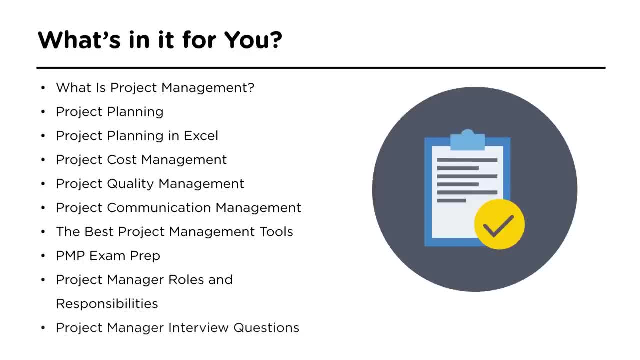 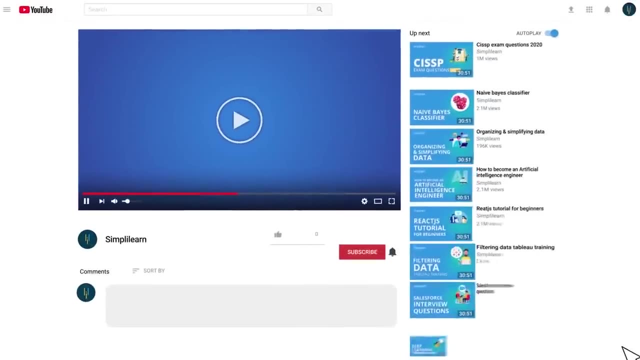 in project management. For this training, with me we have our specialists Chandra, MR and Ishaan. Together. they will take you through these different topics. So let's start by answering our first question: What is project management? So, before we begin, make sure to subscribe to our YouTube channel and don't forget to. 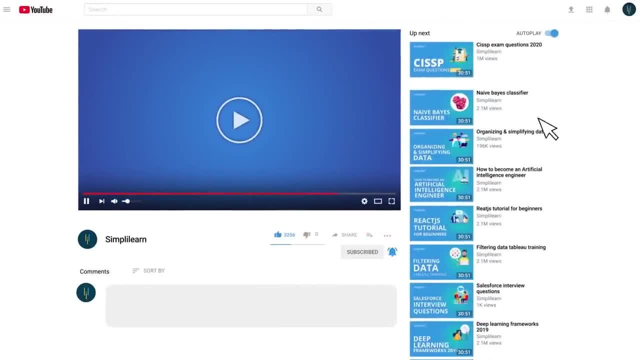 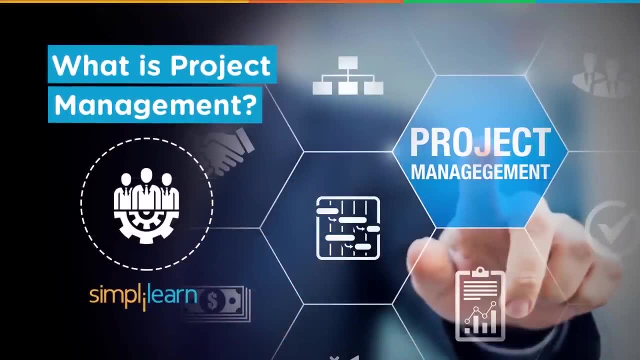 hit that bell icon so that you can never miss an update. Hi, welcome to project management tutorial from Simply Learn. I am Chandra MR, a professional consultant and coach in best practices related to project management and IT service management. Today, as part of this tutorial, we are going to learn the basic understanding about the 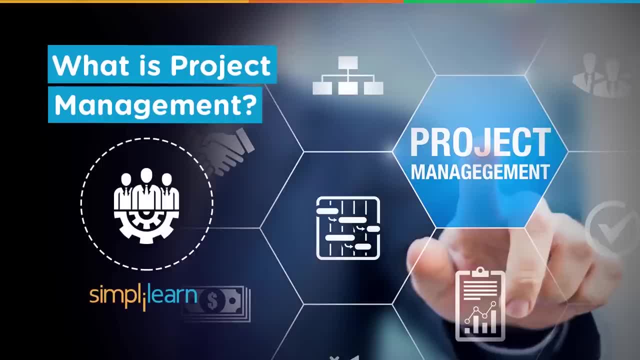 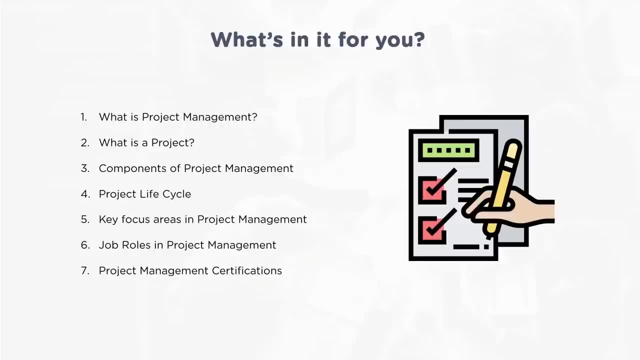 project management and the required knowledge for a project manager to become successful in managing projects. So, as part of this tutorial, we are going to look at: what is project management, What is project, components of project management, project life cycle. key focus areas in project. 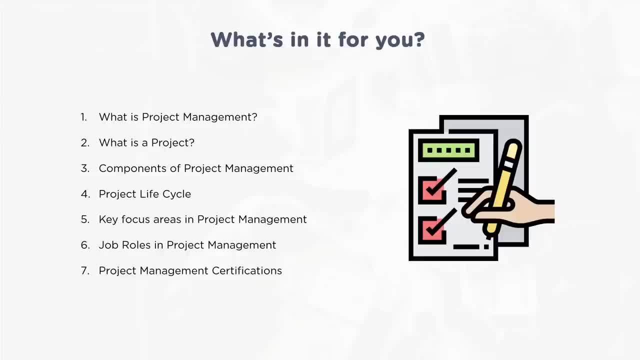 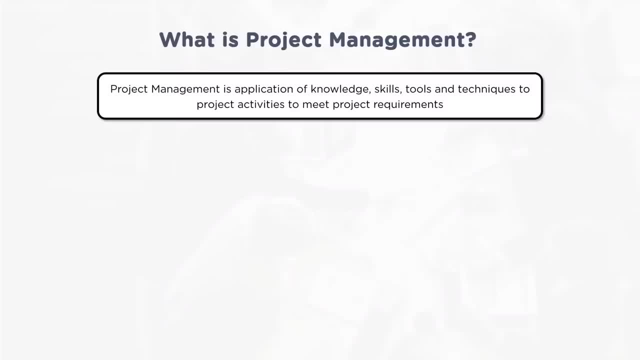 management, job roles in project management and project management certifications. So what is project management? As defined in PMI's PMBOK, project management is application of knowledge, skills, tools and techniques to project activities to meet project requirements. So every project will have an objective to accomplish. Similarly, 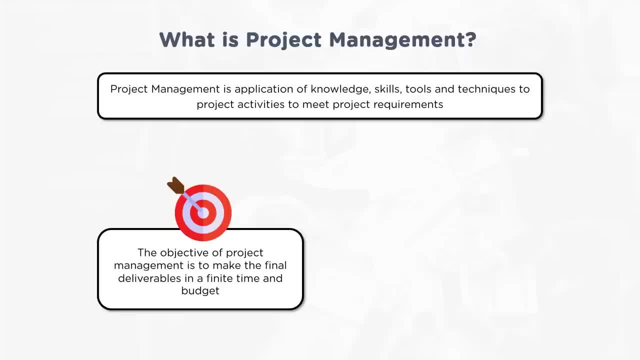 project management is to make the final deliverables in a finite time and budget. This involves having clear understanding about the deliverables of the project, required resources for the project, resource in terms of human resources, technical resources, financial resources, etc. Project manager should have a full picture of those aspects We can call it as constraints. 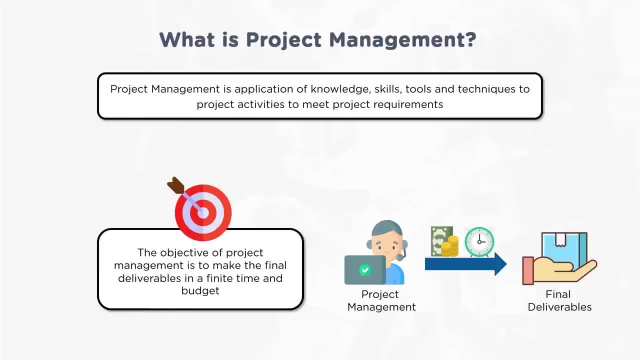 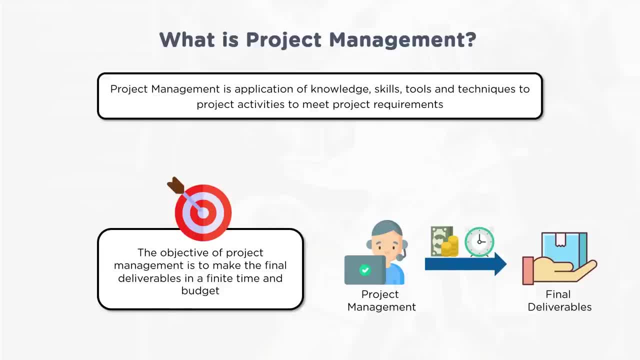 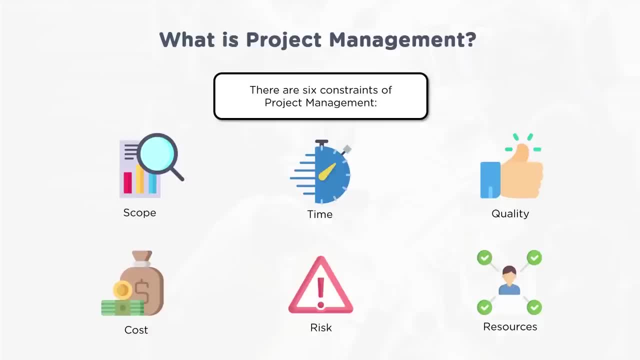 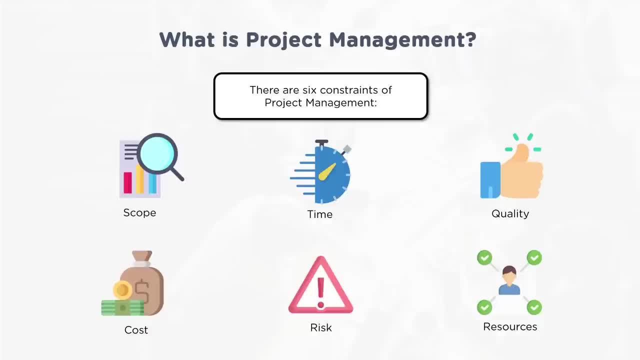 risk and resources. So each of these areas has very important role to play in project management: The clarity in scope, the clarity in terms of schedule within which the project has to be delivered, the cost, what it incurs to that particular project once it is finalized. 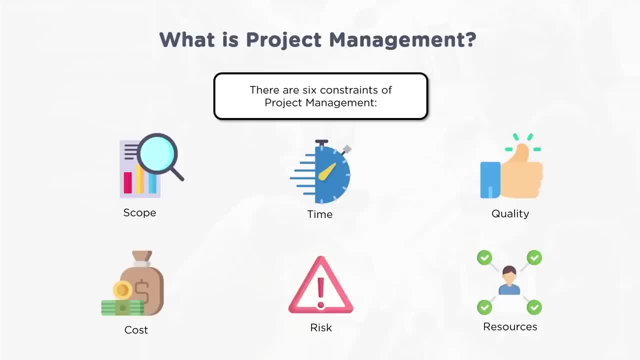 change without any proper approvals. similar to that, we have quality management, which has to ensure the scope, the specifications, what are defined. project output will be accordingly achieved. risk: every project is taken up for a specific reason by organization, so organization should assess the risk associated with the project and similarly, as project progresses, various 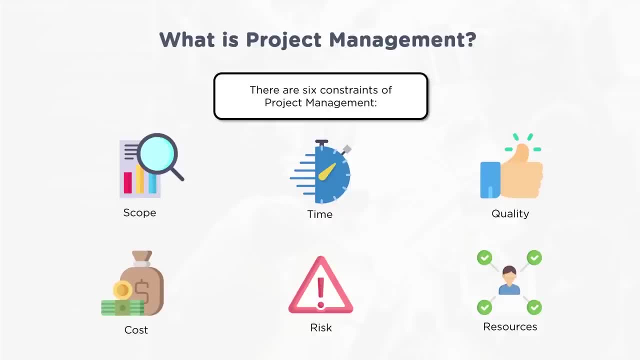 different risks has to be identified, like risk related to project management, risk related to technology area, risk related to resources, risk related to financial things. so broadly, risk management plays a very important role. so there will be something called contingency reserve kept for a identified risk above the cost. what is estimated for various deliverables from? 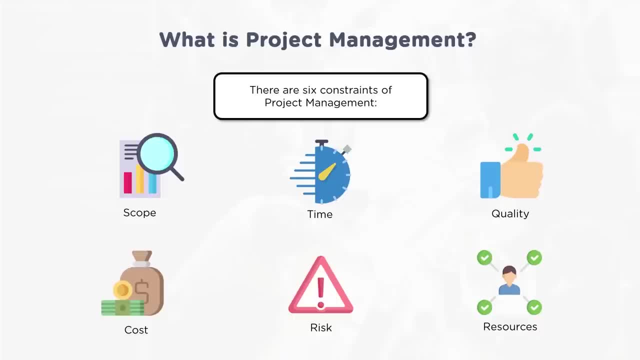 the project. so every projects require resources. resources may be in terms of human resources, financial resources, technology resources, environmental resources. so all these resources are used to produce the output of the project. so these resources has to be managed with the sufficient optimization and standardizations required. now let us understand the definition of a project. 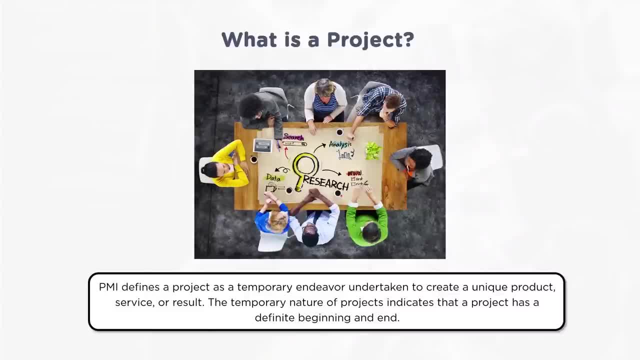 so what is the project? PMI defines a project as a temporary endeavor undertaken to create a unique product, service or result. the temporary nature of a project indicates that a project has a definite beginning and end. so when I say product, unique product, it means every output. it may be similar products you are producing with the same features. 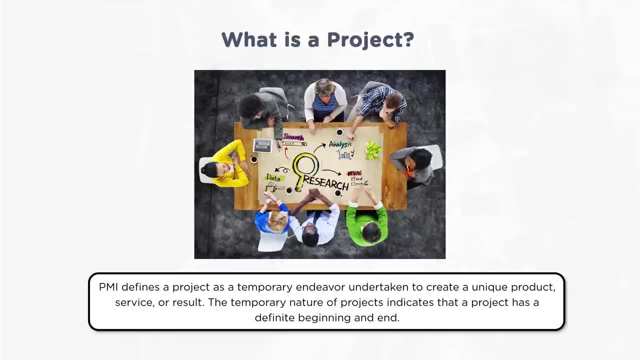 and functionality, but the output of every project is unique because it is unique in terms of all the six constraints, what we just discussed now. now, when I say product, it is very easy for us to visualize: it may be a desktop, it may be a laptop, it may be a car, it may be a machine, etc. but how do I? 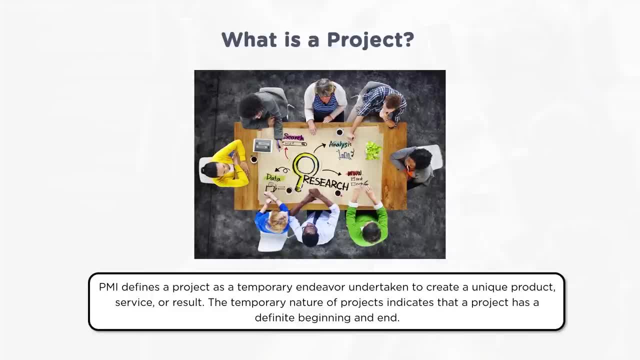 visualize a service, a project. output is a service. now it is. it's about building a capability, a project, by through a project, a capability can be built to ensure services can be provided. that's what the output of project is: service. for example, if I think about a taxi services for 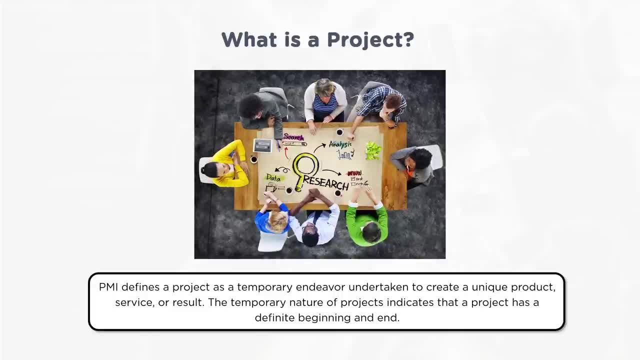 providing a taxi services. I need a mobile app, I need taxi, I need a server, I need a data center. so all these are various different products and services here. service example can be internet service. so combination of all the services and products builds the capability for an organization's who can. 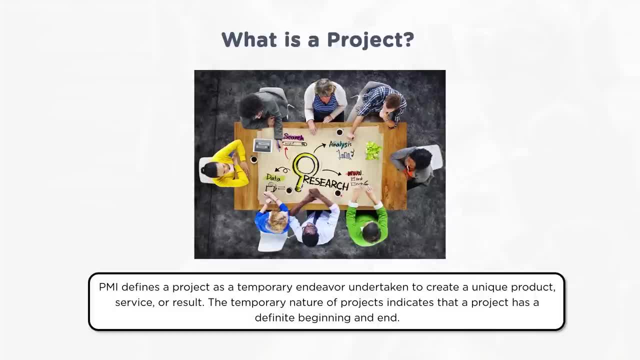 provide the taxi services. so building that capability, we say it is an output of a particular project which is called service. similarly, results can be improvement of something, improvement in customer satisfaction, increase in some specific objectives or specific results needs to be achieved in performance perspective. so output of every project will be unique: product or a service or a 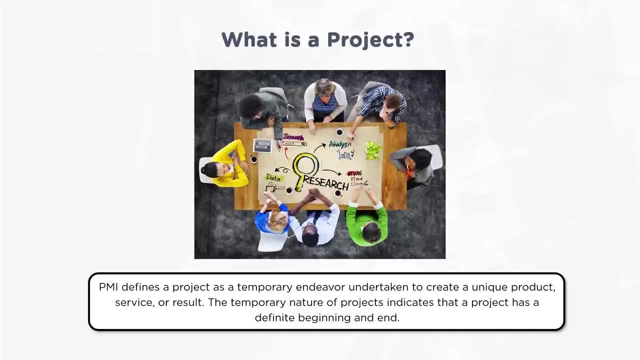 result. this we need to clearly understand. so, when we say there is a definite beginning and end, every project starts at the certain point in time and ends at certain point in time, so it has a definite beginning and end. that is the reason it is temporary in nature. it is not an ongoing. 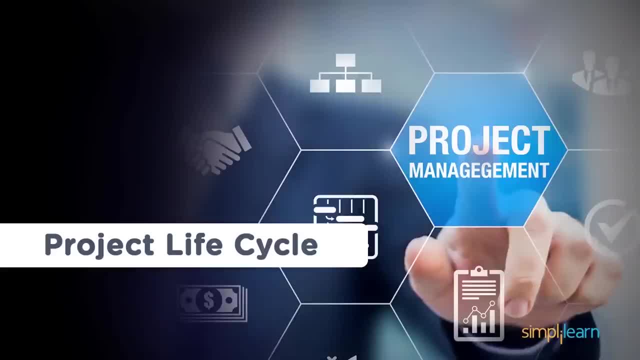 business activity, right. so every project will have a life cycle, a beginning and end. so when it starts till end, until the result, or a service or a product which comes as an output of a project, project life cycle is not ended. so, interestingly, in a product life cycle or in a service life cycle, you come across a 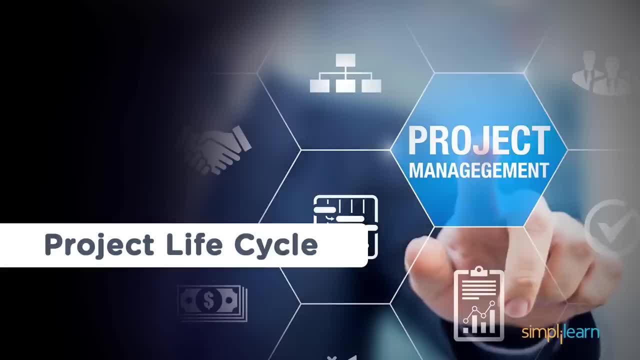 many project life cycles. so one project life cycle means one project is initiated to introduce a product or services. next project, or initiated, would be to enhance the capability of a service or a product. next project initiated after some time is to optimize something similarly at the end of the 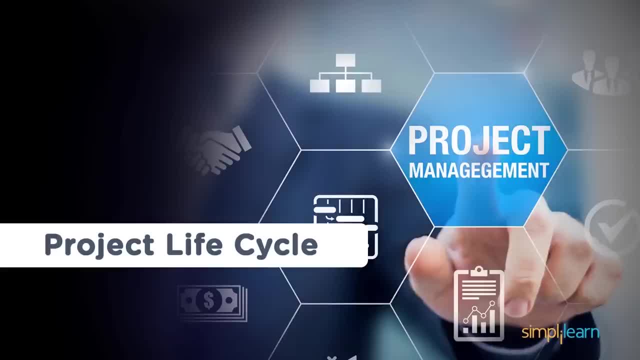 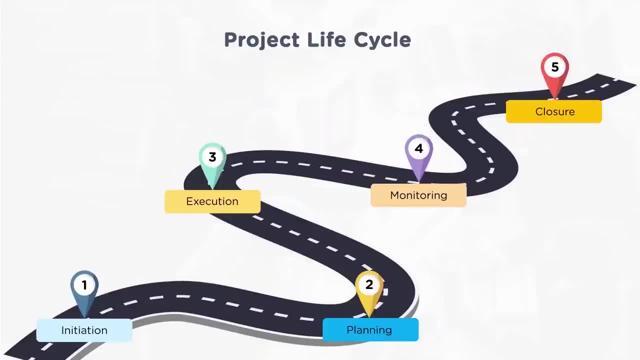 product life cycle, project is initiated to retire that product or services. so in a given product life cycle there may be multiple project life cycle. so what is involved in the project life cycle? it involves five areas, five groups. we can call it a. so initiation, planning, execution, monitoring and closure. so 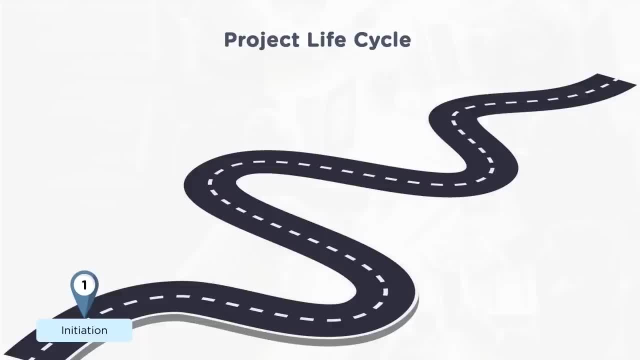 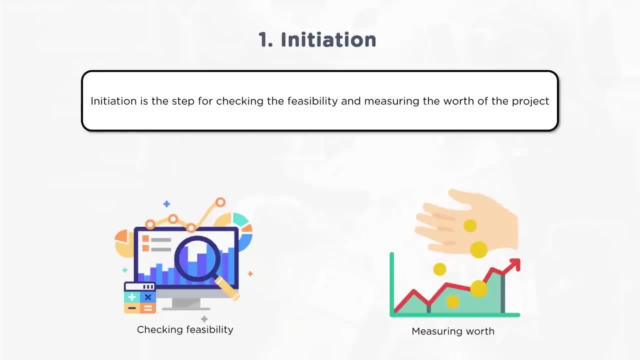 when I say initiation, it's up all about understanding what is project, giving the basic understanding of the project, collating the details and having key stakeholders identified. once that is done one will move towards planning. so here in the initiation, it is very clearly one has to understand: is project? 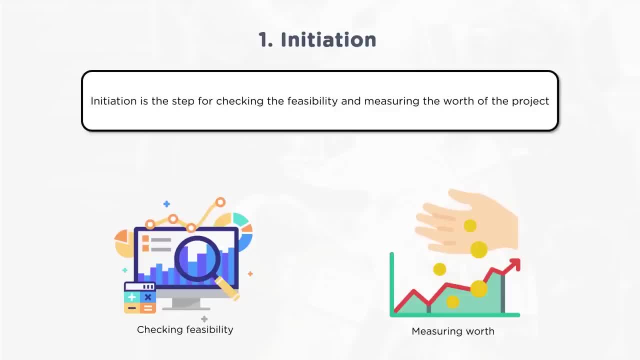 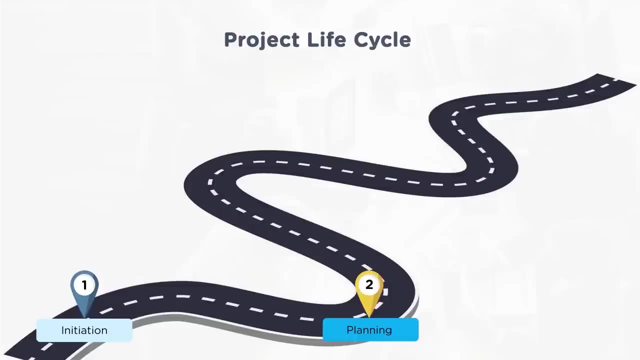 is worthwhile of doing so. one has to check the feasibility, one has to measure that particular investment is making sense and then confirm, yes, it makes sense to invest now. next planning as we have a basic understanding of- yes, this project has to be done, and a discussion with the key. 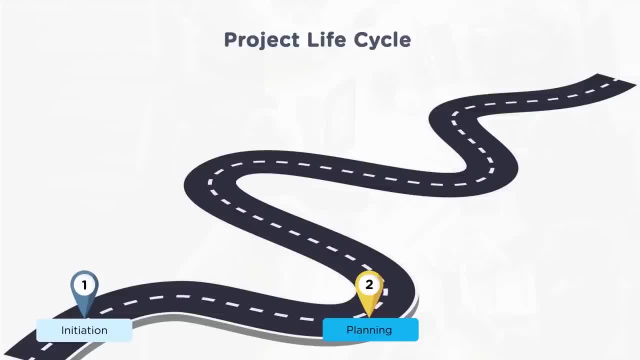 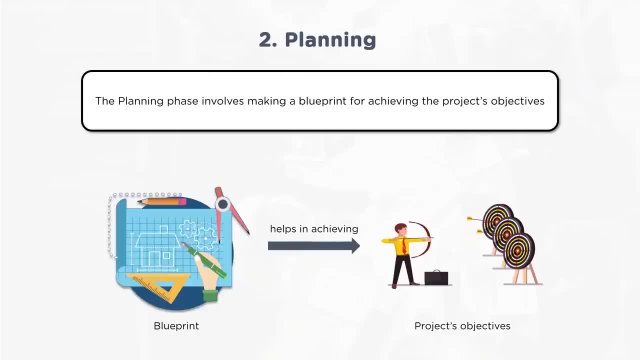 stakeholders have happened. now that moves towards planning. now in planning one will understand the project in entirety. if it is a waterfall approach, one has to have a clear articulation of entire project, a comprehensive details, holistic approach. now, if you go for going in a project in a agile way of approach now in this planning, you may. 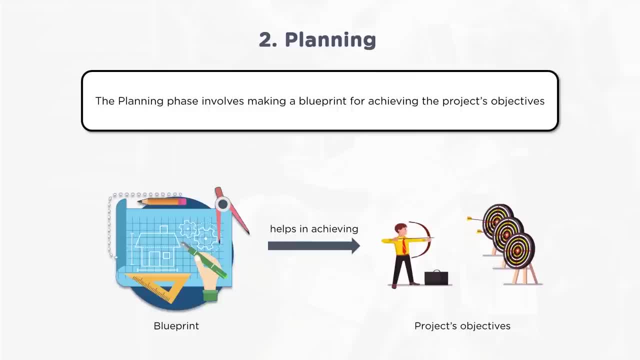 have a big skeleton. as you go in each of the iteration, you may go deep, dive into detailed planning if it is a agile approach. so planning provides you the clear insight towards what needs to be done in this project, how it has to be done and what are the results which can be achieved out of that particular. 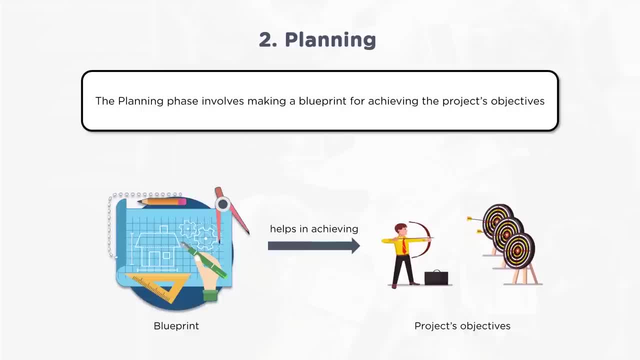 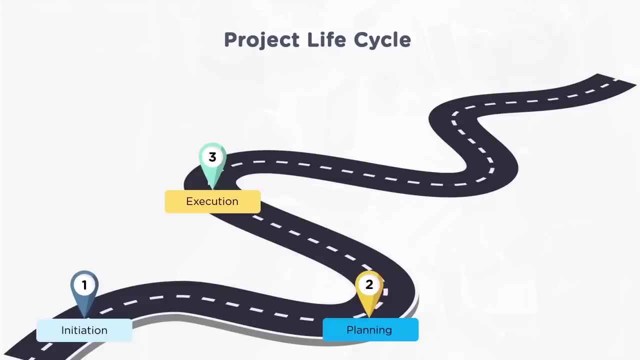 project. so this involves making that a clear blueprint of an project objectives, what we are supposed to achieve. so this will become a reference point throughout the project lifecycle. then execution, as you have a blueprint of the project, as the direction of that project is set, detailing of the project has been made. 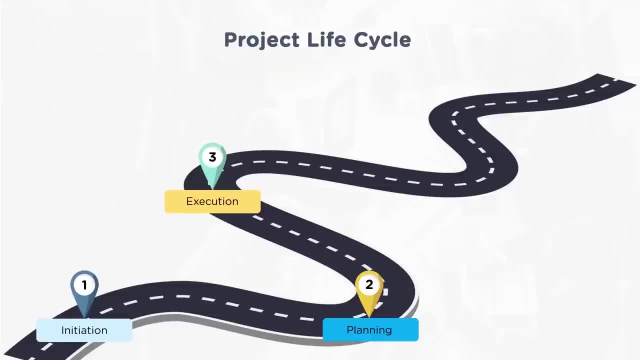 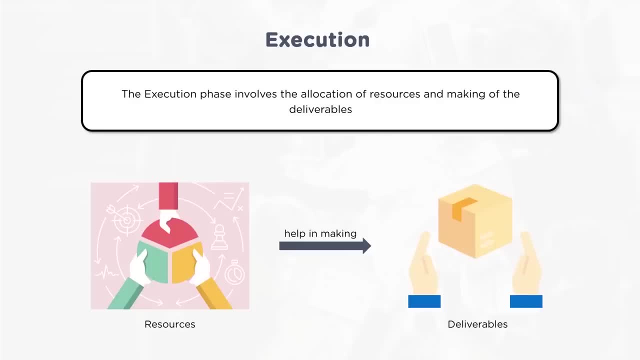 one will go ahead and execute the project. execute in the sense implementation, acquiring resources and implementing it. so execution phase involves the allocation of resources and making the deliverables as required. you acquire resources, you configure a resource, you ensure right resources are acquired. if it is human resource, one has to educate that human resource with the 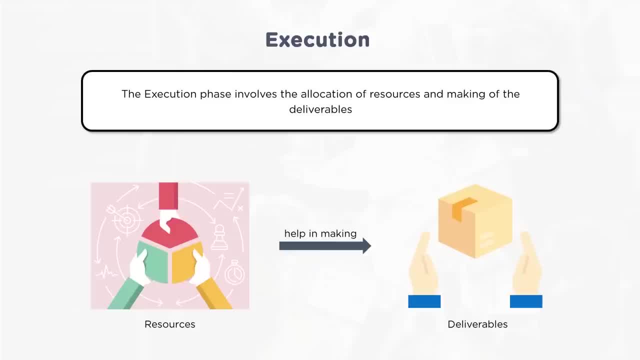 project required knowledge or details, or one has to provide that assignment in such a way that skills of that individuals, what they should have, is acquired by those individuals so that deliverables can happen. and they need to be managed. the entire team need to be managed. for that a clear structure has to be created. similarly, when you do technology, resource perspective. 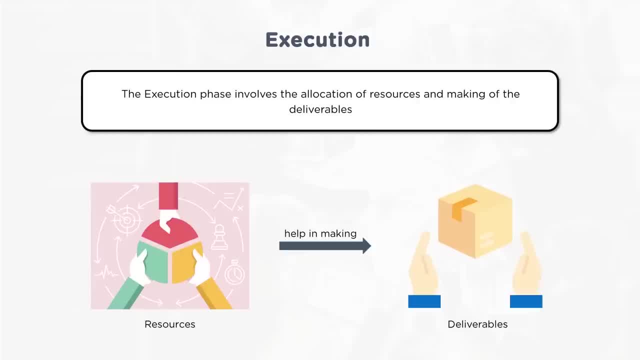 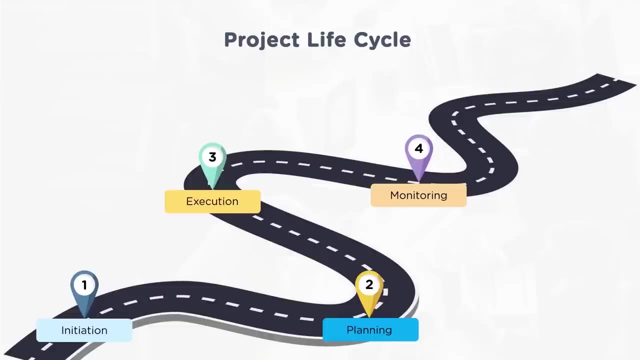 those components has to be tested, configured, then integrated, again tested for and check the performances. so collective action of this results in a deliverable during the execution. so as the deliverables are happening in the execution, it is quite obvious project manager has to monitor, review, control that particular deliverable and also the processes, tools, resources used during. 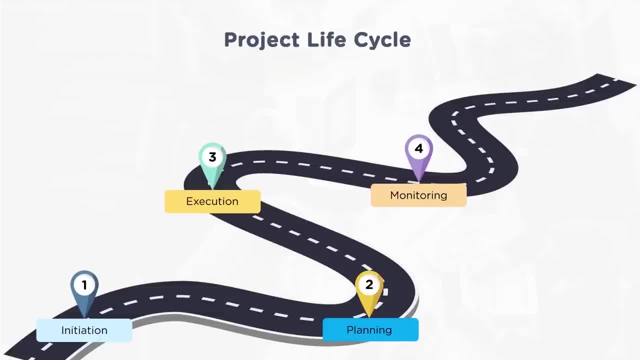 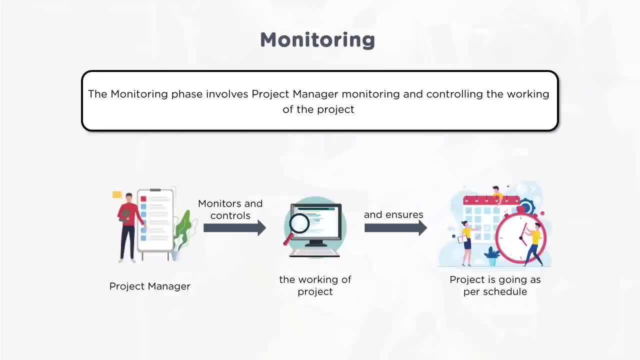 the project, even those needs to be monitored so that they are complaining to the defined processes. so during monitoring there may be a deviation one can found during monitoring there may be. the project is run, running the way it is required. so in this monitoring phase it involves an action from project. 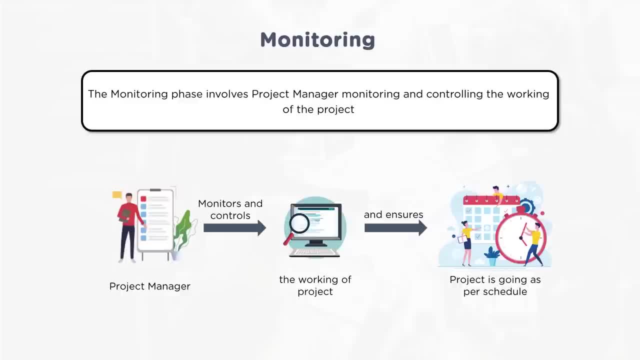 manager to monitor and control the work of the project. so, comparing with the blueprint of plan, what is accomplished, what is created during the planning, the face of this project and as the execution happens, monitoring and control is monitoring it and checking is that activities, what is being done is according to the plan or not. similarly, the deliverables, which comes as an. 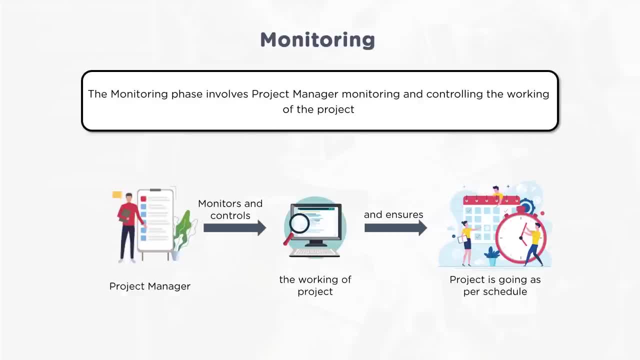 output of a projects are tested thoroughly: whether those have a specific features and functionality and are they functioning the way it is required. now project has to be delivered to the scope: what is defined. it should not go beyond that or below that. similarly, the schedule: what is made for the project within that? 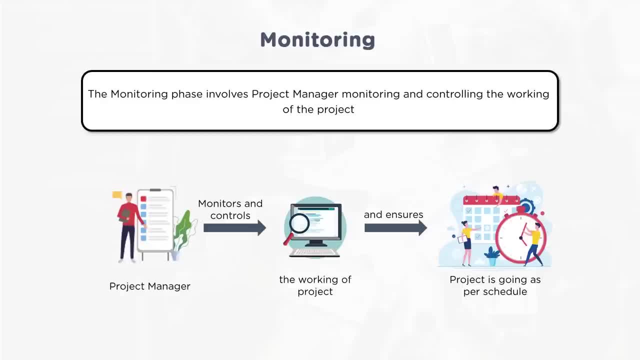 schedule. project deliverables needs to be accomplished within the cost what is budgeted for the project. so during the project you project manager, may find there are certain deviations which are occurred. there are additional challenges which has come in, so for this reason one has to ensure continued monitoring as the execution happens. 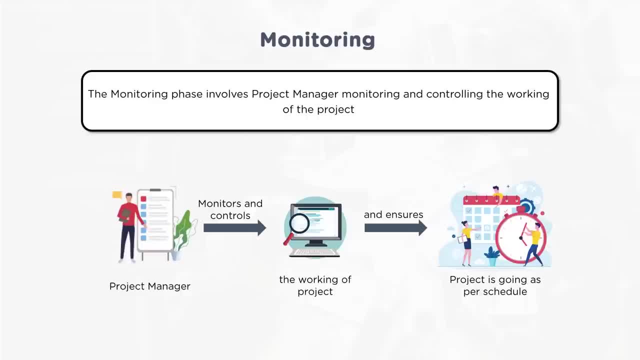 and identify those deviation and ensure whenever there is a deviation there is a correction. whenever there is an additional things coming in, that needs to be considered carefully whether that need to be involved as part of this deliverable or should be taken separately. so this requires lot of conversation with all the stakeholders of the project during the entire project life. 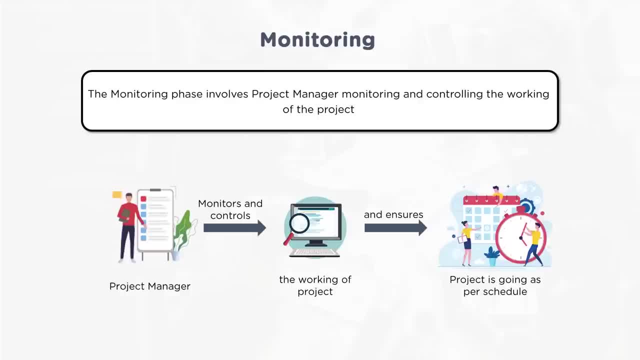 cycle, especially during planning, execution, monitoring and control, since they are not one which is happening in sequence. so planning can also come back again where there is something which you may require to modify, so you may require to have a change in the blueprint itself by adding that new change which is coming in. so you go back to planning. so planning execution. 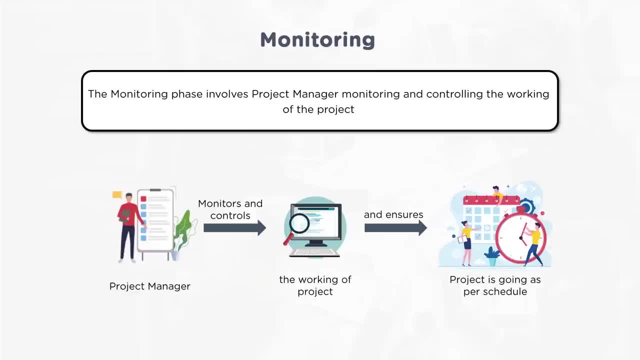 monitoring and control are going hand in hand so that project deliverables are happening as needed. similarly, all the process, work, instructions, all those templates, what is given, are used. one is complying to those requirement- it is very important- and project is done within the scope, schedule and time and the quality matrix defined then as the completion of the project. 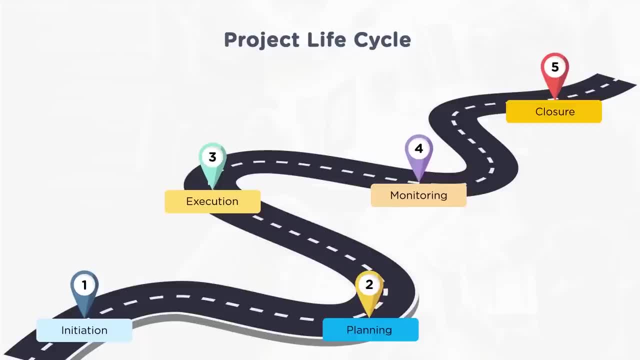 happens as the monitoring and control says: yes, deliverable has happened, according to the requirement, then the project moves to the closure. the closure may be closure of a specific project phase, a milestone deliverable or a phasel deliverable, or it can be a deliverable at the end. 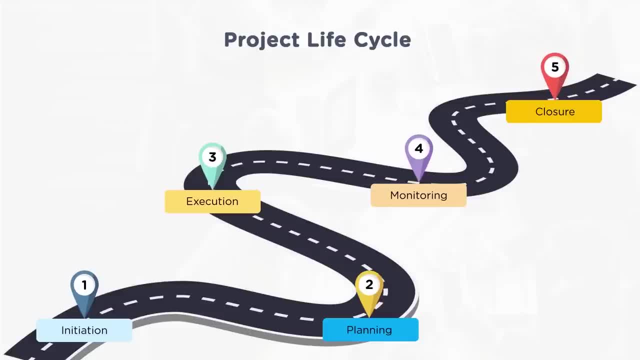 of the project, which is the ultimate end of the project deliverable. so processes in closing has to be triggered whenever there is end of the phase, whenever there is a deliverable to conclude, and also at the end of the project to conclude the entire project. so during the closure one 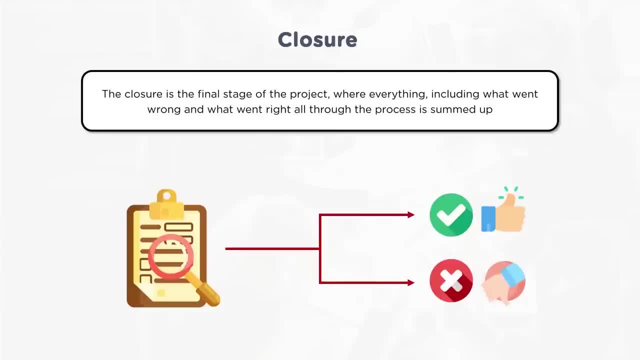 has to ensure capturing all the details in terms of what is accomplished against, what is defined, what went wrong, what went well, what is a learning. one has to take to the next level, or to next phase, or to the next project and, at the same time, a sign-off has to be obtained formally and everything should be. 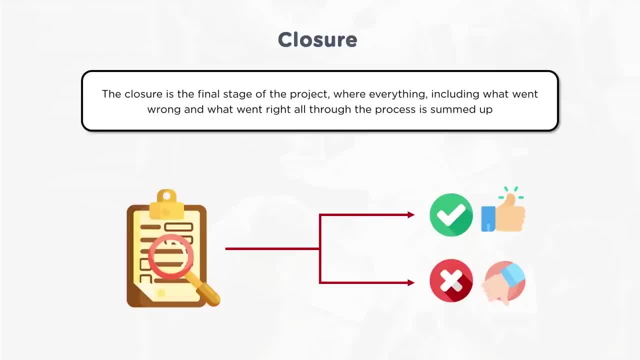 summarized and have a good handshake with the project stakeholder- mainly a business or customer. and also disseminating of team means you will dismantle the entire team and send them back to their specific units or specialization and they may get assigned to new project or, if it is a functional 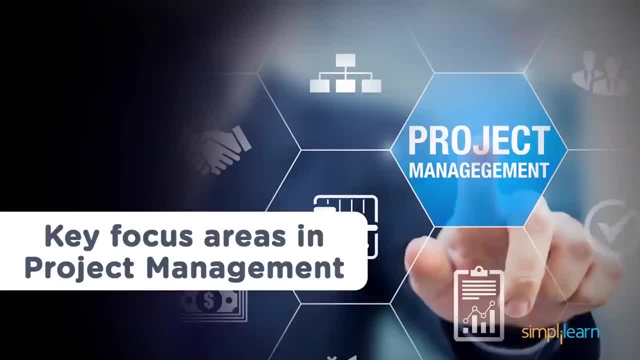 they can go back to their functions to do their functional activities. so that was about entire project lifecycle. what happens now? while doing this, I mentioned there are six constraints, that is, scope, schedule, cost, quality, risk and resources. so, keeping these in mind, one has to ensure project is successful in all aspects. so, to become successful, 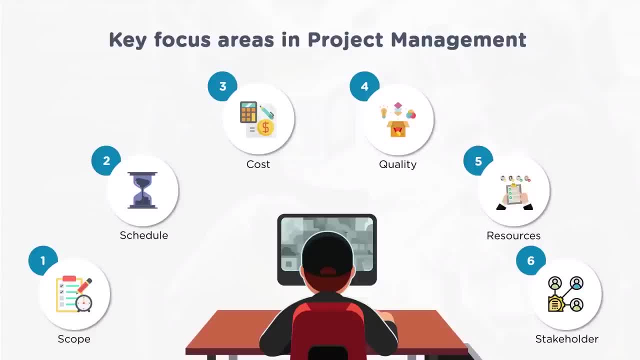 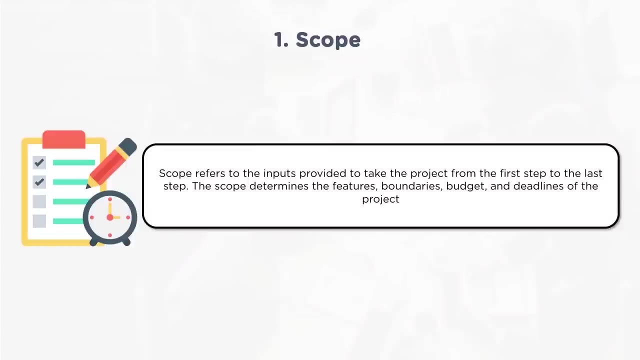 there are few key areas which has to be looked at. so first, six key areas are scope, schedule, cost, quality, resources and stakeholders. now let us look at the scope. what does scope means? scope is about what needs to be delivered, what is in scope, what is out of the scope. so this: 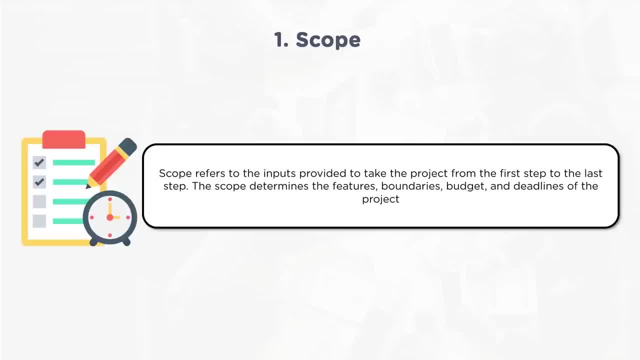 refers to all those deliverable scope, all those activities scope. basically, we speak about two things. one is product scope and project scope. product scope is all about ensuring the features, functionality of products are well defined and understood and signed off and while delivering that product, that is tested against those defined features and functionalities, whereas project 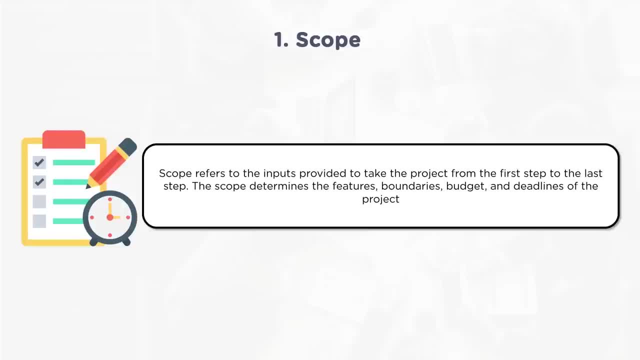 scope focus on all the activities needs to be done, all those templates which has to be used, all the process which has to be complied with, all the skills which is required to be applied. So it is going as defined. So, by doing this activities which is defined as part of project scope, 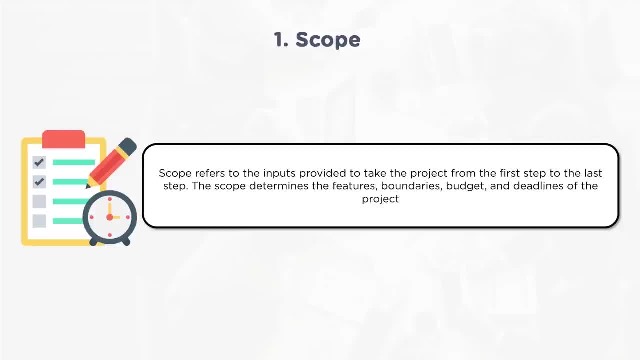 the result, the deliverable will come out, which will be in line with the deliverables features and functionality which is defined as part of product scope. It is very important to ensure entire projects happens within this particular scope. There should not be any deviations from this. 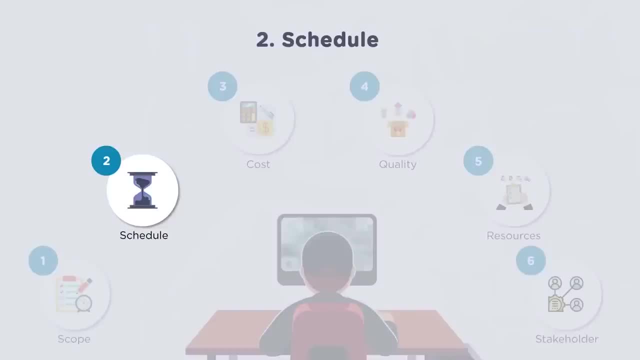 Schedule perspective, for that specifications what we have defined for a product and project. So these needs to be done in a specific point in time, means in a specific schedule. There will be start time, end time, right, So one has to plan how long a project would take. 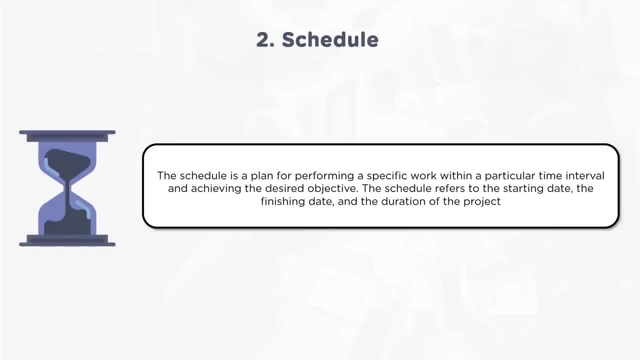 and what are the deliverables, should happen in what sequence? what activities are required to accomplish this? So all these needs to be understood. So while performing the schedule management, one has to look at a specific deliverable at a specific point in time. 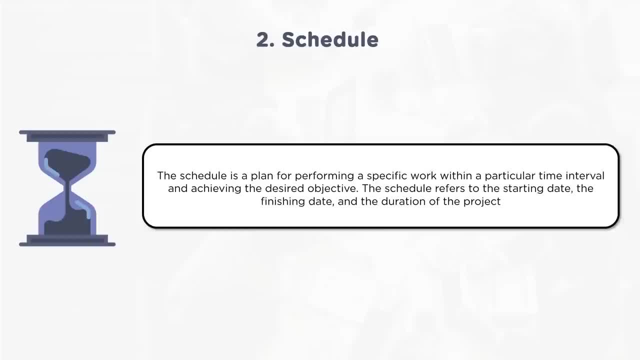 by applying a specific set of activities required. So this will tell you the duration of the project. This will provide you the sequence of project. This will also help you to understand the dependency between one task to another task. This will also help you to understand how the deliverables happening in what sequence. 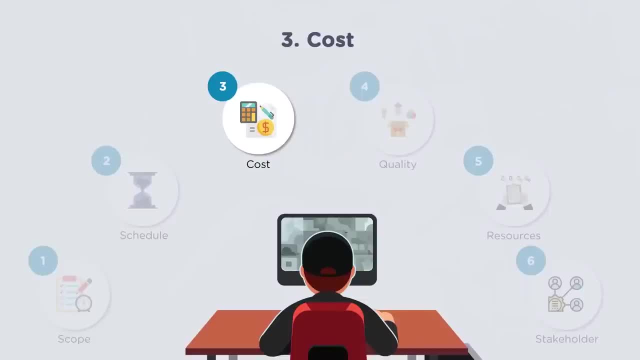 which helps in prioritizing your deliverables. Third is cost. So, as we know, to do any project it is very essential to ensure project happens within that budget. So project cost is estimated initially. Then that estimated cost will be checked. 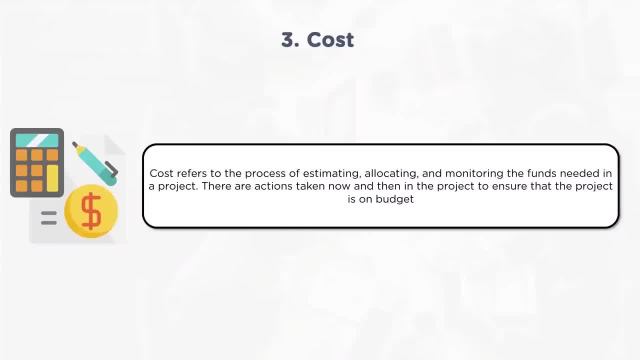 Checked in terms of: is the assumptions, Considerations are right or wrong? Is that really so much of monetary resources are required for the project? And then, after understanding the justification and obtaining the clarity, budget, is- I mean monetary resources- are allocated and confirmed- approved? 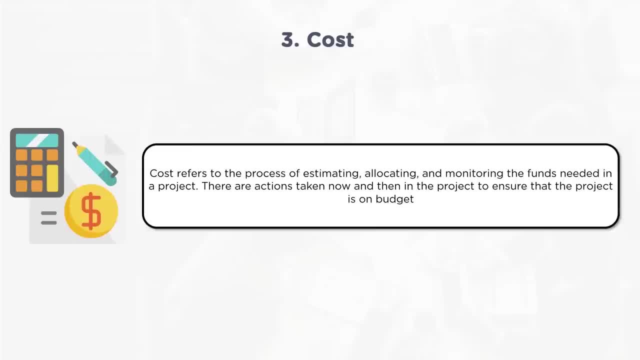 Then it will become a budget That will be a cost baseline. So these estimation, allocation of budget, once it happens that will become a base And any deviations from that cannot happen so easily. So any deviations because of additional of scope. 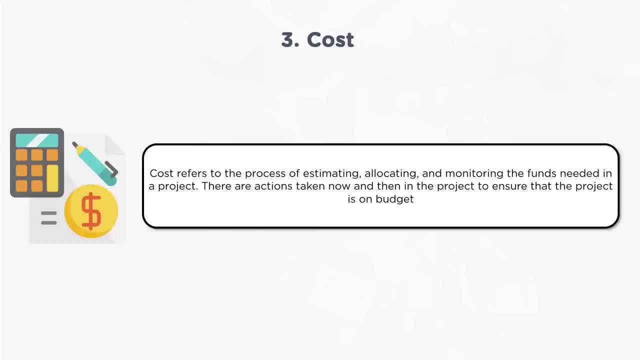 that can be handled through change management, But idealistic scenario- the cost should not escalate or come down. Organization can also set certain tolerances at the project level, Considering various different scenarios, like scenario of risks, scenario of something which deviated from the deliverable. 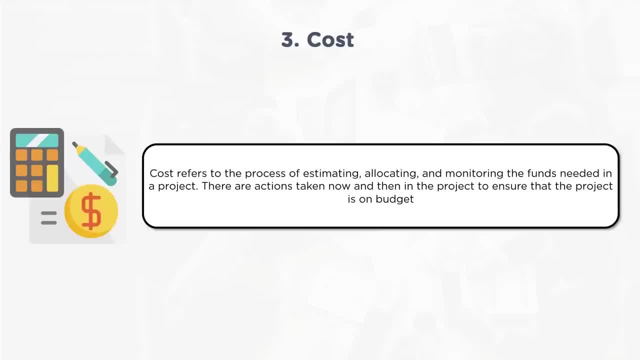 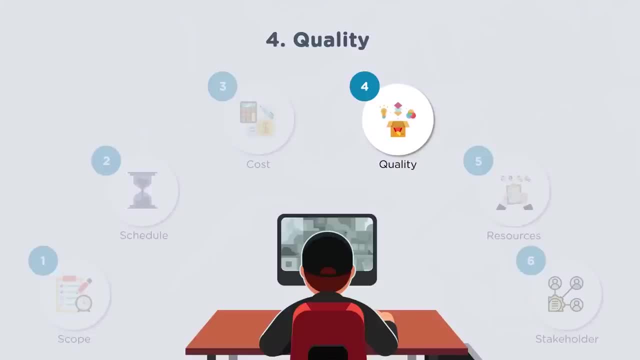 So to what extent it can deviate That tolerance will also be set at the economic or monetary value perspective. That is about cost. Now quality. As we know, quality is a very important area which ensures the project is delivered in time with all the specifications defined. 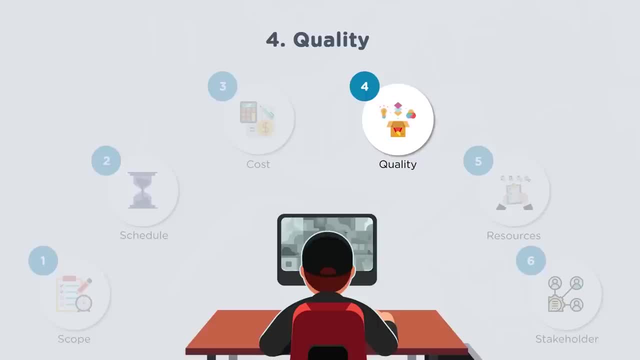 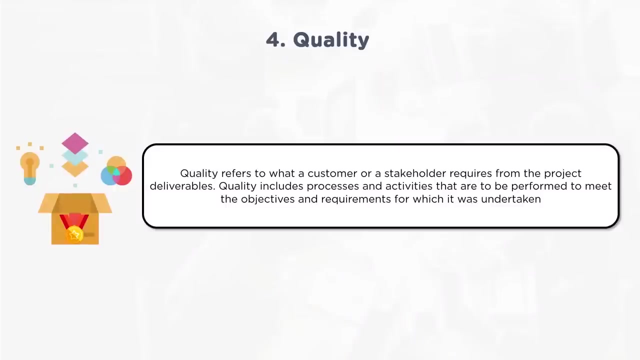 by using all the methods Means by following all the processes, work instructions, templates and delivering as needed Where it enables the project to monitor it easily. So, basically, the requirement of compliance and standardization and optimization is to ensure everyone follows the same steps to the activity. 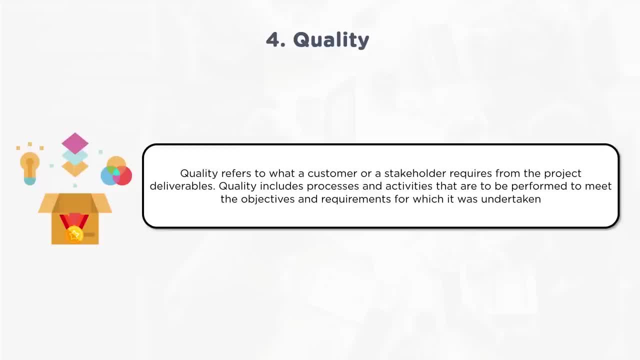 So what quality management focus is To ensure the intended objectives of a project are achieved? Already there is a definition done in terms of various different practices or processes needs to be followed. Similarly, specification of each of the products are defined, And from that there should not be any deviation. 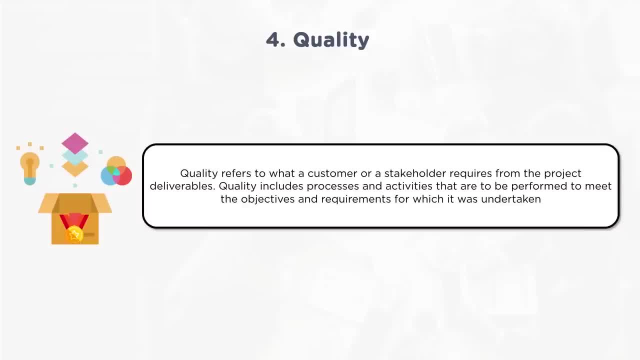 So quality management should focus on ensuring those activities are done as defined, Those deliverables are done according to the specifications, what is defined. It is very important that way. So for that there is a layer of quality management. There should be a layer of quality management. 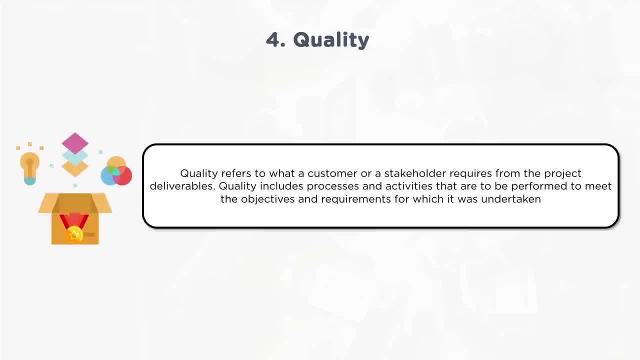 where auditing or control activities are initiated periodically So that any deviations can be seen easily. And remember, a project manager cannot become part of quality management. Like project manager cannot audit. Project manager should have a team or take the help of a team who can able to do. 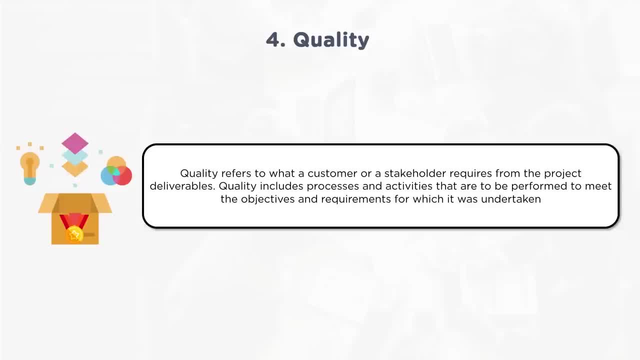 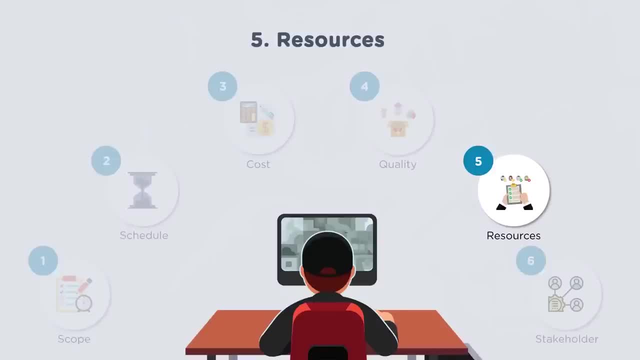 Mostly the one who is not part of the project is always better Resources. Now, as I mentioned earlier, every project need resources. It may be human resources, It may be technology resources, It may be any other resources which are required to do the project. 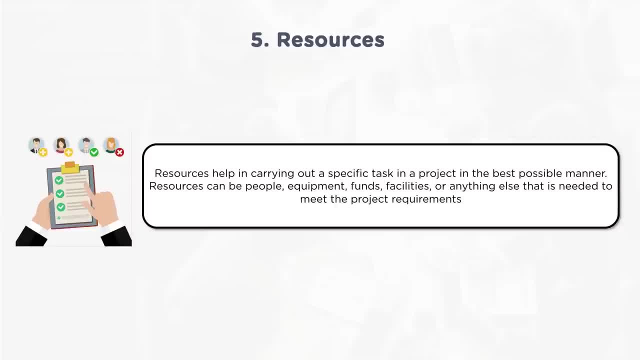 So organization acquires resources, configured and then deployed, For example, in a project. you acquire a server, You configure a server, You deploy a server Technology resource, Human resource is onboarded, Recruited, Project induction is given. Then, at the same time, the skills and capabilities of individuals are according to the requirement of project. 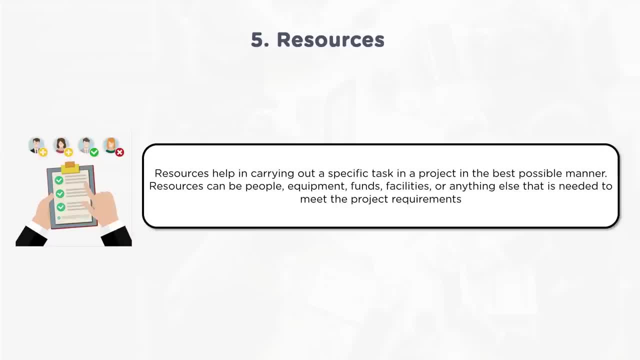 That needs to be ensured And what needs to be delivered And how it has to be delivered should be clear to the particular human resource. So, looking at all the aspects of resources to acquire, to build and manage, It is very important to look at the resource management. 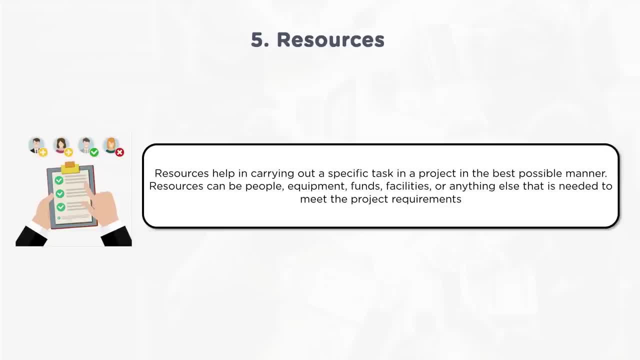 So this will help in carrying out a specific task in the project in the best possible manner. So, interestingly, when I say human resource, always there is a possibility that a conflict can occur. So when I say conflict, Conflict of interest, may be in terms of what that individual needs. 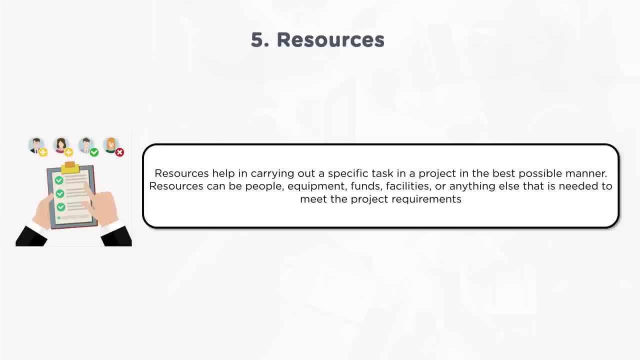 Conflict has to do. Conflict in terms of the preferences, In terms of solutions, What they are looking at. Conflict in terms of using resources, Different opinions, Different preferences, Various reasons. conflict can come across. So it is very important to project manager to understand this dynamics of human resources and manage these conflicts. 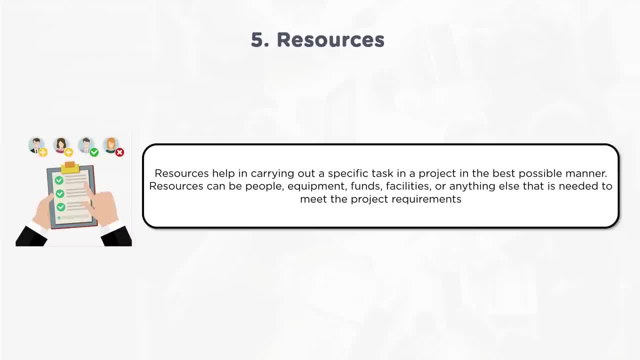 Project manager cannot shy away from handling conflicts. Project manager has to hone and resolve those conflicts in the favor of project, Not in the favor of any individuals. So there are various techniques to look at resolving conflicts. So that is like compromising, problem solving, smoothening, accommodating, 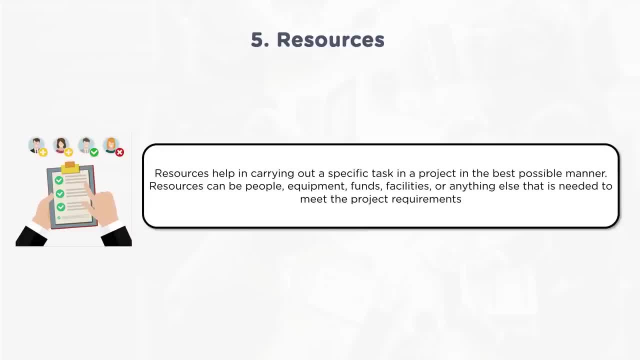 So whichever helps for that project scenario, for the project objectives, That needs to be applied. That technique has to be taken up. So here the resolution is not at the specific individual's preference, It is with the objective of whether projects has any impact. 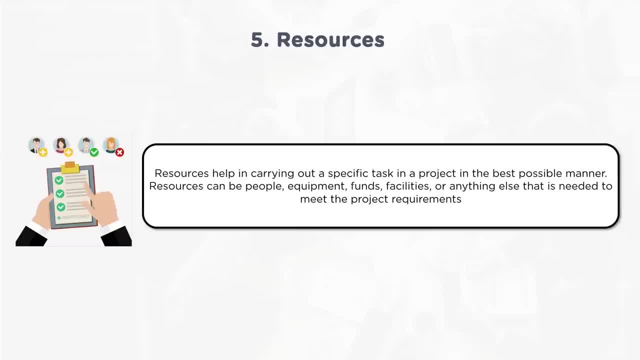 What kind of impact? Positive or negative? If it is negative, No, that is not the direction. The direction should be ensuring project gets that value Through this conflict resolution. So project manager should own it. It is an accountability of a project manager. 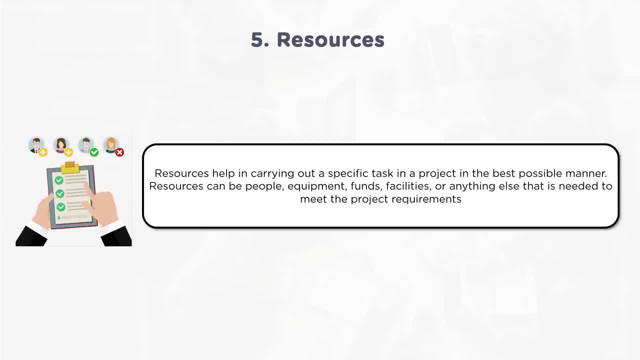 Then as the human resources are acquired. There are five stages. Team dynamics are involved, So one has to bring them, Then educate them about a project. As the education on the project happens, One has to go and do the job on floor. 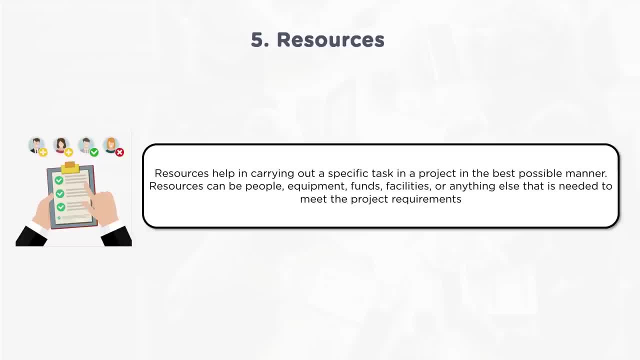 That needs to be observed. Means one has to manage by looking at it And any corrections needs to be done. That needs to be guided. So it is very dynamic thing when it comes to human resources. Similarly in technology resources, Standardization. 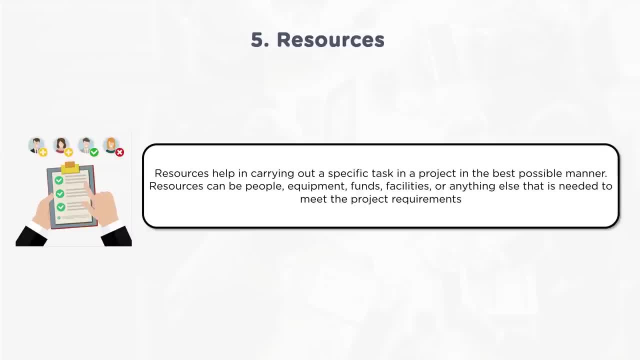 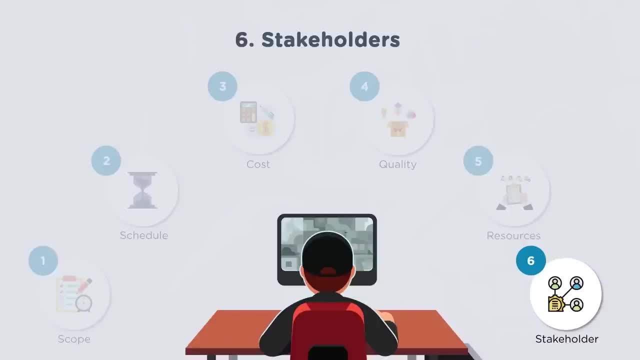 There is no ambiguity as such, But right resources with the right configurations should be acquired. That is very important. The next stakeholders: So who can be stakeholders? Every project will have a stakeholder Who are internal and external to the project. 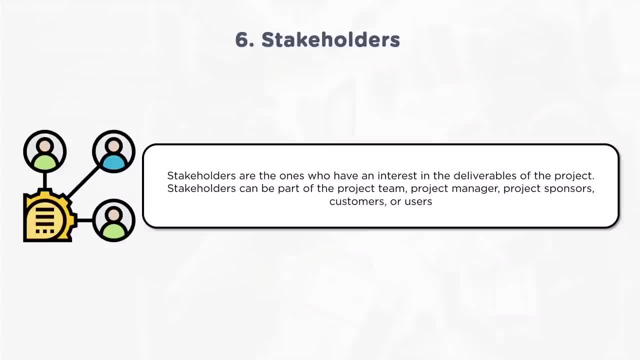 So the internal stakeholders are those Who are part of the project, Who are part of the organization, Who are part of the customer organization, Who are part of supplier organization. A competition to my business Means my organization's business. All these we can call it as a stakeholders. 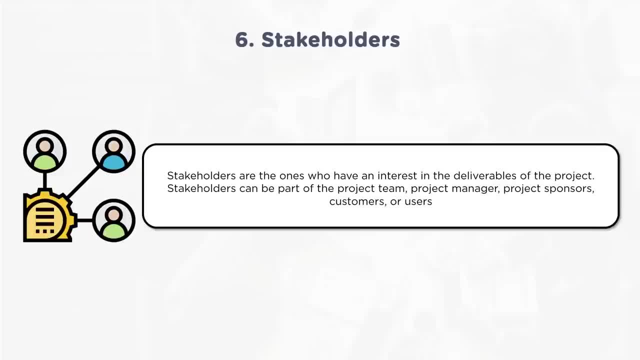 Now, every stakeholders will have a specific interest, A power, An ability to influence. Now, through their position, Through their distance from the project, They will get impacted. At the same time, they will also impact the project. Similarly, they influence. 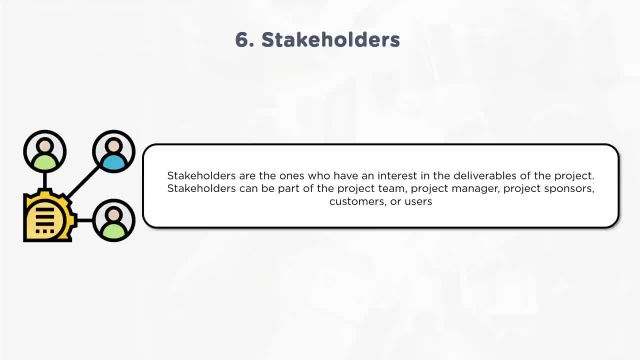 And they get influenced Because of the project. So a project manager should identify all the stakeholders And understand this. What is the kind of stakeholder? is this In terms of power, In terms of legitimacy, In terms of influence, In terms of impact? 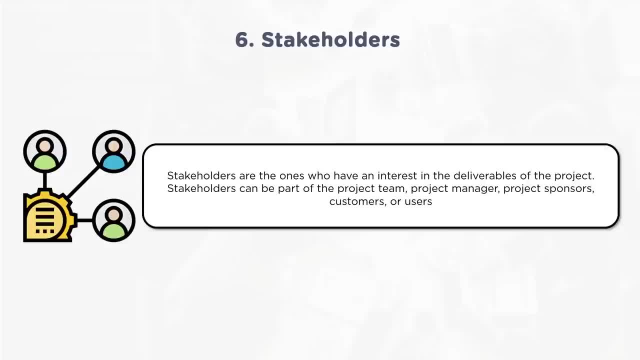 After understanding that There should be a strategy for handling the stakeholders. How am I going to engage with these stakeholders? It is very important And accordingly the engagement should happen And then stakeholder engagement should resolve In the favor of projects again. 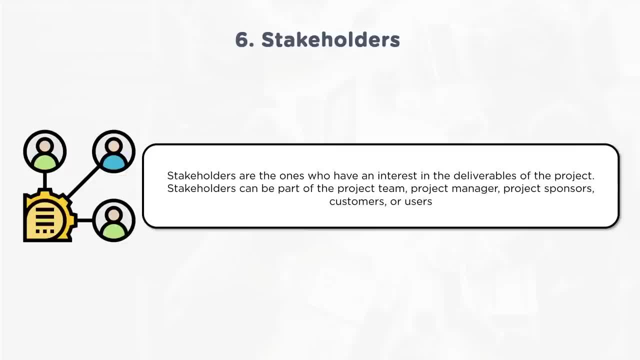 So if it is a customer, Customer should get that inputs required Through review or periodic update, Periodic updates And the engagement required with the customer So that customer is having up to date information about the project. If it is a team, 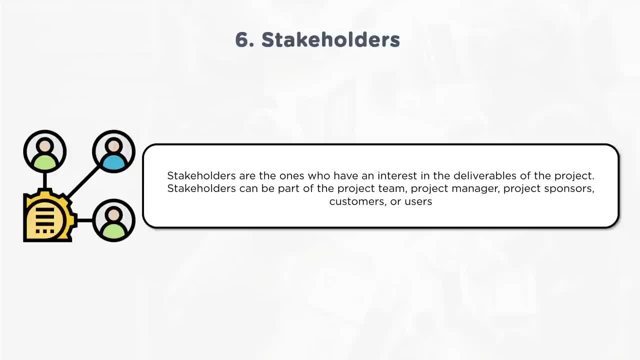 Continued monitoring and control And ensuring team delivers the results. what is required, So focus of a stakeholder should be in such a way That your strategy should enable project to become successful And get a proper response from the stakeholder. Means a supporting engagement. 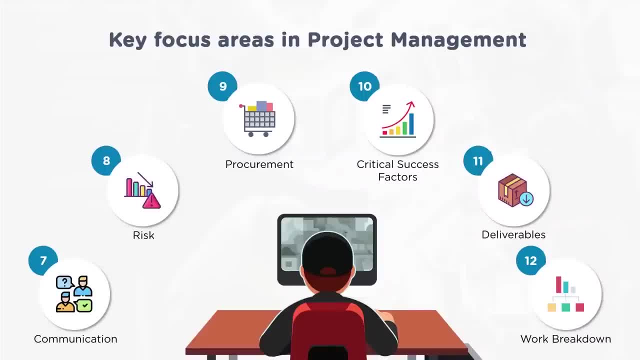 So next few key focus areas to mention is Communication, Risk Procurement, Critical success factors, Delivery Deliverables And work breakdown. So this list is not exhaustive. As we deep dive into project, I think you can just keep listing the key focus areas. more than this. 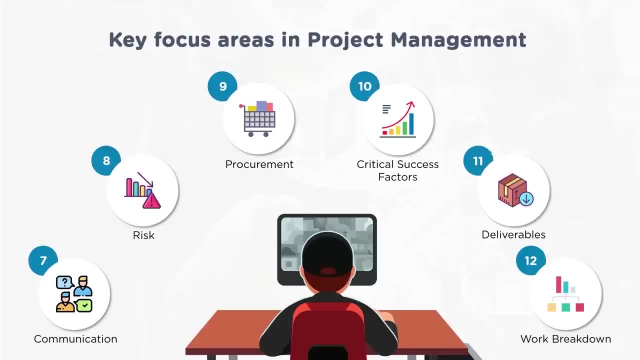 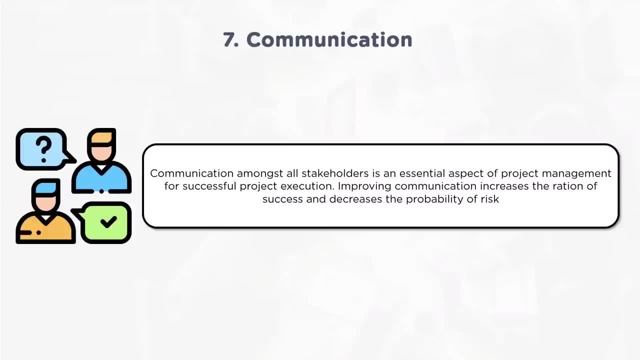 But whatever we have indicated are the minimum Which needs to be looked at. So when I say communication, Communication is basically a conversation, Exchange of message Which happens between two entities. Now, whenever we communicate, It is necessary to understand that. 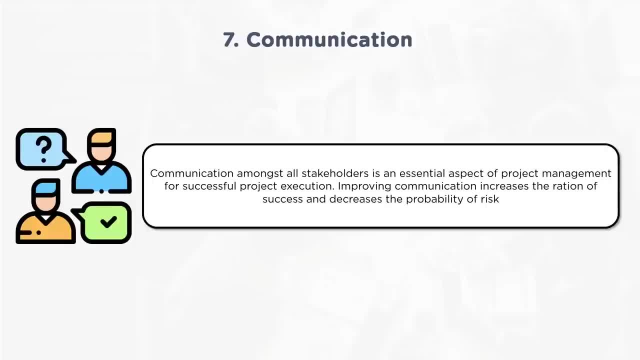 It has to happen with two individuals or two entities. There should be sender, There should be receiver. In the absence of receiver, If sending is happening, That communication doesn't make any sense. There should be a receiver And there should be an acknowledgement from the receiver. 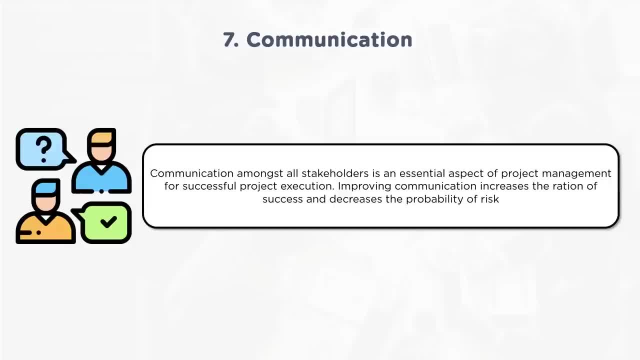 Now this is one of the most ignored area in many of the projects. Even the communication happens more often, More frequently. But what? people face Difficulty in realizing that, As they communicate generally, Informally, Formally, They just take those for granted. 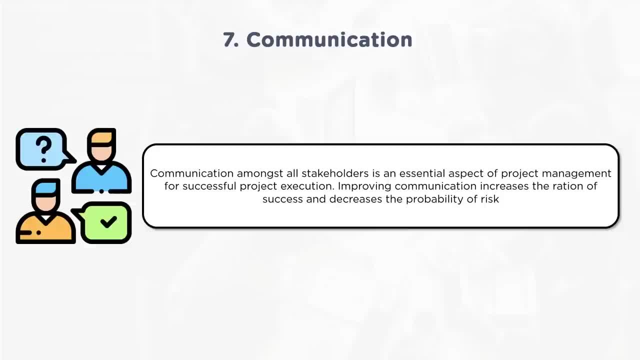 Now, when you identify the stakeholder, One has to understand What is the communication requirement for those stakeholders? What is that communication? Why is that communication? What is the content of that communication? How frequently we should do that? interactions or communications? 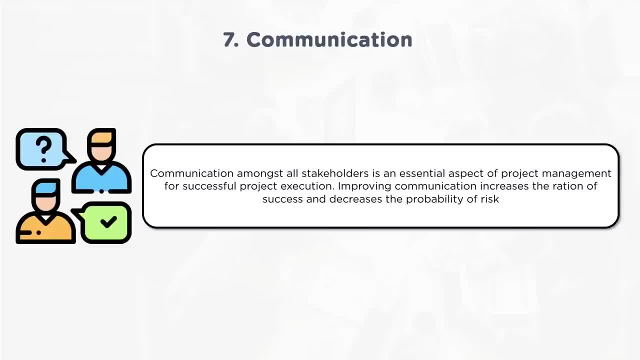 Intent of that particular communication, What is the expected action or response from that communication? All this needs to be very, very clear And this can be articulated. It has to be articulated. So when it is articulated, Once there is a picture, 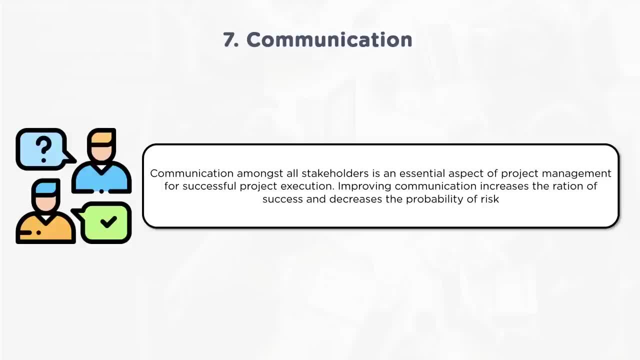 In terms of what kind of communication has to happen. It is quite obvious. There should not be any deviation From the agreed communications requirements And whenever there is a need of change To the communication requirements From the stakeholders, That needs to be updated. 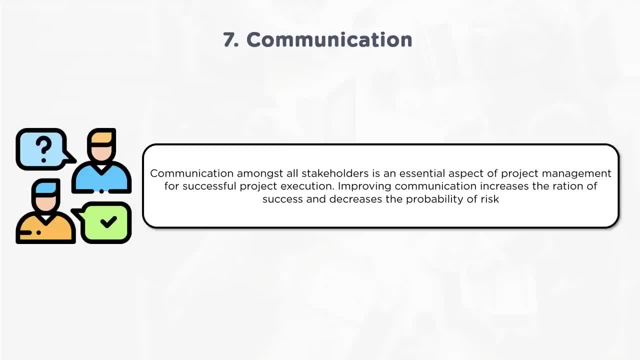 For this One has to have a stakeholders identified. So stakeholder management and communication Are very closely linked, and associated Engagement with the stakeholder will become successful With an effective communication approaches. Next is risk. So every project which is undertaken by organization 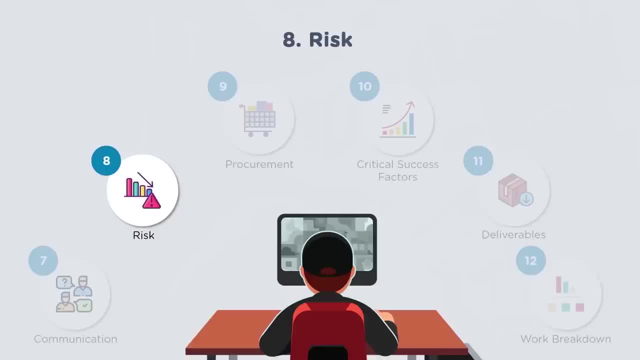 That will have certain amount of risk. Which organization will evaluate? Similarly, within the project life cycle, Lot of risk comes up Which would have certain impact to the project. Now risk refers to, by definition, An uncertain event. It has an uncertainty. 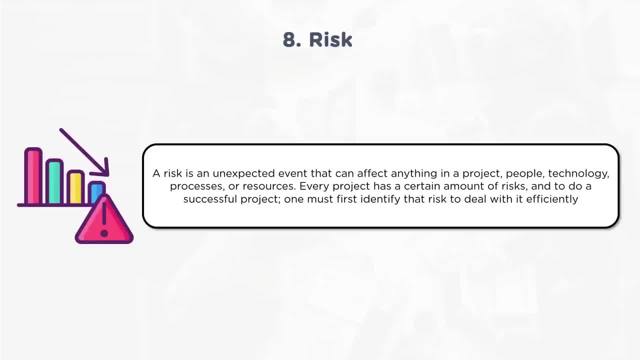 An event which is uncertain And when it occurs, It will have an impact on the project, Positively or negatively. Now, current scenario: In everywhere the projects, What you observe closely- People tend to look at the risk, Which are threats. 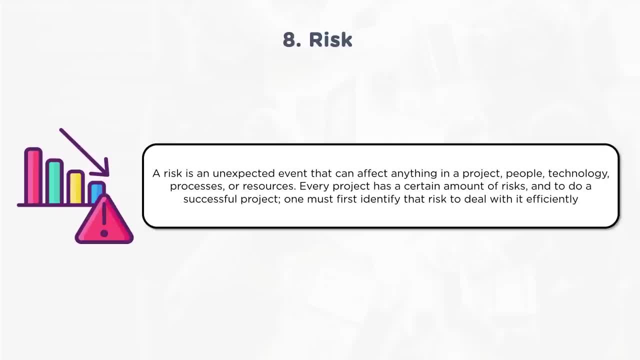 That is negative only. But they fail to recognize the risks Which are opportunities, The positive risks. So another gap which we see: When do the risk management is That is done in the initial phase of the project, As the project is kicked off. 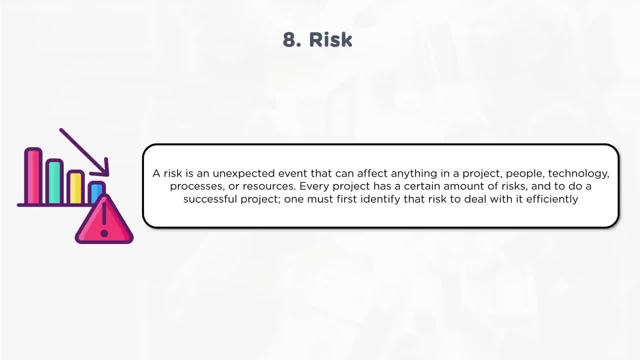 Someone will do the risk assessment, Have a list of risk identified, But unfortunately There is no categorizations for that risk And how is that going to impact the project? That is not clear. Thirdly, risk management Or list of risk? 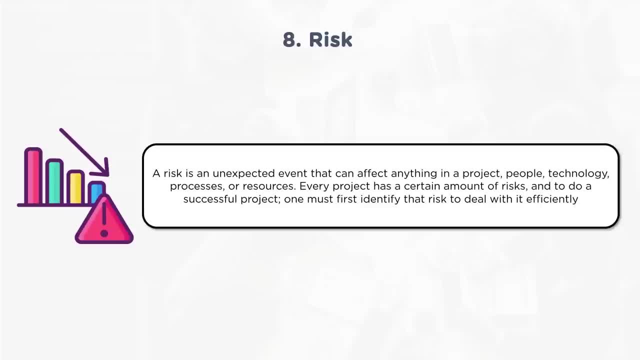 Are created only once, It is not done repeatedly. So risk identification And analysis and assessment Of that risk has to be done Throughout the life cycle of the project, Reason being The risk which looks as an high impact When project is initiated. 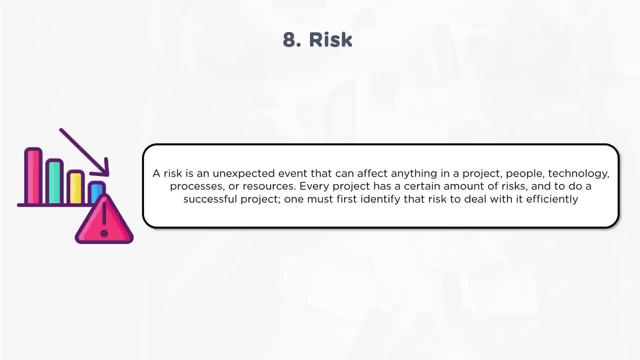 As the project progresses, The impact levels will vary. May be in the middle of the project The impact may be very high or low. So likewise, The impact of the risk will vary Throughout the project life cycle. It may be positive. 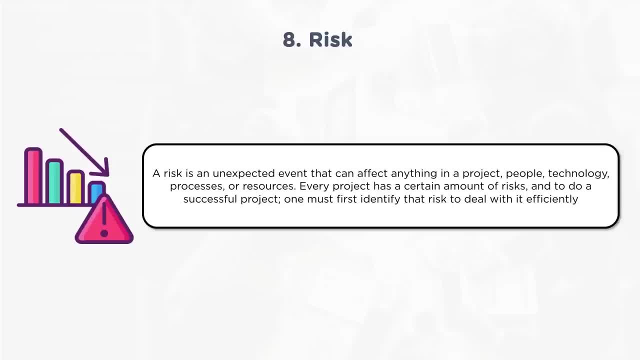 It may be negative. So, as you identify the stakeholder Throughout the project life cycle, As I said, That is also a dynamic. I cannot just have a list of stakeholders And I keep it as it is. I need to update that also regularly. 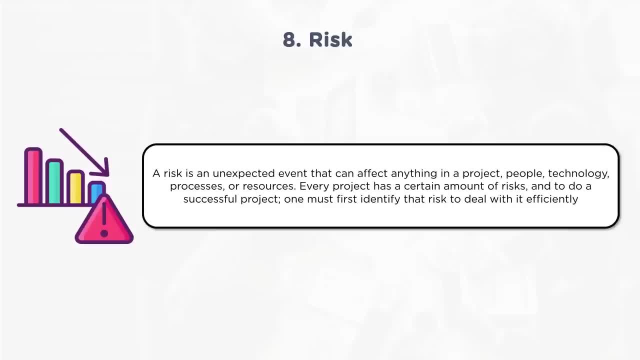 Risk identification, assessment and analysis Should also be done Regularly, Periodically, So that one will have a clear understanding about: Is that risk still valid? Is that risk is there still or not? What is the level of variations in terms of impact of the risks? 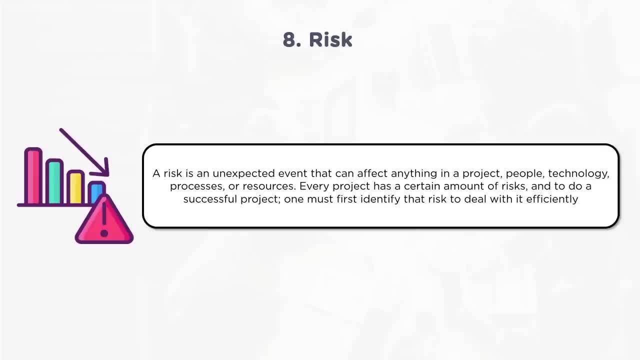 So this clarity will be there, So that organization or project manager can get ready To face those risks. If it is a negative risk, Definitely should have a mitigation or avoidance or acceptance. Whatever the mitigation plan, you have To eliminate the negative impact of the risk when it occurs. 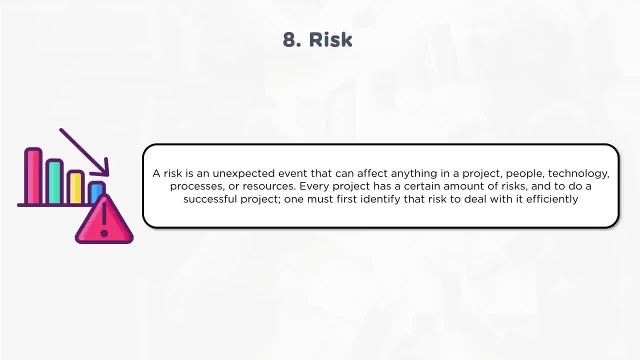 If it is a positive risk, It is quite obvious. One has to take the advantage of that. One has to enhance, exploit, share a positive risk So that organization is benefited Further procurement. So whenever a project is initiated, Whenever a project is taken up, 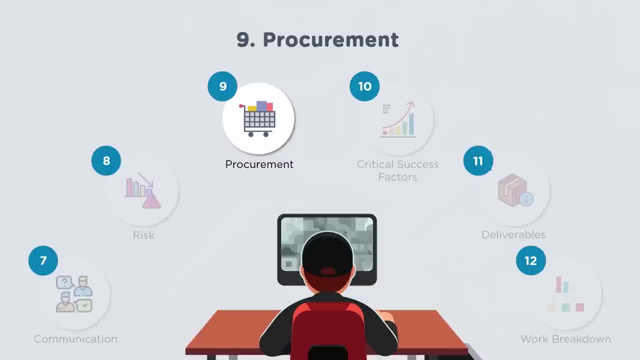 The organization who is doing the project Cannot create everything, Cannot develop everything In that project life cycle. So organization would take a decision, Make a decision stating That some of the deliverables We make ourselves, Some of the products we make ourselves. 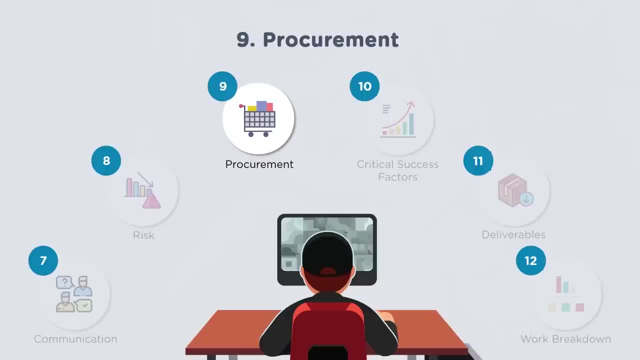 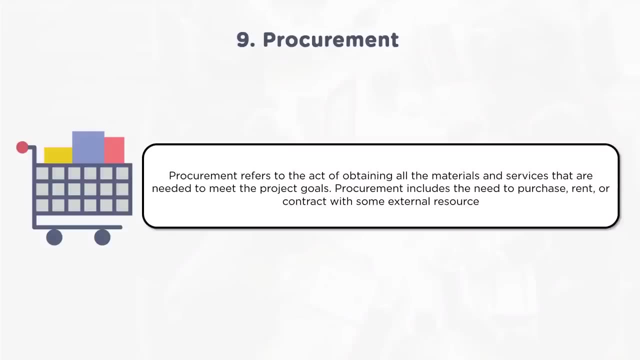 Some of the products we purchase, Some of the services we purchase. So to purchase, That has to happen from a specific supplier. You cannot go with every supplier. You should evaluate the suppliers, Qualify the suppliers And then select on board the supplier. 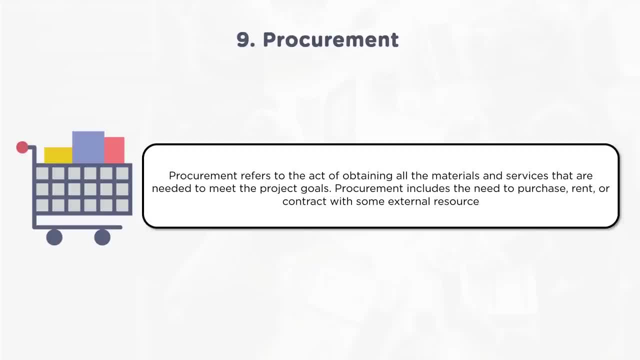 And then get the service, And then get the services or products Supplied by that particular supplier. So while doing this One has to understand What type of contracting they need to enter with. So three types of contracts we speak basically. 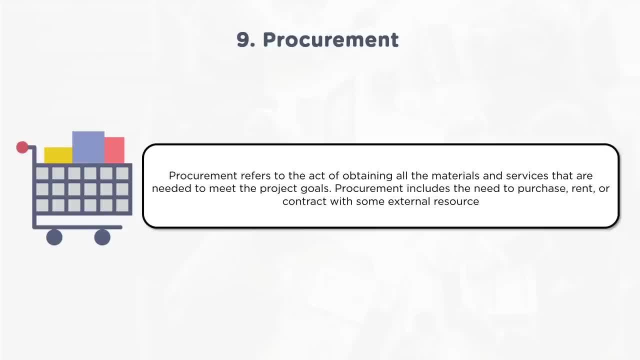 One is about a cost plus contract, Where cost is fully known to the project manager And to the organization. So apart from known cost, A fee will be paid to the supplier. Another one is fixed price, Where project manager or the organization 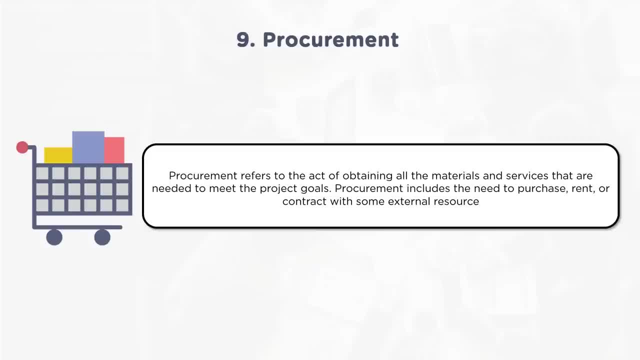 Who is awarding that contract to a supplier Will not know what is the cost. Instead, it is a fixed price. But important here is The scope of work needs to be clearly articulated and defined. Another type of contracting can be time and material. 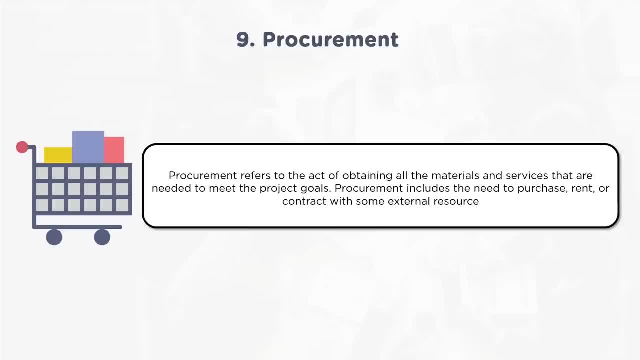 Where the billing will happen, Based on the amount of time one is spent on that particular. I hire a resource or onboard a resource On a time and material basis And what is that effort, That resource has been put? Based on that billing will happen. 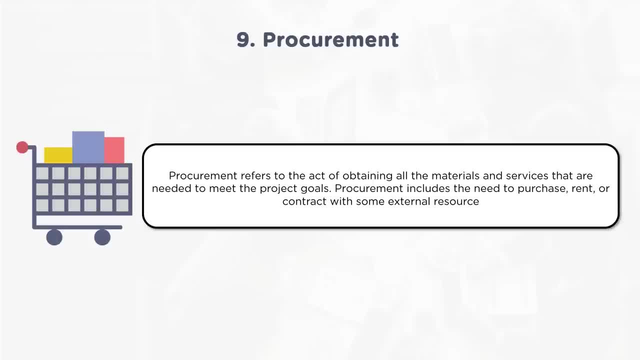 So three types of contracts, Depending on the different scenarios of the project, Will be signed with the contractor. However, Before doing that, It is very essential to identify those suppliers, Sign off with them And monitor and manage them. So if deliverables are not there, 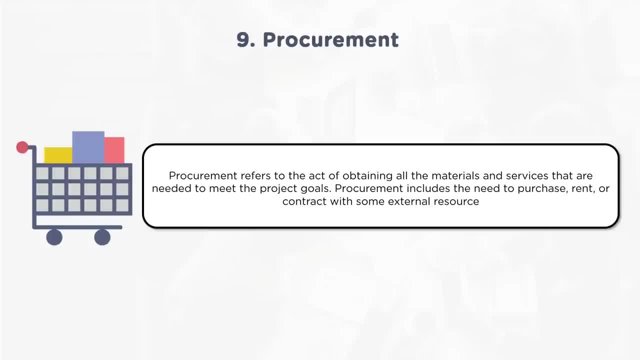 It is very essential to look at the termination. One has to terminate, Otherwise one has to ensure, Instead of terminating Should be able to put some effort To educate them also, So that they come up to the mark, So project is benefited. 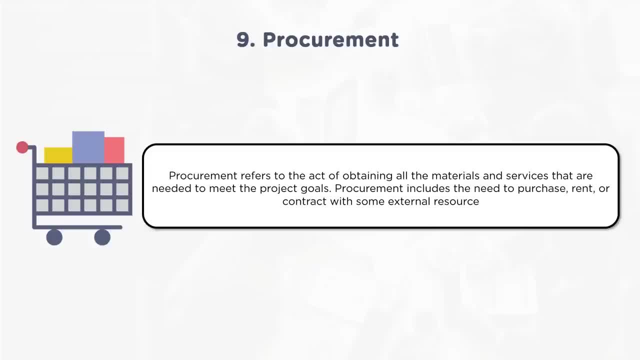 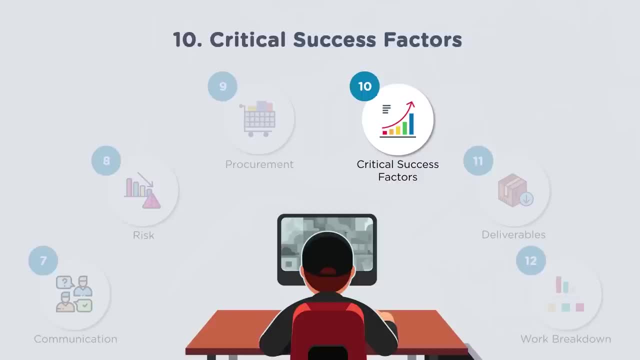 So, depending on what needs to be done, That call has to be taken on a regular basis. Then critical success factor. So for every project There should be an articulation of Critical success factor. So based on that One can confirm: 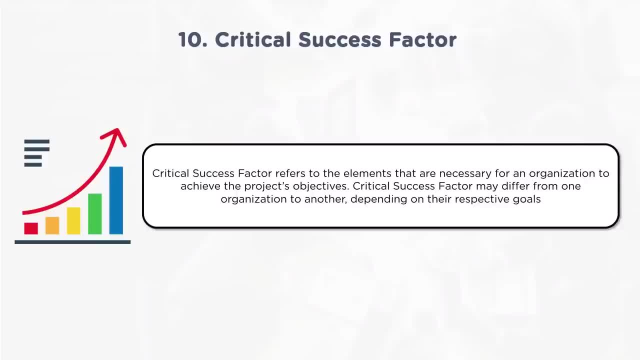 Yes, Project has achieved its objectives Or project has not achieved its objectives. So critical success factor Should be supported through the metrics, Key performance indicators. So key performance indicators Provide those metrics To say critical success factor is achieved. 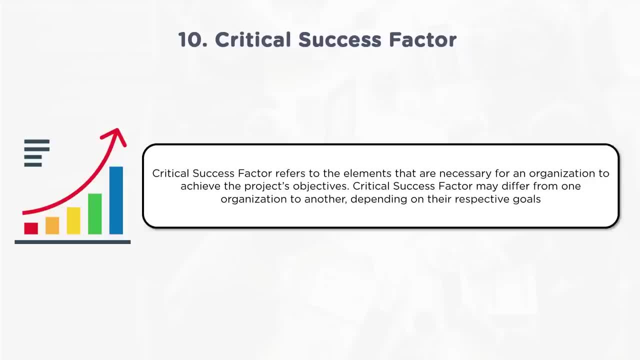 For example, If you want to become successful in an exam, Critical success factor is scoring Or passing the examination. Or let me say, To pass the examination, Key performance indicator is scoring 60% and above. So critical success factor. 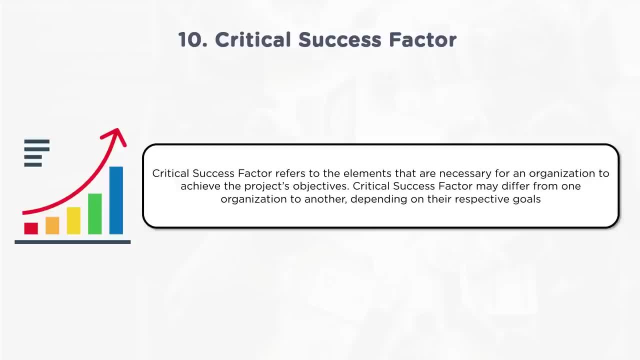 For me to get promoted Is to pass in this particular exam. So to pass in this exam, Minimum I should score is 60%, That is KPI Passing in the exam. That is critical success factor. So how will I measure that success factor? 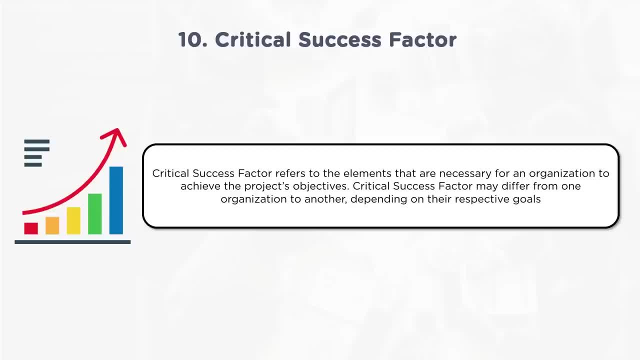 Is KPI, So every project Which it produces a specific product or services By using a specific resources, And each of these- The resources, The processes, The templates, The deliverables, All these Needs to be measured on a continual basis. 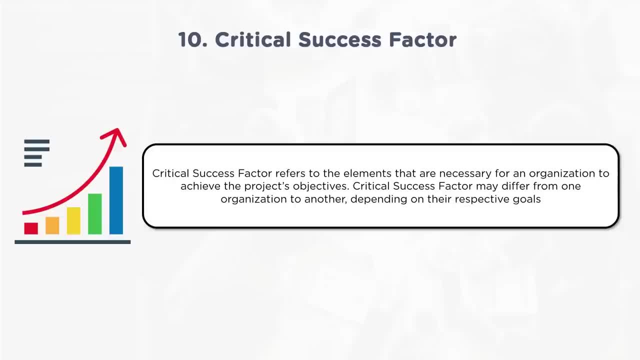 So there are critical success factors defined And those are measured By defining KPIs to that critical success factors. So basically, Critical success factor- provides the insight Towards what needs to be measured And when you measure What should be the focus. 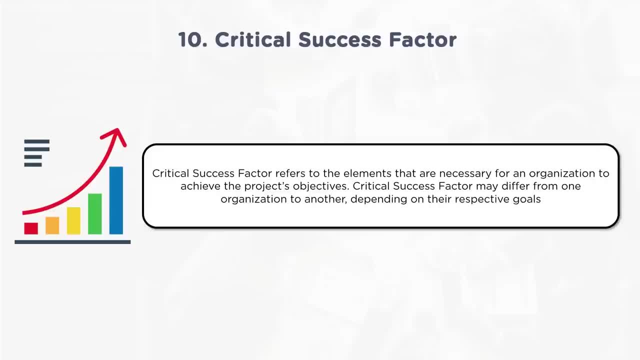 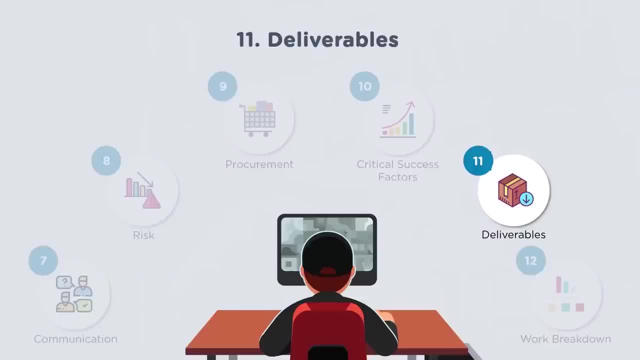 And to achieve those critical success factors, The indicator is Key performance indicators. When you measure, Yes, The moment you achieve that, Your CSF is achieved. Next, Deliverables: So deliverables are those Which comes as an. 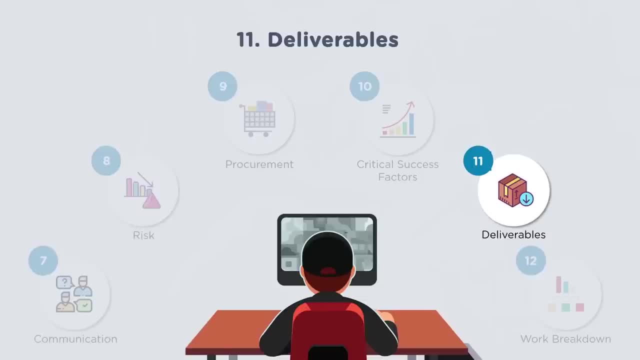 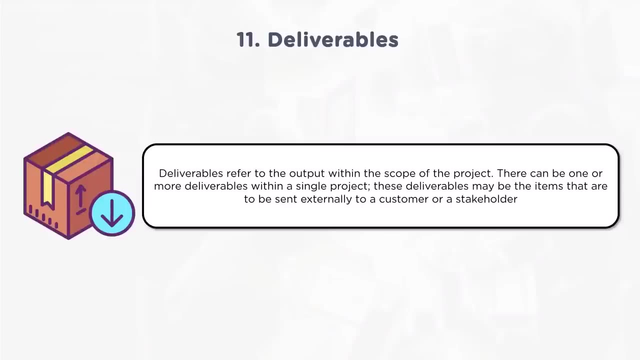 Output of the project. Right, It may be a product, It may be a service, It may be a result. So this refers to the output Within the scope of a project, So there can be one or more deliverables. 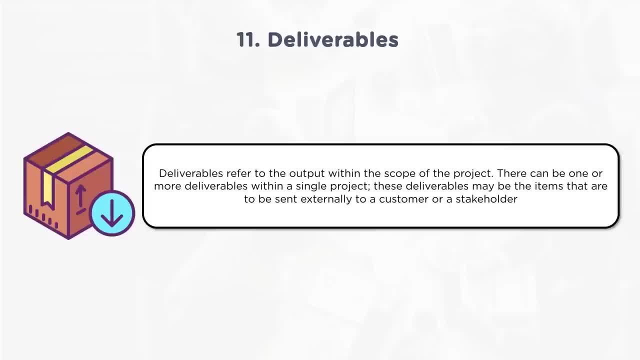 Within a single project. So these deliverables May be the items that are to be sent Externally to a customer or a stakeholder. So every deliverable will have a defined scope, Will have a defined specification. So those deliverables has to be measured. 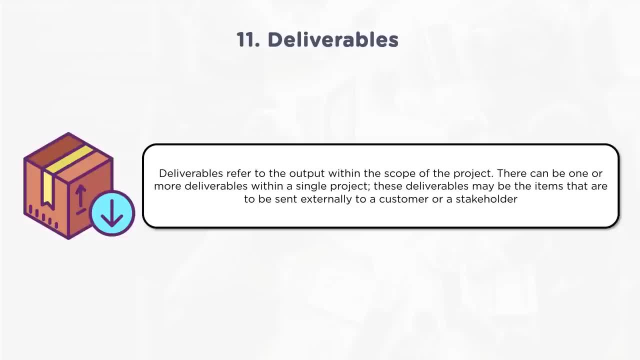 Tested And one has to confirm: Yes, This deliverable is performing As we are intended to have the performance. Accordingly, The decision will happen: Should we accept this particular deliverable Or not. If there any deviation, That has to go back for correction. 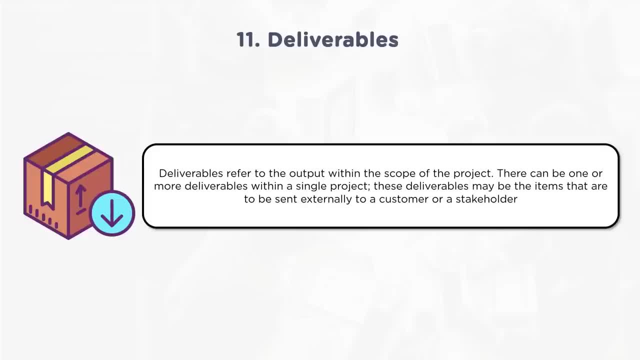 So that's the reason we have monitoring and control, All the control processes, Like control quality, focused on the product trait, Whether it has achieved that results or not, Is that functional as needed or not? One has to ensure these deliverables. 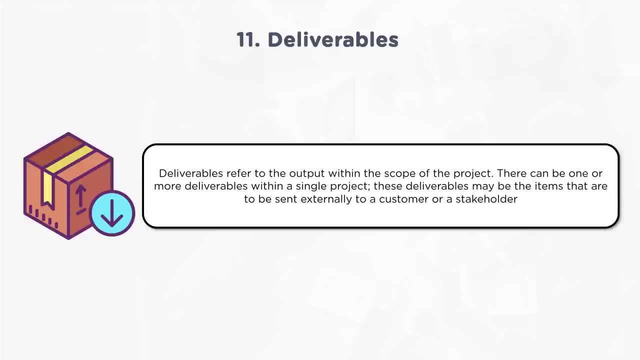 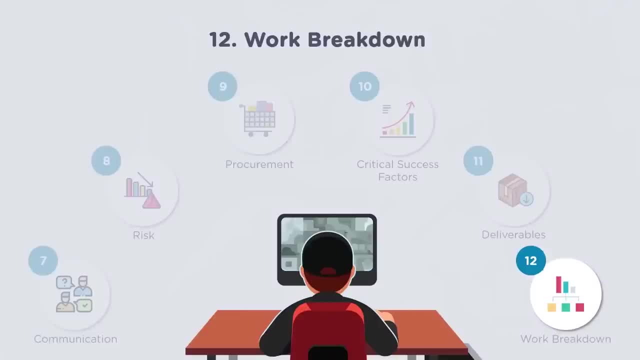 Has all those features and functionalities. Only then that can be handed over to the respective stakeholder, Customer or operation, Whoever the stakeholder it is. Next is work breakdown structure. So when we say work breakdown structure, When I look at a specific piece of product or services, 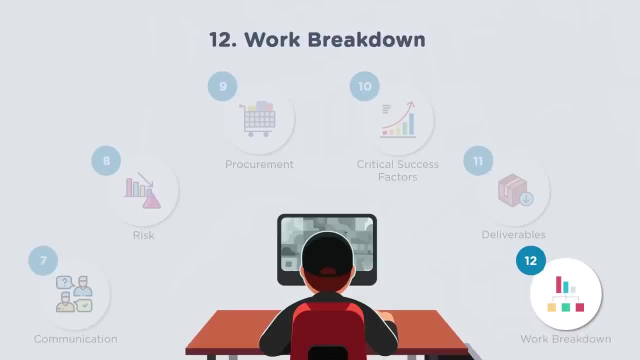 And have a bigger picture. I cannot even visualize the various different components, Various different actions Involved in achieving that bigger deliverable. So if I say a car, So I can think of a body External, I can think of a mirror on that body. 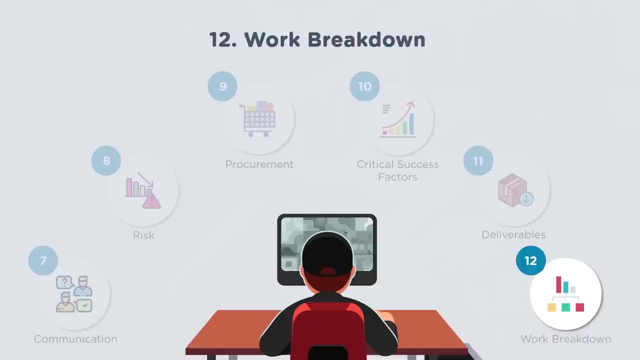 I can think of a glass In the front Side As well as the back side, And also I can think of interiors Like seat, Then accelerator, Steering Dashboard. All these I can visualize, But since I am not a technology expert, 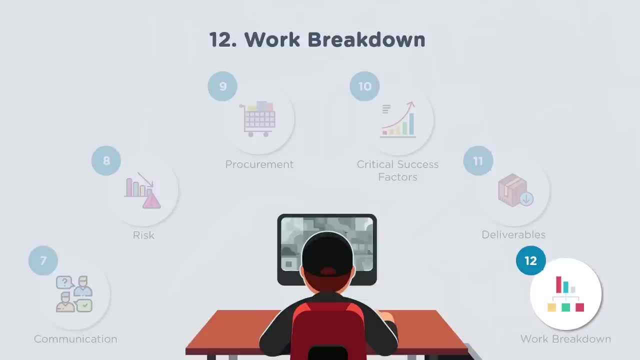 Relating to car. Can I visualize all those parts Which are working inside For car to move, Like engine, The battery assembly? I don't know what to say further. So all these can be visualized by an expert. So every product or services should be broken down into. 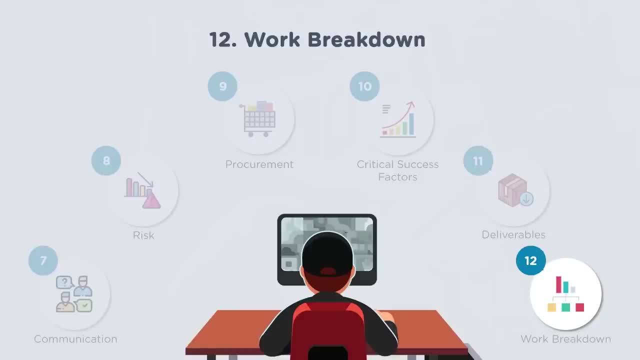 Multiple pieces. I am not saying go and break that product. I am saying That product will have multiple components Which are involved, Those needs to be segregated. For example, If I say Cars Exteriors, Cars Interior. 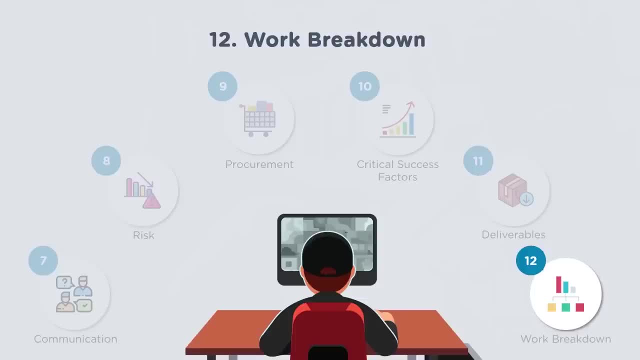 So cars, Exteriors, External items, You can see Whatever you visualize: Body, Body structure, Mirror, Mirror assembly, Headlights, Then tires. So likewise, Whatever I can visualize, I will make it as a. 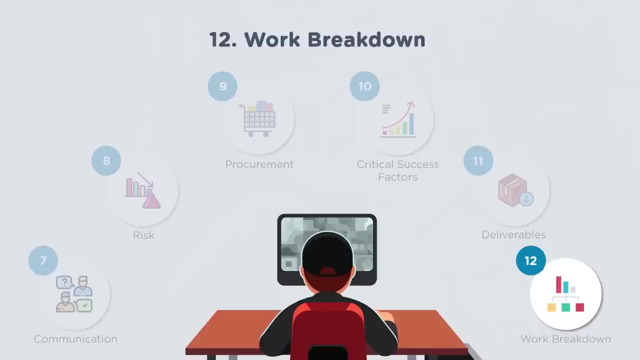 Line items: Mirror Mirror. I can speak about Mirror glass, Mirror cap, Mirror pedestal And mirror Assembly, Where it moves, Where you can move the mirror. So these are the various components Involved in a mirror. 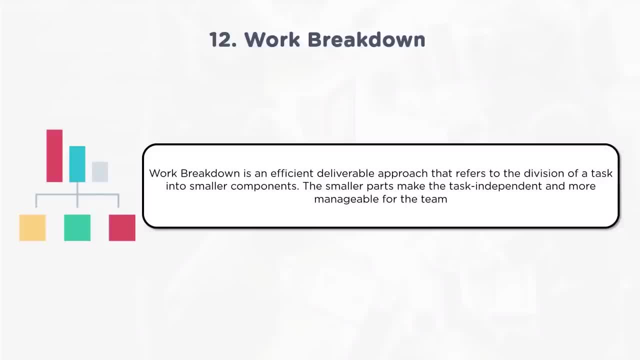 So I need to ensure By breaking down The product Into multiple levels, By decomposing Into multiple levels, I can able to visualize the product Very clearly, What is there In detail. So once I have the details, 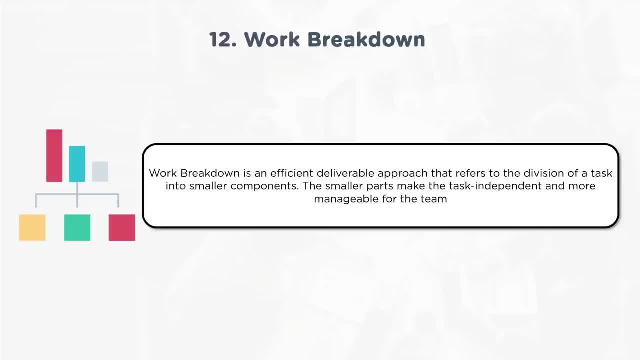 I will Articulate those. What is that particular Work breakdown Element is? Then I will look at What skills And capabilities Required for that product And I will assign the Resources accordingly. So once Activities: 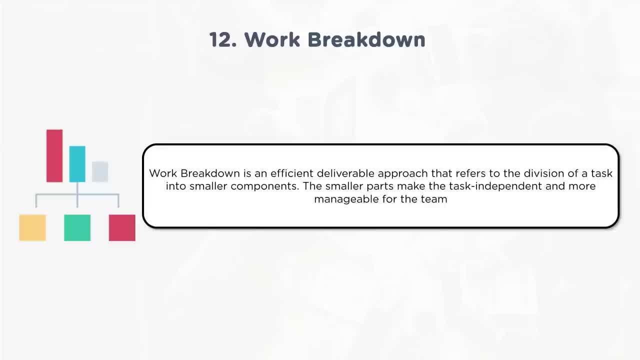 Resources. Everything is assigned Automatically. This will become A work breakdown structure. Further, After creating A work breakdown structure, One will go and Sequence the activity. Look at Sequencing will happen Based on In what priority. 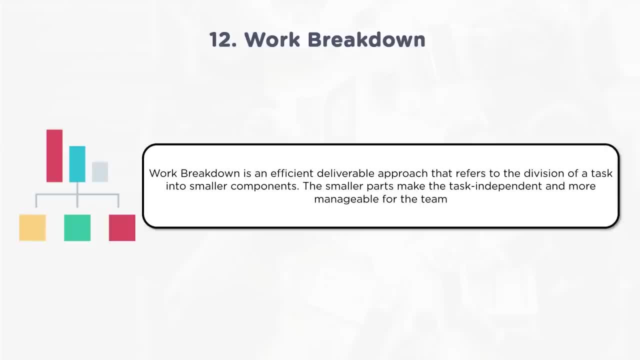 Deliverable should happen. In what order Deliverable should happen? Then, once the sequencing is done, It will be checked To see whether Done in such a way That smooth flow Of the project Can happen. There is no dependencies. 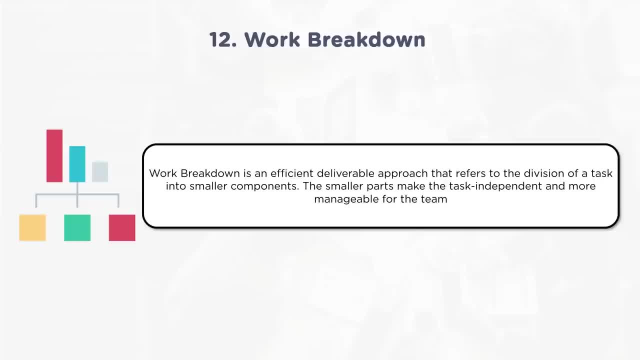 Which will make Project to delay, Like as the flow Happens smoothly. So you would find The Various techniques, Like critical path method, Network diagramming, Critical chain method, So all these are used, The floats. 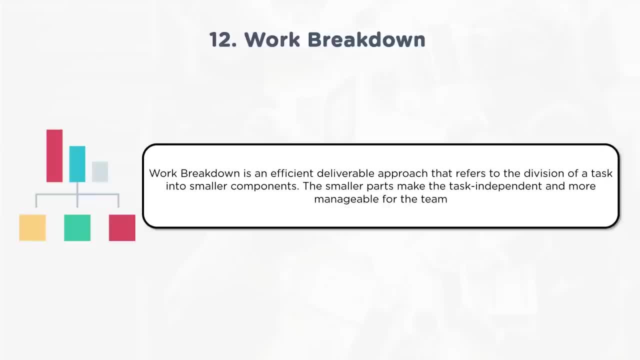 Of an activities Are checked, Then leads And lags Of the activities, The relationship Between activities. So, accordingly, Full visualization In terms of How the project Will flow And how The work will flow. So that is the reason. 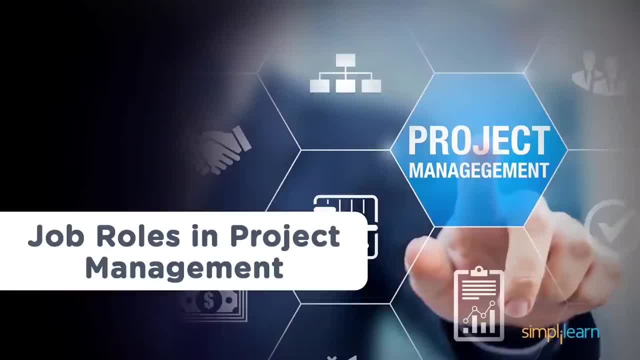 First activity Is to do the Product breakdown, Which would result in Work breakdown structure. So those are the points Till now. Whatever I mentioned Are the basic Understanding One should have About a project And project management. 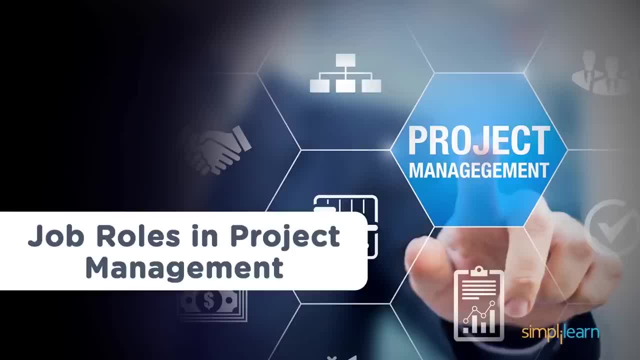 So as you Deep dive into Various best practices Like PMP By PMI PRINCE2.. By axolos Scrum master, Agile scrum master. Similarly, You have Certified scrum master. 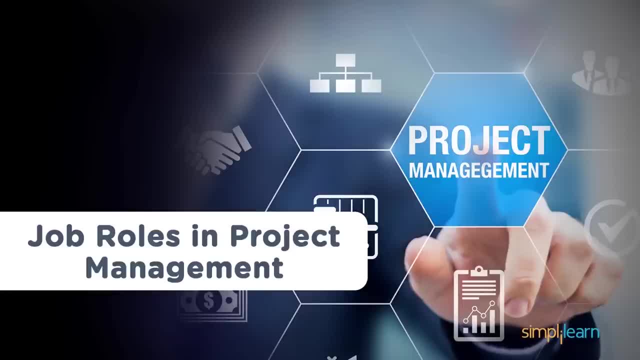 So many agile practices That will tell you Clearly, Articulate, What should be The practice For you To Adopt, And adapt That practices So that your project Can become successful. So any of those, 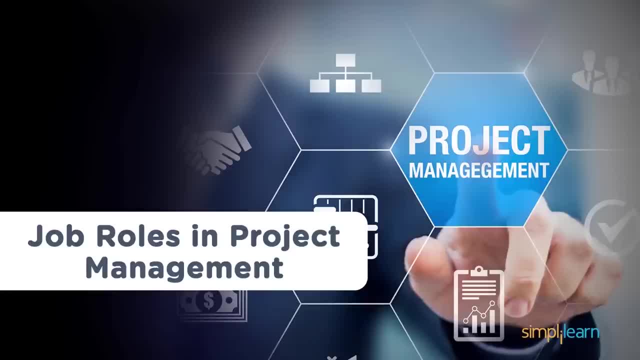 Approach You touch upon All those Refers to These basic Things. In the absence Of these basic Things, None of those Best practices Discusses The project management. Now, Typically In the industry, There are many. 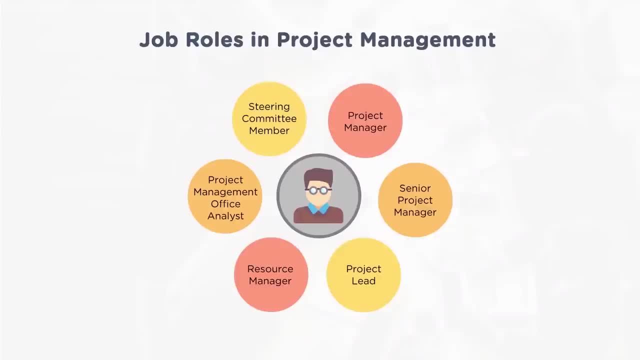 Project managers That are Captured here On various Job rules In a project management. So Some of them Are like Project manager, Senior project manager, Project lead, Resource manager, PMO. That is project management. 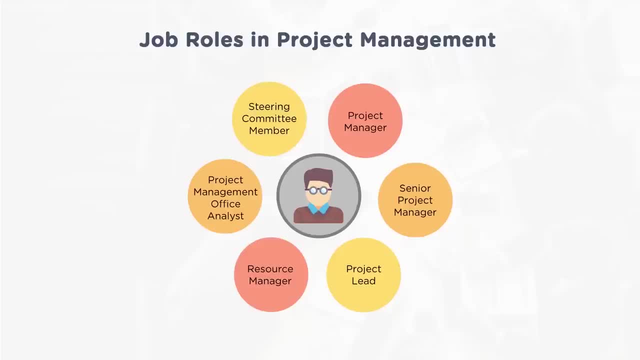 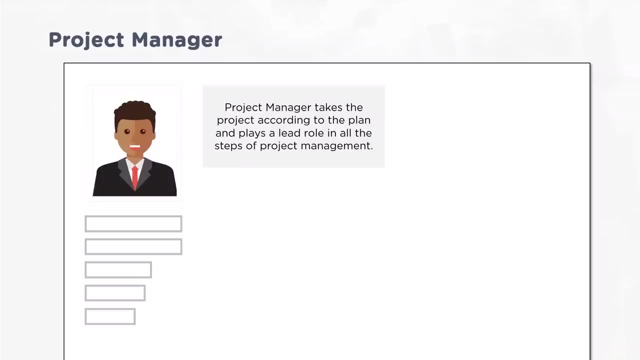 Office analyst. Steering committee member. So Not necessarily All the project management Roles are limited To this. So These are the roles Which commonly You see, And we are trying To capture that. So Project managers. 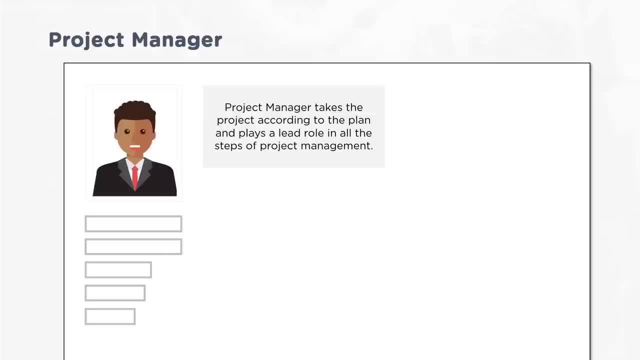 Takes the project According to the plan And plays A lead role In all the steps Of the project management Right, So Responsibilities Would be Managing, Reviewing And prioritizing The task Wherever necessary. 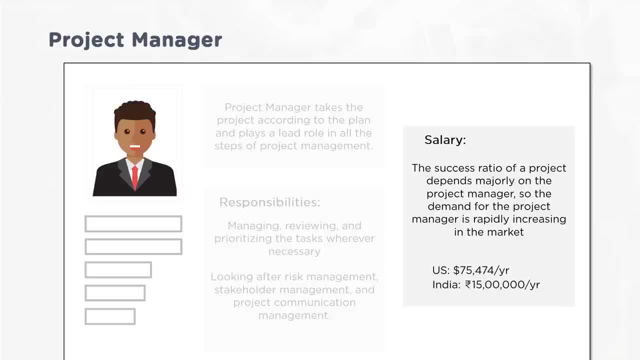 Looking after Risk management, Stakeholder management And project Communication management. Some of the Salary, What we found While We were Doing the survey, The success Ratio Accordingly: Seventy five Thousand Four Seven. 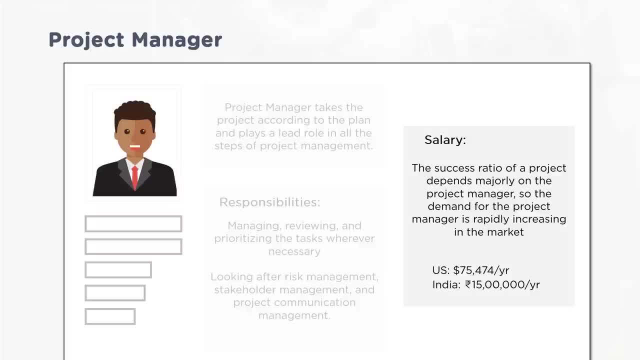 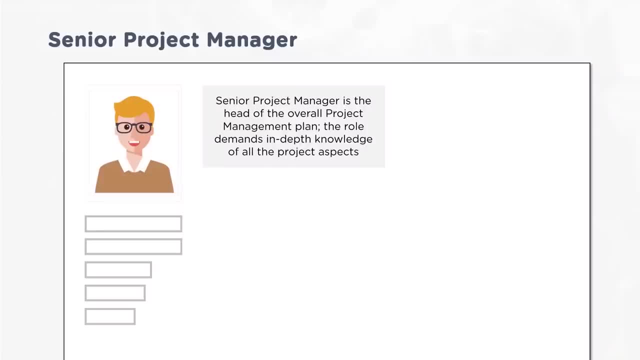 Four Per Year. That is The USD. In INR It is Fifteen Hundred Thousand. So This Is What The salary, On an approximation What Was Found? Next Role: 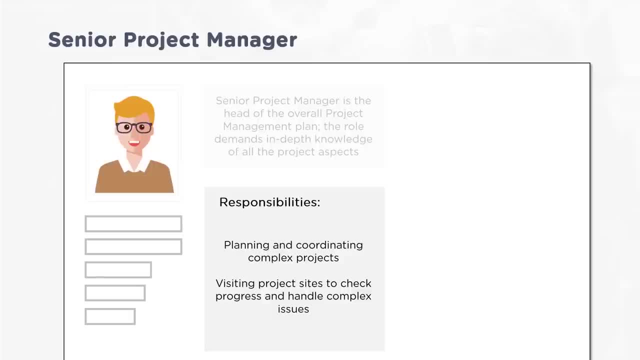 We look At Senior Project Managers And Handle Complex Issues, So Salary Looks Like One, Not Four, Thousand Dollars Per Year. Year Twenty, Ninety, Two Thousand. 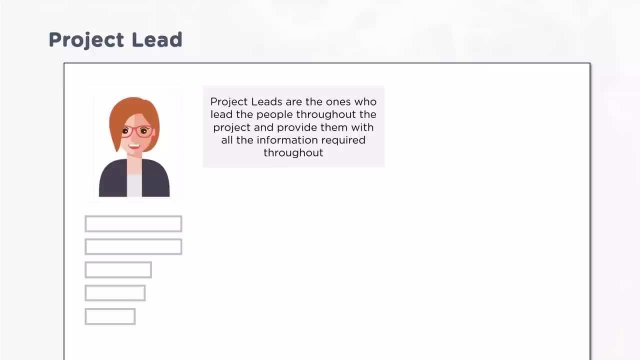 INR Per Year. So The Role Of Senior- And Provide Them With All The Information Required Throughout. So Responsibility Is Involved. Motivating The Team. 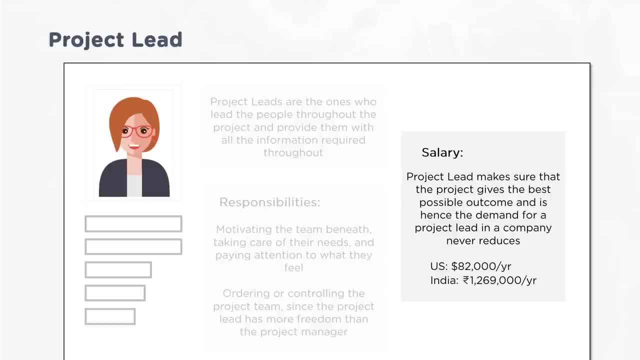 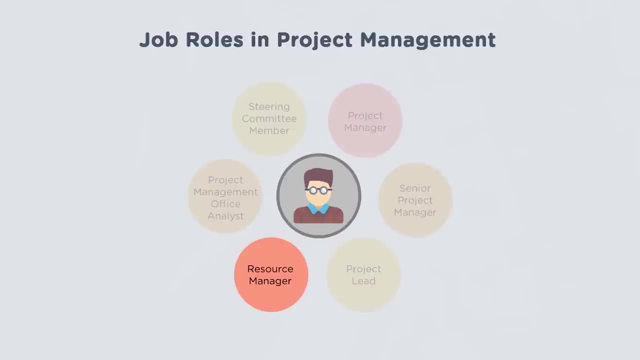 Beneath, Taking Care Of Their Needs And Paying Attention To What They Feel Is One Million Two Sixty Nine Thousand Per Year. Next Role: 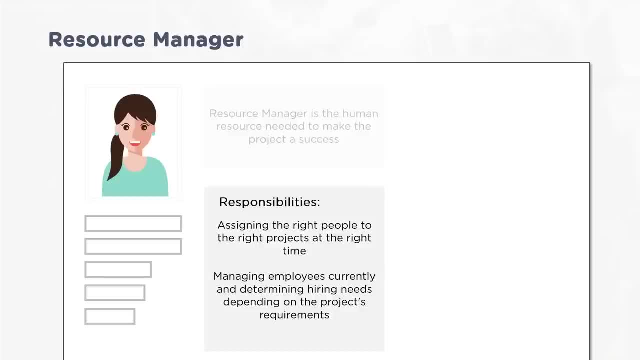 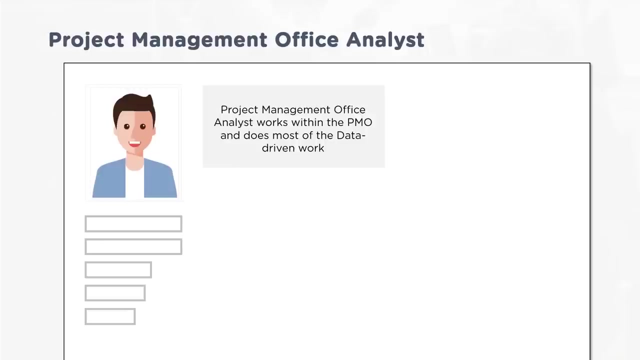 Look At On Resource Manager. So Resource Manager Is The Human Resource Needed To Make The Project Success. Project Management Office Analyst For This Role, The 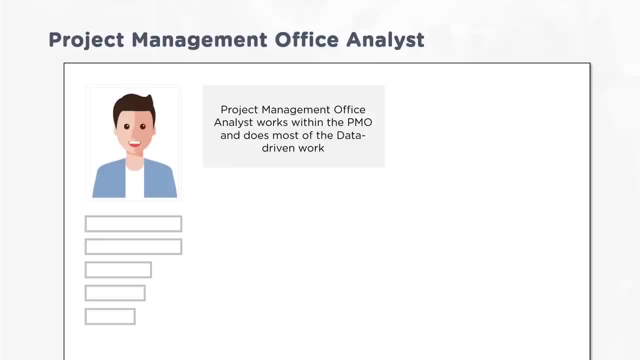 Project Management Office. Analyst Works With PMO, Means Project Management Office And Does Not Look At The Project Or Manage The Project Management. So Salary: 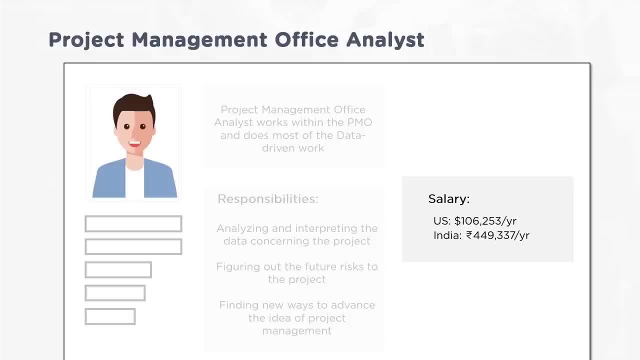 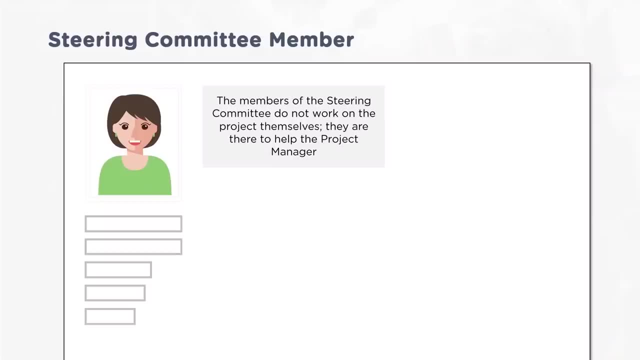 Would Be $106,253. Per Year In USD, Whereas $449,337. In INR Per Year. So Steering Committee Member. So The Steering Committee Members. 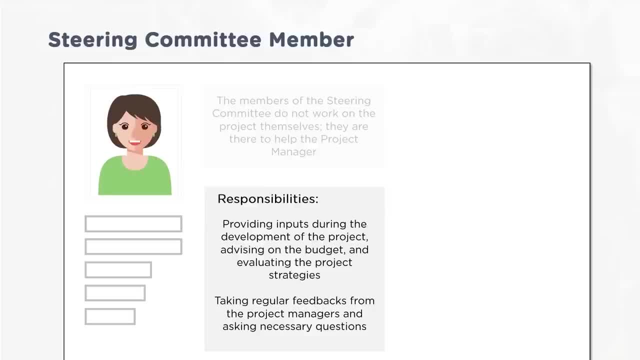 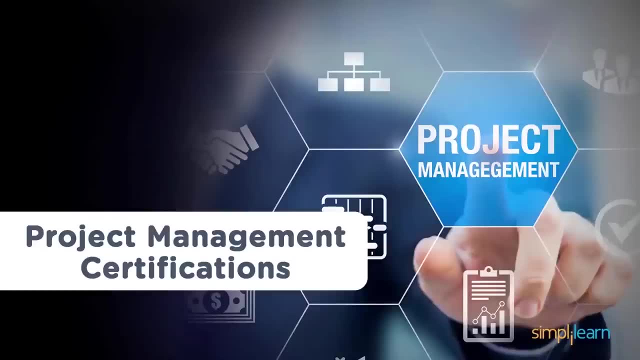 Are The Members And Asking Necessary Questions. So Salary Would Be Around $68,497. Per Year. So Those Were The Various Roles And That Is. 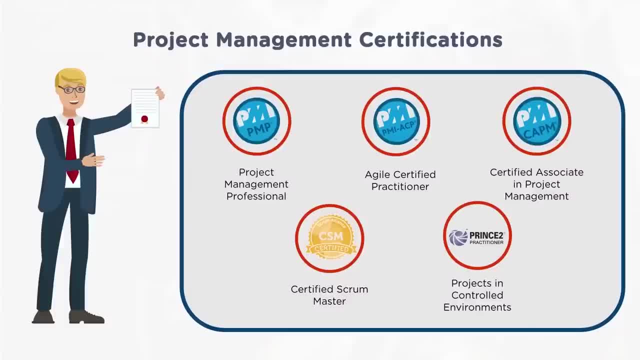 Not An Exhaustive List, Various Different Roles. We Have Topic For You As At In In The Project Management Is As One Project Management In. 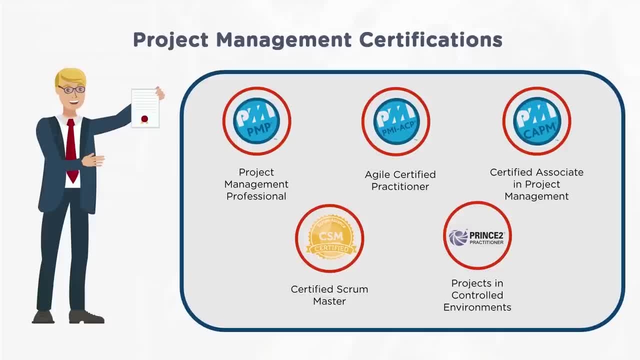 The Project Transition In The Program. This Is A More Important In scrum master certificate, which will explain the role of a scrum master in detail. similarly prints to a certification from axelos, which also 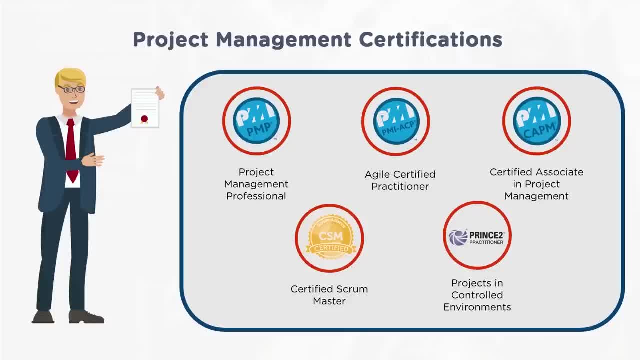 speak about all the aspects of the project, what we discussed and provides the framework for project management. axelos also provides prints to certification in agile- also agile prints to certification. so we will look at each one of this, certain details which are required for us to know. so project. 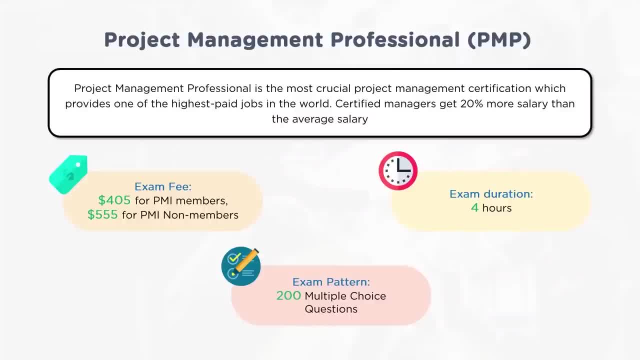 management professional, as I mentioned, is most acknowledged and value the certificate, value what it carries, which has resulted to the certified professionals in landing up in highest paid jobs in the world. so certified managers gets 20% more salary than the average salary. so to take up an 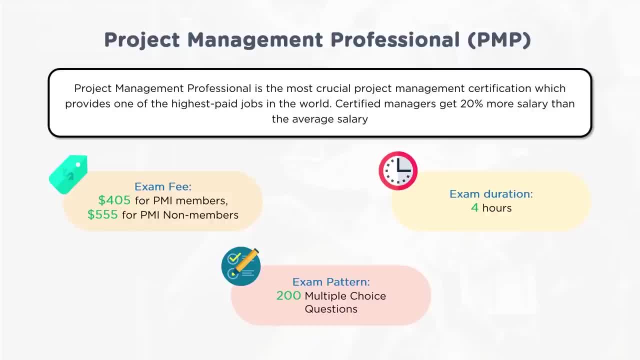 examination one has to go through the formal training of 35 hours. that is one of the prerequisites and there should be some experience of 4500 hours of project managing by leading the various activities of the project. and once the person becomes eligible with that prerequisites person will become registered in the PMI's. 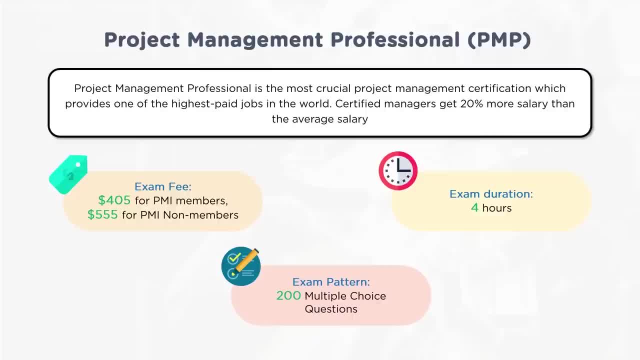 website, becomes member and then go for examination. so examination fee for PMP would be 405 dollars for the members who are registered with PMI and for those who are not registered as a member with PMI it is 555 dollars. the duration of the examination is 4 hours and the number of questions will be 200, which 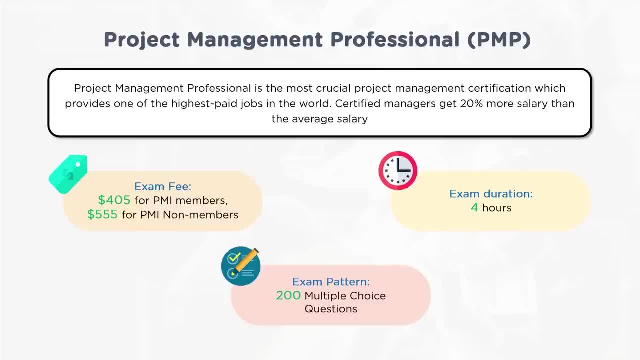 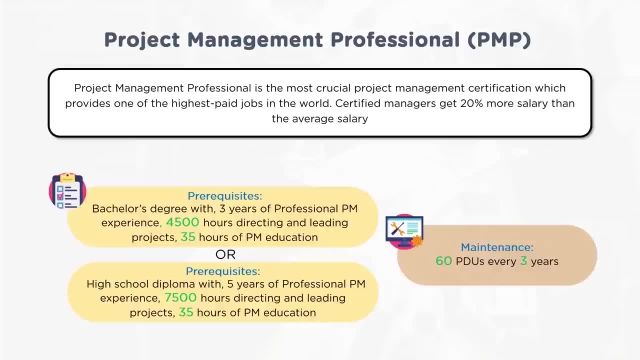 are multiple choice questions, so each each questions carries one marks. there is no negative score. now prerequisites: one has to have four thousand five hundred hours directing and leading the projects. that experience has to be filled in while filling the application if a person is a bachelor degree holder and along with that, thirty five contact. 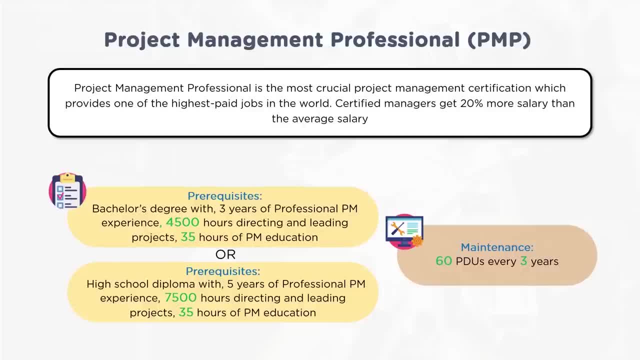 arts of PMI, PM education. now, prerequisites for the one who is not a graduate, who may be high school or diploma, is seventy five hundred hours of directing and leading project, thirty five hours of PM education. so those are the prerequisites before one will go on appear for examination. so once an 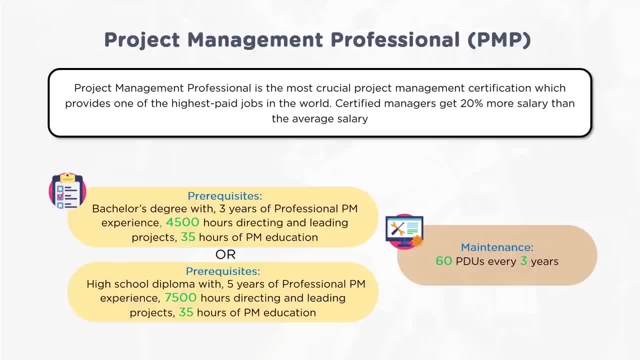 individual passes PMP examination, that certificate is valid for three years. so now, after three years, if the person aspires to keep the certificate continued, they need to produce 60 PDUs- professional development units- which has to be acquired during those three years. how to acquire one has to go through. 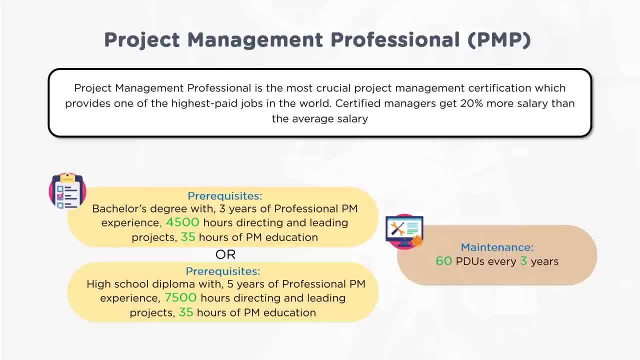 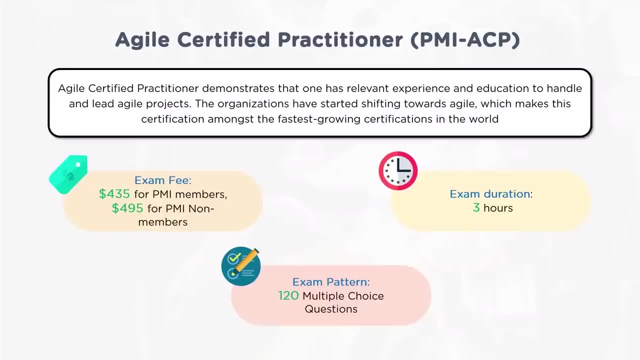 additional learning. one has to contribute towards project management knowledge base, so those needs to be evidenced and then renewal fee has to be paid and certificate has to be renewed. then agile certified practitioner, as we saw for PMP here, agile certified practitioner demonstrates that one has relevant experience and education to handle and lead agile projects. the organization has 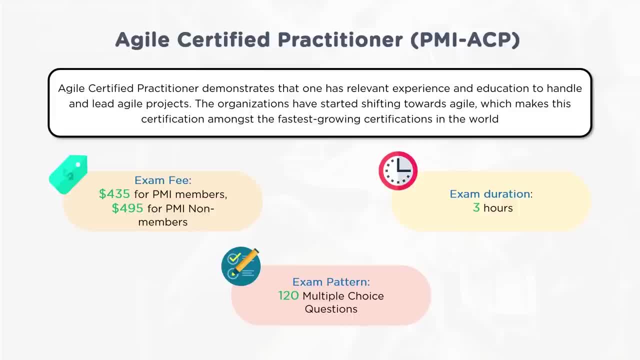 started shifting towards agile, as we know in today's industry, which makes this certification fast growing in the world. so examination fee would be four thirty five dollars for PMI members, four ninety five, four hundred and fifty five dollars for PMP. so that means that one has to be. 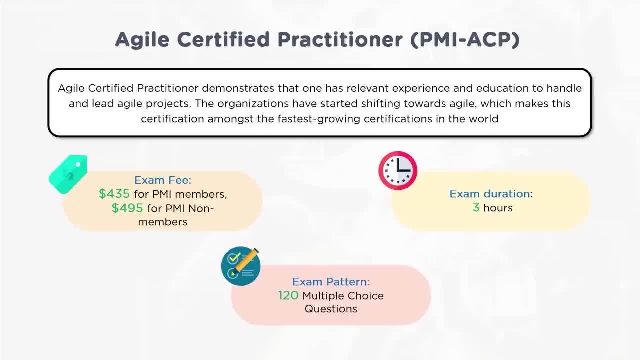 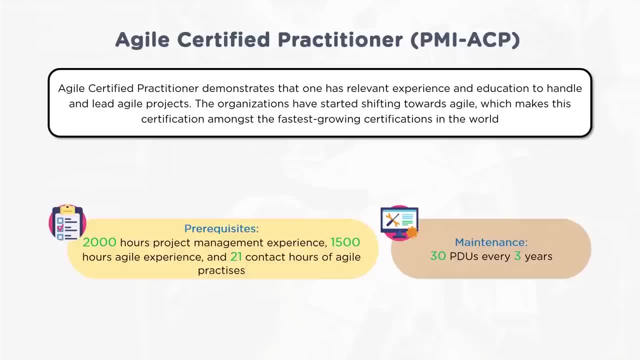 certified for non-PMI members. duration is three hours and multiple choice questions: 120 questions. prerequisite says two thousand hours project management experience with thousand five hundred hours agile experience and 21 contact hours of agile practices. so maintenance: 30 PDUs are required for every three. 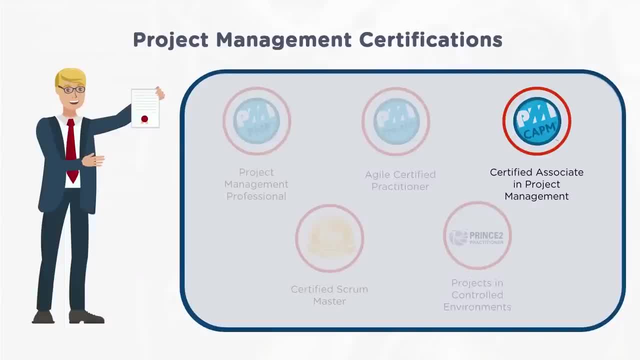 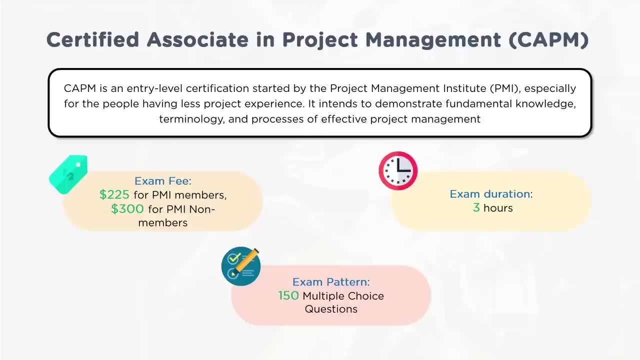 years and, after paying the renewal fee, that can be renewed now. certified associate in project management. so here this is an entry-level certificate of PMI, especially for those people who has less project experience. it intends to demonstrate fundamental knowledge, terminologies and processes of effective project management, so examination fee would be. 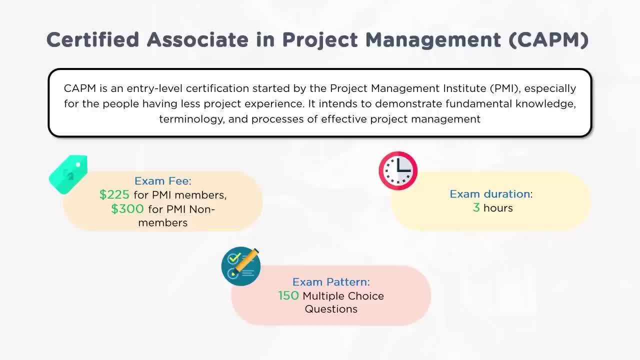 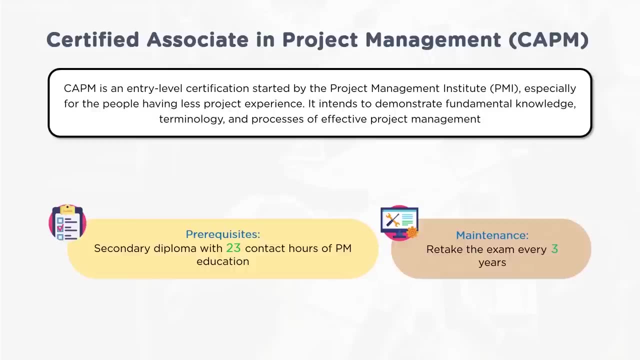 dollar 225 for pmi members, whereas 300 dollars for non-members of pmi. so duration of examination is three hours and examination will have 150 multiple choice questions. so prerequisites: someone who has secondary diploma, 23 contact hours of pm education is enough. there is no experience of doing the. 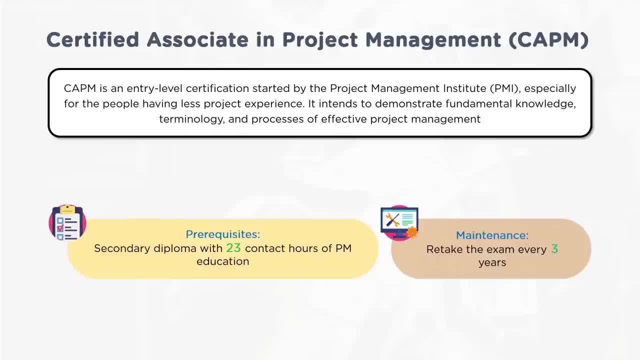 project is required, as we saw in pmp. so maintenance is again three years. someone who need to continue the certification has to retake the examination every three years. next, certified scrum master. so certified scrum master is an entry level certification that helps the professionals to. 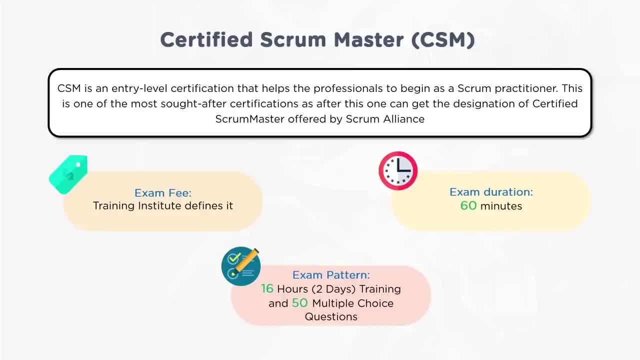 begin as the scrum practitioners is one of the most sought after certifications as other. after this one can get the Designation of certified scrum master, which is offered by scrum alliance. so examination fee which will change time to time, which is not revealed, So one has to approach the training organization where they will get trained on certified scrum master. 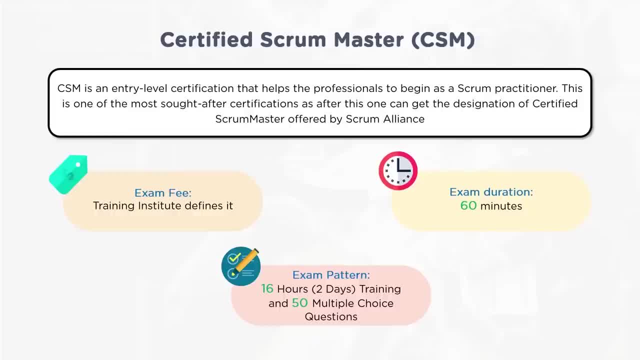 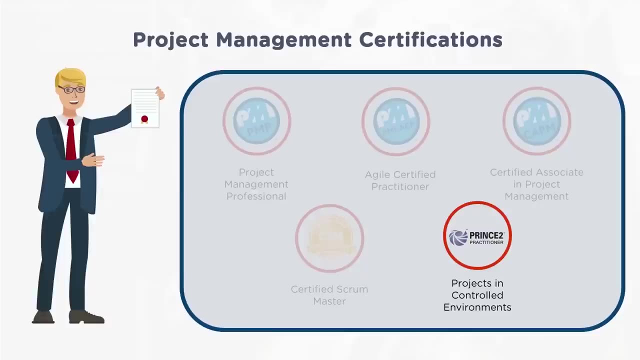 So duration of examination is 60 minutes and pattern would be 16 hours, two days of training and 50 multiple choice Questions. after that particular two days of training, then prerequisite is done for maintaining these credentials. So one has to ensure it has renewed every two years. then projects in controlled environment. 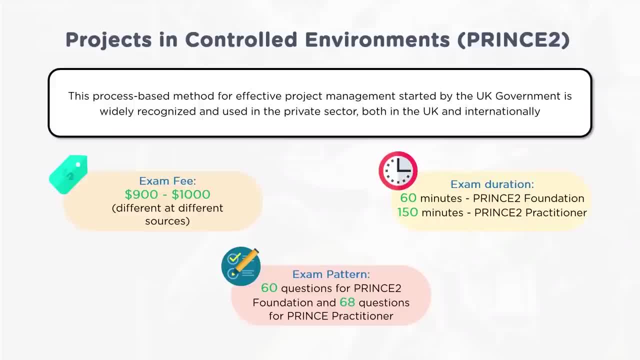 That is prints to. so prints to is a method which is effective mostly from the base of UK- all the organizations Who are from UK region refers to a prints to Certification and it is as popular as any other project management certifications like PMP. So examination fee would vary from nine hundred dollars to thousand dollars depending on where exactly you're taking the examination and 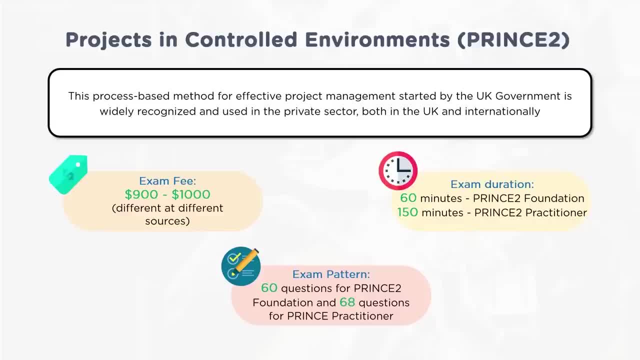 Certification will happen at two levels. one is at foundation level and other one is practitioner. So in foundation it is 60 questions, multiple choice, and in practitioner It is 68 questions. now 60 questions or 68 questions: each carries one marks for correct answer, any wrong answer. 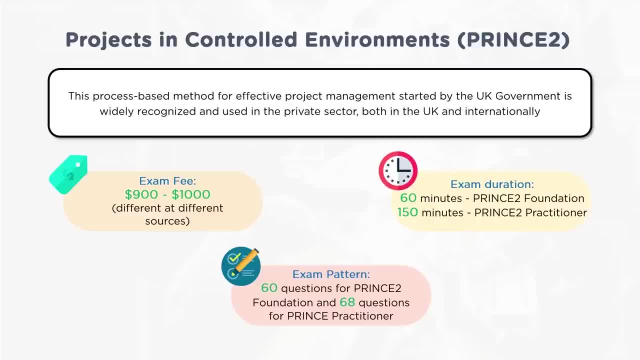 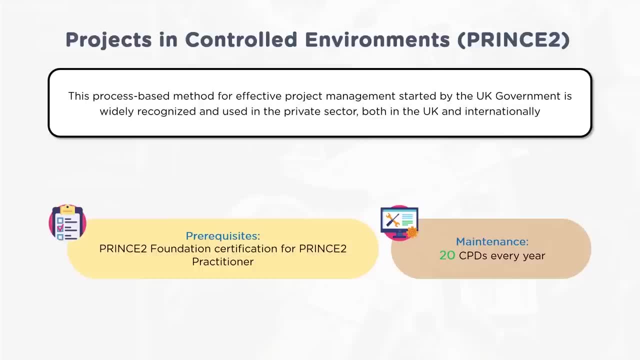 There will not be any negative scoring. one has to score 55 percent to clear the examination. So prerequisites for prints to foundation is none, whereas prints to foundation is a prerequisite for prints to practitioner examination. So to maintain the certificate one has to achieve 20 CPDs every continued professional development. 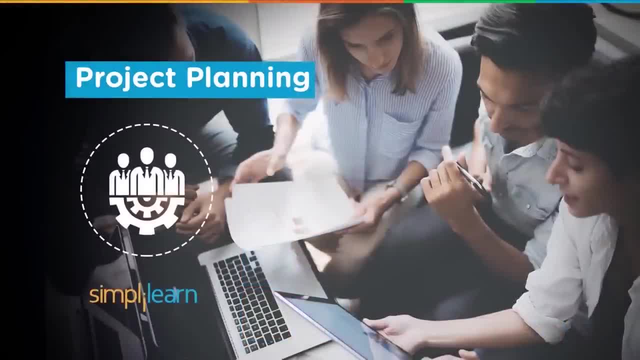 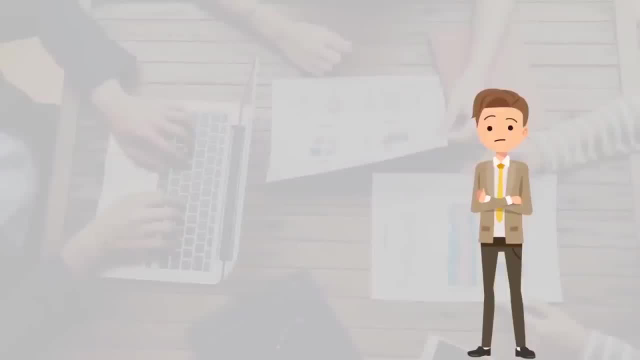 Hi guys, my name is Ishan and I welcome you all to this session of project planning. today We will be learning about different aspects of project planning, but before we begin, Let's have a look at an incident. Here's max, an assistant project manager, who looks tensed and is pacing around the room. 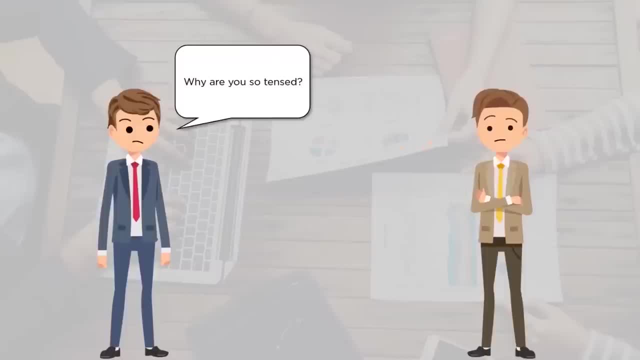 Then Jack, a project manager who works with him, walks into the room and asks him: Why does he seem so tensed, Do it? Max replies he's facing difficulty in estimating the budget. Jack responds It might be because he is not planning the project properly. Jack reassures max and begins to tell him about project planning. 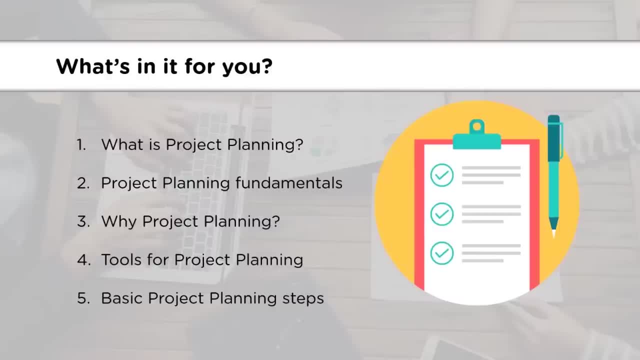 So today we will be learning about what is project planning and check out the fundamentals of project planning. Then we will see why project planning is so essential for a project to be successful. after that We will check the tools for project planning and finally, we will have a look at these steps for project planning. 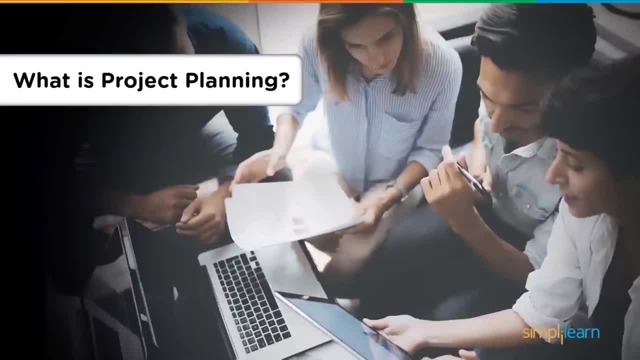 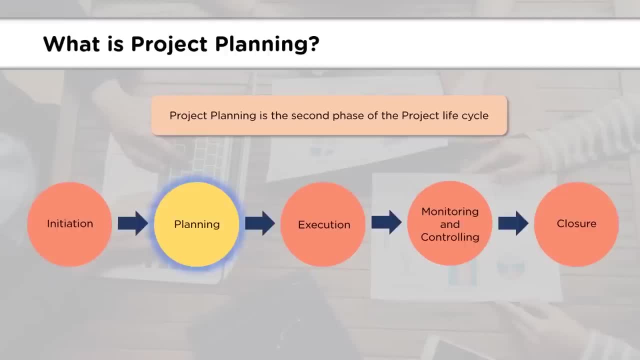 So, without any further ado, let's begin with. what is project planning? project planning Is the second step or phase of the project life cycle. project life cycle as five different phases, from initiation to closure. today, We will be learning about this phase that comes immediately after initiation, in which the project plan is. 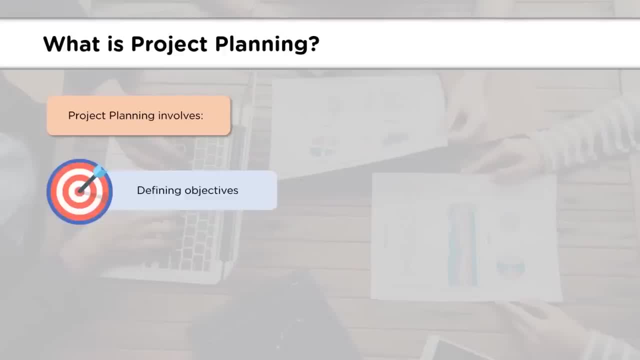 Documented and further requirements are defined. project planning includes the following things. The first and foremost thing is describing the objectives or outputs We are expecting the project to yield. Second we have is the elaboration of the scope, to make sure what the project is all about and what all can be expected. 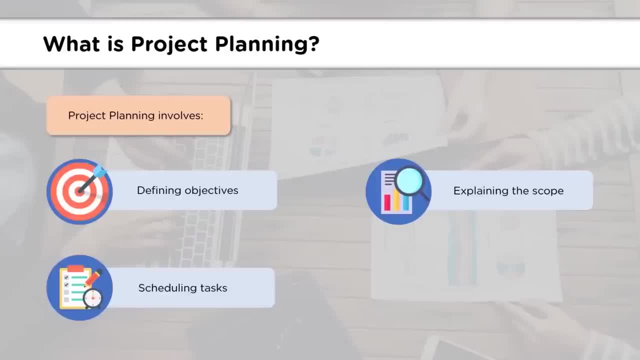 From the project. the third step we have is forming a schedule. This schedule is important to run or perform different tasks of a project, each task having its own start date and end date. This helps a project to finish in the scheduled time and limit. Lastly, we have making and generating progress reports, in which all that went during the tenure of the project is documented. 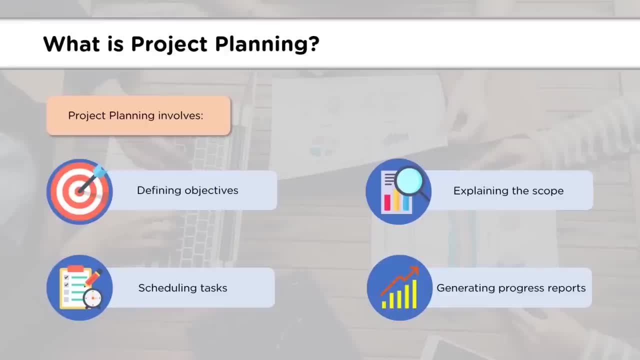 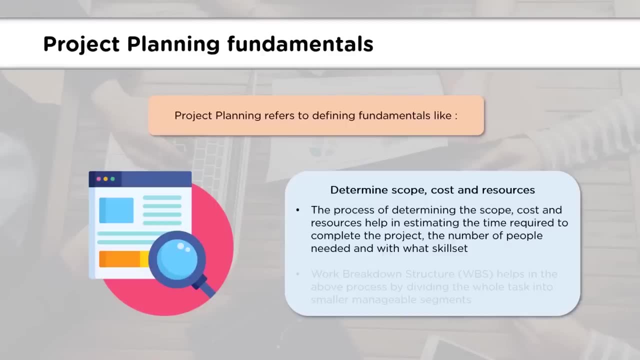 This helps in evaluating the project and helps in the forthcoming projects. Now let's have a look at the project planning fundamentals. The first fundamental that we have is the determination of success, Scope, cost and resources. their determination helps us in having a rough estimate about the time that is required to finish the project. 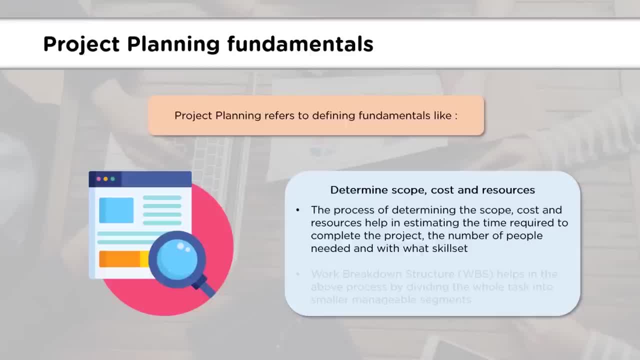 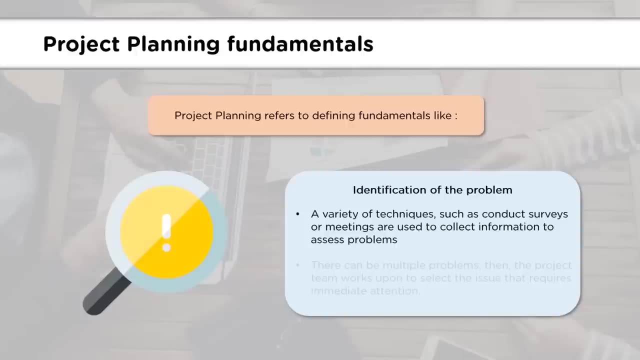 It helps us in determining the number of people required and what should be their skill set. We can divide the project into smaller, manageable sections, and this is made possible with the help of work breakdown structure. The second fundamental refers to identifying the problem. There are several techniques by which we can collect information and discover issues. 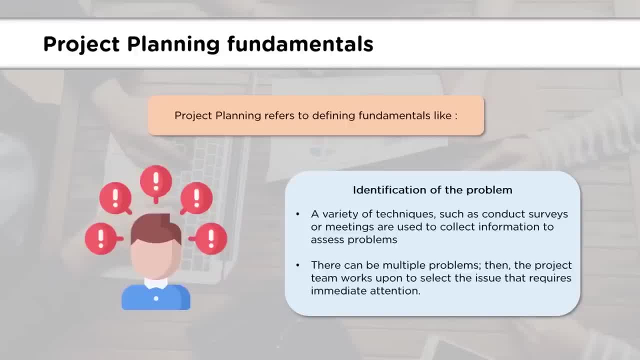 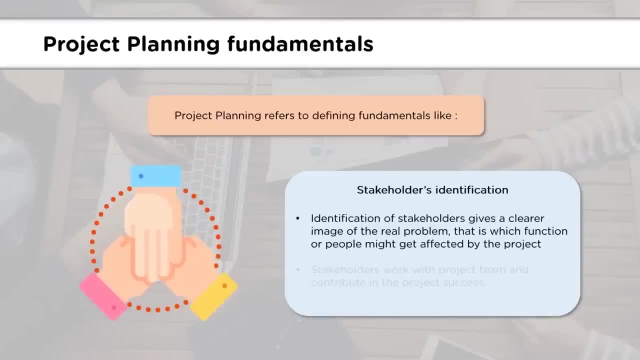 There may be several problems in a project and in that case several risks or issues are prioritized and the risk that requires immediate attention is dealt with first. Then comes identification of stakeholders. When we can identify the stakeholders, we can know who all will be affected and in what way. 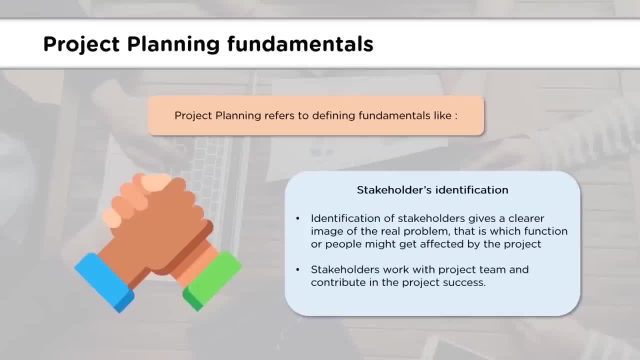 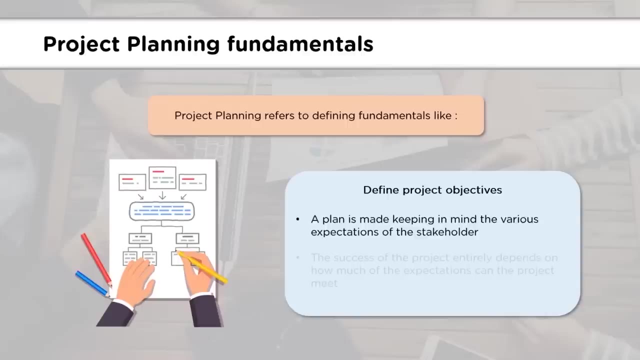 which helps us having a better understanding of the project. Stakeholders may be anybody. They may be the part of the project team, or project managers or customers. They help during the project and contribute to its success. Then the last fundamental we will discuss is defining project objectives. A project plan is made keeping in mind the requirements of the project. 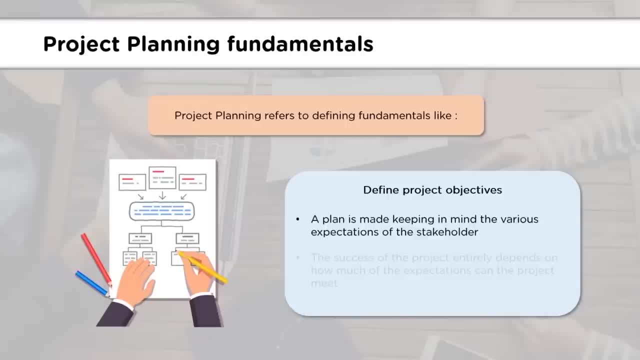 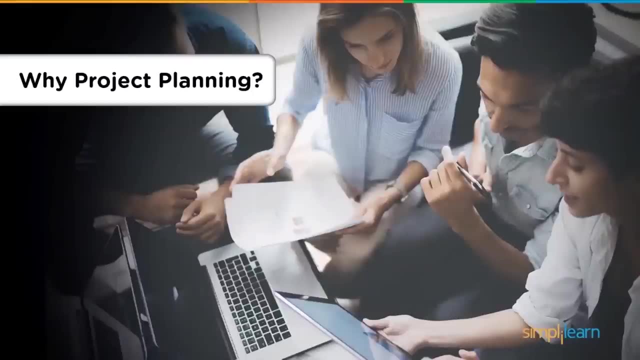 A project plan is made, keeping in mind the requirements of the project, The project team and expectations of the stakeholders. If the project team can meet the expectations of the stakeholders, then only we can say that the project is successful. Now, when we know about project planning and its fundamentals, 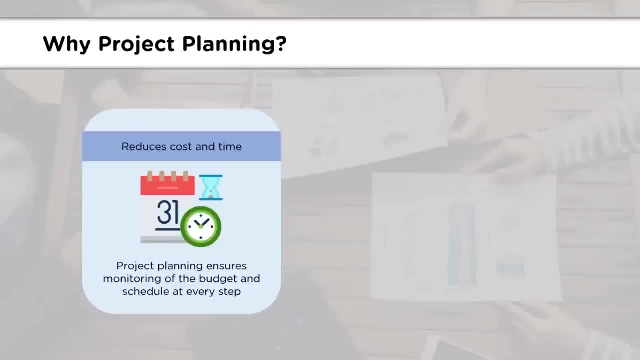 It's time to see why project planning is so important. Project planning reduces the cost and time of the project, as every step is monitored and optimized in the best possible manner. Project planning increases employee satisfaction as every employee who is a part is engaged in the team for improved project performance. 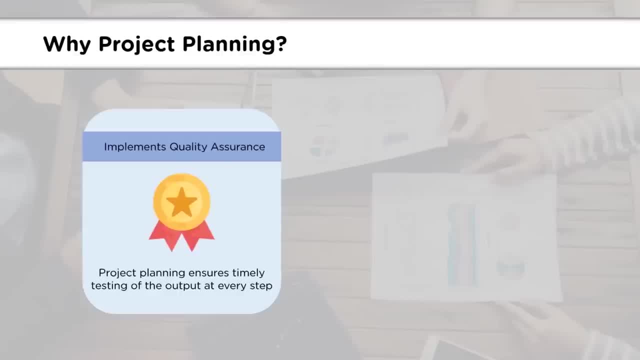 Project planning helps in the implementation of quality assurance, as the output of every step is duly tested. Lastly, project planning helps in reducing project risk, as planning helps to analyze, prioritize and deal with that risk. Moving on, let's have a look at the tools for project planning. 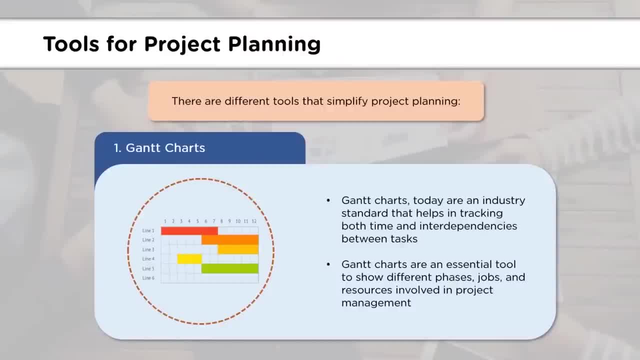 The first tool that we have is a Gantt chart. Today, Gantt charts are one of the most popular project management tools. They help in tracking the status of the work at a particular time and their independencies on each other. Gantt charts help in showing different phases and steps involved in a project. 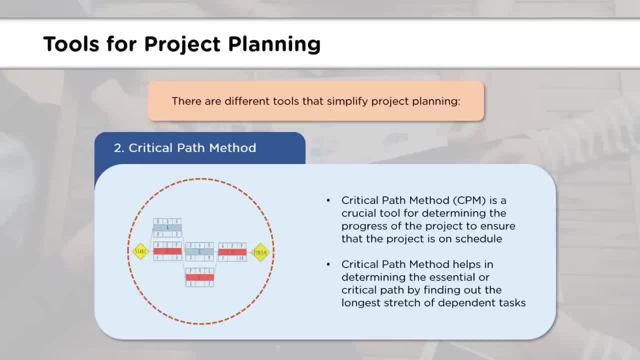 The second tool we will talk about is Critical Path Method or CPM. Critical Path Method helps in scheduling the project activities so that the project runs properly. The Critical Path Method focuses on the longest stretch of dependent tasks and determines the time needed to complete them. 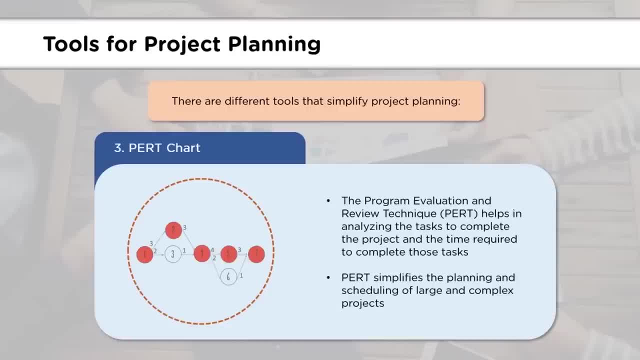 The next tool is Project Evaluation and Review Technique, or PERT chart. PERT provides a graphical representation of the project's timeline, explaining the independencies of different tasks. This tool not only helps in making a schedule, but also helps in coordinating with all the team members. 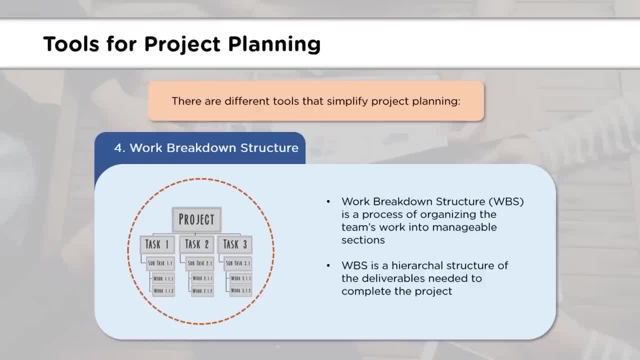 The fourth tool we will check is Work Breakdown Structure. Work Breakdown Structure is a very common tool that makes it possible for the team to break its work into manageable sections. Work Breakdown Structure is a step-to-step process that helps in completing the project efficiently. 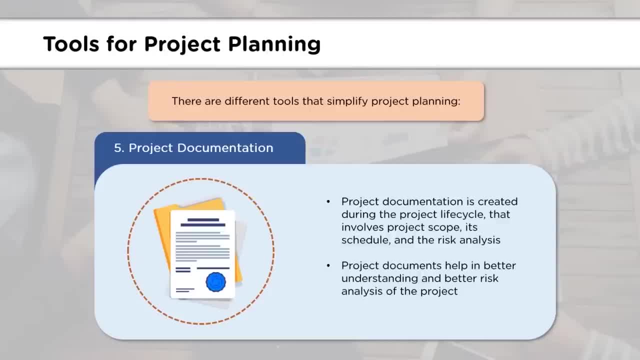 The last tool we will see is Project Documentation. Project Documentation is an integral part of the project lifecycle. Project Documentation helps in understanding the mistakes done during the project and, more importantly, provides guidelines for the upcoming project. Now, when we know about different tools for project planning, 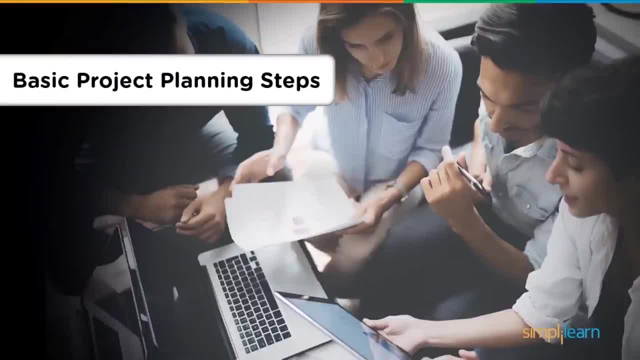 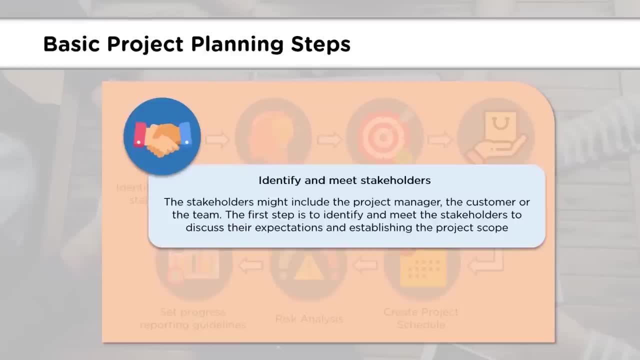 it becomes essential that we know the necessary steps of project planning. There are seven steps in project planning. Let's have a look at each of them in detail. The first step is Identification of Stakeholders. As we have discussed, stakeholders could be anybody. 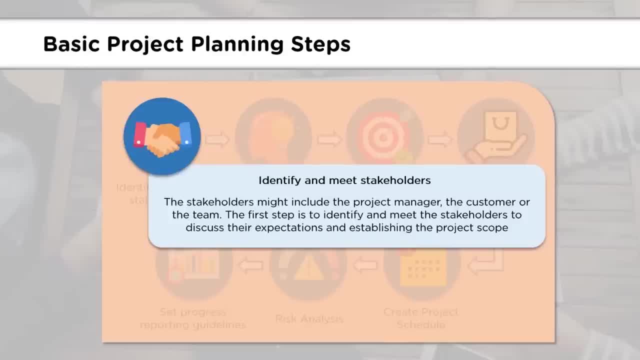 They could be a part of the team or a project manager or a customer. When we identify stakeholders, we can find out the expectations and requirements that are to be looked upon in this project. This gives us a clearer picture of the project and helps in establishing the project scope. 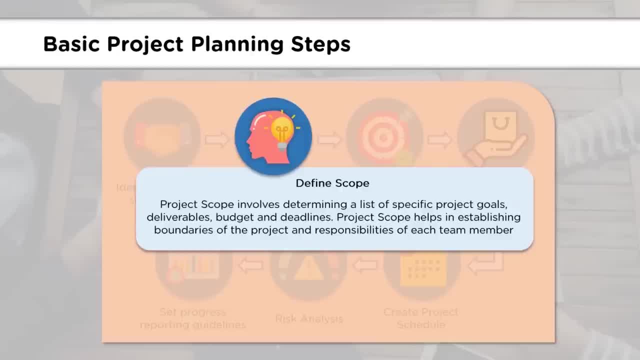 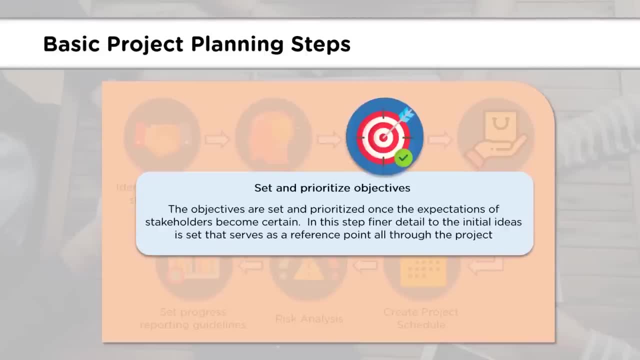 So the next step we have is Defining the Project Scope. This helps in determining a list of specific project goals and deliverables that are to be achieved during the course of the project. After we have defined the project scope, it is time to set project objectives and prioritize them. 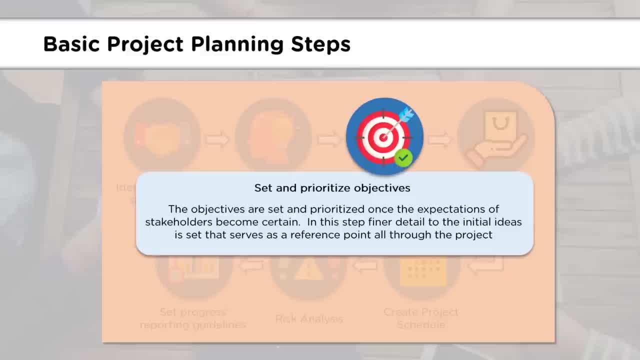 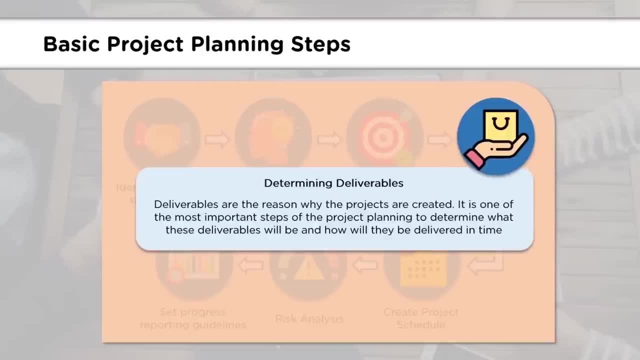 The initial ideas that were there before are now elaborated and final steps to complete the project are defined. In the next step, the deliverables are determined. After all, project deliverables are the only reason why the project is being created. This step involves finding out what these deliverables will be and the deadlines of their delivery. 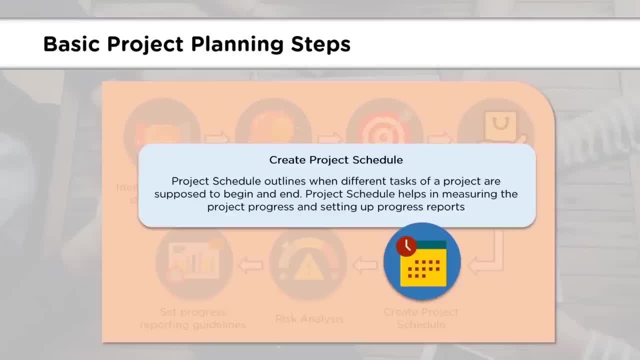 Then the step that comes into picture is Creating a Project Schedule. The project schedule refers to the guidelines when a particular task is to be started and when it is supposed to end. This helps in monitoring the growth of the project and later helps in generating progress reports. 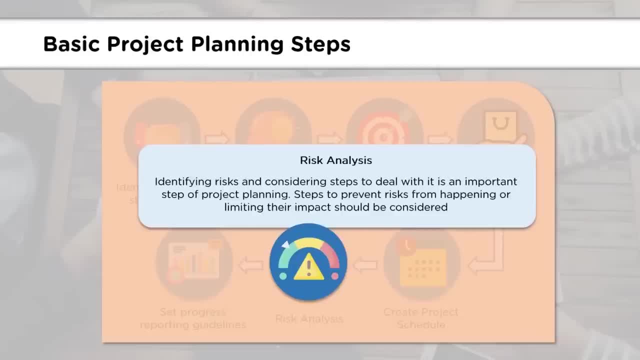 The next step is the step of Risk Analysis. This step plays an extremely important role in the success of the project. This step plays an extremely important role in the success of the project. This step plays an extremely important role in the success of the project. 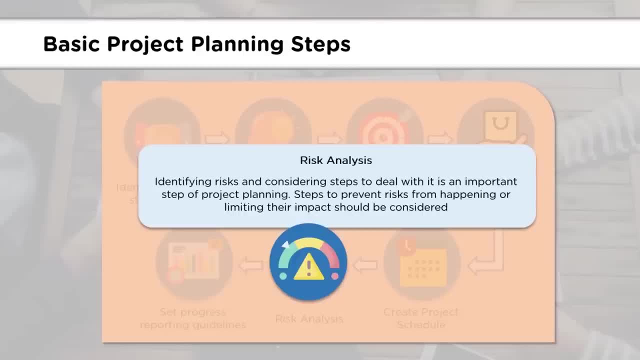 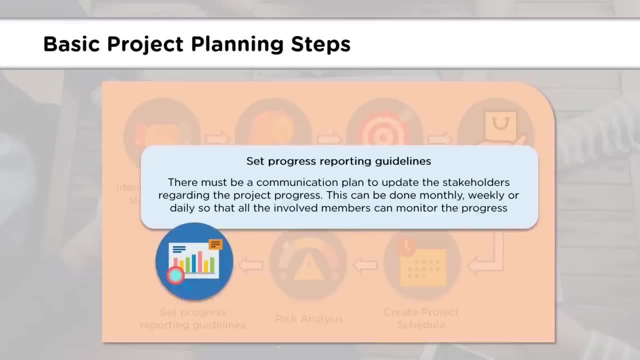 of the overall project. It helps in identifying the risk, prioritizing them and taking steps to limit them. The last step in project planning is to generate progress reports. In this step we update the stakeholders about the project growth and it is done so that all the concerned team 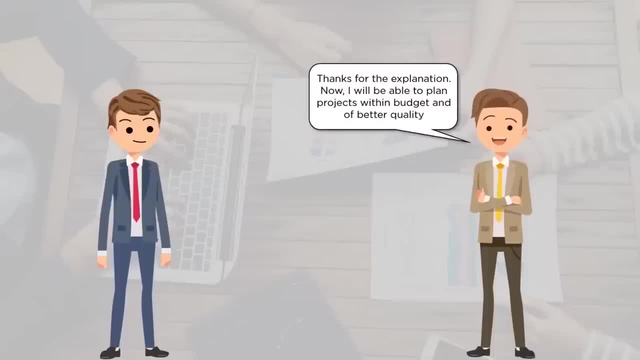 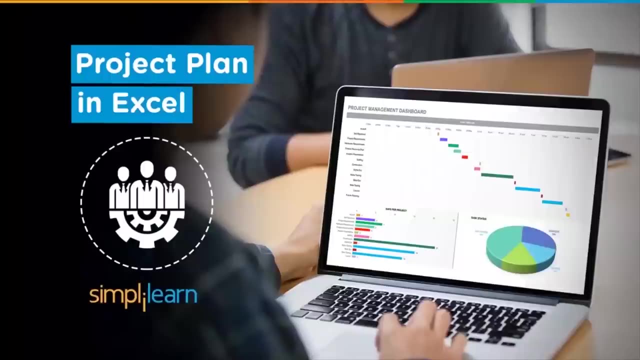 members can have a look at the progress of the project After all this information. Max thanks Jack for the explanation and looks forward to plan projects within the budget and of better quality. In this session we will talk about project plan in Excel. We will learn about a project. 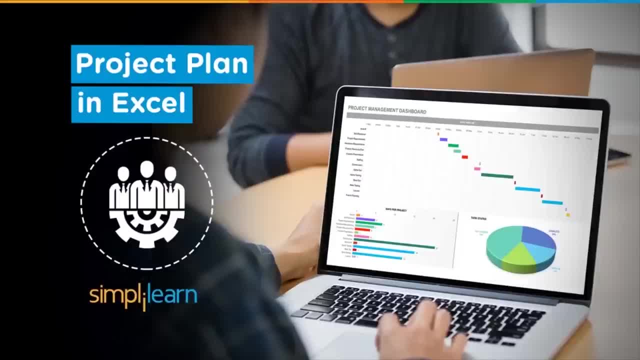 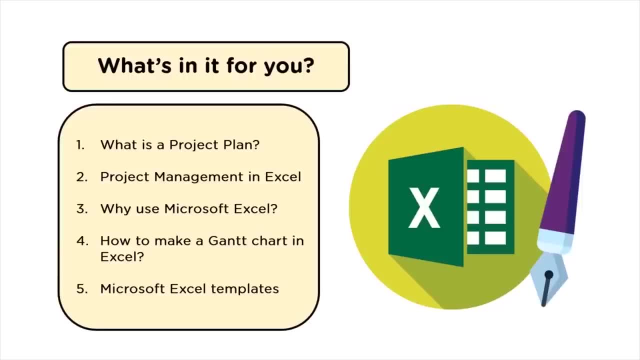 plan and how we can make an effective plan in Microsoft Excel. Before we begin, let's have a look at all the topics we will be covering today. First we will see the basics of a project plan. Then we will check the process of project. 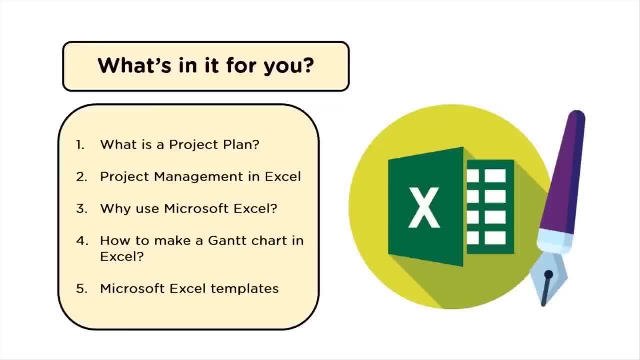 management in Microsoft Excel. and why should one refer to Microsoft Excel? Apart from this, we will learn about how to make a Gantt chart in Excel. Towards the end, we will check some Microsoft Excel templates. So, without any further ado, let's get started. 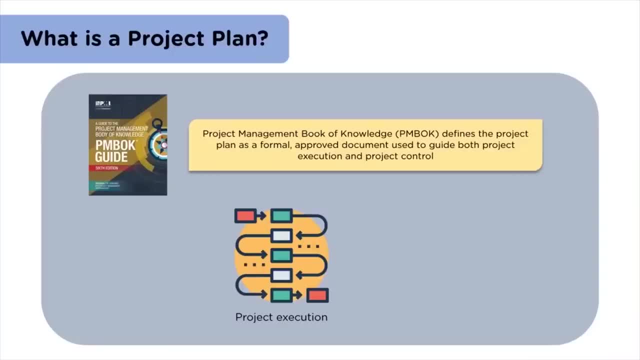 Let's see what is a project plan. Project plan is a basic thing that is needed to execute a project. According to project management book of knowledge, a project can be defined as an approved elaborative document that guides the team during project execution and project control. 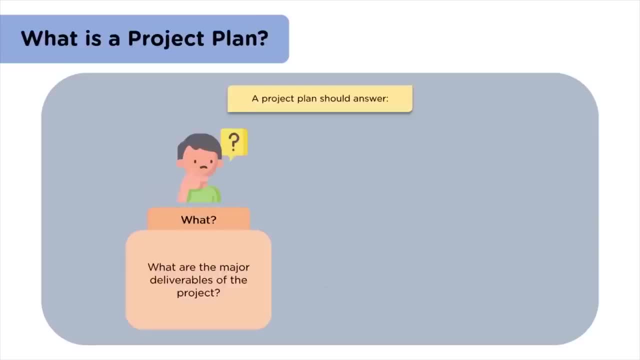 When we are making a project plan. a project plan must answer several questions. for us, These questions are like: what are we expecting our project to deliver? How are we expecting to get our deliverables within the desired time? Who all will be a part of our project? 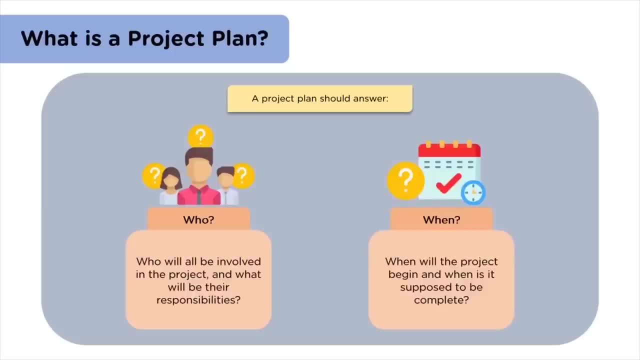 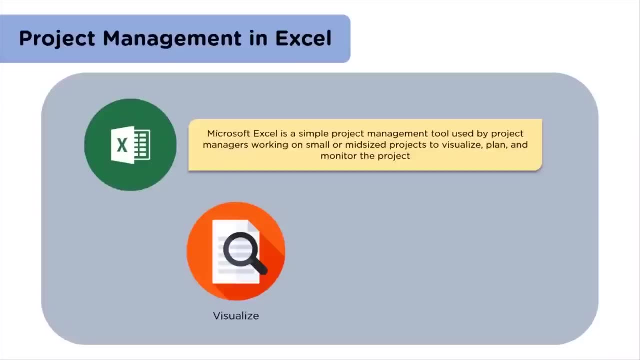 and what tasks they will have in the project. When will the project start and when it is expected to end? That is the deadlines of the project. Now let us learn about project management in Excel. Microsoft Excel is one of the most common applications these days. It is used in both. 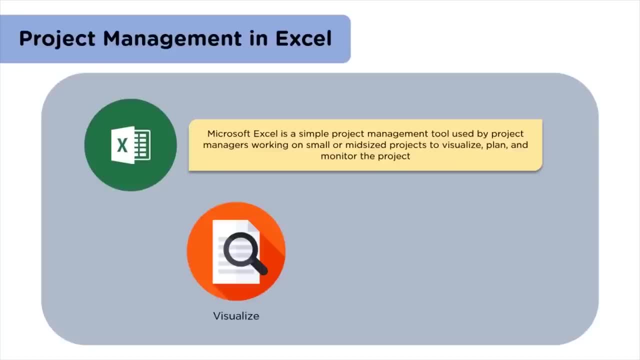 offices and at homes. Microsoft Excel is an easy project management tool that allows the team members to easily see the tasks in a project, develop a plan and track its progress. Before we learn more about project management in Excel, let's first have a look why we 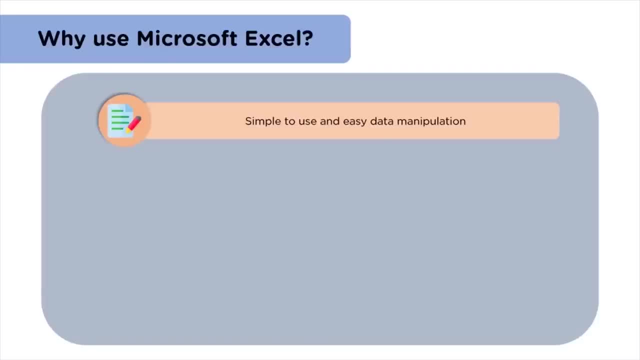 use Excel. Microsoft Excel is an easy tool to plan a project, so it can be used by people who are beginners in terms of project management. One can find several analytical tools like concatenate, len and counter, so this makes data analysis easy and effective. 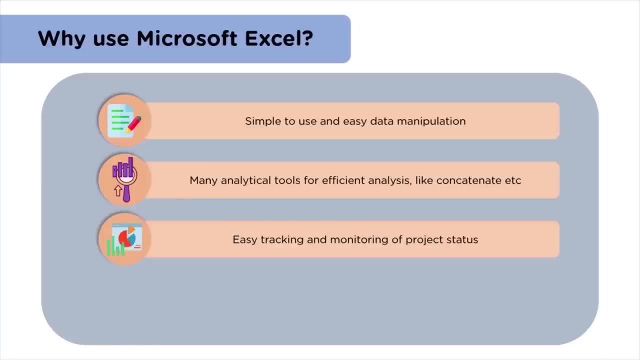 As the entry of data is easy, same is tracking and controlling of project status. Then there are several project management templates in Excel that help us to have an effective distribution of project data. We will be checking several project management templates towards the end of this video. 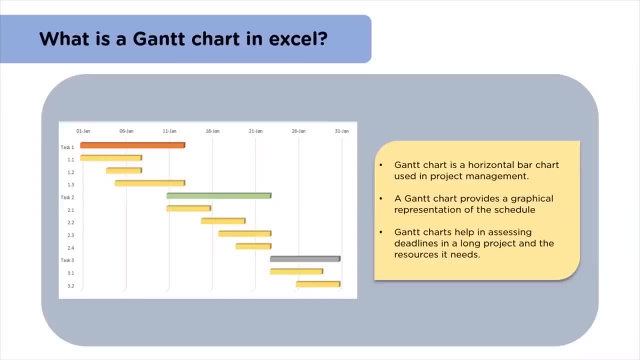 Now let's have a look at the process of making a Gantt chart in Excel. Before we begin this, it's important we know what is a Gantt chart. A Gantt chart is like an horizontal bar chart that is used for project management. 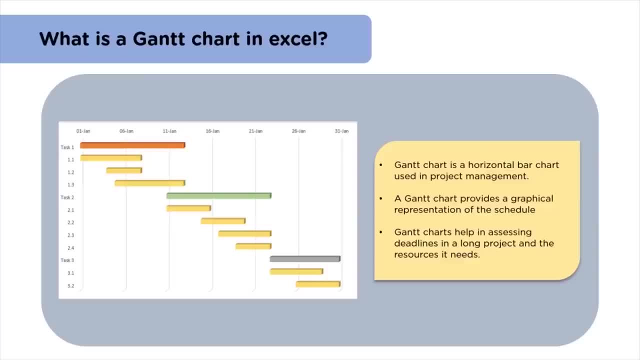 With the help of a Gantt chart, we can check the status of the task, the date they start, the date they end and their dependencies on each other. Gantt chart helps in coordinating and monitoring different tasks in a project. Now let's have a look at the steps that will help us in making a Gantt Chart. 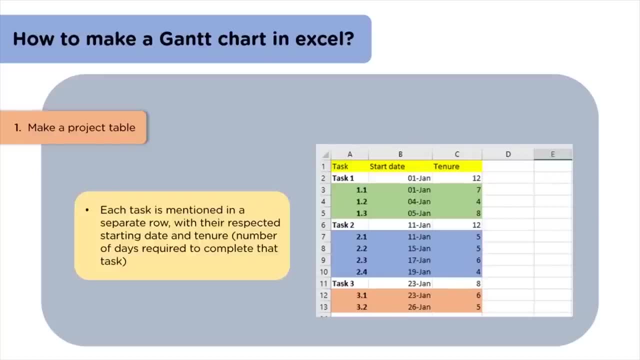 First step we have is make a project table. We have several rows and columns, like here: we have three columns: In the 1st column we have the task, in the 2nd we have our start date and in the 3rd column 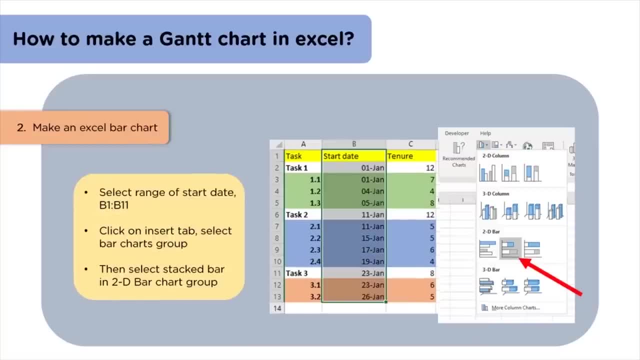 We have the duration or tenure of the task. The second step is to make a bar chart in Excel. For this we will select the entire second column. Then we will go on the Insert tab and click on the Bar Graph chart. There we can select stacked bar graph in 2D bar charts. 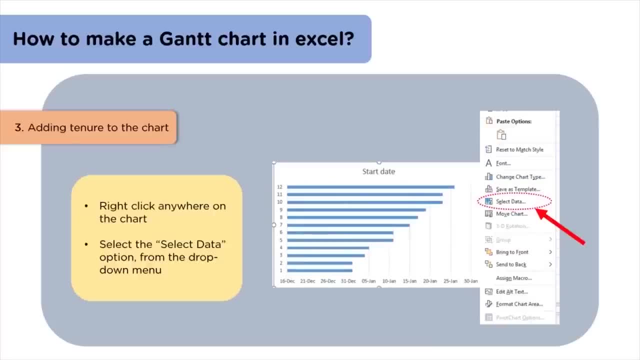 As a result, we will have the entitled bar graph on the screen. In the third step, we will add the duration to the bar graph. We will right click on the chart and in the menu that appears, we will select Select Data option. 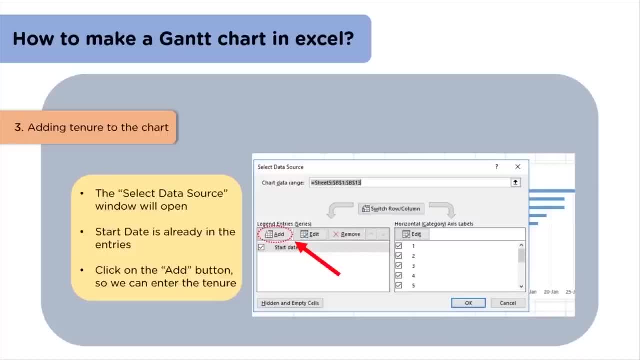 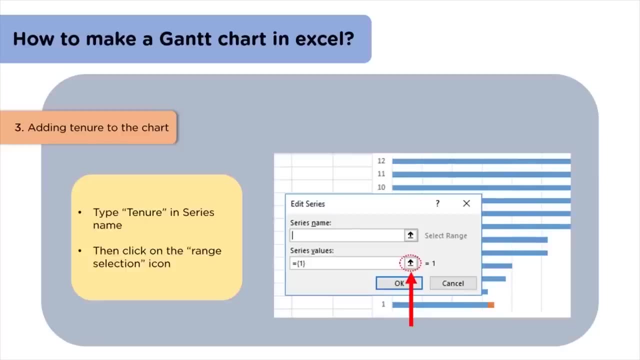 A window that appears on the screen. in that window we will select Add option as shown. We can also see the start date is already in the entry section. Then in the dialog box that appears, type tenure in the series name and click on the. 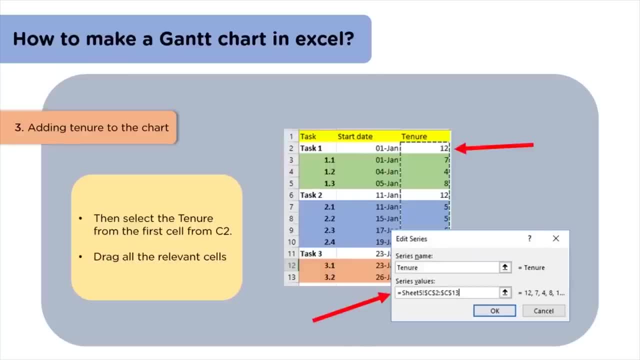 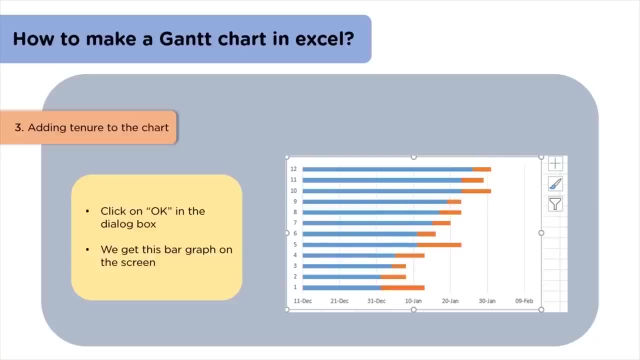 range selection icon that's shown in the figure. Now select the relevant data from the tenure column and click on OK. Now we can see a bar graph that has two colors on the screen. This bar graph now has the duration of the tasks. 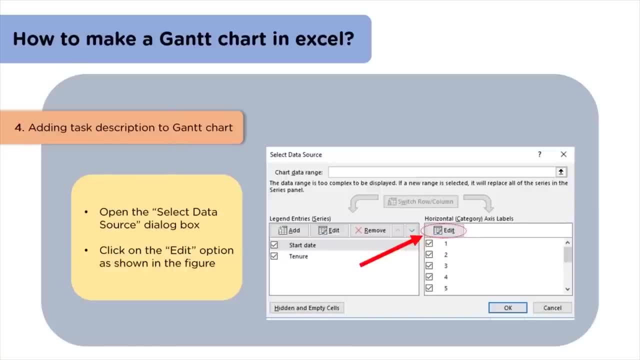 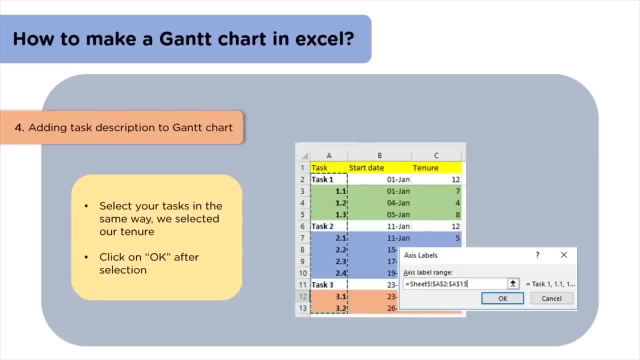 The fourth step we have is adding description to the Gantt chart. Now we will open the box again and in that box we will select the Edit option as shown in the figure. Then we will select the tasks as we had selected the duration of the tasks before, and click on OK. 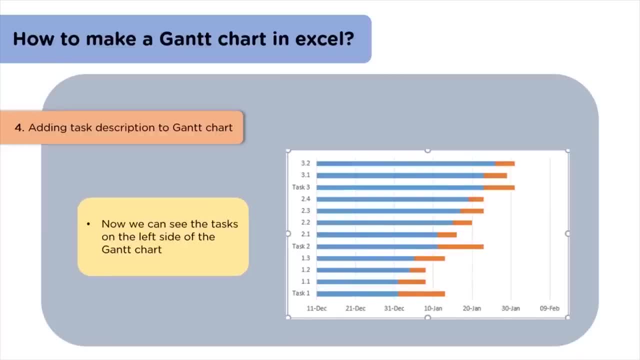 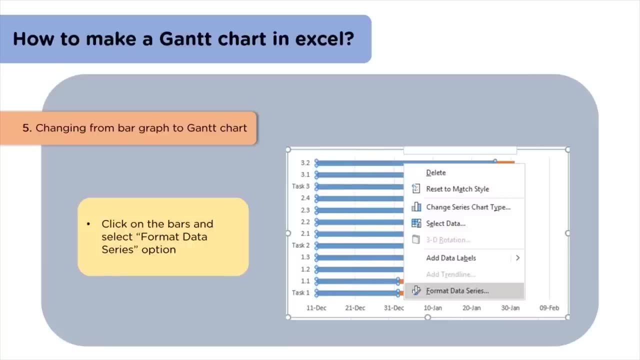 We can now see the tasks have appeared towards the left side of the Gantt chart. The fifth and the remarkable step will help us convert this bar graph into a Gantt chart. We will now click on the bars and select the Format Data Series option from the menu that appears. 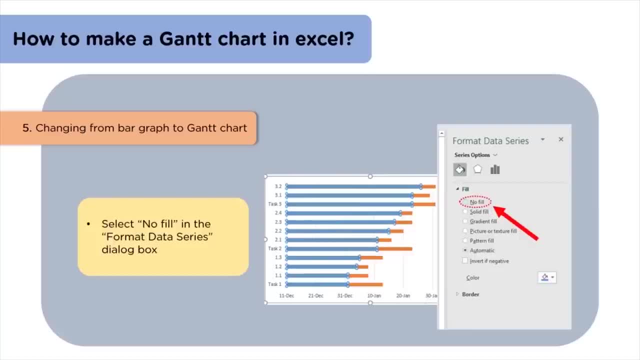 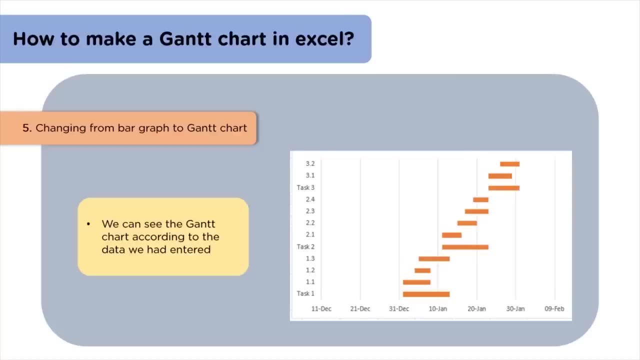 Then in the Format Data Series dialog box, we will select No Fill option. We can find our Gantt chart on the screen now, in accordance with the data that we had entered. Now we can see the tasks on the left side are in the reverse order. 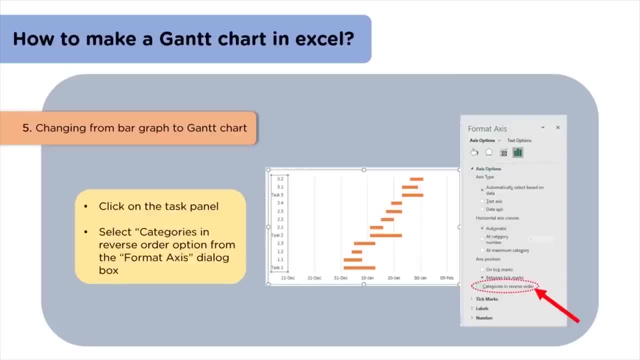 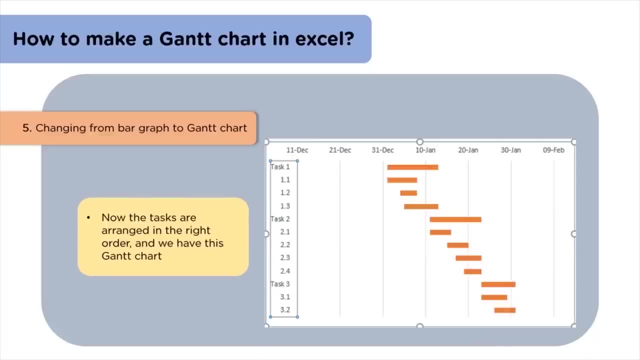 So what we will do next is we click on the task panel, then go to the Format XS dialog box and select the Categories in Reverse Order option. Now we can find our tasks in the right order. One more thing we can notice is Gantt chart is starting with some other date and not with the dates that we had entered. 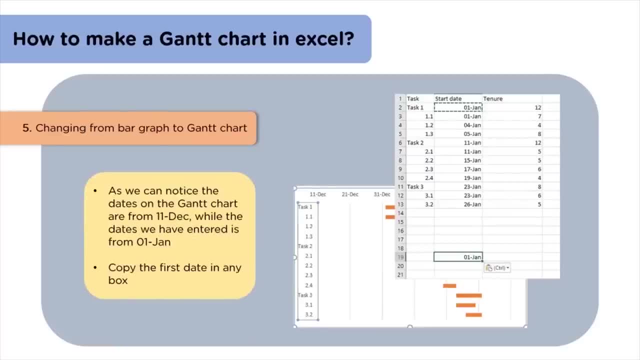 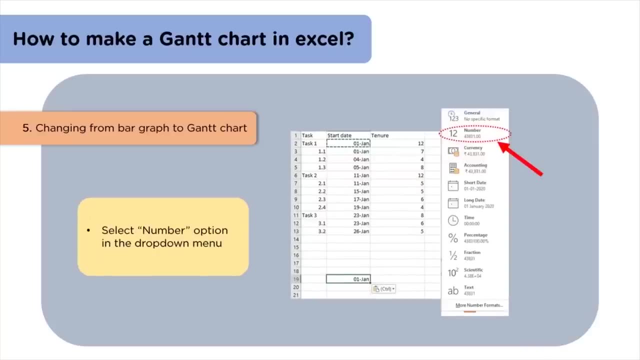 So for this we will copy the first date in some other cell. Then, clicking on the copied cell, we will go to the Home menu to select the dialog box as shown in the figure. Then in that drop-down menu we will select the Number option. 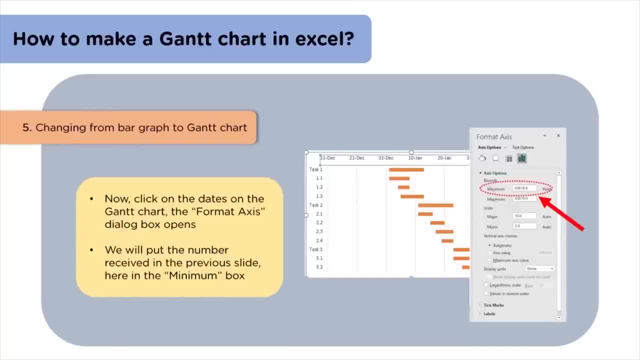 We can now find a value displayed in the copied cell. We will copy that value. Click on the dates on the chart and, as the Format XS dialog box opens, we will paste that value in the box that says Minimum shown in the figure. As a result, we will have our final Gantt chart on the screen. 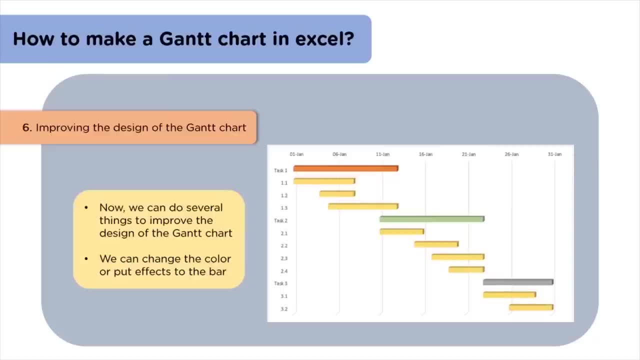 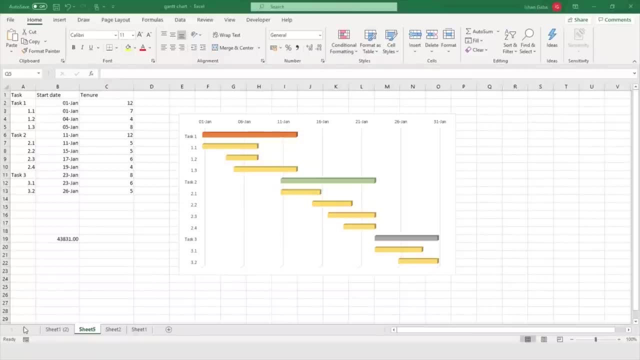 In the last step we can give several designs to a Gantt chart, change colors and make it more presentable for us. Now, when we know the basic steps of making a Gantt chart, I will show that practically to you in Microsoft Excel. 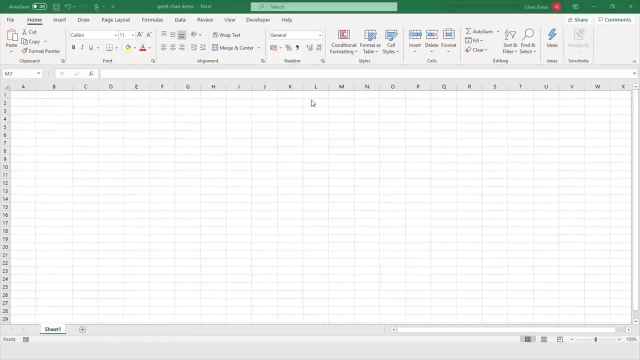 Our first step is to open Microsoft Excel and in Microsoft Excel we will make a project table. In a project table, we will have three columns. The first column will be Task. The second column will have the start date. The third column will have tenure, or the duration of the task. 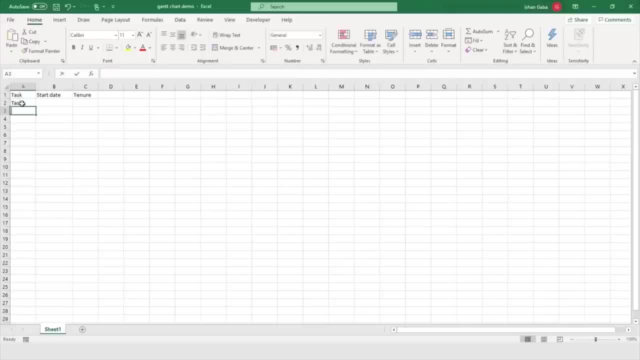 So, beginning with tasks, we have Task 1.. In Task 1, we have 1.1, 1.2, 1.3.. Then comes Task 2.. In Task 2, we have 2.1, 2.2, 2.3 and 2.4.. 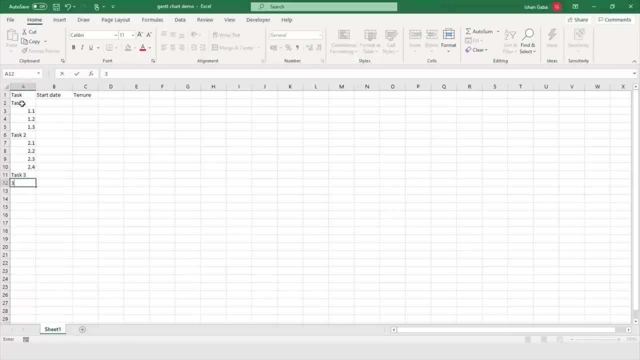 Then we have Task 3.. Then we have Task 4.. Then we have Task 5.. Then we have Task 6.. In Task 3, we will have two subsections: 3.1 and 3.2.. Then we will start with the starting dates. 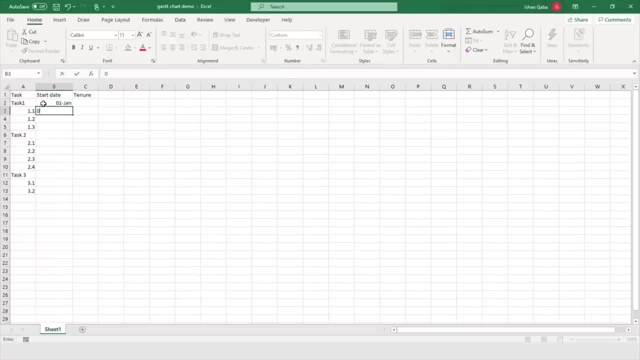 In starting dates we will put 1st January. The Task 1.1 will be 1st of January, Then this will be 4th January. Let's say this is 5th January, Then we will put this as 11th of January. 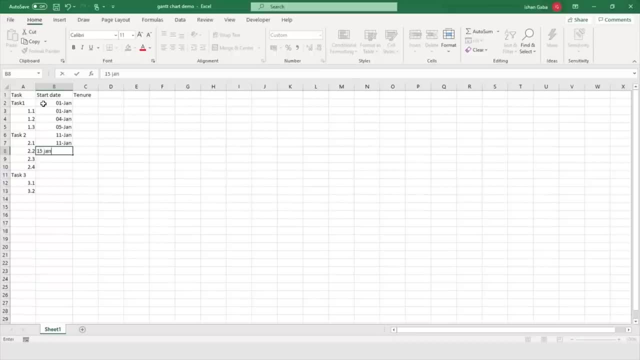 And this will be again 11th January. only This will be 15th January. Let's put this as 17th January. this be 19th january. task 3 begins on 23rd january and it- the 3.2 section- begins at 26th of january. 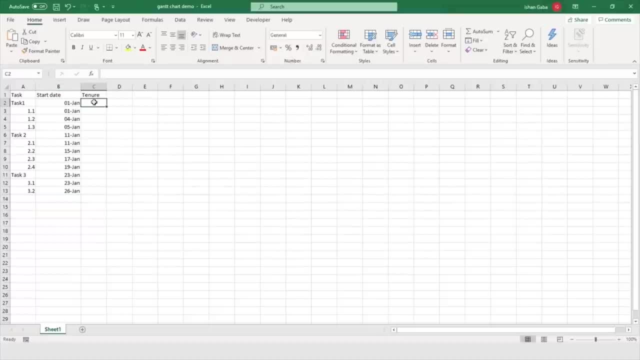 now let's put the tenure, or the duration of the task. we will begin with task 1. it takes 12 days. then 1.1 takes 7 days. we say this takes 4 days and this takes 8 days. then for task 2, it again. 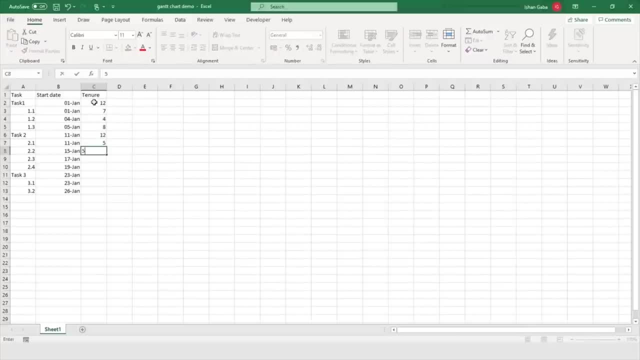 takes 12 days. it takes 5 days, 5 days and let's say this takes 6 days and this takes 4 days. then we come to task 3. this takes 8 days and let's say this takes 6 days, and the 3.2 section. 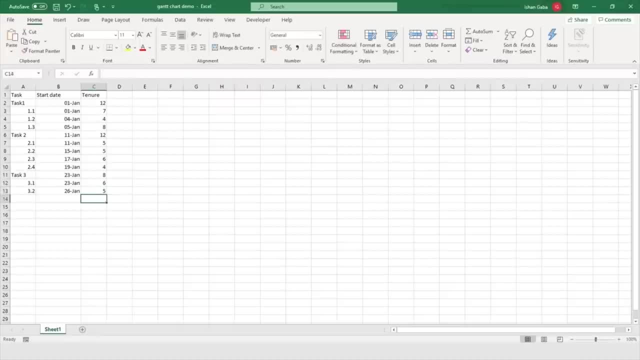 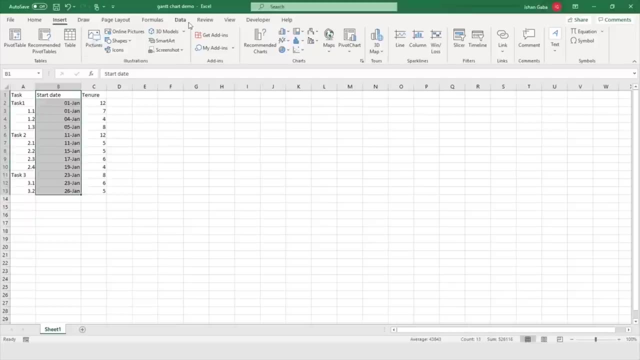 takes 5 days. so this is how our project table is ready. in the second step we will select the entire second column. after we have selected this column, we will go to the insert tab. in the insert tab we will go to the bar columns and in this we will select: 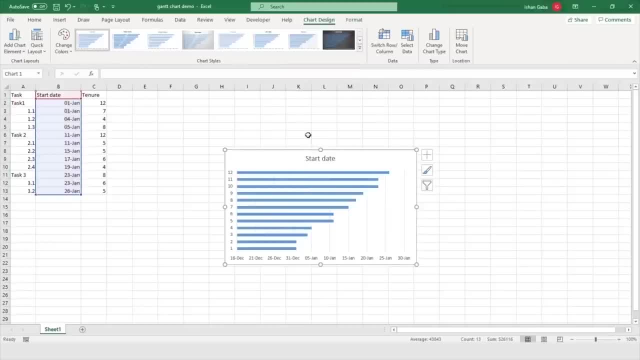 2. D- stacked bar charts. now we have the entitled bar chart in accordance to our data on the screen. then comes the third step. we will add the duration of the tasks to the bar graph, we will click on the chart and after we click on the chart, 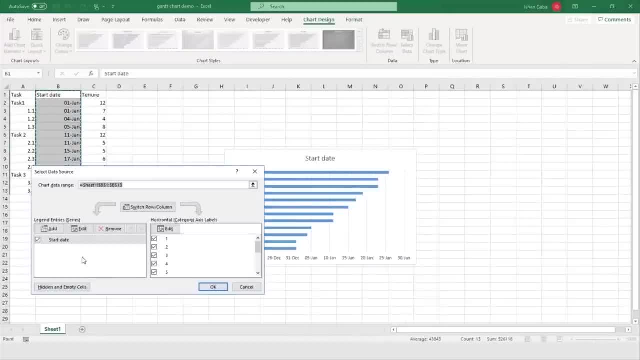 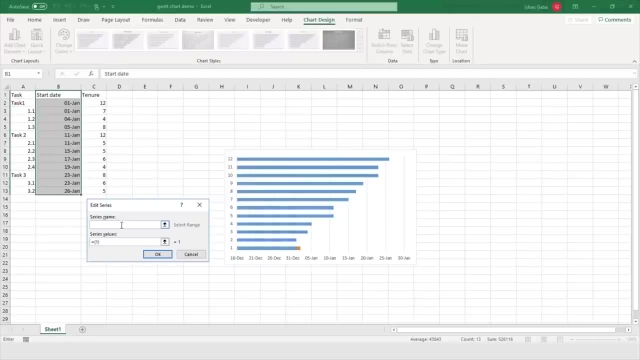 we will select select data option. in the select data source dialog box we find the start date is already there. now we will click on add and after we click on add in this series name section we will put tenure. then in the series value we will click on this. 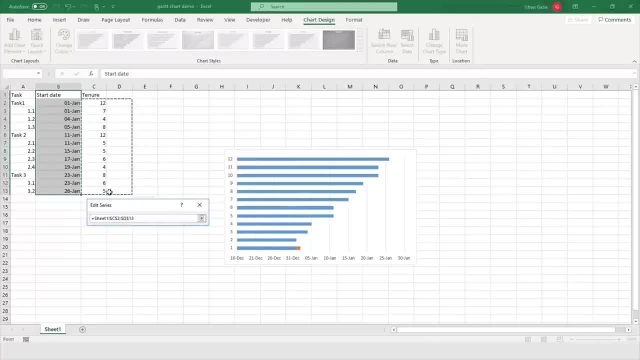 icon and select the entire tenure series and click on OK. So this is the bar graph that we have now. This is now in two colors: the orange color and the blue color. This bar graph now has the duration of all the tasks in our project table. 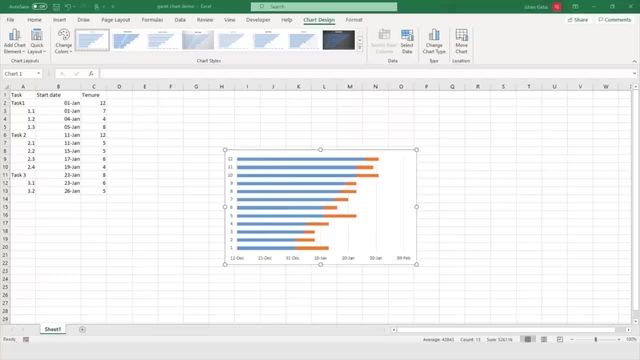 Now in the fourth step. now it's time for us to add description to our Gantt chart. Instead of this: 1, 2,, 3,, 4, 5, we will put task 1,, task 2 and the subtasks. 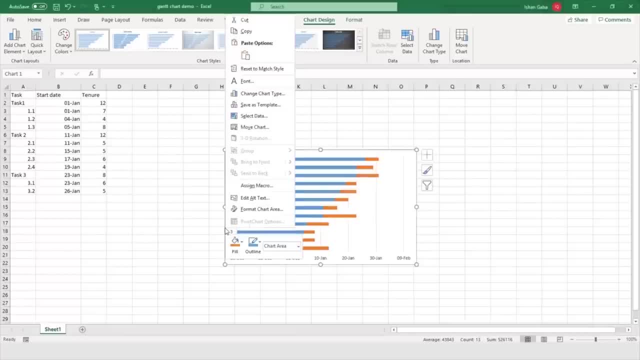 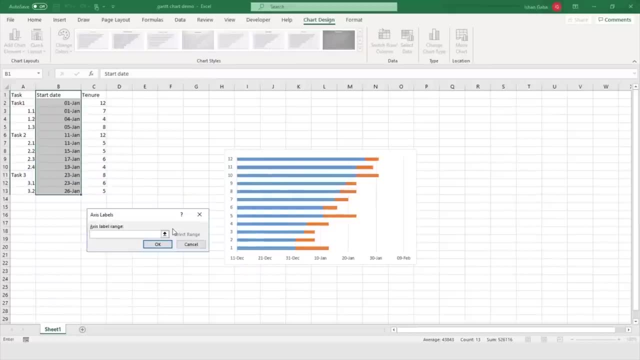 So what we will do is we will again go to that box, We will left click on the Gantt chart, select the select data option and then we will go to the start date. Here we will select the edit option. In the edit option we will select all the tasks and click on OK. 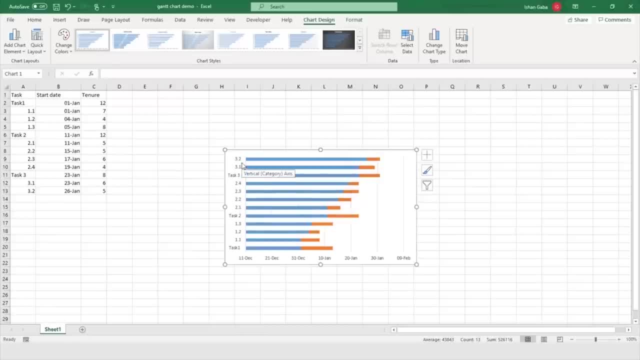 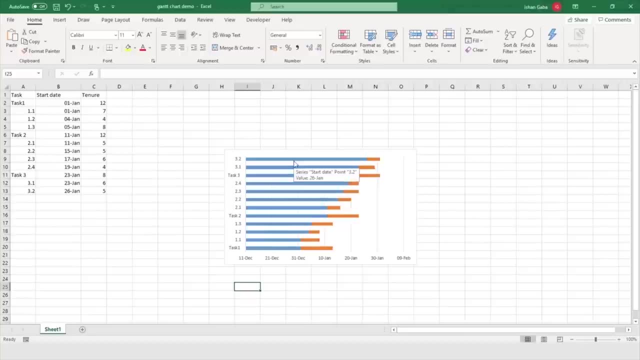 Now we can see, all the tasks are aligned towards the left of the bar chart. As we can see, this is a bar chart or a bar graph, and not a Gantt chart. The next step we have is converting this bar graph into a Gantt chart. 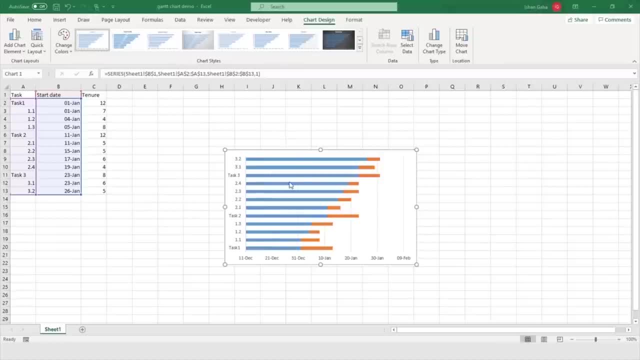 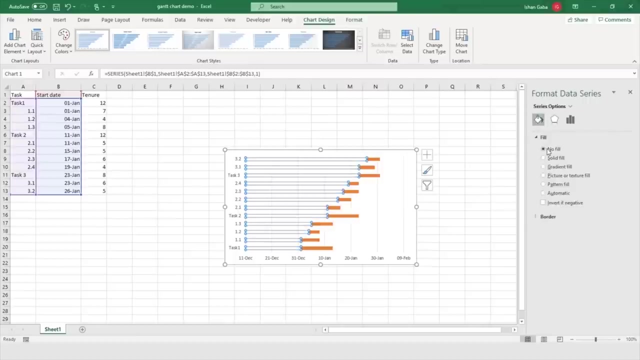 So we will click on the bars and select the format data series option from the menu that appears Here. we have this format data series option. Now we can see the dialog box on the screen. Here we will go into the color section, fill section, and then we will select no fill. 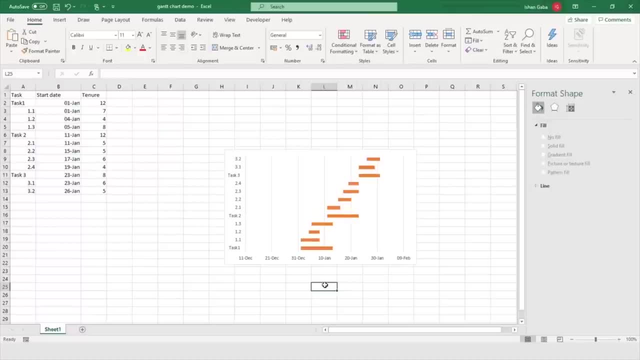 Now we can see the blue lines have disappeared, So this looks like a Gantt chart. So now, when we have a Gantt chart on the screen, we can notice that the tasks here are in the reverse order. So what we will do is: 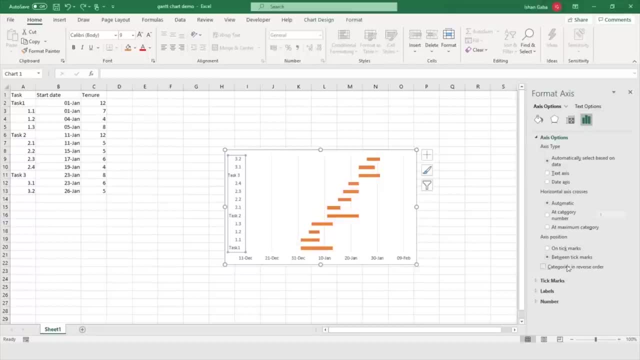 we will click on these tasks and select the format axis option. Here we will select categories in reverse order. We can see our Gantt chart is now in order, Like we have our task 1 on the top and task 3 at the bottom. 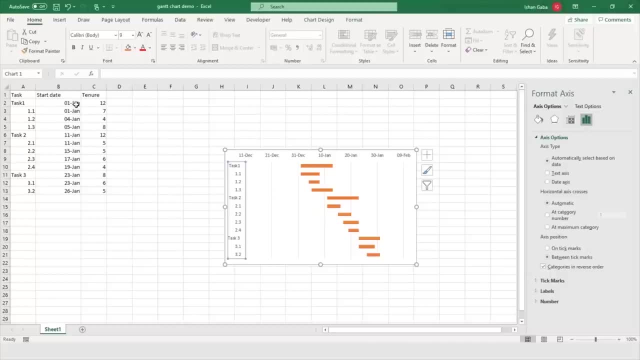 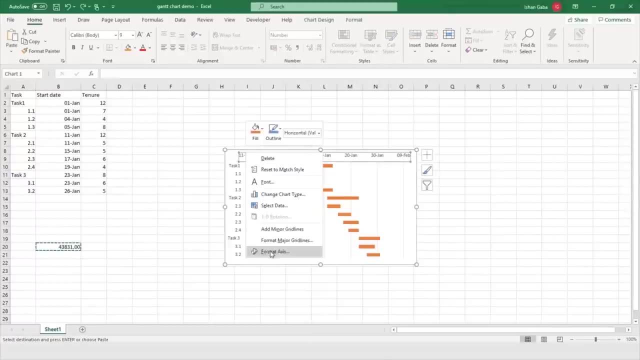 The dates are starting from 11th of December, but the dates we have provided are from 1st of January. Now we will copy this cell, then go on the dates box. Here we will go to format axis. In the format axis we can see minimum. 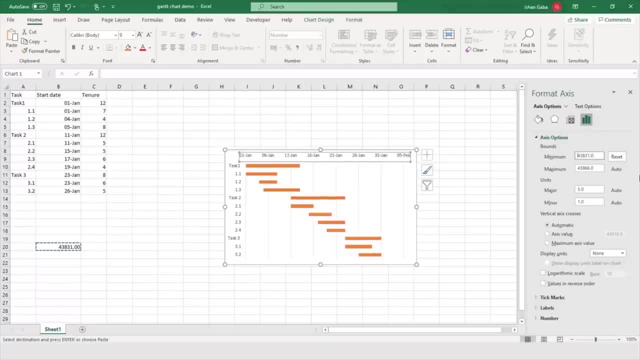 In this minimum. we will paste this value and press enter. As we press enter, we can see our Gantt chart, starting from the date that we wanted to start and that, too, in the correct order, starting from task 1 to task 3.. 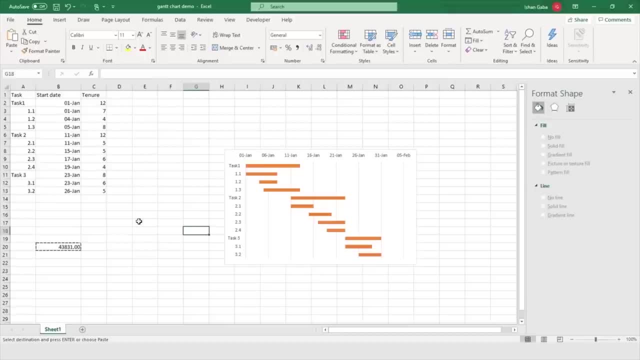 Now, as a result, we have our final Gantt chart on the screen. In the last step, what we can do is make our Gantt chart more representable. We can change the color of these bars, we can give them shapes and we can do many other things to make it more presentable. 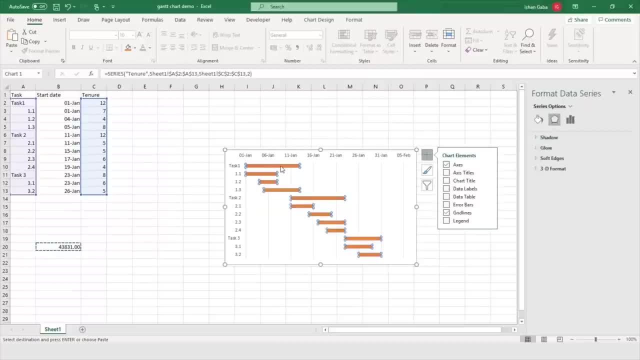 We will first select the bars, Like. what we will do is we will select task 1 and let's say we give it the color blue, Then task 2, we will give it color green and in task 3, we will give it the color black. 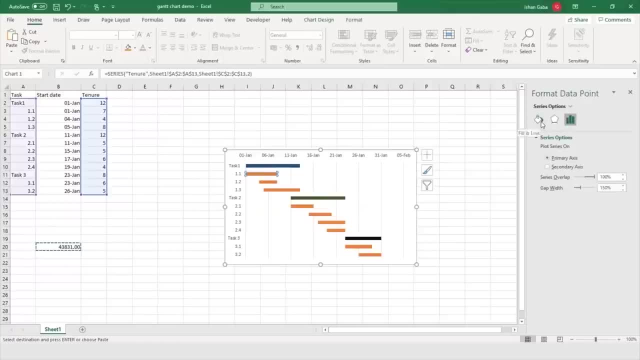 So here the subsections will give different colors to the subsections as well. Then we come to task 2.1.. This is how we can change the color of these cells. or, apart from changing colors, we can select a bar graph and do the gradient fill. 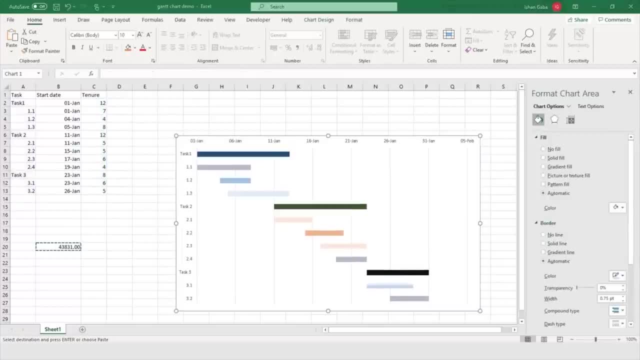 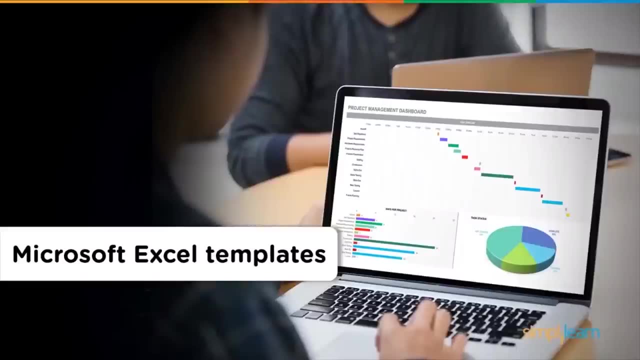 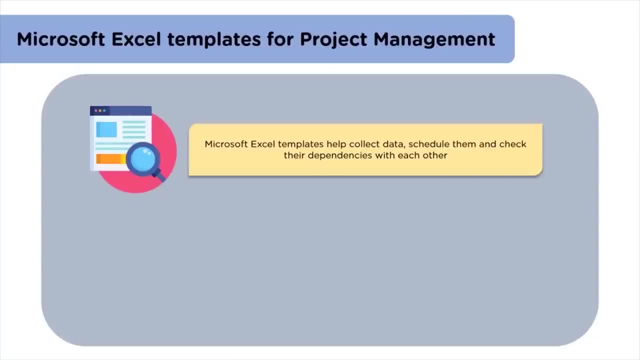 So this is how we can make a Gantt chart. After changing the colors or changing the shapes, we have our final Gantt chart on the screen. Finally, let's have a look at some Microsoft Excel templates for project management. Microsoft Excel templates help in collecting data, putting them into order and check their dependencies with each other. 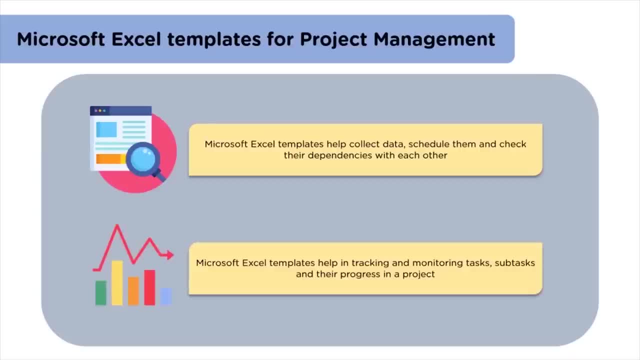 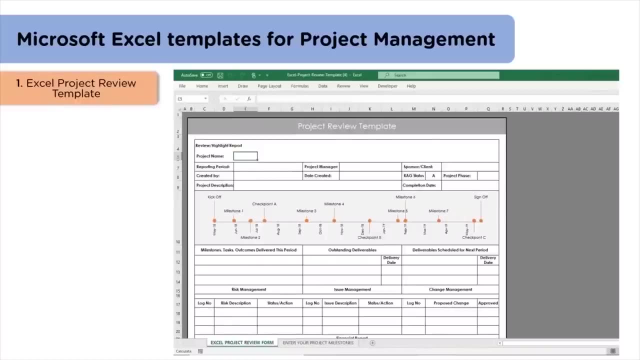 With the help of these templates we can monitor the status of the tasks and we can also check the progress our project has made Moving forth. we will check some important Microsoft Excel templates. The first template we have is Excel project review template. This template helps us have an overview of the project. 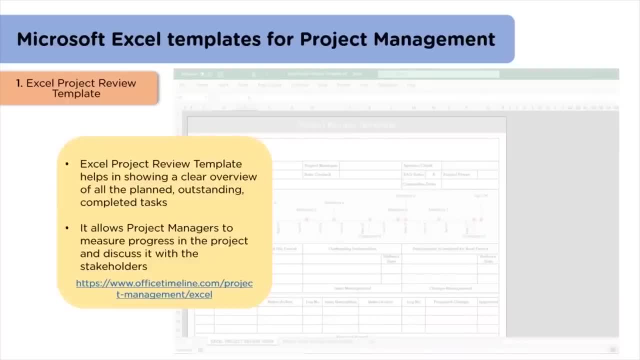 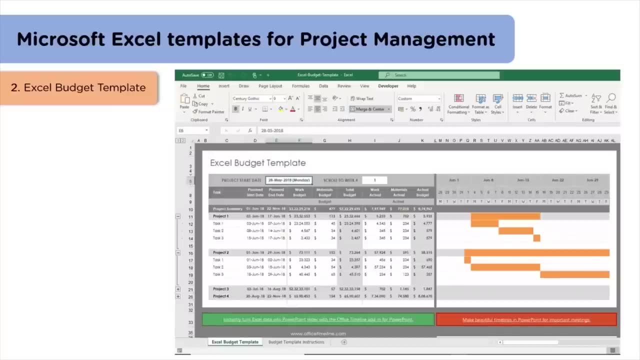 We can have a clear understanding of all the tasks that are planned and that are completed. This helps project managers to measure the progress of the project and take further steps accordingly. Second template we will check is Excel budget template. In this template we can monitor all the expenditures of our project. 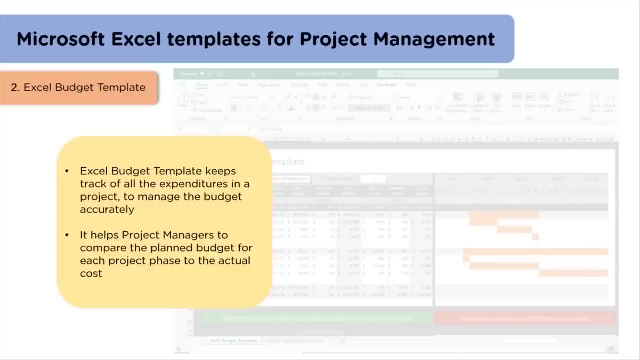 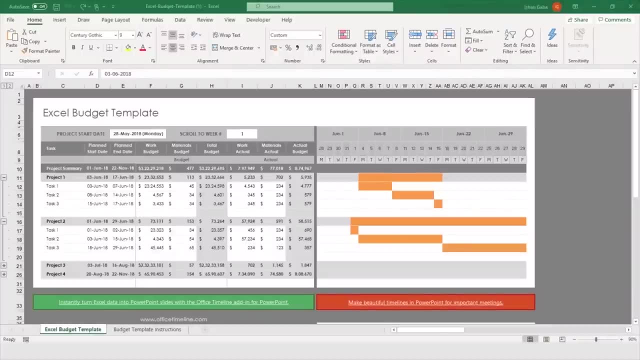 It helps us in managing the budget of our project and also helps in comparing the budget of our project at different phases. Let's have a look at the budget template in Excel, once We can download this template from officetimelinecom. The Gantt chart towards the right is in accordance with the dates towards the left. 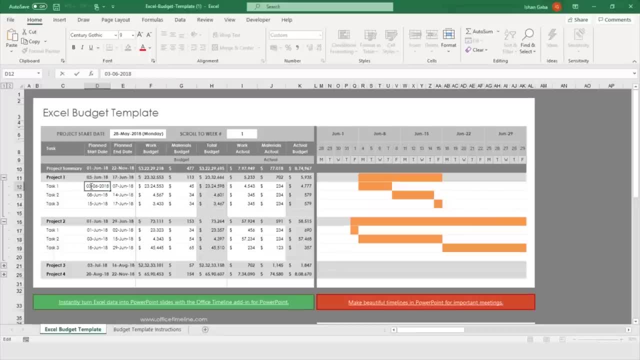 If we fluctuate the date, we can see the template working. The start date for task 1 could be changed to 10th June. If we change this date to 10th June, we can see the fluctuation in the Gantt chart. 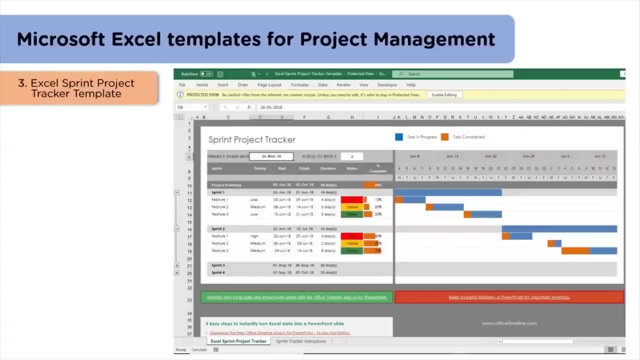 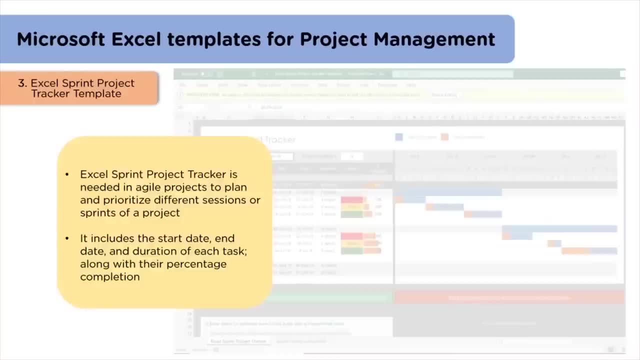 So this is how we can use this template directly. Let's have a look at the third template now. Third template we will see is Excel sprint project tracker template. This template is used majorly in agile projects where the project is made in several sprints or sessions. 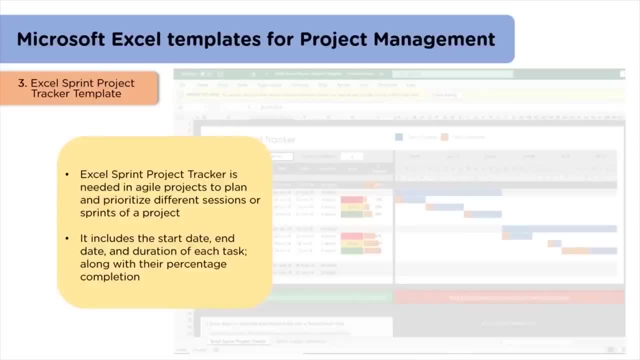 This template includes the sprint project tracker template, The start date, the end date and the duration of each task. We can also see the percentage completed of each task. Let's have a look at this sprint project tracker template as well. We can see the Gantt chart towards the right and the data towards the left. 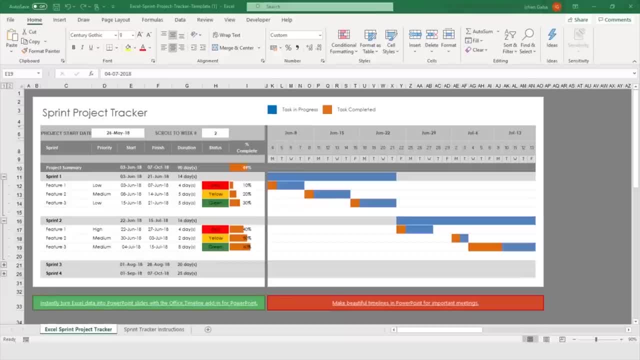 So if we change any data, we can see the Gantt chart changing. For example, we can change the data in sprint 2, feature 3.. Let's change the start date to July 2nd: We can see the Gantt chart changing. 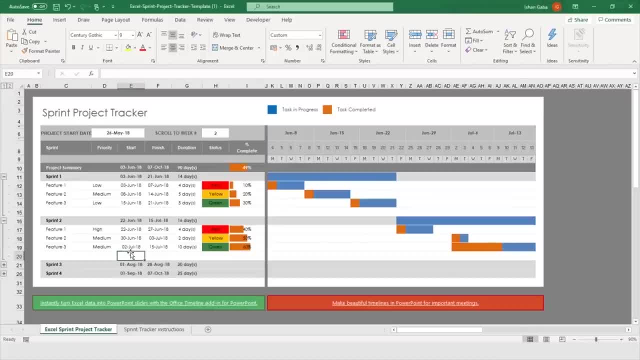 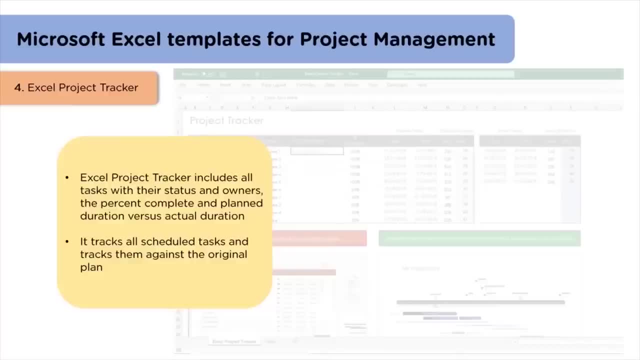 This is how we can use this template directly to track our sessions. Let's have a look at the fourth Excel template. This template is Excel project tracker. In this template we have the data of all the tasks with their status and owners. We can track the percentage of tasks completed and also compare the planned duration of the task to the actual duration of the task. 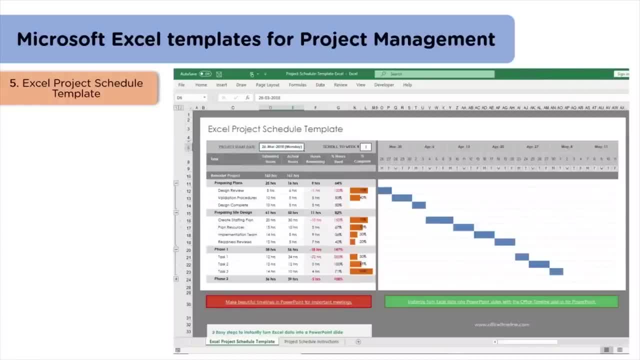 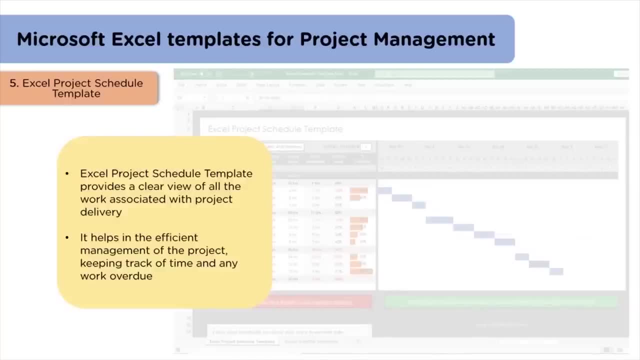 After the critical part tracker, let's check the Excel project schedule template. This template helps in effective management of the project as it helps in monitoring the time that each task of the project takes. It provides a clear view of the tasks. It provides a clear view of all the work associated with the project. 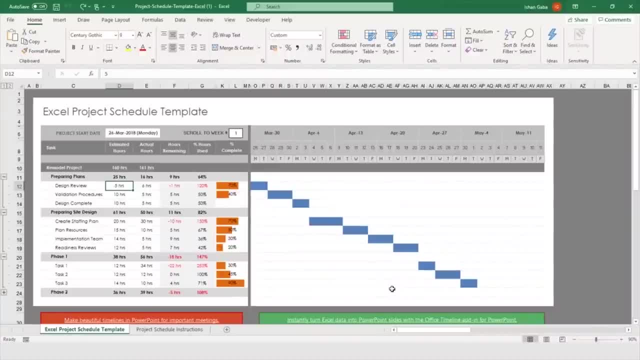 Let's have a look at this template in Excel once We can see the Gantt chart. in accordance to the data, If we change the estimated hours at two places- let's say at the design review, we make it 15 hours instead of 5 hours- 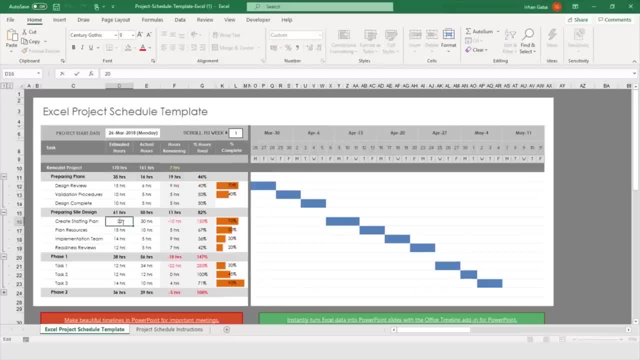 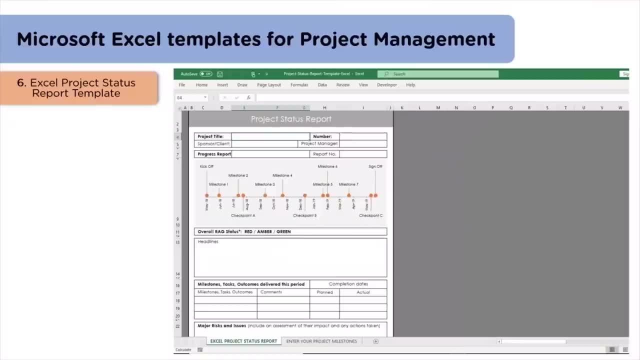 And at the create staffing plan we make it 2 hours instead of 20 hours, We can see the Gantt chart fluctuating. This is how we can use this template to manage the schedule in a project Moving forward. the next template we will see is Excel project status report template. 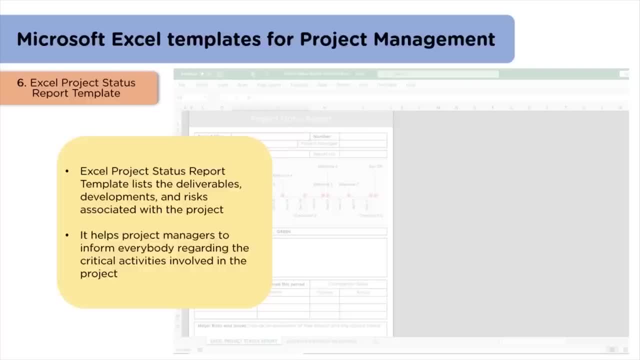 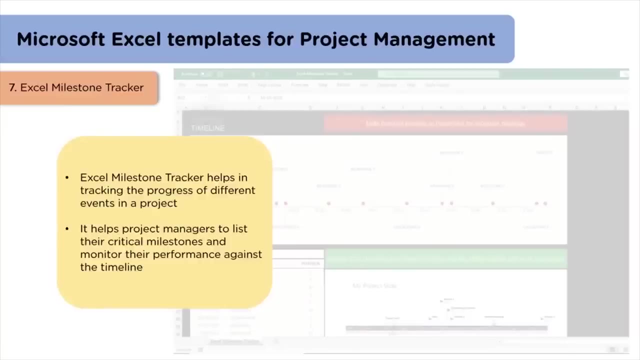 This template helps us having a list of project deliverables and the risks associated with that project. This template helps the project managers about different crucial activities involved in a project. After this we have Excel milestone tracker. The milestone tracker helps us in tracking or monitoring different tasks in a project. 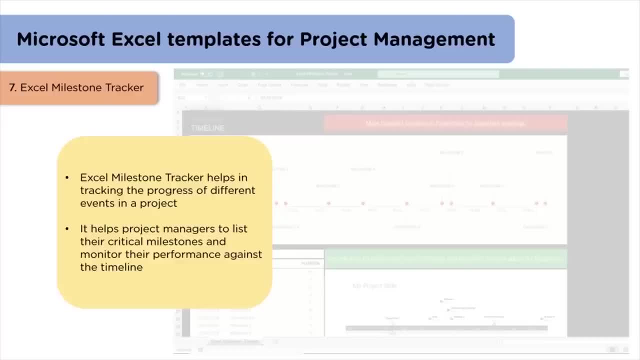 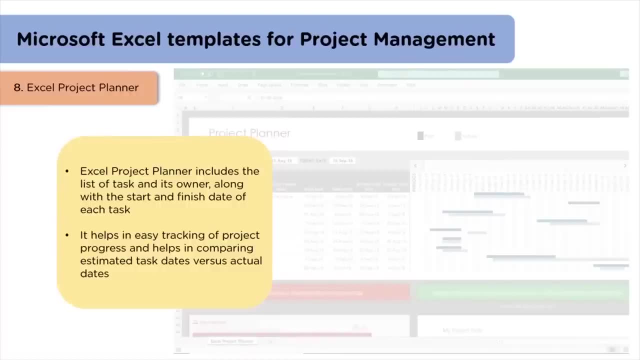 Project managers use this template to monitor the project performance with respect to the timelines. The last template we will see is Excel project planner. Excel project planner includes a list of tasks with the respective owner, Along with the start date and the end date of that task. 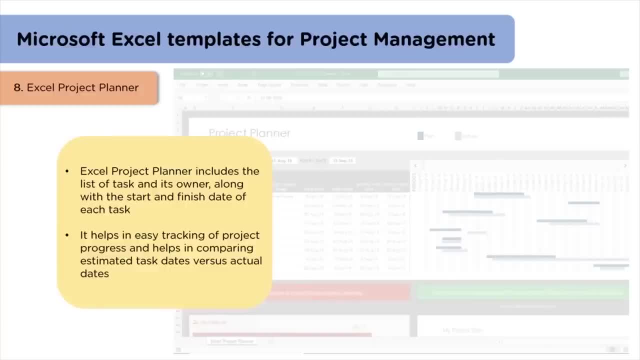 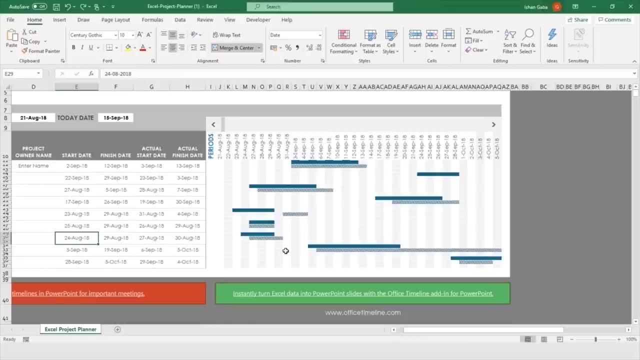 This helps in monitoring each task and comparing the estimated task date with the actual ones. Let's have a look at this template in Excel. We can see the Gantt chart with respect to the data entered. Let's make changes at several places in the data. 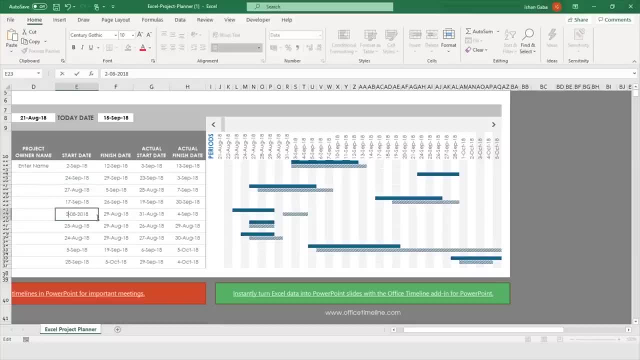 We can make this 22 to 24.. We will make this 23 go to 2. And we can make this 5th September go to 15th September. And when we make the changes, we can realize the Gantt chart is fluctuating. 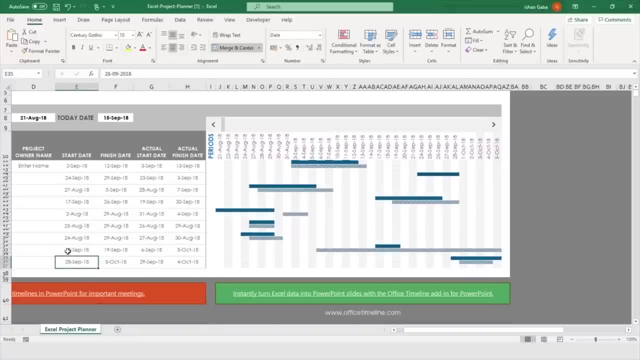 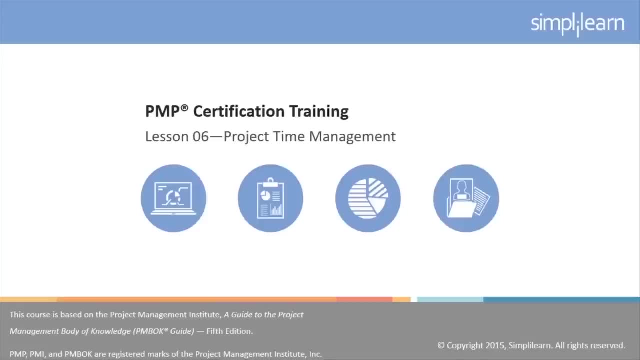 So this is how we can make changes. We can use this template to plan a project effectively and efficiently. In this lesson, we will focus on project time management. Let us begin with the objectives of this lesson. After completing this lesson, you will be able to: 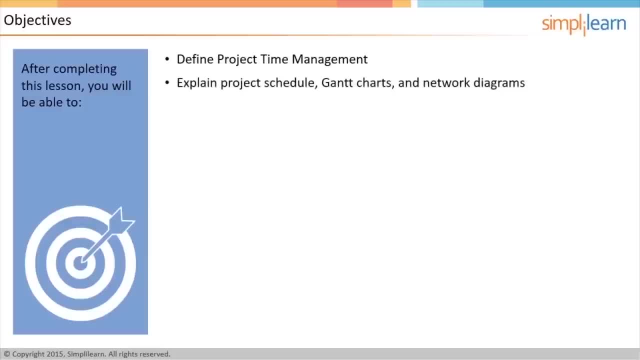 Define project time management. Explain project schedule, Gantt charts and network diagrams. Identify the key terms used in project time management. Describe the project time management processes. Explain various schedule network analysis techniques. In the next screen, let us take a quick look at the project management process map. 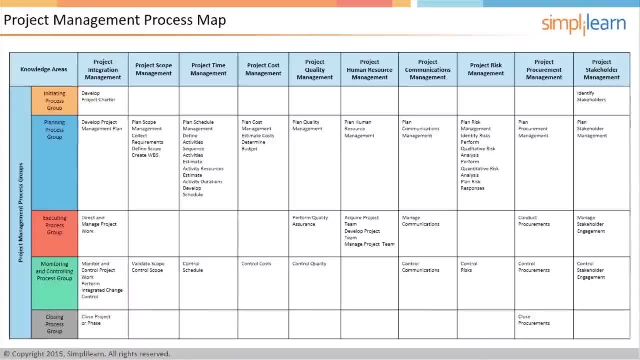 There are 47 processes in project management, grouped into 10 knowledge areas and mapped to 5 process groups. In this lesson we will look at the third knowledge area, that is, project time management and its processes. Let us begin with the first topic of this lesson. 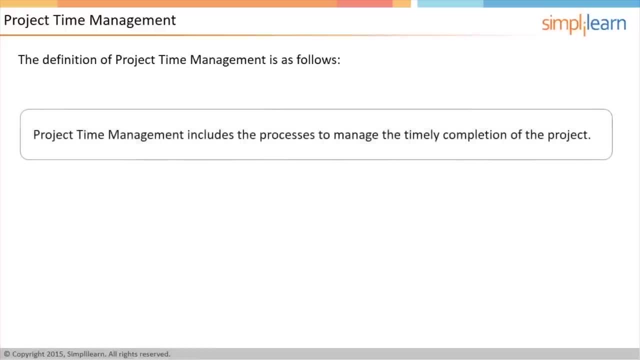 Project time management. The purpose of project time management is to ensure that the projects get completed on time. This knowledge area is primarily concerned with developing a project schedule and ensuring that project goes as per the agreed schedule. If there is a need to change the project schedule, the change should happen by following a proper change control procedure. 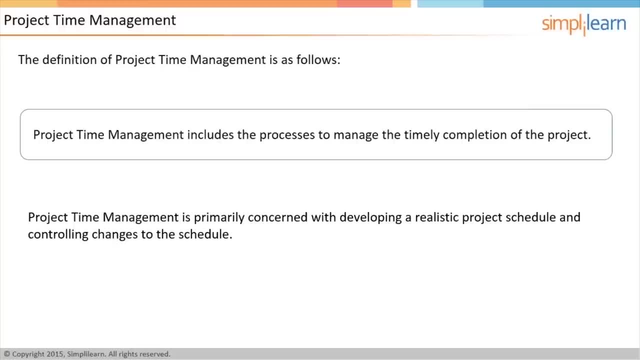 Another term used in the PMP examination is schedule management plan. Schedule management plan is part of the project management plan and has information on the planned project schedule and its management and control. Let us discuss the key activities of project time management in the next screen. 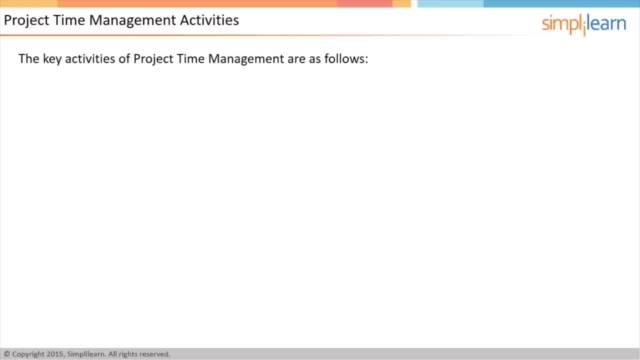 The key activities that are part of the project. time management include identifying activities, estimating time and resources, and sequencing activities. It is important to identify a list of activities that would be a part of the project. Next, an estimation of time and resources required for completing the identified activities are done. 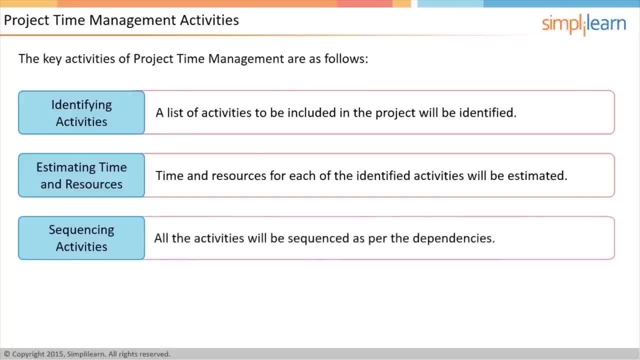 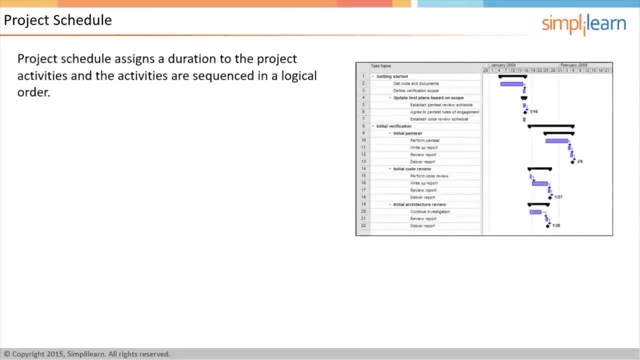 Finally, these activities need to be sequenced as per the dependencies In the next screen. let us discuss project schedule. Project schedule represents the time dimension of the project plan and has information like when the project would start, when each of the project activities would happen. 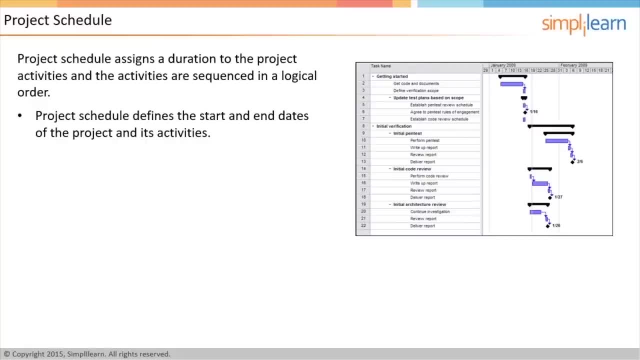 in what order the project activities would happen, when project would be completed, etc. Usually, software system is used to develop the project schedule. The project team can enter the list of activities in the software, as well as their dependencies, and the software can produce the project schedule as the output. 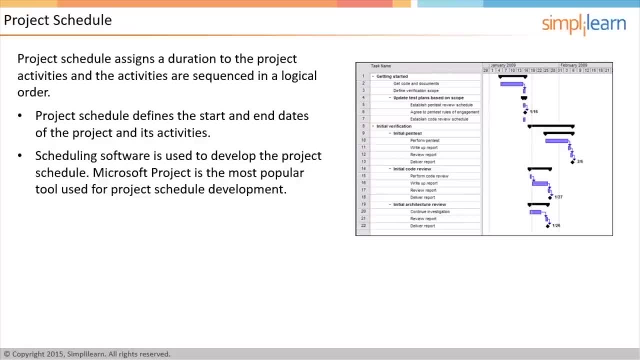 Microsoft Project is the most popular tool used for project schedule development. Generally, project schedule is considered similar to project management plan. Project management plan is different from project schedule. Project management plan not only has information about the project schedule, but also other important project-related plans. 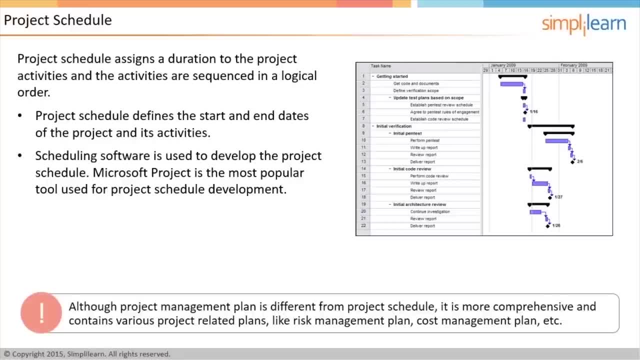 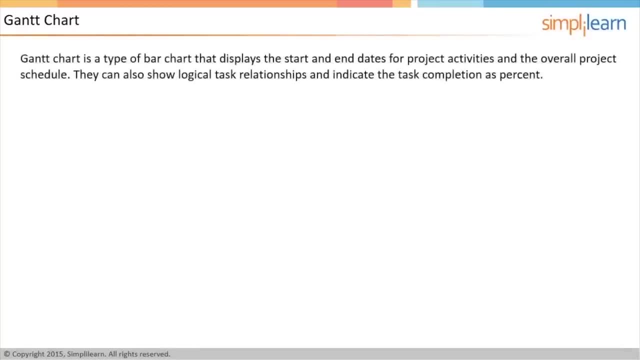 like risk management plan, cost management plan, etc. Let us focus on Gantt chart in the next screen. Gantt chart is a list of activities and is a type of bar chart that illustrates a project schedule. It shows the dependencies between the project activities. 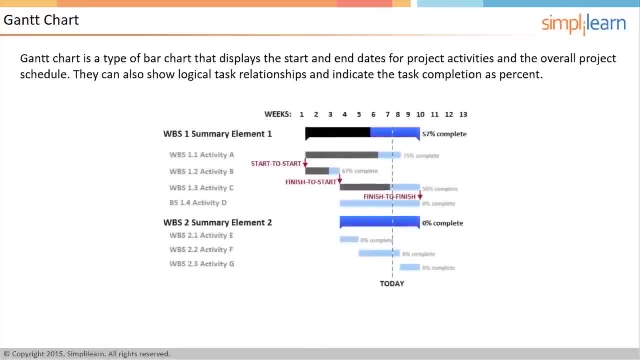 as well as their percent completion. A sample Gantt chart is shown on the screen. Two summary elements of the work breakdown structure are depicted. To complete those elements, there are a number of activities under them. Some of these activities have dependencies. For example, activity B and C have a dependency. 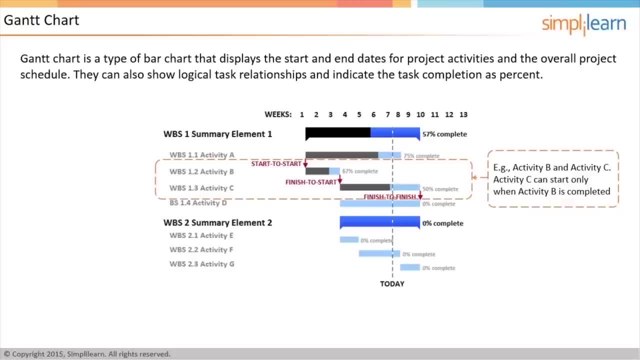 Activity C can start only when activity B is completed. The chart gives you an idea about when specific activities are planned to finish and when the overall WBS element will get delivered. Create tasks and work with the Gantt chart. This will make answering Gantt chart-based questions easy and fun. 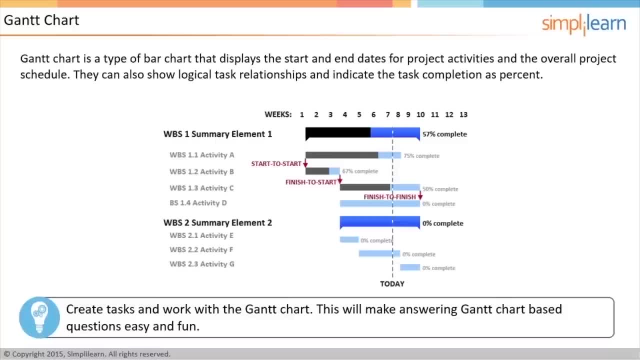 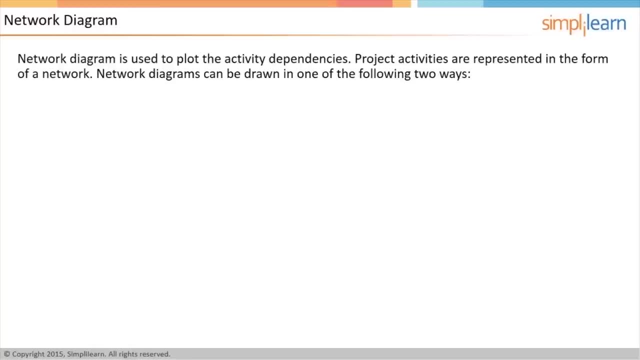 In the next screen. let us understand the relationships that exist among project activities. Network diagram is extensively used in the project time management knowledge area to plot the activity dependencies. This is a graphical representation of the project activities in the form of a network. There are two ways to draw a network diagram. 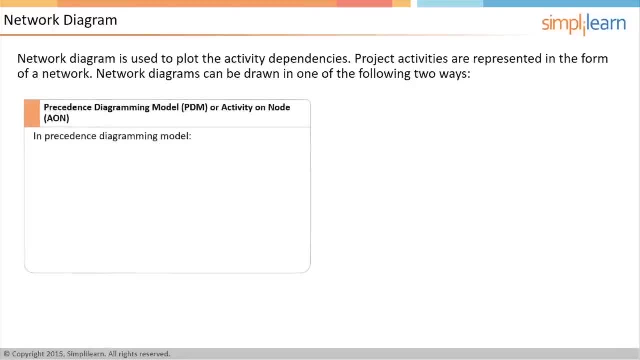 In Precedence. Diagramming Model or Activity on Node. boxes represent activities and the arrows indicate the dependency. This type of network can have all four types of relationships between the activities. In Arrow Diagramming Model or Activity on Arrow, the arrows represent activities. 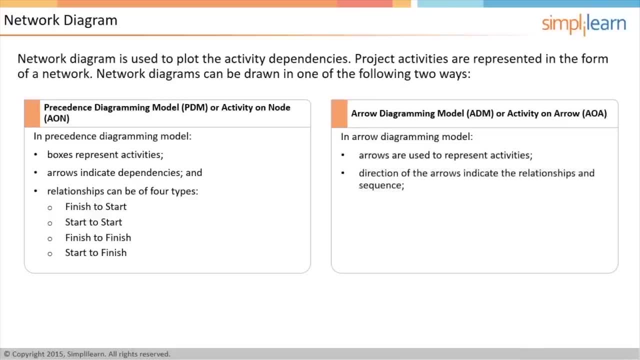 The relationships and sequences can be inferred from the direction of the arrows and linkages between the activities. In such types of network, only finished-to-start relationships can be shown. Such diagrams may need to make use of dummy activities to indicate some dependency between the activities. 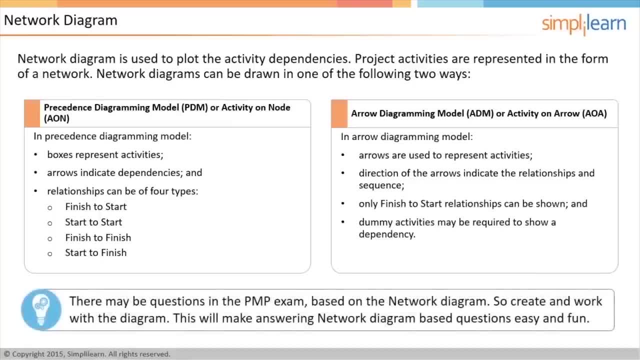 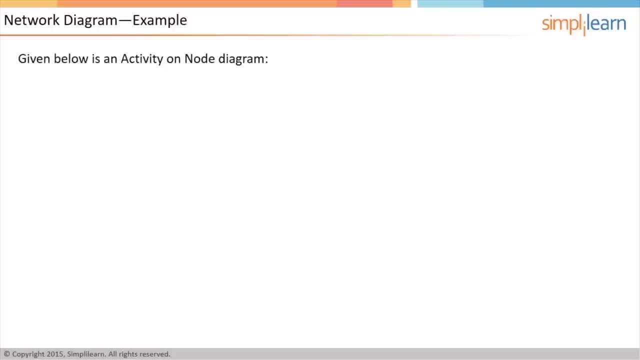 There may be questions in the PMP exam based on the network diagram, so create and work with the diagram. This will make answering network diagram-based questions easy and fun. In the next screen, let us look at a network diagram. A sample network diagram is shown on the screen. 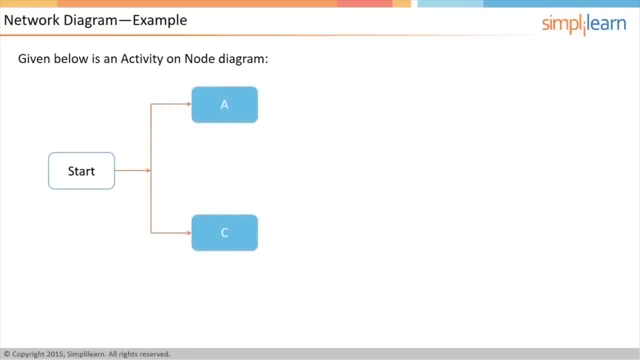 Activities A and C can happen in parallel. B and D require both A and C to complete, whereas E requires both B and D to complete. Activity on Arrow Network Diagram makes use of hammock activities. They are used to show a comprehensive summary activity. 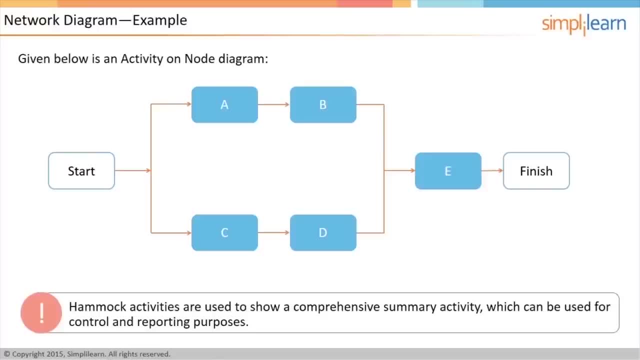 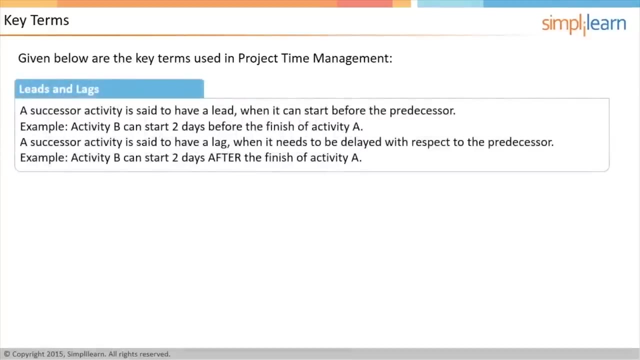 combining several other activities underneath for control and reporting purposes. In the next screen let us look at a few important terms in time management. When a successor activity can start before the predecessor activity can complete, it is considered lead. For example, you can start preparing the test environment. 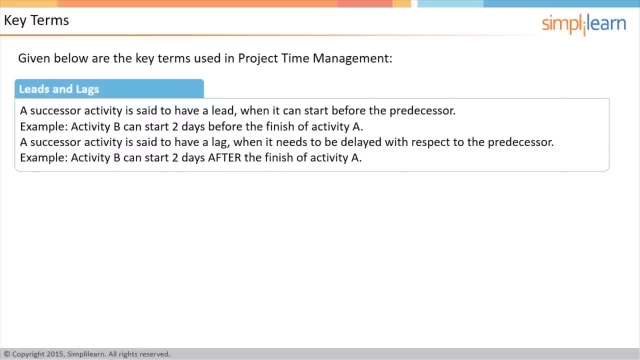 two weeks before the development activity finishes. When the successor activity has to wait for a few days after the predecessor activity has been completed, it is considered lag. For example, one needs to wait for two days for the foundation to settle before work on the pillars for the next floor starts. 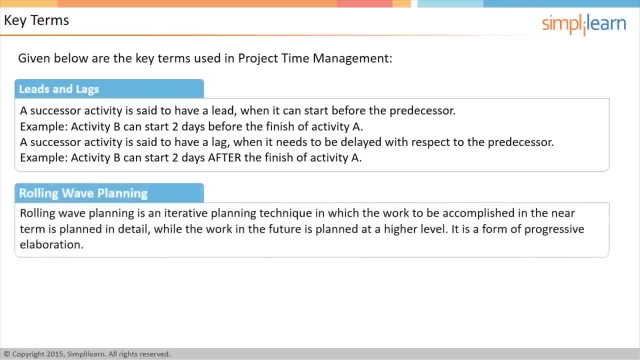 Rolling wave planning is an iterative planning technique in which the work to be accomplished in the near term is planned in detail, while the work in the future is planned at a higher level. It is a form of progressive elaboration In the context of estimating techniques. 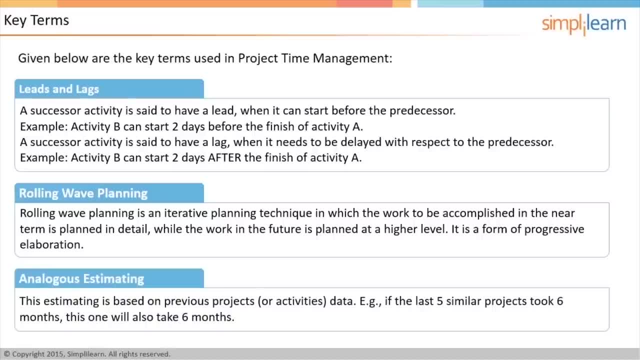 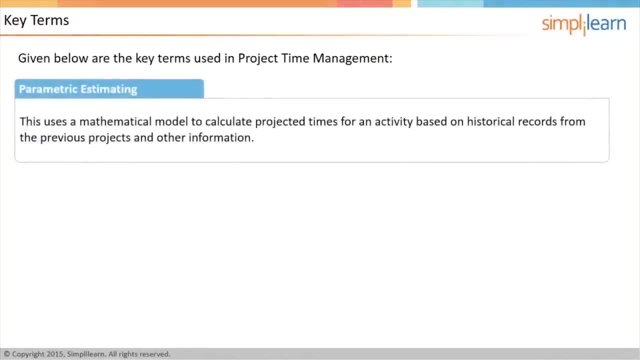 analogous estimating is based on the previous project data. Therefore, if the last five similar projects took six months to complete, the next one will also take six months. This technique employs expert judgment. Another estimating technique is parametric estimating. This technique uses a mathematical model. 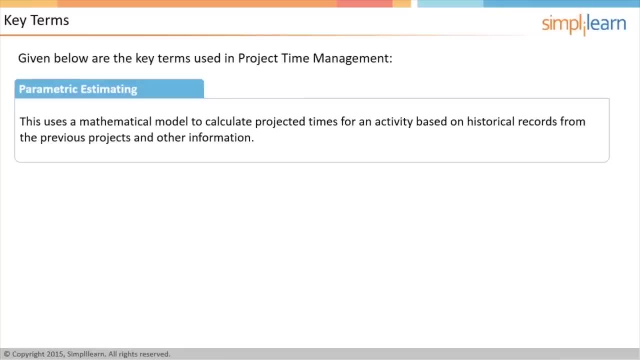 to calculate projected time for an activity based on the historical records from previous projects and other information. A few common parameters are identified based on the previous project data, and that parameter is used to predict the time required to complete the next activity or project, For example. 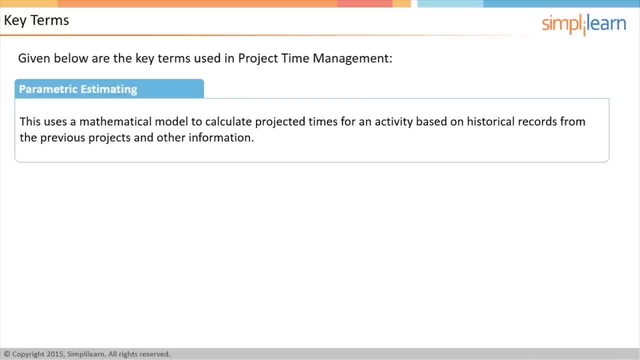 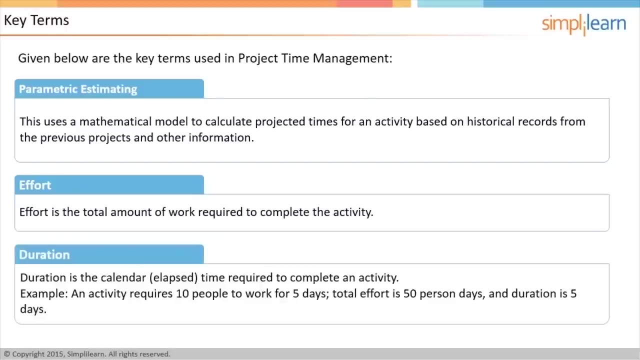 you can normally complete 10 kilometers of highway construction lanes a week. Effort is the total amount of work required to complete the activity. Duration is the amount of time it takes in terms of a lab store calendar days If you have an activity that requires. 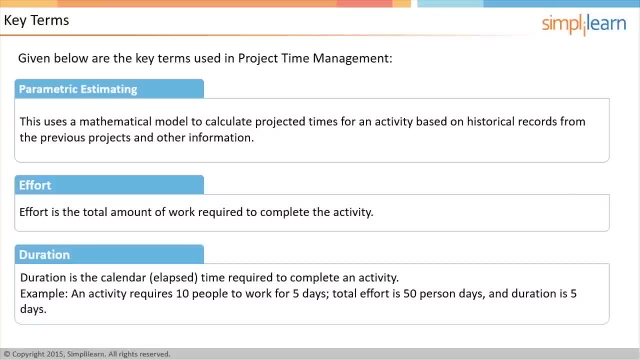 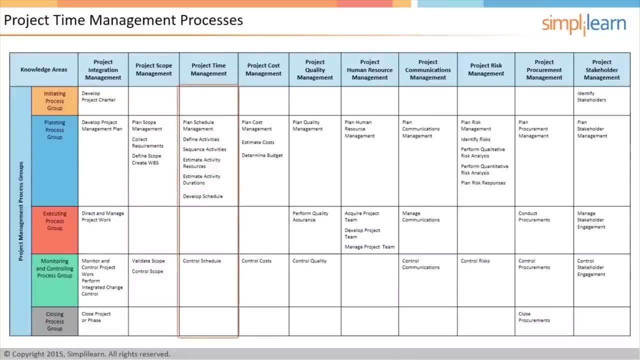 10 people to work for five days. the total effort is 50 person days, but the duration is only five days. In the next screen let us look at the project time management processes. There are seven project time management processes. They are plan schedule management. 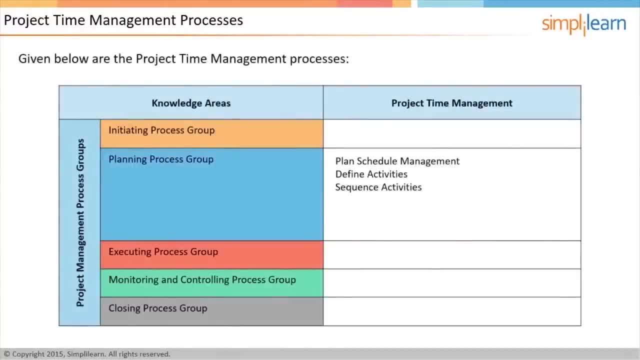 define activities, sequence activities, estimate activity resources, estimate activity durations, develop schedule and control schedule. The first six processes are executed during the planning process group. The ultimate goal of these planning processes is to develop the project schedule. The seventh and the last process: 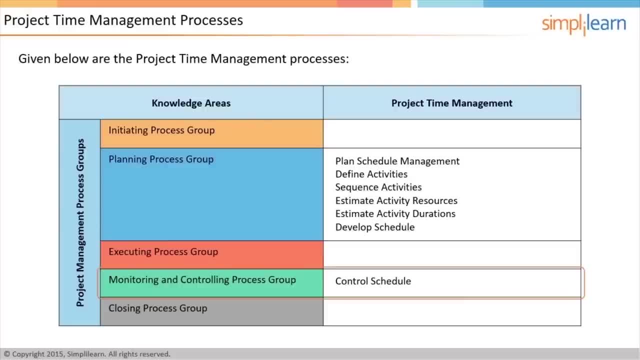 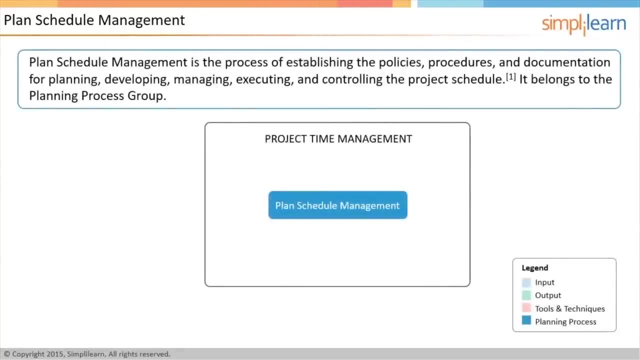 is a part of the monitoring and controlling process group. In the next few screens let us discuss these processes in detail. We will begin with plan schedule management. As defined in PMBOK Guide, plan schedule management is the process of establishing the policies. 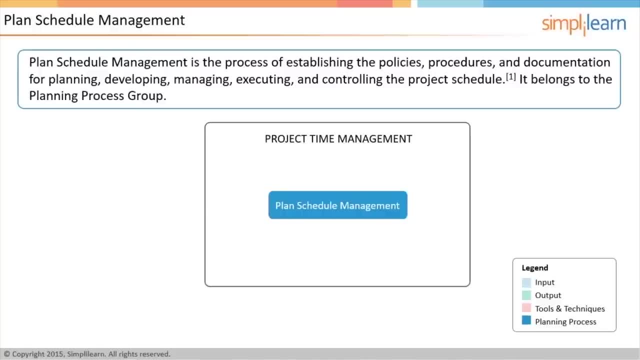 procedures and documentation for planning, developing, managing, executing and controlling the project schedule. It belongs to the planning process group. Let us look at the inputs to this process. The project management plan provides other subsidiary plans and will guide the schedule planning. 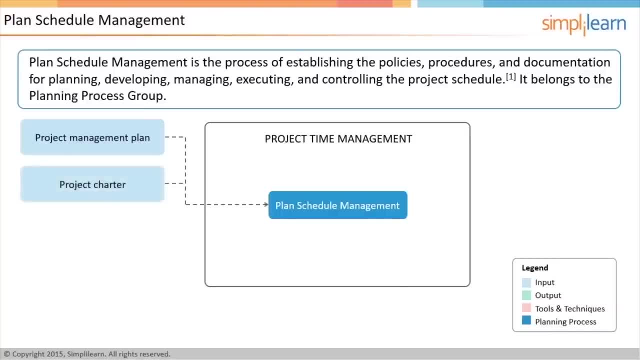 activities on the project. The project charter provides an overall context and the high-level product and project description which might help determine the approach for schedule management. Few projects might have scheduling constraint. For example, projects of Olympics 2016 should be completed at the same time. 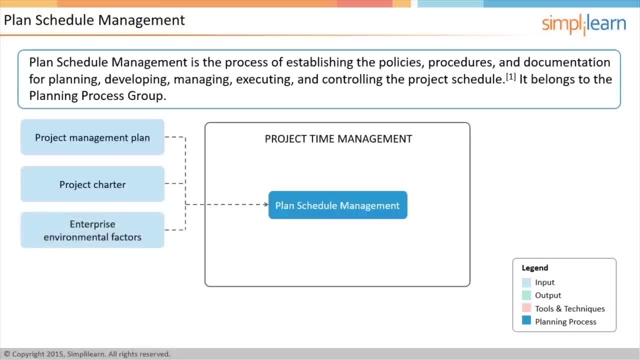 Enterprise. environmental factors provide the organizational context to the project, including the culture of the organization, the infrastructure, like scheduling systems, available key personnel and so on. Organizational process assets provide inputs such as policies and procedures, templates, past performance data and estimates. 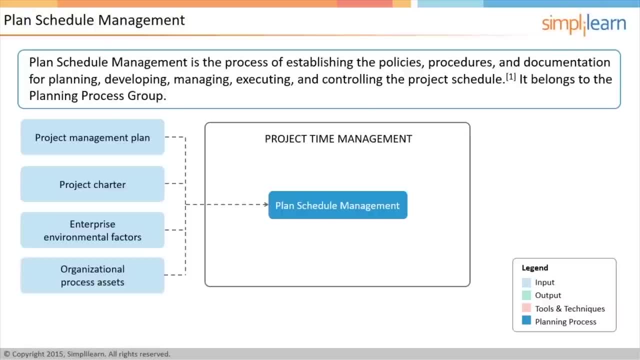 historical information and knowledge base. Now let us look at the tools and techniques employed in this process. Expert judgment refers to input received from knowledgeable and experienced resources. Experts can draw from their previous experiences the proper approach to govern the schedule on a project. 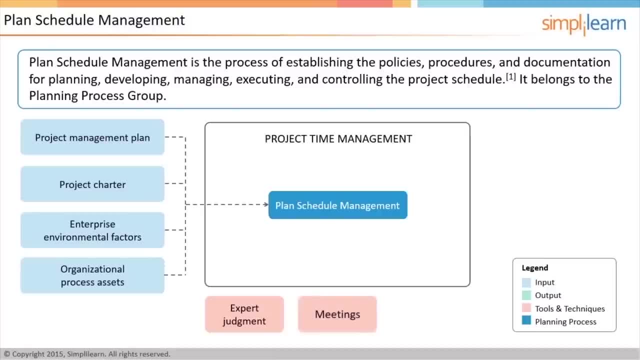 Meetings may be organized to determine the schedule management plan. Anybody responsible for the project schedule management, such as the project manager, sponsor, customer and other stakeholders, must attend these meetings. Several analytical techniques may be used to determine the schedule management plan. These may include different planning approaches. 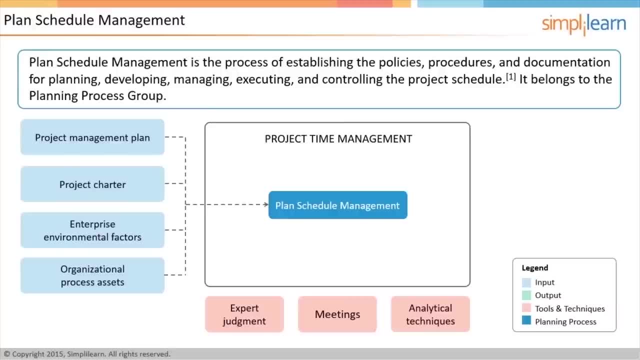 and philosophies, such as rolling, wave planning or different scheduling software that allow to build what-if scenarios and study the effect of advanced scheduling techniques like leveling, fast tracking and crashing. Now let us look at the outputs of this process. Schedule management plan is a component. 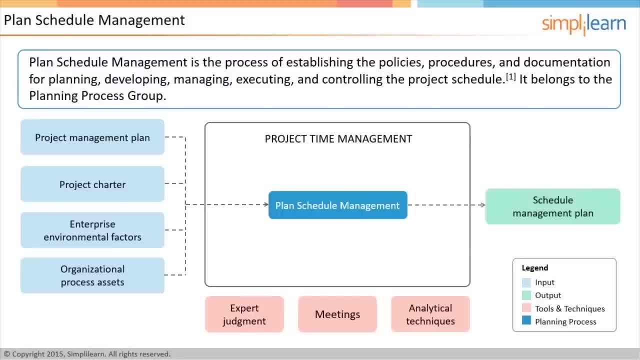 of the project management plan that describes the criteria and activities required to arrive at the project schedule, as well as how the project may be baselined, monitored and controlled. In the next screen, let us define activities process. Define activities is the process of identifying. 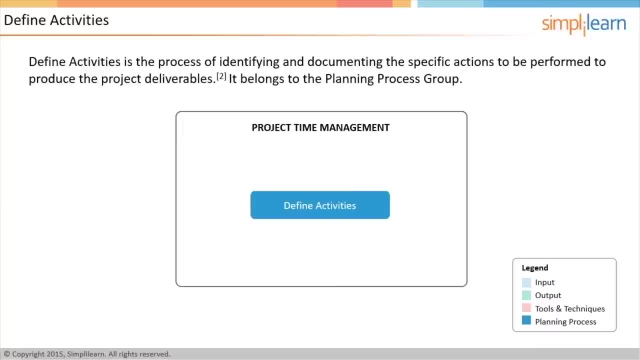 the specific actions to be performed to produce the project deliverables. It belongs to the planning process group. The important input for the define activities process is the scope baseline. Scope baseline is a term used collectively to refer to project deliverables, constraints and assumptions of the project. 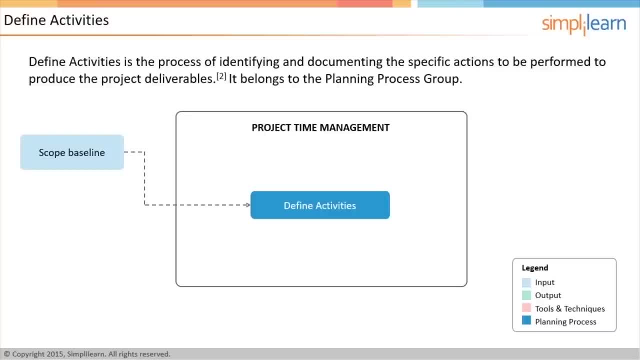 In addition to the scope baseline, the other inputs in this process are enterprise environmental factors, organizational process assets and schedule management plan. A reason why enterprise environmental factors is an input to define activities is because the organization might be using project management software to define activities. 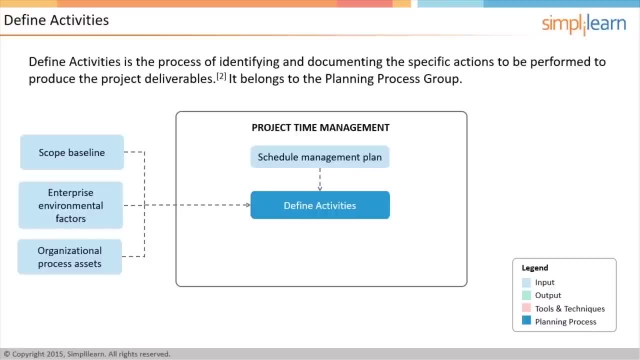 and that may influence the activity definition process. The knowledge base containing historical information regarding activities lists used by previous similar projects is a good example of organization process assets applied to scheduling. The tools and techniques used in defining activities are decomposition and rolling wave planning. The last technique is expert judgment. 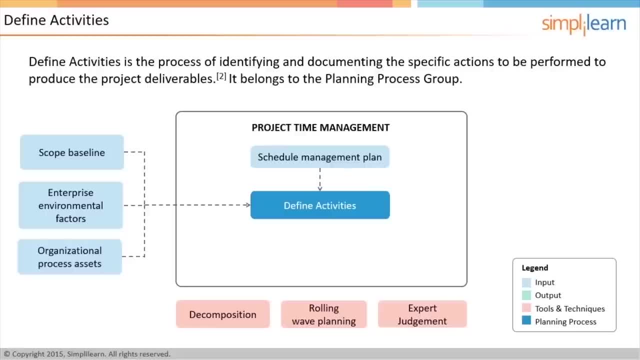 where the experience of project team members is used in developing detailed activity lists. The output of the process is activity list, activity attributes and milestone list. Activity list contains a list of identified activities. Activity attributes are the additional information about the activity itself. 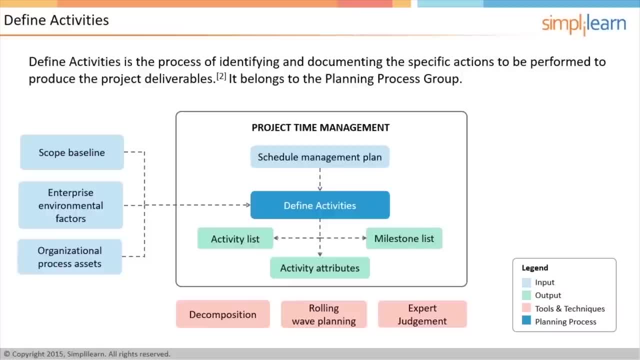 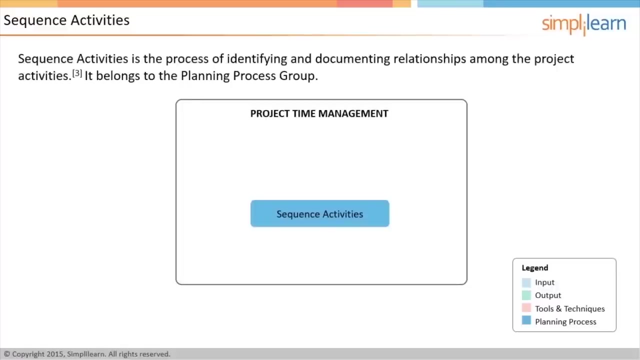 A milestone is a significant point or event in the project. A milestone list identifies all the milestones and indicates whether the milestone is mandatory or optional. Let us move on to the next process: sequence activities. Sequence activities is the process of identifying and documenting relationships among the project activities. 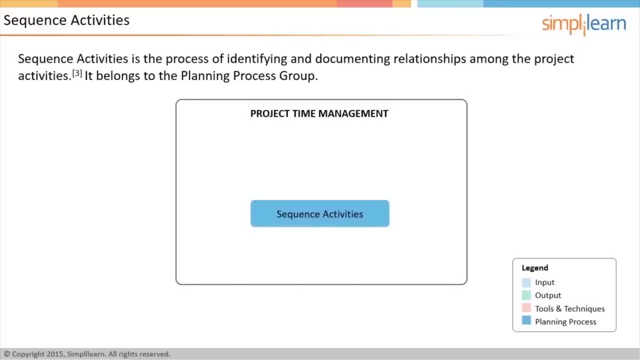 and is also part of the planning process group, For every activity and milestone, except the first and last one, is connected to, or at least one predecessor and one successor. The inputs to this process are activity list, activity attributes and milestone list. 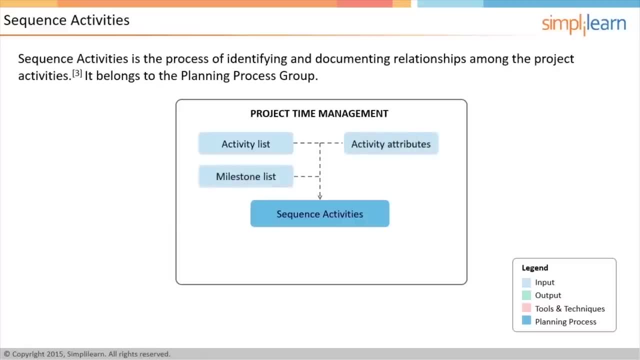 All these are the outputs of the defined activity process. The other inputs are schedule management plan and project scope statement. Schedule management plan provides guidance in terms of methodology to be employed for many of the scheduling activities on the project Organization process. assets are also an input. 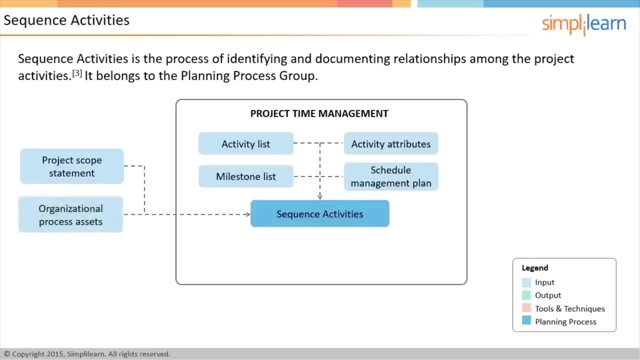 to sequencing activities because the organization might have some kind of knowledge base for scheduling project activities. The enterprise environmental factors relevant to this process may be scheduling tools in use, project management information systems, work authorization systems, etc. One of the important tools and techniques used: 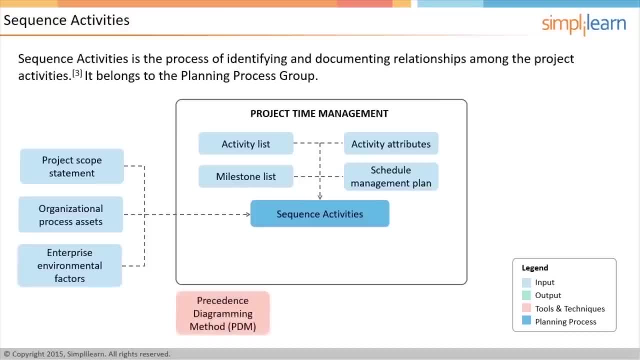 in sequencing activities is the precedence diagramming method. In this method, the activities are drawn on a network diagram and all the different kinds of dependencies between the activities are determined. While determining activity dependency, it is important to identify the type of relationship or dependency between the activities. 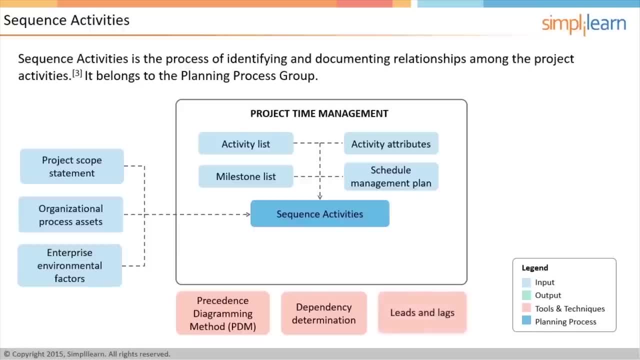 The other technique is leads and lag, which is widely used for sequencing activities. The output of the process is the project schedule network diagram, which is a graphical representation of the project activities in a form of network which also shows the activity dependencies. While designing the network diagram, 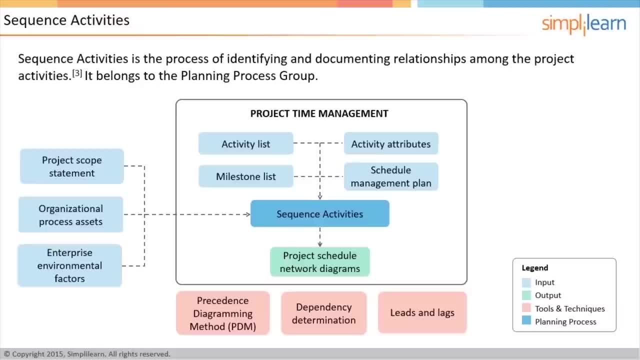 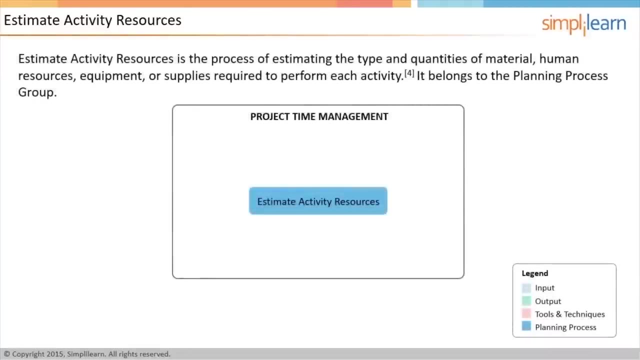 new activities might be identified and that would result in some of the project document updates, especially the ones that list all the project activities In the next screen. let us look at the estimate activity resources process After sequencing the activities. the next step in project time management is 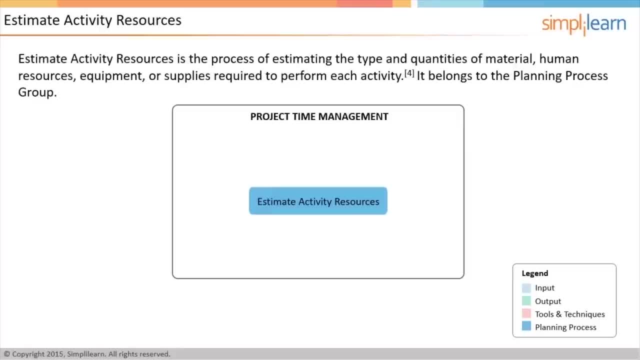 estimating the resources required to accomplish each of the identified activities. Estimate activity resources process also belongs to the planning process group. Here resources do not mean only the human resources but includes all other resources like equipment, raw materials, machinery, etc. Schedule management plan is the first input. 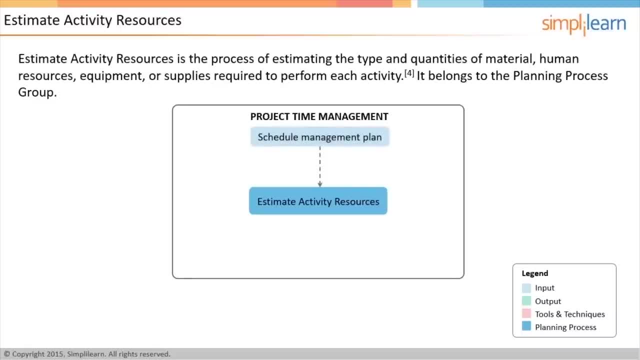 Schedule management plan provides guidance in terms of methodology to be employed for many of the scheduling activities on the project. The other inputs to this process are an activity list and activity attributes that are the outputs of the time management processes. Risk register is another input. 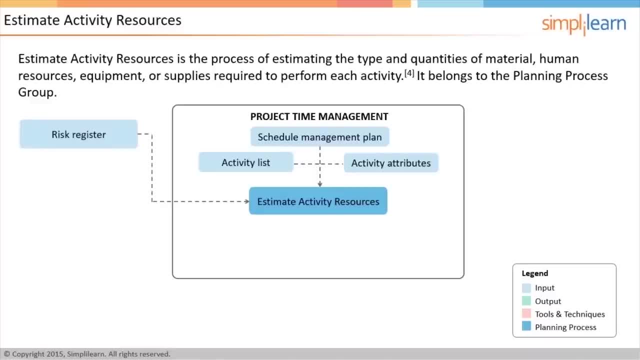 Risks to the project may influence the decisions about the resources that need to be deployed. Hence risk register becomes an input to this project. In addition, activity cost estimates are another input. Cost and resource estimates on a project are interrelated and influence each other. 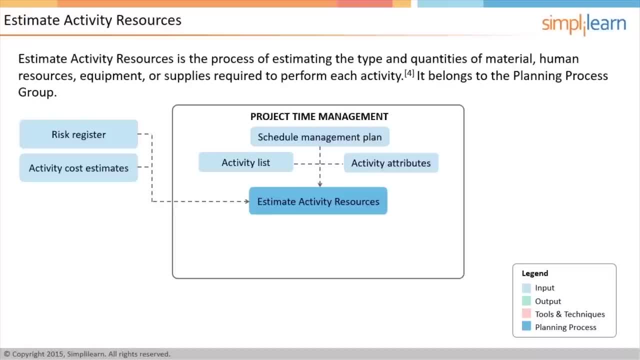 For example, the cost might dictate the number and type of resources that can be employed, or the time might dictate the cost that may need to be incurred. Along with this, the resource calendar is also an important input because it has the information about the availability of each of the resources. 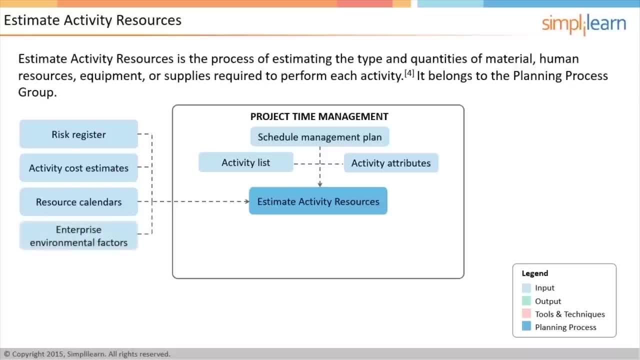 Some of the enterprise environmental factors that can influence estimating activity resources are: availability of required resources within the organization. The organizational process- assets- is also an important input, as the organization might have standard policies for staffing or for hiring contractors on the project. With all these inputs available, 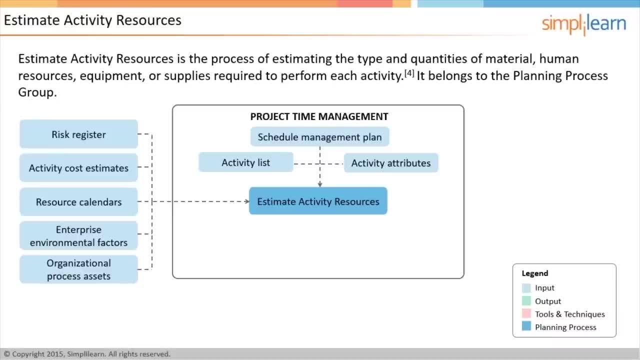 for estimating activity resources. there are various techniques used for estimating the required resources. The first technique is using expert judgment. In this technique, an expert in resource planning and estimating can estimate each of the activities. The next technique used is alternative analysis. In this the activities are analyzed. 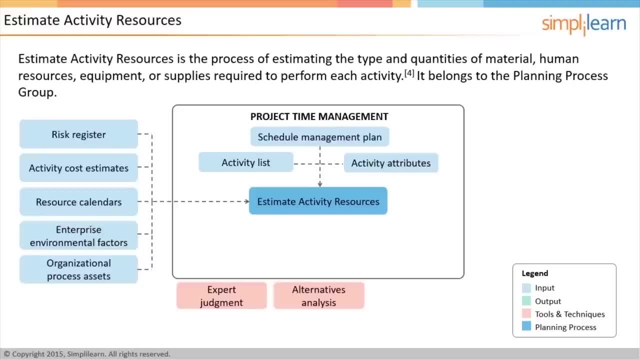 to identify different ways of completing them. This is to ensure only the required resources are assigned to each of the activities. This helps in resource optimization. Along with the two techniques, many organizations routinely publish their estimating data, and this could be used in activity resource estimation. 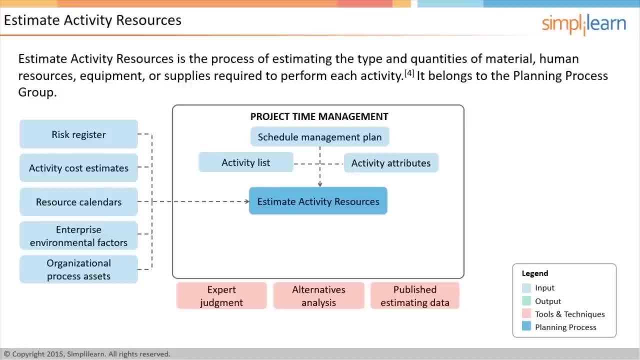 Another technique that is routinely used in activity estimation is bottom-up estimating, which is decomposing the activity further down to understand it in more detail and estimating at that level. Later all such estimates are added to arrive at the estimate of the activity In real projects. 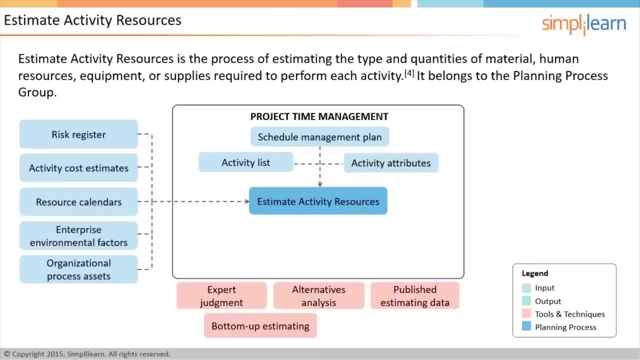 one has to use all the estimates to estimate each of the activities. Sometimes the project management software also helps in estimating. The software estimates are based on the inputs provided to it. Software should only be considered as a supporting tool in estimation and never fully rely on its output. 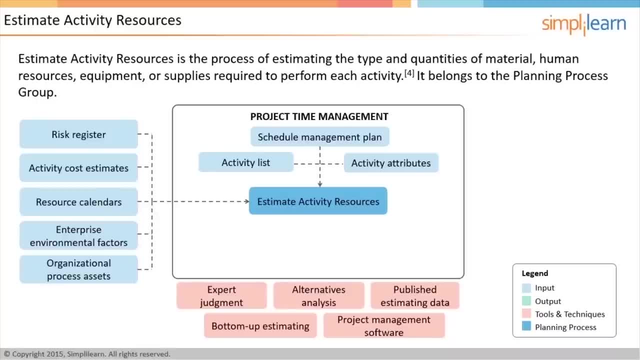 Clearly, the output of this process is the activity resource requirements. Along with this, resource breakdown structure is also prepared. The resource breakdown structure is the categorization of all the required resources in various categories, that is, human resources, equipment, raw materials, etc. 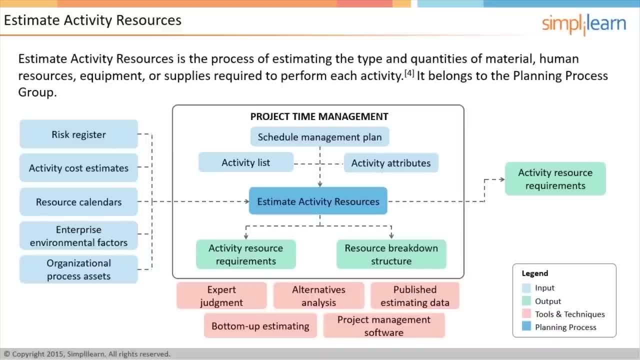 In the process of estimation, several other project documents may also be updated. For example, the resource estimates are directly correlated with cost estimates. Let us now move on to the next process: estimate activity durations. The next process is to estimate the duration required. 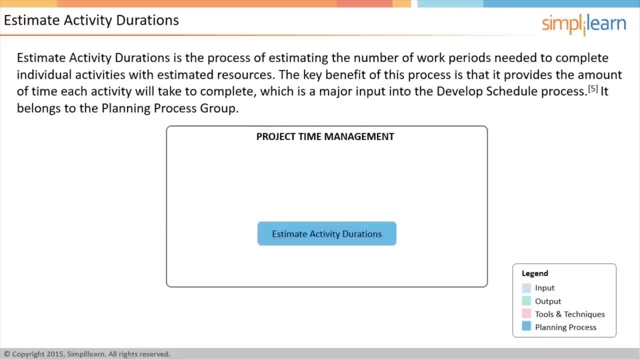 to complete each of the activities. The duration estimation should be done by someone who is familiar with the project. For example, the same activity, if done by a high-skilled resource, would take less time compared to a less skilled resource. This may vary. 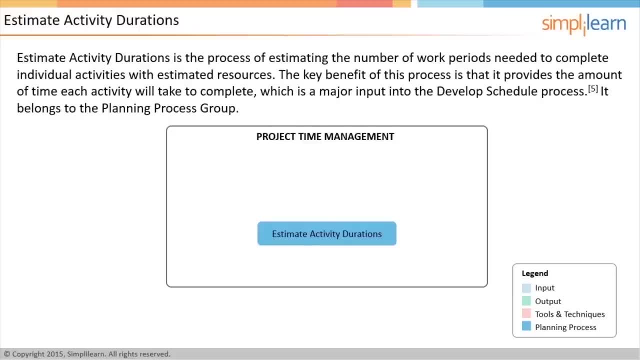 regardless of the resource used due to the project requirements. In addition, the activity duration estimation should be updated continuously as you move ahead with the project, because as the project progresses, there will be more clarity on the project. The inputs of this process are similar to the ones 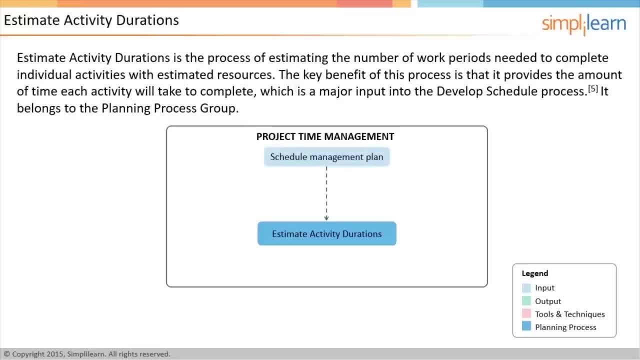 in sequence activities process. Schedule management plan is the first input. Schedule management plan provides guidance in terms of methodology to be employed for many of the scheduling activities on the project. For instance, it may contain information about the estimation techniques to be employed and the people who need to be involved. 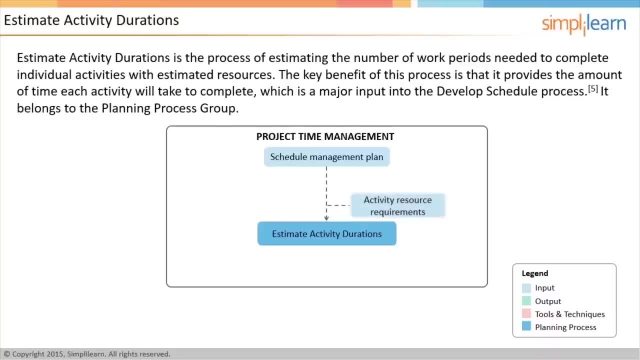 in the estimation process. Activity resource requirements is also an input to this process, because resources assigned to an activity would significantly affect the activity duration, That is, the lower-skilled resources would take more time than the high-skilled resources. The other inputs include activity list. 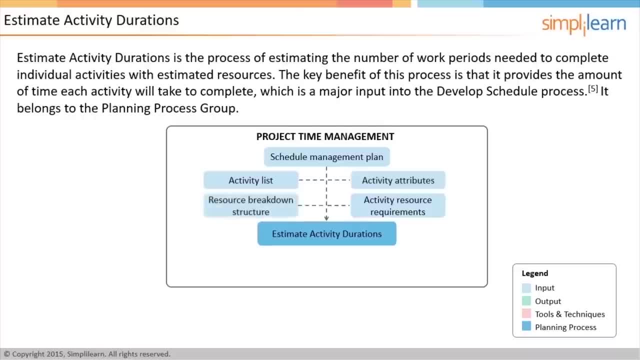 activity attributes and resource breakdown structure. Resource calendars are also an input to this process. The type and skill set of resources available to the team may have an impact on the time it would take to complete the activities. Risks to the project may influence. 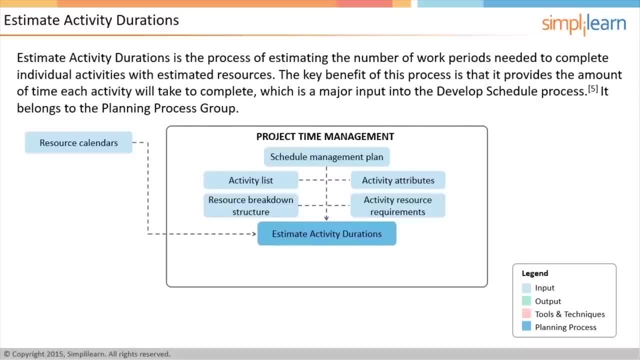 the decisions about the time required to complete the activity. Hence risk register becomes an input to this process. The project scope statement defines the constraints and assumptions affecting the project duration. An example of enterprise environmental factor that can affect duration is organization's productivity metrics. 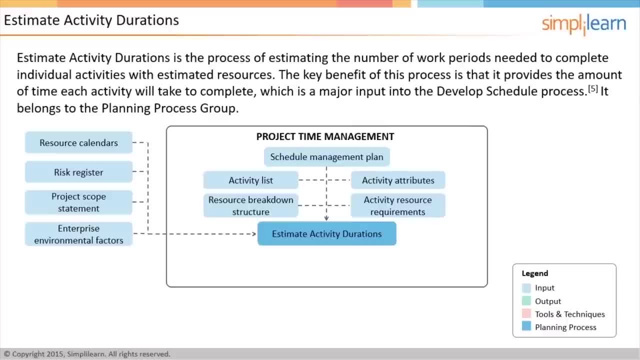 which is collected based on the experiences from multiple projects. The last input in this process is organizational process assets. Now let us look at the tools and techniques used for estimating activity durations. First is the expert judgment, which means using previous project experiences in estimating the current project duration. 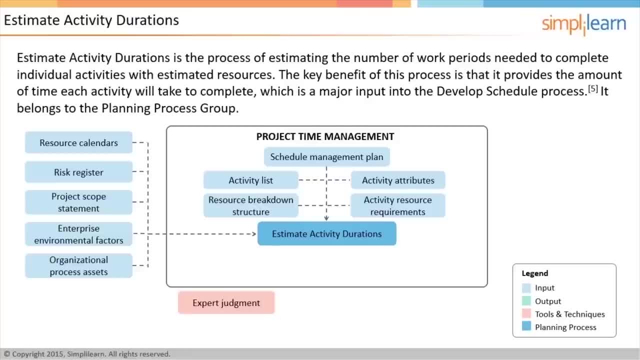 This can be used with other estimation techniques and used to reconcile differences if different techniques result in different estimates. Three-point estimating is a method where three estimates are used instead of one. It is part of a project management philosophy known as Program Evaluation and Review Technique. 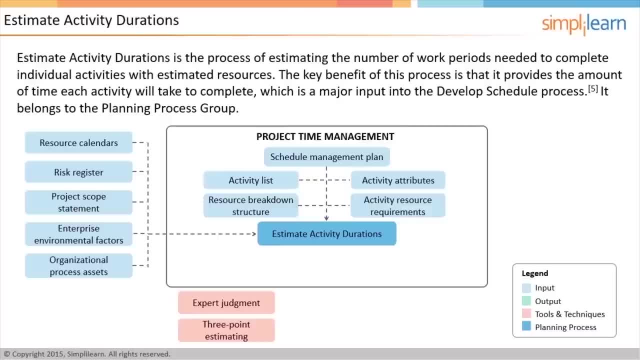 Estimating activity durations is often done as a team exercise, as each activity may require multiple skill sets to be applied. Therefore, it is important to use group decision-making techniques to arrive at a consensus or at least an estimate that is acceptable to all the team members. 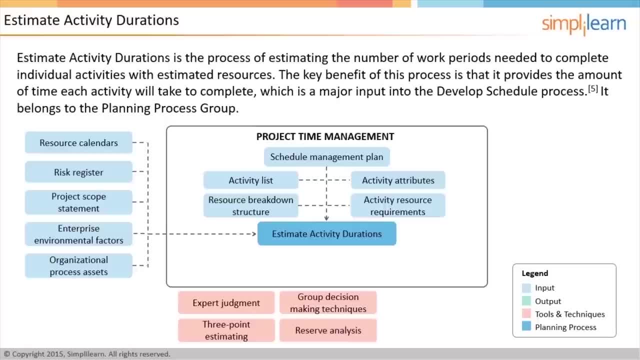 Reserve analysis adds buffers into the project schedule to deal with any uncertainty. The contingency reserve may be added as a percentage of the activity duration or fixed number of work periods. The other tools and techniques are analogous estimating and parametric estimating The outputs of this process. 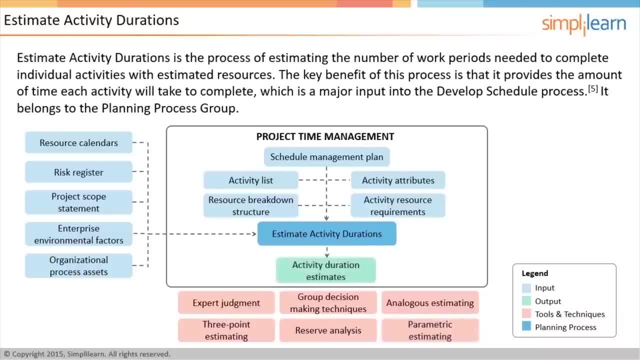 are the activity duration estimates and project documents updates. The activity duration estimates is represented in terms of the range of possible results. For example, 10 days plus minus 2 days. that is, the activity would take minimum 8 days and maximum 12 days. 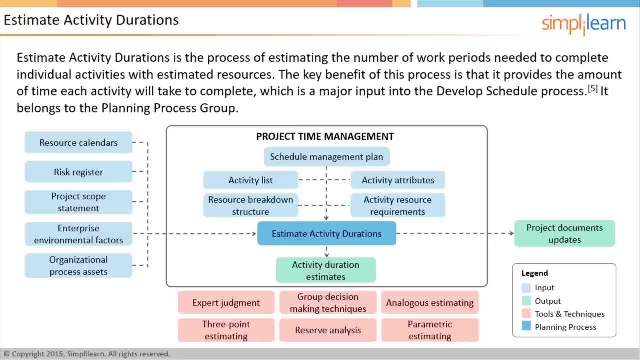 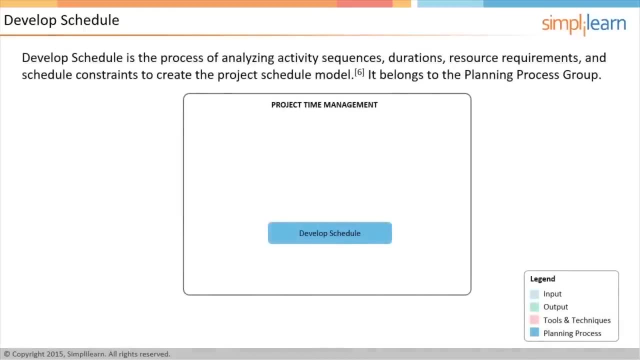 In the next screen. let us look into a business scenario to understand this concept better. After reading the problem statement, click the Solution button to look at a possible answer. Develop Schedule is the process of analyzing activity sequences, durations, resource requirements and schedule conditions. 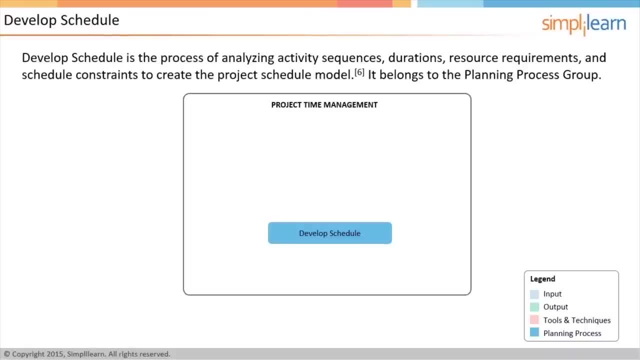 Schedule is the process of creating a project schedule. It belongs to the Planning Process Group. Generally, scheduling software is used for developing the project schedule. Entering the activities, durations and resources into a scheduling tool generates a schedule with planned dates for completing project activities. 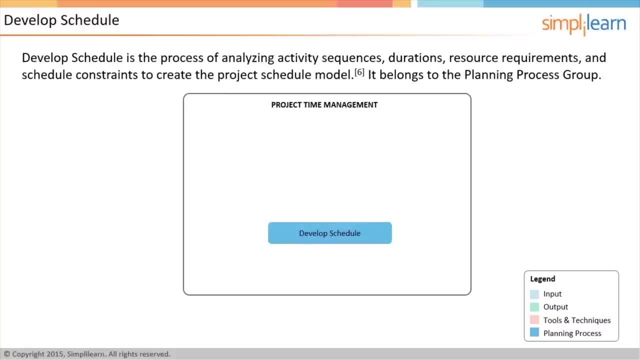 Developing a project schedule is an iterative process. Revising and maintaining a realistic schedule is a task in itself and it continues throughout the project as the work progresses. The most of the inputs of this process are the outputs of Estimate Activity Durations process. 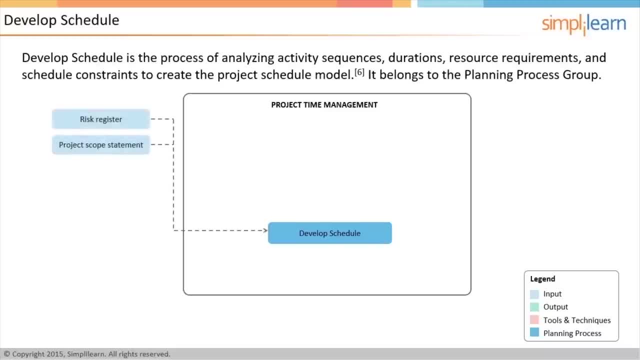 They are: Risk Register. Project Scope Statement. Project Staff Assignments, Resources, Calendars, Organizational Process, Assets, Enterprise, Environmental Factors. Schedule Management Plan. Activity Lists. Activity Attributes. Project Schedule- Network Diagrams. Activity. Resource Requirements. Resource Breakdown Structure. 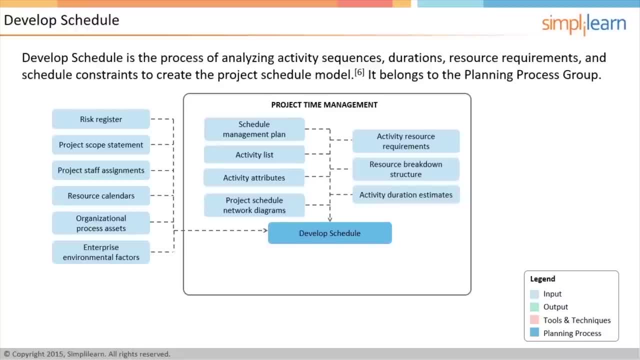 and Activity Duration Estimates. Various tools and techniques are used to develop schedule process Schedule Network Analysis is a technique that generates project schedule. It employs various analytical techniques, such as critical path method, critical chain method, modeling techniques and resource optimization techniques. It also uses optimization techniques. 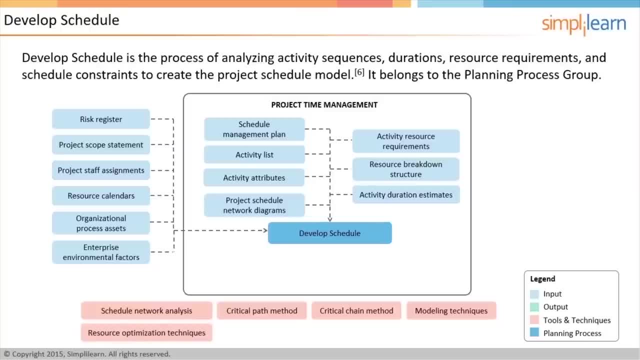 to create the project schedule. The other tools and techniques include Leads and Lags, Schedule Compression and Scheduling Tool. Let us now look at the outputs of this process. The project schedule consists of a minimum planned start date and planned finish date for each activity. 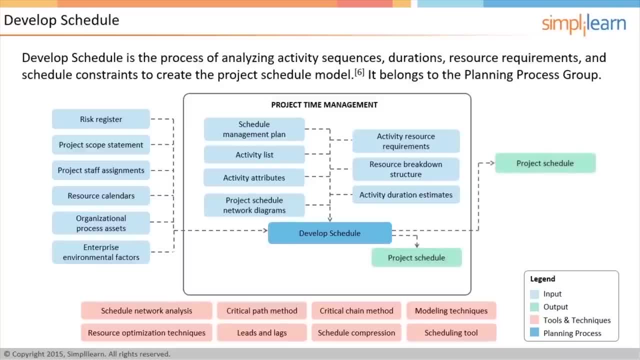 Although project schedule can be represented in tabular format, it is more often represented graphically, using either bar charts and network diagrams, or a combination of the two. The final schedule, which is the output of the developed schedule process, is also called schedule baseline. 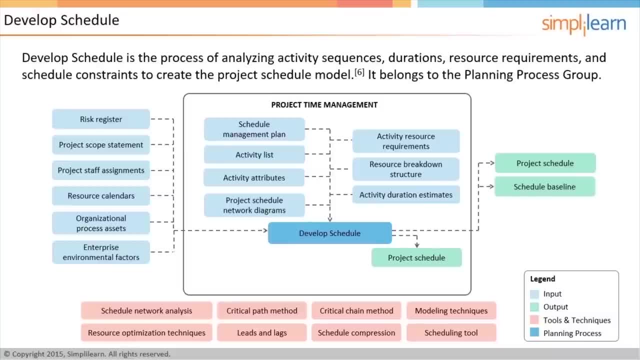 Once the schedule is baselined, it can be changed only through formal approvals. Meeting the schedule baseline is one of the measures of project success. Scheduled data produced may include number of resources, key milestones, etc. Project calendars specify the available working days. 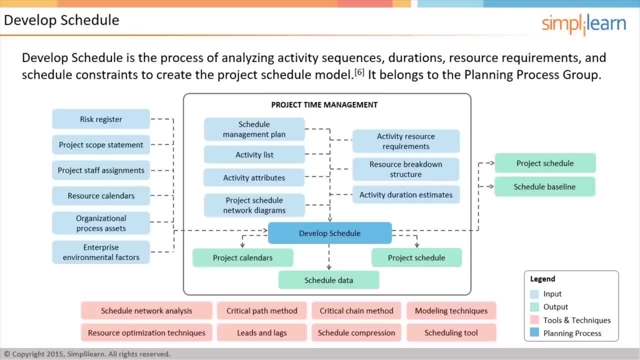 and the number of shifts in each day. It indicates how many hours and days are available for the work of the project to be completed. Project management plan updates are a result of the developed schedule process. Many of the other subsidiary plans of the project plan may get impacted. 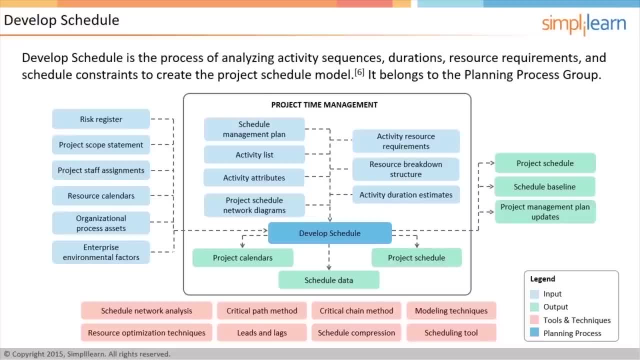 which may include cost management plan, scope management plan, risk management plan, etc. This may also result in other project documents being updated In the next few screens. let us discuss schedule network analysis techniques. It is essential to know if the required resources 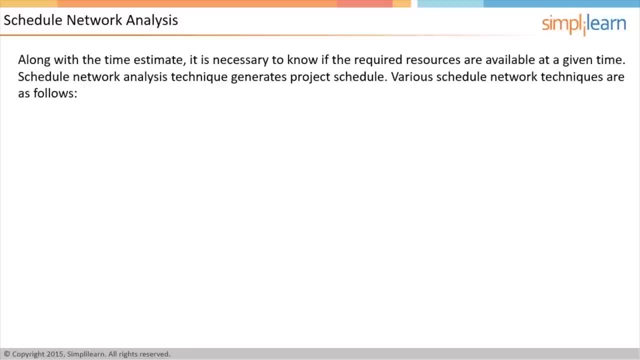 are available at that time, along with the time estimate of each of the activities. Since schedule is calendar-based, it helps in estimating the same Schedule. network analysis technique generates project schedule. There are various schedule network techniques. Critical path method relies on determining. 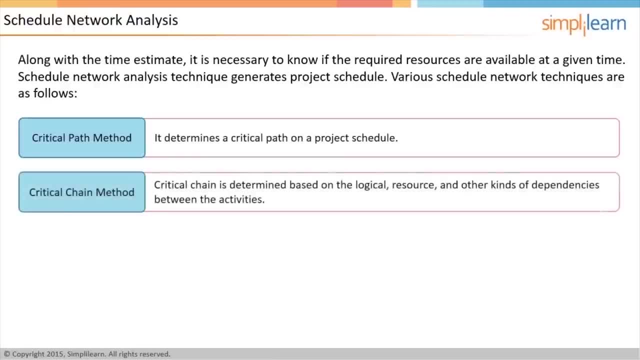 the critical path on a project schedule. Critical chain method is a variant of the critical path method wherein the critical chain is determined based on the logical resource and other kinds of dependencies between the activities. What-if scenario analysis is about trying to vary a certain parameter to observe. 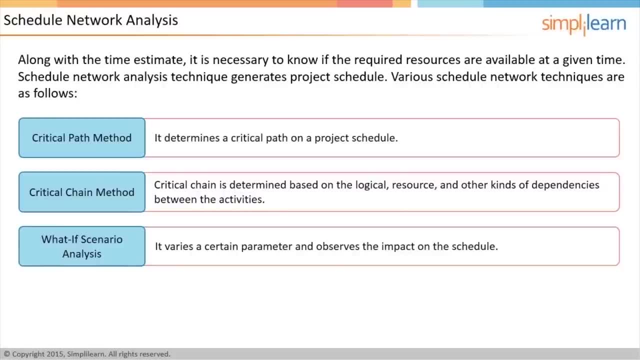 the impact on the schedule. For instance, you may want to check result if you put in more resources on a particular activity to reduce its duration. Resource optimization techniques: try to arrive at the optimal utilization of the resources used on a project. Ideally, you would want the resources. 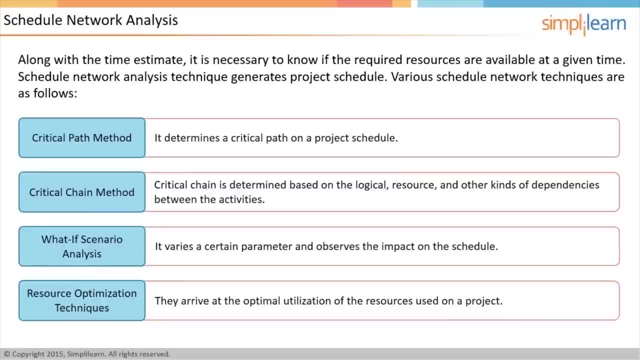 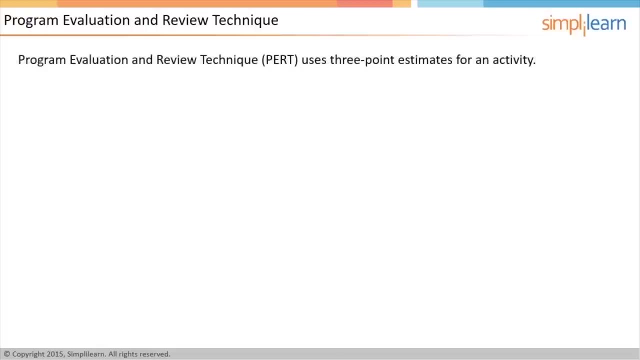 to be fully utilized, but you would also want to build in sufficient buffers in case a certain resource is not available due to various reasons. In the next screen, let us look at the program evaluation and review technique. Program evaluation and review technique is based on three-point estimates. 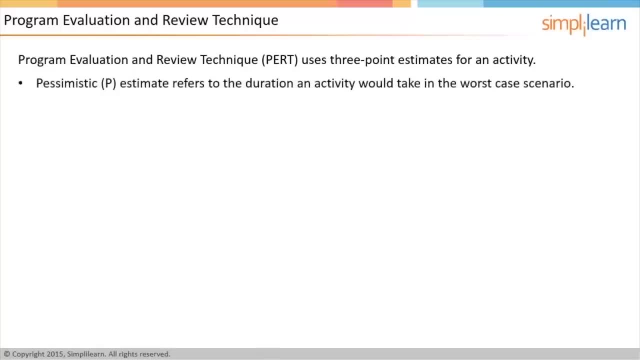 for an activity. The pessimistic estimate refers to the worst-case scenario, whereas most likely estimate is what you expect to happen in a realistic scenario. The optimistic estimate, on the other hand, represents the amount of time an activity would take in the best-case scenario. 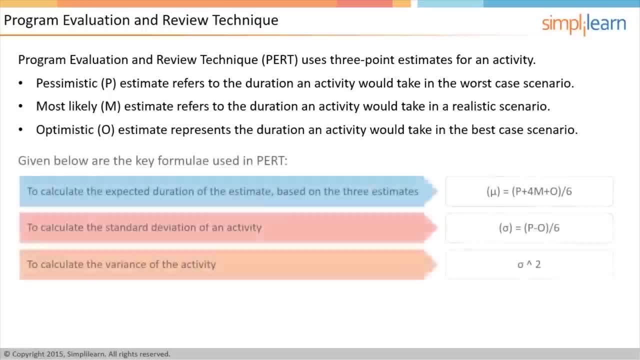 Based on these three estimates. the expected duration of the estimate is the formula given on the screen. The formula for calculating standard deviation of an activity and variance of an activity is also given. There is no question asked on variance, but the formula is important. 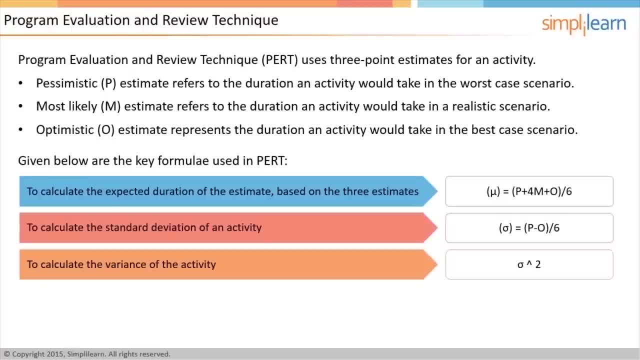 because if the standard deviation of the whole project is to be calculated, the process is to calculate the variance of the whole project and then take its square root to calculate the standard deviation of the project. Concept-based questions on PERT are included in the PMP exam. 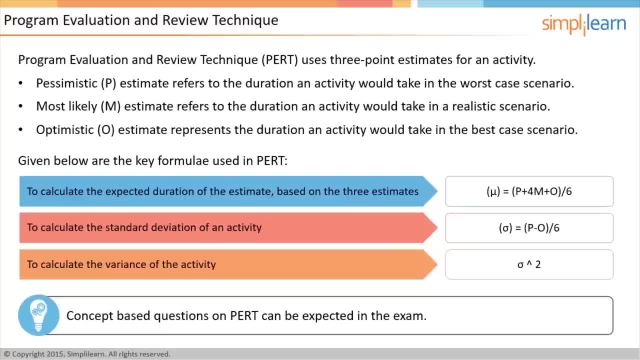 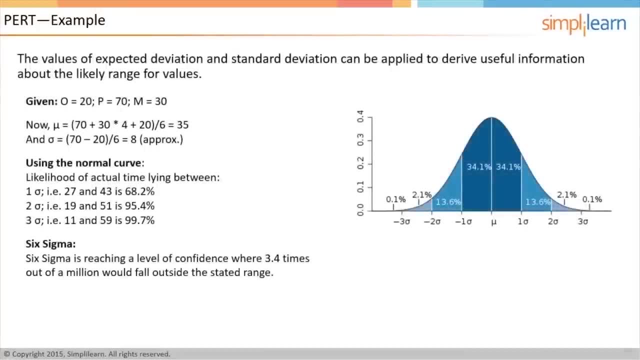 so make a note of the formulae while you prepare for the exam In the next screen. let us understand PERT with an example. Let us now figure out how we can apply the three-point estimation that PERT uses in order to draw some useful conclusions. 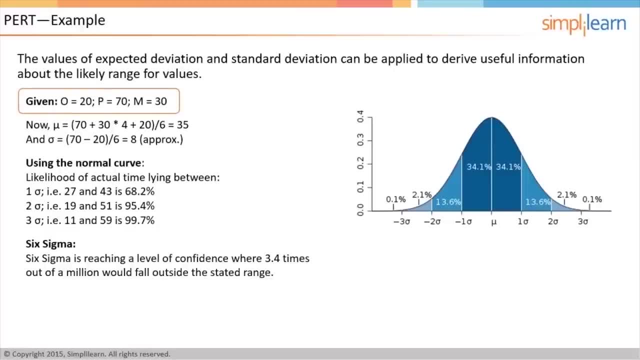 Assume that the optimistic, pessimistic and most likely estimates are 20,, 70, and 30, respectively. Using these values, you can determine the expected duration and the standard deviation as indicated Now if the causes of variation are random. 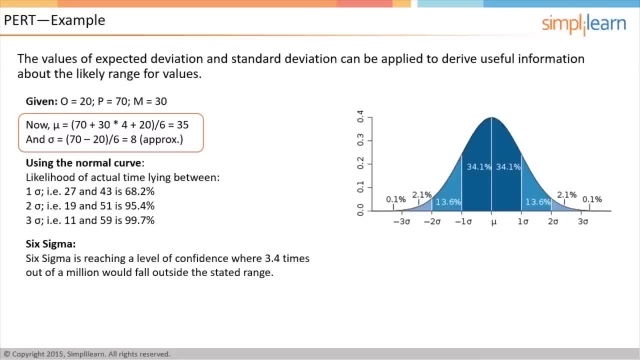 you can assume that the actual values would be evenly distributed about the mean and will follow the normal distribution, sometimes referred to as the bell curve. Further, you can use the properties of the normal distribution. There is a 68% probability of the actual value falling. 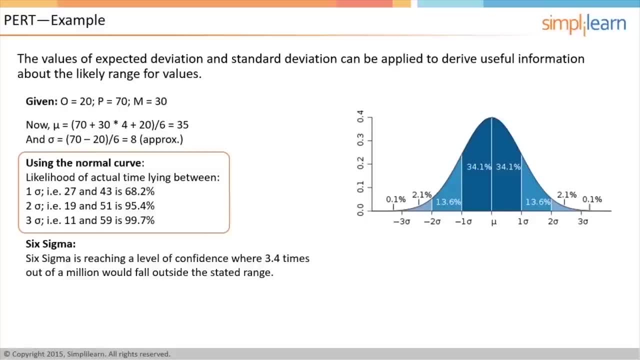 within first sigma from the mean 95.4% probability for the second sigma and 99.7% probability of the actual value falling within third sigma. Extending this logic, the notion of six sigma is reaching a level of confidence that only 3.4 times out of a million. 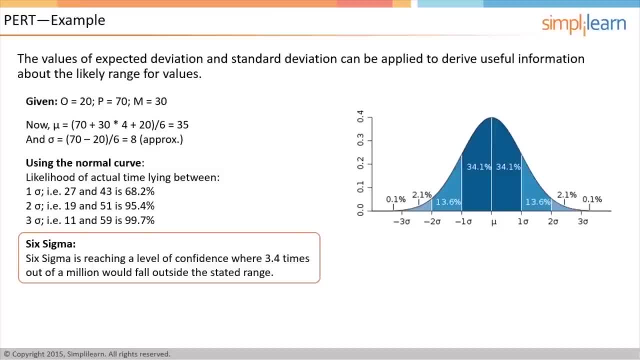 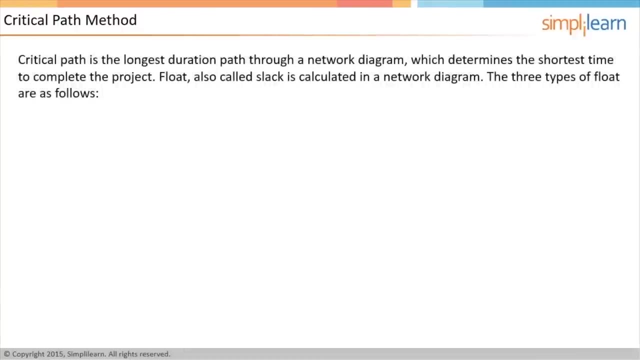 would the actual value fall outside the stated range? PERT allows you to plan based on the intended level of confidence in the outcome and determine buffers accordingly. Let us discuss the critical path method in the next screen. Critical path is defined as the longest duration path. 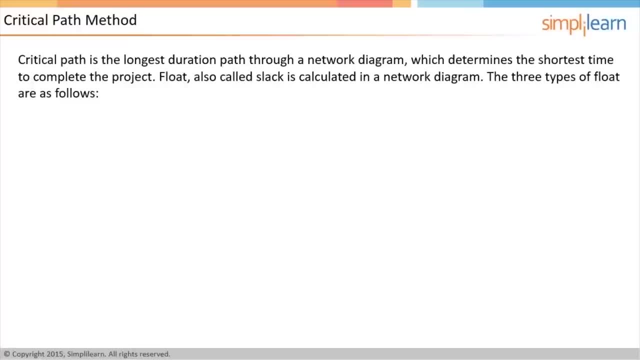 through a network diagram which determines the shortest time to complete the project. Float can be considered as a buffer time available to complete an activity. Float is calculated once the network diagram is ready. It is also called as slack. There are three kinds of float. 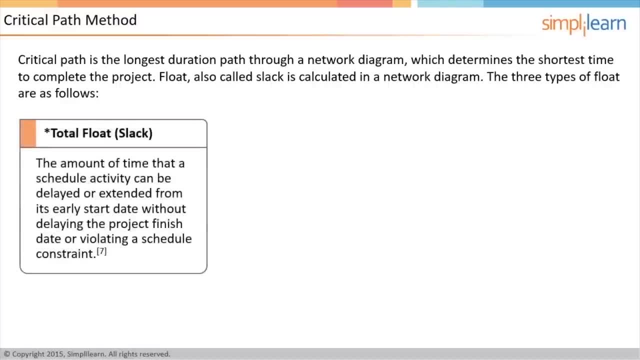 the first being the total float, which is the amount of time an activity can be delayed without delaying the project end date or an intermediary milestone. The second type of float is free float, which is the amount of time an activity can be delayed without delaying. 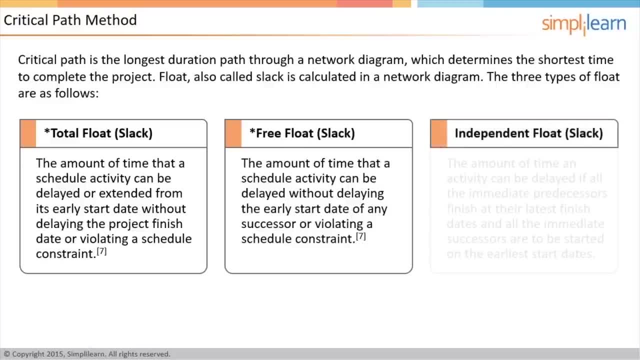 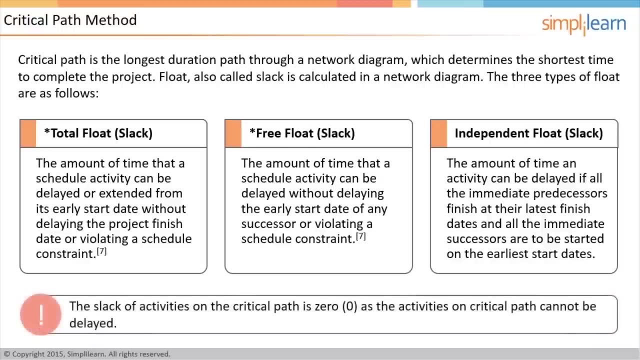 the early start date of its successor or successor's activities. The last type is independent float, which is the amount of time an activity can be delayed without delaying the project end date, and you want to start all the immediate successors at their earliest start dates. 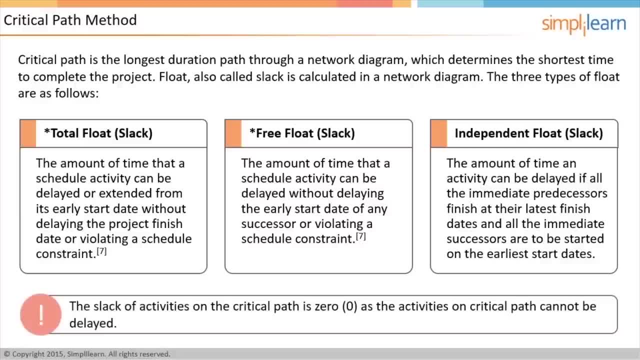 The slack of the activities on the critical path is zero, because there is no scope to delay activities on the critical path. Critical path actually represents the project duration. Delaying activities on the critical path is as good as delaying the project duration. Concept-based questions. 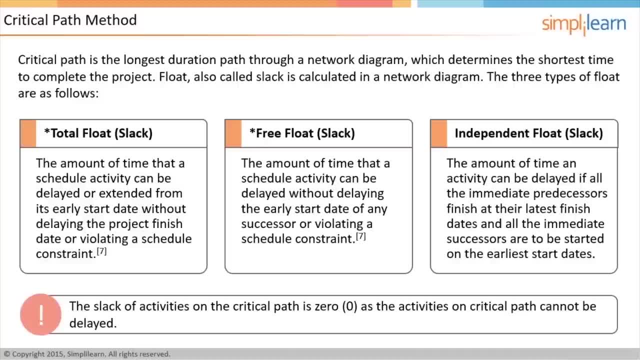 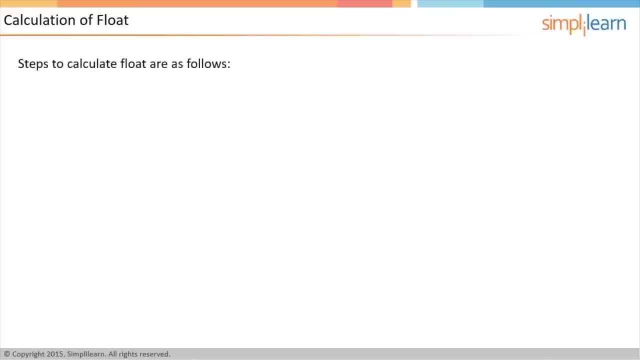 on critical path can be expected to improve your understanding of the concept. In the next screen, let us learn how to calculate float. Float of an activity can be calculated by two methods. However, the first step in critical path method is to identify the critical path. 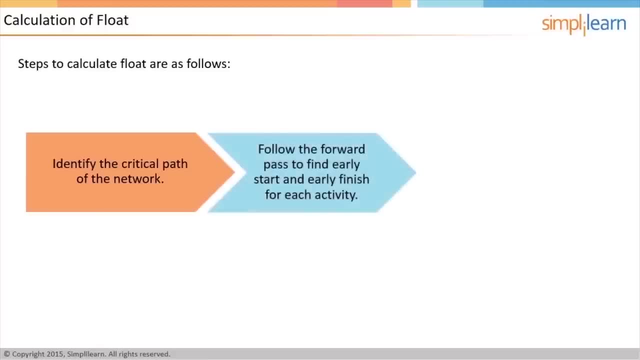 of the network. Once the critical path is identified, follow the forward path to find early start and early finish for each activity. The float of the activities represents the overall project duration. Use forward pass or backward pass to calculate the total activity time. Calculate late finish. 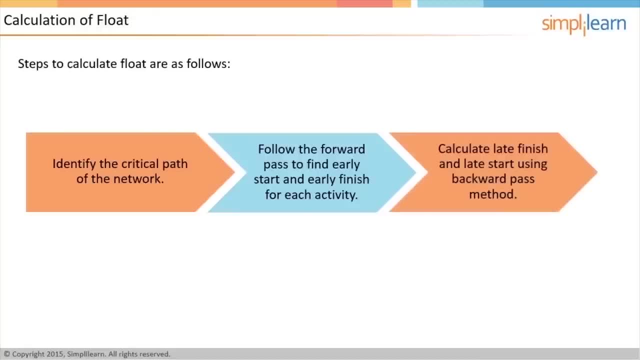 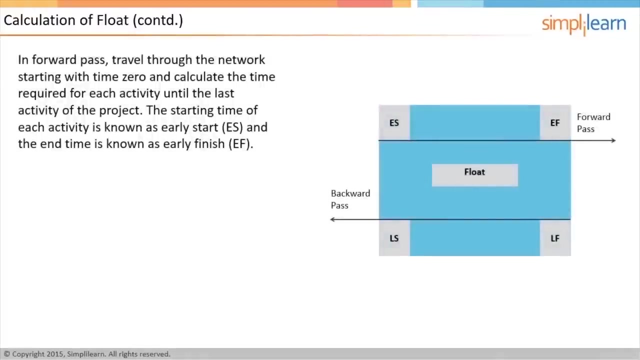 and late start using backward pass method. Note the total float formula before you start for the exam In the next screen. let us look at forward pass and backward pass methods in detail. In forward pass, you can either go through the network starting with time zero. 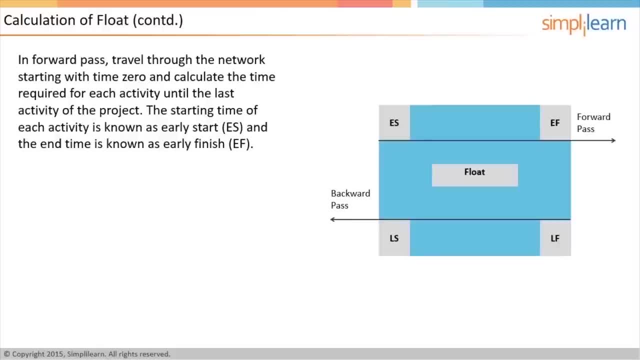 and keep calculating the time required to complete each of the activities until you reach the last activity of the project. The starting time for each of the activity in this approach is called early start and the end time for each activity is called the early finish. Alternatively, 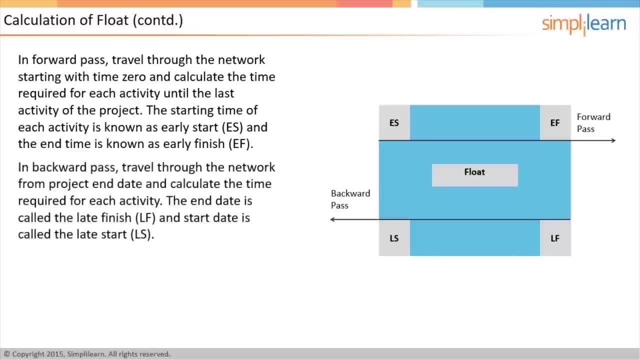 in backward pass, you can travel through the network from the project end date and calculate the time required to complete each activity. The end date in this approach is called the finish and the start date of the activity in this approach is called the late start. 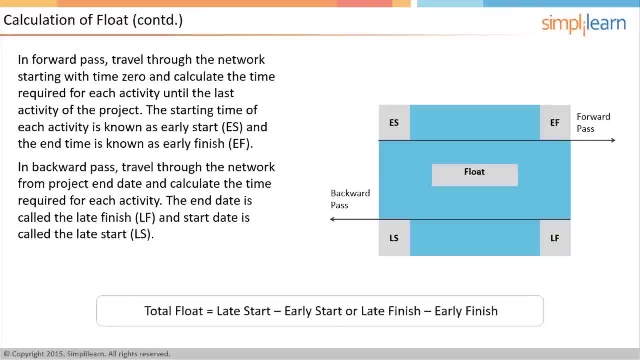 The float of the activity is either the difference between the late start and early start or the difference between the late finish and early finish. Both the differences work out to be the same. Before the start of the PMP exam, please make a note of the total float formula. 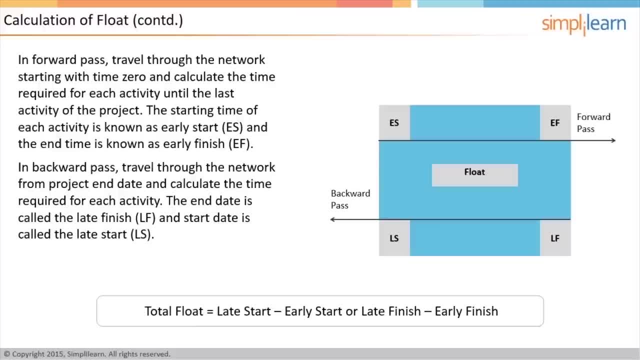 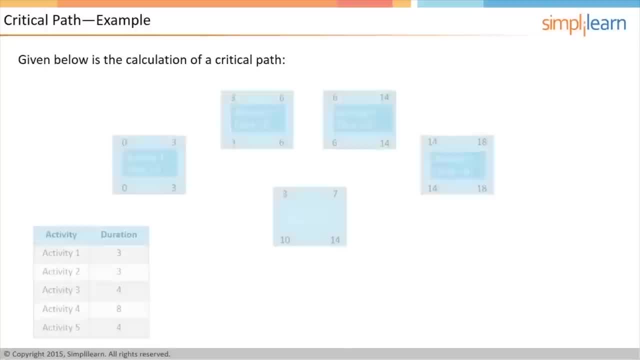 Let us understand the critical path calculation with an example in the next screen. Let us look at an example for critical path. There are five activities in this project and two paths in the network diagram. Start, 1,, 2,, 4,, 5, end is one path. 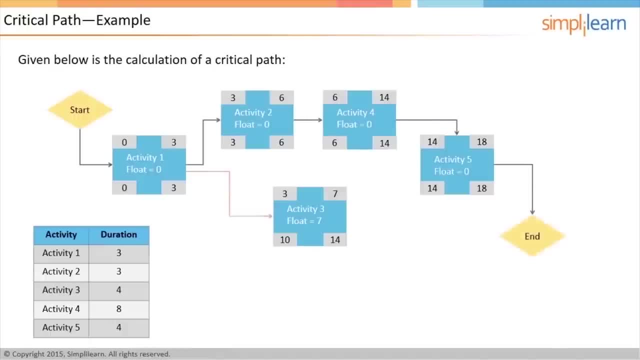 and start, 1,, 3,, 5, end- is the second path, Since the duration of the path- start, 1,, 2,, 4,, 5, end- is 18 days, which is more than the duration of the path. 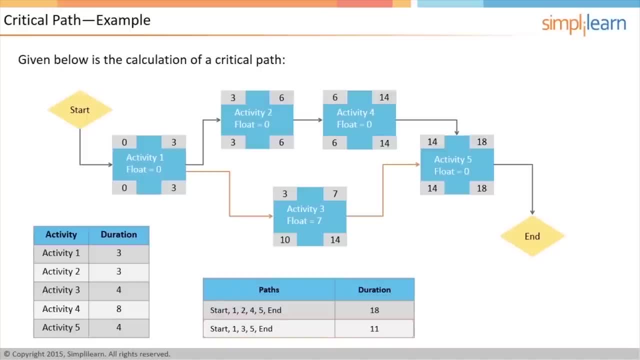 start, 1,, 3,, 5, end. the critical path of the project is start, 1,, 2,, 4,, 5, end. Let us take activity 3 as an example. First, calculate the early start and early finish dates. 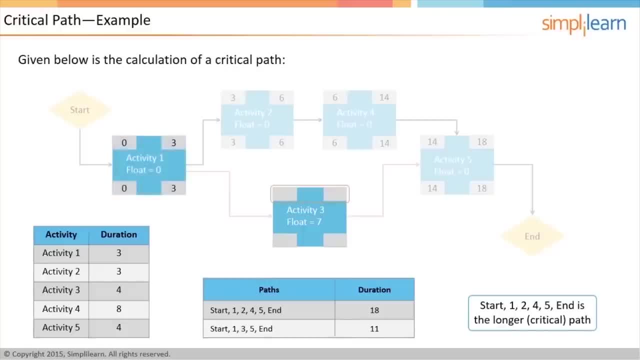 Activity 3 can start only after activity 1.. Since the early finish of activity 1 is 3, it becomes the early start of activity 3.. Activity 3 cannot start earlier than 3 because activity 1 can be completed only by then. 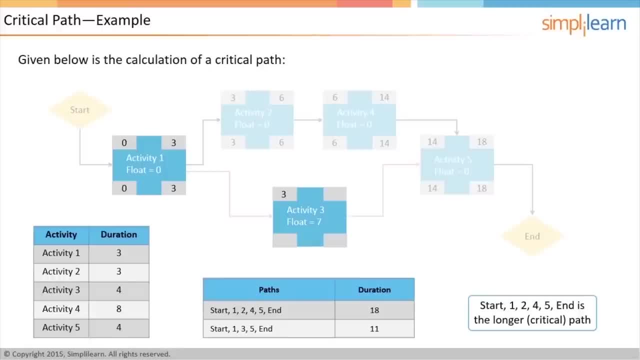 Therefore, early start of activity 3 is 3,. since the duration of the activity is 4 days, The early finish of activity 3 is 3 plus 4, equals 7 days. Now let us calculate the late start and late finish. 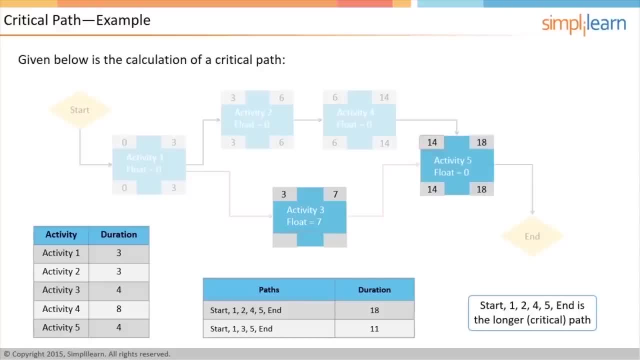 of activity 3.. Late start of activity 5 is 14 days. The activity 3 happens in activity 5, so the late finish of activity 3 is 14 days. To calculate the late start, you can subtract the duration from late finish. 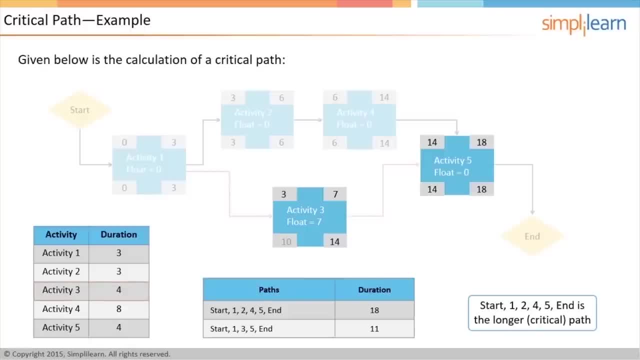 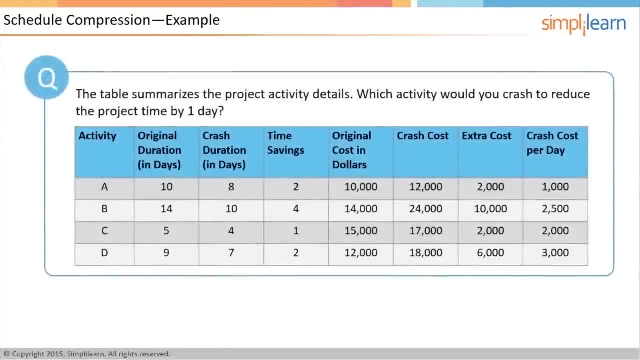 Therefore, the late start of activity 3 is 14 minus 4 equals 10.. In the next screen let us focus on schedule compression. Look at the four activities in the table. The normal cost of executing each of the activities that can be crashed. 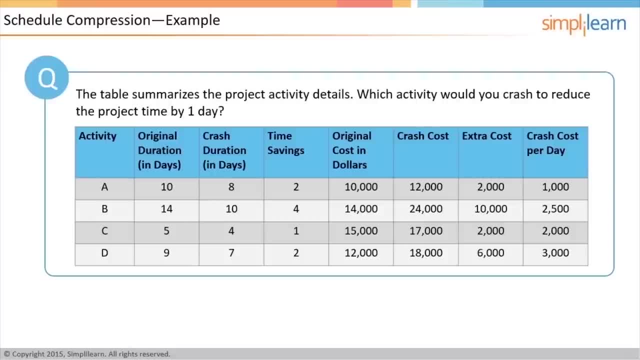 is also provided. Which activity would you crash to reduce the project time by one day? Activity A will be crashed if the duration of the project is reduced by one day. as the per unit cost of crashing the activity A is the least, All the activities are assumed. 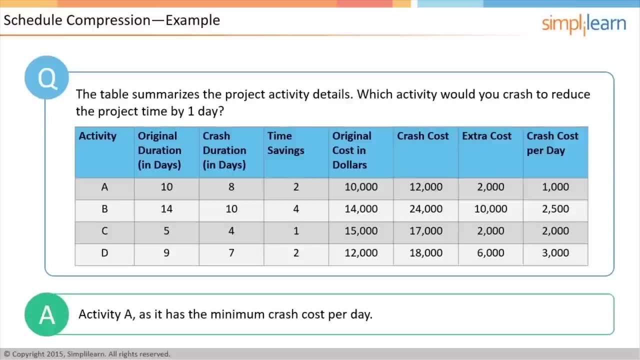 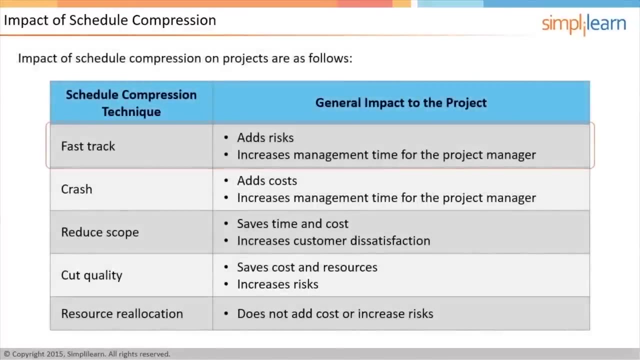 to be on the critical path here. While crashing, you will not end up saving time on the project. In the next screen, let us look into the impact of schedule compression. Different schedule compression techniques have different impact on the project. The impact of fast track. 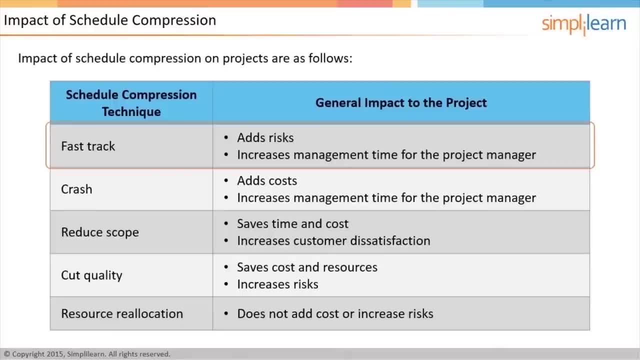 leads to risk additions and increase in management time for the project manager. Crash leads to cost addition and increase in management time for the project manager. Reduced scope, on the other hand, saves cost and resources, but increases customer dissatisfaction. Likewise, cut quality saves cost. 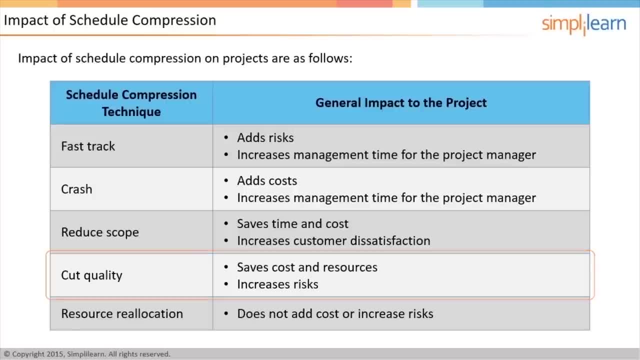 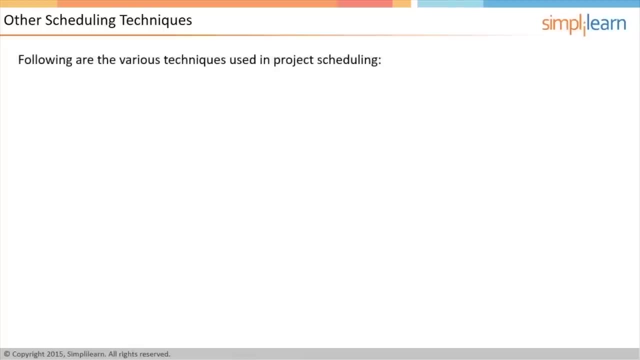 and resources, but increases risk. Resource reallocation does not add cost or increase risk. In the next screen, let us look into the other techniques used in scheduling. There are several techniques that are used in scheduling projects. What-if scenario analysis In this technique. 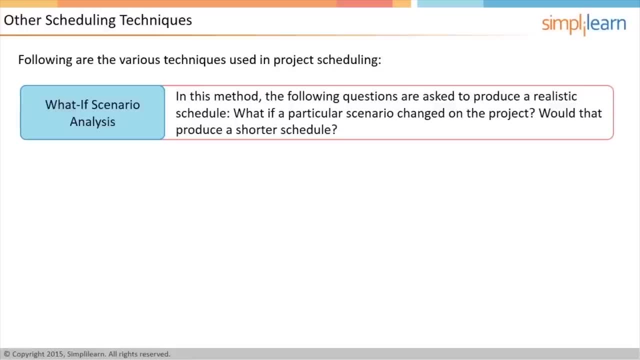 you can ask unique questions like: What if a particular scenario changed on the project? Would that produce a shorter schedule? are put forth to understand the impact of specific changes on the schedule. The goal is to produce a realistic schedule- Monte Carlo analysis In this method. 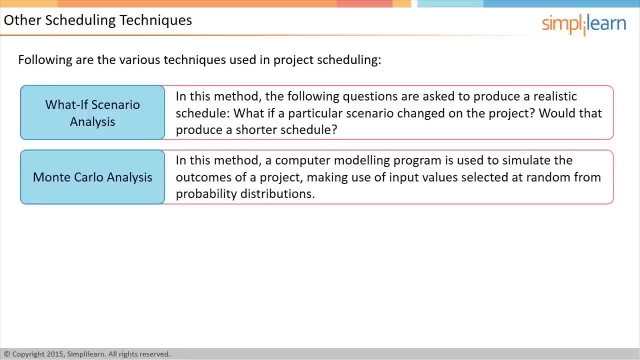 a computer simulates the outcomes of a project, making use of randomly generated values that map the probability distribution of the project. These two techniques are called modeling techniques. Resource optimization techniques. These are also used to produce a resource limited schedule. Resource optimization results. 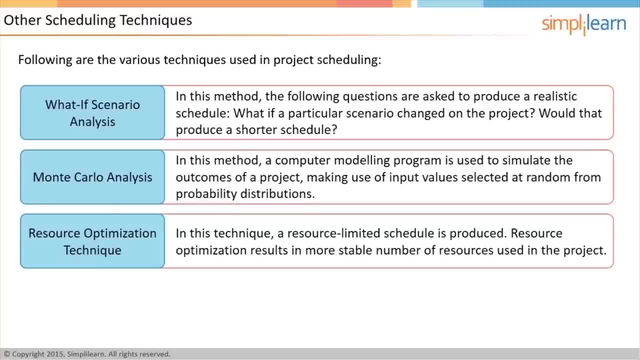 in more stable number of resources used in the project Critical chain method. This technique develops the project schedule that takes into account both the activity and resource dependencies. In the next screen we will look at the last process in project time management: Control schedule. 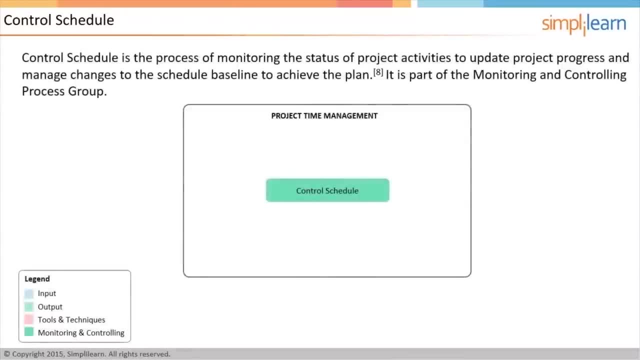 Control schedule is concerned with determining the status of the project schedule, determining that the project schedule has changed and managing the actual changes as they occur. The project schedule is an important input to this process. It is the actual schedule that needs to be controlled. 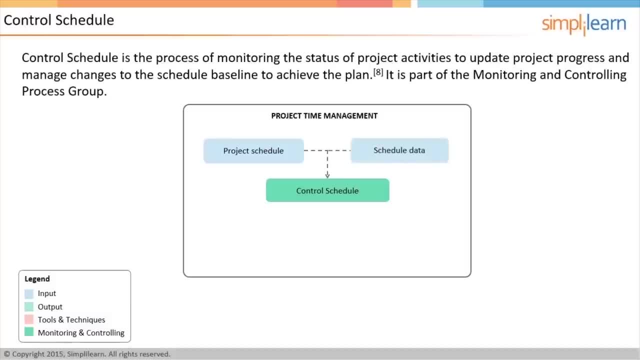 Scheduled data contains information that may need to be monitored in order to take actions to bring the project back on schedule. Project calendar describes the working hours and days for the project. Work performance data has information like which activities have started their progress and which activities have finished. 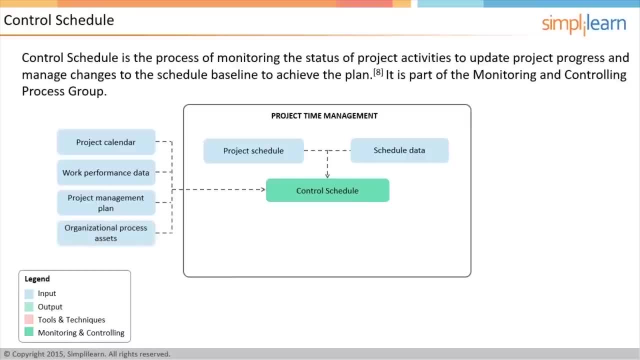 The other inputs of this process are project management plan and organizational process assets. The key tools and techniques are the performance reviews. Performance review is measuring, comparing and analyzing schedule performance, such as actual start and finish dates, percent complete and remaining duration for work in progress. 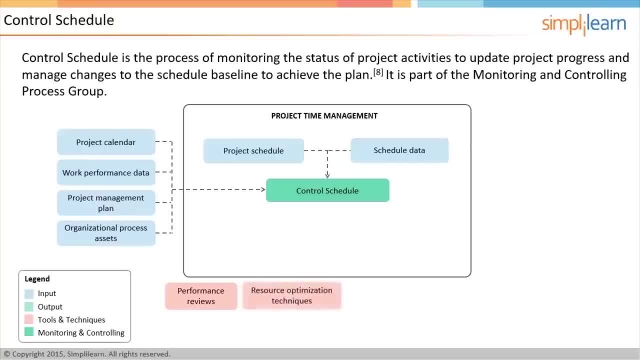 The other tools and techniques include resource optimization techniques, modeling techniques, schedule compression, leads and lags scheduling tool and project management software. In development schedule process, these techniques are used for the first time to develop the project schedule, Whereas in control schedule process. 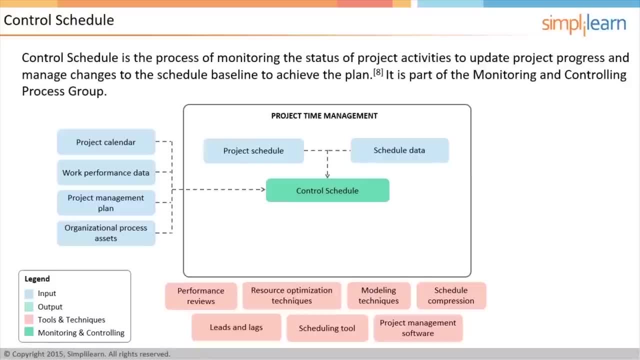 these techniques are used to update the project schedule. The key output of the control schedule process is the work performance information. This is represented in the form of schedule variance- SV- and schedule performance index- SPI, As a part of the control schedule process. 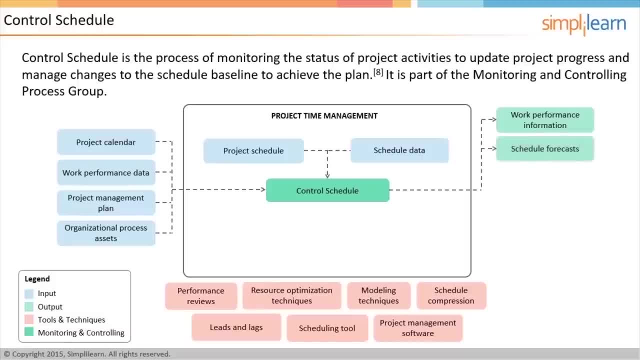 the project team will generate forecasts likely schedule for forthcoming activities and project as a whole. The other outputs include organizational process assets updates, change requests, project management plan updates and project document updates. In the next screen, let us look into a business scenario. 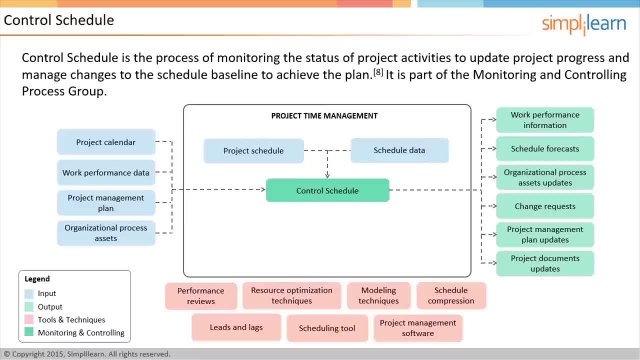 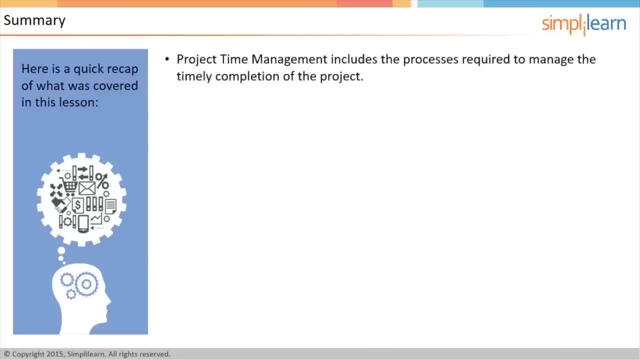 to understand the concept better. After reading the problem statement, click the solution button to look at a possible answer. Here is a quick recap of what was covered in this lesson. Project time management includes the processes required to manage the timely completion of the project. 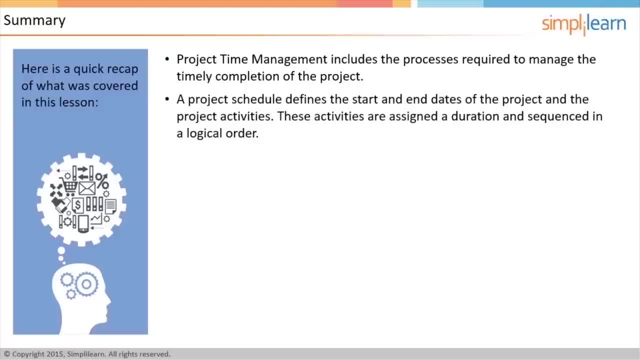 A project schedule defines the start and end dates of the project and the project activities. These activities are assigned a duration and sequenced in a logical order. Chart charts and network diagrams are used to identify project activities and determine the relationships and dependencies between them. 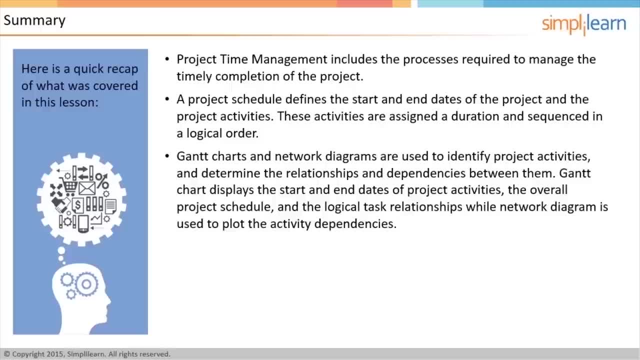 Gantt chart displays the start and end dates of project activities, the overall project schedule and the logical task relationships, while network diagram is used to plot the activity dependencies, Plan, schedule, management, define activities, sequence activities, activity resources, estimate activity durations, develop schedule and control schedule. 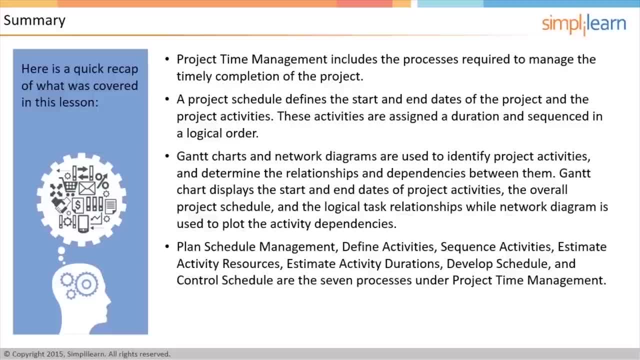 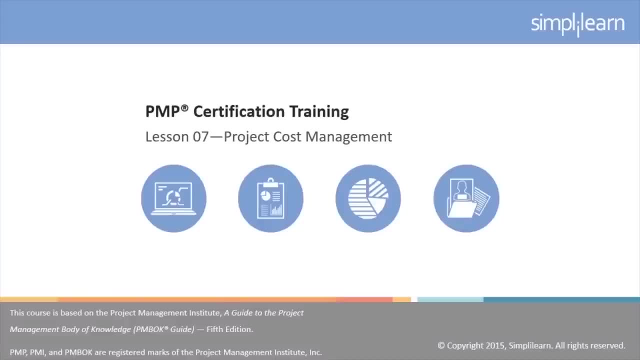 are the seven processes under project time management Schedule. network analysis technique generates project schedule based on the estimates of time and resource requirements. In this lesson, we will focus on project cost management. Let us begin with the objectives of this lesson. After completing this lesson. 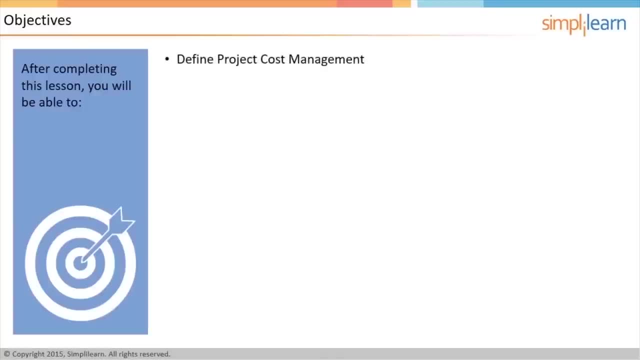 you will be able to define project cost management, differentiate between cost estimation and cost budgeting. explain control accounts. describe the project cost management processes. apply earned value management technique to track project performance. identify key terminologies used in project cost management. In the next screen. 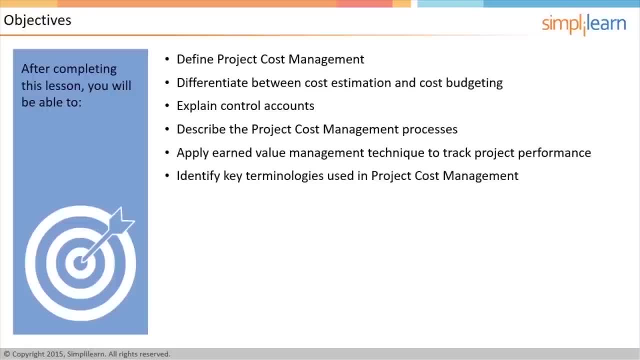 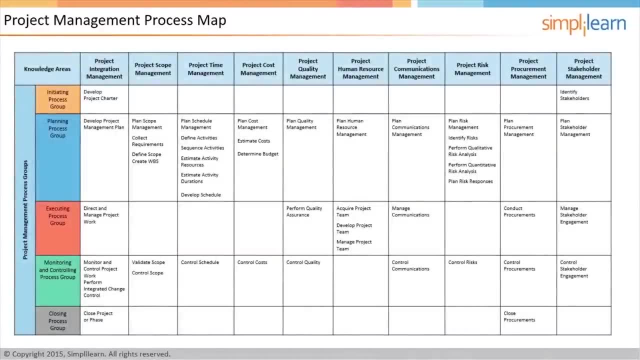 let us take a quick look at the project cost management process map. There are 47 processes in project management, grouped into 10 knowledge areas and mapped to 5 process groups. In this lesson we will look at the fourth knowledge area, that is. 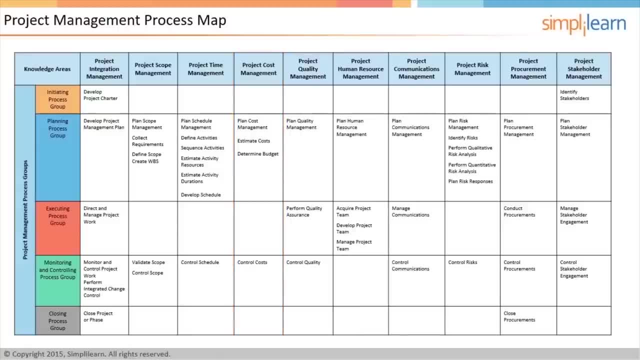 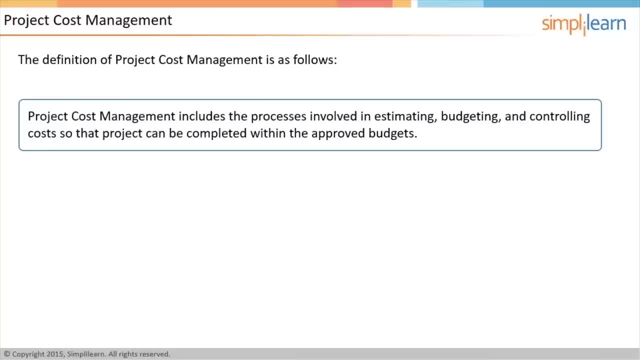 project cost management and its processes. In the next screen, let us understand the concept of project cost management. In the next screen, let us discuss cost management plan. The cost management plan is a vital step in project cost management. It contains information like planning the project cost. 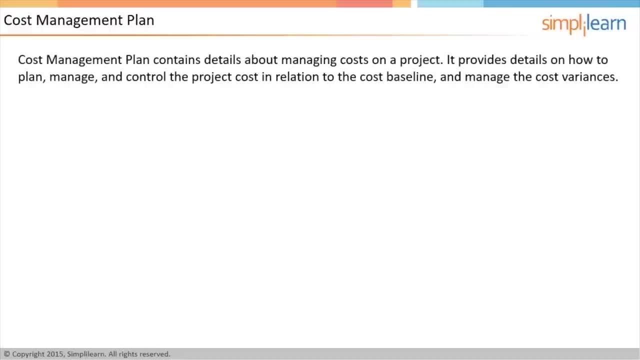 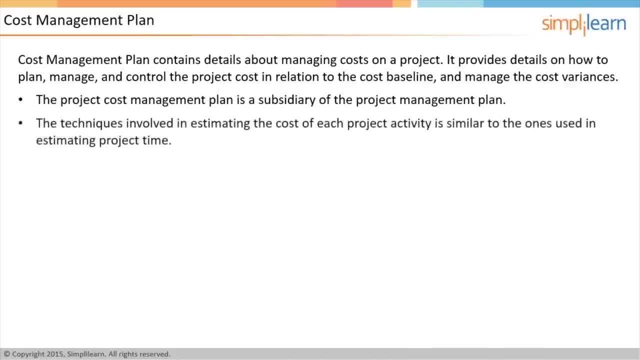 is a part of the project management plan. The methods used in estimating the cost of each of the project activities are similar to the ones used in estimating project time, For example, time estimation methods like expert judgment, analogous estimating, bottom-up estimating and two of the techniques. 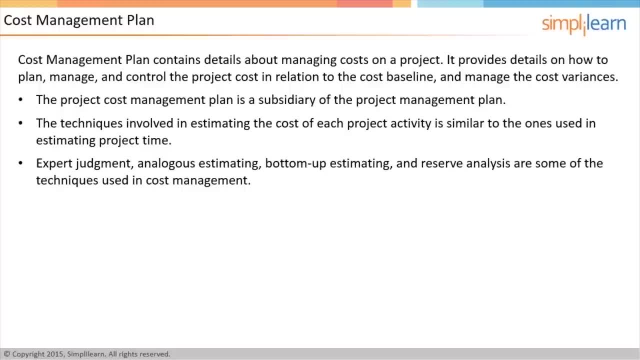 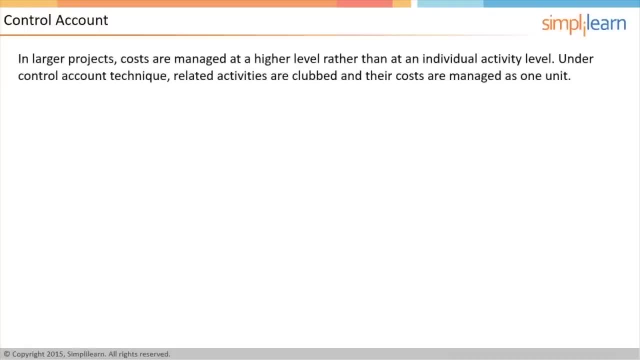 that are also used in estimating activity cost. Let us discuss control account in the next screen. Control account is an important concept in the project cost management. Project cost is generally estimated at individual activity level. It becomes difficult to manage cost at the activity level. 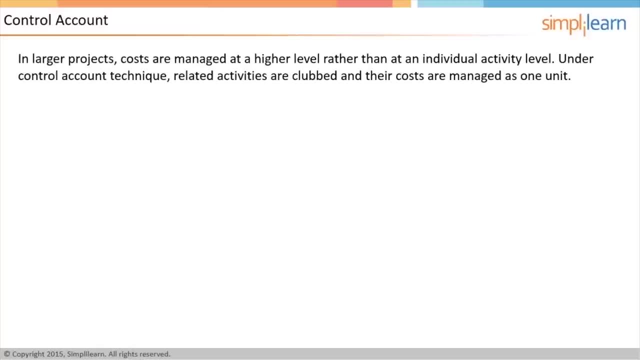 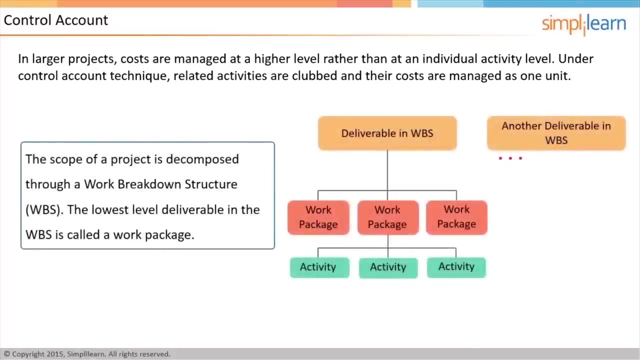 in large projects. Therefore, the cost is managed at a higher level. This requires related activities and their cost being managed together as one unit. This unit is called control account. While estimating the project time, WBS is created to break down the project into smaller deliverables. 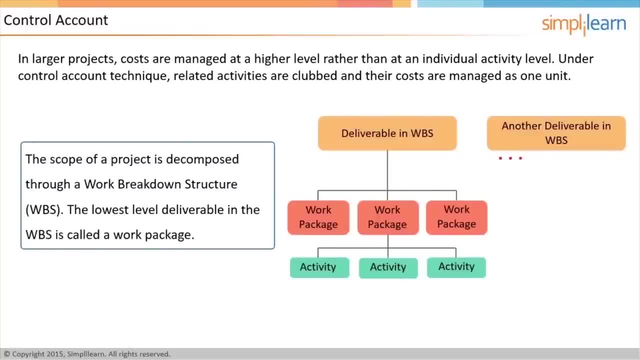 These deliverables are broken down into work packages, and these work packages are in turn broken into activities. Control account is defined at a level higher than the work packages. For example, for the one control account, the cost of all activities belonging to these five work packages. 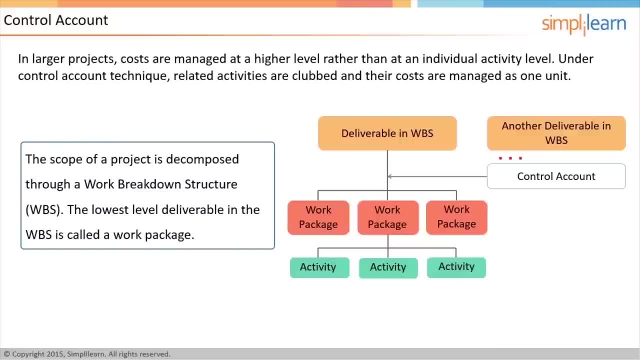 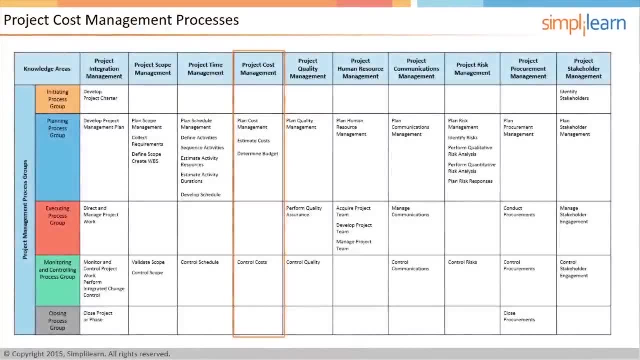 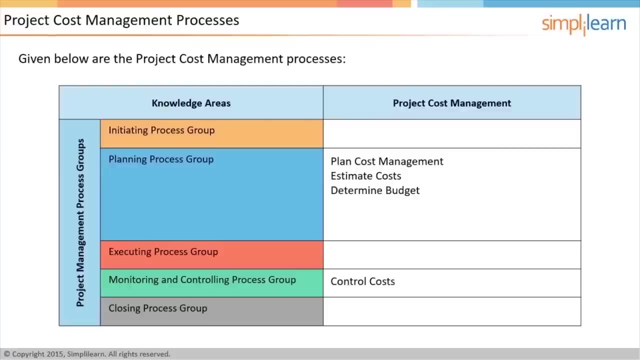 are managed as one unit. In the next screen, let us discuss the project cost management processes. Project cost management has four processes. They are: plan cost management, estimate costs, determined budget and control costs. The three processes: plan cost management, budget. 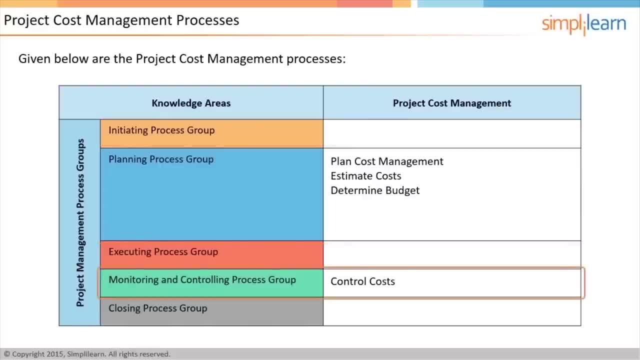 are a part of planning process group, and control cost process is a part of monitoring and controlling process group. Let us look at each of these processes in detail. Let us begin with the first process, that is, plan cost management in the next screen. 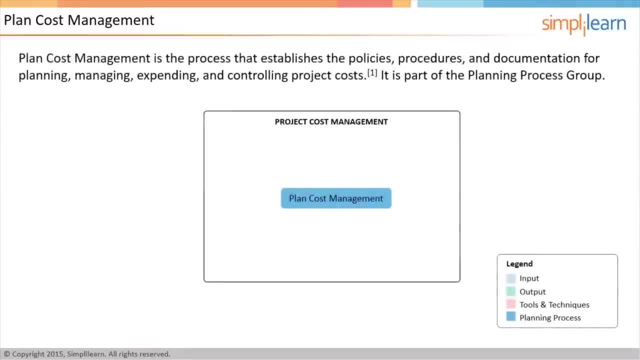 Managing costs on a project is a critical exercise. If the activities are planned well, it becomes easier to achieve harmony between the project cost and budget of the project Plan. cost management is the process of establishing the policies, procedures and documentation for planning. 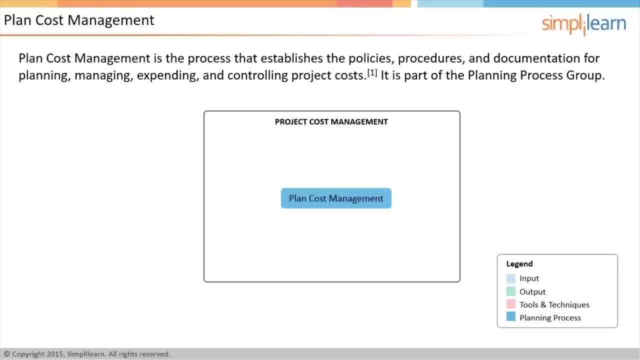 managing expending and controlling the project costs. Let us look at the inputs required for this process. The project management plan provides other subsidiary plans and guides the cost planning activities on the project. The project charter provides a detailed description which help determine the approach. 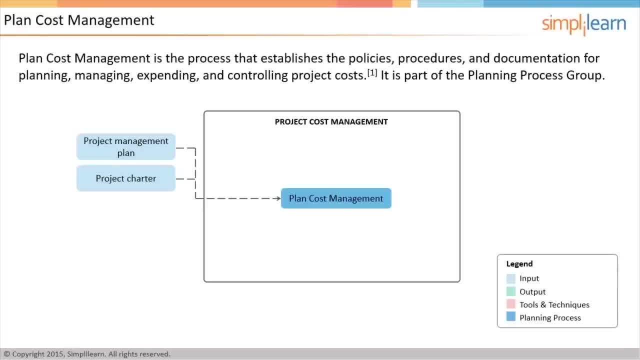 for cost management, For example, for some projects budget could be a constraint, whereas for others budget would not be a constraint but subject to the other objectives. Enterprise environmental factors provide the organizational context to the project, including the culture of the organization. 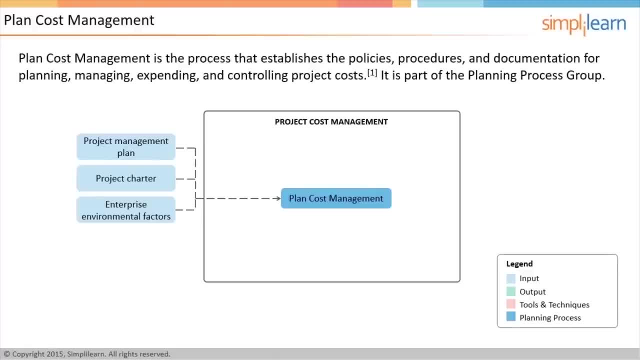 and the infrastructure, for instance, the scheduling systems available, the key personnel and so on. Organizational process assets provide inputs such as policies and procedures, templates, past performance data and estimates, historical information and knowledge base. Now let us look at the tools. 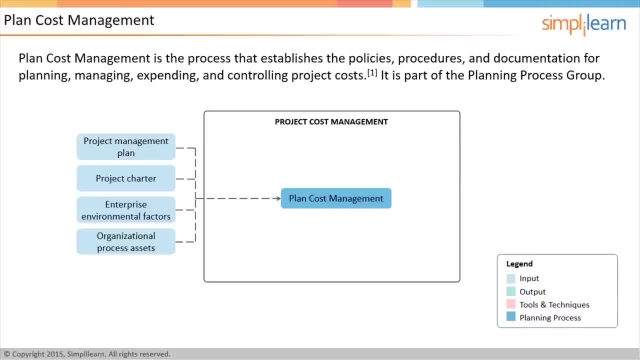 and techniques employed in this process. Expert judgment refers to input received from knowledgeable and experienced resources. Experts can devise an approach to govern the costs on a project by using their previous experiences. Meetings may be organized to determine the cost management plan. Everyone responsible for the project schedule management. 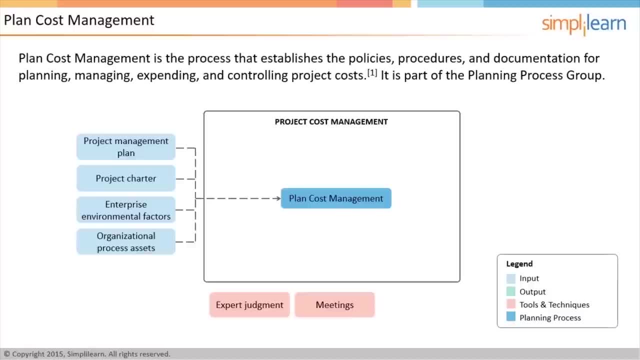 such as the project manager, representatives from the appropriate accounting or financial organization, sponsor, customer and other stakeholders must attend these meetings. Several analytical techniques may be used to determine the cost management plan. These techniques help to map the impact of various decisions on the project. 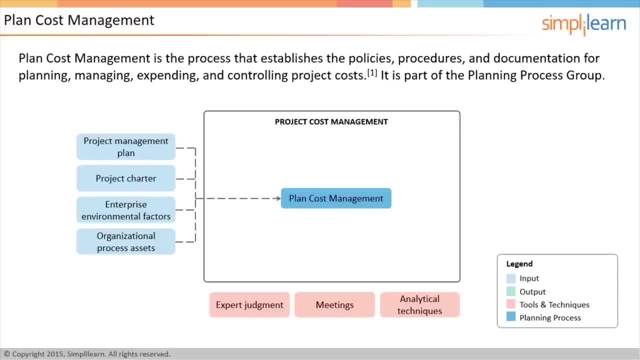 For example, how do risk management processes impact cost, etc. Cost management plan is the primary output of this process. It establishes the units of measure, levels of precision, organizational process, links, control accounts to be used, rules for performance measurement and reporting. 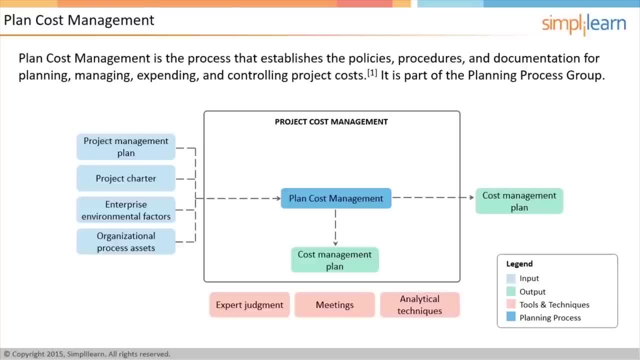 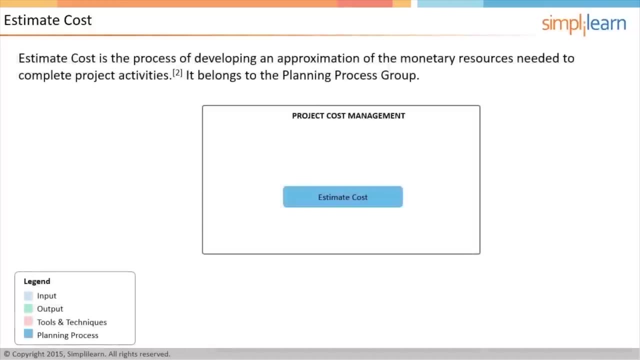 frequency and methodology of monitoring the costs and various other details that lay on a project. In the next screen let us discuss the second process under project cost management: Estimate cost. Estimate cost is the approximation of the monetary resources required to complete a project activity. 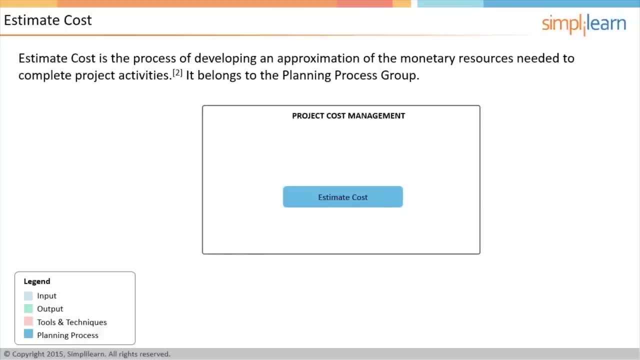 Cost of a specific activity is estimated based on the information available at that point of time. As the project team gets more information about the project, the activity cost estimation is determined. Let us look at the inputs of this process. Scope baseline is the most important. 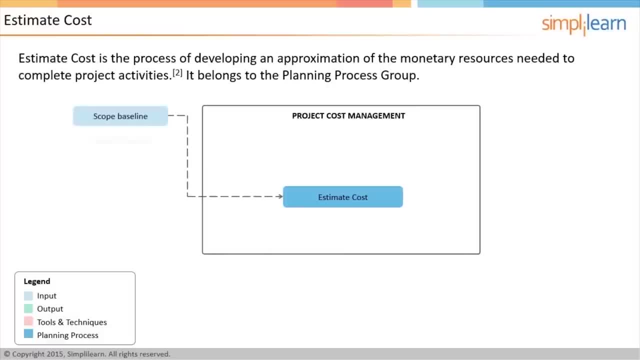 input, as it details out the project scope of work, Along with that project schedule, is also important. This contains information like when and which resource is required for the project. It is good to remember that the same kind of resources may have different costs at different points of time. 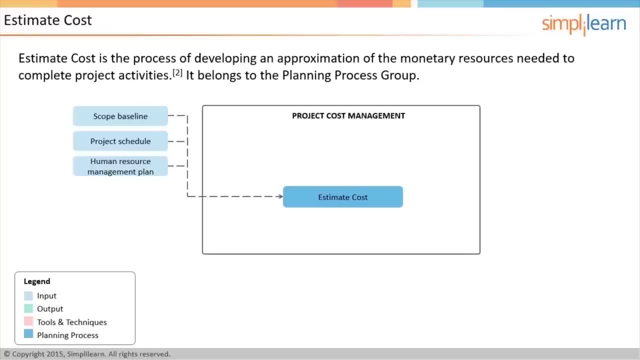 Cost plan is another important input. Various elements like personnel rates, rewards or recognition programs, etc. are covered in the human resource management plan, which is important in approximating the cost estimate. Human resource management plan will be discussed in detail in the human resource management. 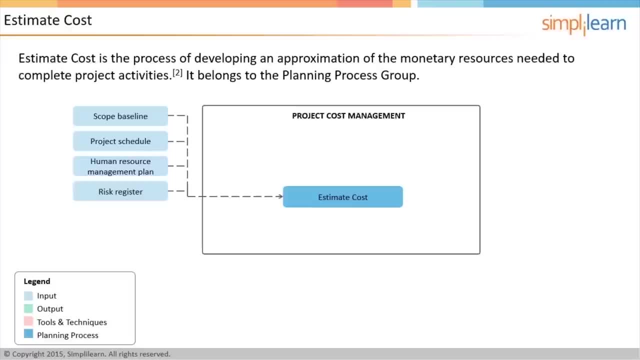 knowledge area. Risk register is also an input because risk mitigation costs should be considered in cost planning. More information on risk and its effect in the project will be looked at in detail in risk management knowledge area. Another input, enterprise environmental factors- provides organizational context. 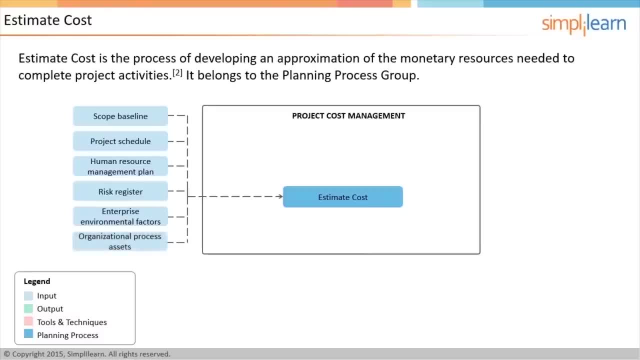 to the project. Organization process. asset is listed as an input, as organizations might have standard set of cost estimation policies or templates. Cost management plan is another important input. The cost management plan lays the framework for the cost management processes in the project. It provides guidelines such as: 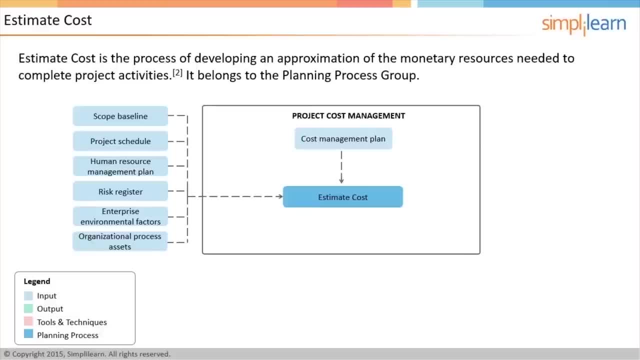 the units of measure, accuracy, desired, methodologies and tools to be used, etc. Let us now look at the tools and techniques used in this process: Expert judgment, reserve analysis, analogous estimating, cost of quality, parametric estimating, three-point estimating. 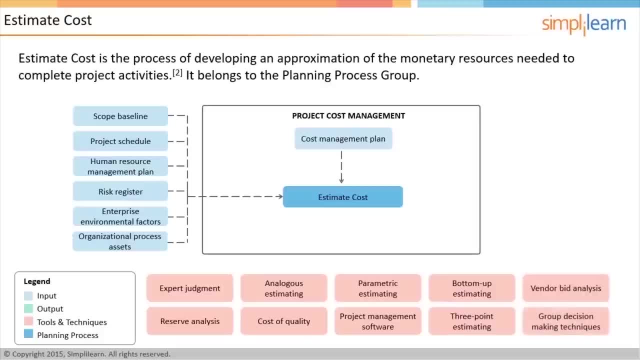 vendor bid analysis and group decision making are the various tools and techniques used in this process. Most of the tools and techniques used here are similar to the ones used in the time management knowledge area. Vendor bid analysis is a technique used to estimate project cost. 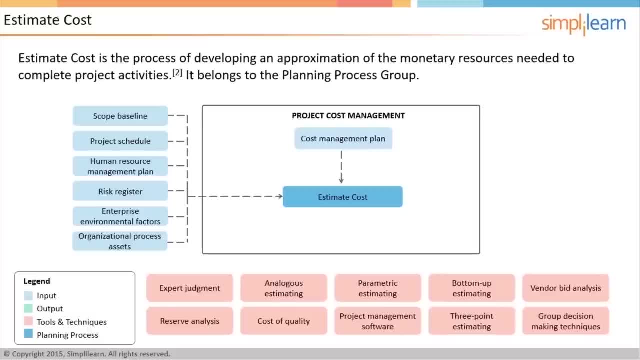 For example, a project requires material procured externally through suppliers. In order to get that, you need to collect bids from three or four suppliers and assess their quotations. Based on their quotations, you can get an idea of the cost that will be involved in getting 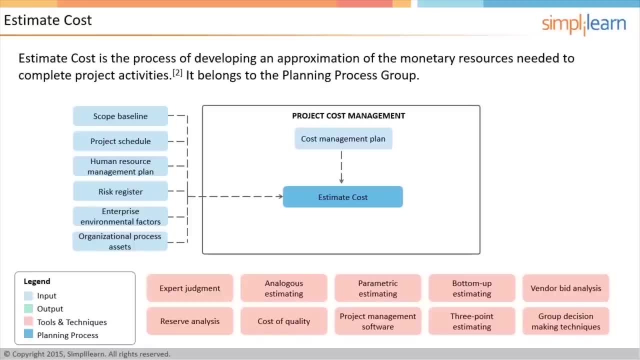 the material for the project. Group decision making technique is another important technique for project cost estimation. Cost estimation is an exercise which may be carried out by a group or committee in order to gather well-rounded input. Therefore, group decision making techniques can be used. 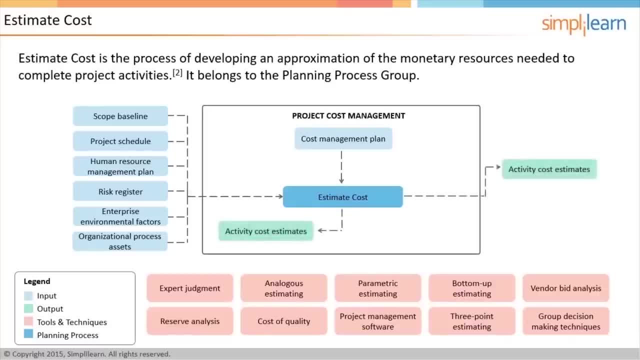 The outputs of this process are quite straightforward. Estimates of each of the activities are arrived at Basis of the estimate. includes things like how the estimate was developed, what were the assumptions made in estimating, etc. Project document updates is also one of the outputs. 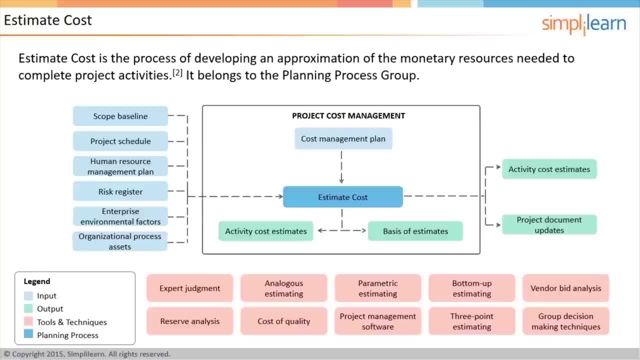 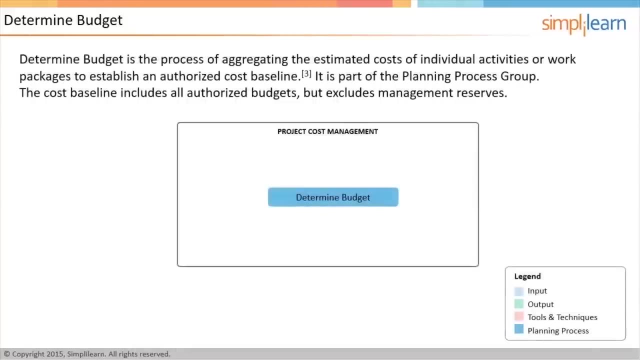 because the cost estimates may result in updates to other aspects of the project, For example, quality, risk, etc. In the next screen let us discuss the third process under project cost management: determine budget Once the estimate of each of the activities. 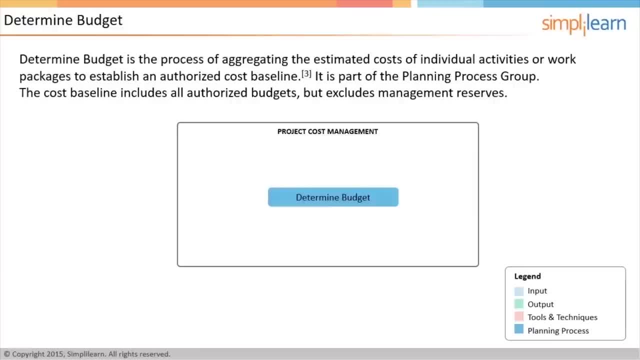 is arrived at. the next project cost management process is to determine budget. It is the process of aggregating the estimated costs of individual activities or work packages to establish an authorized cost baseline. This is where the control account concept comes into picture: The costs of the activities. 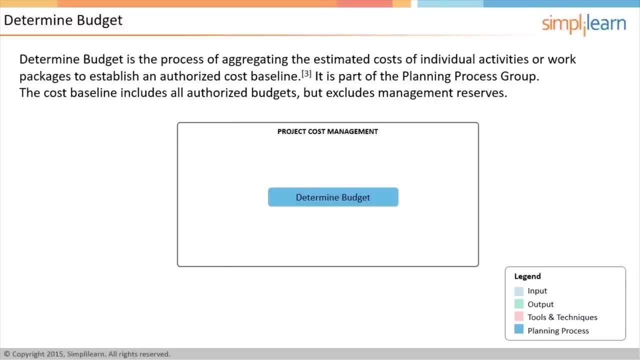 are aggregated to arrive at the cost budget at the control account level. Once approved, this cost budget becomes the cost baseline of the project. Project cost performance is measured against the cost baseline. that is, how much more would the project cost be compared to the original cost baseline? 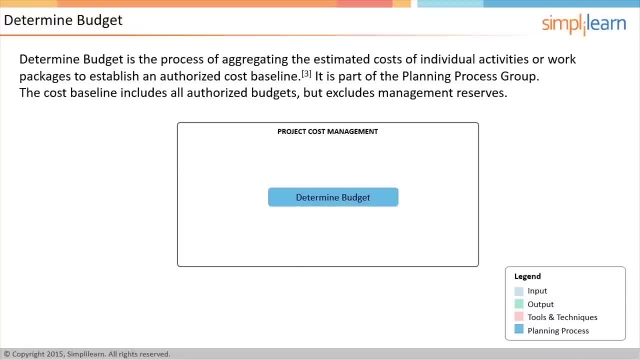 The cost baseline includes all authorized budgets but excludes management reserves. The cost management budgets are the activity cost estimates and the basis of estimates which are the output of the previous cost management process. The cost management plan lays the framework for the cost management processes in the project. 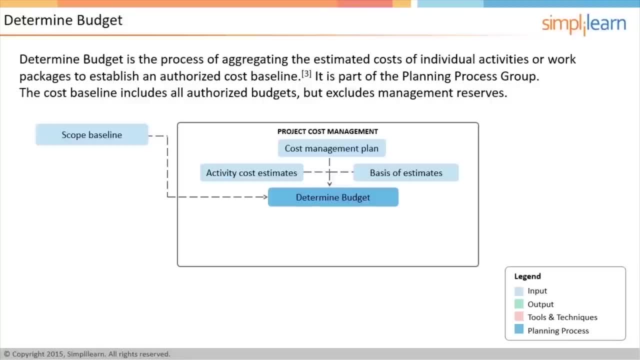 It provides guidelines such as the budgeting cycle, tools and techniques used to prepare and approve the budget, etc. In addition to these two guidelines, the project schedule provides aggregate costs in a particular calendar period to ensure how much money can be made available during that time. 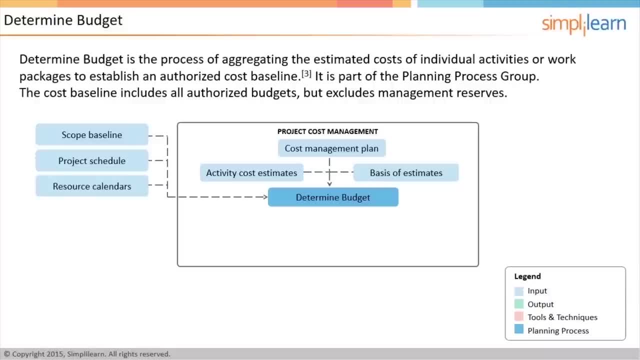 Similarly, resource calendar provides information on the resource which is assigned to the project at a particular point of time. This information is then used to indicate resource costs over the duration of the project, Therefore, the level of contingency reserves that need to be built into the budget. 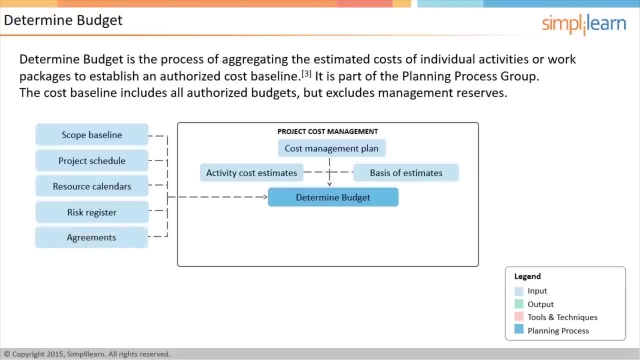 Agreements entered into with the suppliers are also required to finalize the budget. Again, organizational process asset is an input because organization may have few policies for reporting the cost budget or there might be some cost budgeting tools being used. There are various tools that can be used. 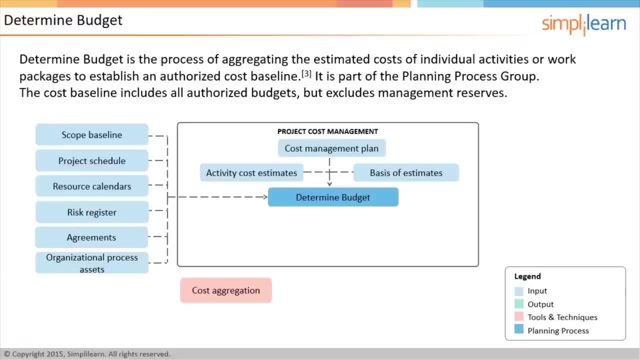 The cost aggregation technique involves adding up the cost and aggregating them at the control account level so that the cost can be managed in a better way. In reserve analysis, once the costs are estimated, some extra amount is added to the estimate as a management. 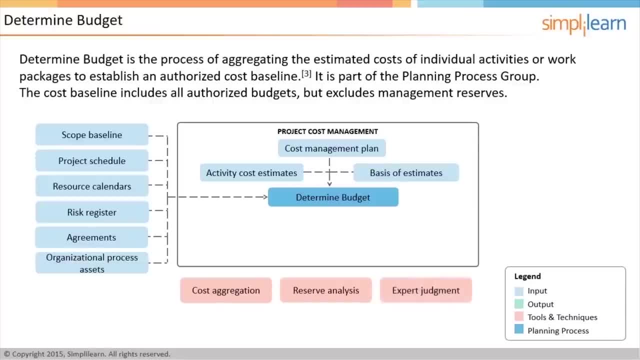 reserve to take care of any unplanned activities. Expert judgment is a technique in which an expert's help is spent on a similar project in the past and has a good idea to estimate the activity cost involved. Historical relationships are used to predict the total project costs. 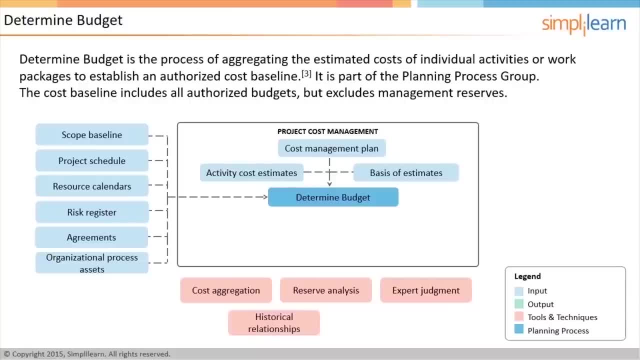 using mathematical model. This is similar to analogous estimate or parametric estimate method. Funding limit reconciliation technique is used to ensure that cost on the project is budgeted or spent as per the availability of the fund. If the project can get the funding of only $50,000 a month, 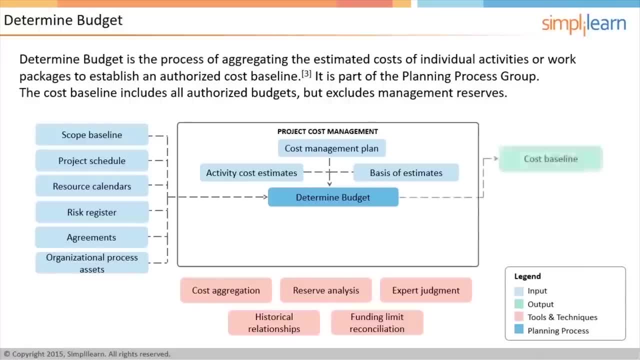 the project budget should be planned accordingly. The output of this process is the cost baseline. This is an authorized project budget over a period. This is used to measure, monitor and control overall cost performance of the project. In addition to this, the project funding requirements. 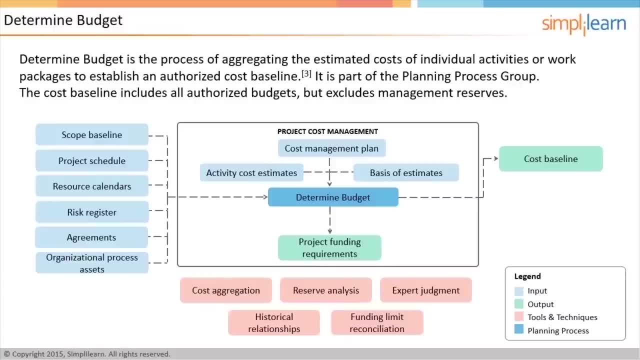 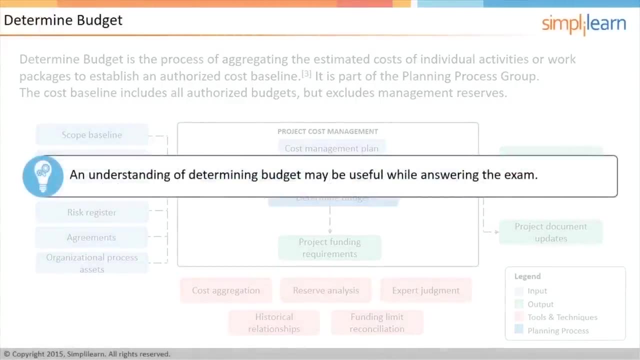 are also arrived at. Funding requirements means how much the project budget should be spent annually or yearly for the execution. The last output of this process is project document updates. An understanding of determining budget may be useful when answering questions in the PMP exam. 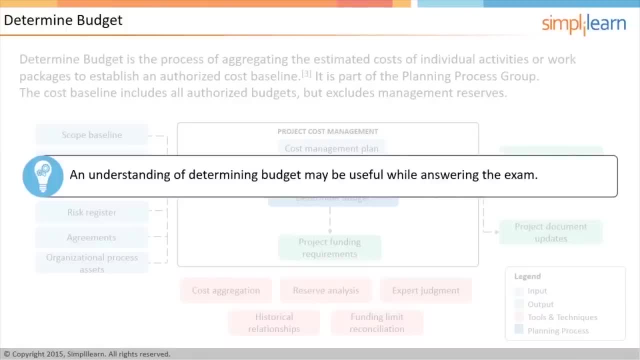 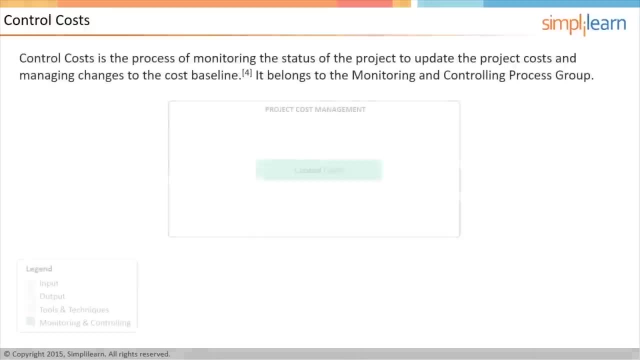 so make a note of the inputs, tools and techniques and outputs of determining budget. In the next screen, let us discuss the last process of project cost management, that is, control cost. In the next screen, let us discuss the status of the project to update. 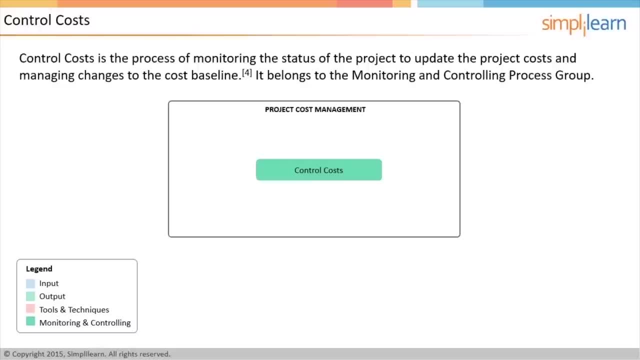 the project budget and managing changes to the cost baseline. Updating the budget involves recording actual costs spent until date. Any increase to the authorized budget can only be approved through the perform integrated change control process. Some of the typical activities that happen as part of the 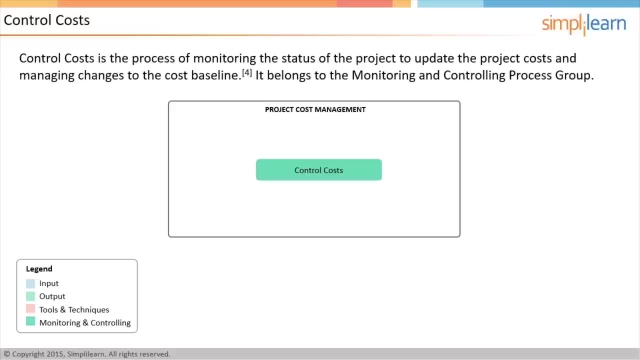 control cost process are ensuring that the project budget is spent annually, monitoring the cost performance to understand variance and monitoring the work performance against the funds expended. The inputs to the process are project management plan, organizational process assets, project funding requirements and work performance data. 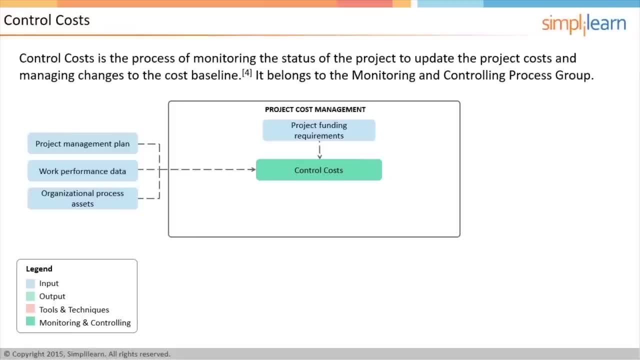 Work performance data contains the information about the project progress. The important tools and techniques are project management forecasting to complete performance index. Other important aspects of controlling costs are the review, the performance, analyze the reserves to make sure the project has enough budgetary. 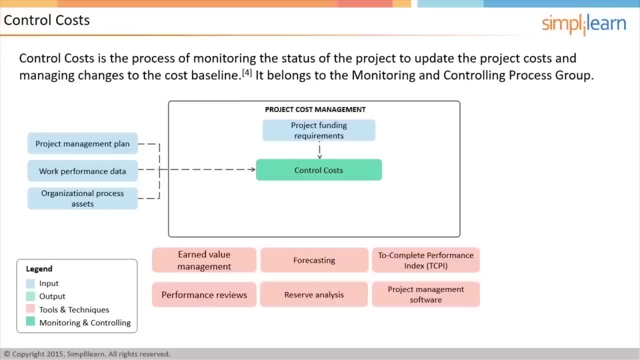 reserves to meet the expenses, and project management software, which helps in tracking and managing costs. Now let us look at the output of this process. The key outputs of this process are cost evaluation in terms of cost variance, schedule variance and earned value. 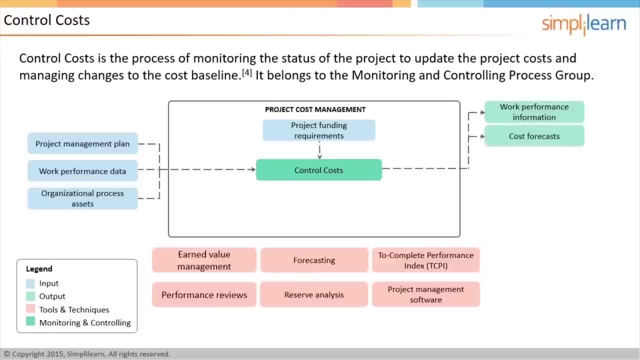 and forecasts about the cost performance. This process may also result in change requests arising out of cost control measures, as well as updates to project documents, the project management plan and organizational process assets. Business scenario-based questions on project cost control can be highlighted in the exam. so if 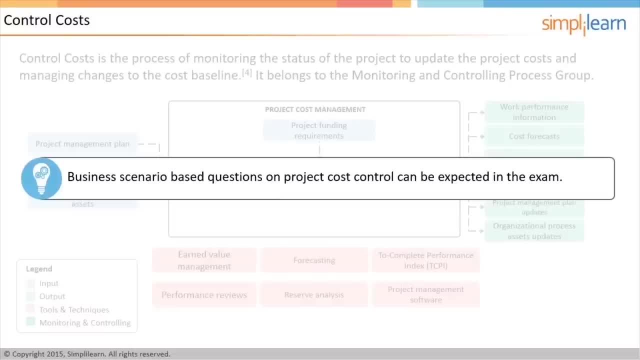 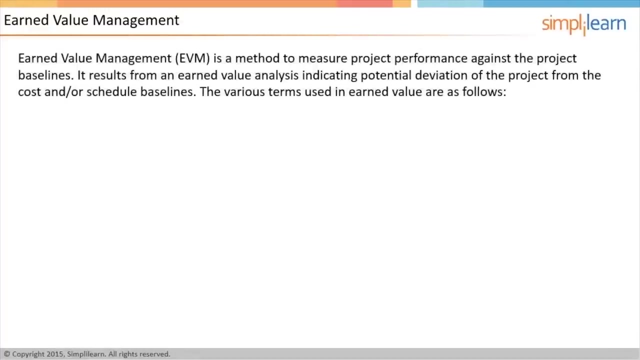 you have questions on these concepts, get them cleared, as that will help you score higher In the next screen. let us learn about earned value management and its related terms. Earned value technique is an excellent way to track the project progress against the project plan. It is a method of 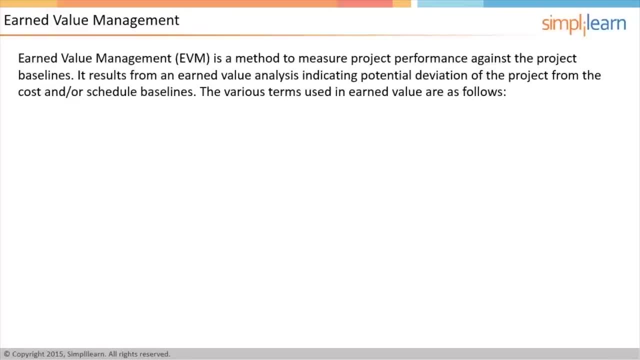 measuring the project performance objectively and comparing it against the project baseline. Results from an earned value technique include the evaluation of the project from cost and schedule baselines. Baseline is the initial approved value along with approved changes. Therefore, schedule baseline is the first approved project schedule. 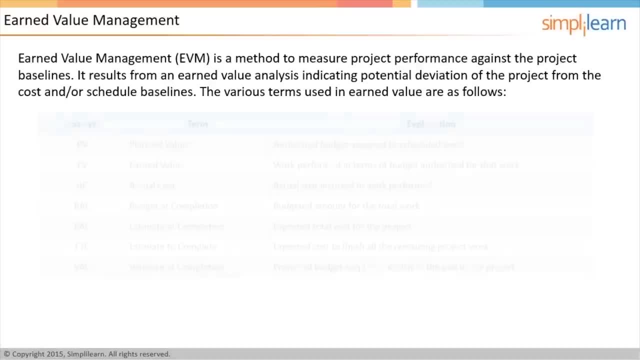 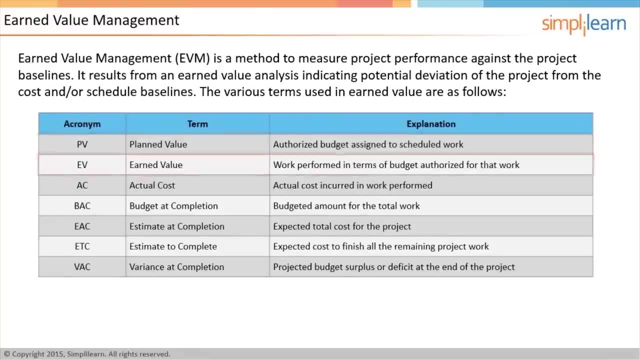 along with approved changes. There are various terms used in earned value technique. Planned value is the authorized budget assigned to the scheduled work. Earned value is the work performed in terms of budget authorized for that work. Actual cost is the cost incurred and work performed. 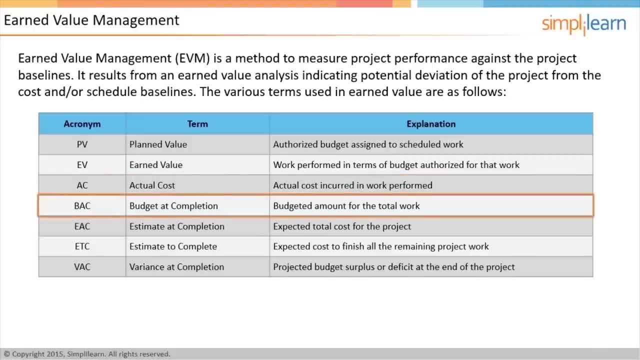 Budget at completion is the budgeted amount for the total work. Estimate at completion is the expected total cost for the project. Estimate to complete is the expected cost to finish all the remaining project work. Variance at completion is the projected budget surplus or deficit at the end of the project. 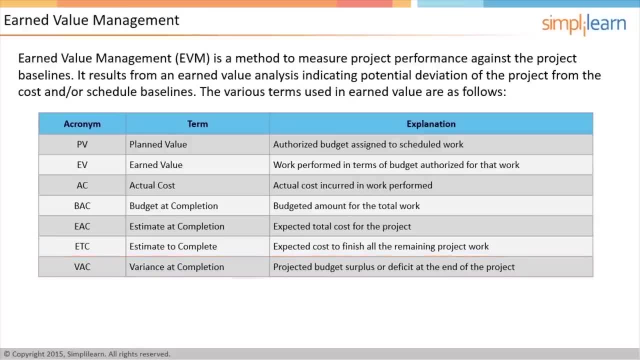 All the parameters displayed on the screen are measured in terms of cost. You may come across business scenario based questions on earned value management in the PMP exam, So ensure that you develop a clear understanding of this topic. Let us look at an example of a planned. 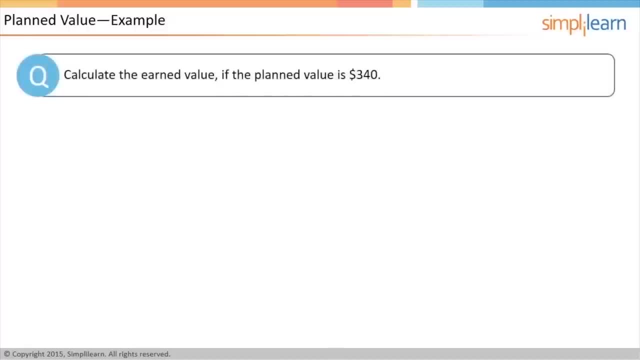 value in the next screen. Planned value is the estimated value of the work planned. This value is measured in terms of currency, say dollar. If the planned value is $340, then the work planned is worth $340.. How do you calculate earned value? 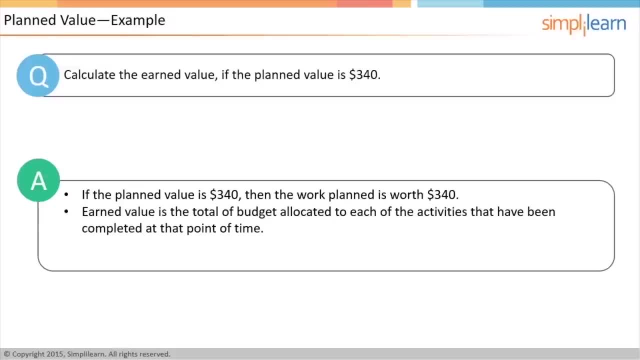 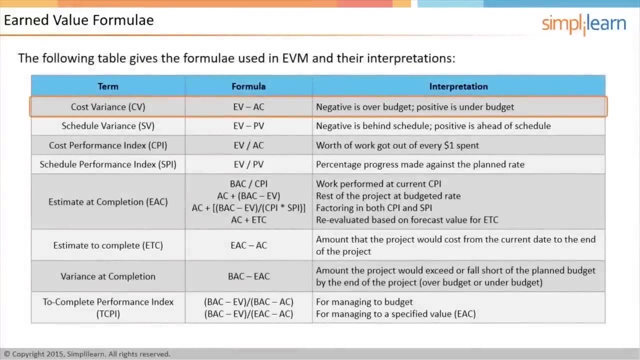 The solution is add the budget allocated to each of the activities that have been completed at the point of time. The resulting value is the earned value. In the next screen, let us look at the formula used to calculate earned value In cost variance. negative means. 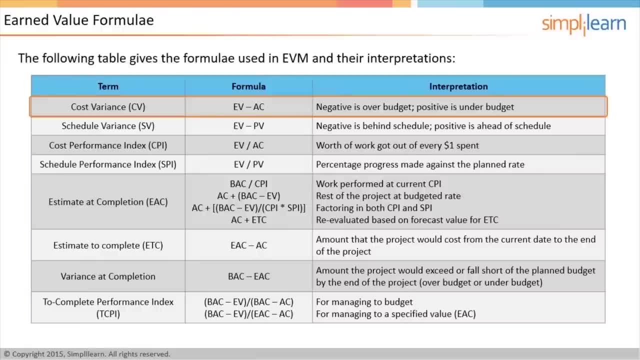 the project is over budget. Positive means the project is under budget. Similarly, in schedule variance, negative means the project is ahead of schedule, whereas positive means the project is ahead of schedule. The value of the next two parameters- cost performance index. 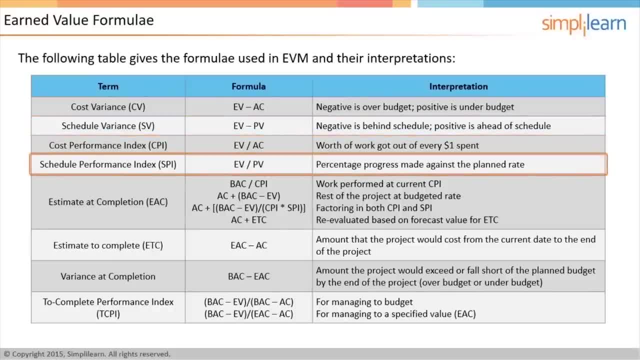 CPI and schedule performance index. SPI values vary between 0 and 1.. For example, a CPI of 0.8 implies that 80 cents of work is obtained for every dollar spent in the project. Similarly, if SPI is 0.9,. 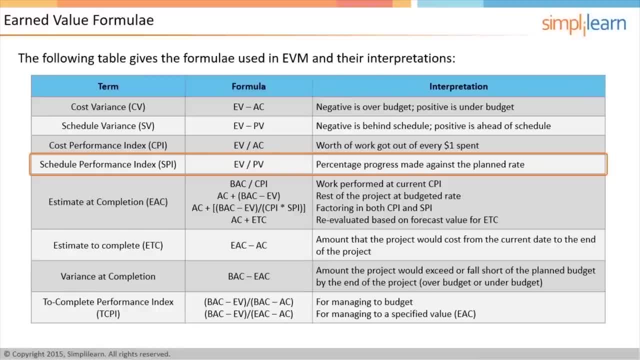 it implies that project is progressing at only 90% of the speed originally planned. The next parameter is estimate at completion, or EAC. There are different ways of calculating the EAC value. The method used depends on how the cost and schedule variances are expected to play. 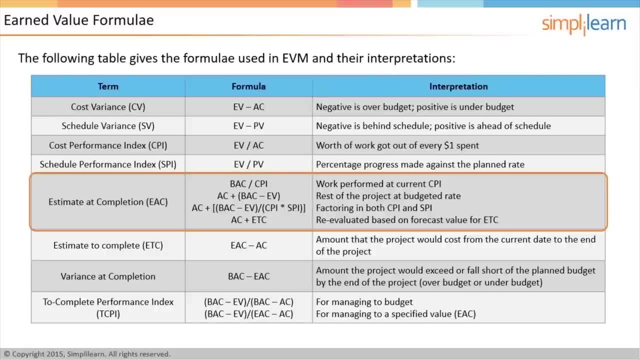 for the rest of the project. BAC by CPI is used if you expect that the current cost performance will continue until the end of the project. AC plus BAC minus EV is used if you expect that the rest of the project will be managed at the budgeted rate. 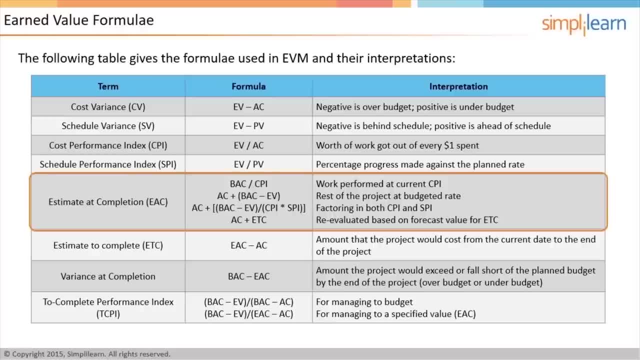 AC plus BAC, minus EV by the product of CPI and SPI is used if you want to factor in the impact of the cost as well as schedule variances. AC plus ETC is used if you want to re-evaluate the project based on a forecast value. 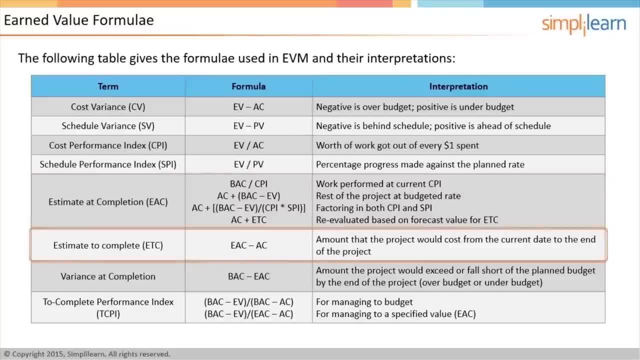 for the estimated cost of the remainder of the project. The next parameter is estimate to complete or ETC, which is the cost of project from this point to the end. This is calculated by subtracting the actual cost from the estimate at completion. In addition, 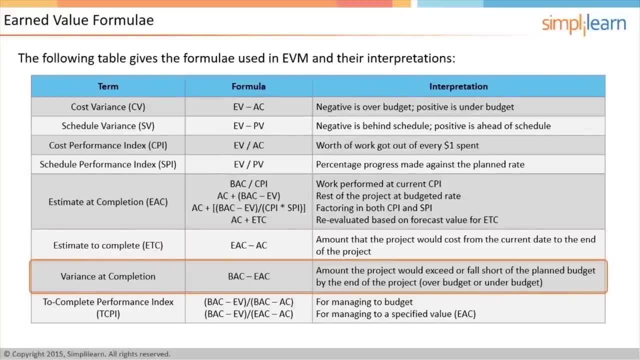 variance at completion can be calculated by subtracting the estimate at completion from the budget at completion. Variance at completion is the cost estimation, whether it is over or under budget. Another parameter is the to complete performance index, or TCPI. This is the 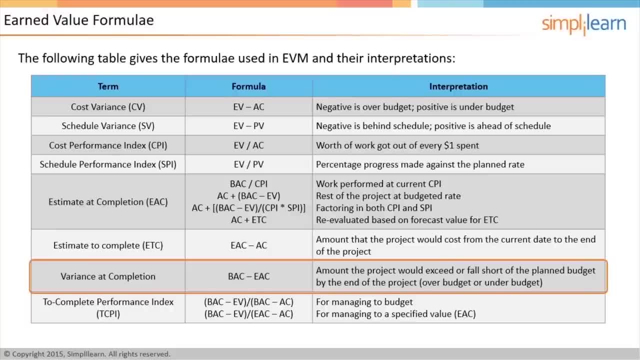 cost performance needed to achieve a desired outcome. For example, if the project needs to be managed to the original budget BAC, then TCPI- that is, the CPI that must be maintained for the rest of the project- is calculated as BAC minus EV. 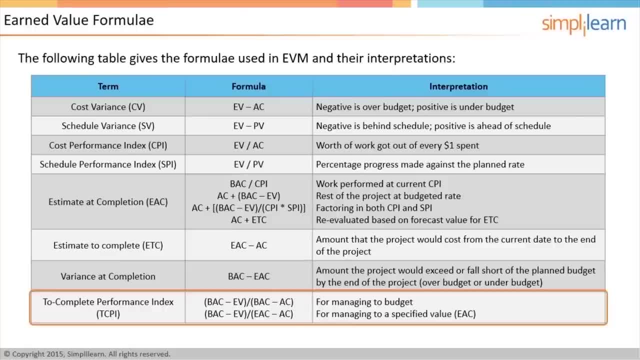 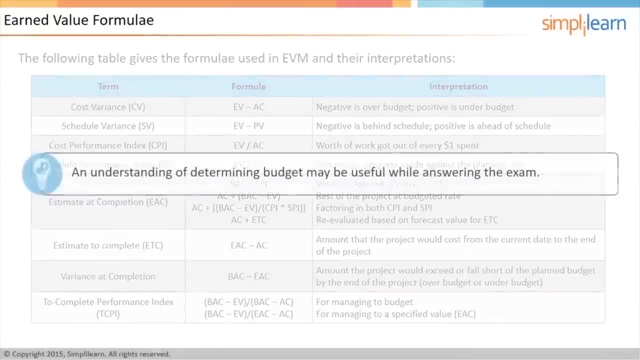 by BAC minus AC. Similarly, if it has to be managed within a revised target, say AC, then TCPI is calculated as BAC minus EV, by EAC minus AC. Before the start of the PMP exam, please make a note of the formulas of: 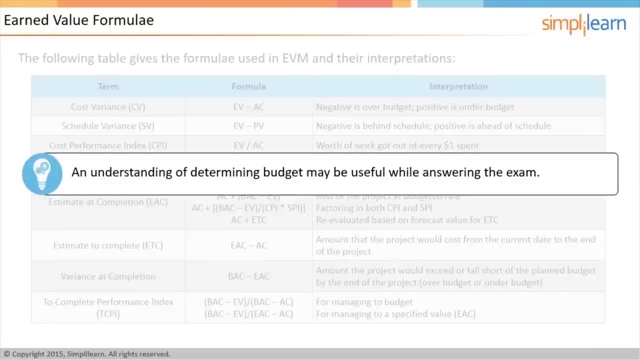 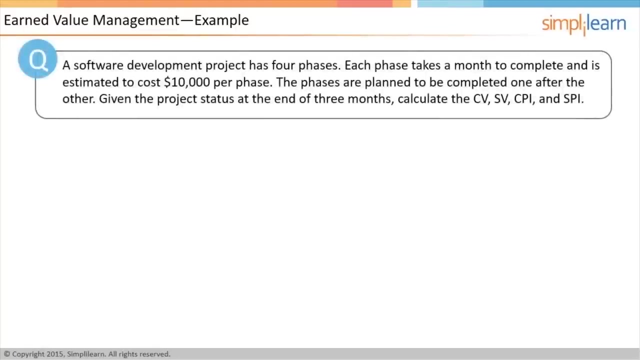 earned value technique. In the next screen, let us look into a business scenario to understand this concept better. After reading the problem statement, click the solution button to look at a possible answer. Let us take the example of a software development project. There are four phases. 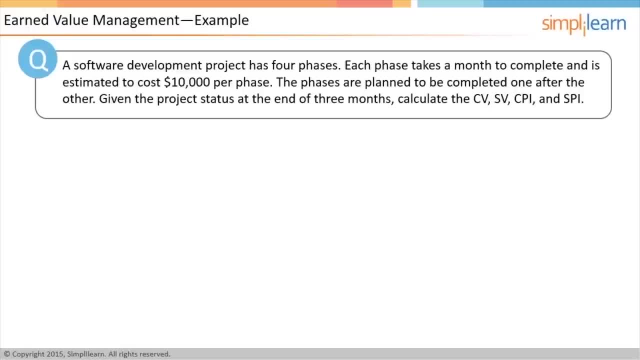 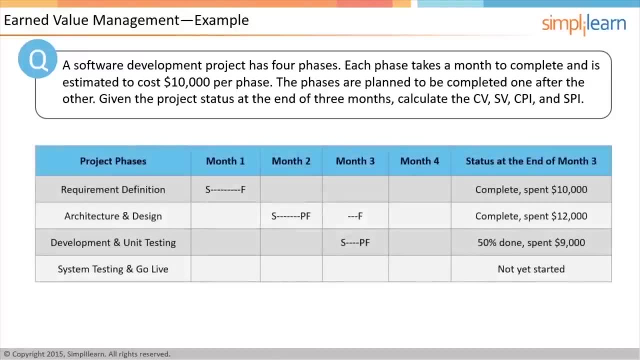 and each phase takes a month to complete and is expected to cost $10,000.. The phases are planned to be completed one after the other. The status of the project at the end of the month three is summarized in the table. Requirements definition is. 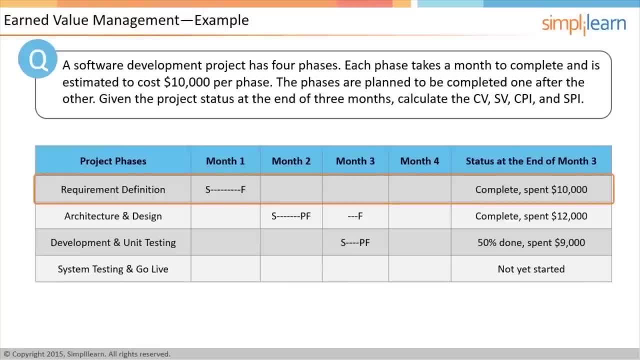 completed, and actual spending on this is $10,000.. Architecture and design is done, and actual spending on this is $12,000.. Development and unit testing is only 50% done, though it was supposed to be completed by third month. It. 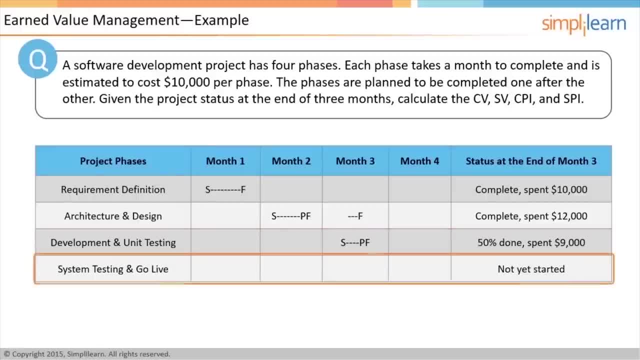 has cost $9,000 until date. System testing and go live has not yet started. Note S indicates start time, F indicates finish time and PF indicates that it is partly finished at the end of the month. Based on the above information, calculate the. 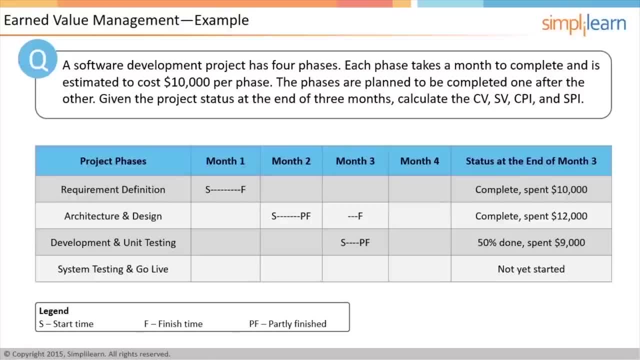 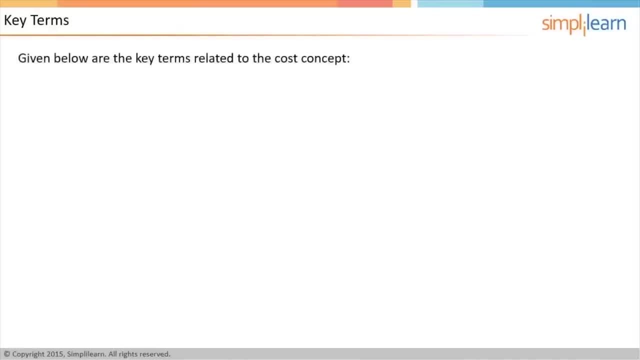 CV, SV, CPI and SPI of the project. Let us look at a solution in the next screen. Before we end this lesson, let us also look at a few definitions that might be useful for your PMP examination. Law of diminishing return- This. 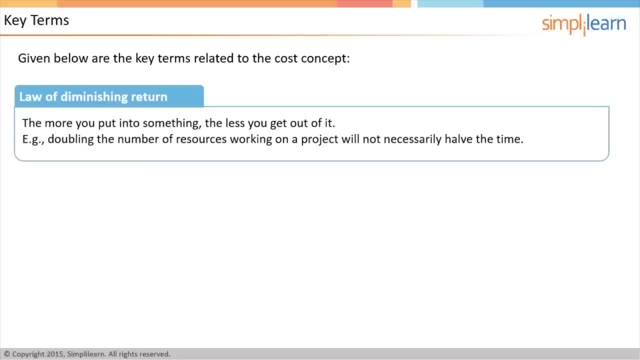 means the more you put into something, the less you get out of it. For example, doubling the number of resources working on a project will not necessarily halve the time Working capital, The amount of money the company has to invest on the project. 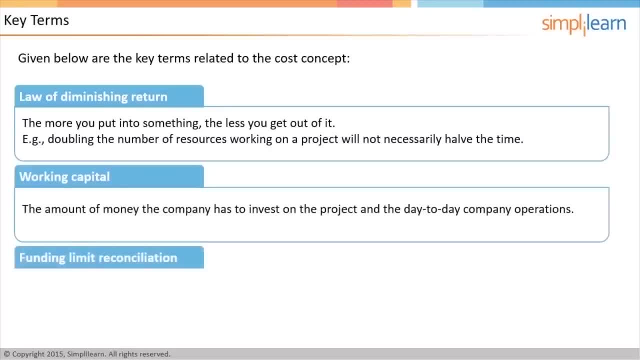 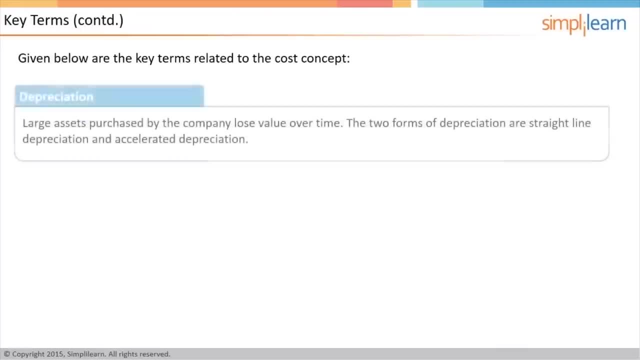 and the day-to-day company operations. Funding limit reconciliation: The process of comparing the planned expenditure in a given period with the available funding for that period. Large assets purchased by the company lose value over time. This is called depreciation. There are two forms of depreciation. 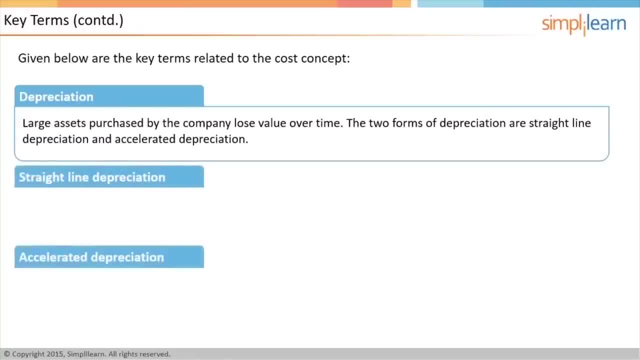 Straight line and accelerated. Same amount of depreciation is taken every year. For instance, a car with a price tag of $10,000 and useful life of 10 years is depreciated $1,000 per year. At the end of the 10th year, the value of the car is. 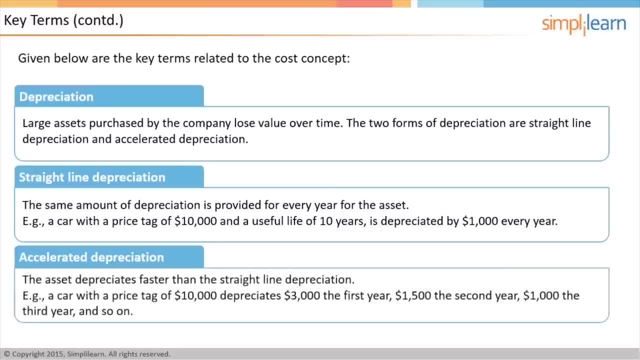 considered zero for all accounting purposes. Accelerated depreciation Depreciates faster than the straight line depreciation. For instance, a car with a price tag of $10,000 depreciates $3,000, the first year $1,500, the next year $1,000. 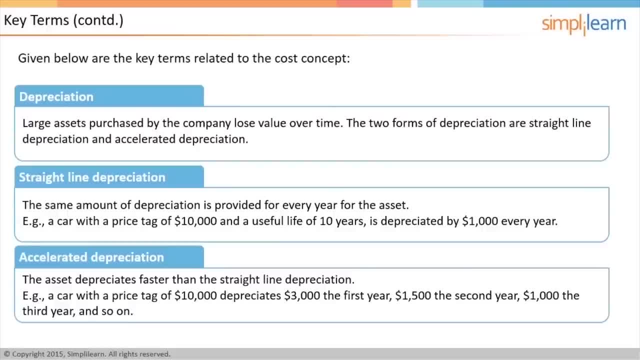 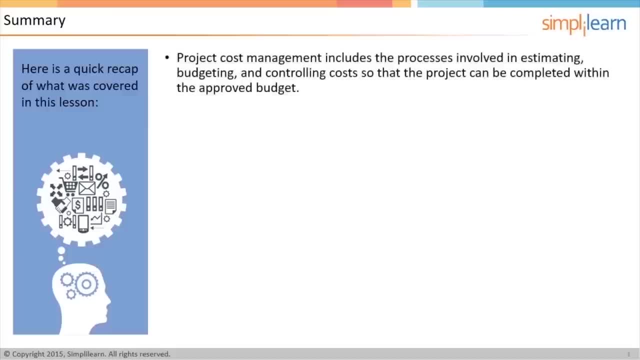 the third year, and so on. Let us now check your understanding of the topics covered in this lesson. Here is a quick recap of what was covered in this lesson. Project cost management includes the processes involved in estimating, budgeting and controlling costs so that the project 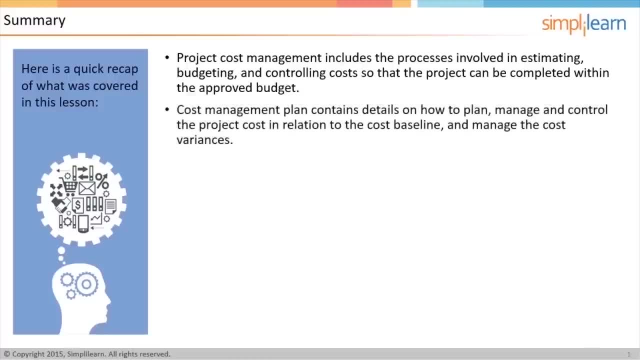 can be completed within the approved budget. Cost management plan contains details on how to plan, manage and control the project cost in relation to the cost baseline and manage the cost variances. Cost estimate is an educated guess of how much an activity or project will cost. 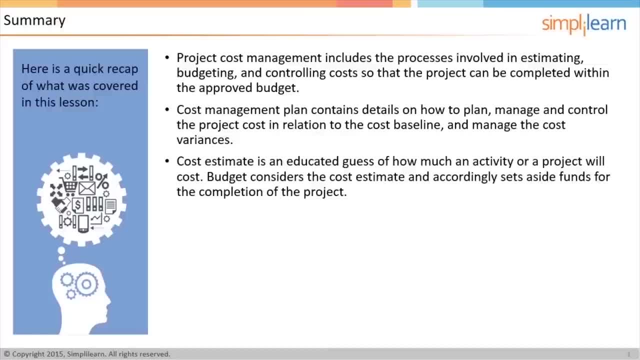 Budget considers the cost estimate and accordingly sets aside funds for the completion of the project Under control. account technique related activities are clubbed and their costs are managed as one unit. The four project cost management processes are: plan cost management, estimate costs. determine budget control costs. 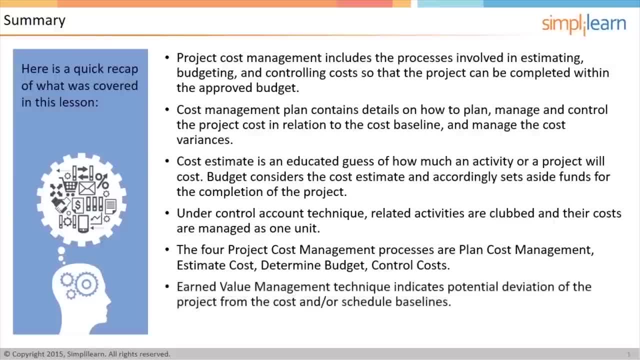 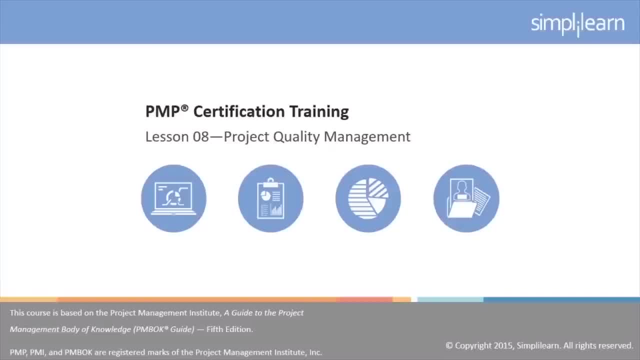 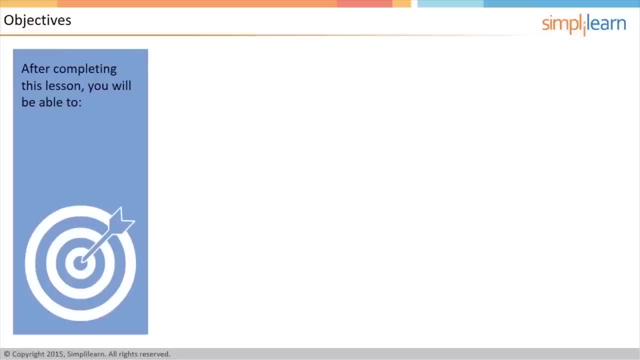 Earned value management technique indicates potential deviation of the project from the cost and or schedule baselines. In this lesson, we will focus on project quality management. Let us begin with the objectives of this lesson. After completing this lesson, you will be able to define quality. 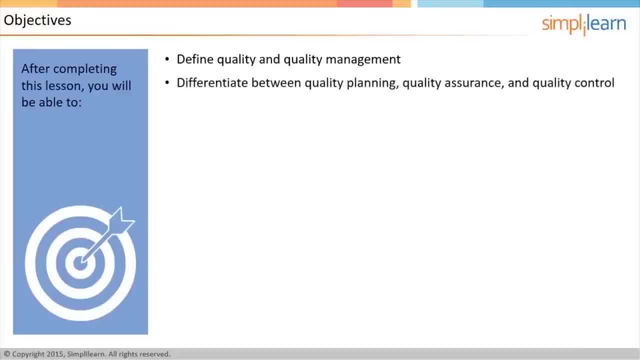 and quality management. Differentiate between quality planning, quality assurance and quality control. Explain cost of quality and its categories. Describe the project quality management processes. Explain the seven basic tools of quality. Explain Six Sigma In the next screen. let us take a quick look. 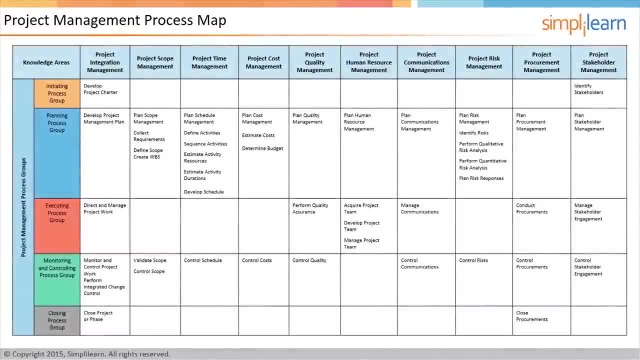 at the project management process map. There are 47 processes in project management, grouped into ten knowledge areas and mapped to five process groups. In this lesson we will look at the fifth knowledge area, that is, project quality management and its processes In the next. 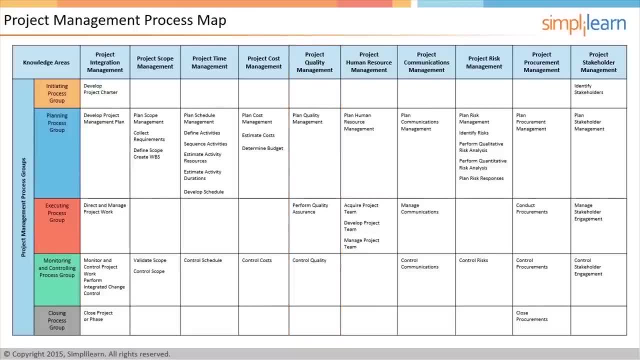 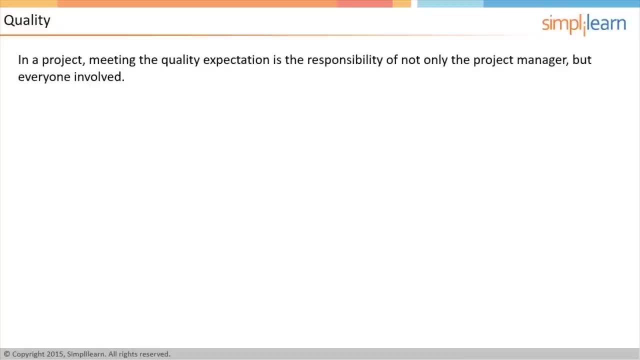 screen. let us understand what quality is. The project manager is responsible for quality in a project. However, it is also the responsibility of each and every one in the project to ensure that whatever they do meets project quality expectations. Quality is defined as the degree. 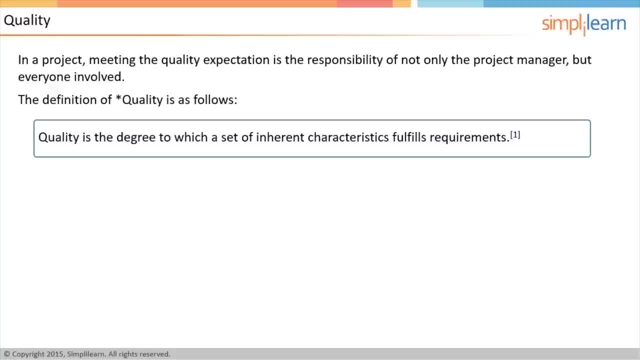 to which a set of inherent characteristics fulfills requirements. A project is said to meet quality expectations when all the project requirements agreed in the beginning of the project are met and the resulting product is usable. Usable means that the intended users can use the product without any problem. 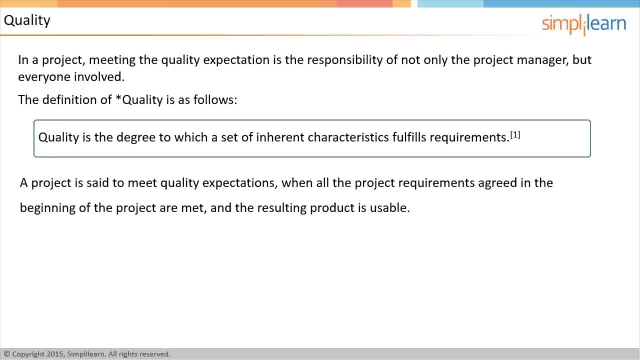 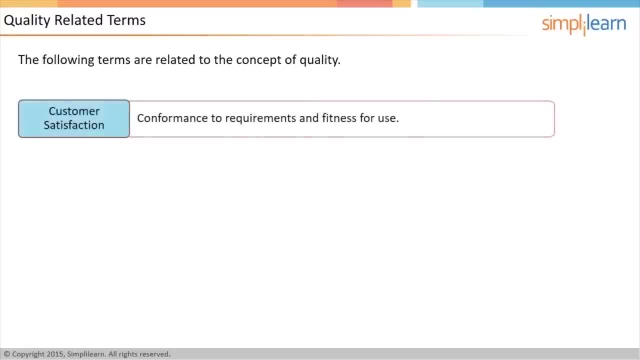 In the next screen. let us look at some quality related terms. It is important to discuss a few terms to understand the concept of quality. better Customer satisfaction is defined as conformance to requirements and fitness for use. It is important to understand the subtle 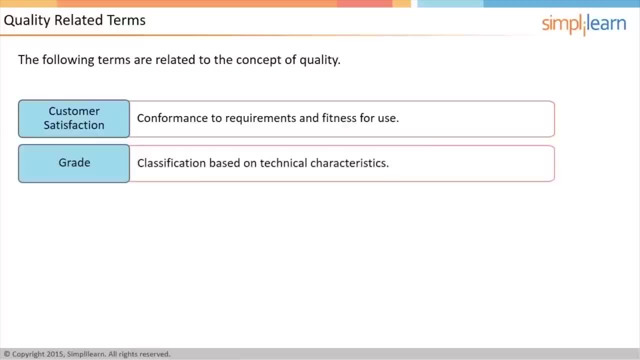 distinction between quality and grade. Grade is a classification based on technical characteristics. Low quality is always a problem, but low grade may not be a problem. Rather, it would be a matter of choice. Similarly, it is important to understand the distinction between precision and accuracy. 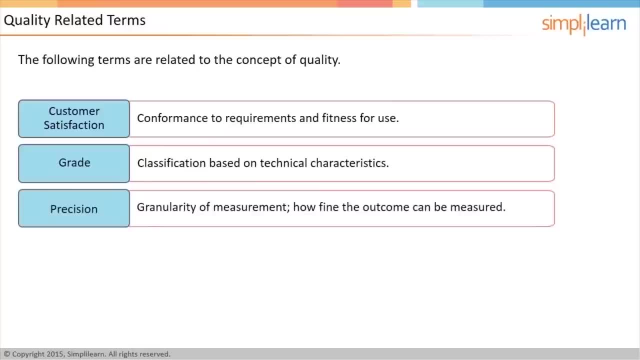 Precision is the granularity of measurement. That is, how fine-grained can you measure the outcome. Accuracy is how correct you are. That is how close you are to the desired value In the next screen. let us understand the concept of optimal level. 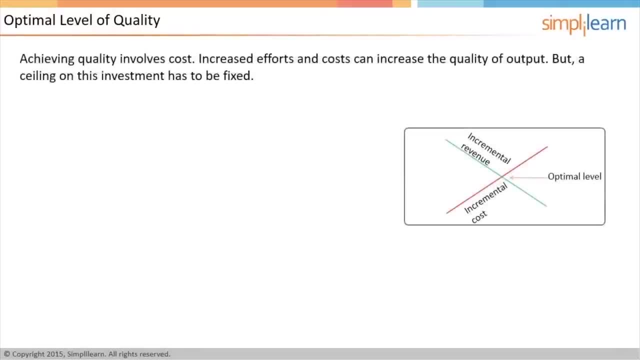 of quality. Quality comes at a cost. More effort put in quality will give better results. However, you cannot keep on investing on increasing the quality, as there is no limit to how much a product can be improved. Investment in quality is determined by knowing. 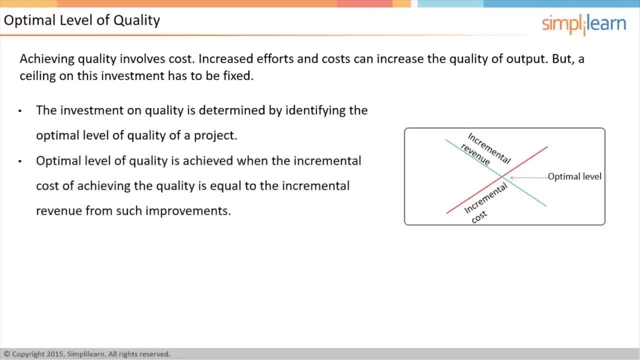 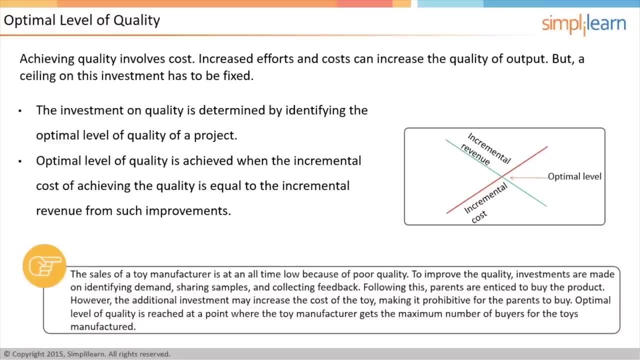 the optimal level of quality. Optimal level of quality, as shown in the diagram, is said to be achieved at the point where the incremental revenue from improvement equals the incremental cost to secure it. Suppose you are the manufacturer of toys, but the toys are. 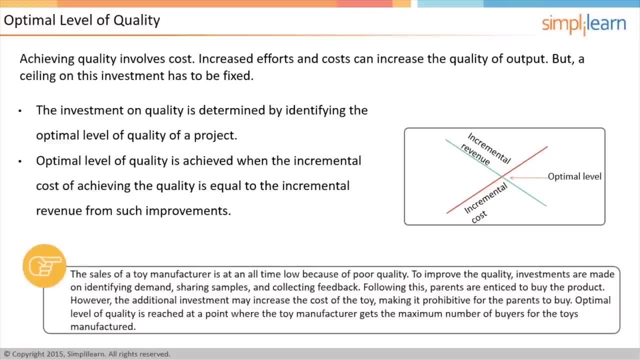 below quality and the sales are low. To improve the quality, you invest in identifying the demands of children, sharing few samples and recording their feedbacks. Once all these are captured and implemented in the products, you lower the parents to buy them. 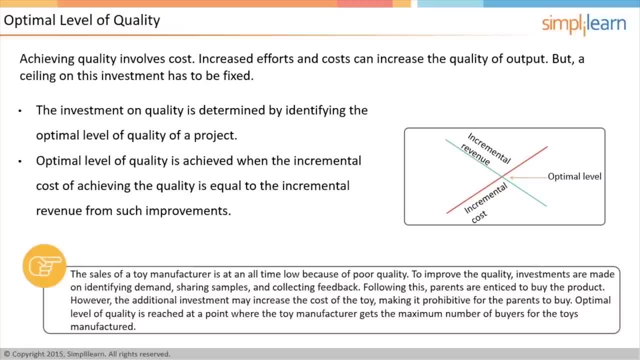 As the investment is increased to manufacture good quality toys, the cost will therefore increase and it might become prohibitive for parents to buy. Optimal level of quality is reached at a point where you get maximum number of buyers for the toys manufactured. Now that we are clear on the 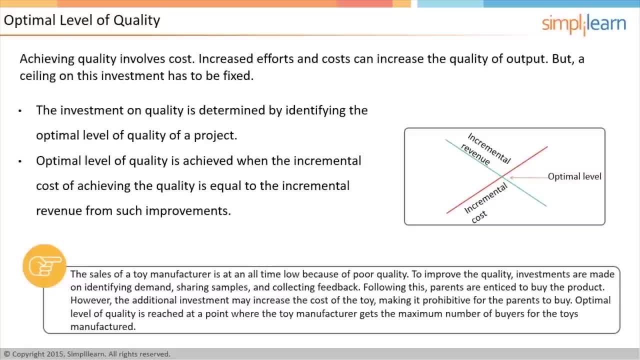 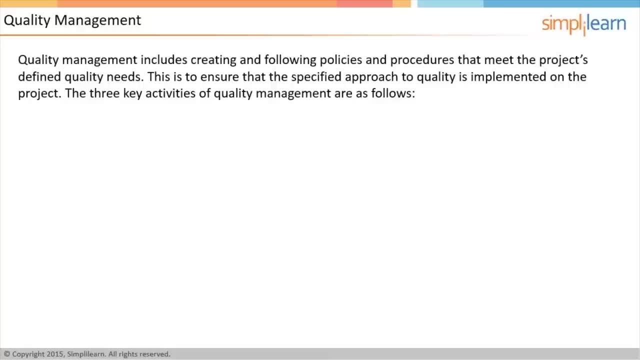 concept of quality. in the next screen let us discuss quality management. Quality management involves performing activities like creating standard policies and procedures and ensuring that those standard procedures are being followed properly in the project. It aims to ensure that project meets all the initial 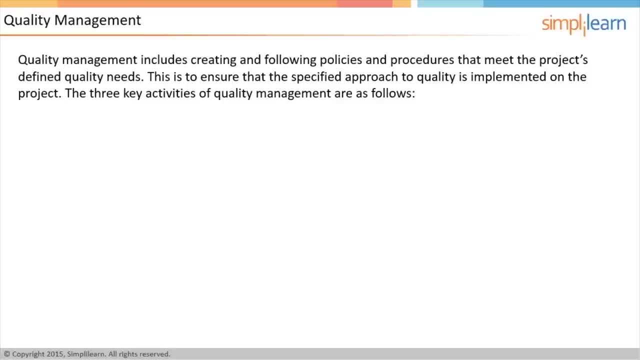 agreed requirements without any deviation and that the specified approach to quality is implemented on the project. Three broad activities are done as part of quality management. They are quality planning, quality assurance and quality control. Quality planning is the first step when quality related. 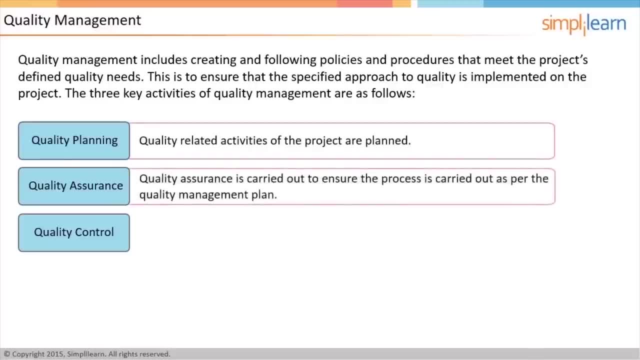 activities of the project are planned. Quality assurance is the next stage of implementing those quality plans and quality control is the last stage when periodic checks are done to see if project quality is improving. In the next screen let us look into the differences. 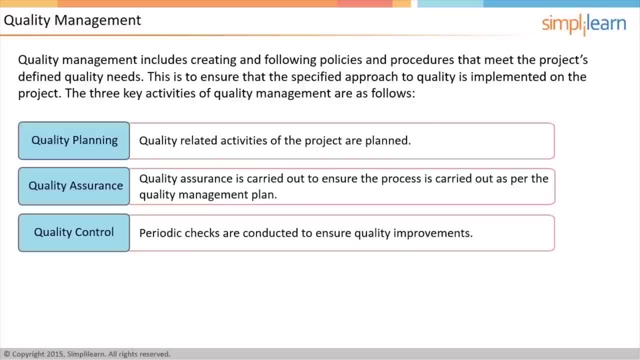 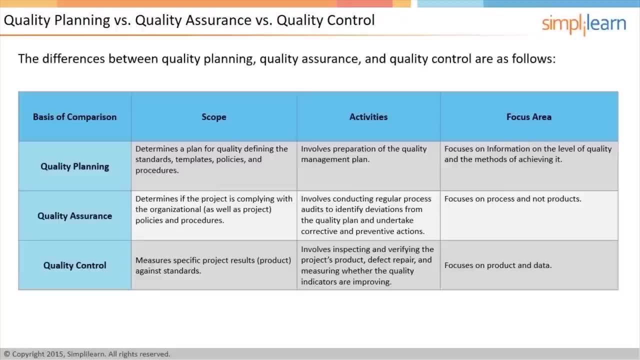 between the three aspects of quality management. It is important to understand the different kinds of activities that come under quality planning, quality assurance and quality control. Once the quality planning is done, the quality management plan is ready. This quality management plan has standards templates. 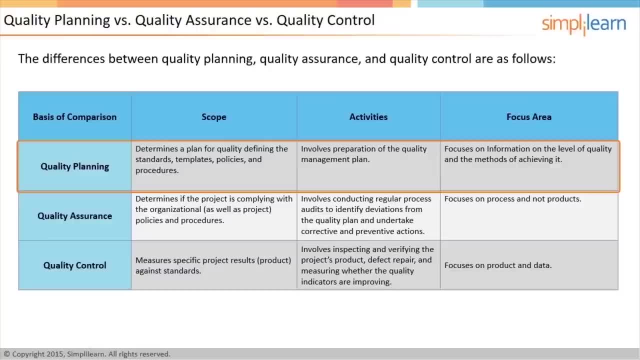 policies and procedures to be followed in the project. It contains information on the level of quality being aimed and the plan to achieve that level. It is the aim of quality assurance activities to ensure that the activities planned under quality planning phase gets executed for the project. 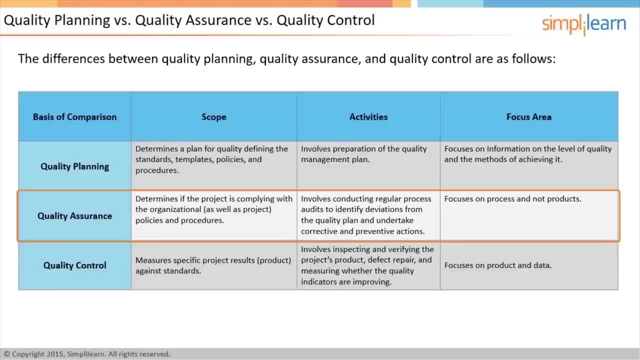 It is the task of quality assurance to determine if the project is complying with the organizational as well as project policies and procedures. This is ensured by conducting regular process audits to identify deviation from what is planned in the quality management plan. These audits are generally done by quality. 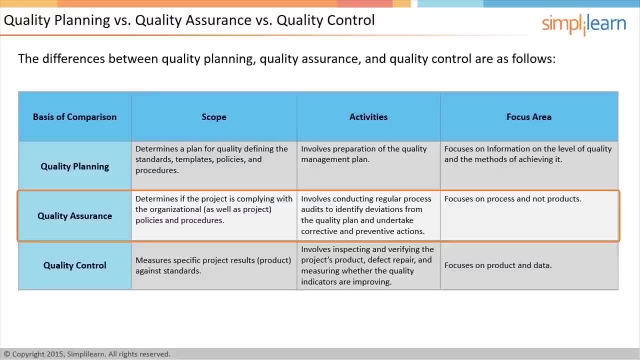 department of the organizations. Quality assurance focuses on the process, not on specific products. The role of quality control is to measure specific project data or results against standards, to inspect and verify the project's product defect repair and measure whether quality indicators are improving. 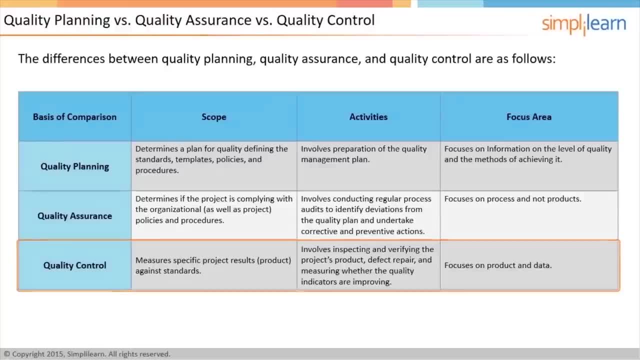 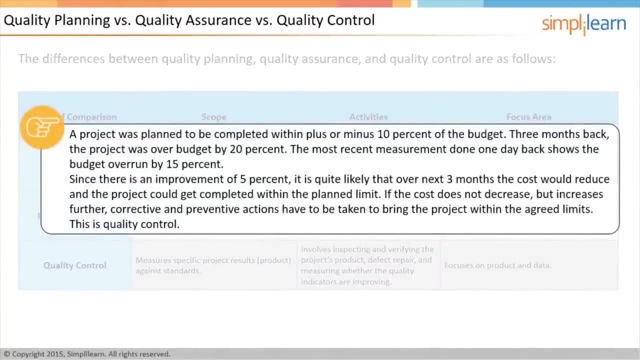 Quality control is about the product and data. For example, it was planned as part of quality management that project would get completed plus or minus 10% within the cost budget. Three months back, when the measurement was done, project was over budget by 20%. 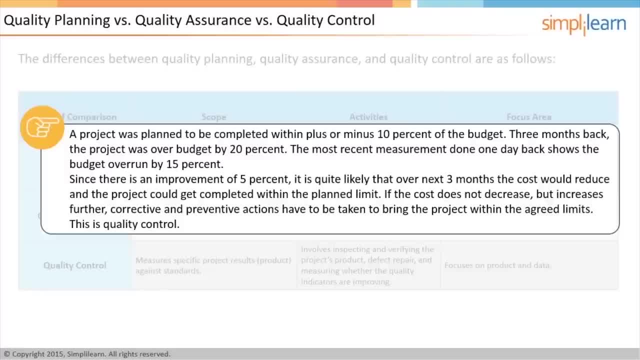 When the measurement was done a day before, it was only 15% over budget. Therefore, the project has showed an improvement of 5% in the last three months and it is quite likely that over the next three months project may get within the. 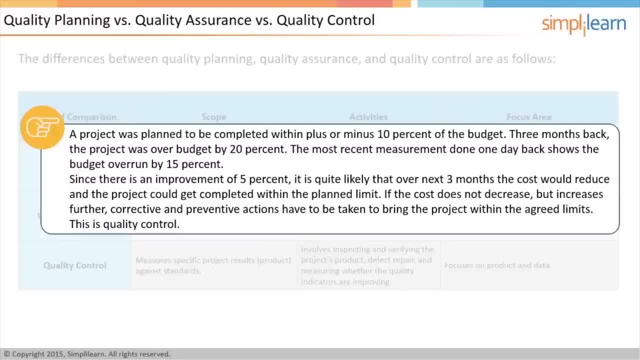 planned limit of 10% Instead of showing improvement. if the data shows cost increase, then corrective and preventative actions are required to get the project within the 10% limit. This is quality control. In the next screen, let us discuss a few. 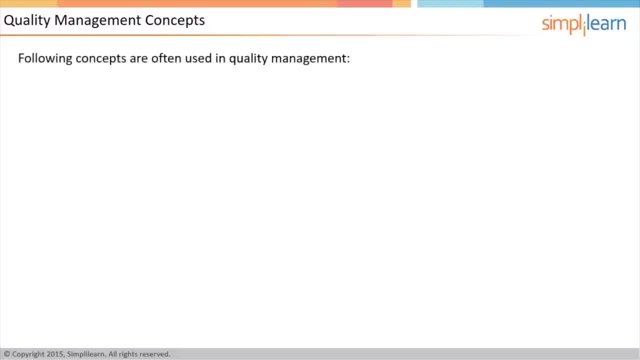 quality management concepts. Let us look at some terms that are commonly used in quality management parlance. Total quality management, or TQM, is a quality management philosophy that involves holistic thinking about meeting the objectives of an organization. It places the responsibility of quality squarely on the management. 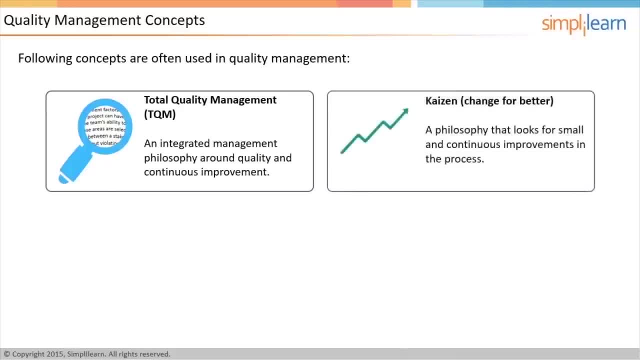 Kaizen is a Japanese term that stands for change, for better. Kaizen philosophy is one that should always be looking for small and continuous improvements in the process Deeming cycle or PDCA cycle, that is, plan, do, check. act is a process control and. 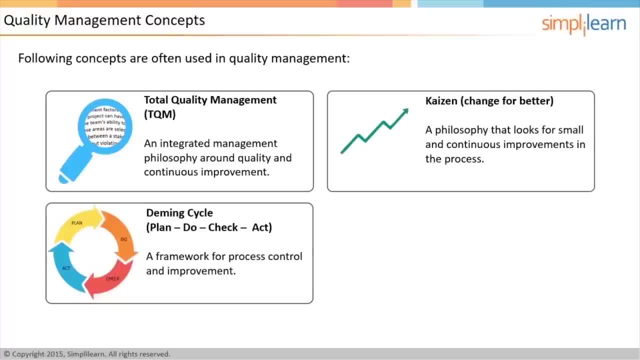 improvement approach propagated by the famous quality guru Edward Deeming. It means you plan for something, execute it, check the output and, based on the lessons, you act to bring the deviations under control. Kanban is a poll-based management system that originated in Japan. 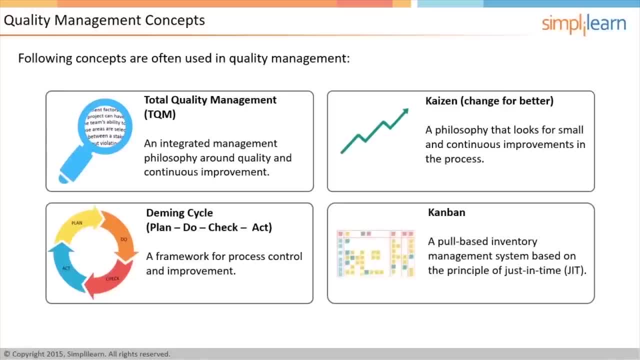 based on just-in-time JIT inventory management. The idea behind Kanban is to minimize the work in progress and achieve a smooth flow in the process from start to finish, Because building up inventory only to paper over the imperfections in the system tends to hide the problems. 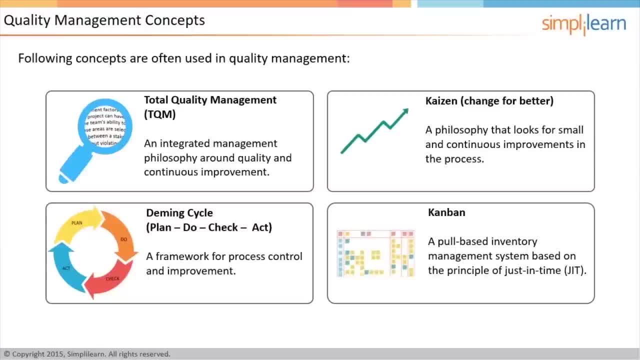 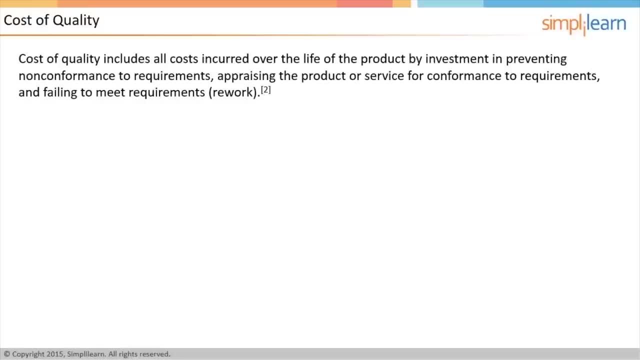 In the next screen. let us focus on cost of quality. Cost of quality is the cost that needs to be incurred to make a quality product. The sum of all the costs incurred is ensuring that project conforms to requirement is cost of quality. Cost of quality. 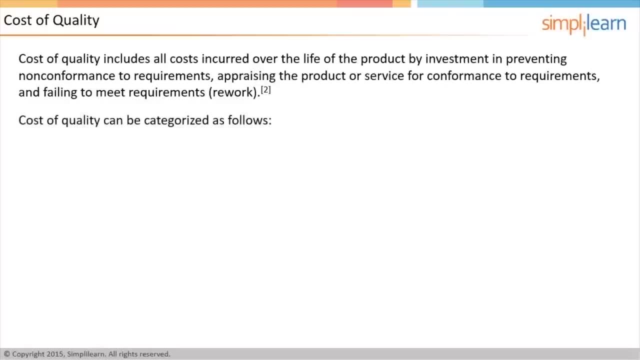 can be broken down into two major categories. First is the cost of conformance, or the money spent during the project to avoid failures. This can further be subdivided into prevention costs, which is the cost to prevent errors, Like training the team, creating documents on equipment. 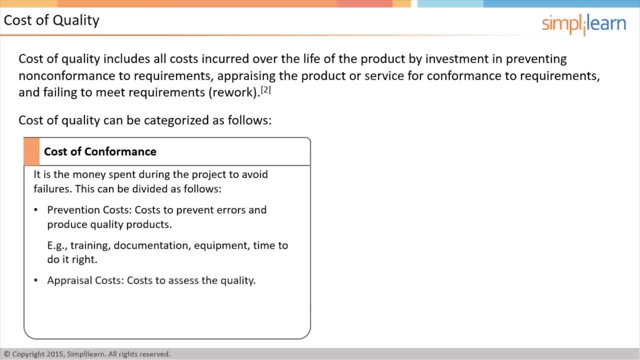 and, in time, to do it right. The other subdivision is appraisal costs or the cost for assessing quality, like testing, destructive testing, loss and inspections. The second category is the cost of nonconformance. It is the money spent during and after the project because of failures. 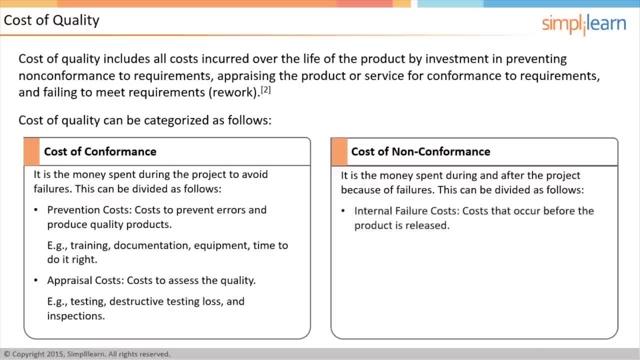 This is subdivided into internal failure costs. It is the cost of failures that occur before the product is released to customers, for example, rework and scrap. The second subdivision is external failure costs. It is cost incurred on failures that occur after it has been released by the. 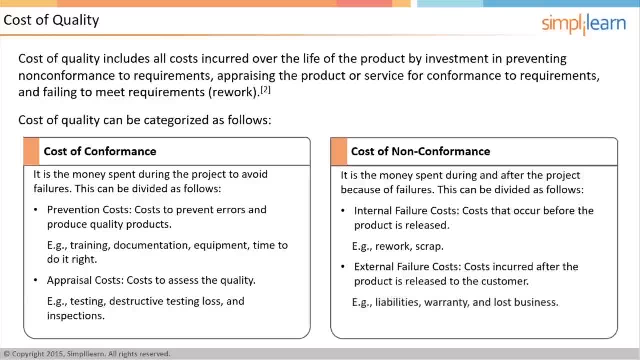 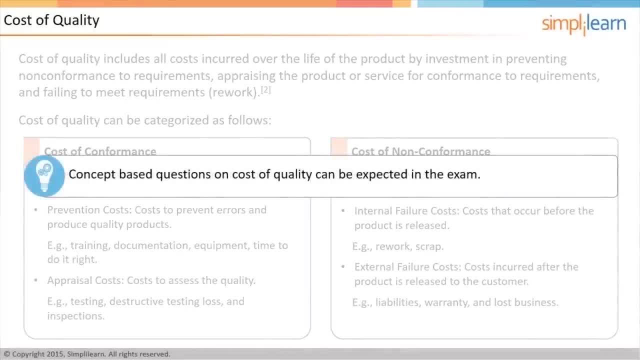 team. for example, liabilities, warranty work and lost business. Concept based questions on cost of quality can be expected in the exam, So please make a note of the categories of cost of quality. Let us look at the project quality management processes in the next screen. 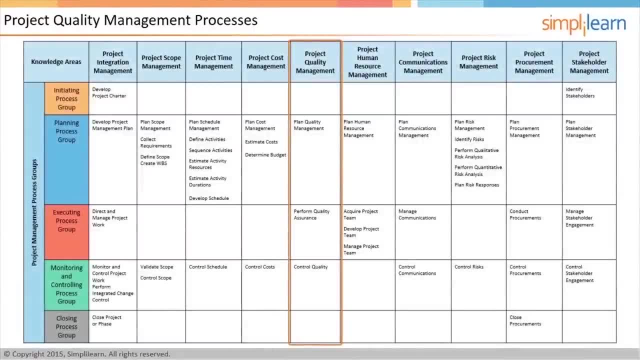 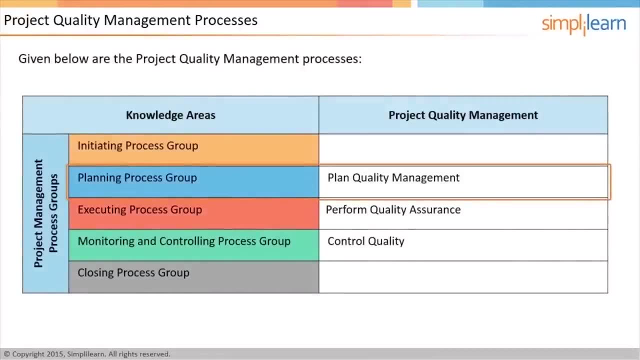 There are three project quality management processes, of which the first process- plan quality management- is done as part of the planning process group. The next process- perform quality assurance- is done as part of the executing process group and the last process. 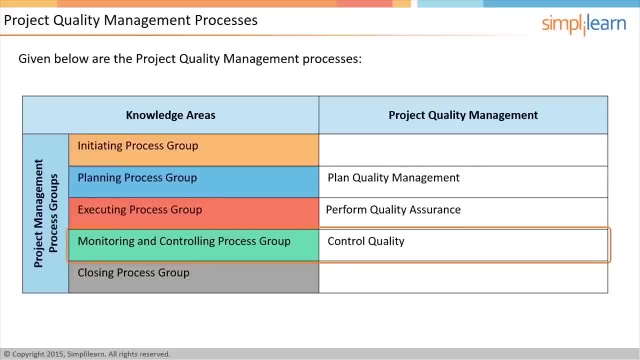 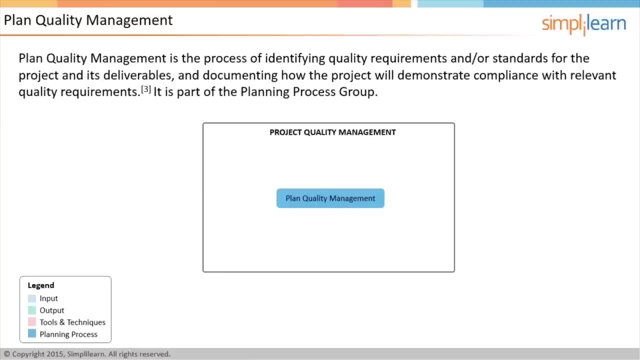 control quality is done as part of the monitoring and controlling process group. In the next three screens, let us look into each of these processes in detail. The aim of the plan quality management process is to identify the relevant requirements or standards to execute the project. 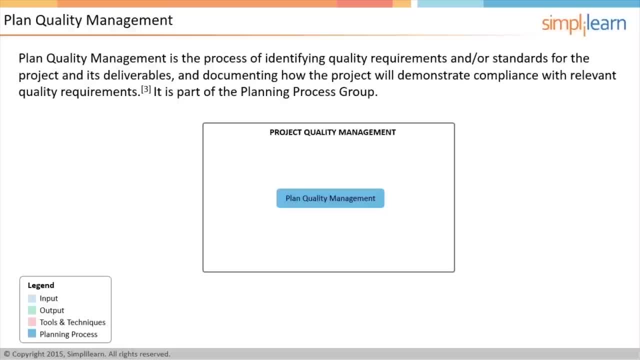 effectively to achieve the desired quality level. Quality planning results in the creation of the quality management plan. Aim of the plan quality process is to identify the standards. A standard is an agreed upon process to work or achieve a result. A standard can be set from within. 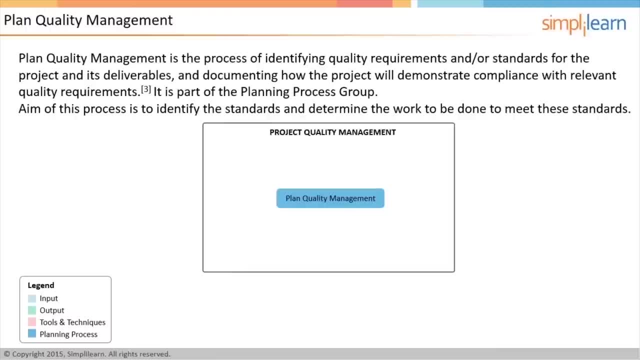 the organization or government. Once all the standards for the project are identified, the aim of the quality planning activities involves determining what work needs to be done to meet those standards. Before adhering to the standards, you should question their relevance with the project Implementing. 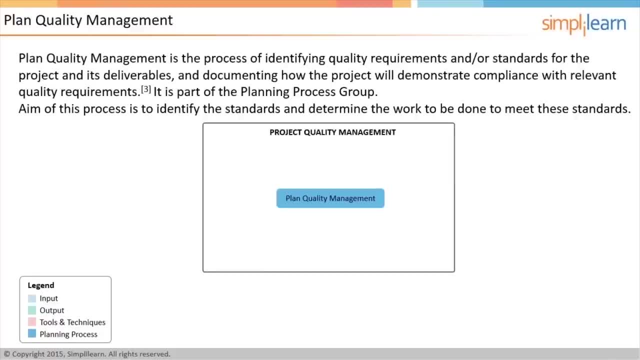 all possible standards applicable to the project in random will have cost and time implications. Let us look at the inputs to this process. The project management plan provides the scope, schedule and cost baseline, all of which have an implication on the quality management plan. 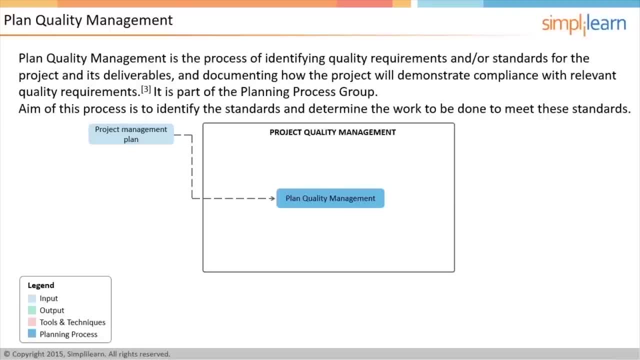 Quality plan has a direct correlation with these. It might also have an impact on and be impacted by other subsidiary management plans, such as risk management. The stakeholders of the project may have specific requirements and views about the quality parameters of the project and these have to be considered. The risk 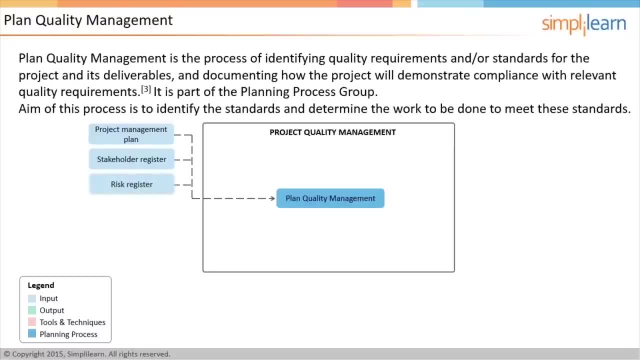 register gives an indication about the kind of risks that are inherent in the project and also those which must be considered while planning the activities to ensure quality. The requirements for the project need to be considered for planning quality related activities, because quality is all about meeting the requirements In addition to 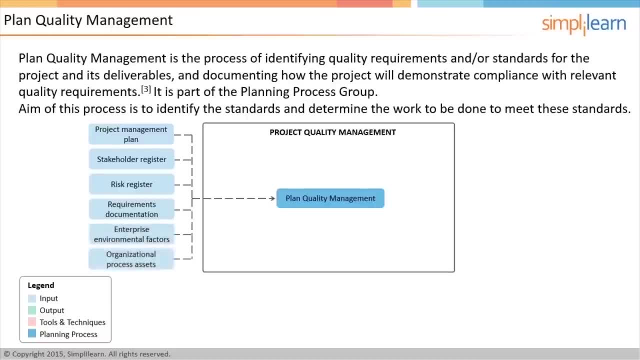 these enterprise environmental factors and organization process assets are also listed as inputs because the standards can be either from within the organization or from government or other external bodies. Standards from within the organizations are usually the best practices learned over a period while executing numerous projects. An example of 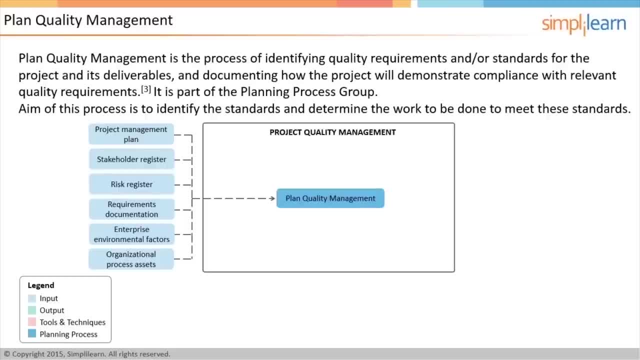 government standards can be standards to control air pollution by the motor vehicles which vehicle manufacturers must adhere to. To accomplish quality planning, first analyze the benefits versus the costs of meeting quality requirements. Next identify the cost of quality and confirm if that kind of investment. 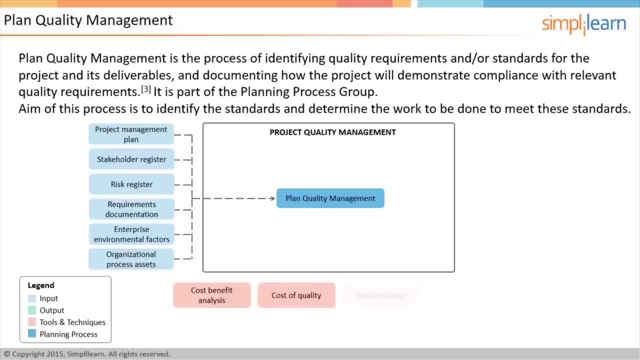 in quality is justified. In addition to these two, benchmarking helps in analyzing the quality of activities of similar projects executed in the past. This helps in identifying the particular quality of output of the previous project, which in turn acts as a basis for the current. 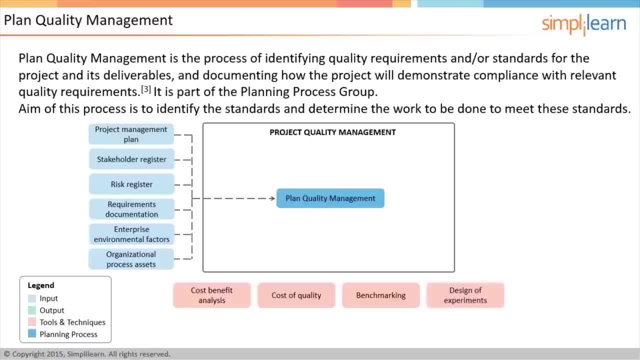 project's quality planning. Design of experiments can also be used for quality planning. This is a statistical way to determine what variables will improve quality the most. For example, in case of manufacturing doors, it can be determined that increasing the quality of the wood can have maximum. 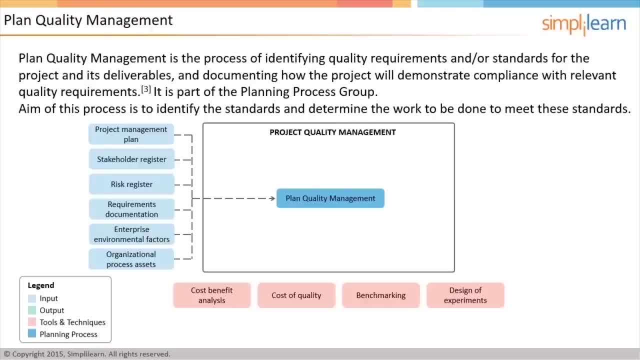 impact on improving the quality of the door. In addition, the seven basic quality tools, also known as the 7QC tools, are used to determine the plan to achieve the desired level of quality. Statistical sampling as a tool becomes relevant whenever the quality 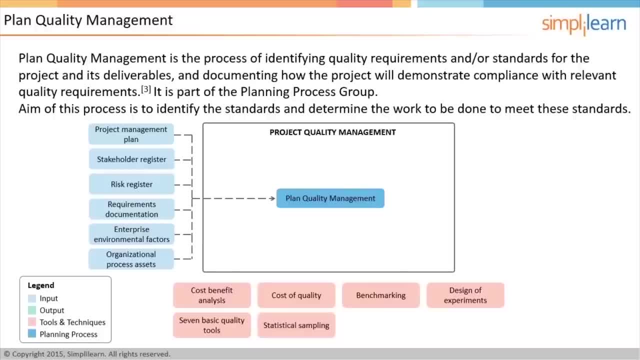 plan cannot be applied to all the artifacts produced. For example, if destructive testing is a requirement, then it can be carried out only on a sample, not on the entire population. Statistical sampling helps in arriving at a representative sample that can give useful information. 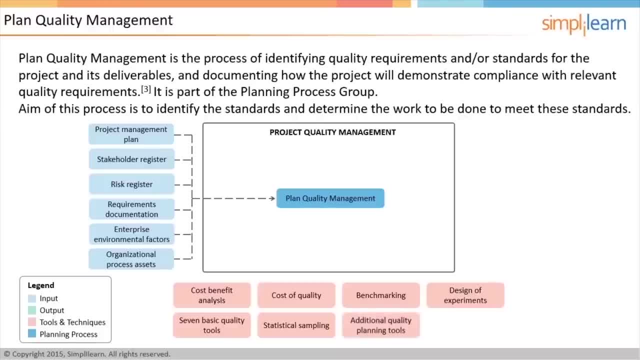 Other additional tools, such as brainstorming, resource field analysis, etc. may be used to determine the quality management plan for the project. Conducting regular meetings is another important tool. The quality management plan has to be determined in a collaborative manner by consulting. 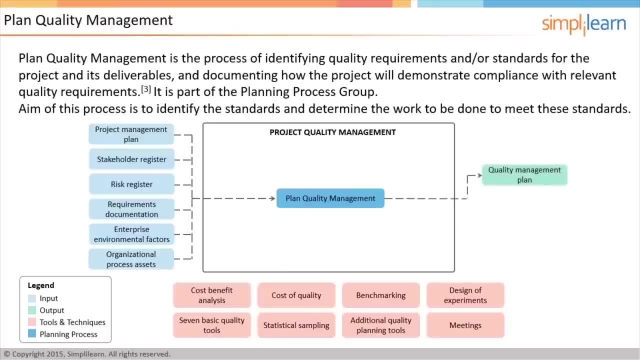 the team members and other stakeholders. Quality management plan is a key output of this process. Checklist is a list of items to inspect. For example, many of the office buildings have housekeeping checklists to ensure that all floors, cabins etc are cleaned. 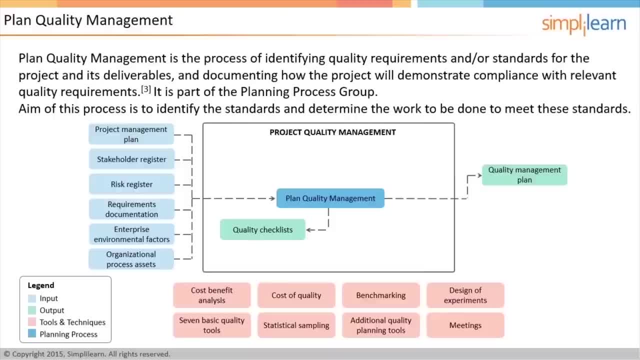 Checklists are created during quality planning and used in quality control. Metrics are project specific data that need to be measured to check the status of the project. The simplest project metrics can be cost and schedule. Metrics are also decided during quality planning and used in quality control. 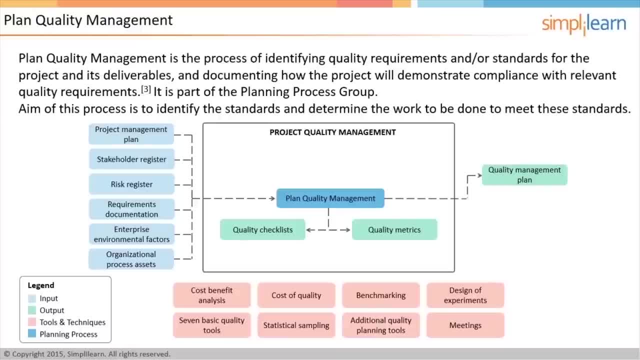 One of the roles of the project manager is to not only manage the project but also improve processes in the project to decrease the instances of defects, which in turn saves time and money. Such activities are listed in the process improvement plan, which eventually becomes part. 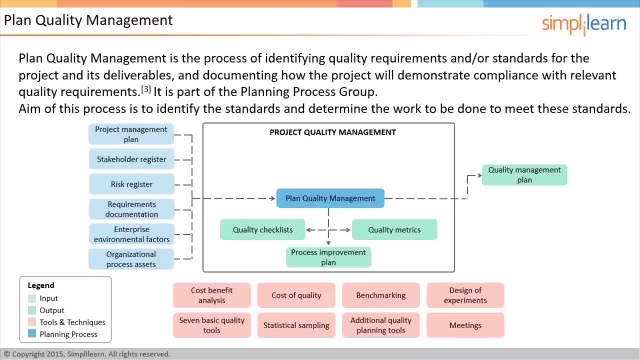 of project management plan. As a result of the planning activities, other project documents may also get updated. For example, the quality management plan may result in updates to the cost or resource requirements. There may be questions in the PMP exam based on the planned quality management. 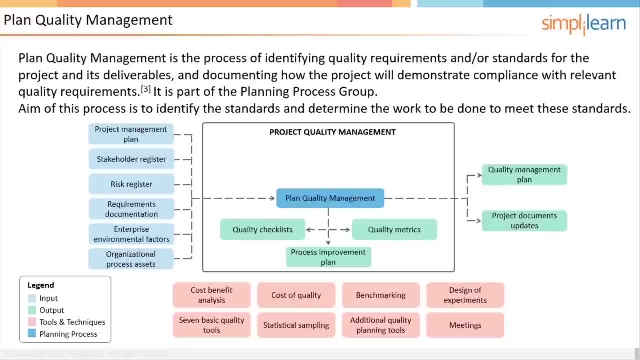 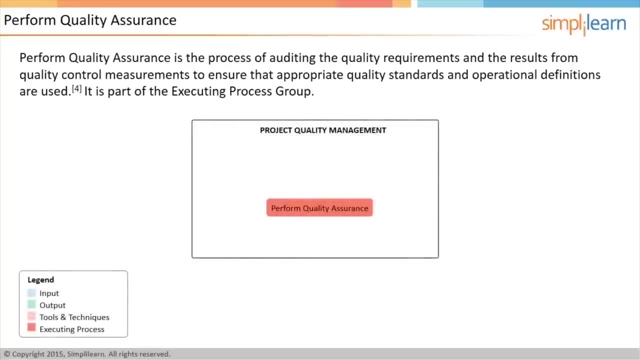 process. so please ensure you have a fair understanding of the concept before you take the exam In the next screen. let us discuss the second quality management process. Once the quality planning is over, the next process in project quality management is quality assurance. 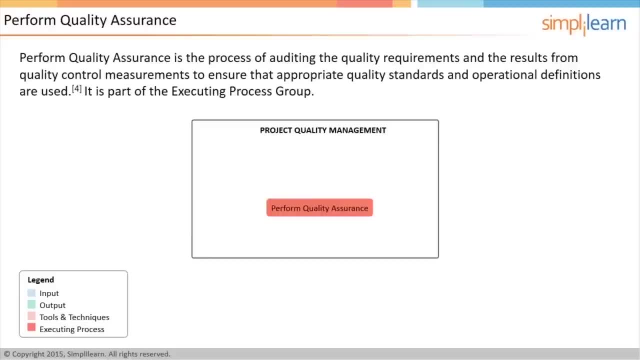 which involves determining whether the standards are being met and the processes are being followed. Therefore, the input for this process is the work that has been completed during the quality planning stage. They are project documents, quality management plan process improvement plan, quality metrics and quality. 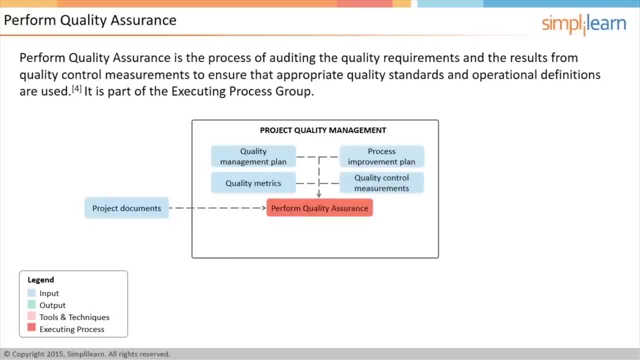 control measurements. Let us look at the tools and techniques used in this process. Quality audit is the process to check whether the project is complying with the organization standards and procedures and determine whether these policies, standards and procedures used are efficient and effective. So a good audit not only looks at 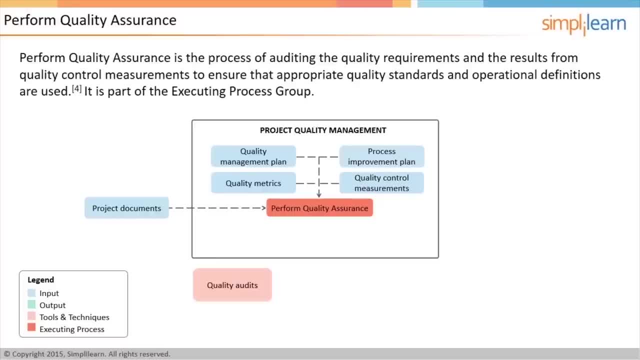 this compliance, but also for the new lessons learned from the current project that can help make the future projects better. Process analysis involves using the lessons learned from doing the initial few work to make the remaining work more efficient, For example, if the project involves installing a software. 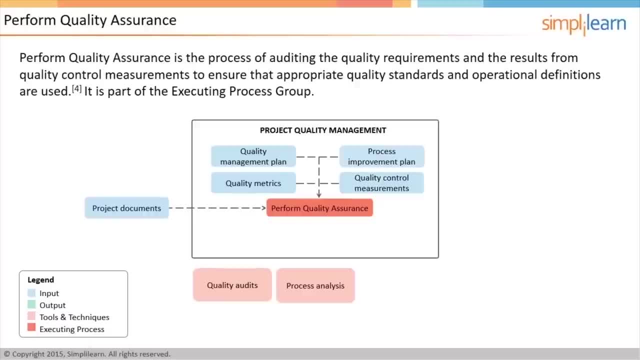 package. then the lesson learned from the first few installations can be used to improve the process on remaining installations. Apart from these, all the quality management and control tools, such as the seven basic quality tools, will be relevant to this process, The key output of this process. 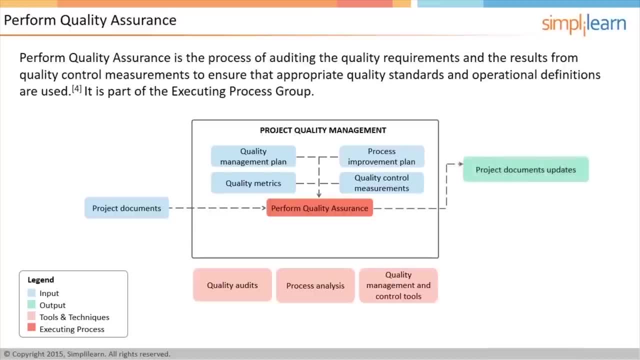 is project documents updates to ensure that if there is any deviation from agreed standards, it is corrected. Also, if there are any lessons learned that can help improve the future projects, the organization process assets get updated. This quality assurance may result in improvement suggestions, change requests. 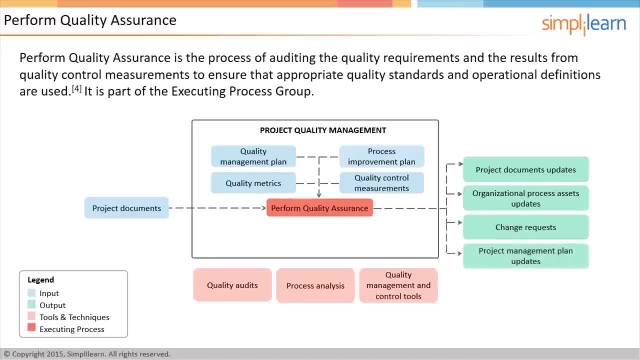 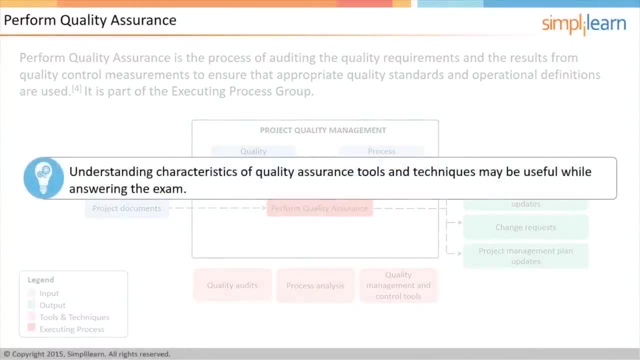 may be generated and the project management plan may need to be updated. Understanding characteristics of quality assurance tools and techniques may be useful while answering the exam, so prepare this topic well before you take the exam In the next screen. let us discuss the last process of 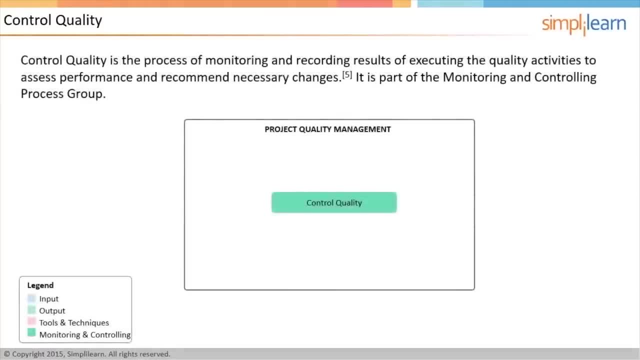 quality management. The key focus of the quality control activities is on the correctness of the work. Quality control helps answer questions like: is everything okay with the project? Does the project plan require changes to successfully execute the project? Will the project succeed, Etc. Let us 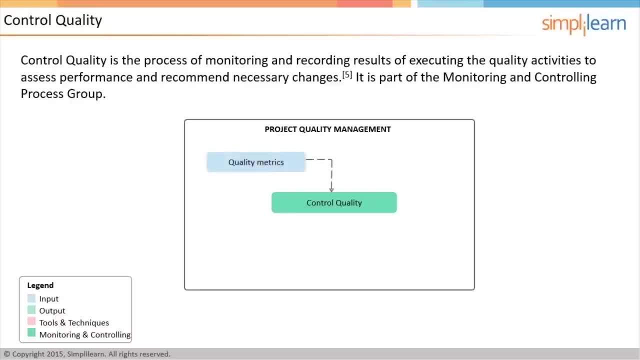 look at the inputs to this process. The quality metrics. measurements are done continuously to see whether the project quality is improving. The project deliverables are inspected against the planned checklists. Quality control acts upon the deliverables and work performance data produced in execution. 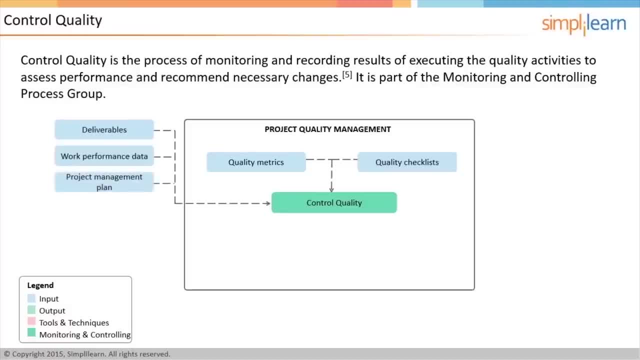 It also refers to the project management plan for understanding deviations from the plan. It also considers the approved change, requests, information from other project documents and organizational process assets. There are seven popular tools and techniques used in doing the quality control activities. They are collectively known as: 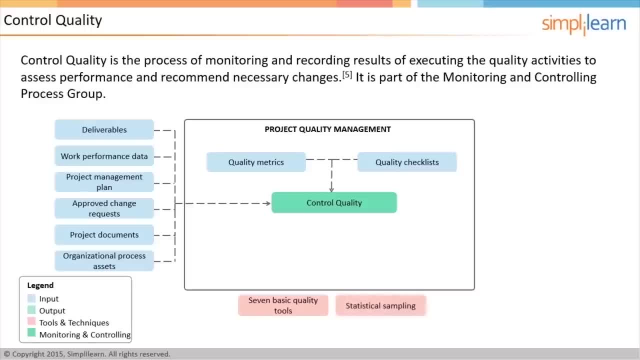 seven basic tools of quality. Other relevant tools are statistical sampling, inspection or testing and review of the approved changes. Quality control activities result in quality control measurements. the verified deliverables. validated changes. information about the work being performed. recommended changes. 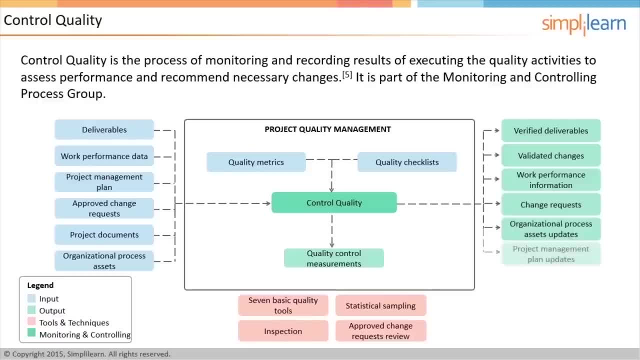 and updates to the organizational process, assets, project management plan and other project documents. In the next screen, let us look into a business scenario to understand this concept better. After reading the problem statement, click the solution button to look at a possible answer. 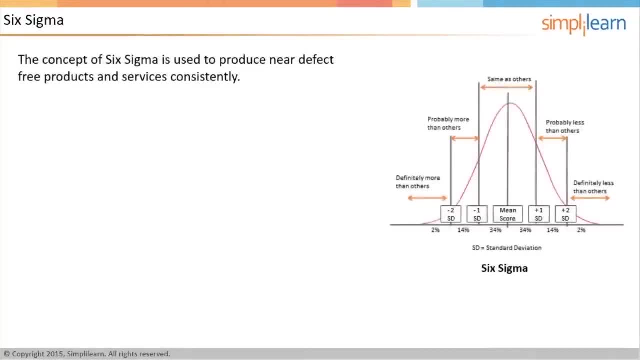 Six Sigma is a highly disciplined process that focuses on developing and delivering near-perfect products and services consistently. If large volume of data is plotted over a period of time, you would most probably have a bell-shaped graph. Such graphs are also called normal distribution graph. 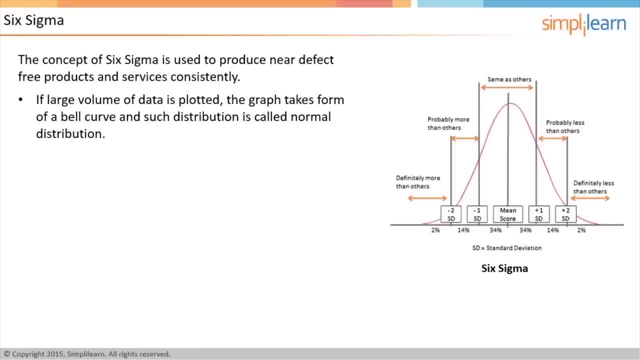 It's called as normal distribution because any large volume of data is plotted with the intent to track variations would most probably be in a bell-shaped curve. The line corresponding to the top of the bell curve is the median of the data sample. Standard deviation concept is used. 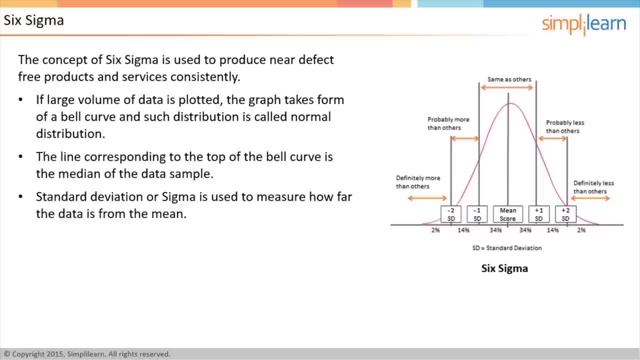 to measure how far any data is from the mean. Standard deviation is also called Sigma. One standard deviation from the mean covers 68% of the data. Six Sigma means six standard deviations from the mean. This would cover 99.99966%. 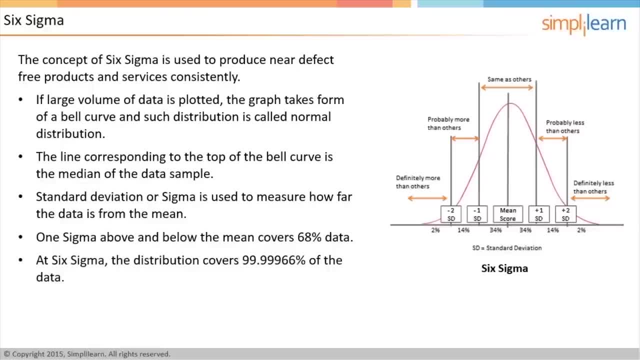 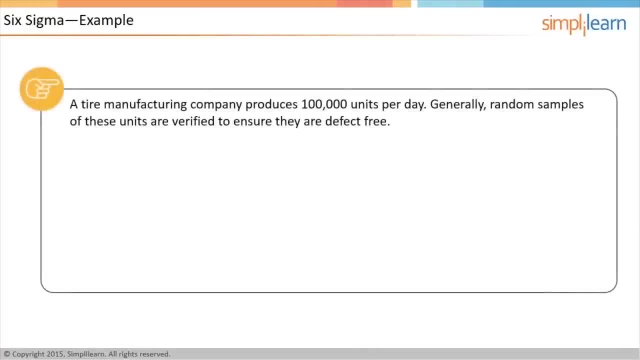 of the data. We will look at an example of Six Sigma in the following screen. To understand Six Sigma, let us look at an example. A tire manufacturing company produces 100,000 tires a day. It is not possible to verify each and every tire. 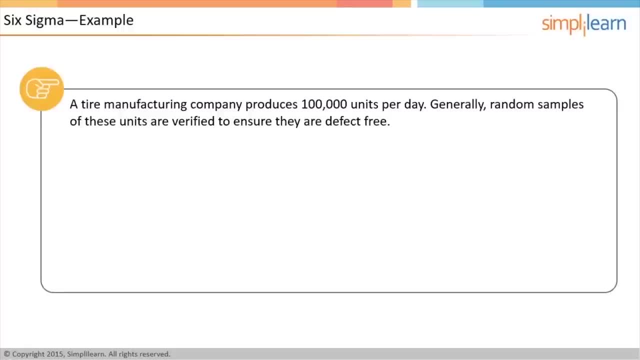 manually to ensure it is defect-free. Instead, random sample of these manufactured tires are taken and checked for defects. Assuming that the thickness of the tires is a parameter to measure defect: any tire that has a thickness more than or less than 10 millimeters. 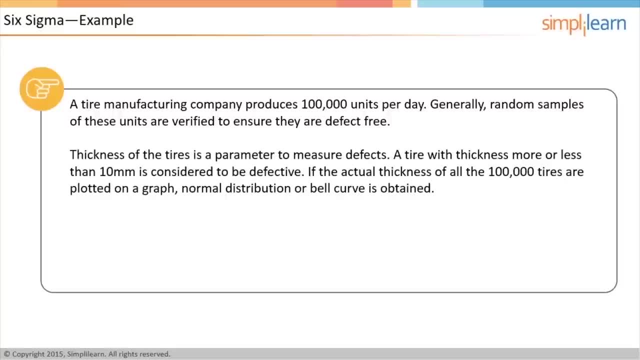 is considered to be defective. Now, if you measure the actual thickness of all 100,000 tires manufactured daily and plot them on a graph, you get a normal distribution graph One: standard deviation from the mean covers 68% of the data Meaning. 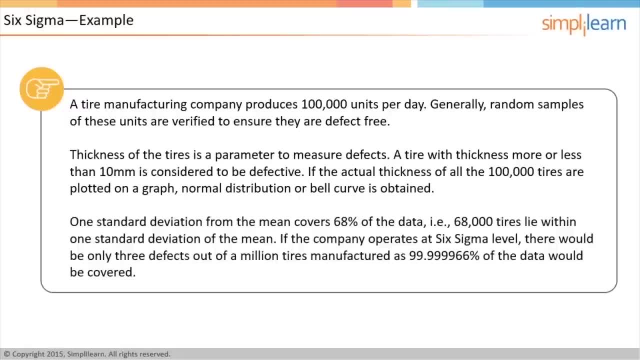 if the thickness of the 100,000 tires are plotted, 68,000 of them lie within one standard deviation above or below the mean. Now, if a company operates at Six Sigma level, they would ensure that all tires that are up to six standard deviations. 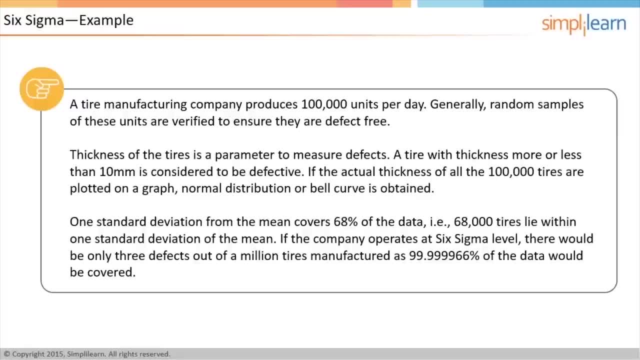 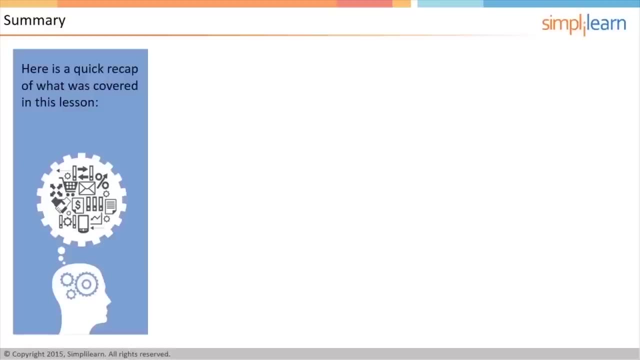 from the mean are defect-free. Therefore, in such cases, you can expect only three defective tires out of a million tires manufactured. Let us now check your understanding of the topics covered in this lesson. Here is a quick recap of what was covered in this lesson. 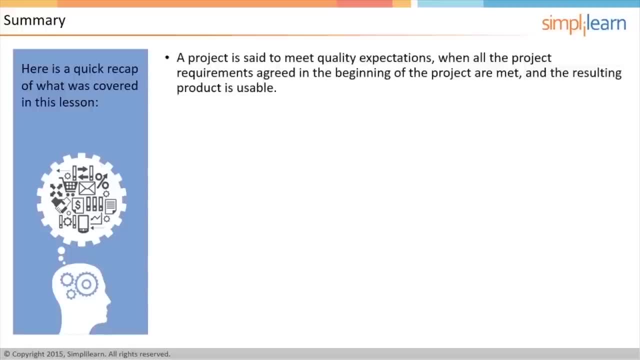 A project is said to meet quality expectations when all the project requirements agreed in the beginning of the project are met and the resulting product is usable. Quality management includes creating and following policies and procedures that meet the project's defined quality needs. Quality planning defines the standards. 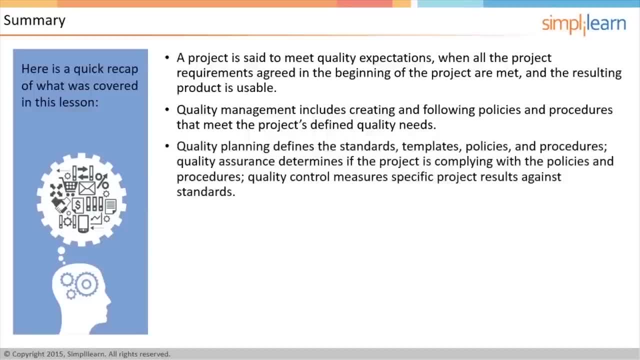 templates, policies and procedures. Quality assurance determines if the project is complying with the policies and procedures. Quality control measures specific project results against standards. Plan quality management, perform quality assurance and control. quality are the three project management processes. Seven basic quality: 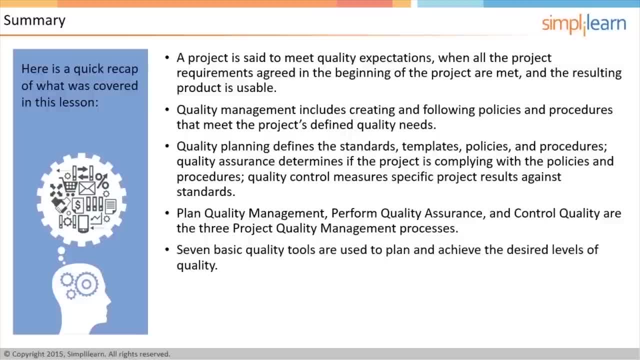 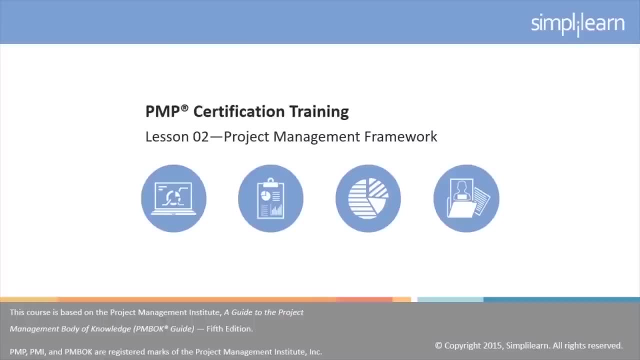 tools are used to plan and achieve the desired levels of quality. At Six Sigma level, there would be only three defects out of a million units manufactured. In this lesson we will focus on project management framework. Let us begin with the objectives of this lesson. 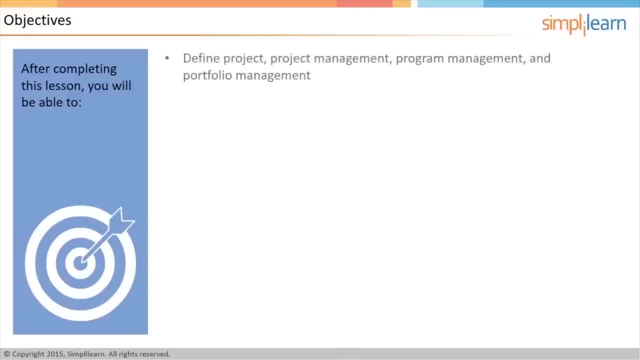 After completing this lesson, you will be able to define project project management, program management and portfolio management. Recognize the roles of project management office. Identify the project constraints and their impact on the project. Explain the role of a project manager in stakeholder management. 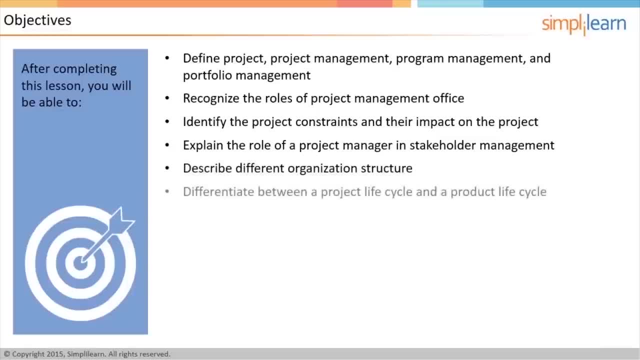 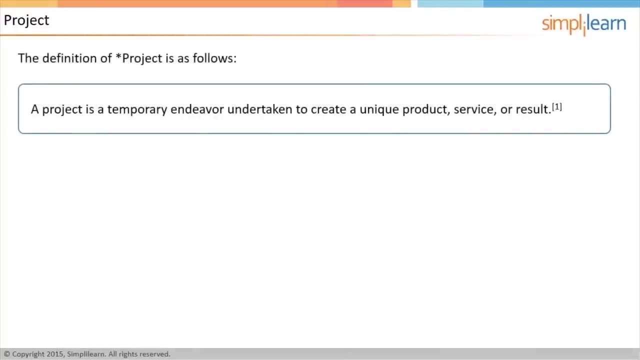 Describe different organization structure, Differentiate between a project life cycle and a product life cycle. Let us begin this lesson with understanding what a project is in the next screen. A project is a temporary endeavor undertaken to create a unique product, service or result, For example, developing. 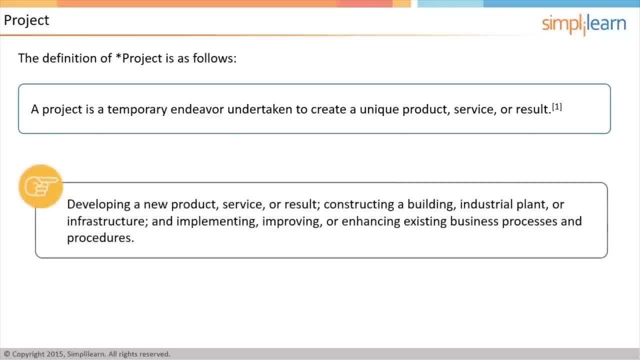 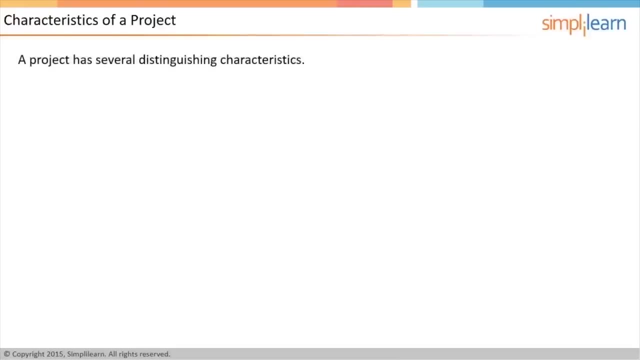 a new product, service or result, constructing a building, industrial plant or infrastructure. and implementing, improving or enhancing existing business processes and procedures. In the next screen, we will focus on the characteristics of a project. A project can be distinguished based on its 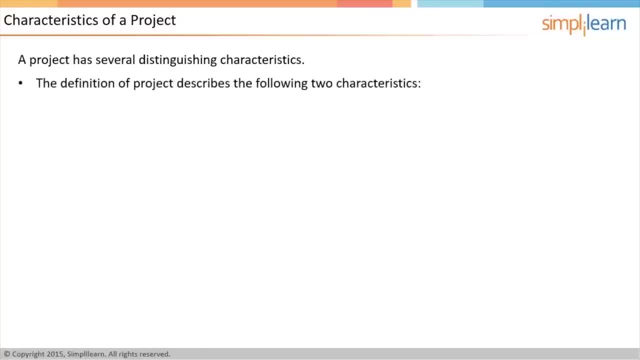 characteristics. The definition describes two characteristics of a project. First, it is temporary in nature. Temporary here does not mean short in duration. A project can extend for long duration based on the requirements, For example creating a new indigenous missile defense system for a country. However, 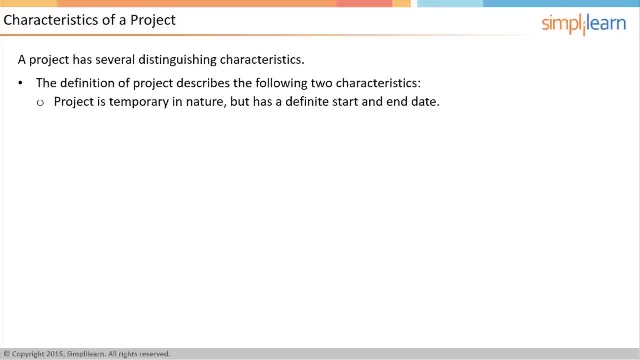 there is always a definite planned start and end date for a project. It cannot go on indefinitely. Secondly, the project is supposed to produce a unique output. The output could be a product, service or result. There can be many common activities between two projects, but the outcome. 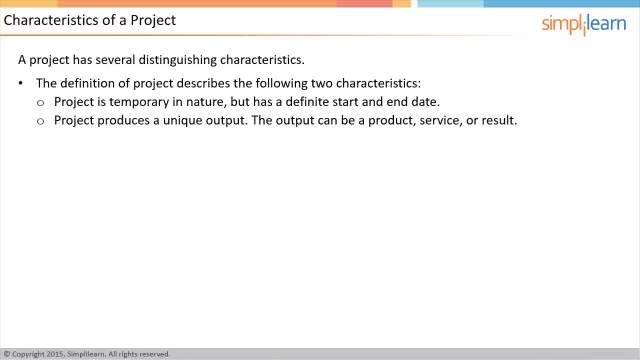 of each project should be unique in some way or the other. Now let us look at what marks the end of a project. A project ends when either the objectives are met or the project is terminated because the objectives will not or cannot be met. 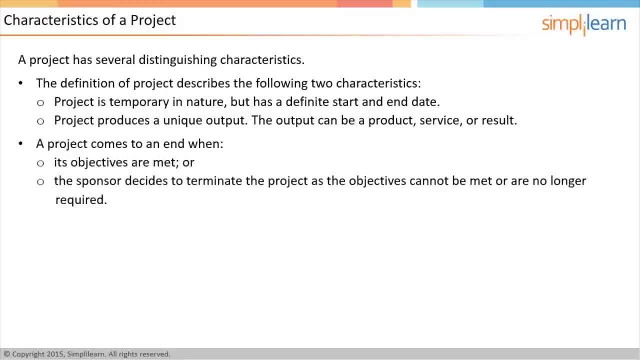 The other reason to terminate the project can be that the need for the output of the project does not exist anymore. Usually, the sponsor of the project takes a call about the closure of the project. It is important to differentiate project work from regular operational work. 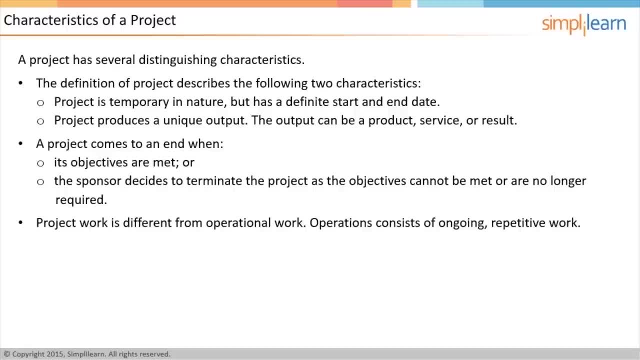 For example, your office receptionist does the same work every day of picking any incoming call and directing the call to the right person in the office. This is an ongoing repetitive work and can be classified as operation. Operations, unlike projects, are neither temporary nor 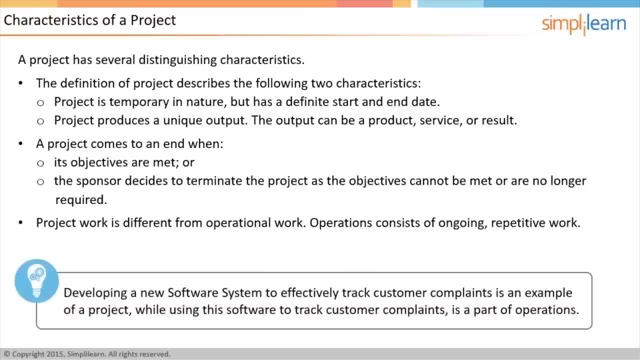 unique. Creating a new software system to effectively track your customer complaint can be an example of a project. When the software is successfully developed, the project objective is met, which marks the end of the project. When you start using this software to track customer complaints, you are entering: 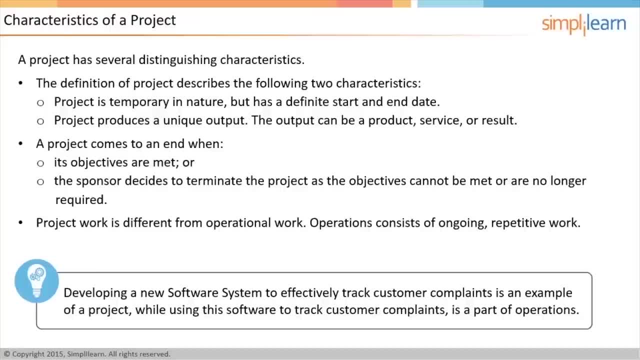 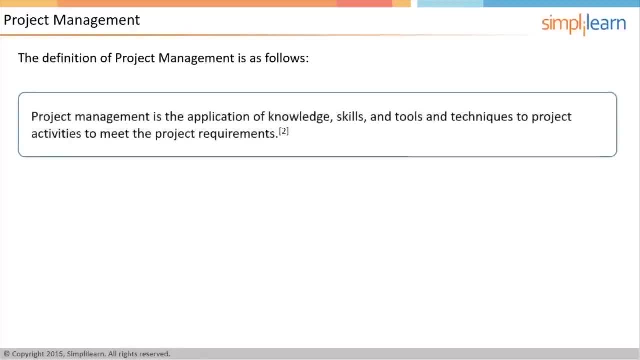 into the operations phase In the next screen. let us now look into project management. As defined in the PMBOK guide, project management is the application of knowledge, skills and tools and techniques applied to project activities to meet the project requirements. 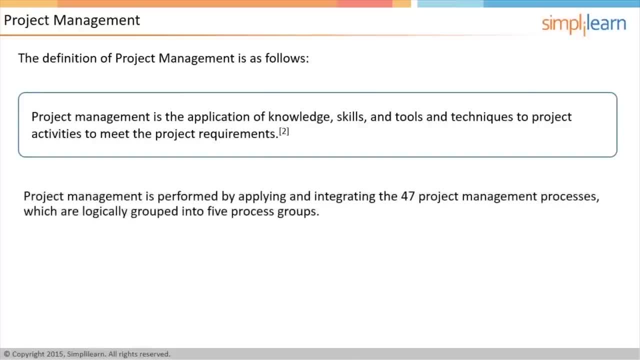 Project management is achieved by proper application and integration of the 47 processes. Project application and integration means these processes should be executed in the right manner, as well as in the right order. In the next screen, let us discuss how to make and manage a project. 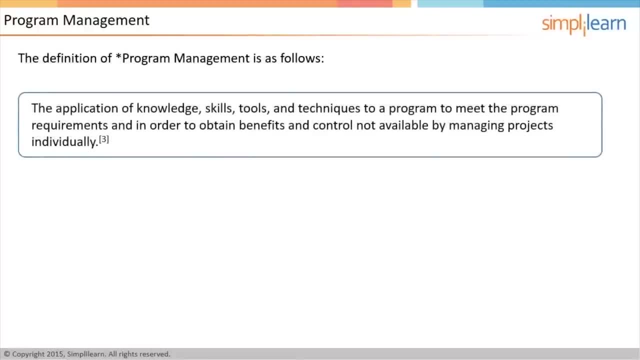 Program management is defined as the application of knowledge, skills, tools and techniques to a program to meet the program requirements and to obtain benefits and control not available by managing projects individually. As defined in PMBOK guide, a program is a group of related 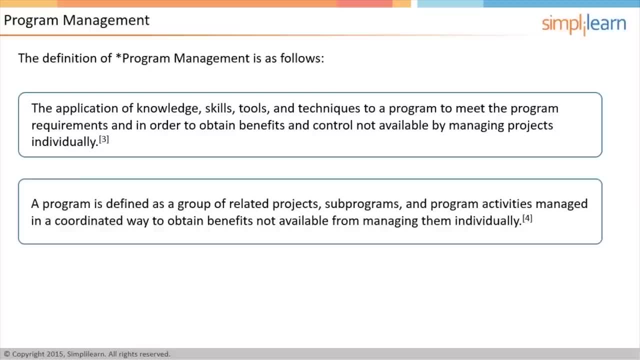 projects which, when managed as a group in a coordinated fashion, provides benefits and control that are not available while managing them individually. These benefits could be from decreased risk, economies of scale, improved management of dependencies, delivery of additional capabilities, optimal utilization of. 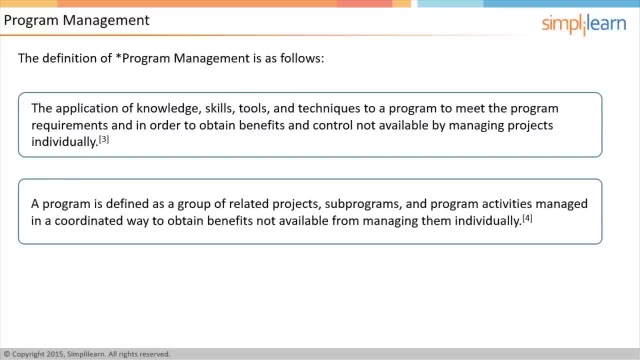 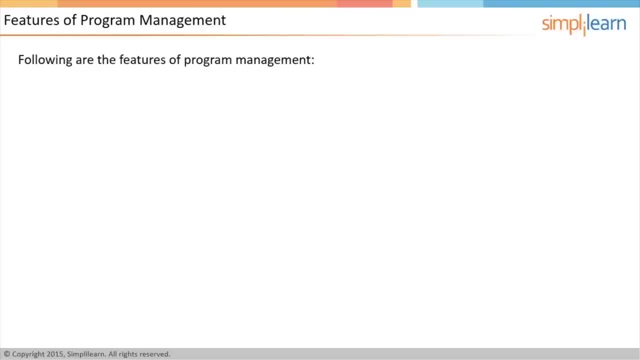 shared resources and so on. Let us now learn the various features of program management. Random projects cannot be grouped together as a program. The projects in a program should be related in some way or the other and there should be some value added in managing. 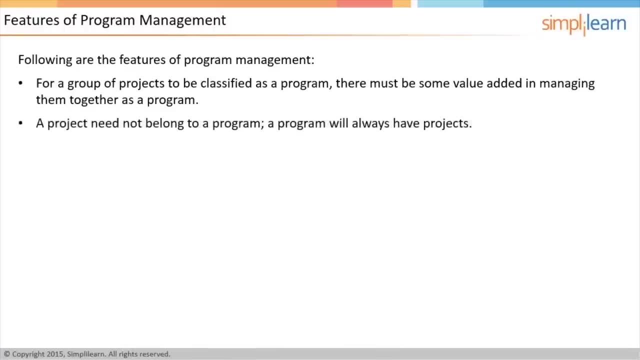 them together. A project may not be a part of any program, but a program will always have projects. A project can also be executed as a standalone project. A program is designed to deliver some strategic benefits value to the organization. These benefits can be tangible or 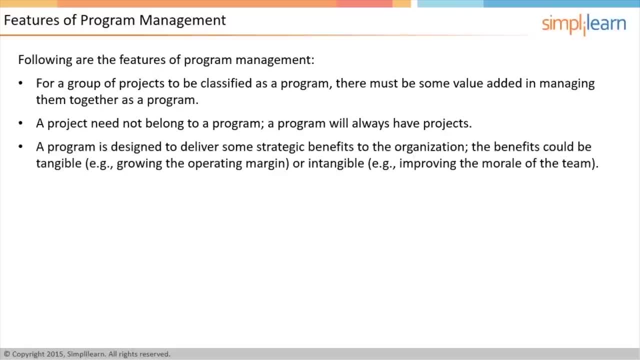 intangible. Examples of tangible benefit could be increased profit margins or operational cost savings. Examples of intangible benefits could be improved team morale or building up certain competencies, While a project manager focuses relentlessly on the fulfillment of the project's requirements, that is, scope, cost, time. 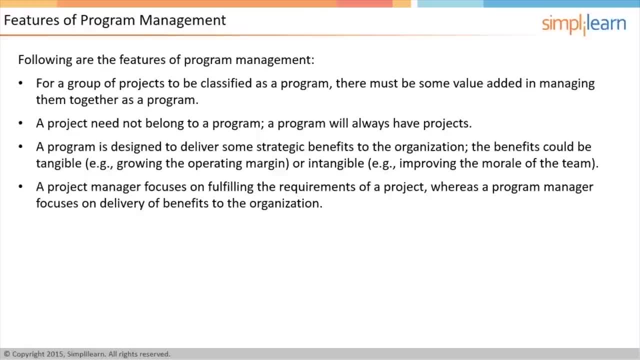 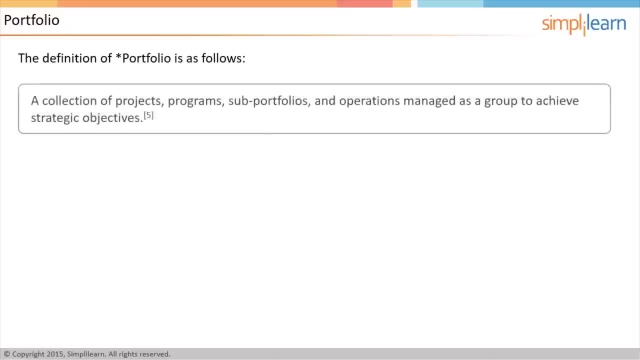 quality. a program manager needs to focus on ensuring that the organizational benefits are realized. In the next screen, let us understand what a portfolio is. Portfolio is yet another term used, along with project and program. A portfolio may have multiple projects and programs that are managed as a. 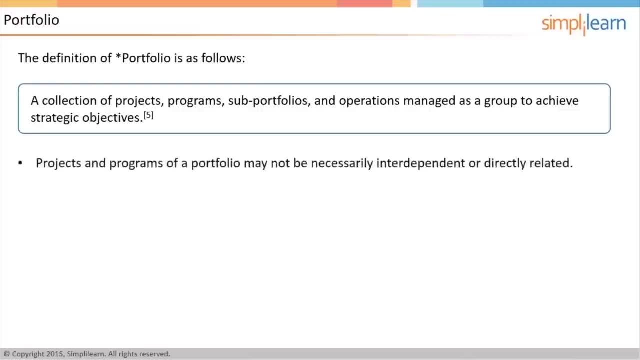 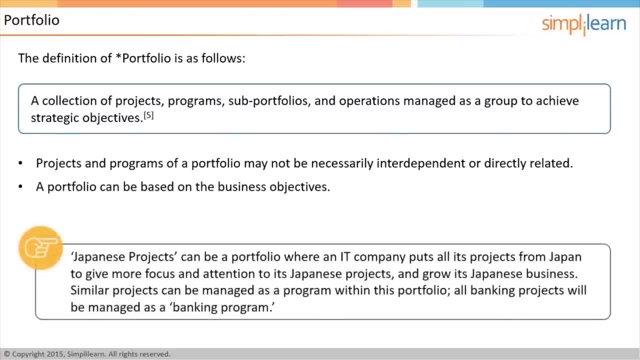 group to achieve strategic objectives. Note that all projects and programs in a portfolio may not be necessarily interdependent or directly related. A portfolio can be created based on the business objectives. For example, an IT service company can have a portfolio named Japanese projects, which is 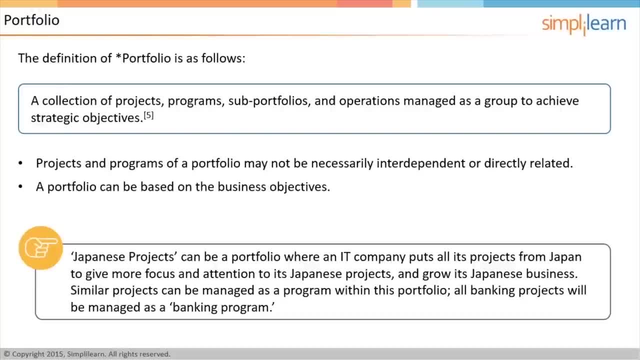 formed with an aim to take over the Japanese market by giving more attention to these projects. Within this portfolio, similar projects can be managed as a program and all banking projects from Japan can be managed as a banking program In the next screen. let us 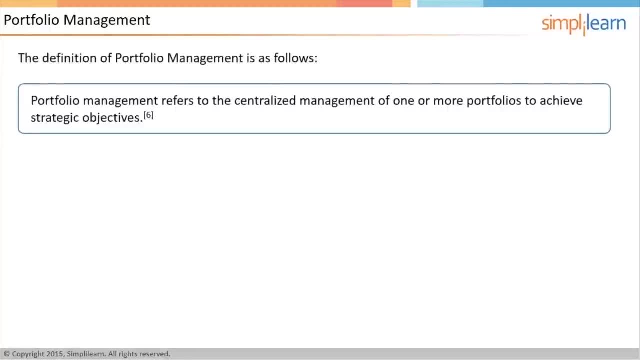 discuss portfolio management. Portfolio management is the centralized management of one or more portfolios. This includes identifying, prioritizing, authorizing, managing and controlling projects, programs and other related work to achieve strategic business objectives. Therefore, whether the company should have Japanese projects as. 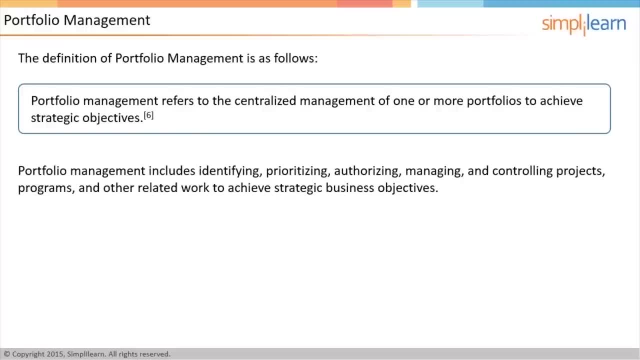 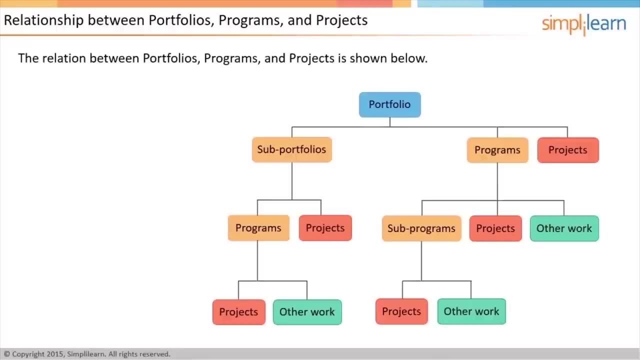 portfolio or not is decided by portfolio management. In the next screen, let us understand the relationship between portfolios, programs and projects. The image on the screen will help you to understand the terms: portfolios, programs and projects. A portfolio is part of an. 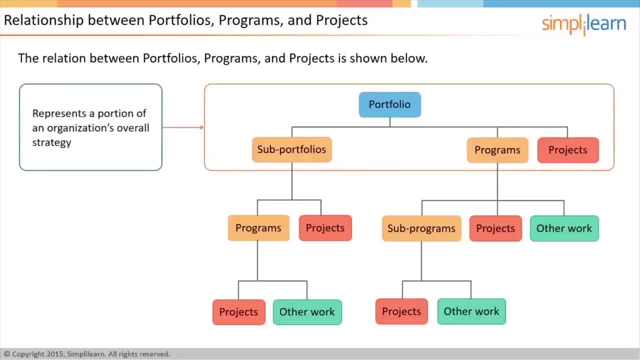 organization's overall strategy. It represents a conscious decision by an organization to invest in the portfolio. The overall objectives of a portfolio are then cascaded down to the lower level components. The components could be sub-portfolios, programs or projects. These components can further be. 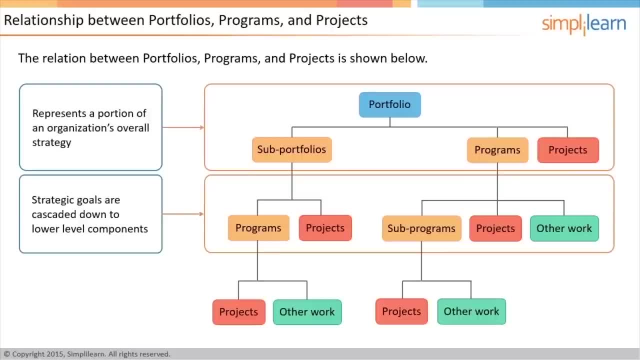 broken down into smaller components for ease of management. Although a project may not contain operations, a program or a portfolio, it can include other work. This other work may comprise training and development, customer support and services, etc. If the other work has synergy with. 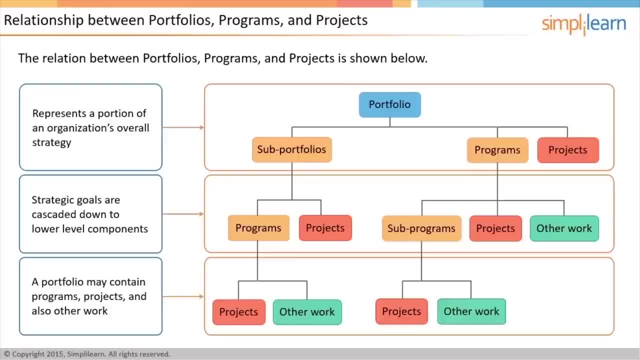 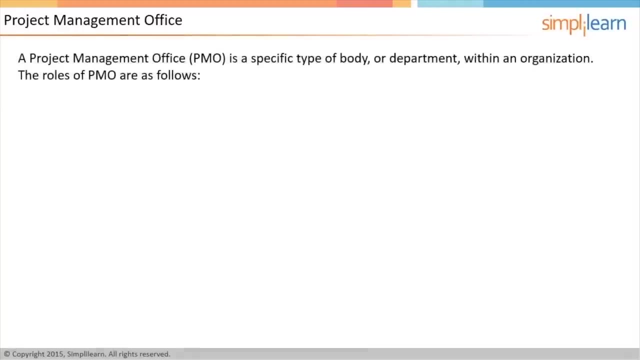 the overall objectives and adds to the capability to deliver the higher level benefits, then it can be included in the program or portfolio as well. In the next screen we will discuss project management office. Project management office or PMO, is a specific 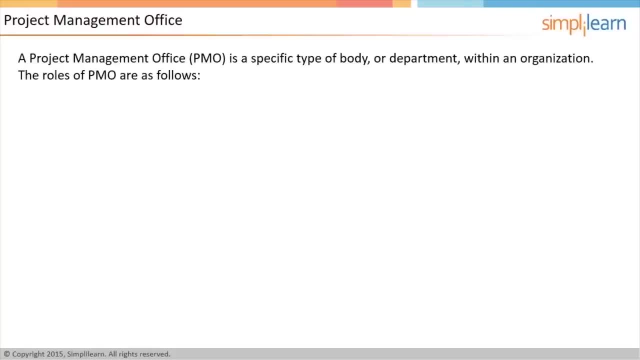 type of body or department within an organization. PMO performs several roles in the organization and these can broadly be classified as primary roles and other roles. Typically, the PMO may take up any one or a combination of the three primary roles It provides. 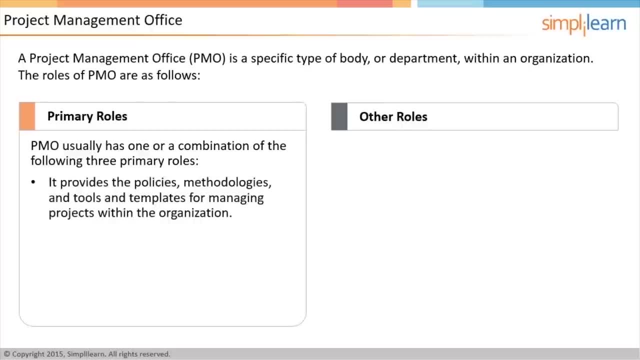 the policies, methodologies and tools and templates for managing projects within the organization. It provides support and training in organization on how to manage projects and, finally, it provides project managers for different ongoing projects in the organization. PMO may also help in managing interdependencies. 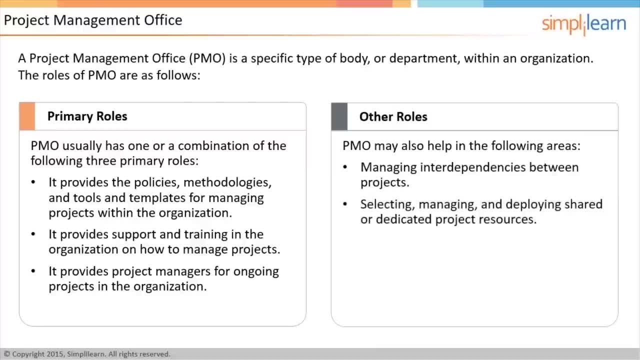 between the projects, selecting, managing and deploying shared or dedicated project resources, if need be, terminating a project and organizing lessons learnt sessions and maintaining the project management knowledge base for an organization. In the next screen, we will discuss how to manage the 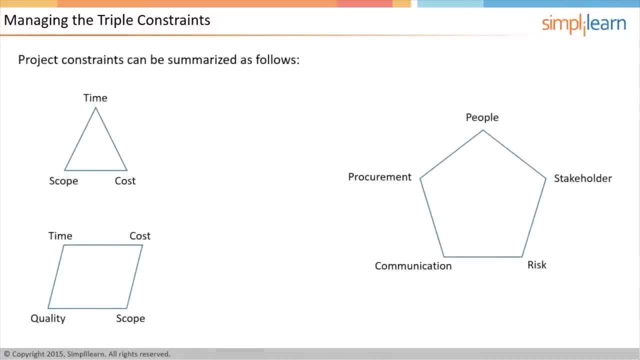 triple constraints. Any project can be done successfully if there is no constraint on time or there is unlimited budget available. Unfortunately, that is not true in real life. A project is performed within some constraint and these constraints are usually competing. Therefore, if you change one, 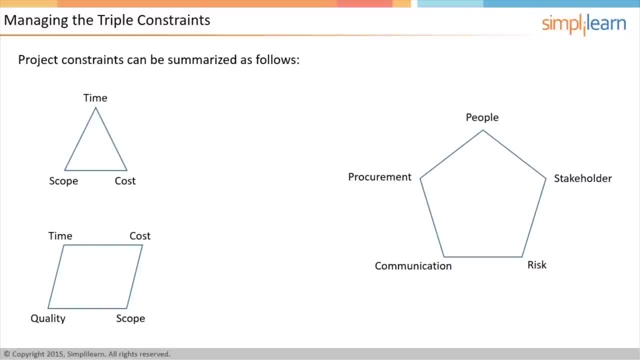 it would affect the other. For example, if the project duration increases, it would lead to increase in the project cost as well. Triple constraint is a term that originally referred to the three competing project constraints within which the projects are performed. These constraints are cost time. 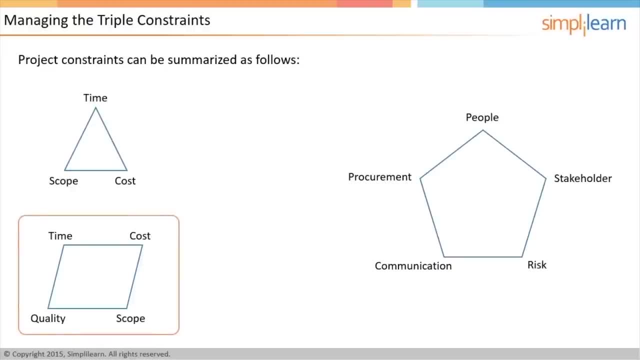 and scope Quality is a primary concern for a project manager. Therefore, the project manager has to make trade-offs to keep the scope, cost, time, quality plane in balance. To achieve the balance, the project manager also needs to manage other aspects of the project, For instance, 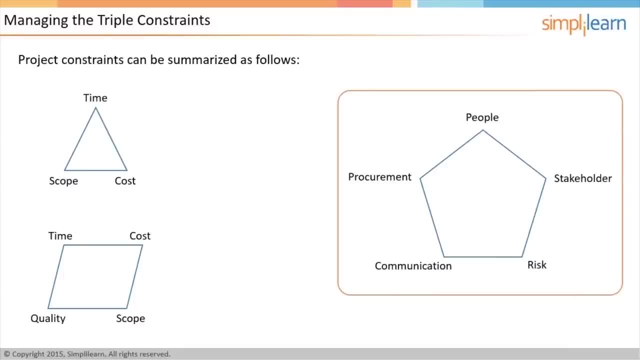 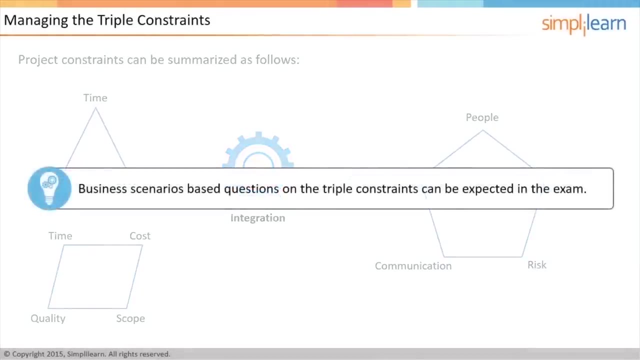 the people, stakeholders, risks, communication and procurements. The project manager plays the essential role of integrating all these different aspects of project management. In the PMP examination, you can expect business scenario-based questions focusing on the triple constraints In the next screen. 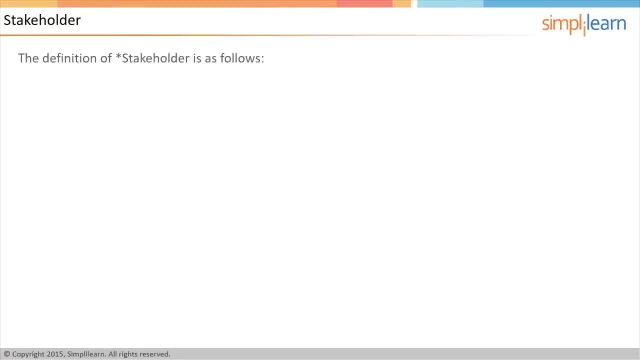 let us understand who a stakeholder is. A stakeholder can be defined as the one whose interests may positively or negatively be affected, or perceived to be affected, by the decision, activity or outcome of the project. As per the definition, the project team, project manager, project. 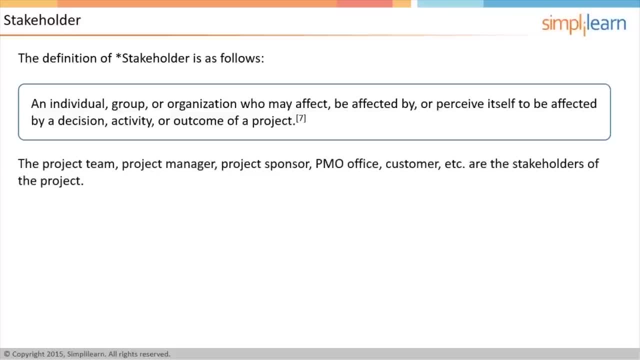 sponsor, PMO office, customer, etc. are the stakeholders of the project. A project sponsor is the one who gives a go-ahead for a project and provides the necessary resources to execute the project. Therefore, the head of projects in the organization who provides a green signal to. 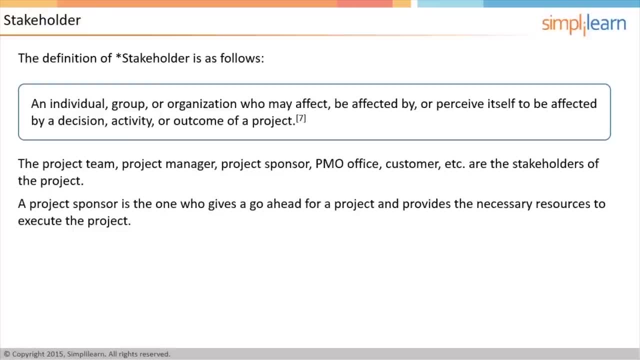 start a project and allocates required resources to the project is the project sponsor. A project sponsor is usually somebody placed high up in the organizational hierarchy of the performing organization, that is, the organization in which the work of the project is being carried out. 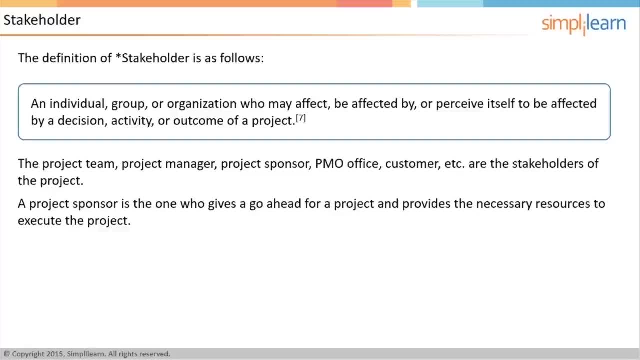 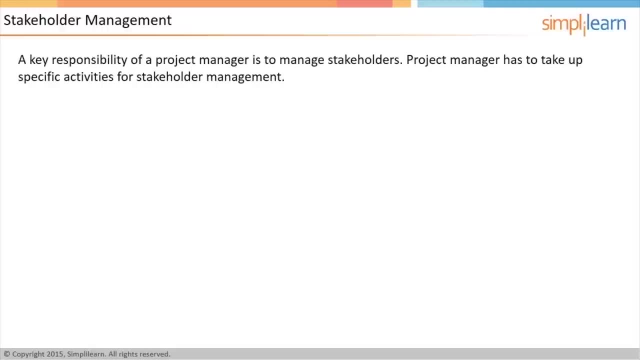 In the next screen. let us look at stakeholder management. One of the key responsibilities of a project manager is to manage stakeholders. A project manager has to involve the stakeholders from the beginning of the project until the end, so they are aware of every step. 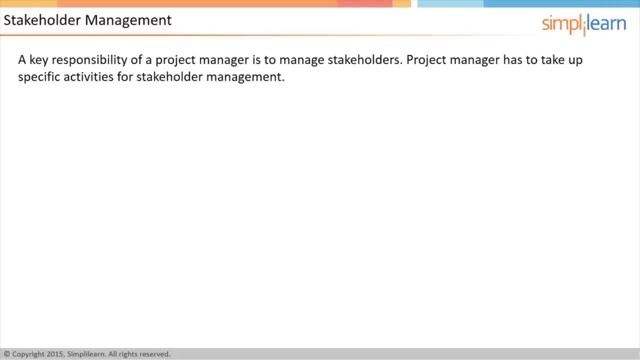 A project manager has to take up specific activities for stakeholder management, Identifying both internal and external stakeholders. Missing out any stakeholder can be disastrous for a project. A stakeholder who has identified towards the end of the project may come up with his own requirement at 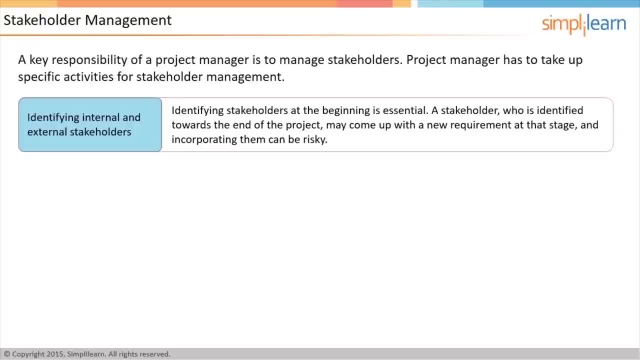 that stage and incorporating them can be risky. Determining stakeholder requirements: After identifying all the stakeholders, the project manager also needs to ensure that their requirements are clearly identified. Sometimes stakeholders might themselves not know of their requirement, and it is the job of the project. 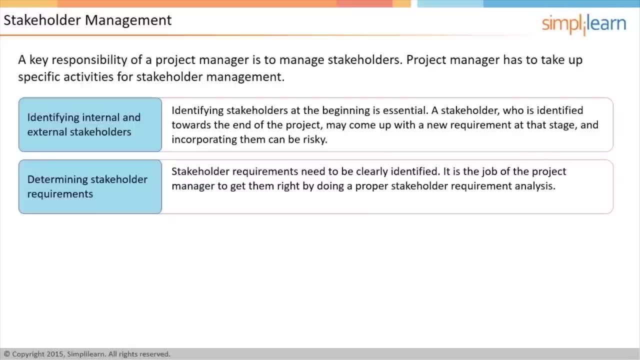 manager to get them right by doing a proper stakeholder requirement analysis, Determining stakeholder expectations. Stakeholders might also have some unstated expectations which need to be clarified to see if it can become a project requirement. It is again the role of the project manager to 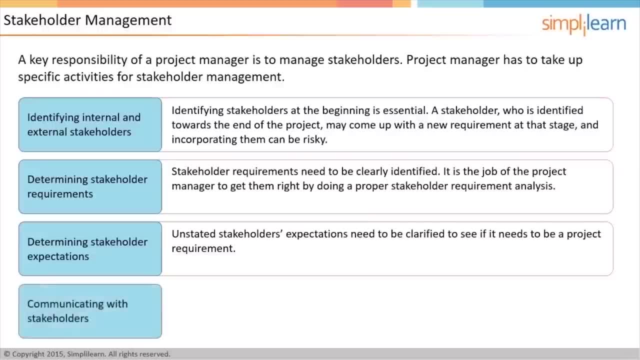 determine the stakeholders' expectation: Communicating with stakeholders. Once all the stated and unstated stakeholder requirements are known, the project manager, as part of stakeholder analysis, should focus on communicating them regularly to keep stakeholders involved in the project. Once you understand, 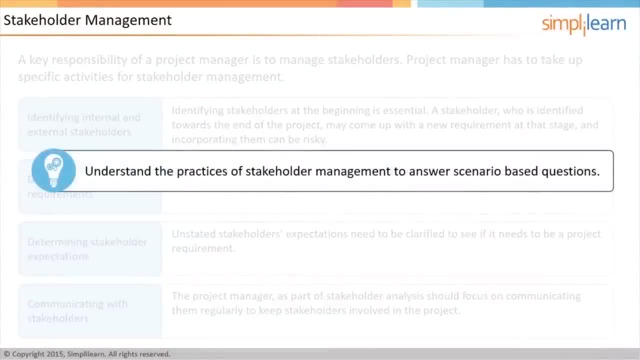 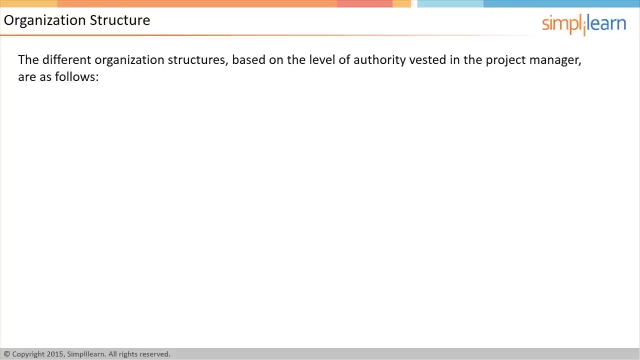 the practices of stakeholder management. it will be easier for you to answer scenario-based questions in the examination In the next screen. let us look at the various organization structure. Projects are performed in an organization and the functioning of the organization might affect the project. 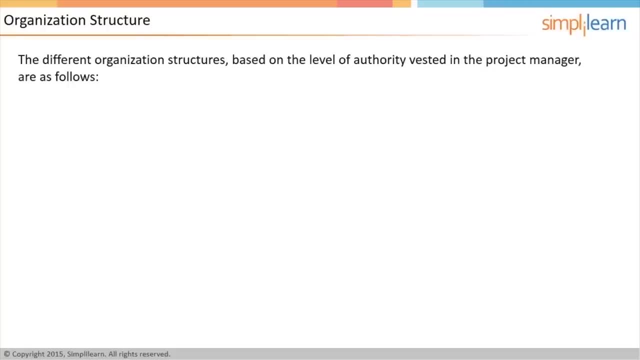 The different organization structure types explained here are based on the level of authority that a project manager gets into in those organizations. In a functional type of organization, the organization is grouped by the area of specialization within different functional areas, For instance marketing, accounting, engineering, etc. 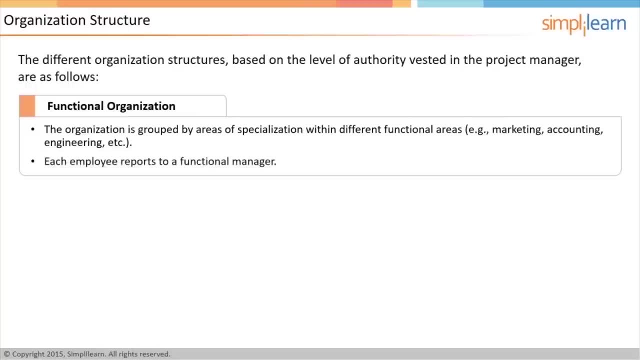 are departments within the organization. Each employee typically reports to a functional manager. In such types of organization, normally projects are undertaken within the department itself. If a project requires any assistance from another department, the request moves from the head of the requesting department to the head of the concerned. 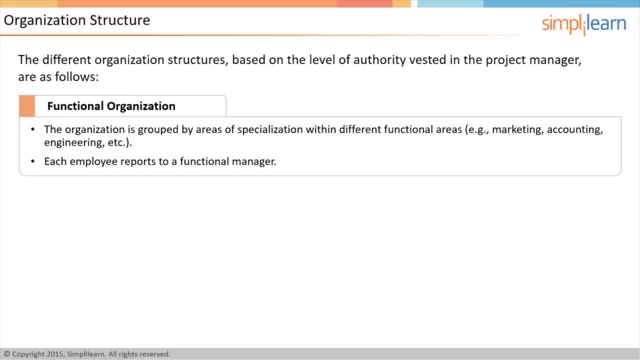 department. The team members do their normal departmental work in addition to the project work. The next type of organization is projectized organization. In such organizations there are no departments. The organization's resources mostly work on projects. Team members report to a project manager. 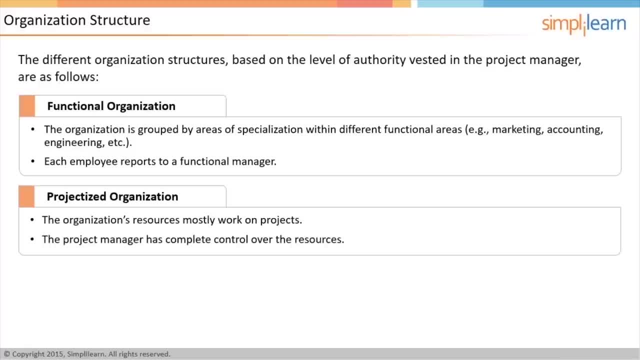 The project manager has complete control over the resources. When the project is completed, either they move on to another project or they look for some job outside the company. They do not have a department for themselves. The third type of organization is a matrix organization. 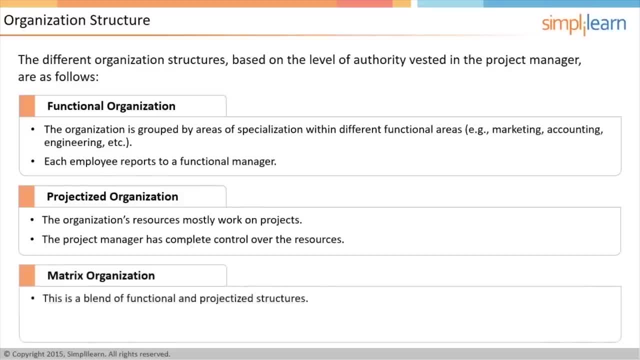 which is a blend of functional and projectized organizational structure. A team member belongs to a department as well as they are part of a project team. In such organization, team members have two bosses: one their department head and the second their project manager. 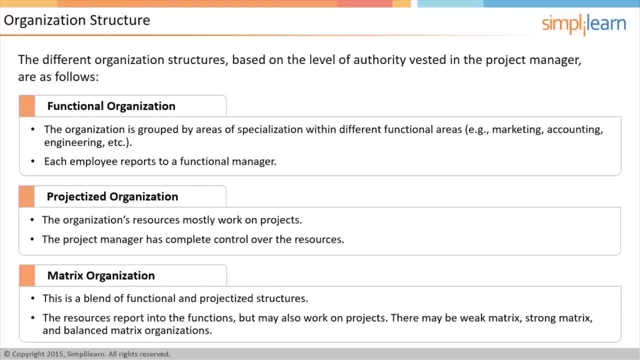 Since there are two bosses here, this type of organization is further classified into three different types. They are weak, strong and balanced matrix organization. So out of the two bosses that team members have in matrix organization, if the project manager has more, 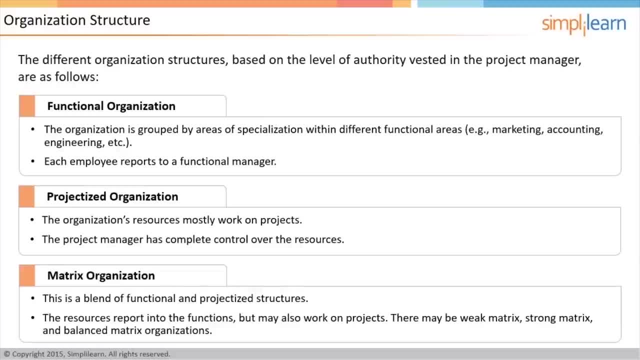 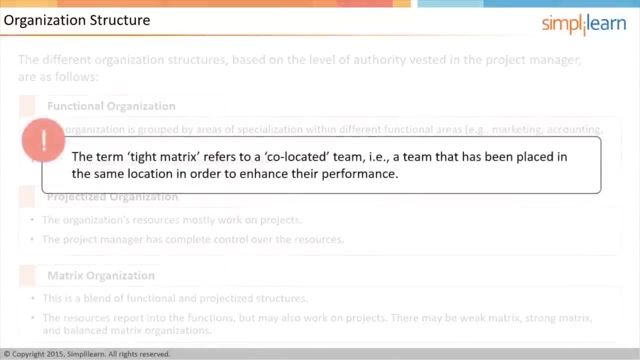 authority over the team member. such organizations are called strong matrix. Where the functional manager has more authority, it's a weak matrix organization. If they both share equal authority, then it is a balanced organization. There is another term that you might find in the exam, called 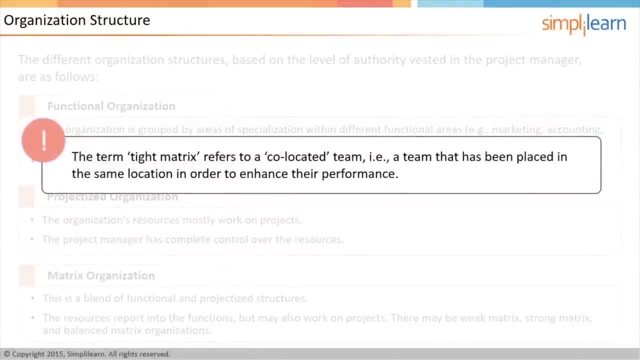 tight matrix. This generally refers to a co-located team, that is, a team that has been placed in the same location to enhance their performance In the PMP exam. if there is no mention of the organization type, you can assume it to be. 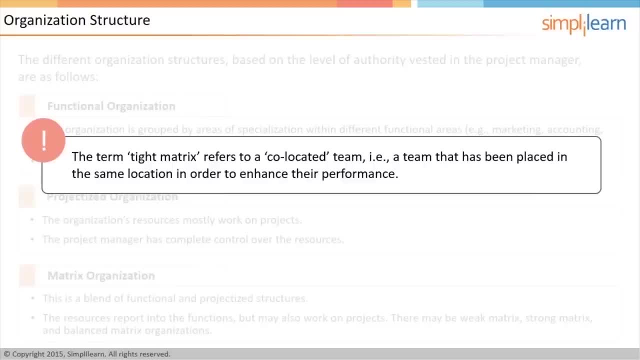 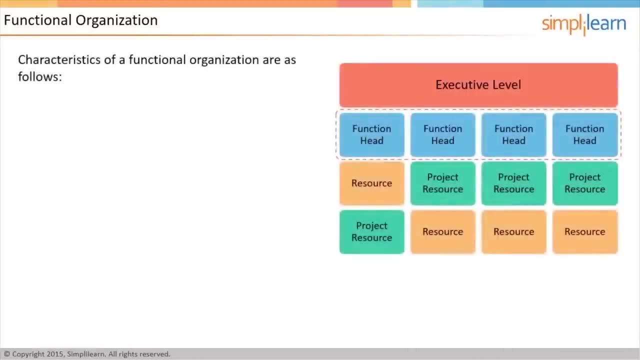 a matrix organization. Let us look at each of these organization structures in detail. In the next screen, let us look at functional organization. In a functional organization, the resources of the organization are grouped by functions, sometimes called departments. Examples of functions could be: 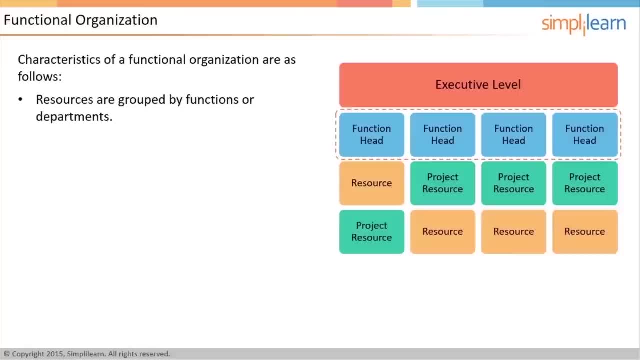 sales, finance, administration, manufacturing, etc. Each function plays a definite role in the organization and is headed by a functional head or supervisor. All the resources in such an organization report directly into their functions. Therefore a salesperson would report into the sales organizational hierarchy. 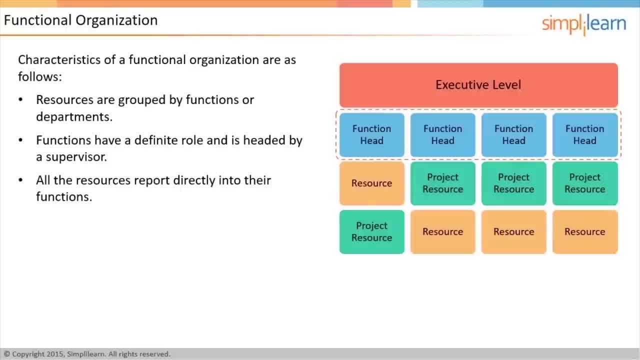 a purchase executive would report into procurement and so on. You would notice that in a functional organization, the project manager's role is not explicitly called out. When a functional organization embarks on a project, each of the functions that are involved may volunteer some resources to work. 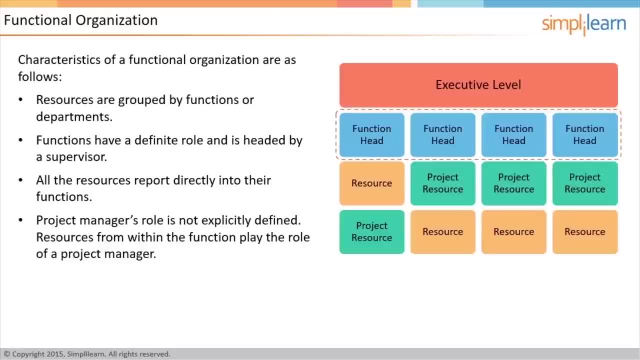 on the project, One of these resources may end up playing the project manager's role. The resource assignments may not even be full-time, and sometimes even the project manager is part-time, Since the project manager has no authority over any of the resources. 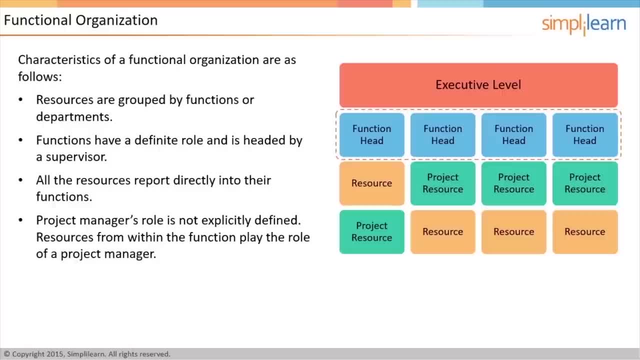 they are dependent on the functional heads. This makes it more challenging for the project manager to coordinate in the team. However, functional organizations provide an opportunity for specialization. For example, if a purchase executive was reporting into the purchase department, that executive would have exposure to all the 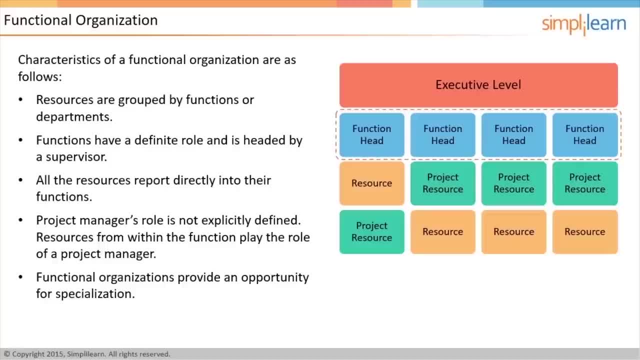 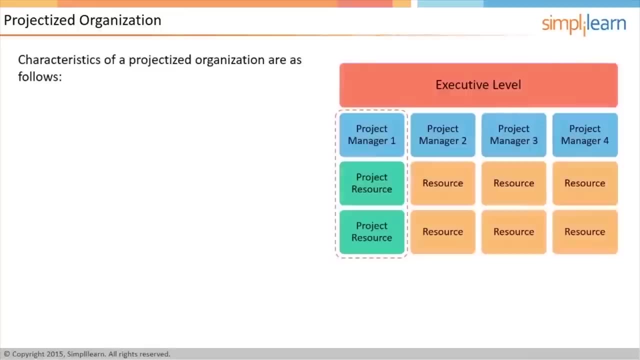 purchasing. that happens within the organization and has a well-defined career path. In functional organizations, project management happens at the functional head level. Next let us look at the projectized organization in the next screen. The projectized organization has all the resources aligned around. 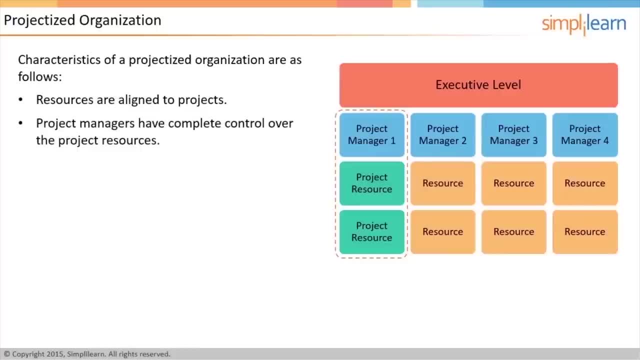 projects. The project managers have complete control over the resources working on their projects. The biggest advantage of the projectized organization is that the resources have loyalty to their projects and project execution becomes easier. This kind of structure is suitable for organizations whose work is in the nature of projects. 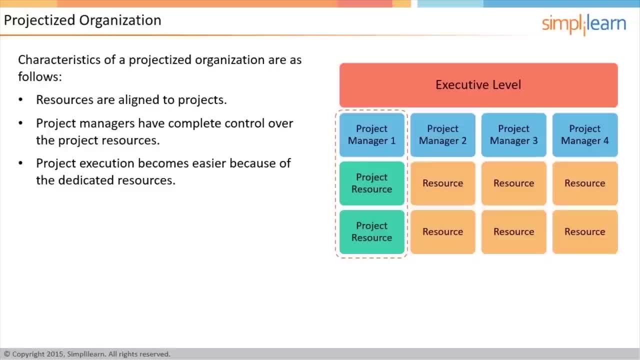 There are few disadvantages in this structure as well. Firstly, the role of the resource is over once the project is completed. Secondly, highly specialized roles within a project may not be fully occupied all the time. For example, a purchase executive may have work for selected periods. 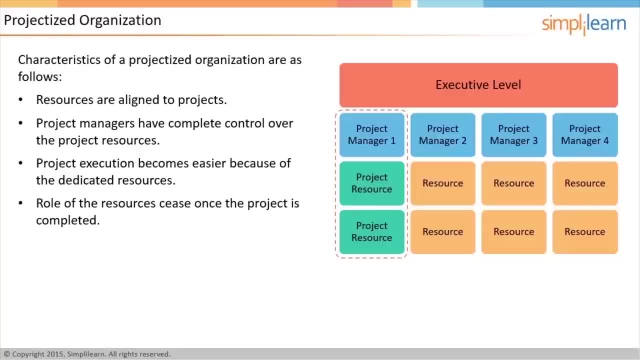 on a project while purchase activities are going on. However, for the rest of the period, their capability may not be optimally utilized. There is less scope for functional specialization, as the project boundaries limit the kind of work for the resources Each project manager is in charge. 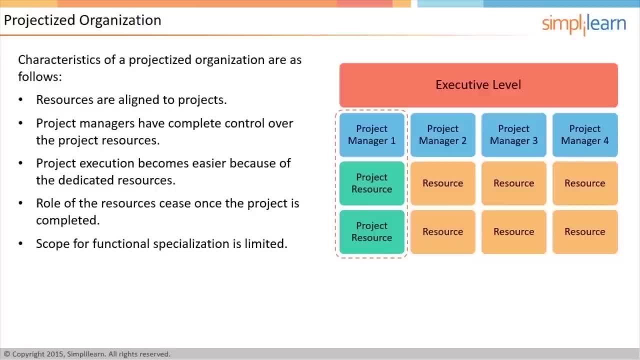 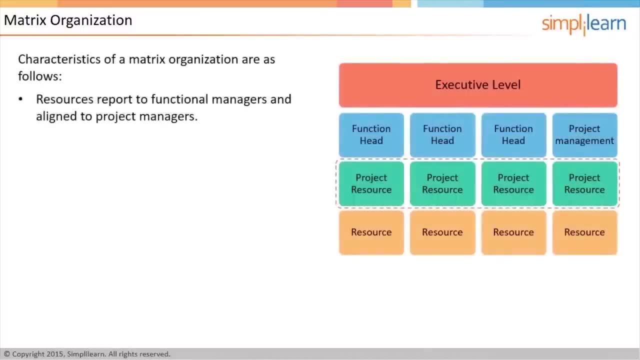 of a project and its resources. Next, let us look at the matrix organization. In a matrix organization, the resources report to the functional managers and are managed by the project managers as well. There might even be a function that represents all the project managers in the organization. 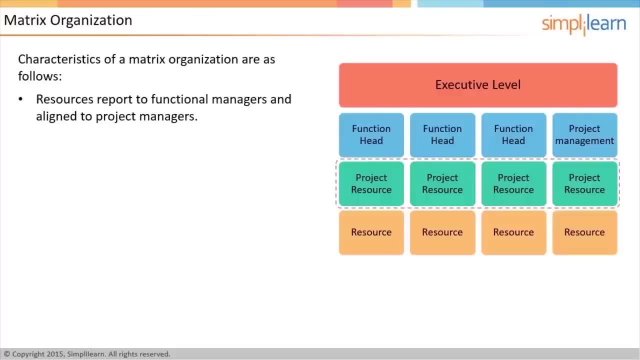 The matrix organization is a project manager that provides project management expertise. The matrix structure has three variants, commonly referred to as weak, balanced and strong. In a weak matrix, the authority of the project manager is the weakest and strongest. in a strong matrix, 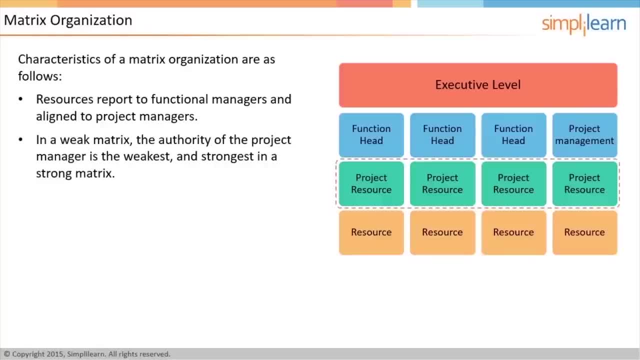 structure. The titles given to project managers in functional or weak matrix organizations are project expediter or project coordinator. They would be called project managers in a balanced or strong matrix structure and have slightly more authority over the time of the team members. The advantage of the matrix. 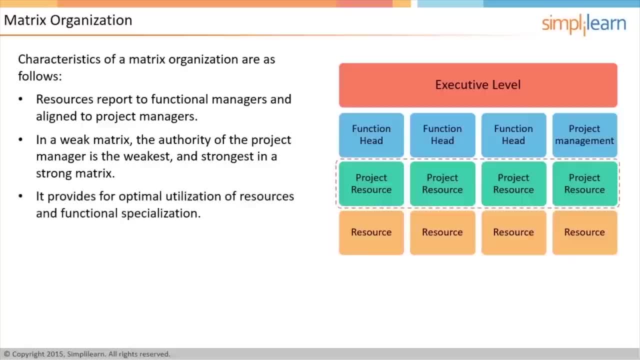 structure is that resources can be optimally utilized while preserving the capacity of the project managers to get projects executed efficiently. Resources can specialize in their functions and have stability in their careers, also contribute to the projects at the same time. potentially The disadvantage of matrix organization is that 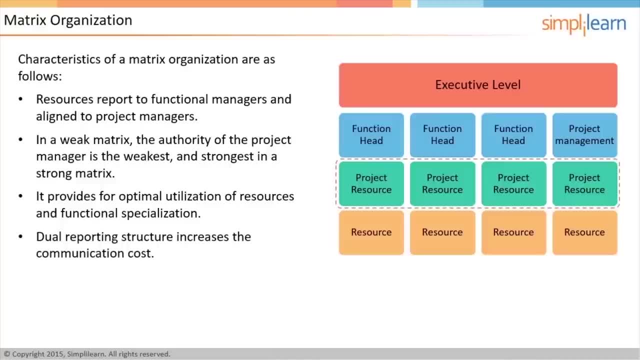 the communication overhead increases significantly. This is because every resource in the organization belongs into a project and into a function, leading to a dual reporting structure. In a matrix organization, project management happens at project resource level. In the next screen let us summarize the advantages. 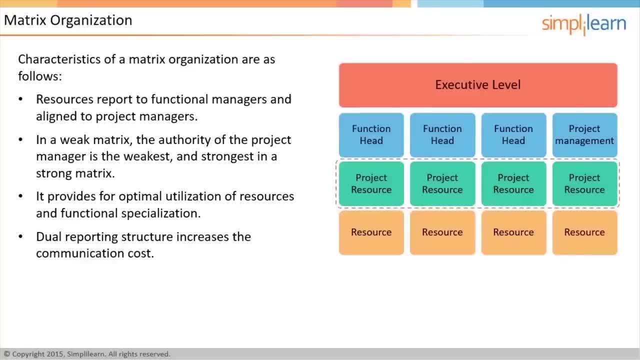 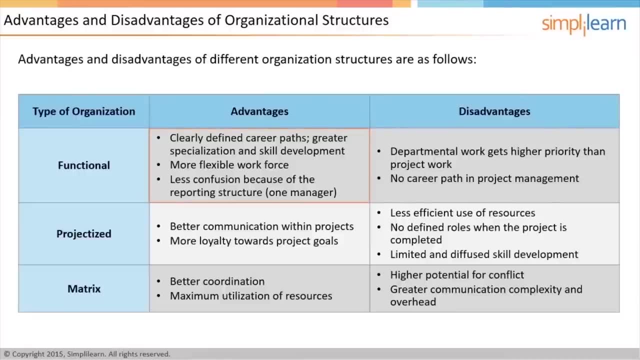 and disadvantages of different organizational structures. Each organization structure has its own set of advantages and disadvantages. The advantage of functional organizations is that resources may find clearly defined career paths and achieve specialization and skill development in their respective fields. It will be a flexible workforce, since 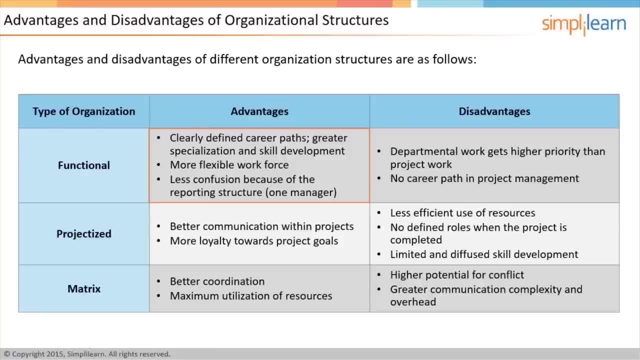 only one manager will be responsible, avoiding confusion. The disadvantage of such organization type is that project work is hampered. Department work is always given higher priority than the project work. In addition, there is no career path in project management, which leads to lower interest in projects. 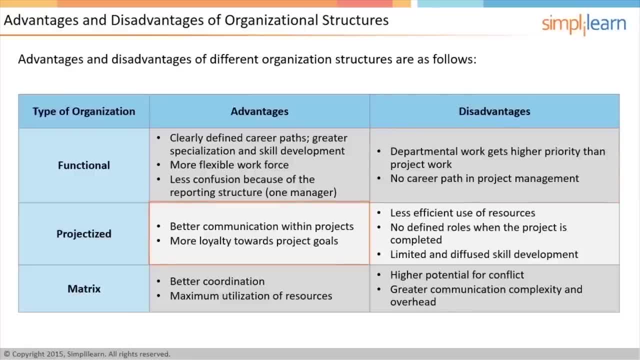 In the case of the projectized organization. one of the clear advantages is better communication within the projects, Since project work is the only work team members are doing. it also leads to loyalty towards the project goals. The disadvantage of such organization type is the inefficient use. 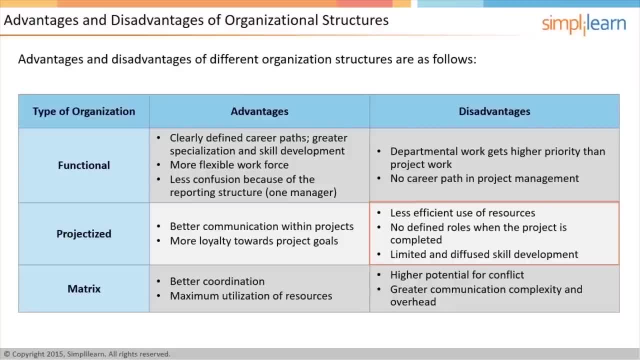 of resources because every project team has their own support function. Therefore, this might lead to the duplication of effort. It also leads to the resources being left with no work, since their roles are over once the project is completed. It also hampers skill development because the 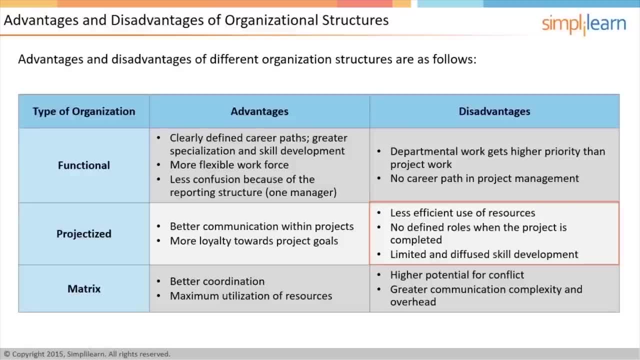 project requirements dictate what kind of work team members perform at different stages on a project. Now let us look at the matrix organization. It also has the advantage of better coordination and maximum utilization of resources. However, the disadvantage is the higher potential for conflict. 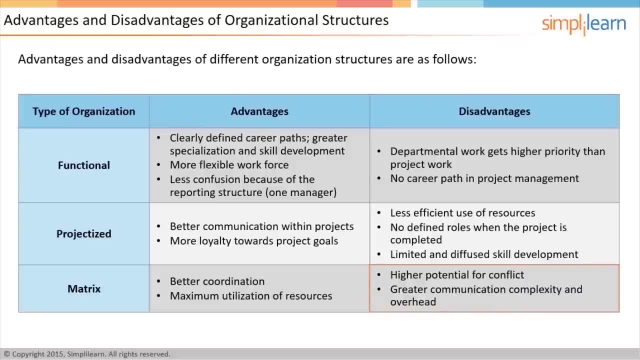 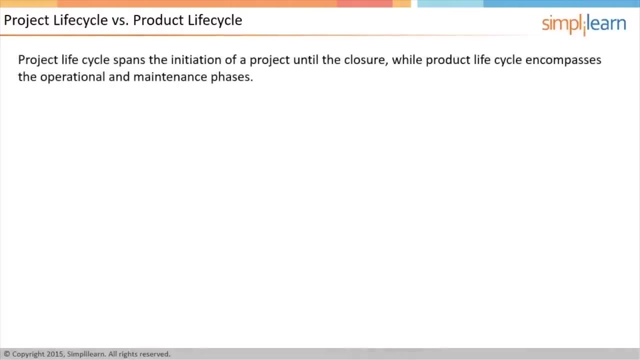 among the managers, which might lead to communication complexity and overhead management. In the next screen, let us focus on the comparison on project lifecycle and product lifecycle. Project lifecycle spans the initiation of a project until the closure of the project. Product lifecycle, on the other hand. 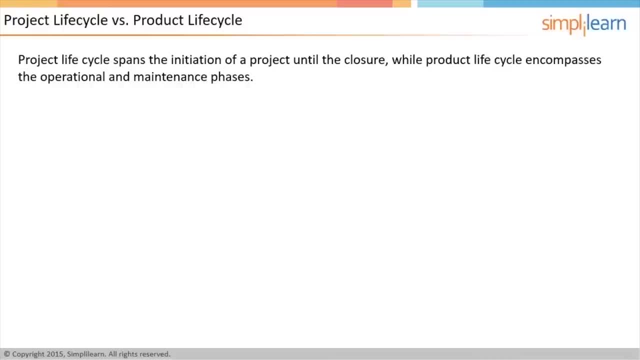 also encompasses the operational and maintenance phases. A typical product lifecycle starts with conception of the product and goes until its withdrawal from the market. The withdrawal might be because it becomes obsolete or there is no further need for the product in the market. A product has a long lifecycle. 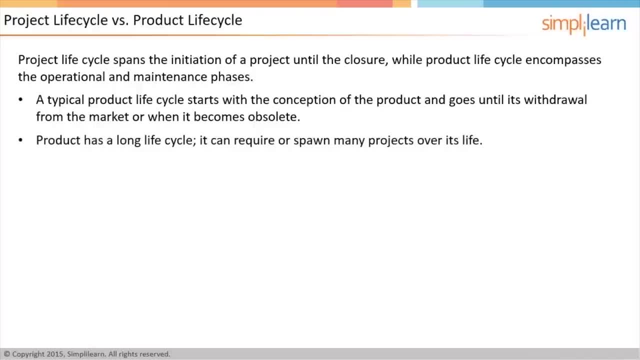 A product can require or spawn many projects over its life. For example, a project in product conception phase could be to determine customer needs, whereas a project during product maturity phase could be used to perform competitive analysis. Typically, a product lifecycle is longer than the project lifecycle. 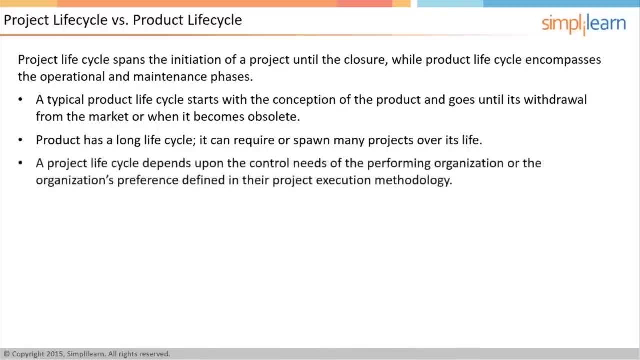 A project also has its own lifecycle, and this lifecycle depends upon the industry and the organization within which the project is being executed. Sometimes, different organizations within the same industry use different life cycles. There can be questions in the exam based on the comparison of project. 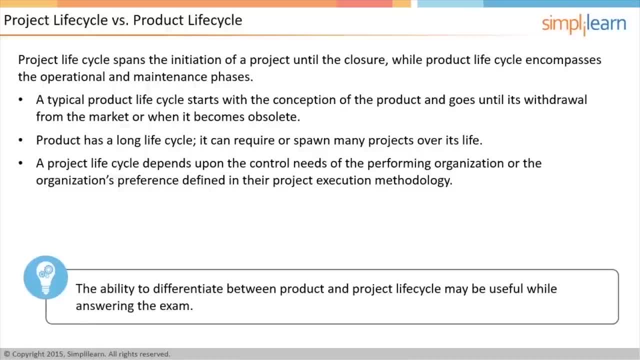 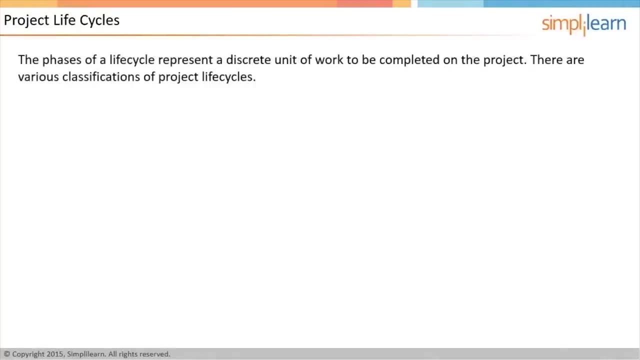 lifecycle and product lifecycle. so understanding the differences will be useful in answering such questions. In the next screen, let us discuss more on project lifecycle. A lifecycle is composed of phases. Each phase represents a discrete unit of work required to be done on the project. 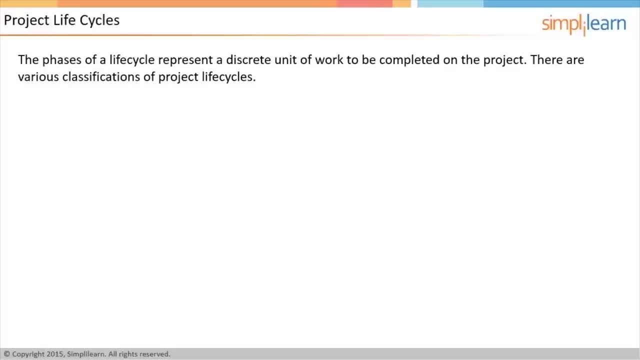 There are different ways of classifying project life cycles. Let us first discuss the sequential versus overlapping lifecycle. In sequential phases, the subsequent phase starts only after the previous phase has been completed, whereas in overlapping phases, two or more phases may run in parallel for some time. 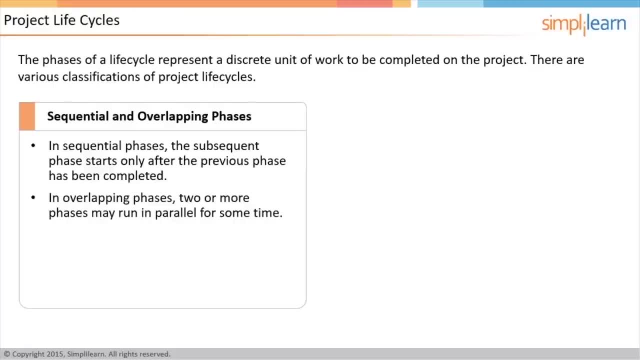 This could help fast tracking and compressing the amount of time required. The other way of classifying life cycles is how they go about the process of planning. In predictive life cycles there is a large upfront planning phase where all the details of scope 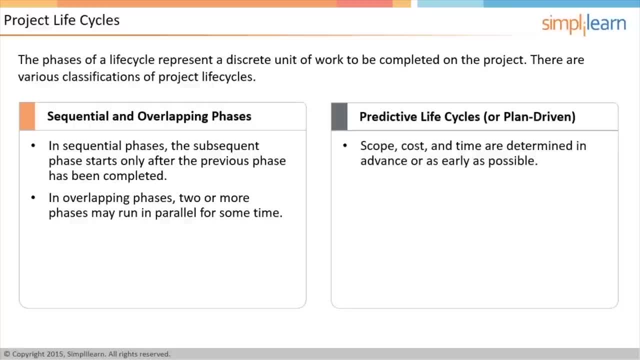 cost time are planned before beginning the subsequent phases. These phases, then, are executed in either sequential or overlapping modes. They are suitable for large projects where all the requirements are likely to be known in advance and where upfront planning effort is required to get the necessary approvals. 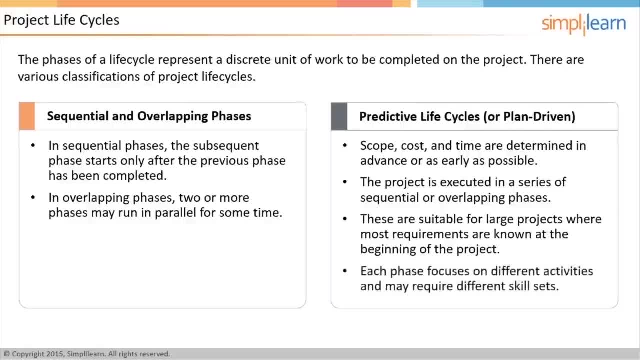 Another feature of predictive life cycles is that each phase may potentially be different in the nature of activities and may require people with different skill sets. For example, traditional software development life cycle has phases like requirements, feasibility planning, design, construction, testing. 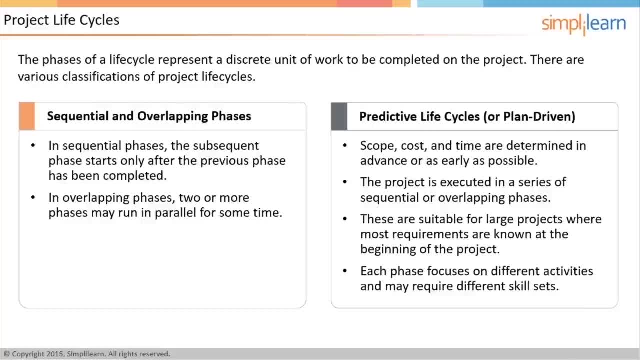 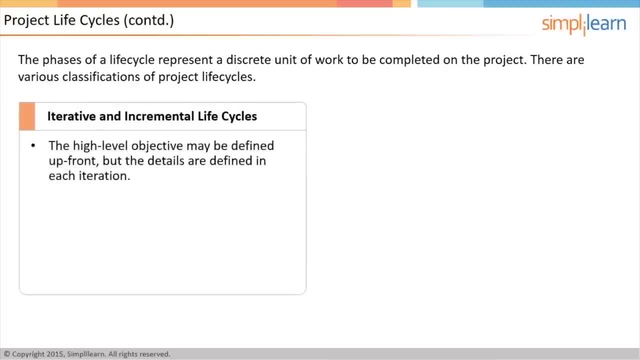 and transition. We will continue project life cycles in the next screen. Incremental and iterative life cycles have a short, upfront high-level definition and planning phase. The product is then developed through a series of iterations where iteration increments or adds to the functionality by a little. 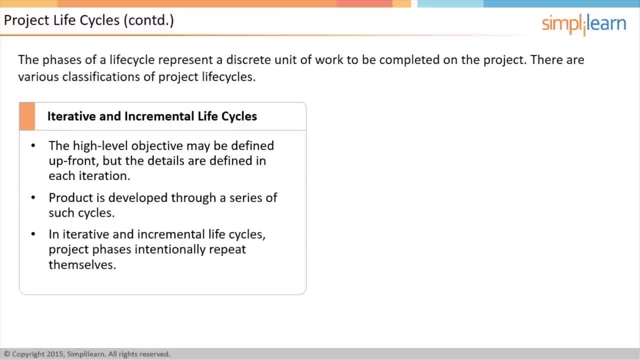 All the activities are intentionally repeated in iterations. Adaptive or agile life cycles are variants of incremental and iterative life cycles where iteration is very short, typically two to four weeks. Agile methodologies are becoming very popular in the software development industry and in other industries where the requirements are highly changeable. 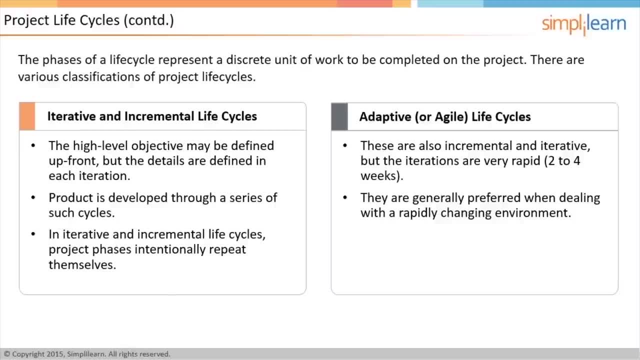 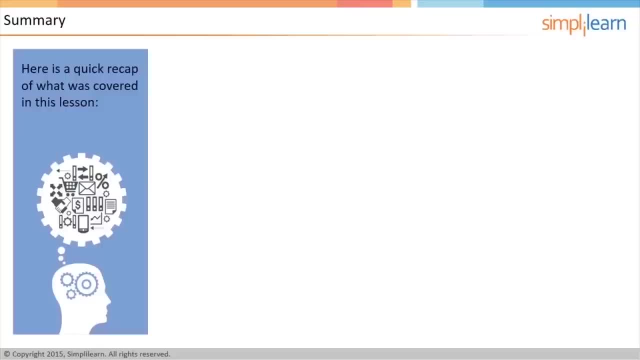 and frequent feedback is beneficial. Let us now check your understanding of the topics covered in this lesson. Here is a quick recap of what was covered in this lesson. Project management is the application of knowledge, skills and tools and techniques applied to project activities to meet the project. 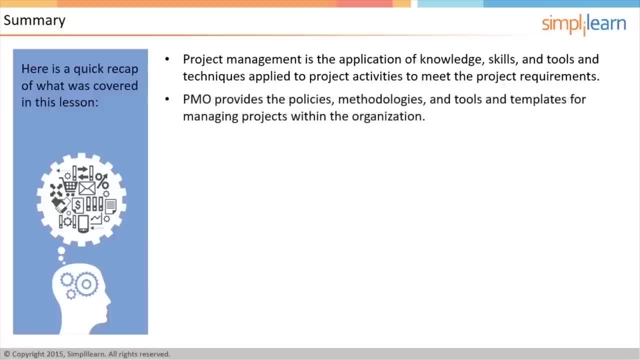 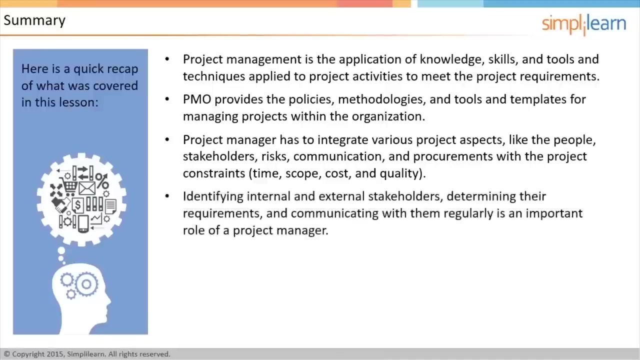 requirements. PMO provides the policies, methodologies and tools and templates for managing projects within the organization. Project manager has to integrate various project aspects, like the people, stakeholders, risks, communication and procurements, with the project constraints, Identifying internal and external stakeholders. 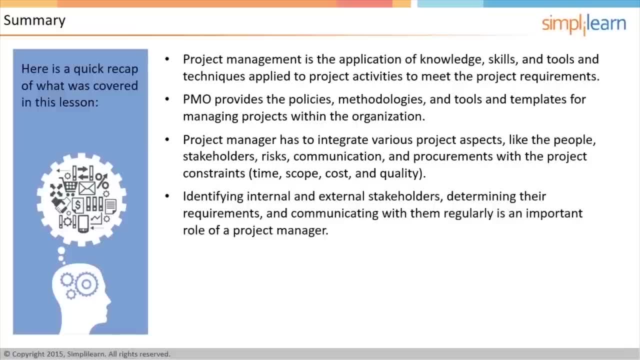 determining their requirements and communicating with them regularly is an important role of a project manager. Functional, projectized and matrix are the three types of organization structures based on the level of authority given to the project manager. Project lifecycle spans the initiation of a project until 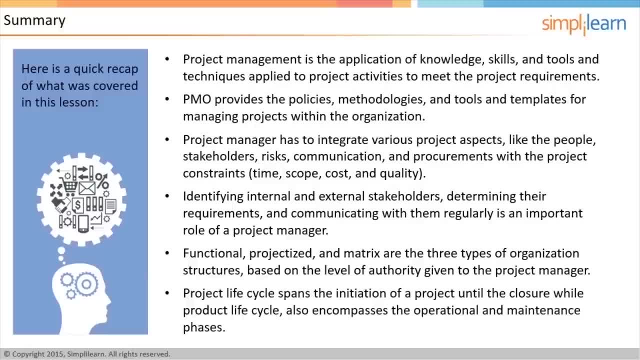 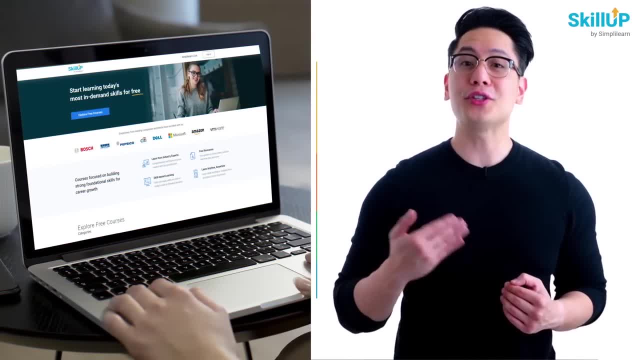 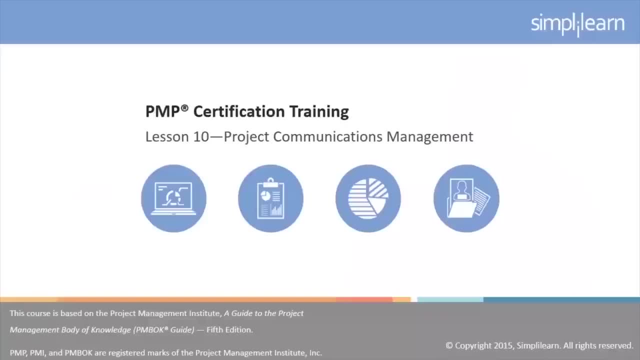 the closure, while product lifecycle also encompasses the operational and maintenance phases. If getting your learning started is half the battle, what if you could do that for free? Visit SkillUp by SimplyLearn. Click on the link in the description to know more. 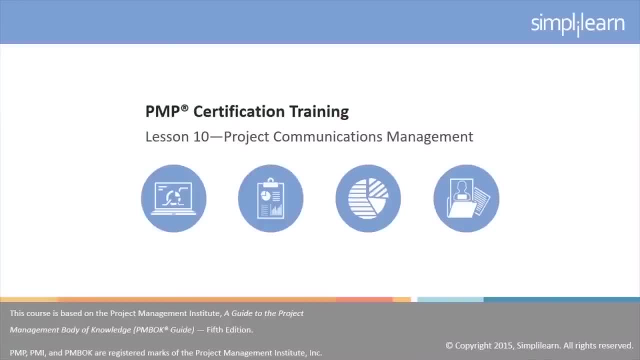 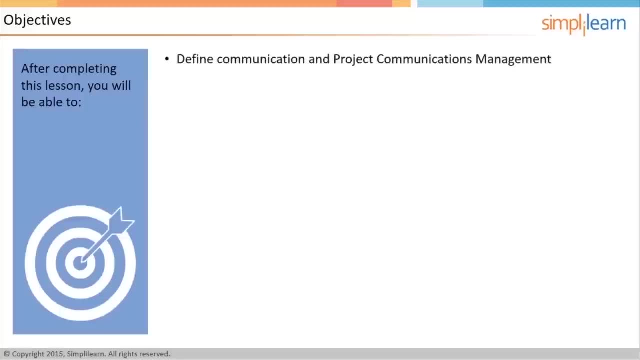 In this lesson we will focus on project communications management. Let us begin with the objectives of this lesson. After completing this lesson, you will be able to define communication and project communications management, identify the different communication methods, technology and channels, explain the 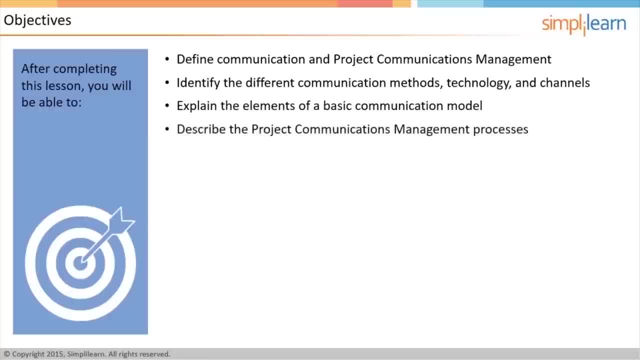 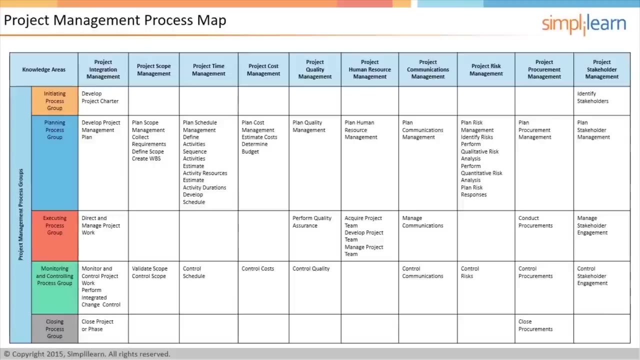 elements of a basic communication model describe the project communications management processes In the next screen. let us take a quick look at the project management process map. There are 47 processes in project management, grouped into 10 knowledge areas and mapped into 5. 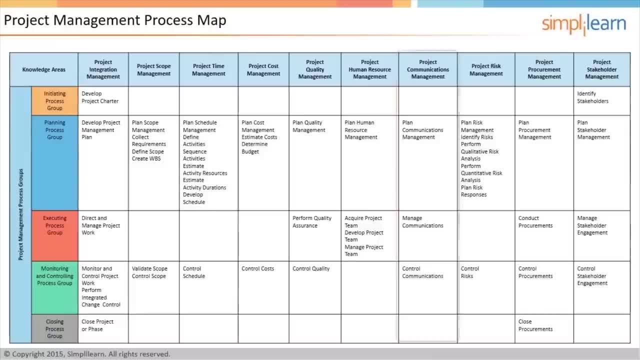 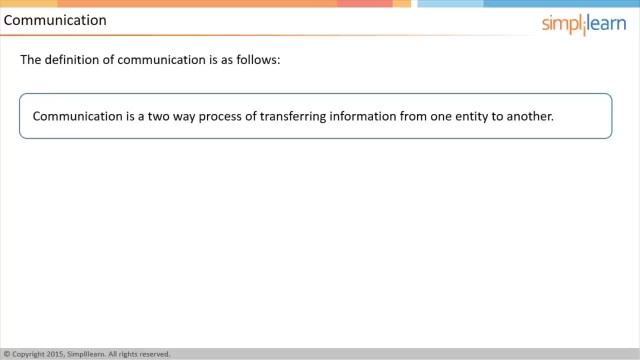 process groups. In this lesson we will look at the seventh knowledge area, that is, project communications management and its processes In the next screen. let us understand communication. Communication can be best defined as a two-way process of exchanging information between two entities. As you can see, 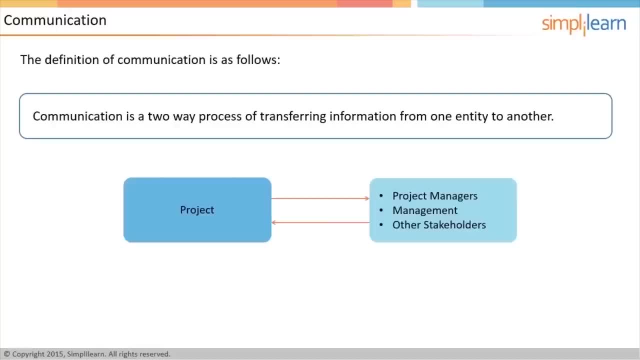 on the screen. if project is an entity, the project needs to communicate with other entities in the organization, like project managers, senior management of the organization and any other stakeholder of the project. Similarly, these entities may also have to communicate with 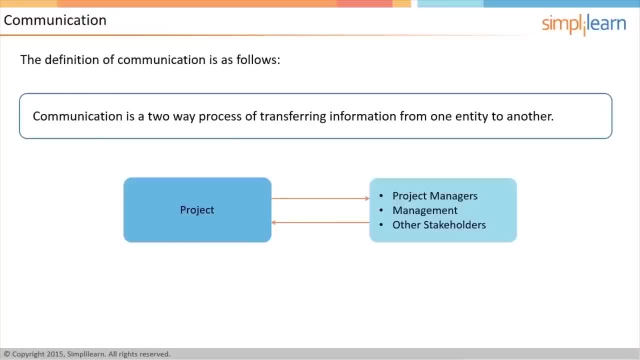 the projects. The communication between project and the stakeholders is always two-sided. Project manager is responsible for ensuring proper communication to and from the project. In fact, a project manager spends almost 90% of his or her time on communication. You can now understand. 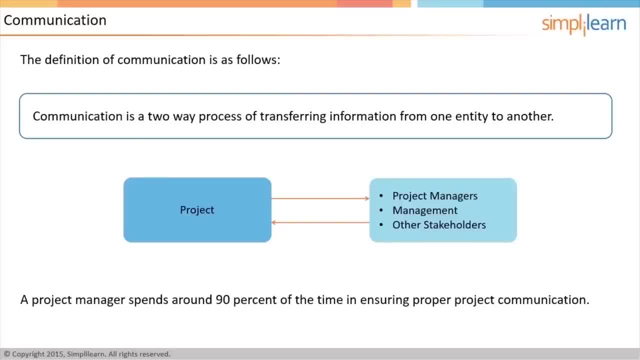 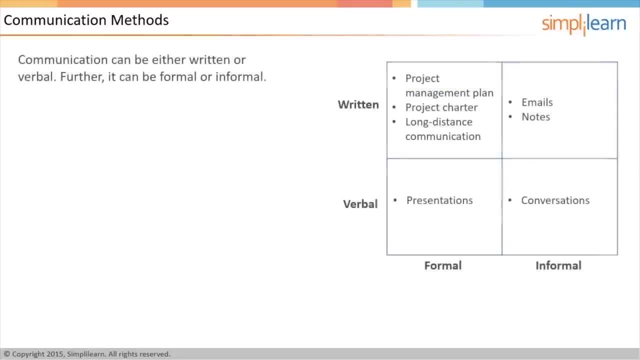 how important it is for a project manager to plan this activity well. In the next screen, let us discuss communication methods. Communication can be done in two ways. It can be done written or verbal. Both written as well as verbal communication can either be. 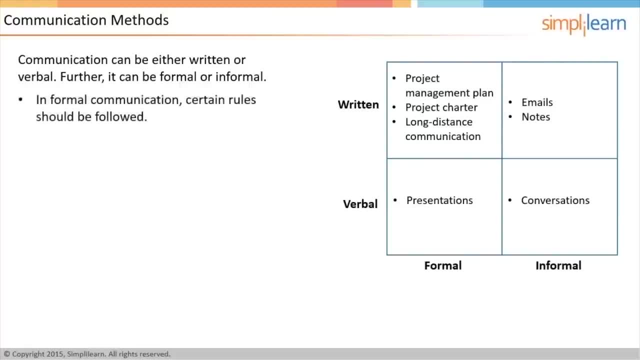 formal or informal. Formal means communicating by following some basic rules, whereas informal means taking a casual approach. These two combinations result in four different communication methods. They are formal, written, formal verbal, informal written and informal. verbal. Formal written method is used for project. 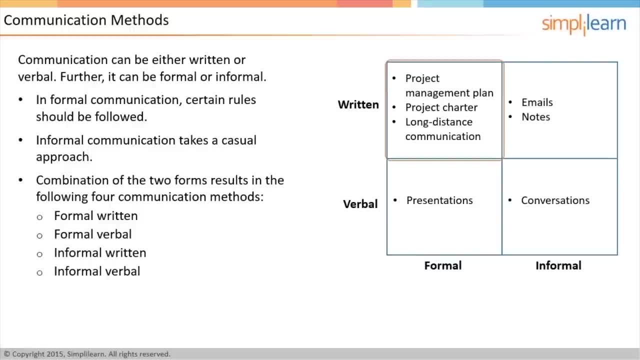 management plans, project charter and over long distance communication. Formal verbal method is used during presentations, whereas informal written method is applicable while writing notes or emails. Informal verbal, on the other hand, is applied during conversations. You can expect questions in the PMP exam. 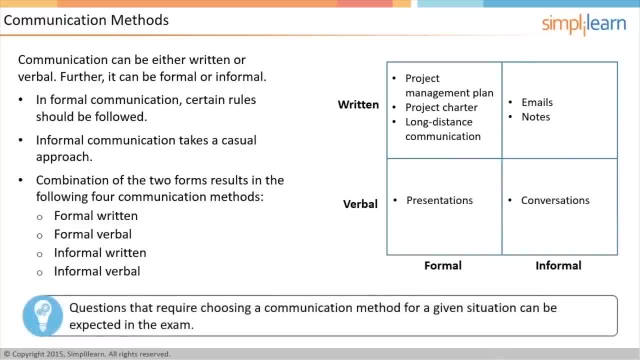 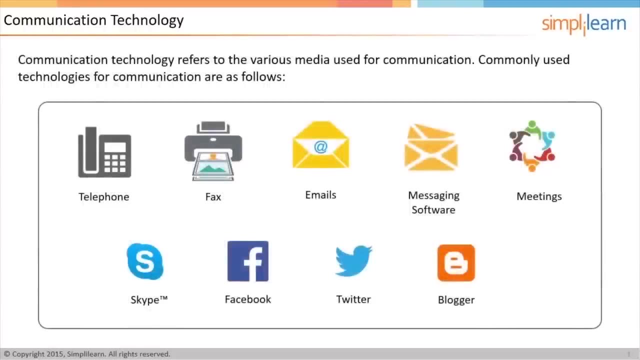 which require choosing a communication method for a given situation. so a fair understanding of the communication methods can help you score higher In the next screen. let us look at the various communication technologies. Communication technology refers to the different media used for communicating. A few such 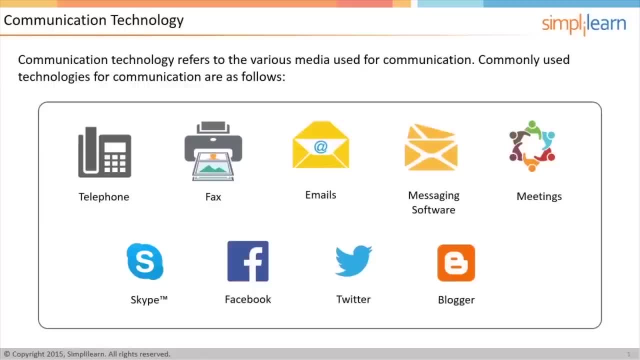 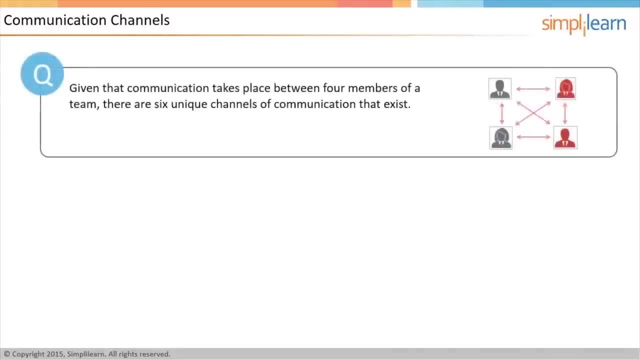 technologies are listed on screen, among which email, fax and telephone are a few popular communication technologies. In the next screen, let us understand the communication channel with the help of an example. Communication takes place between four people in a team, The lines across the. 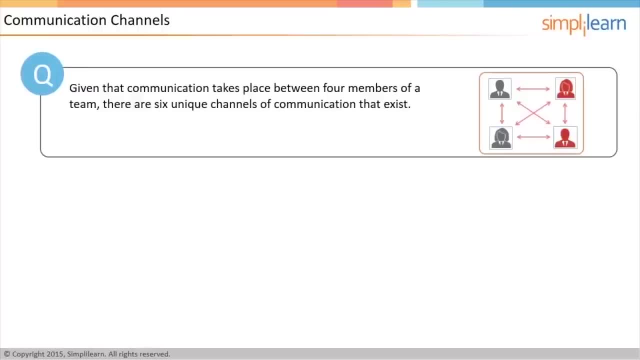 members represent their communication skills. The communication channel can be six unique channels of communication existing within the team. Now, if the team comprises 10 members, how many unique channels of communication will be calculated? You can use the formula n multiplied with n. 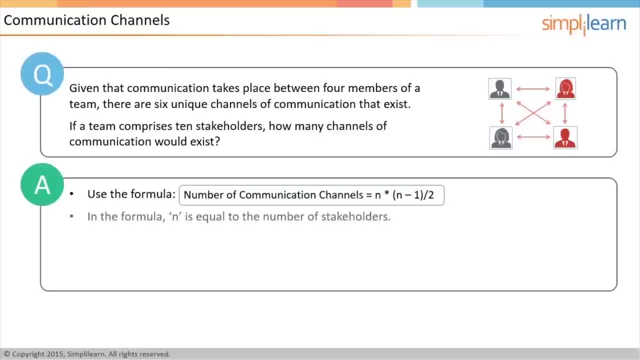 minus 1 and the resulting sum divided by 2.. N is the total number of people involved in communication. In this case, n equals to 10.. If this is put into the formula, you will get 45 as the total number of people. 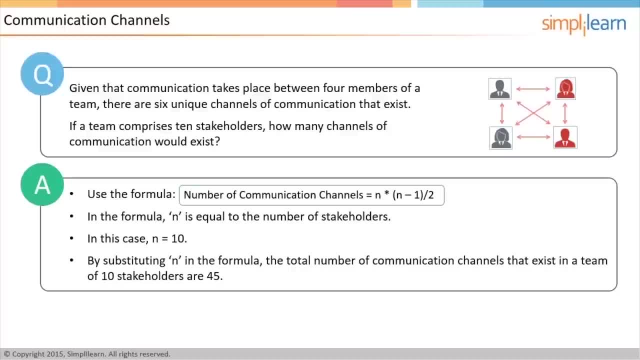 involved in communication. Therefore, 45 unique communication channels exist. in a team of 10 people, It is difficult to manage such a large number of communication channels. Therefore, it is important to structure communication. Otherwise everyone starts communicating everything to everyone, and 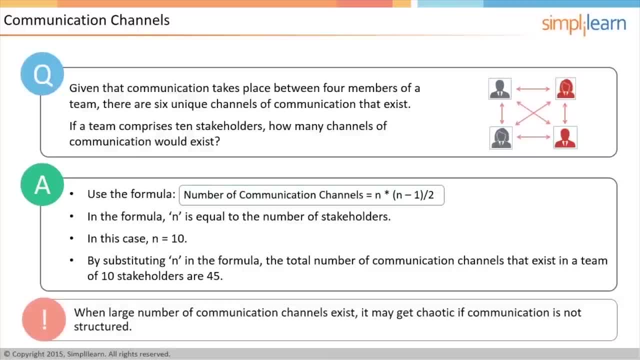 it can become a real chaos in the project. In the PMP exam you may be asked to calculate the number of communication channels in a scenario-based model, so please make a note of the formula to answer the question correctly In the next screen. 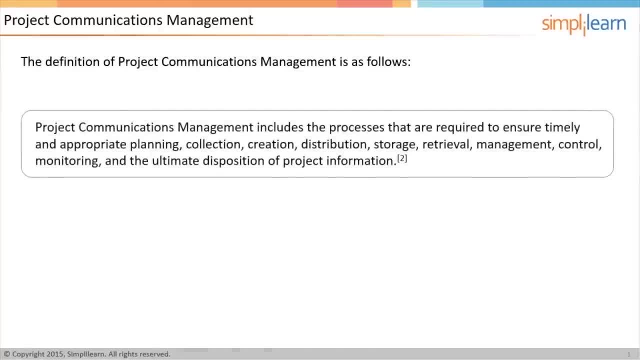 let us discuss the basic communication model. Project communications management includes the processes required to ensure that information about timely and appropriate generation, collection, distribution, storage and ultimate disposition of project is prepared and circulated to all project stakeholders. It is the responsibility of a project. 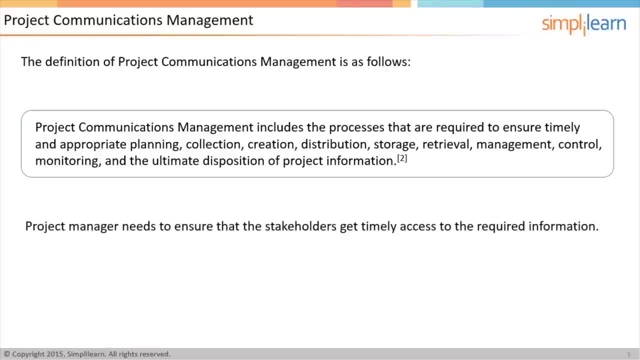 manager to ensure that the information requested by the stakeholder is communicated to them. The frequency at which the information needs to be shared may also vary from stakeholder to stakeholder. For example, think about a simple process of sharing a project status report with the customer and. 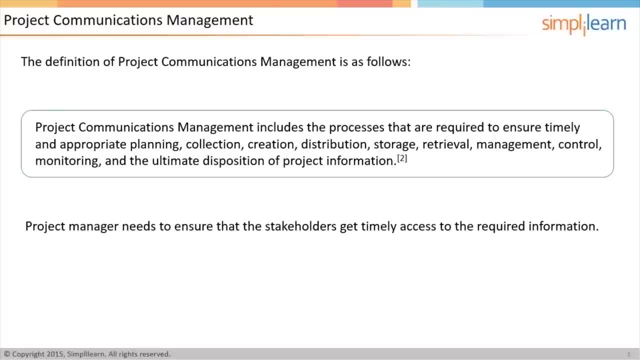 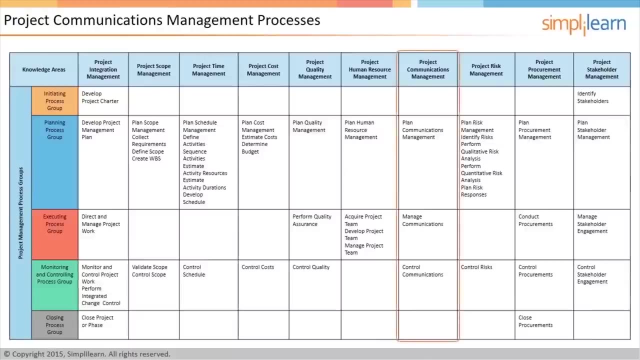 senior management. This knowledge area explains how it should be done as per PMI. In the next screen let us discuss the process management of project communications management processes. There are three project communications management processes. Process is carried during different process groups: Plan communication management. 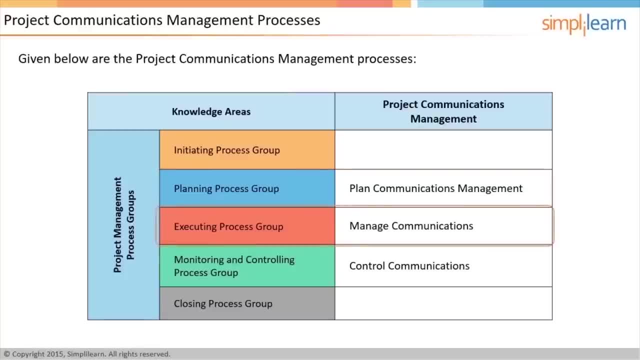 is done during planning process. group Manage communications is done during executing process group And control communications is done during monitoring and controlling process group. In the next few screens we will cover each of these processes in detail. Plan communications management is the process of developing. 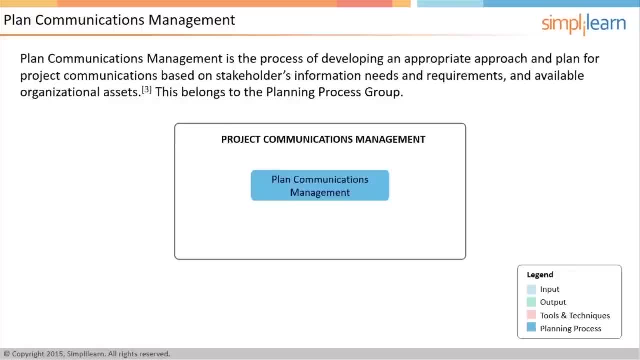 an appropriate approach and plan for project communications, based on stakeholders' information, needs and requirements and available organizational assets. This belongs to the planning process. group Stakeholder register is an important input to this process. It is a list of all the stakeholders, The project. 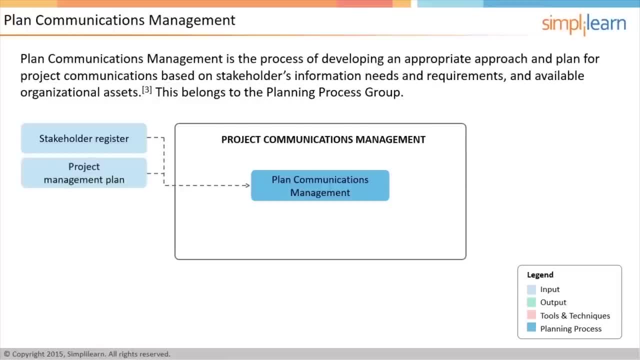 management plan has information about a large number of the project's requirements, and the stakeholders who need to receive communication of various kinds are therefore a critical input to this process. In addition to these two organization process, assets and enterprise, environmental factors are also inputs to this process. 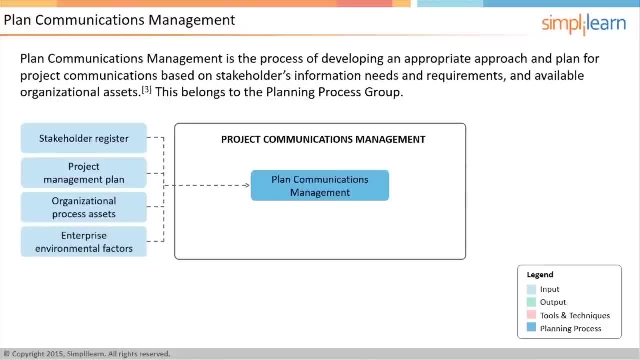 Many organizations have standard templates to prepare communication management plan which are part of the organizational process: assets and enterprise environmental factors. The first technique used in this process is the communication requirements analysis, where the communication requirements of each of the stakeholders are analyzed and categorized. In this you try. 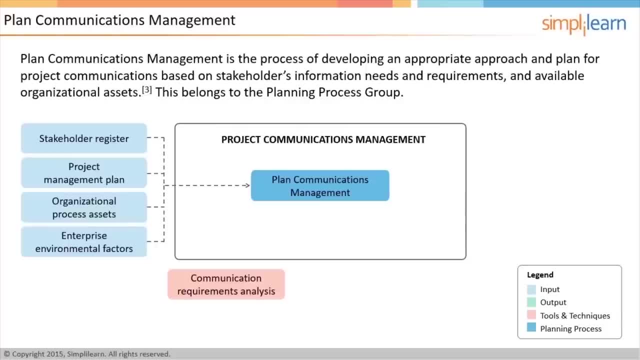 to find how many of the stakeholders need similar kind of information which can be grouped together. If you send information through an email system, all those stakeholders who need similar information can be marked in CC in the email. Next you can decide on the. 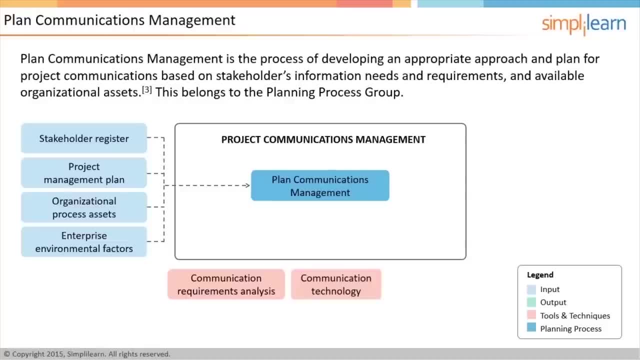 communication technology. These days, email is the most widely used technology, but in few cases you might have to send information using some other technology, like fax or registered post. For example, all government communications are done using registered post to keep a written record. Finally, 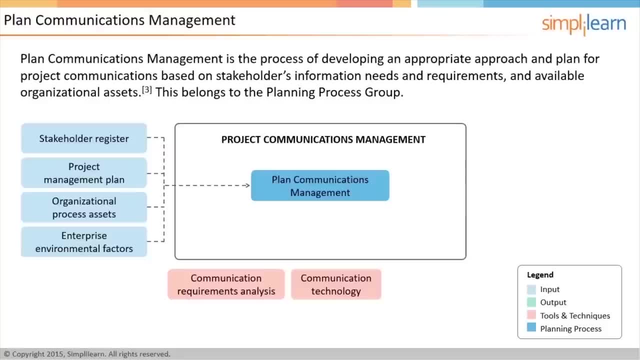 you need to understand how to communicate really happens. that is, the communication models and the various communication methods used. You may need to conduct meetings before agreeing on and finalizing the communications management plan. The communications management plan is the primary output of this process. 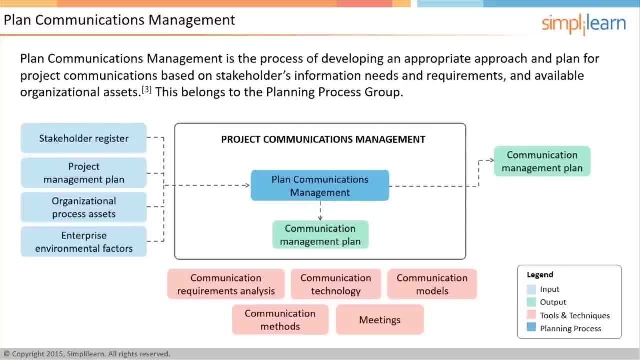 which lays down the procedures around communications in the organization. Communication management plan has information like which stakeholder needs what kind of information, at what frequency and how. As a result of this process, some other project documents may also get updated. There may be 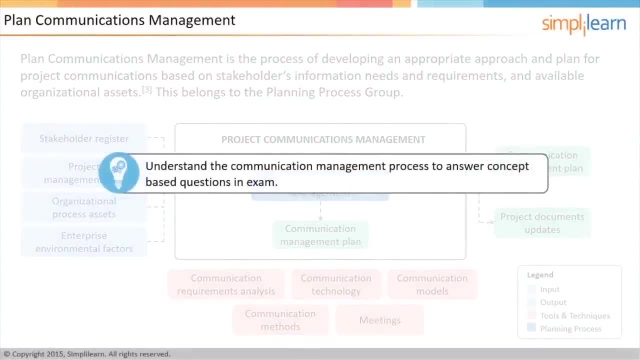 questions in the PMP exam based on the planned communications management process, so a fair understanding of the process will help you answer such questions correctly. In the next screen, let us look into a business scenario to understand this concept better. After reading the problem statement, click the. 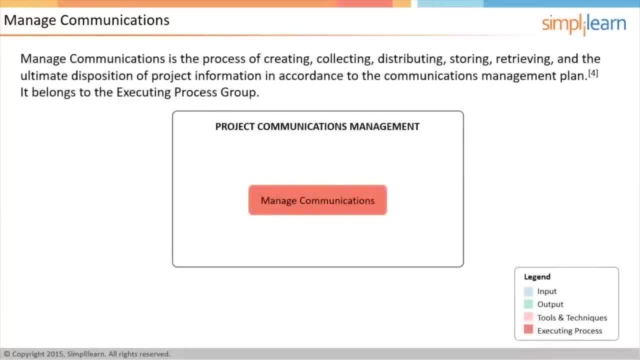 solution button to look at a possible solution. Manage communications is the process of creating, collecting, distributing, storing, retrieving and the ultimate disposition of project information. in accordance to the communications management plan, It belongs to the executing process group. Manage communications is done. 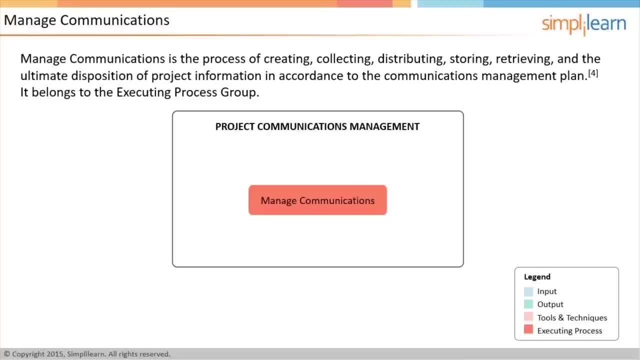 throughout the project life cycle. Everything cannot be planned during communication planning, so manage communications takes care of responding to unexpected requests for information as well. Communications management plan is an important input. Work performance reports have information regarding project performance and status information. Organizational process. 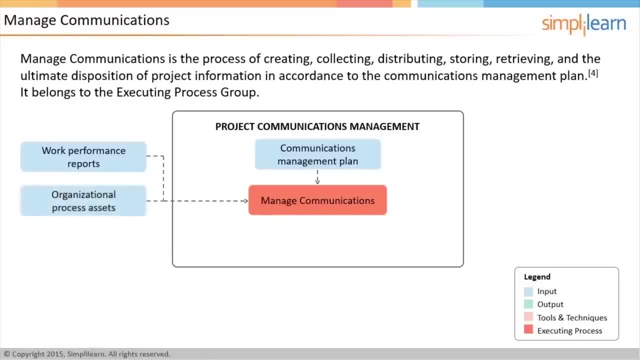 assets are the standard templates created for the status report by organizations. In some organizations there are guidelines for communication distribution. Enterprise environmental factors are the other inputs to this process. Various tools and techniques are used in this process. Communications technology represents the means of technology, that is. 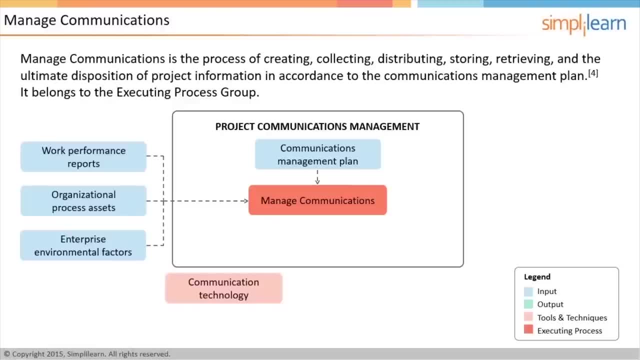 email, instant messaging, telephone conferencing, etc. that are used to exchange information. The use of communication models helps you determine the technique that is best suited for a particular situation. Communication methods are the various methods used to communicate, For example, whether it is interactive or. 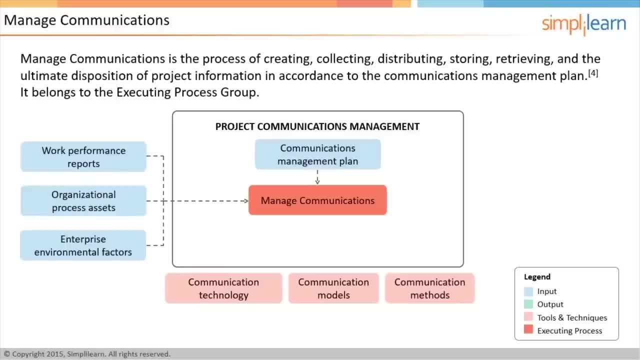 offline, whether information is being pushed by the provider or pulled by the recipient, etc. Information management systems help design a framework for managing the information within a project, that is, how it is acquired, where it is stored and how it is distributed. and. 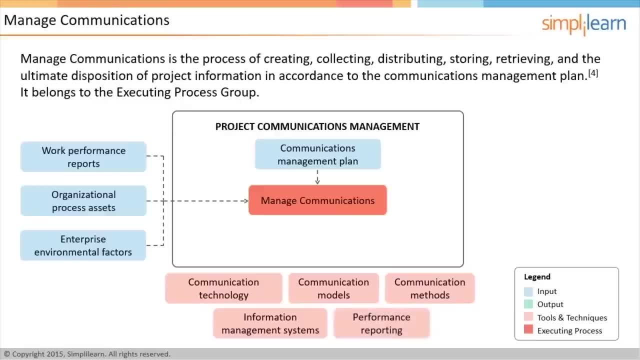 destroyed. In performance reporting, all the information is synthesized in the form of performance reports that are later distributed to the appropriate stakeholders, and forms an important part of the communications strategy on a project. The first and primary output of this process is the communications messages that 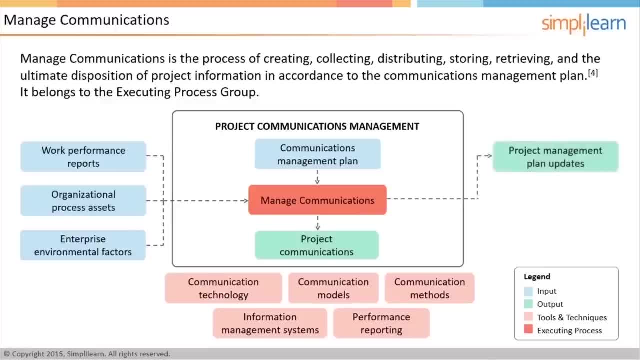 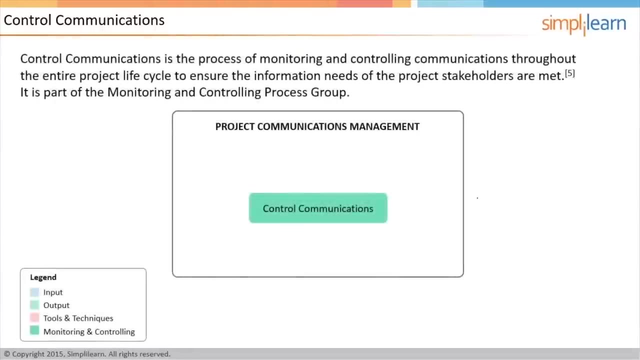 are generated during the project. The other outputs include project management plan updates, project document updates and organizational process assets updates. In the next screen, let us discuss controlled communications process. Controlled communications is the process of monitoring and controlling communications throughout the entire project. 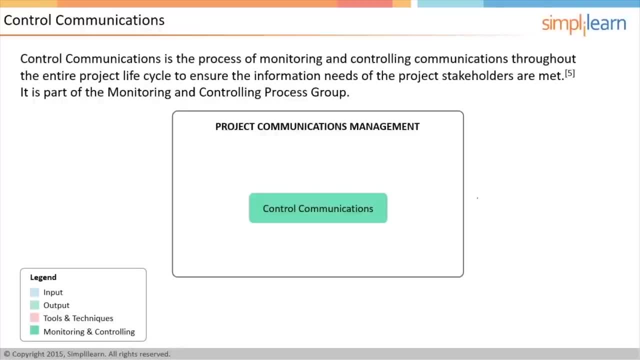 lifecycle to ensure the information needs of the project's stakeholders are met. It is part of the monitoring and controlling process group. The inputs to this process are the project communications, project management plan and issue log, which has a list of issues that are raised by different project. 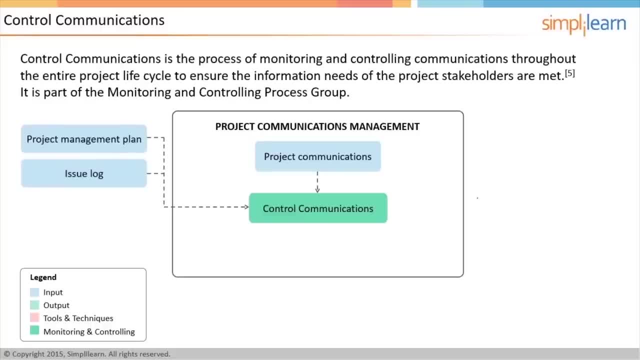 stakeholders, data related to the work being performed on the project and various other project documents which may have to be communicated. Other inputs include work performance data and organizational process assets. Let us look at the tools and techniques in detail. The information management systems provide tools to collect. 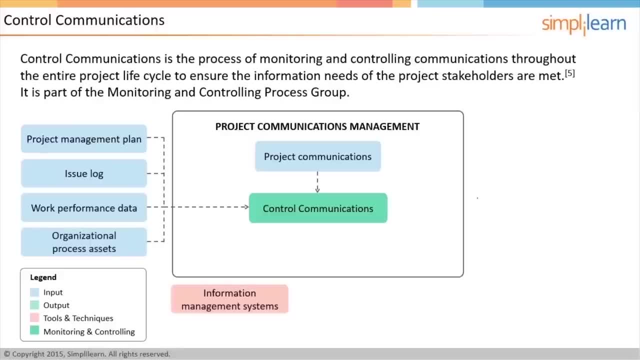 consolidate and present the information in the form of cogent, concise communications. Expertise must be sought from different stakeholders on how you should go about this process. Several meetings may be needed to ensure the efficiency and efficacy of the communications. The major outputs of this 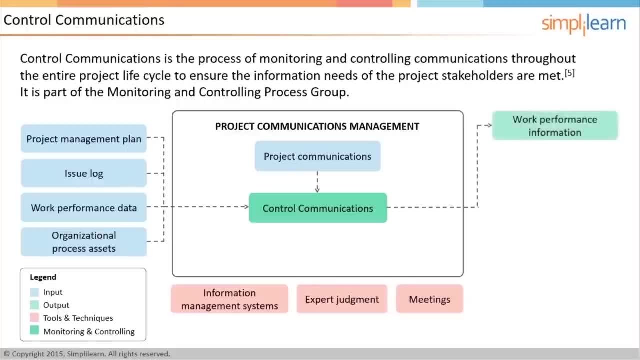 process is the work performance information, which indicates that the work performance data has been analyzed, interpreted and presented in an easily comprehensible form. This process may also give rise to change requests, updates to the project management plan, project documents and organizational process assets. 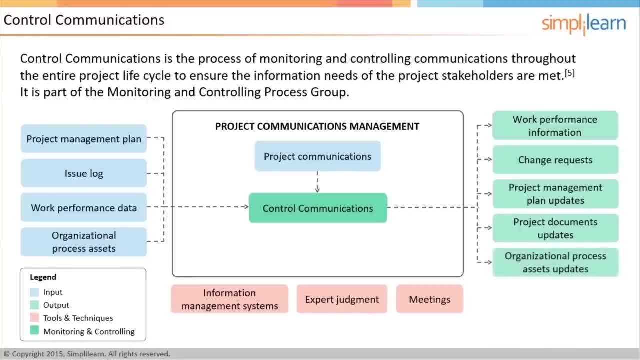 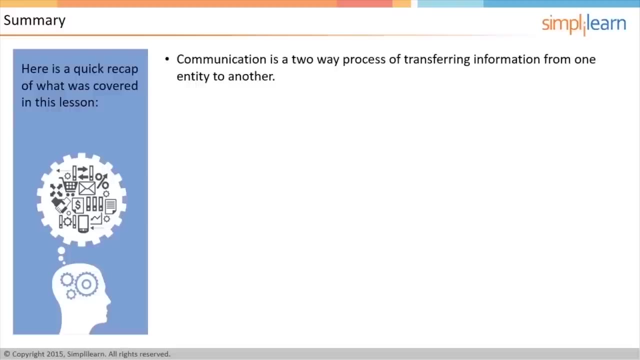 In the next screen. let us look into a business scenario to understand this concept better. After reading the problem statement, click the solution button to look at a possible answer. Here is a quick recap of what was covered in this lesson. Communication is a two-way process. 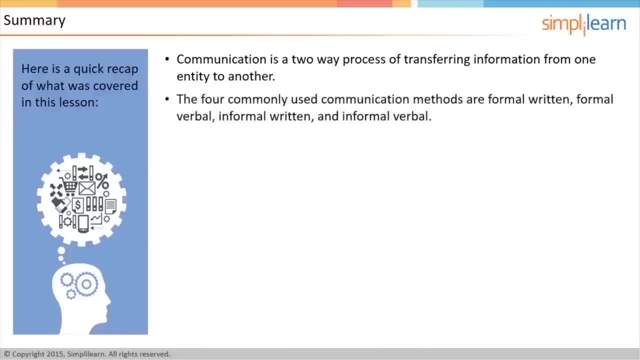 of transferring information from one entity to another. The four commonly used communication methods are formal written, formal verbal, informal written and informal verbal. The total number of unique channel of communication can be calculated using the formula n multiplied with n minus one and the resulting sum. 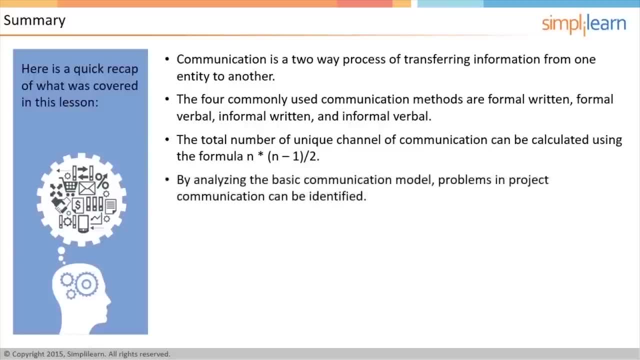 divided by two. By analyzing the communication model, problems in project communication can be identified. Project manager is responsible for timely availability of information to all stakeholders. The three project communications management processes are planned communication, management, management communications and control communications. In this lesson we will focus 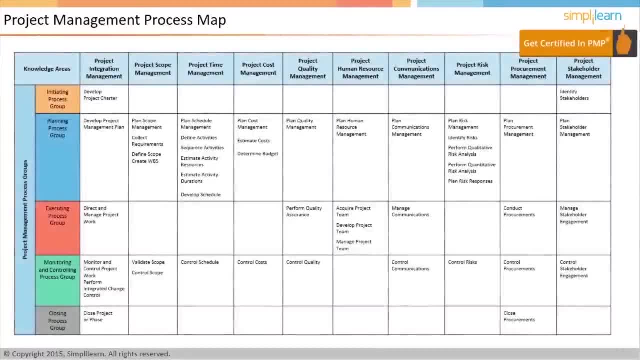 on project human resource management. There are 47 processes in project management, grouped into ten knowledge areas and mapped to five process groups. In this lesson we will look at the sixth knowledge area, that is, project human resource management and its processes, In the next. 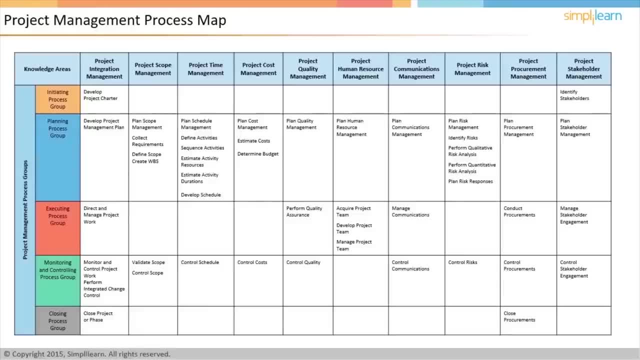 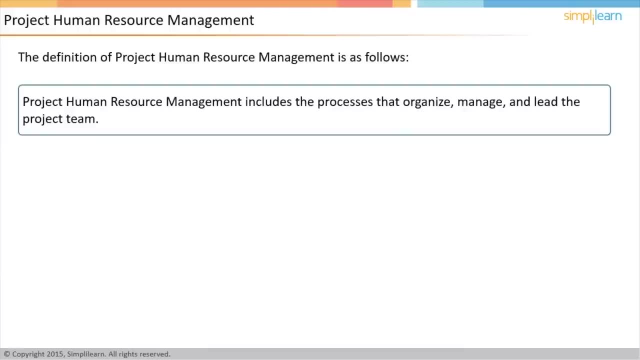 screen. let us understand project human resource management. Project human resource management includes the processes that organize, manage and lead the project team. One of the key elements of human resource management is that each of the project team members should have clear assignment of their 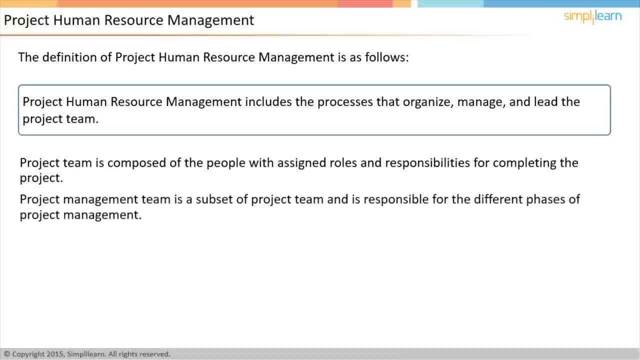 roles and responsibilities. In addition, even the team working on project management tasks should be a part of the project team and they are responsible for project management functions like initiating, planning, executing, monitoring and controlling, and closing, along with other leadership activities In the next screen. 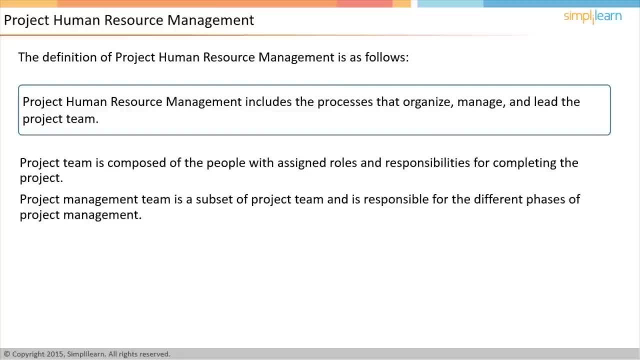 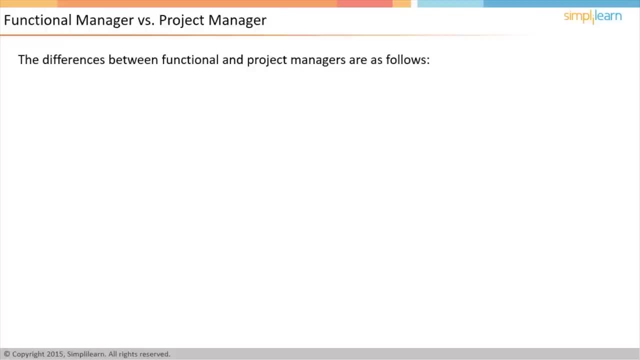 let us understand the difference between functional and project manager. An organization may have both functional managers and project managers. The difference: Functional manager is the one who handles a business function or department. For instance, the HR manager is responsible for the HR department in an organization. 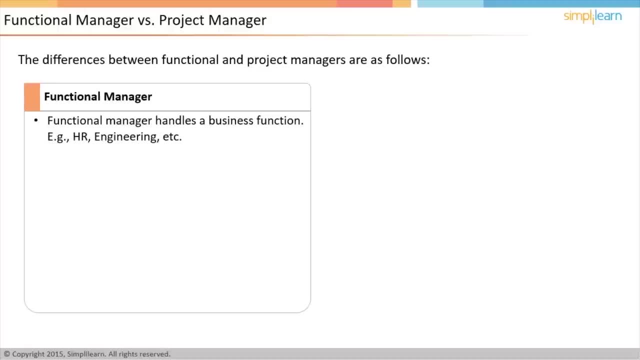 Therefore, an HR manager will be a functional manager. Generally, a functional manager is also a subject matter expert. The roles and responsibilities of the functional manager depend upon the core business of the organization and overall organization structure. Functional managers normally own the resources and provide the 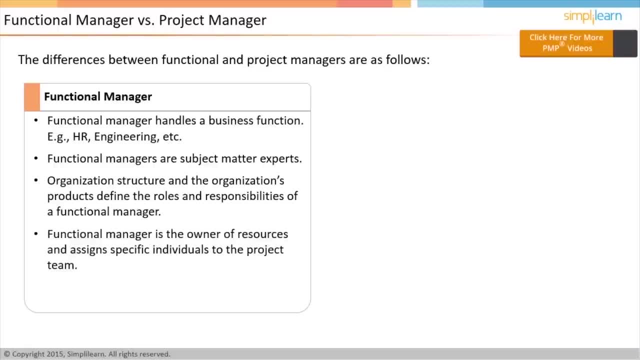 projects with necessary resources. They also negotiate with the project manager regarding resources. The project manager, on the other hand, is responsible and accountable for the success or failure of a project and the quality of the project. They are not technical experts. The project manager may not have. 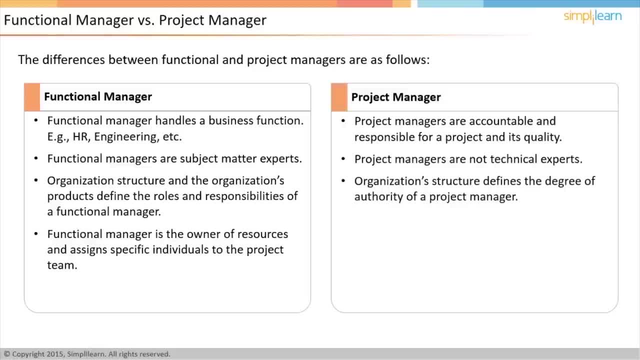 authority over the resources, depending upon the organizational structure. They often have to negotiate with the functional manager for the resources and are responsible for the product quality. A project manager will credit the team of the project and accept the blame for the failure. Now let us look at an example to 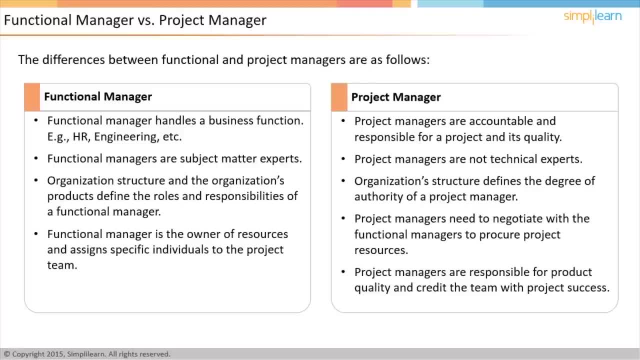 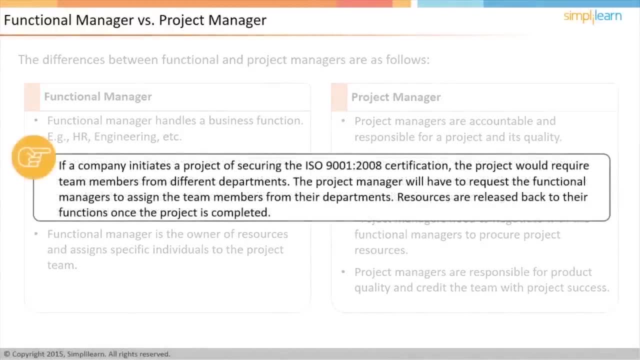 understand the roles played by functional and project managers. The CEO of an organization initiates a new project to secure an ISO 9001-2008 certification for the company. Now this project would require team members from each of the company departments and whoever is the 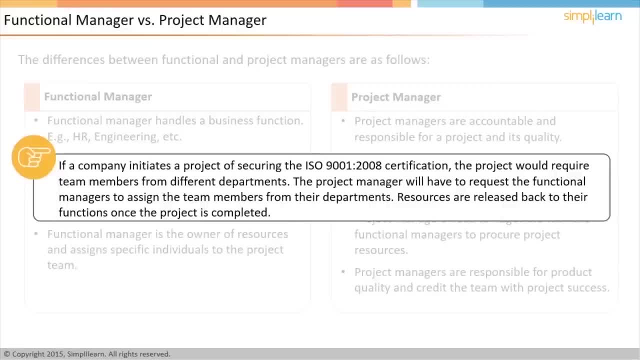 project manager of this project will have to request the functional manager to assign one of their team members to the project. Resources assigned to the project go back to their respective departments once the project is completed. Let us now discuss the project human resource management processes in the next screen. 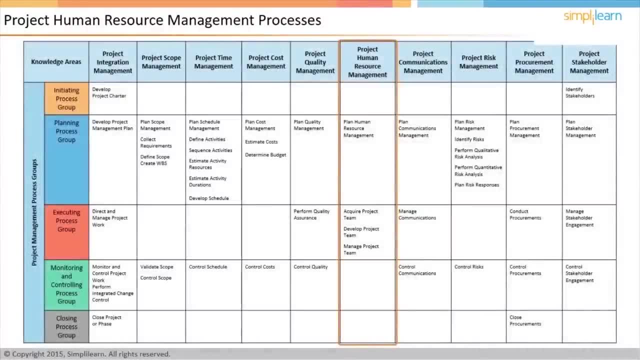 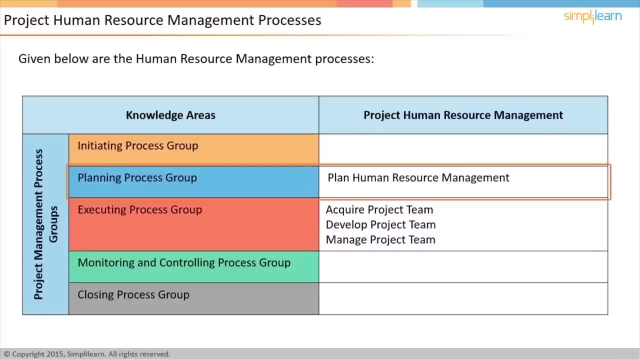 There are four project human resource management processes. The first process, Plan Human Resource Management is done as part of the planning process group. The next three processes are part of the executing process group. These processes are: Acquire Project Team, Develop Project Team. 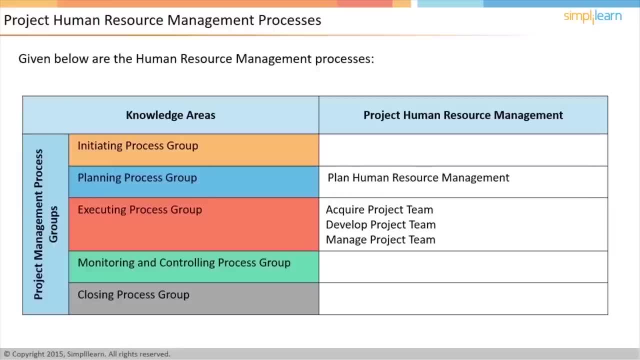 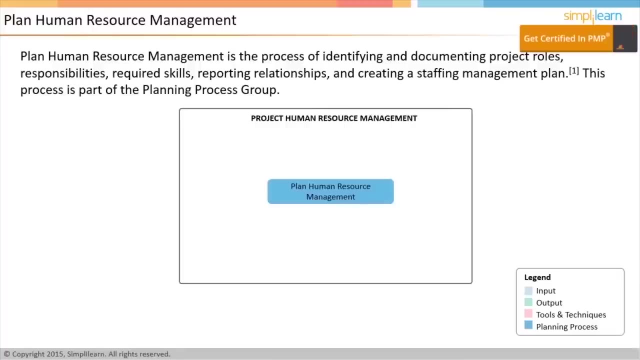 and Manage Project Team. Let us now look into each of these processes in detail In the next screen. let us begin with Plan Human Resource Management. Plan Human Resource Management is the process of identifying and documenting project roles, responsibilities, required skills, reporting. 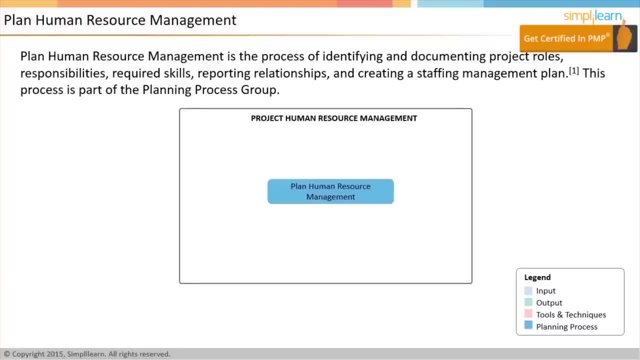 relationships and creating a staffing management plan. This process is part of the planning process group. In addition to that, finalizing the project hierarchy of who reports to whom and designing the staffing management plan is also part of this process. The first input to this process, 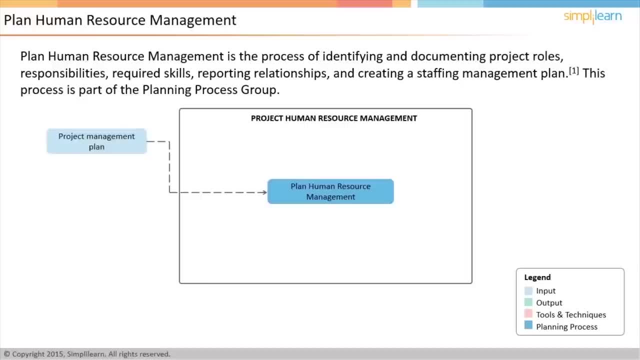 is the project management plan. There could be a lot of information in the project management plan and subsidiary plans that may be relevant to the creation of the human resource management plan, For example, the project life cycle, processes, the timelines, how the work will be accomplished. 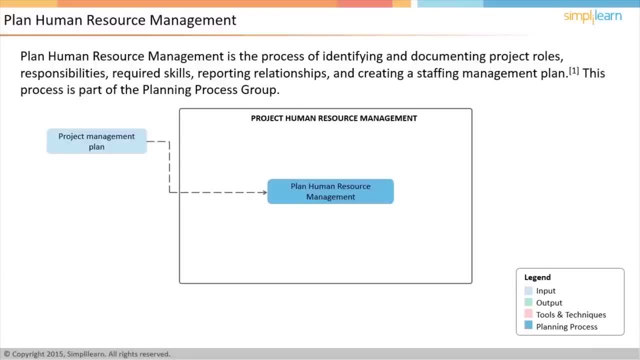 etc. The other key input for this process is the activity resource requirement. Team members can be identified based on these requirements. In addition to this, enterprise environmental factors like current employment outlook, etc. are also important. For example, if the economy is booming and there are 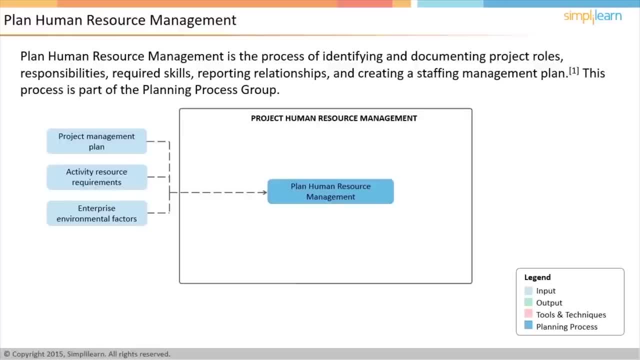 simple job opportunities for the team members. the reward and recognition system can keep the project team interested in the project. Organizational process asset is also an input to this process. An example of the organization process: assets can be template or a form to request for a new resource. 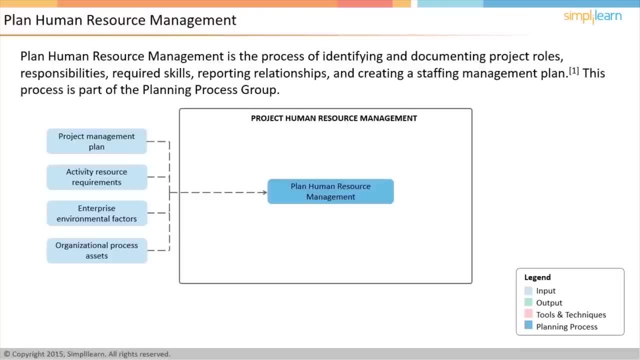 Let us now look at the tools and techniques used to develop human resource plan. The roles and responsibilities are captured in the form of organization charts and position descriptions. There are various ways to draw this chart. It can be either hierarchical chart, which shows the reporting function, or 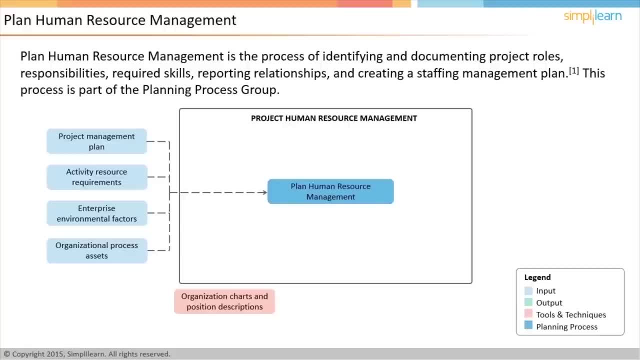 it can be text based. The other technique used for developing the human resource plan is networking. This involves formal or informal interactions within the organization and outside by the project manager to identify the best team for the project, depending upon various interpersonal factors. Organizational theory helps. 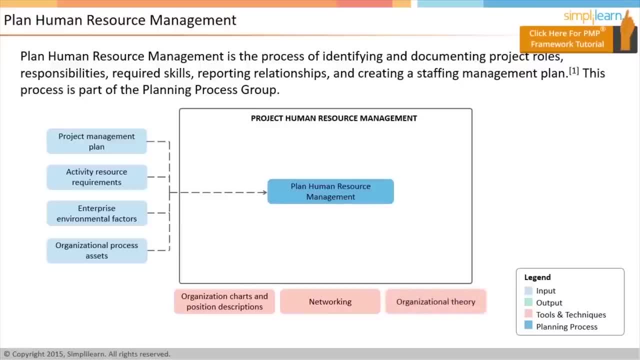 to understand how individuals come together and function as an organization. Expert judgment and meetings are required to put the human resource plan together. The output of this process is human resource management plan. This plan contains documents like staffing management plan, project organization chart and roles and responsibilities. 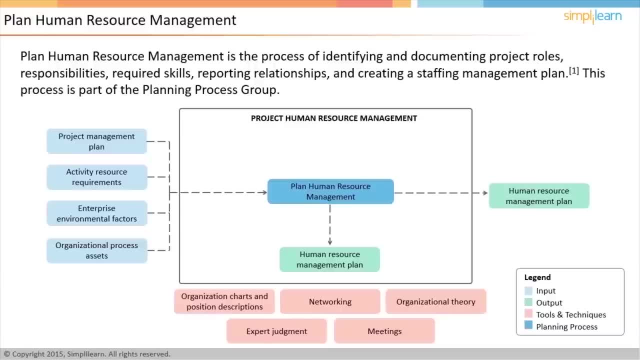 matrix. The staffing management plan is a comprehensive document that describes when and how team members would be added to and released from the project. Another component of the staffing management plan is the recognition and reward system. Recognition and reward system helps project managers motivate their team. The staffing management. 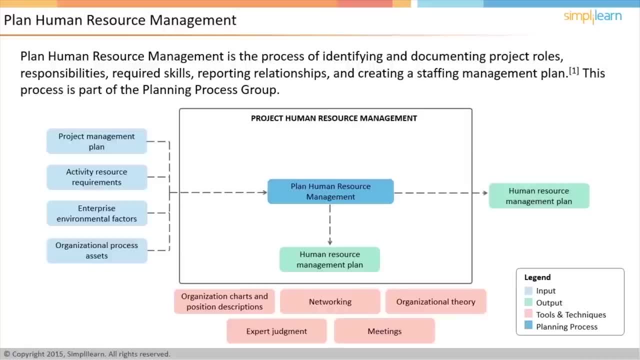 plan is relevant to the projects of a functional or matrix organization, where project team members are always caught in a dilemma about prioritizing project work against regular departmental work. In the next screen, let us discuss organization charts and role descriptions A project manager needs to make. 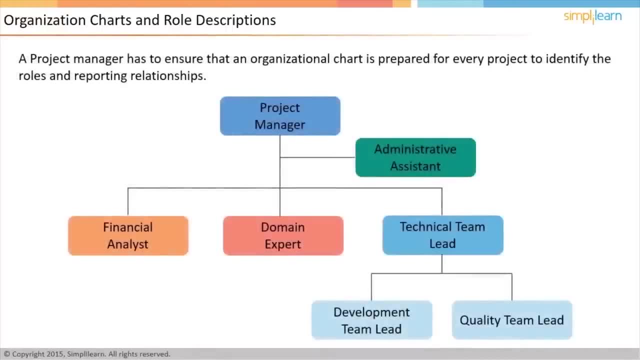 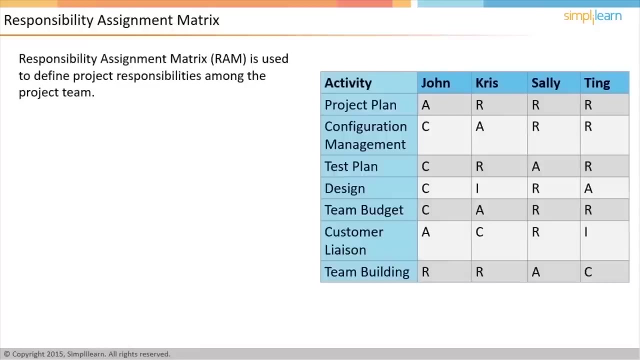 sure that there is an organization chart prepared specifically for the project. It should clearly identify the roles and the reporting relationships between them. A sample organization chart is shown on the slide. Another way of clearly delineating responsibilities among team members is by using a responsibility. 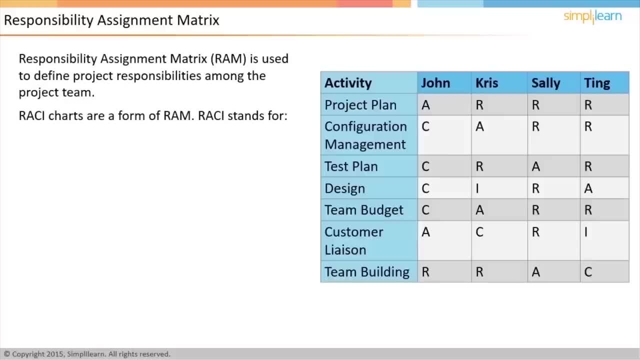 assignment matrix. One form of responsibility assignment matrix is the RACI chart. In the RACI chart, R stands for responsible, A for accountable, C for concerned or consulted and I for informed For each important activity or deliverable on the project. 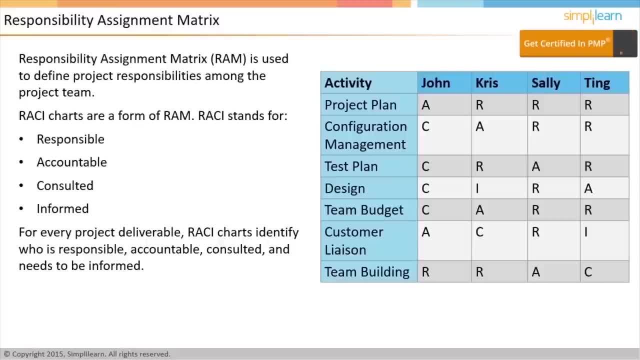 it needs to be clearly identified who is responsible or contributes to it, who is ultimately accountable, who is merely concerned about the success and who needs to be informed or kept in the loop. An example of the RACI chart is shown on the screen. 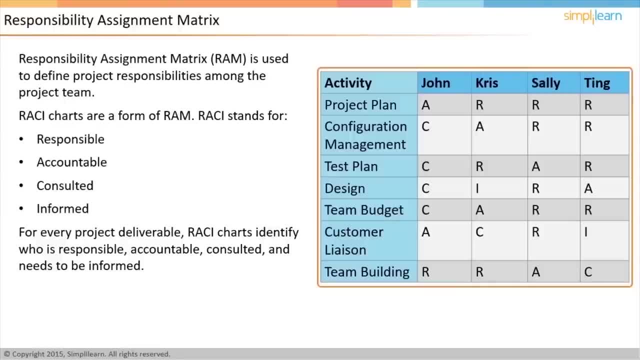 In this case, project manager John is accountable for the project plan, and the other team members, Chris, Sally and Ting are responsible for completing the plan. Similarly, you can note the roles of each resource in the other activities In the next screen. let us 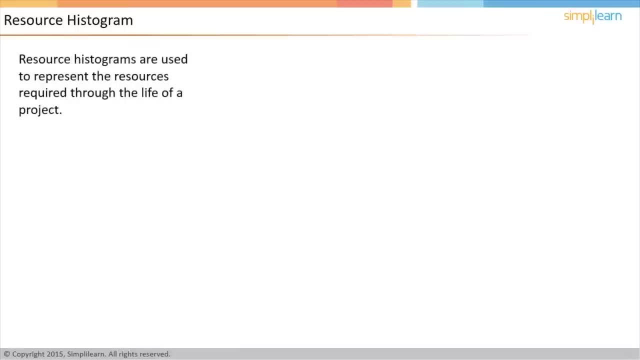 understand resource histogram. Resource histogram is a method of depicting how many resources are required for the life of a project. If you observe the chart shown on the screen, it indicates that the number of staff hours required on the project increases to a peak in 2014 and then slowly. 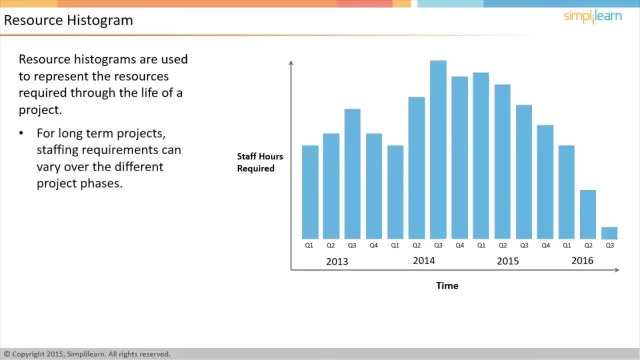 tapers off. Especially for long-running projects, the level of staffing needed may vary considerably over a period. This has implications for other parts of the plan as well. For example, the cost will vary as the number of resources change. This piece of information helps a. 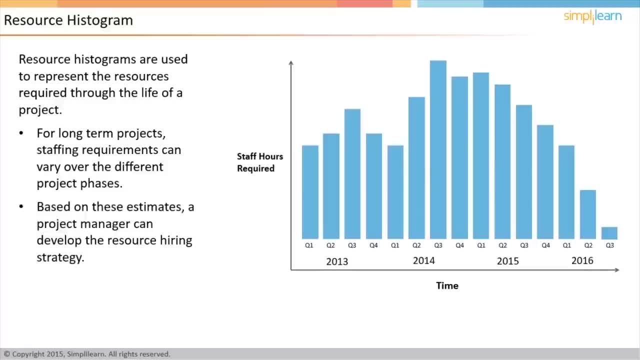 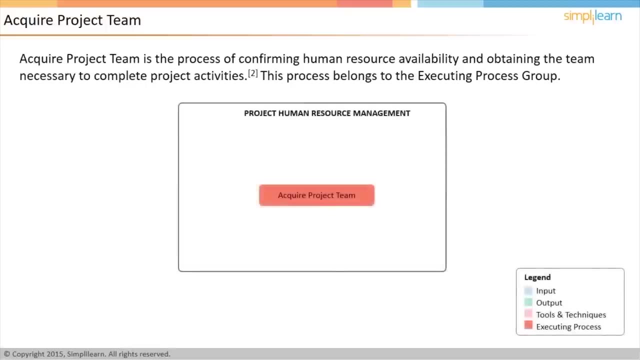 project manager to understand at what time they need to on-board and off-board resources on a project. In the next screen let us look into the second human resource management process, that is, acquire project team. Acquire project team is the process of confirming human resource. 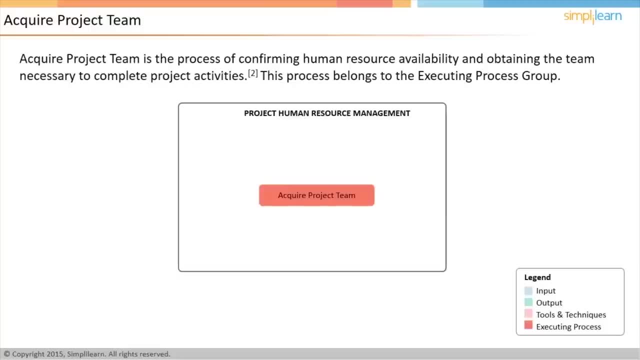 availability and obtaining the team necessary to complete project activities. This process belongs to the executing process group. Acquiring resources may not be required in the planning phase. Therefore it is done in execution phase. Though you may plan to acquire few in the planning phase, major acquisition. 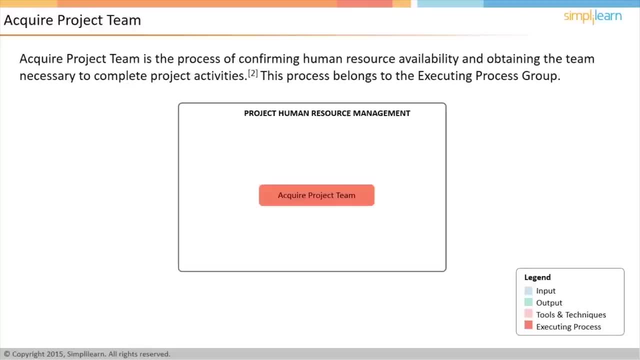 is done in execution phase. This may be true where large projects are run spanning over many years, with several detailed activities. The key input is the human resource management plan. Enterprise environmental factors help understand which team members will be available to work on the project, how much they will. 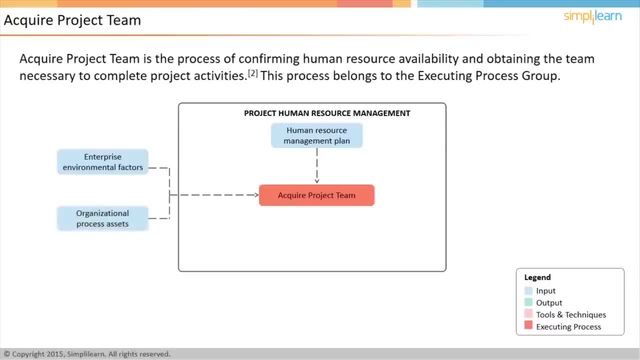 cost, etc. Organizational process assets will help understand the hiring procedure of the company, the policies that govern the use of team members on the project, etc. The key technique for acquiring the project team is negotiation. As a project manager, you have to negotiate. 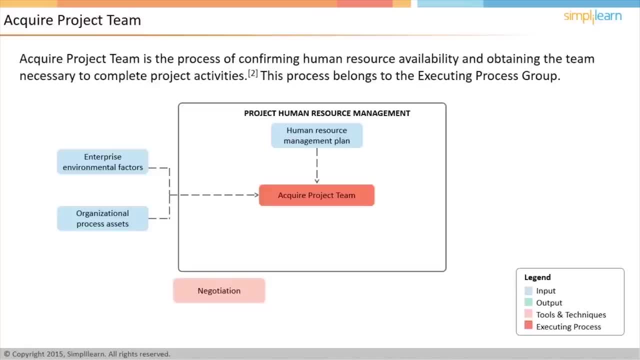 with the company's senior management, resource manager or with prospective candidates to secure the most suitable resources on the project. Sometimes the resources may be pre-assigned to a project. This typically happens when they are the key resources without which the project cannot take off. 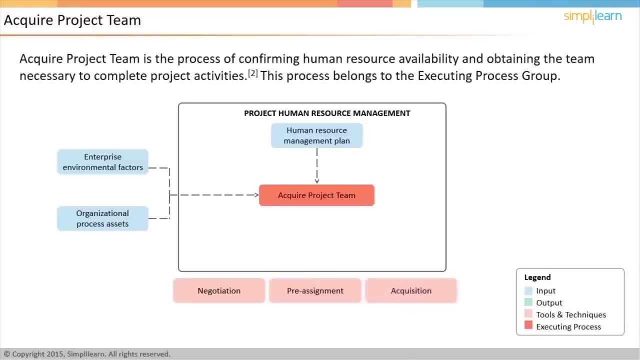 Sometimes the project team is acquired by getting required resources through external vendors. Most of the bigger organizations have approved list of vendors who provide resources on a contract basis. Nowadays the concept of virtual team is also quite popular to get a project team. So even though the project is 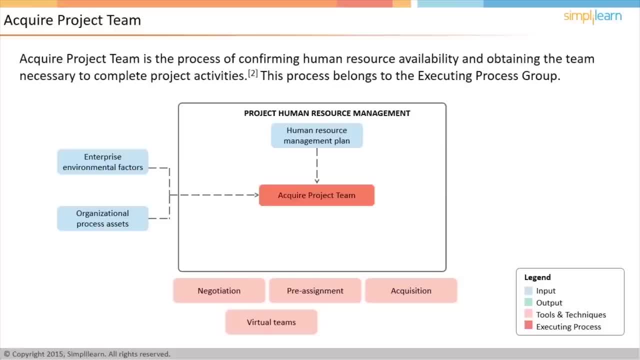 being conceived in one country, a big part of the team can be in another country. For example, if the project is conceived in the USA, majority of the team can be in Germany, and both the teams can coordinate over the phone, email, chat etc. 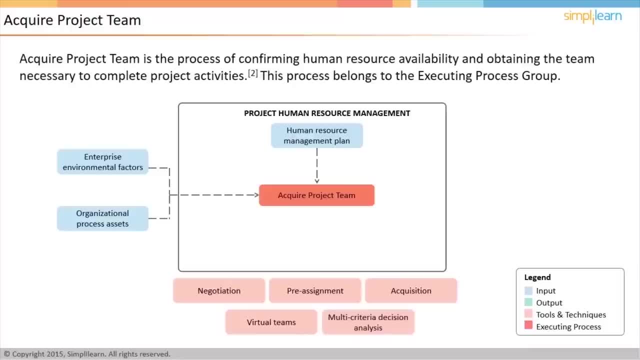 Multi-criteria decision analysis is also an important part of the project. While acquiring the human resources for the project, it is important to consider a number of factors such as availability, cost, skill set, experience, attitude, relocation needs, etc. 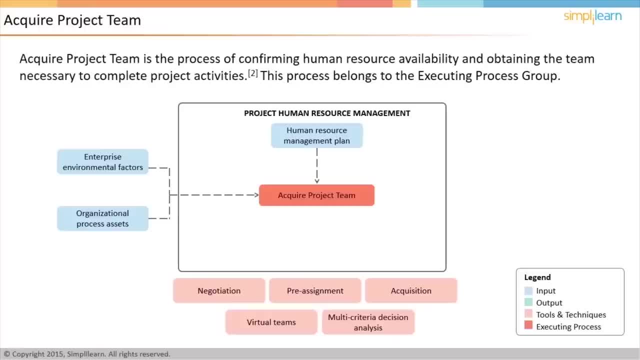 These criteria have to be considered in totality and balanced out against the project's requirements. The output of this process is project staff assignments, resource calendars and updates on project development and development Project management plan. Let us now discuss the next process: develop project team. 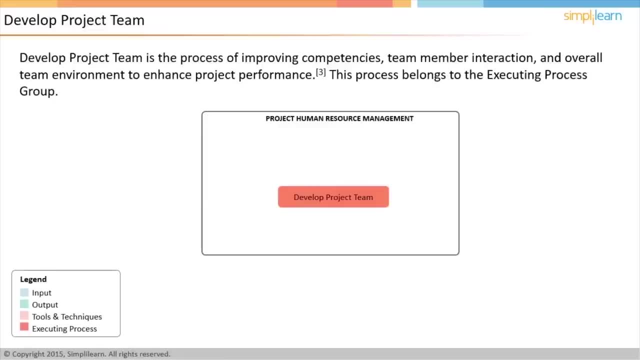 Once the project team is acquired, the next step is developing the project team. Develop project team is the process of improving competencies, team member interaction and overall team environment to enhance project performance. This process belongs to the executing process group. The inputs: 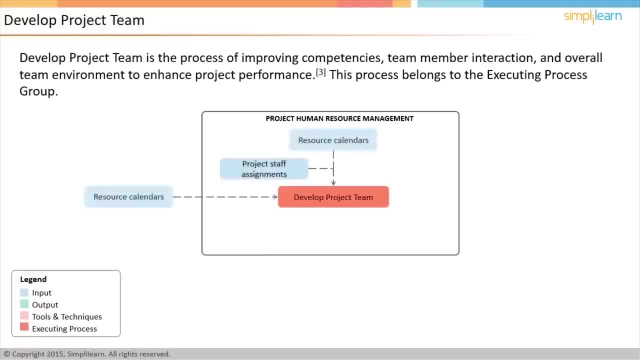 to this process include project staff assignments, resource calendars and human resource management plan. One of the techniques used in developing project team is interpersonal skills. It is more of an art than a science, and this is where individual characteristics of project managers matter a lot. 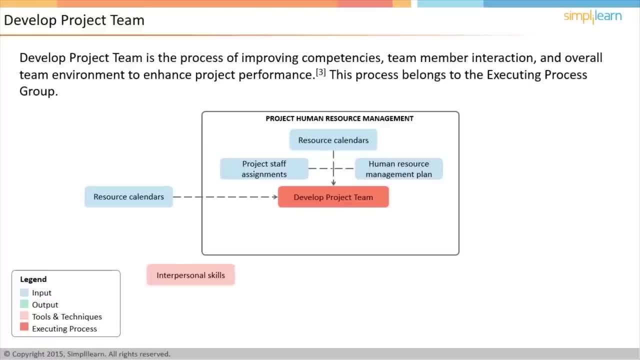 If the project manager genuinely commands trust and respects the team members, developing the team becomes easy. Team members look up to the project manager not only for getting projects, specific instructions, but also for their career advancement as well. Social activities like celebrating a team member's birthday going. 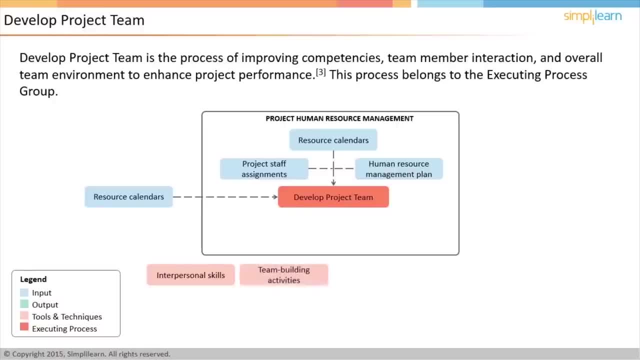 for parties outside the office, etc. helps in team building. Training is also an important tool for developing the project team, as it helps in increasing the knowledge of competencies of the team members, Sometimes co-locating the team members at a single place also. 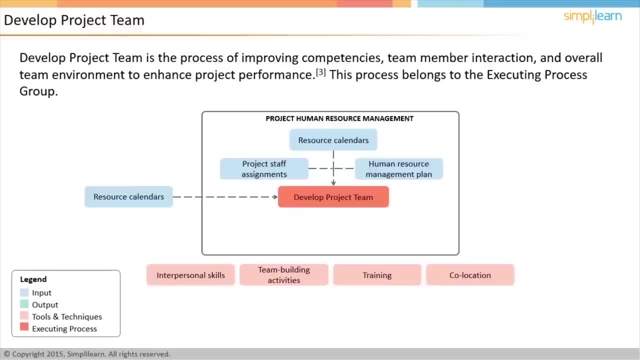 helps in developing team bonding. This is especially important if team members work from different geographical locations. Knowing a person face-to-face does help in reducing conflict. Project managers can also encourage the team members by providing recognition and rewards. Personnel assessment tools give the project manager insights into 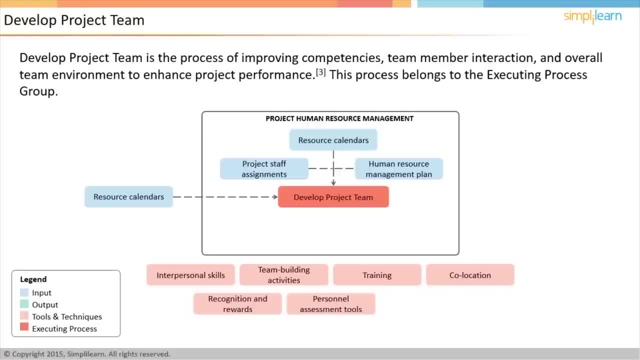 the strengths and opportunities for improvement in the team members. These tools also help in understanding members' aspirations so that the project manager can better align the project goals with the individual aspirations. Finally, the project manager should also set some ground rules in the project to ensure that team 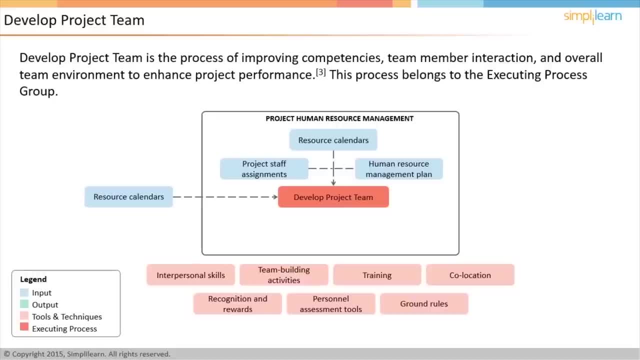 performs their work without any problems. Some such rules can be: everyone should reach office for daily meeting by 9.30 am sharp. If there is more than a 10% delay in completing any activity assigned, it should immediately be escalated to. 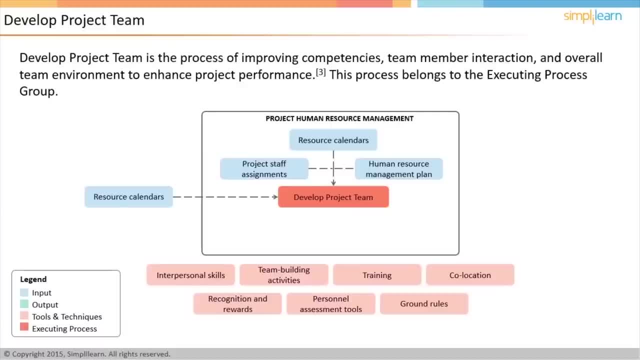 project manager. If there are any unforeseen circumstances, it should be immediately brought to the notice of the project manager, etc. The output of this process is team performance assessments. This is done by the project manager to evaluate and enhance the effectiveness of the team as a whole. 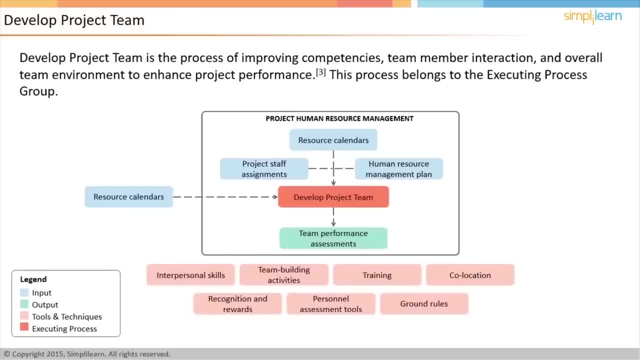 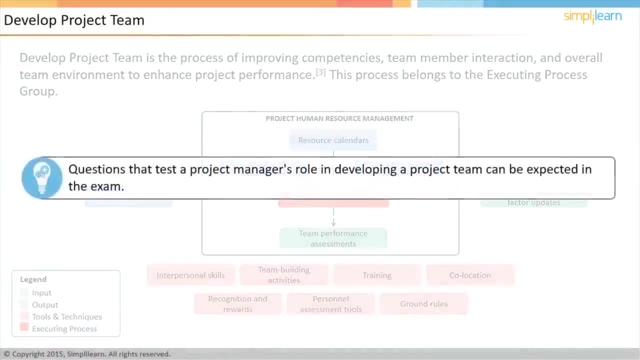 This is a document which explains team effectiveness. As information about the team evolves, the enterprise environmental factors may also be updated. Questions that test a project manager's role in developing a project team can be expected in the PMP exam. So ensure that the team. 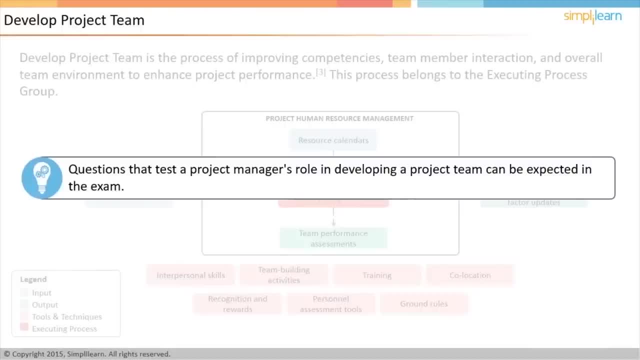 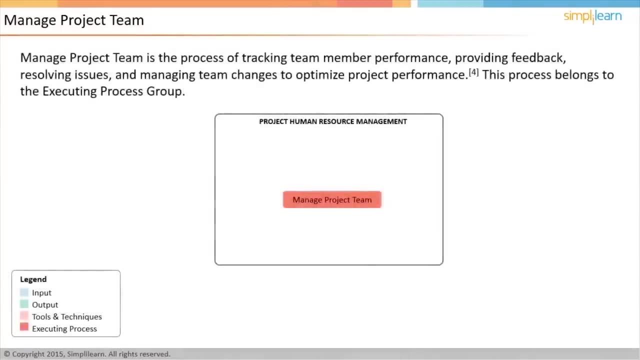 has a fair understanding of the role. before you take the exam In the next screen, let us discuss the Manage Project Team process. Managing the project team is different from developing the project team, though it is also done during the execution process group. It relates to measuring team members'. 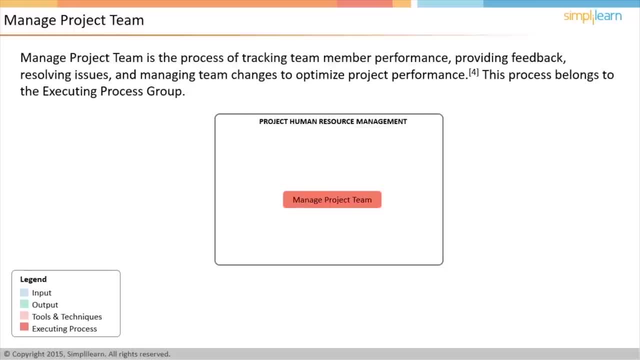 performance, providing feedback, resolving issues and managing changes to optimize project performance. To measure team members' performance, the manager should know the work assigned to them, as well as their performance on the assigned work. Hence project staff assignments and team performance assessments. 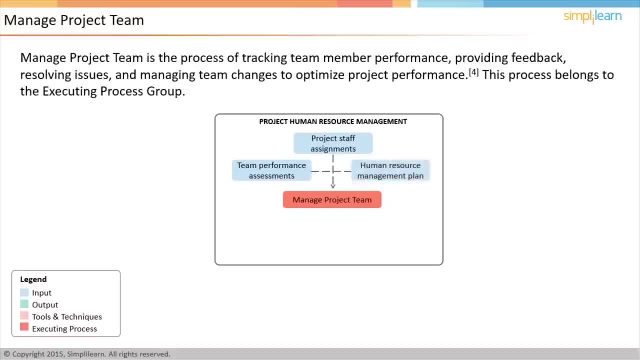 are listed as input to this process. The Human Resource Management Plan serves as a guideline for managing project teams. Some organizations have templates and procedures to do such assessment, and that being the reason why Organization Process Asset is also one of the inputs to this process. 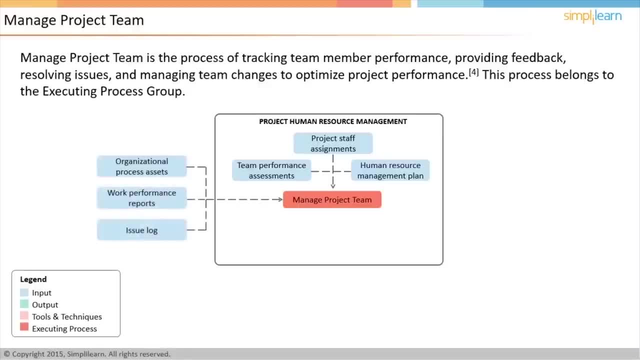 The work performance reports, as well as issue logs, will be inputs because the team management activities have to be performed. in this context, Observation and conversation is a technique where the project manager monitors and discusses the tasks done by the team. This does not imply formal. 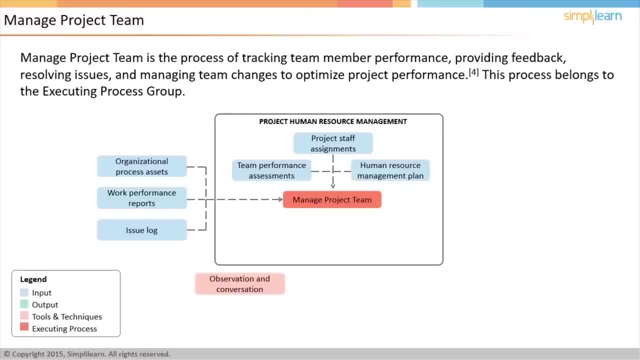 project status reports, but having an informal interaction with the team before documenting the project status report. Knowing about the issue early, helps in resolving them early. Formal performance appraisals are helpful in evaluating the team members' performance on the project. The project manager creates these. 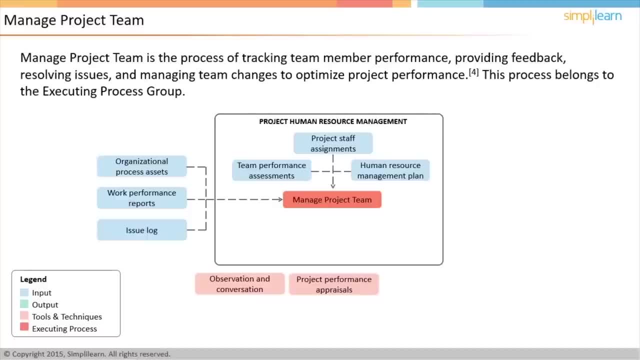 with the help of the team supervisors. It is an established practice in most organizations to evaluate team members for their work. This may have a bearing on their future assignments, salary promotions, etc. Since the power of appraising lies within the project manager. 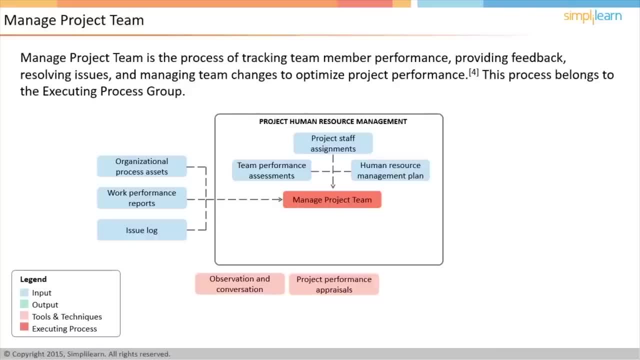 the project manager can use this as an effective tool for managing the team. Since multiple resources on a single project, it is quite natural to expect conflicts. It is the responsibility of project manager to resolve conflicts. Conflict management has been discussed in detail later in the lesson You can expect. 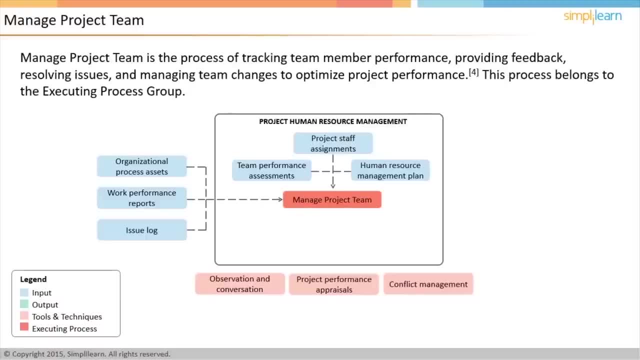 questions on conflict management in the exam. The other tool is interpersonal skills. The output of managing a project team includes corrective action, recommendations like which team members to be changed, implementing some reward system to motivate the team, etc. Updating the project management plans documents. 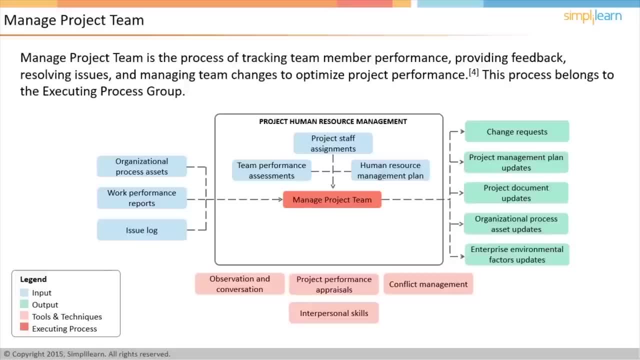 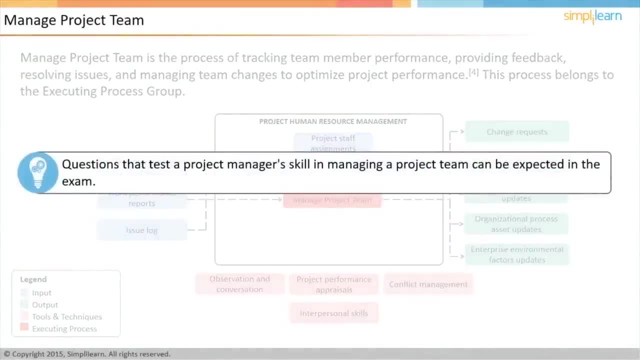 organization, process, asset and enterprise environmental factors are the other outputs of this process. There can be questions in the PMP exam that test a project manager's skill in managing a project team. So ensure that you are aware of the inputs, tools and techniques and outputs of 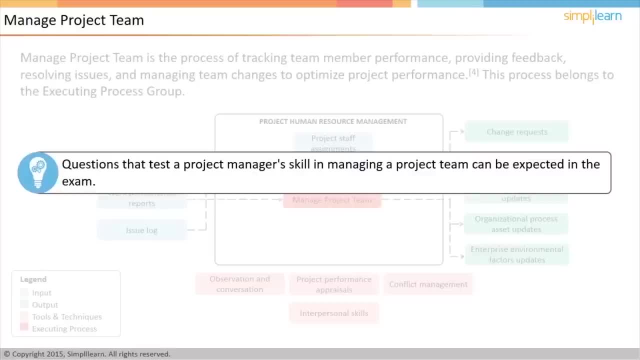 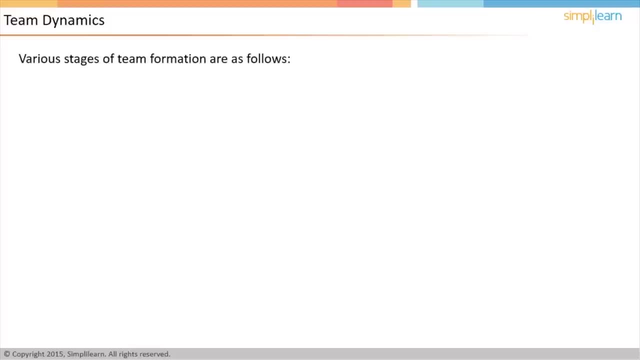 managing a project team. Let us discuss team dynamics in the next screen. Any team naturally goes through several stages as it gets together. These stages are forming, storming, norming, performing and adjourning. In forming stage, a team formally comes together. 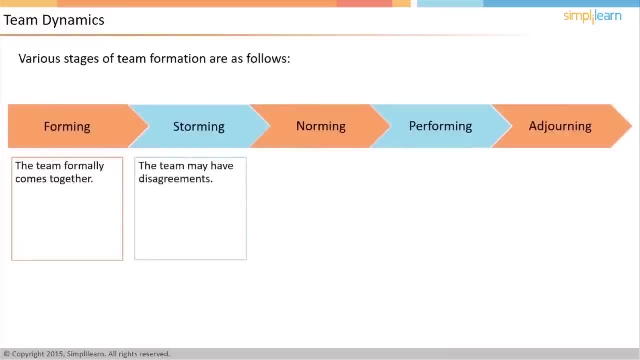 for the first time In storming stage, disagreements start to surface. This is followed by norming. when the teams start working together and trusting each other In performing stage, they are able to deliver results as a team. Finally, the team is. 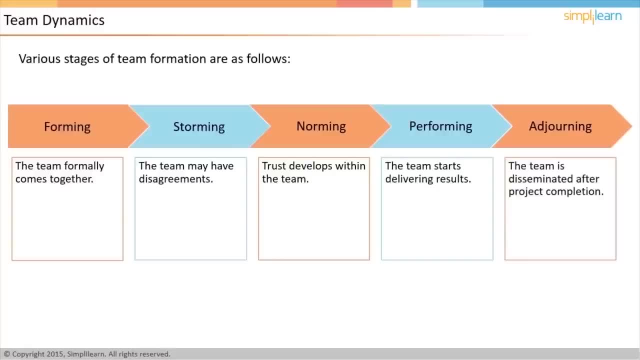 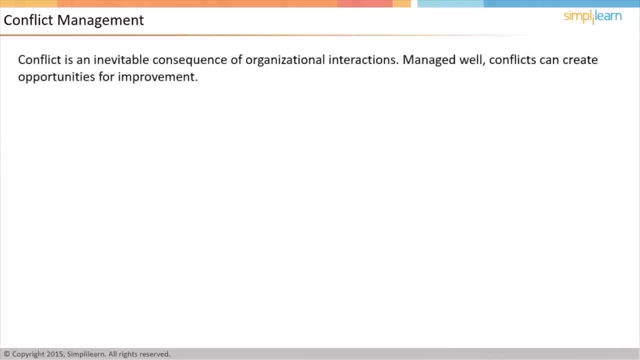 adjourned when the work of the project is completed or the project is terminated. In the next screen, let us discuss conflict management. Many organizations look for people with diverse backgrounds to get different perspectives about work. If people with diverse backgrounds and culture work on a project, it 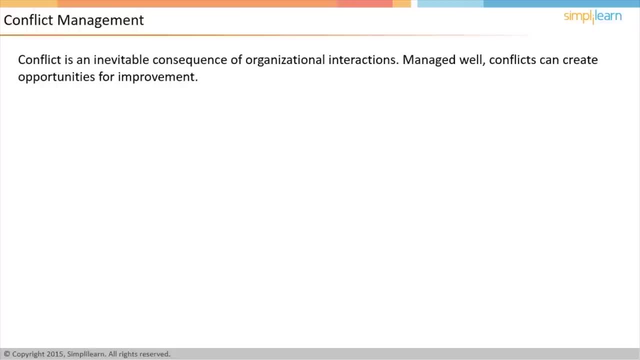 is quite natural to expect conflict. Conflict often results in opportunities for improvement. The root causes of conflict can be scarce resources, scheduling priorities and personal work styles. While the popular belief is that personality or ego can be the key reason for conflict, it is. 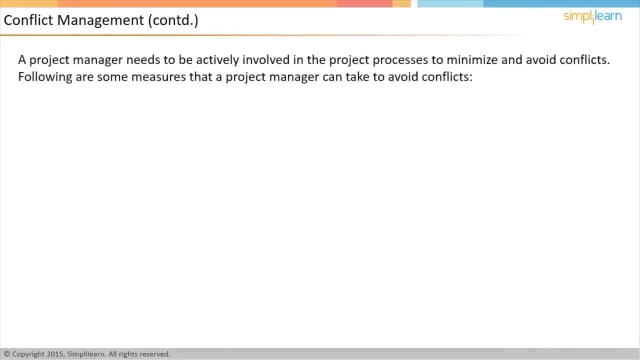 the least possible reason for conflict. As a project manager, if you find yourself in between a conflict with a team member, sit across the table and resolve it. If not, they should get their immediate managers involved and try to resolve it To avoid conflicts a project. 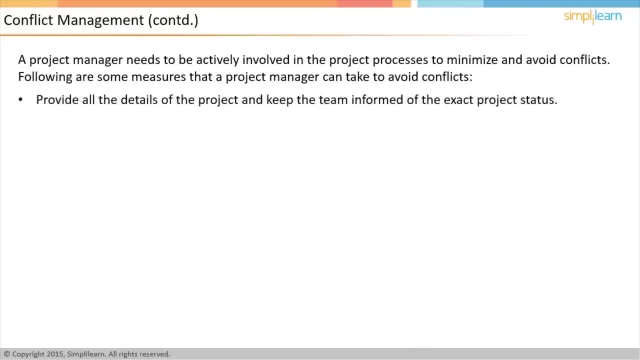 manager should let everyone involved have complete clarity about the project, Assign the roles and responsibilities to each of the team members. clearly Ensure that there are no overlapping responsibilities, which could be a possible cause for conflict. Sometimes, boredom at work can also lead to conflict, So one of the 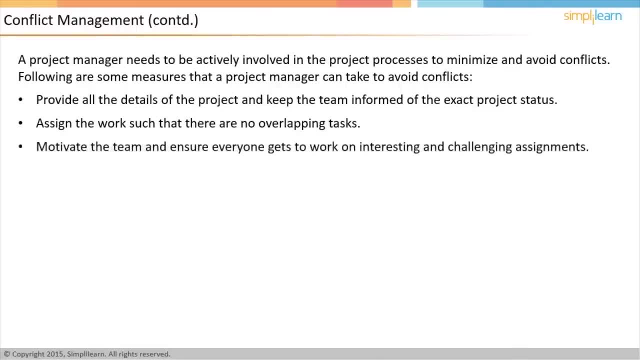 responsibilities of project manager is to keep motivating the team members and let them work on interesting and challenging assignments. Business scenarios based questions on conflict management can be expected in the PMP exam, so it is essential to have a fair understanding of the topic In the next screen. 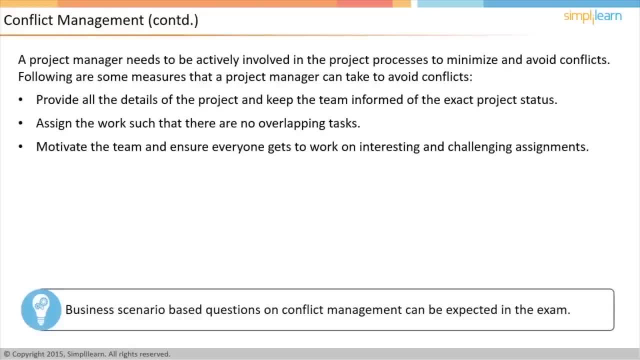 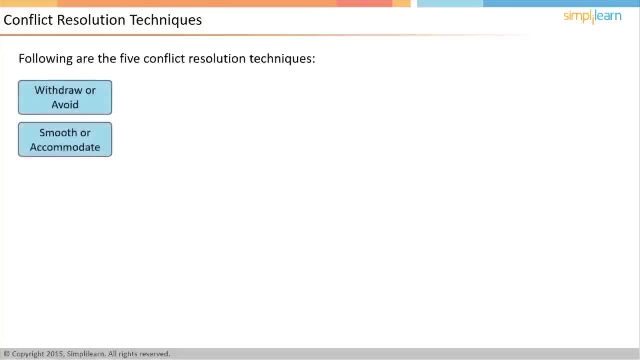 let us look at conflict resolution techniques. There are five techniques of resolving conflict. They are: withdraw or avoid, smooth or accommodate, compromise or reconcile, force or direct, collaborate or problem solve. In withdraw or avoid, one retreats from a potential conflict. 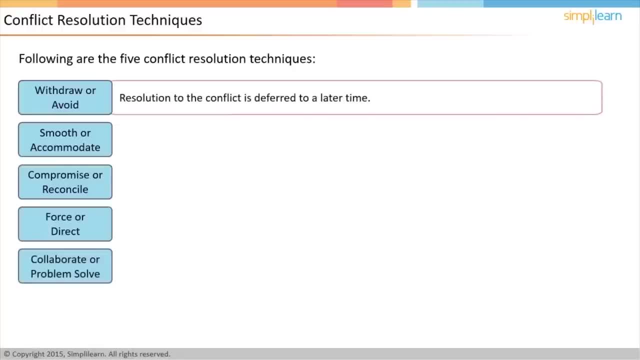 situation or defers the resolution to a later date. This does not resolve the conflict but allows for more time In smooth or accommodate. areas of agreement are emphasized to reduce the intensity of the conflict. Again, this does not on its own 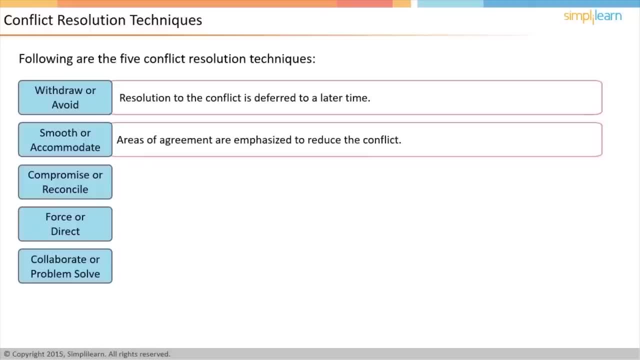 result in a resolution, but it may succeed in changing the perceptions about the situation. In compromise or reconcile, there is some give and take in order to bring some satisfaction to all parties. Depending on how the process went, this may be perceived as a 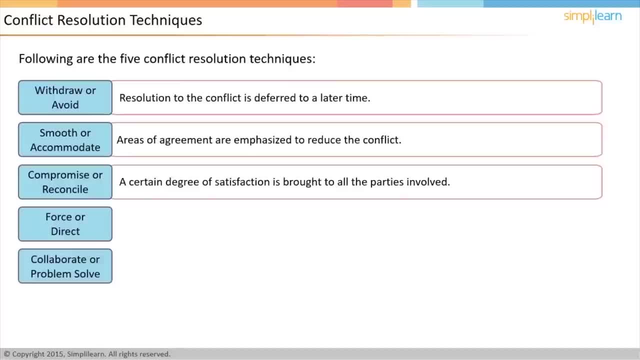 win-win or a lose-lose situation because none of the parties really get what they want In force or direct. a person in a position of authority directs how the matter should be resolved. It may be necessary to do this when the matter has to be resolved immediately. 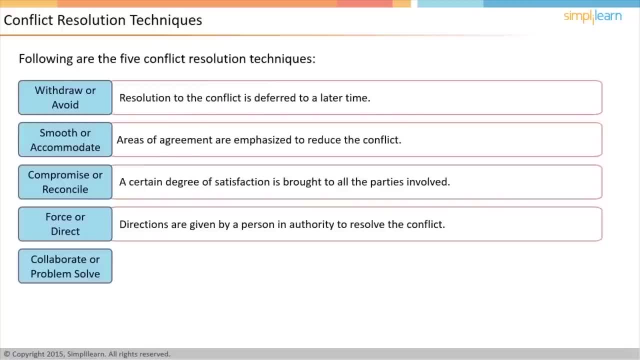 However, this may result in upsetting one or more of the conflicting parties In collaborate or problem solving. the parties in the conflict are asked to come together to collaborate and look for a resolution to the problem. This offers the greatest likelihood of a satisfactory and permanent resolution. 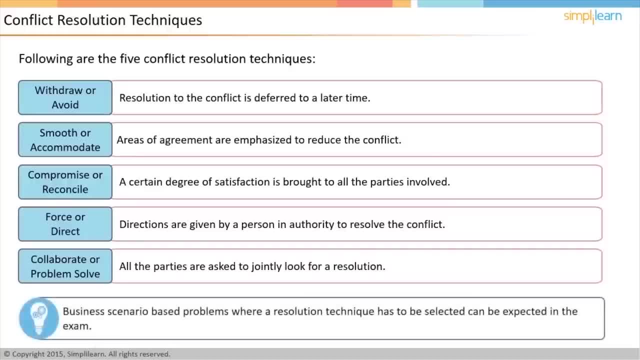 and should be resorted to whenever possible. Business scenario-based problems where a resolution technique has to be selected can be expected in the PMP exam. So understanding the conflict resolution techniques is essential. In the next screen, let us look into a business scenario. 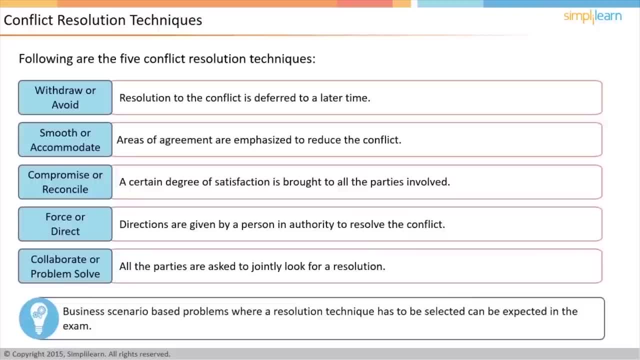 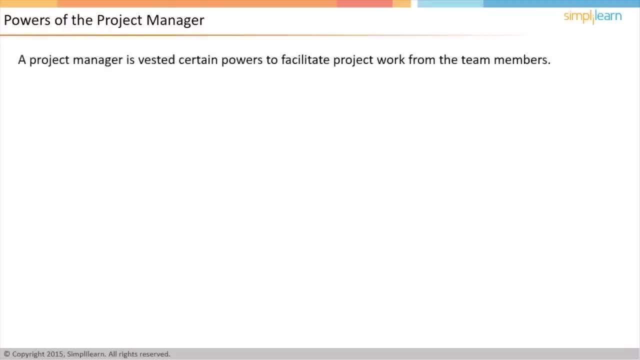 to understand this concept better. After reading the problem statement, click the solution button to look at a possible answer. The first thing to do is to get the work done by the team. There are certain powers that a project manager can use to get the work done. 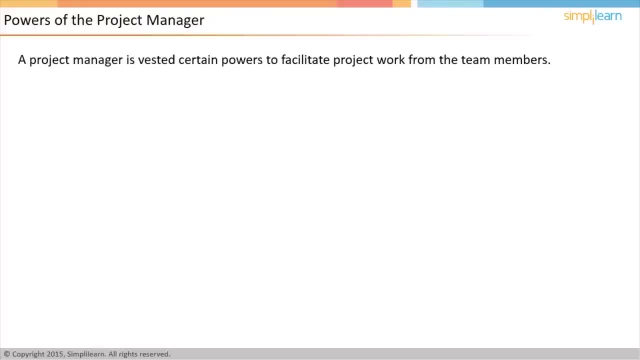 A project manager has to use a combination of techniques to get this accomplished. Various powers of a project manager are legitimate or formal, reward, penalty, expert and referent. In legitimate or formal project manager can formally assign a work to a team member. 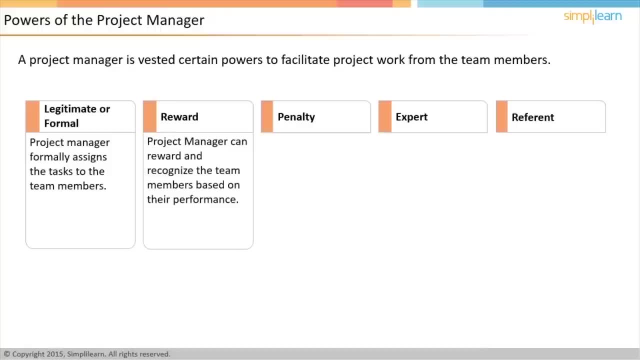 that he or she has to do. The reward could be as simple as assigning challenging or sought-after work to a team member. This can motivate good performers on the project. Sometimes project manager can penalize the team members for poor performance. Some project managers are able. 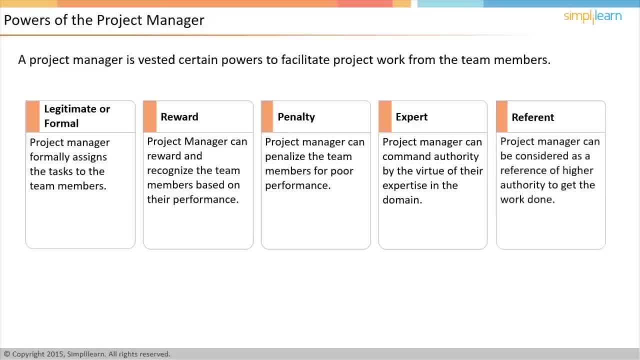 to command authority because of their expertise in a certain field, Project manager can be considered as a reference of higher authority or personal charm or charisma of the project manager. Legitimate reward and penalty are the powers derived from the project manager's position in the company. 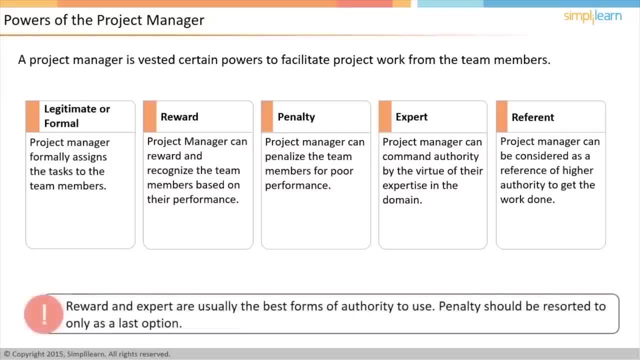 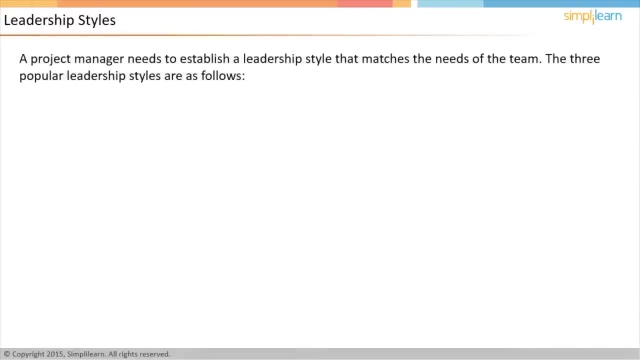 Expert power exists when the project manager is an expert on the subject matter. Reward and expert are usually the best forms of authority to use. Penalty is the worst way of influencing and managing the team. A project manager should resort to this only as a last option. 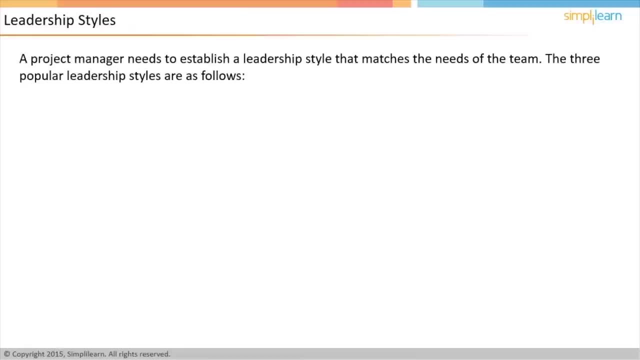 Having formal reporting authority over the team, they are naturally looked upon as the leaders for their projects. Project managers need to be familiar with the leadership styles and be able to tailor their style according to the needs of the project and that of the team. There are three leadership styles. 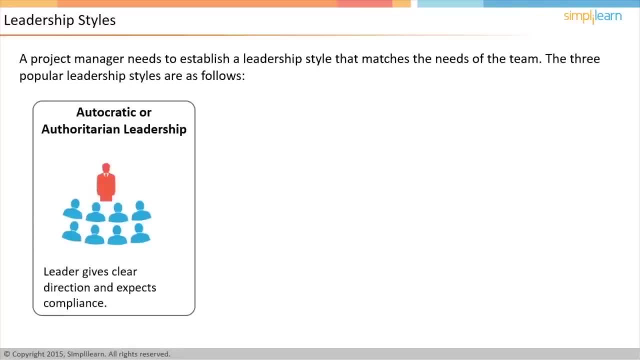 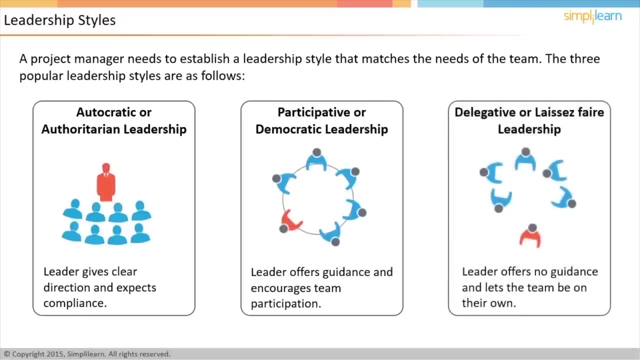 The first one is authoritarian or autocratic. In this style, the leader sets clear expectations of the team and expects complete compliance. The leader offers guidance, but also involves the team in decision making. In a delegative or laissez faire style, the leader leaves the work to the team. 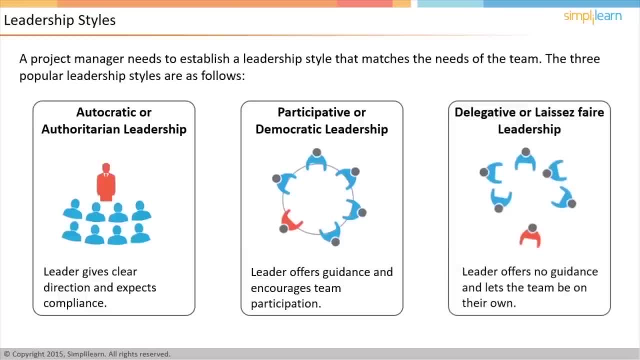 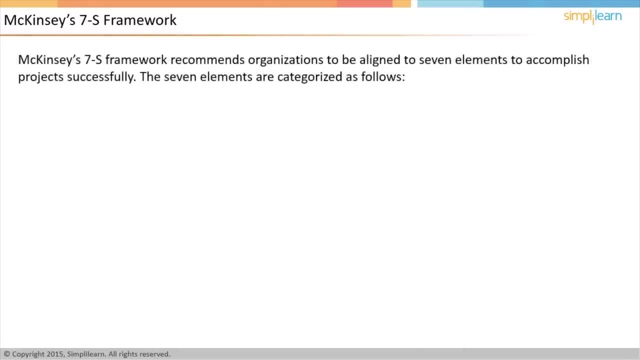 without offering much guidance. In most circumstances, you would want your leader to employ a participative style, but there may be occasions when other styles might be appropriate. In the next screen, let us discuss McKinsey's 7S framework, A popular framework in management science. 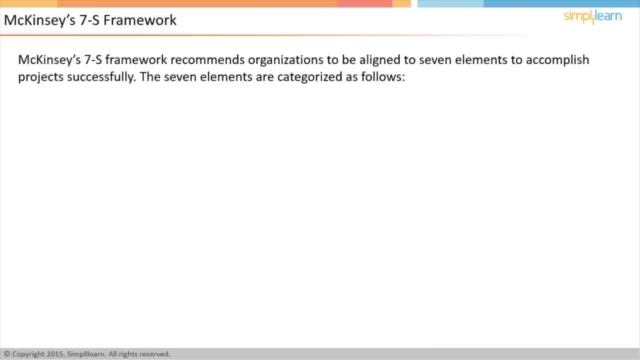 is the McKinsey's 7S framework. There are seven elements that are divided into two categories. An organization working on a project will have these elements already in place and hence these become the hard elements, The first three elements of the 7S framework. 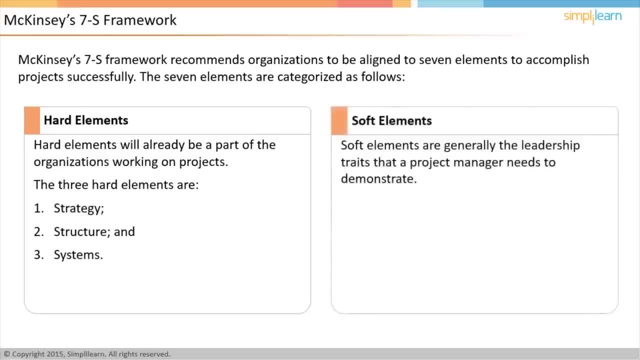 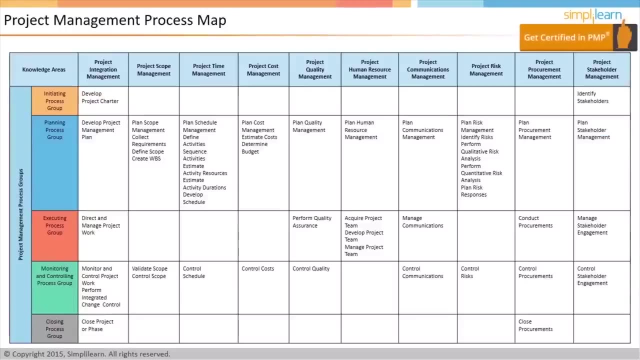 are the strategy, structure and systems. The leader or project manager is expected to step in and exhibit soft elements to earn the mantle of leadership. The next four elements are shared values, skills, style and staff. There are 47 processes in project management. 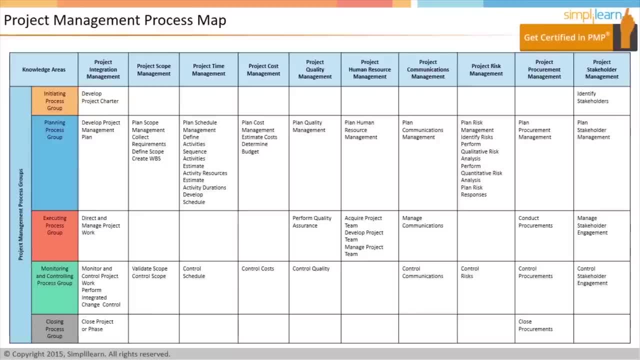 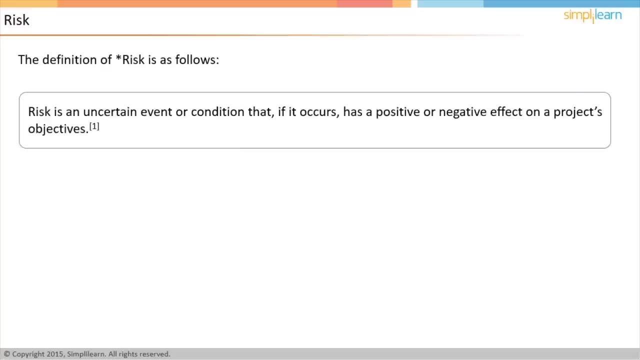 grouped into ten knowledge areas and mapped to five process groups. In this lesson we will look at the eighth knowledge area, that is, project risk management and its processes. Risk is an uncertain event or condition that can affect a project positively or negatively, Although most of the time 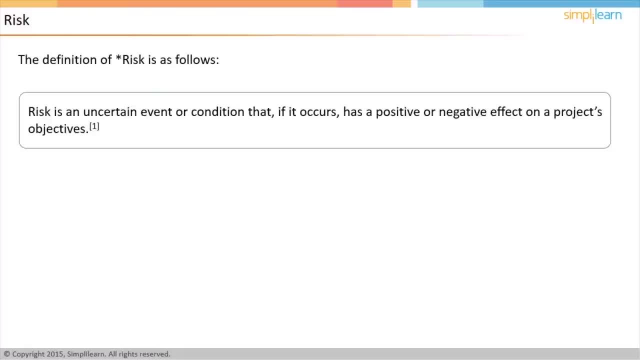 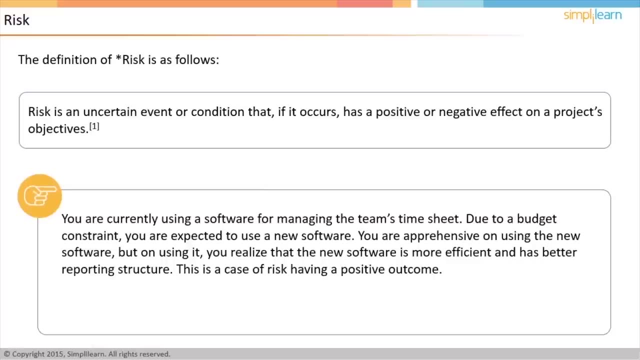 you view this uncertainty as bad. sometimes it also has a likely positive outcome. Risk is an example of risk having a positive outcome. You are using a software for managing timesheet of your team members. Due to budget constraints, you are forced to use a new software. 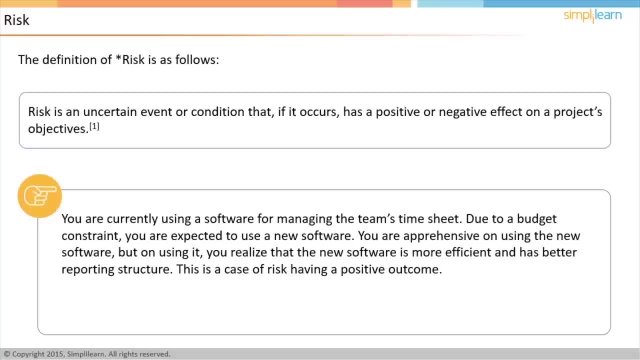 Though you were initially reluctant to use it, you found the new software to do better than the current one. It is more efficient and has better reporting facility. An example of bad uncertainty can be swine flu. Government declares a mandatory holiday to check flu spread. 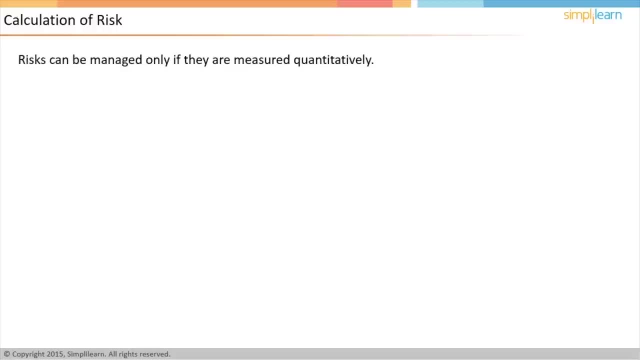 but the government does not allow it. Risk can be managed only if they are measured quantitatively. Suppose there are many risks identified in a project and you have limited resources to manage them. You should know which risk is most important that has to be managed first. 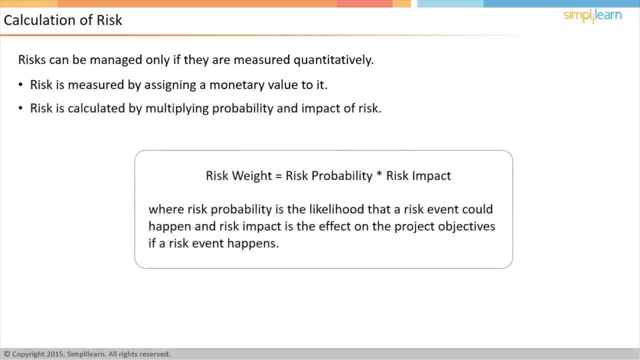 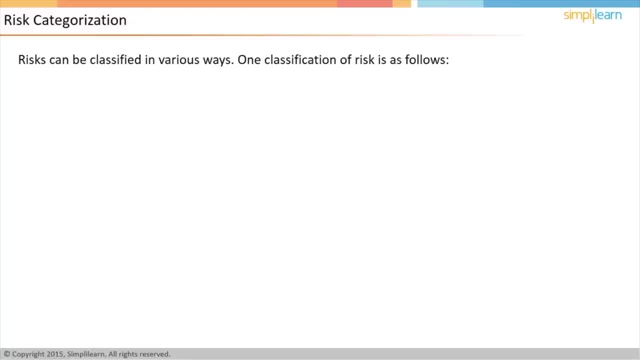 Therefore, measuring risk becomes very critical. Risk is measured by assigning a monetary value to it, which can be categorized in various ways. One such categorization is external, internal, technical or project management related risk. External risk arises out of external policies or regulations. 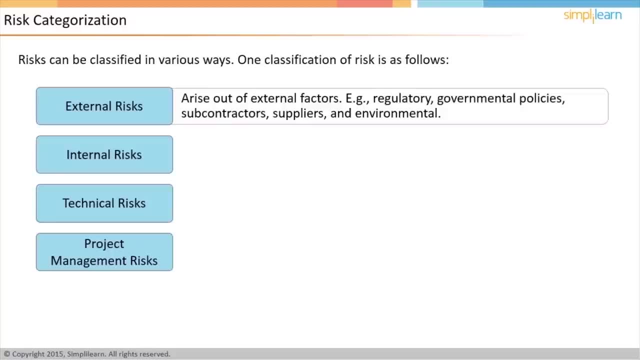 For example, government policy that the river water can be used for drinking purposes may hinder your production, which is dependent on the river water. Internal risk arises from within the project. For example, the complexity of the project may result in time and cost escalation. 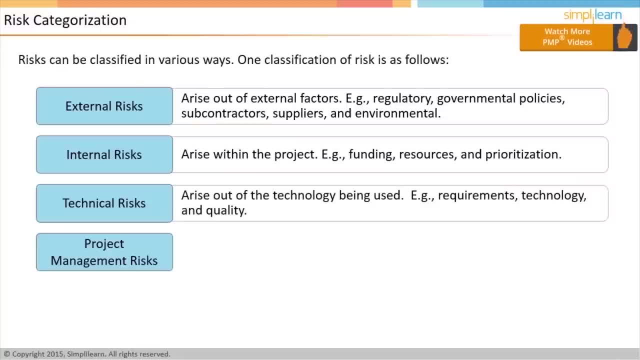 Technical risks arise from the technology being used. Projects in space exploration have a lot of technical complexity. Risks could be related to project management. For example, if there are many interdependencies between the sub-projects, it is a risk from the project. 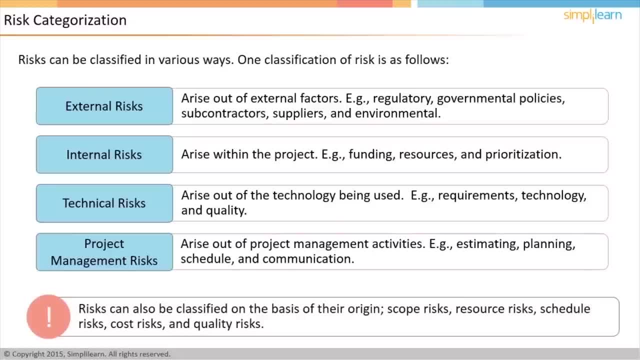 management standpoint. The categorization of risk can be based on the origin. There are two types of risk: Resource risk, schedule risk, cost risk and quality risk. Scope risk can include redoing the same task if the scope is not well understood. 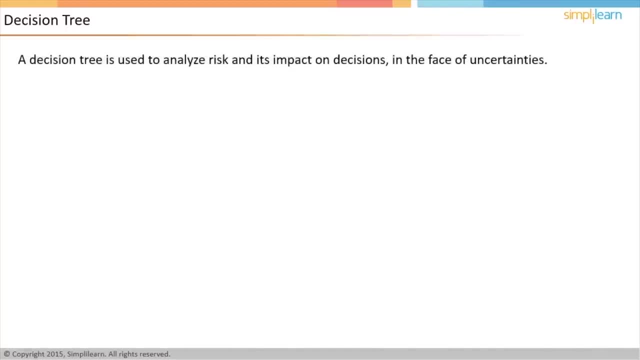 When the only resource is assigned to some other project, it is called resource risk. A decision tree helps in analyzing risk and its impact on making decisions in a scenario where there is uncertainty on the outcome. A new car or an old car? Which one should you buy? 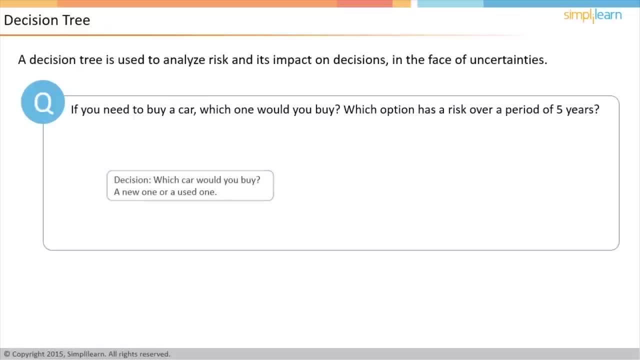 Which has more risk over a period of five years. Consider the concept of decision tree to solve this problem. The initial cost of buying a new car is $20,000, and the cost of buying an old car is $15,000.. For a new car, 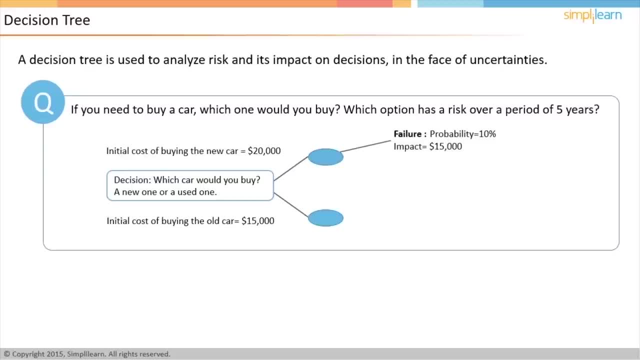 the probability of it having any problem is only 10%. That is, there is a 90% likelihood that the car will not work without any problems- past scenario- and if it does have any at all, the impact of the problem is $15,000. 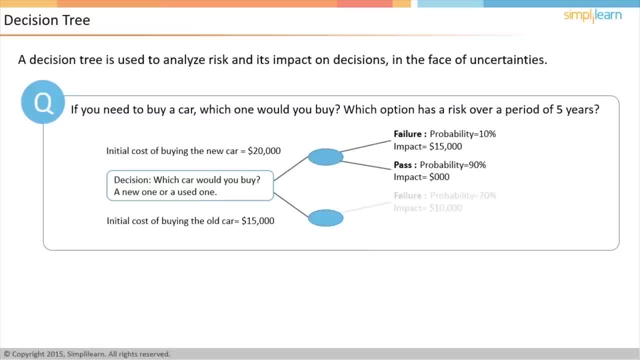 The reason is that it was bought at a higher cost. An old car has 70% probability of having a problem, The reason being. the probability is high because the car was already used by someone else in the past. However, the impact here is low. 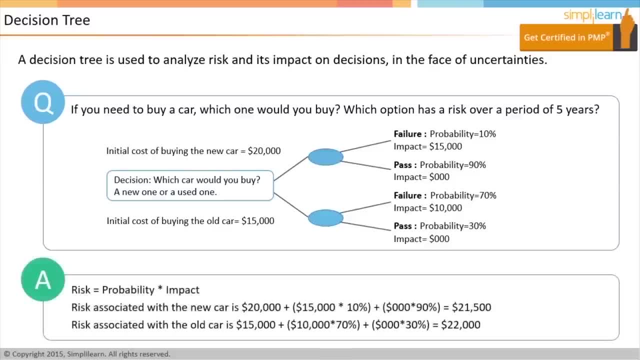 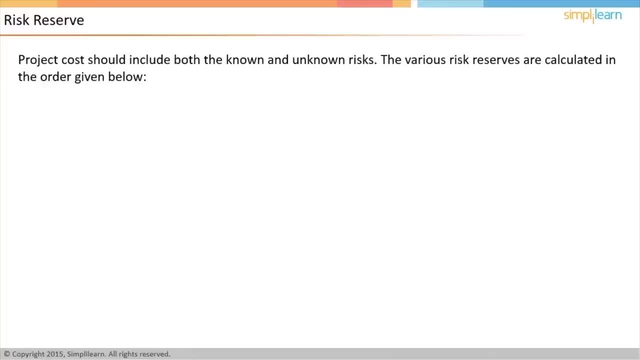 say $10,000.. Considered by impact of both the options at the decision nodes, you will find buying an old car over a period more risky than buying a new car. The project cost will be arrived at after considering the risk reserves of both the known risks. 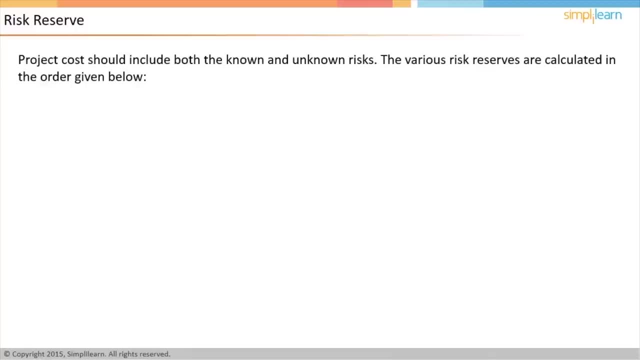 and unknown risks. There is a specific order in which these reserves are calculated in the project cost. First, the cost of all activities is identified. Activities are the smallest and all the activity costs add up to the cost of the work packages. Work packages are the last level. 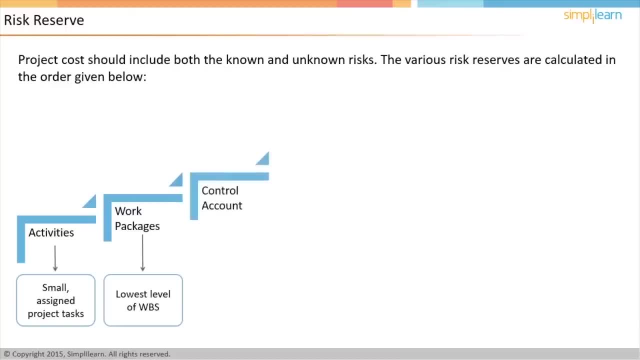 of classification. in a work breakdown structure, Work packages cost adds up to the control account cost. One or more work packages are clubbed together to create a control account and manage the cost of the work packages. Next the project costs are identified. There can be multiple control accounts. 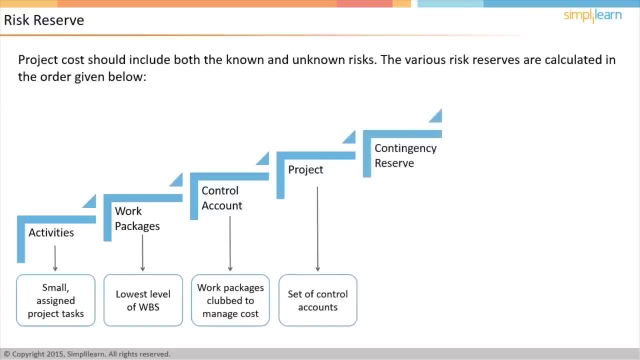 in a project. Now, once the project cost is calculated, some reserve is added to take care of any uncertainties. You may have made some assumptions to calculate the cost of the activities and by adding some reserve you would want to take care of those uncertainties. 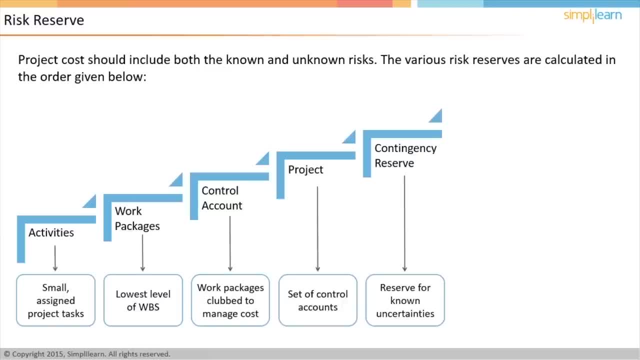 In this case, make a note that you are accounting for the assumptions made and it can be said that this reserve takes care of known uncertainties. This reserve is also called contingency reserve. It is the cost for the project that will be used for budgeting and tracking purposes. 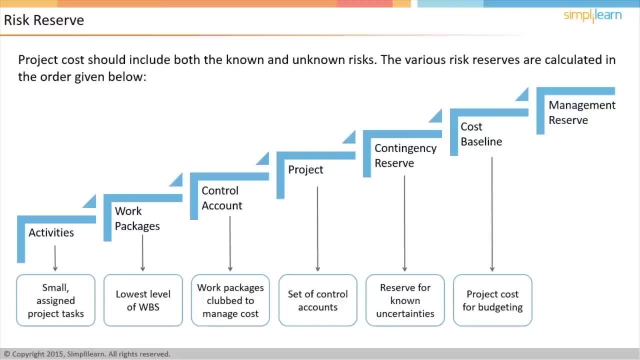 Once the planned cost is arrived, there is another reserve that gets added, called management reserve. Note that management reserves are not part of the cost baseline and are used during emergencies only. By adding contingency reserve, you have taken care of known uncertainties, and by adding management reserve 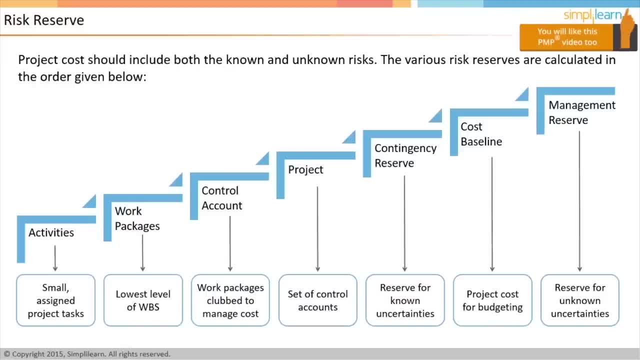 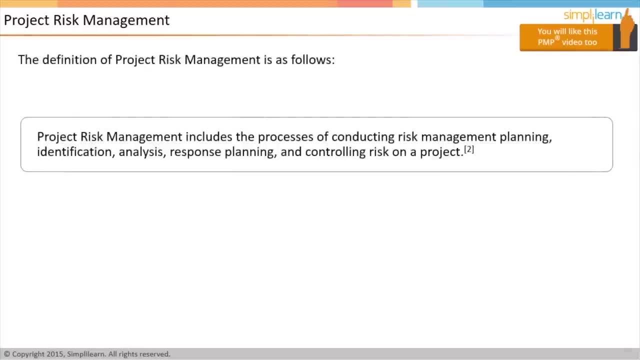 you take care of unknown uncertainties which perhaps have not yet been identified. Unknown uncertainties are added based on experience or expert judgment. Project risk management includes the processes of conducting risk management, planning, identification, analysis, response planning and controlling risk on a project. 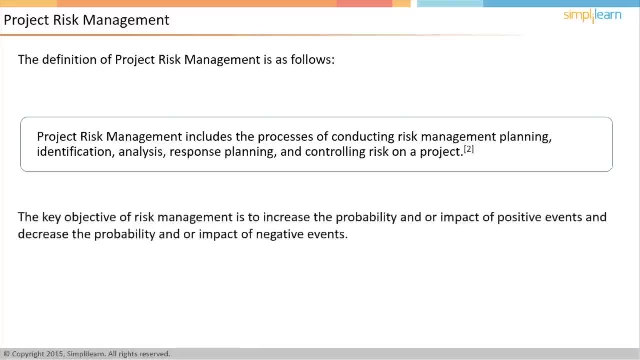 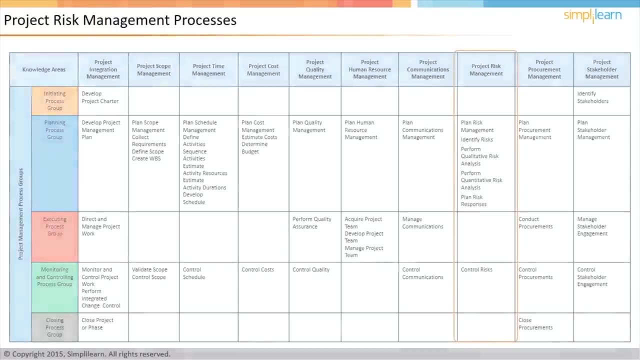 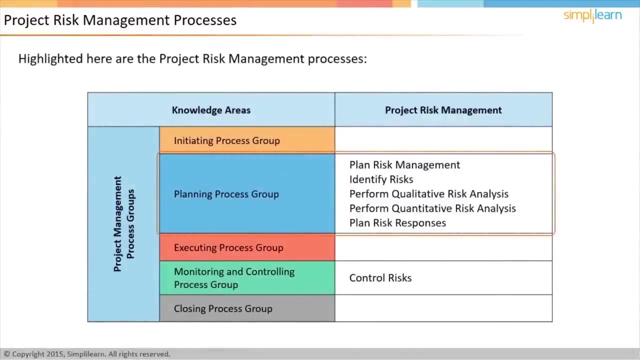 The key objective of risk management is to increase the probability and or impact of positive events and decrease the probability or impact of negative events. There are six risk management processes: Plan risk management. identify risks. perform qualitative risk analysis. perform quantitative risk analysis. 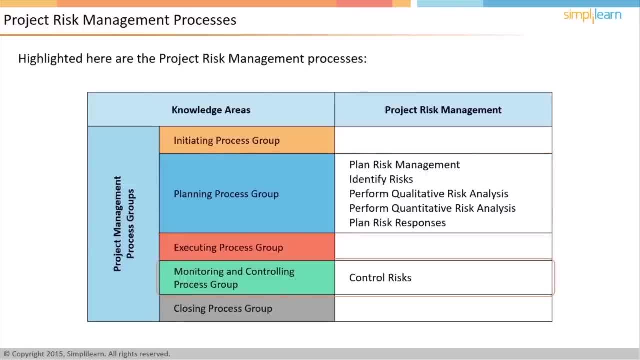 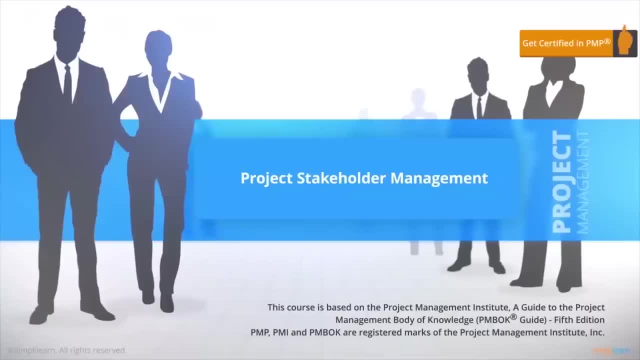 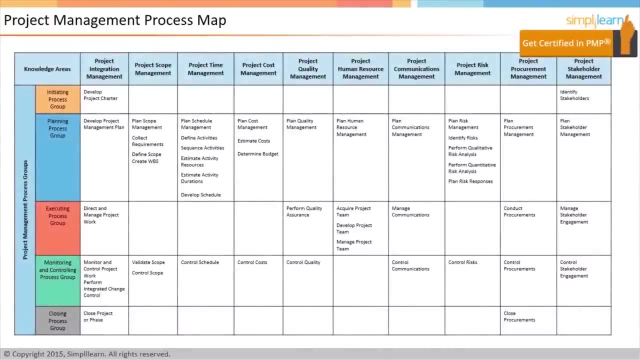 and plan risk responses belong to the project planning group and control risks belong to the monitoring and controlling process group. In this lesson we will focus on project risk management. There are 47 processes in project management, grouped into ten knowledge areas and mapped to five process groups. 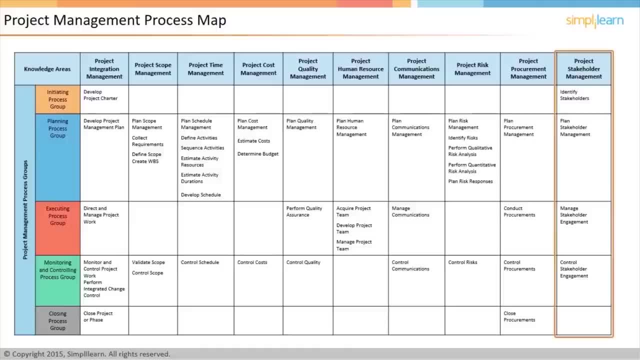 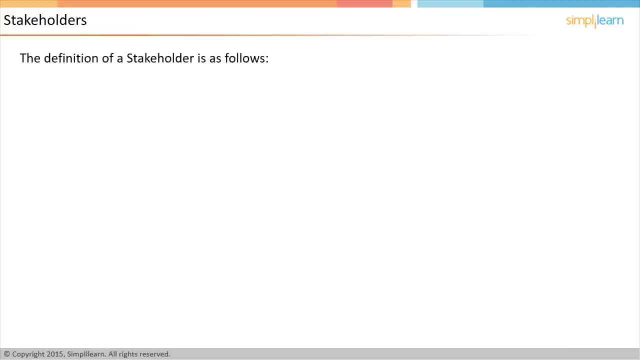 In this lesson we will look at the tenth knowledge area, that is, project stakeholder management and its processes. In the next screen let us understand who stakeholders are. A stakeholder is anybody who has a stake in the project. A stakeholder may be an individual. 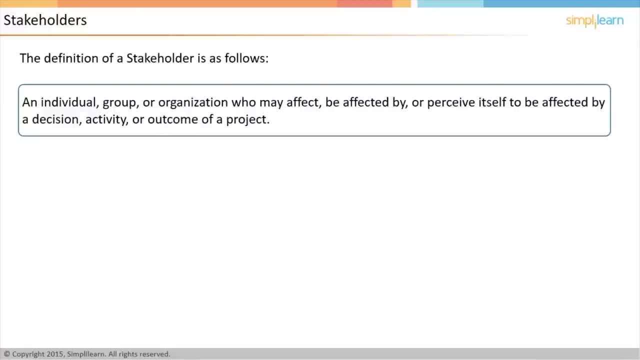 a group or an organization, or perceived to be affected by a decision, activity or outcome of a project. Further, the nature of the impact can be positive or negative, thus giving rise to the notion of positive or negative stakeholders. Irrespective of whether a stakeholder 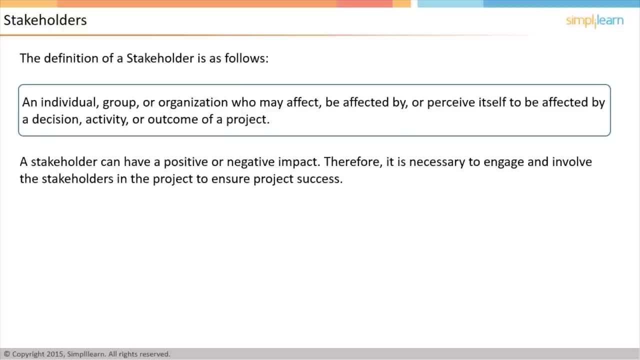 is positive or negative. it is important to engage with the stakeholders and get them involved in the project. This can make a critical difference to the success or failure of the project. A single disgruntled stakeholder can bring the project to its knees. 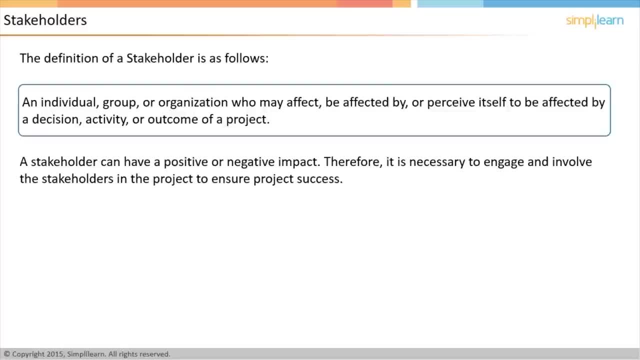 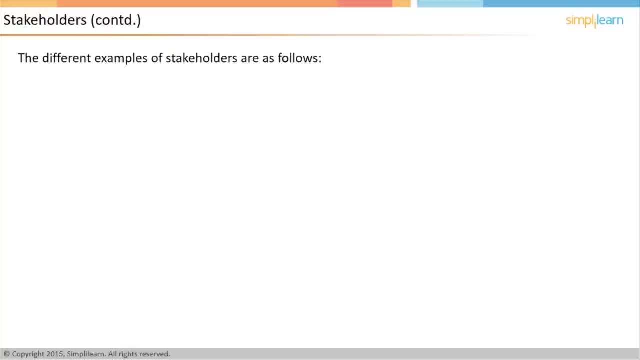 whereas an actively engaged and influential stakeholder can have the opposite effect. Let us understand who the common stakeholders of a project are. There are several categorizations of stakeholders. The project managers themselves are important stakeholders. The project team members represent stakeholders in the project. 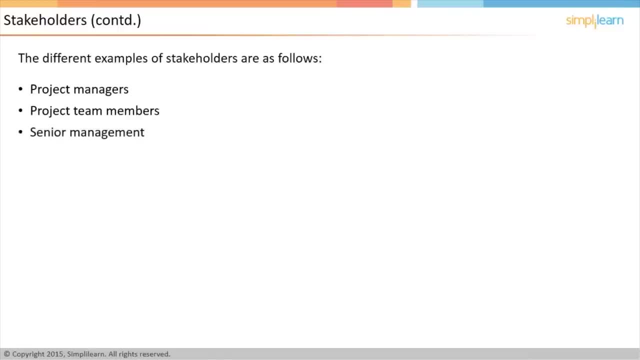 The senior management of the organization which is working on the project has a stake in the project. The person or entity that provides the money and resources for the project and essentially champions the project is an important stakeholder- The customer, which may be different. 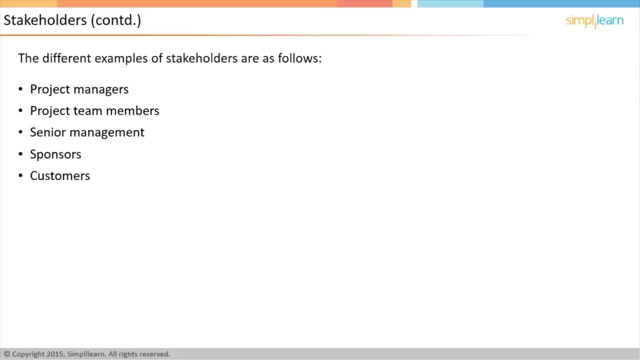 from, the sponsor is a stakeholder as well. For instance, in many of the projects in the social sector, the sponsor may be the government or a development agency, whereas the customers would be the people who actually benefit from it, The end users, which may be different. 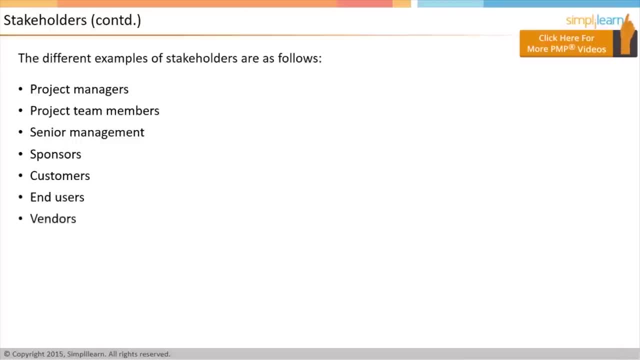 from the customers or the sponsors are important stakeholders. The vendors or suppliers who provide goods or services to the project are important stakeholders. People whose lives may be impacted by the output of the project are also stakeholders. For example, if a highway project requires possession of privately owned land. 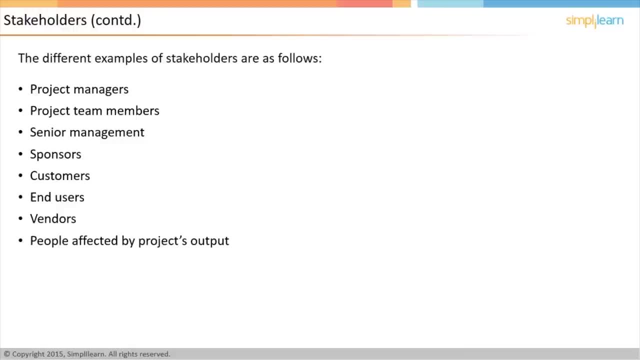 people whose land is being taken away are the stakeholders. If the construction of a dam or water reservoir benefits the downstream farming communities, they are the stakeholders here. Other alternative goods or services are stakeholders too. Sometimes environmentalists or other social groups may become stakeholders. 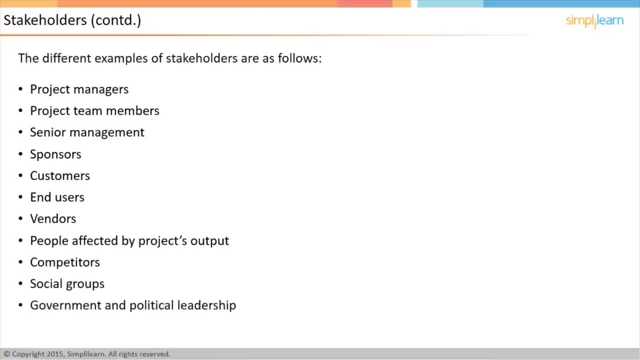 The government or political leadership may become stakeholders for projects in the public domain. It is sufficient to state that there could potentially be hundreds of stakeholders for a large project. It is in the interest of the project manager and the project team to clearly identify all such stakeholders up front. 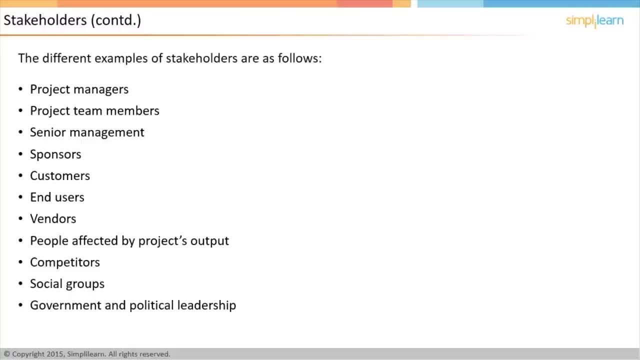 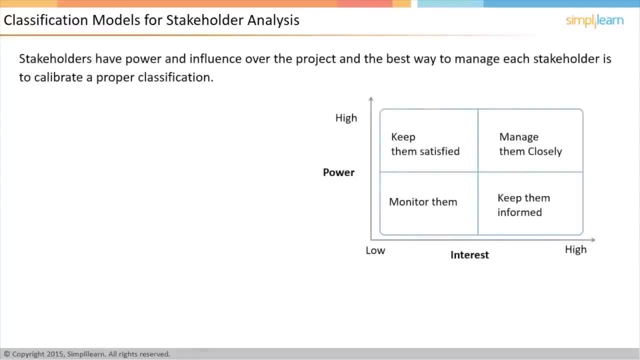 and then actively manage them throughout the project. In the next screen, let us discuss the classification models for stakeholder analysis. Not all the stakeholders have the same amount of influence or power over the project. Therefore, the way to manage each stakeholder needs to be calibrated. 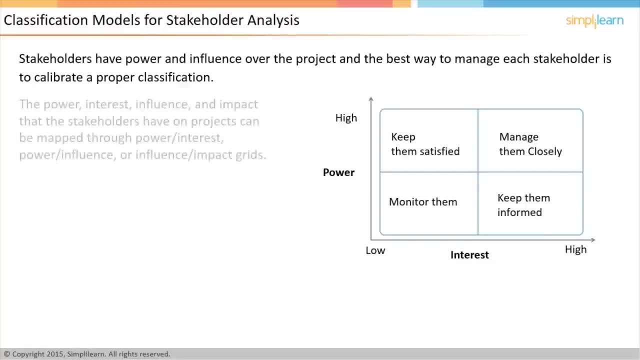 based on a proper classification of the stakeholders. This is the role of the classification model. You can come up with a grid that maps the power of the stakeholders, the interest they have and the impact that they can have on the project through the power interest. 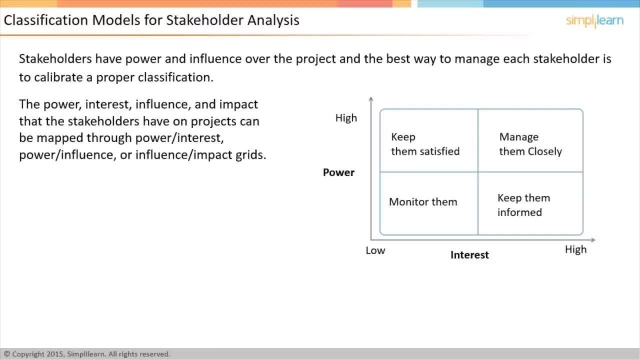 power, influence or influence impact grids. It can be represented by mapping stakeholders to a power or interest grid. The diagram on the screen has X-axis, which represents interest level, and Y-axis, which represents the power level Based on the various combinations. 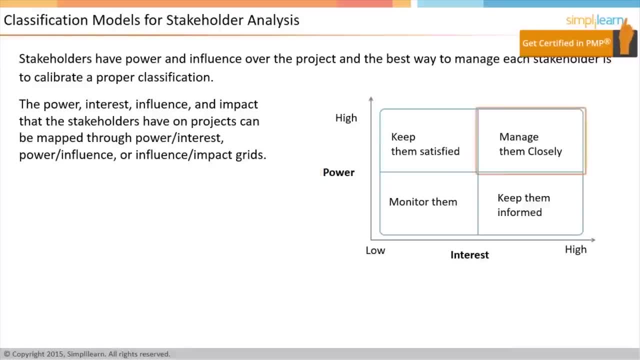 of power levels and interest levels. the grid can be divided into four quadrants. The quadrants with high power and high interest need to be managed closely, That is, you have to monitor their involvement and engagement very closely. The stakeholders on the bottom right quadrant. 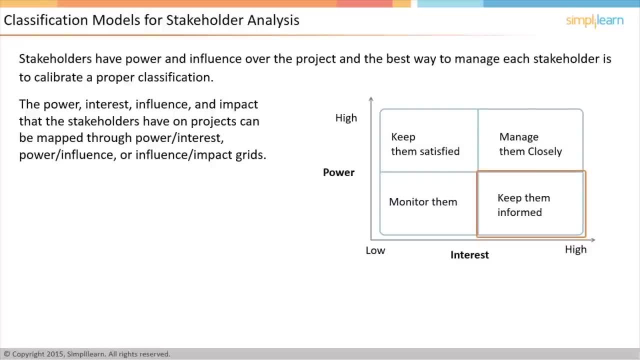 with high interest but low power need to be kept in the loop, That is, you should share information with them and keep them regularly informed. The stakeholders on the top left quadrant with high power but low interest, can be managed by keeping them happy, for example, by making sure 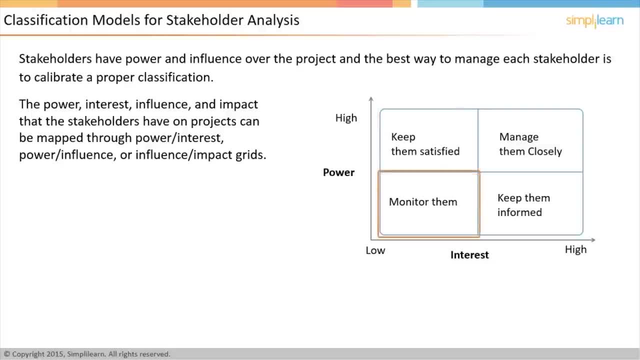 they are taken into consideration. The stakeholders on the left bottom quadrant with low power and low interest may be managed less actively by simply monitoring how things are going with them. The salience model describes classes of stakeholders based on their power, urgency and legitimacy. 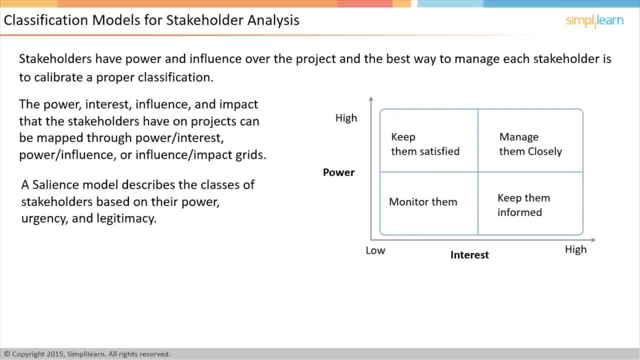 This is a useful framework to guide the stakeholder management strategy on a project Practice, creating power grids for business scenarios. This will help in understanding the level of engagement a project manager needs to maintain with various stakeholders. In the next screen, let us discuss. 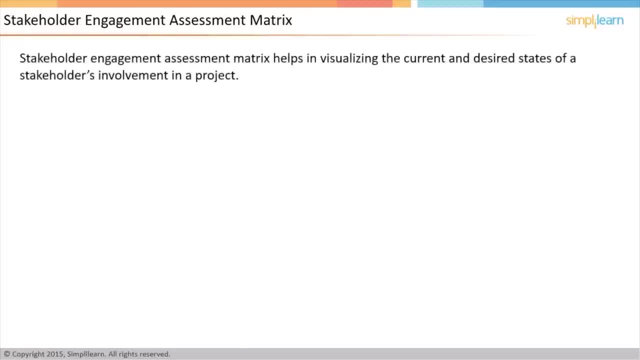 the stakeholder engagement assessment matrix. The stakeholder engagement assessment matrix allows visualizing the current and desired states of a stakeholder's involvement in the project. The five levels of involvement are as unaware, supportive and leading. Unaware is where the stakeholder 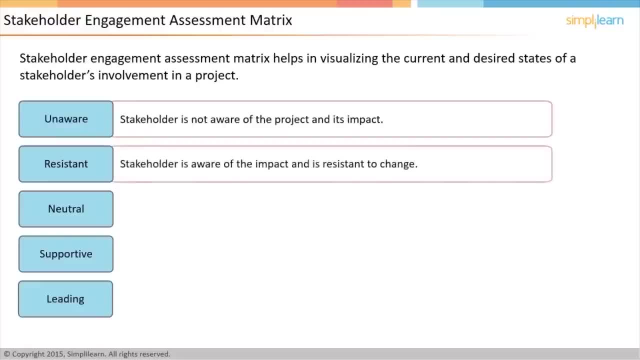 is not aware of the project or its impact. Resistant is where the stakeholder is aware of the impacts and is resistant to change. Neutral is where the stakeholder is aware of the project and is neither supportive nor in opposition to the project. Supportive is where the stakeholder 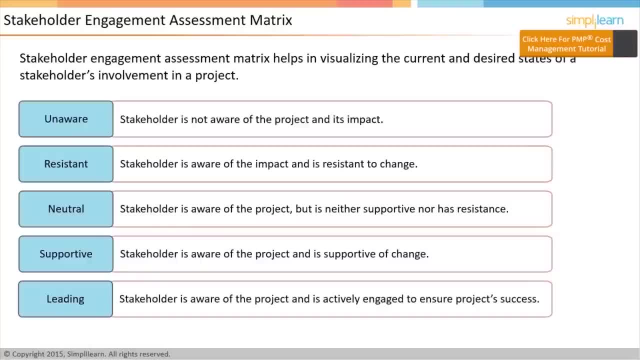 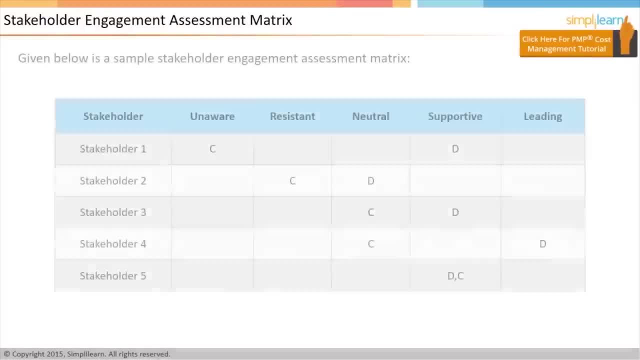 is aware of the project and its impact and is supportive of the change. Responsive is where the stakeholder is actively engaged to ensure that the project is successful. Let us now look at the matrix. The table has one row per stakeholder identified. You place C in the column. 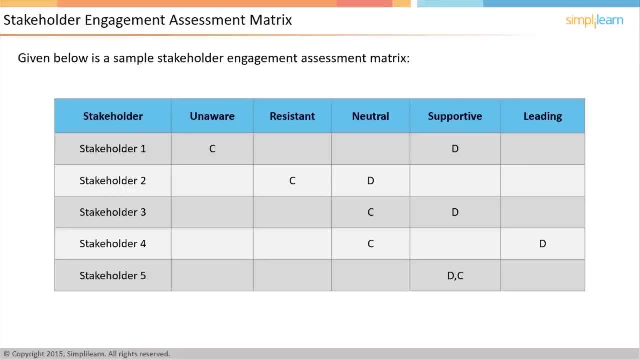 which best indicates the current level of engagement for that stakeholder. Then you place D in the column, which best indicates the desired state of engagement. This table can be a quick visualization tool that helps understand how stakeholders interact with each other. Next screen: let us discuss. 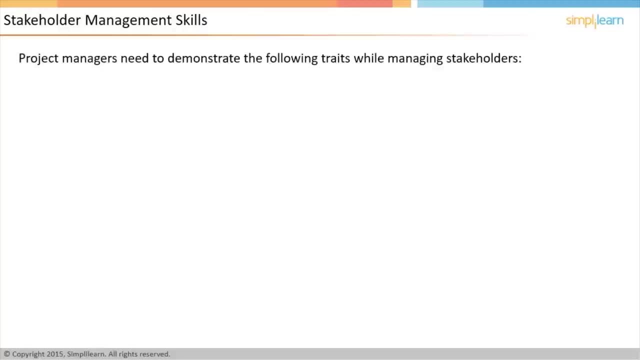 the skills required for stakeholder management. Stakeholder management is both an art and a science, Since it involves dealing with people, and people are inherently non-linear and unpredictable. there is no one size that fits all, strategies or tools that will work while managing them. 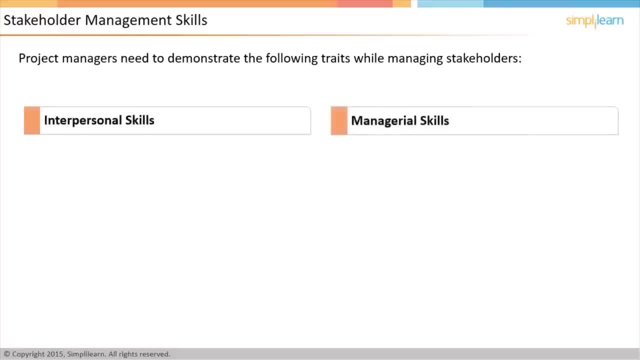 However, a project manager must possess good interpersonal skills and managerial skills. A project manager must possess good interpersonal skills, That is, must invest the time and energy to build trust. This involves multiple things, such as establishing a personal rapport following through on commitments. 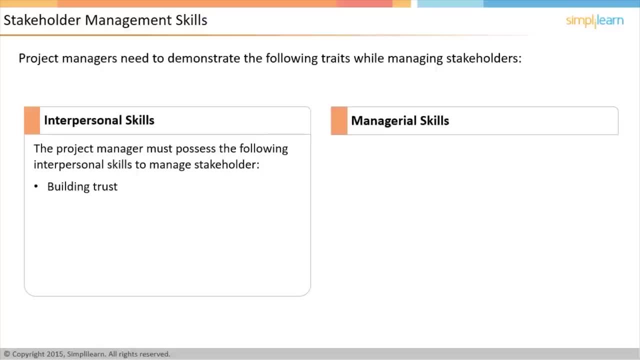 being punctual, etc. Once the trust is established, it helps in smoothing many difficult bends. Conflict management is an important skill for a project manager Stakeholders- the project manager must practice active listening. They must not assume that they have all the answers. 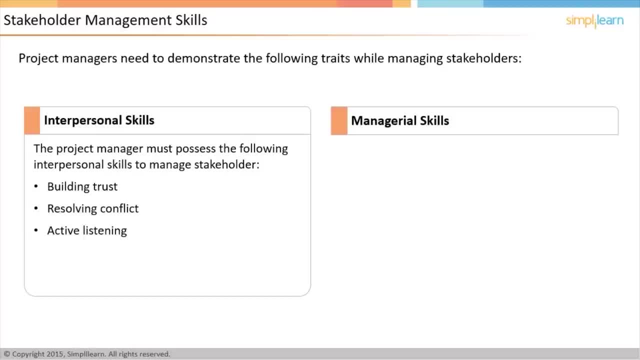 Instead, they should spend some time to understand the issues and the stakeholders' points of view. This alone can go a long way in smoothing ruffled feathers and building constructive relationships. Resistance to change is natural. A project manager must know how to convert that into a positive. 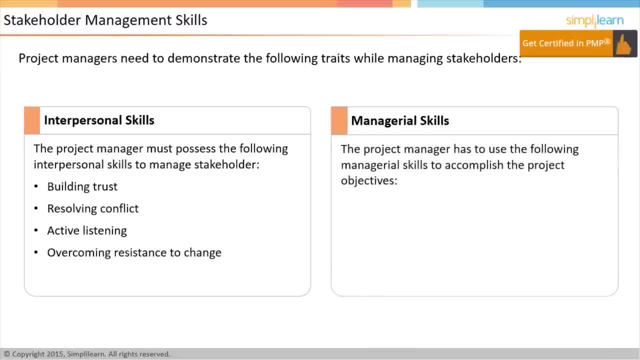 energy in its favor, Managerial skills that may help them achieve their objectives. A project manager must be able to build consensus among the group. While absolute uniformity may not always be possible or desirable, the project manager must use techniques to ensure widespread discussions. 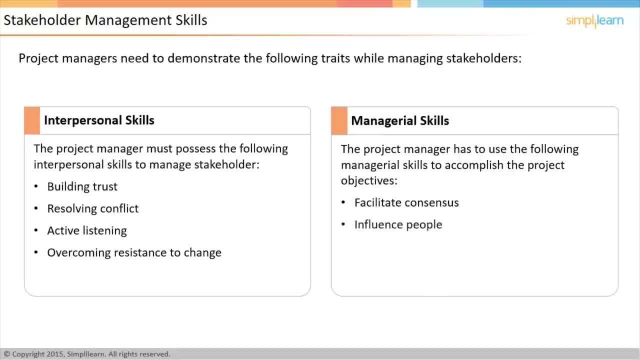 and arrive at a path that the group can buy into. The project manager must be able to influence people, often without necessarily being in the position of authority. The project manager must be skillful at understanding and modifying organizational behavior in order to move the project. 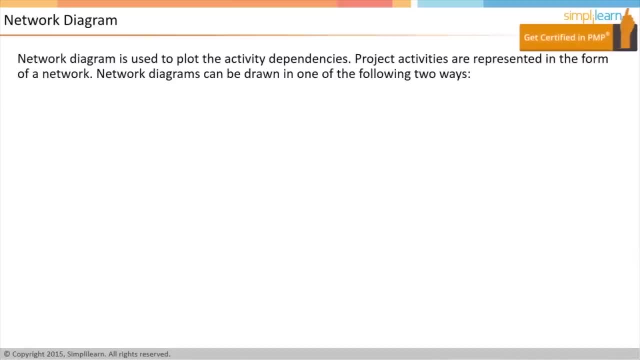 in a certain direction. Network diagram is extensively used in the project time management knowledge area to plot the activity dependencies. This is a graphical representation of the project activities in the form of a network. There are two ways to draw a network diagram. In Precedence, Diagramming Model. 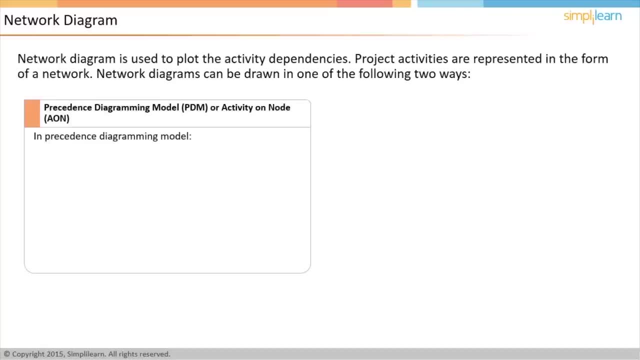 there are two ways to draw a network diagram. In Precedence Diagramming Model or Activity on Node, boxes represent activities and the arrows indicate the dependency. This type of network can have all four types of relationships between the activities In Arrow Diagramming Model. 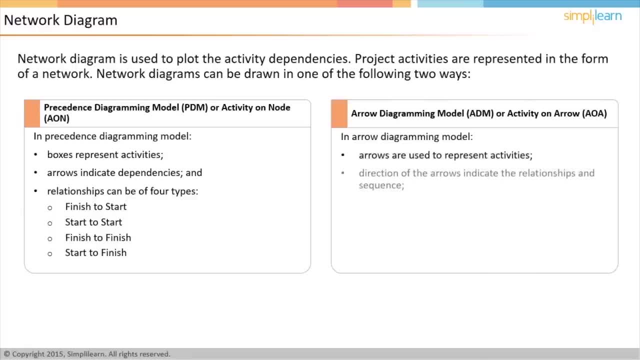 or Activity on Arrow, the arrows represent activities. The relationships and sequences can be inferred from the direction of the linkages between the activities. In such types of network, only finish-to-start relationships can be shown. Such diagrams may need to make use of dummy activities. 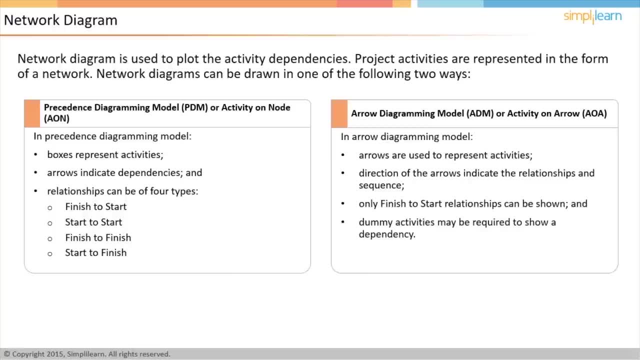 to indicate some dependency between the activities. There may be questions in the PMP exam based on the network diagram. so create and work with the diagram. This will make answering network diagram-based questions easy and fun. Let us look at a network diagram. 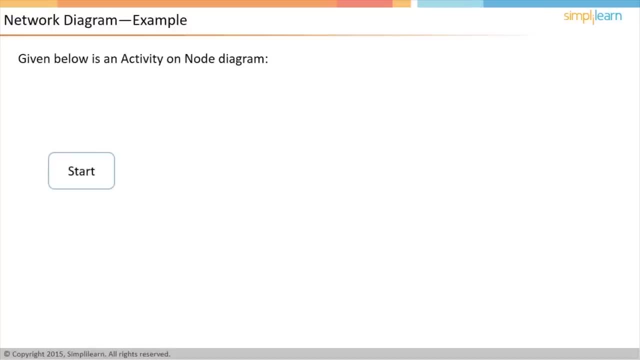 A sample network diagram is shown on the screen. Activities A and C can happen in parallel. B and D require both A and C to complete, whereas E requires both B and D to complete. Activity on Arrow Network Diagram makes use of hammock activities. 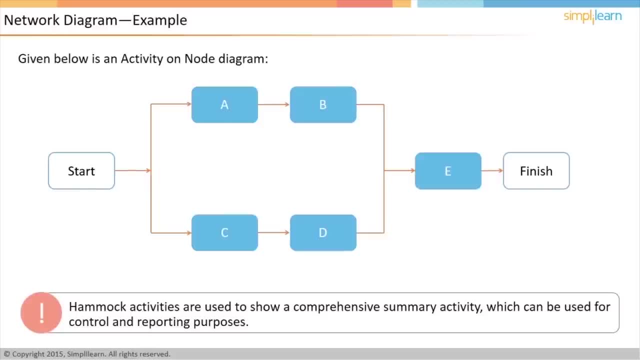 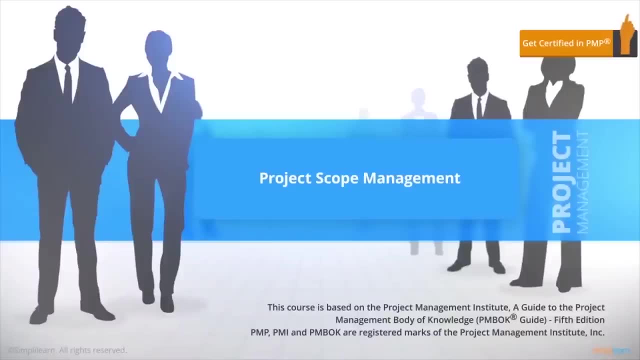 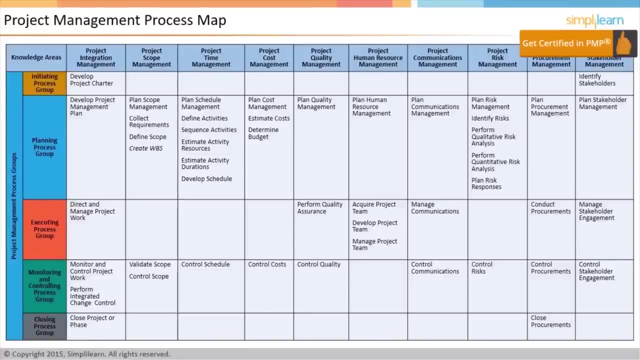 They are used to show a comprehensive summary activity combining several other activities underneath for control and reporting purposes. In this lesson we will focus on project scope management. There are 47 processes in project management, grouped into 10 knowledge areas and mapped to 5 process groups. 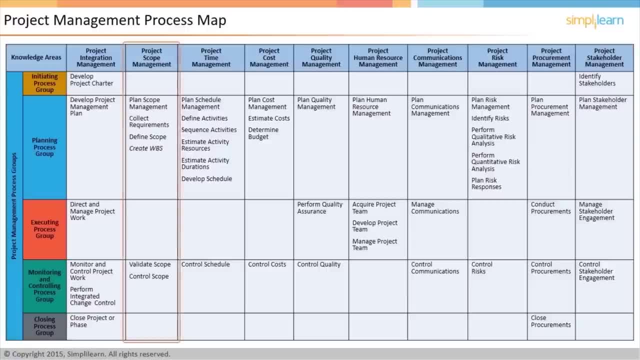 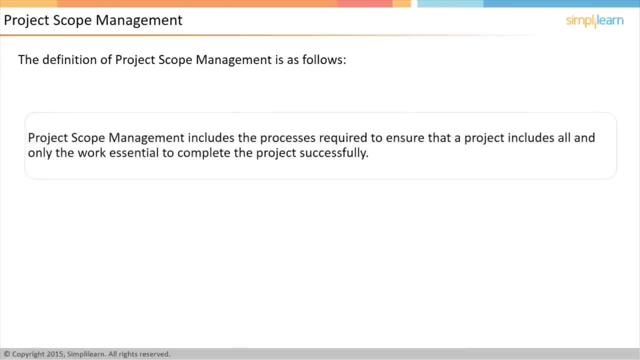 In this lesson we will look at the second knowledge area, that is, project scope management and its processes. Let us begin with the first topic of this lesson, that is, project scope management. Project scope management includes the processes required to ensure that a project comprises. 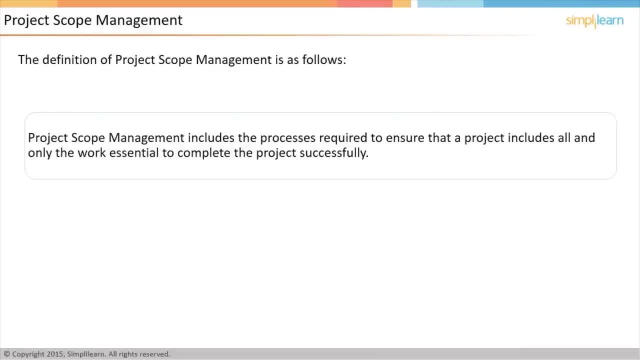 all and only the work required to complete the project successfully. The project scope management is concerned about the scope. What is not there in the scope is also clearly identified In the next screen. let us look at the key activities performed under project scope management. 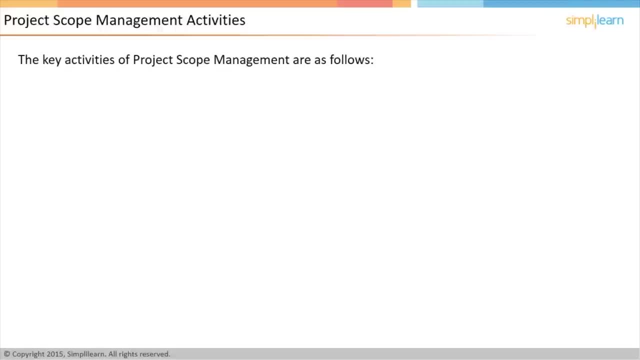 Let us look at a few of the typical activities that are part of project scope management. Constant monitoring is essential to make sure that all the project work is being completed. The gradual, uncontrolled increase in scope of the project is referred to as scope creep. 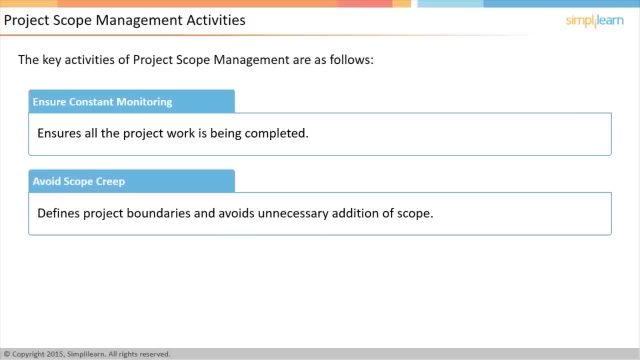 It is necessary to define the project scope boundaries and not let people randomly add to the project scope. Gold plating is doing more than what is required and this has to be avoided in projects. As per the published statistics about projects done globally, less than 40% of projects. 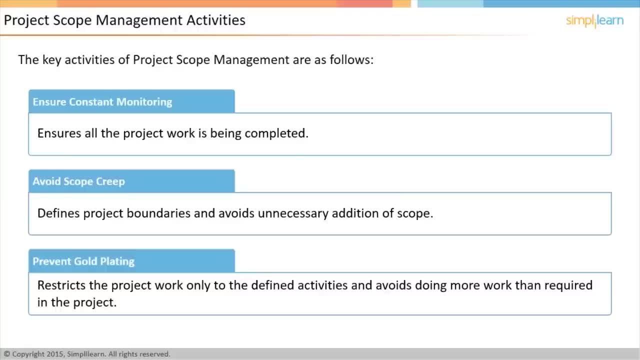 can be considered successful. Therefore, the focus should be on what is required rather than squandering around with what is not required. 40% might be considered less, but a project is classified as successful only if it meets all its objectives and is done within time. 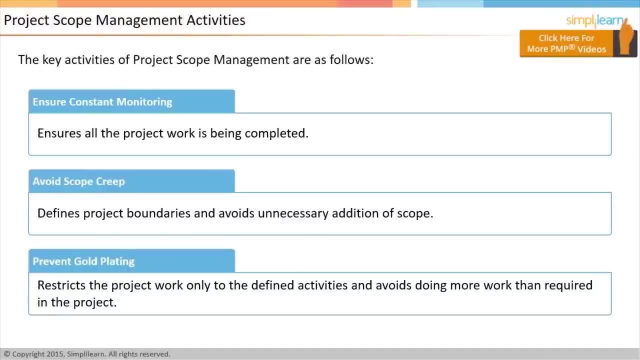 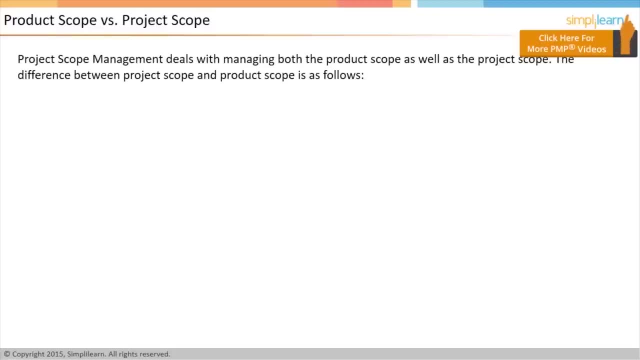 The next screen. let us understand the differences between product scope and project scope. Project scope management deals with managing both the product scope as well as the project scope. Product scope refers to the features and functions that characterize a product, service or result. The word product. 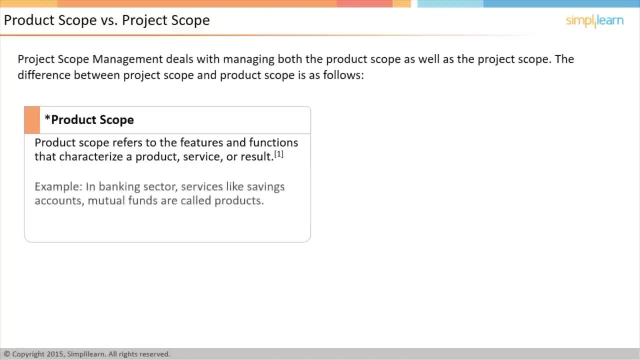 may also include creation of a service, For example, in the banking industry. each of their services is a product. Likewise, a savings account is one of their products, Mutual fund is another. On the other hand, project scope is the work that needs to be accomplished. 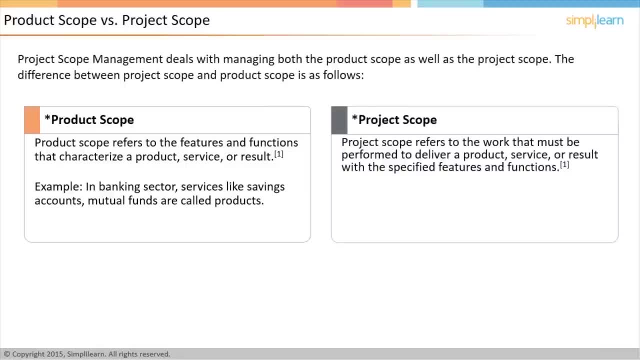 to deliver the output of the project, which could be a product, service or result, with the specific features and functions. For instance, to deliver a product, you may also need to produce a requirements document or a design document. In the next screen. 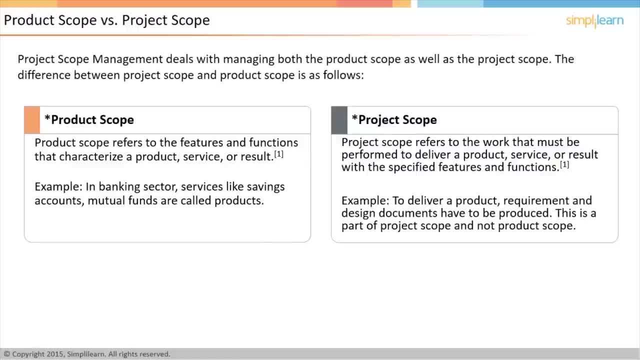 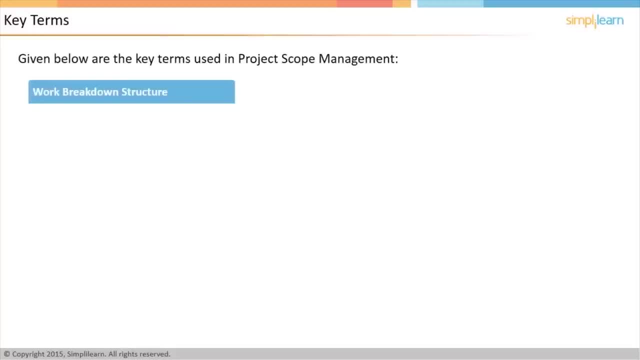 let us discuss a few key terms used in the project scope management. WBS stands for Work Breakdown Structure. It means breaking the project deliverables into smaller and more manageable components called work packages. The last level of work in such subdivision is called work packages. 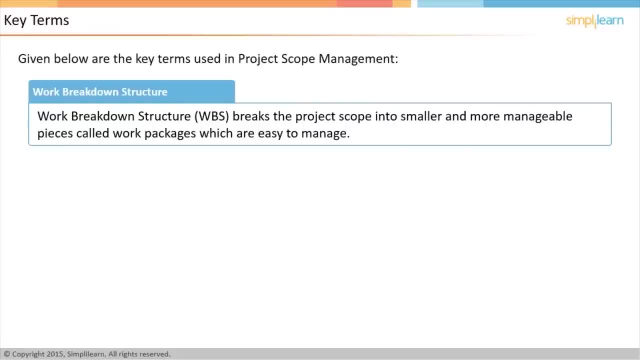 and the whole structure is called WBS. For example, a typical project would have various activities like finalizing requirements, designing the new system, coding, testing and going live with the new system. Each of these translates into high-level deliverables which can be further subdivided. 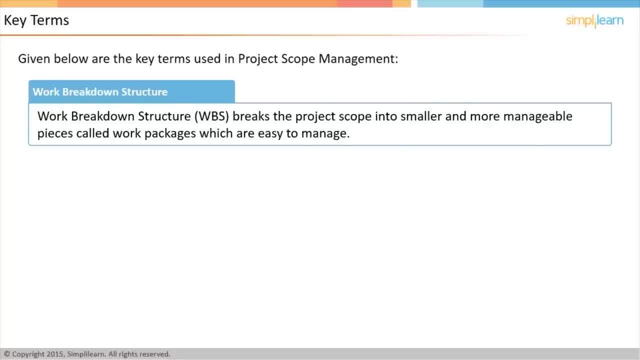 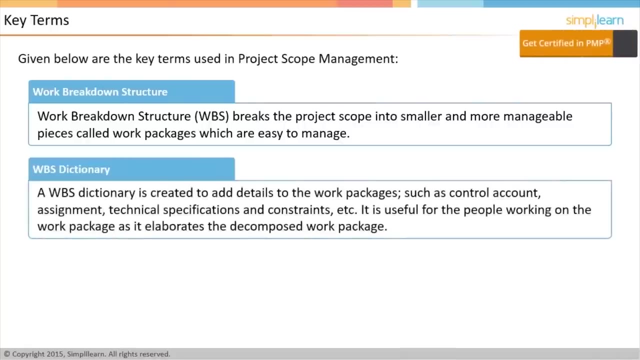 into smaller activities which are more predictable. WBS dictionary. like any dictionary, contains the explanation of the terms used in WBS. A typical WBS dictionary has details like the control account. name of the work package, description of the work package. 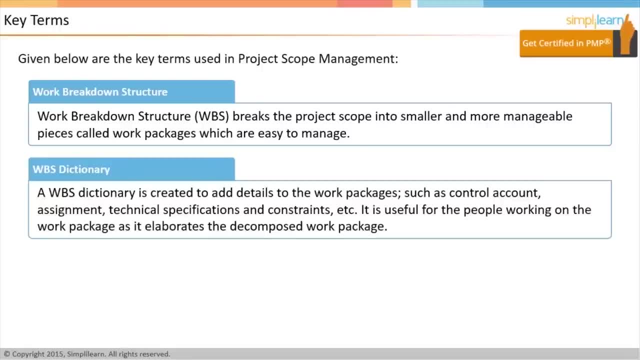 resource assigned, if there are any assumptions or dependencies to complete the work package, the due date to finish the work package, technical dependencies and so on. WBS dictionary is useful for the person or group working on the work packages of the project. 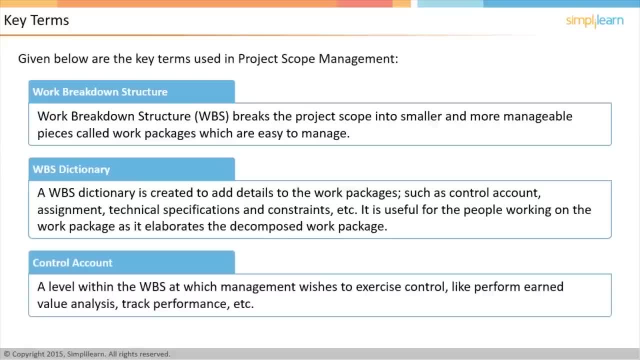 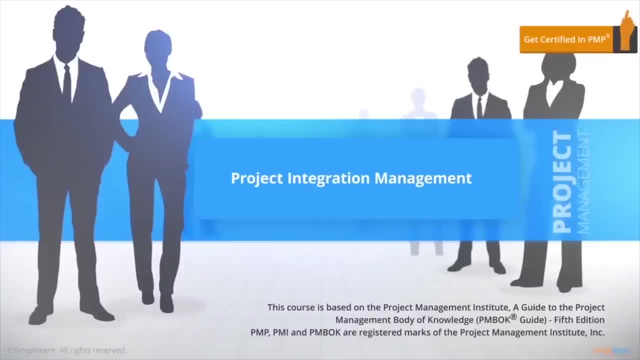 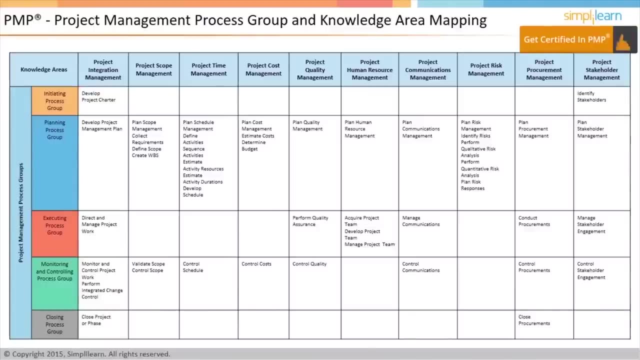 The control account is a level within WBS at which management wishes to exercise control, For example, perform earned value analysis, track performance, etc. In this lesson we will focus on project integration management. There are 47 processes in project management grouped into 10 knowledge areas. 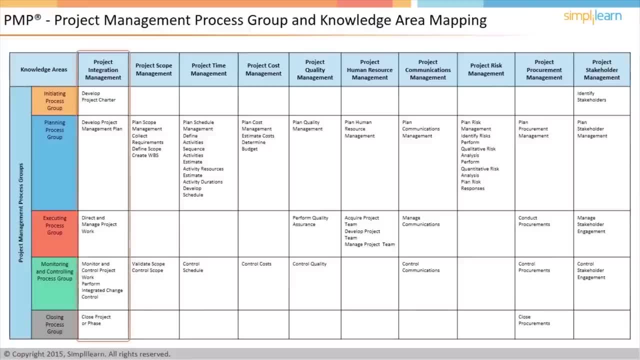 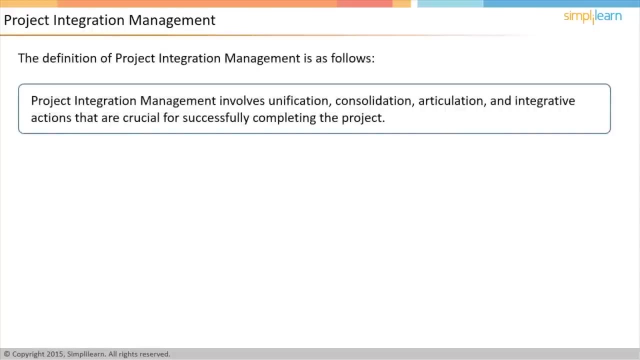 and mapped to 5 process groups. In this lesson we will focus on project integration management and its processes. In the next screen, let us understand the concept of project integration management. Project integration management involves unification, consolidation, articulation and integrative actions. 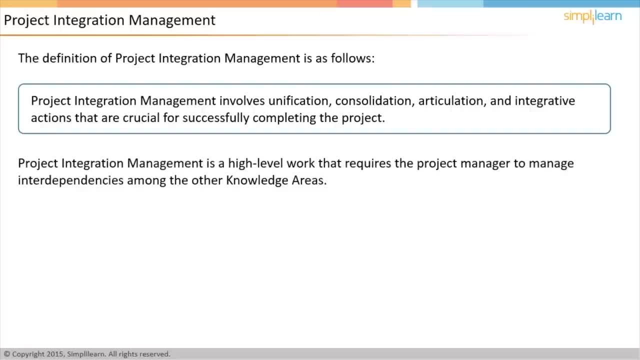 that are crucial for successfully completing the project. The project integration management is high-level work. among the other knowledge areas, The other nine knowledge areas involve detailed work in a specific direction. For example, project cost management deals only with how to manage cost in a project. 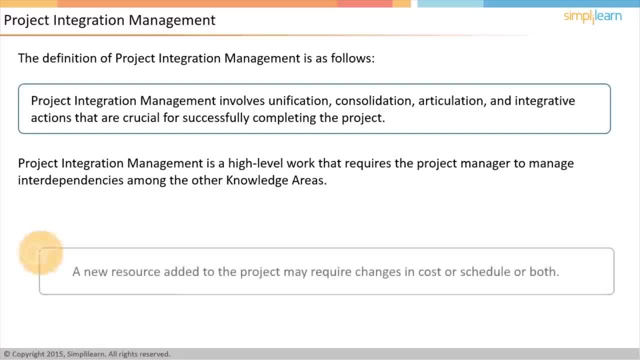 The project management processes do not happen independently. For example, a new resource added to the project may require changes in cost or schedule or both. In dealing with such situations, the project manager integrates with project management. The need for integration drives much of the communication. 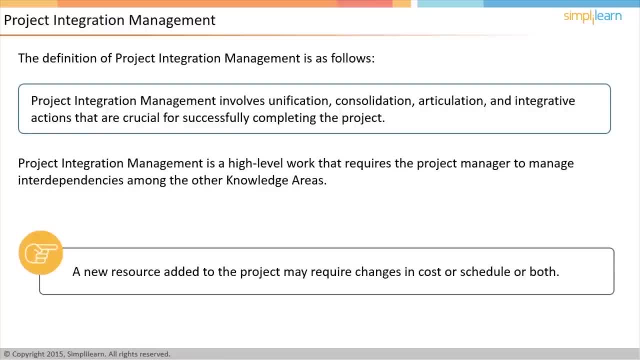 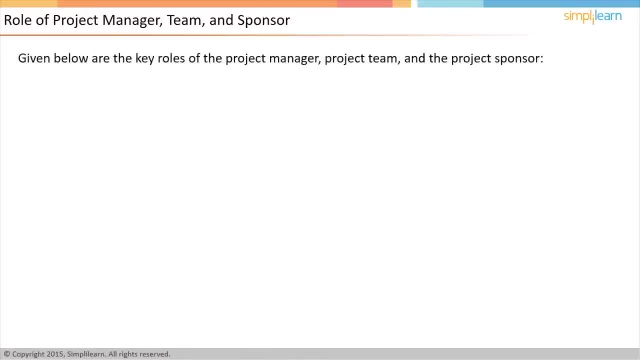 and the work of the project manager. Let us discuss the key role of project manager, sponsor and team in the next screen. Project manager, team members and project sponsors have different roles to play in a project. The project manager is supposed to play multiple roles in the project. 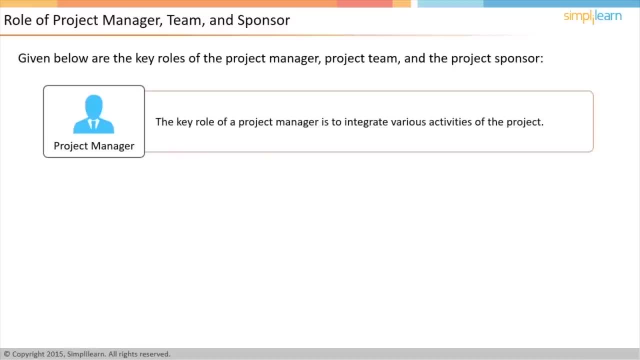 The key role is to perform integration. The project manager puts the pieces of the project together into a cohesive whole. In doing so, the project manager tries to ensure that the project is done faster, cheaper and utilizes resources optimally, while meeting the project objectives. 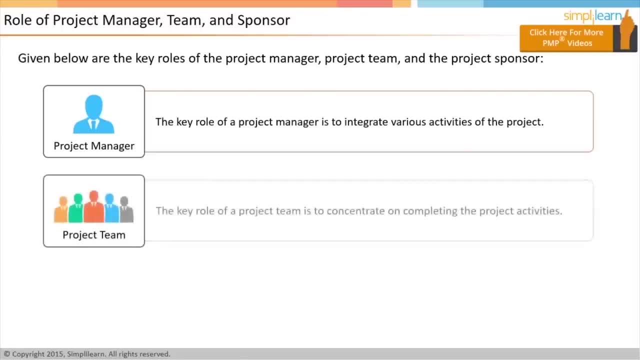 As the project progresses, the team members work on completing the project activities. The role of the project sponsor is to protect project from any unnecessary changes and to ensure that it has the required resources for completion. The project sponsor is the champion for the project within the performing organization. 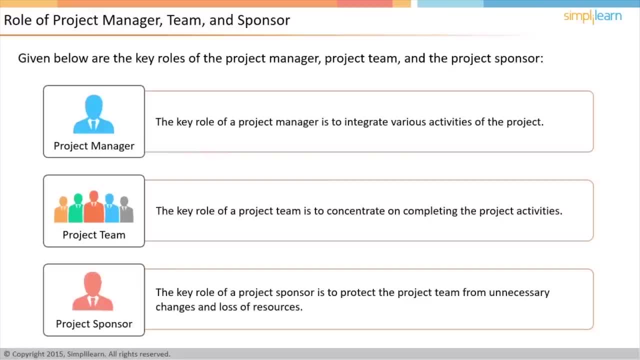 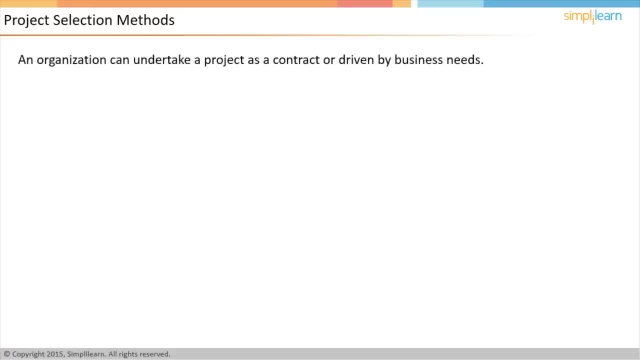 that is, the organization in which the work is being performed. In the next screen we will cover the project selection methods. An organization can undertake a project under contract with an external organization or take up a project driven by internal business needs. There should be a formal process. 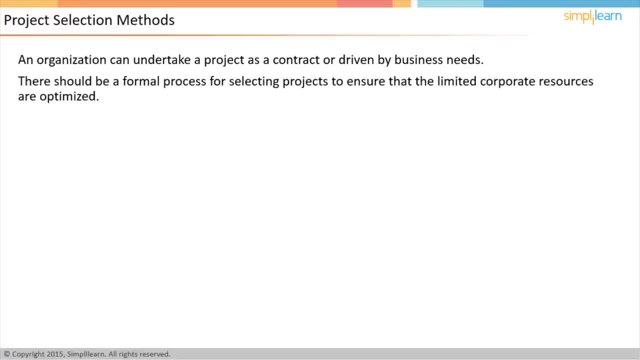 of selecting project organizations to ensure that it is making the best possible use of limited corporate resources. For example, if the organization has an option to take up any one out of the two projects, both of which use the same corporate resources, the organization would naturally 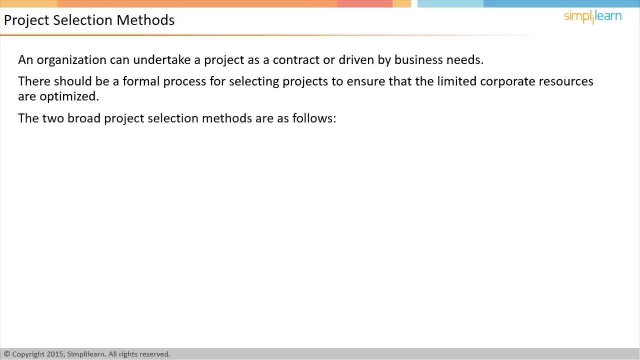 select the one which is more profitable. There are two broad ways to select a project. One way is the benefit measurement method, where one project is compared to other projects. Another approach is based on mathematical models, wherein you examine the most optimal selection of projects by trying to optimize a goal. 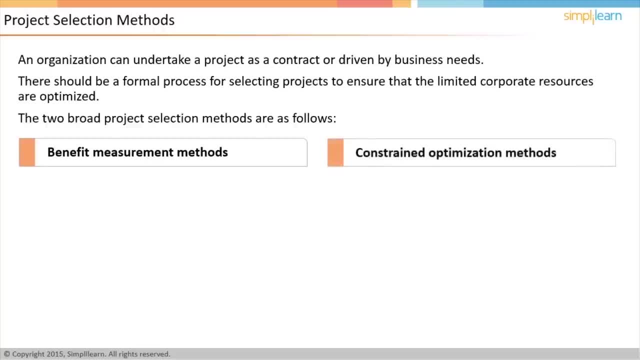 For example, maximize operating profits. Such methods may be called constrained optimization methods. There are different methods under both these categories and you should be familiar with the names of these methods Broadly. the benefit measurement methods are based on the benefits of undertaking the project. 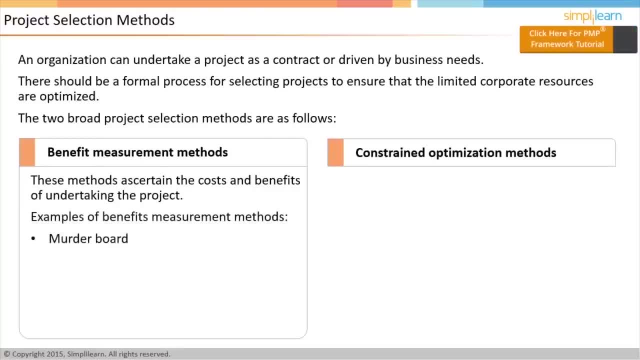 The methods under benefit measurement method include murder board, where a panel of experts shoots down a new project idea, peer review, scoring models, economic models and benefit compared to cost. The constrained optimization methods rely on mathematical modeling techniques to determine the best selection of projects to achieve. 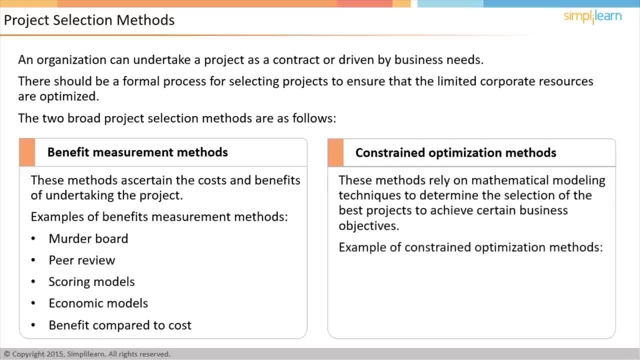 certain business objectives. The methods of constrained optimization method include linear programming. In reality, you might not have seen these methods to be followed in project selection. Often personal relationship with the sponsor may be more important than anything else. This is quite normal, and any organization worldwide. 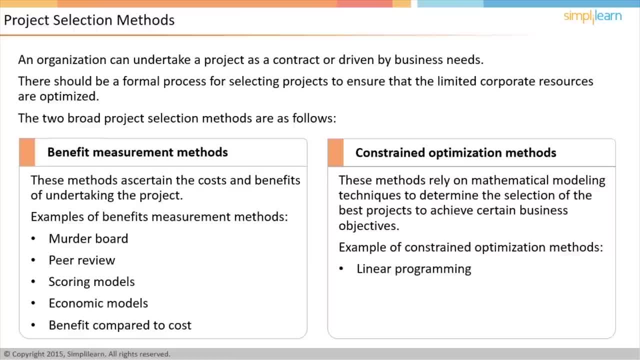 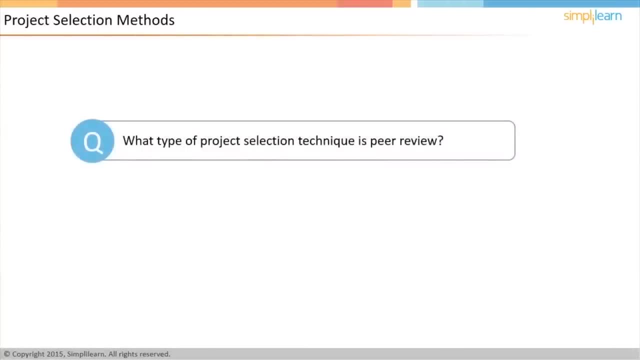 works this way. However, as a certified project manager, it is important for you to be familiar with more scientific methods of project selection. The question on the PMP exam could be: what type of project selection technique is peer review? And the right answer is: 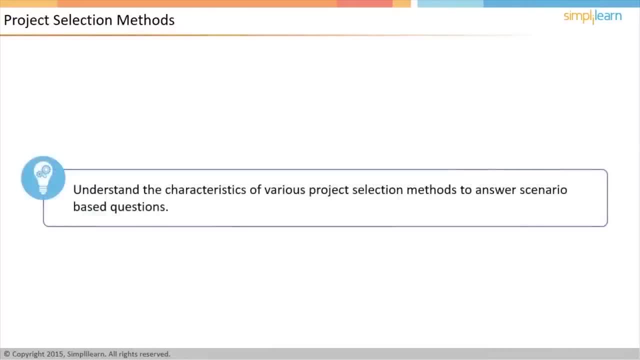 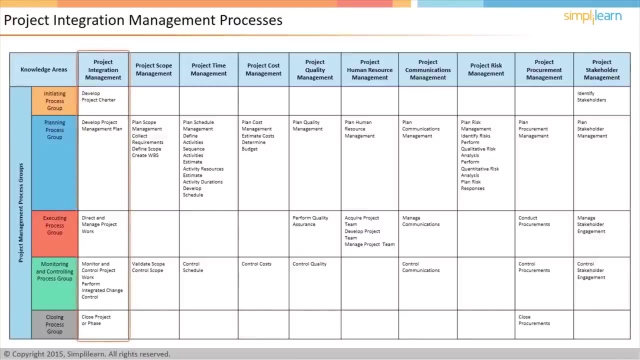 benefit measurement method. You need to understand the characteristics of various project selection methods to answer scenario-based questions. In the next screen, we will focus on the project selection methods. There are five project management processes which are part of project integration management knowledge area. 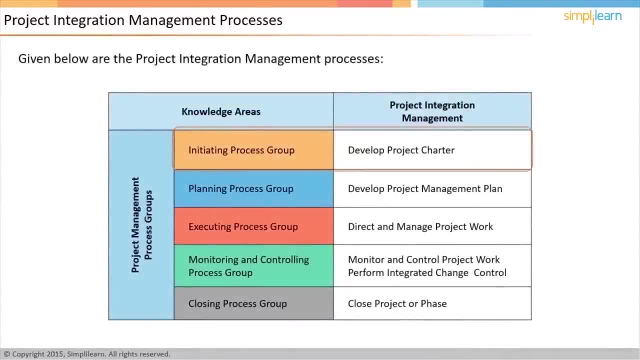 They are: the: develop project charter done in the initiation process group. develop project management plan undertaken in the planning process group. direct and manage work carried out in the executing process group. monitor and control project and perform integrated change control undertaken in the monitoring and controlling process group. 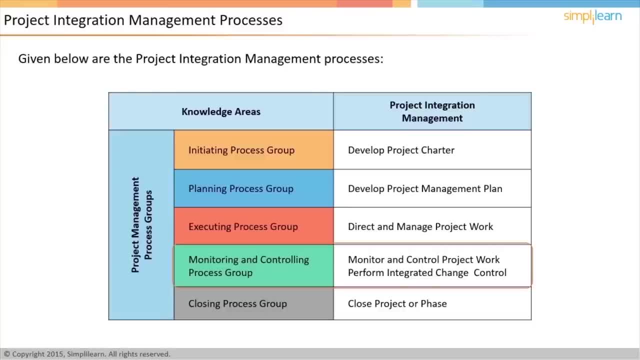 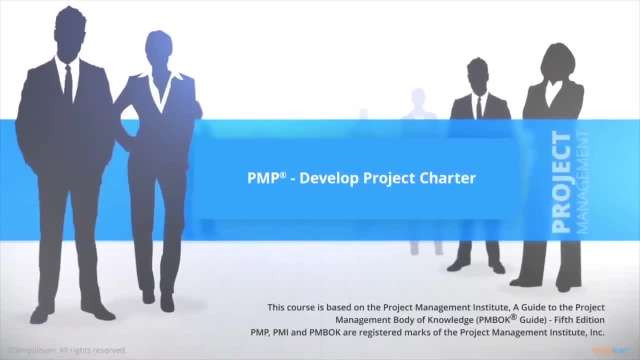 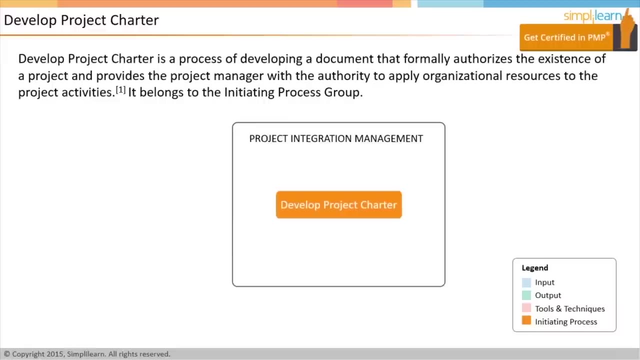 and close project or phase done in the closing process group. The project management process is a process of developing a project charter. Develop project charter is an initiating process. A project charter is essentially a document that authorizes a project. Once a project has received a charter. 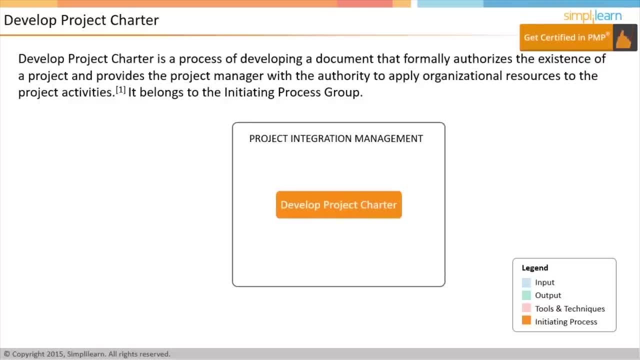 it means that the project manager can start employing the organization's resources for the project activities. Let us look at the key inputs to be considered in preparing the project charter. The first input is the project statement created by project sponsor or the customer describing their needs, project scope. 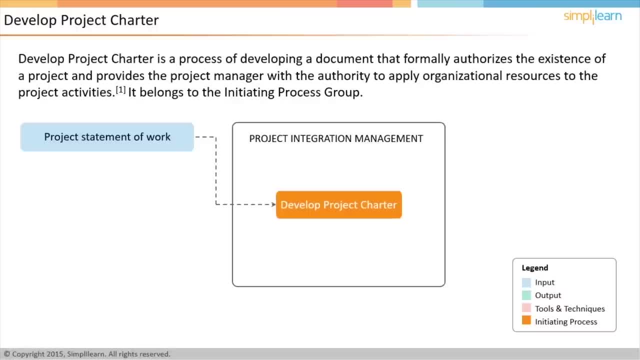 and how the project fits into their strategic goal. If the project is taken up under a contract, the request for proposal can be considered as project statement of work. The next input is the business case. This document establishes whether the investment in a project is worth from a business point of view. 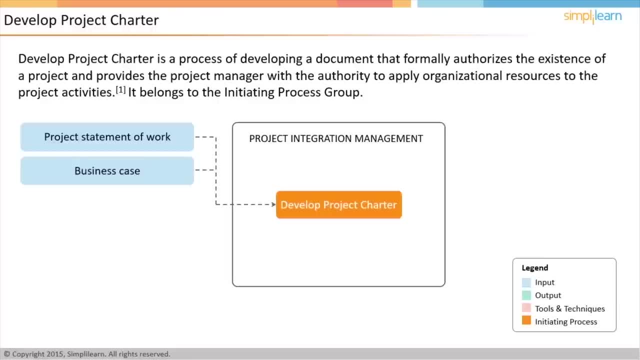 the business need for the project and the cost-benefit analysis. It provides important information to the project manager about the goals of the project and the boundaries in terms of the desired results, cost, etc. If the project is being undertaken as part of a contract. 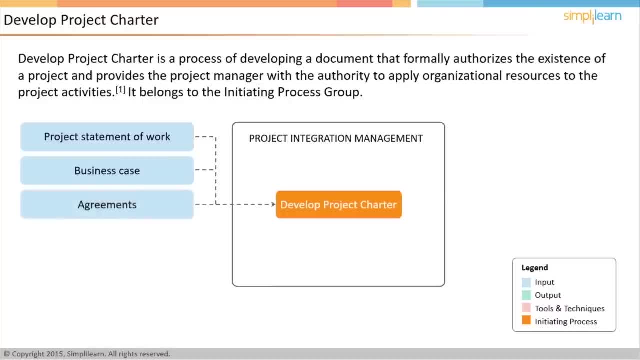 or agreement. the agreement provides an important input for the project manager that establishes what must be done in the project. The next input to be considered for project charter is organizational factors. Any project to be executed within the organization has to deal with the organization culture. 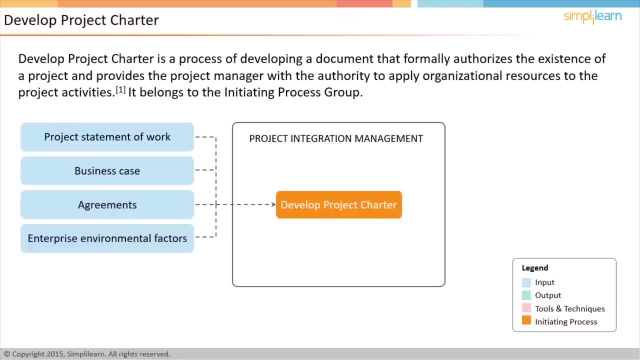 and existing systems. You can consider this as an organization baggage that comes with the project. This is the reason a project being executed in two different organizations may be done differently. Another factor to be considered is organizational process assets. This is a broad term and includes all the 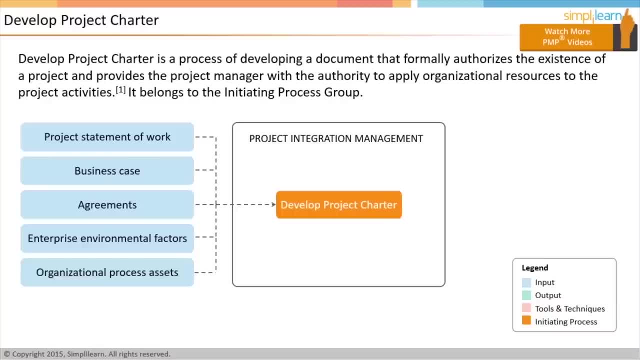 organizational processes, procedures and policies, corporate knowledge base and historical project information. Every organization develops a set of processes, procedures and policies that are based on the best practices learned by the organization over time. The historical information includes past project management plans, risks, lessons learned. 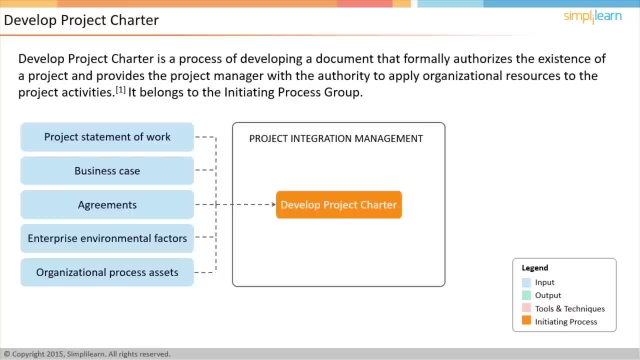 etc. of similar projects executed. Now let us look at the tools and techniques used in this process. The first technique is expert judgment. Expert judgment is an invaluable input to the process of formally authorizing a project, because an expert can provide insights into why a project 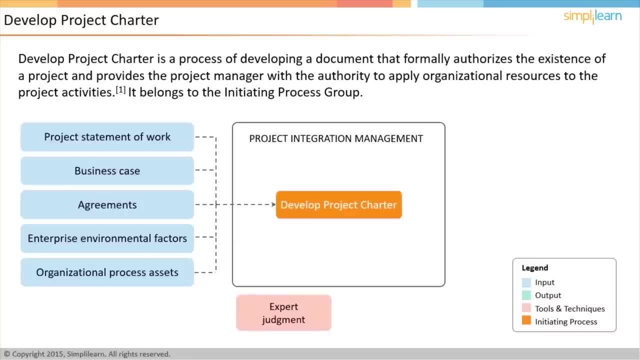 makes business sense or why it does not. From experience, they may be able to shed light about the validity of the business drivers, feasibility assumptions and goals considered for the project. Facilitation techniques is another technique used. The chartering process is often. 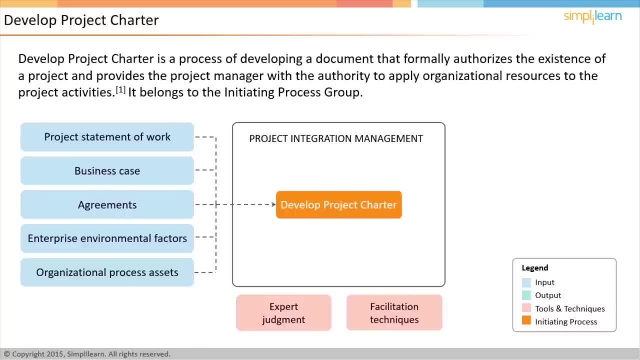 a collaborative activity involving many influential stakeholders in an organization. Facilitation techniques help bring all these stakeholders together and engage in fruitful discussions in order to arrive at an informed decision whether to go ahead with a project or not. The only output of this project is the project charter. 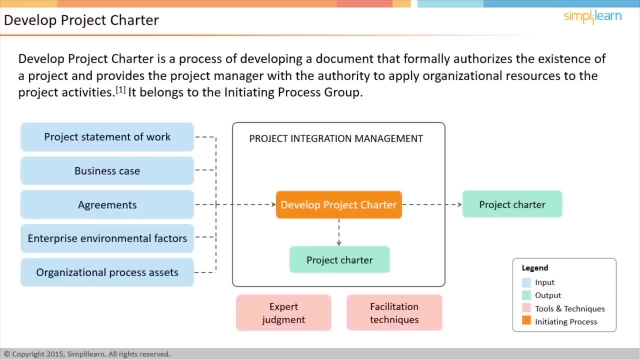 Let us try to understand what the project charter might contain. The project charter usually contains the high-level project requirement and it should be created by the project sponsor and handed over to the project manager. The project manager can do the groundwork to prepare the project charter. 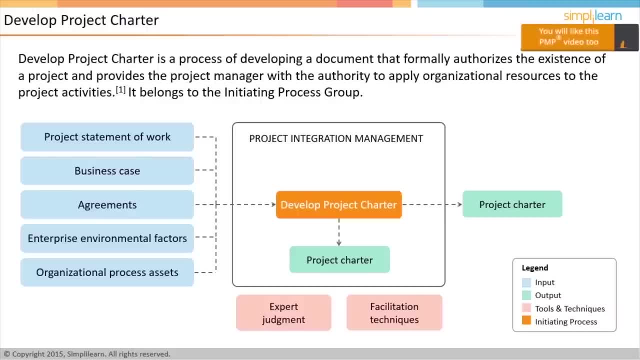 but it must be signed by the project sponsor or somebody in the performing organization who is higher in authority than the project manager. It is important to point out that a project charter is not a project management plan: The detailed risk schedule, cost analysis, etc. 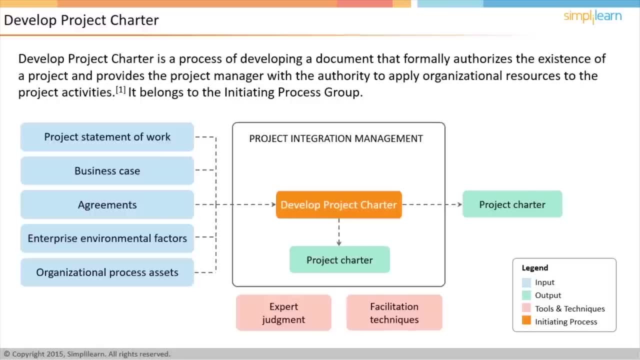 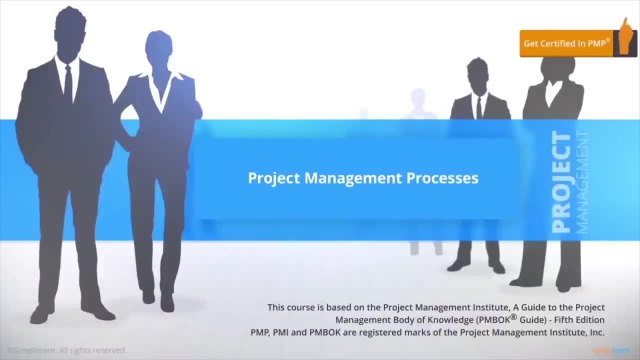 is part of the project management plan and should be done during the project planning phase, when there is more detail on the availability of the project to do so. The charter should be sufficiently high-level to accommodate the minor changes that might arise in the project. Project life cycle addresses. 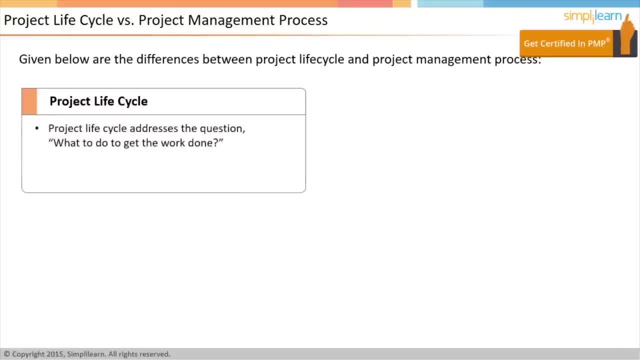 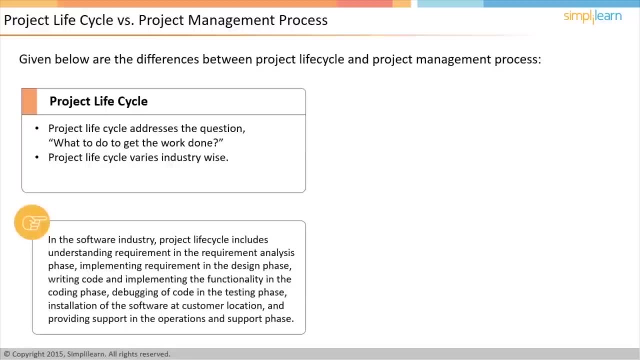 the question what to do to get the work done. It varies industry-wise, For example. let us look at a typical project life cycle in a software industry. First, you understand what is required and analyze it as part of the requirement analysis phase. 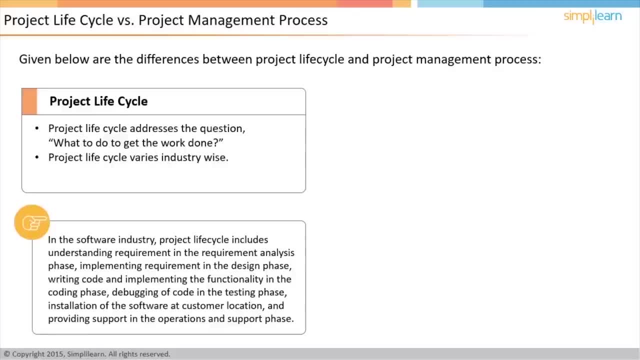 Then, as part of the design phase, you figure out the implementation of it and arrive with the approach. Next, you implement the functionality by writing the code as part of the coding phase. The code is then verified to ensure it works right as part of the testing phase. 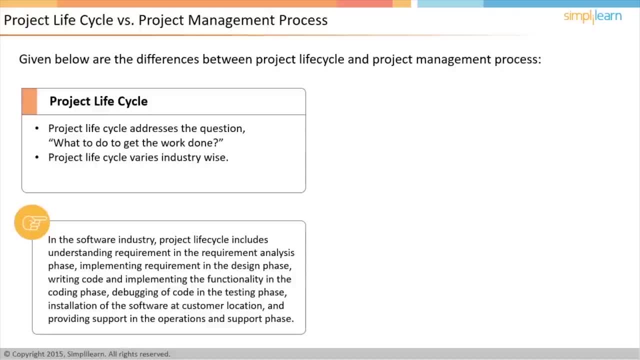 The tested and verified software is then installed at the customer locations as part of the installation phase. After the installation, the system then moves into operations and support phase. The project management process addresses the question of the project. The processes for managing the projects are likely. 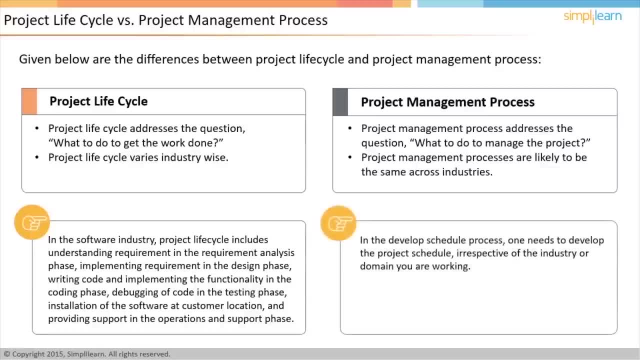 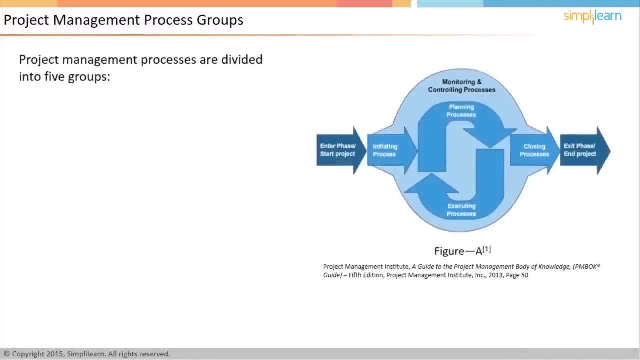 to be the same across industries. For instance, in the develop schedule process, one needs to develop the project schedule irrespective of the industry or domain you are working. In the next screen let us understand the project management process groups, The project management processes. 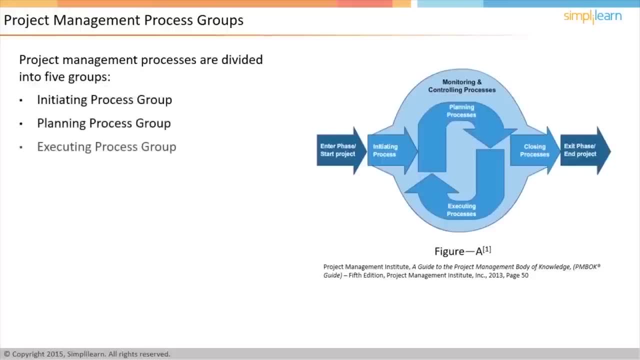 are divided into five process groups: The planning process group, executing process group, monitoring and controlling process group and closing process group. The initiating process happens at the beginning of the project or a phase. The planning, executing and monitoring and controlling processes go together. 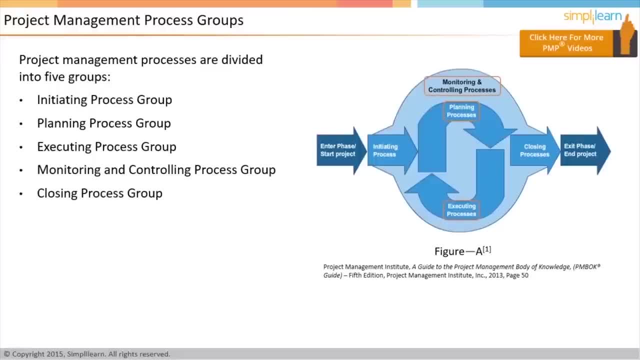 Therefore, you plan, execute and replan based on the execution result. The project closing processes are performed when the project is completed. The typical project management process in the closing phase releases resources back to the resource pool so the team members can be assigned. 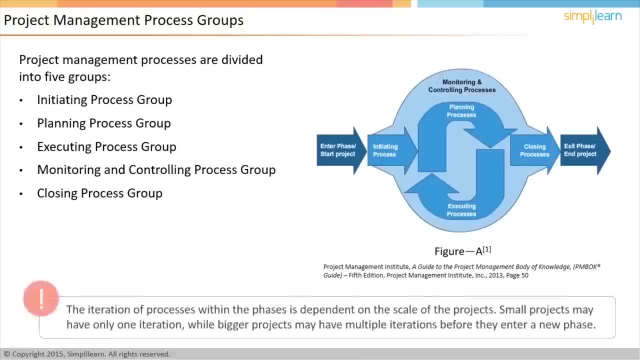 to another project. Note: the iteration of processes within the phases is dependent on the scale of the projects. Small projects may have only one iteration, whereas bigger projects may have multiple iterations before they enter a new phase. Project management processes are overlapping activities. Let us look at the interaction. 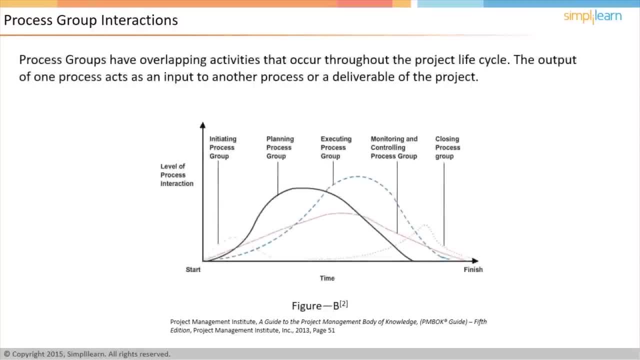 between these activities in the next screen. Process groups have overlapping activities that occur throughout the project lifecycle. The output of one process group is generally the input to another or a deliverable of the project. For example, project management plan is an output of planning process group. 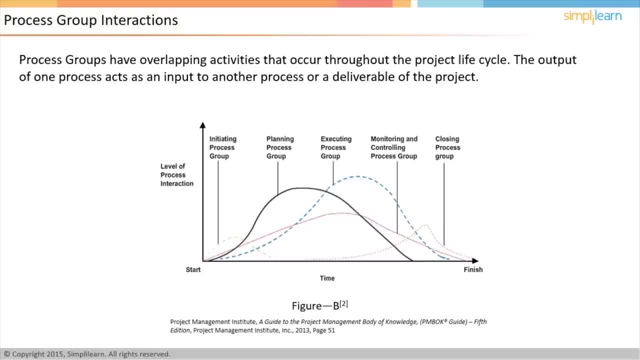 and an input to execution process group. Note that production of the plan is not a one-time activity. As the project progresses, the project management plan may get updated as a result of the monitoring and controlling processes. The updated project management plan once again forms: 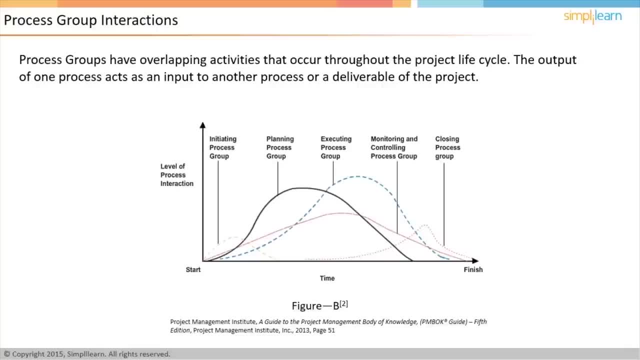 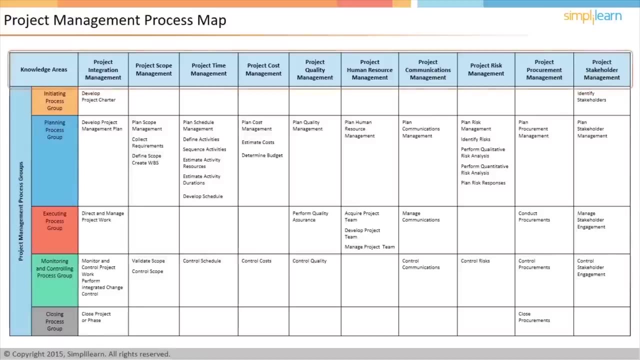 an input to the execution process group. In the next screen we will discuss the project management process group, knowledge area and project management process mapping. Given on the screen is the list of the 47 project management processes, 10 knowledge areas. 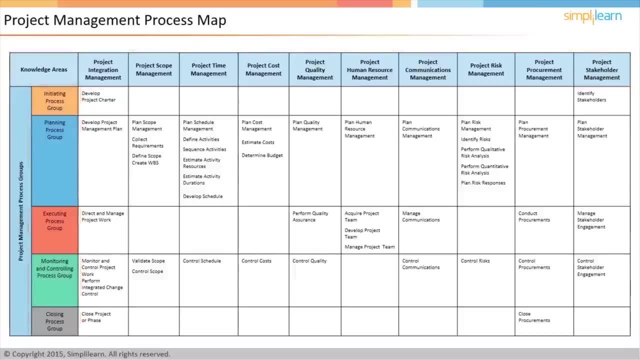 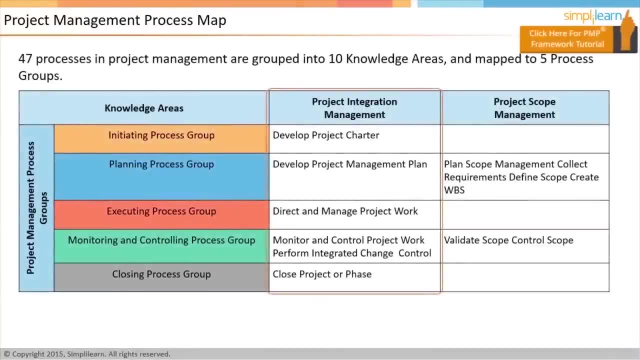 and 5 process groups. The table shows how each of them is interrelated. You can see that the project integration management processes can be mapped back to all 5 process groups, while project scope management processes are mapped back to only planning and monitoring process group. 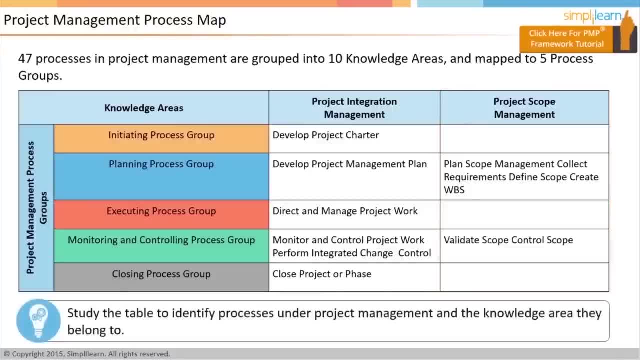 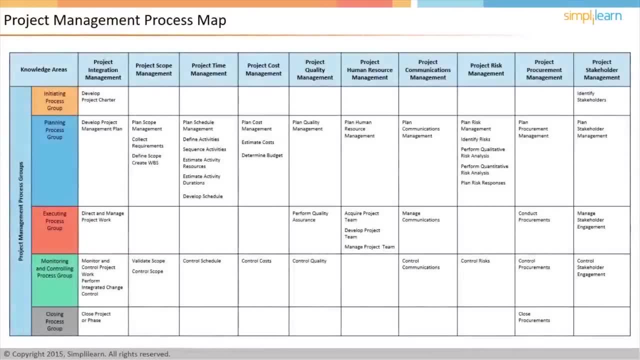 Study the table to identify processes under project management and the knowledge area they belong to. All the 47 processes are described in detail in this tutorial. Each knowledge area is covered in detail as a lesson. It also covers how the processes map to process groups to help. 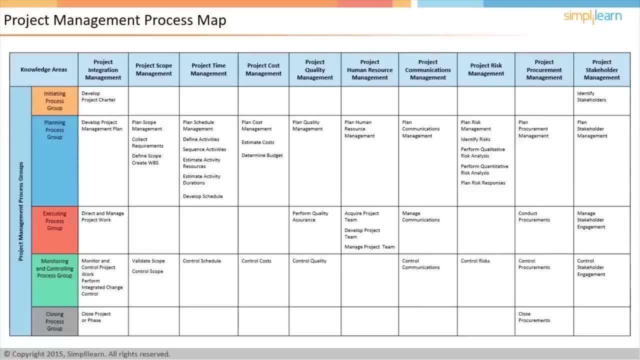 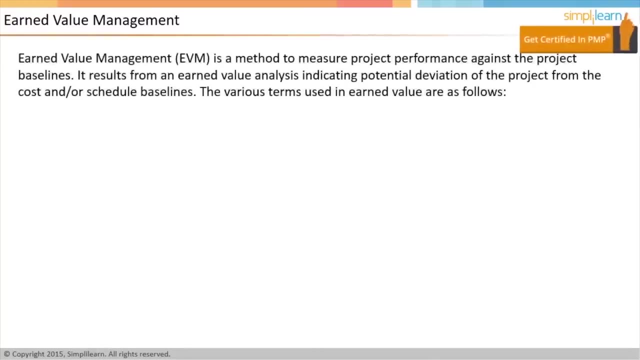 you understand the big picture. Further, the inputs and outputs of each of these processes, tools and techniques that are used in these processes and what exactly happens during these processes are also discussed. Earnings- An earned value technique is an excellent way to track the project progress. 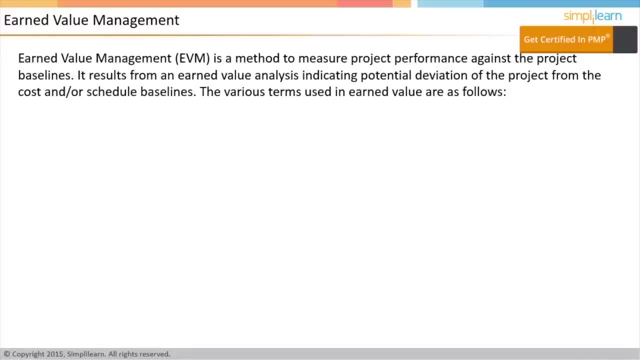 against the project plan. It is a method of measuring the project performance objectively and comparing it against the project baseline. Results from an earned value analysis indicate deviation of the project from cost and schedule baselines. Baseline is the initial approved value, along with approved changes. 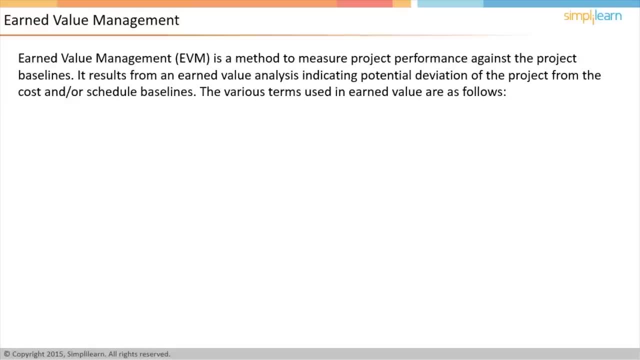 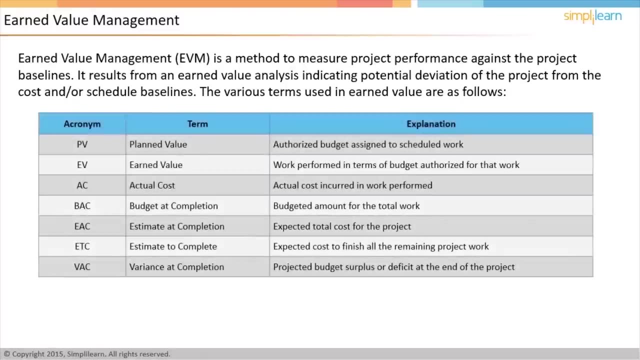 Therefore, schedule baseline is the first approved project schedule, along with approved changes. There are various terms used in earned value. technique. Planned value is the authorized budget assigned to the scheduled work. Earned value is the work performed in terms of budget authorized for that work. 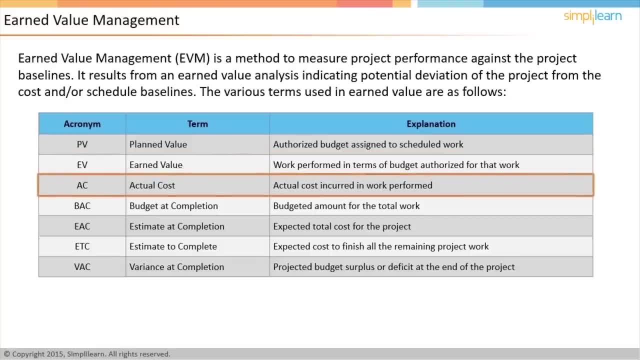 Actual cost is the cost incurred in work performed. Budget at completion is the budgeted amount for the total work. Estimate at completion is the expected total cost for the project. Estimate to complete is the expected cost to finish all the remaining project work. Variance at completion is the projected 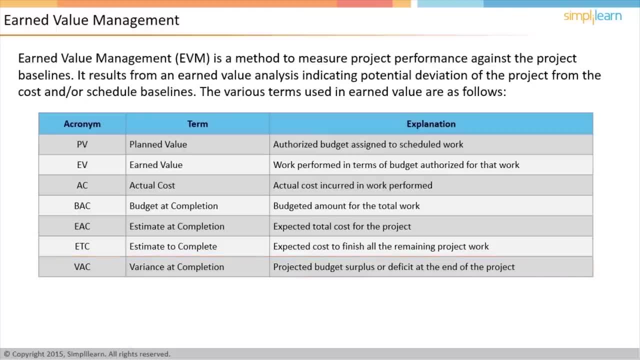 budget surplus or deficit at the end of the project. All the parameters displayed on the screen are measured in terms of cost. You may come across business scenario based questions on earned value management in the PMP exam, So ensure that you develop a clear understanding of this topic. 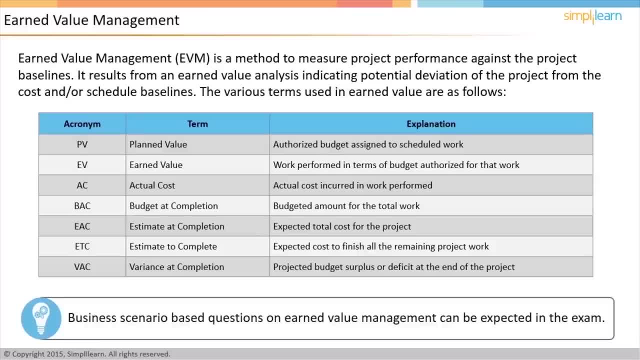 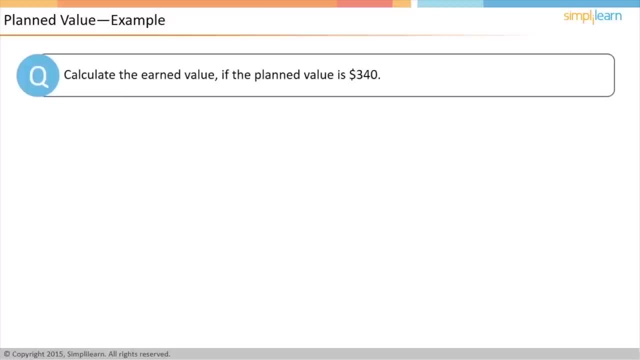 Let us look at an example of a planned value in the next screen. Planned value is the estimated value of the work planned. This value is measured in terms of currency, say dollar. If the planned value is $340,, then the work planned is worth $340.. 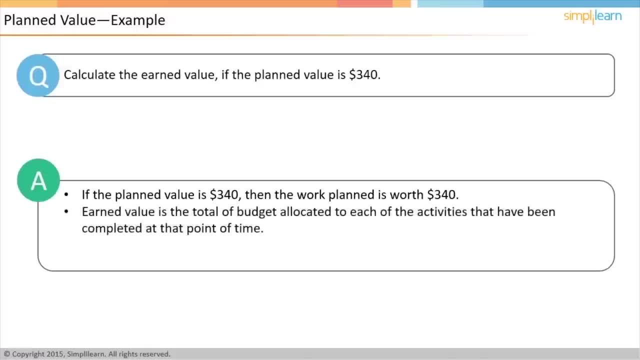 How do you calculate earned value? The solution is: add the budget allocated to each of the activities that have been completed at the point of time. The resulting value is the earned value. In the next screen, let us look at the formula, The formula used to calculate earned. 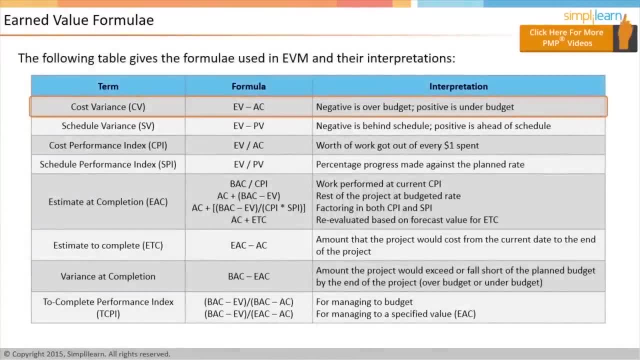 value. In cost variance: negative means the project is over budget. Positive means the project is under budget. Similarly, in schedule variance: negative means the project is behind schedule, whereas positive means the project is ahead of schedule. The value of the next two parameters: 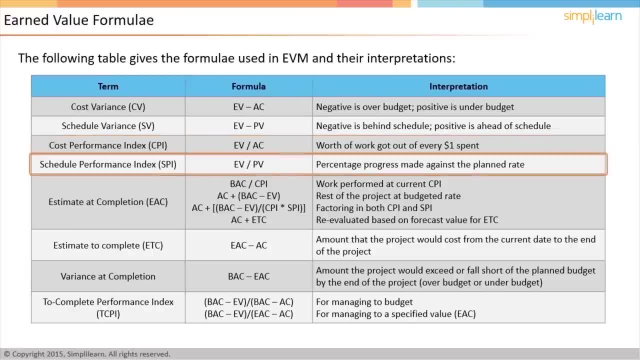 cost performance index, CPI and schedule performance index. SPI values vary between zero and one. For example, a CPI of 0.8 implies that 80 cents of work is obtained for every dollar spent in the project. Similarly, if SPI is 0.9,. 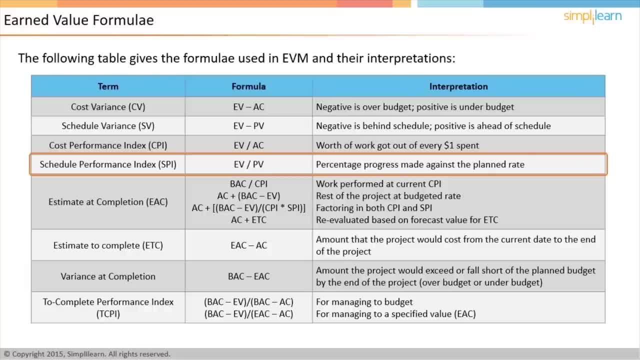 it implies that project is progressing at only 90% of the speed originally planned. The next parameter is estimate at completion, or EAC. There are different ways of calculating the EAC value. The method used depends on how the cost and schedule variances are expected to play. 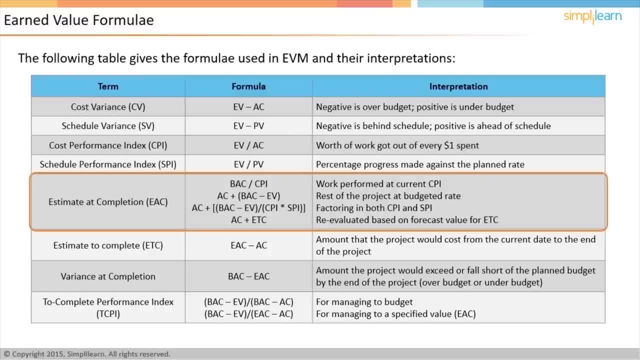 for the rest of the project. BAC by CPI is used if you expect that the current cost performance will continue until the end of the project. AC plus BAC minus EV is used if you expect that the rest of the project will be managed at the budgeted rate. 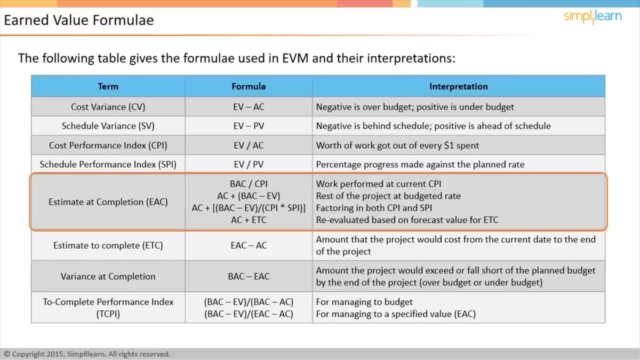 AC plus BAC, minus EV by the product of CPI and SPI is used if you want to factor in the impact of the cost as well as schedule variances. AC plus ETC is used if you want to re-evaluate the project based on a forecast value. 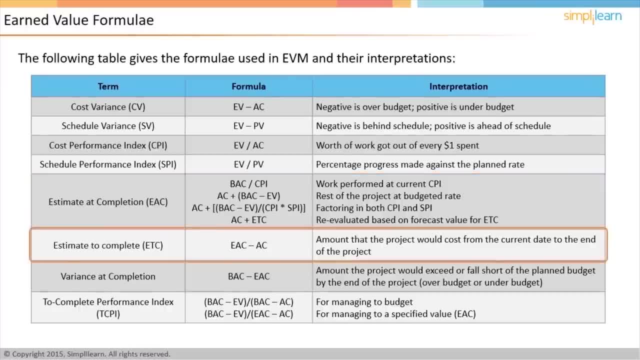 for the estimated cost of the remainder of the project. The next parameter is estimate to complete or ETC, which is the cost of project from this point to the end. This is calculated by subtracting the actual cost from the estimate at completion. In addition, 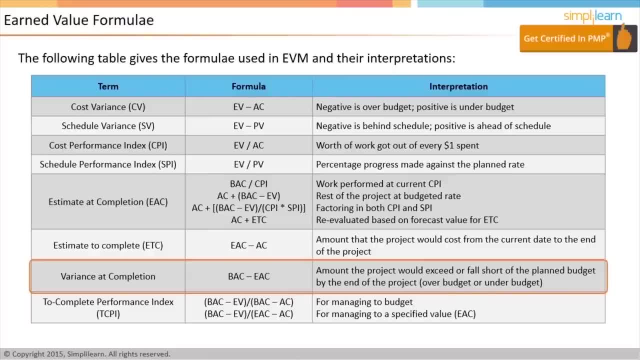 variance at completion can be calculated by subtracting the estimate at completion from the budget at completion. Variance at completion is the cost estimation, whether it is over or under budget. Another parameter is the to complete performance index, or TCPI. This is the cost. 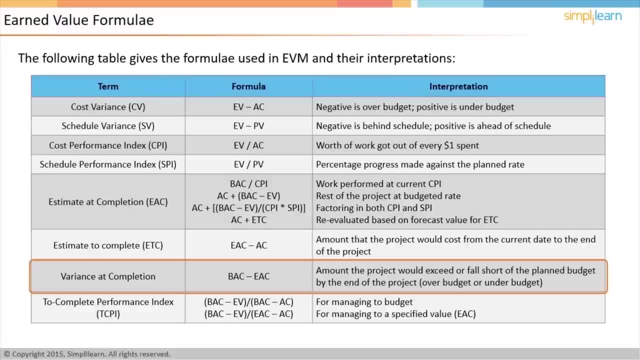 performance needed to achieve a desired outcome. For example, if the project needs to be managed to the original budget BAC, then TCPI- that is, the CPI that must be maintained for the rest of the project- is calculated as BAC minus EV by BAC minus AC. 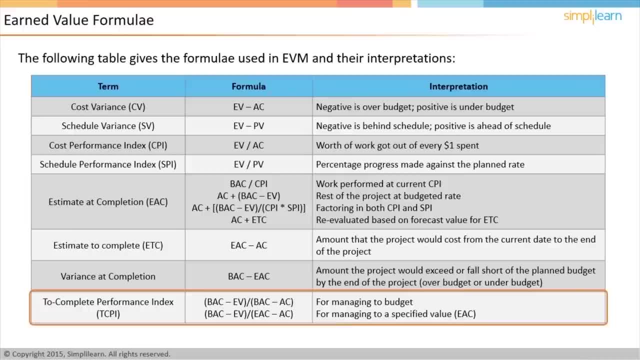 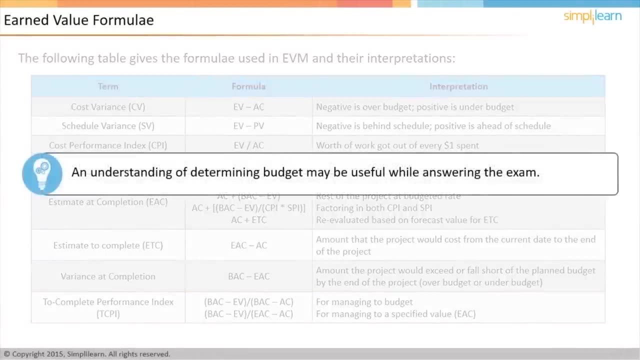 Similarly, if it has to be managed within a revised target, say EAC, then TCPI is calculated as BAC minus EV, by EAC minus AC. Before the start of the PMP exam, please make a note of the formulas of earned. 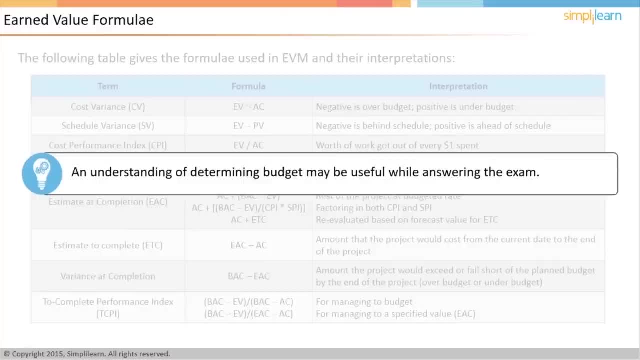 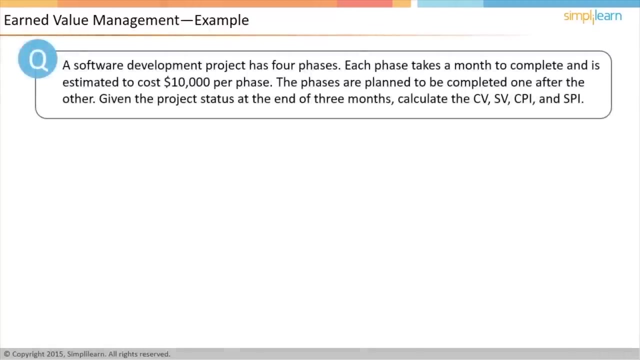 value technique. In the next screen, let us look into a business scenario to understand this concept better. After reading the problem statement, click the solution button to look at a possible answer. Let us take the example of a software development project. There are four phases and 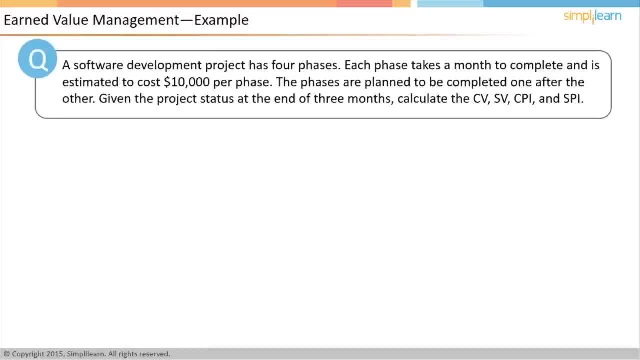 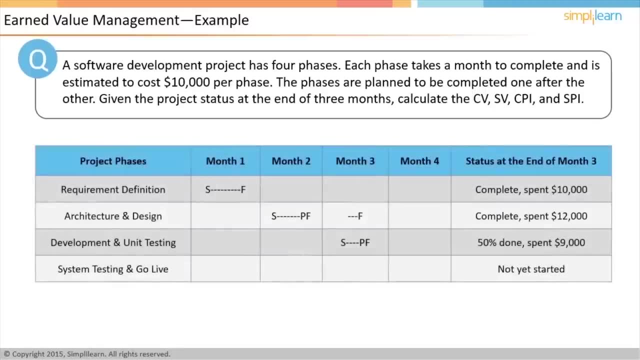 each phase takes a month to complete and is expected to cost $10,000.. The phases are planned to be completed one after the other. The status of the project at the end of the month 3 is summarized in the table. Requirements definition is completed. 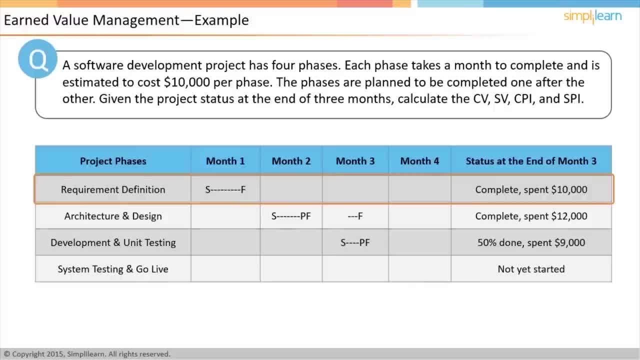 and actual spending on this is $10,000.. Architecture and design is done, and actual spending on this is $12,000.. Development and unit testing is only 50% done. though it was supposed to be completed by third month, It has. 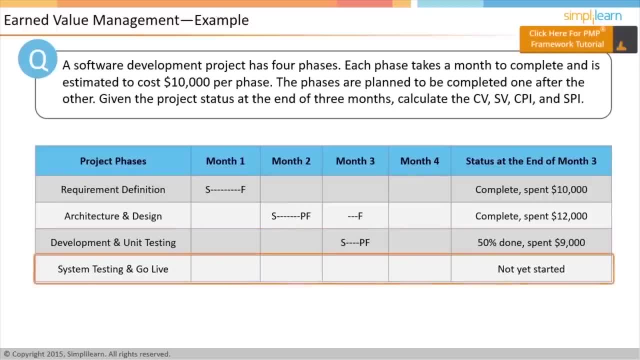 cost $9,000. until date, System testing and go-live has not yet started. Note S indicates start time, F indicates finish time and PF indicates that it is partly finished at the end of the month. Based on the above information, calculate the. 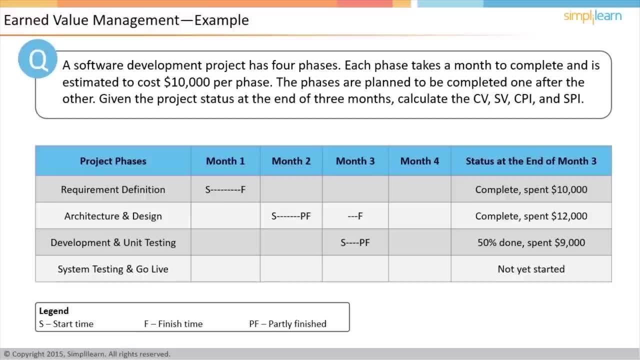 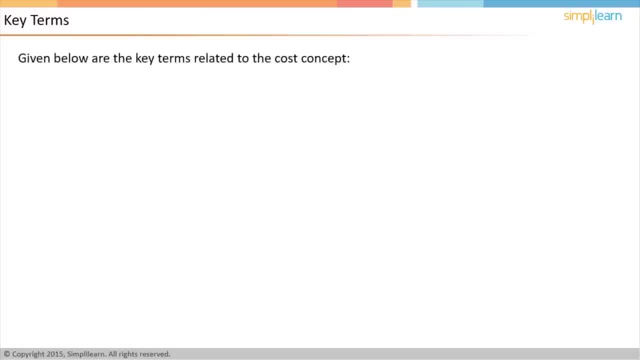 CV, SV, CPI and SPI of the project. Let us look at a solution in the next screen. Before we end this lesson, let us also look at a few definitions that might be useful for your PMP examination. Law of diminishing return. This means: 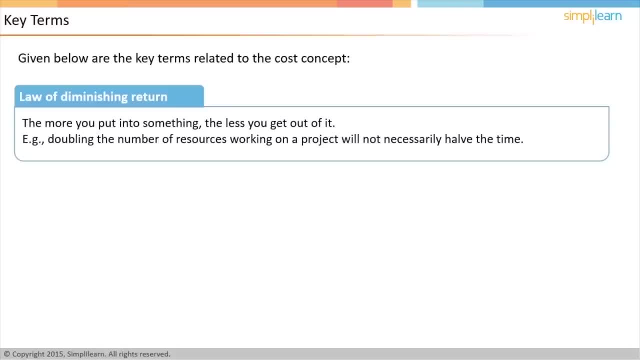 the more you put into something, the less you get out of it. For example, doubling the number of resources working on a project will not necessarily halve the time Working capital, The amount of money the company has to invest on the project and the 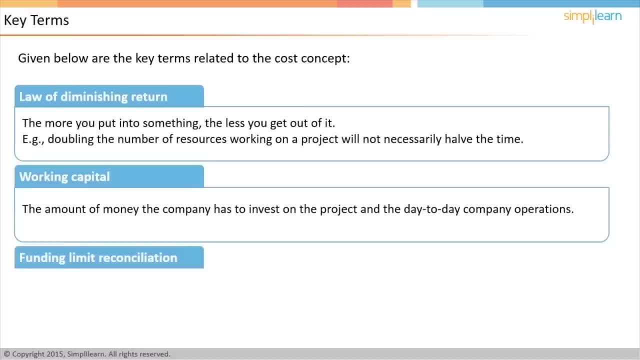 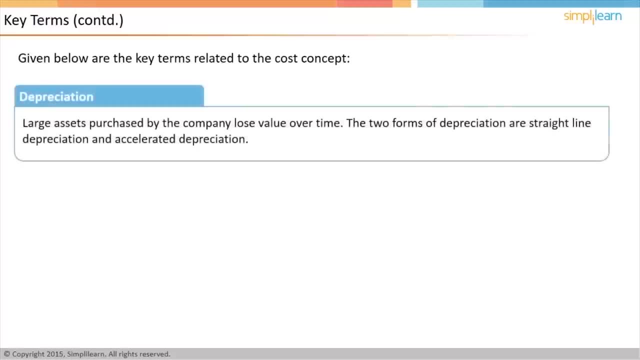 day-to-day company operations. Funding limit reconciliation: The process of comparing the planned expenditure in a given period with the available funding for that period. Large assets purchased by the company lose value over time. This is called depreciation. There are two forms of depreciation. 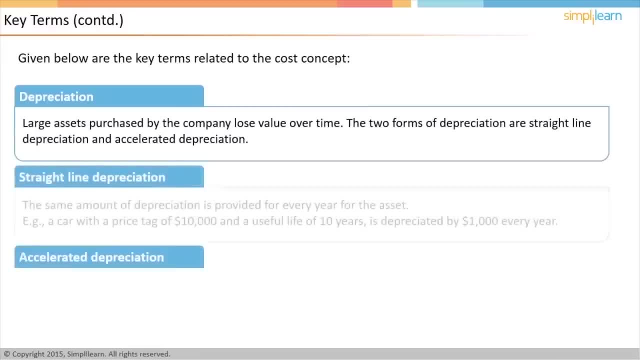 Straight line and accelerated. Same amount of depreciation is taken every year. For instance, a car with a price tag of $10,000 and useful life of 10 years is depreciated $1,000 per year At the end of the tenth. 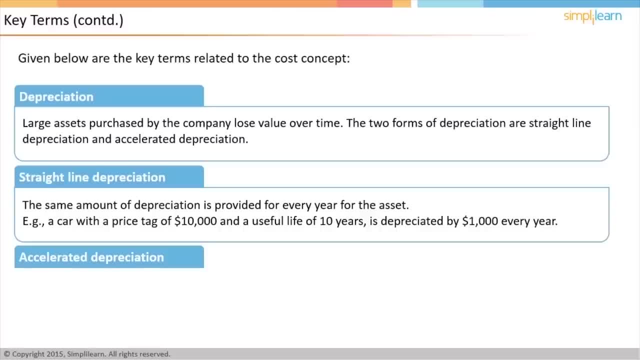 year, the value of the car is considered zero for all accounting purposes. Accelerated depreciation Depreciates faster than the straight line depreciation. For instance, a car with a price tag of $10,000 depreciates $3,000. the first. 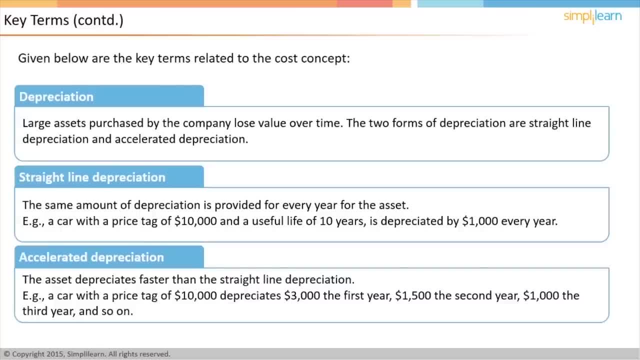 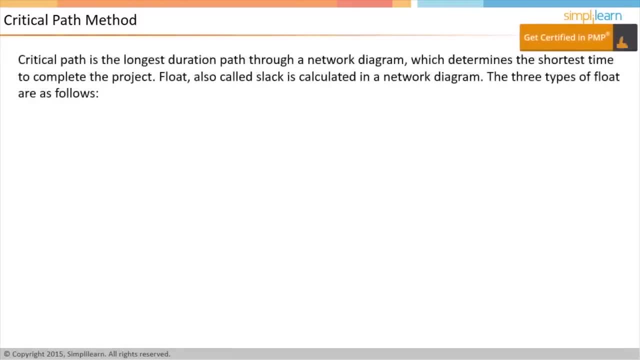 year $1,500, the next year $1,000, the third year and so on. Critical path is defined as the longest duration path through a network diagram which determines the shortest time to complete the project. Float can be considered as: 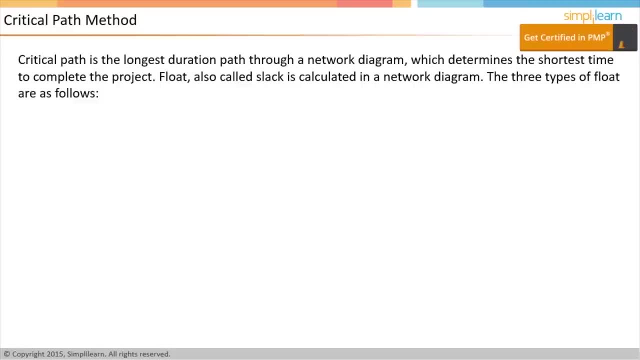 a buffer time available to complete an activity. Float is calculated once the network diagram is ready. It is also called as slack. There are three kinds of float, The first being the total float, which is the amount of time an activity can be delayed without delaying the. 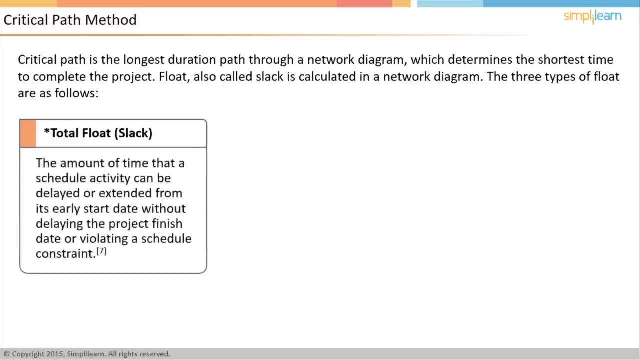 project end date or an intermediary milestone. The second type of float is free float, which is the amount of time an activity can be delayed without delaying the early start date of its successor or successor's activities. The last type is independent float, which is the amount of time 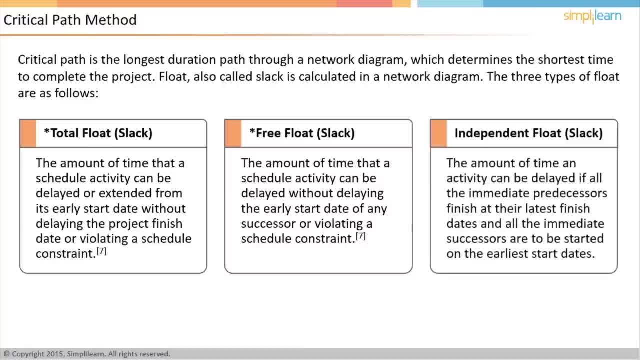 an activity can be delayed if all the predecessors finish at their latest finish dates and you want to start all the immediate successors at their earliest start dates. The slack of the activities on the critical path is zero, because there is no scope to delay activities on the 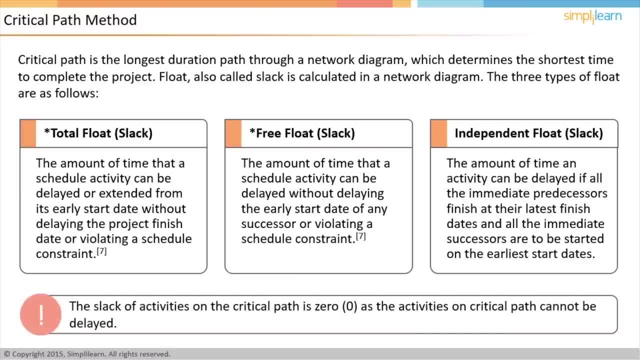 critical path. Critical path actually represents the project duration. Delaying activities on the critical path is as good as delaying the project duration. Concept-based questions on critical path can be expected in the exam, so it is essential to have a clear understanding of the concept. 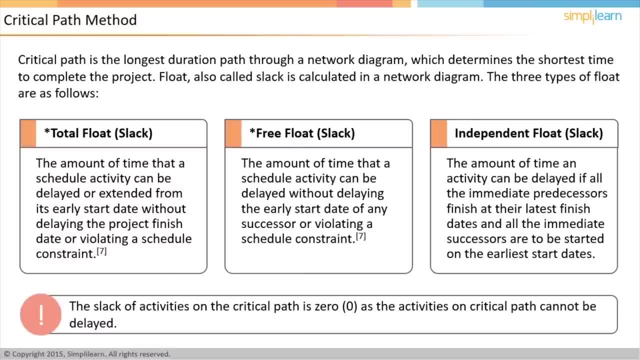 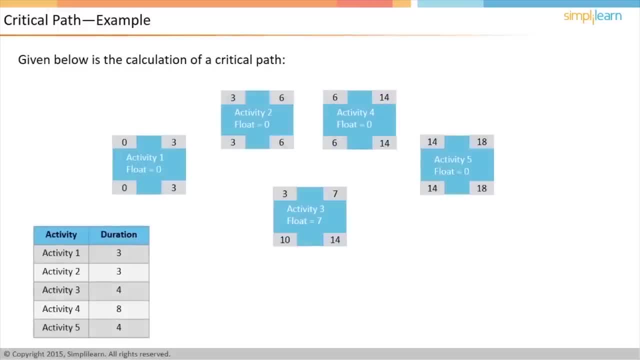 In the next screen. let us learn how to calculate float. Let us look at an example for critical path. There are five activities in this project and two paths in the network diagram. Start, 1,, 2,, 4,, 5, end is 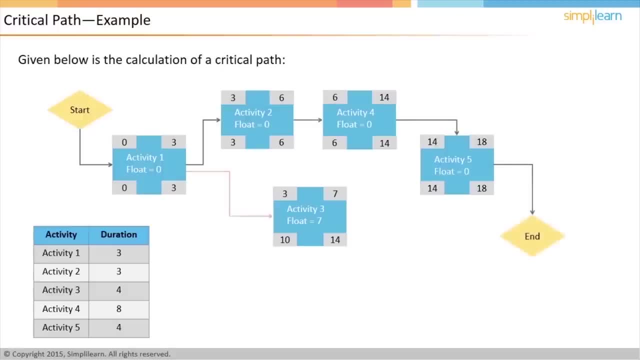 one path, and start, 1,, 3,, 5, end is the second path, Since the duration of the path- start 1,, 2,, 4,, 5, end- is 18 days, which is more than the duration of the path. 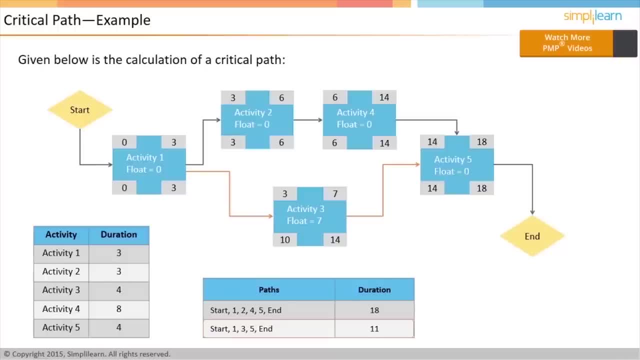 start 1,, 3,, 5, end. the critical path of the project is start, 1,, 2,, 4,, 5, end. Let us take activity 3 as an example. First, calculate the early start and early finish. 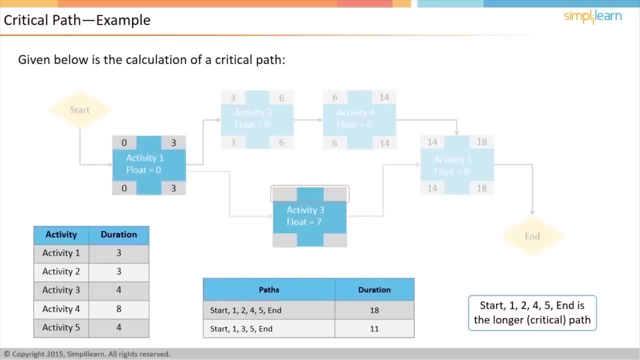 dates. Activity 3 can start only after activity 1.. Since the early finish of activity 1 is 3, it becomes the early start of activity 3.. Activity 3 cannot start earlier than 3 because activity 1 can be completed. 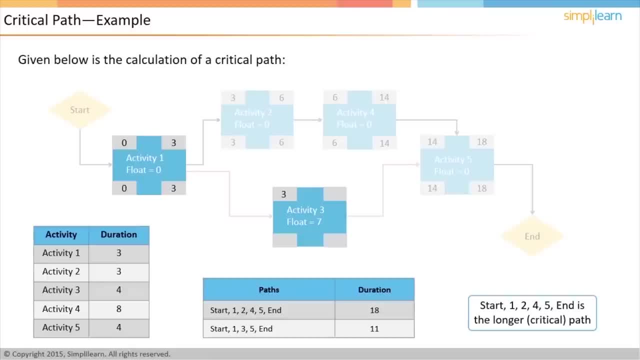 only by then. Therefore, early start of activity 3 is 3,. since the duration of the activity is 4 days, The early finish of activity 3 is 3 plus 4 equals 7 days. Now let us calculate the late start and late finish. 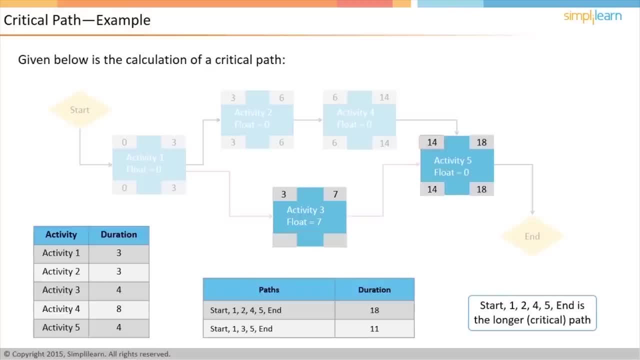 of activity 3.. Late start of activity 5 is 14 days. The activity 3 happens just before activity 5.. So the late finish of activity 3 is 14 days. To calculate the late start you can subtract the duration from late. 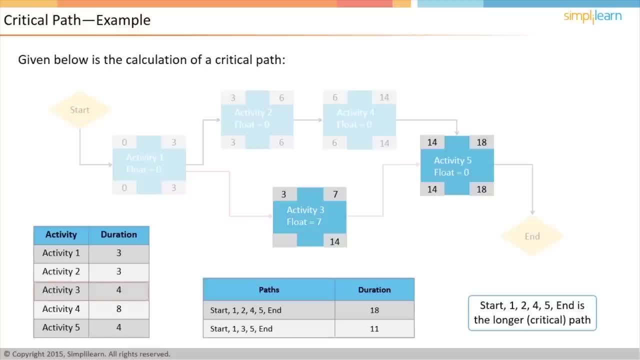 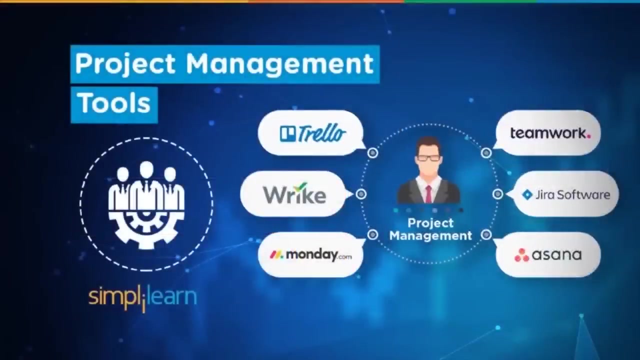 finish. Therefore, the late start of activity 3 is 14 minus 4 equals 10.. In the next screen, let us focus on schedule compression. Hi, welcome to project management tools tutorial from SimplyLearn. I am CMR Chandra MR a. 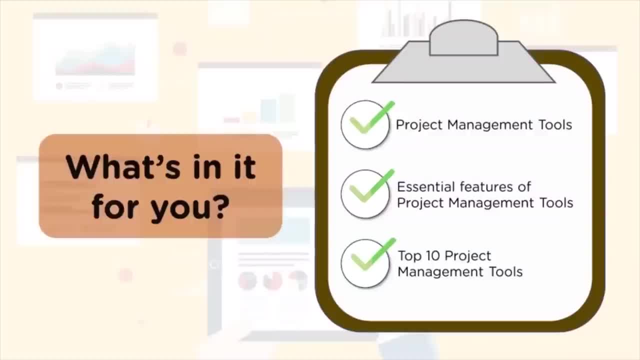 certified project management professional. As part of this tutorial we are going to look at about project management tools, essential features of project management tools, top 10 project management tools currently used in the industry. So what is project management tools? Why should we use? 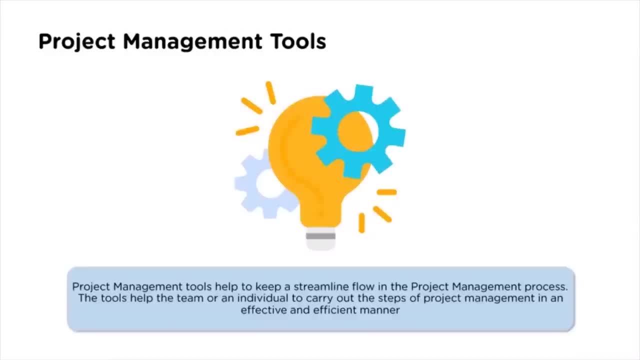 project management tools while doing project management. So project management tools help to keep a streamlining flow in project management processes. The tools help the team or an individual to carry out the steps of project management in an effective and efficient manner. So project 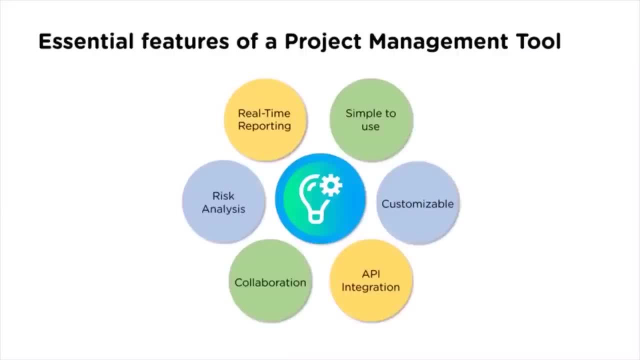 management tools features and functionalities. So basically, a project management tool should have minimum fulfilling these features and functionality. They should be simple to use, customizable. They should have API for integration. It should help in collaboration. It should help in risk analysis and real-time reporting. 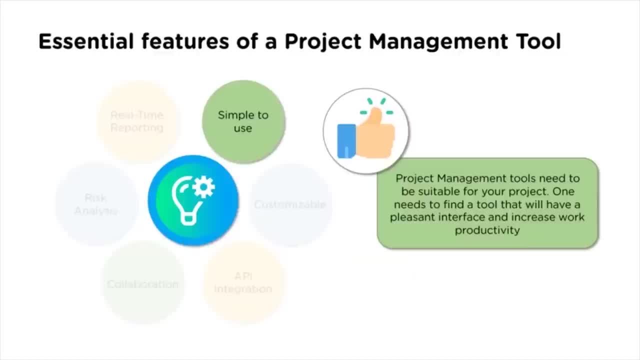 When we say simple to use, the project management tools need to be suitable. for every project we do, One needs to find a tool that will have a pleasant interface and increase work productivity. The project management tool must be easy to configure according to the organization needs Every. 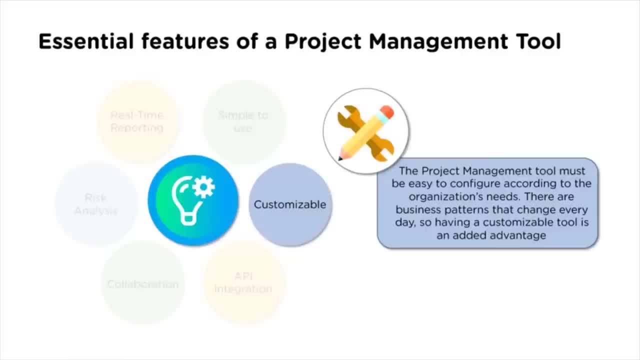 project management approach, every project management templates, every artifacts needs tailoring and adaption before adopting as part of the practice. There are business patterns that change every day, So having customizable tool is an added advantage. API or application programming interface enables the sharing of data. 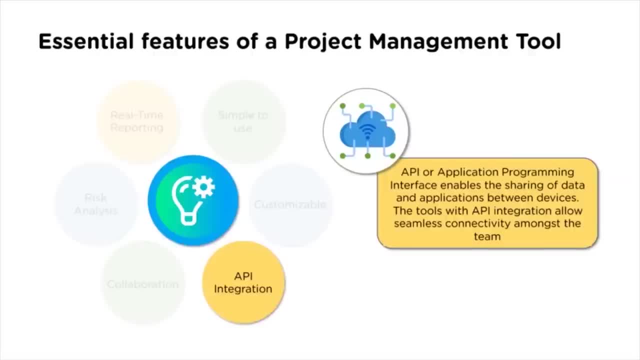 and application between devices. The tools with API integration allow seamless connectivity amongst the team. The project management tools must allow for collaboration so that whole team can work together. Collaboration not only makes the task easier, but also increases the productivity of the project. Risk analysis helps to identify. 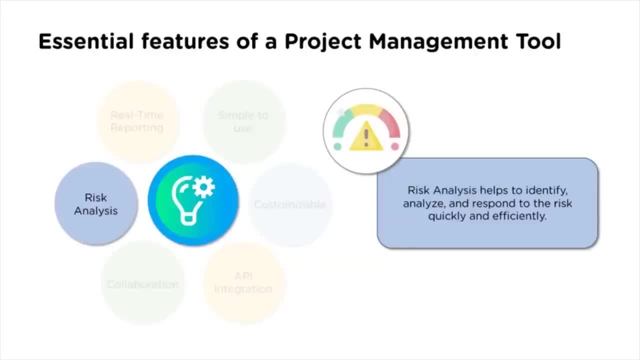 analyze and respond to the risk quickly and efficiently, It needs to capture all the details of the risks, their impacts, the probability of occurrence of the risk and risk responses, and tracking them throughout the project life cycle. The real-time reporting enables the access of data at different locations. 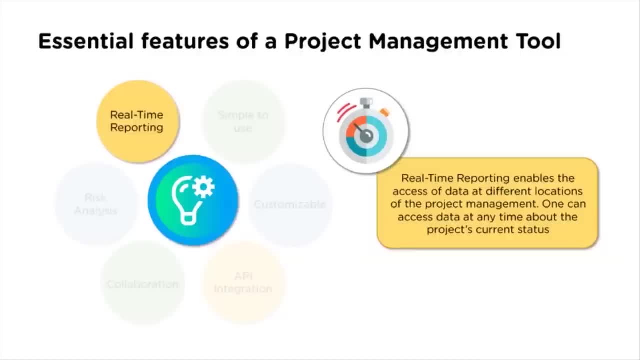 of the project management. One can assess or access data at any time about the project's current status. This will help in having a real-time update about the project status to the stakeholders of the project. The top 10 project management tools: what we have today. 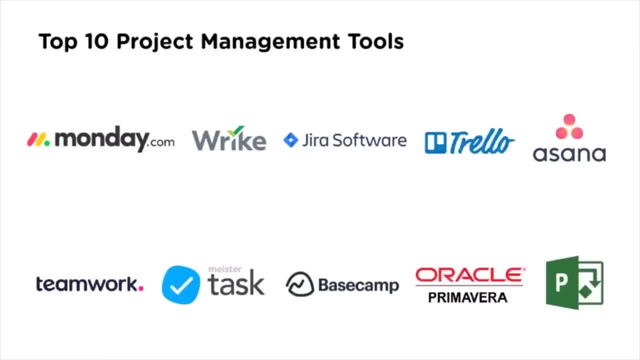 in the market are Mondaycom, RIC, Jira Software, Trello, Asana, Teamwork, MeisterTask, Basecamp, Oracle's Primavera and Microsoft project management tool. So let us look at these one by one. 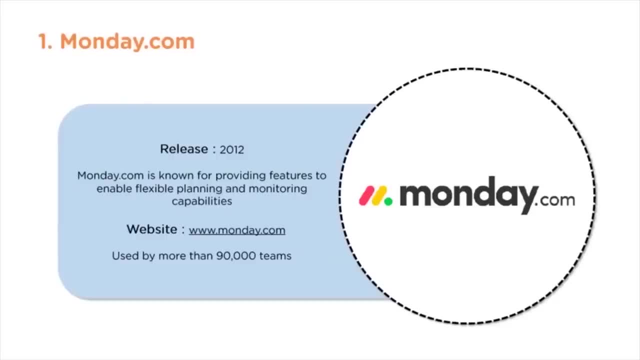 So Mondaycom was released during the year 2012 and it is known for providing features to enable flexible planning and monitoring capabilities. The website where you can find Mondaycom access the tool is wwwmondaycom, So this tool is used by more than. 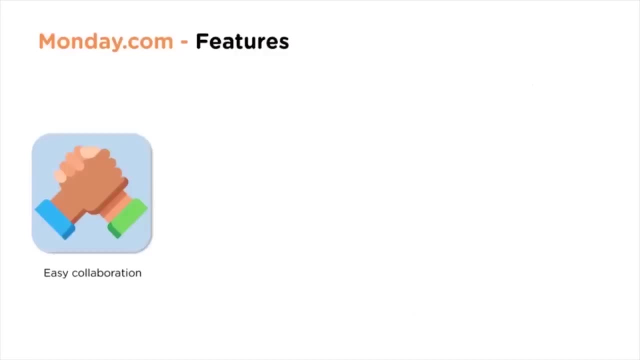 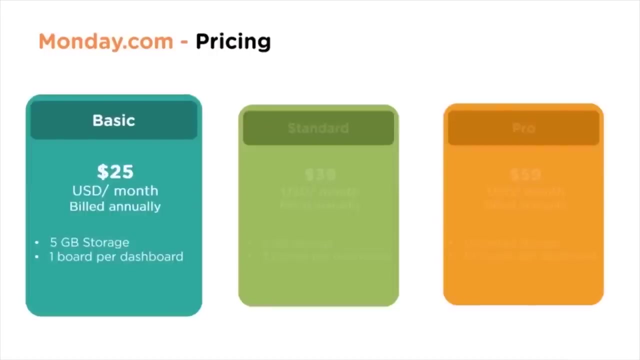 90,000 teams across the globe. Mondaycom features and functionality includes: it is easy for collaboration, highly customizable, excellent for analytics. integration with Dropbox, Google Drive and Pipedrive is possible. So pricing: the basic version is $25 on monthly basis, so which will. 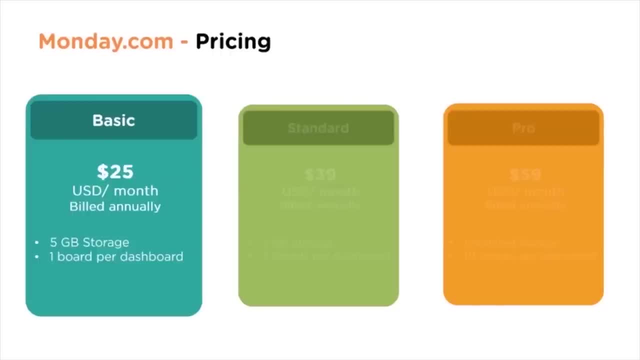 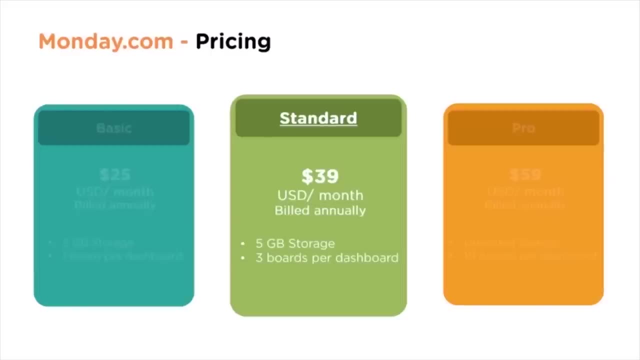 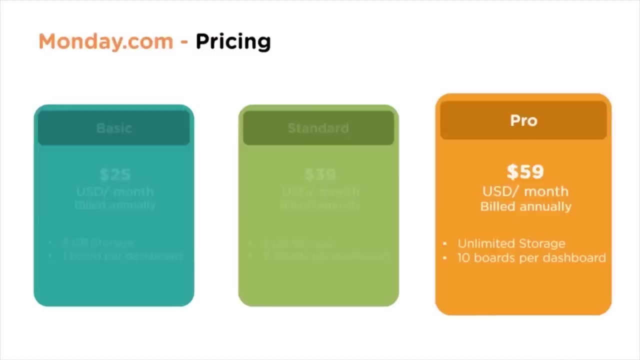 provide you 5 GB storage, one board per dashboard, and it is billed annually. The standard package includes 5 GB storage, 3 boards per dashboard, and it is $39 per month, which is billed annually. Professional includes unlimited storage: 10 boards per dashboard. 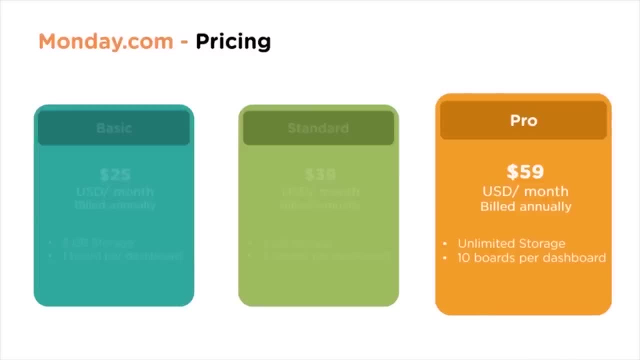 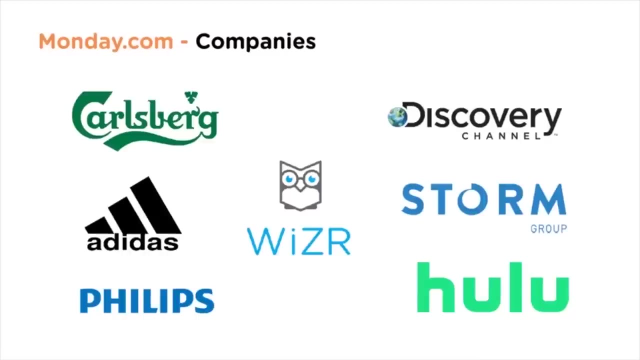 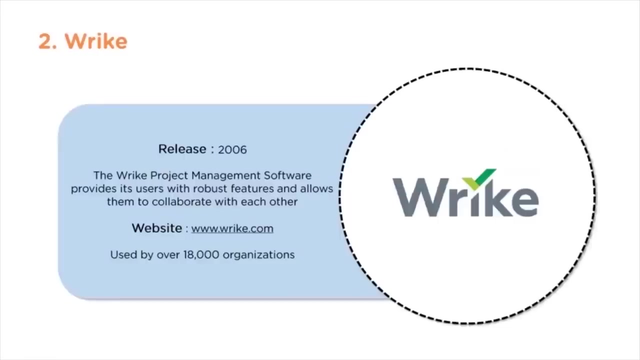 and it costs $59 per month and it is billed annually. Mondaycom is used by the following customers: organizations of Mondaycom, that is, Girlsburg Discovery Channel, Adidas, Tom, Philips, etc. Rick is another project management tool which was released in 2006.. 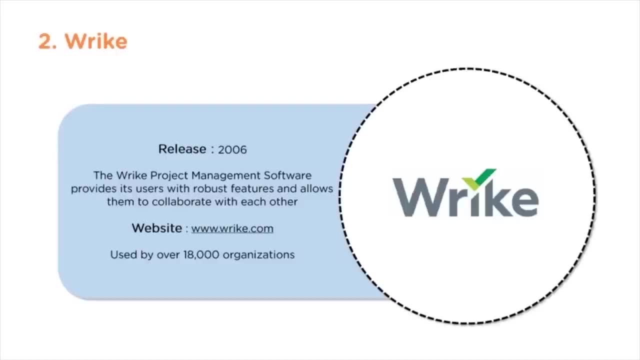 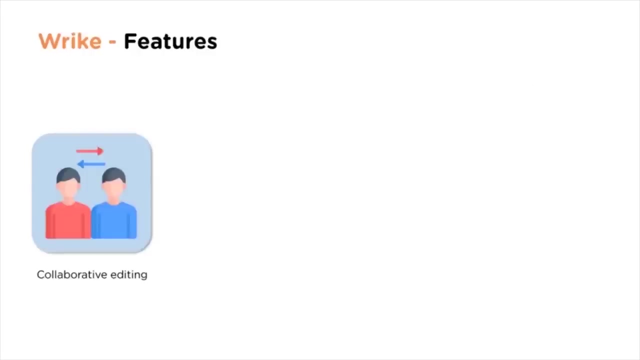 So this application provides its users with robust features and allows them to collaborate with each other. The website to access the tool is wwwrickcom, and this is used by over 18,000 organizations across the globe. The features of Rick includes: it has collaborative editing. 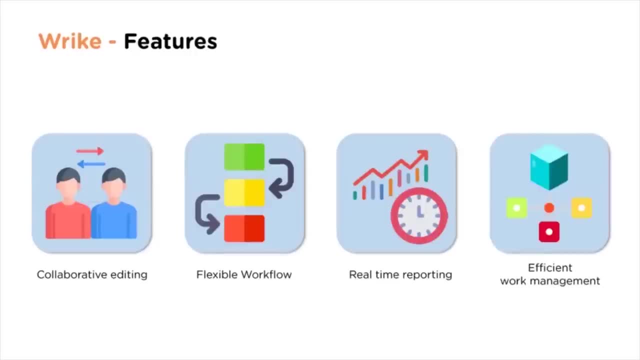 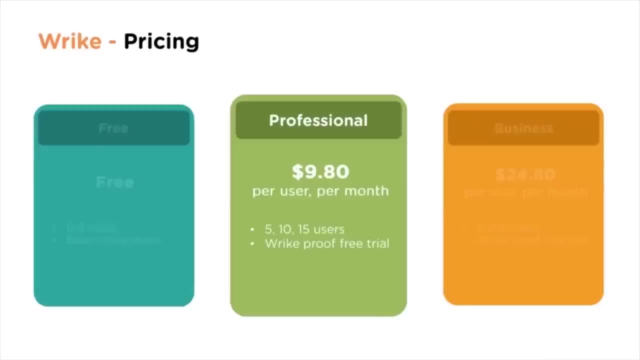 flexible workflow, real-time reporting and efficient work management. The pricing includes 0 to 5 users, it has basic integrations and which is free, whereas professional includes $9.8 per user per month, which has a slab of 5, 10 and 15 users. 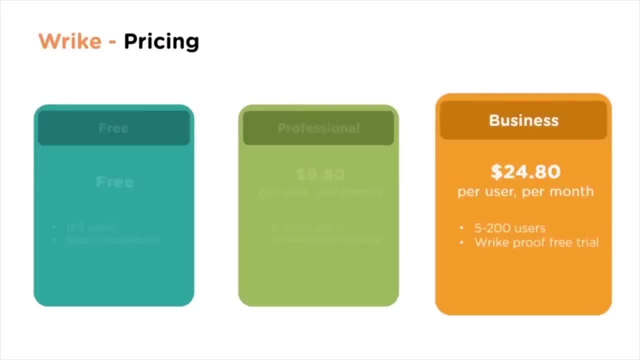 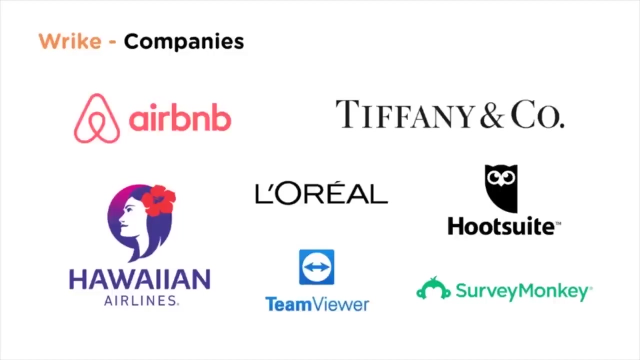 and Rick proof free trial. Business version has 5 to 200 users and Rick proof free trial, whereas $24.80 per user per month. The companies which uses Rick tools are Airbnb, Laurel, Teamviewer, Tiffany & Co, etc. Now let us look at Jira software. 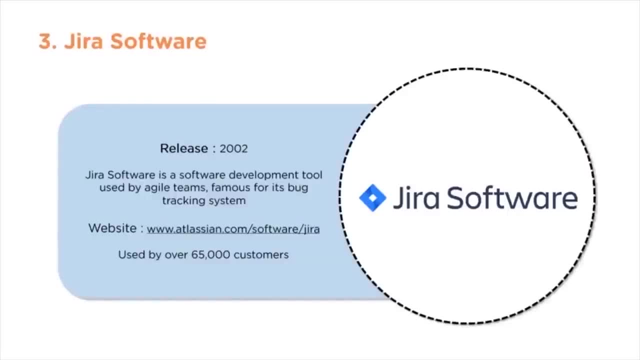 Jira software was released during year 2002.. It is a software development tool used by Agile teams, famous for its bug tracking system. The website to access this tool is wwwatlassiancom. slash software- slash Jira- used by over 65,000. 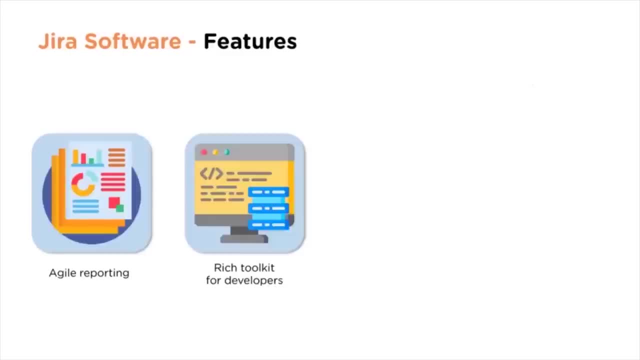 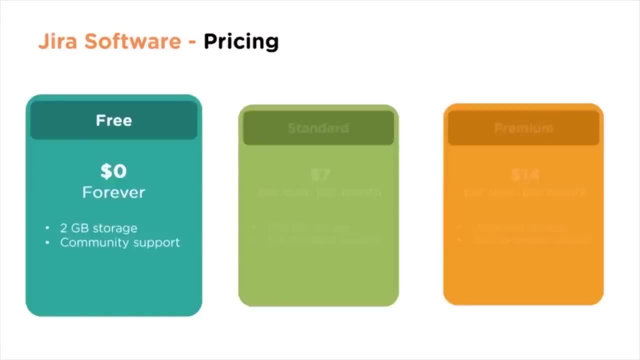 customers. The features of Jira software includes Agile reporting, rich toolkit for developers, bug tracking, mobile applications. So the pricing of Jira software is as follows: So for forever, 2 GB storage and community support which cost $0, whereas standard is around. 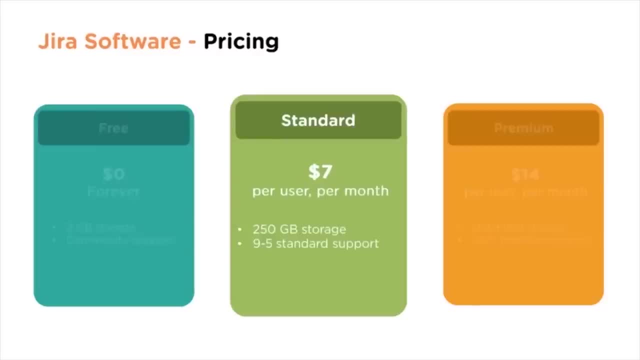 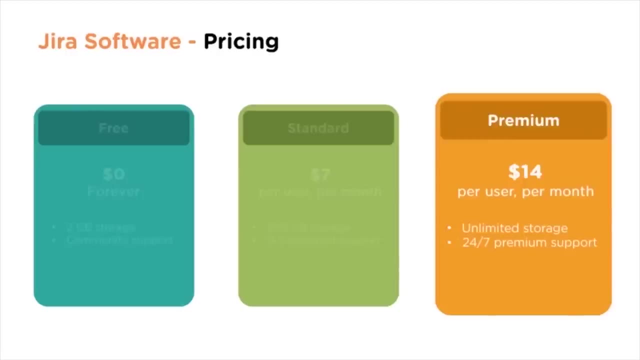 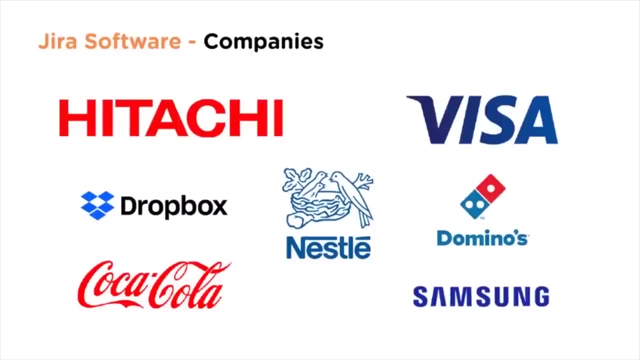 $7 per user per month, which includes 250 GB storage and 9 to 5 standard support. Premium is $14 per user per month unlimited storage and has 24.7 premium support. Jira software is used by the organizations, that is: Itachi, Visa, Dropbox. 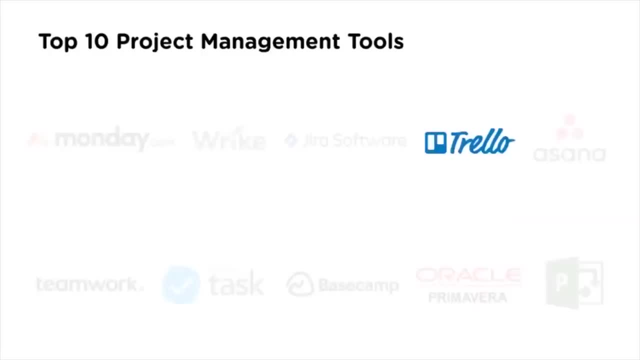 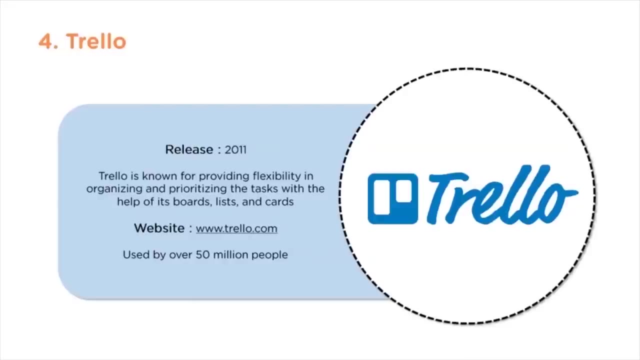 Nestle, Domino's, Coca-Cola, Samsung, etc. Now let us look at the tool Trello. So this application was released in 2011.. It is known for providing flexibility in organizing and prioritizing the tasks with the help of its boards. 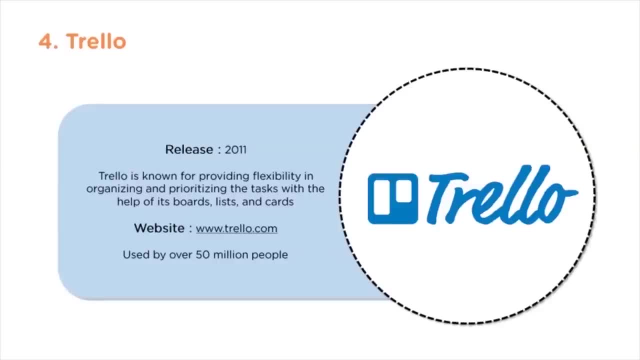 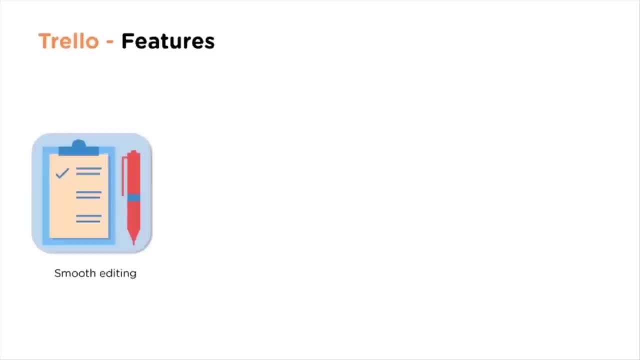 lists and cards. Website to access the tool is wwwtrellocom, used by over 50 million people. The features of Trello include smooth editing, easy file uploads from Dropbox or Google Drive, high security standards and easy data searching techniques. So the pricing includes: 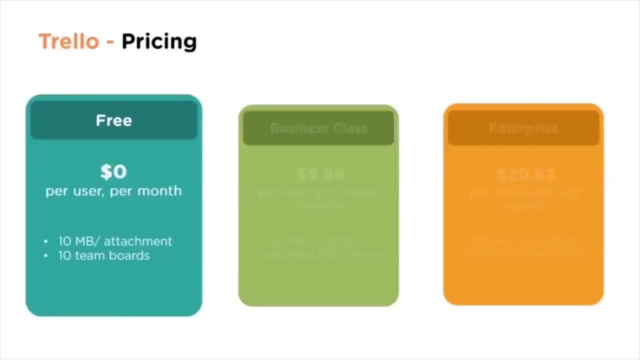 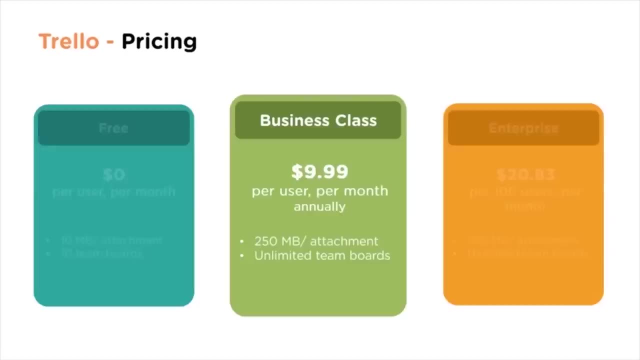 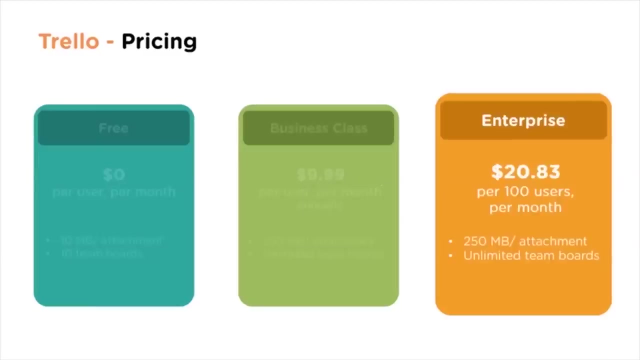 it is free for 10 MB per attachment and 10 team boards. Business class includes 250 MB attachment, unlimited team boards and it cost $9.99 per user per month annually. Enterprise version provides 250 MB per attachment, unlimited team boards and costs around. 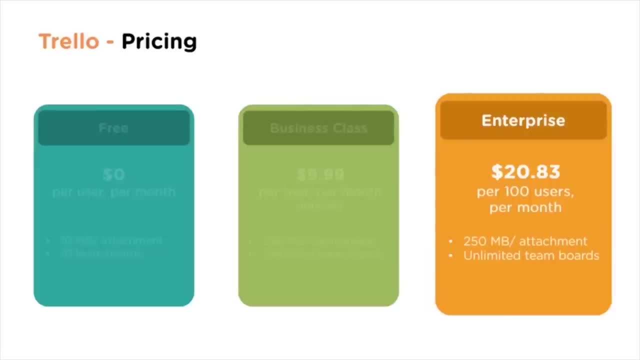 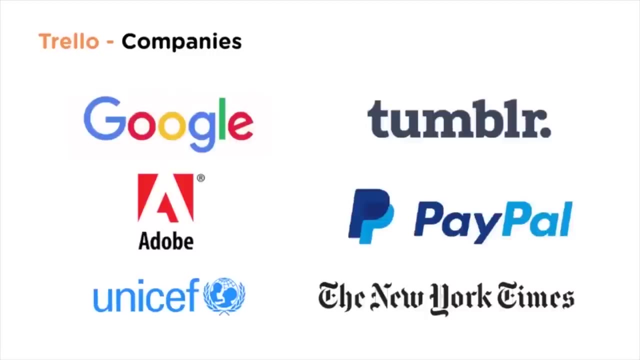 $20.83 per 100 users per month. The companies who use Trello are Google, Adobe, PayPal, Unicef, The New York Times, etc. Now let us look at Asana. The Asana tool was released during 2008.. 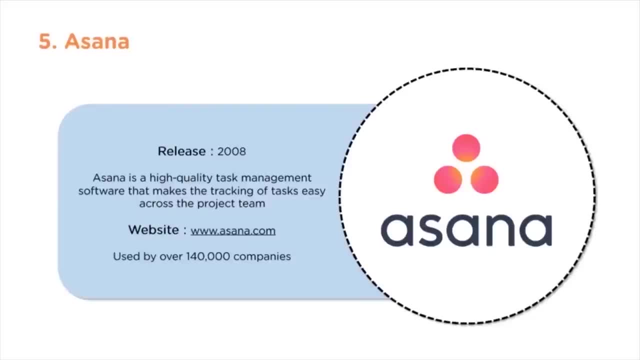 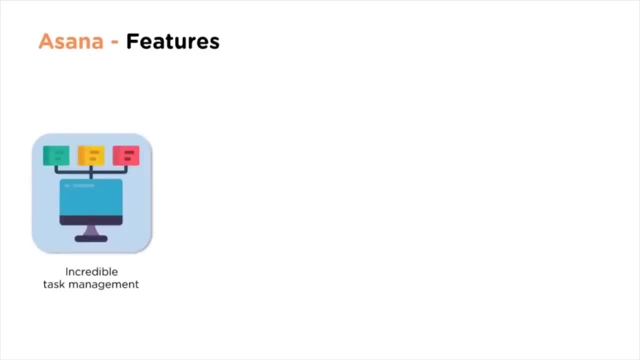 It is an high quality task management software that makes the tracking of tasks easy across the project management. The website to access this tool is wwwasanacom, used by over 140,000 companies. The features includes incredible task management, Gantt charts, privacy controls. 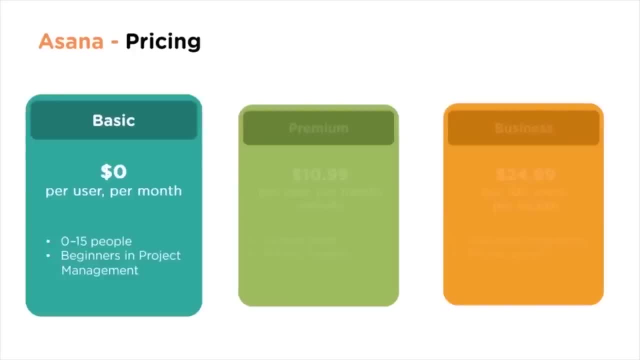 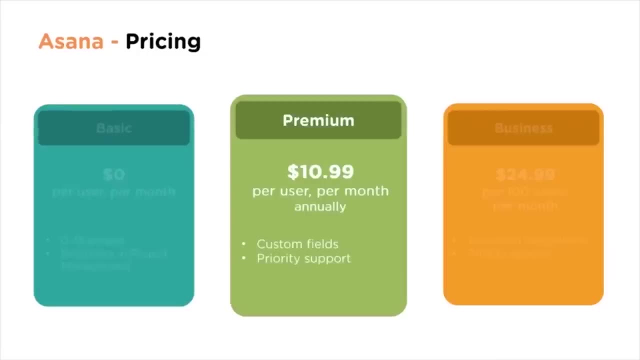 easy progress tracking. The pricing includes the basic model. Asana is provides 0 to 15 people beginners in the project management, So premium includes custom fields priority support, where the pricing is $10.99 per user per month annually. The business version includes advanced 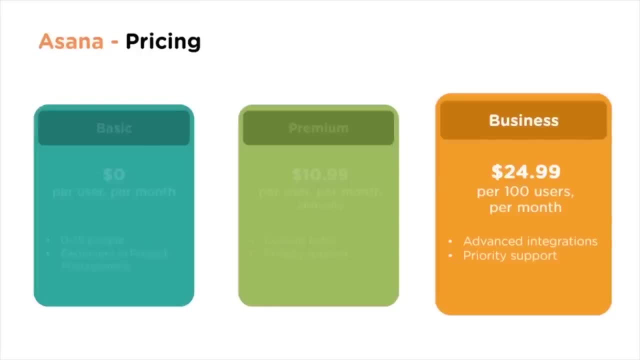 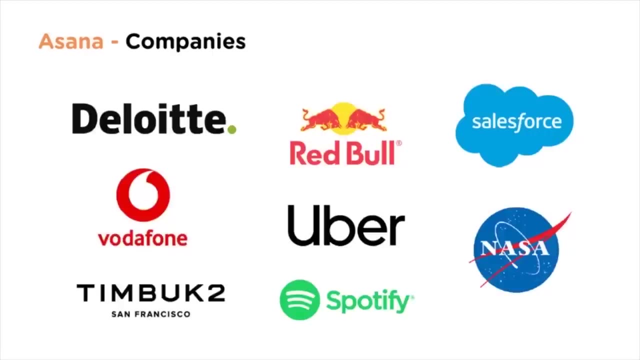 integration priority support and it costs $24.99 per 100 users per month. The companies which uses Asana are Deloitte, Vodafone, Red Bull, Uber, Salesforce, NASA, etc. Let us look at Teamwork tool. Teamwork was 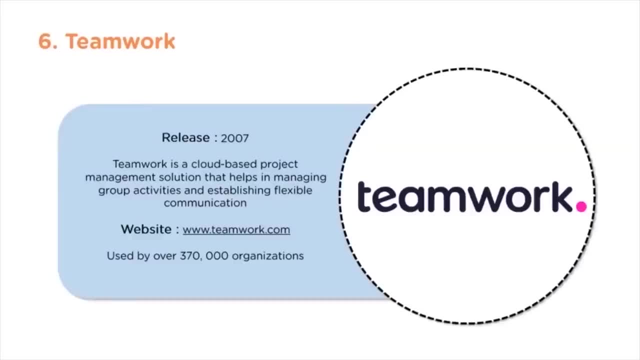 released during year 2007.. It is a cloud based project management solution that helps in managing group activities and establishing flexible communication. The website to access this tool is wwwteamworkcom, used by over 370,000 organizations. The features of Teamwork includes: 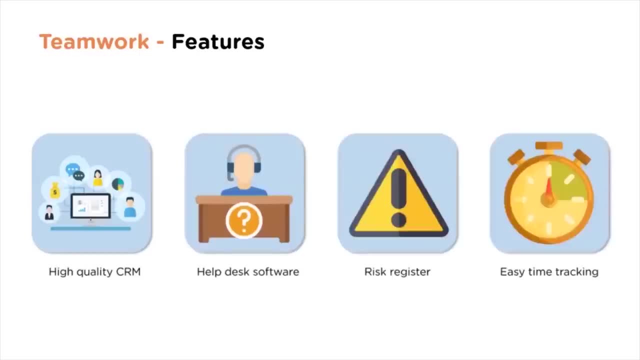 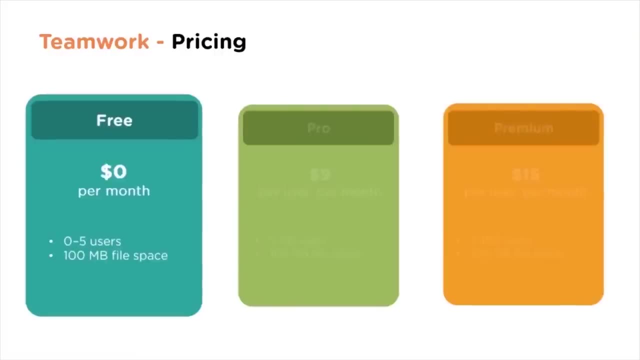 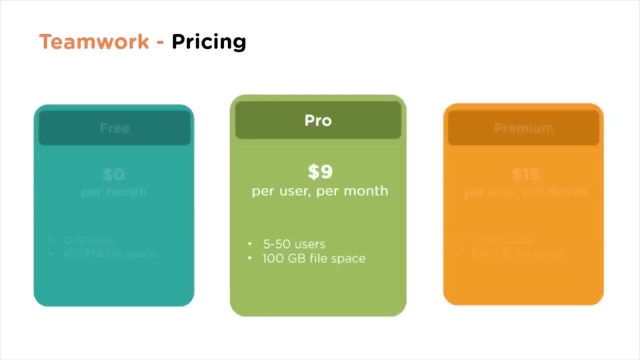 high quality CRM help desk software, risk register and easy time tracking. The pricing includes 0 to 5 users and 100 MB file space is provided free of cost, whereas pro version includes 5 to 50 users, 100 GB file spaces, which cost $9. 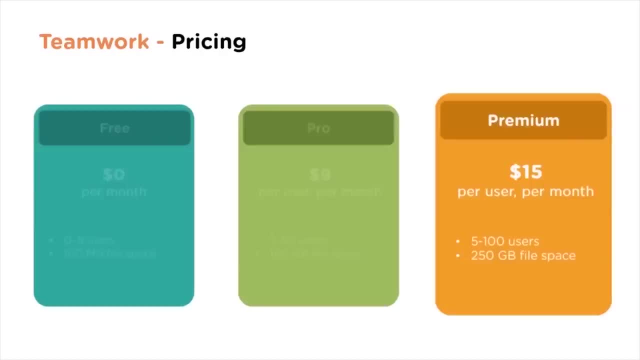 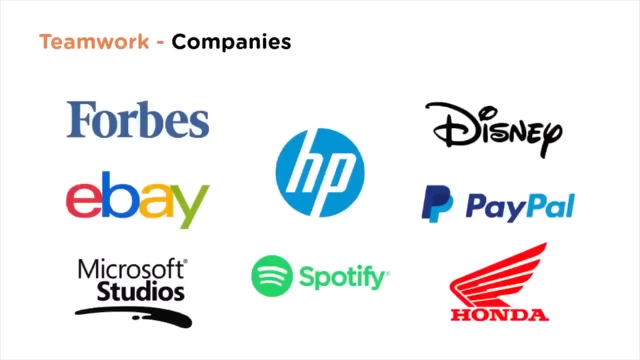 per user per month. Premium version costs around $15 per user per month, which includes 5 to 100 users and 250 GB file space. The organization who use Teamwork are Forbes, eBay, Microsoft Studios, HP, PayPal, Disney, Honda. 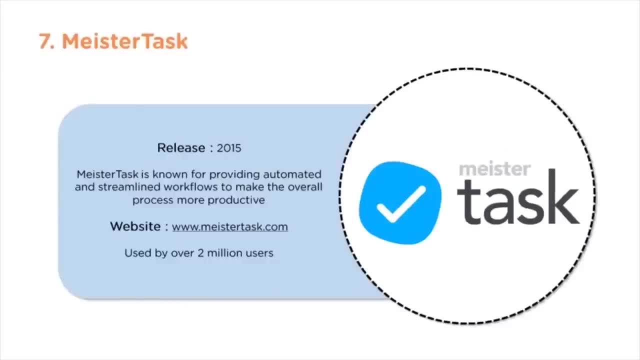 Now let us look at the tool MeisterTask. So this tool was released during year 2015 and it is known for providing automated and streamlined workflows to make the overall processes more productive. The website to access this is wwwmeistertaskcom. 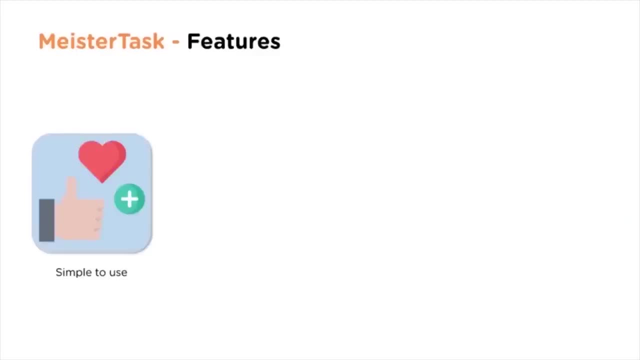 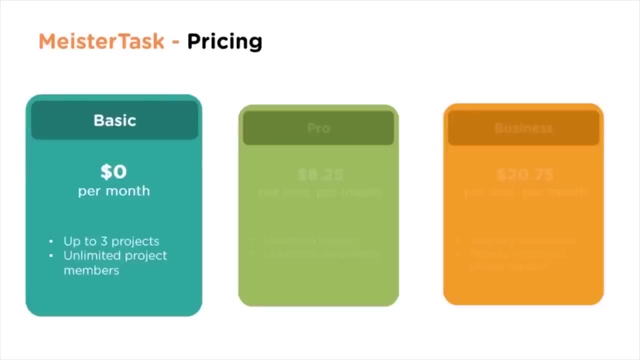 used by over 2 million users. The features of this tool includes: it is simple to use, seamless workflow, Gantt charts, flexible project boards. The pricing: it is $0 per month, up to 3 projects and unlimited project members. The pro version includes: 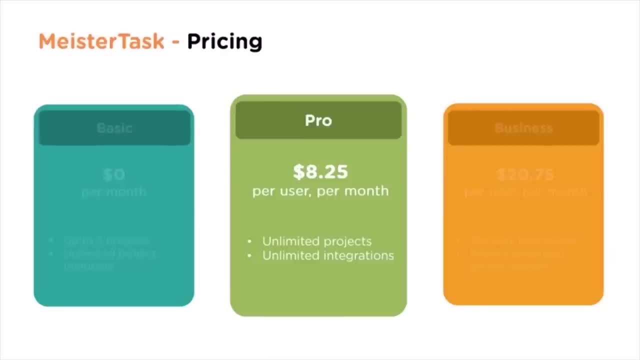 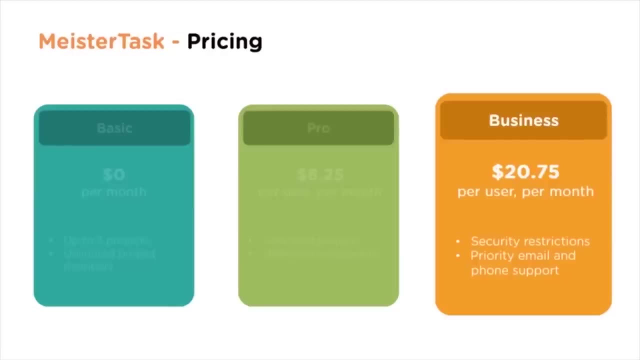 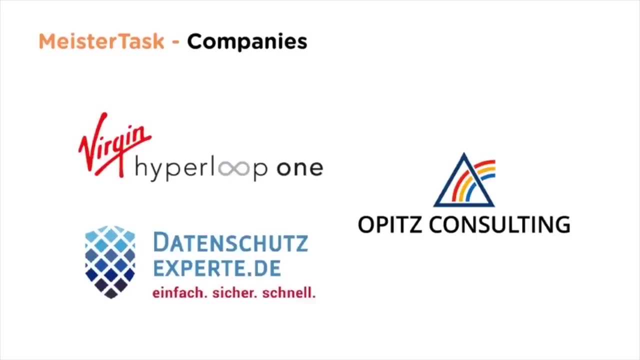 unlimited projects, unlimited integrations, which costs around $8.25 per user per month, whereas business costs $20.75 per user per month, which has security restrictions, priority email and phone support. The organization who use the tool are Virgin Optics Consulting and. 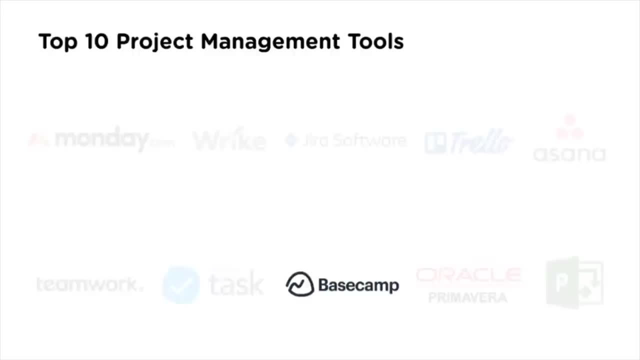 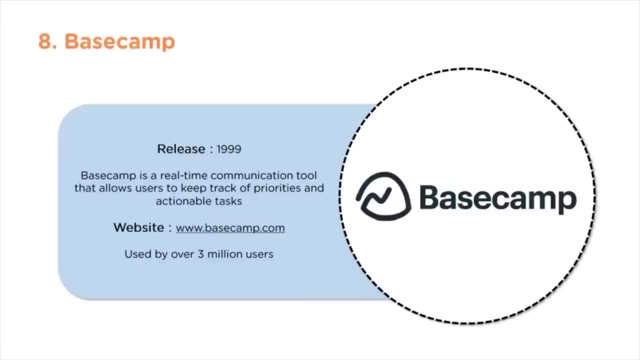 datansuchartsexpertde, etc. BaseCamp: The BaseCamp tool was released during the year 1999.. It is a real time communication tool that allow users to keep track of priorities and actionable tasks. The website to access this tool is wwwbasecampcom. 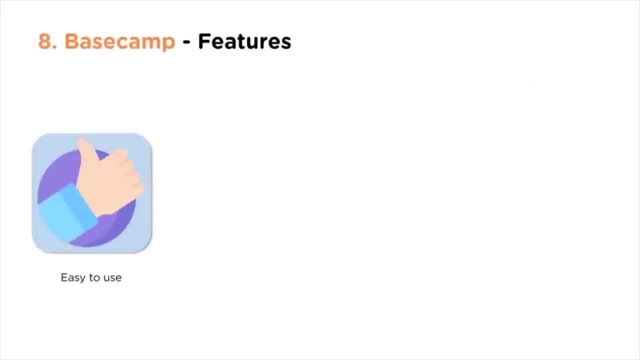 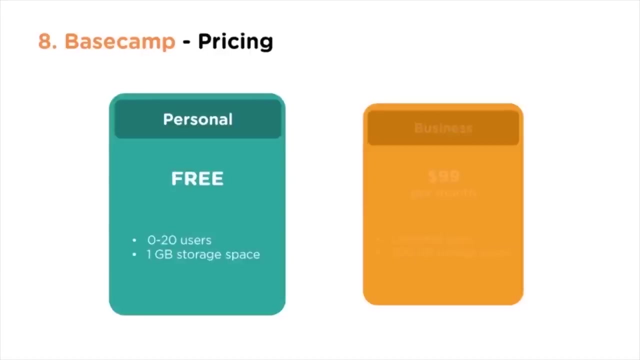 used by over 3 million users. The features of BaseCamp includes easy to use various third party integrations, daily backups and comprehensive project calendar. The personal version is free and 0 to 20 users and 1 GB storage space is provided. 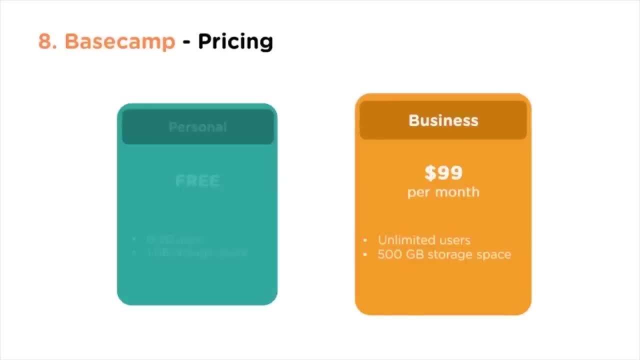 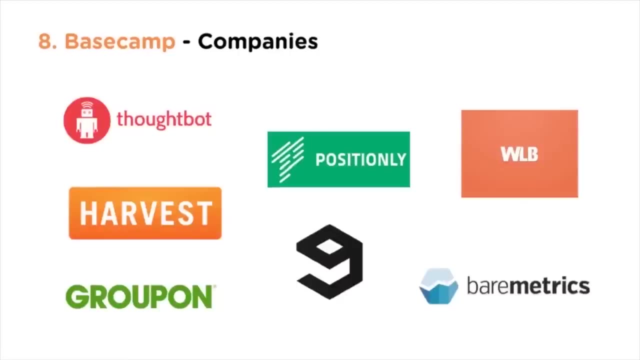 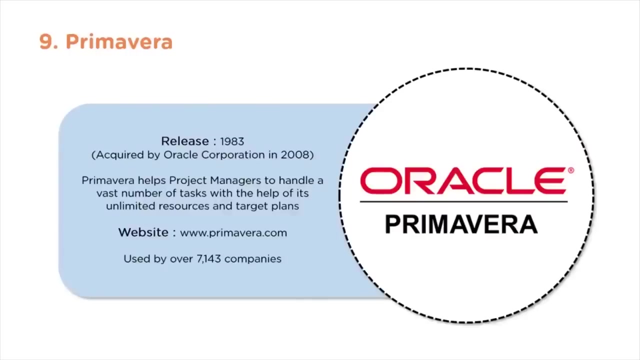 In business version it is $99 per month for unlimited users having 500 GB storage space. The companies who use BaseCamp is Thoughtpot, Harvest, WLB Groupon, etc. Oracle, Primavera. So this tool was released during the year 1983. 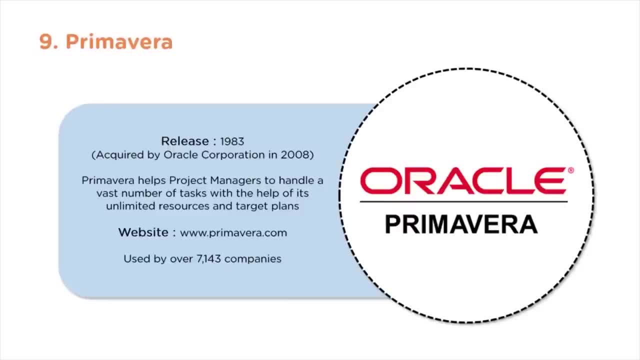 which is acquired by Oracle Corporation in the year 2008.. Primavera helps project manager to handle a vast number of tasks with the help of its unlimited resources and target plans. Website to access this tool is wwwprimaveracom, which is used by over 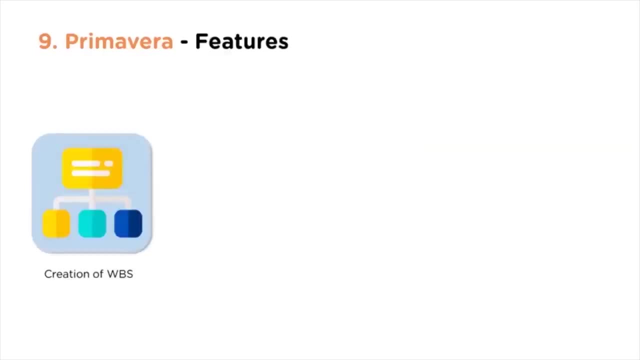 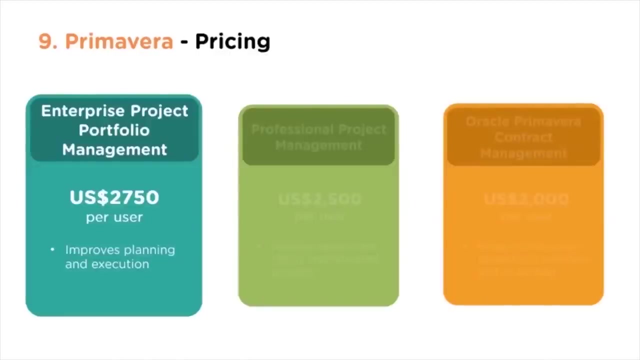 7143 companies. The features of Primavera includes creation of WBS, the work breakdown, structure issues and risk recording, supports large number of activities and easy collaboration with project users. The enterprise project portfolio management version costs around $2750 per user. 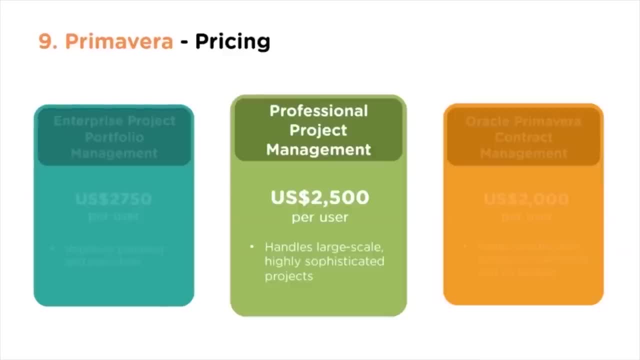 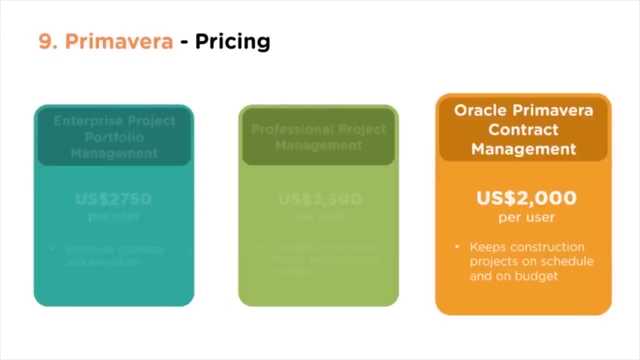 which improves planning and execution. Professional project management version is USD 2500 per user. handles large scale, highly sophisticated projects. So Oracle Primavera contract management version module costs around USD 2000 per user. keeps construction projects on schedule and on budget. 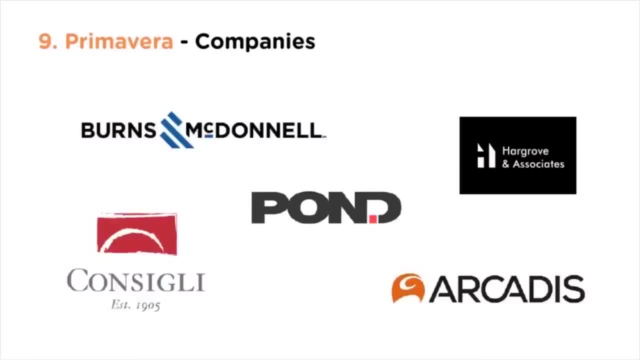 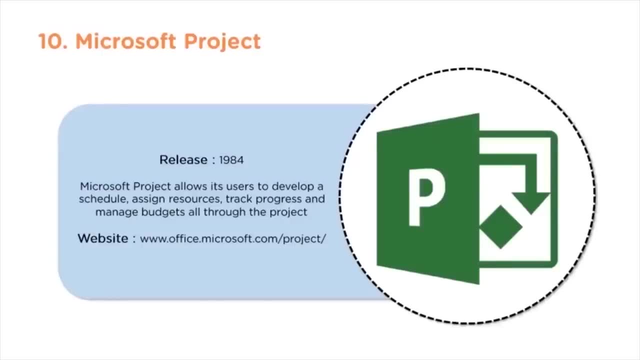 So the companies which use Primavera are Burns, McDonalds, Pond, Arcadis, etc. Microsoft Project. So Microsoft project management tool was used during the year 1984. So this tool allows users to develop a schedule, assign resources, track progress and manage budgets. 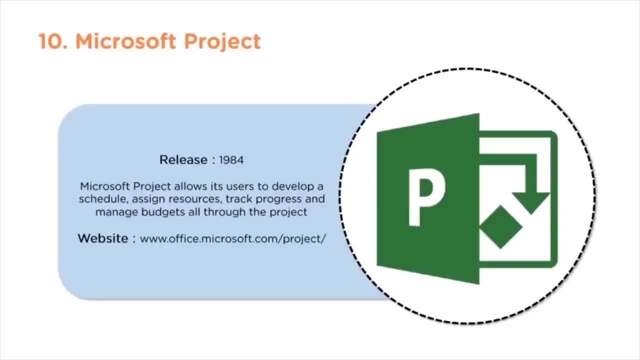 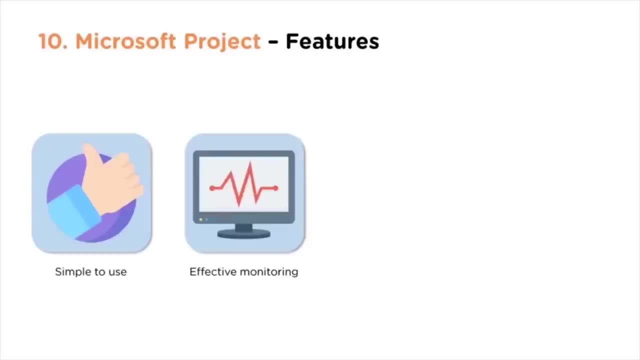 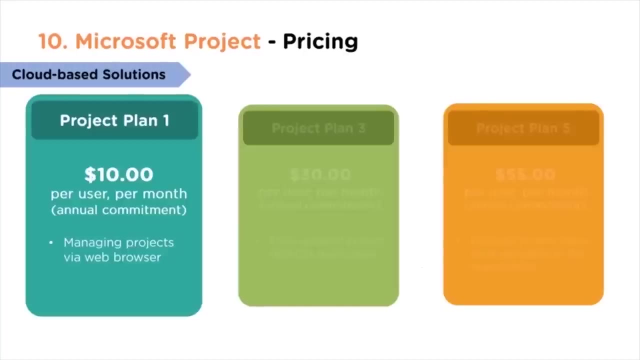 all through the project. The website to access this tool is wwwofficemicrosoftcom slash project. The features of Microsoft project includes simple to use, effective monitoring, easy communication, enhanced decision making. So this is a cloud based solution and the pricing is project plan 1. 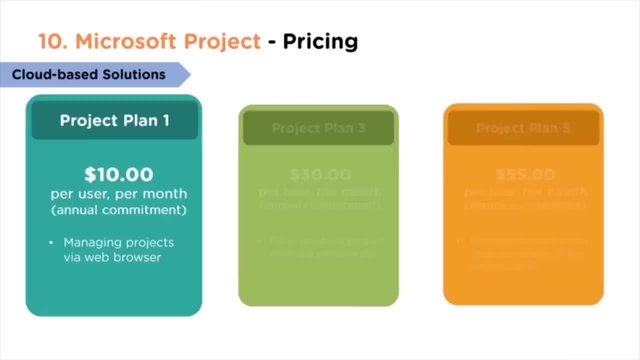 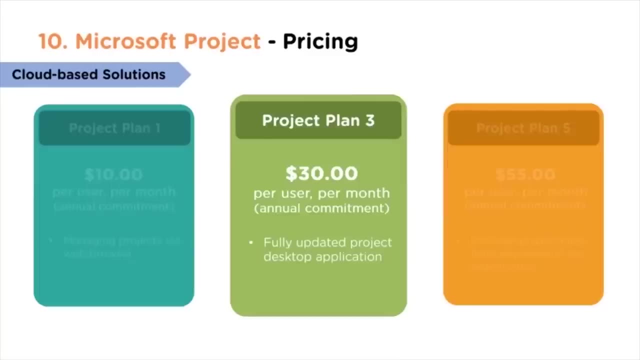 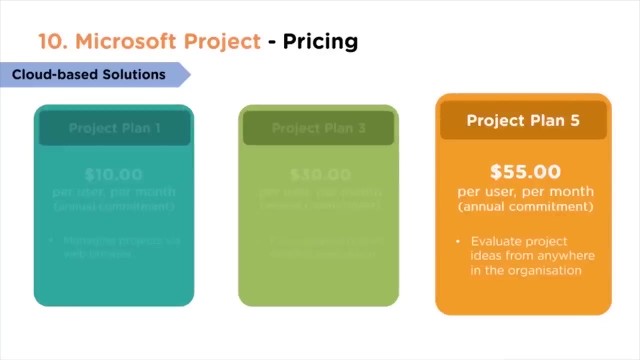 costs around $10 per user per month on an annual commitment. Managing projects via web browser is the feature- Project plan 3- which costs around $30 per user per month with annual commitment, which is fully updated project desktop application- Project plan 5- which costs 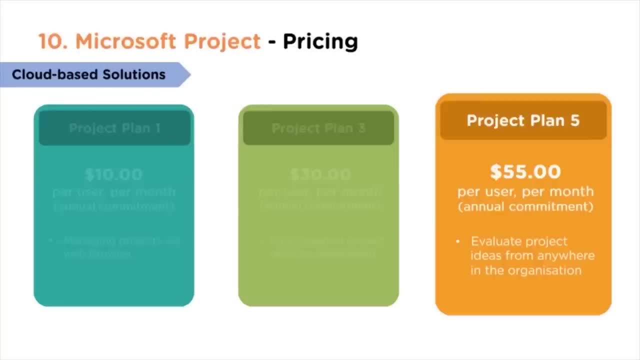 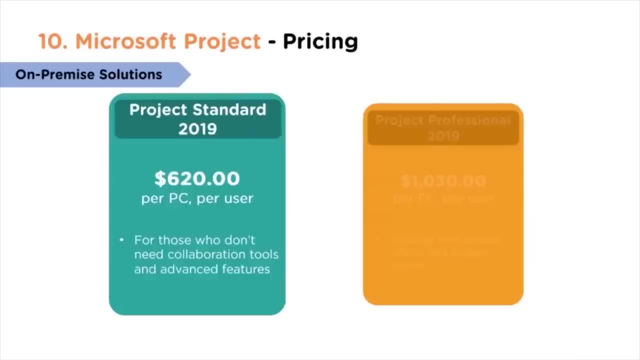 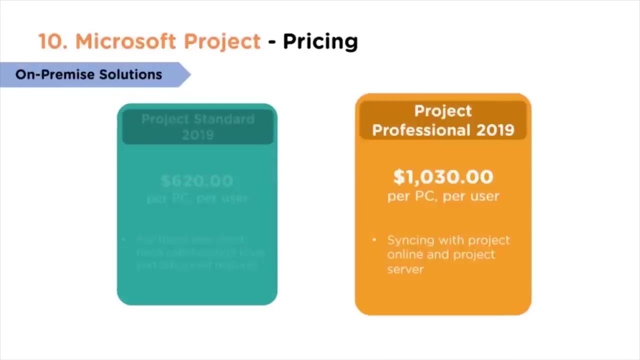 around $55 per user per month with annual commitment. Evaluating project ideas from anywhere in the organization is possible through this Project. standard 2019 version costs around $620 per pc per user for those who don't need collaboration tools and advanced features. 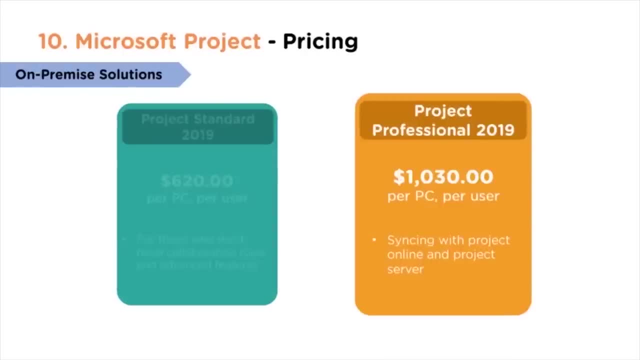 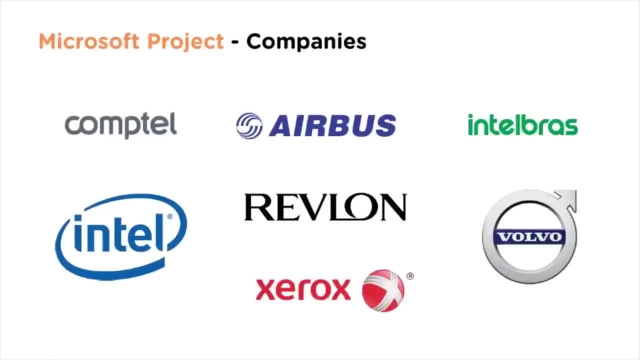 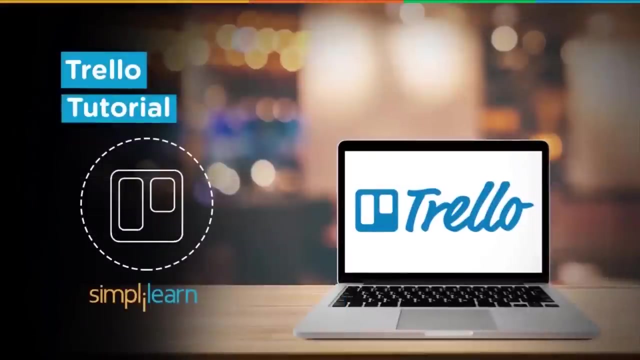 Project professional version 2019 costs around $1030 per pc per user syncing with project online and project server. The organization which uses Microsoft projects are Comptel, Airbus, Intel, Volvo, Xerox, etc. Hey guys, welcome to this Trello tutorial by 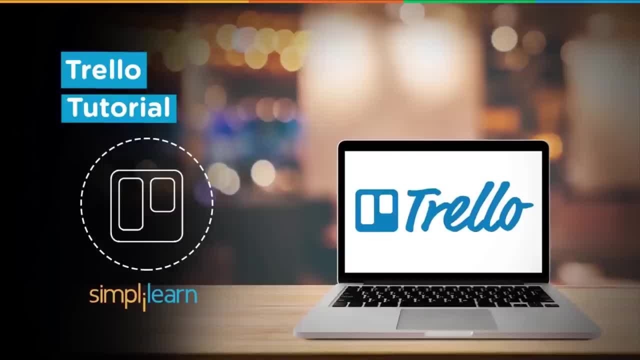 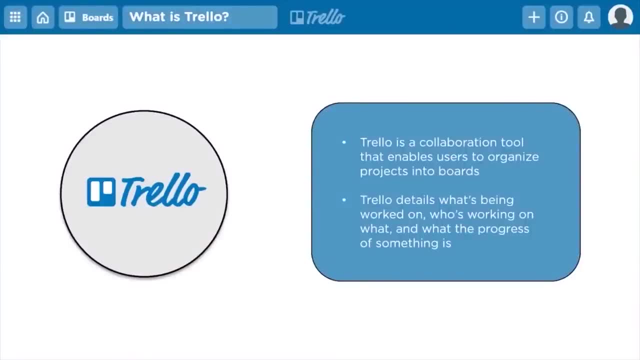 Prelearn. So, without further ado, let's get started with what exactly is Trello? So Trello is a simple and easy to use collaboration tool that can enable you to organize projects and everything related to it into boards. With Trello, you can find all kinds. 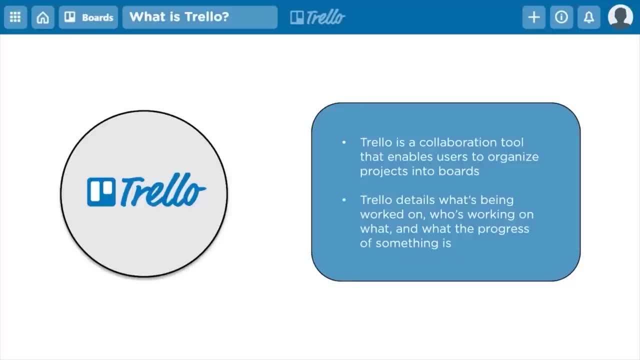 of information like what's being worked on, who's working on what and what progress the project is making. Now we'll learn about that in a little bit. while we're talking about the Trello demo, Now let's talk about the advantages of Trello. 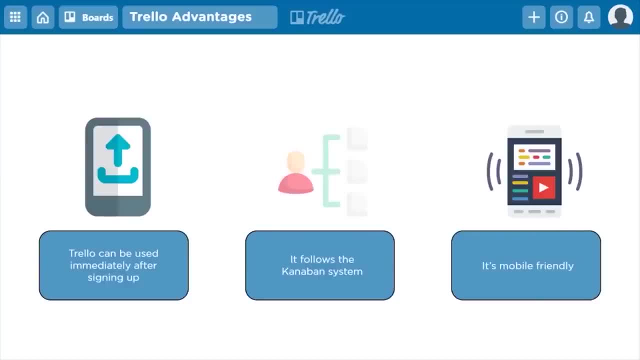 Now, first off, Trello can be used immediately after signing up. So Trello offers you a free sign up, after which you get access to almost all of Trello's features. Now it does have a premium service, but most of Trello's important features are available. 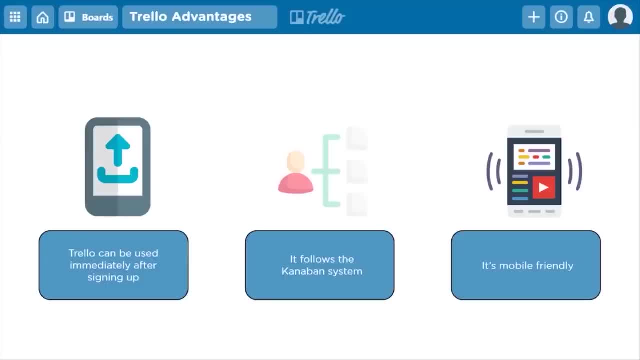 in the free account. Secondly, it follows the Kanban system. So the Kanban system is a popular methodology that can be used to achieve lean. So with Trello you can also achieve lean. Now Trello also has a very popular mobile application, which 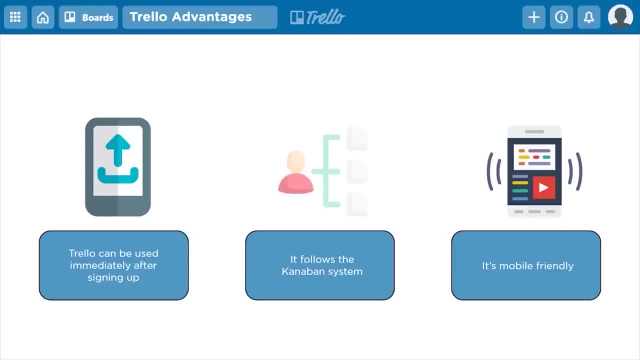 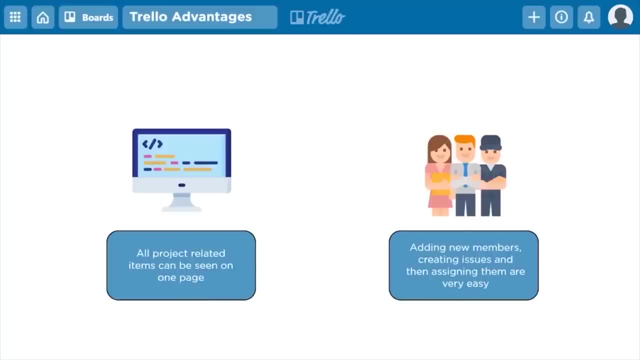 also has the same features as the interface that you see on the desktop. It's very user friendly. Now, the fourth advantage is that all project related items can be seen on one page, Which means everything you need about the project is available in one place. 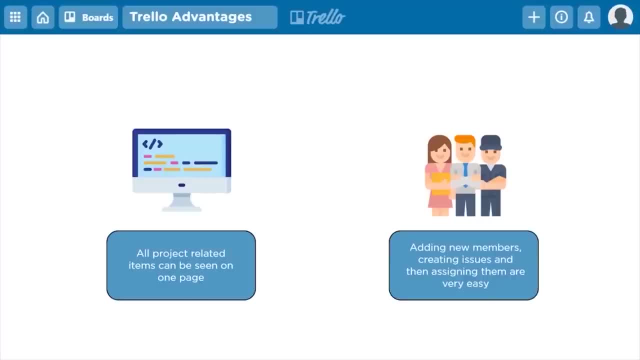 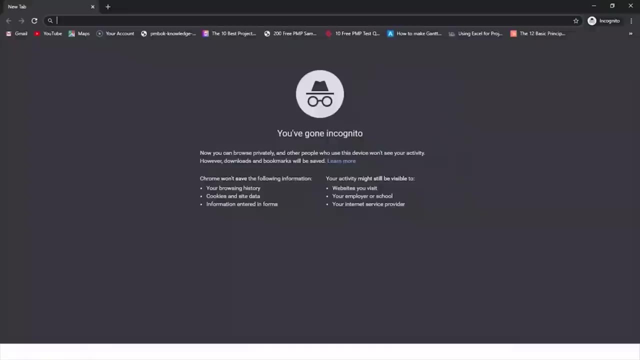 Next, adding new members, creating issues and assigning them are very easy with the help of Trello. Now that we had a look at all the advantages that are provided by Trello, let's have a look at a live demo. So first off, let's go to Trellocom. 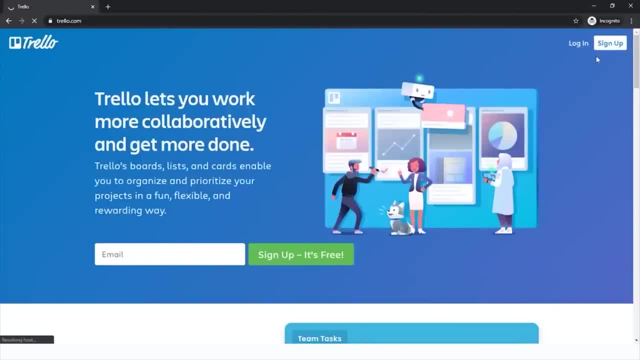 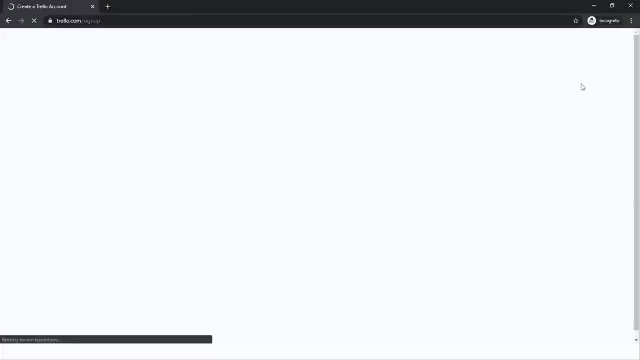 So here you can see two options: to login or sign up. So first of all, if you've never used the website before, go to sign up. So here you can enter your email, or you can go through Google or Hotmail or Outlook. So it's very simple. 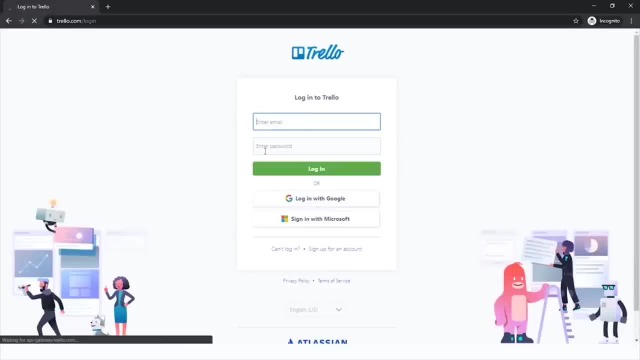 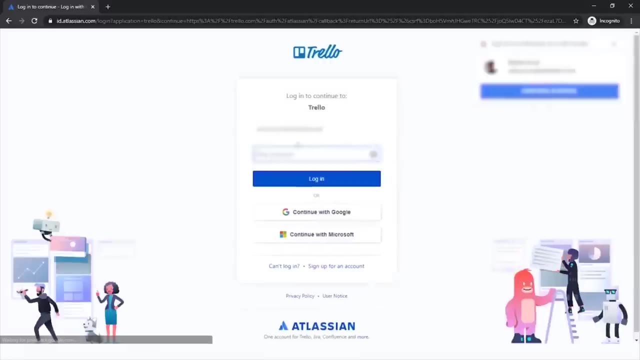 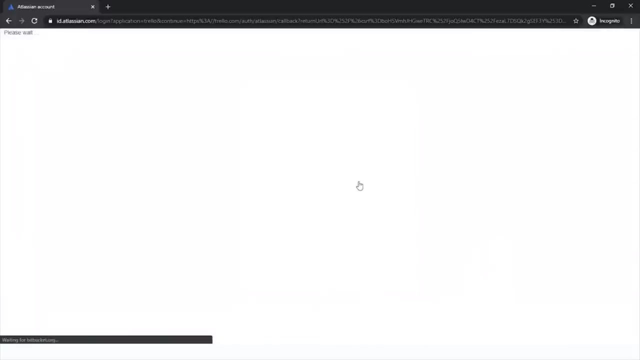 I already have an account, so I'll just login. So I'm just going to login. So if you're using Trello for the first time, this is what it would look like. So here you have personal boards, templates, home and so on. 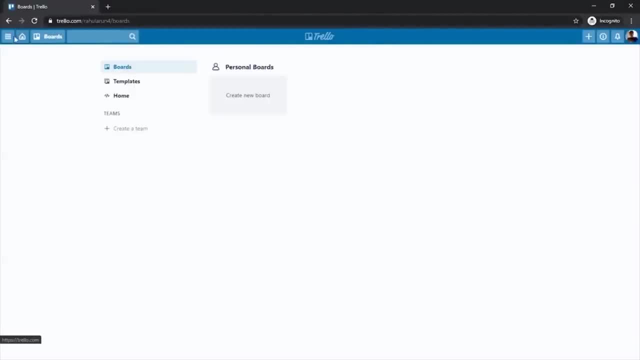 So let's go one by one. Firstly, the most important thing that you need to know about is boards, Which is right here. So let's assume you're using this for a team, Which means that you need people to share your content, So let's assume you're using this. 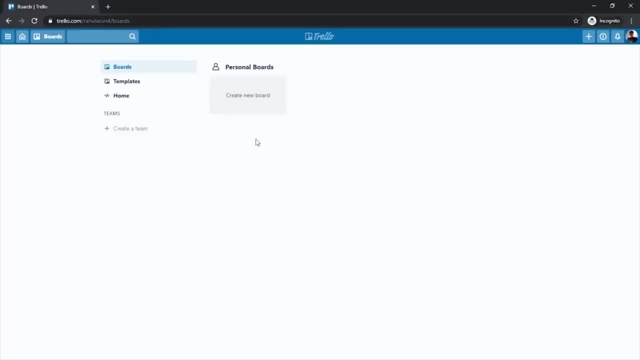 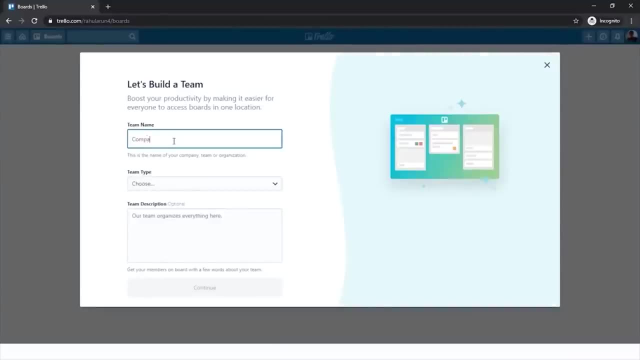 for a team, Which means that you need people to share the board along with. So first of all, let's create a team. So here I'm just going to name the company called CompanyCo. Say, we do EngineeringIT, Let's write a. 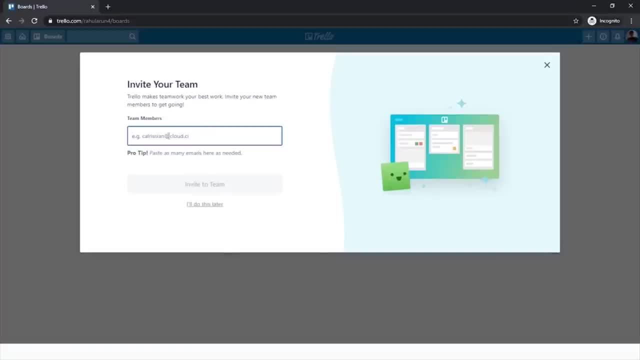 brief team description And continue. So here, say, I have four members, So I have Bob. I'm adding them here. Depending on what your team is like, you can add those team members. So this is important so that you can connect with them while you're on the board. 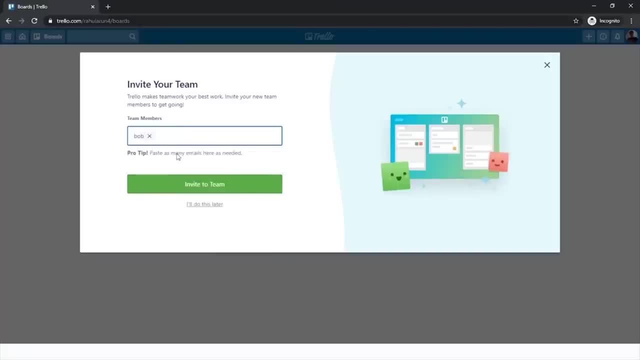 So this is companycom, so we'll just add them. So the team members that you're going to invite will get an invite email very soon, As soon as you're done by clicking the invite to team button. We'll also add Bill, Who also works at my company. 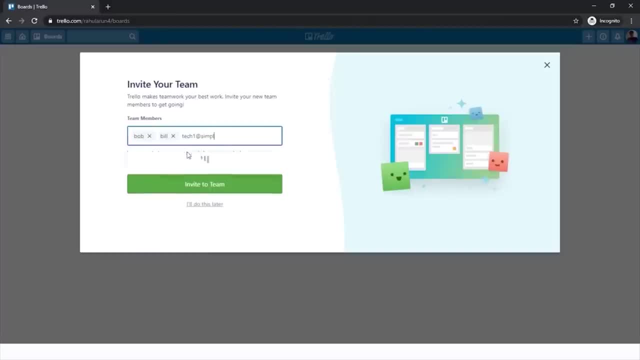 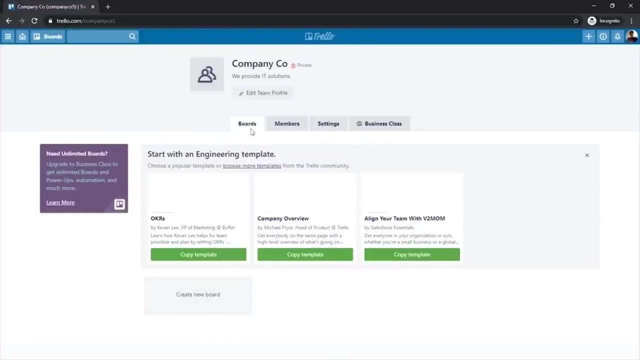 There's Technician1.. Who works at companycom. There's Technician1. Who works at companycom. We'll add anybody who's required later. So invite to team And there you go. There's some details here about the team and all that. 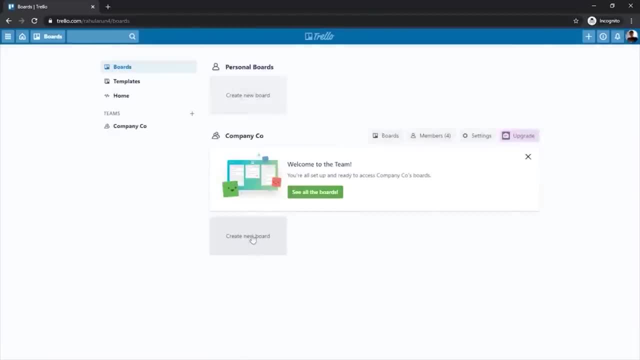 Let's go back to home And now let's create a new board under CompanyCo. So the difference here is that for personal boards is that, like the name says, it's personal. You can also add the team if you want later on, But here you have the option. 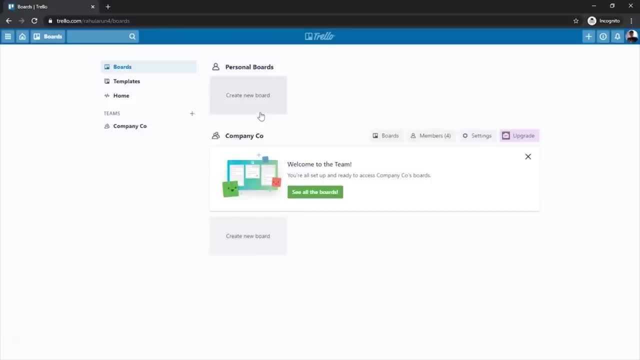 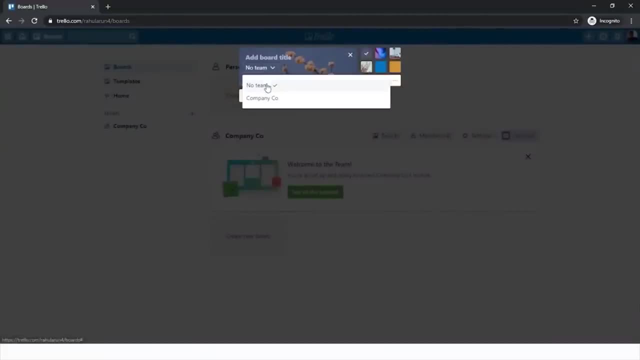 for creating a team board. So I'll show you how you can create a team board from personal board. So you've got create board Here you can show. as this is by default selected as no team because it's under personal, Change it to company. 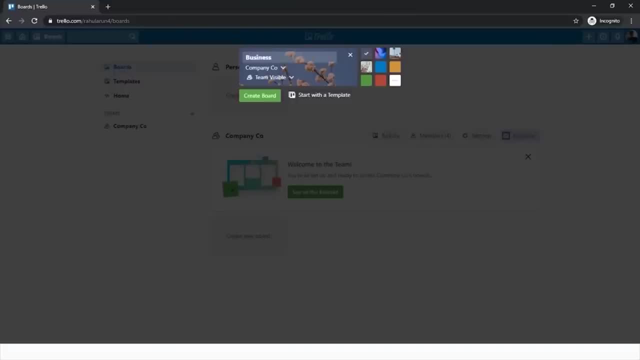 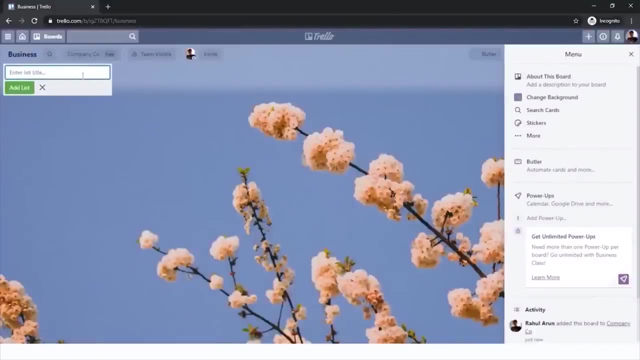 And you can write business- Anything else like that- And then you create a board And there you go, The board has been set up. So now, first things first, It's that you can make this team visible, Which is either only board members. 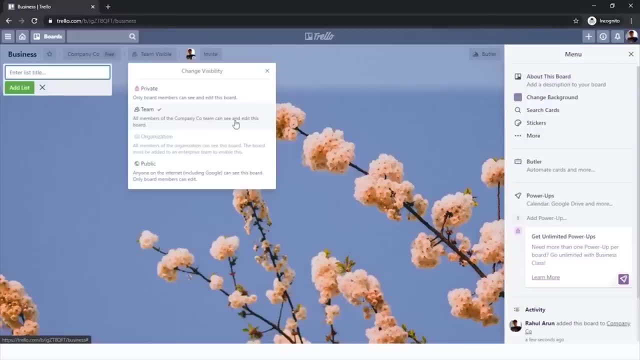 can see it or, since it's a small team, the entire team can see it. So it's up to you how you want it. There's the public option, which everyone can see, which I don't think is necessary, But if you feel like it, you can do that too. 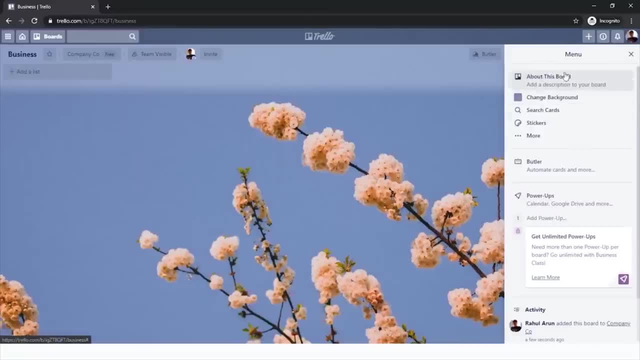 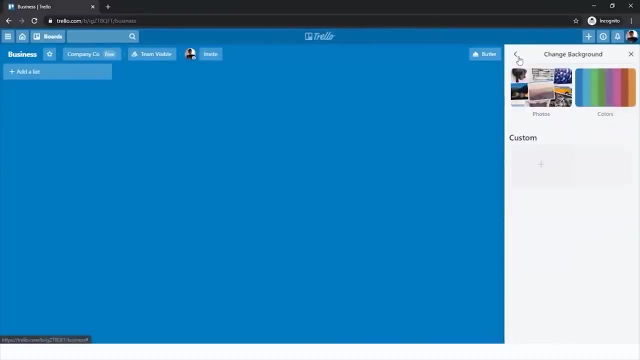 First of all, you can even write description of the board. which is what you want to achieve with this board. For example, this is business or sales or something like that. You can change the background into something more colorful or less colorful, like this, And then: 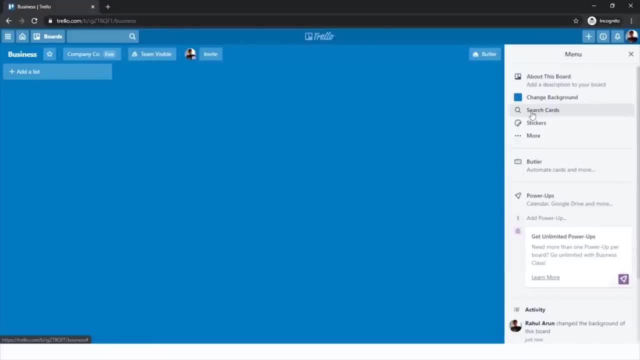 there's search cards, which we haven't added anything so far, so there's nothing to search. There's stickers, which again is, I feel, unnecessary at the moment. You can also see something called Butler. So, based on your usage or how you're using Trello, 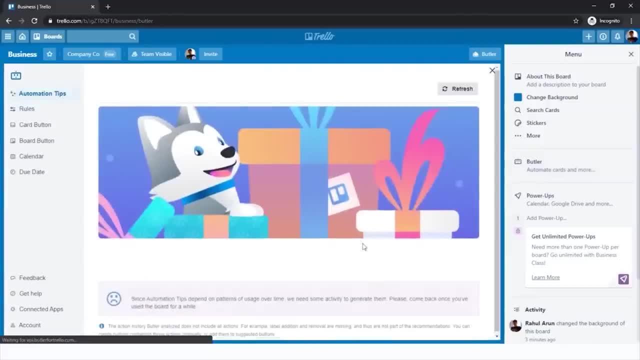 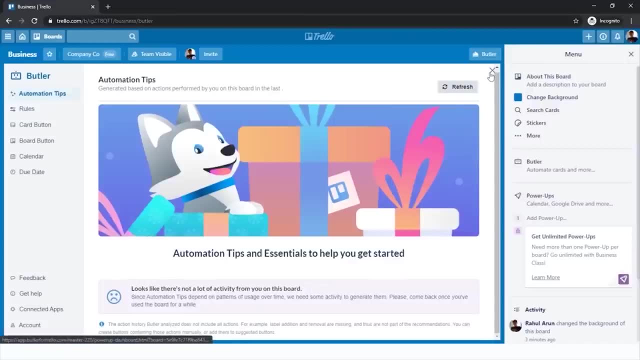 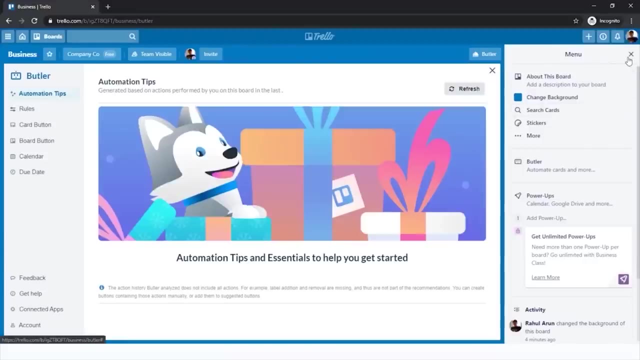 Butler can provide you suggestions like what you can add here. Like you can see here, The tips haven't been added so far because we haven't used Trello so far. So, based on your usage, it'll give you suggestions. Now let's go back. 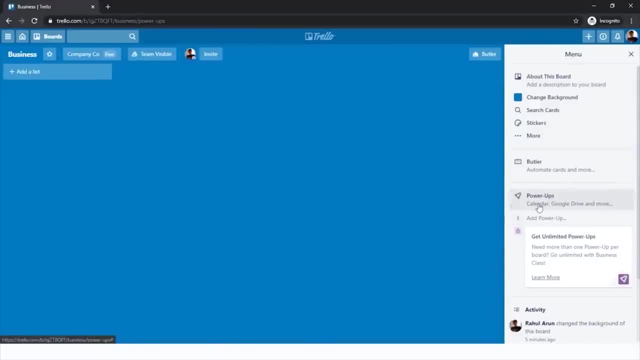 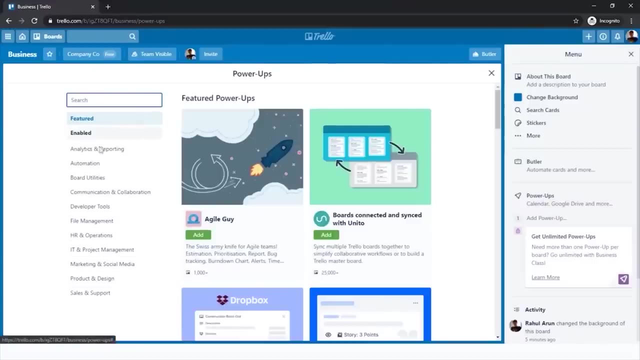 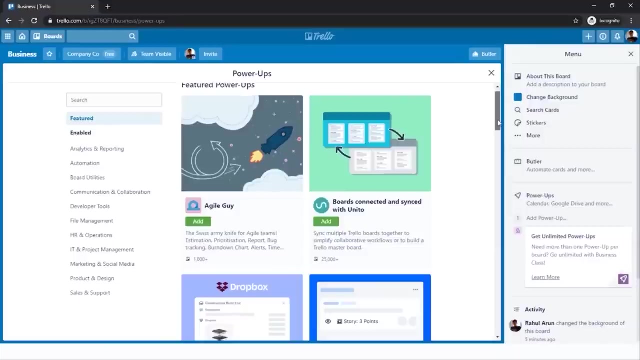 So here you see powerups. So powerups are basically additional features that you can add to your board. So there are features that are connected to a number of different features. There's analytics, automation, utilities, tools and so on. So as a free user, you get access. 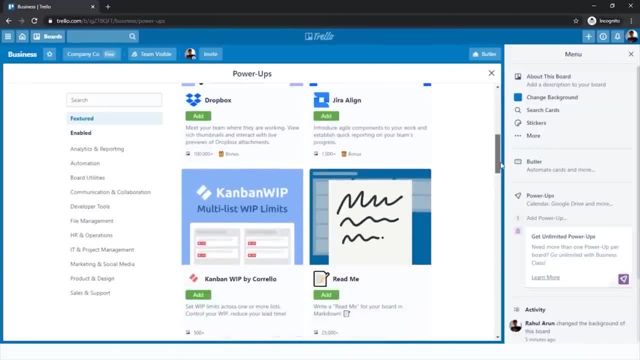 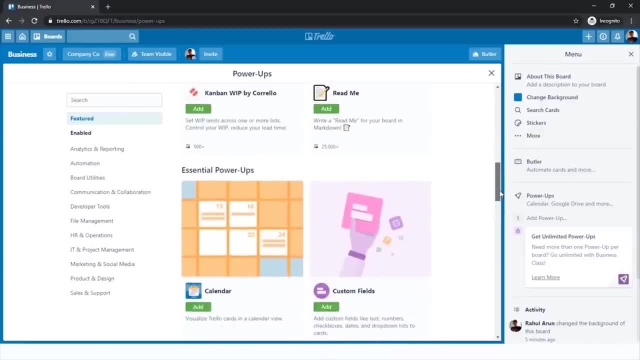 to one powerup, but still we don't have to use it so far because we don't have anything on our board. but, based on your requirement, you can go through these powerups and decide on one of them. So now let's get back to business. 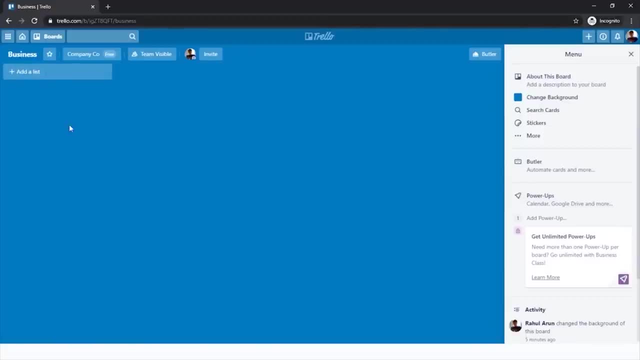 or our board. So first you can see: add a list. So this basically refers to the different processes that you want to follow in this board. So first of all we'll add a list title I'm going to add to do. That's the first. 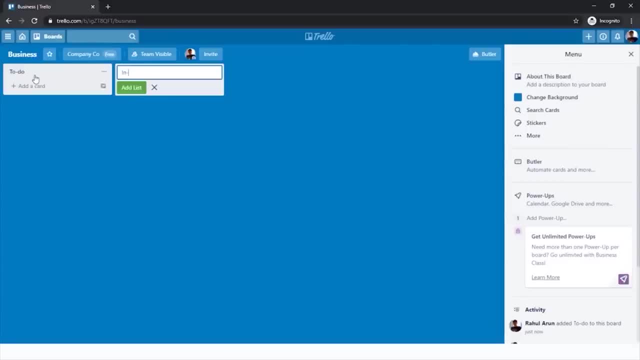 list, Then there's in progress, On hold And completed. So here we have four lists which represent the processes in this business. So if you want, you can even add another list, depending on your requirement. So in these lists there are things called cards. 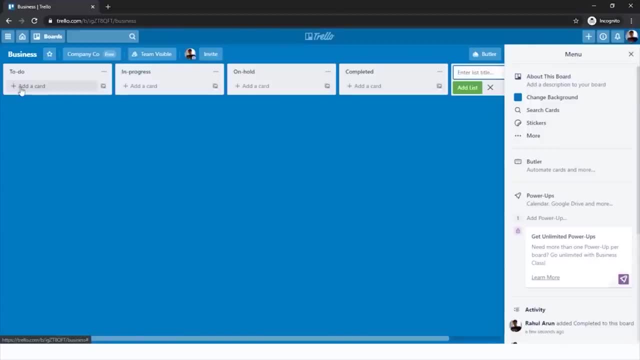 So which are like subtopics. So, first of all, let's add a very simple title. For example, deliver product, company A. This is again very simple. Deliver product to company B, Like this, So on and so forth, if you want it, So here. 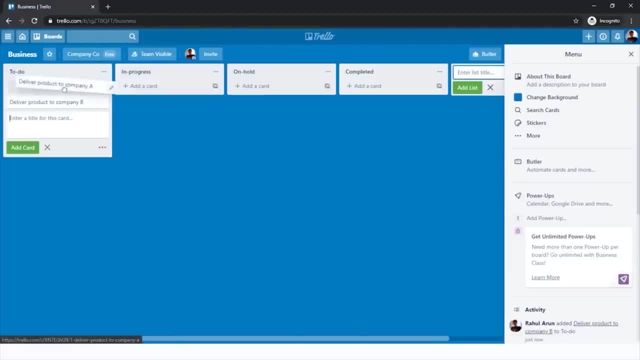 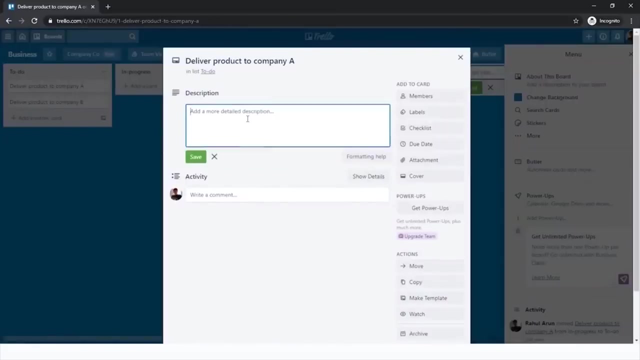 this is a card, So this card can be moved from each stage to another as it progresses. So this isn't the to do stage, since we've not started with anything. So once you click on a card, so this popup shows up. So here you can add a description. 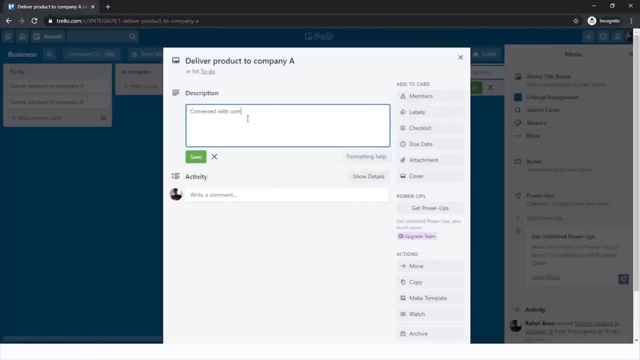 like conversed with company A Ready to go, Just some details that you want to add. You save Now one thing you can see add to card. So there are number of different things you can add to this card. So, members Now. 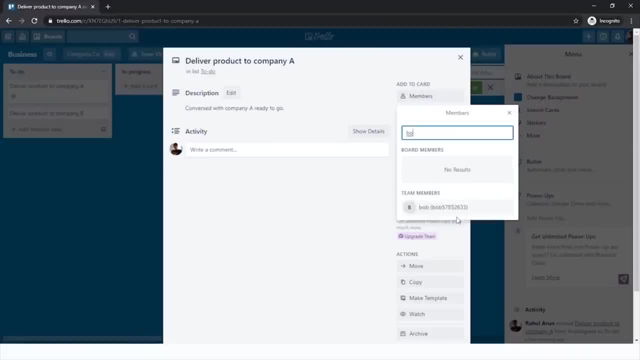 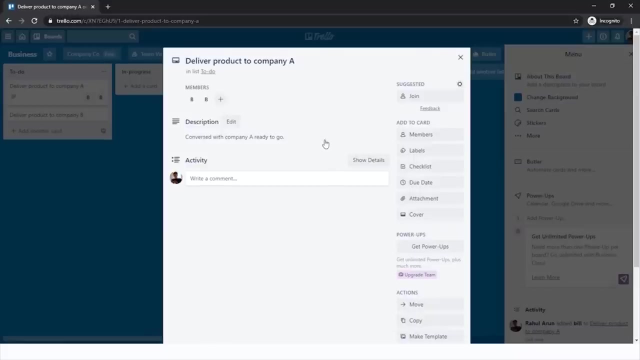 I have four team members. I can add Bob here. I want Bob in on this. I want Bob to see the activity as it happens. I want Bill to also see as things proceed Right. So the Bob and Bill are in on this right now. 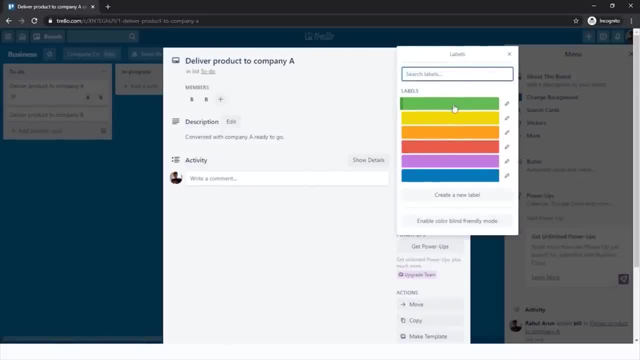 Next, you have labels. So, depending on what you want to use this for- For example, I want to use this to represent that it's important or immediate- Put it as red Save So I can select this label to indicate that this is now very important. So, depending on, 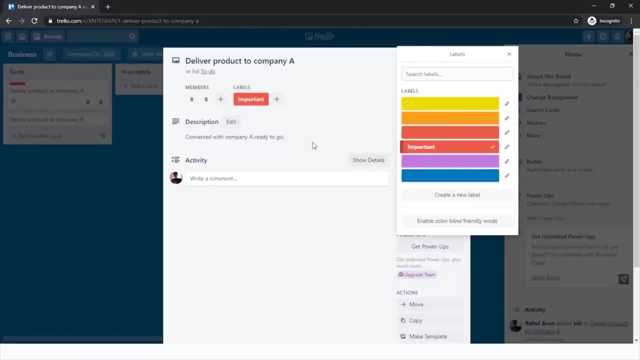 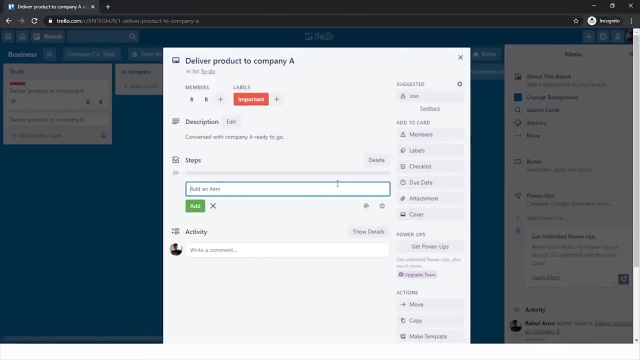 your company's style or depending on your requirements, you can add the labels. Then you have a checklist, So different steps can be focused on with this checklist. For example, I am just going to write steps. So we are delivering a product, for example. So let's just 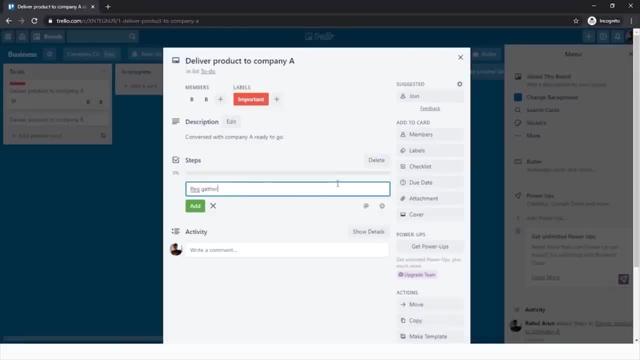 use steps. I am just going to write the software life cycle steps: Analysis, Design, Implementation, Testing, Employment And maintenance. So yeah, we have all the steps. So one thing is that once each of these steps are done, you tick it. 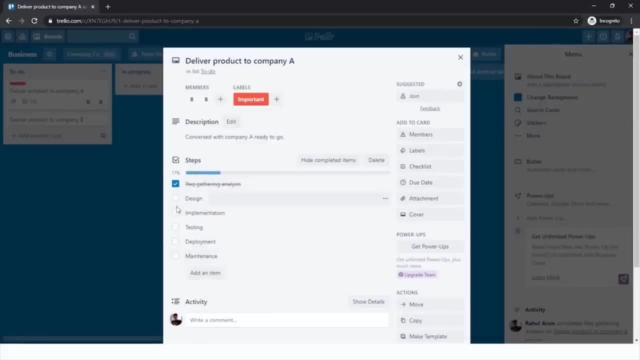 So a percentage increases. So until you are done with 100%, you can just keep ticking. Finally it will show 100% and you are done. So another thing is a due date, So this is basically by when you want it completed. 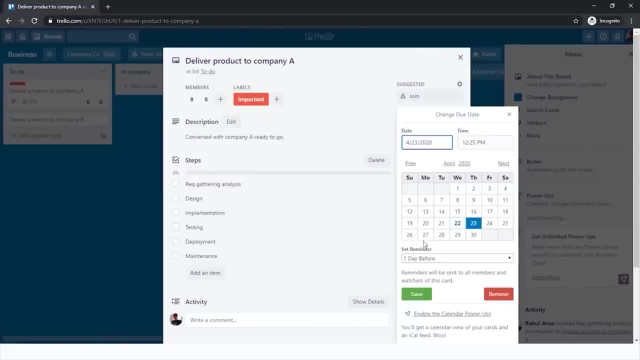 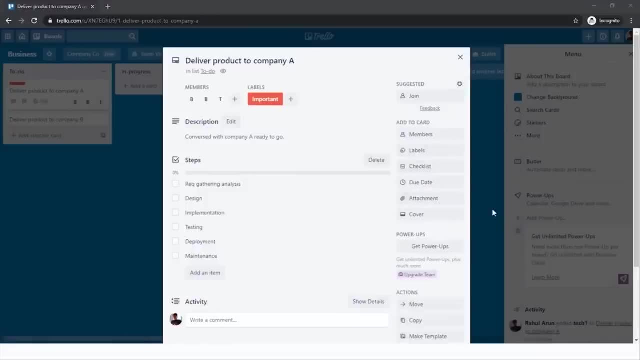 So this is basically a reminder that we need to complete it before a particular date is done. So I am not adding a due date as of now, but that's up to you. Next, you have something called attachment. So say, for example, all your requirements have been. 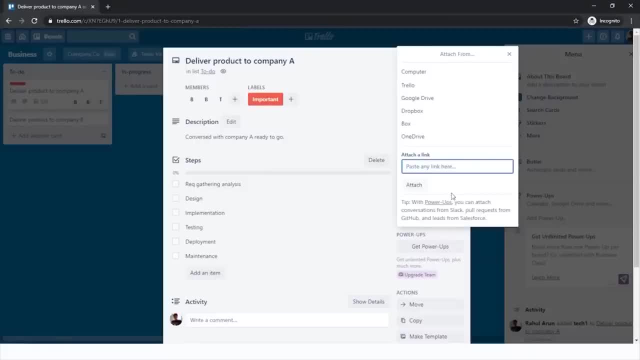 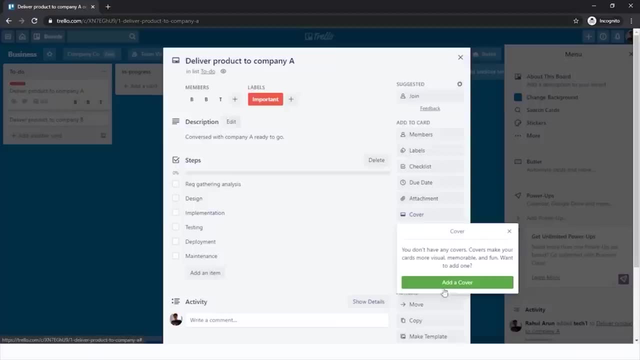 gathered into one PDF. So where all the requirements that are required by the company are shown in that PDF, You can attach it here so that everyone has access to it. Then a cover can also be added to your card, which is just basically beautifying it. 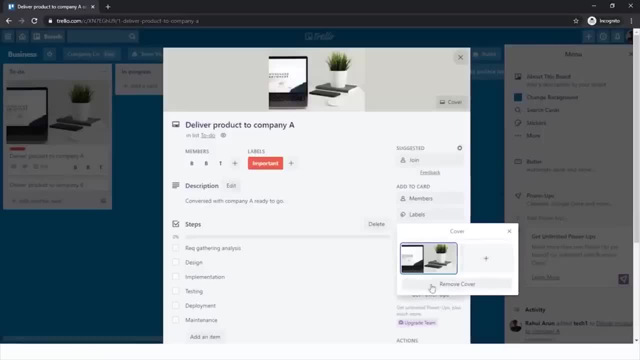 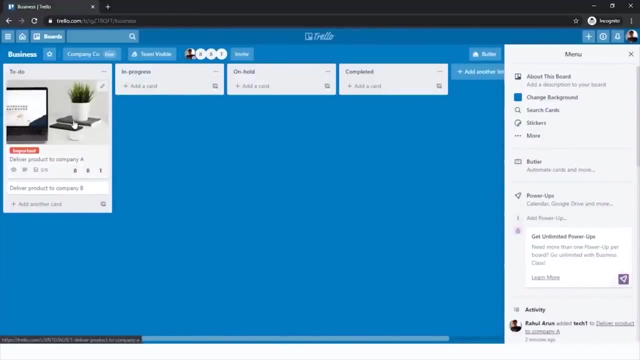 So we can find one. So for example, this: And there you go. There is a pretty good looking cover here. Now we have all the information, So let's get started. So to officially mark the beginning of the project, we will just go and put this to in progress. 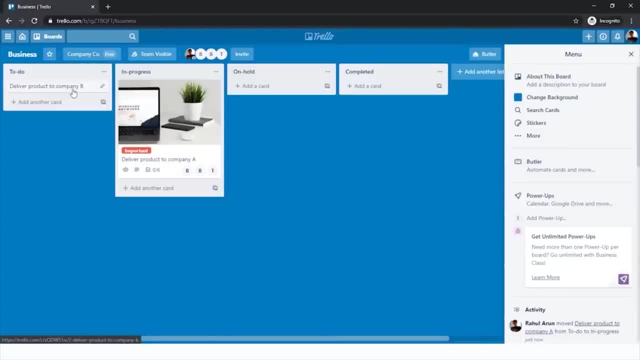 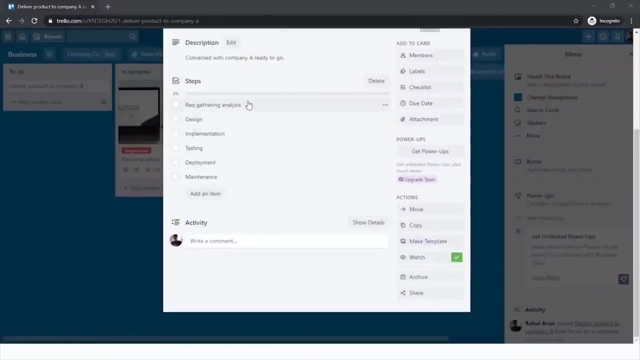 So at the same time, you can do the same thing with this card as well, about company B. So let's just focus on company A now. So say the steps have already started. Requirement gathering is done, Designing is done, Implementation is also done. 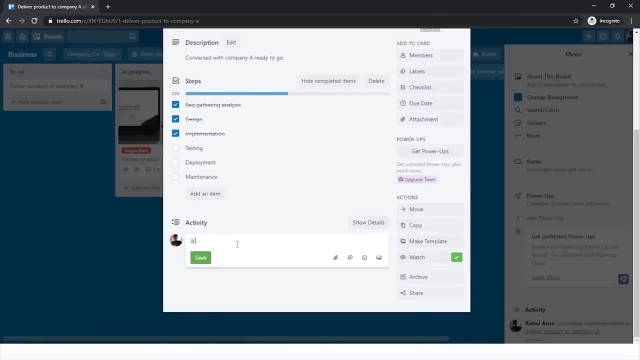 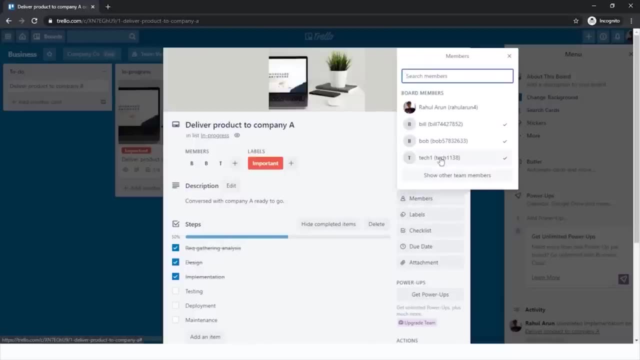 So, depending on the person, you know the technician, So the technician could respond that you know we have already started. So before that, we need to add the technician. He is already on this, but if you had to add him, you search for members And you have board members, who is already in the. 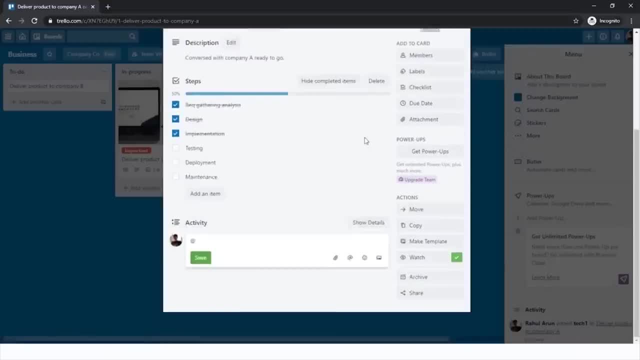 board. You can add the technician. Now. you can also, you know, add activity details like technician 1.. How is it going? How is the process going Now? he could respond here with its name. So each time one of us you know adds. 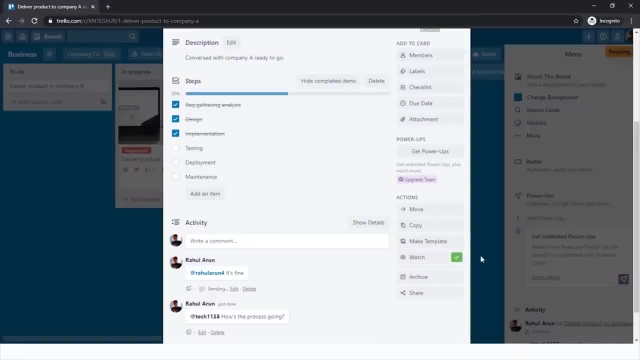 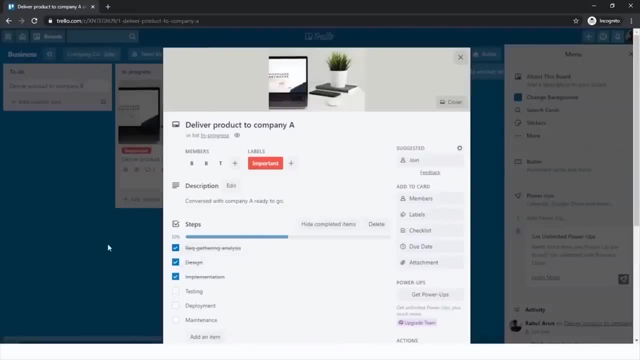 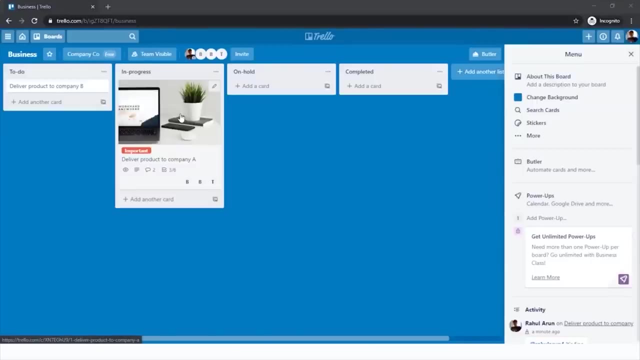 the other or says something to the other. they get notifications so that you know they get to respond as well. They get to know what's happening Now. Now say, for example, the technician is not able to complete the project or complete his work, So it's put on. 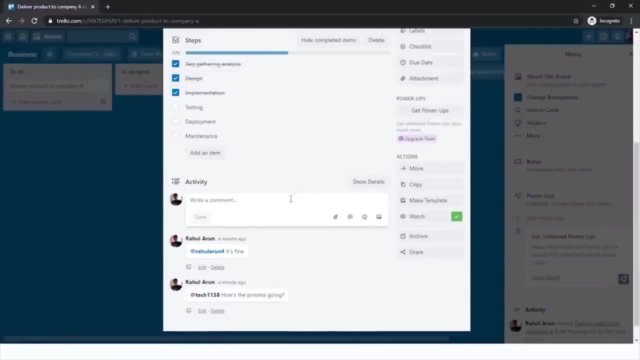 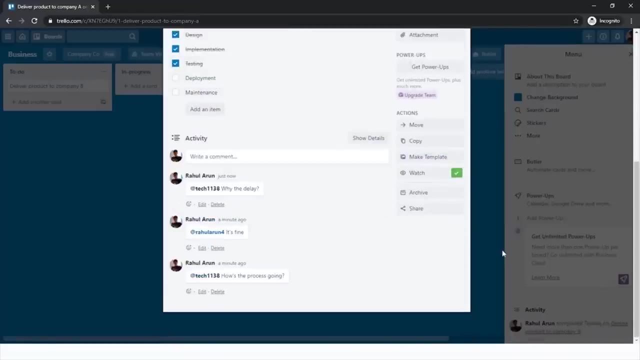 hold. So here I could say: so testing isn't done. So you can say test by the delay or what's going on And he would give in a proper response. And once he is ready he can finish the testing and put it back to in progress. 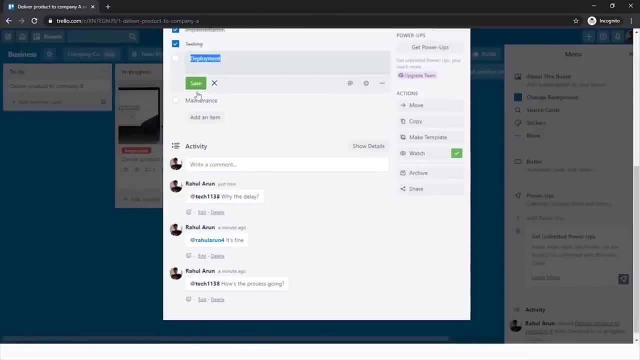 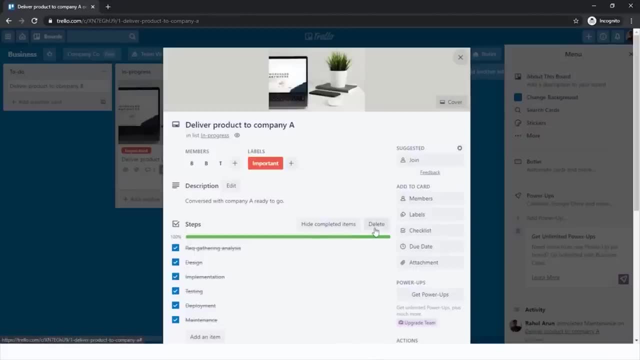 And eventually all of it is done: Deployment and maintenance. So here you have an option to hide complete items. That's up to you. You can also delete them if you feel like it. You can close this And then, after everything is done, 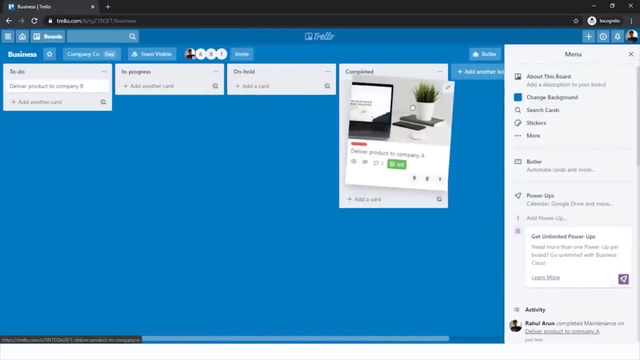 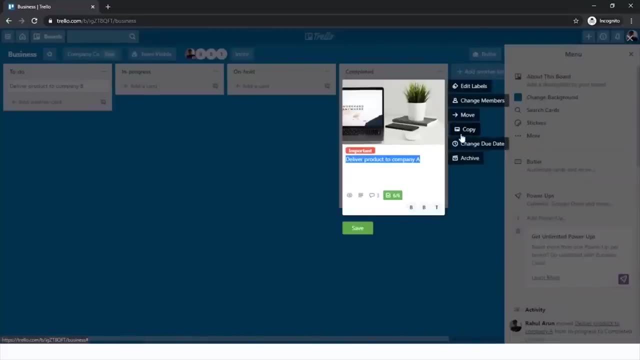 and you feel that everything of the process is done, You can put it on completed. So if this is a recurring process, you can, you know, make a copy of this, which you can find by doing this copy, Or you could just put this on archive. 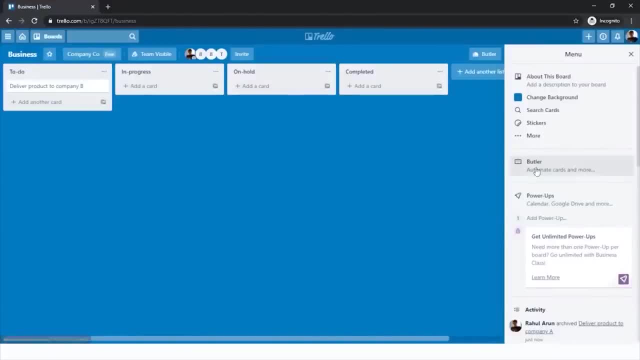 Indicating that it's done. You can even get it back by just going to more archived items, and then there you have it. You can send it back to board. That's up to you, And there you go. That's most of everything you need to know. 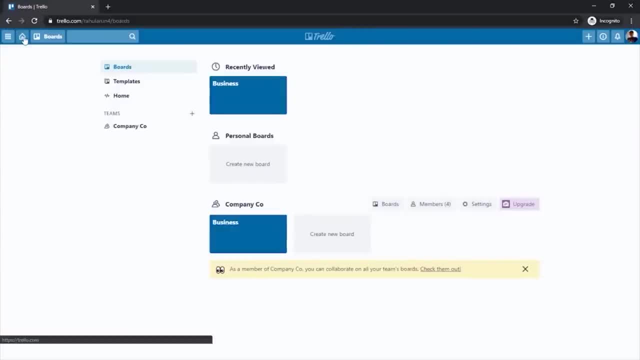 about Trello One. another thing is that right now, you can only add 10 boards on this feed as of now, Because you are using a free membership. Also, depending on the intensity or the difficulty of the board, you can also have different boards for different projects. 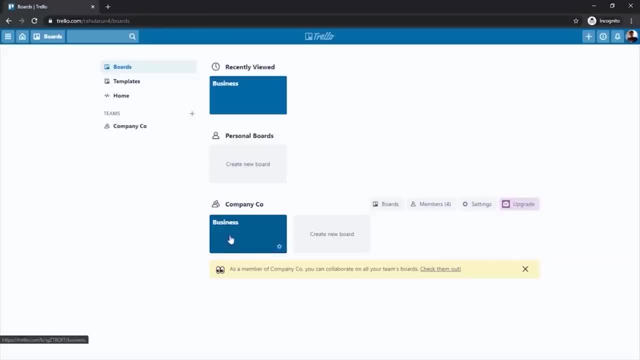 I've just used one for multiple projects, but it's entirely possible for you to have one board per project. You can also- you know- favorite this indicating that this is a very important one that you need to focus on every day. So this is where you get. 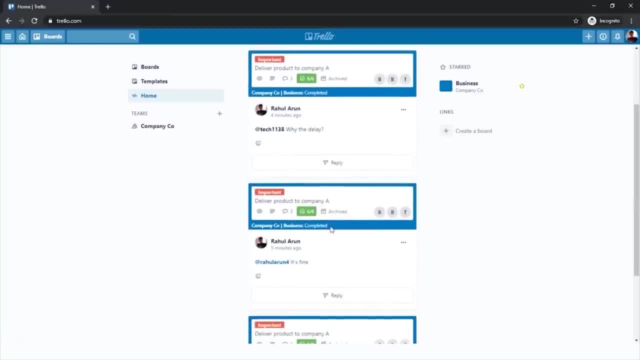 all the notifications that X has changed. There you go: All kinds of responses. everything that you need is available on this home screen, Which is basically like a home feed. You can also find templates depending on your requirement, So you can choose a template from a wide 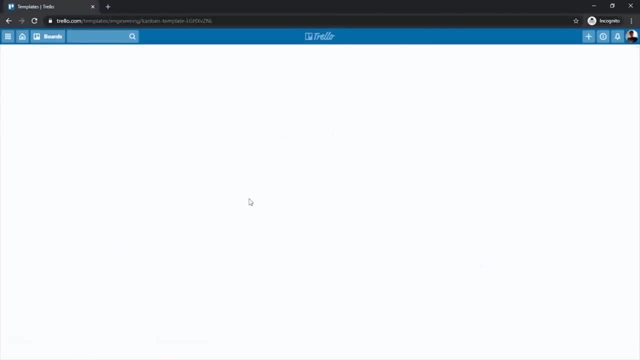 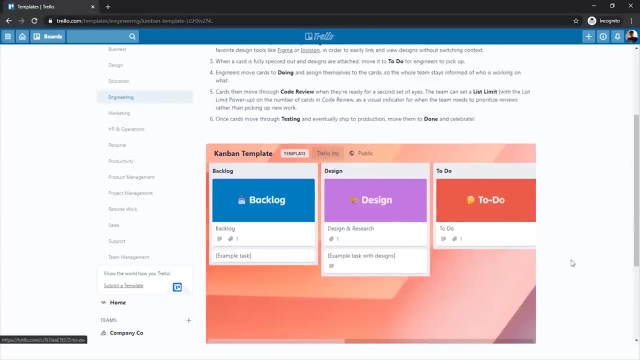 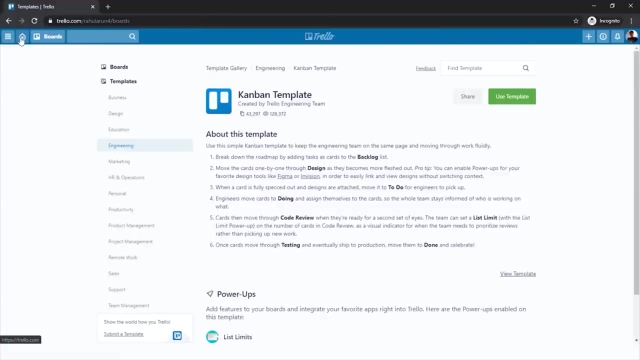 variety of options. So I'm just going to show you the Camden template. So here you have details about the template, Example of what the template looks like, and so on, And there you go. That's everything you need to know about Trello. 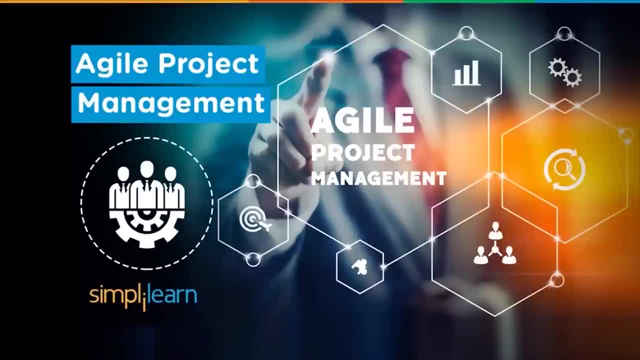 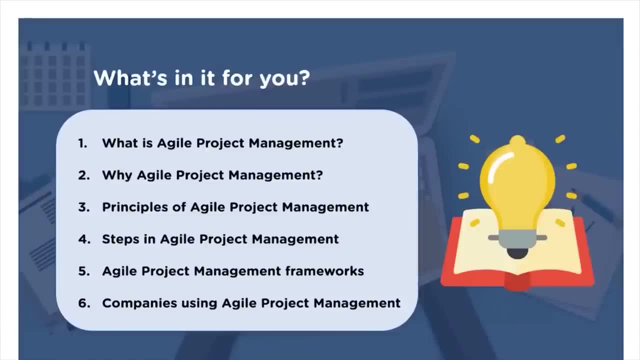 In this session we will be talking about Agile project management and several other things related to it. Before we begin, let's have a look at all the topics we will be covering today. First, we will see the basics of Agile project management. Then we will check the relevance and 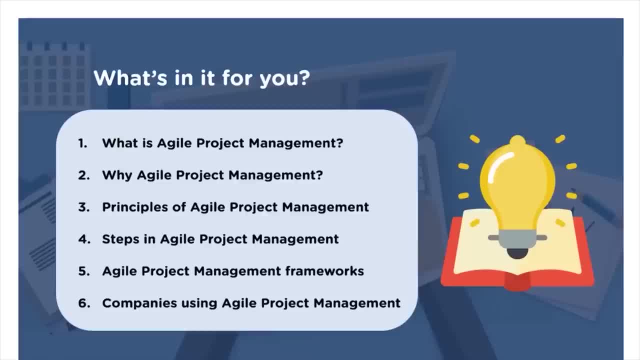 principles of Agile project management. We will then see necessary steps to implement Agile methodology. Along with that, we shall also see different frameworks involved in the process, and finally, we shall see some companies that use Agile project management. So, without any further ado, let's get. 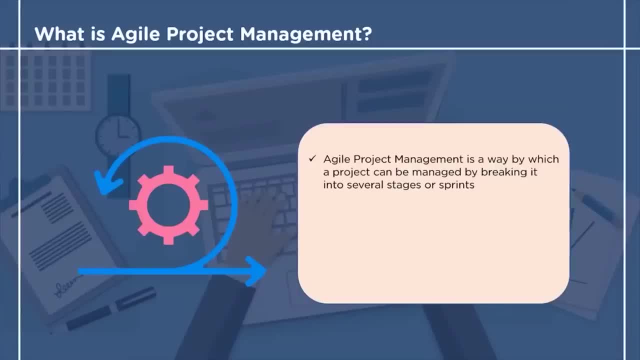 started with. what is Agile project management? Agile project management, as the name suggests, is a flexible approach to building a project. In Agile project management, the project is broken down into several stages or sprints. Agile does not work on the principle of delivering the final product at the end of 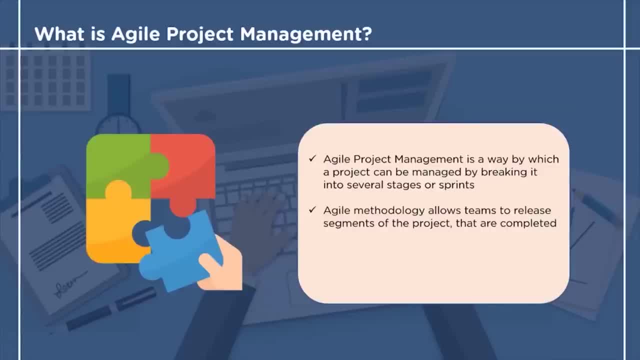 the project. It works on delivering sections of a project or mini projects. The process of project management in the case of Agile is Agile based, So there won't be any central control of project manager, as it was there in the traditional way of working Before we move. 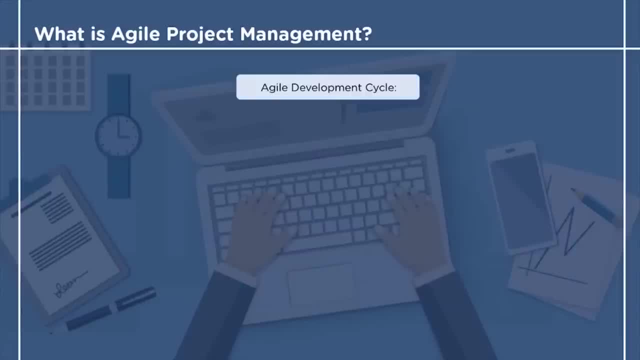 forth. let's have a look at the Agile development cycle. Agile methodologies consist of several small cycles, or sprints. At the end of each stage, we get a mini project. There's a product backlog that explains new features, changes in the existing features and several other improvements. 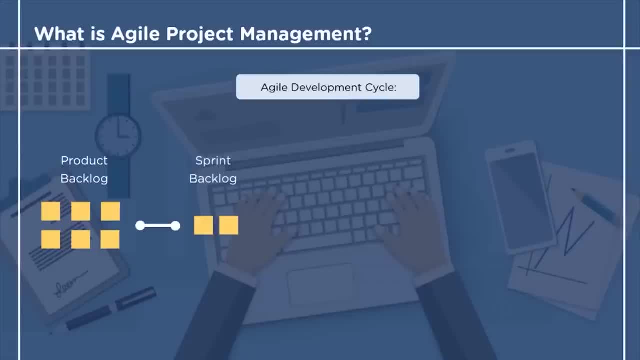 in the project. Then we have a sprint backlog, which has a list of tasks that are to be completed during each sprint. The sprint consists of planning, designing, execution, testing and deployment stages, And at the end of each sprint, a mini project is delivered With. 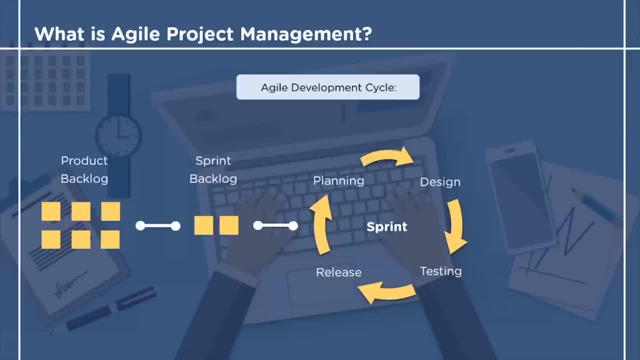 every sprint, new features are added to the product, which plays a significant role in the overall project growth. After all the sprints and early validation in the development, a final deliverable has a fewer chances of failure. Let's now have a look at some reasons. 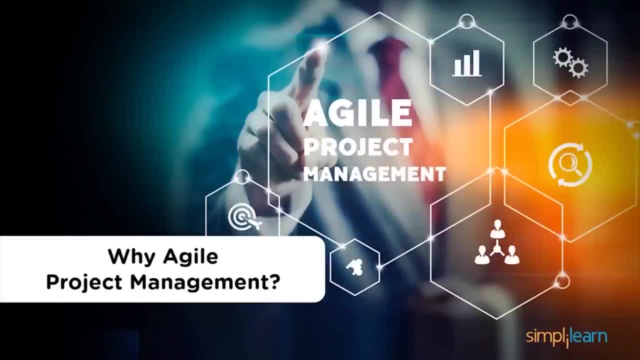 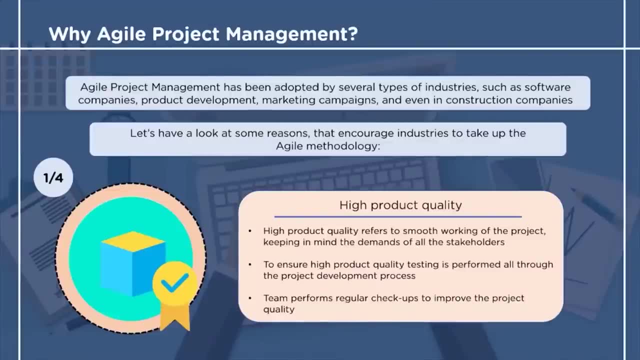 why industries are started moving towards Agile project management. The first reason is high product quality. When we talk about high product quality, we refer to the build of the product as per stakeholders demands. Testing is performed at short intervals of time wherever needed to ensure high quality. 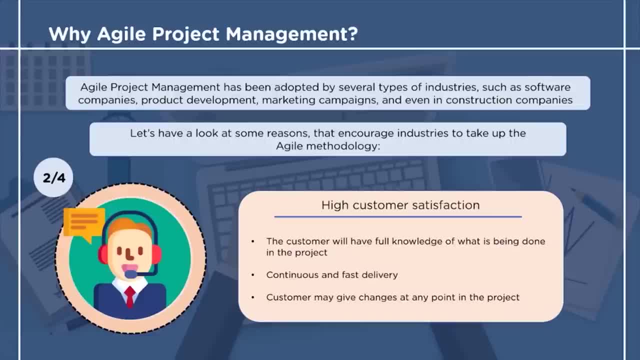 of the product. Then another reason is customer satisfaction. Whatever is done in the project is known by the customer. The deliveries don't take longer durations as they used to take in the case of traditional ways. The changes may be provided by the customer in the execution phase. 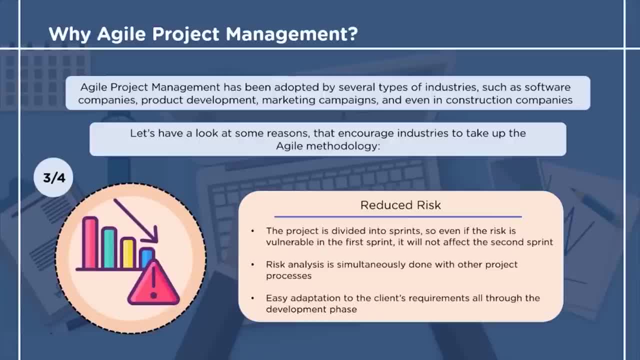 of the project. Third reason is reduced risk, Since the project is divided into sprints. so if the risk affects one sprint, it doesn't mean whole of the project will be at risk. The process of risk analysis continues to take place with all the other. 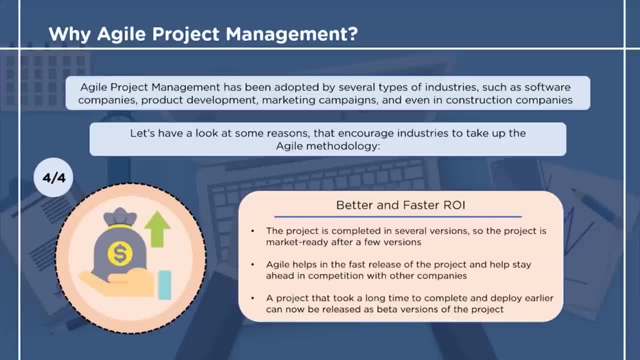 processes. Another significant reason for Agile project management is better and faster return on investment. The project is now developed in several sprints, and each sprint has its own version. Therefore, the project becomes market ready after few sprints only, Since the projects can now be released with ease and 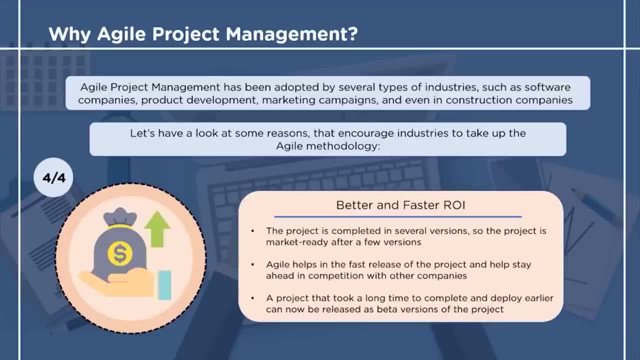 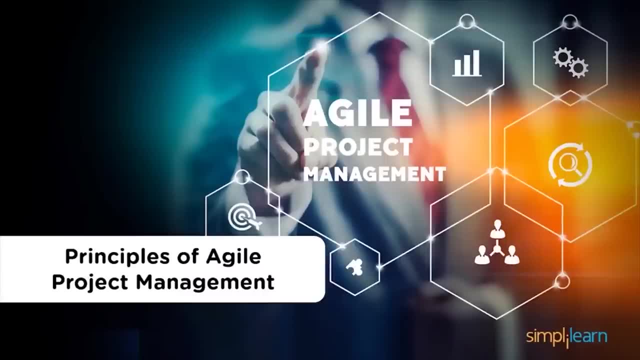 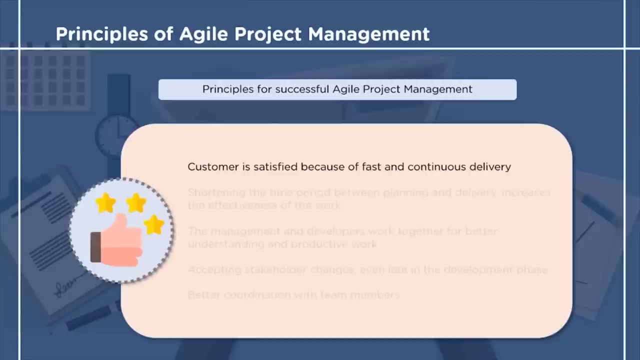 in shorter duration. this helps the organization to stay ahead in competition with respect to other organizations which have still not moved to Agile methodology. Now we shall check the principles of Agile project management. There are 10 principles for successful Agile project management. The first principle is the satisfaction. 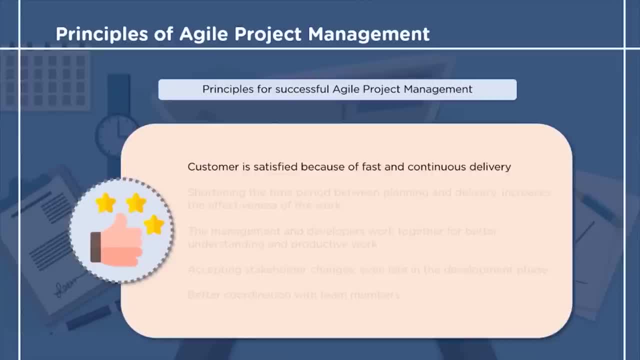 of the customer by delivering the project fast and with least number of errors. The next principle refers to decreasing the amount of time between the phase of planning and delivery. The third principle states that the team of managers and developers work together and increase the productivity of their work. The next principle states: 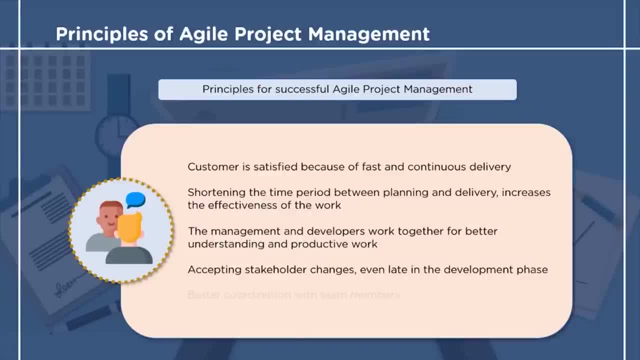 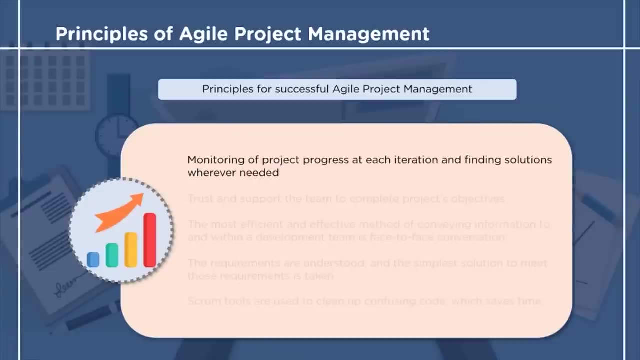 that the changes requested by the stakeholders can be taken into consideration and worked upon during the development phase as well. The fifth principle pays attention to the factor of coordination among the team members. Then the sixth principle refers to the process of monitoring and tracking the progress of the project at the end. 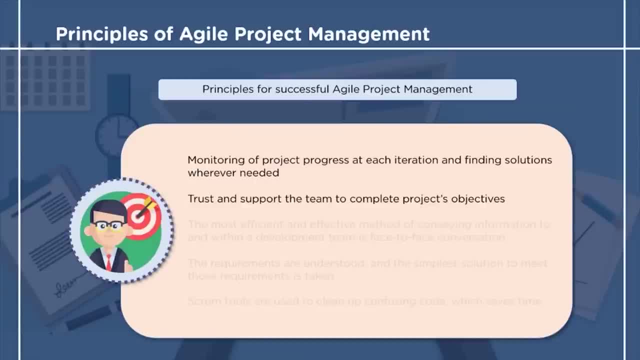 of each sprint and making amendments wherever needed. Moving on, the next principle states that there must be a feeling of trust and support towards the team to complete the project's objectives. The next principle emphasizes on face-to-face conversations with the development team. The 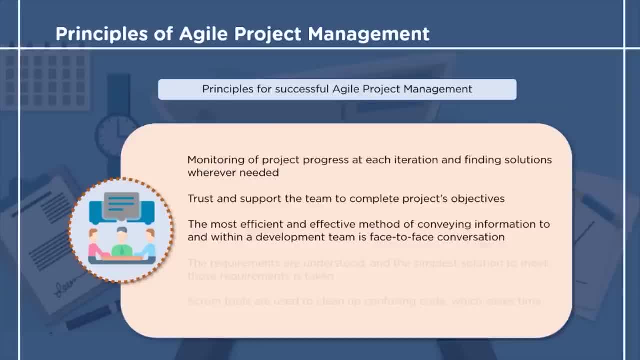 face-to-face conversation helps in both solving problems and easy knowledge sharing. Then the ninth principle emphasizes on finding solutions and maximizing the amount of work done with simplicity. This ensures timely completion of tasks by all the team members. The last principle states that scrum tools like 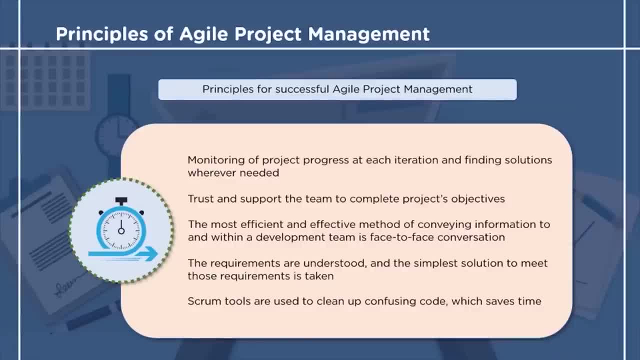 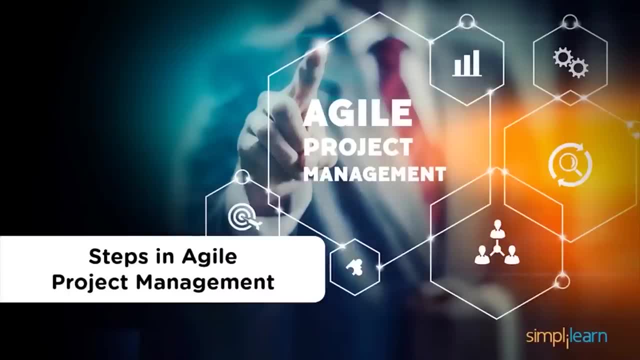 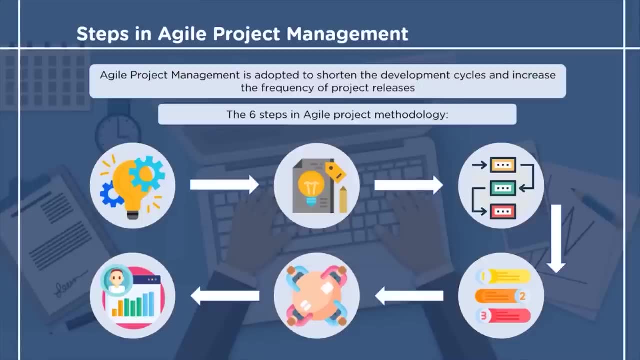 mondaycom or Zoho's must be used to simplify the complicated codes, which further helps in saving time. We shall now see the steps in agile project management. The goal of agile methodology is to produce shorter development life cycles and more frequent product releases than traditional waterfall. 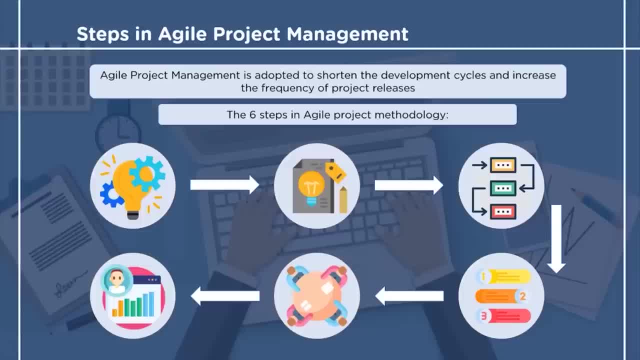 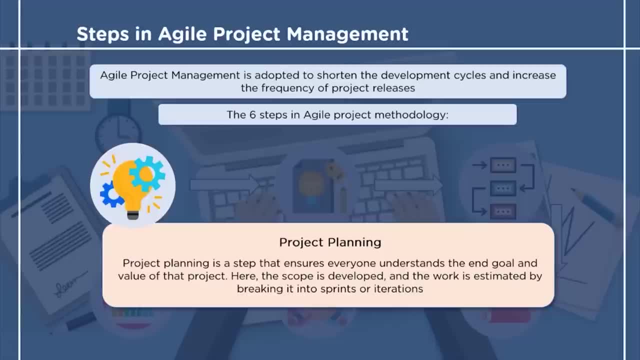 project management. So we will now check six steps in agile project methodology. The first step in the process is project planning. Project planning includes feasibility study, development of scope, breaking the project into executable tasks or sprints, and then estimating the amount of time needed to complete those. 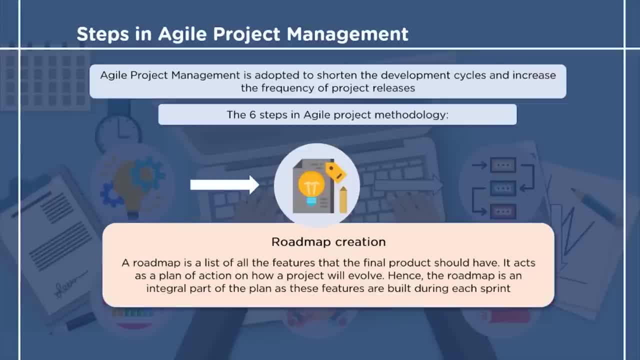 sprints. The second step is the step of roadmap creation. A roadmap is a plan of action that shows how a project shall evolve over time. A list of all the features that the final product should have is created, and the steps to achieve those features are taken. 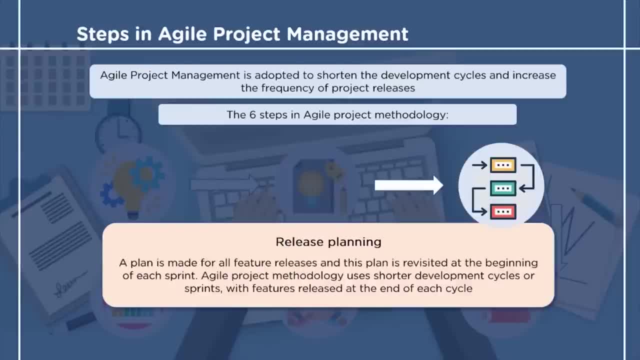 The next important step is release planning. Since we are doing the project keeping in mind the agile project methodology, the project will complete in sprints. That means there will be the release of features at the end of each cycle and, unlike the traditional waterfall model, the development cycles. 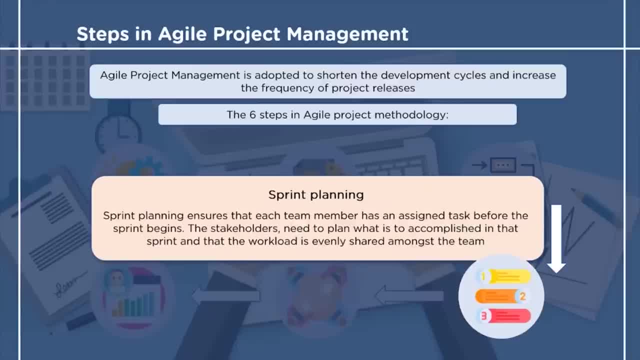 will be smaller. The fourth step in agile project management is sprint planning. The sprints are made keeping in mind what all is to be accomplished in that particular step. At the beginning of each sprint, the goal of that sprint is decided and steps to achieve that goal are taken. 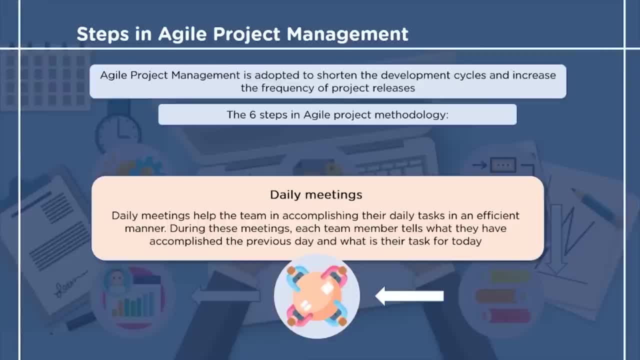 The next step in the process emphasizes on daily meetings. There are short meetings every day to discuss if the team was able to finish the task for each sprint and check if there are any amendments that are required. Each team member talks about what they achieved in the last. 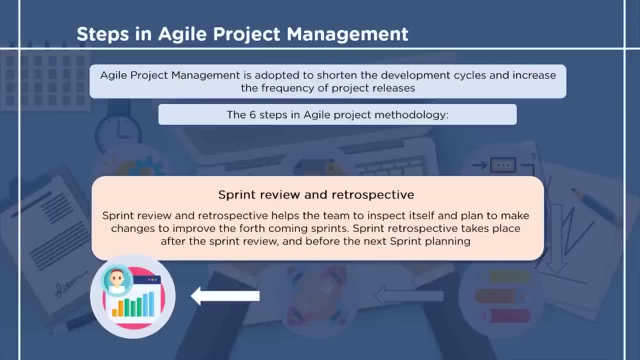 sprint and what are they going to work on in the next sprint? The last step is the step of sprint review and retrospective. There are two meetings after each sprint. First meeting is for the sprint review. This meeting is with the stakeholders to show them the finished 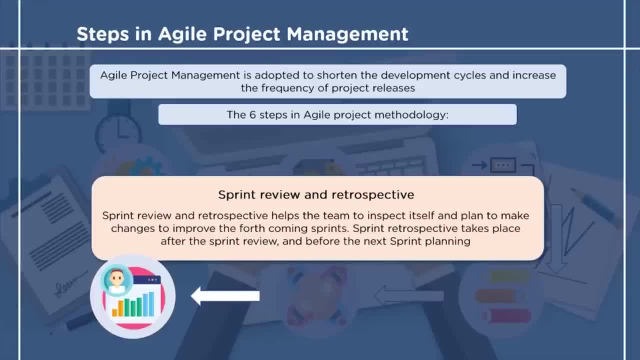 product. This helps both sides to build a relationship and discuss if there are any issues in the end product. The second meeting is for having a sprint retrospective. This meeting involves the stakeholders to discuss what went well and what went wrong during the sprint Sprint retrospective. 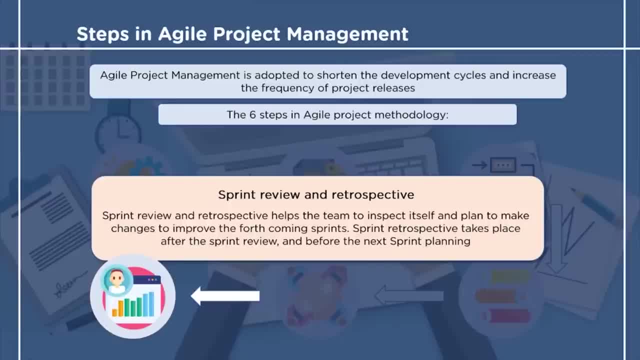 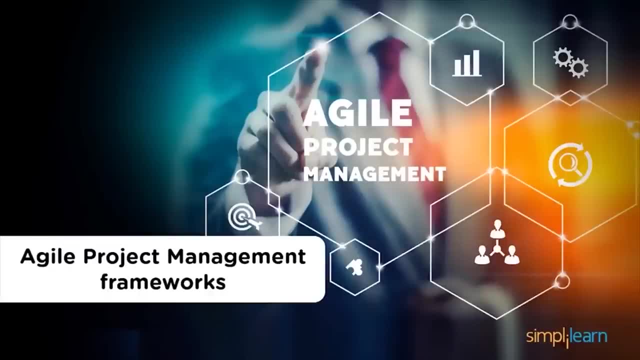 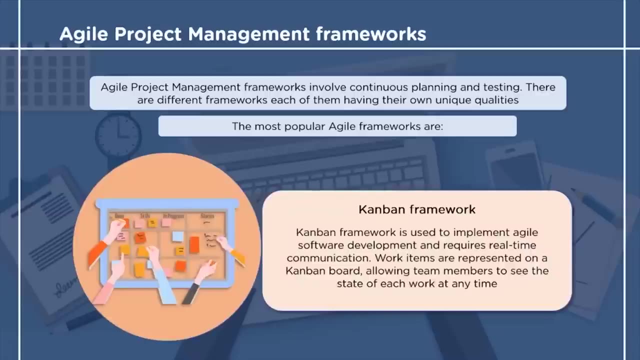 takes place after the sprint review and before the next sprint planning. Now, when we know the steps needed for agile project methodology, we must understand some agile project management frameworks. There are several frameworks available today. Here we will be discussing some of the most popular frameworks. The first framework: 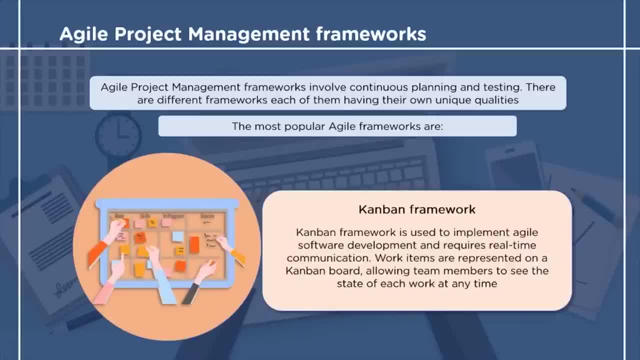 we will discuss is the Kanban framework. Kanban framework is a well-known framework for implementing agile software development. In the case of Kanban framework, work items are represented on the Kanban board, which helps all the team members to see the state of every piece. 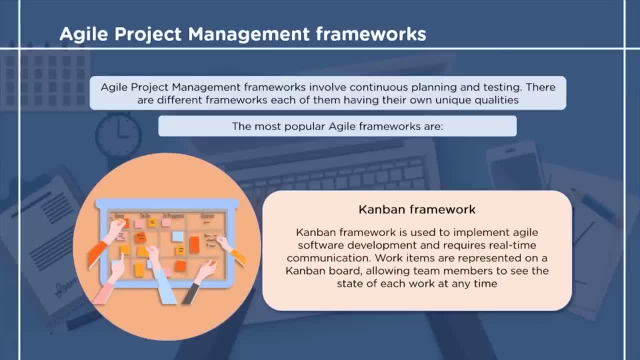 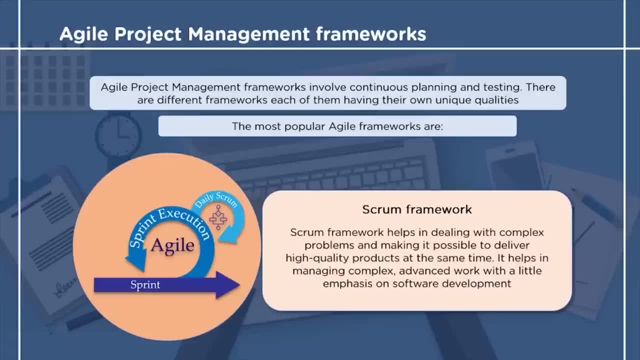 of work at any time. Kanban board not only helps in visualizing the work, but also optimizing the workflow among the team. The next framework we will discuss today is the Scrum framework. Scrum framework is a popular framework for managing complex knowledge work. 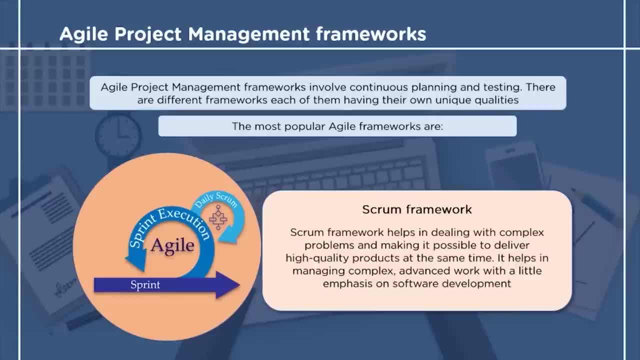 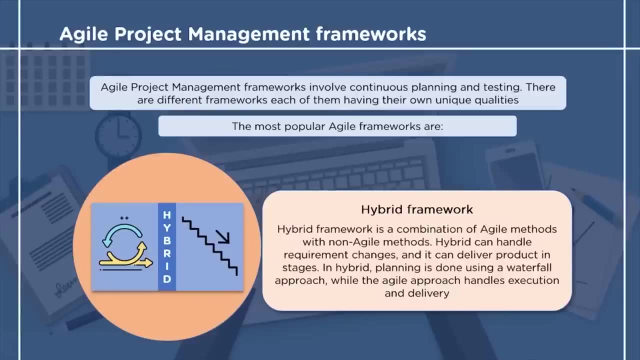 like in the field of research and advanced technologies, Scrum is a simple framework that helps team work together and learn through their experiences gained while working on a problem. The third framework we will see today is the hybrid framework. The hybrid framework is a combination of agile methodology. 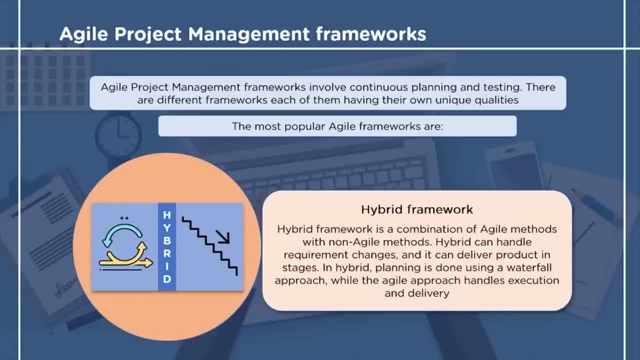 and non-agile methodology. In the case of a hybrid framework, planning is done using the traditional way of project management, while the execution and delivery is done using the agile methodology. Since the hybrid is a combination of the two, it handles the requirement changes. 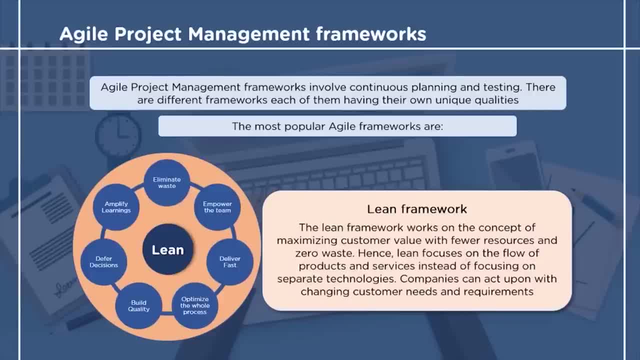 and delivers the product in different stages. The fourth and the last framework we will see is the lean framework. The lean framework works on the principle of providing maximum customer value and creating zero waste. It focuses on optimizing the flow of products all through the value stream. This helps in eliminating 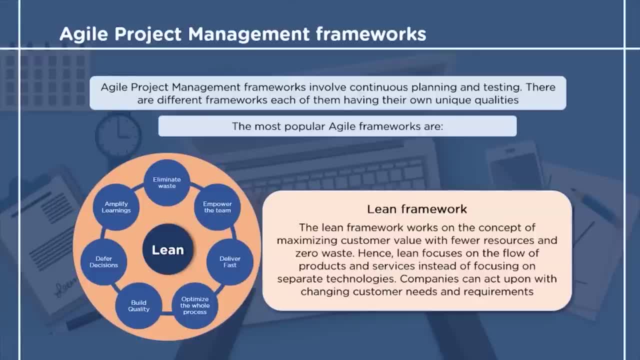 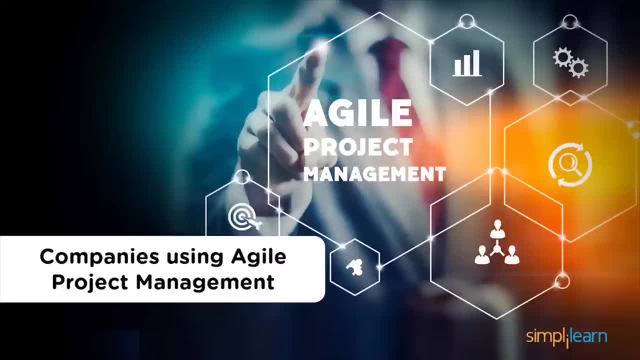 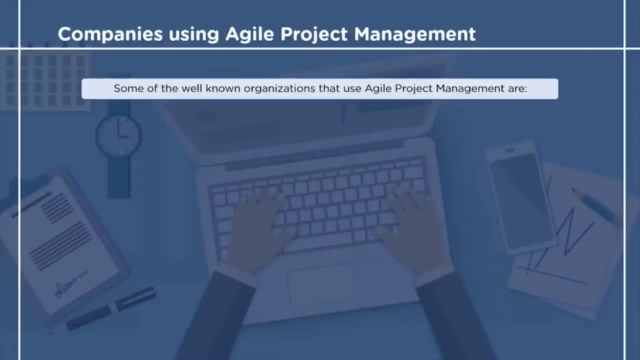 waste all through the process and create processes that requires less human efforts. This also simplifies the process of information management and makes it more accurate. Finally, let's have a look at some companies that have opted for agile project management. Today, around 22% of the organizations 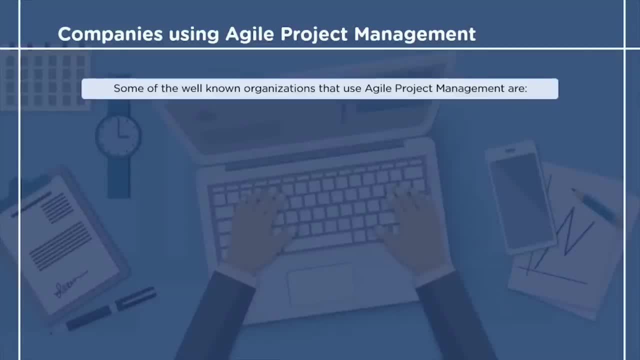 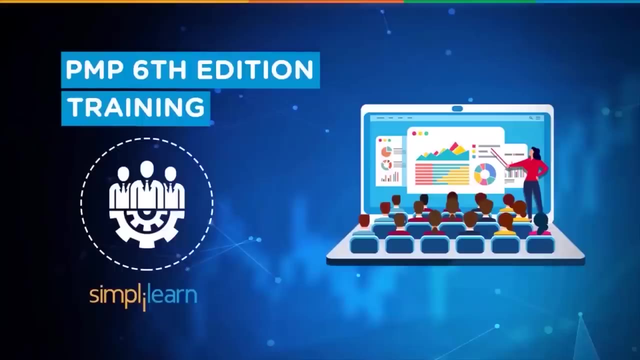 worldwide have all their teams working on the principle of agile project methodology. Let's have a look at some of the most prominent companies in the world that use agile project management. In the list we have IBM, Cisco, AT&T, Microsoft, Philips and Samsung Welcome. 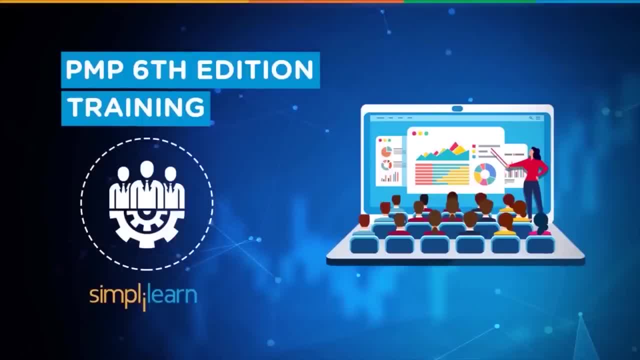 to SimplyLaunch PMP 6th Edition training tutorial. I am CMR Chandra MR, a certified project management professional, Princeton practitioner, ITL expert, ITL4 managing professional COBIT 5, and DevOps. Today we are 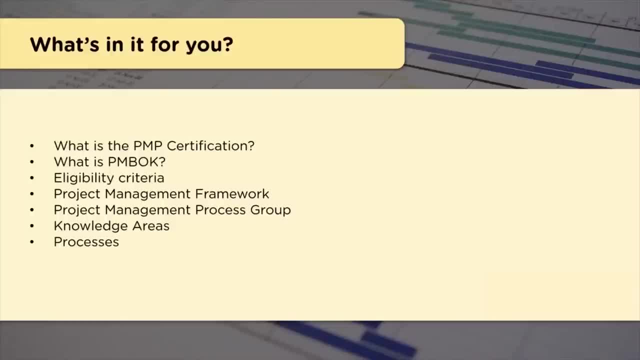 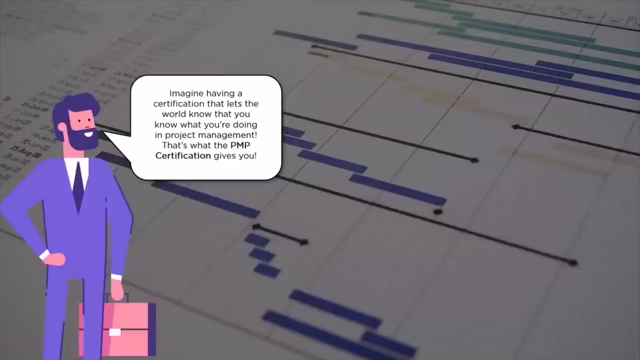 going to look at understanding. what is the PMP certification? what is PMBOK eligibility criteria to appear in PMP examination? the project management framework, the project management process groups, knowledge areas and processes. So now imagining the world where 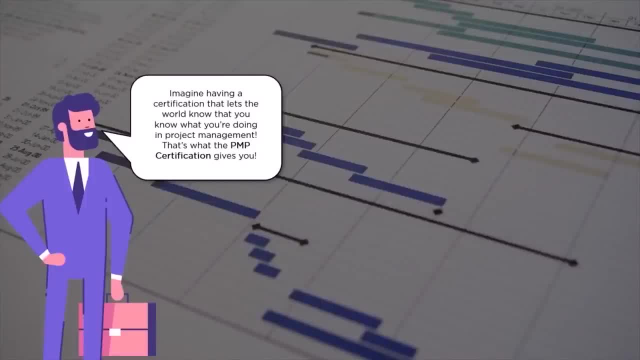 you have a project being done and you are the project manager, and how best a project can be conducted. So to make a project successful, it is required to follow a best practice. So if you have a certification, just imagine having a certification that. 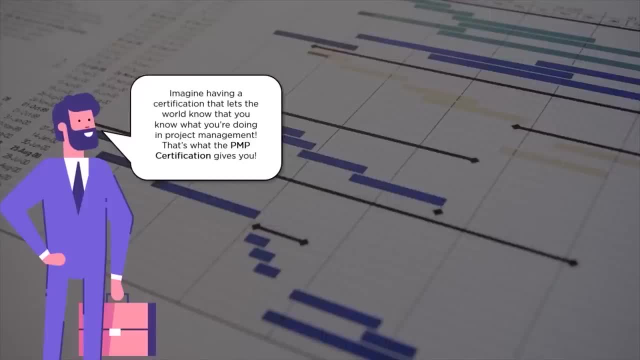 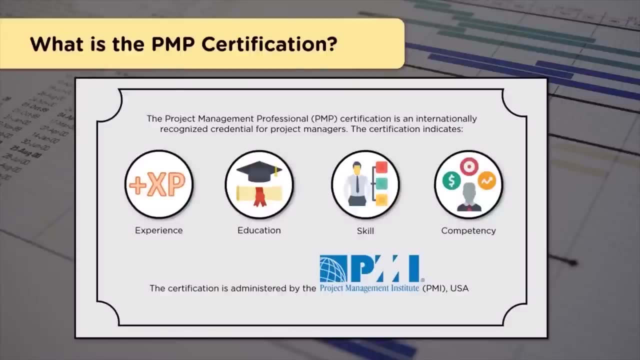 lets the world know that you know what you are doing in project management. So PMP certification gives you all. So what is PMP certification? So the PMP, the project management profession certification, is a certification of PMI. 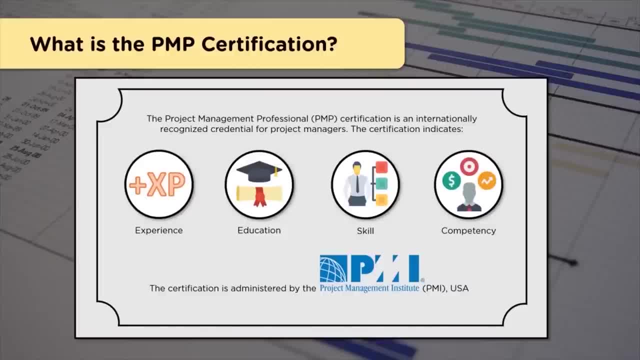 the project management institute, which is at USA. So it is an internationally recognized credential for project managers. See the certification indicates that the certified professional has a sufficient experience, education, skills and competency. Reason being before going for PMP certification, it asks. 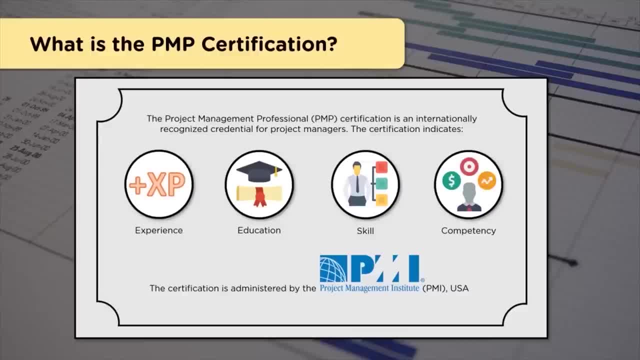 for specific prerequisites, which involves experience in project management, as well as formal education of project management and demonstrated skills. So, that being a prerequisite for project management professional certifications, it is very essential that one need to understand what it takes to become eligible for PMP examination. 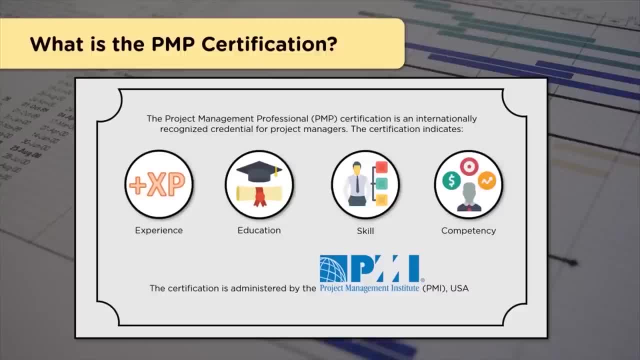 So that we will go through in the subsequent slides. So the moment one has the PMP certification, that itself indicates the prerequisites to take up a PMP certification is accomplished already before going for certification, And then the individual will go for a certification and become 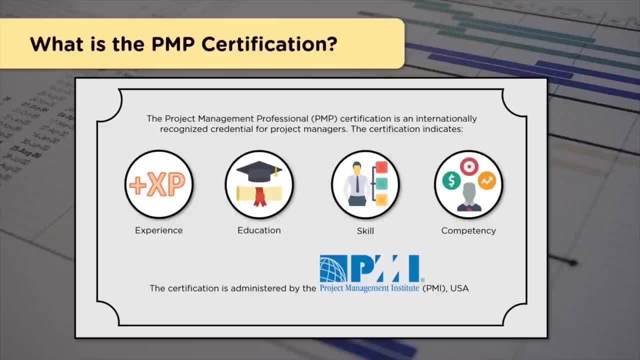 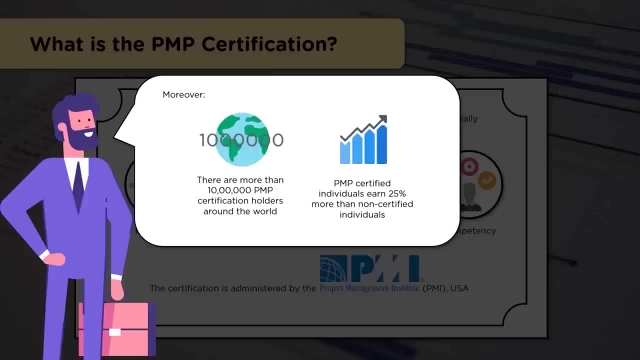 certified professional. So that way it concludes, it also indicates that person who holds the PMP certification has sufficient experience, education, skills and competency. Moreover, there are more than 10,000 PMP certification holders across the globe. 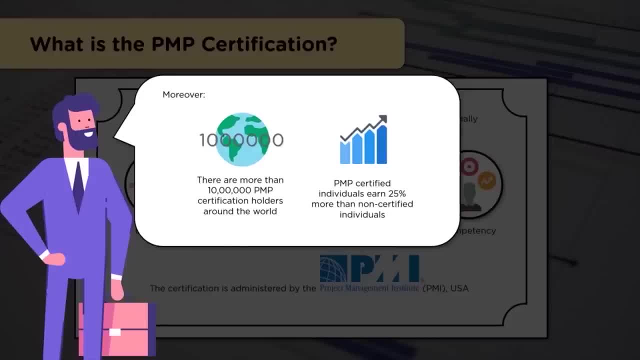 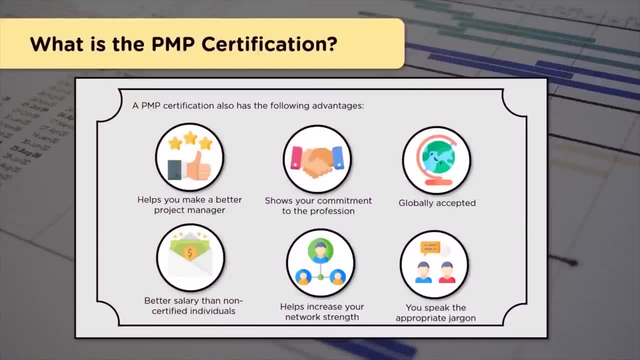 So PMP certified individuals earn 25% more than non-certified individuals. So now PMP certification also has the advantages which are given here, like: helps the project manager to practice the project management better, create the results better, demonstrate the project management capability. 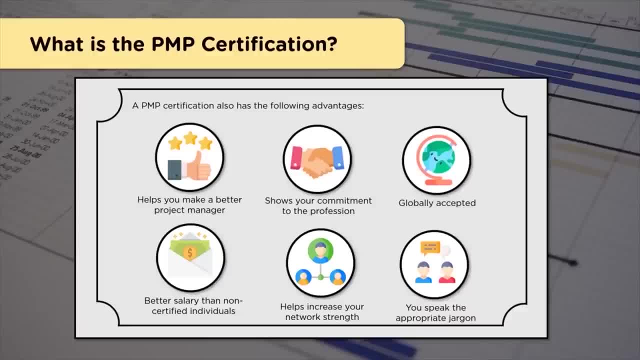 better. So this also helps project manager to show the commitment towards the project management profession and having PMP certification provides the recognition across the globe which helps in getting better salary compared with people- the professionals- who are not certified, and also helps in increasing the network project management. 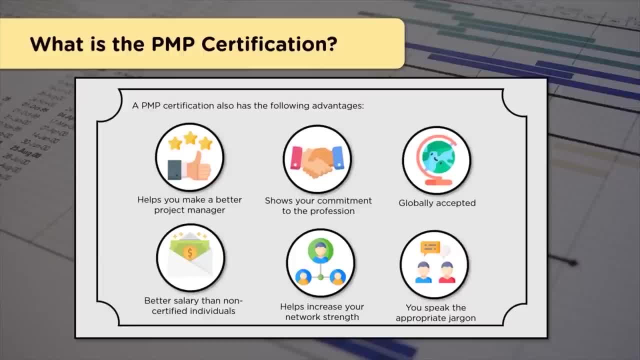 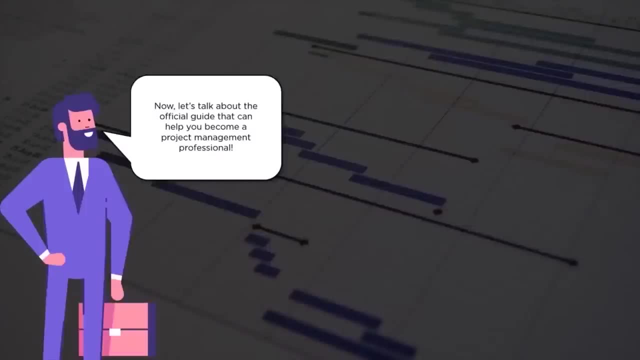 network who actually practices project management, the fellow project managers who are practicing the project management. So there are certain vocabularies, jargons, which are used specifically while doing the project management. PMP helps to understand those. So now let us look at 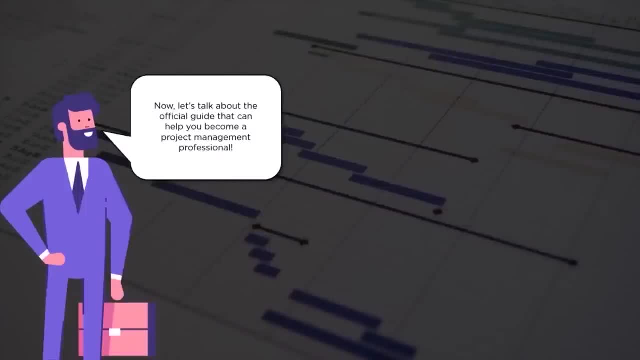 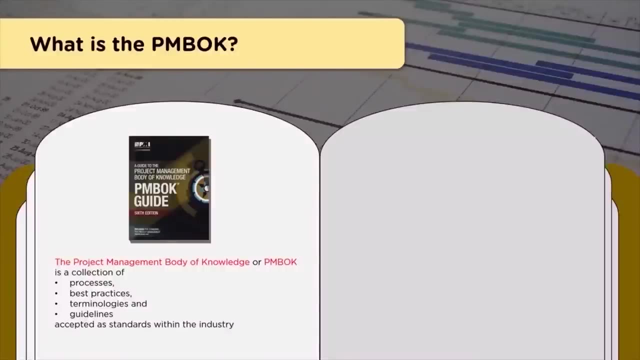 what does the official guide which is used in PMP that can help to become a project management professional? So that is PMBOK, which is referred as project management body of knowledge, or PMBOK, which is the collection of processes, best practices. 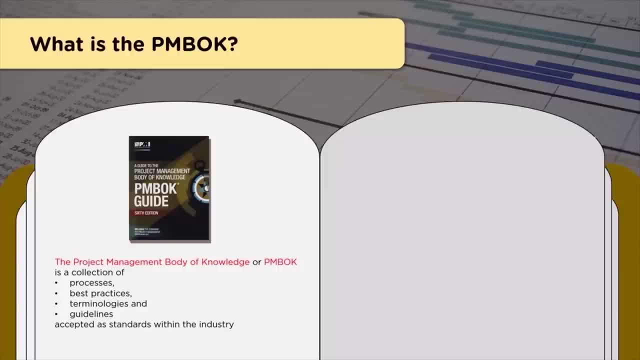 terminologies and guidelines accepted as standards within the industry. So the latest edition of this is 6th edition, which was released in 2017.. The first edition of PMBOK guide was published in 1996 and the 6th edition, as I mentioned. 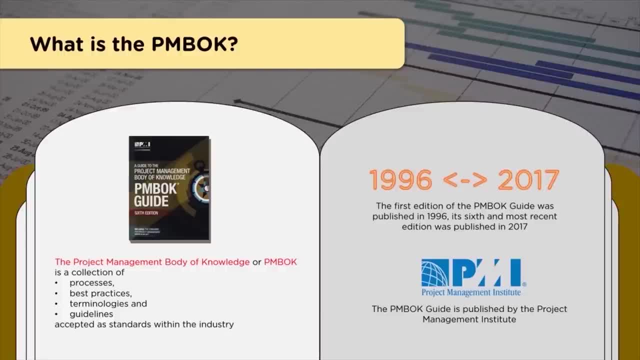 was released in 2017 and exam format was revised from 26th March 2018.. So PMBOK guide will become the basic reference to appear in the PMP examination. So one needs to go through the training based on PMBOK guidelines. 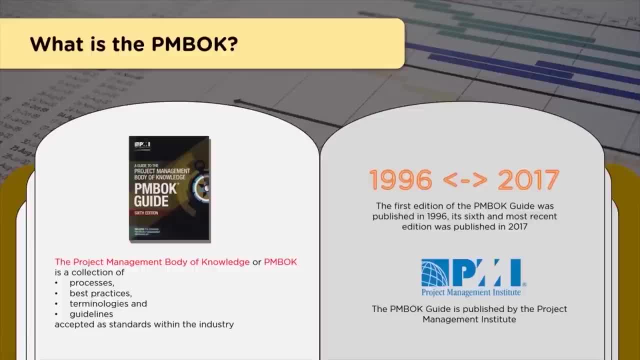 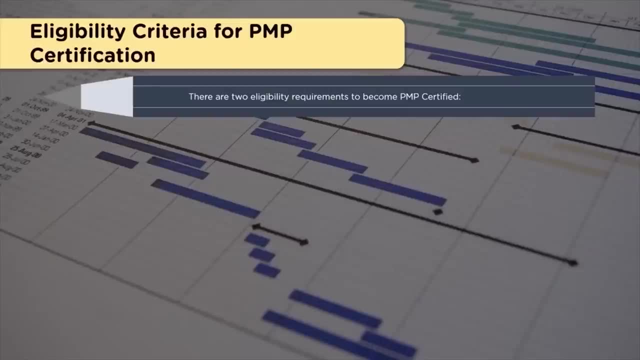 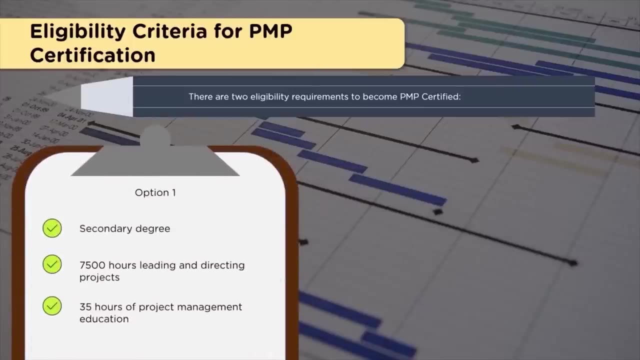 so that will help them to pass the examination easily. So eligibility criteria for appearing for PMP certification examinations. So you can have two types of eligibility which PMI defines. So option 1 includes someone who has secondary degree should have 7500 hours of. 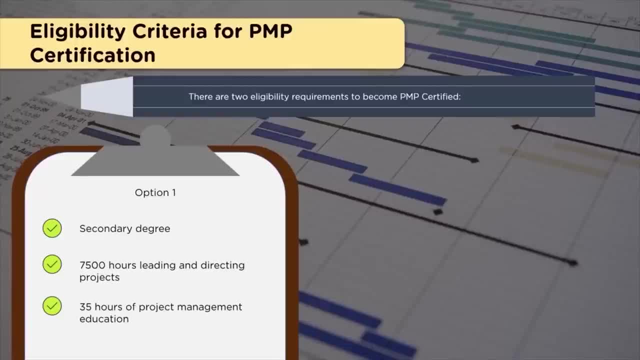 leading and directing project. That is an experience. what it is asking as a prerequisite before the professional go for examination, Plus 35 hours of project management education formally from a registered education provider Like SimpliLearn Option 2, someone who has 4 year degree project management. 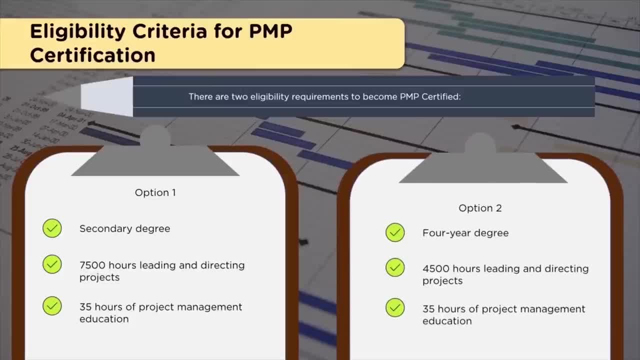 experience leading and directing project. This experience will be 4500 hours, whereas, as we saw in option 1.. In option 2, 35 hours of project management education is required, and that is from registered education provider like SimpliLearn, as I mentioned earlier. 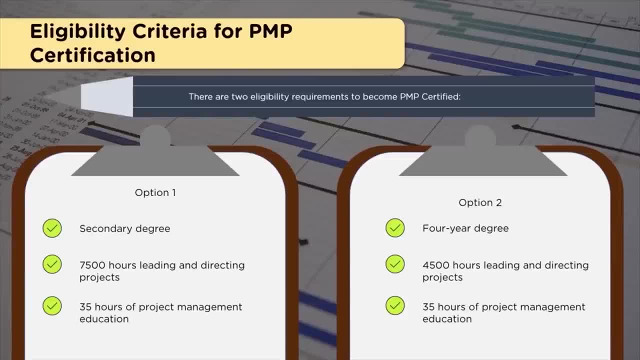 So this training, which is conducted by registered education provider, will have their trainings aligned with PMBOK, the latest edition. So SimpliLearn enables people to learn what are the topics in PMP framework, plus make the professionals ready to appear the examination. 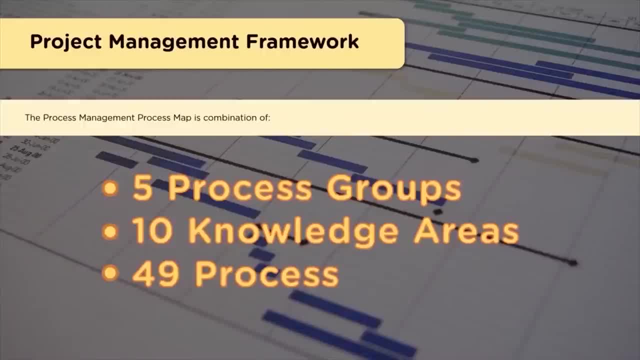 and become successful. The project management framework which is defined in PMBOK includes 5 process groups, 10 knowledge areas and 49 processes. So when we say 5 process groups, this indicates the way the project flows, How each of these process groups are connected. 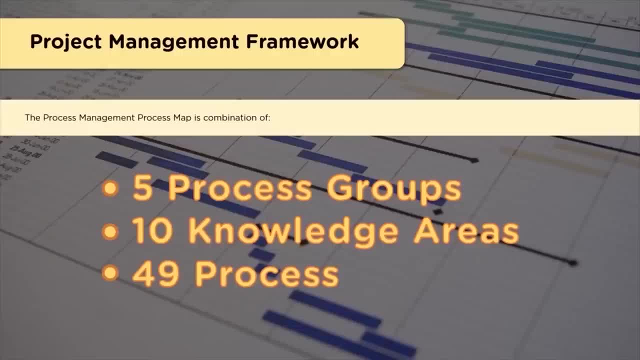 while project happens, in the project life cycle, Whereas 10 knowledge areas are the one which needs to be looked up, to demonstrated up, to considered while doing the project management and the 49 processes distributed across 5 process groups and 10 knowledge areas, has 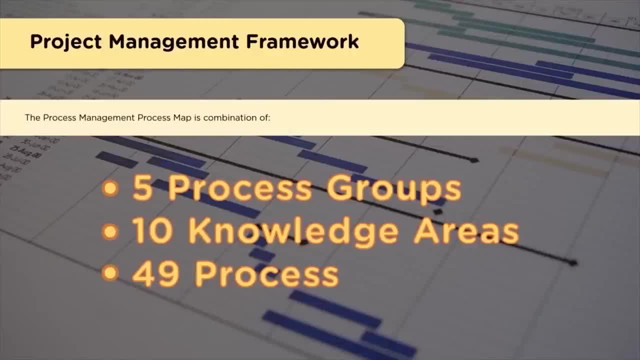 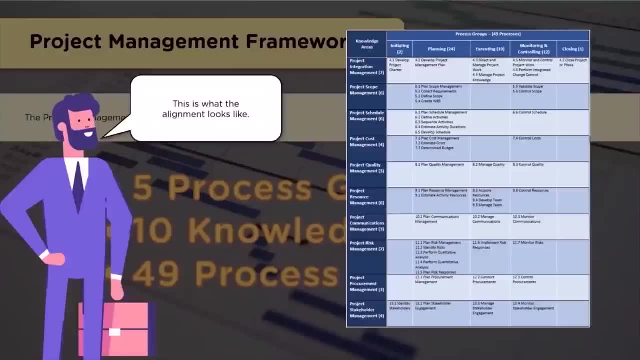 the activities, the objectives, the inputs, outputs, tools and techniques clearly defined so that those can be applied while doing the project management. So those are aligned the way it is shown in the table. So 5 process groups, that is, initiating planning. 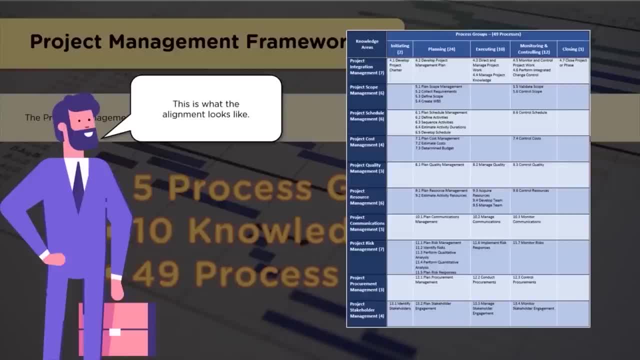 executing, monitoring and control and closing. These are the process groups, whereas 10 knowledge areas includes project integration management, project scope management, project schedule management, project cost management, project quality management, project resource management, project communication management, risk management, project procurement. 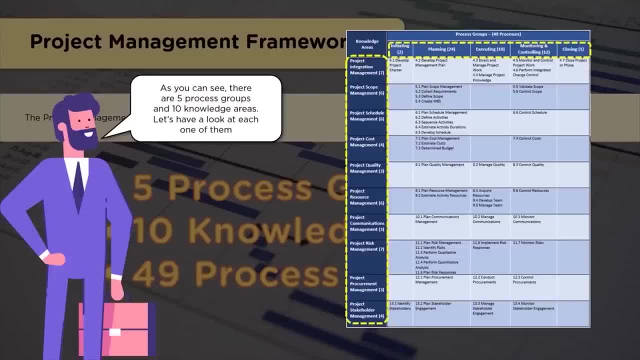 management and project stakeholder management. So each of these knowledge areas and process groups are aligned in such a way where the processes align with a specific process group and knowledge area can be demonstrated accordingly If you look at a process which goes from initiating to planning. 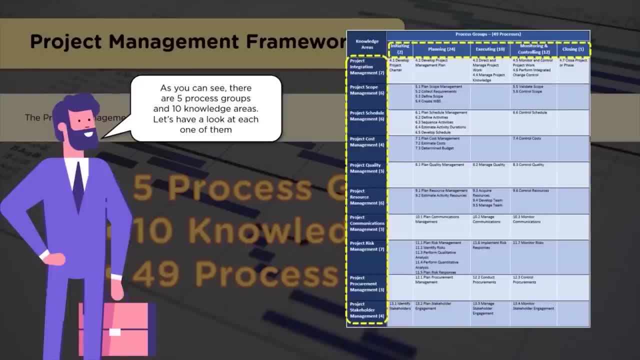 planning to executing and then monitoring and control. While you do monitoring and control, if there is anything found as a deviation, it may come back to planning or executing for necessary corrections. Once the necessary corrections happens again, it moves to monitoring and control to check whether it is. 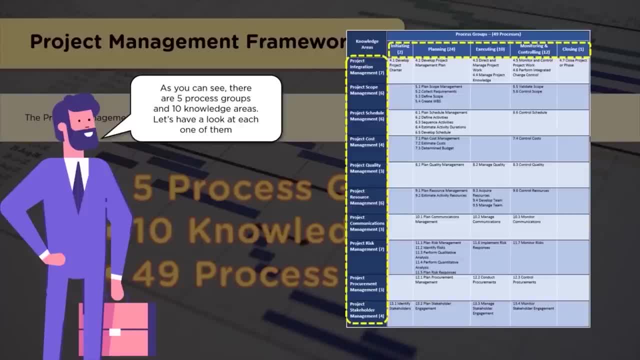 completely done as expected or not. If it is confirmed everything is done as per the requirements defined, then it moves to closing. This is how the project flows in the project life cycle, Whereas all the 10 knowledge areas happens in parallel. So now, if you look at 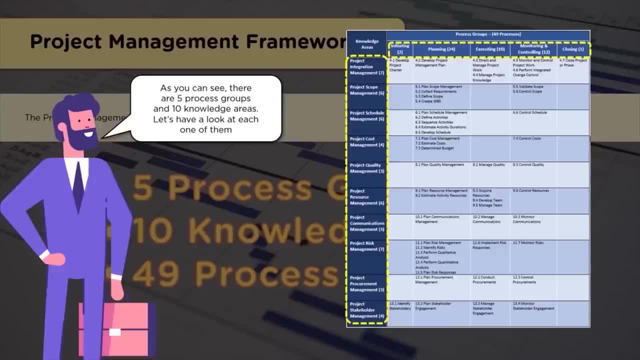 initiating process group you can see two processes. that is, develop project charter and identify stakeholders. So develop project charter and identify stakeholders basically defines project charter required for the project as well as initial identified stakeholders who are required to move forward in the project. Similarly, if you look at 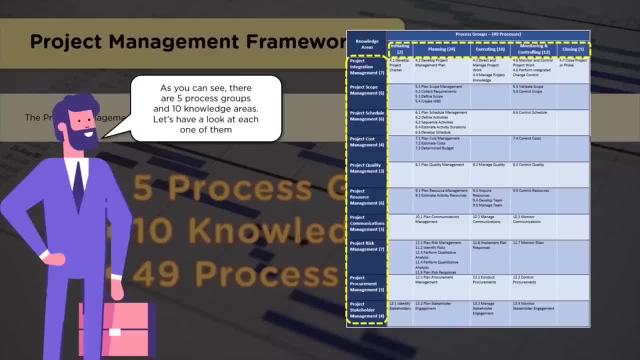 planning process group. you have 24 processes which are distributed across all the 10 knowledge areas. So these processes creates a plan for the project which involves scope, baseline, schedule, baseline cost, baseline, quality management approach. then resource management approach Means the plan. 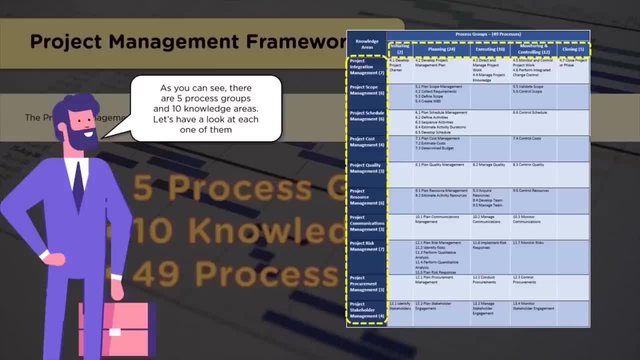 I mean to say When I say approach, I am speaking about the plan. Similarly, communication management plan, risk management plan, procurement management plan, stakeholder management plan and all of these will get consolidated into project management plan in the integration management knowledge area. Once. 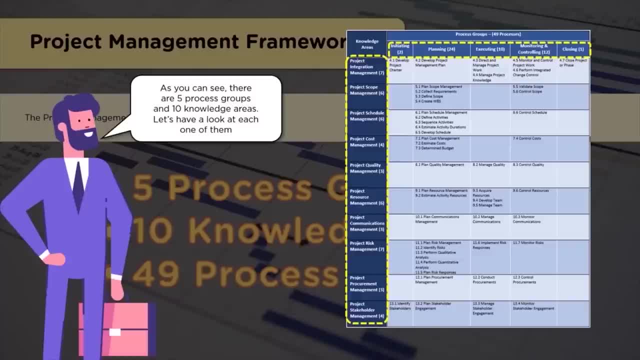 this plan is done and approved, then it moves for execution. All that project manager do during execution is directing and managing project work and managing the project knowledge. At the same time, project manager would take responsibility of managing quality, acquiring resources, developing team managing. 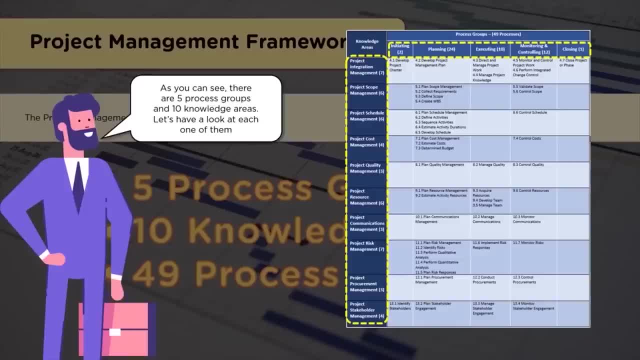 team. then communications, which are planned as per the communication management plan. communication should happen during execution. So, similarly, implementation of risk responses defined while doing the planning and conducting the procurements as planned, and then managing stakeholder engagement. So actual execution of those work packages, execution. 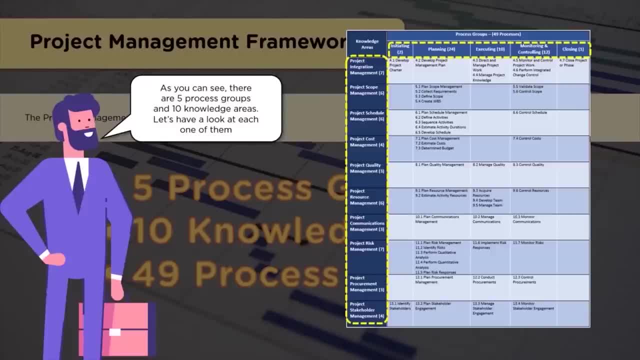 of those deliverables happens from the team. Now, as those deliverables happens, the delivered products are checked, monitored and controlled. You can see validate scope, control scope. Likewise, for each knowledge areas, there is a control process which checks: is that happened in execution? 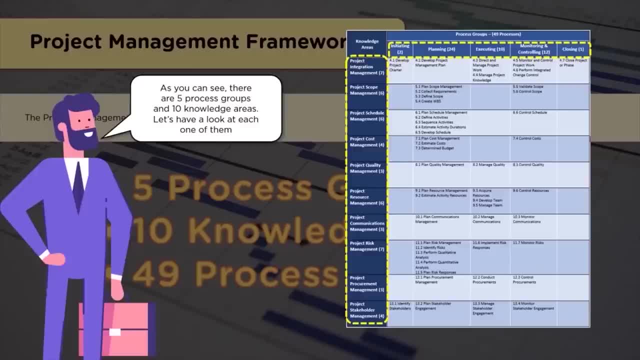 as it was planned in planning process group. So then that is consolidated here for monitoring and controlling the project work in entirety, integrated, Similarly performing integrated change control, any deviations found in any of these checks, which is being done in the control now that 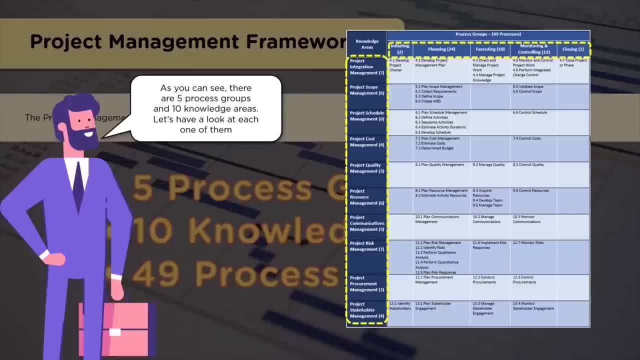 deviation needs to be corrected, So change will be raised. So request for change will be raised and that will be approved and controlled and necessary directions are given, approvals are given, and that moves towards execution for implementation. Once it is implemented, again validation happens. 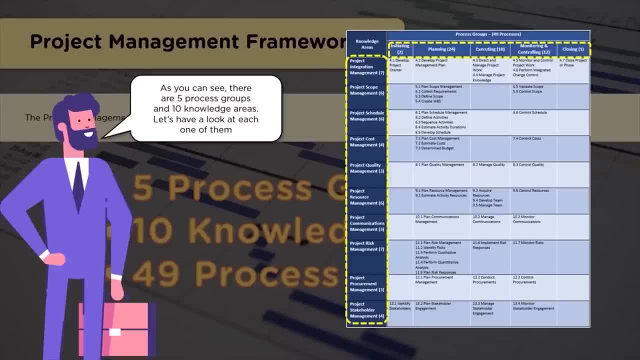 Once control checks if everything is okay, then it moves to the closure. Now activities in closure. a project or a phase involves just an activities of closure. The products or services or results which are created from the project does not go to closure until those are validated, checked. 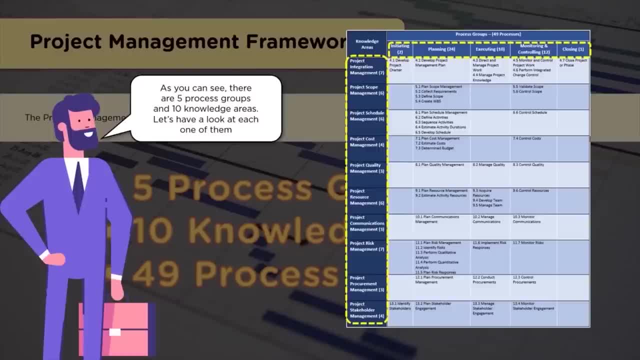 confirmed and signed off. Only then it goes to closing project or phase, and necessary formalities which are required to be completed before conclusion, will happen in closing project or phase. This is how the project flows. Second point which you should keep in mind is: a project manager is also. 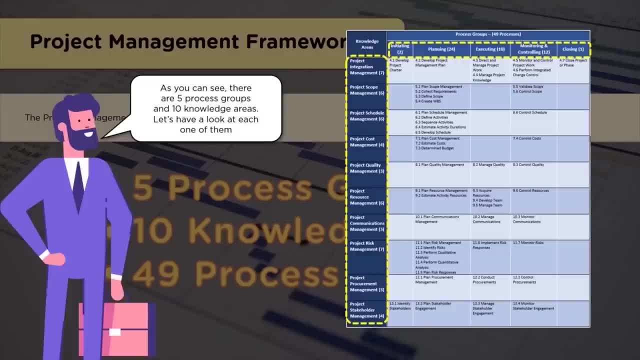 called as an integrator. So main focus, the umbrella view, the bird's eye view project manager should have from project integration management. So this layer project integration management where project manager should have an umbrella view, total view about entire project. 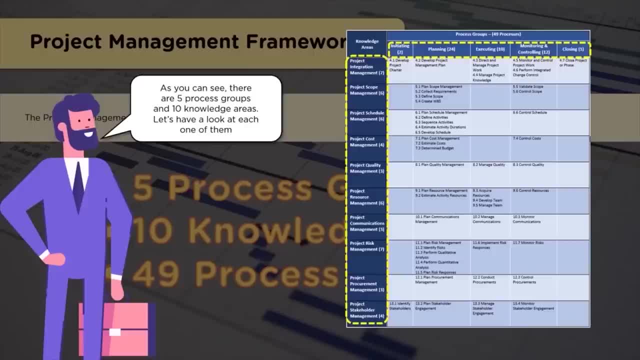 what is happening. So bigger picture: only when project manager has a bigger picture, project manager can come to the lower levels and see: are they progressing the way it is supposed to? So then go back, look at the bird's eye view again and see, is it going in the right? 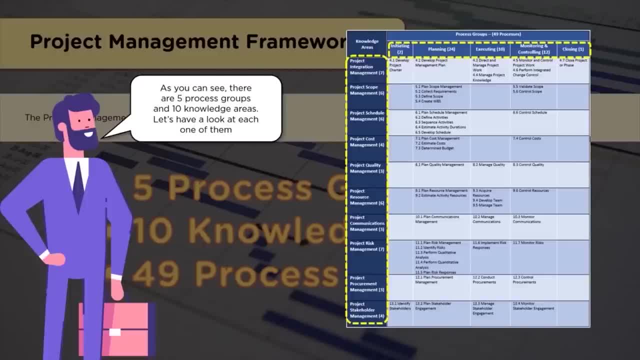 direction, which is very essential. So further, I guess we will look at each of these process groups and what happens in each of the process groups, similarly in knowledge areas. So let us move forward Now: project management process groups. So these process groups. 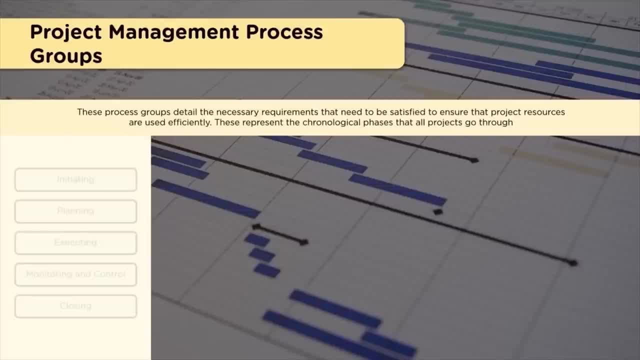 details, the necessary requirement that need to be satisfied to ensure that project resources are used efficiently, and these represents the chronological phases that all projects go through during the project life cycle. So, starting from initiating stage, it moves to planning. Once the plan is ready, then it moves. 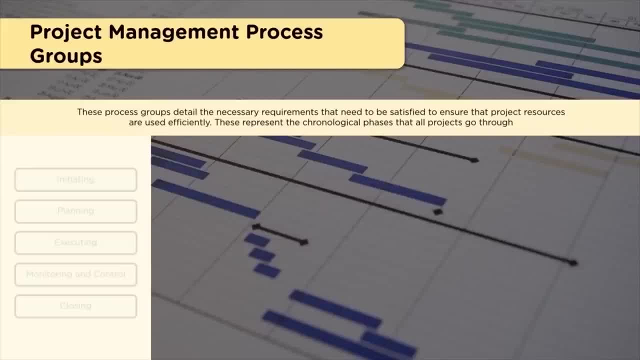 to execution. As the execution happens, validation checks happens in monitoring and control and as you find some deviation in monitoring and control, for correction of the deviation it comes back to execution or if any necessary changes needs to be done in planning also, while doing these, 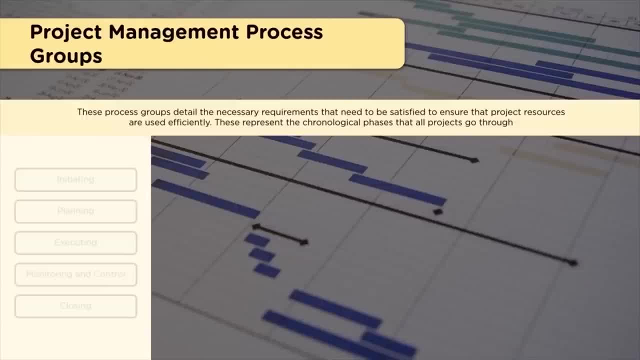 corrections, then it may move to plan, then execution and then monitoring and control. So this loop continues until the confirmation: yes, it is delivered as per the plan and then it moves to closure. So that is how the project flows and the project life cycle. 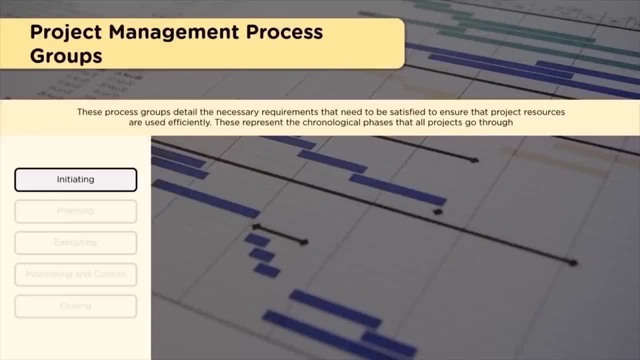 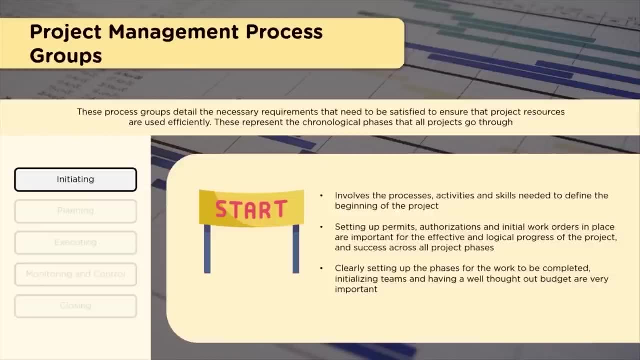 would be like that. So initiating process group. So initiating process group involves the processes, activities and skills needed to define the beginning of the project. As I mentioned earlier, in initiating process group the creation of project charter happens and identification of. 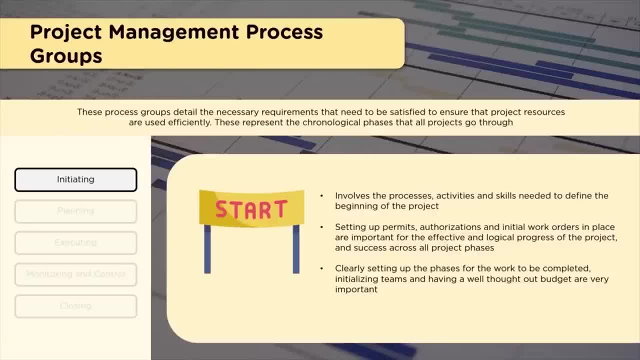 the basic stakeholders, main stakeholders who are required to understand the further requirements in detail. who needs to be engaged, So those are identified. So setting up permits, authorization and initial work orders which should be in place and are important for effective. 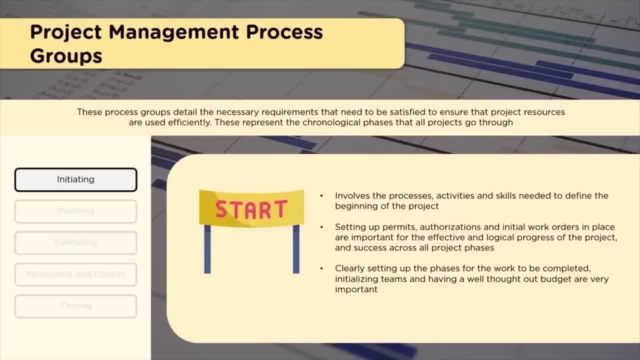 and logical progress of the project and success across all project phases. So this clearly sets up the phases for the work to be completed: initializing teams and having a well thought out budget, which is very important. So this gives that view in totality, but it may. 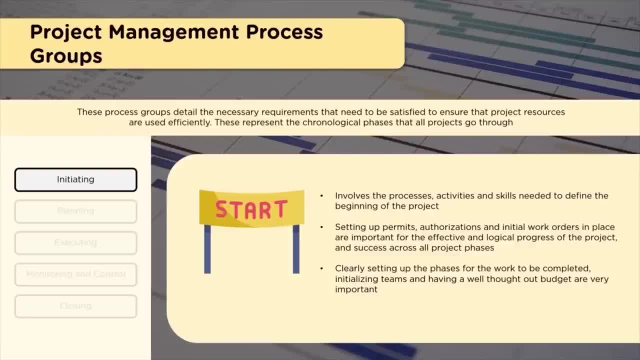 not give you the full granular details, but it sets the directions, provides that insight and also one important thing we should keep in mind is in initiation stage, appointment of project manager happens, The formal declaration of appointment of project manager happens and project charter will be formally handed over to project. 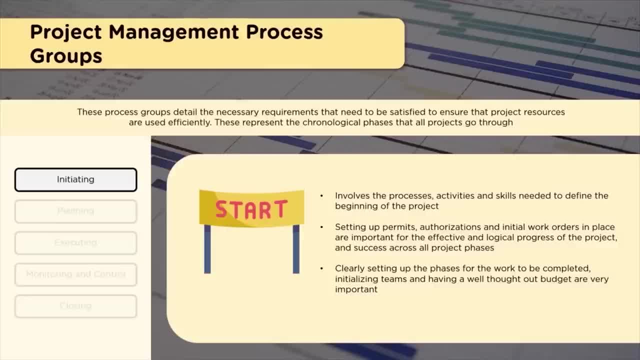 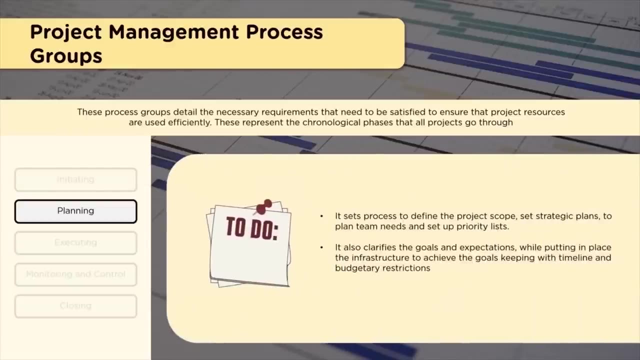 manager and that formal declaration of assignment of project manager happens. From then project manager takes over and first activity project manager does is identification of stakeholders. So next process group is planning process group, where we have around 24 processes to define the project scope. 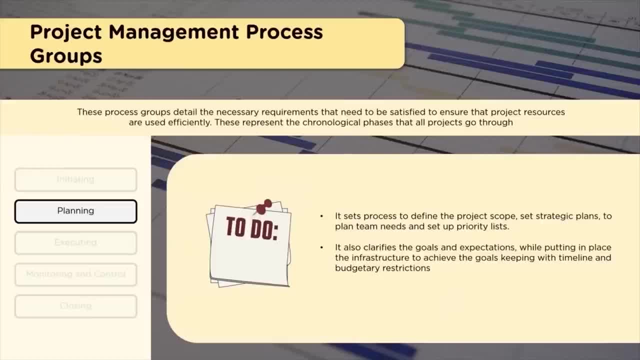 cost schedule, quality, resource risk, then procurement, stakeholder engagement. So comprehensive plan if it is waterfall approach, or basic skeleton plan, which is required if it is agile approach. So it also clarifies the goals and expectations while putting in place. 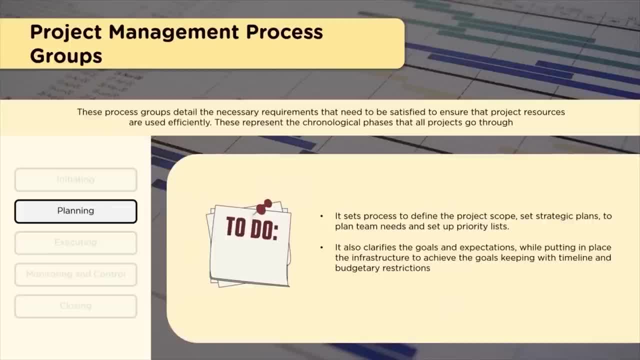 the infrastructure to achieve the goals, keeping in timeline and budget constraints. The end to end view of the project is provided in planning. So this perhaps as a basic reference, while the execution and monitoring and control happens. So, based on the planning, the way it is done, execution will happen. 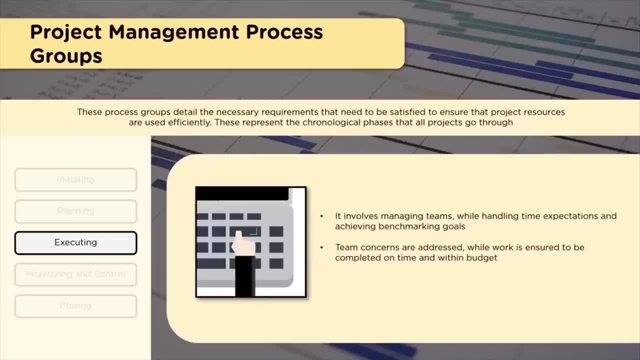 Now next process group is executing process group, where the role of project manager is to direct and manage project work and manage the project knowledge main activities, being an integrator of a project. Secondly, acquiring resources. it may be human resource or technology resource or any other resource required. 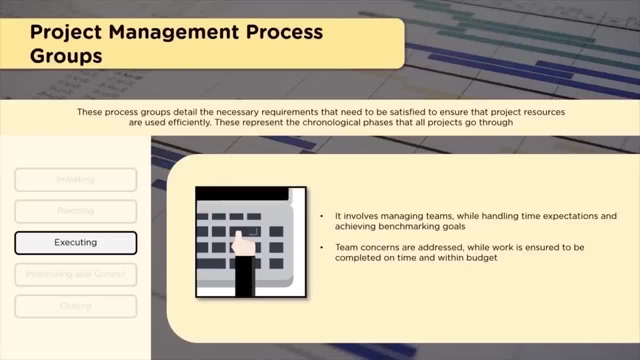 for the project, Then if it is human resource, there needs to be necessary training, development of the team and then managing them. So lot of team dynamics are involved that needs to be handled. So this involves managing teams while handling time expectations and achieving 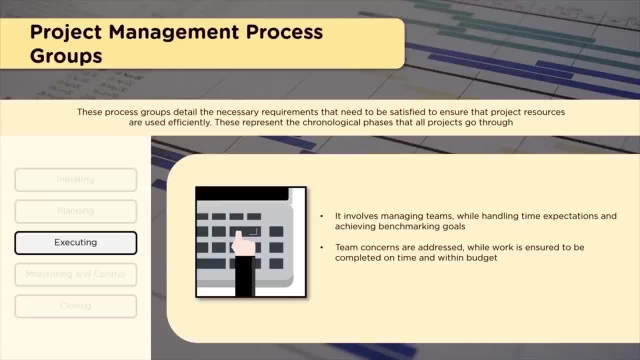 benchmark goals. Team members delivers those results. Team members does all the activities and then creates that results. So team concerns needs to be addressed because, as you see, the people together, the team members together, it is quite obvious conflict may occur. So conflict: 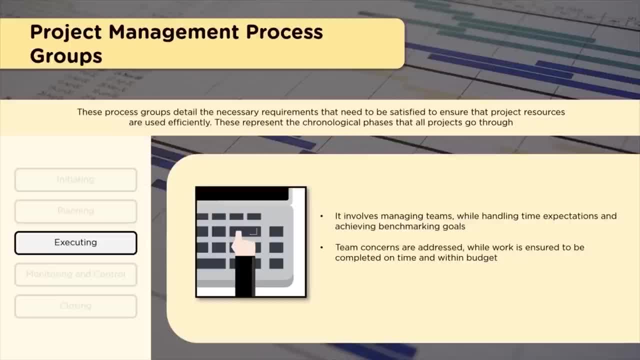 resolution should happen. The engagement with the team member should happen. So demonstration of work which is done by the project team that needs to be monitored and controlled. Parallelly, which happens during the execution, monitoring and control is also happening. So project manager should look at both. 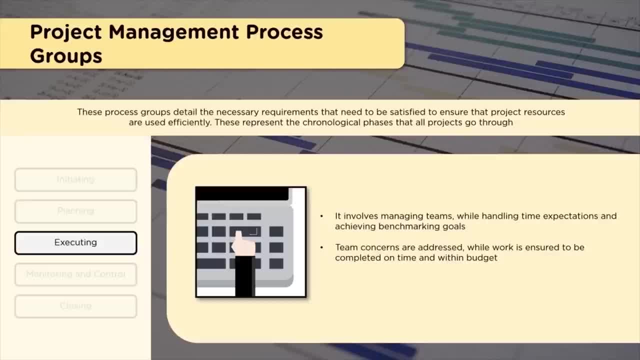 So concerns needs to be addressed. Execution- is that happening as per the plan? has to be checked as part of monitoring and control while execution is happening. So birds of view in entirety, which says how the execution should happen, that needs to be directed and monitored. 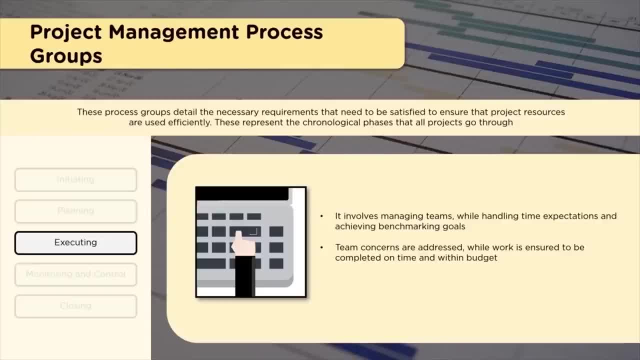 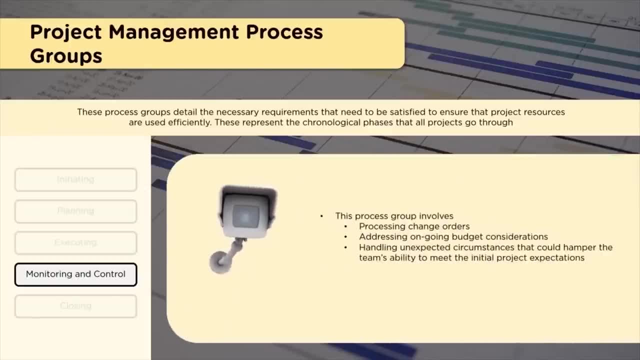 whereas coming on ground seeing, is that happening the way it is required? that is also very essential. So next is monitoring and control process group. Now, as part of these process group, as I mentioned, while execution happens, it is very essential to check, validate, 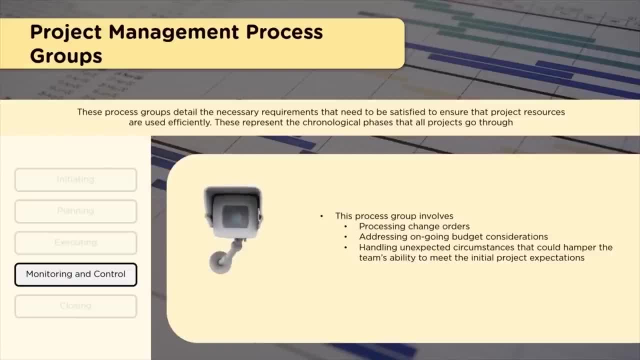 and control. So this process group involves processing change orders. Any deviations being found, change requests are raised and if that change request needs some modification or changes in planning, then it goes to planning. If no such planning requirements simple change, then it straight go to execution. 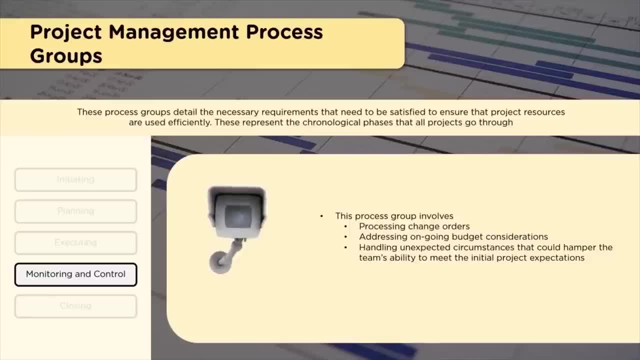 change get executed and then again validation happens. So integrated change management, which is there in this particular process group. So this also focuses on addressing ongoing budget considerations, handling unexpected circumstances that could hamper the team's ability to meet the initial project expectations. So it goes on throughout. 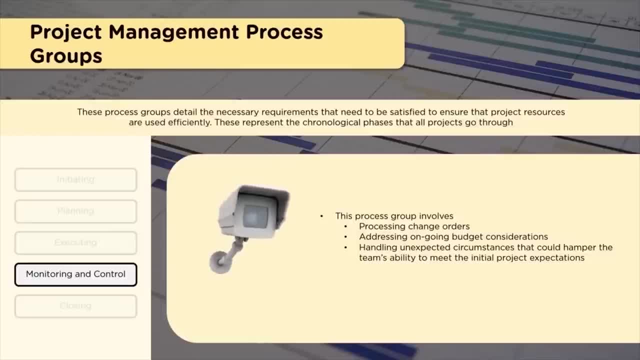 the project life cycle. So two process groups. if you closely observe, planning process groups and monitoring and control process groups are the process groups where you see processes in all the knowledge areas. Otherwise, if you see an initiating process group, it is only two process One: 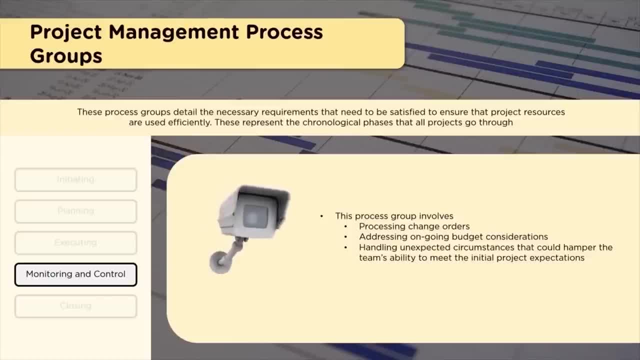 is an integration management. other one is stakeholder management. If you look at execution, you don't see in scope, time, cost and risk management. Similarly, if you see closing process group, only one process which is in initiating process group. So these are the only two. 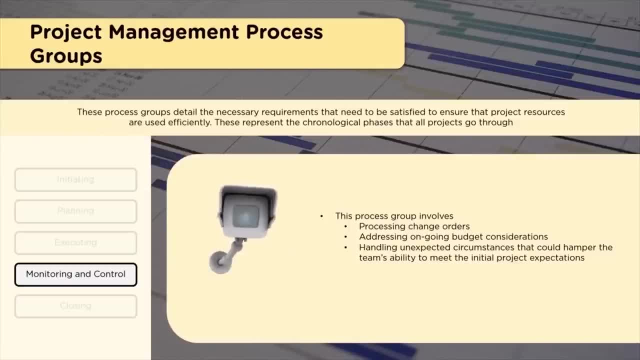 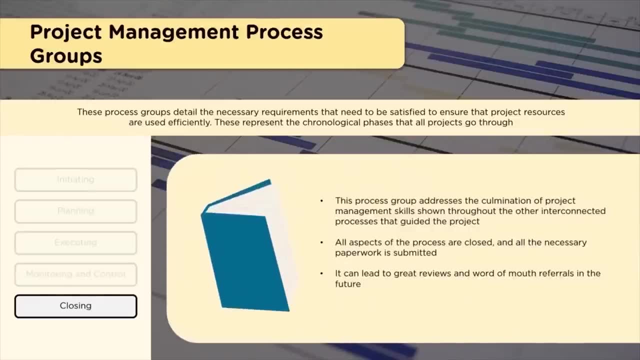 process groups, planning process groups and monitoring and control process group, where you see the most of the processes. So next process group is closing process group. So closing process group, closing project or phase, is a process. what we have in this process group, which 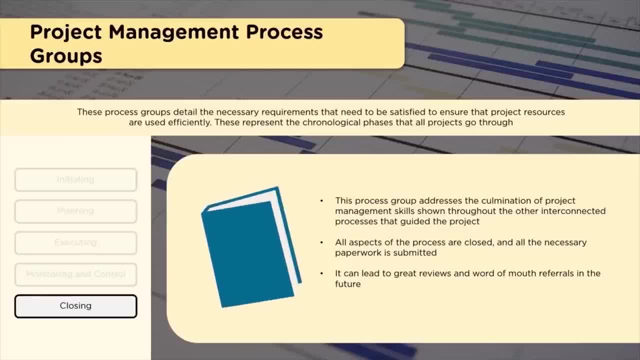 basically focuses on addressing the culmination of project management skills shown throughout the other interconnected processes that guided the projects. So all the aspects of process are closed and all the necessary paperwork is submitted. So it can lead to great reviews and word of mouth referrals in the future. 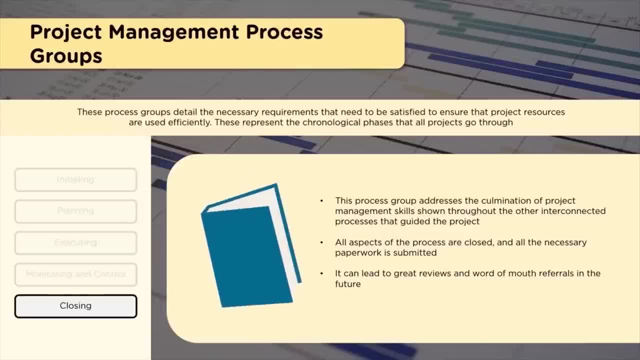 So all the activities which is to be done for formal closure and conclusion, which is done in the closing process group. So this is about all the five process groups defined in the PMP framework. So now let us move towards understanding each of the knowledge areas. 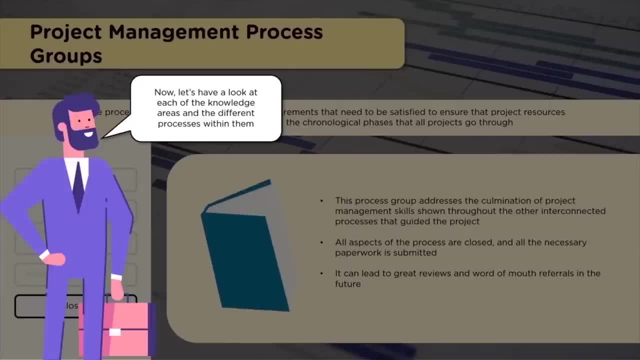 and the different processes within it. So how many processes in each of the knowledge areas, aligning with the process group we just saw in the table? but we will look at it. understand what are those exactly. So now, knowledge areas are necessary for effective. 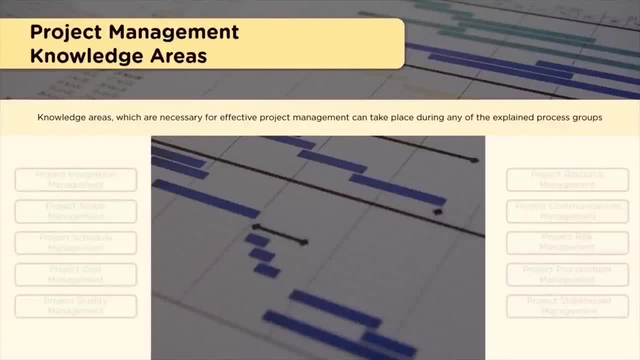 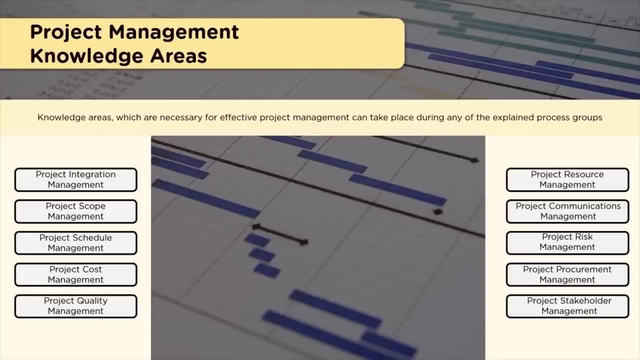 project management which can take place during any of the explained process groups. So they are ten. So those are: project integration management, project scope management, project schedule management, project cost management, project quality management, project resource management, project communication management. 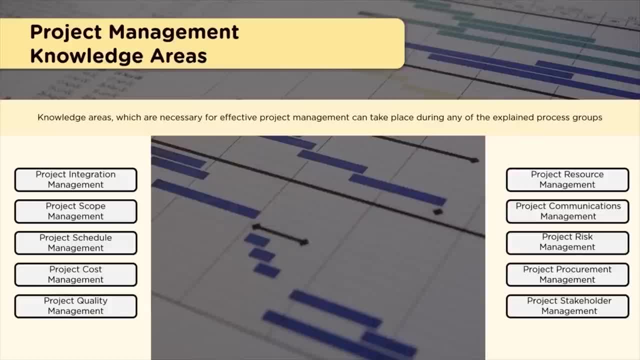 then project risk management, project procurement management, project stakeholder management. So many people ask me when I train the people. they ask me: how do we remember all of this? So remembering process group will be easy because it is the flow. 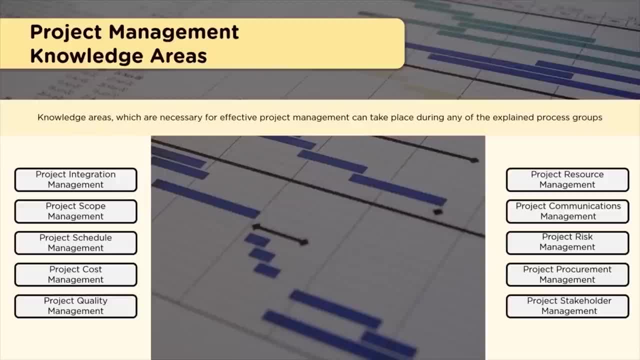 which you can remember. then remembering the process group will be easier, But to remember the knowledge areas. So one thing you should keep in mind is initially, when PMP was defined, mostly in until third edition or fourth edition, we used to focus on triple constraints. 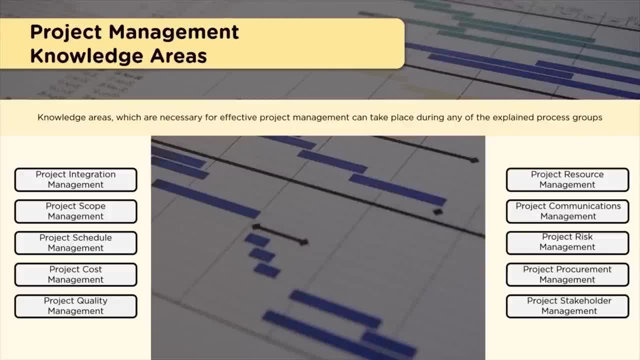 So when we say triple constraints, we used to tell scope, cost and time. Now, later, when, as the best practices evolved, as the PMBOK evolved. so it did not limit on triple constraints, it actually said six constraints. What are the six constraints? 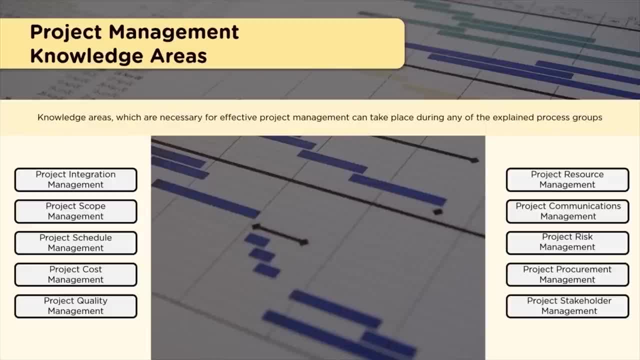 Scope, cost, time, quality, resources and risk. So, if you can able to remember the six constraints, so each of associated with each of these constraints there is a knowledge area, Like you have, project scope management, which is one of the area of constraints. 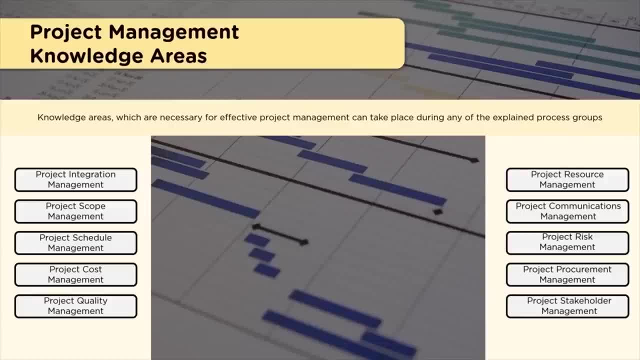 Similarly, schedule management linked to time, cost management, quality management, resource management and risk management. So out of ten easily you can able to remember six Further there are four Now. integration management by default integrates all the nine knowledge. 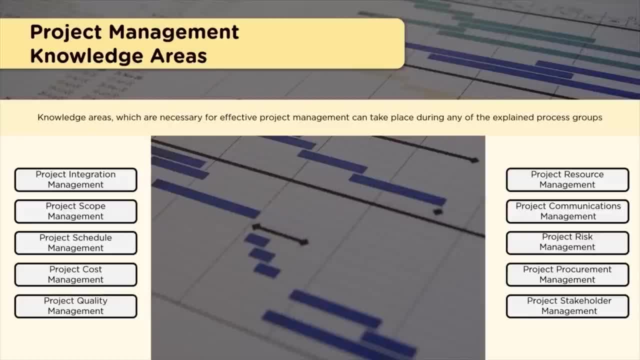 areas. So remembering that may not be difficult. So to consolidate this, to conduct the project properly, you need stakeholders, You need to procure something and you need to communicate. So other three knowledge areas: remembrance should happen by linking to this. 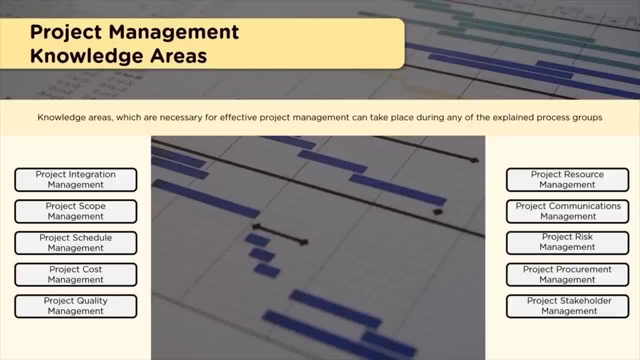 So firstly, remember six constraints, that is, scope, time, cost, quality, resource and risk. Then you have communication, which needs to happen. To communicate, there should be stakeholder and also there should be supply, which needs to happen to the project. So, if you can link like this: 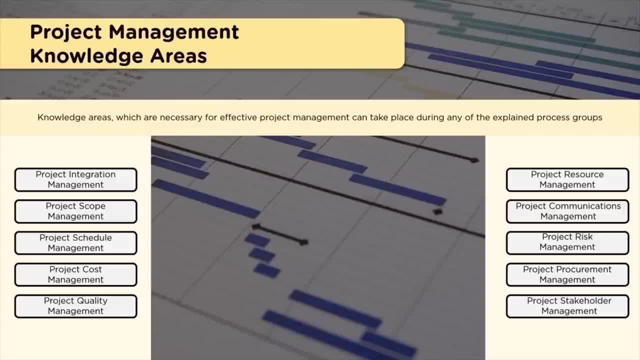 nine knowledge areas you can remember. So all these nine knowledge areas you will integrate and manage in integration management. So in fact all the plans which are defined in rest of the nine knowledge areas except integration management, So all those plans are called. 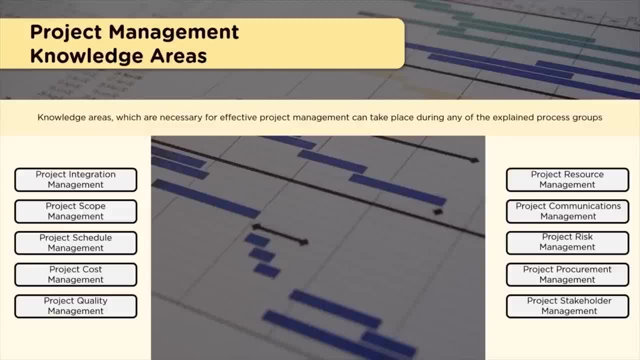 as subsidiary plans. So all these nine subsidiary plans, that is, scope management plan, schedule management plan, cost management plan, quality management plan, resource management plan, communication management plan, risk management plan, procurement management plan and stakeholder management plan. So all these. 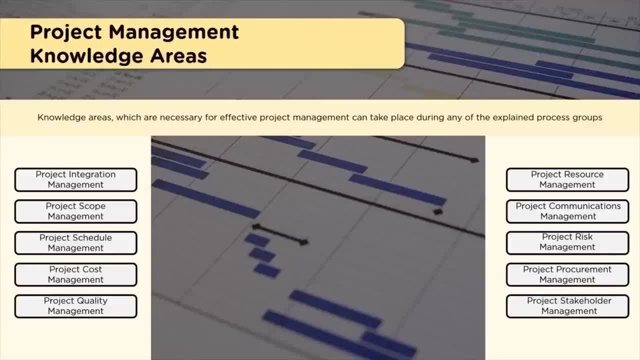 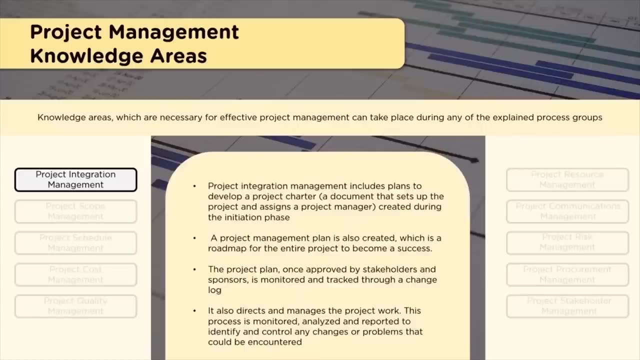 nine subsidiary plans are integrated together and consolidated in project management plan. So that happens in project integration management. So this we should keep in mind. So project integration management- what does it do? So project integration management basically includes plans to develop project. 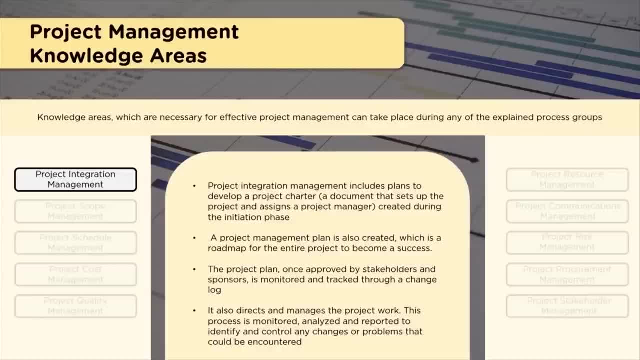 charter, a document that sets up the project and assigns the project manager created during the initiation phase. So a project management plan is also created, which is a roadmap for the entire project to become a success. So the project plan, once approved by stakeholders. 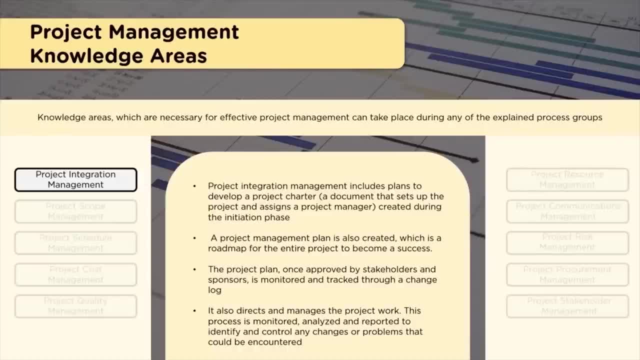 and sponsor is monitored and tracked through the change log. It also directs and manages the project work. This process is monitored, analyzed and reported to identify and control any changes or problems that could be encountered. So one thing we should keep in mind when we say: 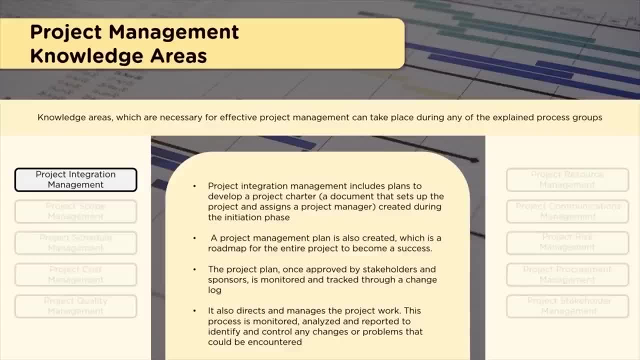 project integration management. this is the only knowledge area where we see processes in all the process groups. So we have processes in initiating process group, we have processes in planning, we have processes in execution process group, we have processes in monitoring and control process group and also. 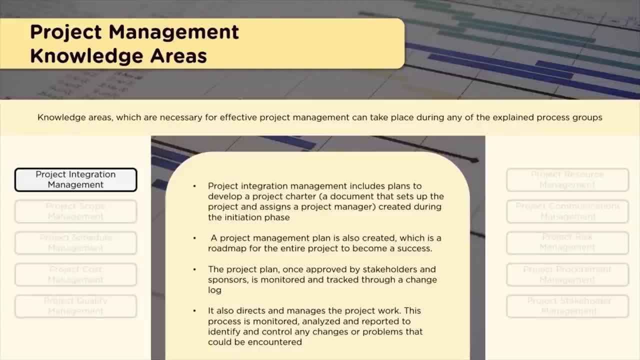 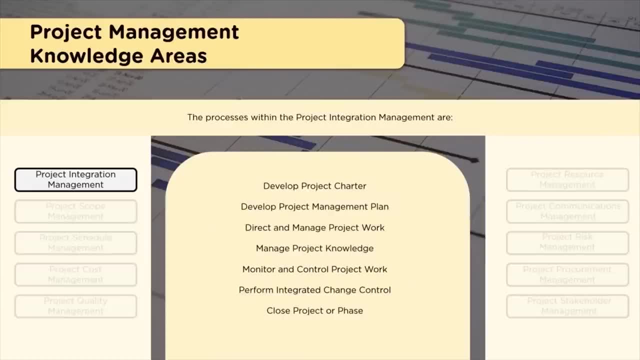 in closing process group. So project integration management is only knowledge area where it has processes in all the process groups which we don't see in any other knowledge area. Now next we will look at the list of processes like develop, project starter is in initiation process. 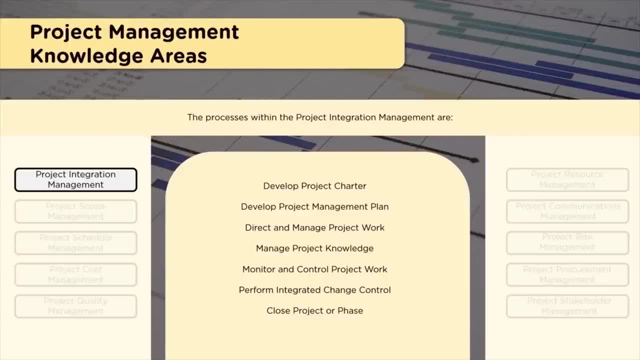 group: develop project management plan which consolidates all the nine knowledge areas is in planning. process group direct and manage project work. manage project knowledge: These two processes are in executing process group monitor and control project work. perform integrated change control: These two processes are in monitoring. 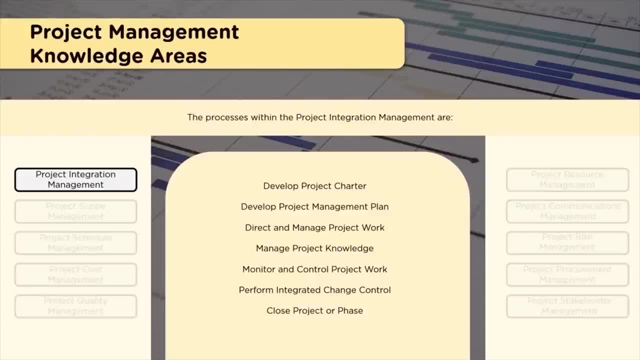 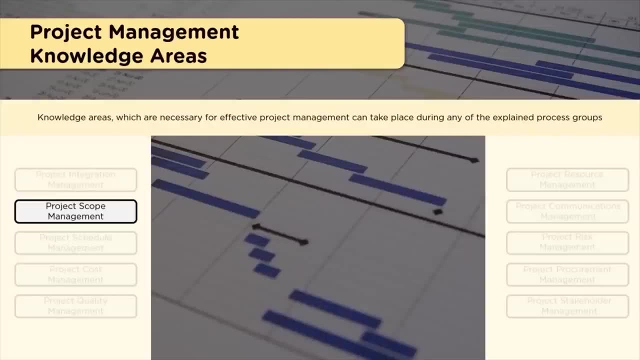 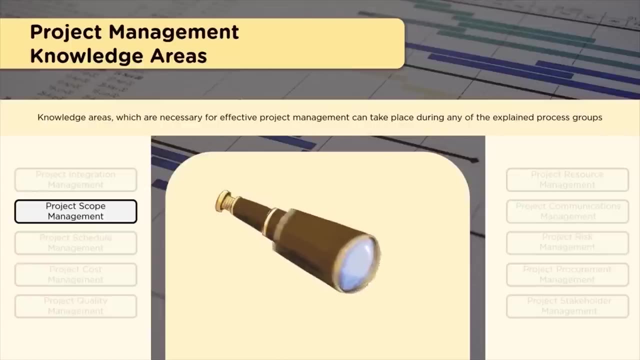 and control process group. So close project or phase is in the closing process group. So now we will move to project scope management. So when we use the term scope, the term scope refers to the boundary within which we need to do something. So first thing, we 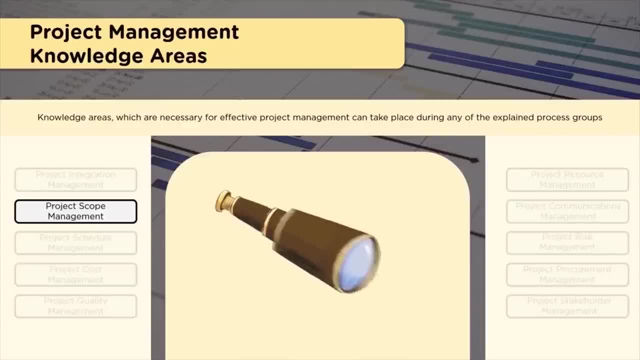 should keep in mind, when we say project scope, two things. One is the scope of that product, service or results which we are creating, which comes out as a product or a service or result out of a project, which comes out What is getting created. So 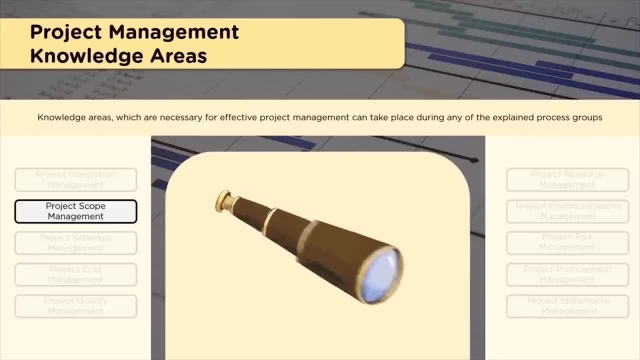 scoping that part of it. So other scope. part of it the processes, the tools, the resources, what is being used during the project so that deliverables happen. So two part of the scope we should look at. So project scope management. 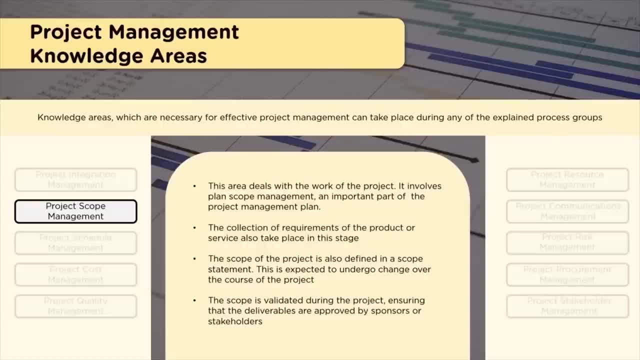 involves those areas deals with the work of the project and involves plan scope management, an important part of project management plan. The collection of requirements of the product or service also takes place in this process group and also project scope management knowledge area. deals with work of the project, which involves 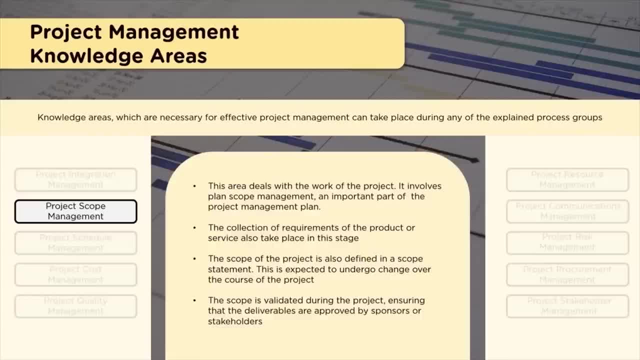 plan. scope management an important part of the project management plan, So the collection of requirements of the product or service also takes place in this stage. The scope of project is also defined in the scope statement. This is expected to undergo change over the course of project. 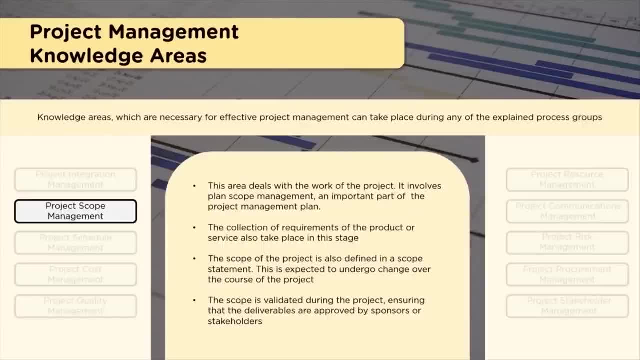 The scope is validated during the project, ensuring that the deliverables are approved by sponsors or stakeholders. So, as I mentioned earlier, it involves the scope of the results, what is being created, and also scope of those processes, resources, tools which are used during the 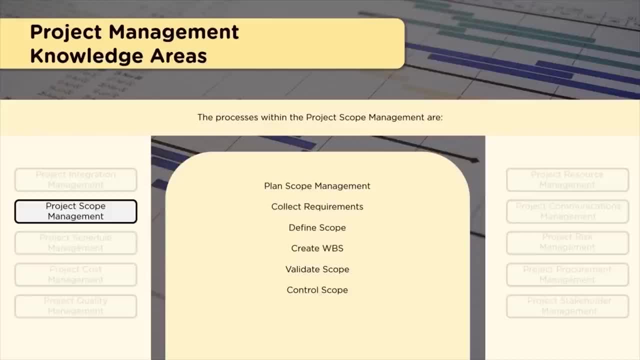 project, So processes in project: scope management, knowledge area, So plan scope management, which is in planning process group, collect requirements, define scope, create WBase. Even these three processes are in planning process group. In total four processes in planning process group. 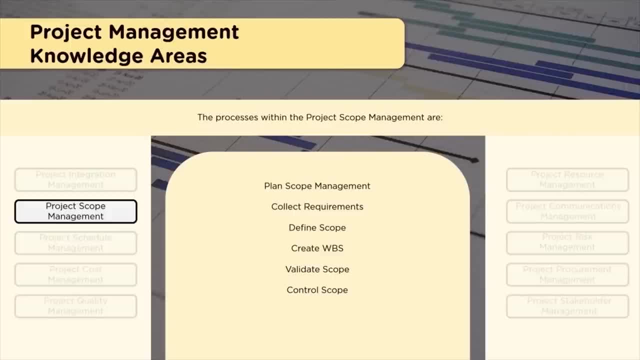 Whereas validate scope and control scope. these two processes are in monitoring and control process group. So when you say plan scope management, it's about defining how to collect the requirements, how to manage those entire scope management planning and requirements management plan also has to be defined Then. 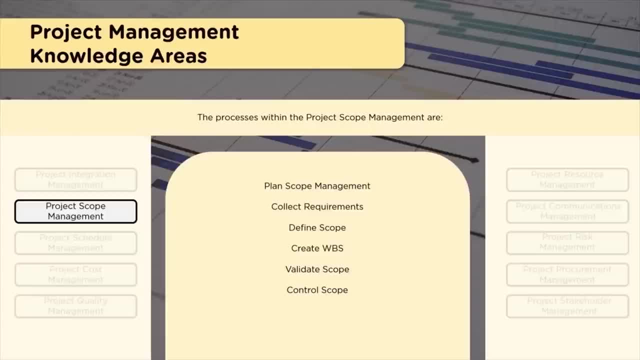 requirements are collected from the stakeholders, who are being identified, and then scope will be defined. Now, very important thing here is about work breakdown structure. So we have a product or a service or a result which we are working on to create as a result of the project. 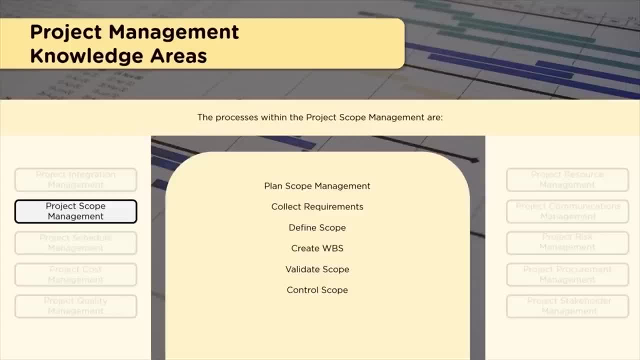 So how will you understand all the parts of it That needs breaking down, that particular product or services or results, which we are going to create into multiple pieces in a structure which would look like a tree, So that you will get a necessary insight. 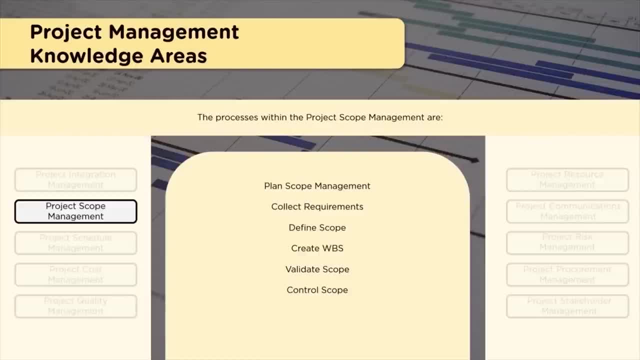 towards what is being delivered. So, firstly, product breakdown structure is made and for each of the layers of this product breakdown structure you will be assigning an activities: assigning resources, effort estimation, cost estimation, sequencing those. All this will be done later. Basic thing: 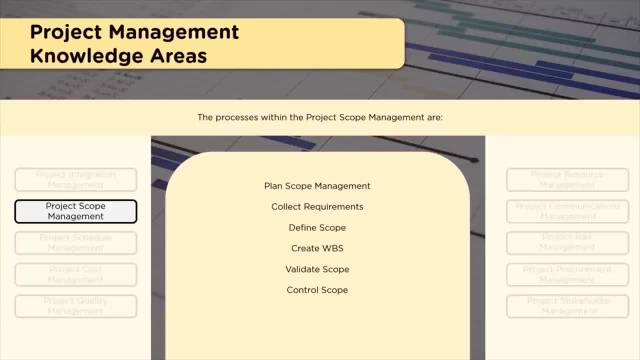 needed is work breakdown structure for that. So to create WBS, the technique called decomposition is used and this approach is top down approach. Next, validate scope and control scope, As WBS provides that structure of various things which needs to be delivered. referring to that, 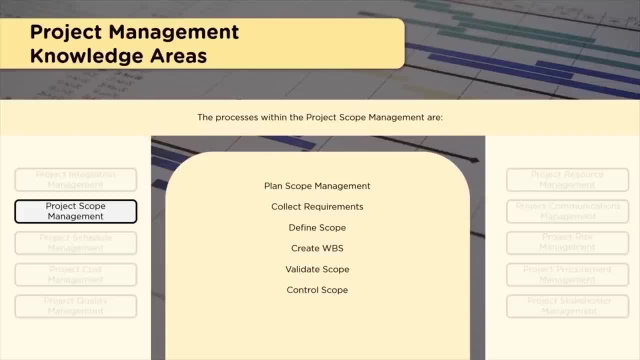 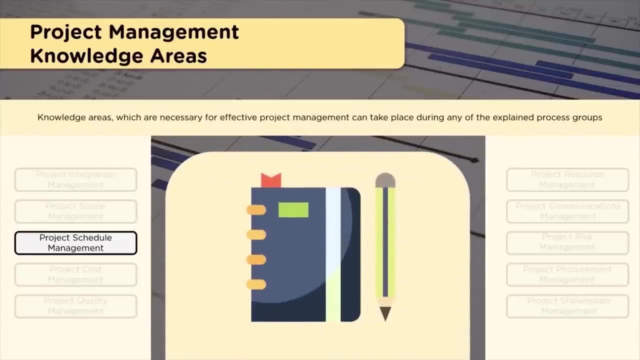 as the execution happens. validation should happen Whether it is delivered accordingly or not, And is that scope management is being done according to the plan? Control scope will be checking that. So next is the project schedule management. When we say schedule, it's quite obvious. 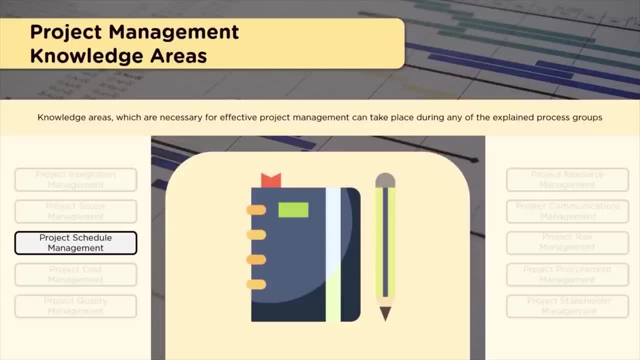 for us to understand when what needs to be done. So what needs to be done is already told in scope. and when are we going to do that? For that you need to have a specific schedule, the timeline So the project will have. 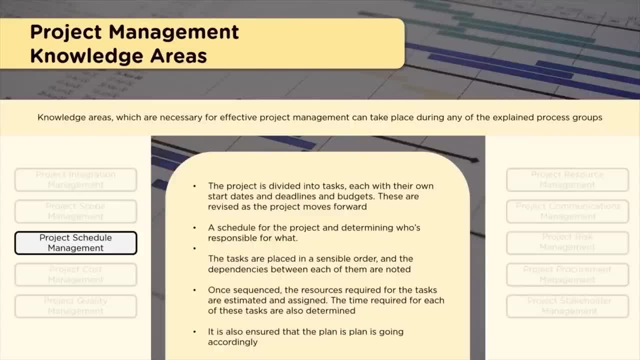 various different activities, tasks which is assigned to the particular WBS element. So these activities will have a specific start date, end date and this will have a specific output which is coming out as part of those actions which happens. So the project is divided into. 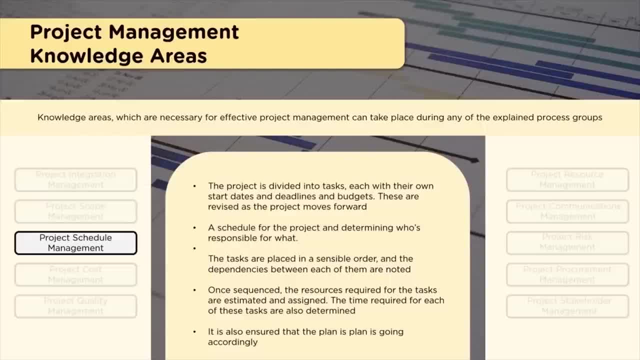 tasks, each with their own start dates and deadlines and budgets, So these are revised as the project moves forward, depending on how the project is progressing. A schedule for the project and determining who is responsible for that So helps us to understand which resource 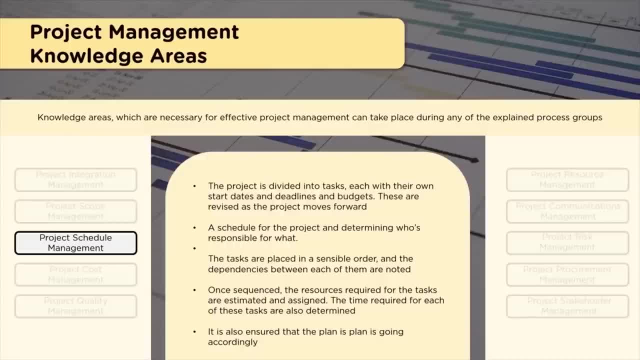 is required at what point in time. Similarly, the cash flow requirement can also be understood by having a defined schedule, So the tasks are placed in a sensible order and the dependencies between each of them are noted, Once sequenced the resources required for the tasks. 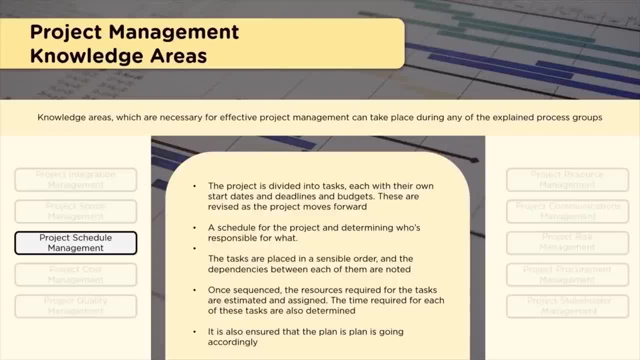 are estimated and assigned. The time required for each of these tasks are also determined. Now, when we say this, we are required to understand and visualize, while doing a project. the WBS structure is defined and in what sequence each of these elements are. 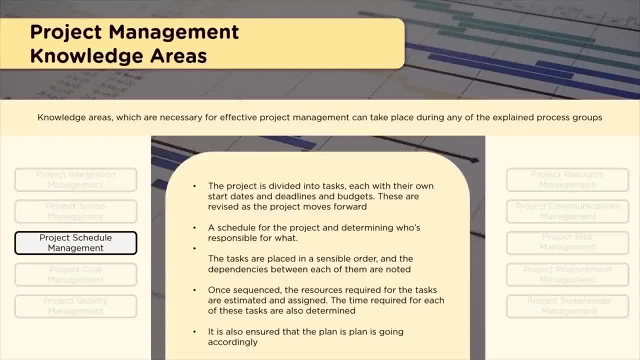 delivered and what timeline- start time, end time- and how each of these are connected to other WBS elements, In what sequence What activities required, What resource required, What effort required, What competency skill required. So all these are put in. So, since we schedule, 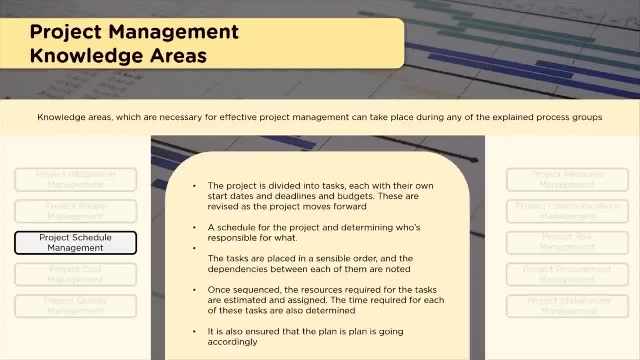 and sequence it. we know when is that required. So this requires working with other knowledge area very closely. When I say WBS element, it's quite obvious it comes from scope management. When I say allocation of resources, obviously it has to work with resource. 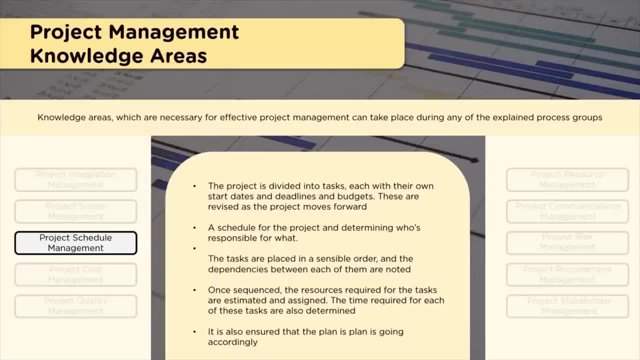 management to create a resource calendar. If it's a cost management, to understand the flow, money flow, cash flow. So budget should be there for the project. So cash flow when what amount is required to understand that cost is linked to schedule. 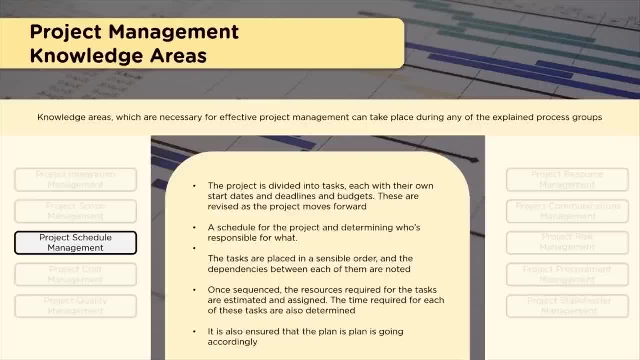 So all these knowledge areas should work very closely, With coordinating with each other, Interfacing with each other. So project schedule management also uses an very important technique called network analysis technique, where we speak about critical path, then forward pass. 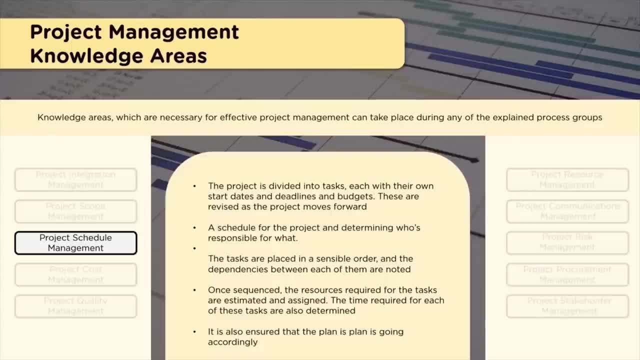 backward pass, then identification of floats. So when I say critical path, critical path refers to the longest path in the established network diagram of a project And that will be the minimum time required for project to complete. So this critical path needs to be closely monitored. 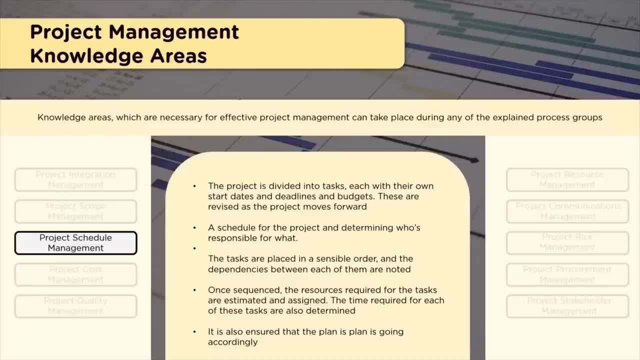 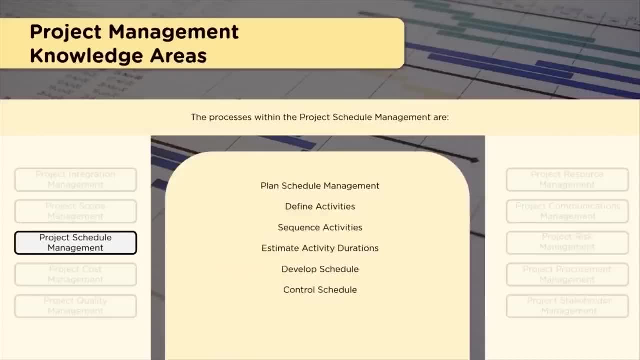 as the execution of the project happens, Because any delay in this critical path will delay the project itself. So that's about some summary about schedule management. Now let us look at the processes which are involved in schedule management. So plan, schedule management. 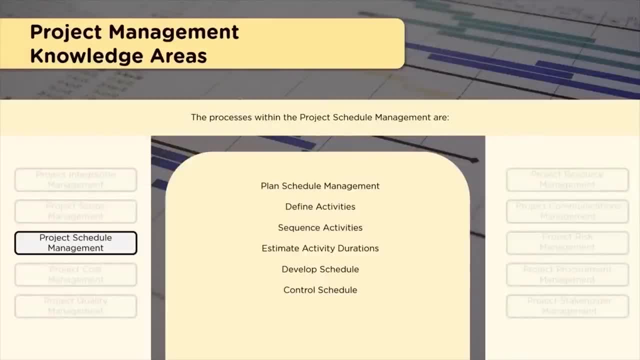 define activities, sequence activities, estimate activity durations, develop schedule. So all these five processes are in planning process group. So schedule management, how it has to be done, needs to be clearly planned as part of plan schedule management. Then, when to define activities, 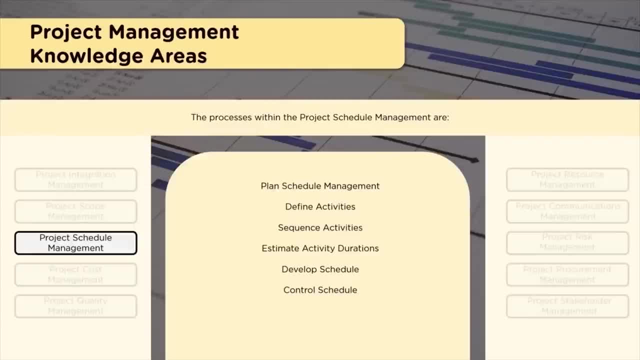 it is quite obvious we need to know what needs to be delivered. So WBS element helps us When the scope baseline is provided as an input here, so taking that activities are defined, Then the sequencing happens. Then when we say estimate. 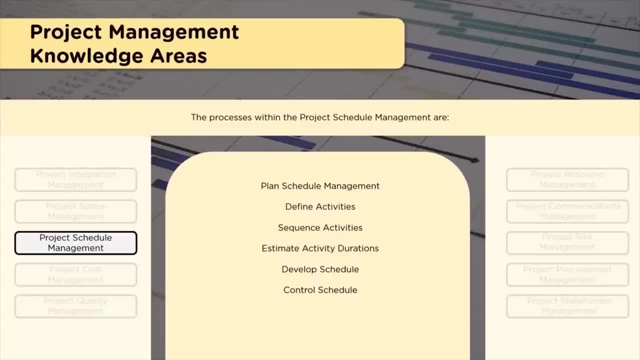 activity durations. so we speak about two terms like effort and duration. If I want to deliver something- let me assume to deliver X for a person, it requires one day. Or for a person, it requires 10 days. if we say: 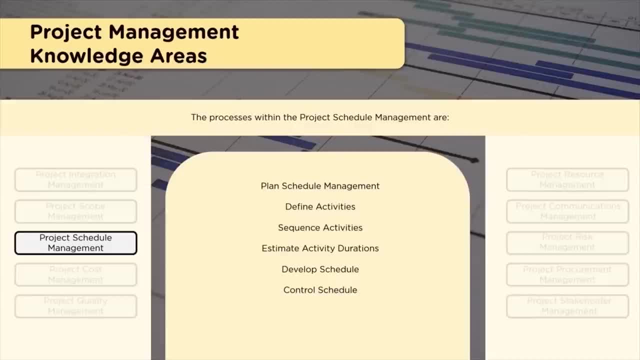 So to create that working piece of a product it takes 10 man days. we will say, That is an effort. Now, if I have 100 pieces of such needs to be created, how many man days I need? So 10 into. 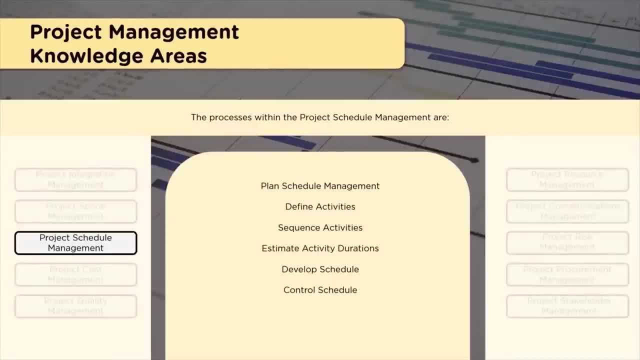 100 piece 10 days into 100 piece, So 1000 man days. Now how many resources I have? I may have around 25 resources Now, 1000 divided by 25. It will be around 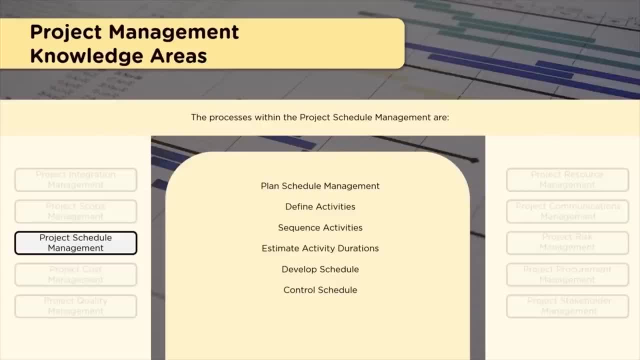 I guess 400.. 400 man days? No, I think 1000 divided by it's about 4. 40. So 40 man days of effort, That is duration, Whereas effort is 1000 man days. 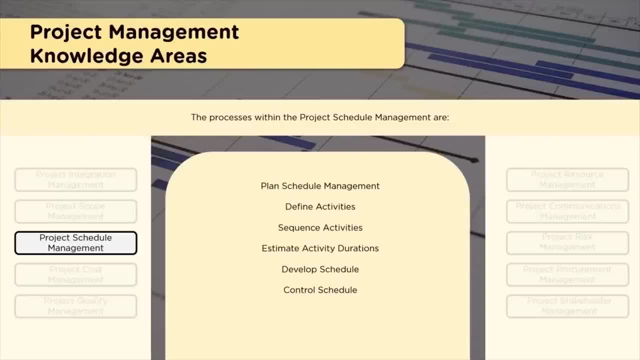 40 days will become duration. So, likewise, looking at how many resources we have, how many, what is that effort is actually required, It is involved, And then what is the duration within which we need to complete it, Either 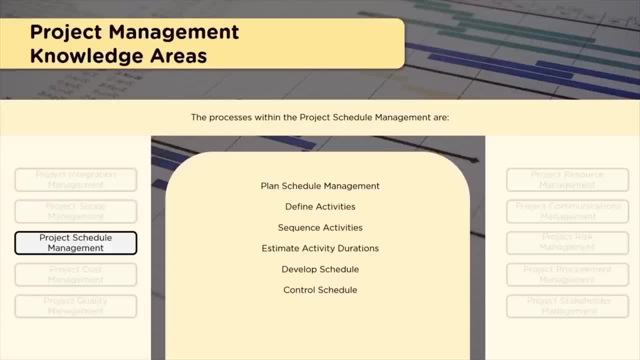 you look at how many resources I have. Based on that, I will look at the duration Or I will look at the target date. Mainly, target date is given by customers, as we discussed, When the project needs to be completed. 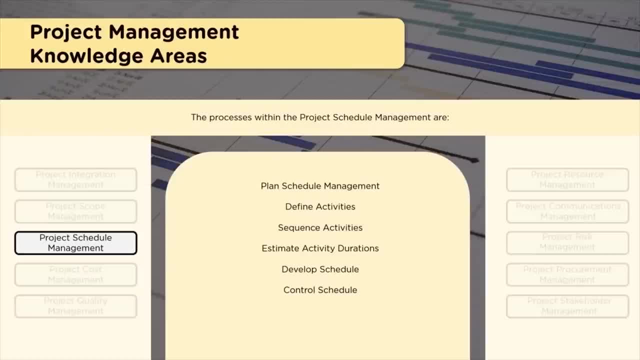 Accordingly, we are required to acquire the resources. So this itself is showing us: these knowledge areas now work very closely. Now, without scope, you cannot define activities. Now, without understanding the activities, you don't know what is the effort. So now, once you. 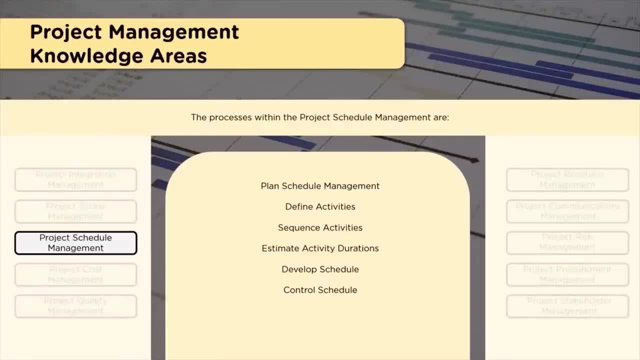 understood the effort. you know what resource, what competency, when. So you need to work with resource management. So to have those resources onboarded or acquired you need to have money cost. So what cost it takes. So likewise it goes. 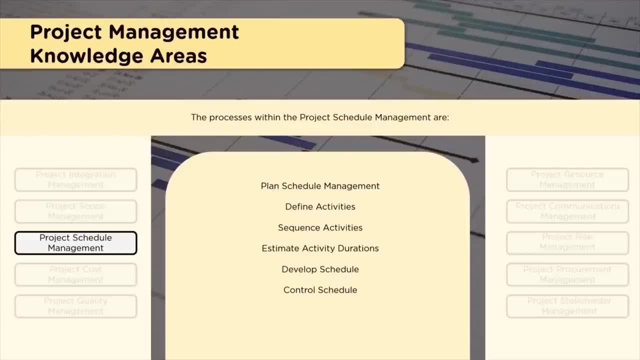 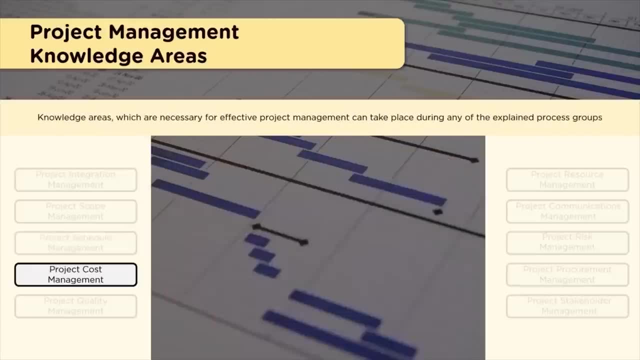 one by one elaborating. That's why you see 24 processes in the planning process group distributed across all the 10 knowledge areas. So this is about schedule management. Now I will look at the cost management Project cost management. So when we say 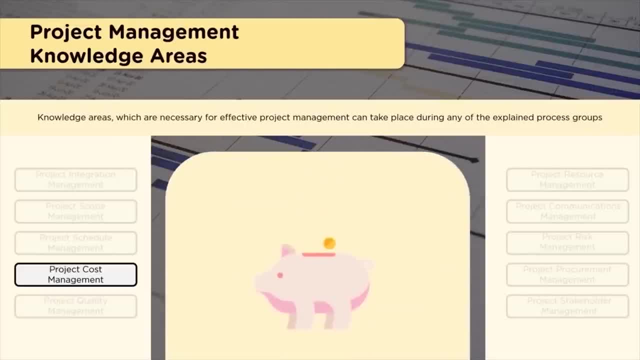 cost. it is quite obvious. it's all about money, What money, The expenditure, the outgoing money. So project incurs cost, If any individuals. I keep getting these questions in lot of trainings. So is checking the revenues? 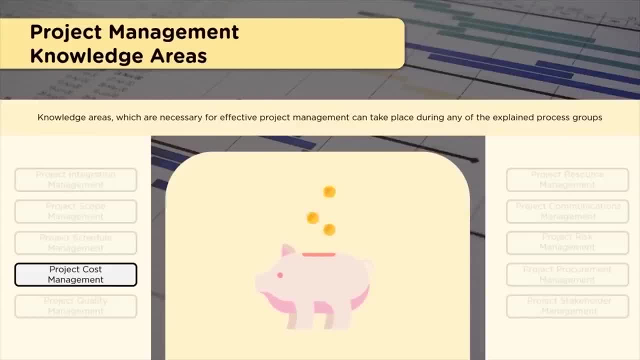 the invoice raising and collection of payment. is that a job of a project manager? Now, when we say the project management and look at it as a project management activities, Now it's all about delivering the results of the project. So when we say 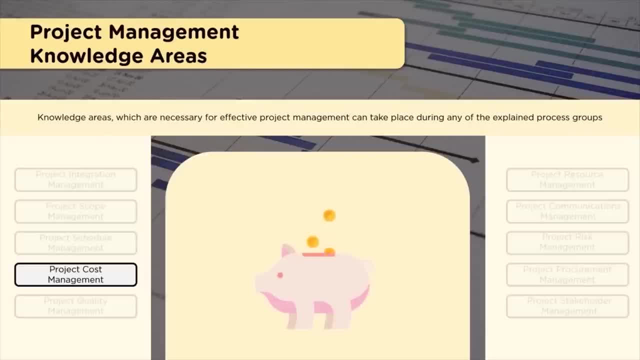 I need to collect invoices and to submit invoices, collect payments. when you say that, So that doesn't mean it is part of a project management role. No, Now, if in your organization, if you have a designation of project manager or some manager or something, 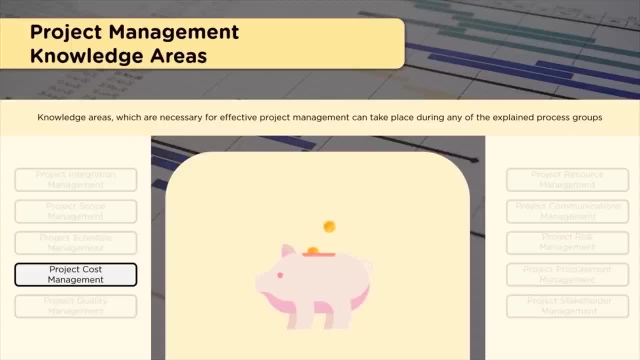 and invoice, submission and collection of payment is also part of your job description. you have to do, You don't have any choice. So designation is totally different when compared with the meaning of the role called project manager, So any other things which are associated with. 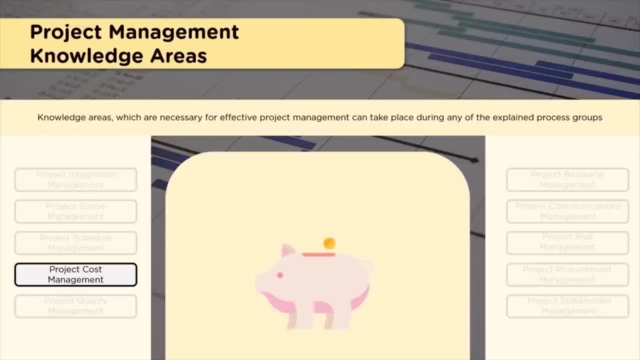 your designation in the organization. It may be project manager also designation possible Depending on what job description, what job activities are associated with it. accordingly, you have to do. But when you do a project management activity, in specific when you involve in the project, 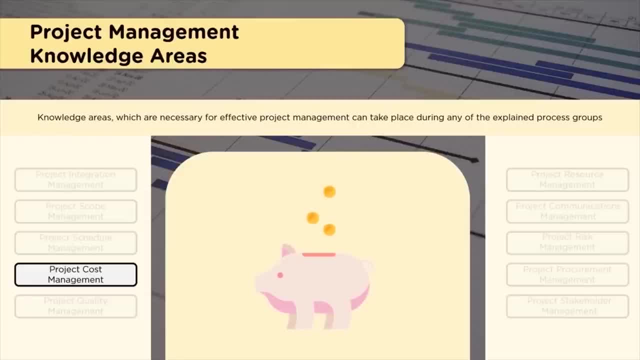 So all these aspects, what we are defining, that needs to be taken care 100%, Along with that raising an invoice, collection of payment or coordinating with some other department to find out new opportunities in the existing customer, Those are all additional things which are 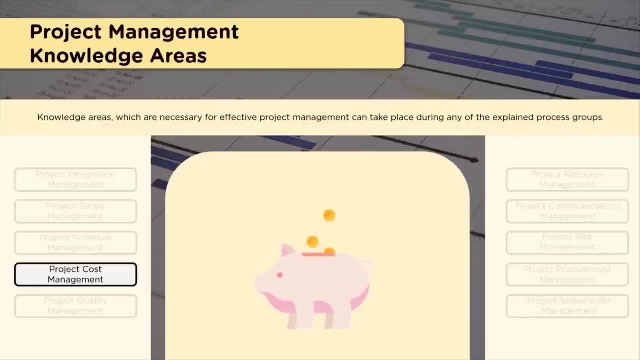 given to you as an individual with that designation to justify many things. So as a professionals, I have a position in organization with some designations and there is a CTC salary which is given and that needs to be justified To justify that various different 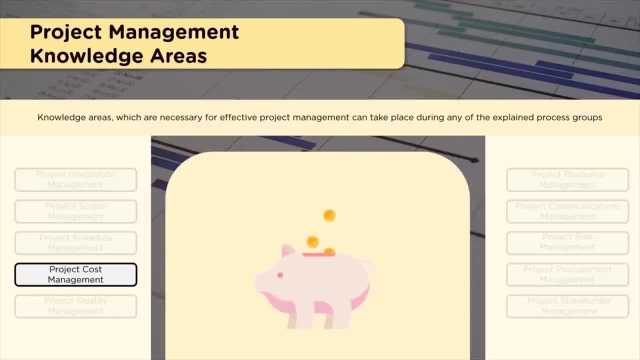 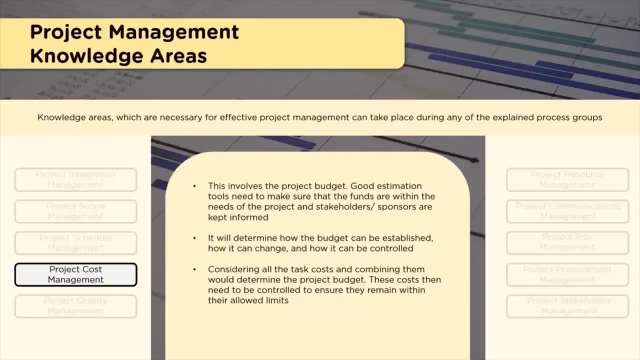 roles are attached to you for your designation, So that you need to look up to Accordingly you need to deal with. Now let us come back to project cost management. So it's about expending money, what we are speaking about, Which, basically? 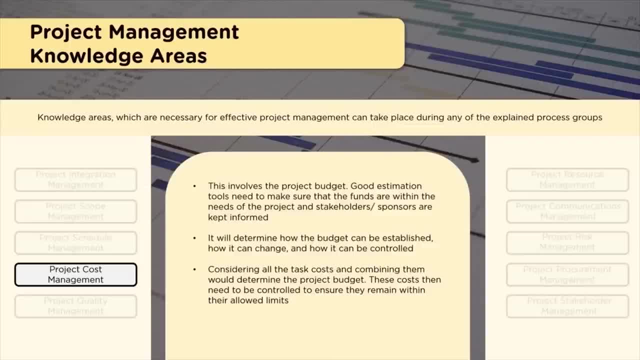 focuses on estimating and allocation of budget to the project. That is first thing. One needs to estimate, approximate what cost it takes for a project. Now, what are those cost components? So where is that cost incurred? So, cost is incurred. 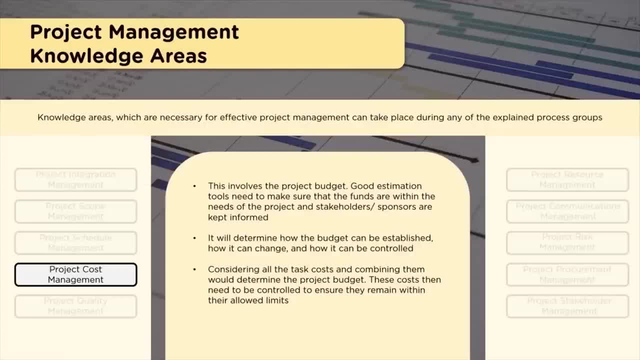 to the resources acquired. Cost is incurred to the tools. Cost is incurred in all that activity. what we do Right, So everywhere, the one we create a result for raw material, what you acquire, The people, the technology resource, what you acquire. 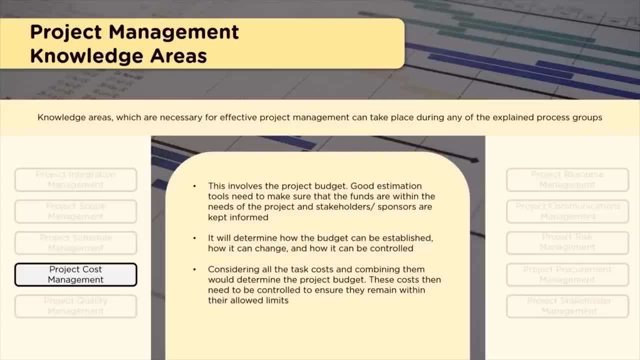 the facility, what you have. So all this involves money, the cost expenditure. So approximation of the cost needs to be done, What it takes to complete this project and confirm budget it. So this involves project budgeting, So good estimation tools need to. 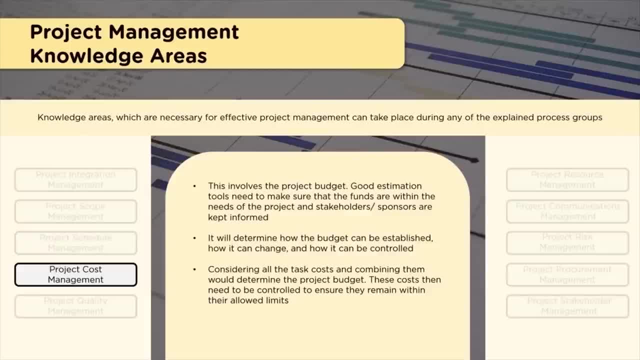 make sure that the funds are within the need of the project and stakeholder sponsors are kept informed. So estimation and budgeting cannot happen in isolation. Project manager cannot do alone. It requires to involve the experts, the divine experts, who can determine how the budget can be established. 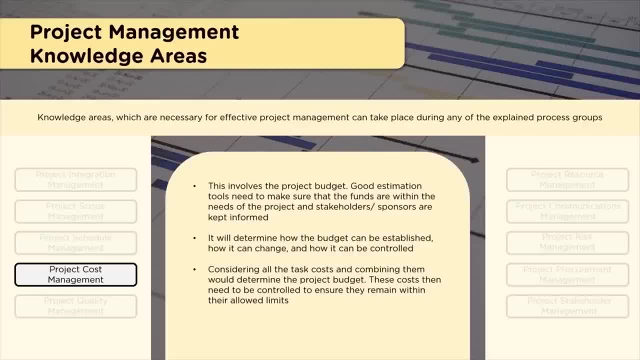 how it can change, how it can be controlled, what are the regulators needs to be kept in mind. So it considers all those processes required to do that, All the tasks which are involved, like cost, and combining them would determine project budget. So, firstly, 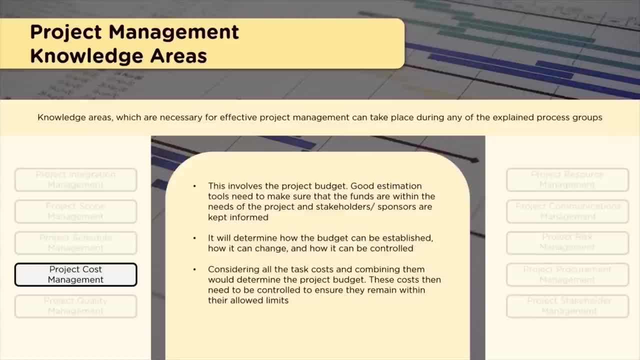 approximation would happen. Based on that approximation, then the approximation of that will be submitted. Then the budget is confirmed after allocation. So this needs to be monitored and controlled throughout the project life cycle. So initially, I also mentioned earlier about triple constraints. 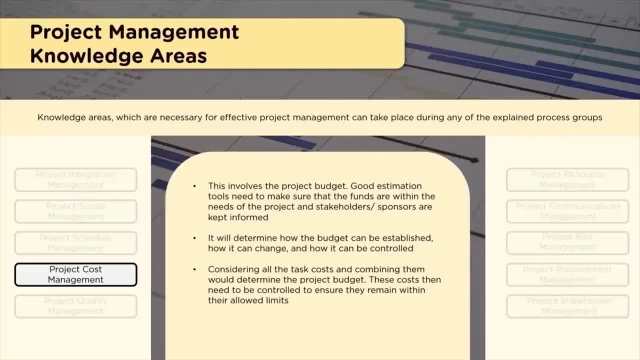 scope, time and cost. So it is very important to monitor these three critically. So for that, there is a technique which is used, which is very popular: earned value management, Which speaks about or provides you the insight towards how the project is progressing. 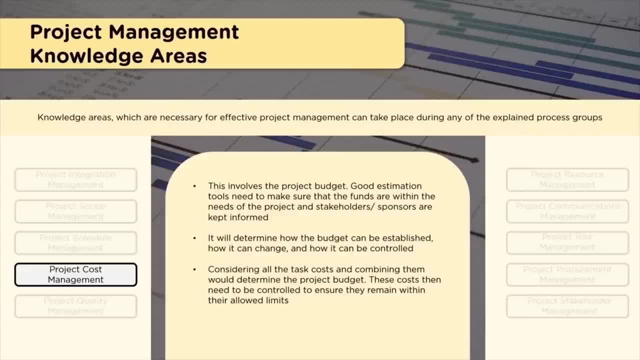 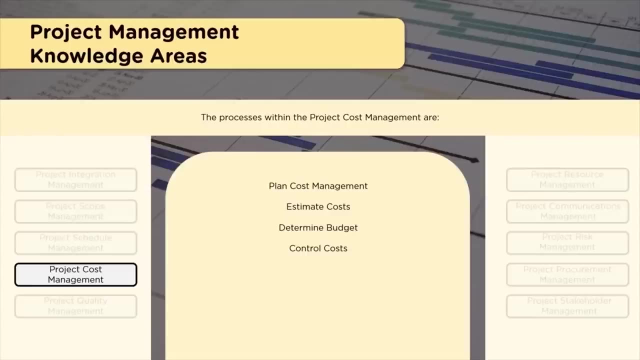 in terms of scope, time and cost, Which are basically very important ones. Then comes rest of the things: quality, resource, risk, which complements to this. So project cost management involves four processes, that is, planned cost management, estimate, cost determine. 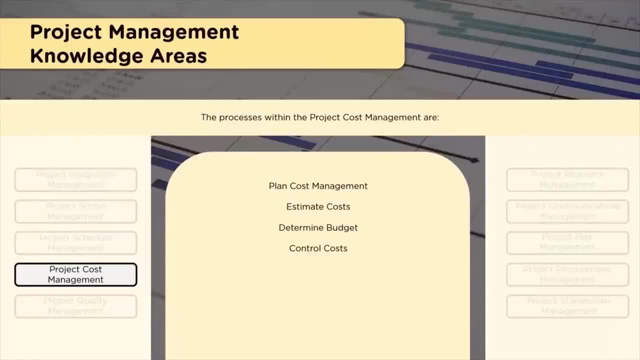 budget, which are part of planning process group, and control cost is part of monitoring and control process group. Now, next knowledge area is project quality management. So when we say quality, it is all about ensuring that rates are set, requirements are clearly. 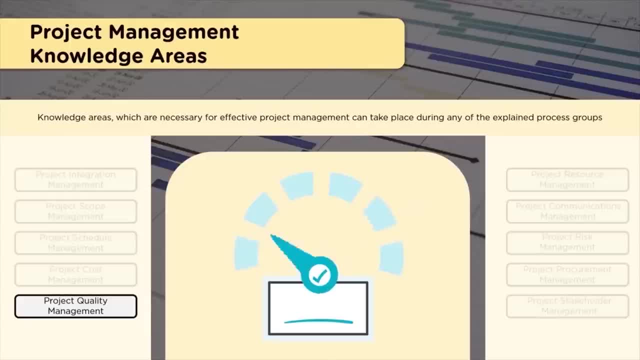 defined and how are you going to ensure that inherent characteristics- what are defined- are accomplished? So you need to have a quality management approach, quality management plan in place. Now what quality management I should follow? There are lot of standards, lot of best. 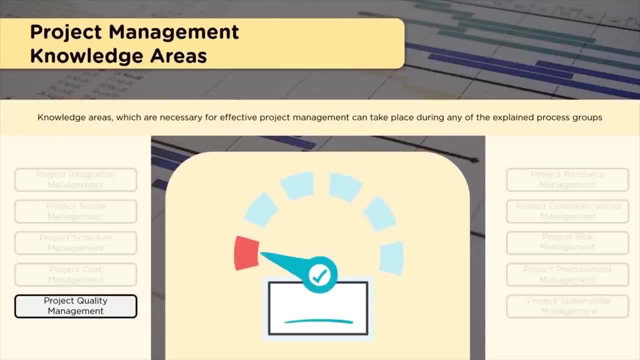 practices. So that is based on the project environment in which organization are you doing. In any given organization, there will be quality management practices which are followed and approach that may require to get reflected in the projects which is being done in that environment or 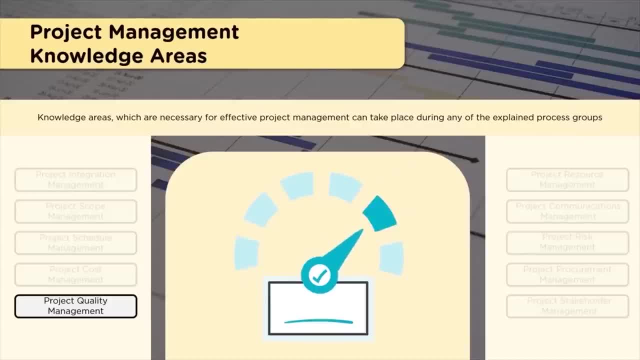 if project has a specific requirement that specific quality management standard or practice needs to be followed, then that needs to be defined. Accordingly, the quality management should happen. So quality management is a part of entire project management plan, which speaks about quality specifications, products or 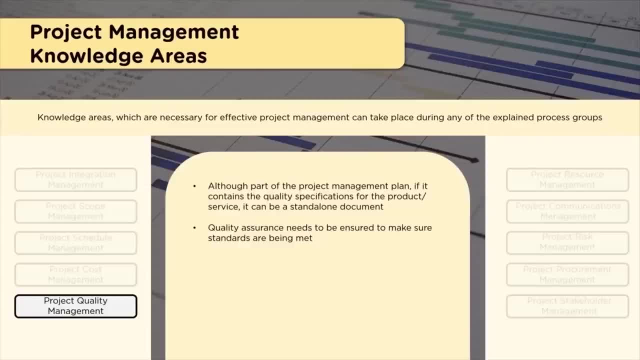 service, the artifacts which are used as part of the project. So when we say quality management approach, we speak about many terms like acceptance criteria, quality criteria, customer quality expectations, then quality assurance, quality control. So all these needs to be kept in mind. 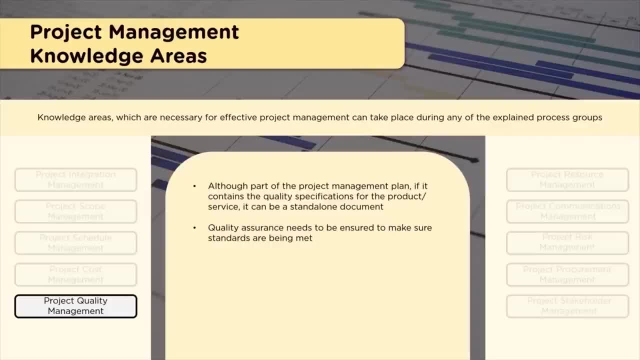 and brought in place, And this in execution. if you look at, there is a process called manage quality. When we looked at scope, schedule and cost, there was no processes defined in execution. But since the accountability of ensuring quality is with project manager, 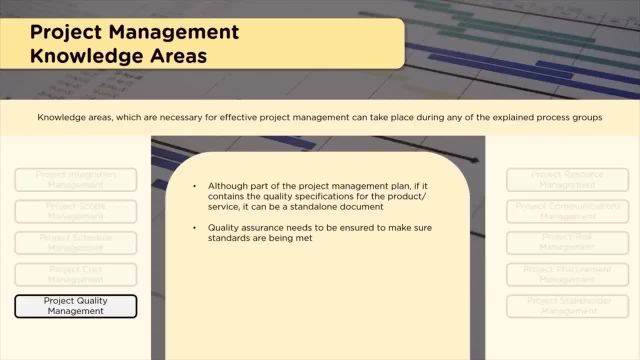 there is a process. Now remember: all these 49 processes defined in PMP are project management processes. These are not the processes which are for execution. So these are all project management processes. If any team member is configuring something, creating something, delivering something, 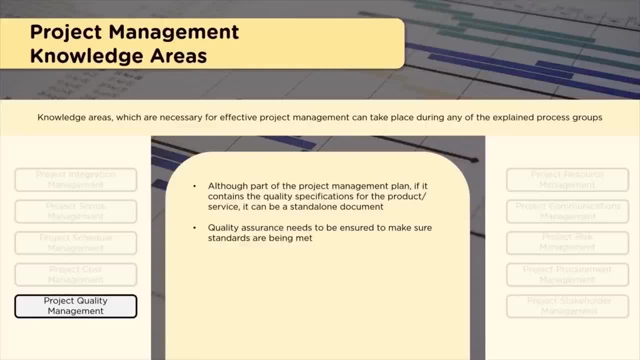 none of those activities are defined as part of these processes, As plan. when you make a clear plan, like when I said, create WBS, where you have the elements which needs to be delivered are defined, When you putting an activities into it, adding activities into it, that anyway. 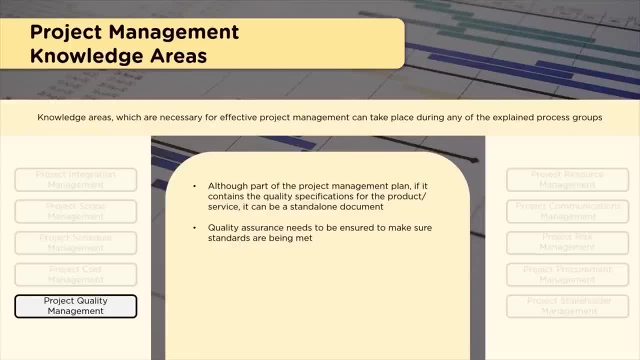 you have a domain expert to do it. Accordingly, execution happens by team members, But as a project manager you are not involved in that in entirety, In execution. I am saying So. project quality management will have the processes like plan quality management. 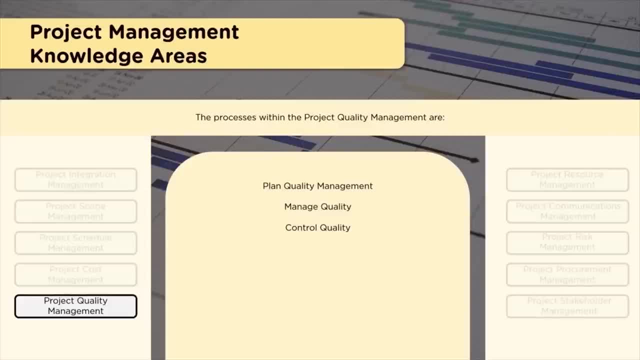 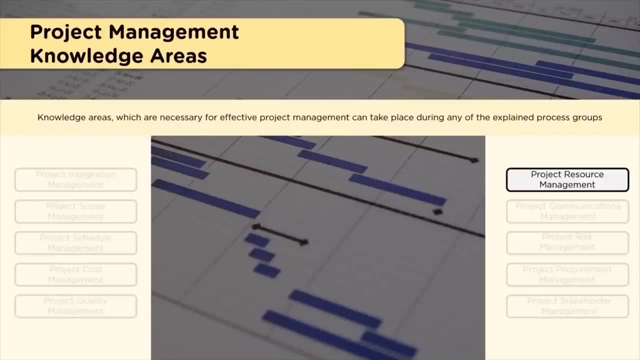 manage quality and control quality. So plan quality management is part of planning process group, Manage quality is part of executing process group, Whereas control quality is part of monitoring and controlling process group. So the next knowledge area to look at is project resource management. 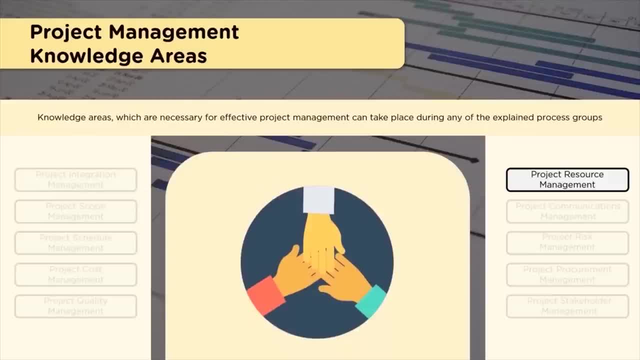 So when we say resource, by default we think about human resources. So that's how the knowledge area was in the fifth edition. So it was called as project human resource management. But as the discussions happened, as the realization happened, 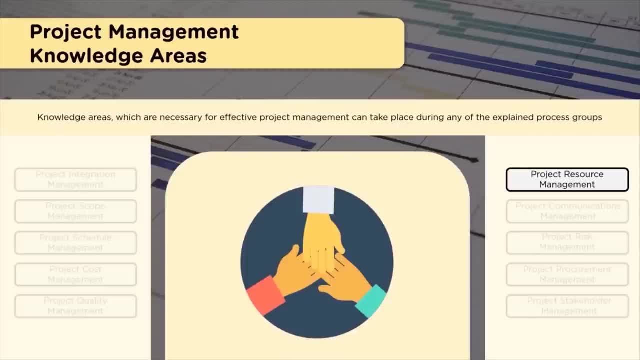 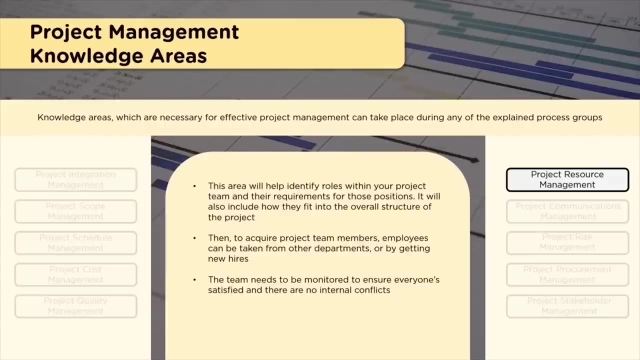 it is not about just human resource. many resources involves Technology resources, facility resources. so the renaming of that knowledge area happened in sixth edition as project resource management. So project resource management focuses on ensuring identification of those roles, Identification of those resources. 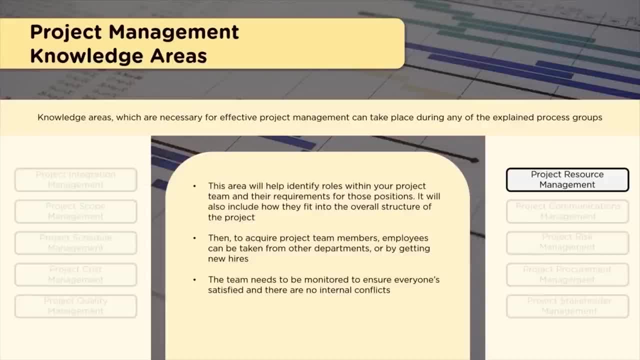 Having a plan in place so that resources can be managed better. So, predominantly, when we say resource, it's quite obvious we think about human resources, So which is very, very unpredictable kind of resource, Whereas when it comes to technology resource, 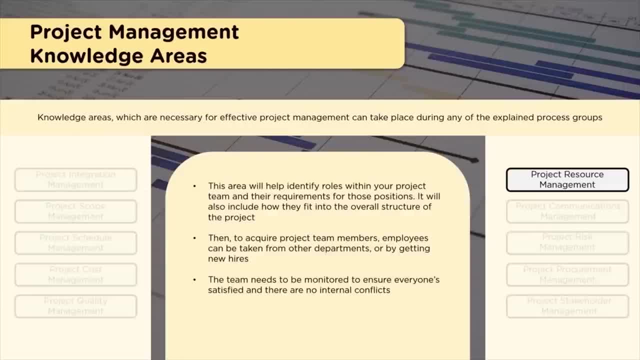 it is predictable. The nature, the behavior, the configuration, everything is predictable. But only those human resources are the one which requires a special treatment, a special approach to engage with them. So this knowledge area helps to identify roles within the project team as per the project. 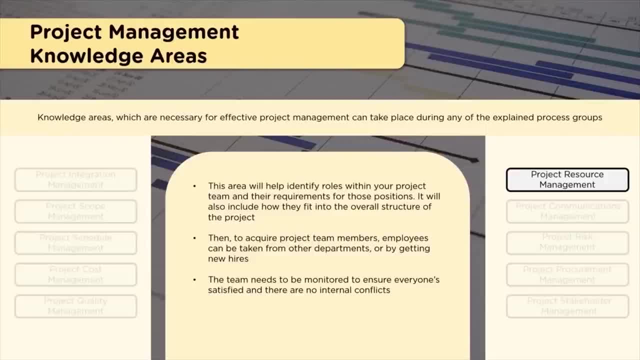 management team structure defined. So there should be project management team structure defined And what needs to be delivered from which are the roles, which also include how they fit into overall structure of the project. So these team members or resources needs to be acquired. 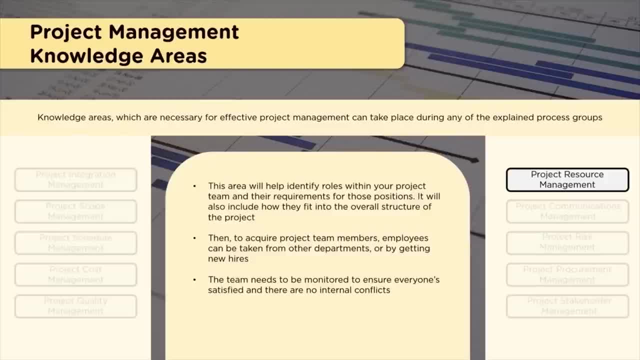 If it is human resources, those needs to be educated and induction needs to be done about the project And they needs to become fit into the project. So when I say people, it's quite obvious conflict occurs, various different preferences they come across with. 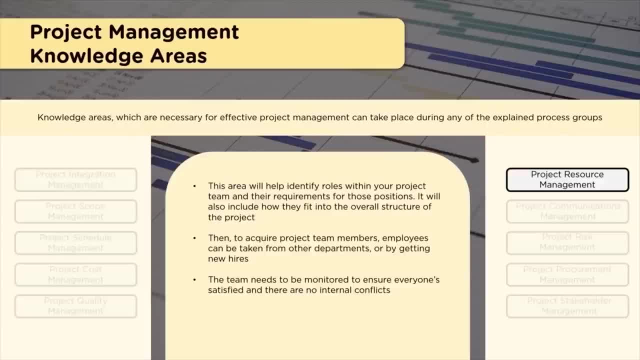 They have their own experience, backgrounds and dynamics associated with them. So close monitoring is required, mentoring is required, demonstration of leadership skills are required. So, generally, we speak about three main ways of demonstrating leadership, which involves authoritarian leadership, then lazy fare leadership. 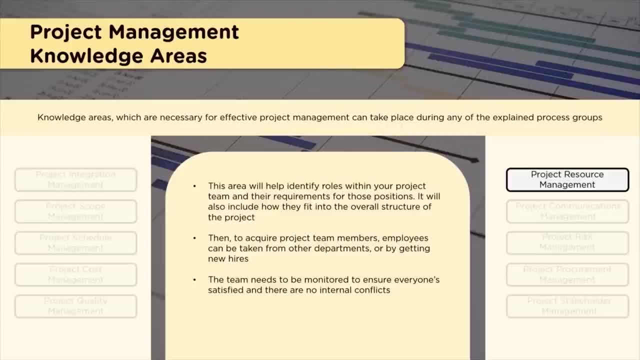 and participative leadership. So authoritarian is also called as autocratic, which means the project manager will become hold that authority power. with that power the project manager demonstrate this is how it should be makes the decision, So such power demonstration may be required. 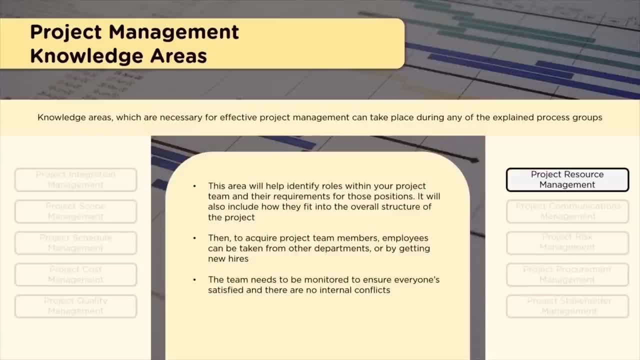 when something needs to be influenced strongly and direction needs to be set and decision needs to be made. But when it comes to participative leadership, when some problems needs to be resolved, when people's involvement is required, that needs to be increased. that is very essential. 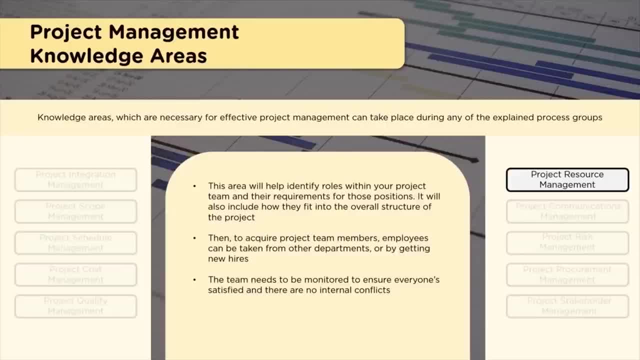 Reviewing or creating solutions. that approach, leadership style, is required. But when it comes to lazy fare, delegative approach. so where there are specific domain experts who will do it, so assign to them and then monitor review with them. that is delegative approach. So these 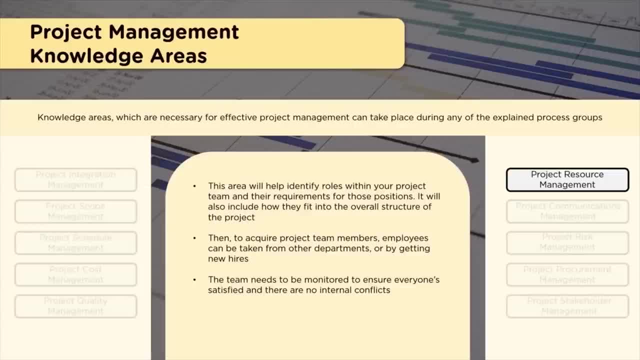 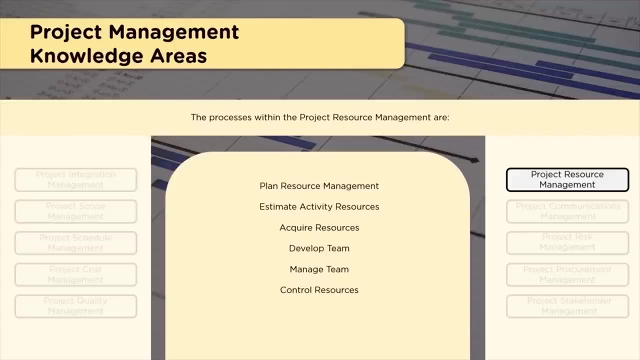 three leadership styles has to be demonstrated effectively while doing project resource management. So team will have their own dynamics, so that needs to be understood and accordingly dealt with. So this knowledge area has around six processes, that is, plan, resource management, estimate, activity resources. 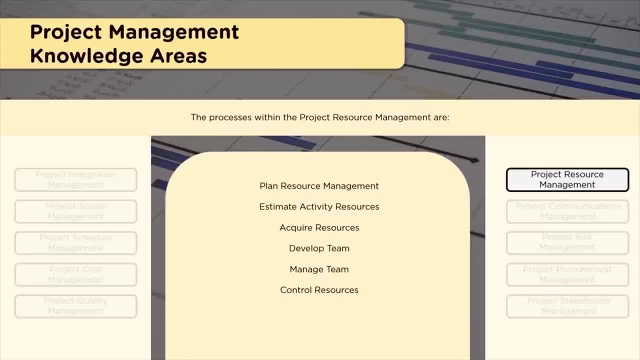 acquire resources, develop team, manage team and control resources. So plan resource management and estimate activity resources are part of planning process group. Acquire resources, develop team and manage team are part of executing process group, whereas control resource is part of monitoring. 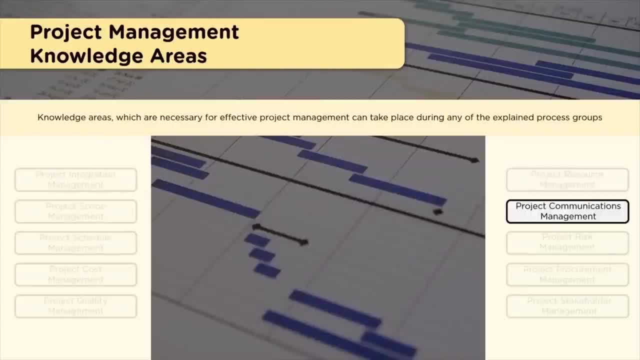 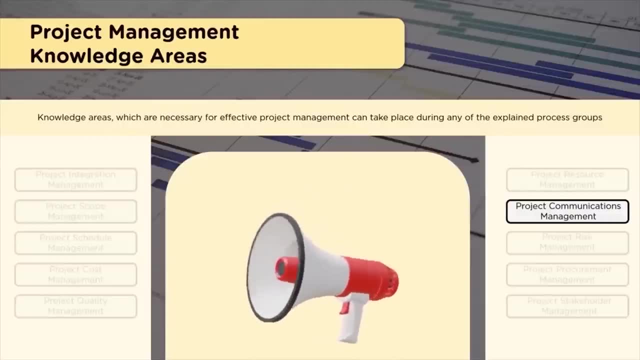 and control process group. So next knowledge area we are going to look at is project communication management. So when we say project communication, firstly we need to understand what is this communication is all about. So communication is used to convey something to someone. 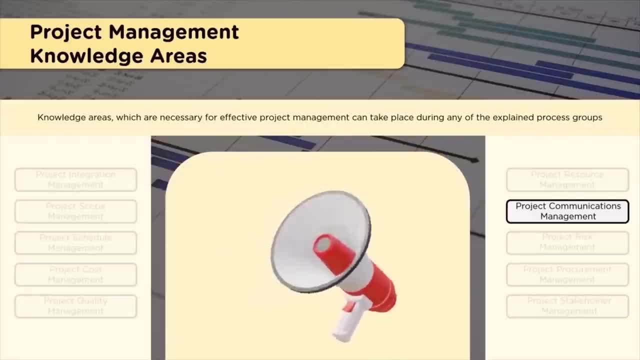 So there should be two parties: the communicator and the one who receives. it means sender and receiver. So very important here is, when sender sends certain message at the receiver's end, how it is received. Is the meaning what is actually perceived? 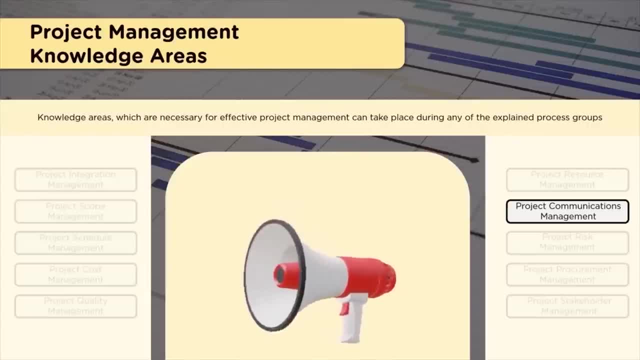 by a receiver is same as what is meant by the communicator means sender. So this will become a big gap if what I told versus what someone understood. if there is a gap, then the communication is not effective. So it is very essential. 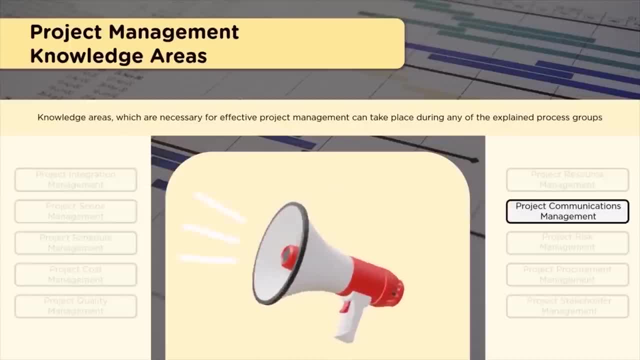 to understand this dynamics, Communication should be very effective and based on that communication there is always a resultant action. So always communication will have two parties. minimum one is sender and receiver, and in the receiver's perspective one is to understand who would be the receiver generally. 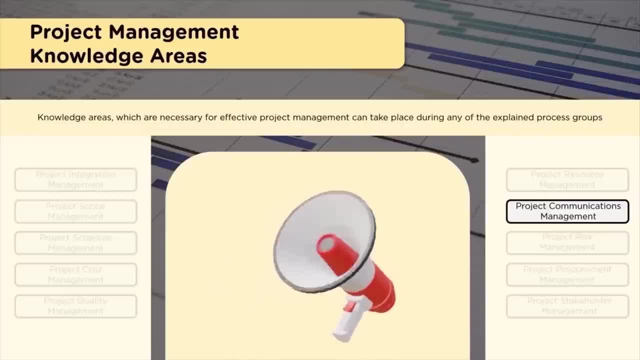 when I say project manager, project manager communicates with sponsor. project manager communicates with team members. project manager communicates with customers. project manager communicates with other functions within organization, suppliers, who are external to the organization. Now, each of these communications will have a specific. 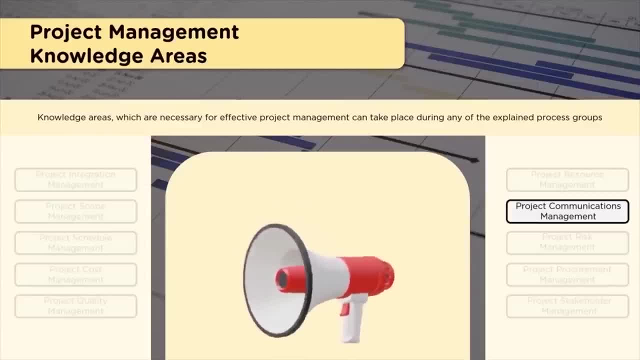 objective and intention. So project manager should understand that. and what sorts of vocabularies, jargons, which needs to be used while communicating, the words, the communication methods which needs to be used, the communication channel, the language, the syntax. 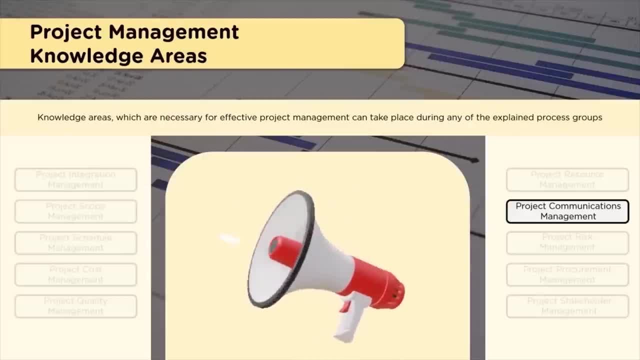 Understanding all of these will become very important while doing the communication in the project. So project communication management is the area that informs the team and stakeholders about the project. So communication management system is determined, along with how it is done and how often it is done, how frequently. 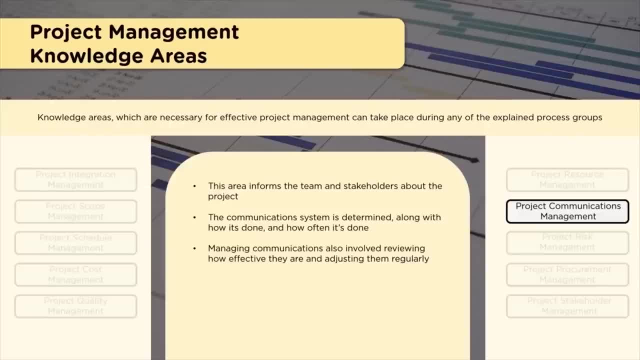 the communication has to be made. So managing communication should also involve reviewing how effective the communication is and how the regularly the modifications are being done to ensure the communication is actually fulfilling the requirements of communication needs. That needs to be discussed regularly and looked at. Is that helping? 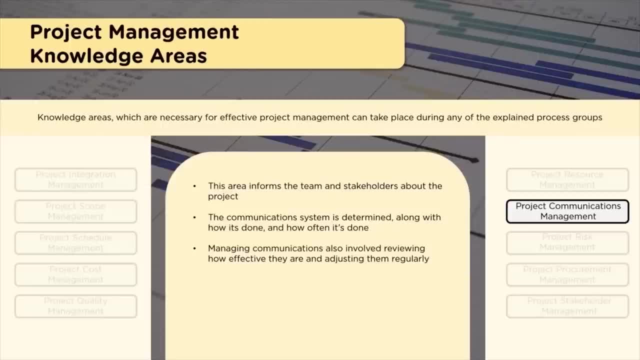 So it is very essential, as the stakeholders are identified, that communication requirement should also identified. and what communication? why is that communication? how often, how frequently the communication has to be made, what channel, what template which has to be used and what language. So all these. 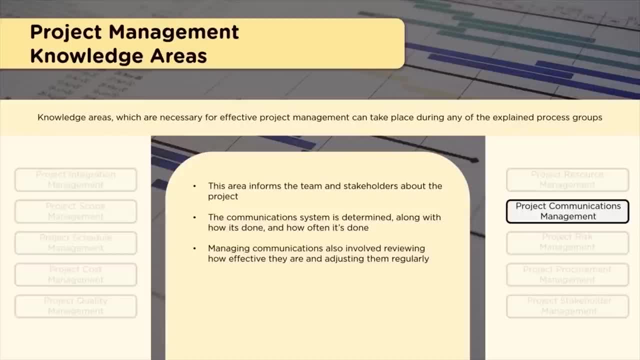 needs to be understood: signed off. So when you go and inform or send some message to the sponsor, it will have specific objective of that communication. Similarly, when you send it to team member, specific objective Here in these two aspects, the frequency. 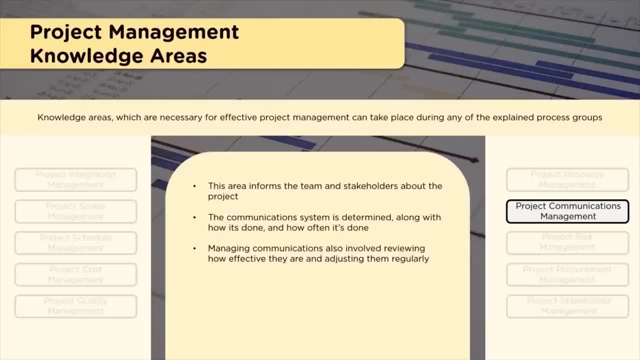 will change the language will change the stakeholders to whom the communication is made. changes and impact it has to create in that communication will also change, So that needs to be understood. The project manager should be very sensitive about it. So communication 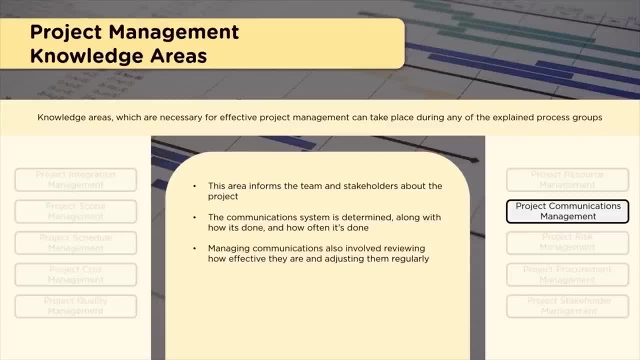 management plays very important role, whereas 90% of the time, project manager will be spending his effort and time in communicating. If that is not effective, it is difficult to become successful in project management. Now let us look at the processes in project communication. 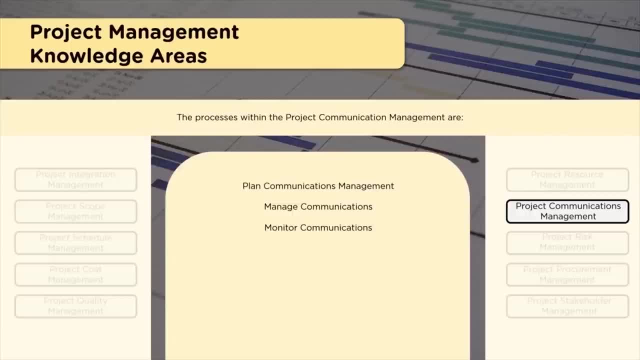 management. So there are three processes, that is, plan communication management, manage communications and monitor communications. So plan communication management is part of planning process. group Manage communication is part of executing process. group Monitor communication is part of monitoring and control process groups. 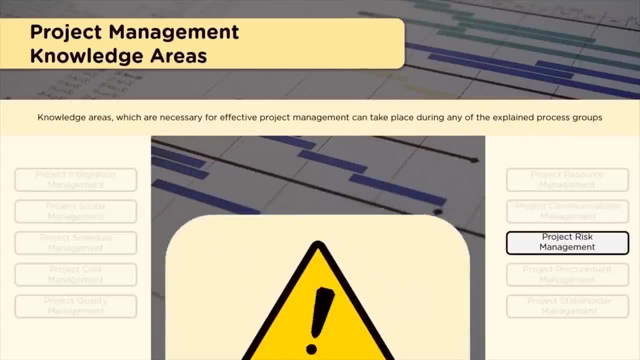 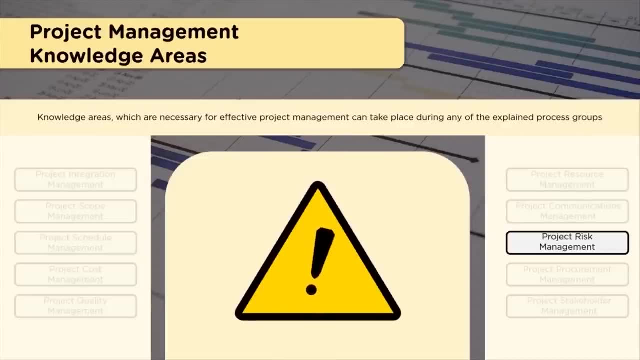 The next knowledge area is project risk management. So when we use the term risk, it is all about an uncertainty what we are speaking about. So every assignment we take up, every initiative we do, everything involves risk. Similarly, project 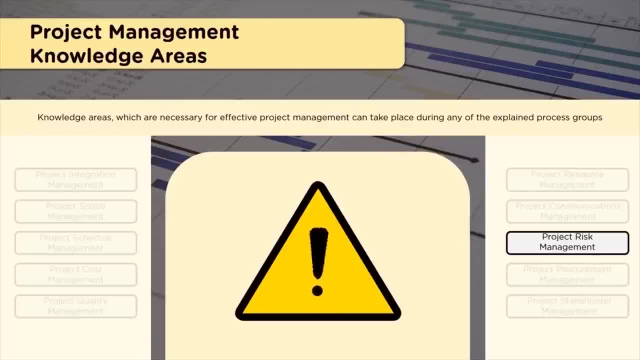 also involves risk. So risk, which is termed as an uncertainty of certain occurrence, are both positive as well as negative. The positive risk we call it as opportunities, whereas negative risk we call it as threats. So each of this risk has to be treated. 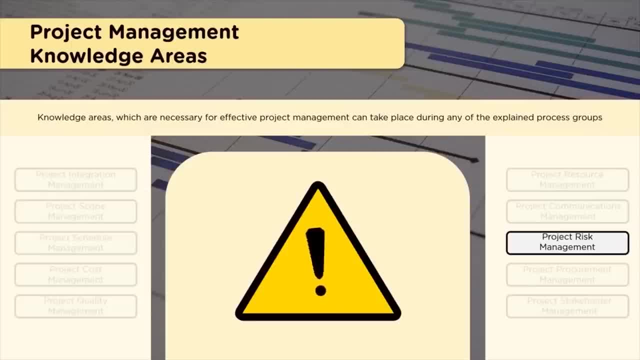 certain way. So before you treat or decide on certain treatment of the risks identified, risks needs to be analyzed. So qualitative analysis, quantitative analysis has to be done and risk responses has to be planned. So the project, risk management, is the 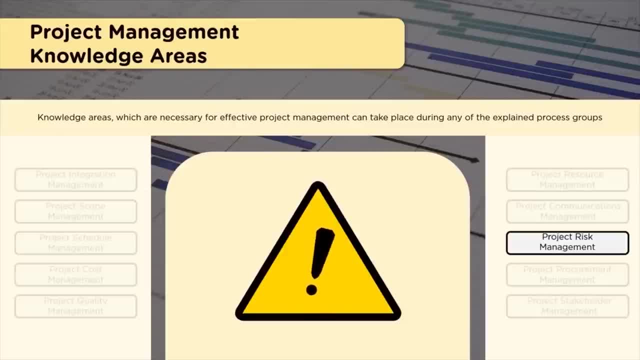 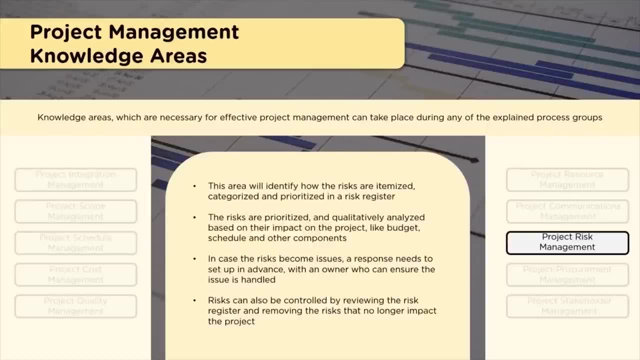 knowledge area which will identify how the risks are itemized, categorized and prioritized in the risk register. Similarly, risks are prioritized and qualitatively and quantitatively analyzed. So, based on their impact on the project, the necessary response plan will be. 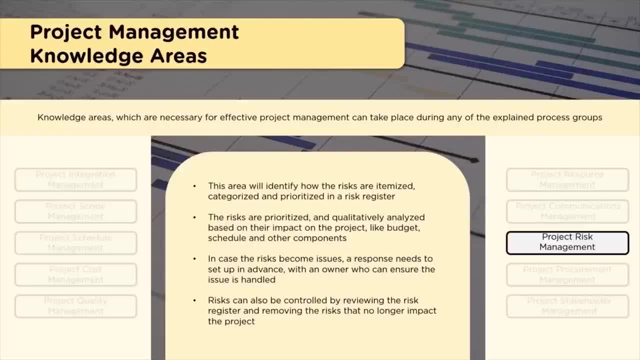 defined. So risk has to be controlled by reviewing the risk register regularly and removing the risk that no longer impact the project. Now the risk once identified, mainly risks- are identified. some set of risks are already identified, captured in project charter. 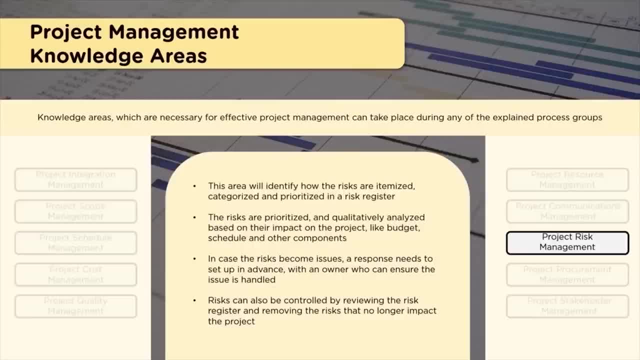 whereas in detail, risks are identified during the planning associated with many different aspects of the project: The risk related to scope, schedule, time, cost, quality, resources, maybe procurement stakeholders. So risks are categorized accordingly and identified. Now, this is not the list. 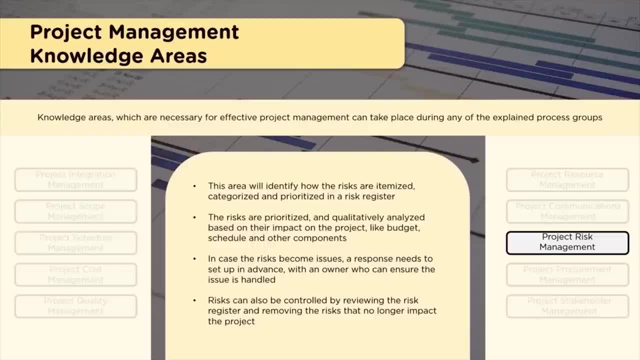 which is made. it is not an exhaustive list which is made in one go, So this acts as a basic list. As the project progresses, all these identified risks needs to be evaluated on continual basis and also new risks needs to be identified regularly, So that what are the? 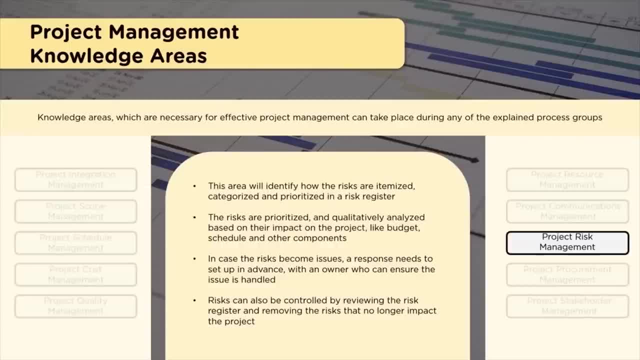 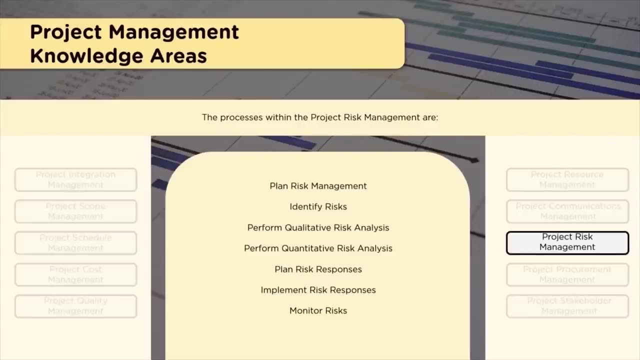 kinds of risks which comes up are understood and then response plans are accordingly taken, So this helps in managing the risks effectively and efficiently. The processes involved in risk management knowledge area are: plan risk management, identify risk, perform qualitative risk analysis, perform quantitative risk analysis and. 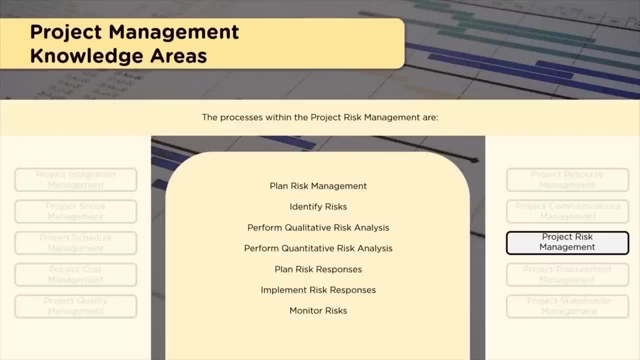 plan risk response, which are part of planning process group, Whereas implement risk response will be part of executing process group and monitor risks: This will be part of monitoring and control process group. So when we say identify risk, this is when you identify the risk here. 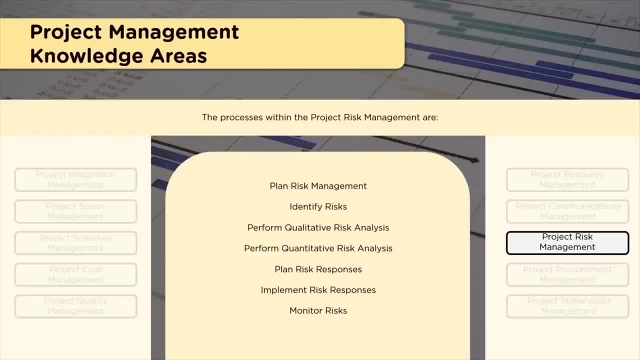 and captured in the risk register and, as I mentioned earlier, this is not a list which is exhaustive. So, at the moment, whatever the risks are being identified, So these risks are analyzed now as part of this planning, qualitatively as well as quantitatively. 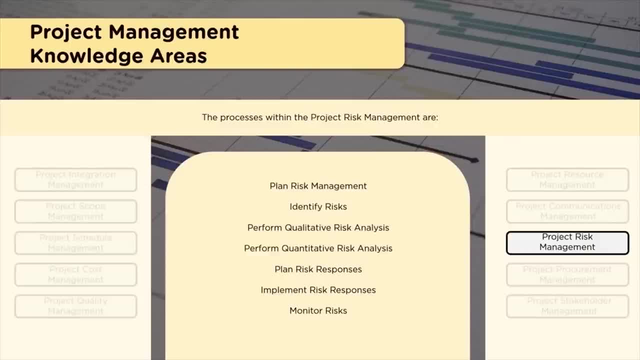 But the analysis of the risk, assessing those risks, should continue throughout the project life cycle, Because the impact level of the risk would vary as it progresses throughout the project life cycle. Now, as we have a risk response plans defined and for some it is already implemented, 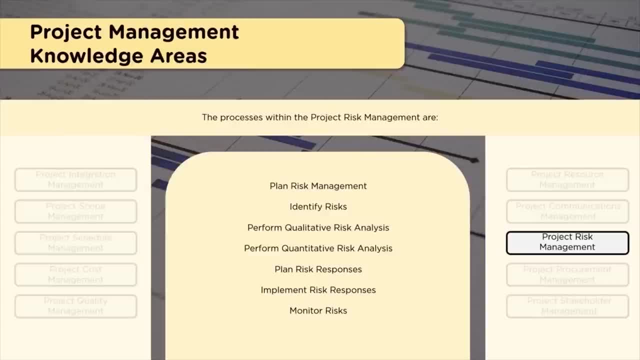 some you cannot implement. You need to make yourself ready to tackle the scenario of issues when it occurs. when risk occurs, You need to handle those. So have that capability built, or having some contingency plans. Any of such actions are taken and project should be ready. 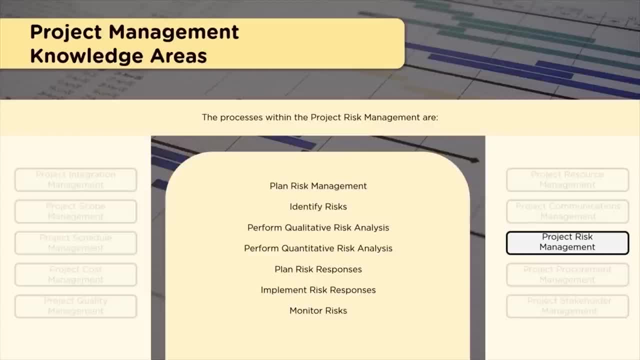 Means when risk occurs, the impact occurred and I am just okay with it. that will not work. So project will get impacted. It may escalate the cost, It may delay the project closure, Many things it will happen. So proper analysis and then 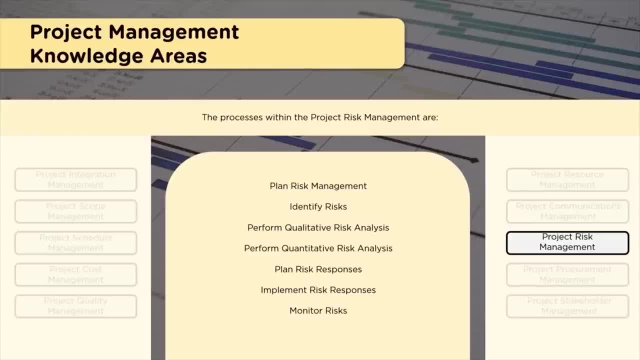 actions in time, Right risk response plans can be implemented. So for positive risk, for opportunities, generally acceptance or exploit or taking advantage of, that would be the kind of response we will see. For the negative risk, the threats, the kind of responses what we would see is 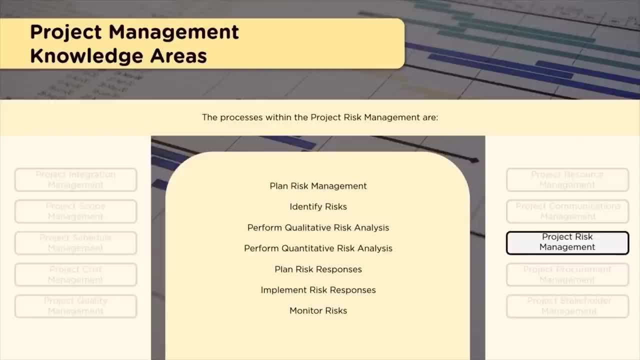 like avoid a contingency plan or mitigate the risk in terms of having some measures implemented. Transfer risk is another thought which is done. So if someone says avoid risk, that behavior is called as risk average behavior, Someone who don't even take risk. 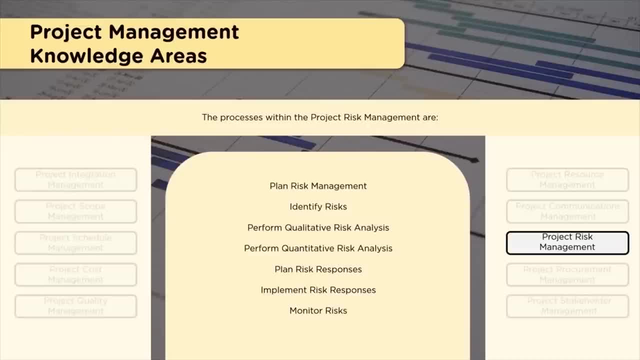 So if I take up this, I have the risk of so much So I will not even take up that Such behaviors- So those are the kinds of risk responses may come across which needs to be implemented as part of executing process group. 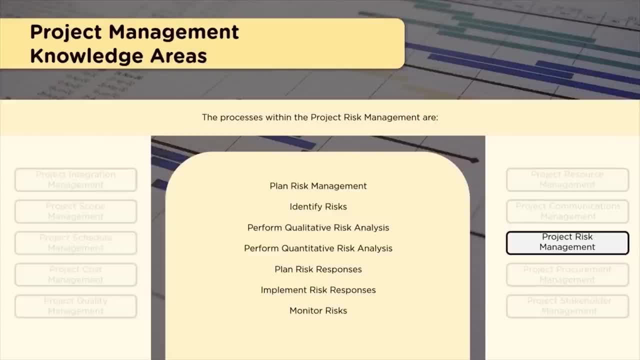 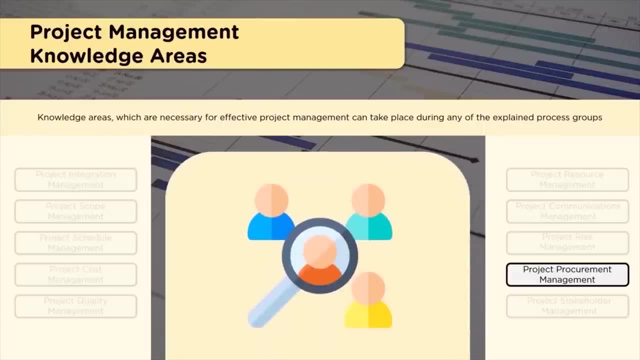 Then whatever the plan, whatever the implementation which has happened, that needs to be monitored as part of monitoring and control. So next knowledge area for us is project procurement management. So when we say procurement, so every project involves procuring something. 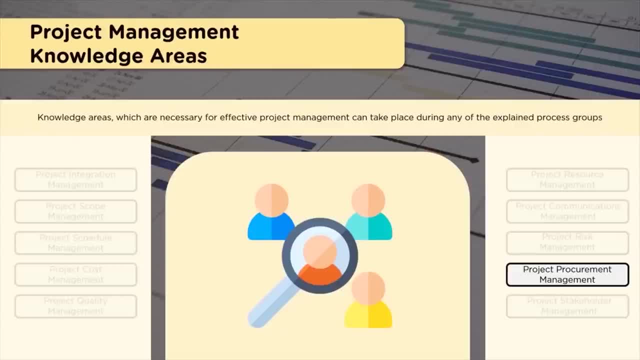 So a main decision which happens here is: make or by decision. So should I make it myself, Should I create myself within the organization, Or should I do something or purchase something? So make or by decision. So when I decide I am going to. 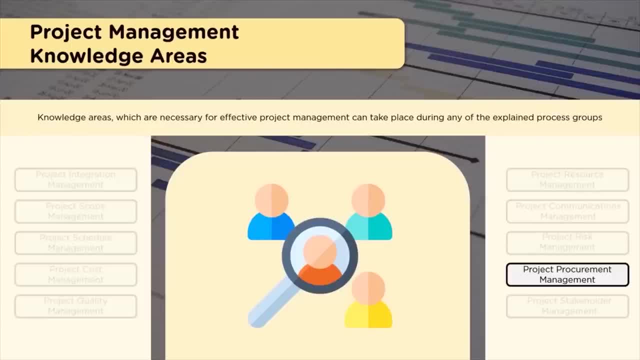 buy certain things from outside, because we cannot make everything as part of our organization, because the direction of the business is totally different. If I am a bank and I am doing an IT project, I need not go and sit and start configuring a server, So I need not hire a people who 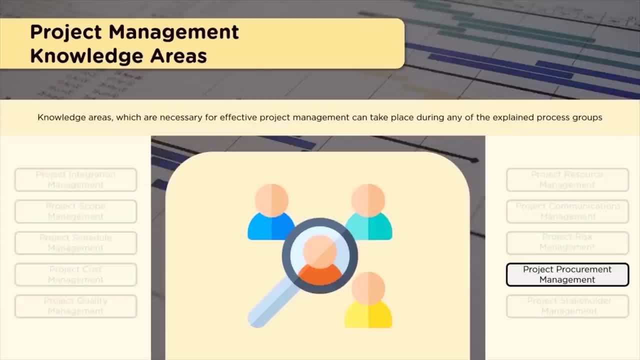 configure, and then they come and sit here and I start managing them. So my entire focus of ranking services, which I need to focus on, will go for TOS. I should not do that, So instead I will give to an experts. So procurement. 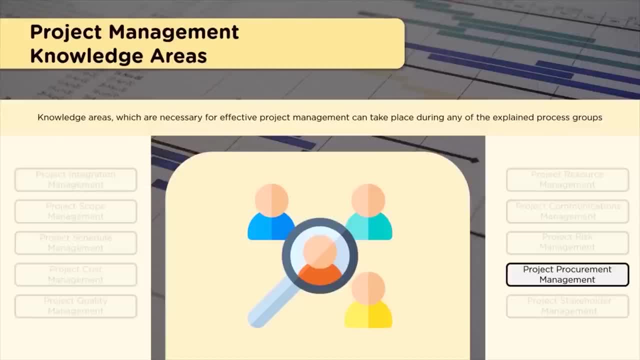 of an IT services from an IT service provider, I will do So to giving it to the experts rather than doing myself, which helps me to have that expertise coming to me. So procurement management involves in identifying those resources, the products or services which needs to be procured. 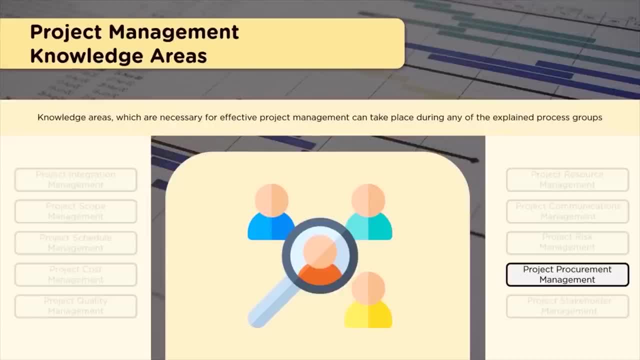 to use in my project So that I need not spend time on that. So this involves identification of the suppliers, having those subcontractors- So they will have an engagement through a contract- and monitoring and managing them and establishing a relationship with them and engaging with them. 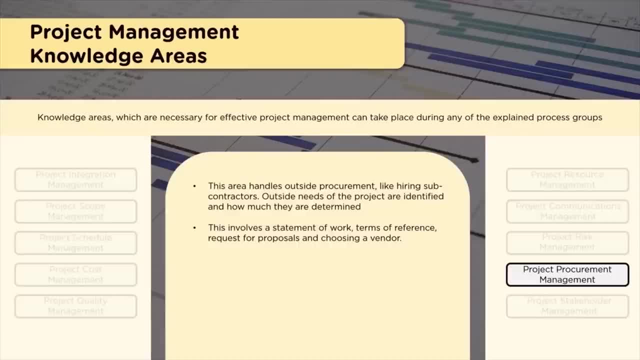 in appropriate way. that is required. It is very essential to be done in every project. So that way project procurement management would guide, in terms of handling all the procurements, what we do from outside, external to the organization. So this knowledge area handles. 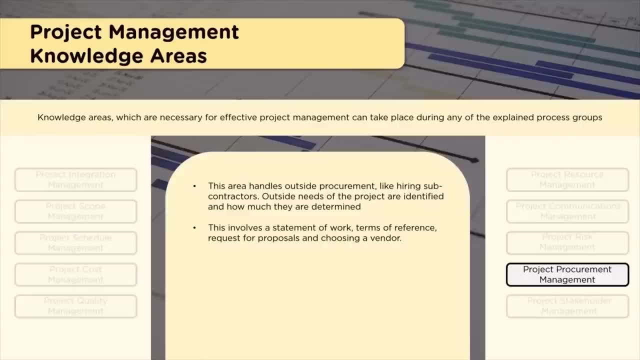 outside procurements, like hiring subcontractors. Outside needs of projects are identified and how much they are determined. This involves a statement of work, terms of reference, request for proposal and choosing a vendor. So to do this bidder conference happens, floating request for proposals can. 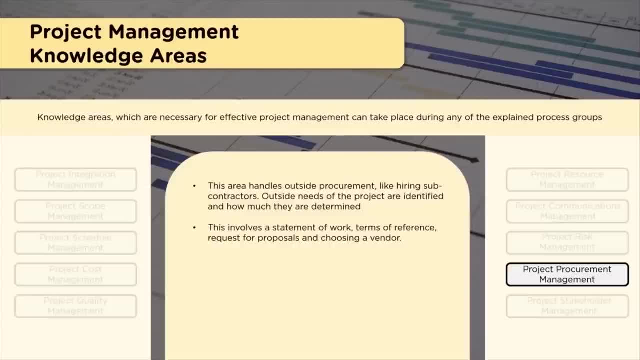 happen. request for quotation can happen. So many such actions are taken and the processes involved here are three mainly So: plan procurement management, which is part of planning process. group Conduct procurement, which is part of executing process. group. And control procurement, which is part of 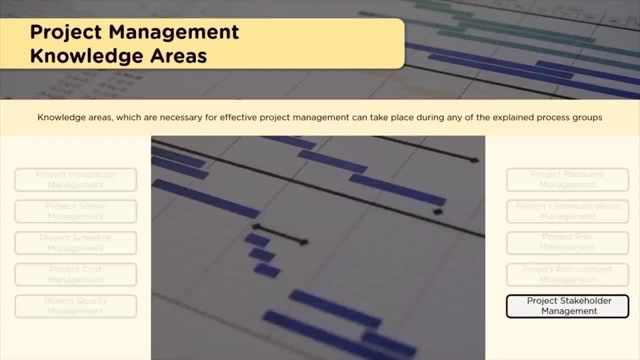 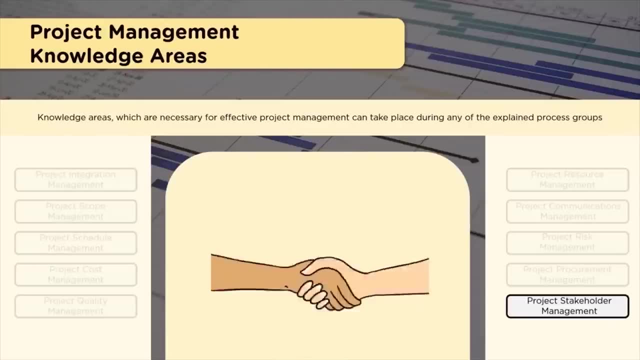 monitoring and control process group. So the next knowledge area is project stakeholder management. So when we say stakeholder, who is the stakeholder? Stakeholders are internal, Stakeholders are external, Stakeholders are the one who influence stakeholders impact. 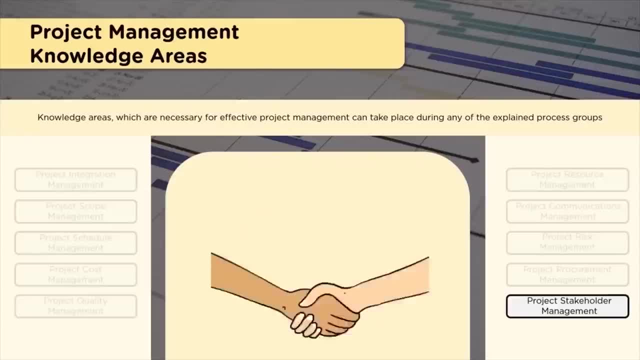 They will get impacted, They are influenced. So, likewise, for every project, every initiative organization takes, there are stakeholders. For me, for my project, I need to identify all the stakeholders. So now: identification of stakeholder. engaging with stakeholder. 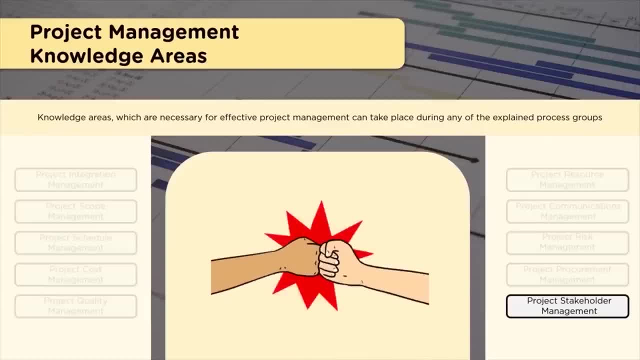 managing the stakeholders will become very essential. So, as part of this knowledge area, after identification of stakeholders, the need of stakeholders needs to be understood. So not every stakeholders identified will have very close to the project. They are not in very close. 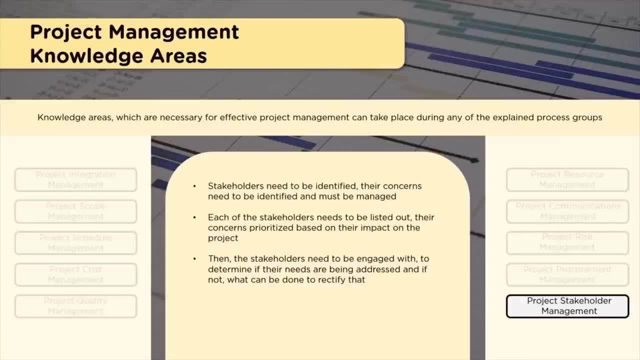 proximity to the project. The distance of the stakeholder from the project may be far Still they may have an impact because of this. We need to understand that If I am building a flyover, construction of flyover is happening. obviously, people living in that region, 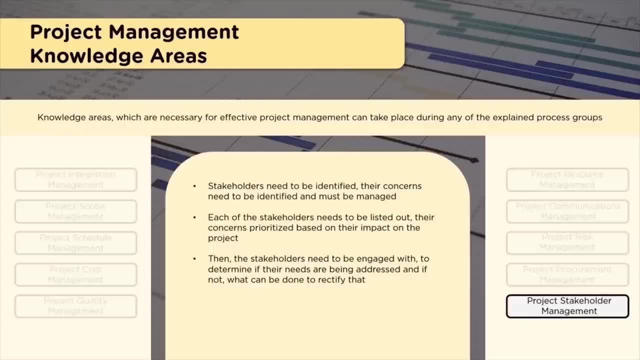 will get impacted, But they have no direct involvement in the project. However, their cooperation is required. So, likewise, as we identify the stakeholders, we need to understand what kind of impact or influence that stakeholder will have on them or on the project from them. This needs to be analyzed. 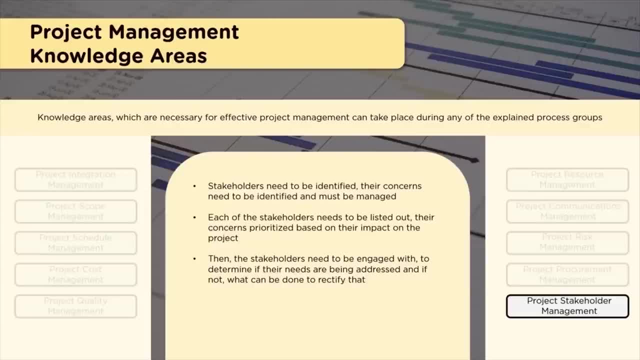 So stakeholders needs to be identified, Their concerns need to be identified and must be managed. Some stakeholders would come up with certain powers, authorities, So we need to understand that as well. So each of the stakeholders needs to be listed out. 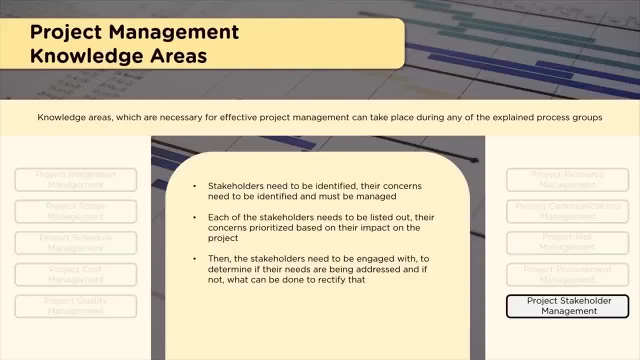 Their concerns prioritized, based on their impact on the project. Then the stakeholders need to be engaged and determine if their needs are being addressed. If not, what can be done to rectify those, if at all any issues exist. So various stakeholders state also can. 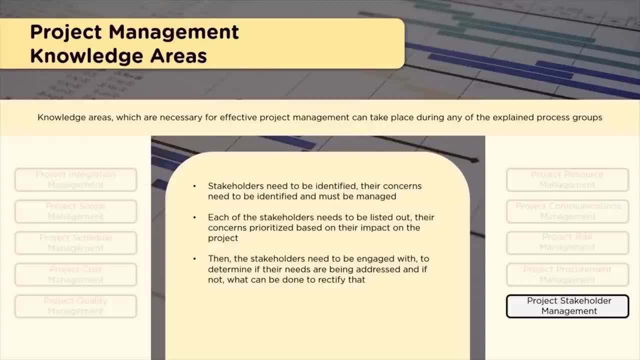 exist. There is a stakeholder who should be very supportive in the project, actively involved in the project, but the stakeholder may be in an unaware state. So we may require to engage with the stakeholder, bring that clarity, explain and then ensure that the stakeholder 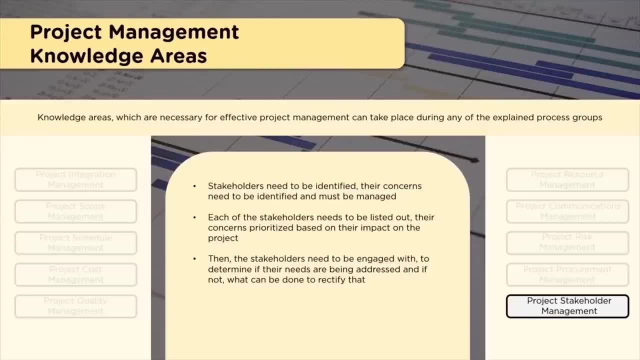 is supportive to the project, Some stakeholders may be resistive, Some stakeholders may be neutral, Some stakeholders will be very supportive, unaware. So various different states of stakeholders would exist, But one needs to analyze what kind of state that stakeholder. 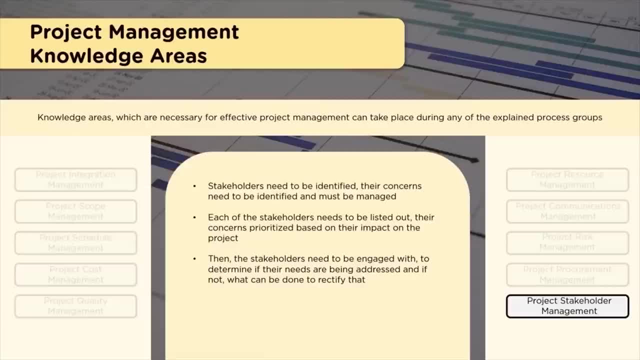 should be in this project. That needs to be discussed, understood and then decide. So accordingly, engagement should happen. So stakeholder engagement plan needs to be defined very clearly. So now, here we have four processes. So one process in initiating, 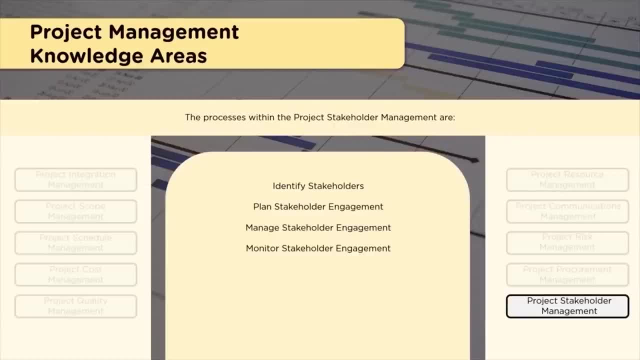 process group, that is, identify stakeholder, Then plan stakeholder engagement, which happens in planning, Manage stakeholder engagement, which is executing process group, and monitor. stakeholder engagement is monitoring and control process group, As I mentioned in risk management, in stakeholder management also. 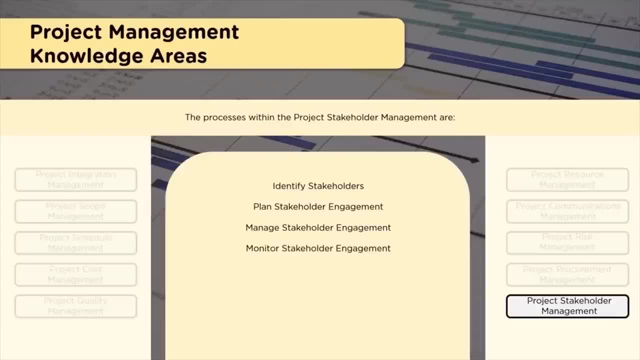 identification of stakeholder, analyzing the way stakeholder engagement should happen and deciding that engagement. This is very dynamic, which has to happen throughout the project life cycle And this is not one time register. what we create like stakeholder register- if we create, It is not. 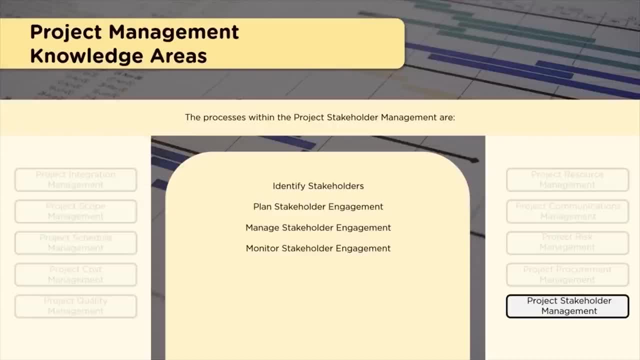 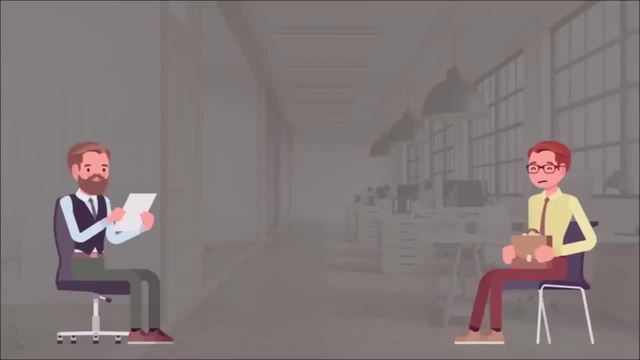 one time register. It is dynamic, which gets updated throughout the life cycle of the project, And today we will learn about PMP certification. Before we begin, let's have a look at an incident where two project managers, John and Ted, are talking to each other. 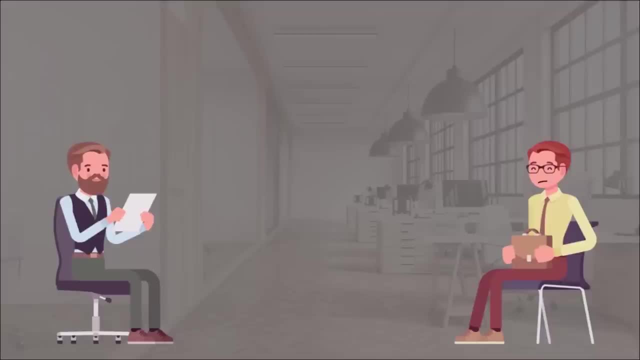 John is a senior project manager, while Ted is a part of his team. John finds Ted to be upset, So he asks him: is there anything he can help him with? To which Ted replies that his project failed. John further asks him what could be the possible reason for the project failure. 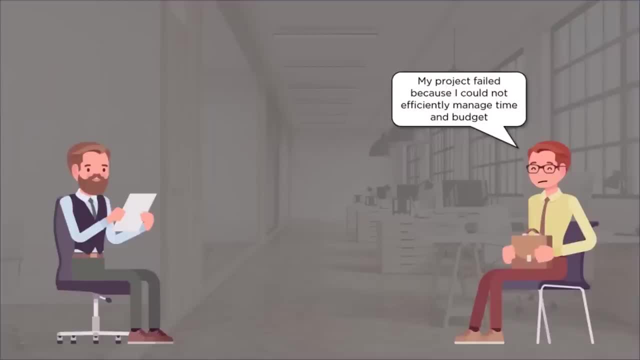 Ted tells him that it's because he was not able to manage the time and budget. Now John asks him if he is PMP certified, To which Ted says he isn't. Then John suggests, Ted, that he must take the PMP certificate. 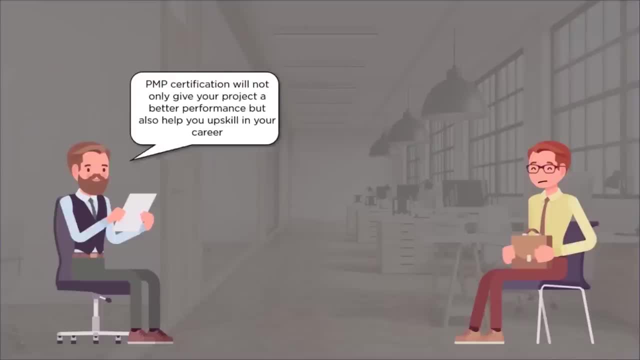 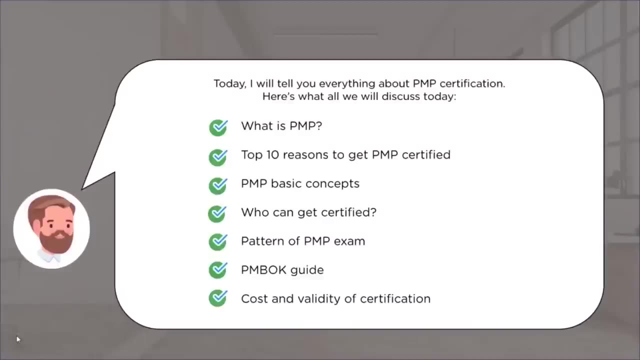 which will not only give his project better performance but also help him upskill in his career. So today we will discuss about PMP certification in detail. Let's first have a look at all the topics we will cover. We will begin with: what is PMP? 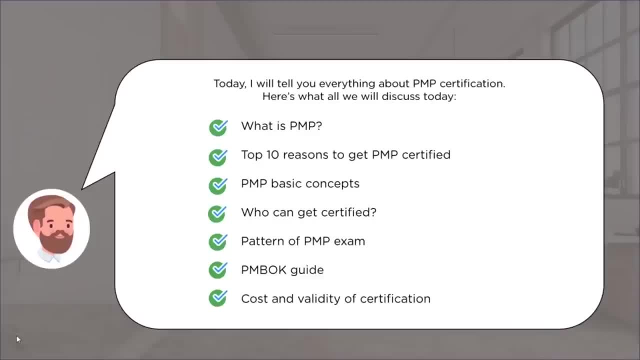 Then we will check top 10 reasons to get PMP certified, followed by the basics of PMP. Then, after we know the PMP basic concepts, we will check who can get this certification and pattern for the PMP exam Then. 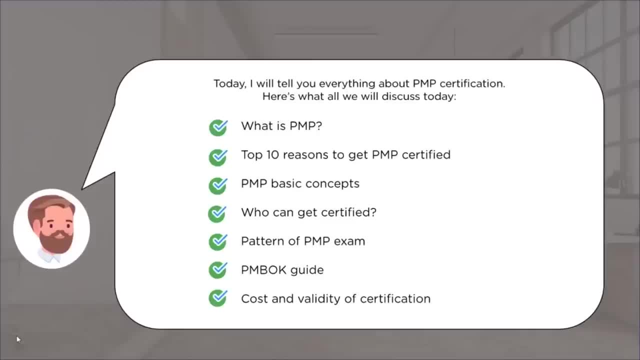 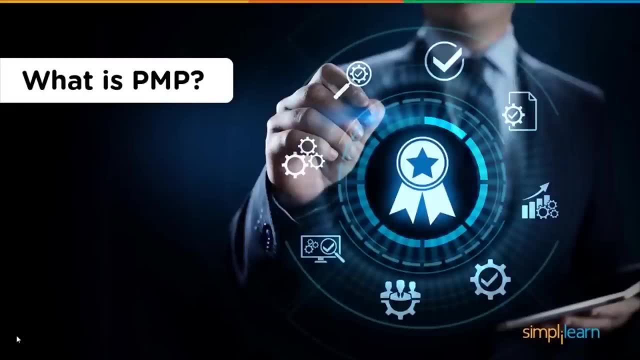 we will learn about the PMBOK guide, which is an integral part to prepare for the PMP exam. Finally, we will see the cost and the validity of the certification. So, without any further ado, let's begin with. what is PMP? PMP- 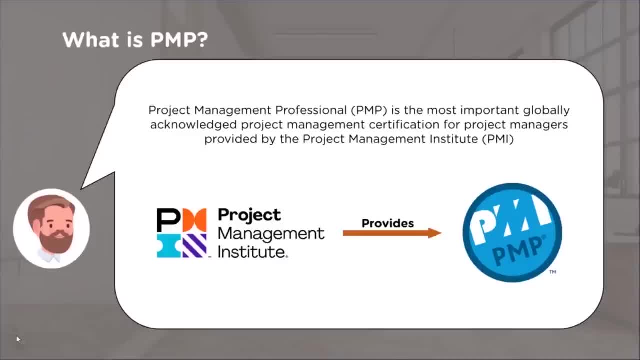 or Project Management Professional, is the world's most renowned project management certification for project managers. This certification is provided by the Project Management Institute. Now, when we know what is project management professional or PMP certification, let's have a look at some reasons why you should. 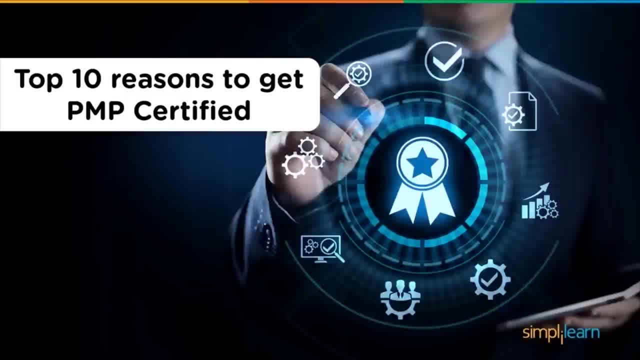 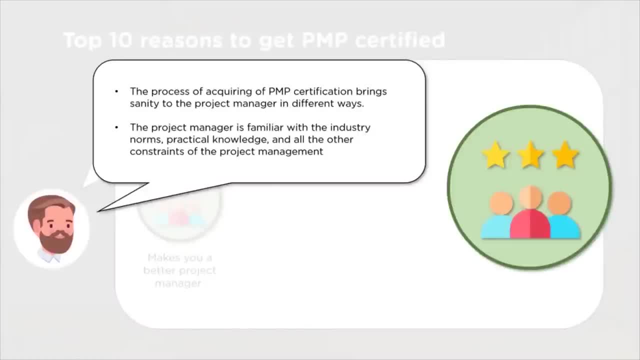 get PMP certified. Today I will give you top 10 reasons to take PMP certification. PMP certification helps you become a better project manager. The process that helps us acquire the certification goes to several phases, like gaining project management experience and passing the PMP exam, which helps. 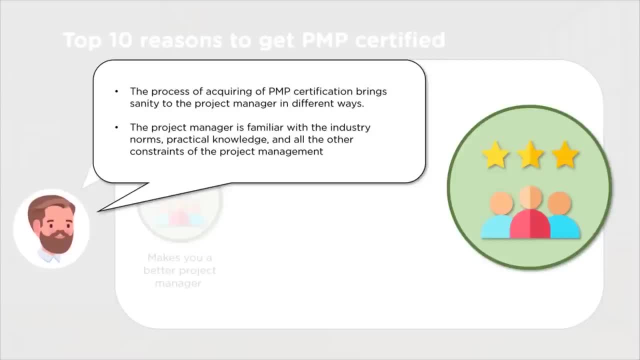 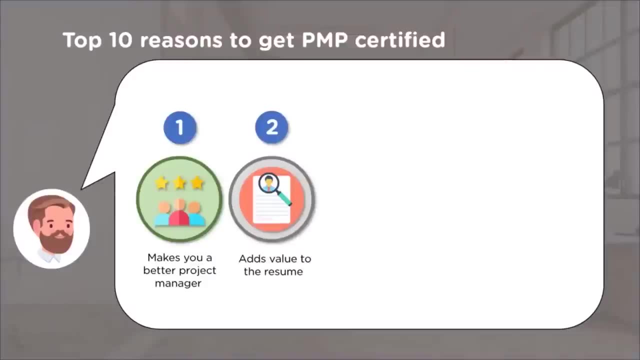 you in bringing sanity to the project manager. The process helps project managers to learn different industry trends, have practical knowledge and several other project management constraints. The second reason that we have is project management certification makes our resume more valuable, As we have discussed earlier. 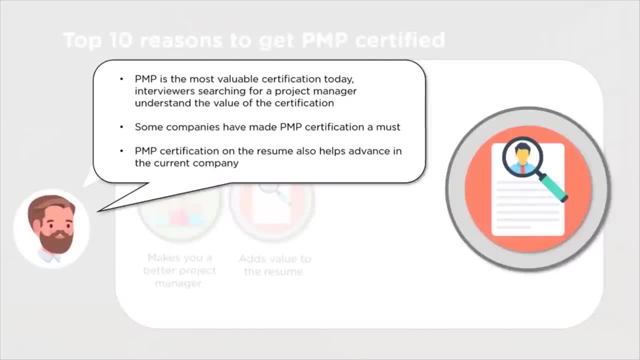 that PMP certification is the most renowned project management certification, so having it on the resume will definitely help the interviewer recognize our skills. There are companies that only accept project managers who are PMP certified. PMP certification not only helps in switching the job or finding a new one. 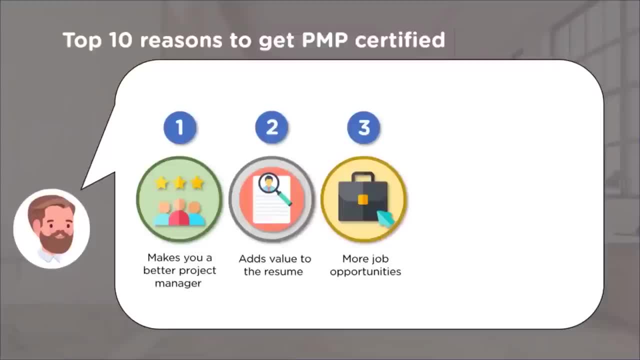 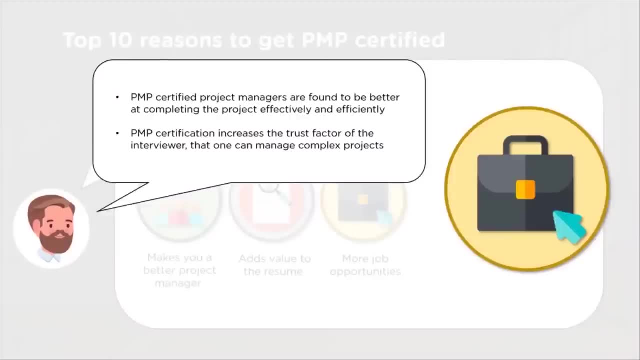 it helps in progressing in the current company as well. The third reason that we have is it provides more job opportunities. When one acquires the PMP certification, it proves that one has expertise in completing the project effectively and efficiently, So the certification increases. 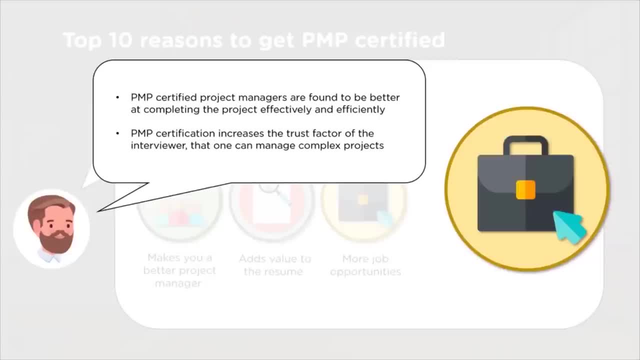 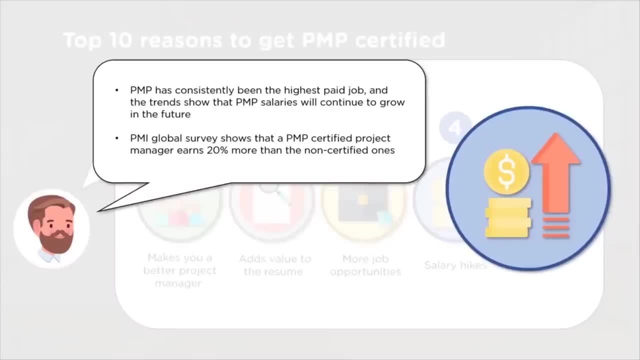 the trust factor of the interviewer in you and increases your probability of getting that job. The fourth reason that we have is salary hikes. PMP certified project manager is one of the highest paid jobs around the globe and this trend will continue to grow. The global survey by the project management. 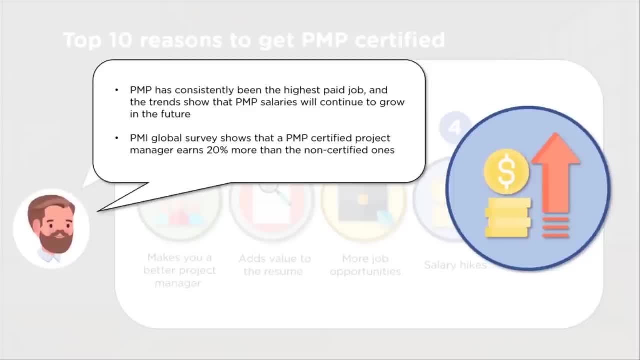 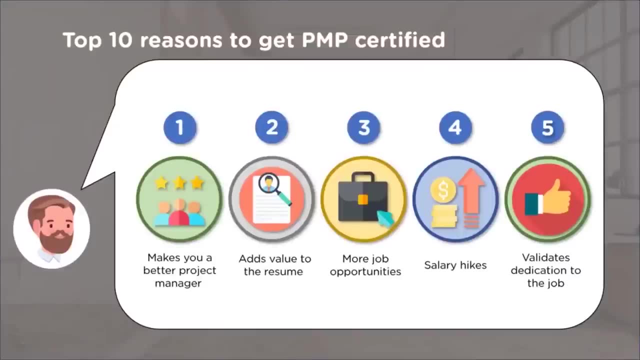 institute shows that PMP certified project managers tend to get 20% more salary than the non-certified project managers. The next reason that we have is PMP certification validates your dedication to the job. The certification requires several months of training. It requires several. 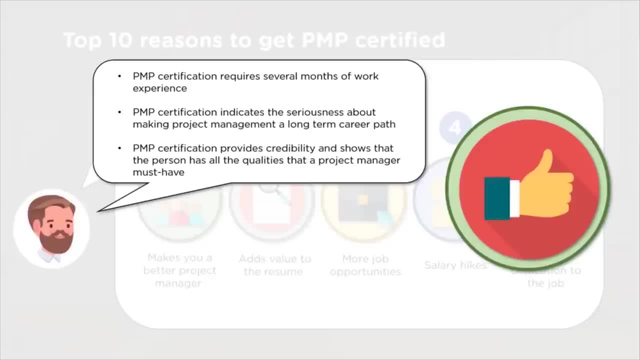 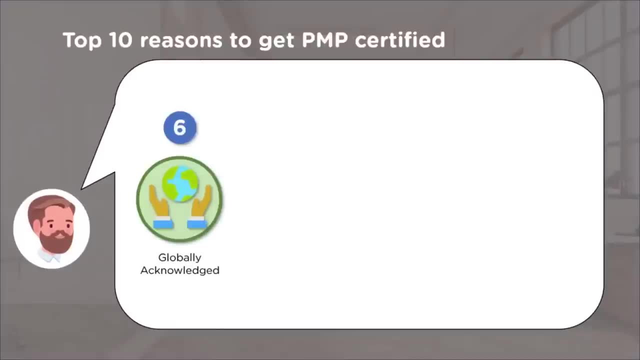 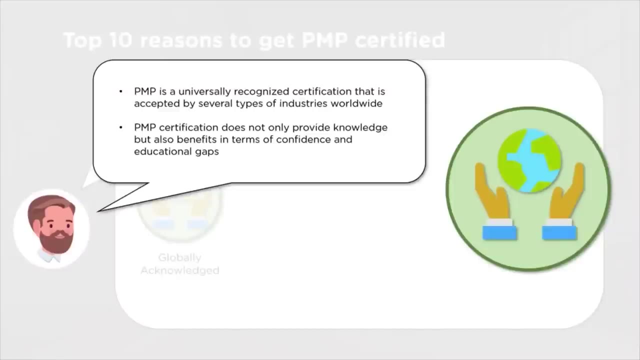 hours of project management experience and exposure. This experience and exposure explains the seriousness of a project manager towards its career path. Then, sixth we have is PMP certification is globally acknowledged. PMP certification is the most renowned certification all over the world. It helps project managers. 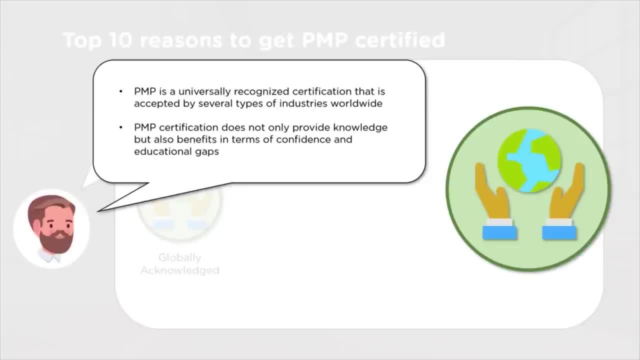 to be a part of different types of industries all over the globe. PMP certification is the most renowned certification all over the world. Project managers who are PMP certified may get jobs in different types of industries all over the world. PMP certification not only provides 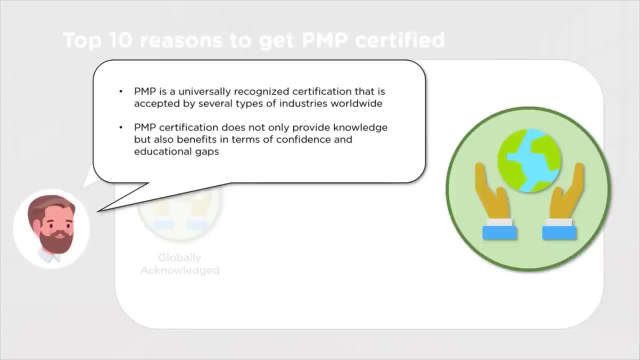 theoretical knowledge, but also helps in gaining practical knowledge, which further helps in increasing the confidence of a project manager. The next reason that we have is better project performance. PMP certified project managers tend to deliver better projects than the non- PMP certified project managers. This is 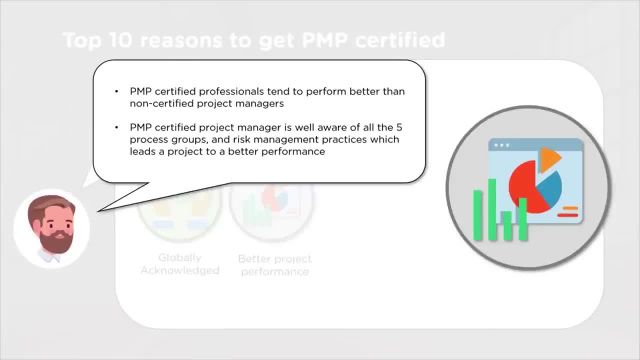 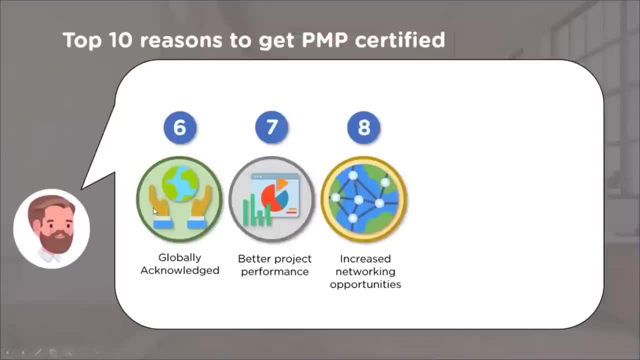 because PMP certified project managers are well aware of 5 process groups, 10 knowledge areas and 49 processes, which helps them have a clear picture of different aspects involved in a project. The eighth reason that we have is that it increases your networking opportunities. 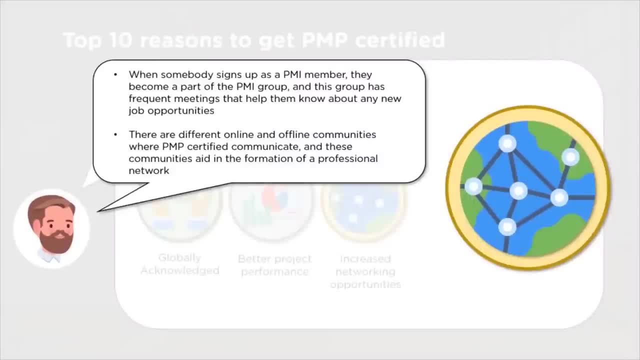 There are several communities that one becomes a part of when they sign up as a PMI member. These communities have meetings regarding new job opportunities and this helps in having a professional network. The ninth reason that we have is job security. Job security is a major reason. 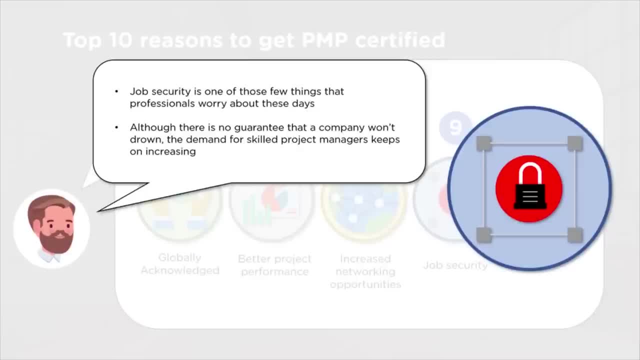 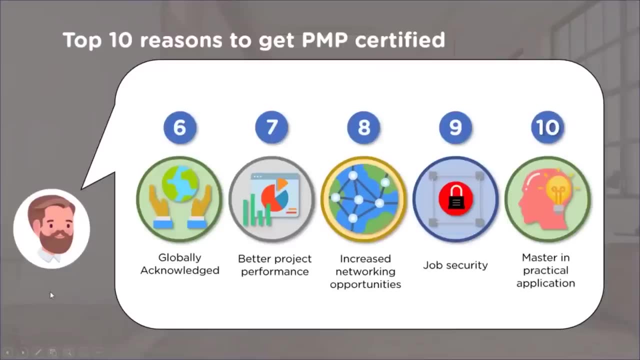 that a professional thinks of before opting for a particular profession. Today, in the world of recession, where companies are drowning, the demand for PMP certified project managers goes on increasing. The last and the tenth reason we have is expertise in practical application When one appears for a PMP exam. 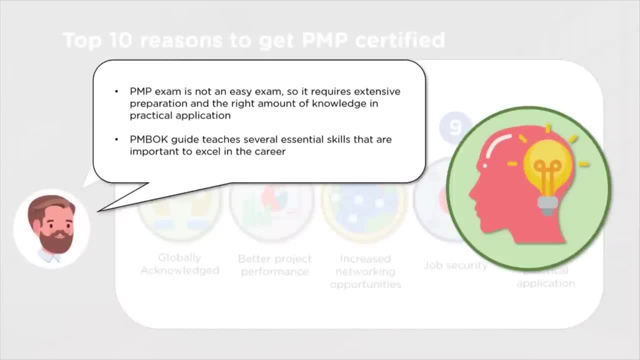 they need extensive preparation. They need to have thorough knowledge of process groups and knowledge areas which help them develop several essential skills and move ahead in their career. Now, as we move further, we will look into the PMP basic concepts. The PMP basic concepts are the five. 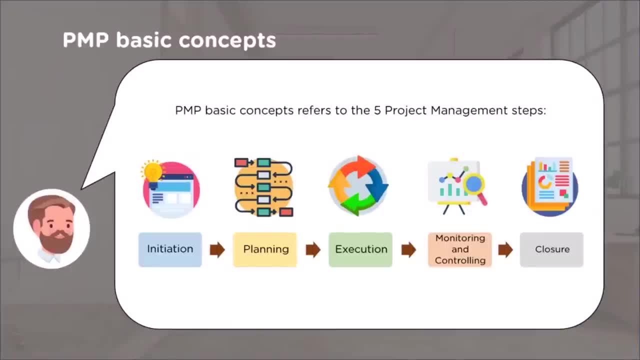 project management steps. These project management steps start from the day we begin our project to the day we end our project. They begin from initiation to closure. The first step that we have is initiation, planning, execution, monitoring and controlling. and closure. Now let's have a look. 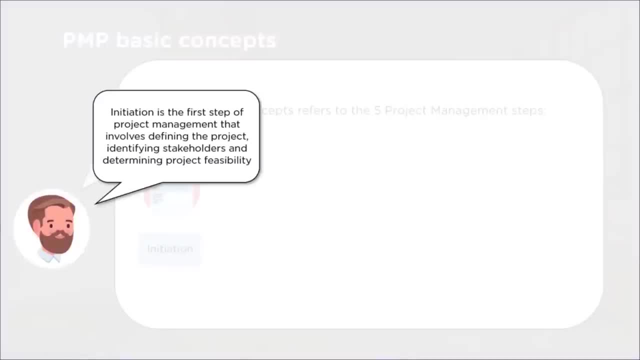 at each of them in detail. The first step we have is initiation. Initiation involves defining the project's scope. This is the step where we explain what our project will have for whom we are making that project. It helps us to identify our stakeholders. 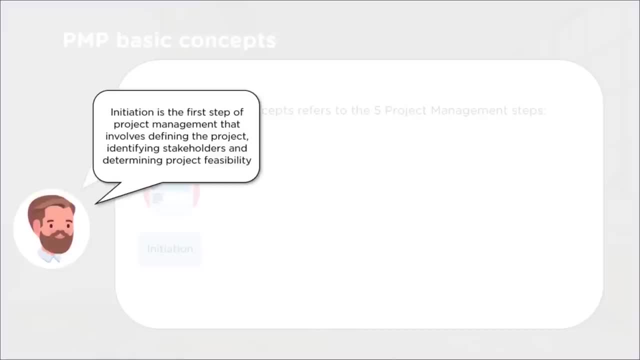 who all will be the part of that project and determine the project feasibility. After the step of initiation, when we have decided the scope of our project, the second step that comes is planning. In the planning phase we define a flow to all the activities of our project. 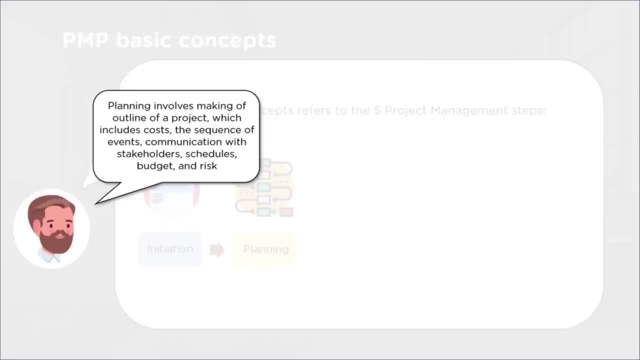 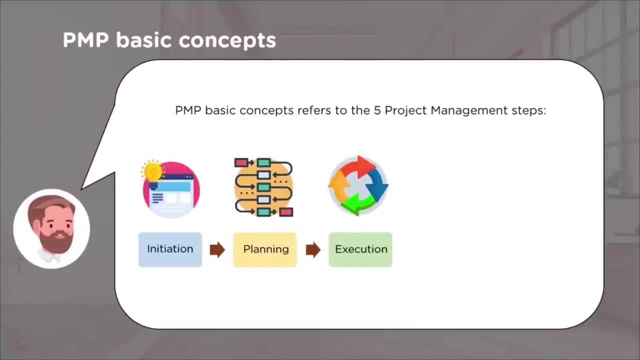 We define this flow, keeping in mind all the constraints of our project, like time, resources and risk. After we have defined the flow of these processes, it is time for us to look at the execution. In the execution phase, we evaluate the plan and. 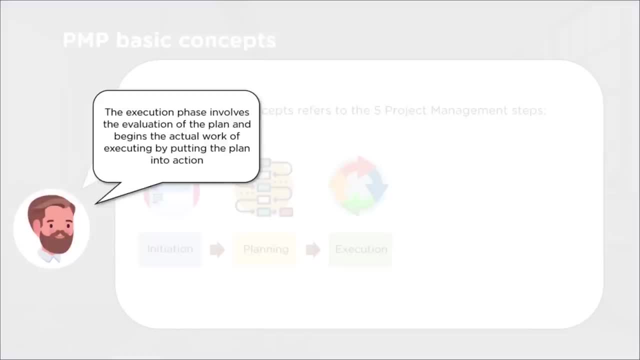 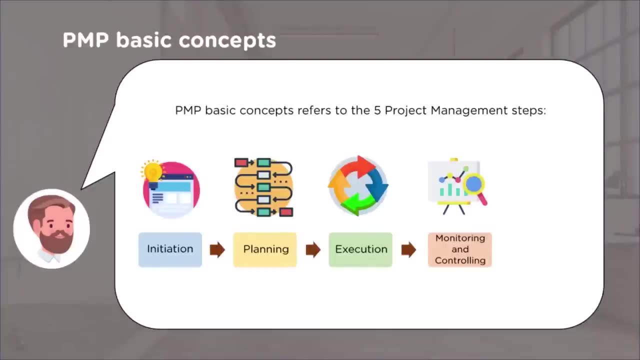 the sequence of the task we have made. We finally put the plan in action and the project tends to start. After the project building has started and the process of execution has started, it is time for the monitoring and the controlling phase. In monitoring and controlling phase, the progress of the 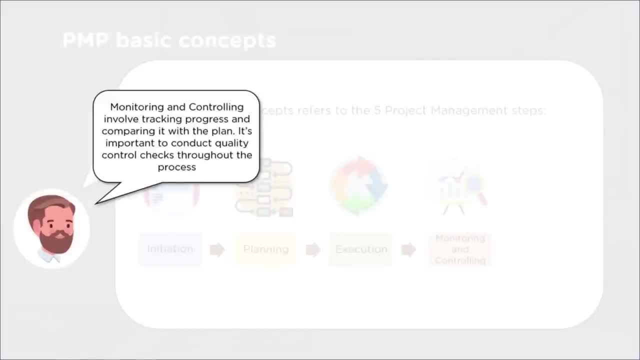 project is tracked and important steps for quality assurance are taken. In monitoring and controlling phase, the work being done is compared with the work as defined in the project plan. In this phase, the progress of the project is tracked and important steps for quality assurance are taken. 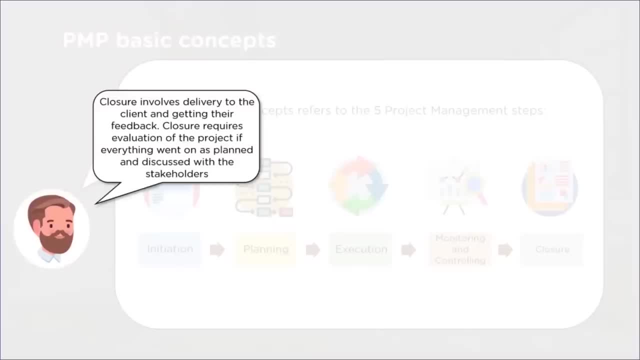 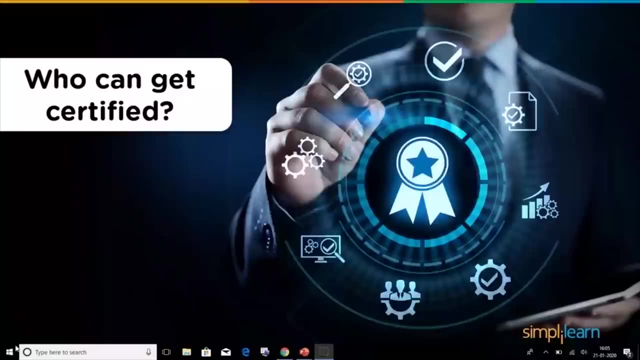 Finally, we have the closure step. In this step, the deliverables are delivered to the client, the documentation of all that took place during the project life cycle is done and project is fully evaluated. Now, when we have seen reasons for getting PMP certified and we 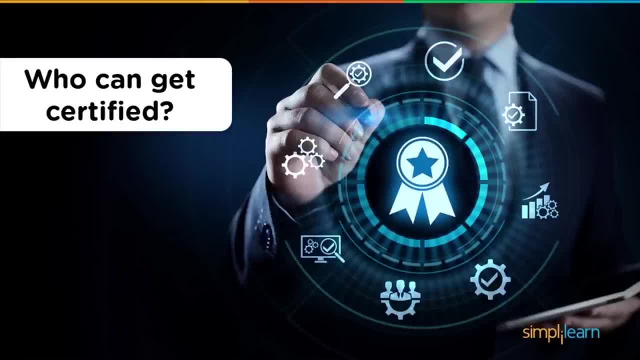 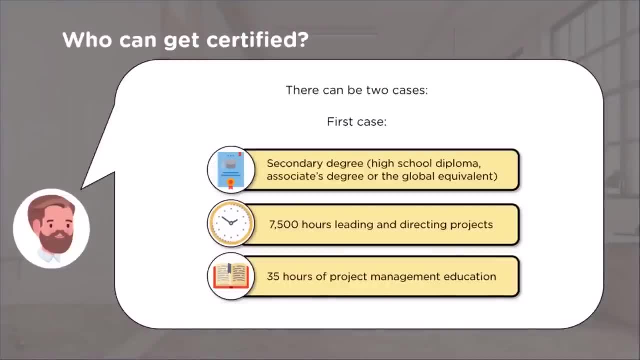 know the basic concepts of PMP, it is time for us to know who can get PMP certified. For getting PMP certified there can be two cases. The first case says you must have a secondary degree. A secondary degree means high school diploma. 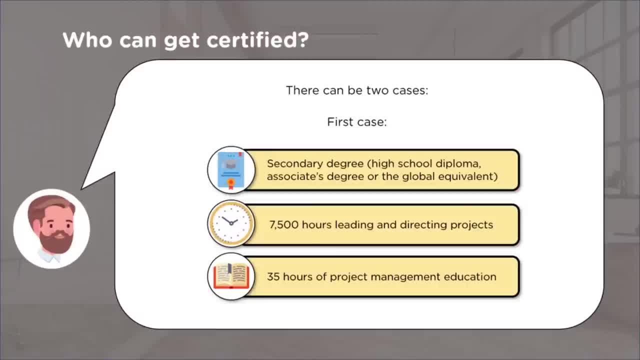 or an associate degree or a degree that is globally equivalent to all of these. Then you need to have 7500 hours of leading and directing projects and 3500 hours of project management education. There can be two cases. First case can be you must have a secondary degree. That 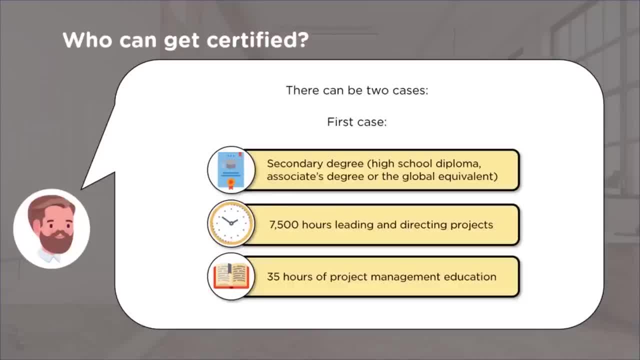 means a high school diploma, associate degree or the global equivalent degree. Then you must have 7500 hours of project management experience and 35 hours of education in project management. The second case can be you must have a four-year degree, along with 4500. 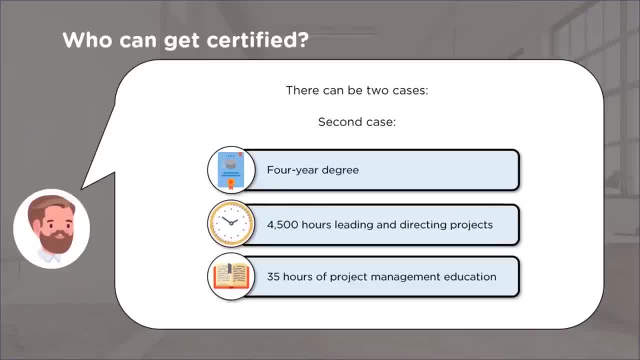 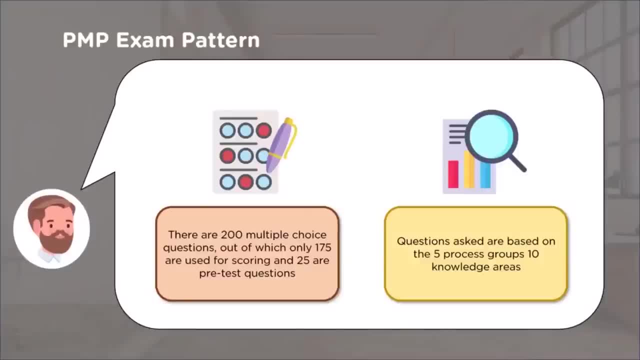 hours of project management experience and 35 hours of education in project management. Now, when we know who can get PMP certified, we will see the PMP exam pattern. The exam comprises of 200 questions, out of which 175 questions are used. 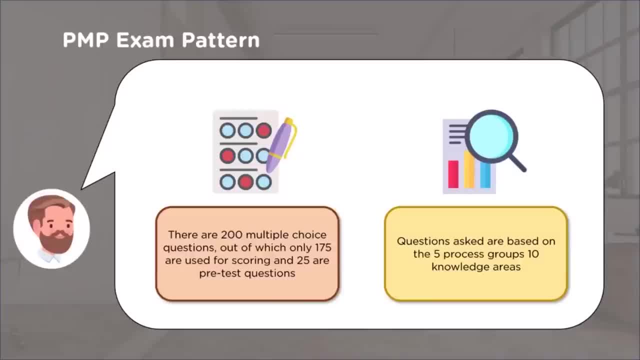 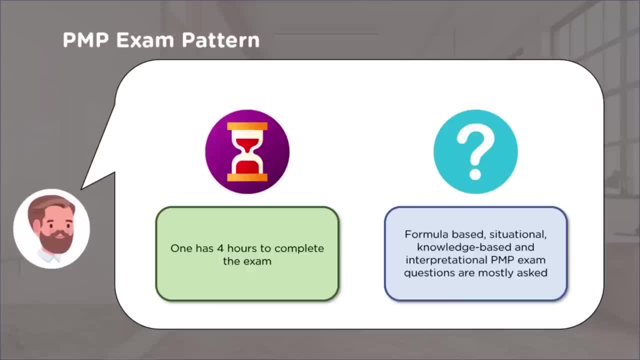 for evaluation. One can answer these questions if they have thorough knowledge of 5 process groups and 10 knowledge areas. The time provided to complete the exam is 4 hours. The questions that are asked are of different types, The most common type being formula based. situation based. 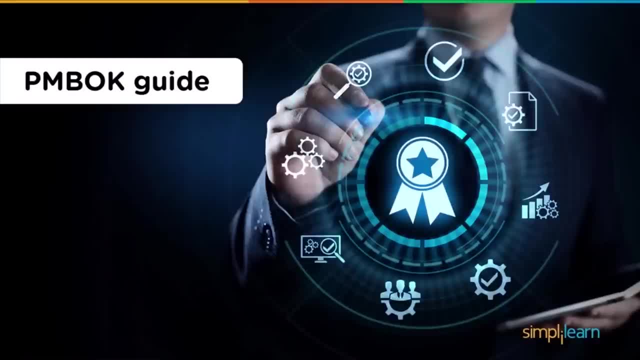 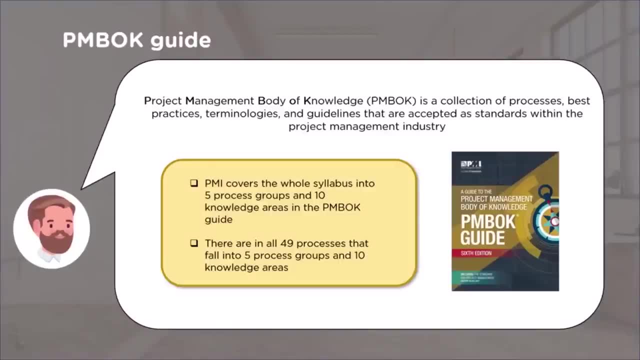 and knowledge based. Now, when we have discussed about the exam pattern, discussing about the PMBOK guide becomes very important, So the next topic that we have is PMBOK guide. PMBOK guide, or project management body of knowledge, is a book that comprises 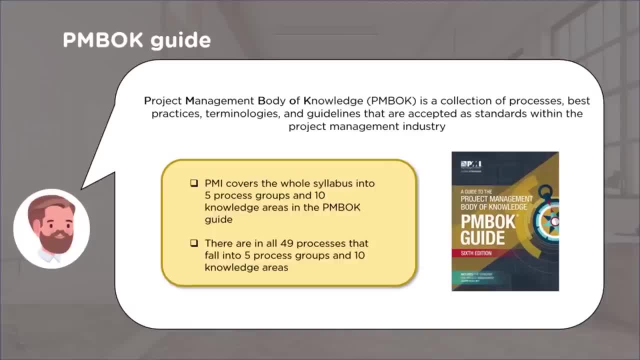 of several processes and different terminologies needed to crack the PMP exam. The whole syllabus of PMP exam is covered in the PMBOK guide by the project management and 10 knowledge areas. Apart from this, there are 49 processes that are divided amongst 5 process 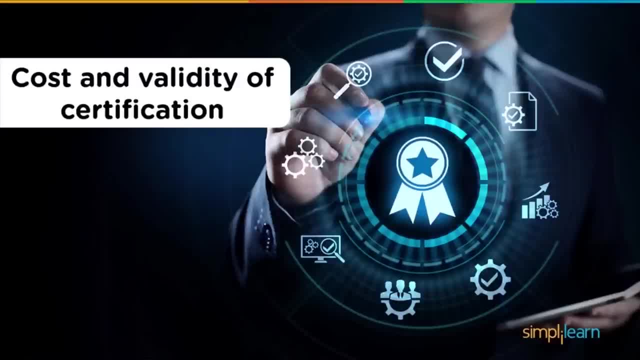 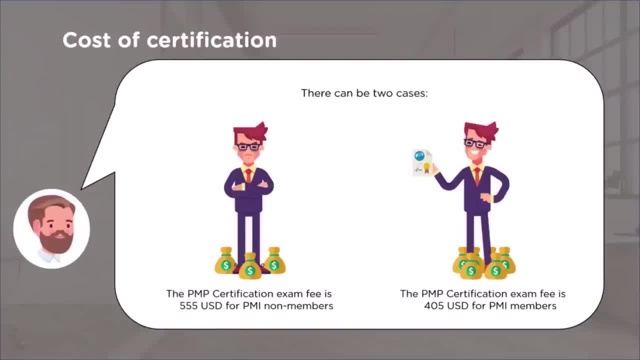 groups: 10 knowledge areas. Finally, let's have a look at the cost and validity of the PMP certification. When we talk about the cost of the certification, there can be two cases. The first case can be if we are not a member of project management. 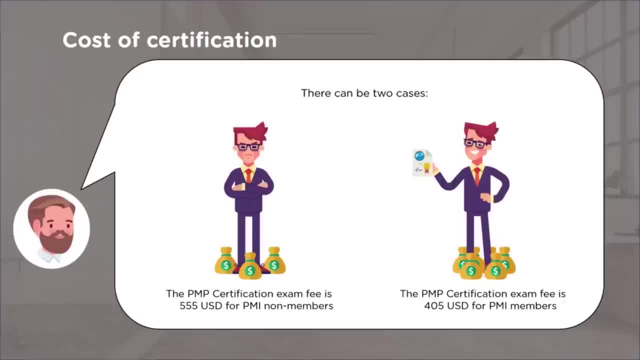 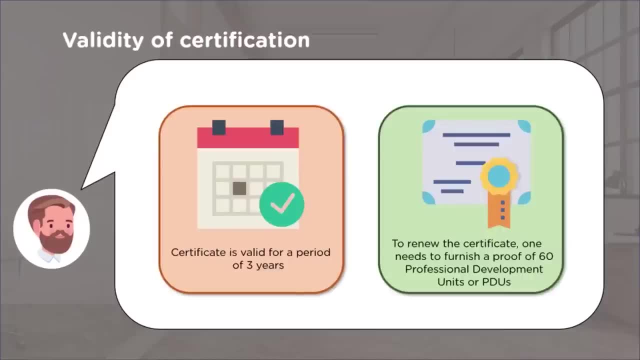 institute, the exam fees is 555 US dollars. The second case can be: if we are a member of project management institute, the exam fees is 405 US dollars. If we talk about the validity of the certification, the certificate is valid for a period of 3 years After every. 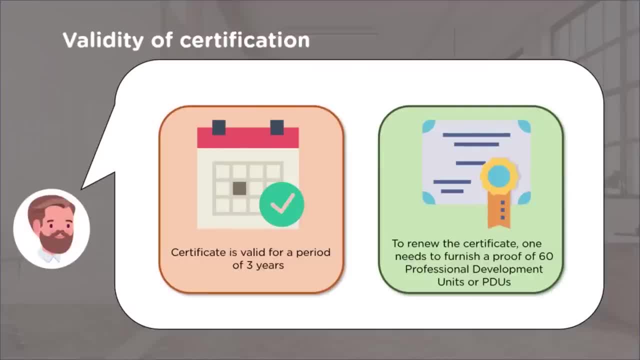 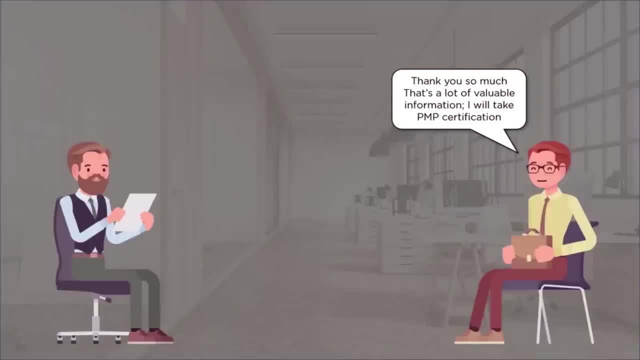 3 years, the certificate needs to be renewed. To renew the certificate, one needs to furnish a proof of 60 PDUs or professional development units. After so much information, Ted thanks John for his time and promises to take the PMP certification at. the shortest notice. Now let's have a look at the salary trends of a PMP certified project manager and a sample resume. If we consider the salary of a non-PMP certified project manager, it is approximately $91,000.. While if we consider the salary, 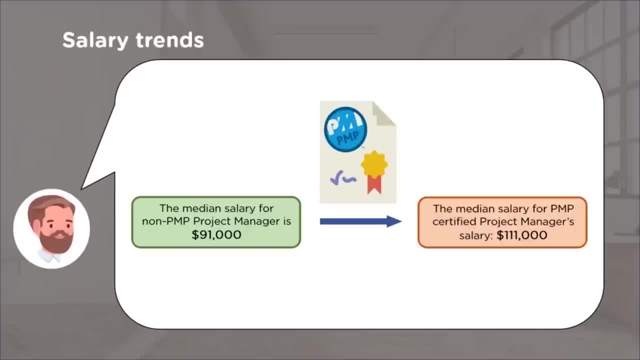 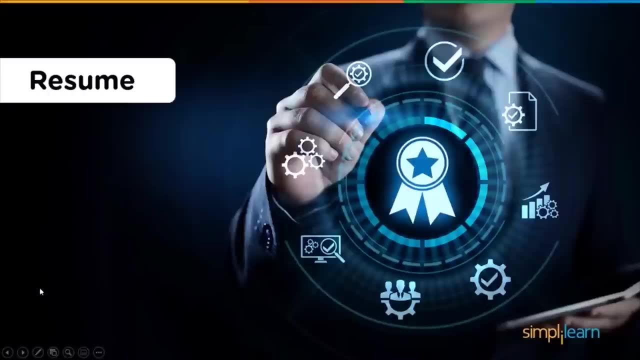 of a PMP certified project manager. it is approximately $111,000, which is approximately 20% higher than the non-certified project manager's salary. Now let's have a look at the resume of a PMP certified project manager. If you are somebody with PMP certification, 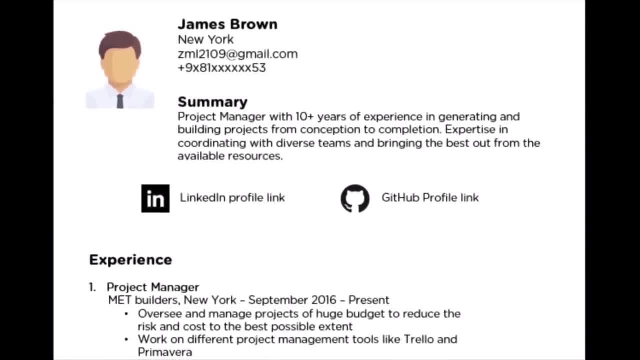 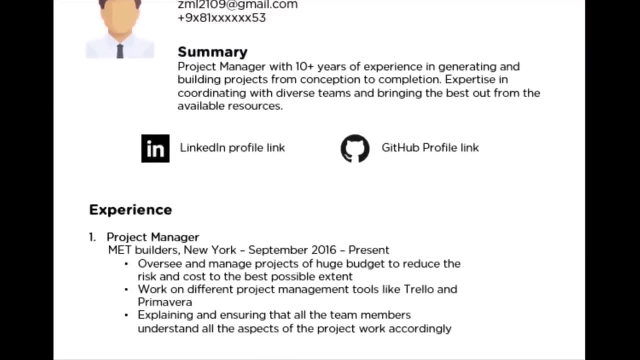 and looking for a project manager or a senior project manager role. your resume should look something like this: The summary in the beginning would include how much experience you have and anything that supports your claim of being a project manager. Like here, James Brown has written, he has: 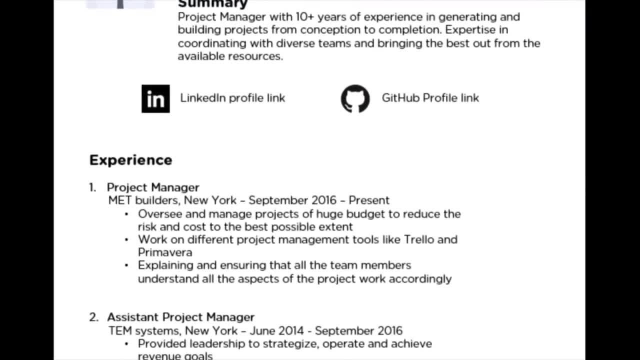 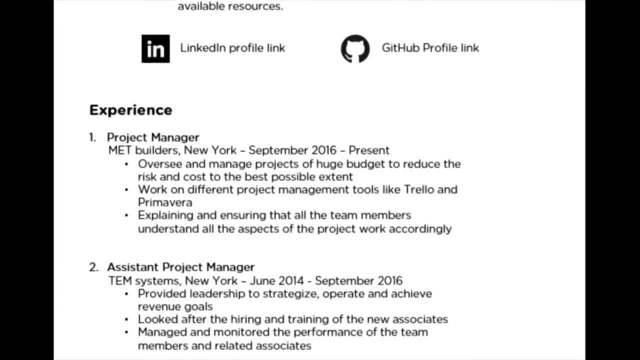 more than 10 years of experience with generating and building projects, Then when you talk about your experience, you should put something that emphasizes on the responsibilities that you had, your area of expertise, put something that shows your skill set for the desired post, and also something 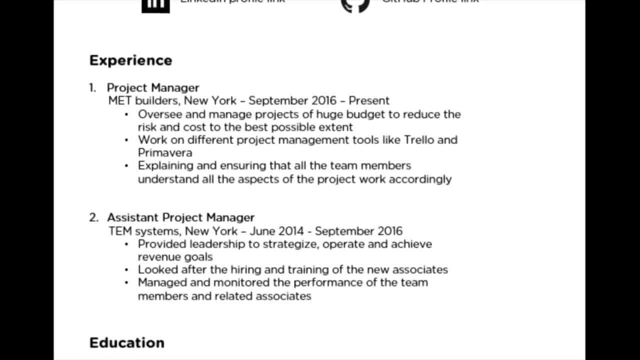 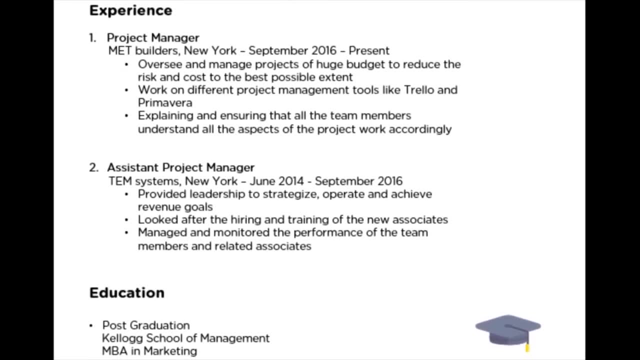 that you learned from your former job role. This shows that you have command over your work and also the determination to skill and upskill yourself, Like here. James Brown has 3 years of experience as an assistant manager, training new associates, and then more than 3 years of experience. 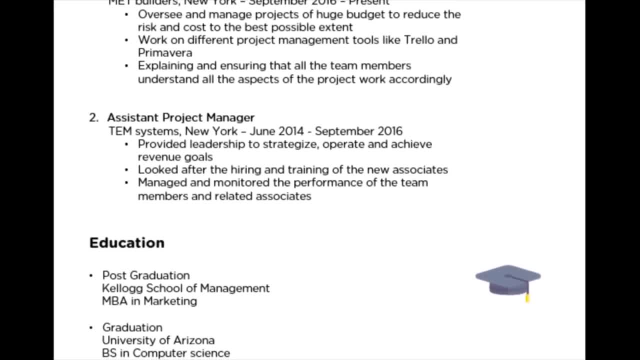 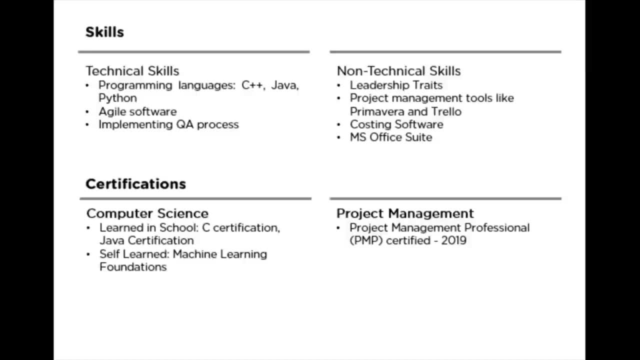 as a project manager, where he not only led projects but also learned new project management tools like Trello and Primavera. After this, add relevant information regarding your education. Your resume must include skills that you have or you have gained in your years of experience. 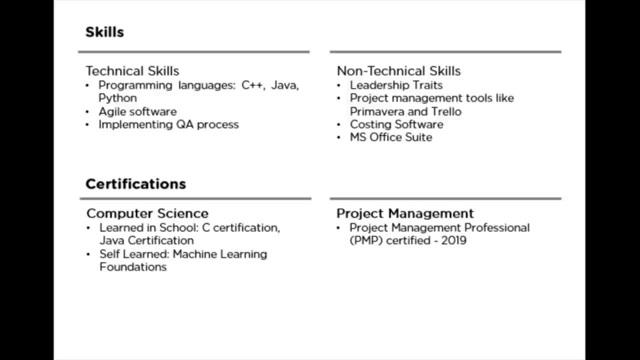 Like here, James Brown has divided his skills into two parts, where he has written his technical skills and non-technical skills. He has included his skill of agile and quality assurance software, as well as he has his knowledge of different project management tools. Then putting your certifications play. 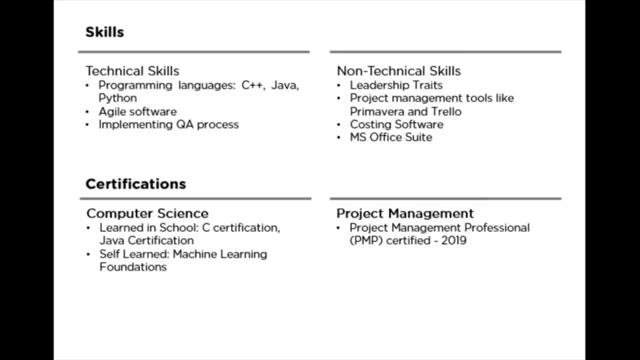 a major role. This proves that you are up to date and updated with current market trends. James Brown has his certifications in C and Java and, more importantly, he has his project management certification- project management professional. In this session, we will discuss about project manager roles and responsibilities. 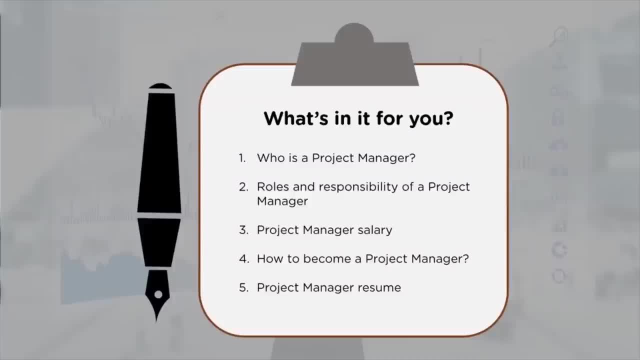 Let's first have a look at all the topics we will be covering today. First, we will see who is a project manager. Then we will check the roles and responsibilities of a project manager. Moving forth, we will analyze the salary of a project manager and the steps that 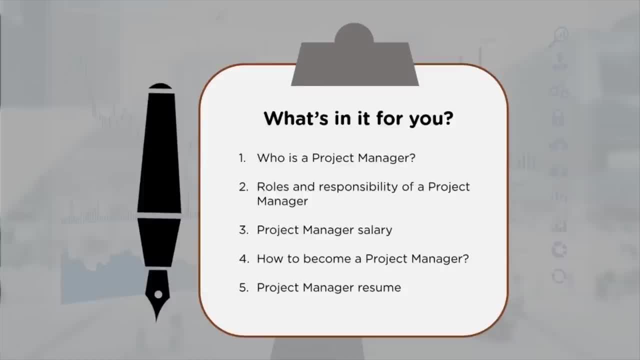 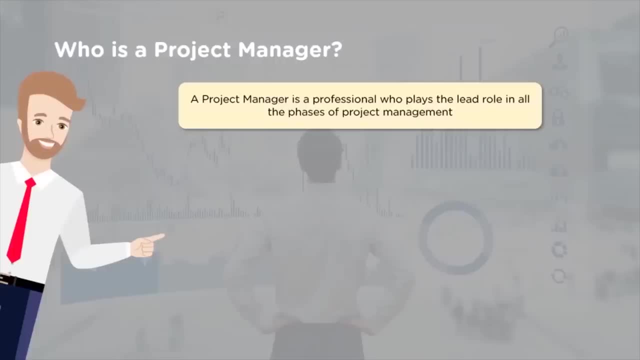 will help us become a project manager. Finally, we will see a project manager's resume. So, without any further ado, let's get started with who is a project manager. Project manager, in simple words, is a professional who manages the project. Project manager plays an integral role. 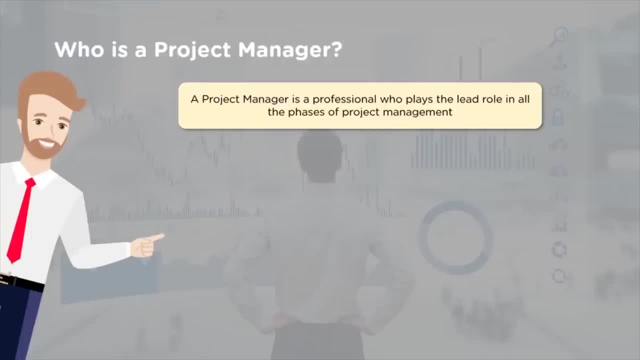 from the first phase of the project life cycle to the last phase of project life cycle. This individual is a part of all the activities that produce the final deliverables and strive towards the success of the project. Now let's get started. Let's consider some must-have skills. 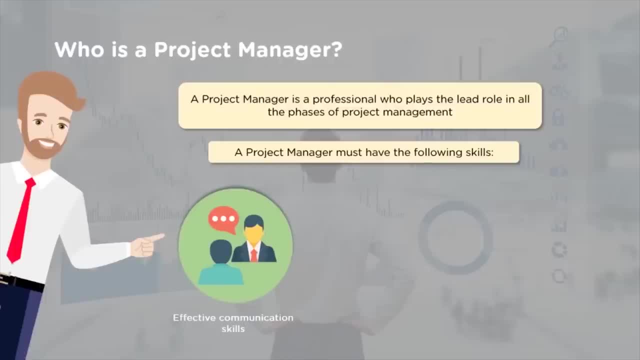 of a project manager First we have is strong communication skills. The communication skills help the project manager to communicate the organization's mission and vision to the team members in a clear, concise manner. These communication skills help project manager to explain their thoughts and. 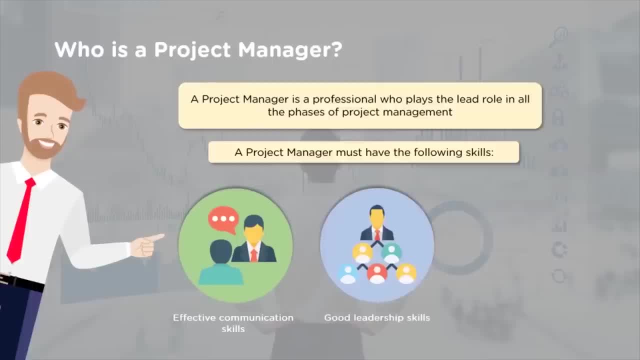 requirements to customers and stakeholders. The next we have is effective leadership skills that helps in forming a team of skilled professionals and lead them in the best possible manner. The next skill that a project manager must have is a team management skill. As a project manager, it is very 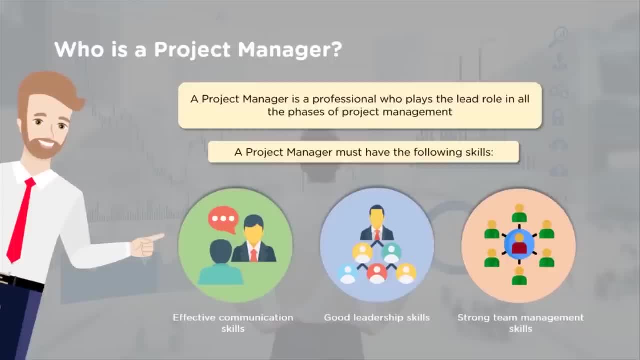 important to know how to manage your team to achieve a common goal with complete harmony. A project manager must have strong negotiation skills, as project managers have to negotiate at each and every step. This negotiation might be with the customers, stakeholders or team members. These negotiation skills. 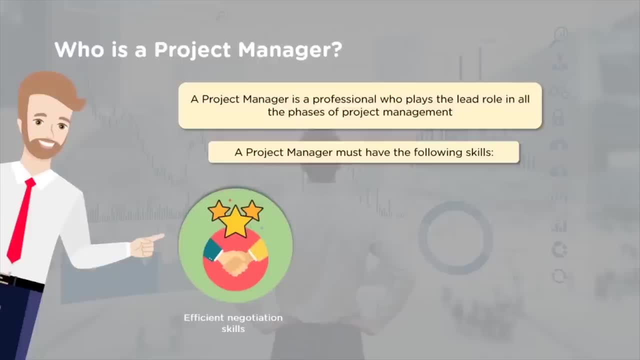 become of utmost importance when project members get into a fight or an argument. Then we have critical thinking. This is a skill that makes a project manager more effective and efficient. in project management, This thinking capability is needed to take difficult steps, talk to stakeholders and resolve. 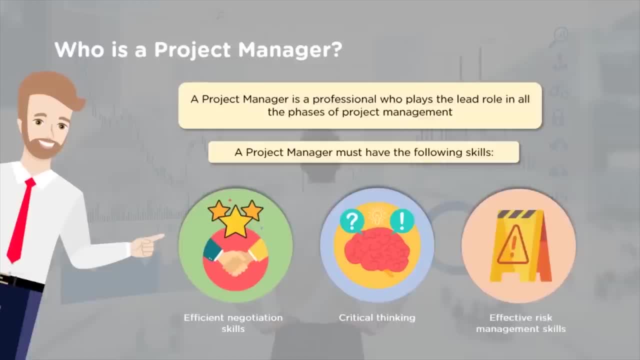 several issues throughout the course of the project. The last skill that a project manager must have is risk management skill. Handling a project is an important step, But what is equally important is risk management. This is the process required to identify, analyze and respond to the risk. 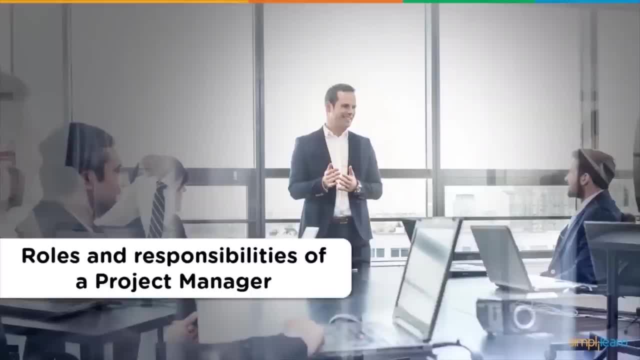 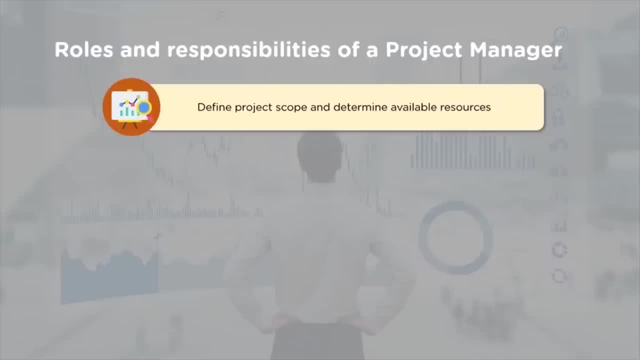 factors throughout the project life cycle. Now, when we know who a project manager is, we must have a look at the roles and responsibilities of a project manager. The first and foremost role of a project manager is to set up a project scope check. 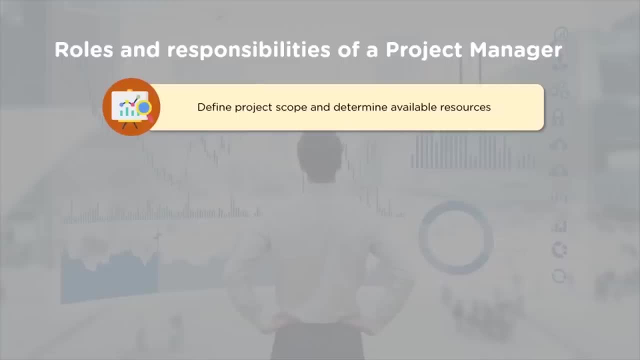 its feasibility and determine the resources that are needed to satisfy the project scope. Second role that a project manager has is the development of a project plan according to the project scope. The plan is needed to encourage the team to hard work with all their dedication. 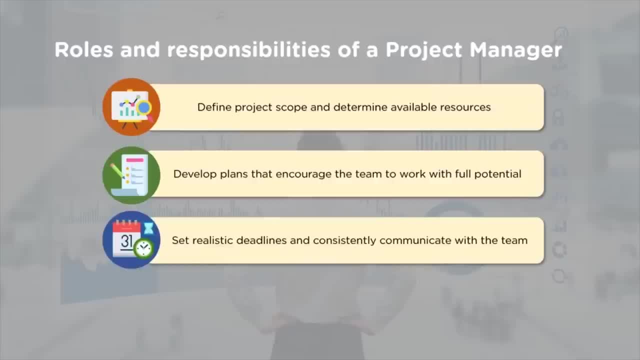 Next, a project manager is supposed to set deadlines for the project deliverables. He or she is supposed to manage time as a priority and communicate with the team at regular intervals. Next important role is to analyze, track and control the budget of the project Project. 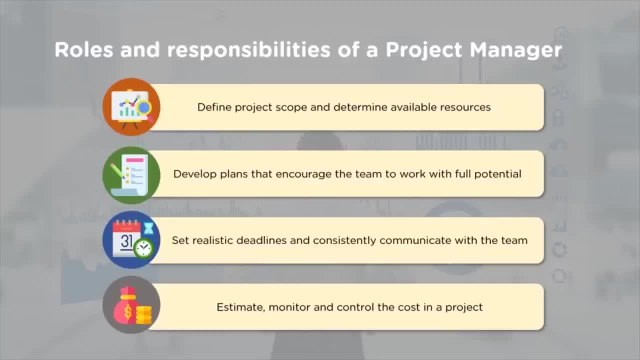 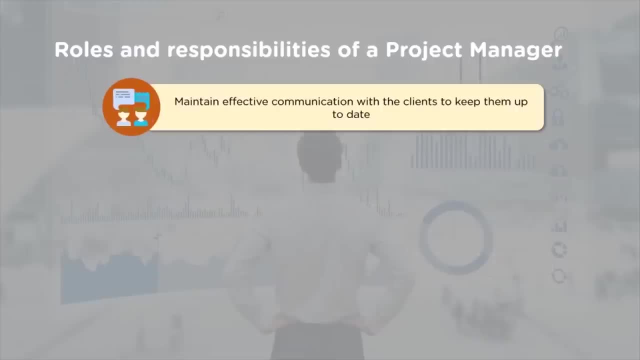 manager has to make sure that the project does not run out of budget and is optimized as possible. Moving forth effective communication is one of the most important skill of a project manager. He or she is supposed to maintain communication with all the stakeholders throughout the project. Then we have is the 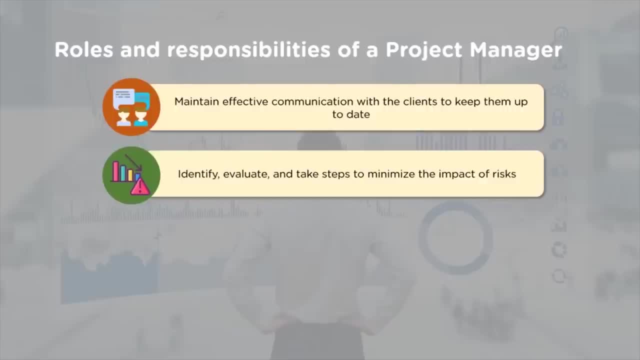 identification and evaluation of risk in a project. Project manager must take steps to minimize the effect of risk in a project. The next role of a project manager is to track and control the performance of the team. This helps in yielding the best outputs with the least number. 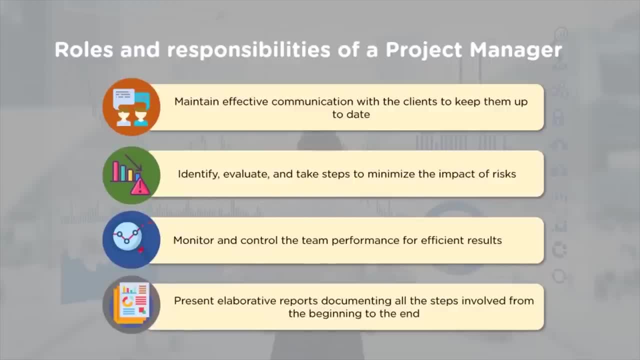 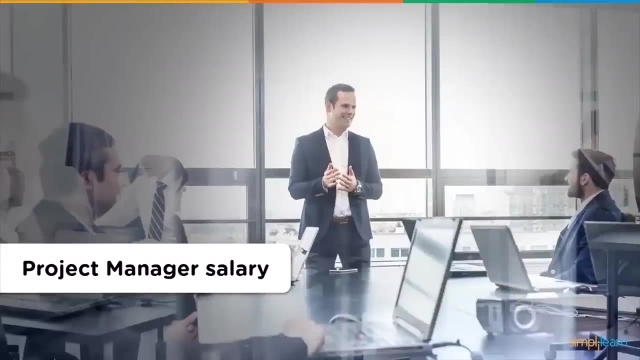 of resources. Last role a project manager must have is to provide reports and documentation of all the steps involved in project management. This helps in future projects and makes sure that the mistakes that happened in the project will not happen again in ongoing projects. Now it's time for us to check. 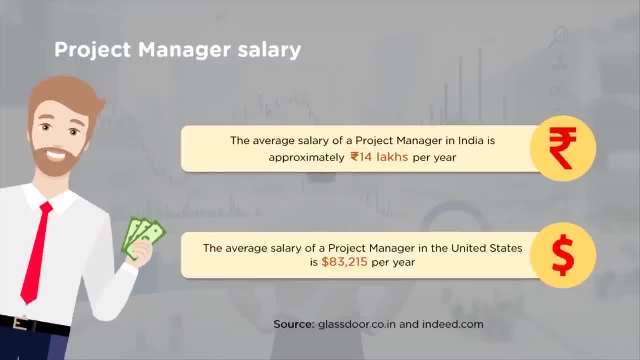 the salary of a project manager. The data shows that an average salary of a project manager in India is approximately 14 lakh rupees per annum, while the average salary of a project manager in United States is 83,215 dollars per year. The next important thing we must learn is: 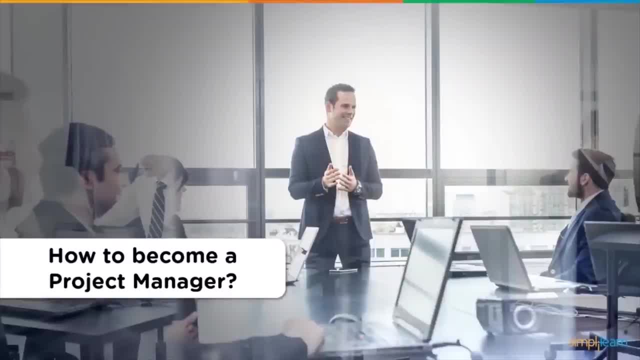 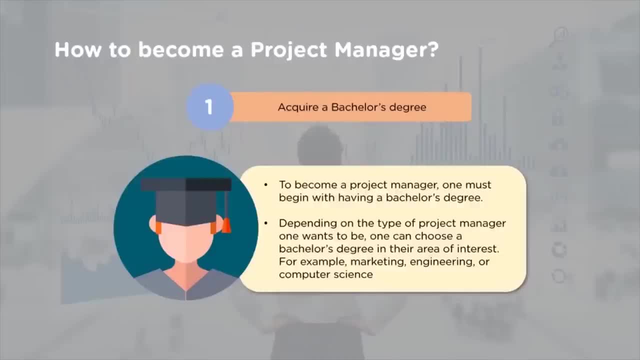 how can we get a project manager's job? There are four important steps that one must fulfill to become a project manager. The first step is to have a bachelor's degree. It is important for a person to be a graduate. One can hold a bachelor's degree. 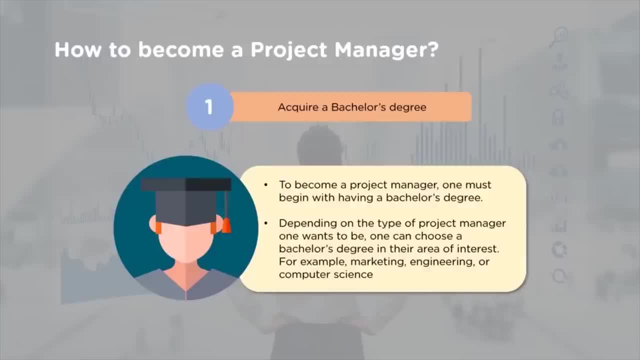 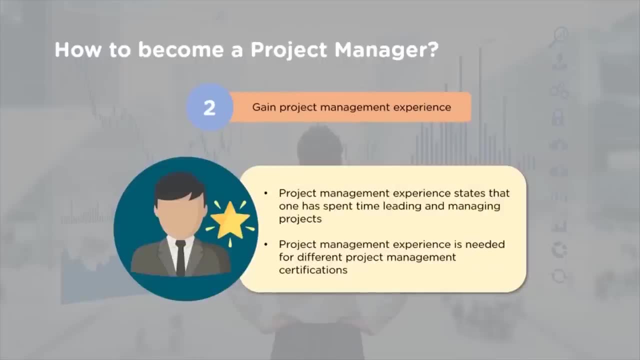 in any area of interest, like marketing, computer science or even engineering. This entirely depends on the type of project manager one wants to be. The second important step is gaining project management experience. This means that a person must have experience in leading and directing projects. Project management experience. 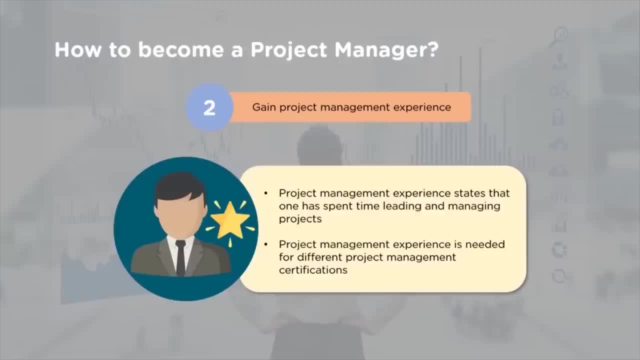 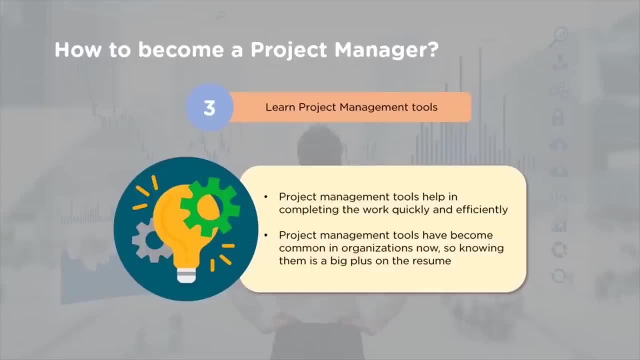 helps in taking different project management certifications, which further help in having a good paying job. The third essential step is to learn project management tools. There are different project management tools for different areas of interest. These tools help in quick and efficient management of work. Project management tools. 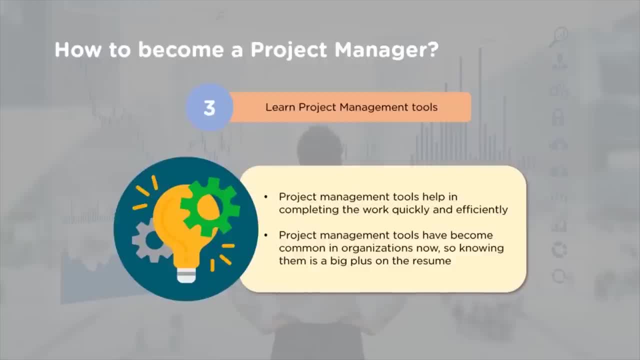 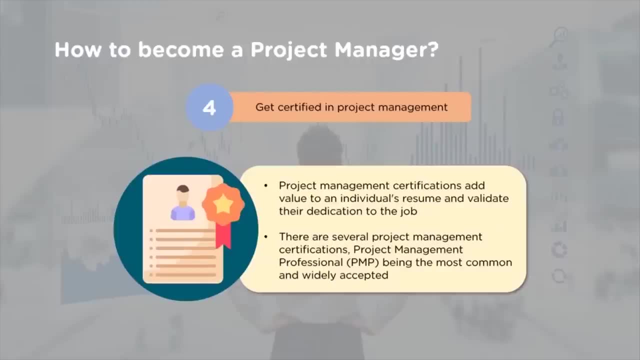 are used widely by organizations. now, Learning these tools will increase the chances of getting selected in one of those organizations. The fourth and the last step is getting project management certified. Project management certifications help an individual to increase the value of their certification and validates their dedication to the job. Nowadays, 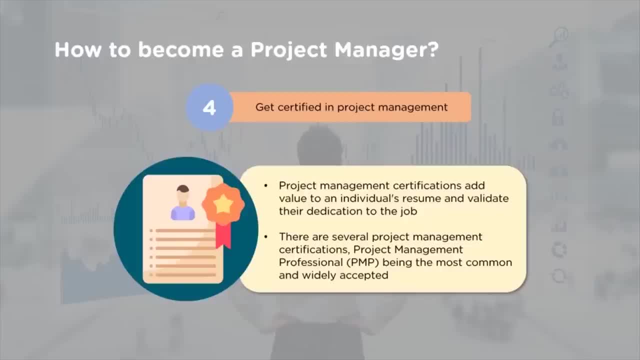 several organizations have made it compulsory for a project manager to be project management certified. There may be several project management certifications, out of which project management professional certification, or PMP certification, is one of the most common and widely accepted certifications. The project management institute, or the PMI. 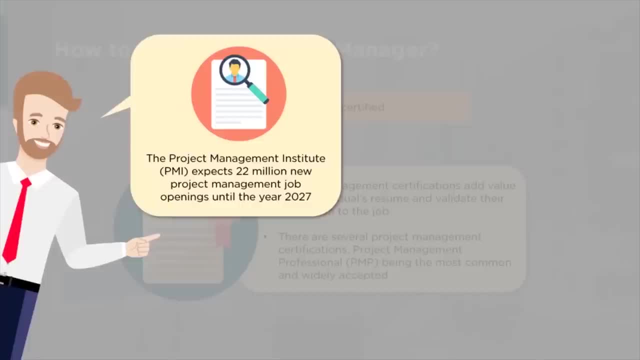 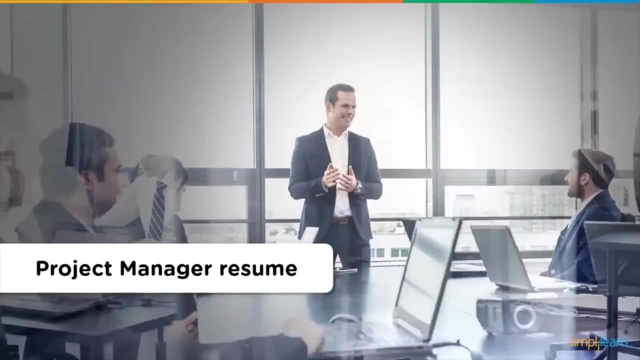 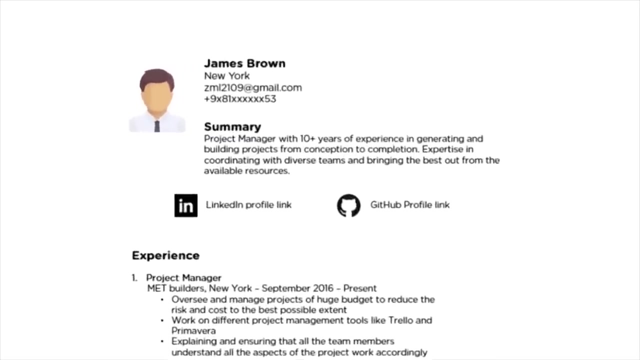 predicts that there will be 22 million new project management jobs by the year 2027.. Now it's time for us to know how a resume of an aspiring project manager looks like. If you are somebody looking for a project manager role or a senior project manager role, then 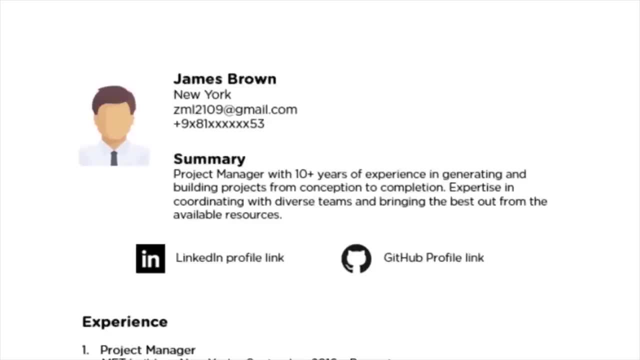 your resume should look something like this: The summary in the beginning would include how much experience you have and anything that supports your claim of being a project manager. Like here James Brown has written: he has more than 10 years of experience with generating. 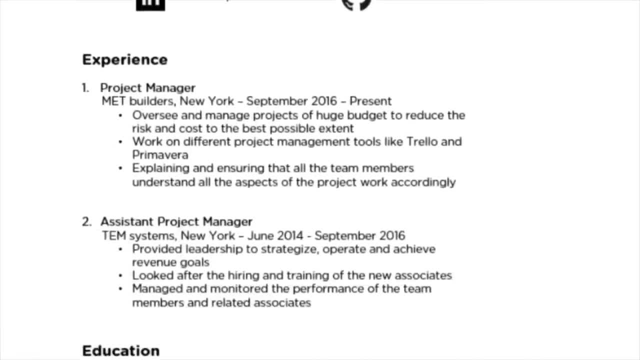 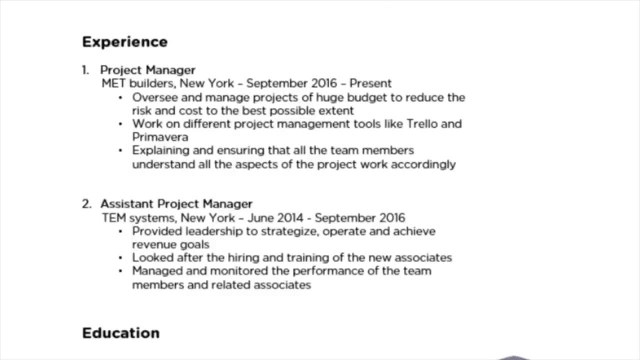 and building projects. Then, when you talk about your experience, you should put something that emphasizes on the responsibilities that you had and your area of expertise. Put something that shows your skill set for the desired post and also something that you learned from your former job role. This: 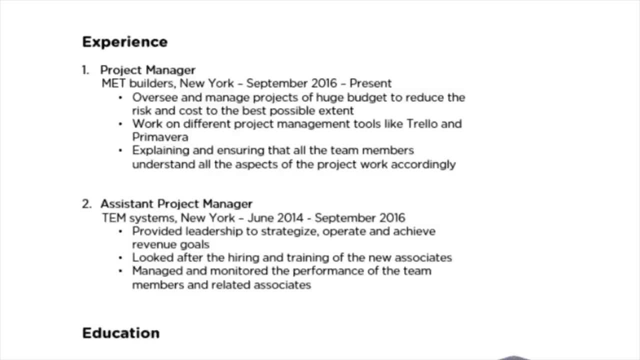 shows that you have command over your work and also the determination to upskill yourself, Like here. James Brown has 3 years of experience as an assistant manager, where he trained new associates, and then 3 years of experience as a project manager, where he not only led projects, but also. 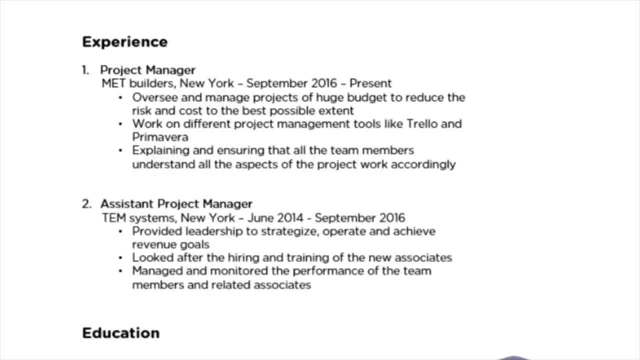 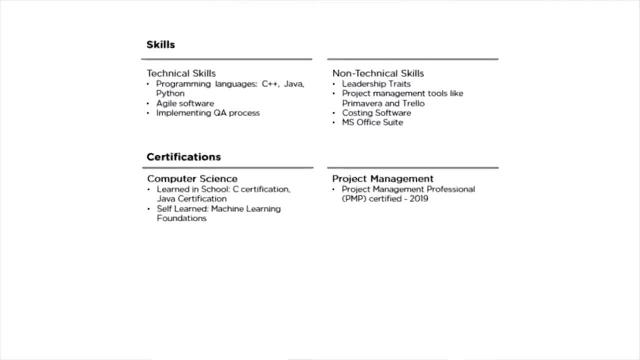 learned new project management tools like Trello and Primavera. After this, add relevant information regarding your education. Your resume must include skills that you have or you have gained in your years of experience. Like here, James Brown has divided his skills in 2. 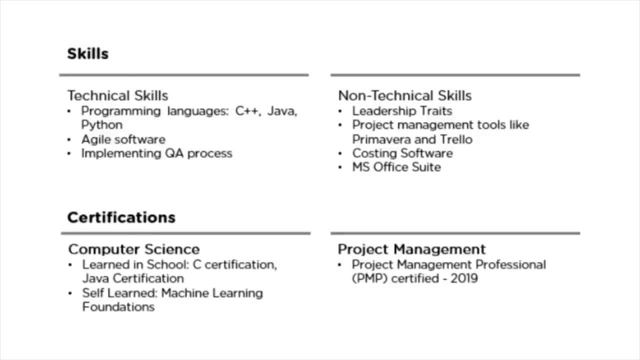 parts where he has written his technical skills and non-technical skills. He has included his skill of agile and quality assurance software, as well, as he has his knowledge of different project management tools like Trello and Primavera. Then put your certifications play a major role. 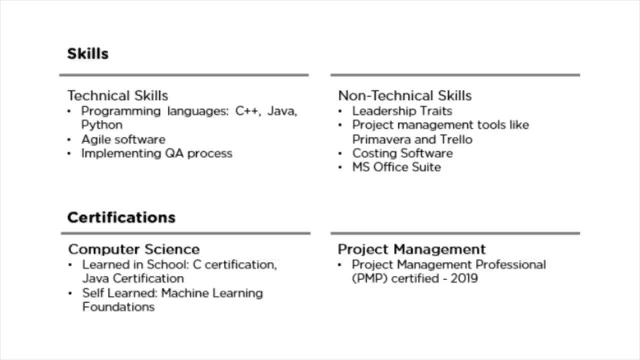 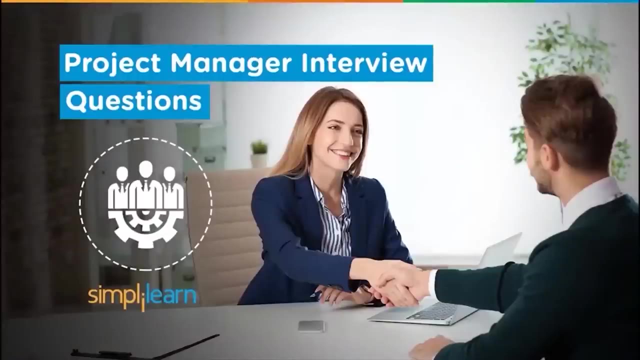 This proves that you are up to date and updated with current market trends. James Brown has his certifications in C and Java and, more importantly, he has his project management certification in project management professional, or PMP. Here, as part of this video, we are going 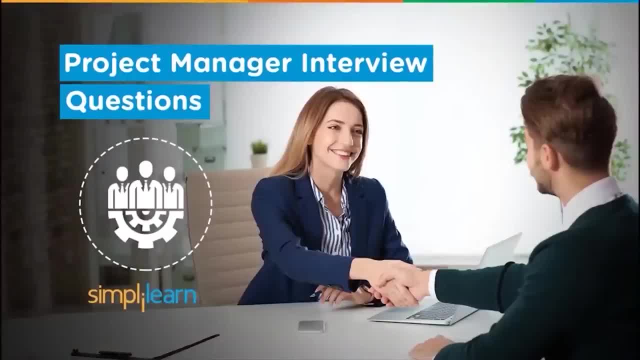 to look at few possible questions which one would face while going through an interview. This will help them to prepare for interview and also help to understand what kind of questions would come across when they face the interview. In addition to that, these questions also has an insight towards: 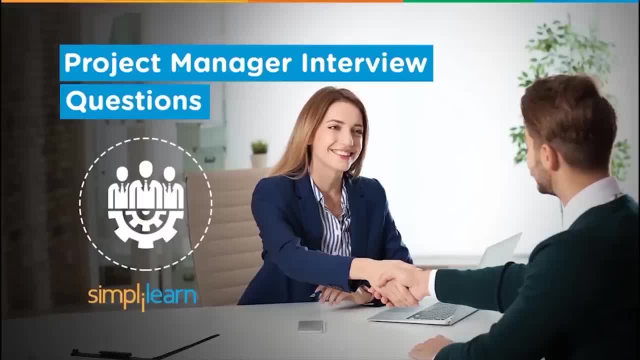 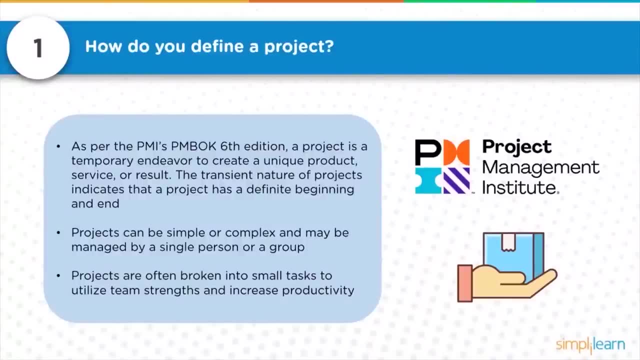 the role of project management itself. So let us look at one by one Question number 1. How do you define a project? So, as per the PMI's PMBOK 6th edition, a project is a temporary end-over undertaken to create. 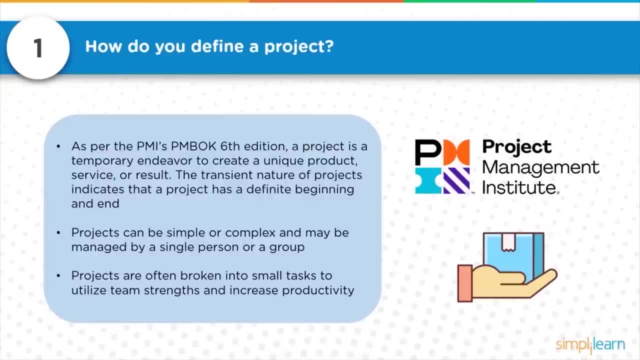 a unique product, service or results. The temporary nature of projects indicates that a project has a definite beginning and end. So when we say this temporary end-over undertaken to create a unique product, service or results, each project will have a definite start date and end date. 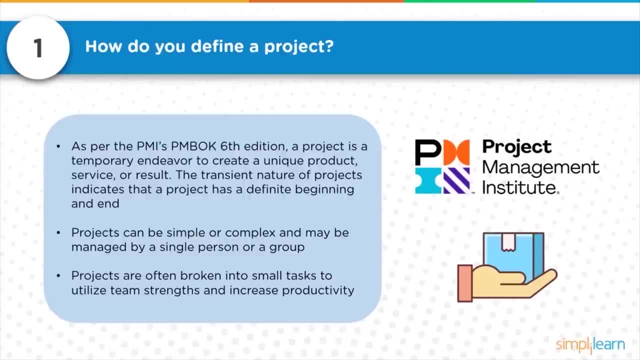 Once the project team is formed, once the project objectives are achieved, so the team which is formed, the human resources which are onboarded to a project, So those are disseminated, sent back to their respective functions or departments and project will be concluded as. 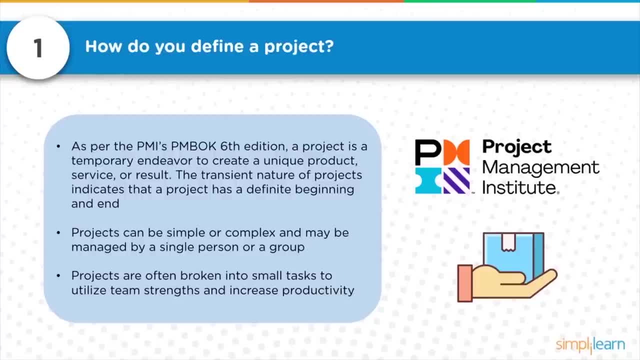 complete. So project can be simple or complex and may be managed by a single person or a group of them. So every project will have a life cycle. So from beginning to end it starts and end where it acquires lot of resources, where it will divide. 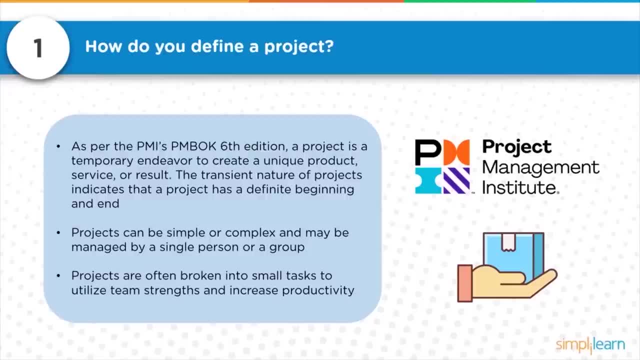 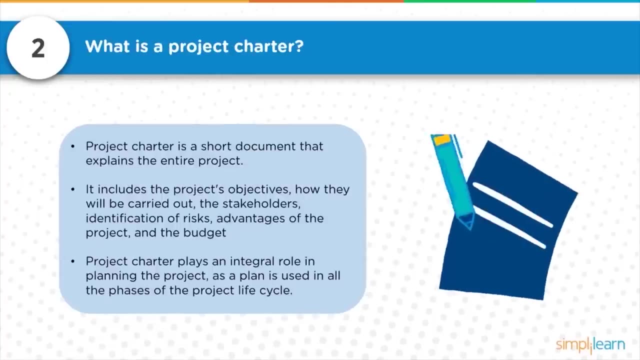 the project life cycle into multiple stages or phases where project is being done and deliverables will happen through the milestones during that life cycle. So projects are often broken into small tasks to utilize team strengths and increase productivity. Question number 2: What is a project charter? 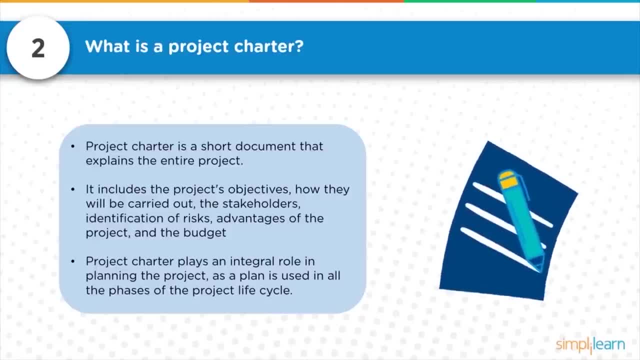 So project charter is a short document that explains the entire project. So this will become a basic document which will be given to a project manager so that a project manager can understand what is a project management is all about. So this document would include the objectives of the project. 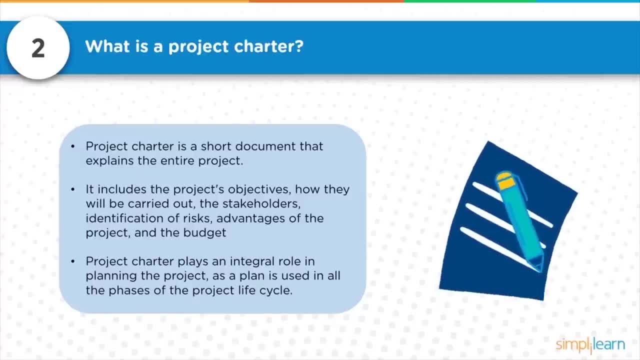 how will they be carried out, who are the stakeholders? identification of risks, advantages of the project and the budget. So project charter plays an integral while planning the project as a plan is something that is used in all the phases of project life cycle. It is very essential. 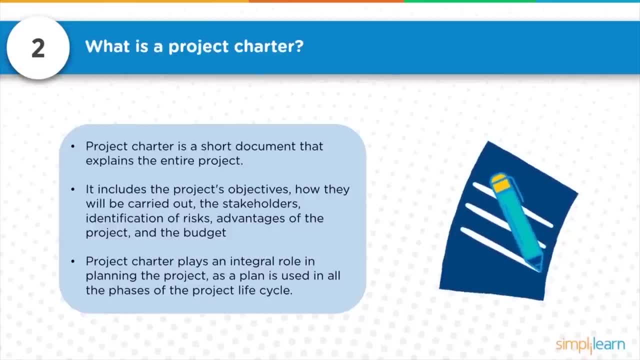 because it provides all the necessary insights. a project manager is needed while taking up the project. After getting the project charter, the first job a project manager supposed to do is to identify the stakeholders, Even though project charter will have a basic list of stakeholders. so, project manager, 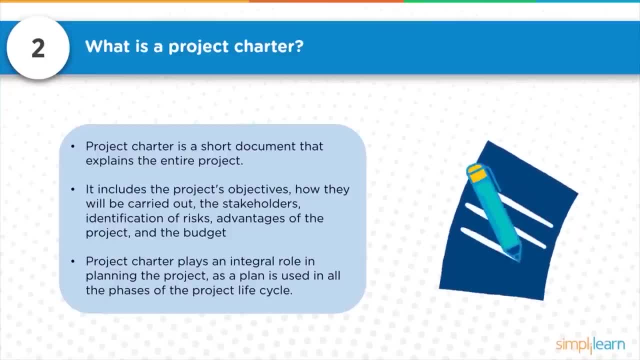 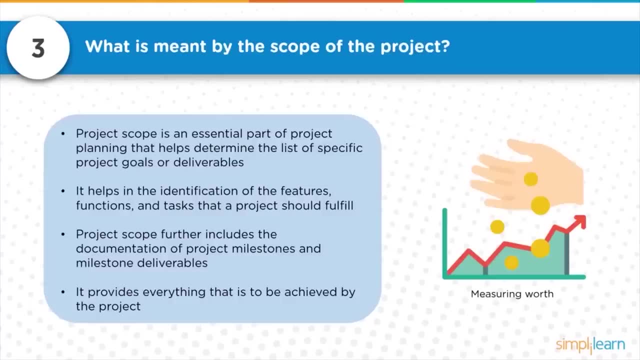 has to contact those stakeholders, establish the list of stakeholders for the project, understand the requirements in detail and further move towards planning What is meant by scope of the project. So project scope is most essential part of project planning that helps in determining the list of specific. 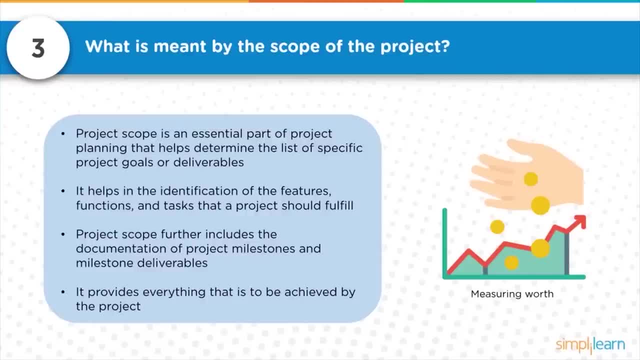 project goals or deliverables. So when we say this project will have a definite unique deliverable which has to be created, So this will have a specific description of the specification as well as the features, functionalities of the deliverable, So to accomplish that features, functionality. 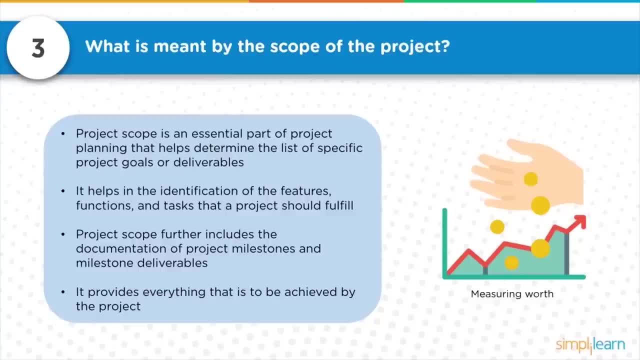 of that output, what we are going to create as a result of a project. within a project, lot of activities are done. The processes, the tools, the resources which are utilized for the project- all falls under this scope. So when we say the term scope, it is very important for us to understand. 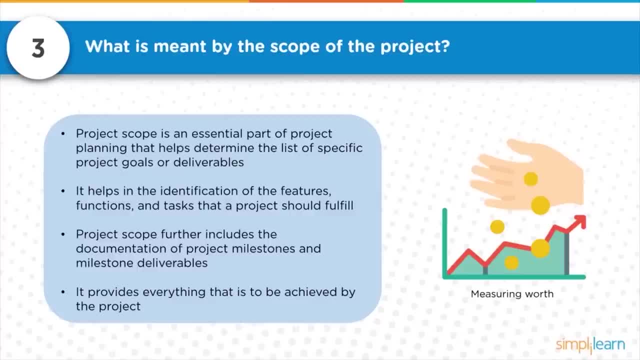 the scope of a project versus scope of the product. The scope of the project involves all those processes, resources and activities, what we do to accomplish the result, Whereas product scope is the one which we speak about, that result itself, the features, functionalities of that result. 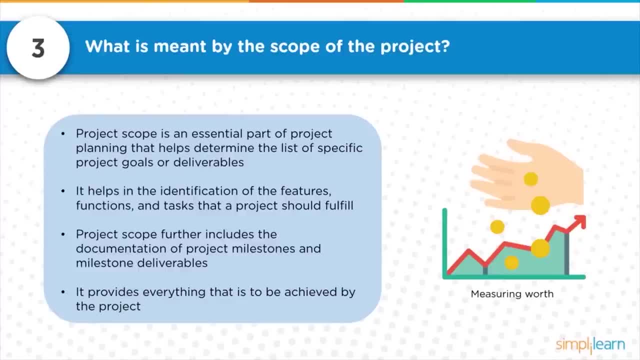 itself. So one needs to understand the difference between this project scope and product scope and define accordingly. So this will help in identification of the project's output and why that output is created and how this particular product or services or results will help organization or business to accomplish their 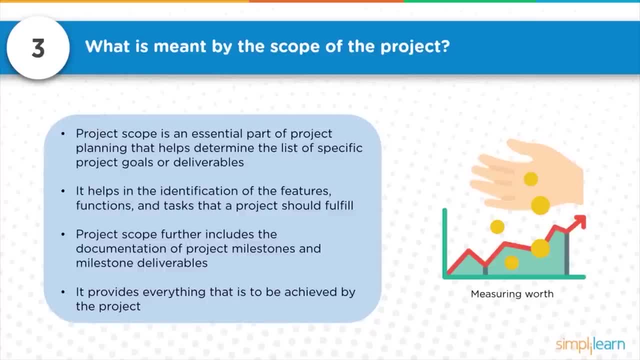 objectives. This should be the basic understanding a project manager should have. So it includes everything that is to be achieved by the project, which means all those results, what needs to be achieved, all those value which has to be created by the results. So we need to keep in mind 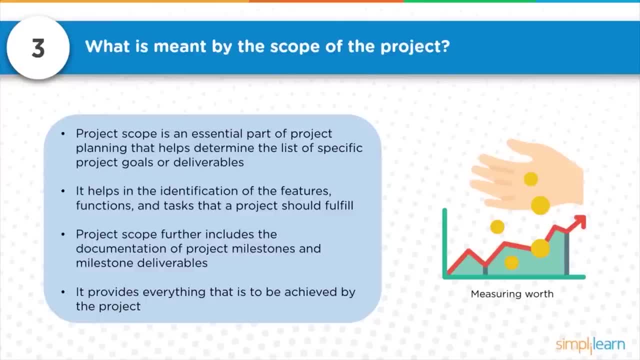 the result itself is not the ultimate objective of an organization. It is not. Instead, the result will help organization to accomplish their objectives. For example, if you take in HR department, if they introduce an intranet portal for claim processing. So the application, what is created as part of the 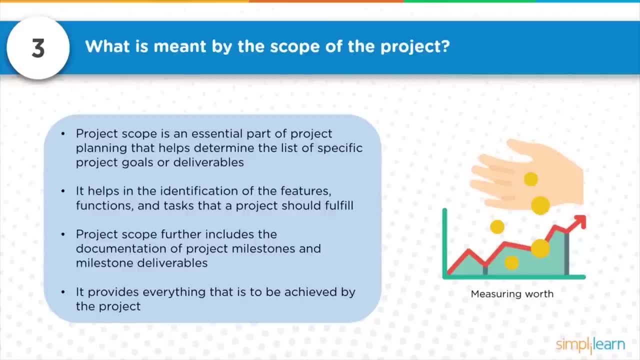 exercise of initiative where my employees should submit their claims through a specific portal. Now, that is to reduce the time, the processing duration, as well as the efficiency and effectiveness of the processed claim, what is submitted. So this is an outcome, So keeping that outcome the objective. 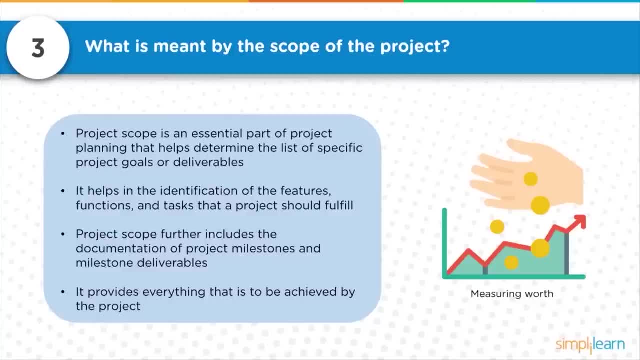 this portal is created. That portal itself has the features and functionalities which project will focus and create that results. So through that result, organization would accomplish their objectives. That should be kept in mind. So understanding the scope is essential. So, while understanding the scope, also need to. 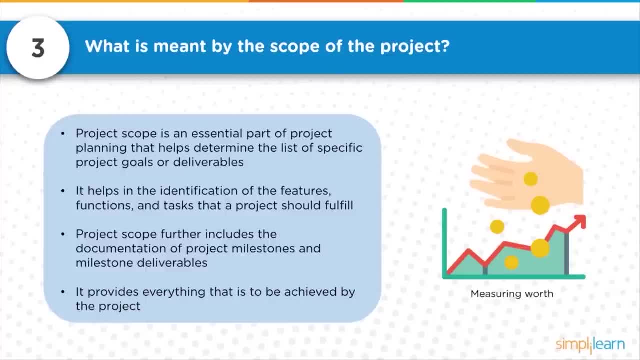 understand how this particular output- the product results- is going to add value to the business. What is the outcome of that? That is also very important to understand. One is understanding the scope, Ensuring the project is delivered within that scope and all that required to be done to accomplish that scope. 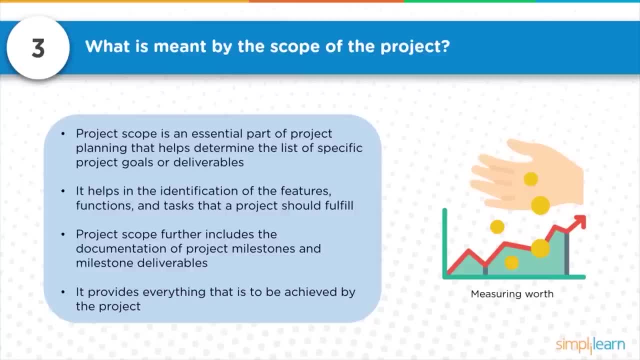 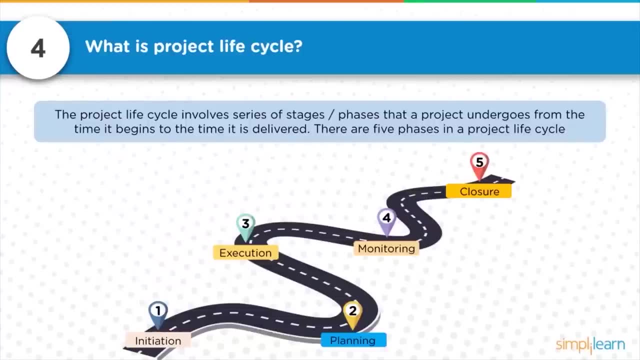 has to be done, and only that, Not anything more than that, Not anything lesser than that. What is project life cycle? As I was mentioning during the question 3, there is a project scope, So project itself has a life cycle, So this project scope falls under. 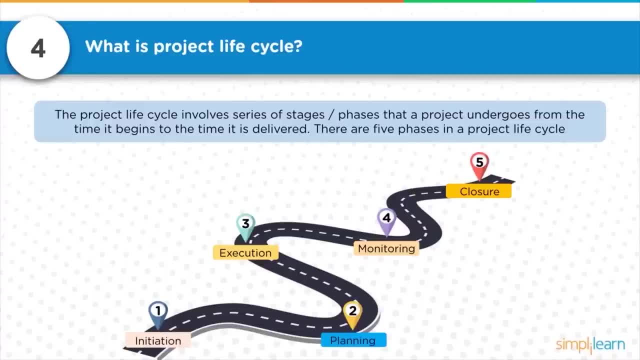 this project life cycle. So project life cycle refers to the beginning and end of the project. So there is a life. So you initiate a project, trigger a project, project is actually started and as it starts, it progresses, creating the results, and then it ends. 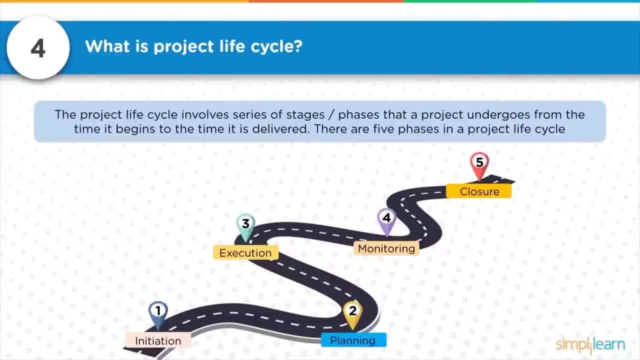 Project can end in various different scenarios. One is by accomplishing the objective of the project, the ultimate results, the deliverable it creates and then ends. Or project may also get closed prematurely. So we are not going to look at the why the project is. 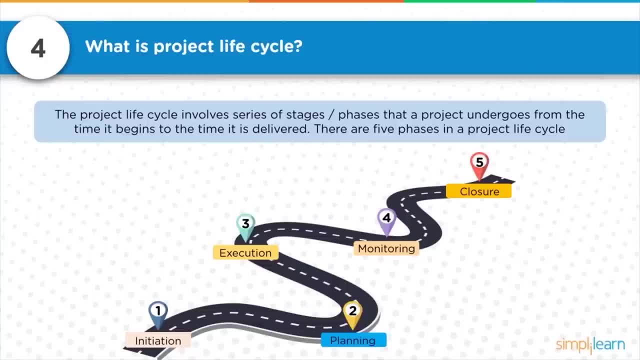 going to close prematurely. at the moment, Our idea is to understand what is project life cycle and to visualize that. So this entire span of time the project spends, from the beginning to end, It involves various different stages or phases, whatever the term you want to call it. 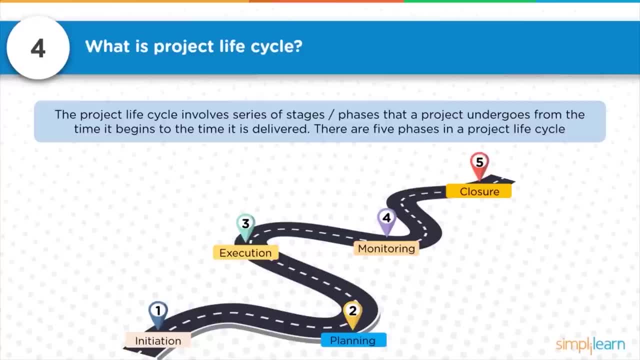 And in each of these stages or phases there is a milestone: deliverables which are measured and that will be part of the ultimate deliverable: What is going to be delivered as a result of a project. So it involves all the activities, all the processes. 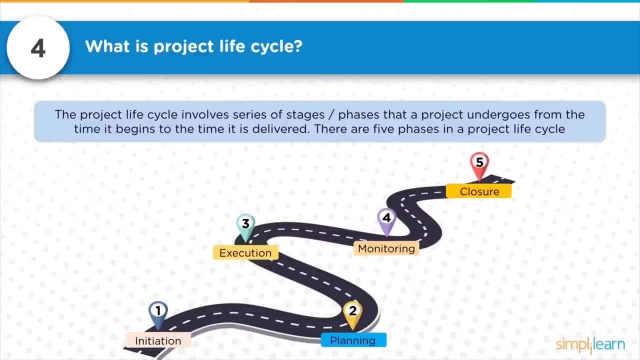 all the resources which needs to be acquired, managed and then the results needs to be accomplished ultimately. So here in a project life cycle. it involves five process groups, which mainly focuses on different, different activities and dynamics of the project, Which we call it as initiation process group. 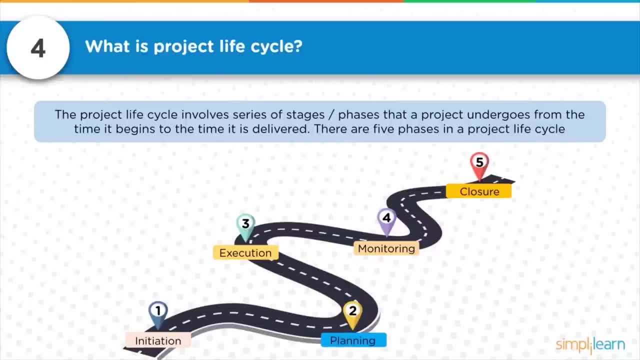 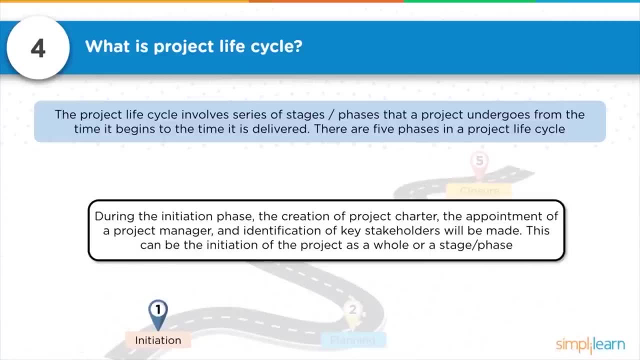 planning process group, execution process group, monitoring and controlling process group and closure process group. So during initiation process group, the creation of a project charter, appointment of the project manager and identification of the key stakeholder will be done. This can be initiation of the project. 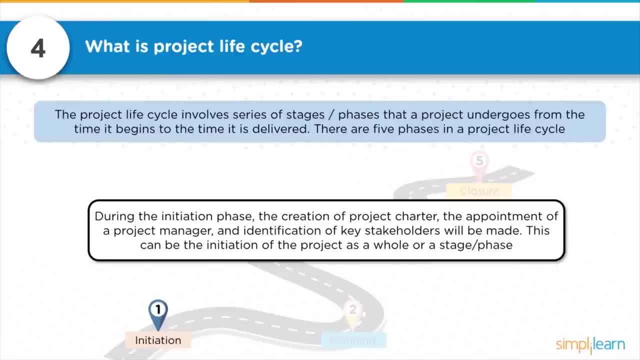 as a whole or as a part of a specific stage or a phase. Now, all this process group, what I mentioned- initiation, planning, execution, monitoring, closure- all of these process groups can be looked at their involvement in the entire project life cycle at the 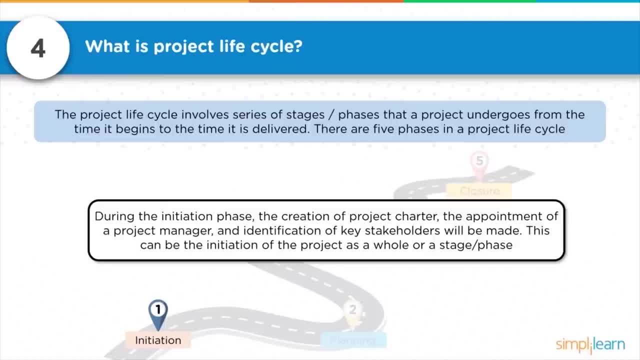 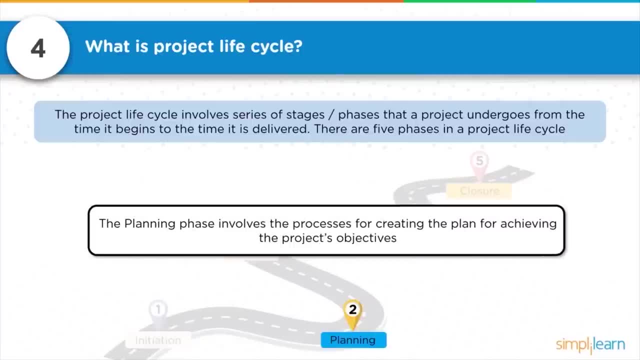 same time it can also be seen as part of a single phase. So each of the process groups are applicable, like initiation of a project, if I say similarly initiation of a stage or a phase. So the planning process group involves the process of creating the plan for achieving the project's objectives. 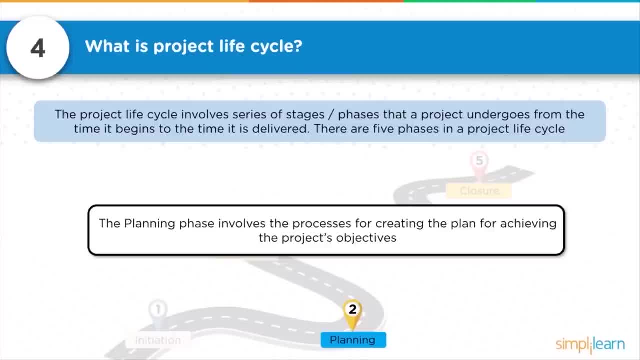 So this would create the detailed plan for entire project or a skeleton plan for a project if it is an agile or rolling wave project. If that approach is taken, like rolling wave or progressive elaboration or agile approaches, then the skeleton of the project plan is created. 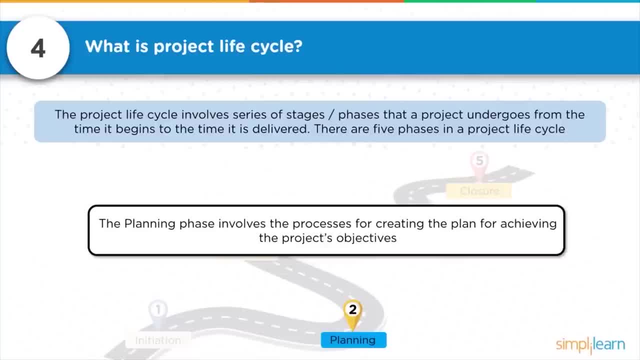 If waterfall approach is taken, it is quite obvious: the comprehensive, the detailed project plan will be created. Project management plan is also involved in this. Now, in addition to this, as you progress in the project, for each stage or a phase, there needs to be a plan which is: 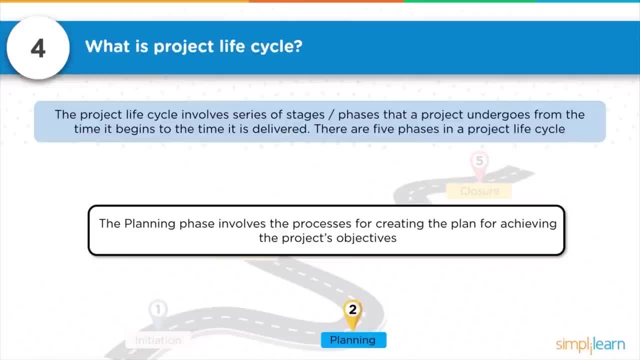 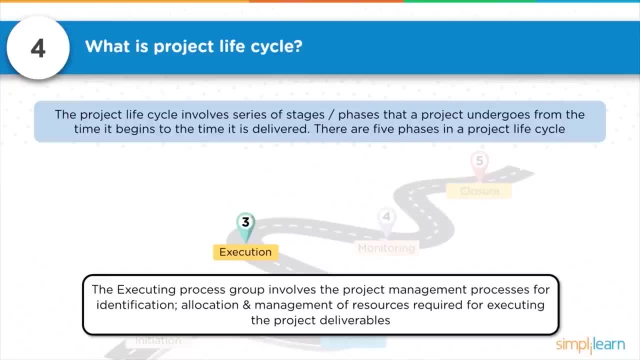 detailed further compared to the project plan itself, Which will become ultimately part of big plan of a project. The execution process groups involves the project management processes for identification, allocation and management of resources required for executing the project deliverables. So here the actual execution happens. 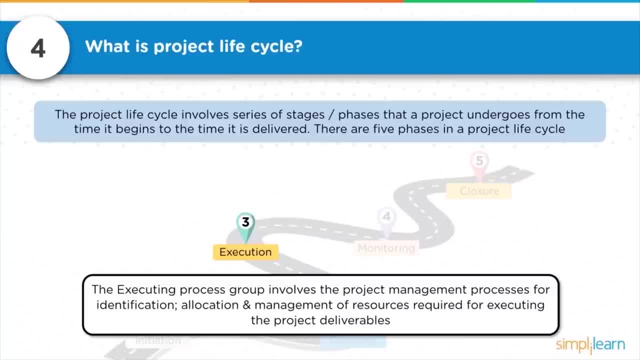 Being a project manager, the focus should be on managing the project. So many a time I have seen project manager is going and doing tasks Looking at the task level- transaction level- which was not project management. so one needs to ensure the project management is not. 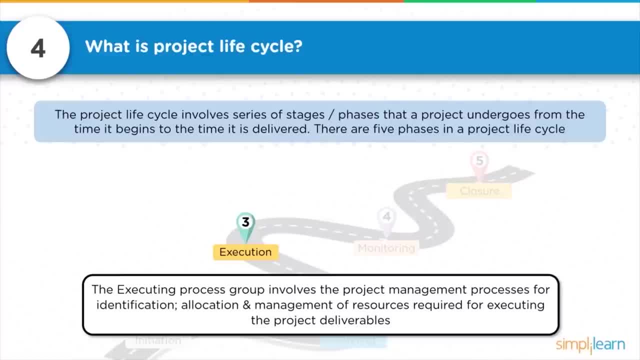 about deliverables in terms of doing the tasks. It is about getting the deliverables from the team. So active involvement in terms of acquiring the resources, checking whether the accomplishment of results has happened, needs to be done throughout the project life cycle. So it is all about directing and manage project works. 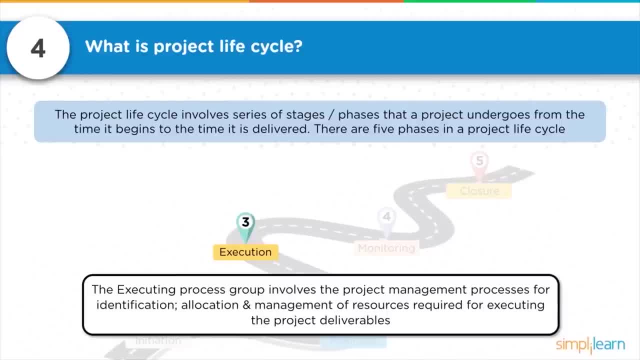 and, at the same time, managing the knowledge which is acquired during the project life cycle. The monitoring and controlling process groups involves the process for project manager to monitoring and controlling the project. Now this involves reviewing. this involves creation of reports. this involves concluding: yes, project has delivered. 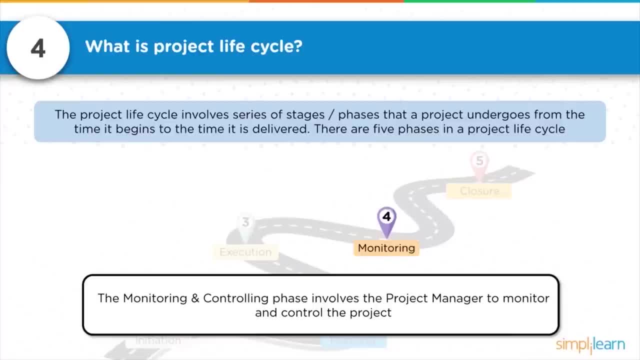 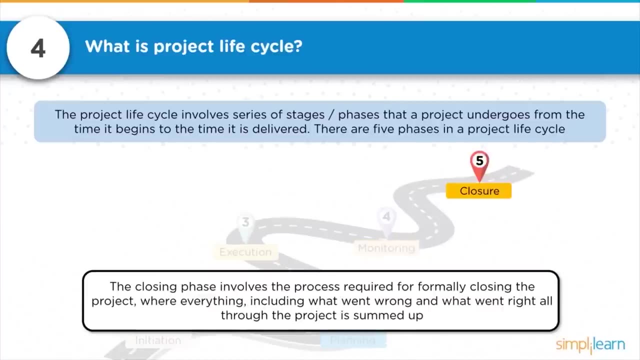 or not delivered, identification of the deviations and initiating with the change request for necessary corrections. So monitoring and control will be done throughout the project life cycle and only with an effective monitoring and control we can see the success in a project. So the closer process groups. 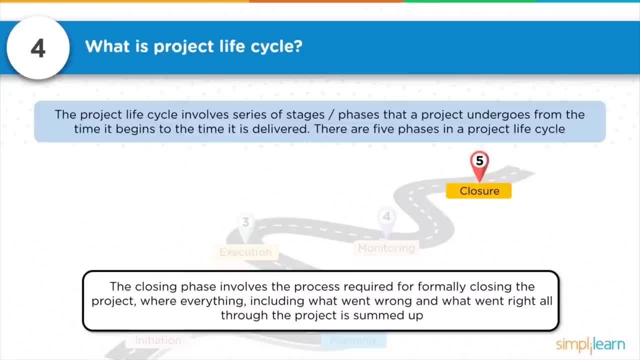 involves the process which is required for formally closing the project, where everything, including what went wrong and what went right all through the project, is summed up. So here, especially in the closing process group, we will not focus on acceptance of the deliverable. instead we will focus on sign off. 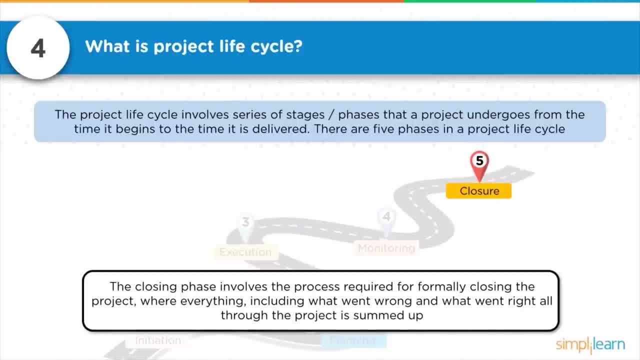 capturing lessons, learnt all the formalities which needs to be completed as part of a closure, Then where are we going to accept the deliverables? this happens in monitoring and controlling. So, while doing the monitoring and control, we will validate against what is planned, comparing with what is being delivered. 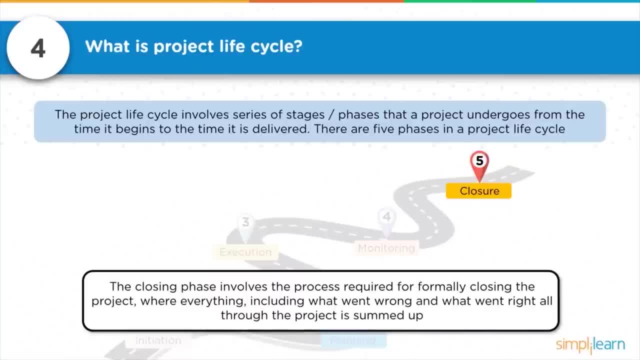 So when we compare both, one would understand what is delivered versus what actually was planned. So there acceptance happens. Once the acceptance happens there, only then the project moves towards closure Project or phase either of that. So when we say closure process group, it involves the process for closure of that phase. 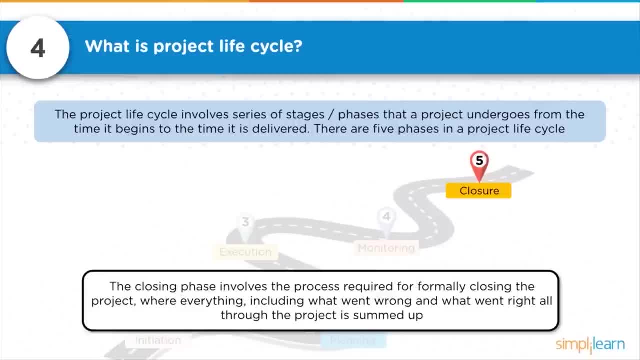 whether accomplishment of all the objectives, all the deliverables of that phase is done or not is checked. if it is a phase, If it is a project in the project perspective, if everything is complete, is checked and then it moves to closing process group, where the lessons learnt, the formal sign off, 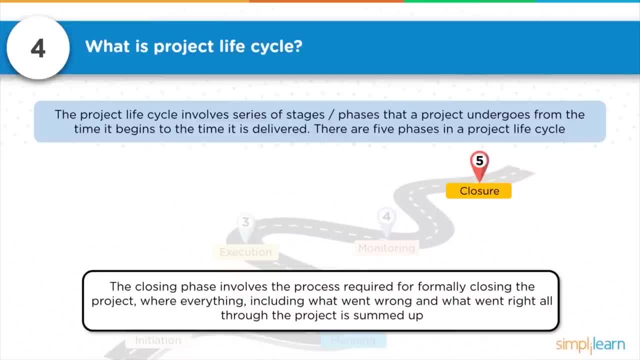 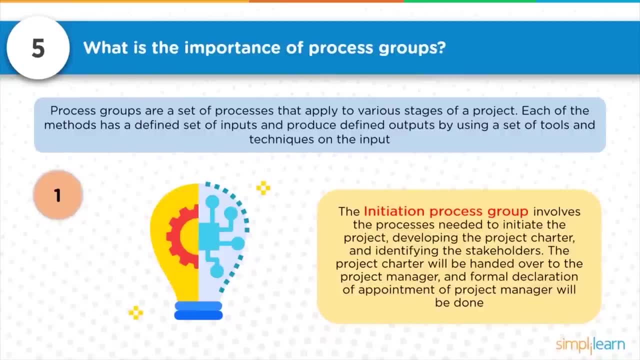 everything will be done as part of this closing process group. What is the importance of process groups? So, process groups are set of processes that are applicable to various stages of the project. as I mentioned earlier, Each of the processes has a defined set of inputs and produced. 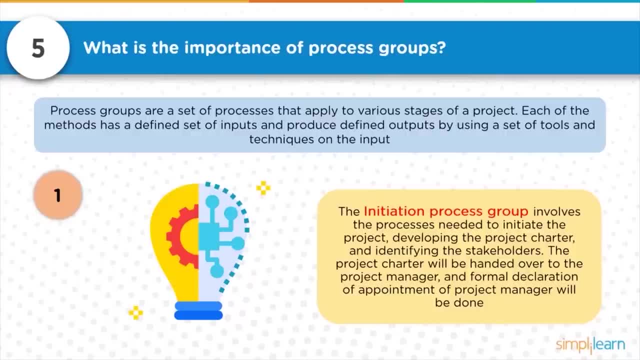 defined outputs by applying a set of tools and techniques. on the input, The initiation process groups involves the processes needed to initiate the project, that is, develop project charter and identify stakeholders. the two processes: The project charter will be handed over to the project manager, and formal declaration of 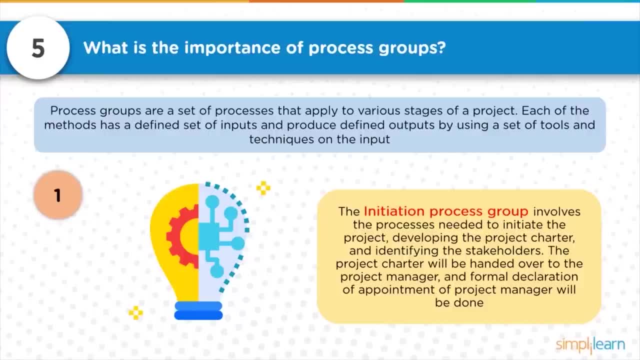 appointment of the project manager will be done. Further, project manager has to identify the key stakeholders and take forward the project as per the direction set in the project charter. So in this group, in this process group, initiation process group, it is a formal declaration. 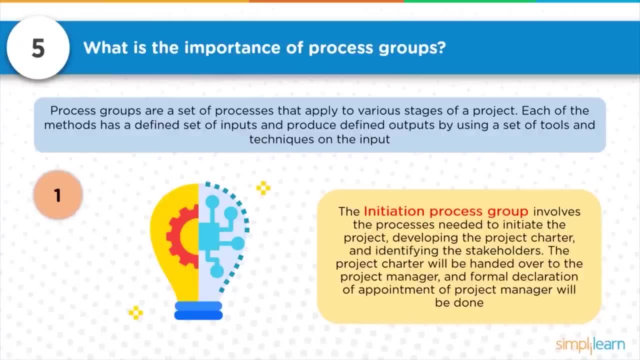 of appointment of project manager to the project. But one needs to remember should not get confused. in real time we see an individual who is about to become a project manager for a project sits and create a project charter. We have seen that in reality. So does it mean? 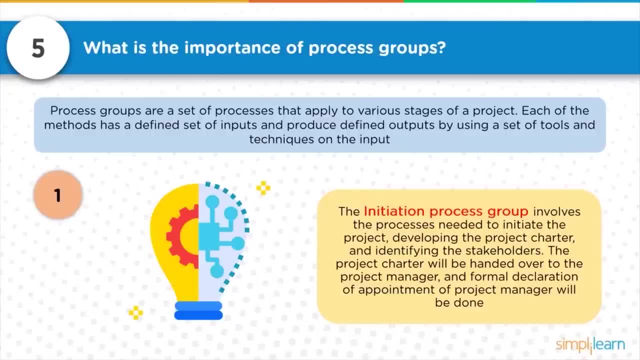 that what is told here is wrong compared to what is practiced. That is not the idea Many organization thinks. if we involve the project manager to be project manager of a project while creating the project charter itself, the level of information, the detail that person will have about a project will be. 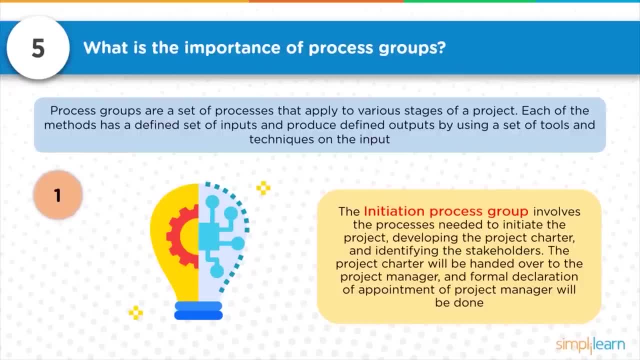 more compared to a person who will become a project manager after handing over the project charter. So there is a difference. The person takes the project charter and become aware of the project. That is one scenario. The person actively involved in creating a project charter. 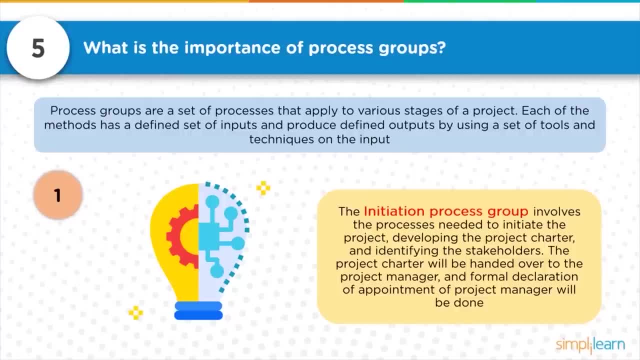 and then become a project manager. That is better scenario where the person will be more informed. But ultimately the accountability of a project charter lies with the sponsor. Formal declaration of appointment of project manager. confirmation of that happens only when project charter is approved and handed over. 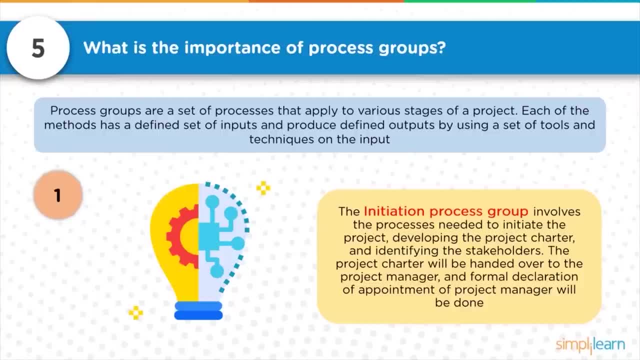 to the person who is to be project manager. So that is where actual initiation of project happens. Then project manager can move out and start identifying the stakeholders and start collecting the details of the stakeholders, their requirements, And stakeholders cannot give all the requirements coming to their mind. They 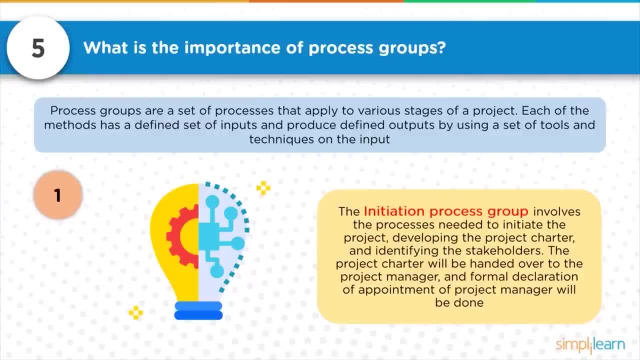 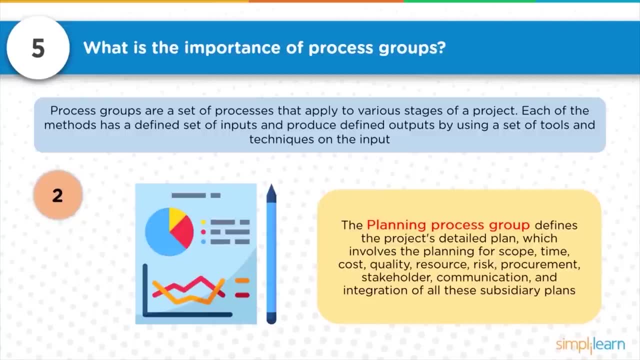 need to restrict to those project detailing what needs to be provided. The planning process group defines the detailed plan of the project, which involves the planning for scope, time, cost, quality, resource risk, procurement, stakeholders, communication and integration of all the subsidiary plans. 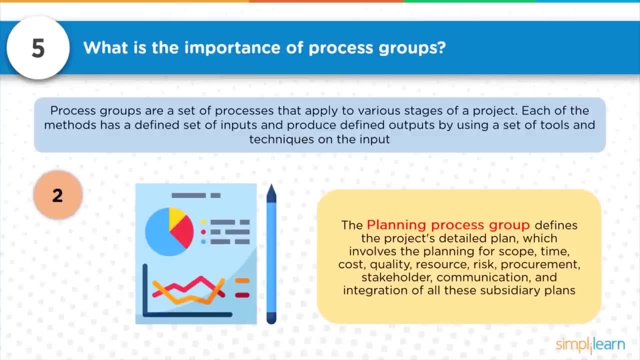 Each of these plans, like scope management plan, schedule management plan, cost management plan, quality management plan, resource management plan, risk management plan, procurement management plan, stakeholder engagement plan, communication management plan. So all these plans are called a subsidiary plans. So all these plans. 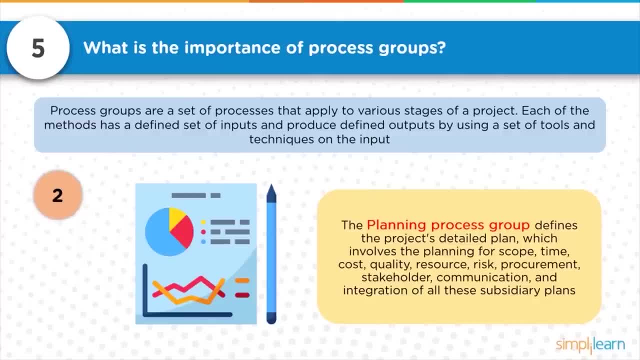 are integrated and detailed project management plan will be created. So this involves various tools and techniques like expert judgment, meetings, analogous estimation, parametric estimation, decomposition, PERT, critical path method, depending on the specific area which is been focused on while planning, For example, expert judgment. 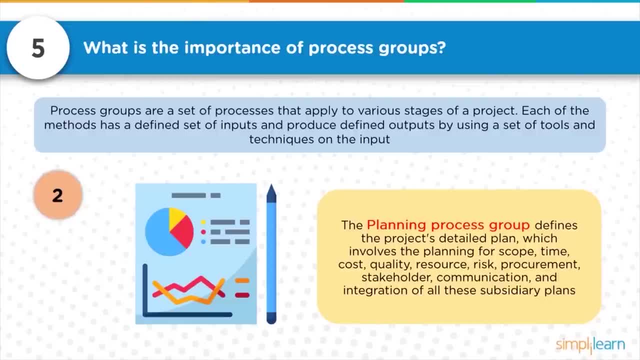 is a common technique used across all the areas like scope, time, cost, quality, all of these nine areas, knowledge areas which I was mentioning- expert judgment meetings are mostly seen as a technique used during each of these planning, Whereas when it comes to critical 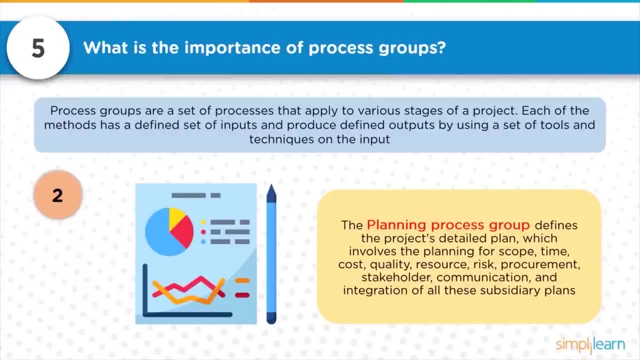 path method. so critical path method is about scheduling. So we will see that technique only mostly in schedule management. Similarly, if I speak about decomposition, we see that in scope management. So likewise there are specific techniques which are specific to a specific knowledge areas. 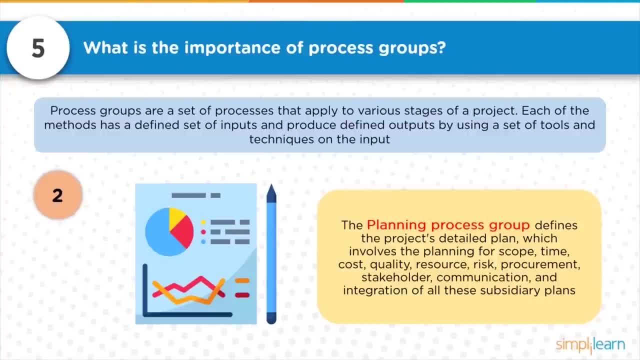 which we need to identify as we go through the entire framework itself. Similarly, there are common techniques used across the knowledge areas which, if we can identify that common techniques which are used across knowledge areas, it is easy for us to remember and recall those. Similarly, specific techniques. 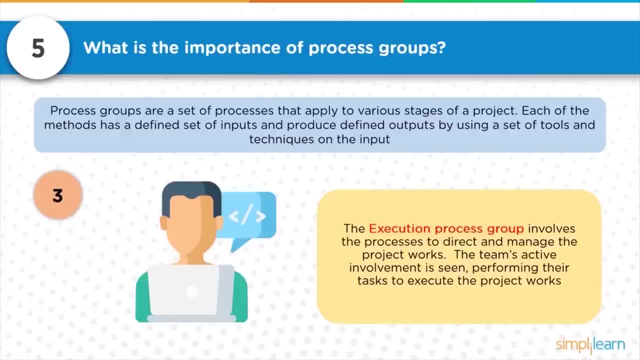 for a specific knowledge area. The execution process group involves the processes to direct and manage the project works. The active involvement of the members of the team is seen performing their task to execute the project works. Although the project plan is finalized, there may be changes in requirements that come. 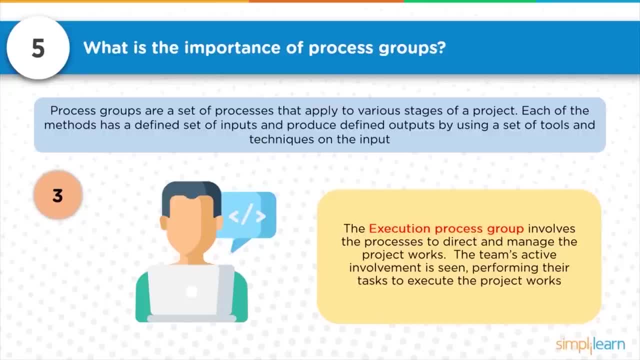 from the stakeholders which are considered for further modifications. So, actual involvement of team delivering something, acquiring the team, onboarding the team onboarding the supplier, identification of them, doing the bidder conference, engaging with stakeholders, all these actions should happen. So, because the main focus of 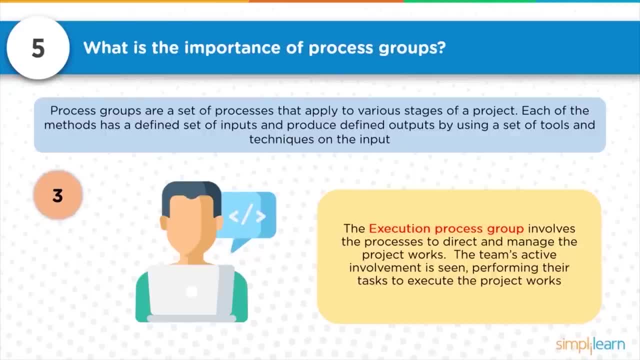 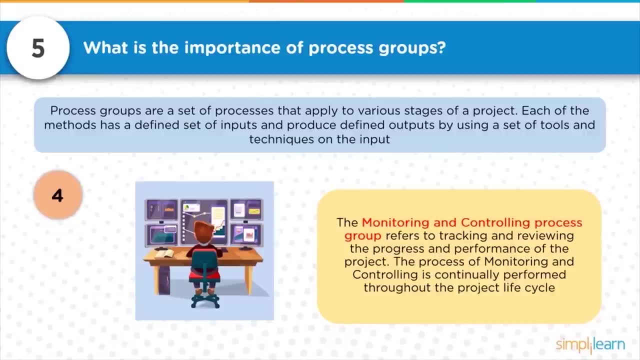 execution process group in project management perspective is directing and managing project work and managing the project knowledge, which is very, very important. The monitoring and controlling process group refers to tracking and reviewing the progress and performance of the project. The process of monitoring and controlling is continually performed throughout. 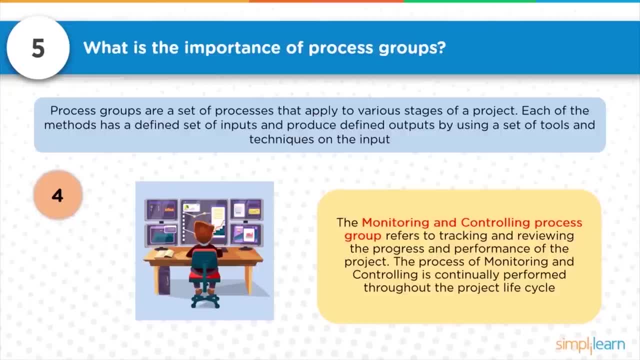 the project life cycle. So here I think, as I mentioned earlier as well, so it is very essential for us to understand whether project has delivered all those required deliverables or not. Are the deliverables are fulfilling all the features and functionality which are defined during the planning, That validation? 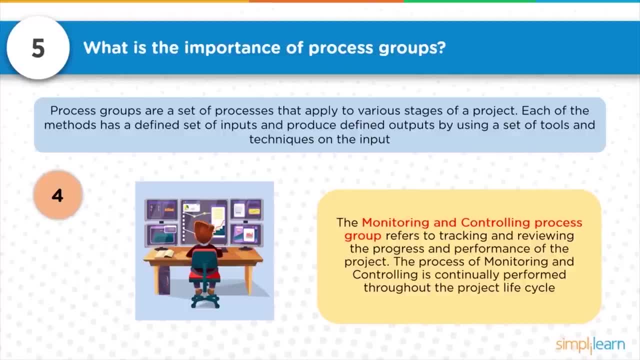 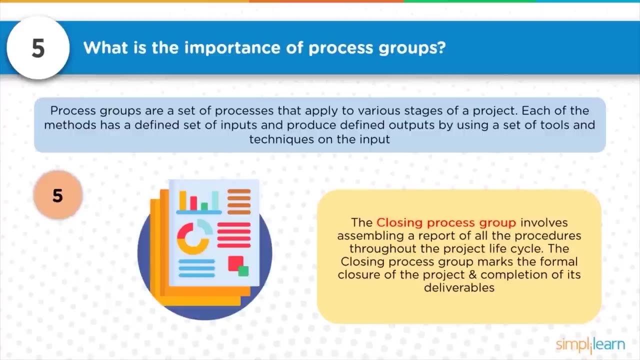 should happen. Any deviations are found, change requests arise and these change requests are approved. Once it is approved, then it comes to integrated change control process, through which changes are executed. Then the closing process group involves assembling a report of all procedures throughout the project life cycle. The closing 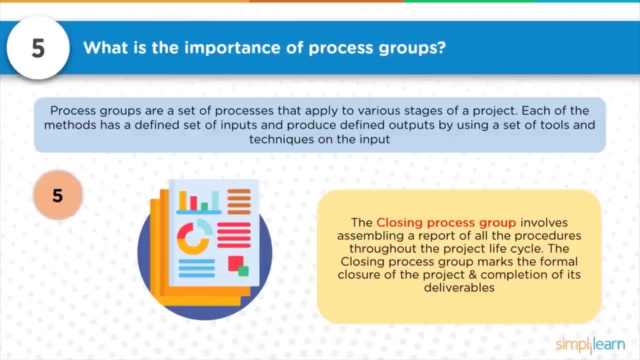 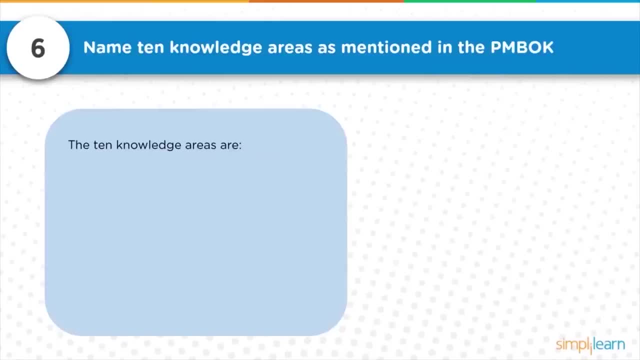 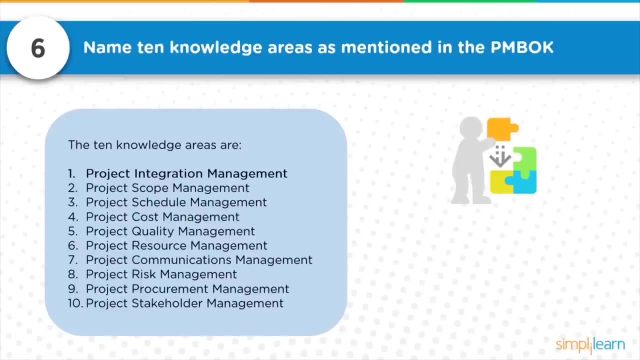 process group marks the formal closure of the project and completion of its deliverables. Now let us move to the next question, So question number 6.. Name 10 knowledge areas as mentioned in the PMBOK. So the 10 knowledge areas are: project integration. 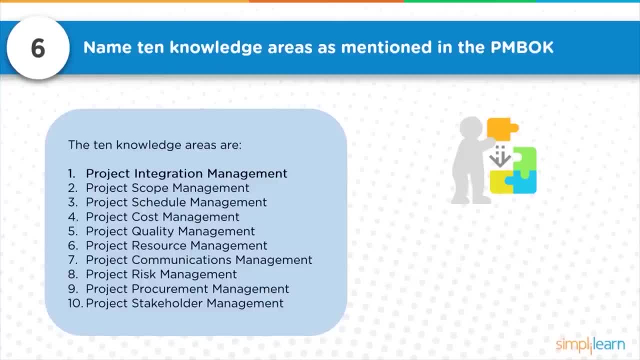 management: project scope management, project schedule management, project cost management, project quality management, project resource management, project communications management, project risk management, project procurement management and project stakeholder management. The project integration management basically focuses on unification and integration. 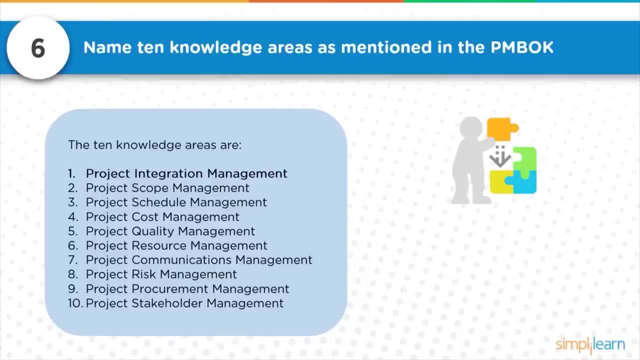 of all the project to manage it in an integrated way. A project manager is also called as an integrator, which means a project manager should have an end to end visibility of the project. So all the rest of the 9 knowledge areas, the plan. 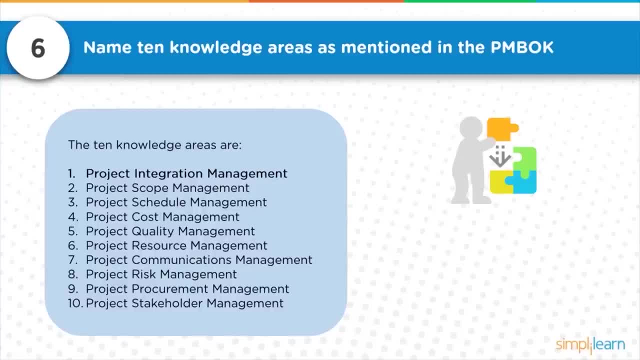 which is created as part of all the next 9 knowledge areas. those are consolidated and a comprehensive project management plan will be created in project integration management. So this is the only knowledge area where we see the processes in all the process groups, Whereas in the rest of the knowledge areas 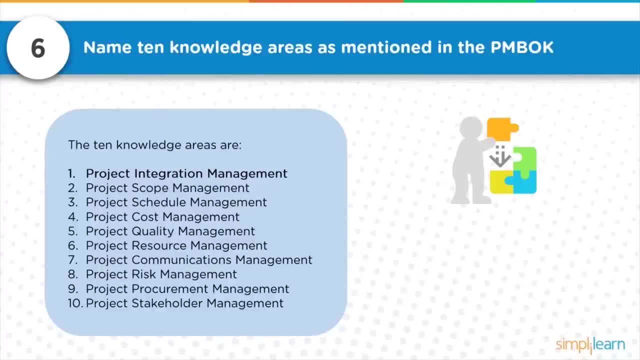 if you see, we don't see any process in initiating process group except stakeholder management. So integration management has one process. similarly, stakeholder management has one process in initiation process group. Similarly, in closing process group only integration management has a process, No other. 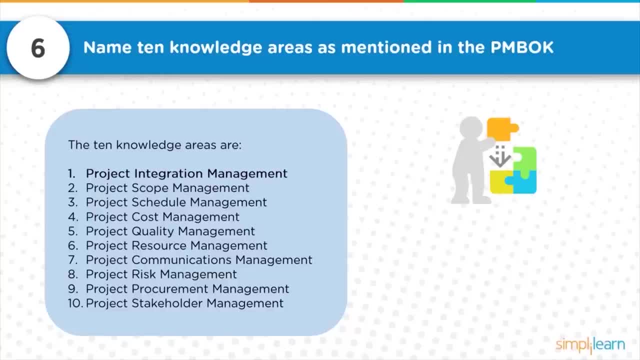 knowledge areas has any processes. So this is the only knowledge area where we find processes in all the process groups, which means it is very important to look at a project in an end to end view perspective. A full view of a project should be known to the project management. 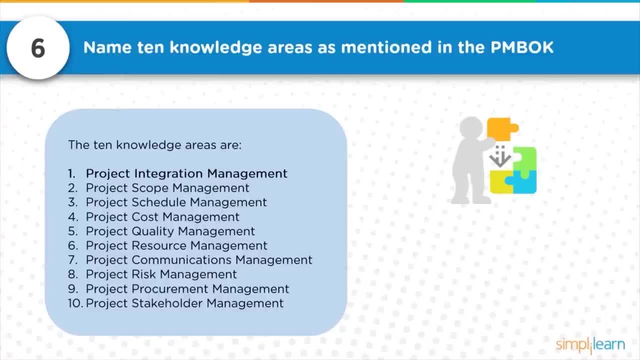 Only the project manager can become successful in doing the project management. The next knowledge area: project scope management, which focuses on ensuring collecting requirements, defining scope, creating work breakdown structures and scope baseline. So scope management focuses on ensuring the necessary scope is defined and provided. 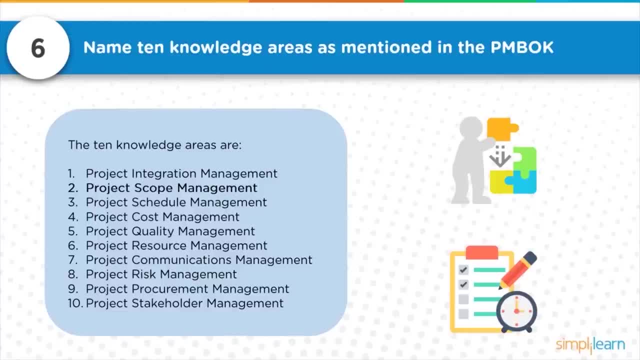 so that during execution, projects are delivered accordingly, and monitoring, controlling of the scope. The validation of the scope will be based on what is defined in the planning, What is planned as part of scope management, Similar to scope management in schedule management. once that work breakdown structure is created, it is very 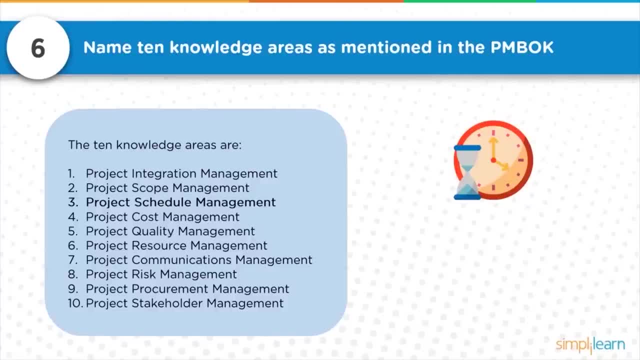 essential to understand what it takes in terms of efforts, what it takes in terms of duration, and in what sequence project deliverables are completed, In what sequence activities are done. So schedule management focuses on that: The critical, the important technique, what we use when it comes to 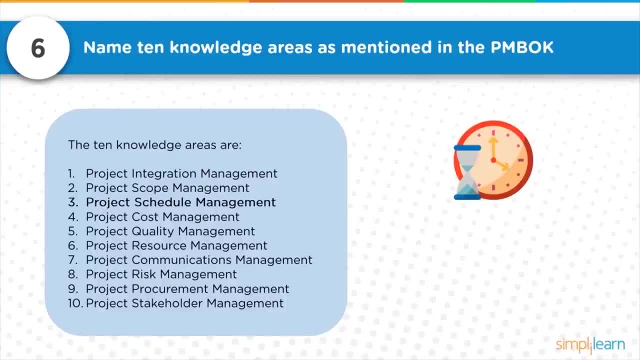 schedule management is critical path method. So in a given project when we establish a network diagram so we may see multiple paths from beginning to end of the project. So some paths will be the longest path which is called as critical path and that will be the minimum time which is required. 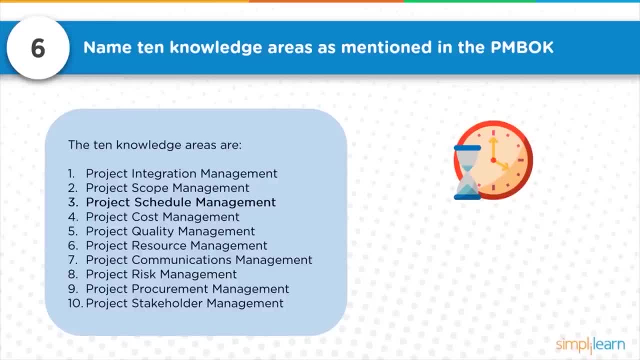 to complete the project. So schedule management plan provides us a detailed schedule of a project, along with sequencing and duration, and at the same time that is considered as a scheduled baseline. Then the cost management. So when we say cost, it is very essential for us to understand. 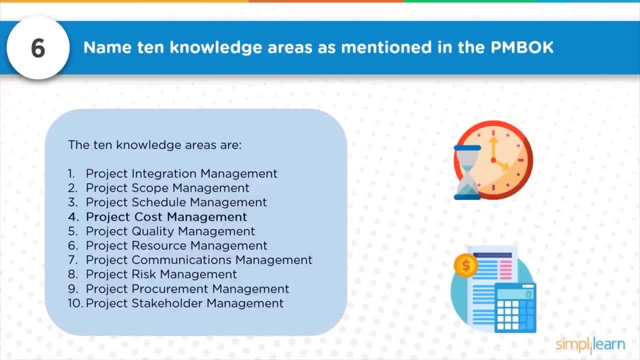 it is an outgoing money, outgoing monetary value. So projects incurs cost. When I say project incurs cost, there needs an investment from the organization who is actually doing this project. So the cost needs to be assessed, means an approximation of the cost needs to be done. A budget has 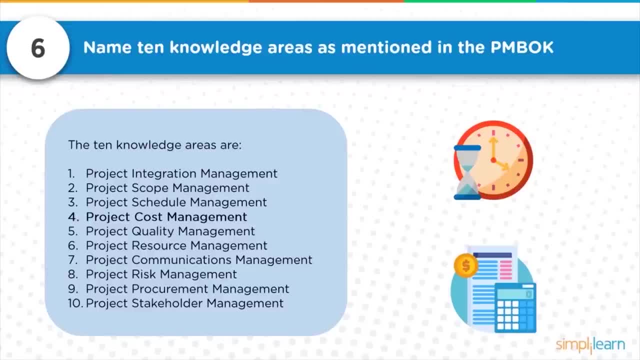 to be allocated to the project and within that budget the project needs to be completed. It cannot go beyond that. So budget is a established allocation of budget and confirmation of budget happens and cost perspective monitoring of the project happens based on what is that specific budget it has within that. 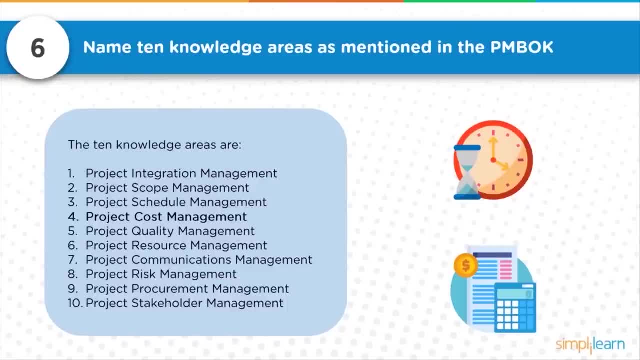 project has to done. That will become a baseline, cost baseline. So to measure the cost and schedule, a technique called earned value management is used, where the terminology like cost performance index, schedule performance index, actual cost, earned value, planned value, budgeted, completion estimate. 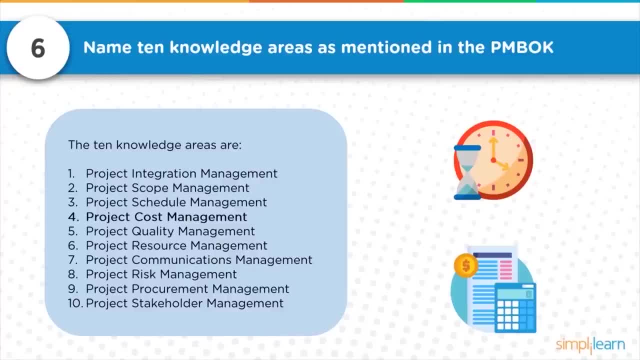 to complete. So these are the terminologies which are used as part of earned value management. Now let us move to quality management, project quality management. So it is very essential for us to ensure all the processes, all the activities, all the templates. 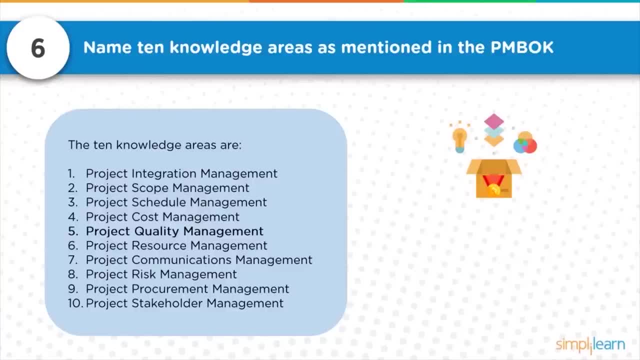 defined for the project are complied with. that is first thing while doing the project during the project life cycle. Similarly, the deliverables which comes out of a project at the end of the project or at the end of the specific phase or specific stage or specific milestone, So those 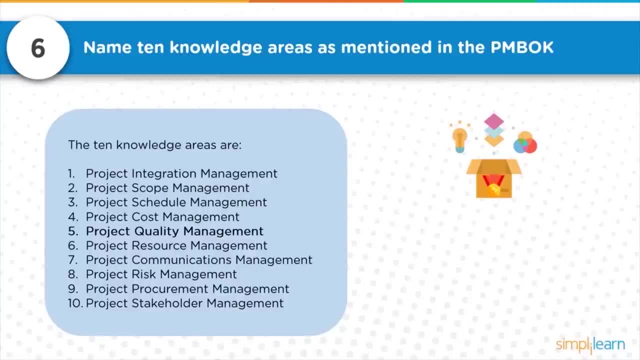 deliverables should be according to the specific specifications defined and agreed upon. So quality management focuses on establishing that quality management approach so that project compliance is maintained. at the same time, The results: what is delivered is as per the specification, what is agreed, The resource. 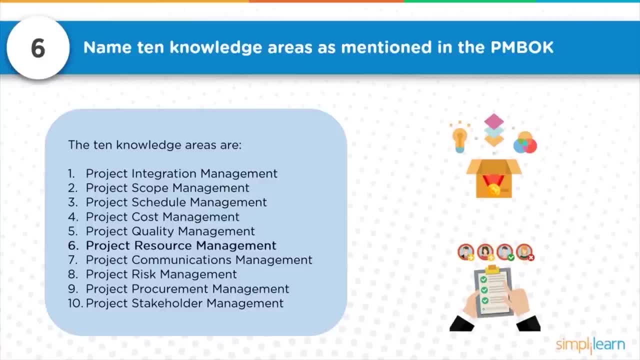 management focuses on ensuring all the resources which are required for the project are acquired, configured, installed, If it is a technology, resources if it is a human resources. the necessary induction of the project. the brainstorming required for team to understand what is the project. 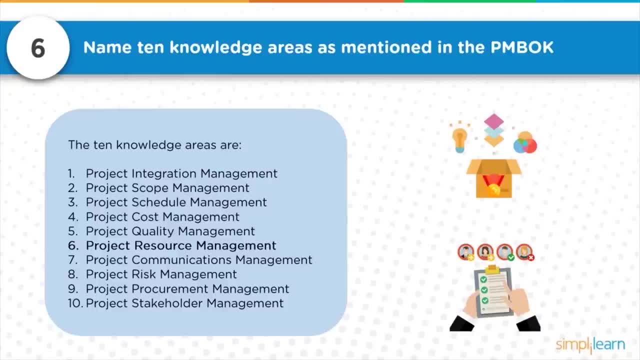 is all about is given and the necessary skills and capabilities are there. with those human resources and these team members execute the task of the project. So project resource management plays very important role. and now here, when we say scope, when we say schedule, when we say cost, 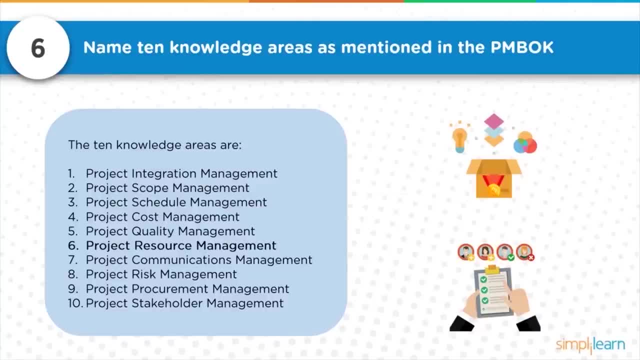 when we say quality in each of this, in other knowledge areas as well, the involvement of each of these resources are essential. So what resources gets into scope management? what resources gets into schedule management? what gets into cost? Likewise, for each of the knowledge areas, we see various different. 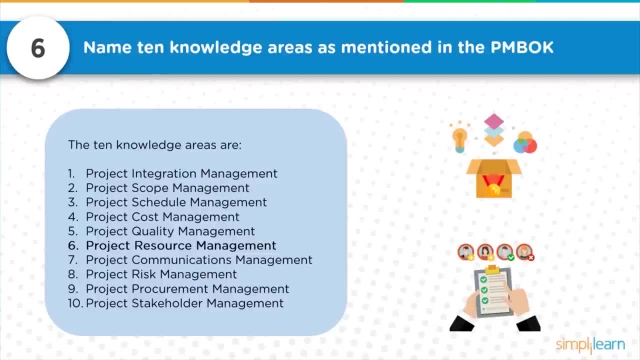 resources used. When I say, in schedule management, effort has to be established. while we establish an effort, it is also required to understand what is the skills and capabilities required. So schedule management definitely work very close with resource management. Similarly, these: each of these resource comes with cost. 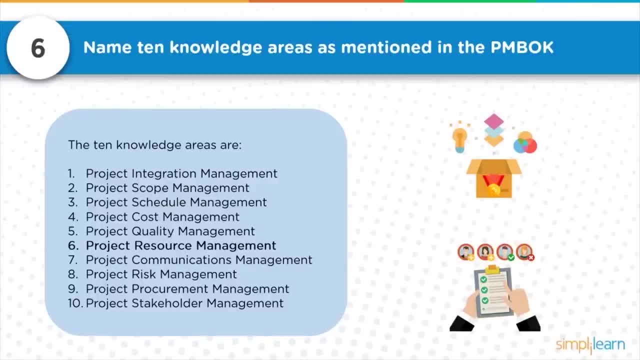 So obviously cost management is involved, Then quality, yes. So who is going to do the quality management? So roles and responsibilities needs to be clearly articulated, defined if it is a human resource in resource management. Coming to communication management, So communication, I think, plays very important. 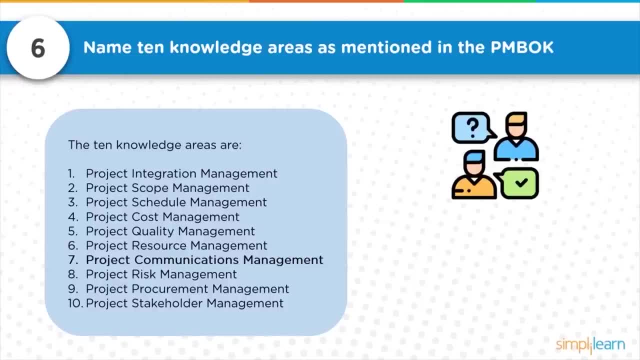 role. as we know, 90% of the time project manager spends on communications. Many times we see project managers like: look only communicating. Many team members have told me mentioning that project manager only does communication, Project manager only ask questions. Now this impression to the team gets created. 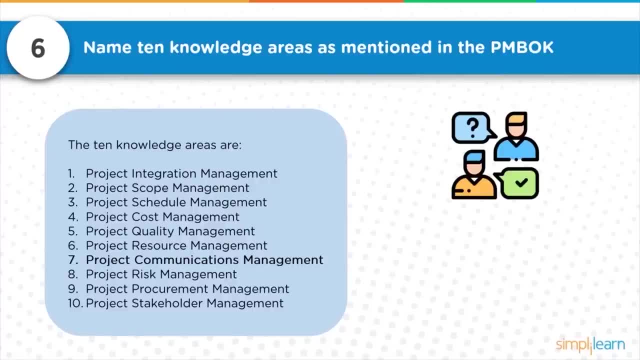 because they only see what project manager is doing is communication, Because team comes in when everything is done, Everything is set right. So they see project manager during the monitoring and control, mainly not during initiation, not during planning, not during closure. So many team. 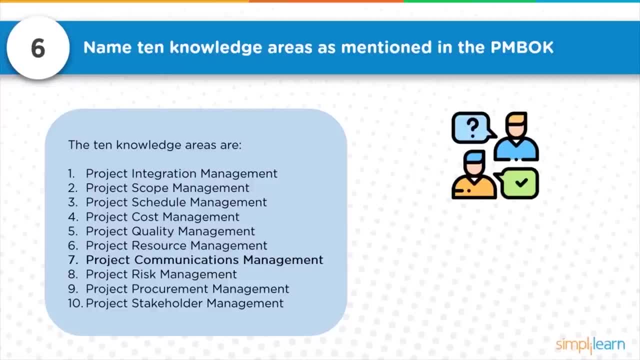 member comes and goes during the project, They only see project managers reviewing and asking the questions. So because of this they assume project manager only communicates, project manager only ask questions. But it is very important to ask questions, but there is a perspective and objective behind it, which already project manager. 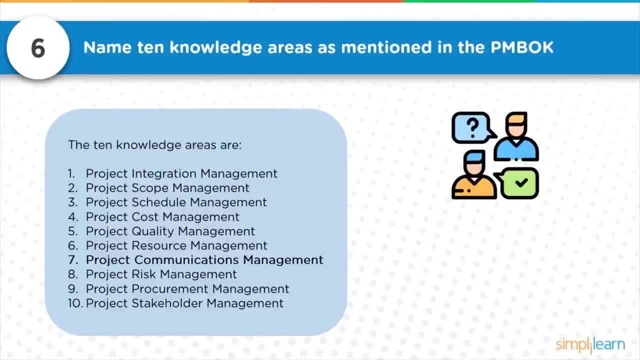 is involved and created like a plan, like signing off, coordinating with stakeholders, understanding requirements. many things has done In all these areas. communication is involved, So it plays very vital role. So then, project risk management: every initiatives organization takes, every investment organization does. there is a risk. 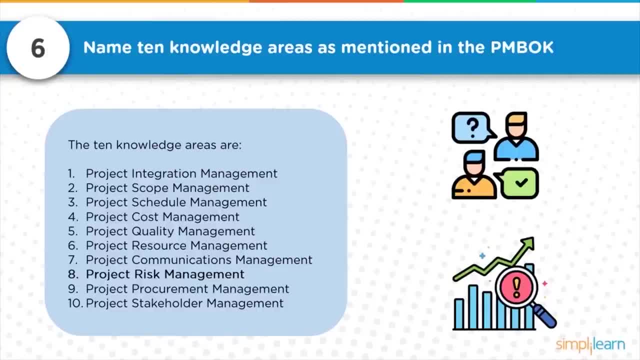 So already the identified risks are evaluated and project is taken up by the organization, which means the business has already understood what is the risk associated with this particular project, Considering that they have taken up a project. But while doing this project, while doing the project management- lot of risk. 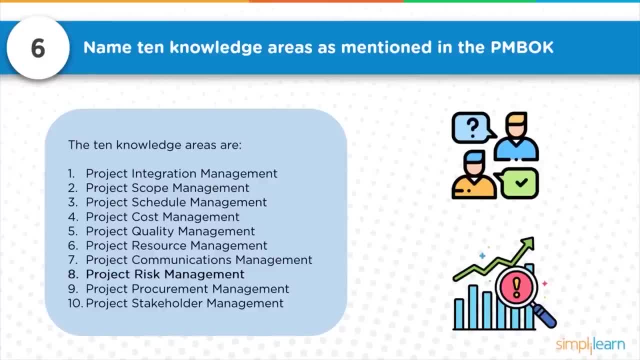 comes across. Project manager should keep identifying the risk, assessing the risk, analyzing the risks qualitatively and quantitatively, depending on the level of impact of the risk. So risk means we already know it is uncertainty of certain occurrence and outcome It may 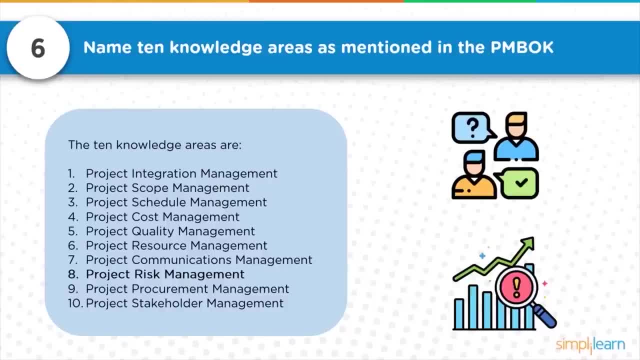 be positive or negative. Positive, you can take advantage of that, You exploit it, you enhance it, Whereas negative, risk, you mitigate, you respond. you will have a response plans like accepting those Or transferring it. sharing it. Transferring means you. 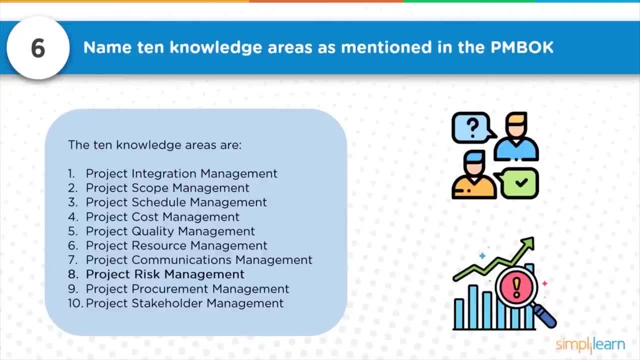 outsource or you take an insurance. So that is negative risk responses. Next, the project procurement management. The projects would involve certain procurement, So we need to ensure for this project what is that I am creating myself and using it. What is that I am going to procure from external? 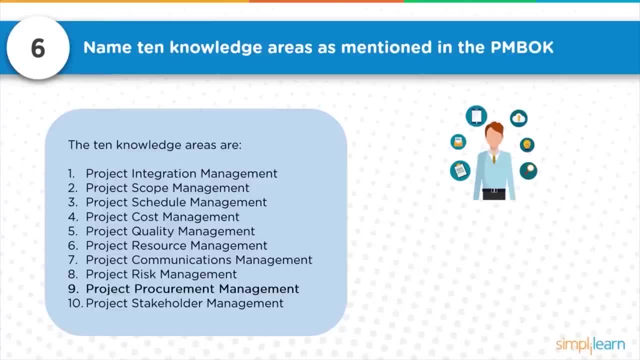 suppliers. So whichever we decided in make or buy decisions, whichever we have decided that we need to procure from elsewhere. So procurement management plays a very important role here. So identification of what needs to be procured, what quantity we need to procure, who would be the best. 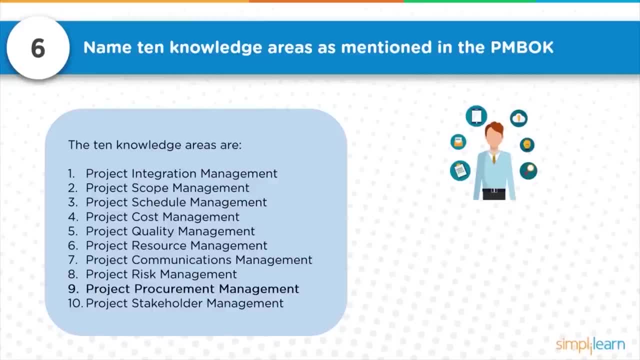 supplier. what are the criteria while selecting the suppliers? You may float an RFP. a proposal request will be respond which will come in. You may float a bid, Then evaluate the best vendor or supplier. You onboard them. Then you start issuing a PO. 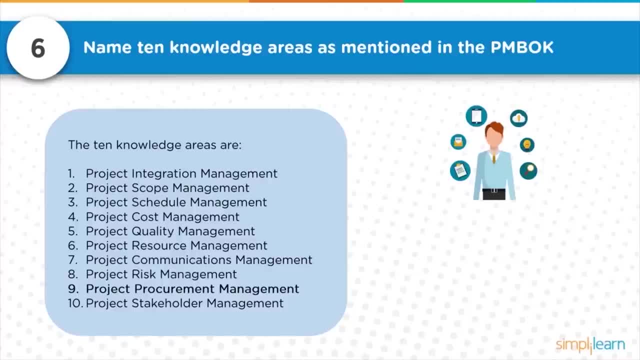 formally for them to supply, And then procurement happens. So end to end management of the supplier, Right from onboarding the supplier to doing the bidder conference, establishing an agreement and then engaging with them for reviewing their performance- All these are involved as part of procurement. 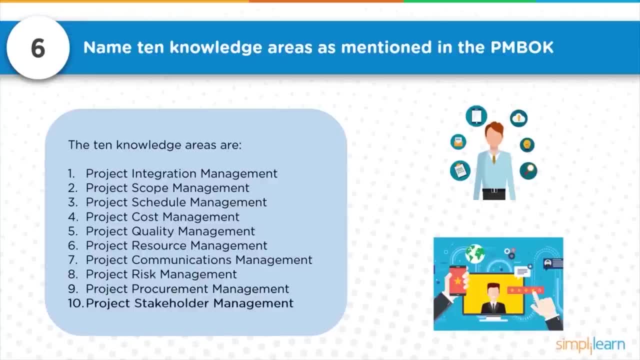 management. The tenth knowledge area, the project stakeholder management. So stakeholder means any entity or individual who involves in the project directly or indirectly. they are impacted, They influence the project and they get influenced. So, very importantly, if you think about a stakeholders, we can think. 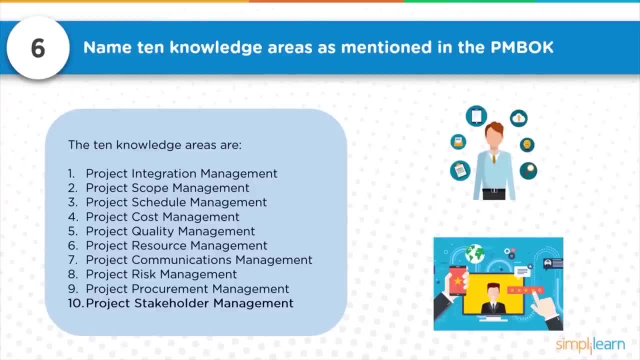 about customers. we can think about sponsor, we can think about team members, we can think about suppliers, who plays very vital role in the success of the project. So, engaging with the stakeholders, managing the stakeholders, plays very important role And if every nine knowledge areas, 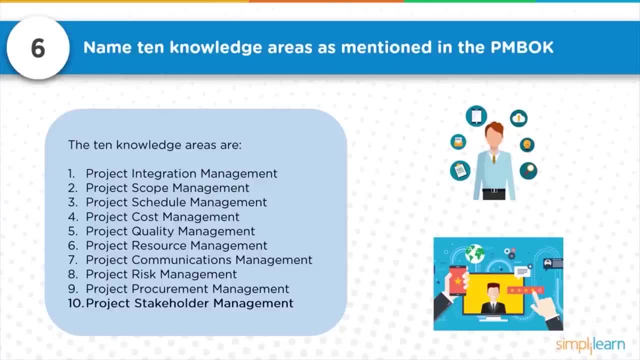 there is something which you have done right but something wrong done with the stakeholder management, entire project may go for toss. So one needs to be very careful, understanding the dynamics associated with each of these ten knowledge areas and then dealt with them accordingly and integration management would integrate all of. 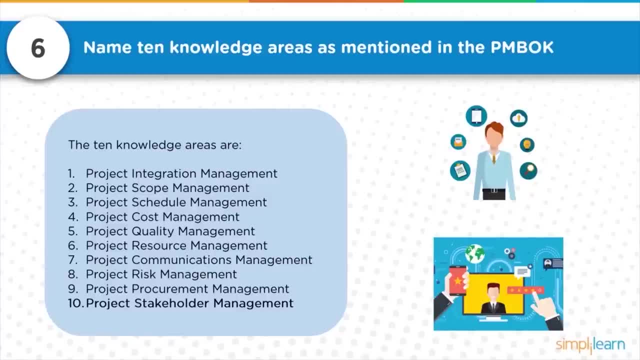 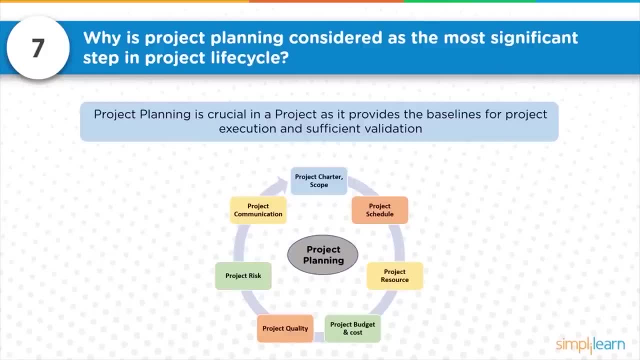 this, as I mentioned earlier, So that end to end visibility of the project can be seen. So that is about ten knowledge areas mentioned in PMBOK. The next question, question number seven: Why is the project planning considered as the most significant step in project life cycle? 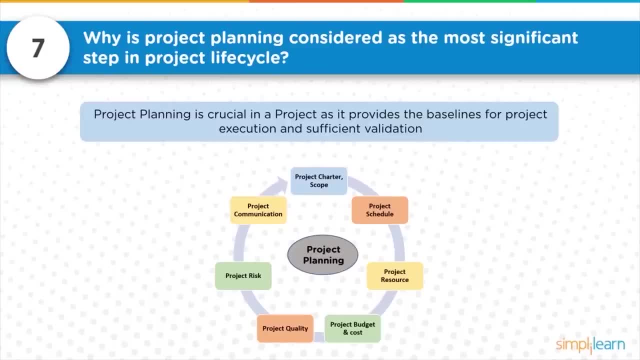 The project planning is more significant. This will provide all the baseline plans, like as we saw in the previous question: Scope baseline, cost baseline, schedule baseline. So all the baselines required which will be referred. Each of the baselines are considered based on these baselines project. 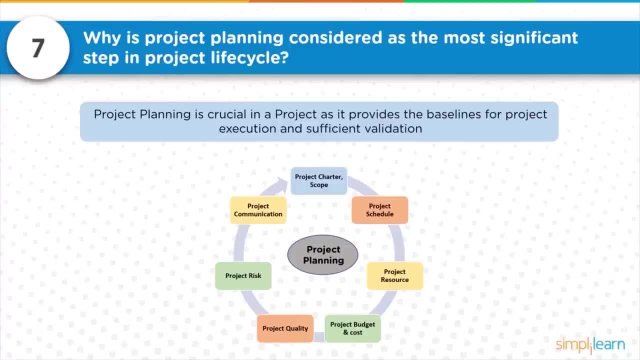 needs to be executed Now. any deviations to this baseline plans need to have a formal approval for necessary corrections. So already we know there are nine types of subsidiary plans for all the nine knowledge areas: Scope, schedule, cost, quality, resource, risk, procurement. 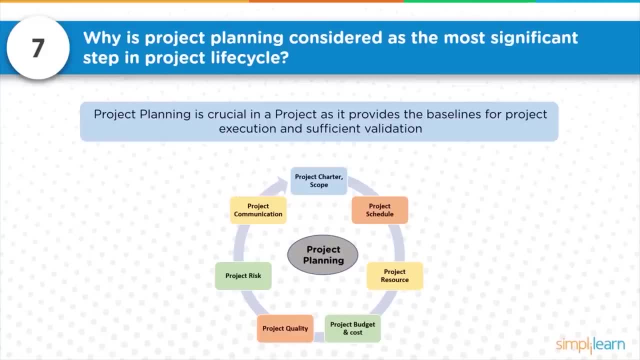 communication and stakeholder. These are the nine knowledge areas which will have a subsidiary plans, which will get integrated in integration management. So without having a clear plan, clear directions, So execution will not have any specific direction to take, So you cannot measure the deliverables. 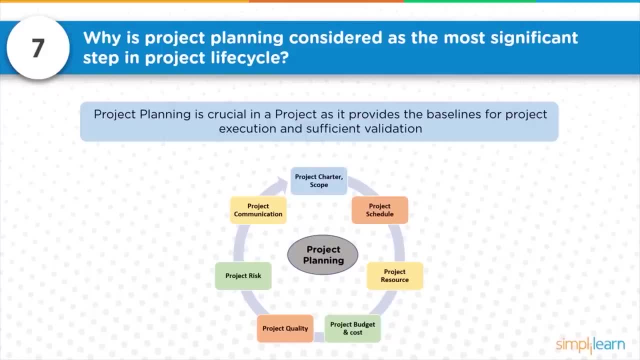 So what to do, when to do, who will do? All these are defined as part of the planning and that plays a very important thing. So if you look at the entire framework of PMP, most of the processes out of 49 processes- we can see in planning. 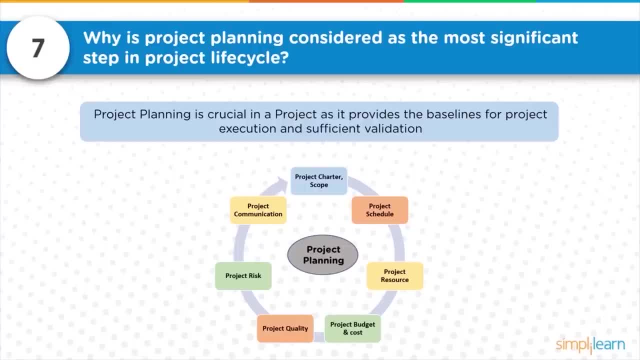 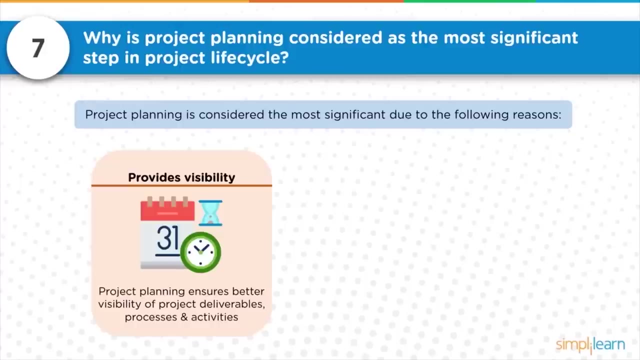 process group, Almost like 24 processes out of 49.. 50% of the processes almost can be seen in planning process group, Which itself indicates how important the planning process group and planning activity for a project. So why the project plan is considered most significant. 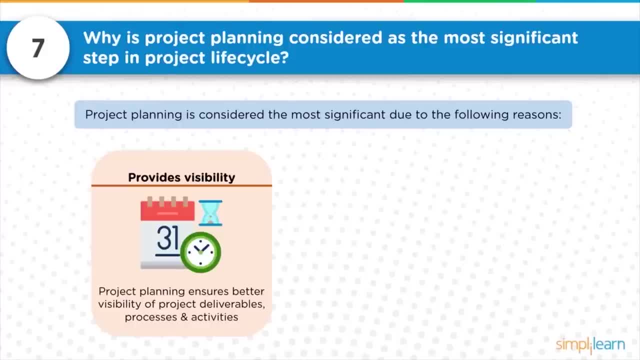 Let us look at few more points. So one is it provides visibility in terms of what project is all about, What is that we are going to deliver and what kind of results are we going to create. What is that we are aiming for? We will get. 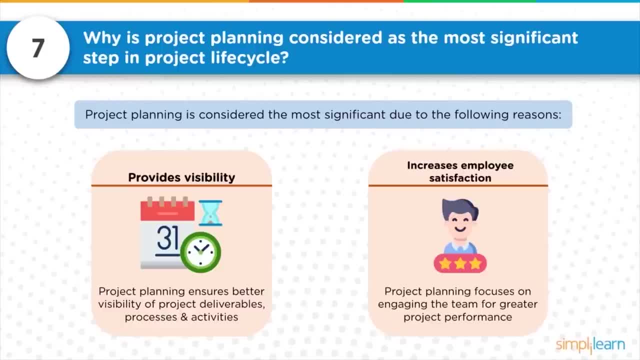 a better visibility. So next increases employee satisfaction, because there is no confusion. Each team member understands what needs to be delivered and what is the performance of the team members. how it is measured is also visible. and that is happening in reality, because you cannot deviate. 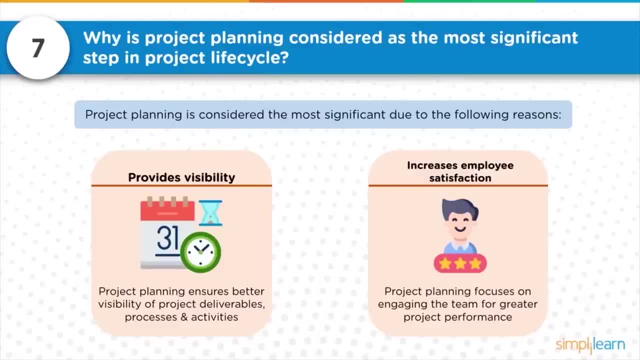 on what is being planned. So that should happen in actual execution as well. So obviously, employees are not confused now. The team members are not confused. They are delivering it according to what is planned and it is easy for them also because it is a better visibility. 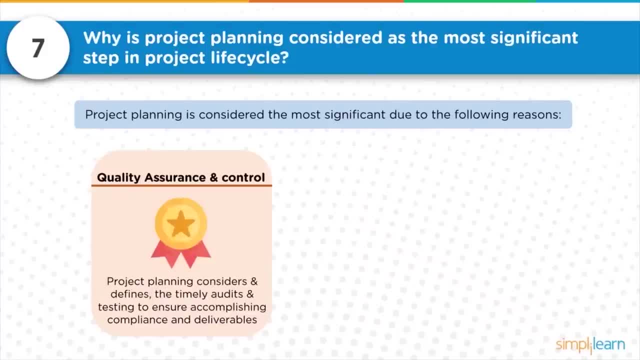 and they have a clarity about it. Next is quality assurance and control. So, as we know, quality management is one of the knowledge areas. So doing timely audits, testing all the deliverables, compliance checks- So all these ensures the approach. what we have selected. covering all of this ensures 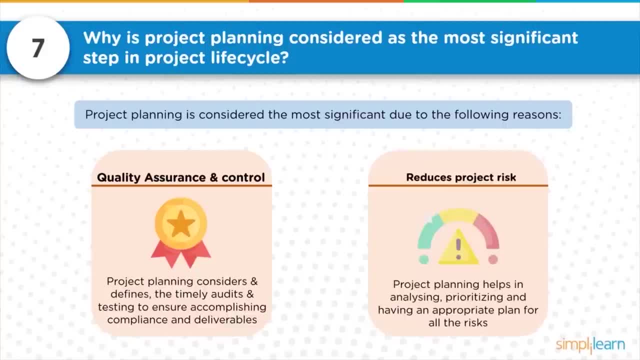 the project is delivered as we planned, Then reduces project risk because all the risks are identified. we have understood what are the risks are and we keep identifying the risk and analyzing those. and when we say risk, there is one unique nature of risk: where exactly the risk occurs. 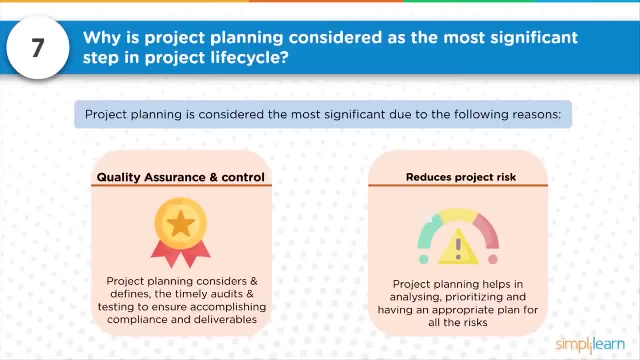 accordingly, the impact to the projects will be there. For example, when I start a project, if there is a risk associated with human resources which I have not even onboarded- Non availability of a specific resource- Very less impact. But when I have onboarded a resource, 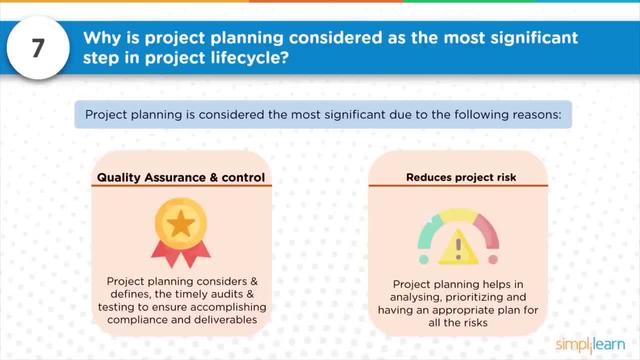 and then project execution is happening and execution is at peak. now what happens? It is quite obvious: Risk impact will be higher compared to the risk which would have occurred in the beginning of the project. So meaning, as we progress in the life cycle of a project, 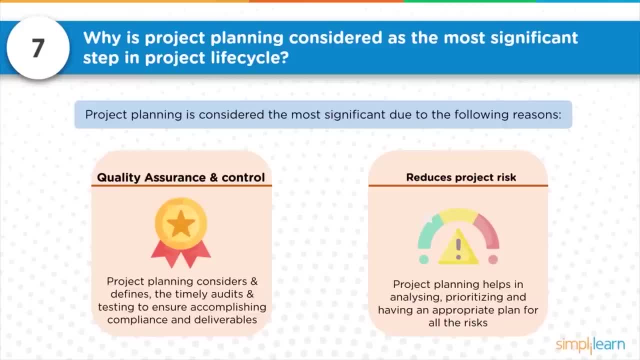 the identified risk will have an impact differently at the different parts of the life cycle, depending on the nature of the risk and state of the project. So, since it is visible to us, we have a risk management knowledge area which emphasizes on doing all of this. So, since we 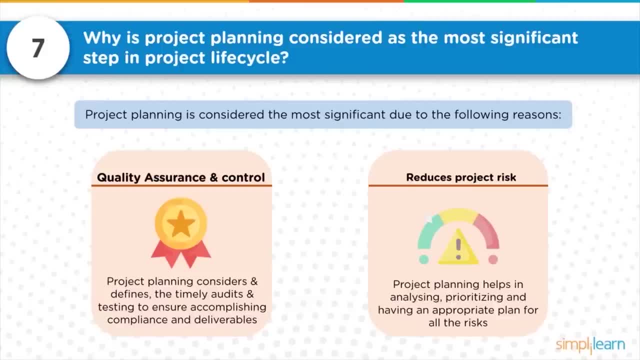 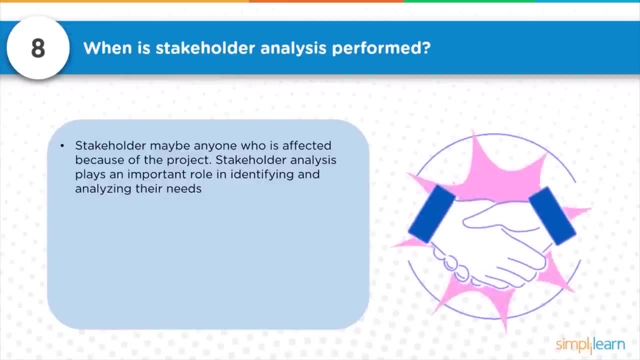 are doing it, it will become visible for us to have an effective risk management. So next question: When is stakeholder analysis performed? Already we know stakeholder means an entity or individuals who involve directly or indirectly, who get influenced, who will get impacted. 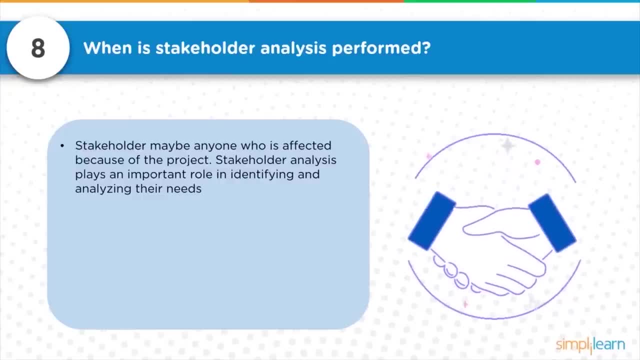 are all called as stakeholders, Understand who are those stakeholders who are basically straight in terms of having impact or impacted. so we need to identify them and manage them. We may have a stakeholder like competition to our organization, but do we really manage them? Not required. 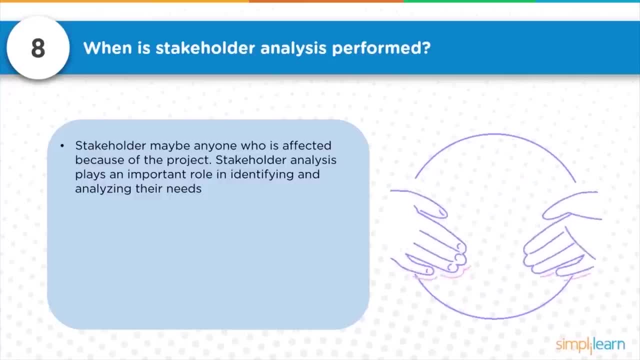 we may require to be sensitive. what competition is doing? Is this project unique, so that the details of this project, the information about this project, is not leaked to the competition, is not shared with competition? in that sensitivity, you need to ensure monitoring it. You need not manage. 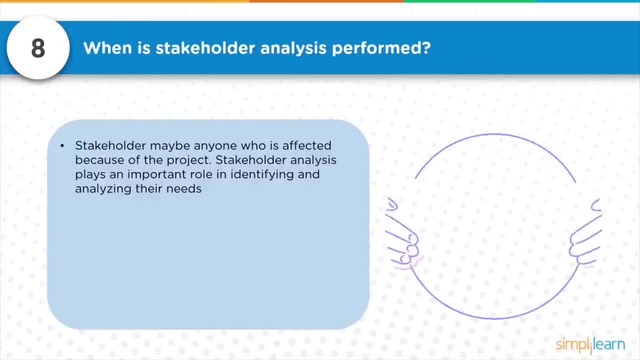 the competition here, but you need to monitor what is happening relating to competition. similarly stakeholder, like team member, so you are required to manage them. You cannot just keep monitoring. You need to manage them so that there can be the results, which is required to be. 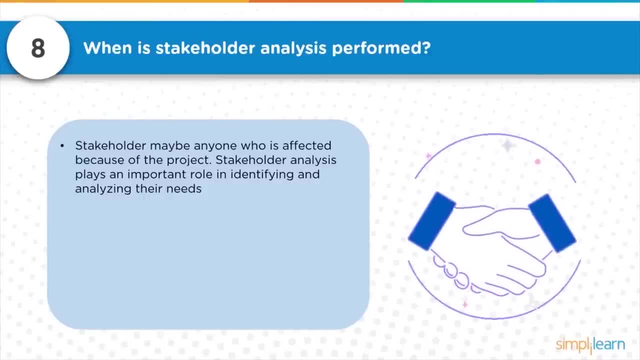 created, has created Now. next is customer. if you say You need to engage with them, you need to discuss with them, you need to review with them that customer is getting what customer is asked for. So stakeholder may be anyone who is affected because of project. 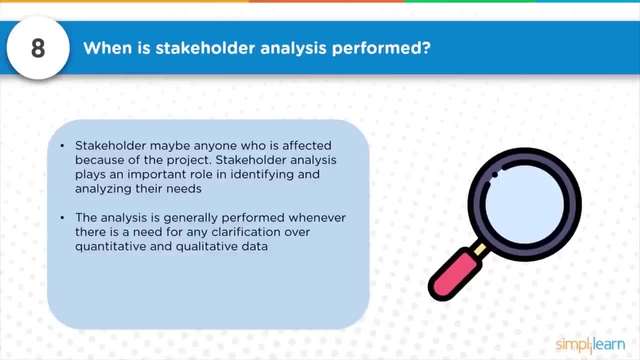 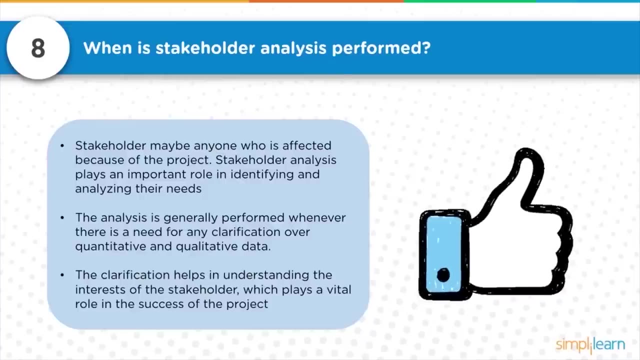 stakeholder. analysis plays a important role to identify and analyze their needs right, so the analysis is generally performed whenever there is a need of any clarifications over quantitative and qualitative data. the clarification helps in understanding the interest of the stakeholders, which plays a vital role in the success of the project, as I mentioned earlier. 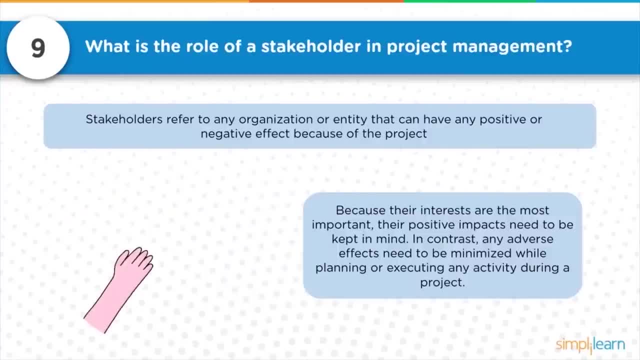 So next question for us: what is the role of stakeholder in project management? So stakeholder, as we know, refers to any organization or entity that can have any positive or negative effect due to project. because their interest are most important. their positive impact need to be kept in mind, while any 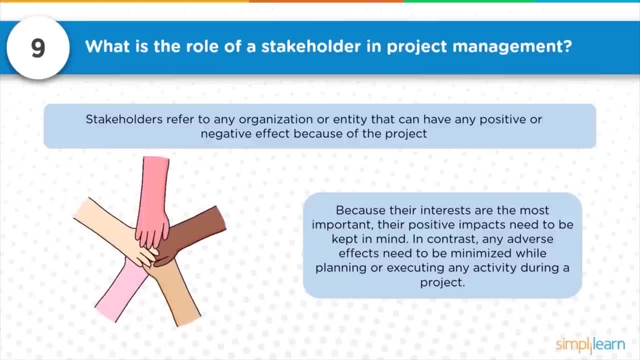 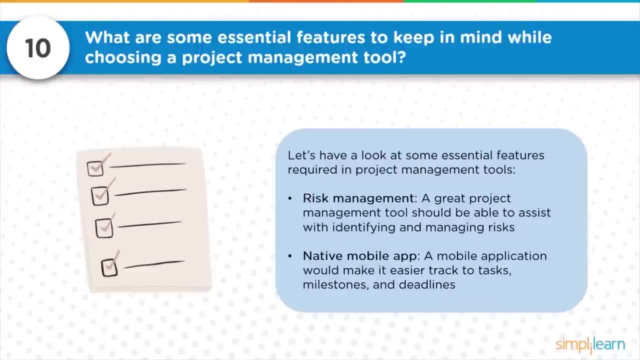 negative impact need to be minimized while planning for executing any activity during the project. So it is very important to understand the stakeholder perspective view. Next question: what are some essential features to be kept in mind while choosing a project management tool? So project management tools basically assist the project. 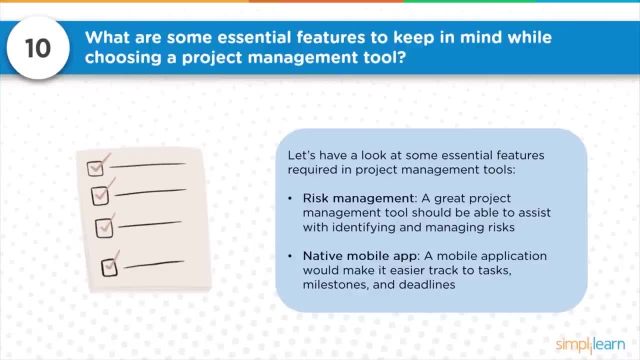 manager and the project team in doing the project effectively. and I think efficient way of doing project is also ensured because many processes are automated and the transaction will become easier. the collaboration become easier, creation of dashboards and reports which will provide the visibility of the performance of the project. so 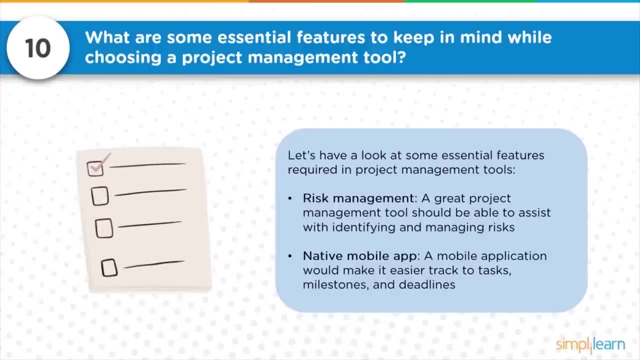 let us look at some of the essential features required by project management tools. so risk management- just now we discussed about risk management and its importance if a project management tool assist while identifying and managing risk, because when we identify risk we update those in a risk register, so if tool has a established risk register. 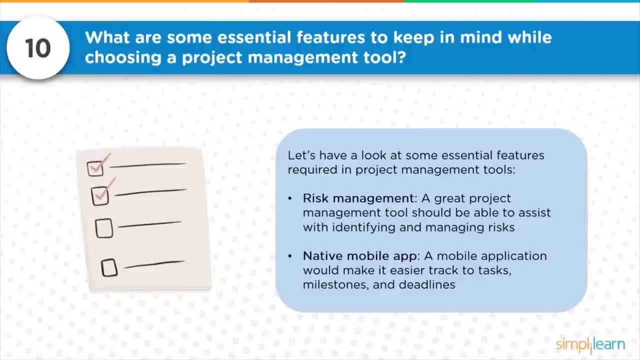 where we can keep inputting this particular risks and keep alerting the specific details about. we have a frequency of analyzing the risk repeatedly, the identified risk, so informing us, reminding us, telling that this risk calendar is like this: you may require to analyze those that will help in 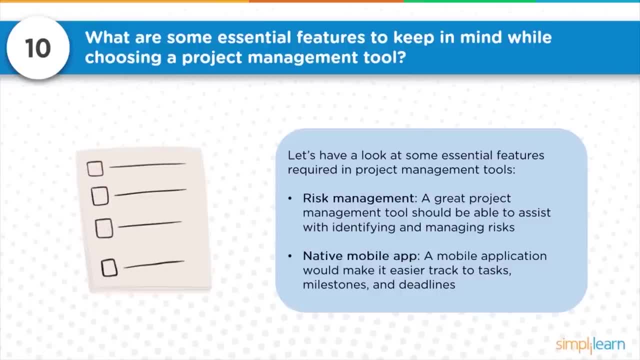 making it better risk assessment, as well as updates in terms of managing the risk, or also lessons learned earlier. some risks which of similar kind which are identified, are managed like this. so lessons learned, recalling those coming to resource management. so tool can able to help us in terms of calculating the 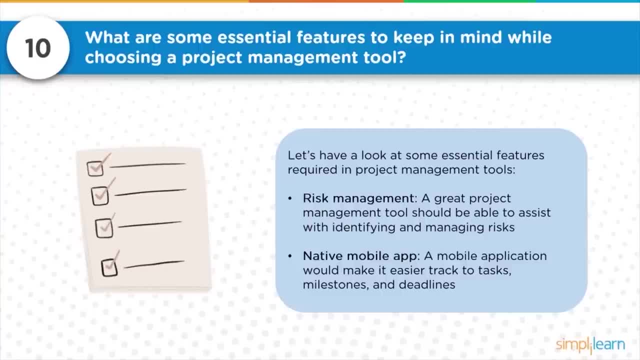 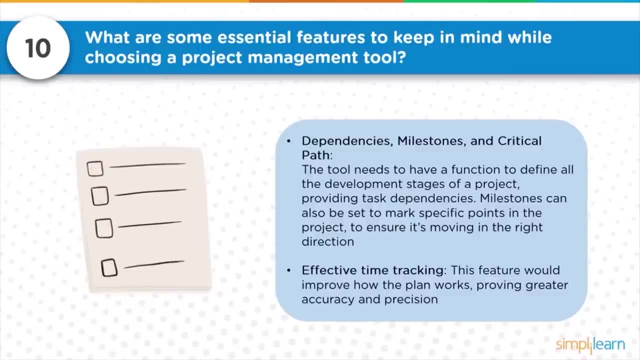 expenditures and distribute them among the tasks so that it is helpful in terms of better management of resources as well as the cost associated with that. then dependencies, milestones and critical path. so most of the project management tools, what we have come across, minimum they will have this capability: establishing a Gantt. 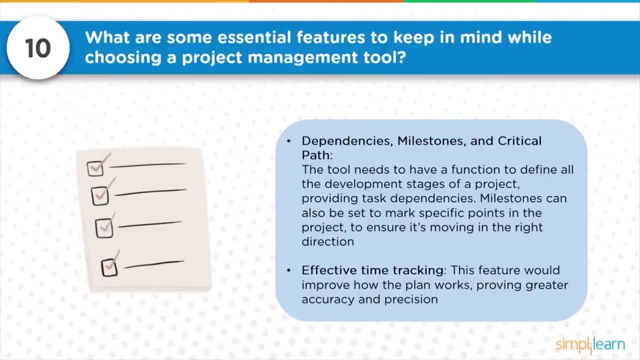 chart, helping in terms of establishing a network diagram which will provide us a visibility in terms of what is that the project flow would be, how the project flow would go on and how the project is going to complete. what are the activities dependent on each other? so what are the relationship between? 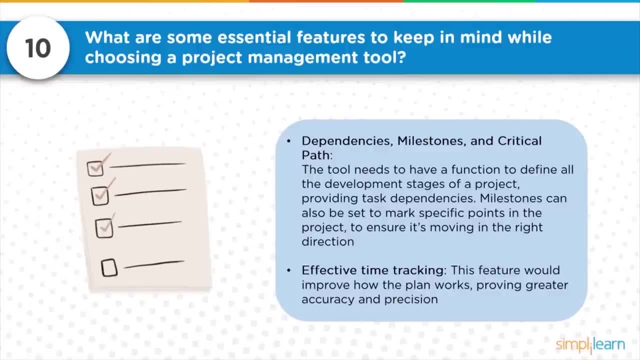 each of the tasks. what are the milestone, deliverables, duration of the project, what are those activities happening in parallel? so visually graphical representation it would give. so it should also minimize, simplify. the tool should have that capability. it should also have a minimal interfaces or ease of doing things like drag and 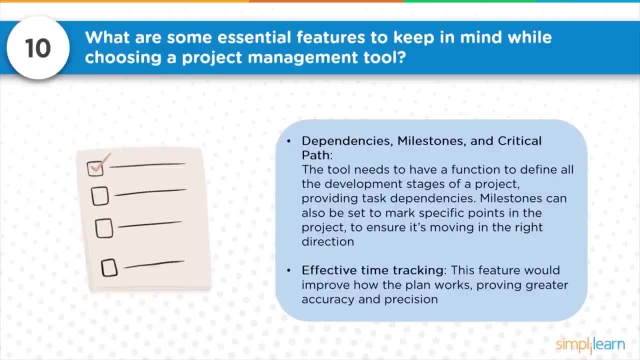 drop interfaces, so ease functionalities, maintaining smooth maintenance and support, which it can help us in terms of doing a project management better. so, basically, tools helps us in terms of assisting to have efficient and effective project management. so all the information should be handy so that it is there with us always. so third part, 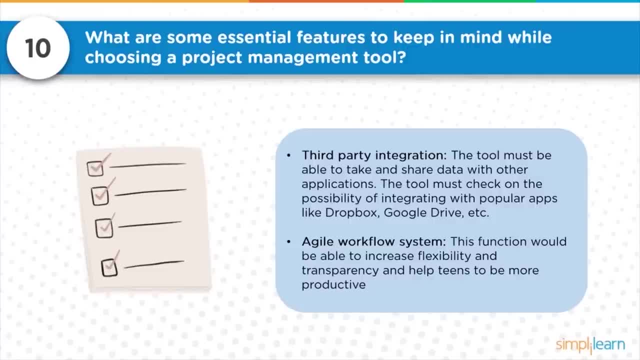 integration like a tool must be able to help us in terms of collaborating with other tools which would help us in sharing information. it would help us in terms of providing better visibility, any other tools which are there in the organization- if I am speaking about documentation, records sharing, or any of the reports or 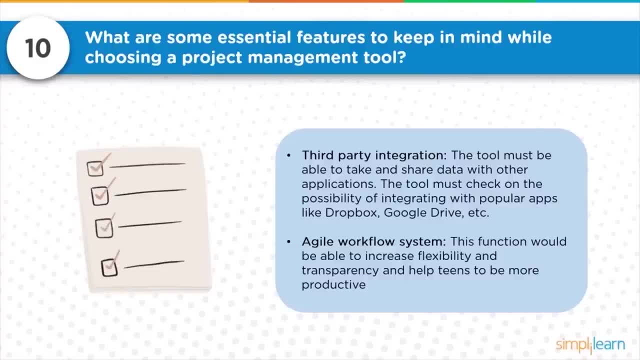 creation of the dashboards. these are the capabilities which a tool can have and, at the same time, this can have an interface with other tools like Dropbox, Google Drive, which will help in have a better visibility and better collaboration. so agile workflow system, when we say the functions. 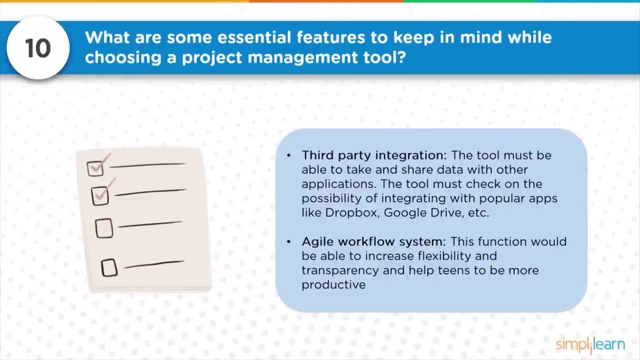 features. functionality of this particular tool should help us becoming agile. so moving faster means quick inputs and feedbacks given, because when we say agile, we are moving faster. when we are moving faster, there should be quick feedbacks which should be coming back so that necessary corrections can be made quickly. 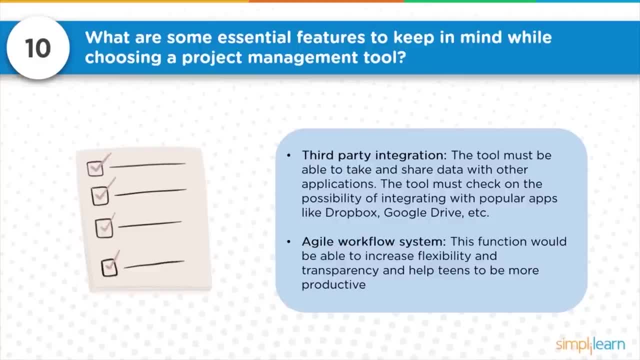 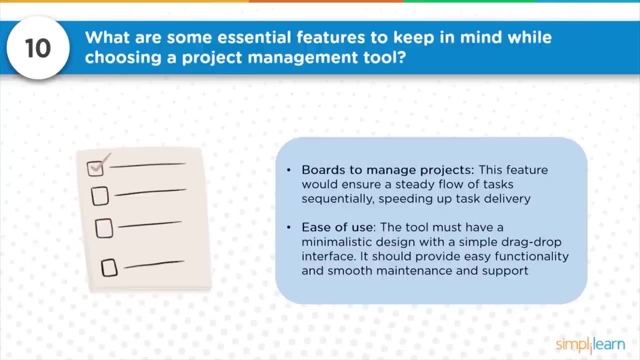 so to do this, if tool can assist us in providing those details of increased flexibility and transparency, so that would help in becoming more productive, then dashboards to manage projects. dashboards which will provide what is complete, what is not complete, what is the status of the project, how is the performance. so, 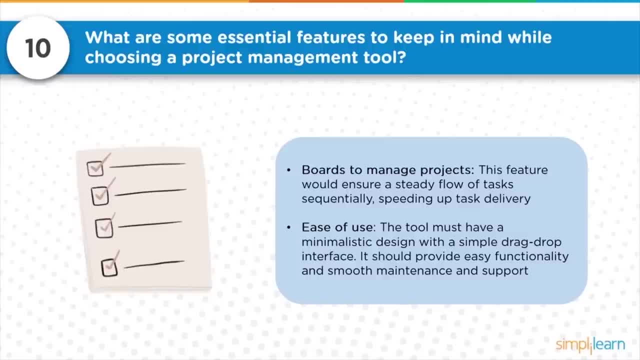 this would help in having a quick visibility into the performance of the project and also the progress of the project, to track them so that what is complete, what is not complete and how it is progressing. is it ahead of schedule, behind schedule, is it within budget or over budget? 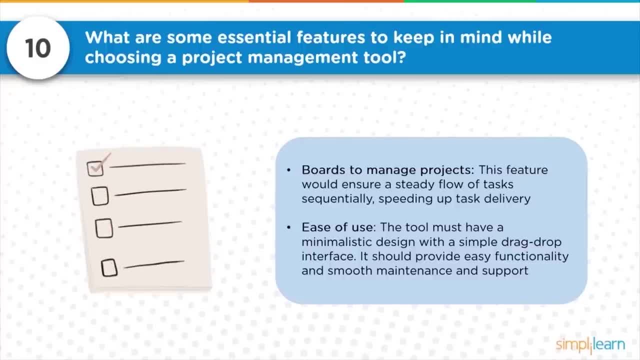 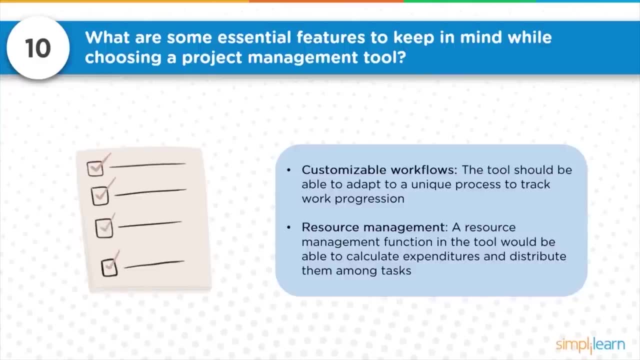 the visibility to that will always help in terms of getting better project management done. then customizable workflows, so the tool should be able to adapt to the unique process to track work progression. so then, if it provides a mobile application integration, so better to have team to know what. 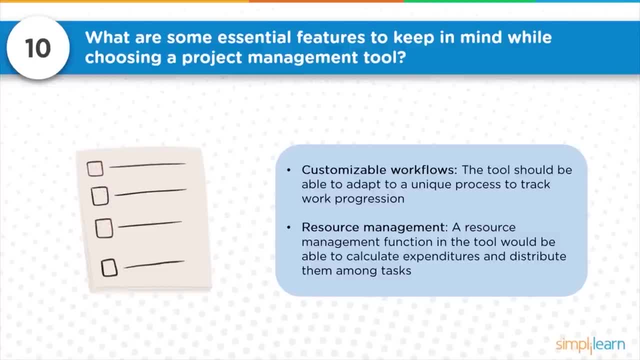 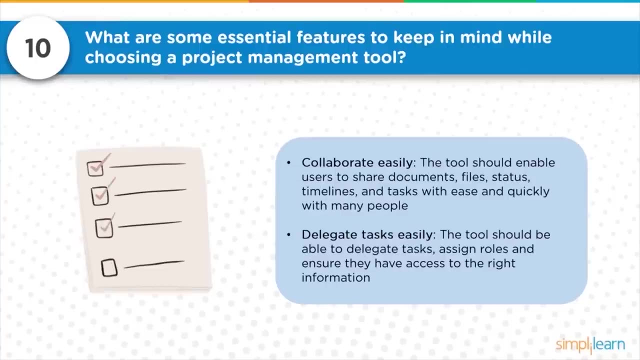 is the status of it anytime anywhere, so that ease of moving forward faster in the project management and making decisions will become easier. because always having right information in right time with the right people is very essential so that decision making can be more informed and quicker then collaborate easily. 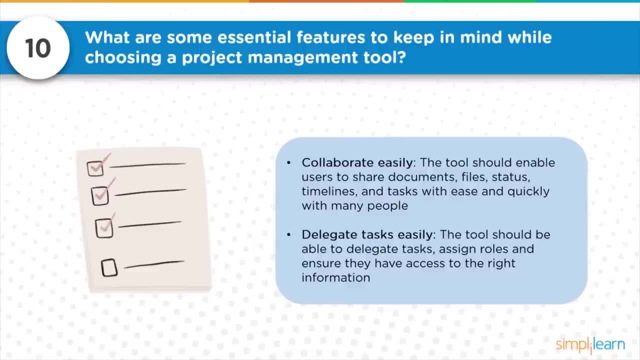 the tool should enable user to share documents, files, status, timelines and tasks with ease and quickly, with many people then delegating task easily. it should be able to delegate tasks, assign roles and then ensure they have access to the right information. so that's all about tools. now we'll move to the next. 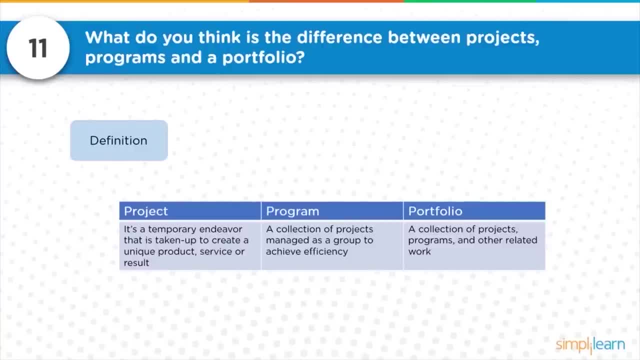 question. so what do you think is the difference between projects, programs and portfolio? so this looks like a very uh, generic question which is asked by any individuals during their interview. but even though this question doesn't focus on project in specific, it is very essential for project manager to understand the difference between. 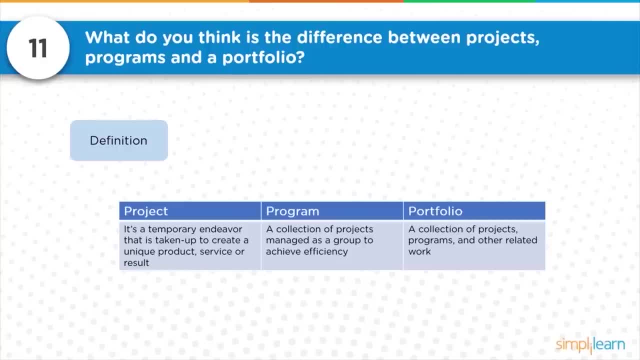 these three so that whom to ask for what will be known to the project manager. so the definition of project is like a temporary end over. it's an activity that is used to create a unique product, service or results. we saw that, we understood already, whereas program is a collection of. 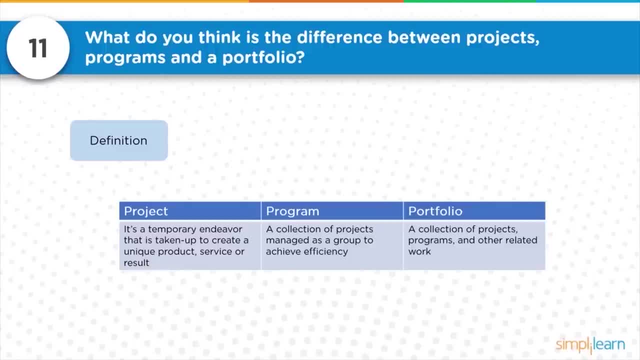 related projects which are managed as group to achieve better effectiveness and efficiency. so when- which you don't get when you manage a project individually, if you group it and manage, you can share resources, you can optimize the resources and cost, you can standardize that you can achieve through. 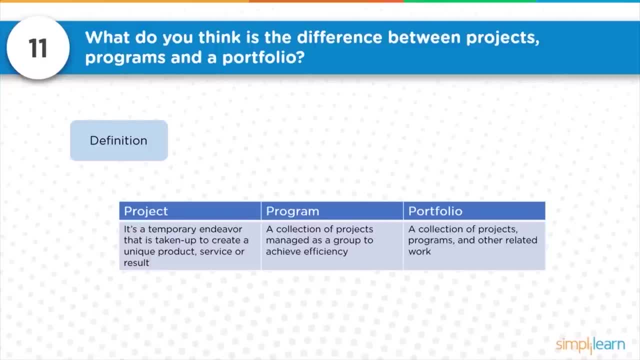 program management. so portfolio management is again a group of projects and programs which may be related, unrelated but strategic objective. accomplishing strategic objectives of the organization is very essential. so all these projects and programs and other related works are grouped together with the common strategic objective organization. so the project manager. 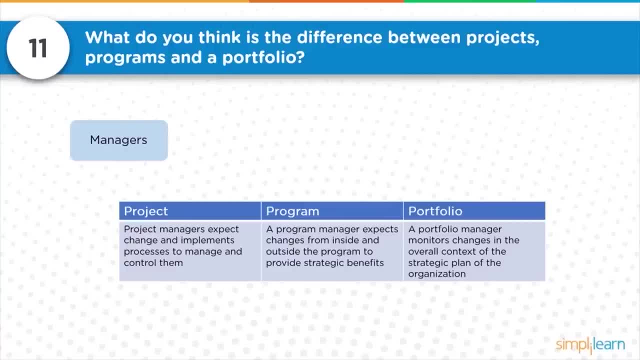 versus program manager versus portfolio managers. what do they do? so? project manager expects change and implements processes to manage and control the project in terms of accomplishing the project objective, whereas program manager expects changes from inside and outside the program to provide strategic benefits, as I mentioned earlier. like 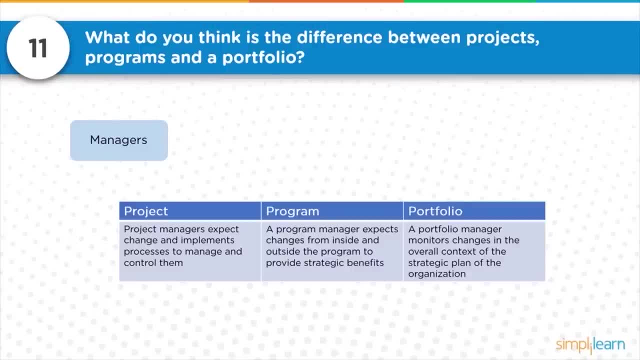 standardization optimization. so portfolio manager monitors changes in the overall context of the strategic plan of the organization. is this projects or programs or whatever we do in this organization? are they aligned to strategic objectives? are they helping to accomplish the strategic objectives? so project managers manages and coordinate. 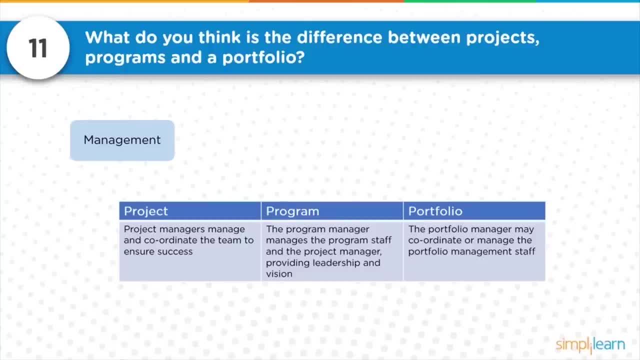 the team to ensure success. whereas program manager manages the program staff and the project manager providing leadership and vision, the portfolio manager may coordinate or manage the portfolio management staff, then monitoring part of it. project manager monitors and controls tasks to produce the products, results or services of the. 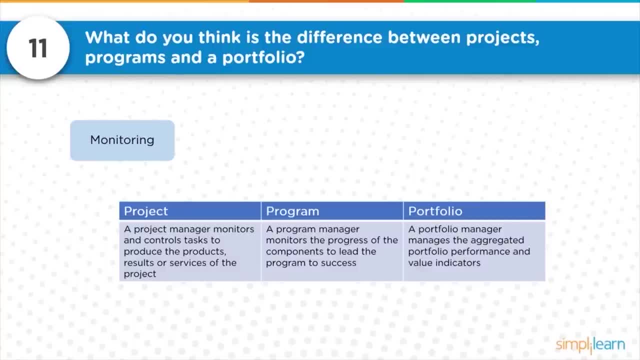 project, whereas program manager monitors the progress of components to lead the program to success. portfolio manager manages the aggregated portfolio performance and value indicators, so planning part of it. project manager develops, monitors and controls project plans throughout the project lifecycle, whereas program manager develops the program plan and performs high-level planning to guide. 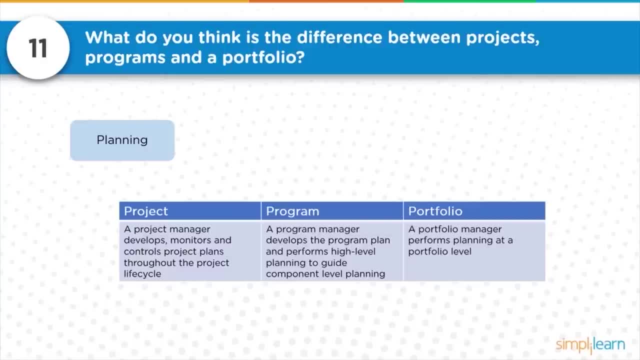 component level planning, whereas portfolio managers perform plannings at a portfolio level. the scope: the project manager will develop, monitor and control throughout the lifecycle of the project, whereas program manager has a program which has a wider scope, aimed at meeting the benefits and goals of the organization. whereas portfolio has a 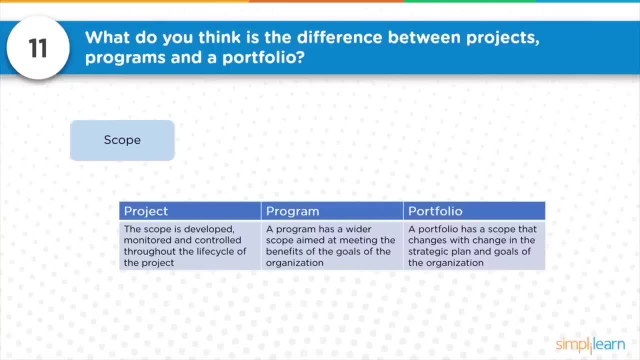 scope. that changes with change in the strategic plan and goals of the organization. so why the strategic goals or plans would change, the directions would change. that has various different reasons, maybe a business scenario, market conditions, etc. the success of the project is based on time taken to finish the project. the 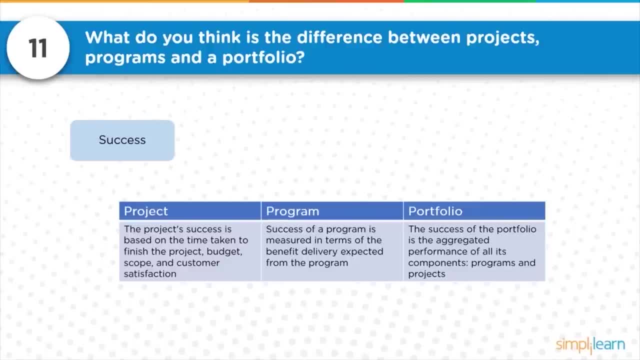 budget within which it is completed. the scope, the customer satisfaction, the quality defines the success, whereas the program success is measured in terms of benefits it delivered, as it expected from the program. then the portfolio success is the aggregated performance of all its components, programs and projects. question number 12: what are the skills? a 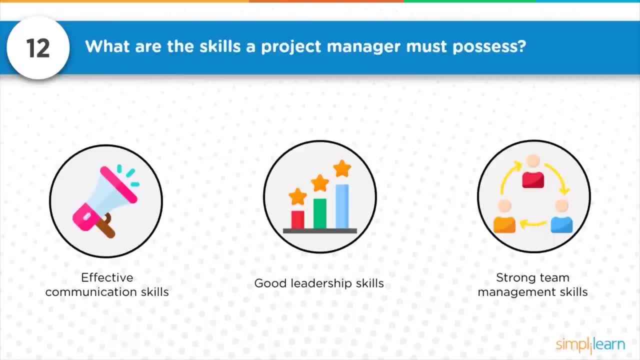 project manager must possess. typically, a project manager would require to have effective communication skills. so communication skills help in terms of establishing better relationship, because it plays a vital role there. what do we communicate, when do we communicate, how do we communicate matters? because it's not about just verbal. 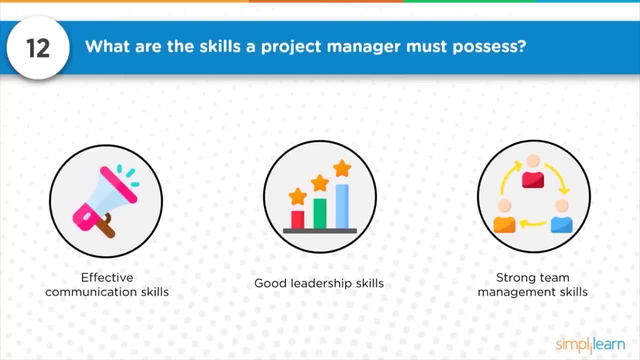 communication or return communication. there is non-verbal communication, through body languages, through expressions, which individuals do the communication. so it is very essential to have a right method and right approach towards communication. so the project manager should possess that skill, good leadership skills, so many times the term. 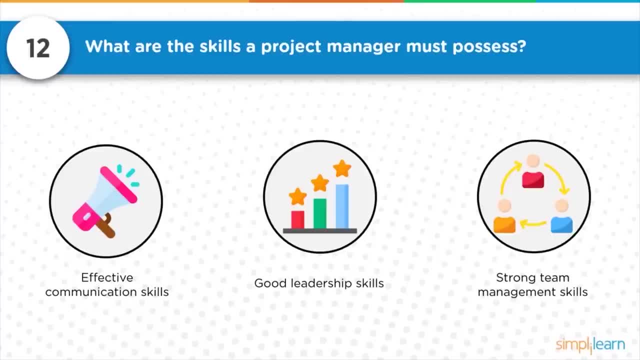 leadership is confused with the position of a leader. no, so leadership is basically capability of an individual. so if a specific individual has a specific individual, having that capability can influence people, can inspire, can motivate project manager, having a leadership skills, it's very essential, it is a must, required skill. 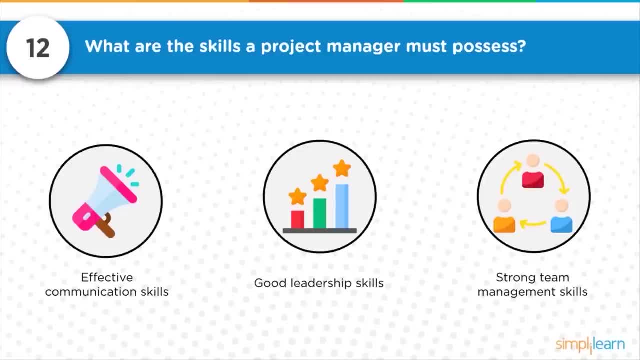 only then project manager can make the people listen to him. people will respect him because the behavior will be guided through that capability. strong team management skill, which requires a, an engagement, which requires a communication and leadership skills work very closely with this team management skills. so understanding the 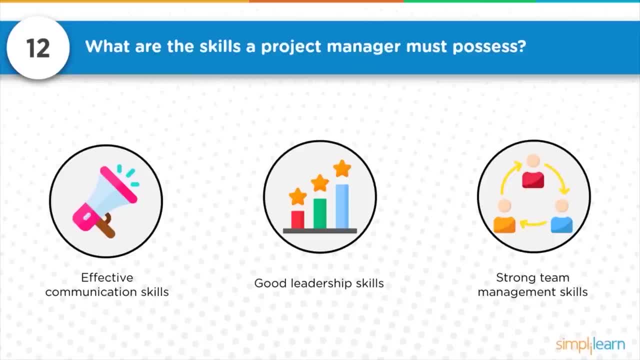 team dynamics ensuring the right education, right skill individuals are in place and they are monitored and managed. it is very important so there should be a little bit of mentoring, which needs to be done to the people regularly so that team gets what is expected out of them and they do. 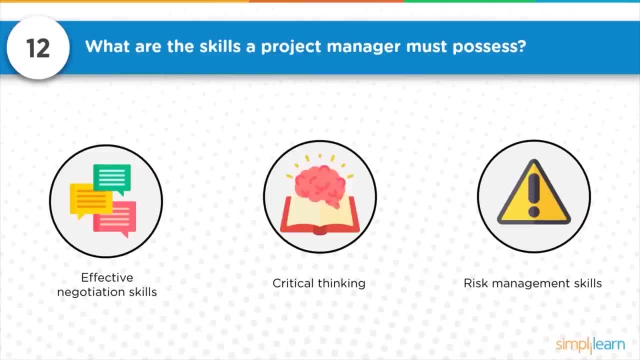 accordingly, then, effective negotiation skills, lot of scenarios, which comes in terms of negotiating in various different scenarios, negotiate to ensure things are been in place or in the interest of both the parties involved in the negotiation. it is very important to involve and make a right discussion, right set of discussion, so that 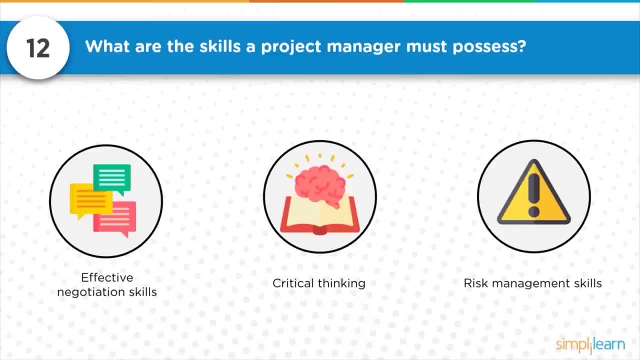 stakeholders are benefited. now, who are these roles we are speaking about? who would involve in negotiation? we can think of customers while establishing an agreement. we can think of teams while having some conflict resolutions which you take, team will have a conflict you may require to resolve. so suppliers. 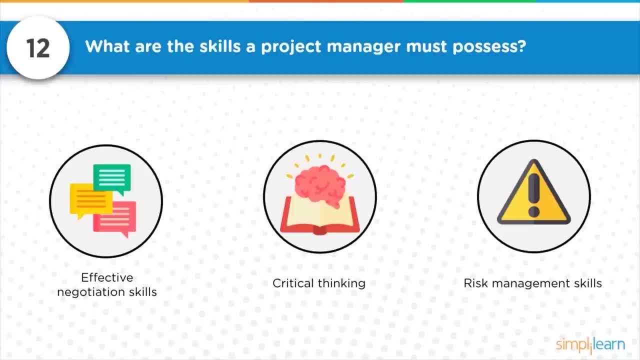 related issues which needs to be resolved. so negotiation is very important, but always negotiation is would be in the interest of both the involved parties. then critical thinking. so critical thinking in the sense not just seeing what is there, it's about how to set it right, how to take it forward. 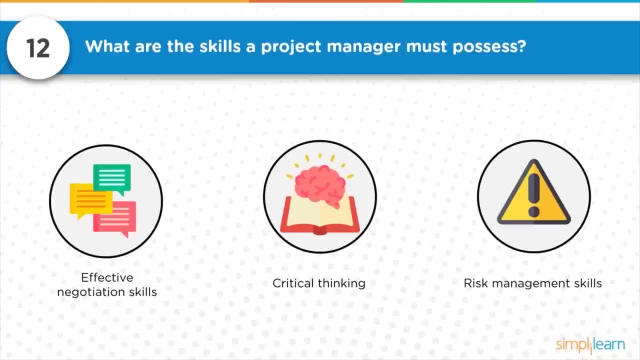 in the right direction. so what could cause? visualizing things is very important. risk management skills: it's quite obvious the most ignored area, what which I have seen throughout, is a risk management. so I don't know what is the reason. risk is ignored. many of the projects, what I have seen- almost like 80. 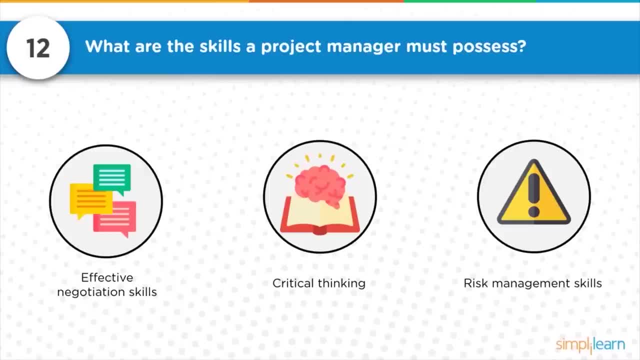 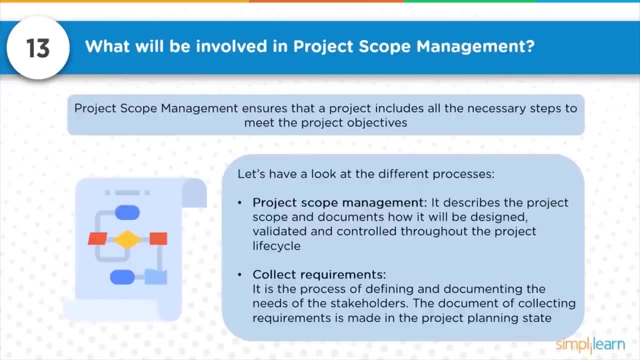 to 85% people don't even look at the risks. so it is very essential to look at the risk and manage the risk. only then project can become successful. so question 13: what will be involved in project scope management? so we already know project scope means it involves. 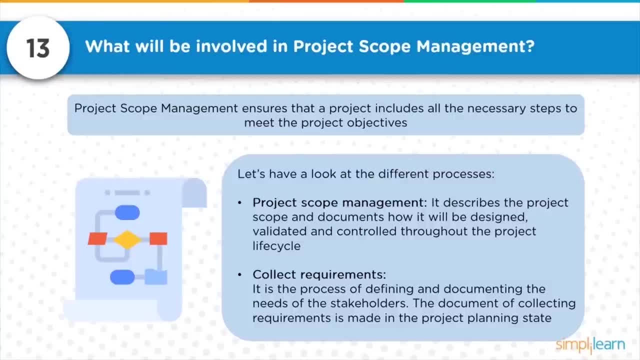 both project scope as well as product scope. now, scope management basically ensures project includes all those necessary things to be done in terms of activities, in terms of processes, in terms of resources, that project objectives can be accomplished. so this particular process- project scope management- describes the project scope. 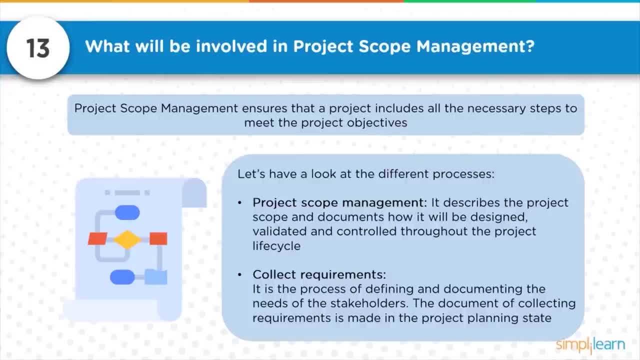 and documents how it will be designed, validated and controlled throughout the project lifecycle. so it collects requirement. so collect requirement process. engages with stakeholders, discusses with them to understand what is the requirement, collect the requirements, document the requirements and establish requirement management plan. then, based on this requirement establishment, 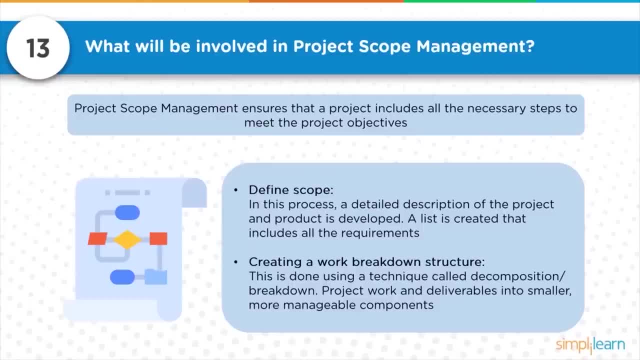 is established. scope has to be defined means the detailed description of the project and product has to be developed and a list has to be created that includes all the requirements, then creating the WBS work breakdown structure once the scope is defined. so now the decomposition of that scope. 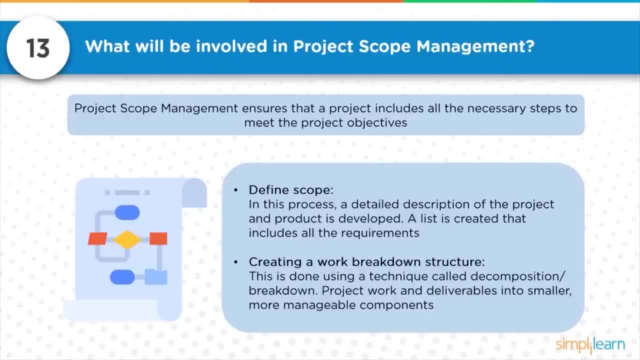 definition. what is given has to be taken into the lowest possible level. it has to be like. logically further, it cannot be subdivided, right? so decomposition basically helps in terms of breaking down those ultimate deliverable to multiple lower level parts. for example, if I consider a car, I 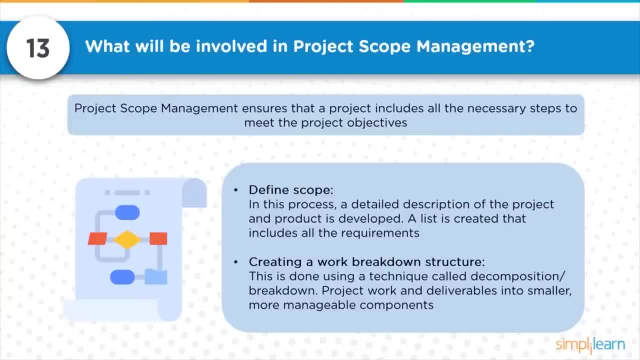 can think about two broad categories like exteriors and interiors. now, in exteriors I can think of a body of the car, the rearview mirror, the wheel, the bonnet, the glass. so I can just decompose like this now until I decompose to the mirror further. I cannot decompose in the 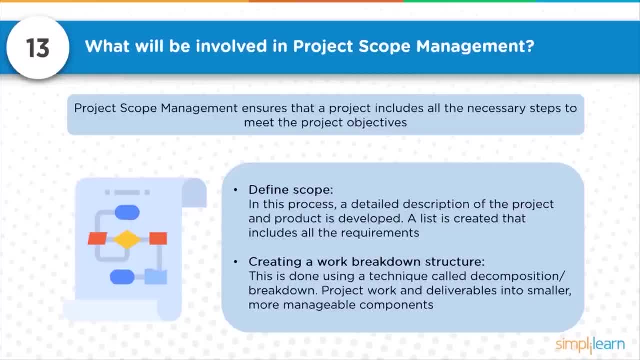 mirror. what are all the things we can think of? mirror cap, mirror glass, mirror mount, so further. can I subdivide this? no, so each of the components involved in all the perspective, in the car perspective, broadly initially decomposed it to the level interior, exteriors, and further down the line we 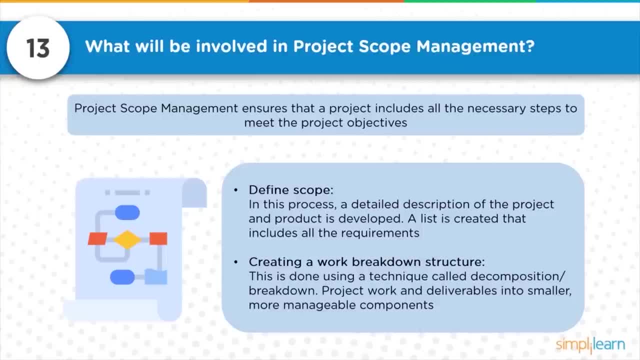 took to the next level of components further down the line. we again decompose it now at the lowest level. we actually look at the effort estimation, activity, resource required. all this we look at and we'll do bottom-up to consolidate to see what is the scope. so it will help us. 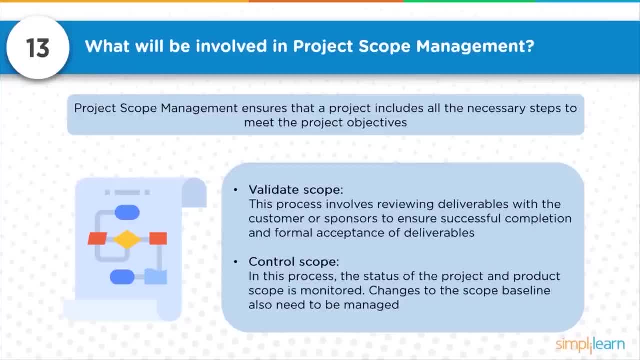 in becoming scope baseline. so validated scope is a process in monitoring and controlling which involves reviewing the deliverables with the customer or sponsor to ensure successful completion and formal acceptance of the deliverables. so formal acceptance is the key requirements when we validate the scope if it is not according to the plan. 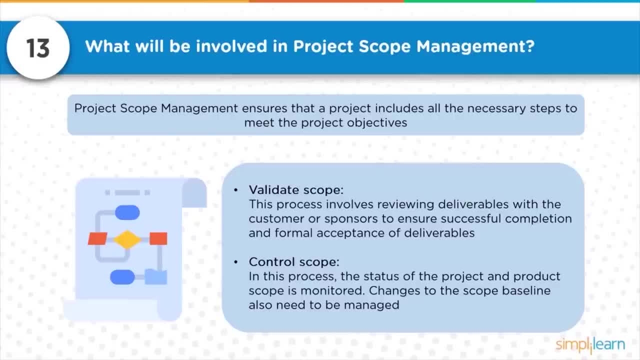 that is rejected and it is sent back for change and necessary corrections. then control scope. so in this process the status of the project and product scope is monitored. changes to the scope baseline, which is actually defined as part of the planning: if anything is seen in terms of deviation, that needs to. 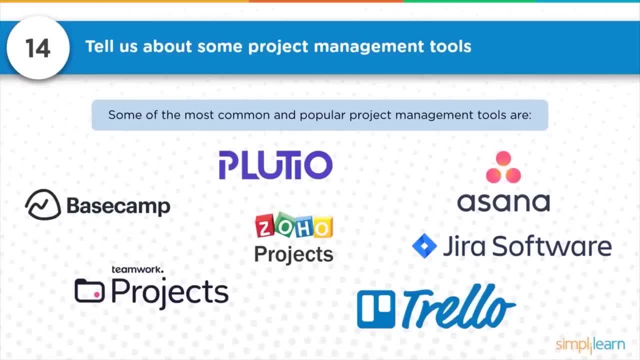 be corrected. the change request would be raised then. next question: tell us about some project management tools. so some of the most common and popular management tools which have come across are listed here, like Plutio, Basecamp, teamwork projects, Zoho projects, Hasana, Jira, software, Trello- I think. details of this. 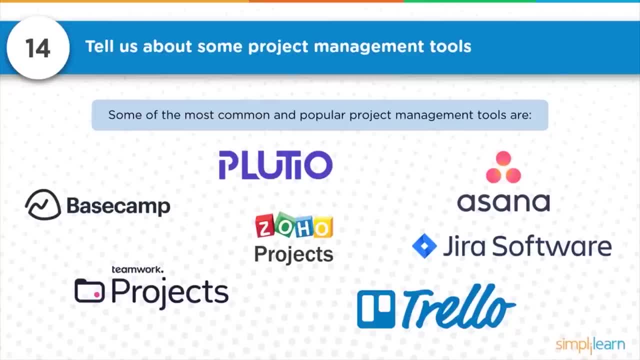 you may require to go to individual tool sections and then review those better. if you can able to create a comparison sheet always helps in terms of understanding what is that features functionality each of this tool has. so one more tool which is not mentioned. it is Microsoft project. 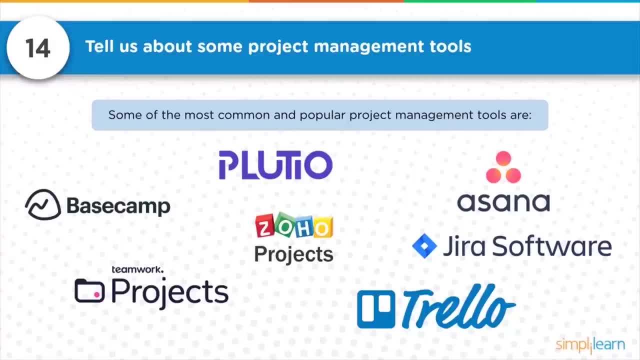 so, which is also another popular tool which is used, and similarly I can mention like Primavera. so each of this has its own advantages- disadvantages, so you may require to list out what do you exactly want in terms of when you take up a tool for project management and 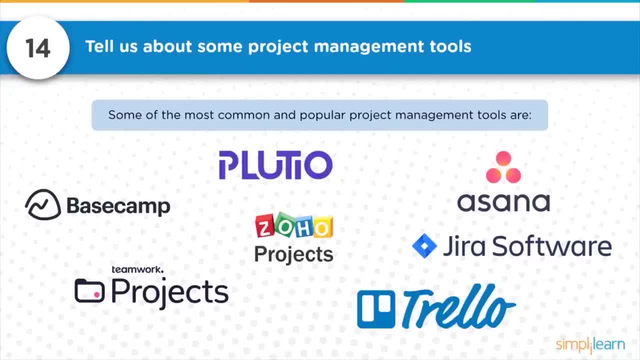 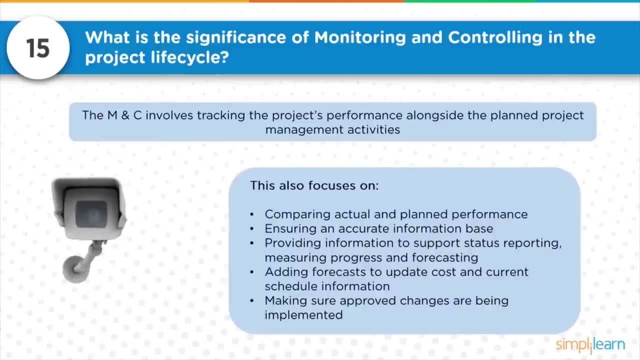 what each of this tool has. if you can able to create a comparison sheet, that would help you in terms of selecting the right tool for your organization and projects. question number 15: what is the significance of monitoring and controlling in the project lifecycle? so, as we know, monitoring and controlling is. 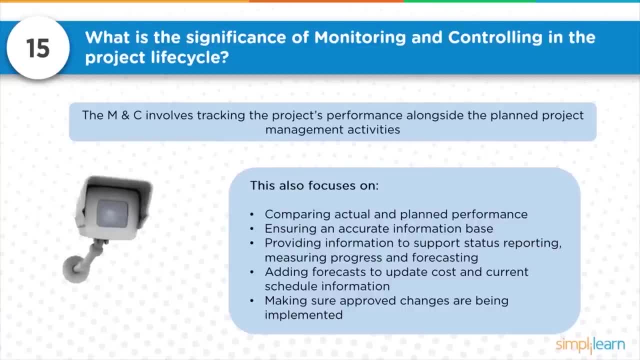 a process group. so this involves tracking the projects performance alongside the planned project management activities. this also focuses on comparing actual and planned performance. so we have defined that in the planning. so what needs to be accomplished, how it has to be accomplished, what templates are to be used, what. 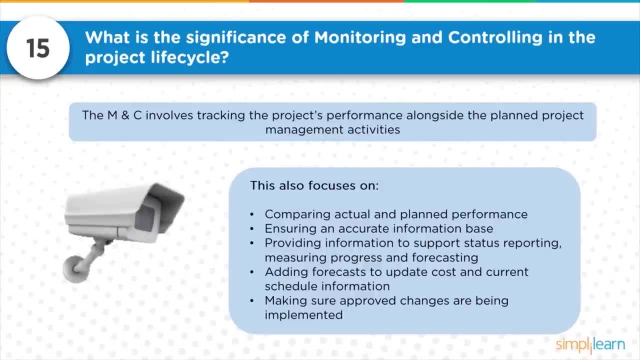 needs to be delivered. we have defined it in planning, so that needs to be compared with actual thing: what is created and what is that? how are we doing this currently? what it is done, is it complied with? assessing performance to determine any corrective actions are identified, their status reported and 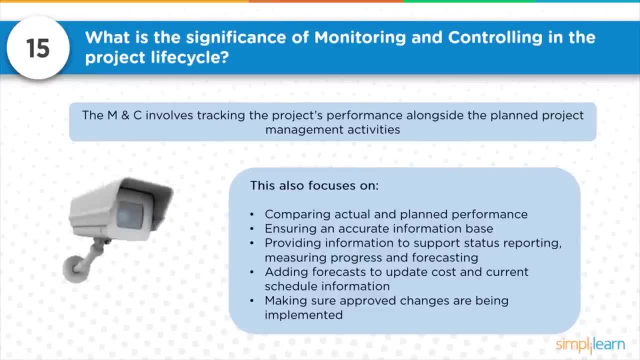 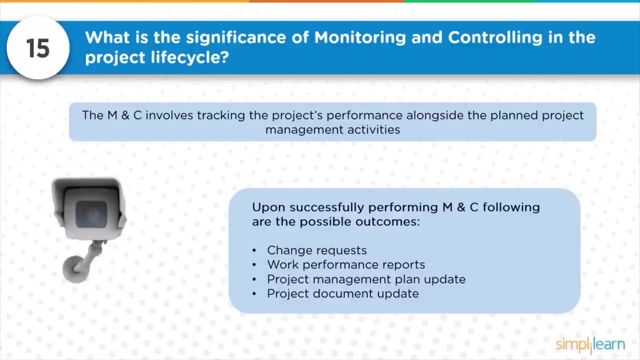 appropriate responses to risks are taken, so ensuring an accurate information base, providing information to support status reporting, measuring progress and forecasting, and then adding forecasts to update cost and current schedule information, making sure approved changes are being implemented upon successfully performing monitoring and control the processes within monitoring and controlling process group. 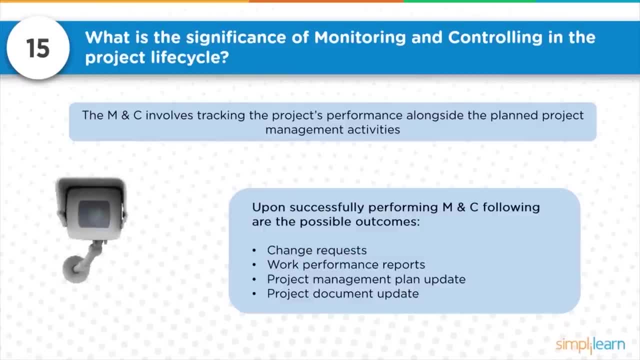 so the possible outcomes would be like the change request, work performance reports, update to project management plan and project documents. maybe, if everything is okay well, for example, validate scope, which comes under this process group. so when we validate if everything is okay as per the plan, then it is accepted, deliverable, which will 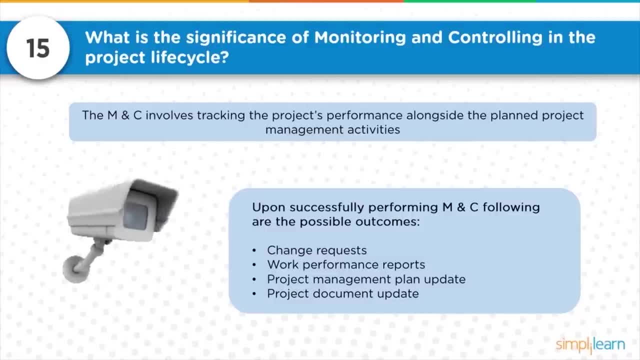 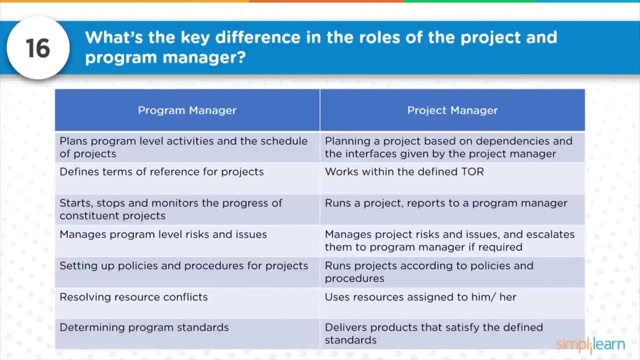 move towards the closure? if it is not, obviously it leads towards change requests. so question number 16: what's the key difference in the roles of the project and program manager? so project manager is basically focuses on projects and its success of the project, as we know already, whereas program 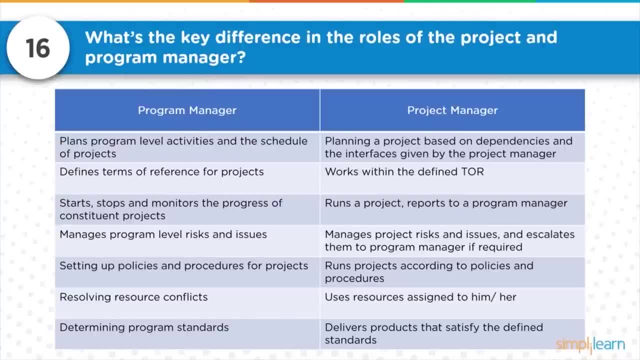 manager looks at all those projects which fall under the program. are managed together and taken forward in the required direction. so program manager plans program level activities and the schedule of projects. so program managers defines terms of reference for projects. they starts, stops and monitor progress of constituent projects. manages program. 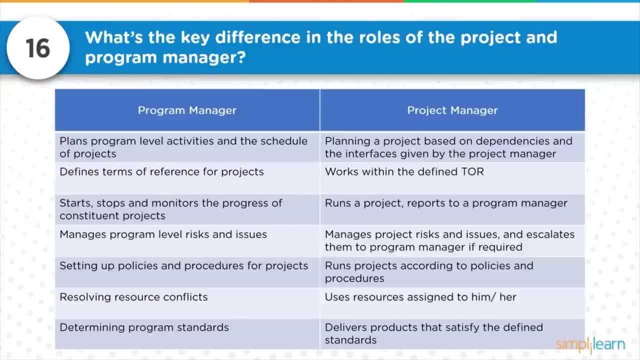 level risks and issues. they set up policies and procedures for projects. they resolve conflicts. they determine the program standards. similarly, project manager focuses on planning a project based on dependencies and interfaces given by the project manager, so works within the defined tar terms of references given for the projects runs. 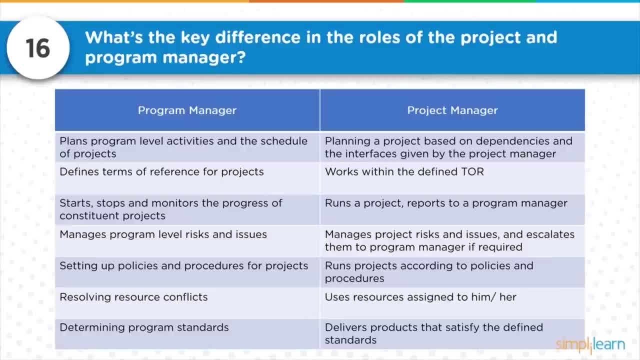 a project, reports to program manager, manage project risks and issues and escalates them to program manager if required. if at all, a project is part of a program. if it is not, then that escalation goes to sponsor. so project manager runs projects according to the policies and procedures, uses resources. 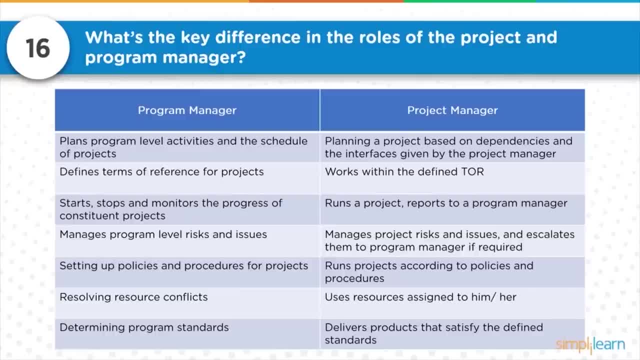 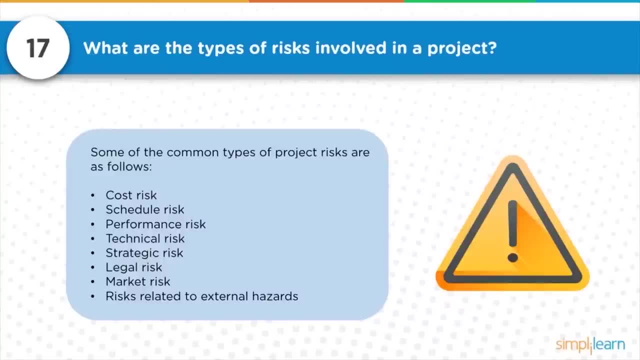 assigned to project manager and delivers the products that satisfy the requirements. question number 17: what are the types of risks involved in the project? so we know that one of the knowledge areas in the project management is risk management. it is very essential for us to identify risk, assess and analyze. 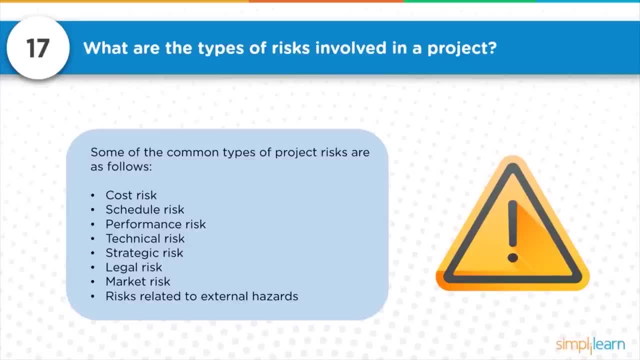 risk and have the risk response plans. so while doing it, it is also very important for us to understand categorizing the risks, depending on where, exactly what category this risk falls into, by depending on the impacts. for example, some of the list which is given, common types of risk. there is categories you can think. 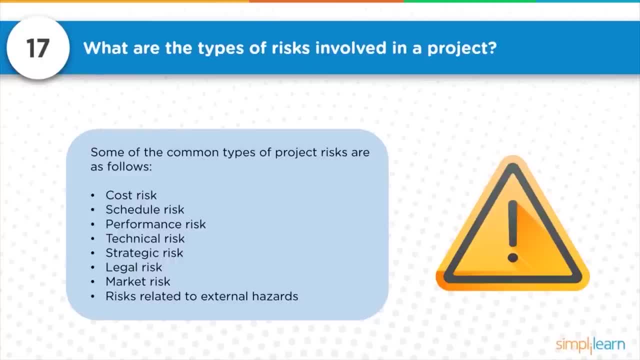 of it may be related to cost, schedule, performance, technology or technical, strategic, legal market risk, risk related to external hazards, and it goes on. so these are the minimum set of list which we can think of in any project. the kind of risk are associated with which area. so when I say cost associated risk, 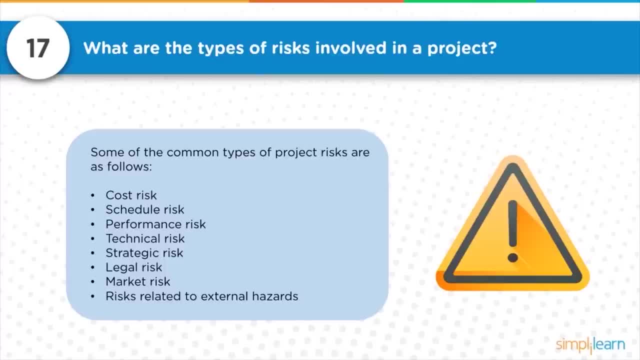 it's all about monetary related, where we invest, where we actually monitor that budget, involve that budget, incur that cost related to that schedule, in terms of doing it faster, doing it slower, doing it as per the plan. so various different details which are associated with the schedule. likewise, each of these types. 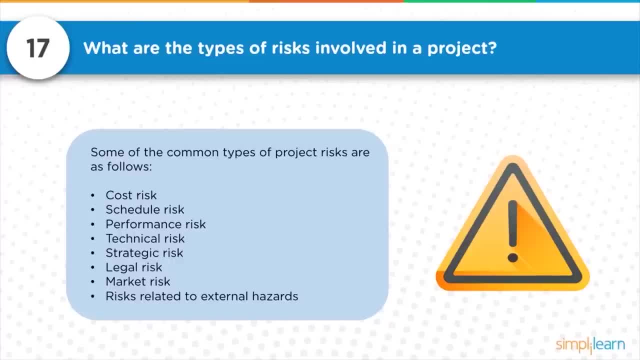 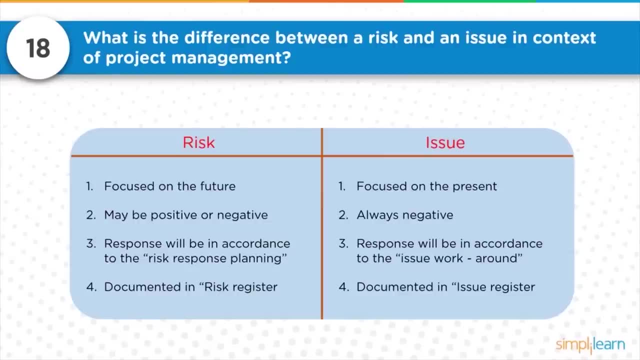 what we have mentioned will have a risk accordingly associated with them. so question number 18: what is the difference between the risk and a issue in context of project management? so when we say risk is always we look at in the future, so it's an uncertainty of outcome. 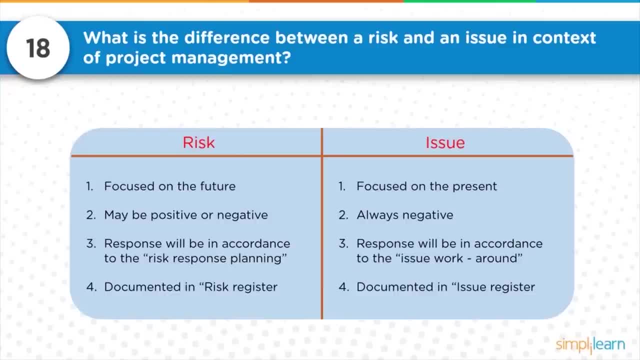 when we say risk, we are looking at a future. it may be next moment in the future, but it is risk which is focused on the future. so risks may be positive or negative. any risk we identify may have positive or negative impact, whereas risk response will be in. 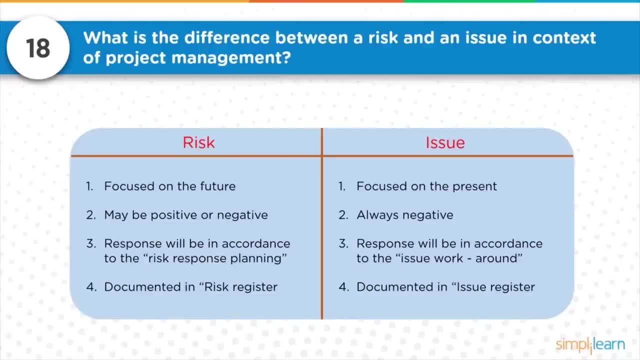 accordance with the risk response planning and this are documented in risk register. so issue is always the one which we have in front of us to manage, so it is focused on present. always negative, it will have negative impacts. so response will be in accordance to the issue workaround provided, and these are: 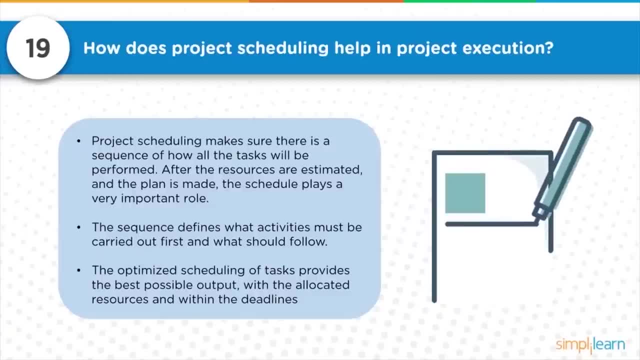 documented in the issue register. so next question, question number 19: how does project scheduling help in project execution? project scheduling make sure there is a sequence of how all the tasks will be performed after the resources are estimated and plan is made. the schedule plays a very important role. 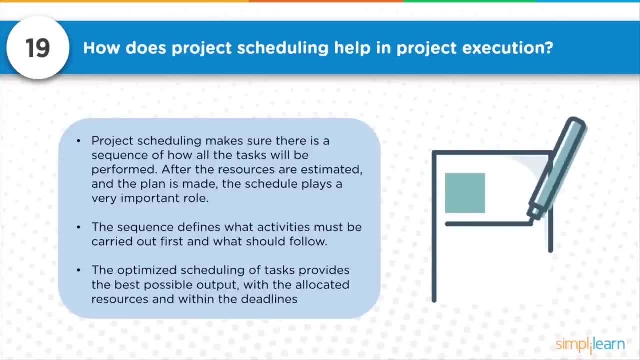 because when to do when it is planned, it is very essential to do accordingly. so providing the sequence- what activity has to be done in what sequence? it's also very important. so this must be carried out first and what should follow needs to be clearly understood. the optimized 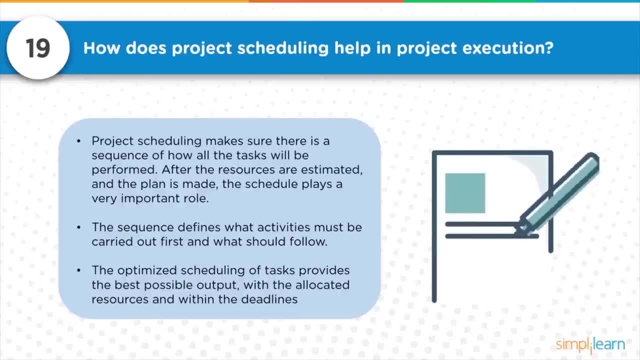 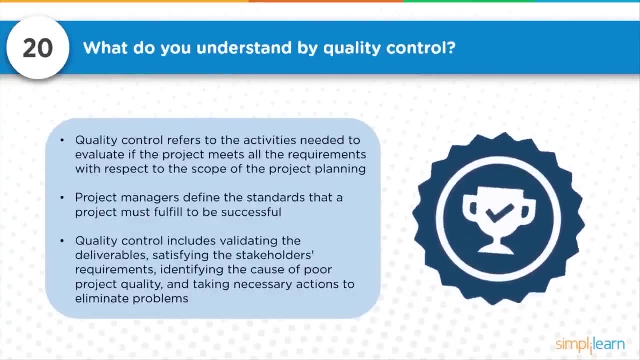 scheduling of tasks provides the best possible output with the allocated resources, and that has to be done within the scheduled time, within the deadline. question number 20: what do you understand by quality control? now, quality control refers to activities needed to evaluate if the project meets all the requirements with respect to the 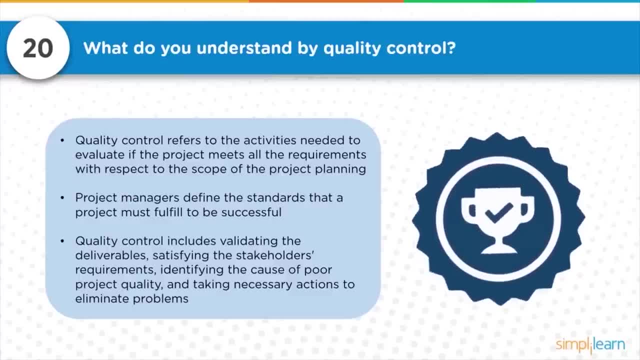 scope of the project planning. now, when we say a control, we should think about the output of a project, the deliverable. it has a specifications, so relating to that specifications, the features, functionalities, what needs to be delivered, is it delivered accordingly? so, project managers, defines the standard that the project must fulfill to be 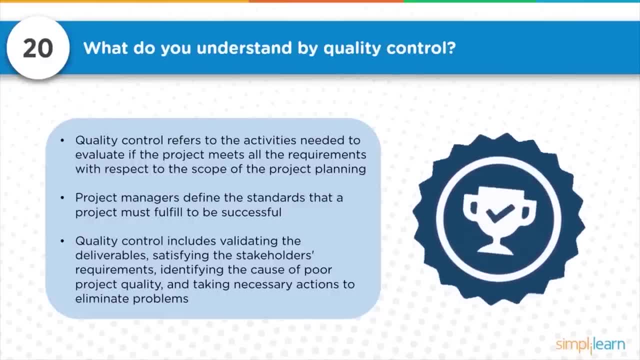 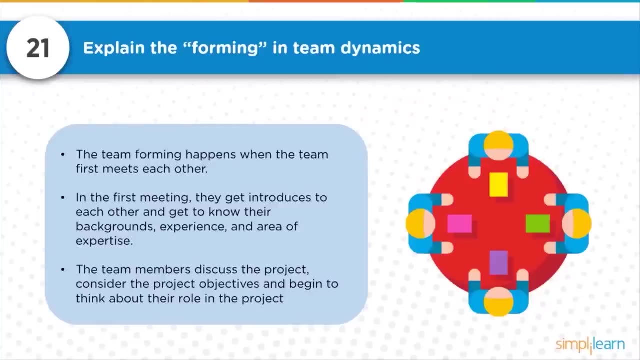 successful quality control includes validating the deliverables, satisfying the requirements of the stakeholders, identifying the cause of poor project quality and taking necessary actions to eliminate problems. right question number 21: explain the forming in team dynamics. basically, when we say team dynamics, it involves various different stages, like 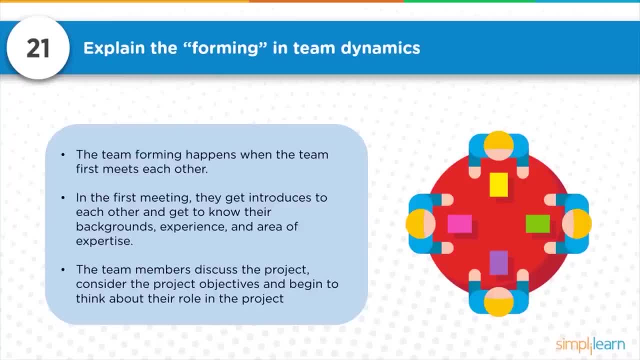 forming, storming, norming, performing and our journey. so forming happens first now. this happens when the team first meets each other. so when they meet each other they get introduced to each other and get to know their backgrounds, experience and areas of expertise. the team members discuss about the project, discuss the 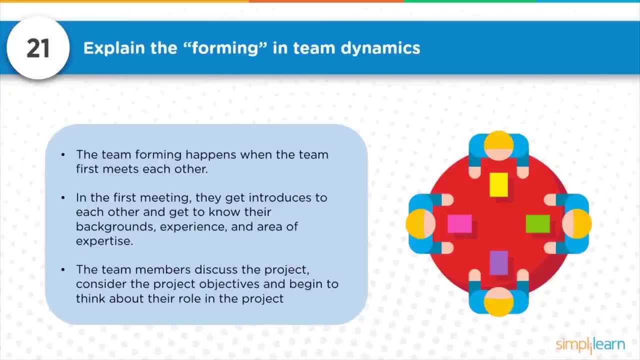 project objectives and discuss the project objectives and beginning to think their role in the project. they beginning to understand. they know what is this project is all about. so, in detail, what is this project is all about will be understood by them in storming, which is the next stage in the team. 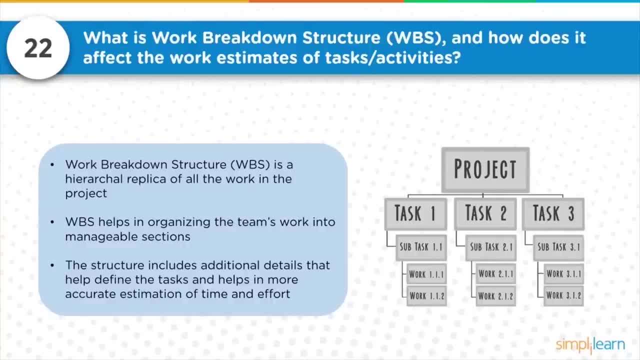 dynamics. question number 22. so what is work breakdown structure and how does it affect the work estimates of tasks or activities? work breakdown structure is a hierarchical replica of all the work in the project. for example, if I take up a specific object, a specific products or services which we are bringing out as a 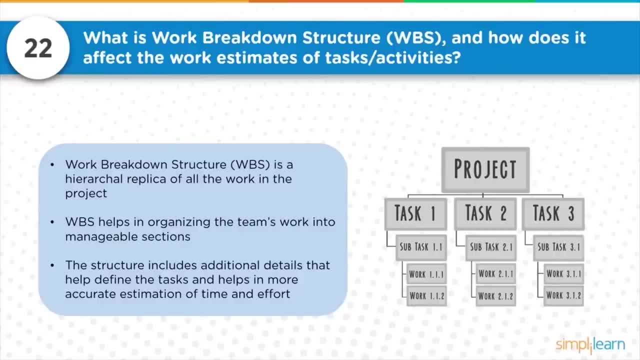 result. for example, if I take a car, so how will I visualize various different parts of the car? it's very difficult in one go in in execution perspective and creation perspective we may require to know every parts of it in detail. so work breakdown structure is established using decomposition as a technique, which 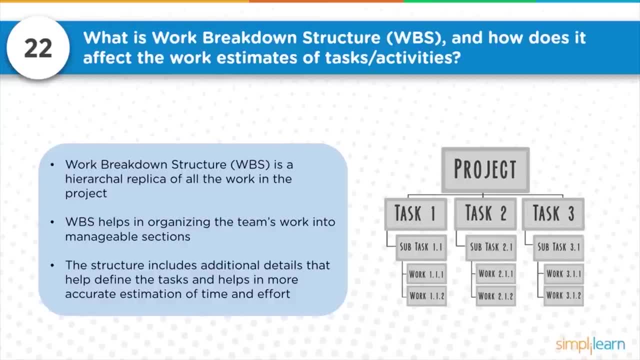 means, for example, if I take car as an example, car has a hole when it is constructed. so I have to visualize broadly. I would classify that into: decompose it to the first level, like exteriors and interiors. after exteriors I can further decompose the exterior. 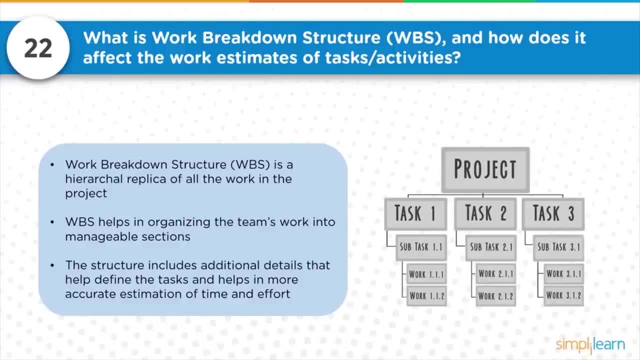 part of it. similarly, after interiors, I will decompose it further in exteriors. what are the things I can think of like exteriors? in terms of glass, in terms of body, in terms of tires, in terms of wheel, bonnet mirror, rear view mirror, which is outside? so, likewise, I love various 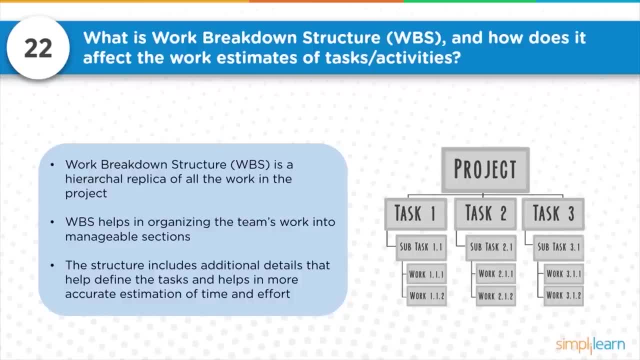 different decompositions level. that is the third level of decomposition, next third level of decomposition. I can go in each of these parts what I said. I can further elaborate those if I take the rear view mirror as an example. so I can think about mirror cap, I can think about 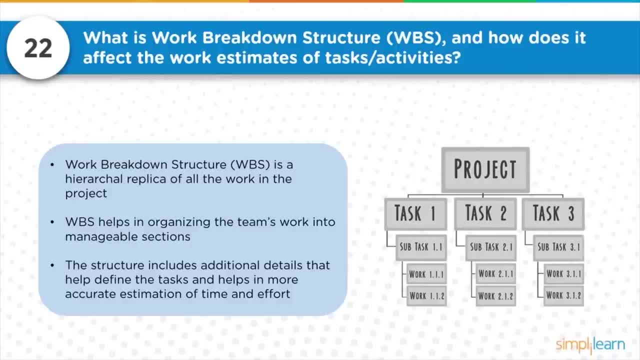 mirror glass, I can think about mirror mount. so these are the various different decomposed levels below mirror. similarly, if I come to interiors, we can think about entertainment system, you can think about seeds, we can think about AC- right, so we can think about anything else like dashboards. now, each of these components. 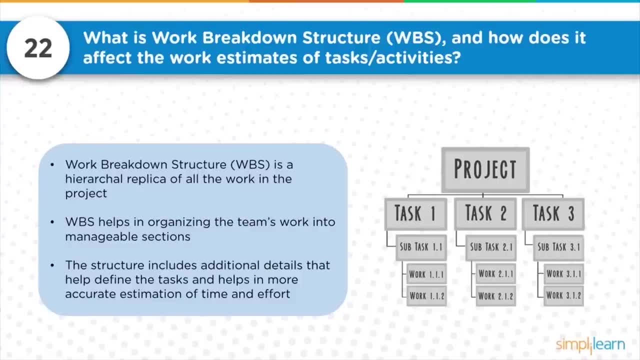 further, I can decompose. so the idea of decomposing is- I am going to understand what are the various product parts are involved to make a bigger product as a whole. so once I accomplished that, I will have a details at each of these levels and consolidate upwards as shown in the 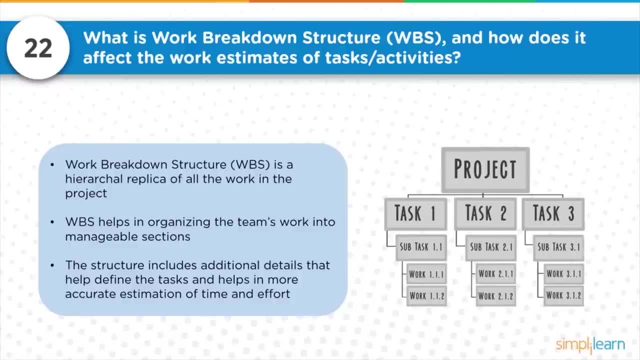 picture here, the first level, task 1, task 2, task 3. before I assign these tasks, I will have the product breakdown structure first and from bottom level I start adding up the activities, effort estimation and then I keep consolidating upwards. similarly, I will put the cost components to it. I will 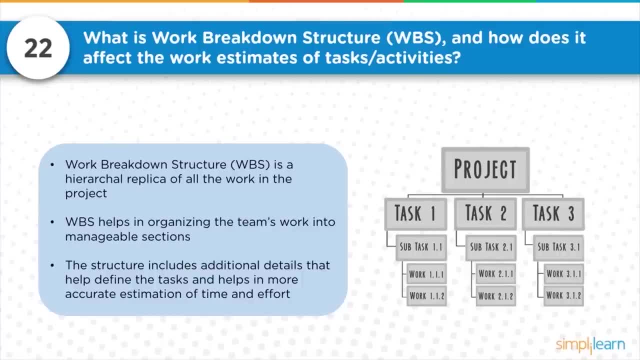 estimate the cost involved with the one which is required and then I go upwards and consolidate. so WBS helps in organizing the work in a manageable sections. so this would help in establishing additional details which would help in defining tasks. helping in estimation helps in when I say 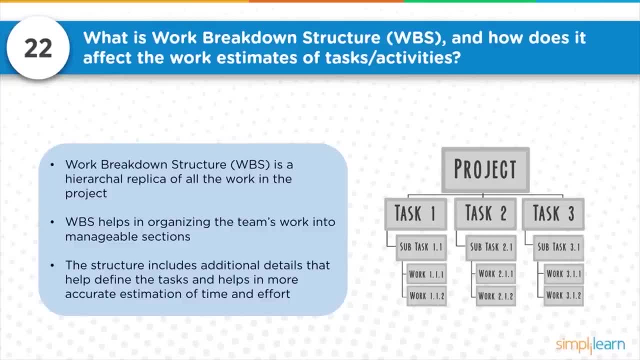 estimation. it is not just specific estimation, it's about cost estimation, schedule estimation, effort estimation, and then this will also help us in terms of sequencing further. so what breakdown structure will also have something called WBS dictionary, which gives the description of all the WBS elements. next question, question number. 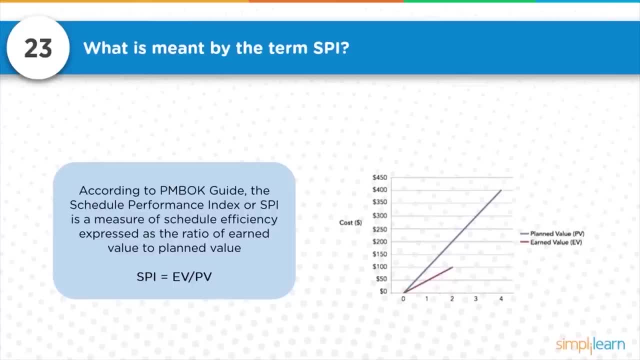 23, what is meant by the term SPI? now, SPI refers to schedule performance index. so schedule performance index is a measure of schedule efficiency expressed as a ratio of earned value to the planned value. so when I say earned value, I mean earned value. earned value is the actual. 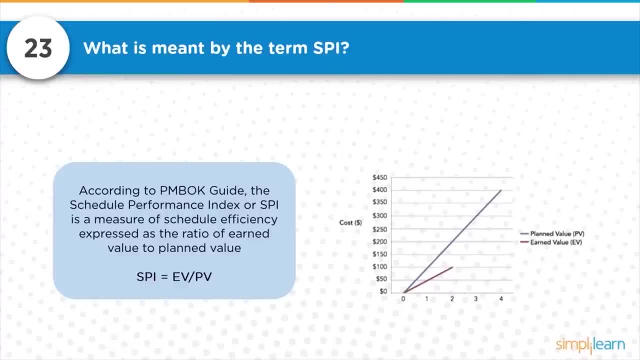 work which is completed. the value- the budgeted value for the actual work which is completed and planned value- is the budgeted value of the work which is supposed to be accomplished as per the plan now. this will help us in understanding how the project is progressing in schedule perspective. if 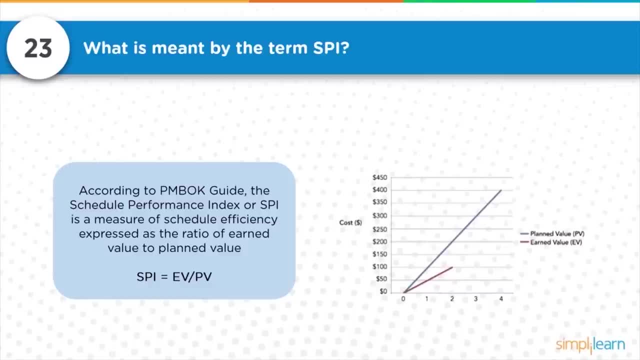 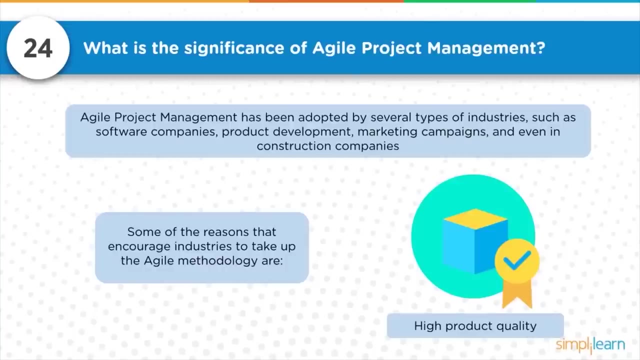 SPI is lesser than one means it is behind schedule. SPI is more than one, it is head of schedule. if SPI is one, it is as per the plan. schedule is as per the plan. question number 24: what is the significance of agile project management? so when we say agile, the 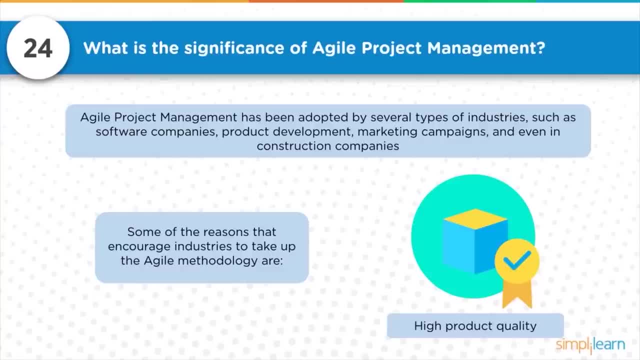 terminology itself refers to quick response, flexible, moving faster. so while we do agile project management, it is very essential to look at the various dynamics around. so it may be a quick response: what you need to give right. so predominantly agile methodologies are today adopted in various types of 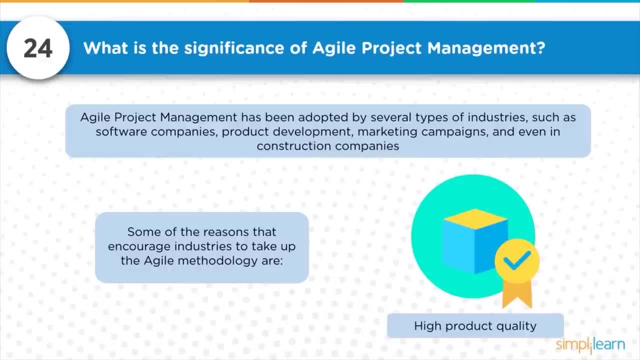 industries. so currently we see more and more in IT and software industry, then product development, marketing campaigns even in constructing companies. some of the reasons that encourage industries to take up agile methodologies are high product quality, high customer satisfaction, reduced risk, better and faster ROI. now let us look at the 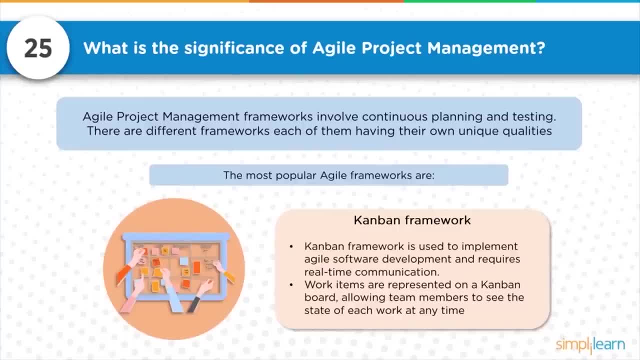 question number 25: what is the significance of agile project management? so the agile project management frameworks involves continuous planning and testing. so there are various different frameworks, each of them having their own unique qualities. so it is very essential for us to understand what are those various different agile 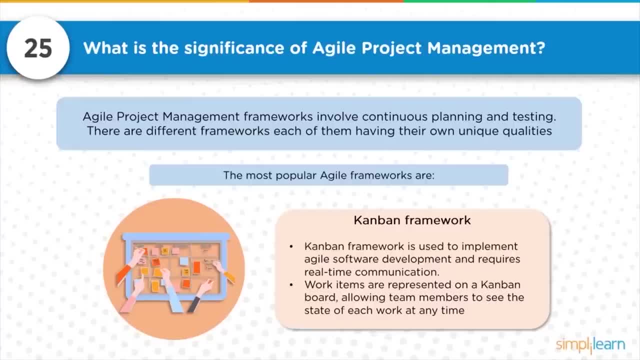 frameworks and how they are going to contribute to become agile. so the most popular agile frameworks, some thoughts which actually depicts and supports organization to become agile are. one of that is Kanban framework. so Kanban framework is used to implement agile software development and requires real-time communication. so work items. 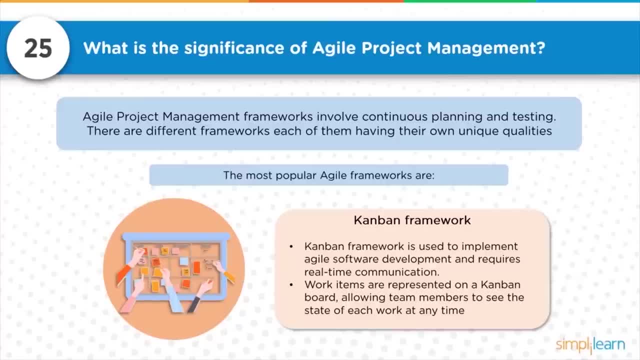 are represented on a Kanban framework, allowing team members to see the state of each work at any time. so this means on the board. so work in progress, work which has to be done and who has to do it- all these details are captured in the Kanban board. now very important. 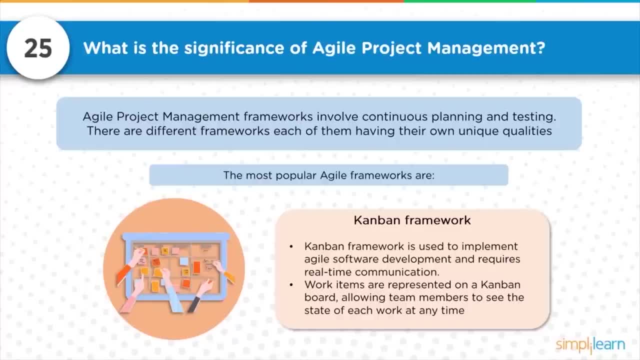 point here is when these are captured is very essential to understand. it is a visual board, so when it is a visual board, it's quite obvious anyone who has actually have a task against them. they don't hesitate. they need to complete it. it forces them, since it is a visual. 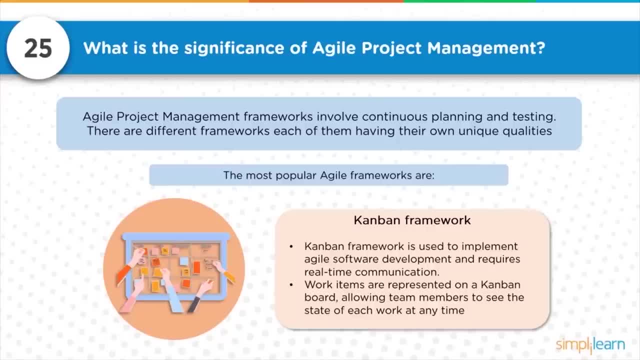 system. since it is a visualized system, it works on their consciousness, so it is also called a spool system. so because people pull the work from that list whatever is given and then accomplish it. so this will also help in tracking the progression of a project, how it is. 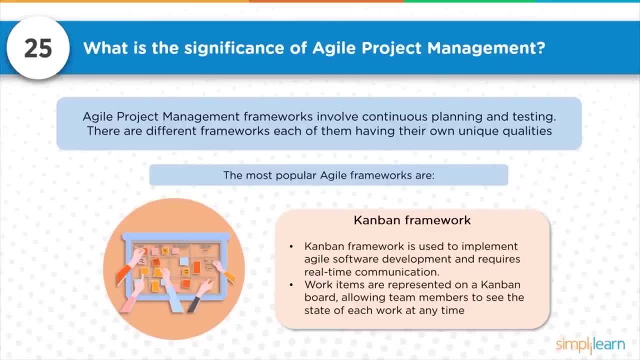 progressing. so how the project is progressing, how the tasks are being completed, how quickly they are completed. so it is easily visible and that makes things to more smoother and faster. so scrum framework, so scrum framework- helps in dealing with complex problems and making it possible to deliver. 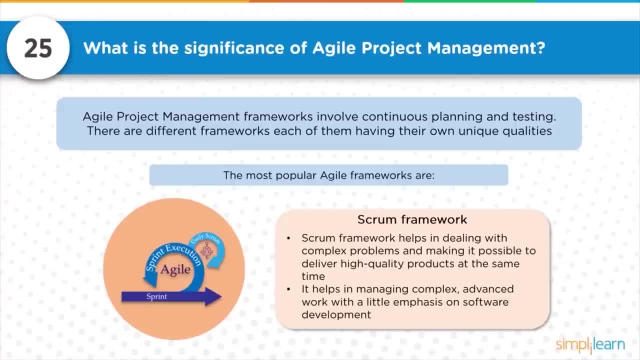 high-quality products. at the same time it helps in managing complex advanced work with little emphasis on software development. so it uses the terminologies like sprint product backlog, sprint backlog, daily scrum, retrospective meeting. so three roles predominantly we come across, that is product owner, scrum master and then self organizing. 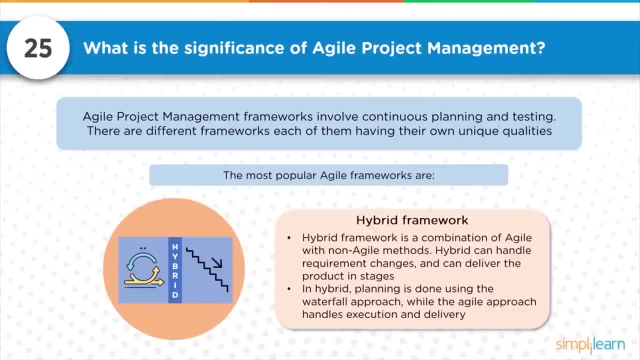 team. so next framework is hybrid framework that you can think of. so it is the combination of agile methods with non-agile methods. hybrid can handle requirement changes and it can deliver products in stages. so in hybrid model, planning is done using a waterfall approach, while the agile approach 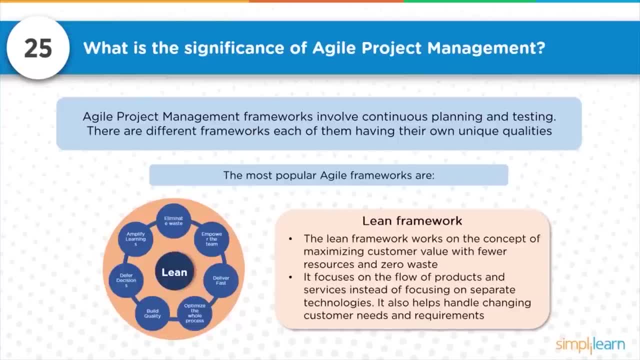 handles execution and delivery, so lean framework. so the lean framework works on the concept of maximizing customer value with fewer resources and zero waste. hence lean focuses on the flow of products and services instead of focusing on separate technologies companies can act upon with changing customer needs and requirements. so very important points. 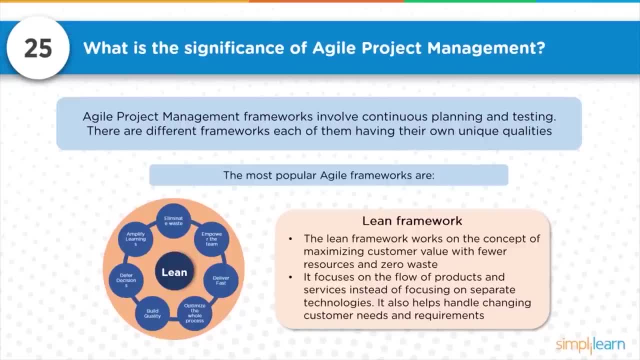 to observe here. zero waste means in the flow, the way the processes are connected to each other in that flow. we should identify what are those which acts as a bottlenecks resulting in waste. so we should eliminate such bottlenecks. so these elimination of bottlenecks helps. 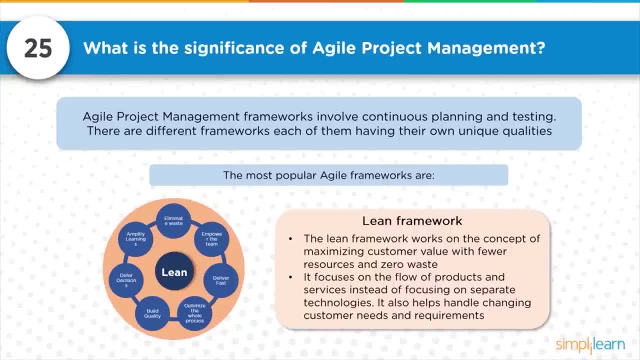 in reduction of waste, at the same time increasing the value to the customers. so in the downstream, from the point of where bottleneck you have, the entire capacity will get limited to the downstream capacity I'm speaking about will get limited to the bottleneck where that particular issue exists. right that? 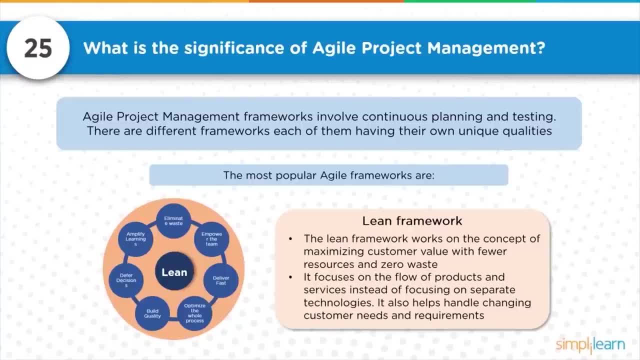 needs to be resolved. elimination of way should happen, so waste is a result of anything which is a non value adding activity, right, so we need to identify. as for the lean perspective, so the defects are not allowed to move forward to the downstream. that is the whole idea behind. 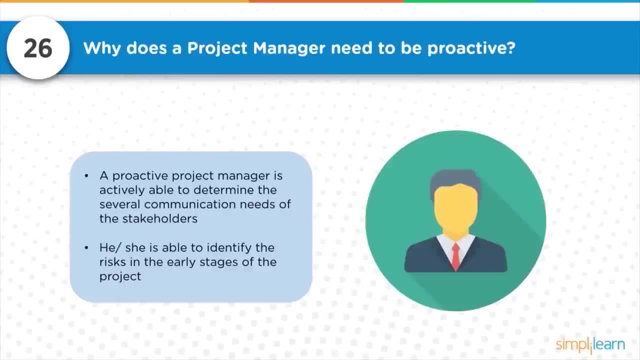 it. so next question 26: why does a project manager need to be proactive? okay, so we always have this question coming around: proactiveness versus reactiveness. when should we be proactive, when should we be reactive? that we need to understand now. more proactive in nature, the project manager or any. 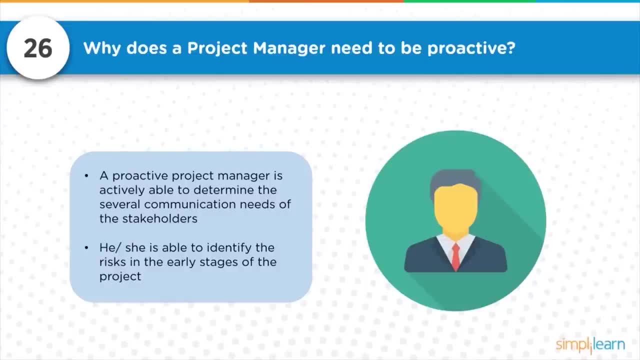 manager who is more proactive will basically visualize the future. so they act today so that tomorrow something negative impact will not happen. so a proactive project manager is actively able to determine the several communication needs of the stakeholders. so a proactive project manager is able to identify the risks in the early. 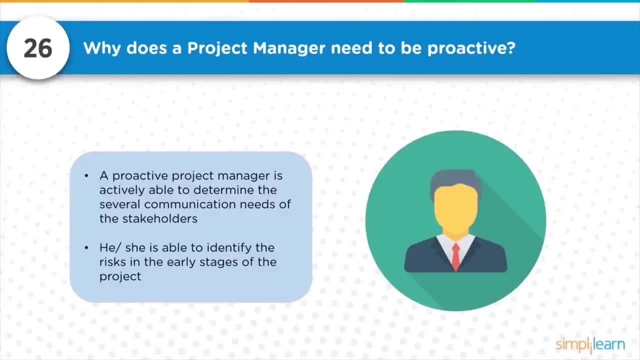 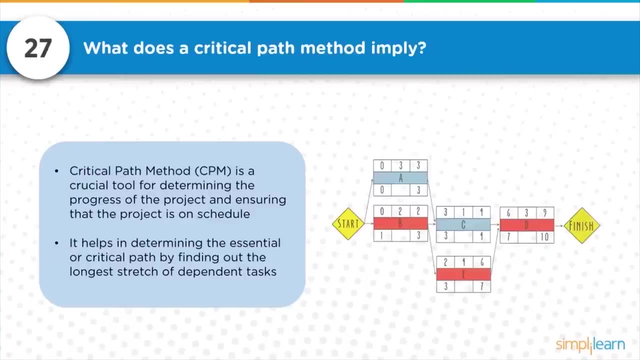 stage of the project. it is very essential. so what is that going to happen in future? that needs to be visualized. act today so that that occurrences can be handled better or eliminated. question number 27: what does a critical path method imply? so firstly, let us understand what is critical path. 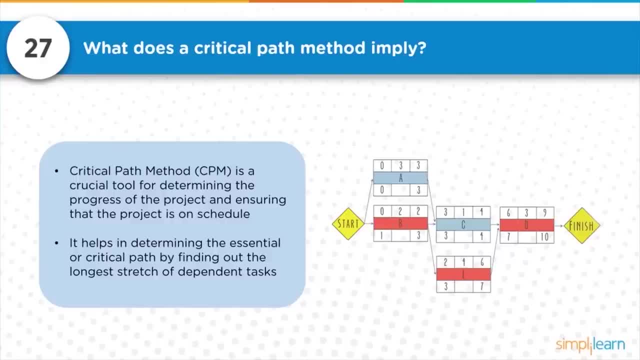 means. so critical path is basically a longest path in a given project network diagram. so that would be the minimum time required for a project to complete. so any delay in any of the activities or tasks in critical path delays the project duration. so in critical path method. so it is a crucial tool for 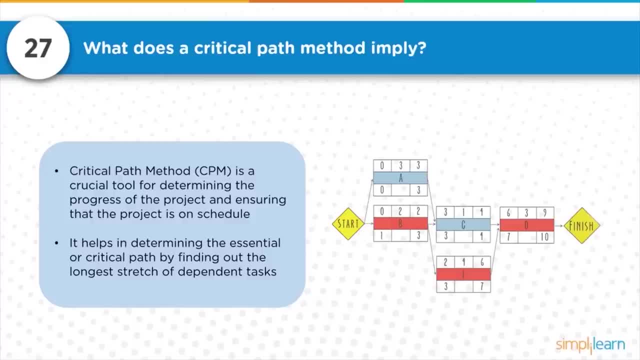 determining the progress of the project to ensure that project is on schedule. so, as I mentioned, any delay in any of the activities or tasks in the critical path delays the project itself. so monitoring on these activities in a critical path will become more important so that project can happen as per the plan. as 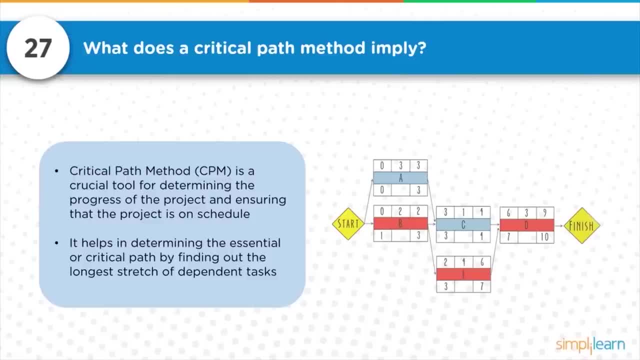 per that date. what is given so critical path method helps in determining the essential or critical path by finding out the longest stretch of dependent tasks so that each dependencies, each flow from left to right, from beginning to end, has to be visualized and monitored very closely so that project. 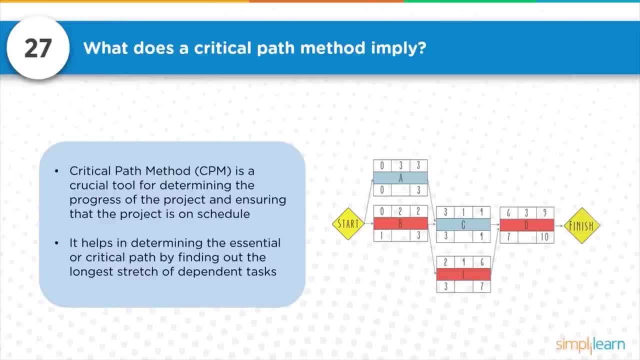 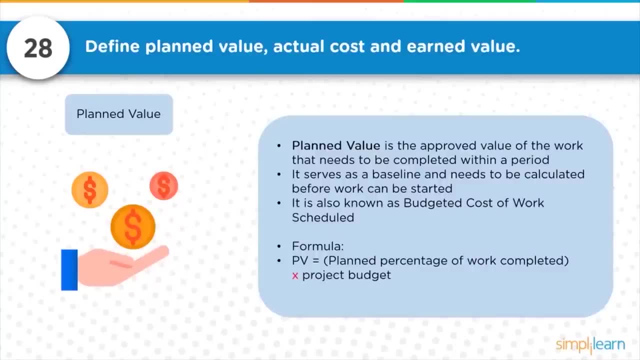 finish date is not delayed. it happens according to the plan. so next question: defined planned value, actual cost and earned value. so when we say planned value, planned value is the approved value of the work that needs to be completed within a given period. it serves as a baseline and needs to be. 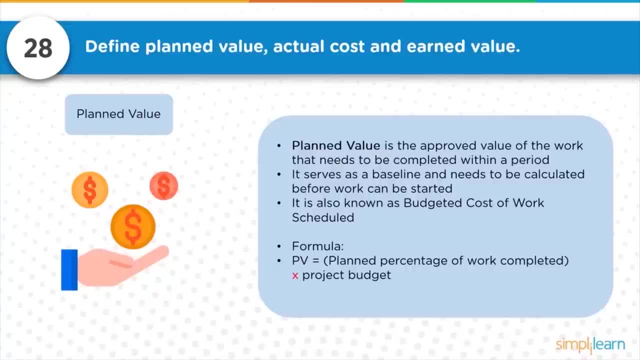 calculated before work can be started. it is also known as budgeted cost of work schedule. so formula to calculate planned values, planned percentage of work completed into project budget. assume your project budget is 10,000, whatsoever the currencies. let us assume 10,000 is my project budget, so my 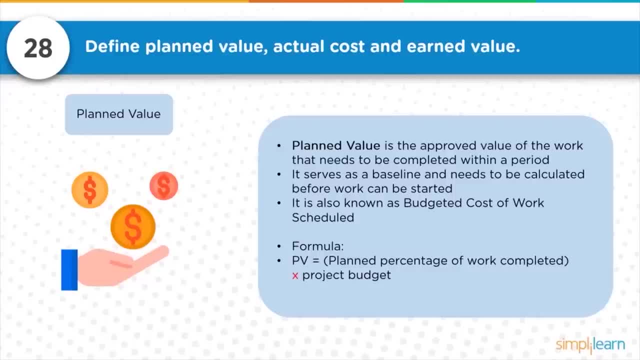 project duration is five months. each month have a plan to complete the work worth of 2,000, so which means that 2,000 is my planned value. the work which is supposed to be accomplished within the end of that first month is work worth of. 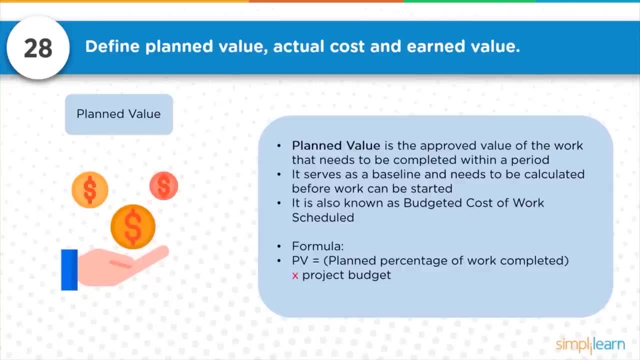 2,000. so if I do the work which is lesser than work worth of, maybe lesser than 2,000, I am behind schedule. if I complete the work worth more than the 2,000, then I am ahead of schedule. so planned value will become that reference. 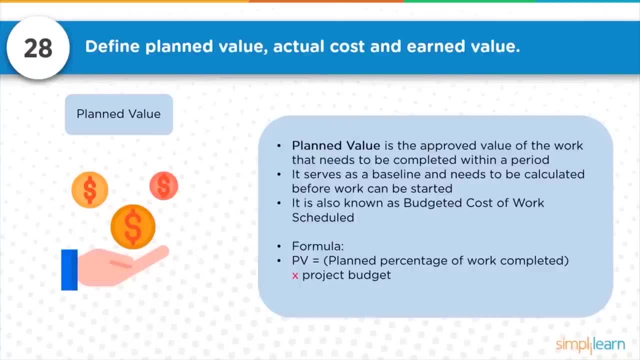 the 2,000. what I mentioned as a planned value, the work worth of 2,000 I'm supposed to complete before the end of the month one. if I say any work which is completed according to the budgeted value, I will make this planned value as. 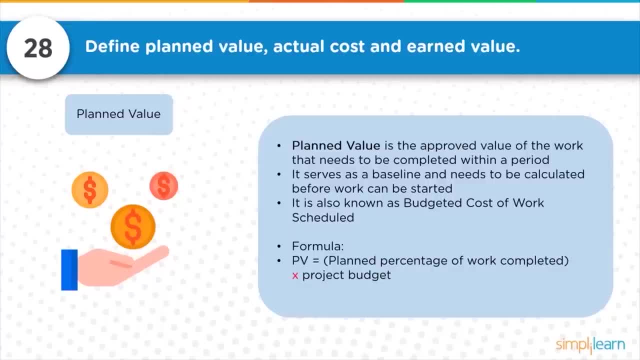 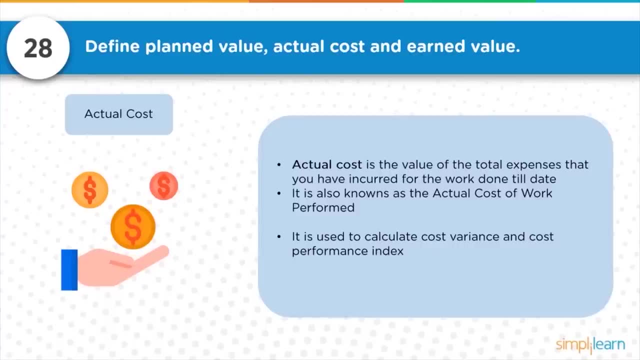 a reference to decide whether I am behind schedule or ahead of schedule: actual cost. actual cost refer to the value of total expenses that you have incurred for the work done till date. for example, in the previous discussion relating to the planned value at the end of month one, the planned value was 2,000. 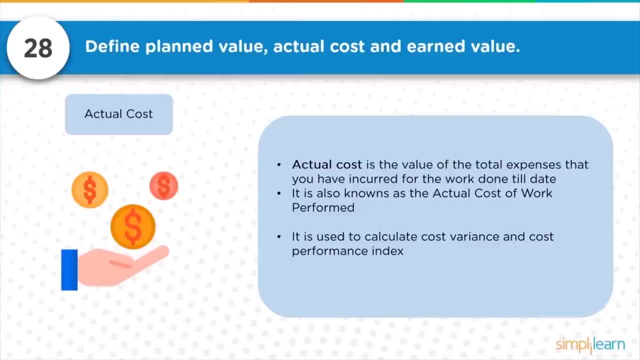 so that is the work worth which was supposed to complete. let us assume we have completed a work where the work worth relating to that actual work completed is around 1,800, means I'm behind schedule, for sure, but at the same time to complete the work worth of 1,800. 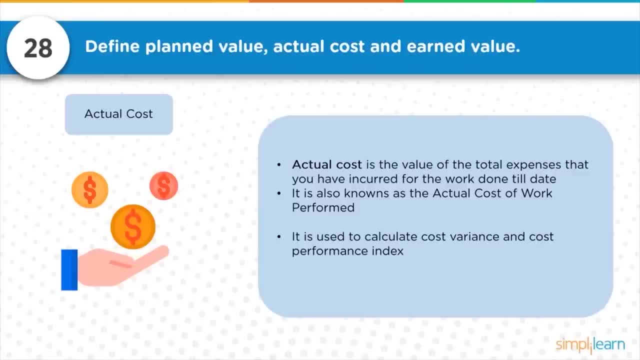 how much I incurred actually. so if I have incurred actual cost, also 1,800, then cost wise I'm according to the plan but behind schedule because I have only completed the work worth of 1,800 against the work worth of 2,000, which is 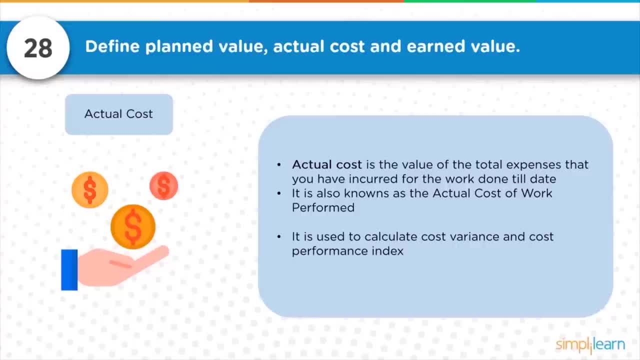 a planned value and behind schedule. but to complete it the actual cost I incurred is 1,800. so cost wise I'm according to the plan. if my actual cost is lesser than 1,800 then I'm doing very good in cost perspective. if my actual cost is. 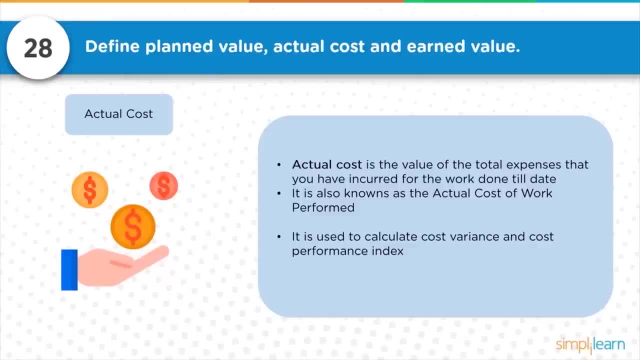 more than 1,800, then I'm using more money means over budget. so actual cost helps us in relating to planned value to define whether cost wise. how am I doing so? it is also known as actual cost of work performed, so this will be used to calculate cost variance and cost. 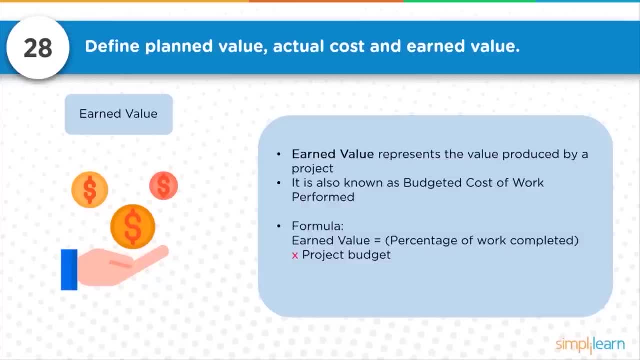 performance index earned value. earned value represents the value produced by a project. it is also known as budgeted cost of work performed. in our example, the earned value is 1,800, meaning I have completed the work worth of 1,800. that is the earned value, which says: 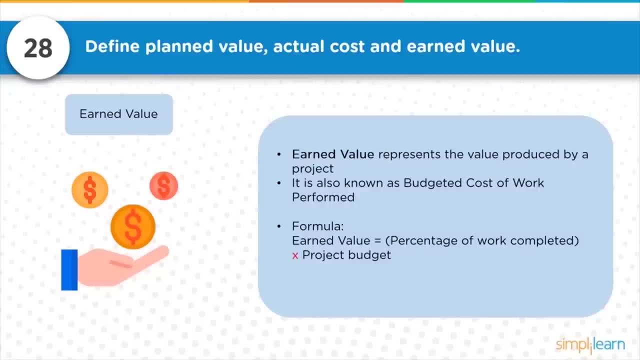 behind schedule. when I compare the earned value with the planned value, it will tell me whether I'm behind schedule, ahead of schedule or according to the plan. now for this earned value of 1,800, if I incur the actual cost of 1,800, then 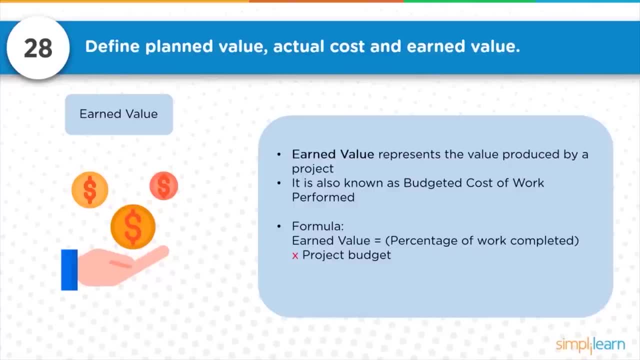 cost wise, I'm doing good. if my actual cost is lesser than earned value, then cost wise, I'm very good, right. if I incur more than earned value, for example, to complete the work worth of 1,800, I incur the cost of 2,000, then I'm not. 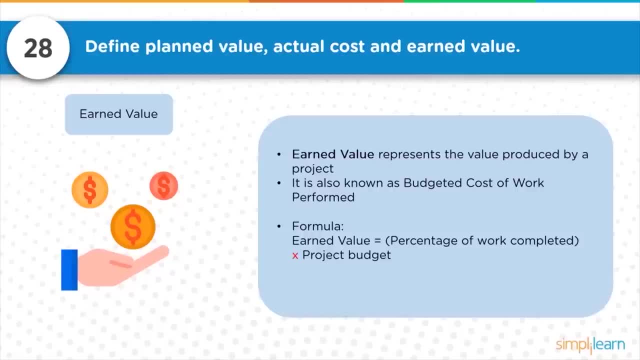 doing good. I'm over budget. so the combination of earned value and planned value helps us to know the schedule perspective of the project is behind or ahead, or according to the plan schedule perspective, whereas the combination of earned value and actual cost helps us to understand whether project is within the 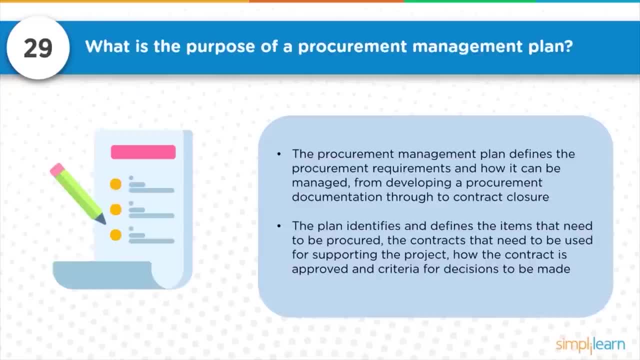 budget over budget or according to the plan? question number 29: what is the purpose of procurement management plan? the procurement management plan defines the procurement requirements and how it can be managed, from developing a procurement documentation through to contract closure. the plan identifies and defines the items that need to be. 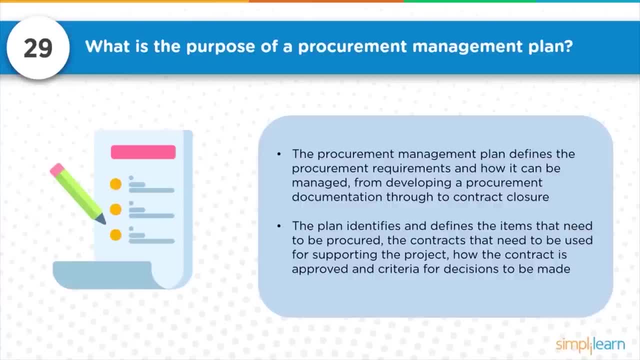 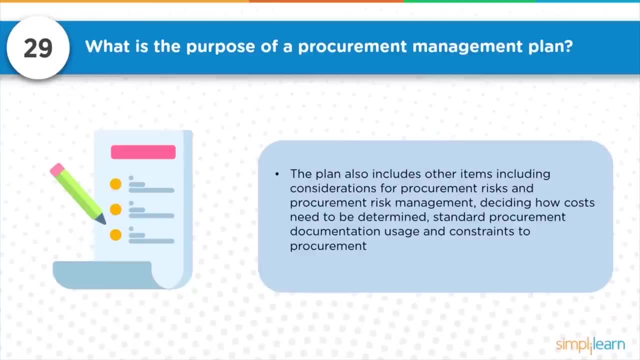 procured, the contracts that need to be used for supporting the project, how the contract is approved and criteria for decisions to be made has to be looked at. the plan also includes other items, including considerations for procurement risks and procurement risk management, deciding how cost needs to be determined, standard requirements and 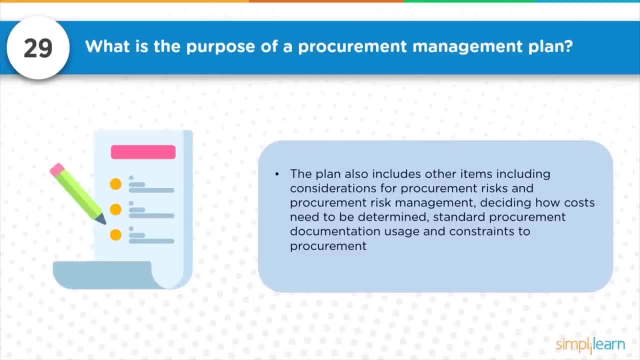 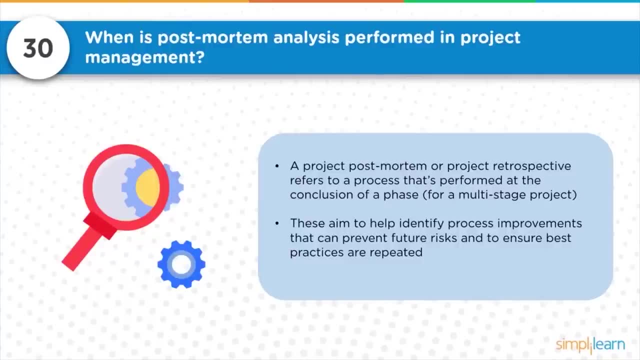 procurement documentation usage and constraints to procurement. question number 30: when is post-mortem analysis performed in the project management? a post-mortem in a project or project retrospective refers to process that's performed at the conclusion of the phase for a multi-stage project. this aim to 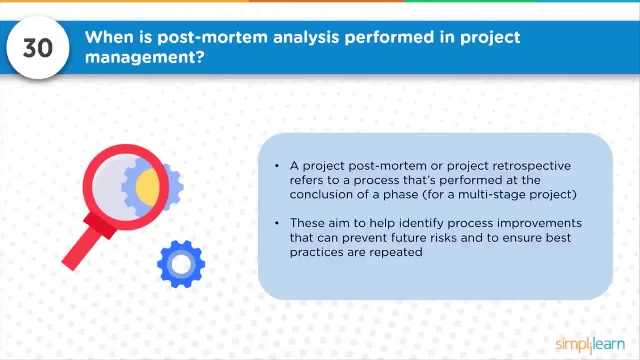 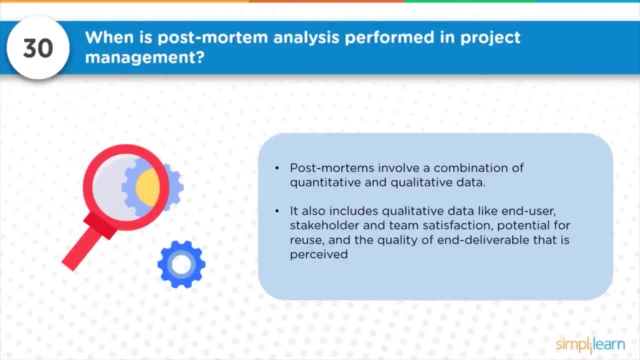 help identify process improvements that can prevent future risks and to ensure best practices are repeated. post martin's involve a combination of quantitative and qualitative data. it also includes qualitative data like end user, stakeholder and team satisfaction, potential for reuse and the quality of end deliverable that is perceived. 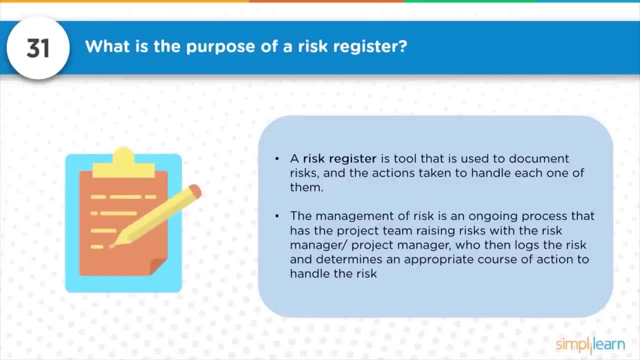 question number 31: what is the purpose of risk register? the risk register is basically a tool that is used to document risks and the actions to handle each of those risks. the management of risk is an ongoing process of risk is an ongoing process that has a project team raising risks with the 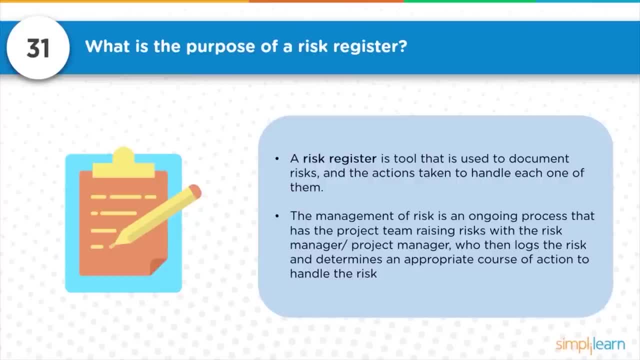 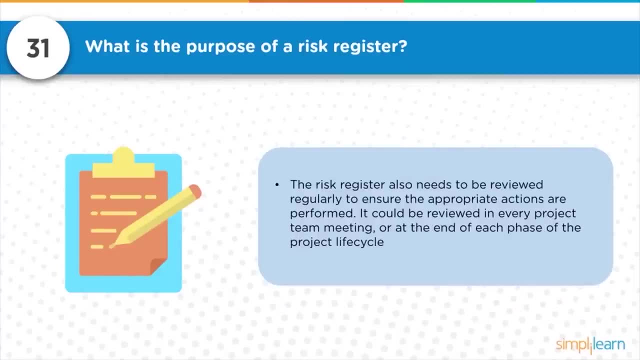 risk manager or a project manager, who then locks the risks and determines an appropriate course of action to handle the risk. the risk register also needs to be reviewed regularly to ensure the appropriate actions are performed. it could be reviewed in every project team meeting or at the end of each phase of. 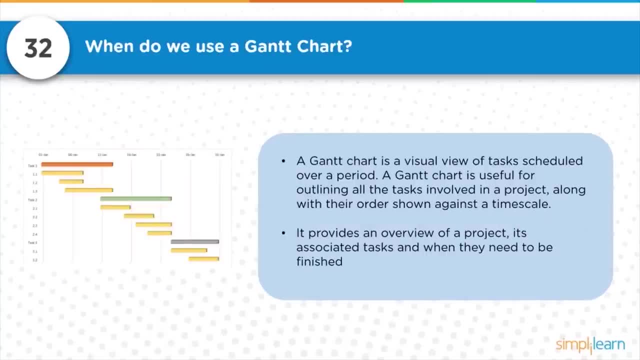 the project lifecycle. question number 32: when do we use a Gantt chart? so, as we are discussing about critical planning, paths, network diagram, critical path method, so by using the project tools, we first establish a Gantt chart. so Gantt chart is basically a visual view of 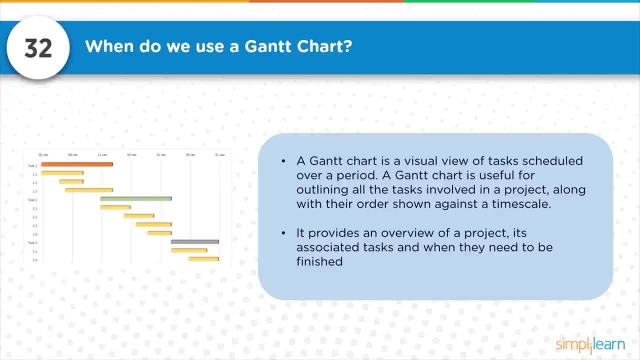 tasks scheduled over a period. a Gantt chart is useful for outlining all the tasks involved in the project, along with their order shown against the time scales. so, since it gives the pictorial representation, it helps us in understanding what tasks will be completed, after which tasks, and how the 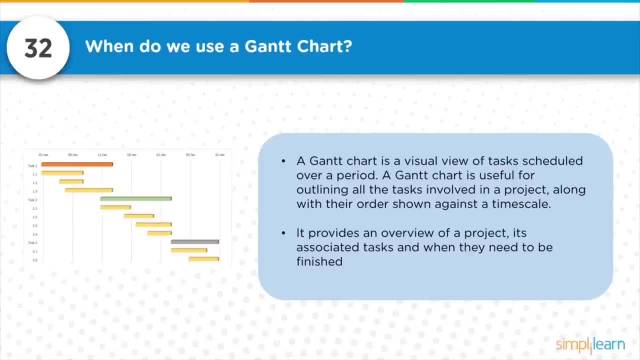 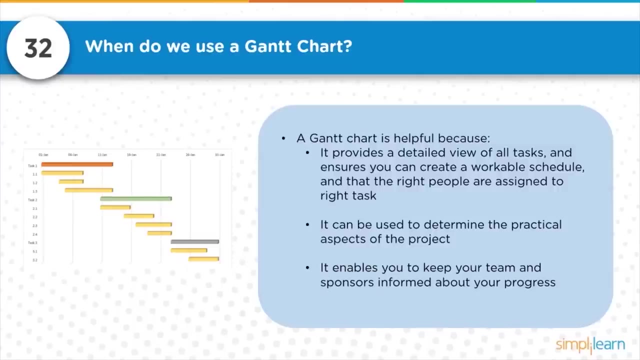 dependencies of each task will be can be easily understood. it provides an overview of a project. its associated tasks and then when they need to be finished are clearly understood. a Gantt chart is helpful because it provides a detailed view of all tasks and ensures one can create a workable schedule and 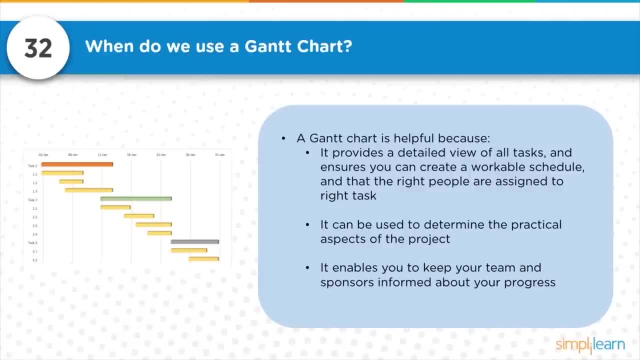 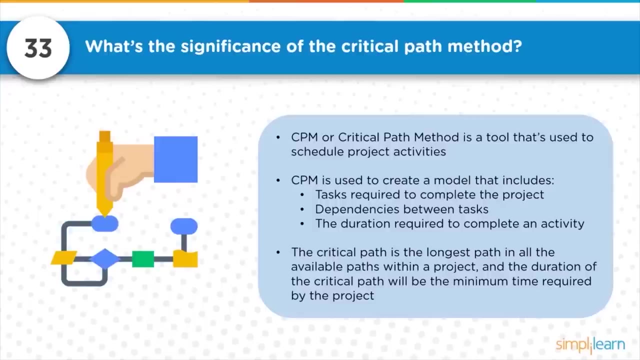 the right people are assigned to right tasks. it can be used to determine the practical aspect of the project. it enables to keep the team and sponsors informed about the progress of the project. question number 33: what is the significance of the critical path method? so critical path method, or CPM, is. 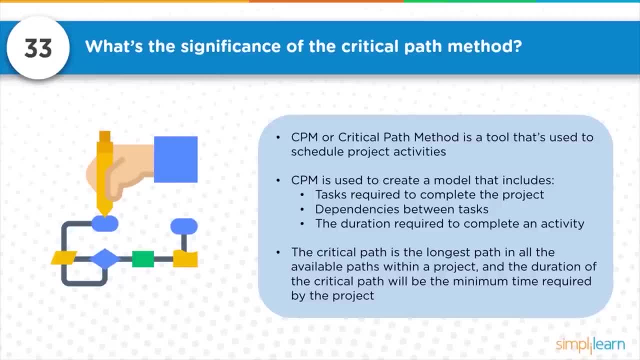 a tool that is used to schedule project activities. so CPM is used to create a model that includes tasks required to complete the project, dependencies between the tasks, the durations required to complete an activity. the critical path is the longest path in all the available paths in the project and the 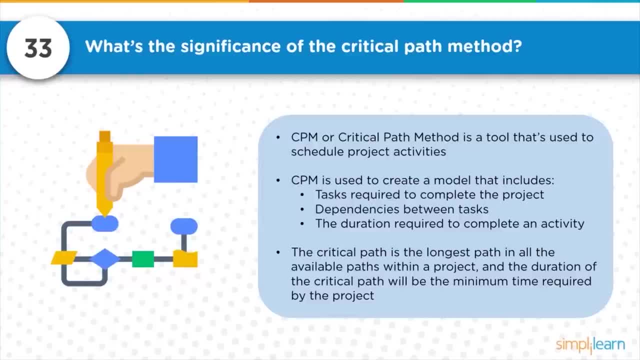 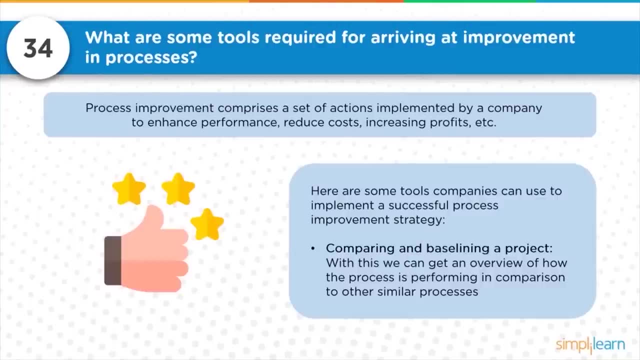 duration of the critical path will be the minimum time required by the project. to complete question number 34. what are some tools required for arriving at improvement in processes? so process improvement comprises a set of actions implemented by a company to enhance performance, cost reduction, increasing profits, etc. so some of the 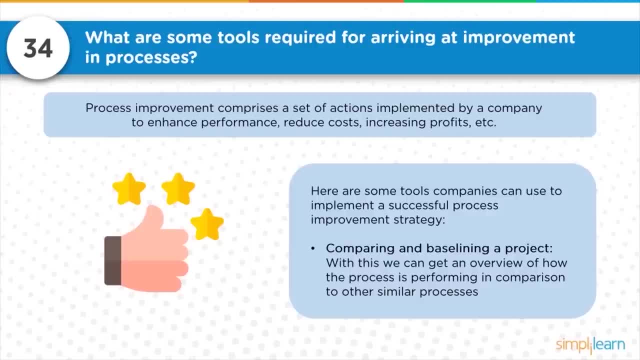 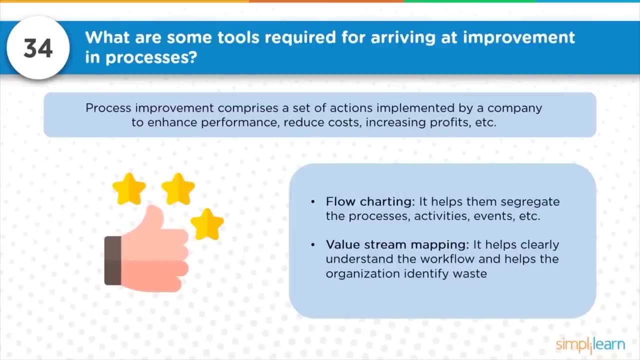 tools some organization can use to implement a successful process improvement strategy can be: comparing and baselining a project, so with this we can get an overview of how the process is performing in comparison with other similar processes. flow charting, which helps them segregating the processes. 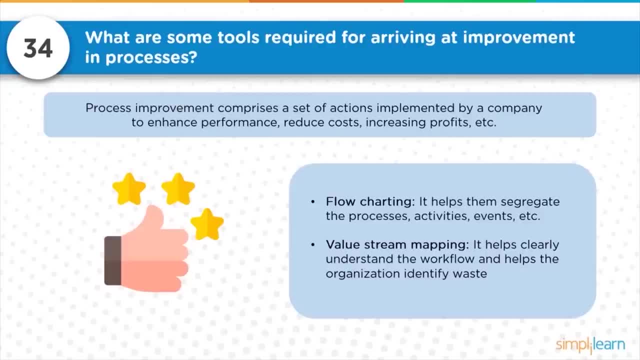 activities, events, etc. value stream mapping: it helps clearly understand the workflow and helps organizations identify waste. cause and effect analysis: these help organizations determine the root cause of any problem. hypothesis testing, which helps in testing to determine whether a hypothesis would be favorable to the organization or not. question 35. 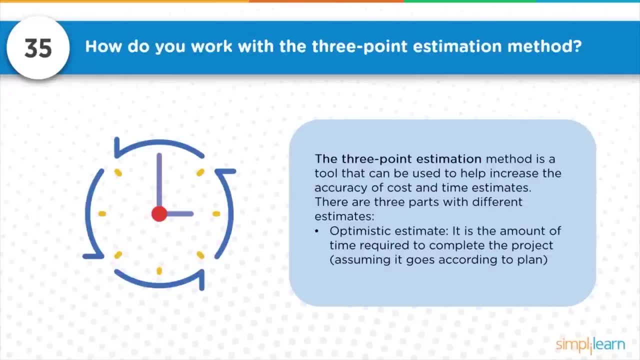 how do you work with three-point estimation method? so the three-point estimation method is also called as pert estimation, which is a tool that can be used to help increase the accuracy of cost and time estimates. there are three parts with the different estimates: that is optimistic, pessimistic and most. 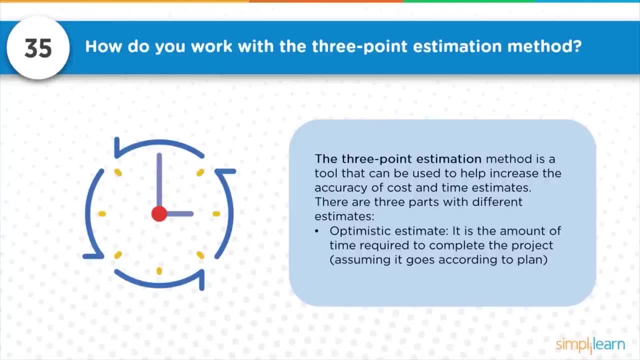 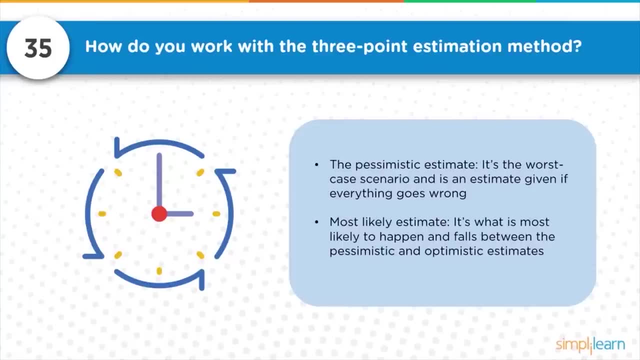 likely. the optimistic estimate is the amount of time required to complete the project, assuming everything in the project goes according to the plan. according to the plan, pessimistic estimation is estimation considering the worst-case scenario and is an estimation given in everything goes wrong. that is the assumption, so most 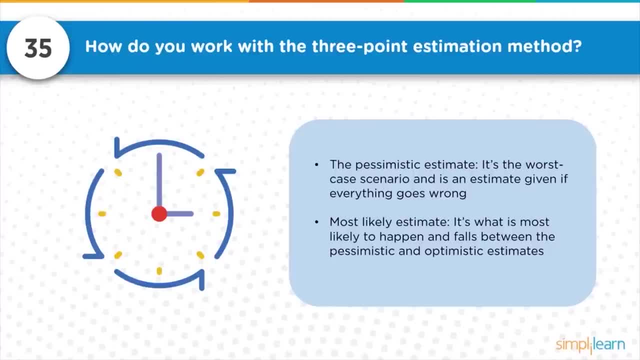 likely estimation. so this is most likely to happen and falls under the pessimistic and optimistic estimates. it falls in between that pessimistic and optimistic. so the formula to calculate three-point estimate would be: pessimistic plus optimistic plus four, most likely divided by six, will provide the three-point estimation. what 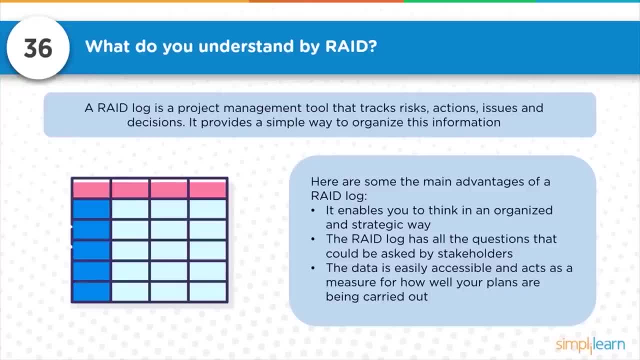 do you understand by the term raid? raid log is a project management tool that tracks risks, actions, issues and decisions. it provides a simple way to organize the information. so the main advantages of raid log is to enable you to think in the organized and strategic way. the raid log has all the questions. 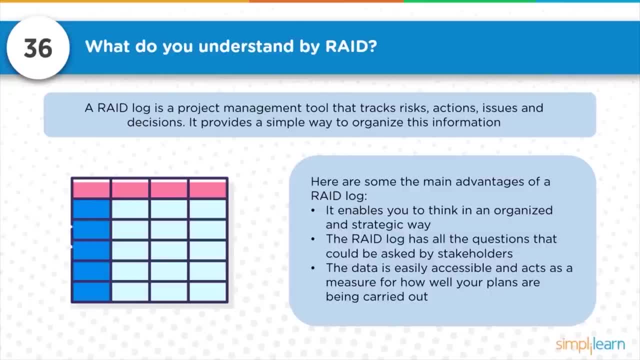 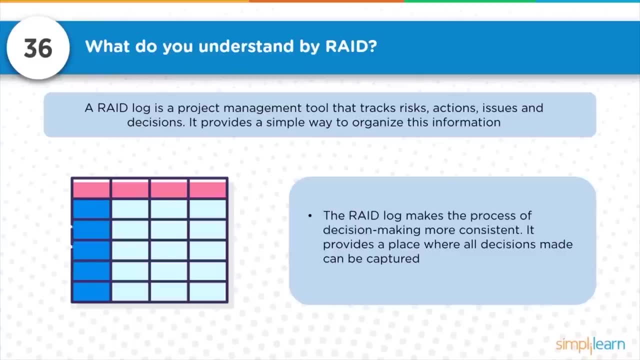 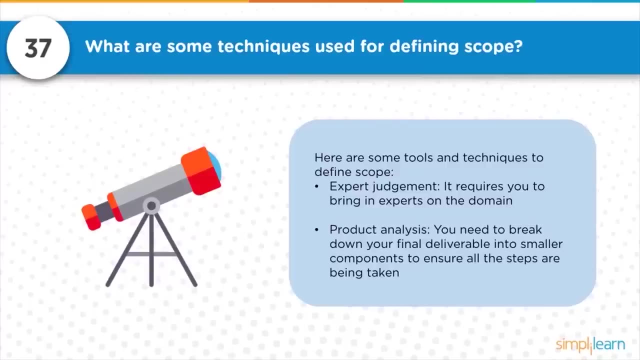 that could be asked by stakeholders. the data is easily accessible and accessible and acts as a measure for how well the plans are being carried out. the raid logs makes the process of decision making more consistent. it provides a place where all decisions made can be compared. question number 37: what are 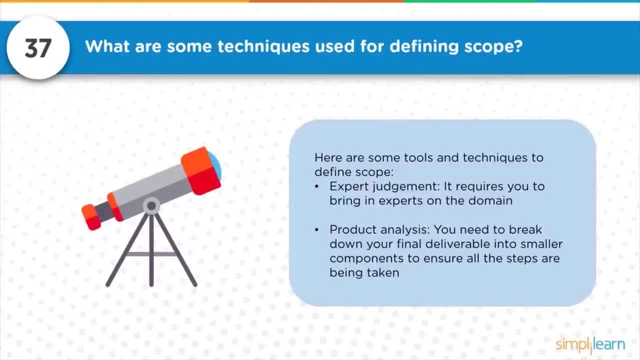 some techniques used for defining scope. so here are some tools and techniques to define scope. that is, expert judgment, it which requires to bring in experts on domain. product analysis, which needs to break down the final deliverability into smaller components to ensure all the steps are being taken. alternative: 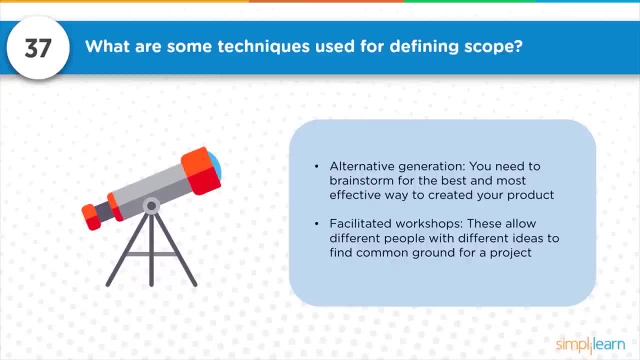 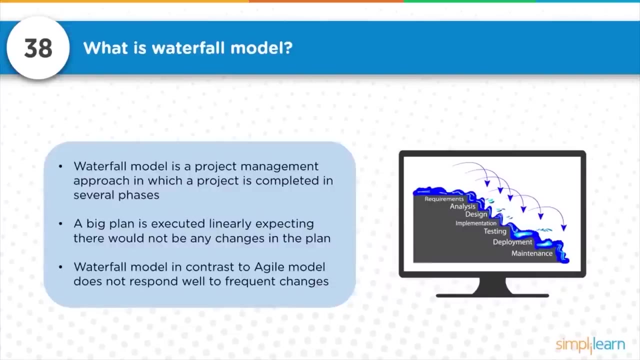 generation, so in alternative generation, it's need to brainstorm for the best and most effective way to create it for the product. facilitated workshops which allow different people with different ideas to find common ground for a project. question number 38: what is waterfall model? waterfall model is a. 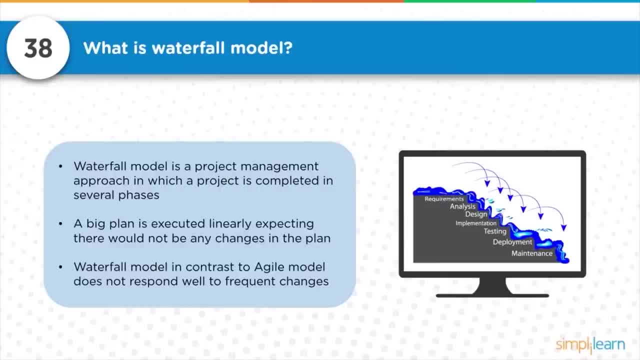 project management approach in which a project is completed in several phases, a big plan is executed linearly, expecting there would not be any changes in the plan. waterfall model is in contrast to a gel model. does not respond well to frequent changes, any changes which comes in between, while 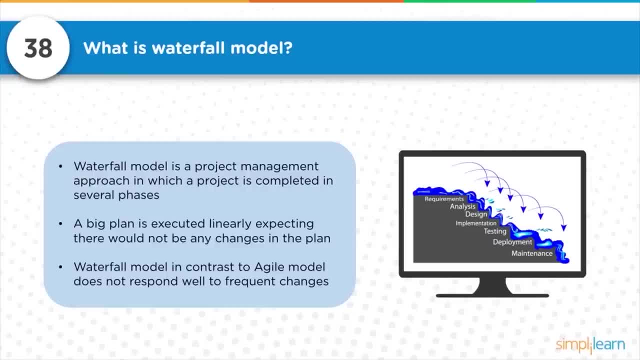 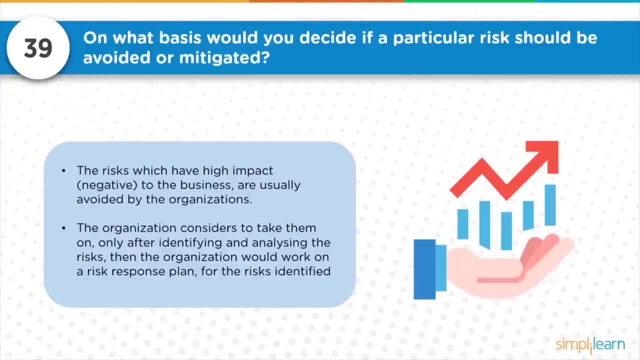 following the waterfall methodologies. making that changes will be difficult and bit complex. question 39: and what basis would you decide if a particular risk should be awarded or mitigated? the risks which are having high impact, negative to the business, are awarded by the organization's usually so. 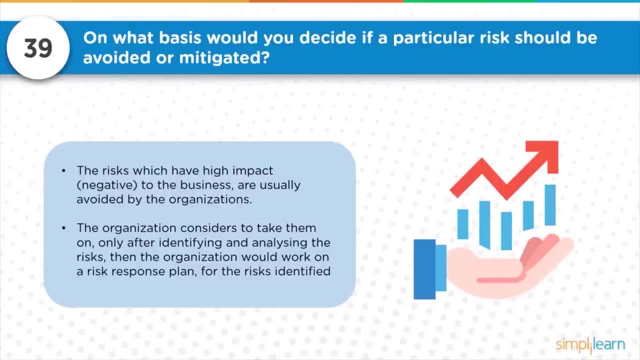 awarding is the first decision. what organization makes for sure? but, however, there may be some discussions which are made before the decision of being made relating to awarding that risk, instead having some workaround for that risk or making certain arrangement so that impact of the risk can be reduced, or 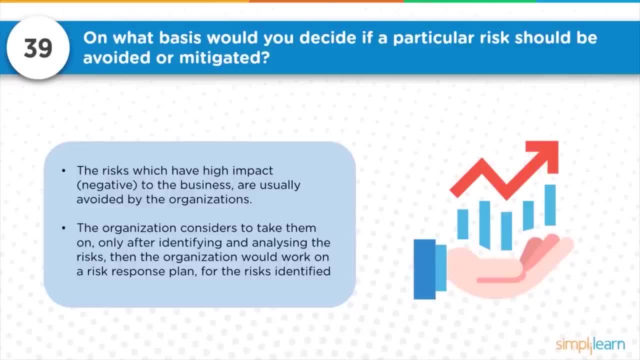 bringing down the probability of occurrence of the risks, considering something which will have higher negative impact. they may not be worthwhile to take up, so it's important in that case. I think awarding is the best decision once the organization is considered to take up after identifying and analyzing the risks. 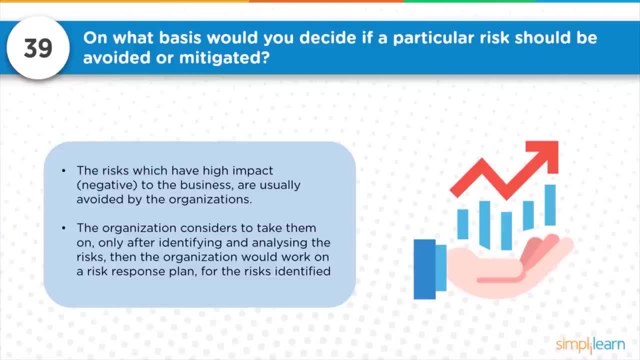 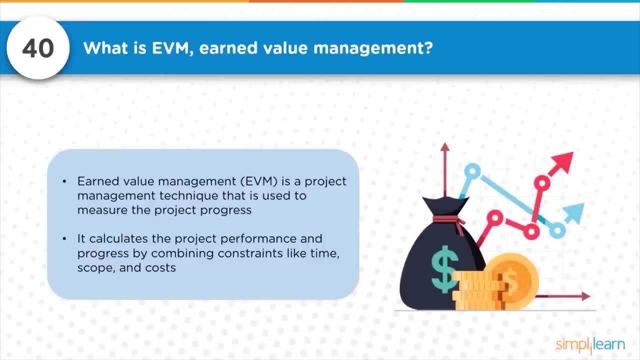 then organization would work on risk response plan for all the risks which are identified. so what is EVM? the earned value management? so, earned value management, it is a project management technique that is used to measure the project progress, if you recall the terminologies like earned value planned. 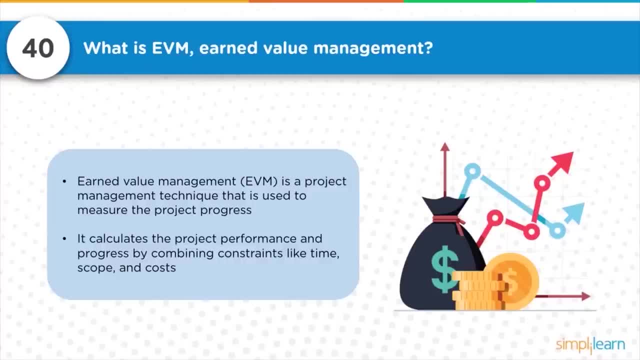 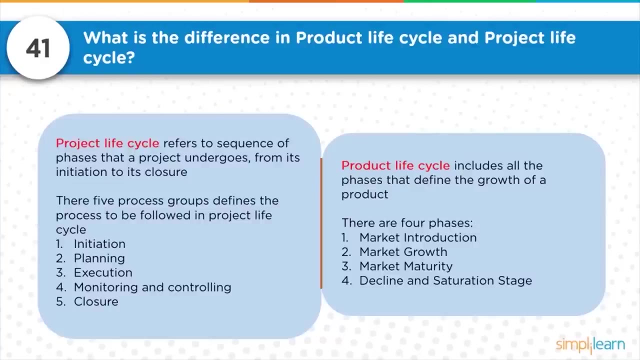 value. actual cost schedule. performance index, cost performance index, cost performance index- these are the terminologies which comes as part of earned value management. it calculates the project performance and progress by combining constraints like time, scope and costs. so question 41: what is the difference in product lifecycle and 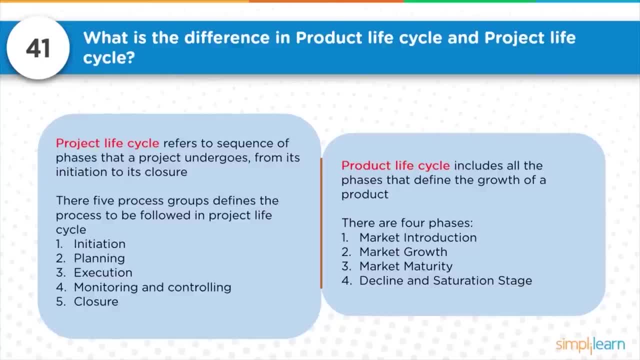 project lifecycle. so project lifecycle refers to the sequence of stages or phases the project undergoes from the time it is initiated till it is closed. so this project lifecycle is the process of the project. so project lifecycle involves five process groups, which is initiating process, group planning process, group executing process. 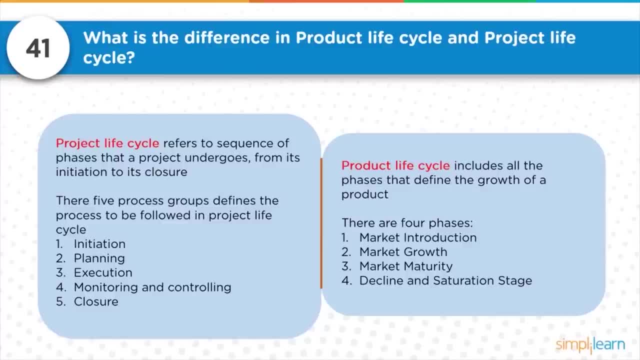 group, monitoring and controlling process group, closure, process group, which should be there throughout the project lifecycle, along with the 10 knowledge areas and 49 processes. product lifecycle includes all that, phases that define the growth of a product. so creation of the product till expiry of the product. so 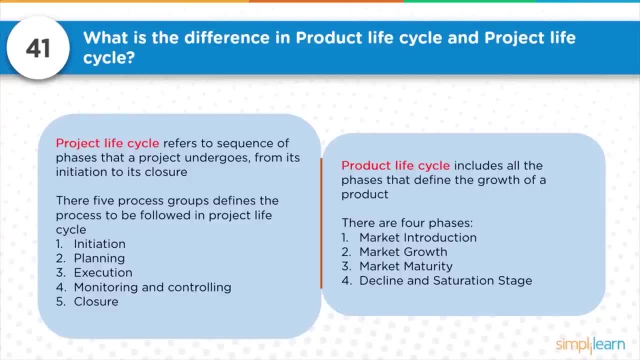 within the product lifecycle we may have multiple project life cycles. so one project lifecycle for introduction of product, one project lifecycle for modifying or updating the existing product. one project lifecycle may be for improvement. one project lifecycle may be for removing the product from the production. so in product lifecycle there 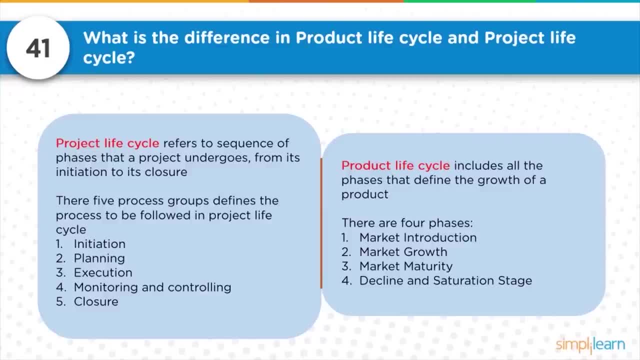 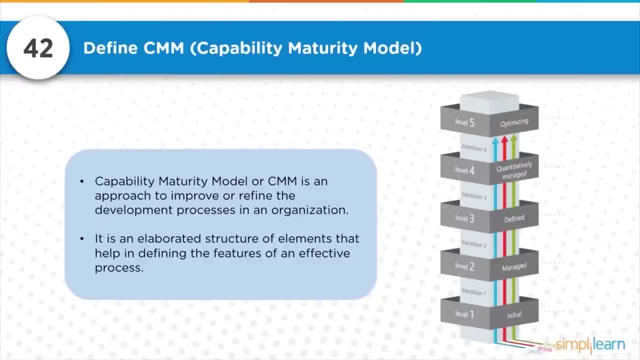 are four phases, that is, market introduction, market growth, market maturity and decline and saturation stage. question 42 define capability maturity model. so capability maturity model is an approach to improving or refine development process in an organization. so it is an elaborated structure of elements that helps in. 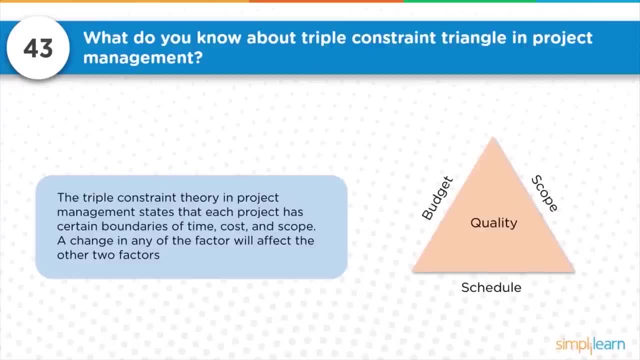 defining the features of an effective process. next, question 43: what do you know about triple constraint, the triangle, in project management? so basically, the triple constraint refers to scope, schedule and cost. right, so it helps in actually analyzing the project status, the way project is progressing, and these are the three critical. 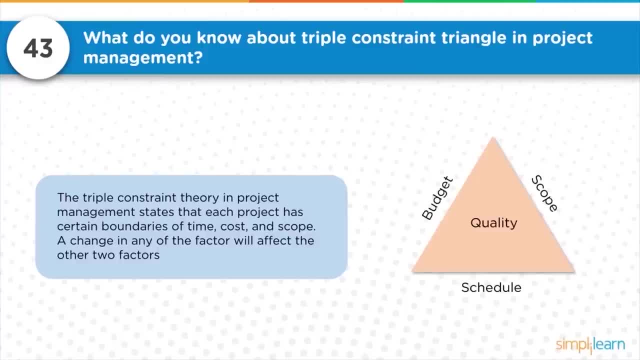 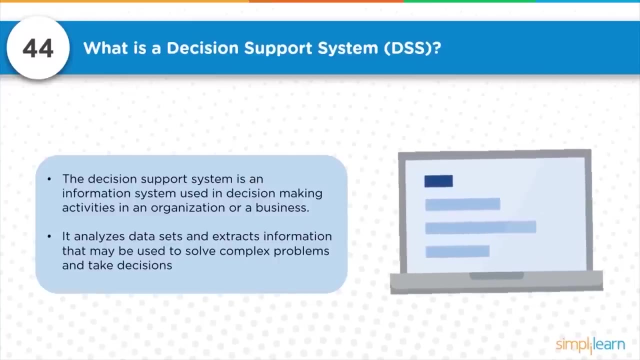 considerations mainly which needs to be made. so, further to these triple constraints, scope, time and cost, quality, resource and risks are also considered as a constraints. so any change in any of the constraints would have an impact on other constraints. question 44: what is a decision support system? decision support. 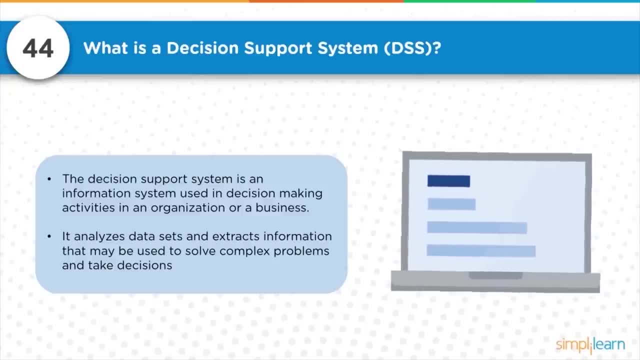 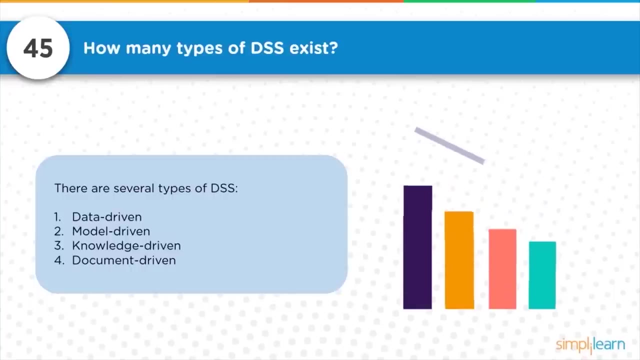 system is an information system used in decision-making activities in organization or business. it analyzes data, sets and extracts information that may be used to solve complex problems and take decisions. how many types of DSS are there? so there are several types of DSS, that is, data driven. 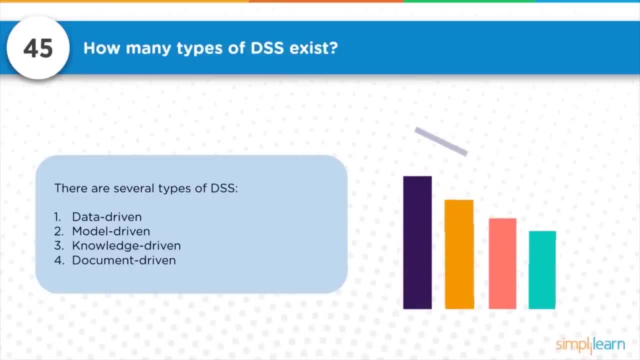 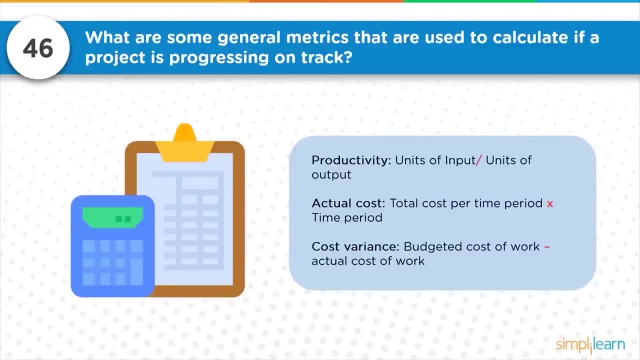 model driven, knowledge driven and document driven. question 46: what are some general metrics that are used to calculate if a project is progressing on track? so, if a project is progressing on track, it is very essential to consider the productivity, which means units of input, units of output, actual cost, that 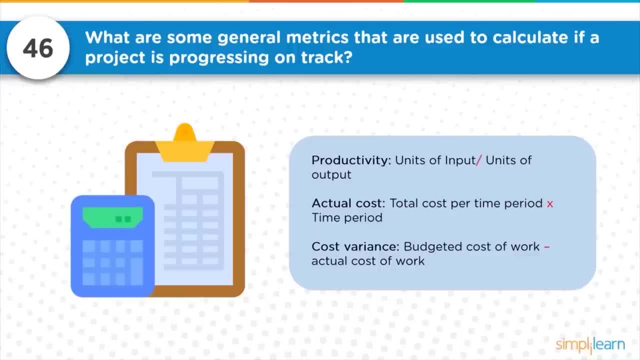 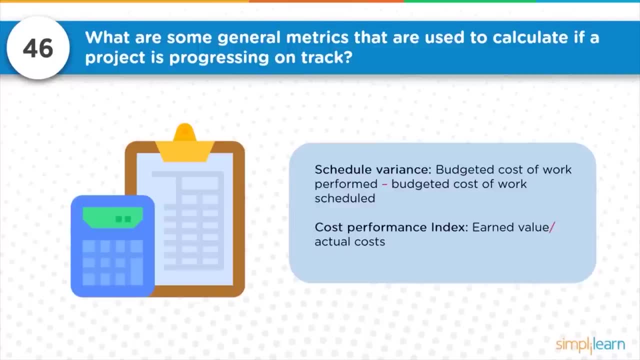 is total cost per time period to time period. cost variance, which refers to budgeted cost of work versus actual cost of work. schedule variance, which is the difference between budgeted cost of work perform and budget cost of work. scheduled cost performance index, which is earned value to actual cost. question 47: what is? 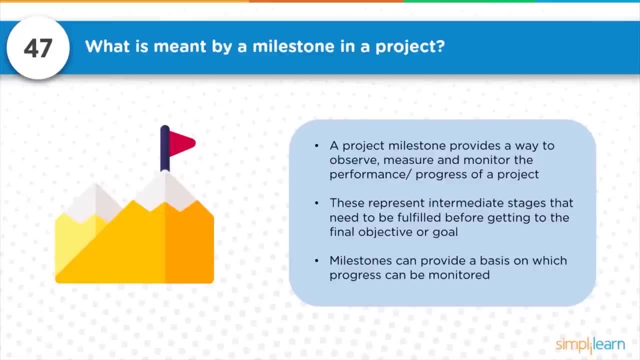 meant by a milestone in a project. a project milestone provides a way to observe, measure and monitor the performance progress of the project. these represents intermediate stages that needs to be fulfilled before getting to the final objective or goal. milestones can provide a basis on which progress can be monitored. they can also 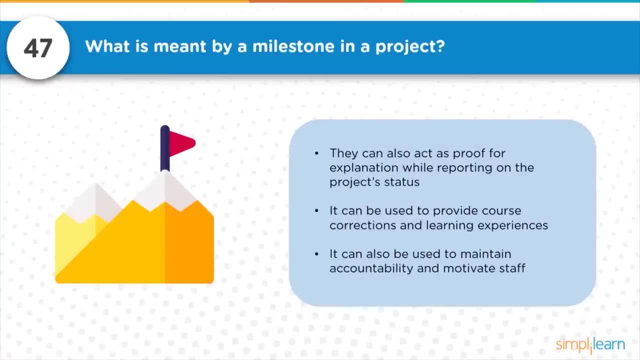 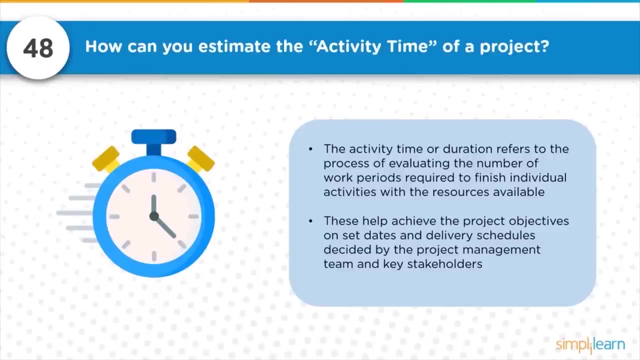 prove for explanation while reporting on project status. it can be used to provide course corrections and learning experiences. it can also be used to maintain accountability and motivate staff. question 48: how can you estimate the activity time of a project? the activity time or duration refers to the process. 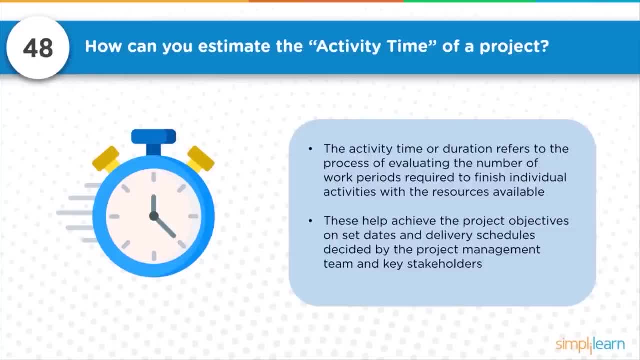 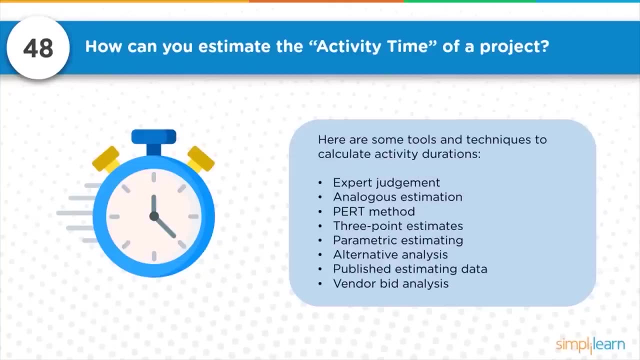 of evaluating the number of work periods required to finish individual activities with the resources available. these help achieve the project objectives on set dates and delivery schedules decided by project management team and key stakeholders. here are some tools and techniques to calculate activity durations. so those are expert judgment analogous. 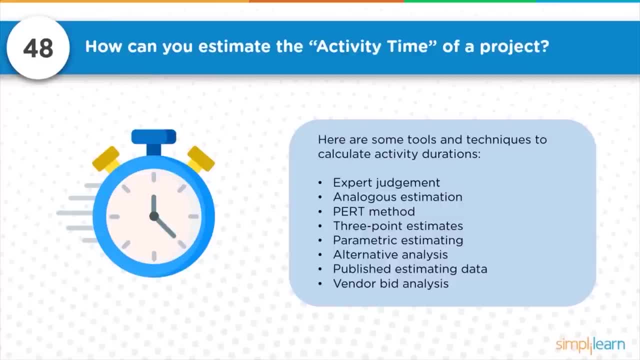 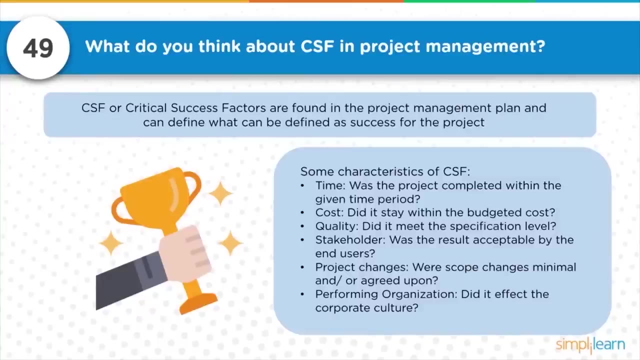 estimation, PERT method, three-point estimates, parametric estimating, alternative analysis, published estimating data, vendor bid analysis, etc. question 49: what do you think about CSF, critical success factor, in a project management? so CSF or critical success factor are found in the project management plan and can define what can. 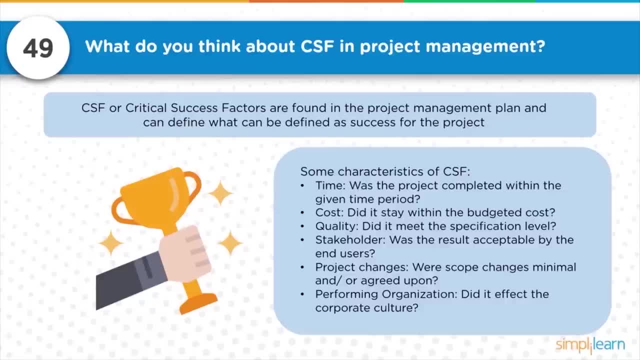 be defined as success for the project. some characteristics of critical success factor involved, for example, time: was the project completed within the given time period? cost: did it stay within the budgeted cost? quality: did it meet the specification level? stakeholder: was the result accepted by the end user project? 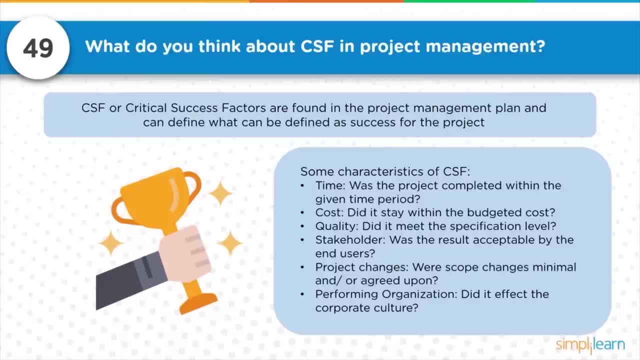 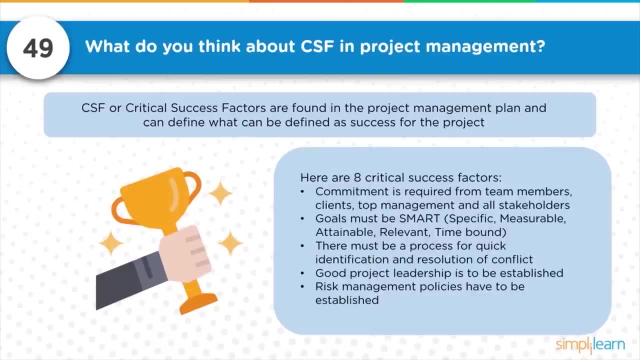 changes were scope. changes are minimal and are agreed upon performing organization. did it affect the corporate culture? commitment is required from team members, clients, top management and all stakeholders, which is very essential and it is one of the main critical success factors. goals must be specific, measurable, attainable. 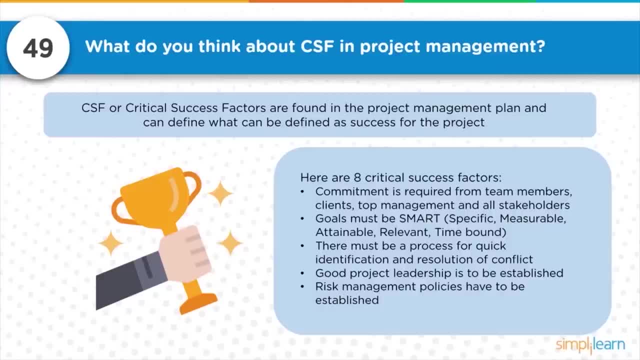 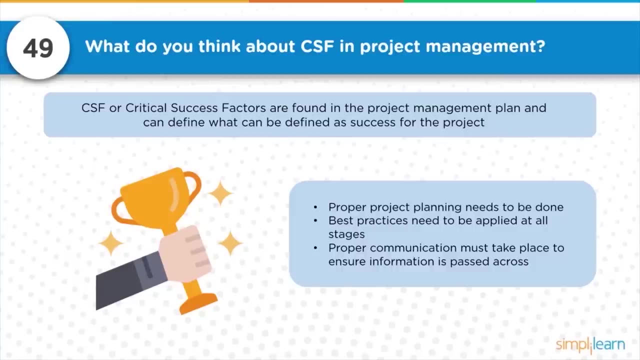 relevant and time bound. there must be process for quick identification, resolution of conflict. good project leadership is to be established. risk management policies have to be established. there must be proper project planning. that needs to be done. then best practices need to be applied at all stages. proper communications might take. 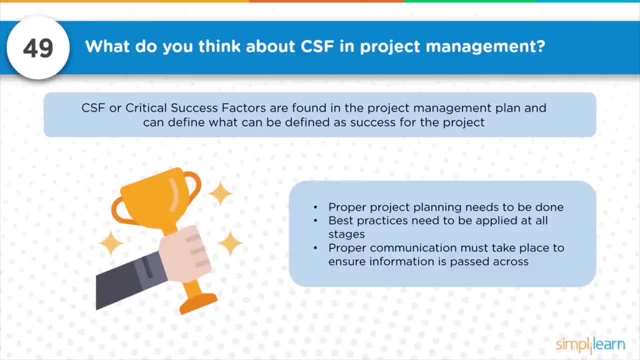 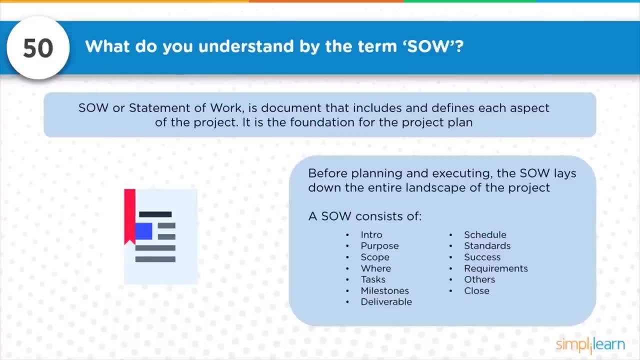 space to ensure information is passed across. question number 50: what do you understand by the term sow? so sow or statement of work is a document that includes and define each aspects of the project. it is a foundation for the project plan. so, before planning and executing, the sow lays down the entire. 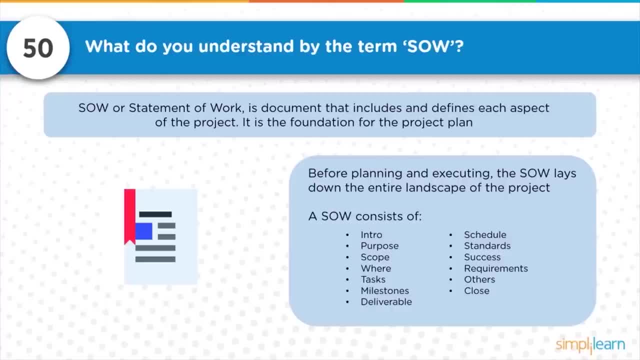 landscape of the project. so it consists of introduction, the purpose of the project, the scope of the project, the project when it is done, where it is done, the tasks, milestones, deliverables, schedule, standards, success: how are you going to determine the success means? how do you know the project is success? what 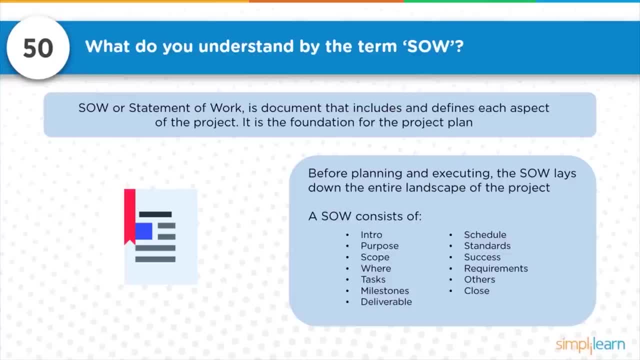 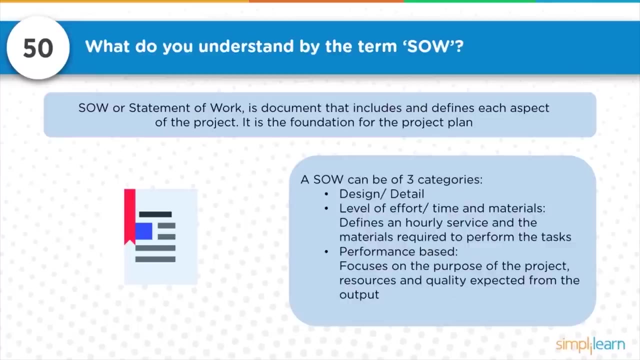 is that you're going to measure or consider for measurement requirements, then any other things which needs to be considered as part of a sow, as part of that specific project and then closing. so sow can be of three categories, which will have design details, level of effort, time and materials, which defines an 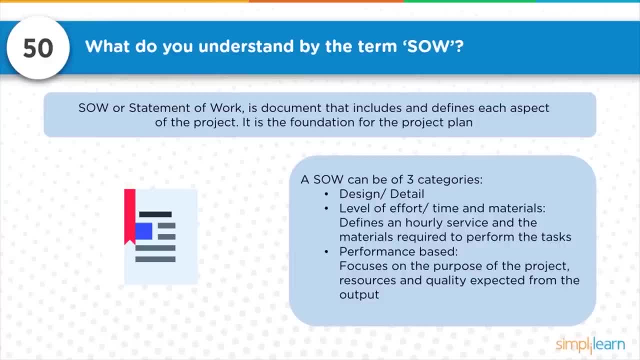 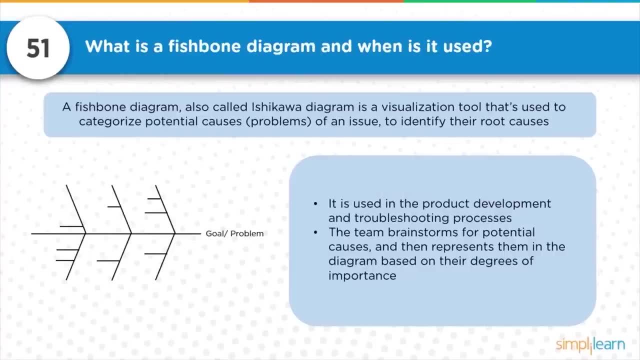 hourly service and the materials required to perform the tasks, which may be performance based. focuses on purpose of the project, resources and quality expected from the output. question 51: what is a fishbone diagram and when is it used? so fishbone diagram, which is also called as Ishikawa diagram, is a 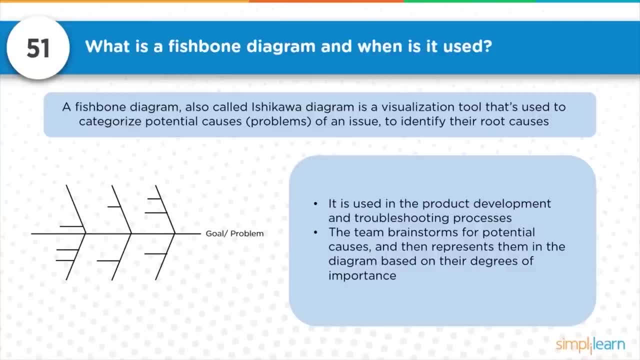 visualization tool that used to categorize potential causes. that is, problems for an issue, to identify the root causes. so fishbone diagram is used in product development and troubleshooting processes. it helps in team brainstorming for potential causes and then represents them in a diagram based on their degree of importance. so 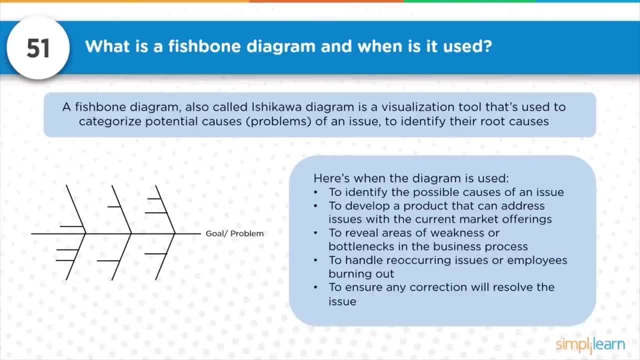 when this diagram is used, it helps us in identifying the possible causes of an issue. to develop a product that can address issue with current market offerings. to several areas of weakness or bottlenecks in the business process. to handle recurring issues or employees burnout to ensure any correction will. 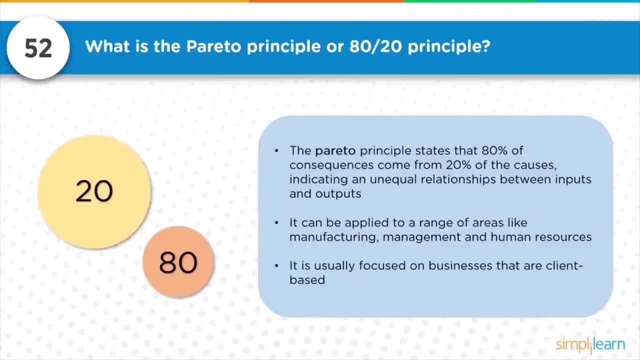 resolve the issue. so question 52: what is the Pareto principle or 80-20 principle? so, as the name itself indicates, the Pareto principle states that 80% of consequences come from 20% of causes, indicating an unequal relationship between inputs and outputs. it can be: 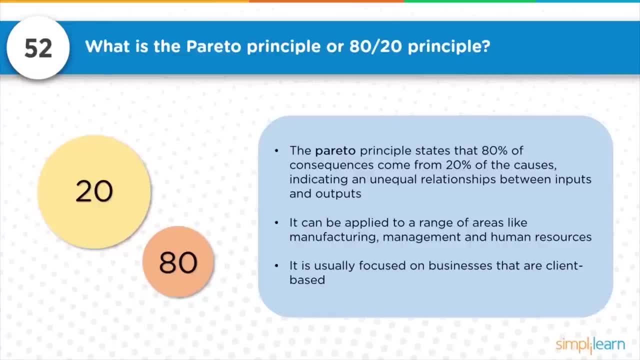 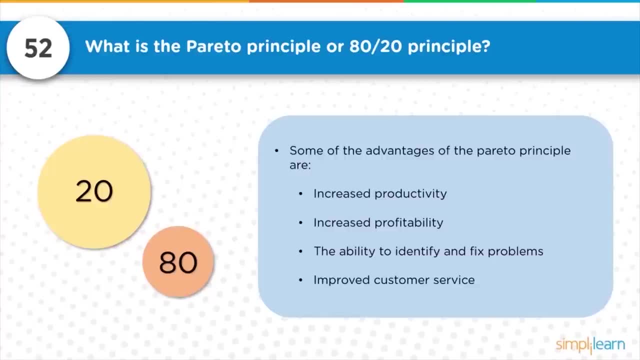 applied to range of areas like manufacturing, management and human resources. it is usually focused on businesses that are claim based. some of the advantages of Pareto principles are increased productivity, increased profitability, identifying and fixing problems and improved customer service. question 53: can you tell us about your? 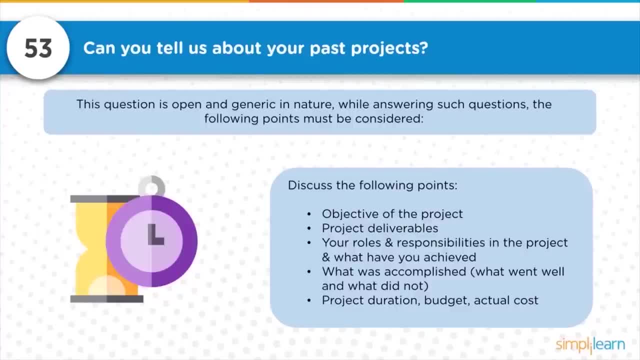 past project. so now, while answering these type of questions, firstly we need to understand this question is open and generic in nature. so while answering such questions, following points has to be considered. so: identify what is that project you have done so. state the objective of the project project. 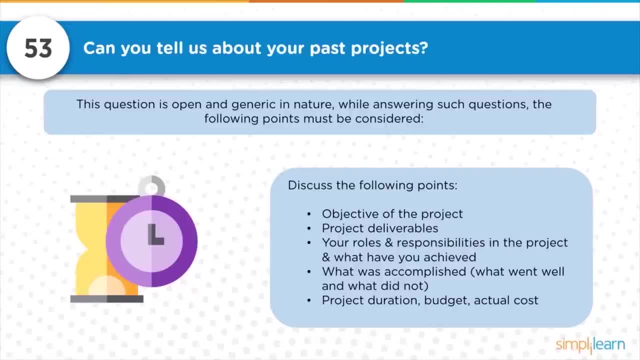 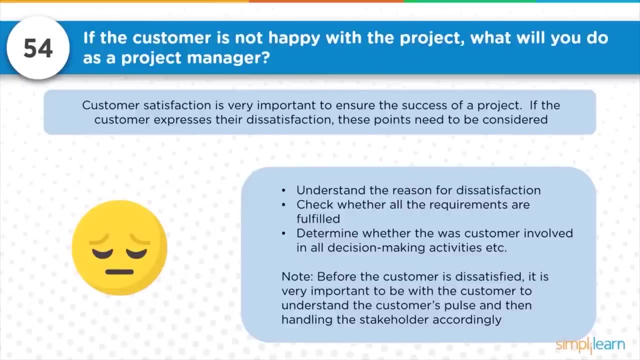 deliverables, your roles and responsibilities in the project and what have you achieved in that project? what was accomplished, what went well, what did not go well? then, project duration, project budget and actual cost incurred in the project. question 54: if customer is not happy with the project, what will you do? 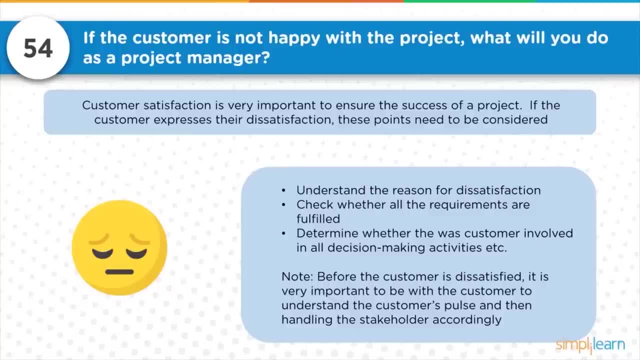 as a project manager. so in any given project, customer satisfaction is very important to ensure success of a project. in the scenario where customer expresses their dissatisfaction, one has to ensure understanding the reason for dissatisfaction. so are all the requirement fulfilled or not? project manager has to confirm that first was 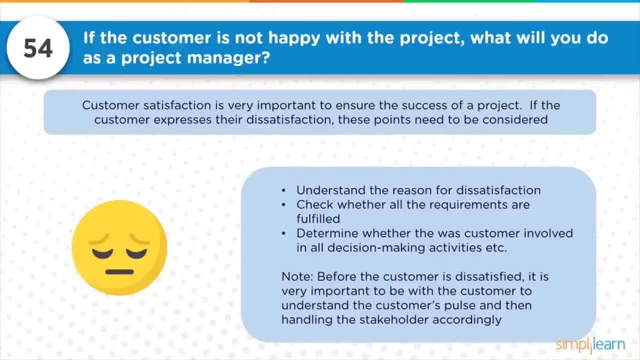 customer involved in all decision-making activities etc. to confirm that this customer is informed about everything. so before customer is dissatisfied, it is always good and important that customer is satisfied. that needs to be ensured. so it is very important to be customer to understand and customers pulse is. 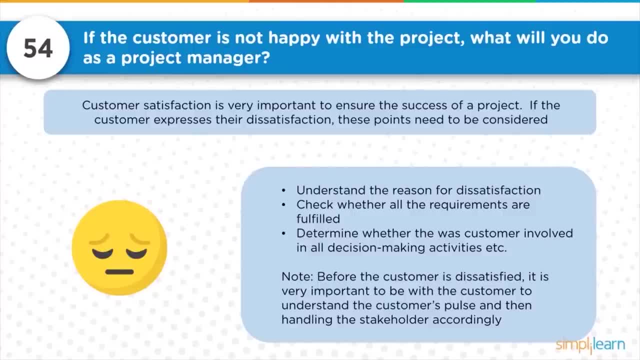 understood and handling the customer's accordingly. so allowing customer to become a dissatisfied customer is not a choice to have. so one needs to ensure customer is not at all dissatisfied in the first place, beyond your control. if customer is still dissatisfied, better you work on it to understand why the 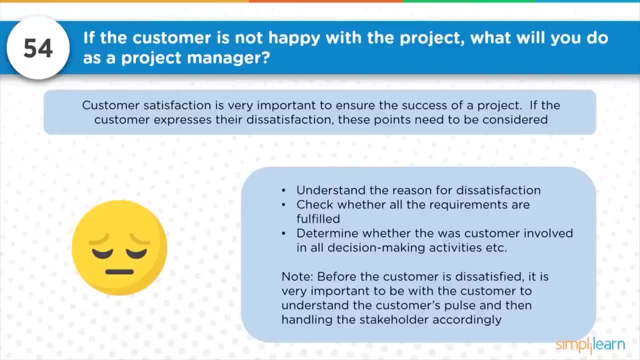 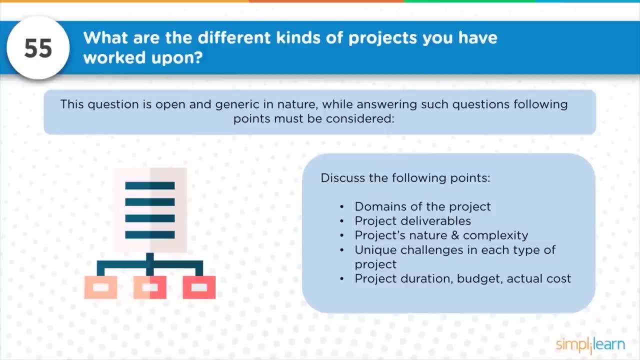 customer is dissatisfied, what is the cause of it and address it? question 55: what are the different kinds of project you have worked upon? so these type of questions are again generic in nature. while answering those questions, the questions, please ensure you speak about various different domains of the 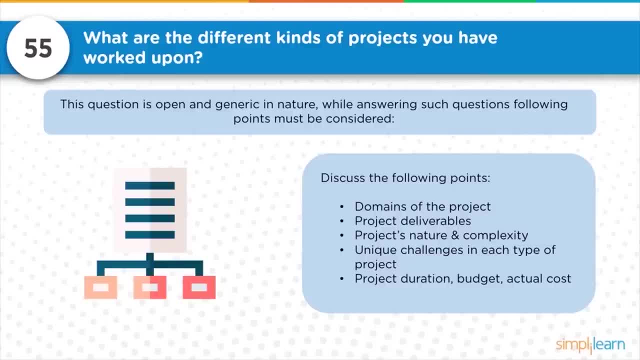 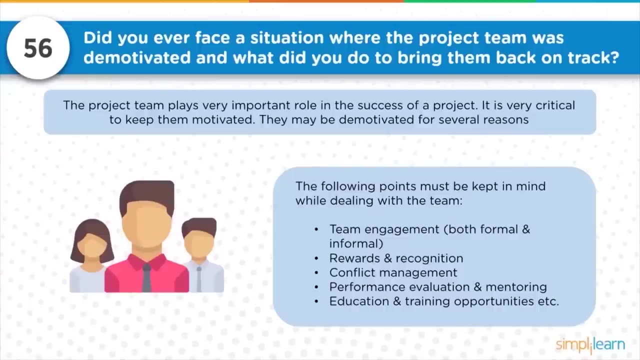 project which you have and that should have variation in different- I say different- domains of the project. what were the deliverables of those projects? projects nature and complexity, unique challenges in each different type of projects. then project duration, budget and actual cost. question 56: did you ever 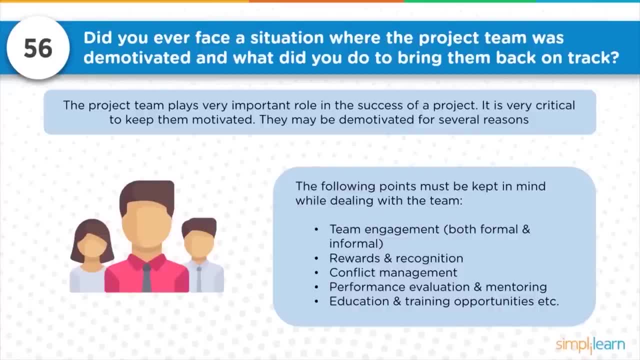 face the situations where the project team was demotivated, and what did you do to bring them back on track? so, as you know, project team plays very important role in success of any project. it is very critical to keep them motivated. the demotivation may happen for various 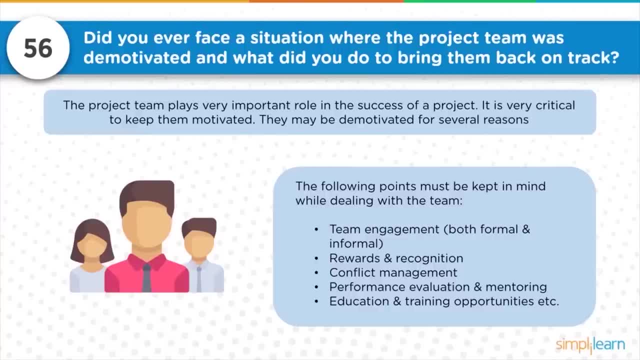 reasons. so one is to keep the following points in mind while dealing with the team. that is, team engagement. so engagement may be both formal and informal. so rewards and recognitions for the team for the good job they have done. conflict management wherever the conflict occurs. it is quite obvious. 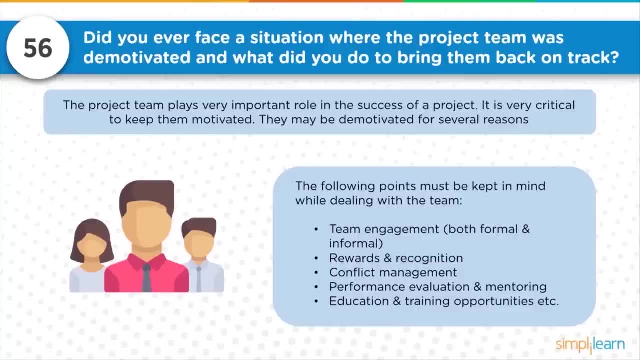 whenever the team is involved, conflict occurs, performance evaluation and monitoring. mentoring is very key. so wherever it is required to mentor, wherever it is required to give them a good perspective of the project and their learning and capability, so mentoring and coaching is very essential and also providing opportunities for 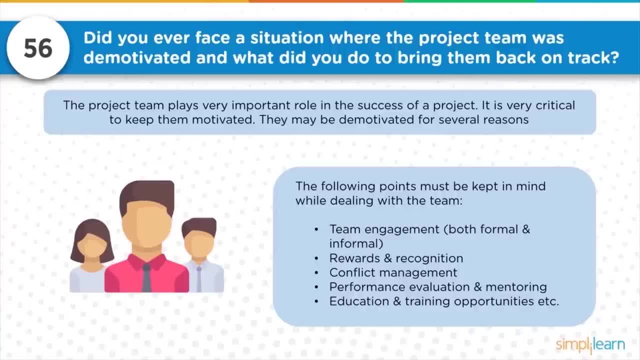 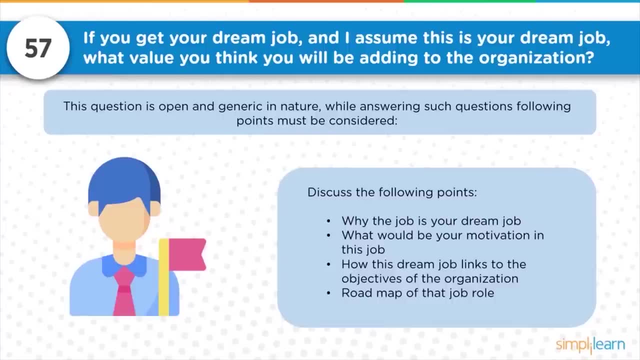 education and training so that they will have a better learning and accomplish or acquire the required skills. question 57: if you get your dream job- and I assume this is your dream job- what value you think you will you be adding to the organization? so this question is very. 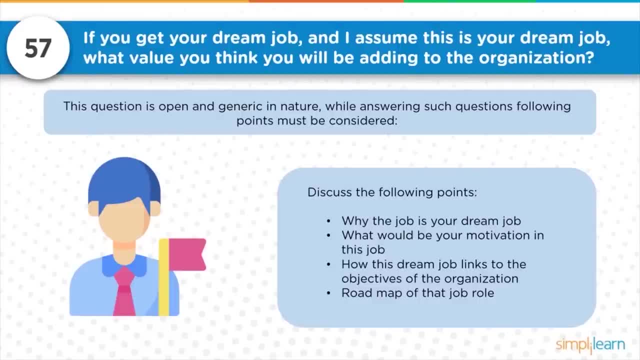 tricky one and also a generic question. so one is to ensure, while answering this question, to discuss the following points: why the job is your dream job. whatever the job you are speaking about, why do you say that that is your dream job? what is the reason why? what would be your? 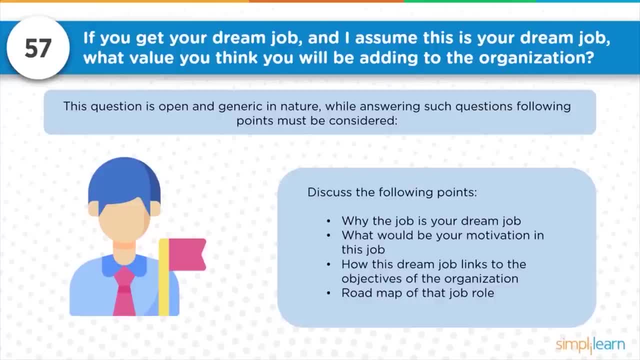 motivation point in this dream job. what exactly is motivating you there in this particular job? how this dream job can link to objectives of organization and the profession, and roadmap of the job role. so what is that you are going to become while you become this in future? what could be the roadmap of this role? 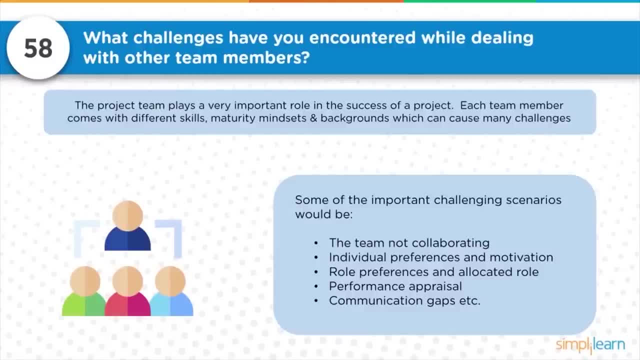 question 58: what challenges have you encountered while dealing with other team members? as already mentioned, project team plays very important role in success of a project. each team member comes with the different skills, maturity, mindsets and background which put across many challenges, such as some of the important changing scenarios. 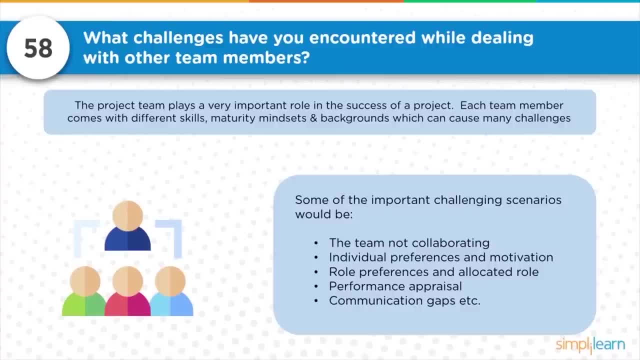 means challenging scenarios. is team not collaborating individuals, performance and motivation levels in each of the projects, role preferences and the allocated roles, performance appraisals, communication gaps, various things which actually brings the challenges and also motivates people to behave certain way they are behaving? question 59, share from 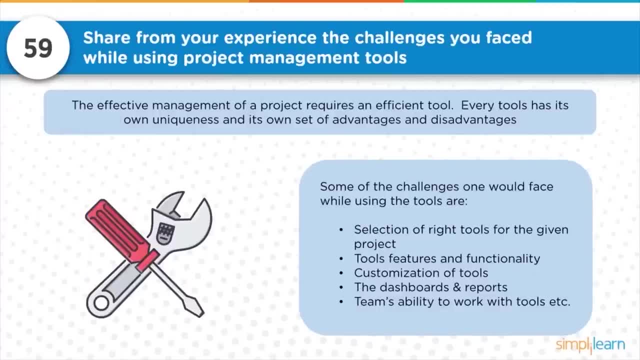 your experience, the challenges you faced while using project management management tools. so we all know that tools plays very important role in our management activity. similarly, the effective management of project requires an efficient tool. every tools has its own uniqueness and has its own advantages and disadvantages. so some of 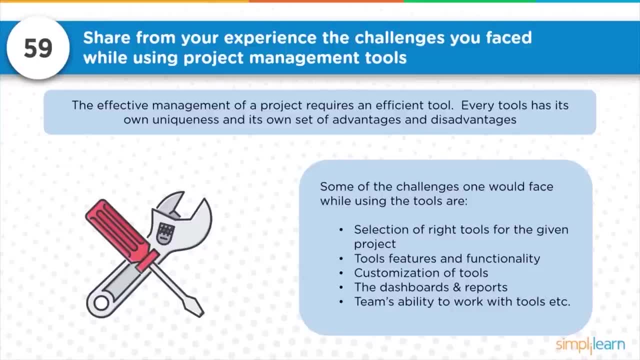 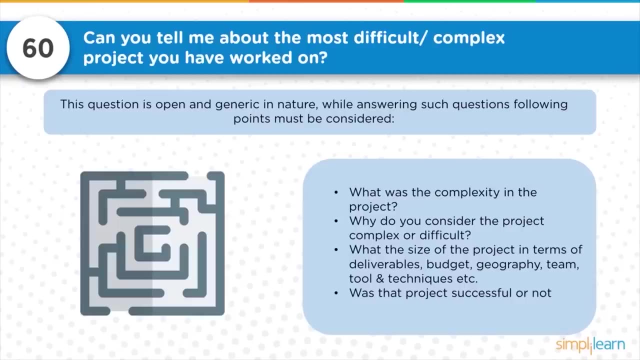 the challenges one would face while using the tools would be: selection of right tools for the given project. tools features and functionalities. customization of tools, the dashboards and reports. teams ability to work with tool. their skills and capabilities matters. question 60: can you tell me about the most difficult, complex? 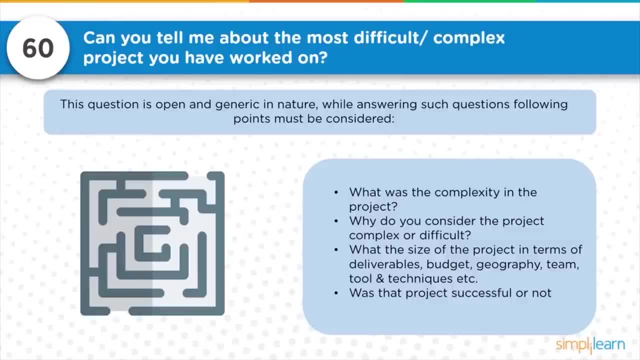 project you have worked on. this question is open and generic in nature. again, while answering such questions, please ensure to discuss the following points. what was the complexity in the project? whichever the project reference you are taking, why do you consider that project as a complex or difficult? what was the 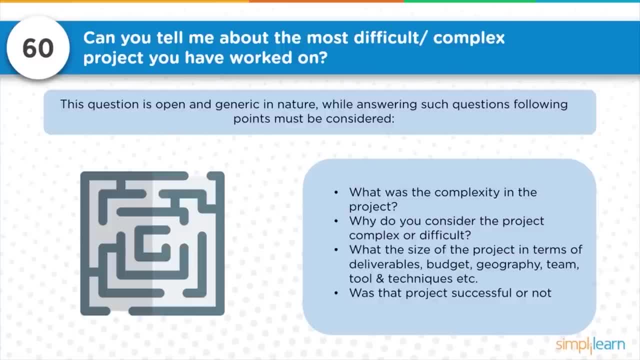 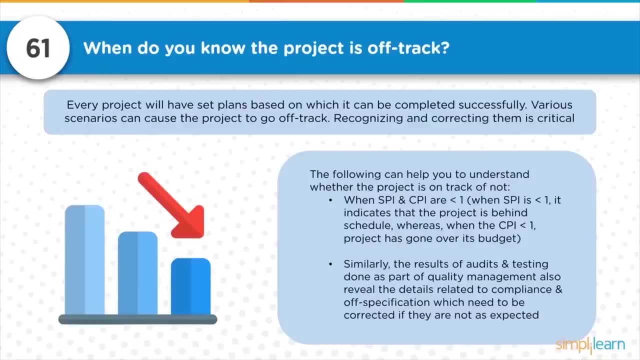 size of the project in terms of deliverables, budget, geography, team tools and techniques, etc. was the project successful or not? and why question 61? when do you know the project is off-track? so it is very essential for every project manager to ensure project is going as per the plan. so there should. 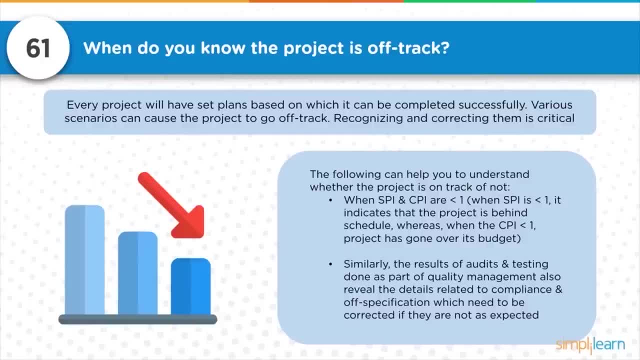 not be any deviations from the actual plan. so every project will have a set plans based on which project have to be completed successfully. due to various different scenarios, project go off-track. recognizing and correcting those is very critical and crucial. so one needs to follow a specific approach and then 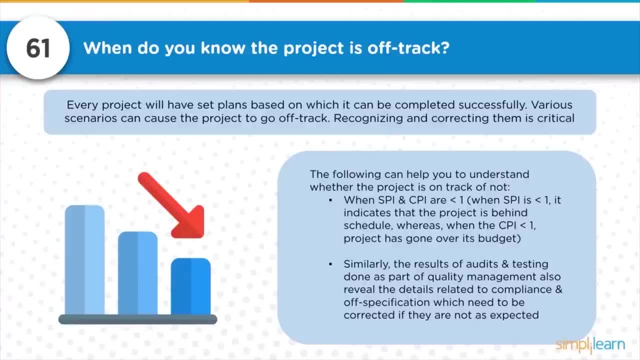 specific approach to ensure project will not go off track. so, but we need to understand whether project is going off track or not. so one of the key thing which we need to know is SPI and CPI. so SPI is the schedule performance index, the CPI the cost performance index. so when? 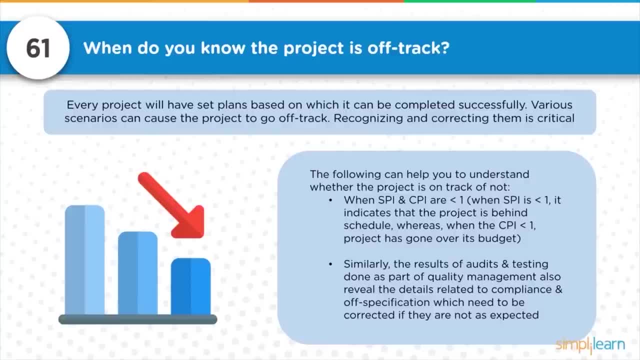 SPI is lesser than 1, which means project is behind schedule. when SPI is 1, then it's as per the schedule if SPI is greater than 1, which means project is ahead of schedule. similarly for CPI, if CPI is lesser than 1, project is over. 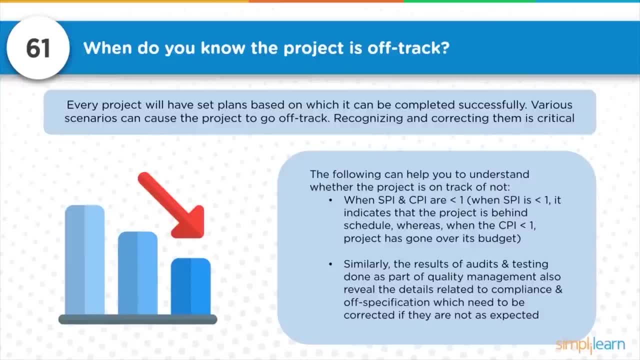 budget CPI is more than 1 project is under budget. if CPI is 1 project, budget is as per the plan. so, similarly, the results of audits and testing done as part of quality management also reveals the details related to compliance and of specifications which needs to be. 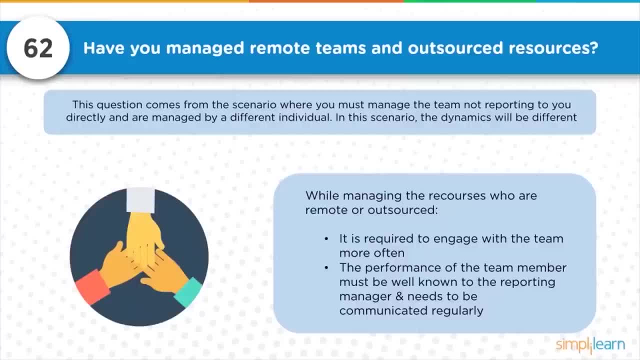 corrected if they are not expected. next question: have you managed remote teams and outsource resources? so these questions come from the scenario where you have to manage the team, not reporting to you directly, and they are managed by different individuals. while having such resources, the dynamics will be different. so, while 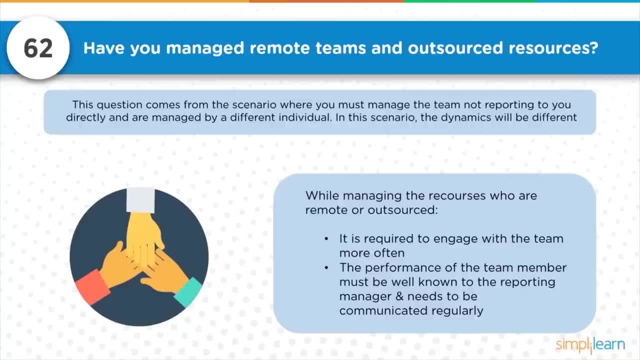 managing such resources, one has to ensure the engaging with them is different than the way the individuals are engaged- the internal teams. so it is required to engage with that team more often. the performance of the team members has to be well known to the reporting manager and that needs to be. 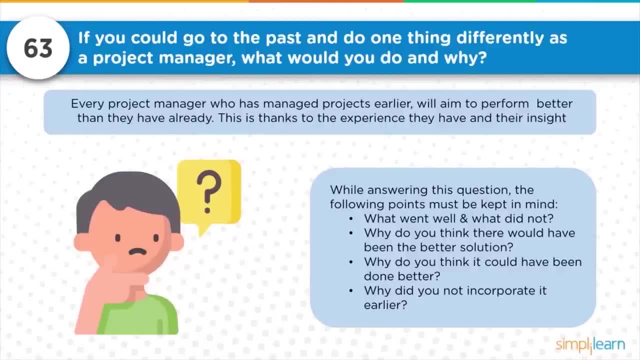 communicated regularly. the next question: if you would go to the past and do one thing differently as a project manager, what would you do, and why so? every project manager who has managed several project earlier will think of doing better which they have done already. so this is because of the